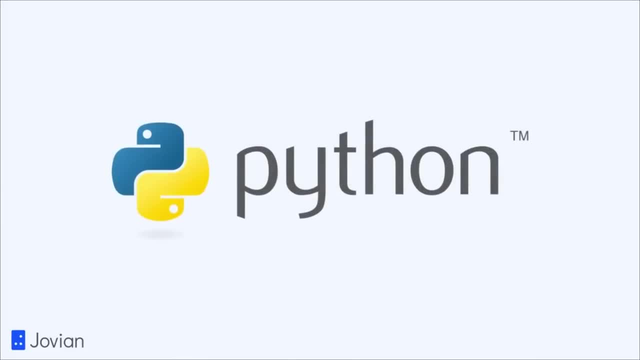 using the Python programming language. You will get a chance to practice and improve your coding skills with weekly programming assignments consisting of real interview questions, and you will also build a course project that you can showcase on your resume or LinkedIn profile. This is a beginner-friendly course and some basic programming skills. 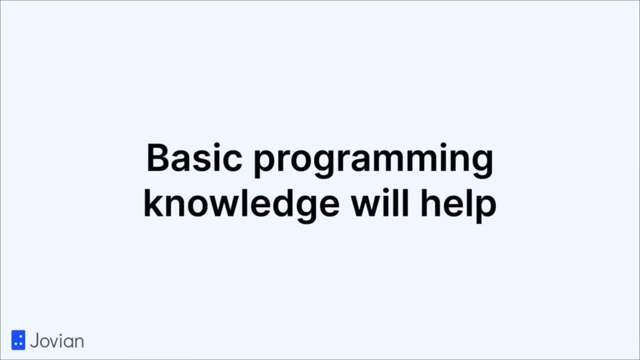 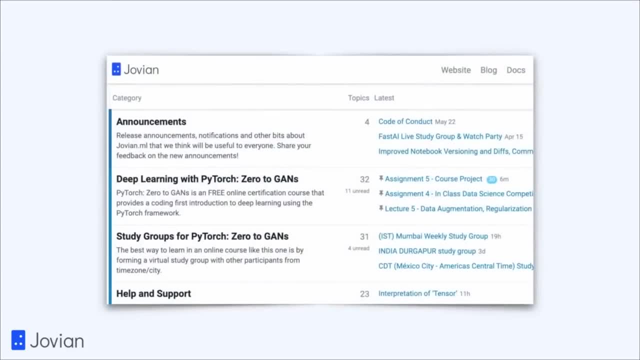 This course will help you follow along with the course. Don't worry if you're new to programming. you can learn it as you work on this course, with a little extra effort. You will also get to access the course community forum where you can ask questions. 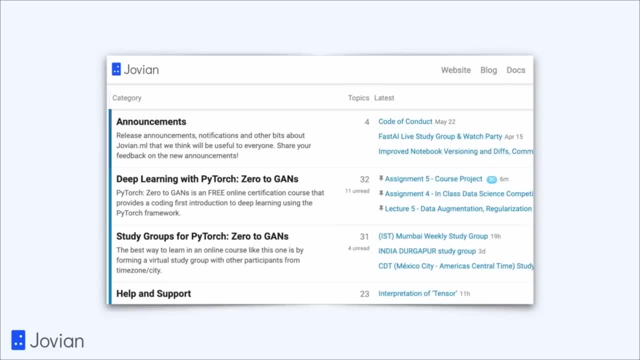 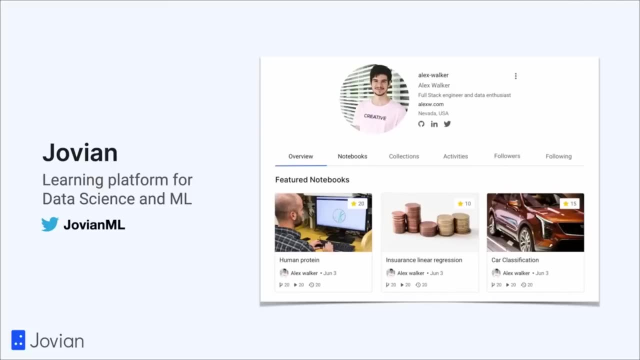 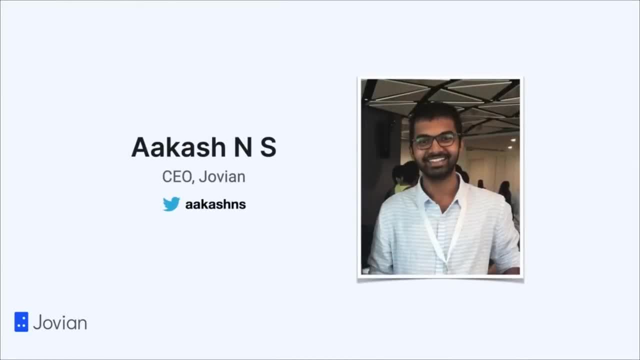 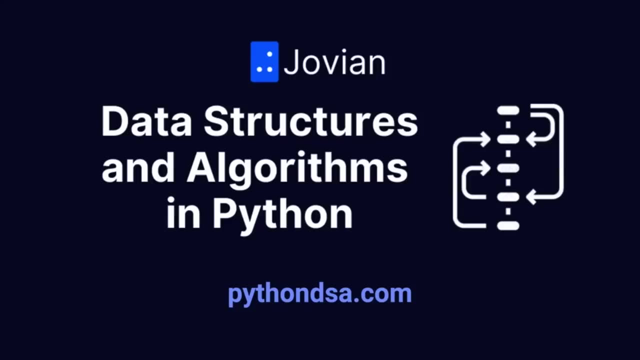 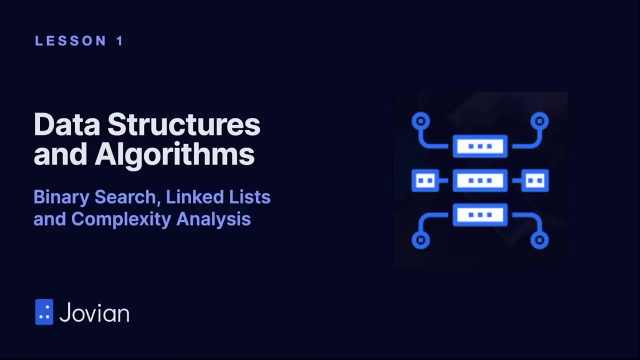 Thank you for watching this video. If you have any questions, feel free to ask them in the comments section below. Hello and welcome to Data Structures and Algorithms in Python. This is an online certification course brought to you by Jovian, And today we're at lesson 1: Binary Search, Linked Lists and Complexity Analysis. 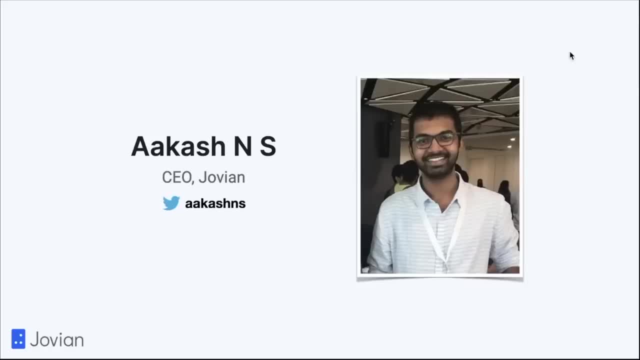 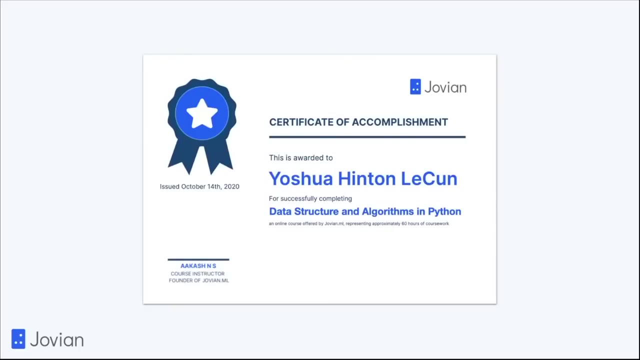 My name is Akash, I'm the CEO and co-founder of Jovian and I will be your instructor. You can find me on Twitter at at AkashNS. This course runs over six weeks and over the six weeks if you enroll with for the course. 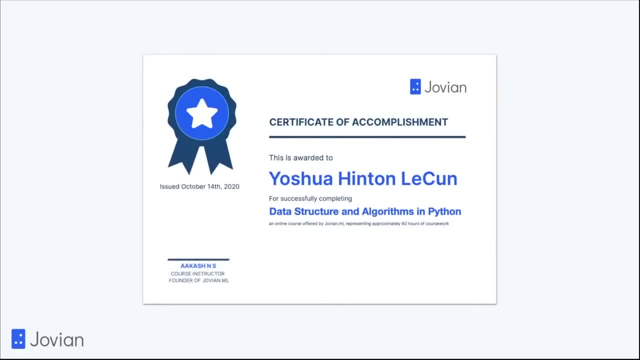 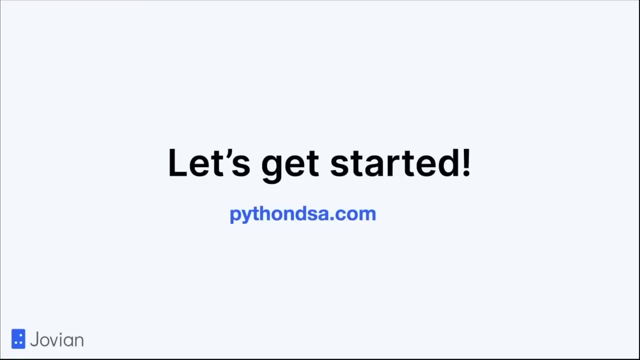 work on four programming assignments and build a course project. you can earn a certificate of accomplishment. Along the process, you will also learn about common data structures and algorithms in Python and how to use these skills to ace coding, interviews and technical assessments. So let's get started then. 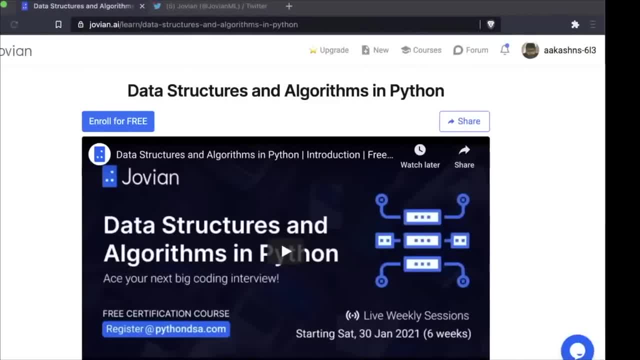 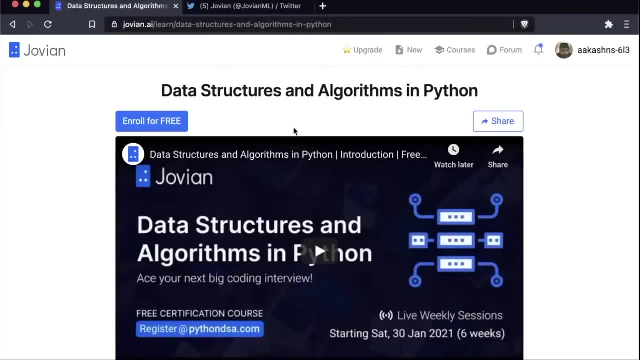 To begin, we need to go to the course website pythondsacom. So if you open up pythondsacom in your browser, that will bring you to this page. This is the course page and you can watch an introductory video about the course here. 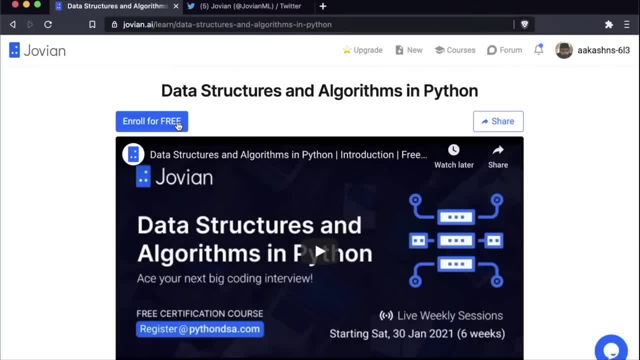 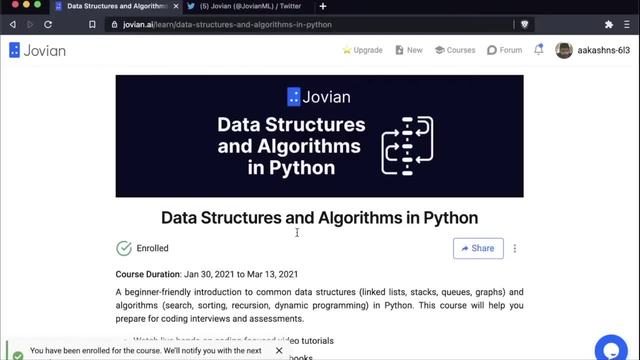 You can enroll for the course for free. You will need to sign in into Jovian. You can use your Google, GitHub or email to sign in into Jovian And once you're enrolled into the course, you can also invite your friends to join the. 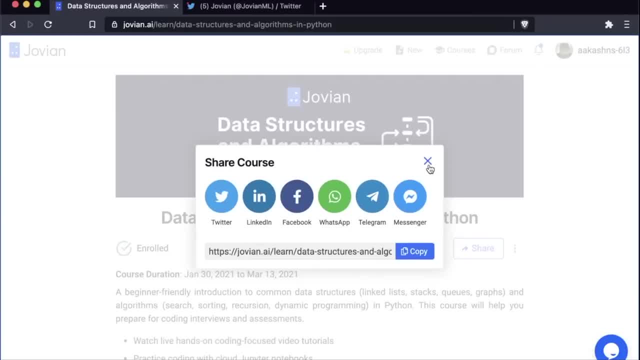 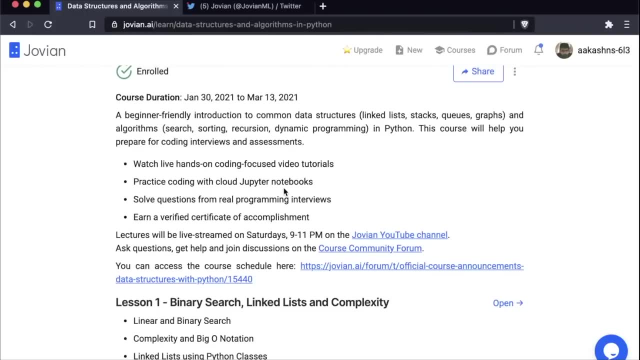 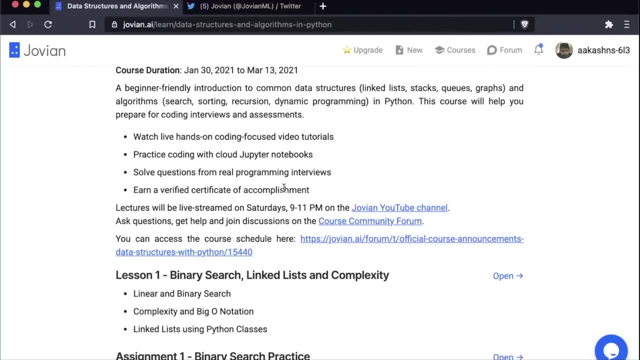 course. The course is still open for enrollments, So please invite your friends and colleagues. This course is a beginner friendly introduction to common data structures and algorithms in Python, and this course will help you prepare for coding interviews. We have coding focused hands-on video tutorials every week. 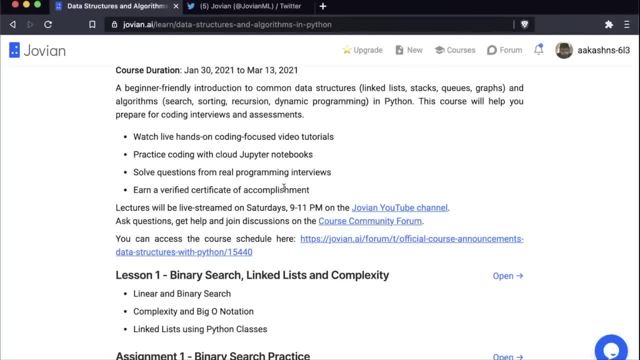 So you can either follow along with this video, You can pause and run the code as we speak And you can practice coding on the cloud, or you can watch the video right now and you can practice later. In this course, we will solve questions from real programming interviews and you can earn. 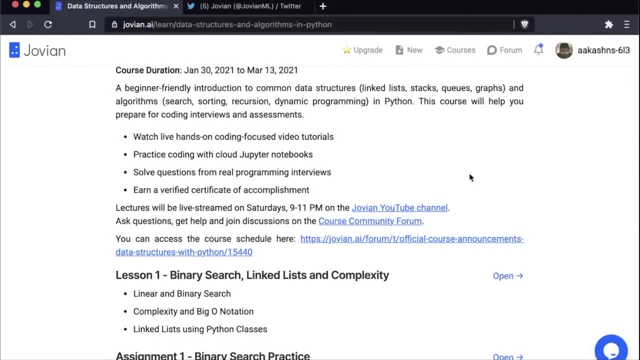 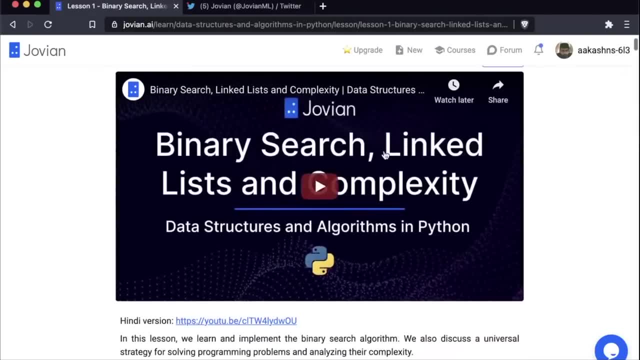 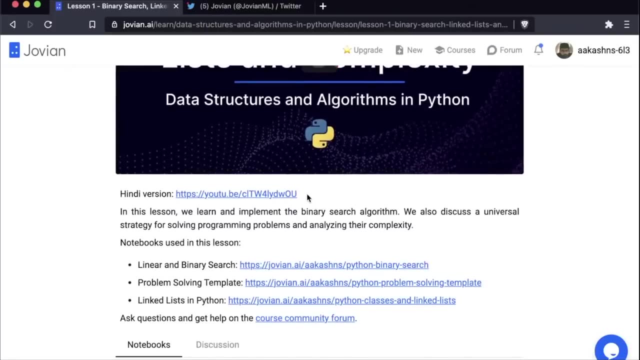 a verified certificate of accomplishment. So let's go to lesson one: binary search. link lists and complexity. On the lesson one page, you can see a recording of the lesson once it is completed. Okay, You can see a Hindi version here, and all the code used in this lesson is linked below. 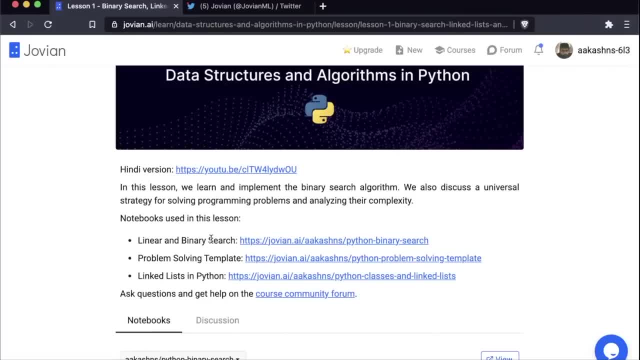 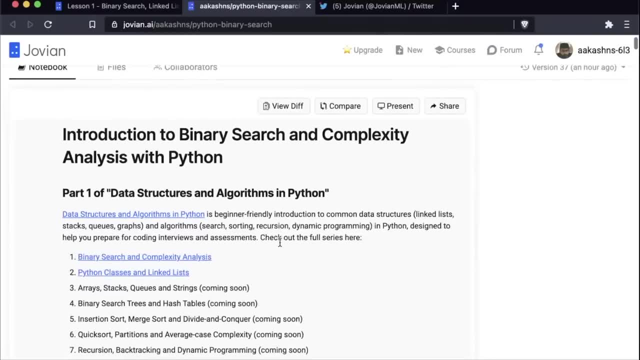 So the first set of code that we will look at today is called linear and binary search, So let's open it up. So this is the first tutorial that we will work through in this lesson, and you will be able to walk through it as well. 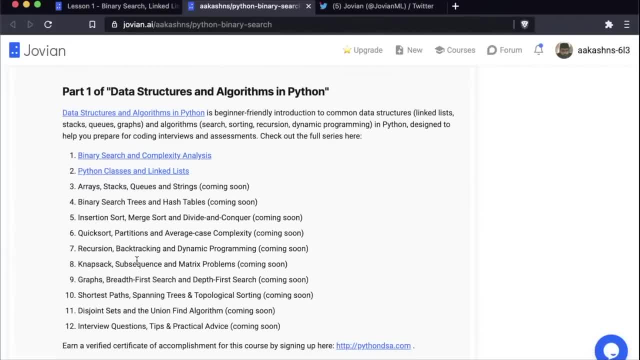 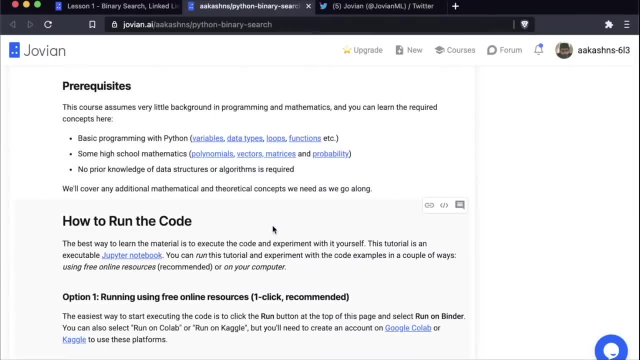 And this is part one, and there are a total of 12 notebooks or 12 tutorials we will go through Now. this course assumes very little background in programming and mathematics, but you still do need to know a little bit. For instance, you do need to know basic programming with Python, things like variables, data types. 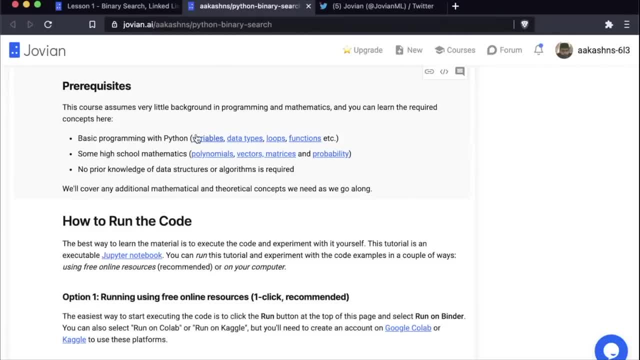 loops and functions, And don't worry if you don't know them already. you can click through and follow these links. Each of these is a separate tutorial. The tutorial will take you about half an hour or so each of these and you can learn the. 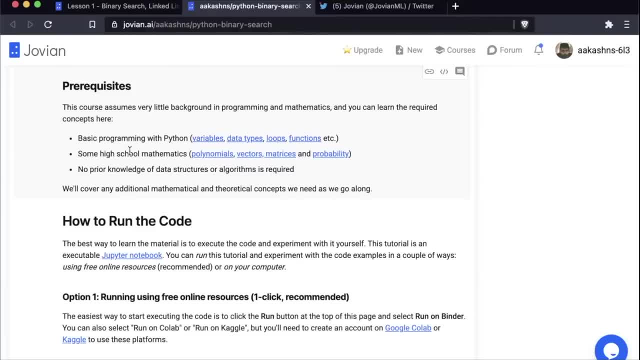 basic programming with Python in just a couple of hours. You will also need to know the basic programming of Python in just a couple of hours. Okay, So you will need to know some high school mathematics and if you want to brush up things like polynomials, vectors, matrices and probabilities, you can click through and read these, but no. 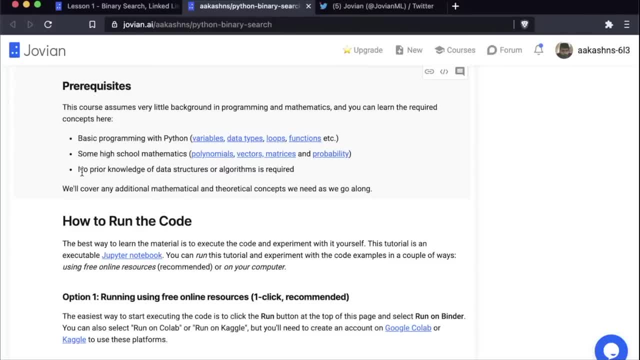 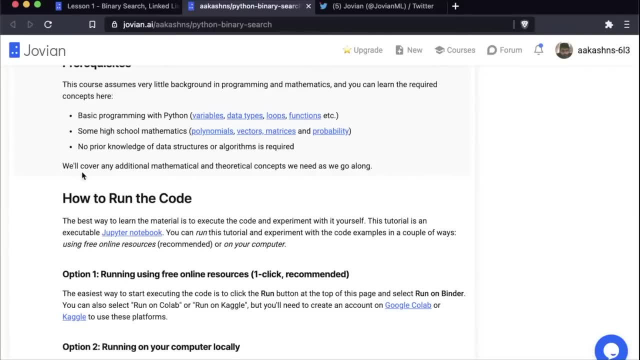 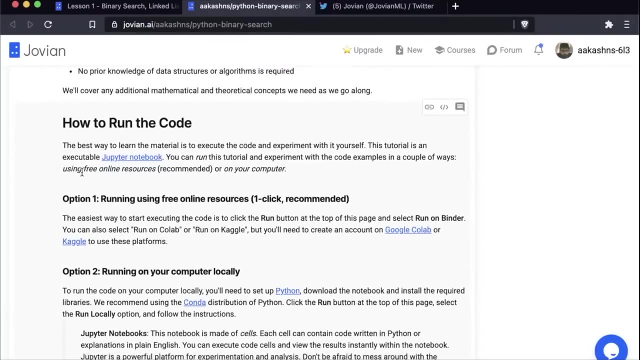 prior knowledge of data structures or algorithms is required. You do not need to have an extensive coding background, and we'll cover any additional mathematical and theoretical concepts as we need as we go along. So how to run the code. What you will see here is that: some explanations. 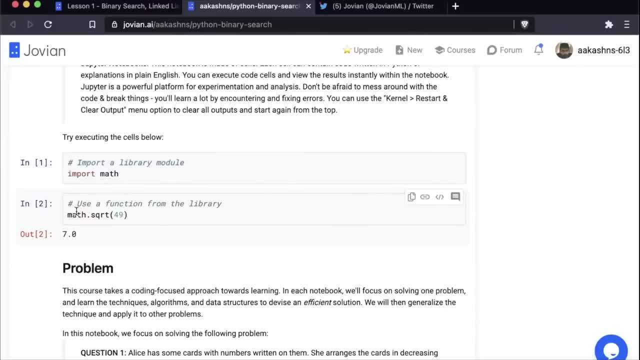 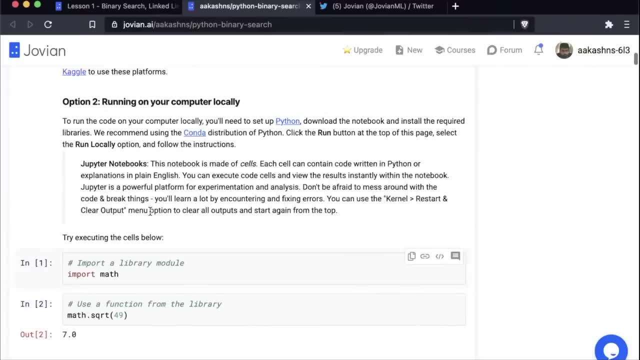 And then you will also see some code. So you can see here that there is some code written here and there is some fun. So the library is imported and a function from the library is used here. Now to run this code, you have two options. 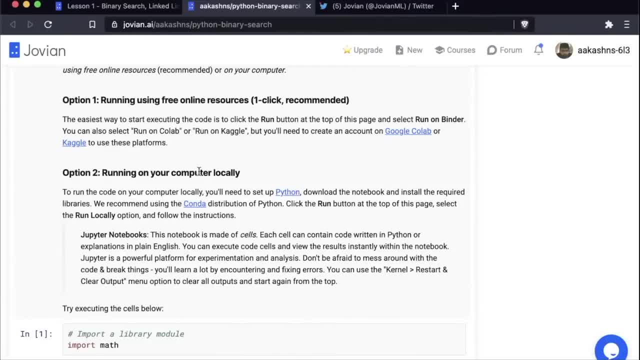 You can either run this code using free online resources, which is what we recommend, or you can run it on your computer locally and you can read these instructions. I'm going to use free online resources provided by Jovian, So we just scroll up here at the top of this page and click run. 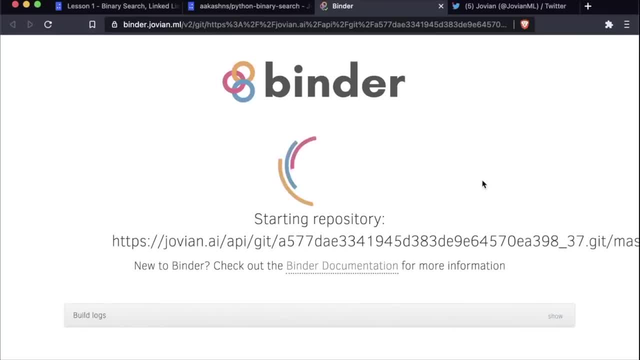 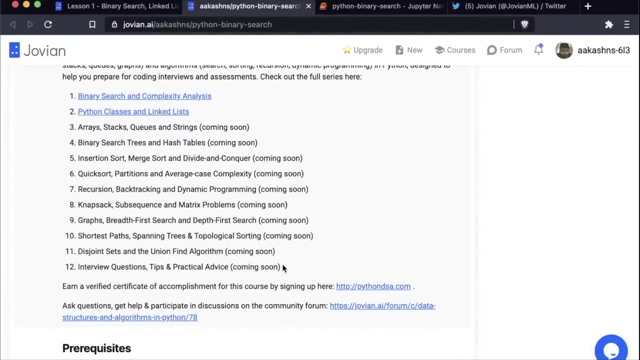 And then click run on binder. So this will take a second or two, And what we're doing here, essentially, is setting up a machine for you on the cloud using a software called binder. It's an open source software. And now what you were looking at here, this was actually not a blog post. 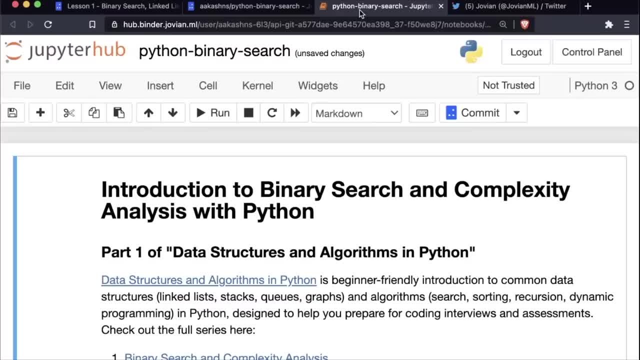 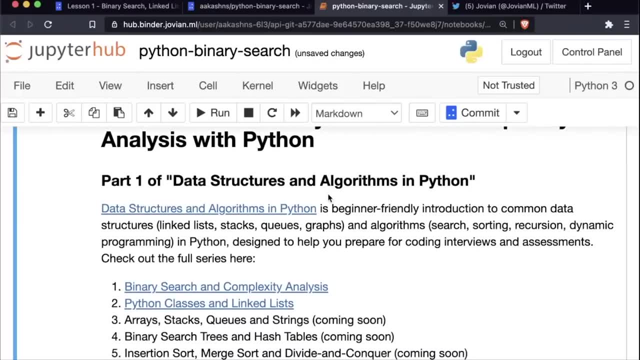 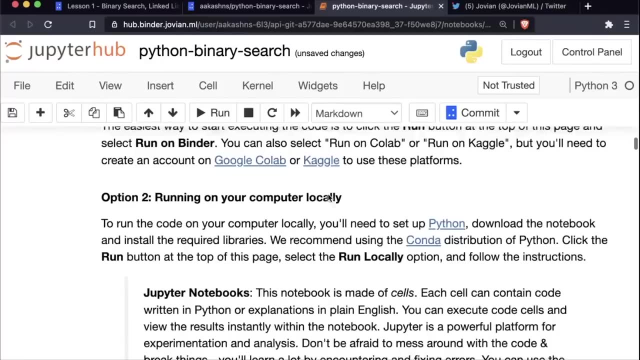 This is actually something called a Jupiter notebook. A Jupiter notebook is something that can not only contain explanations, but can also contain code, And it's outputs right here in an interactive fashion. So if I scroll down here, you can see that we have all the same content that we were. 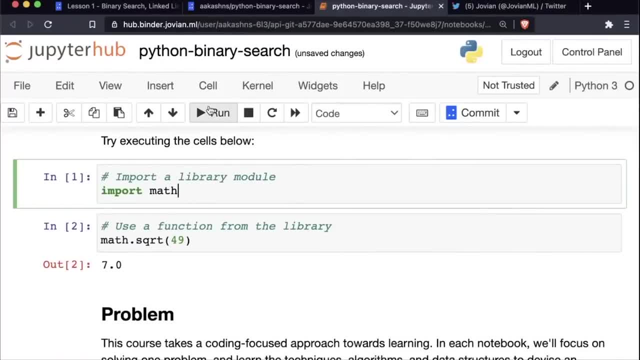 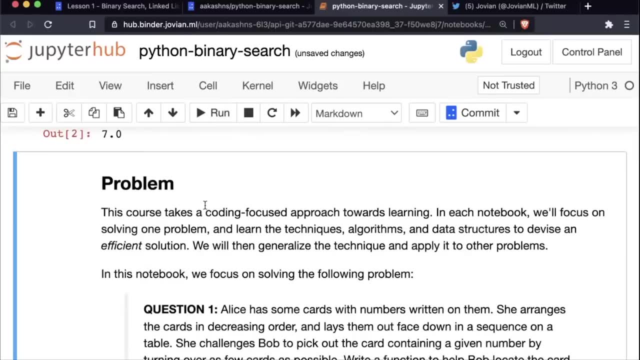 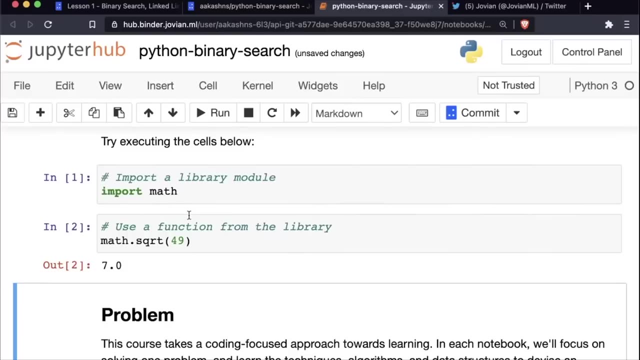 looking at, except this time we can actually run this code. So we can click the run button here and the run button will run the code. And here we click the second run button that is going to run the second line of code. Now we will be using Jupiter notebooks extensively throughout this course, because Jupiter notebooks 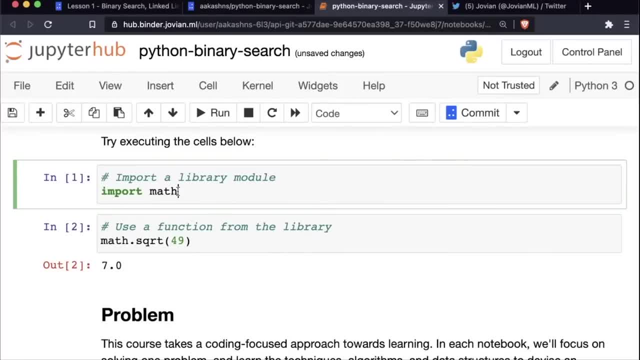 are a great way to do interactive programming. You can change the code. For example, instead of the mat mat dot square root, you can use mat dot seal and you can change the value here. So Jupiter notebooks are great for experimenting with code. 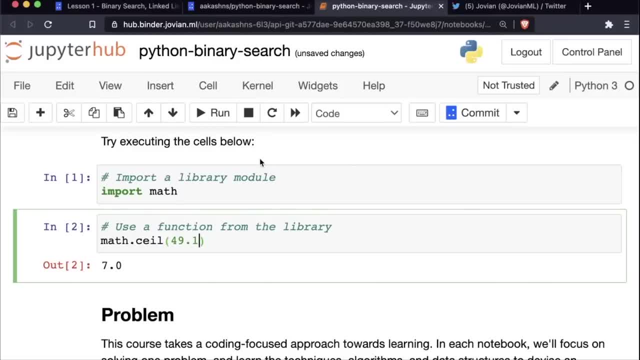 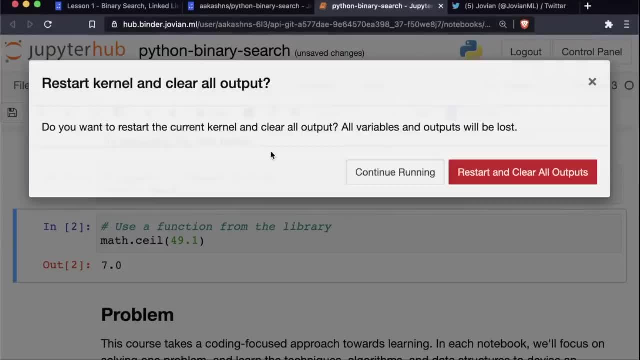 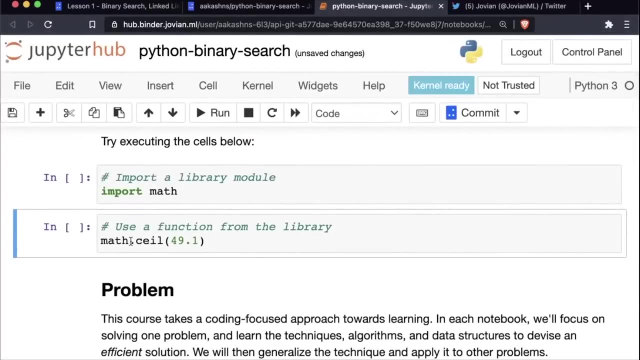 Now just a couple of tips that you want to do. as soon as you run a Jupiter notebook, you can click on Colonel and click restart and clear output. What this will do is this will remove all the pre-executed outputs from your code. So you can now see that. 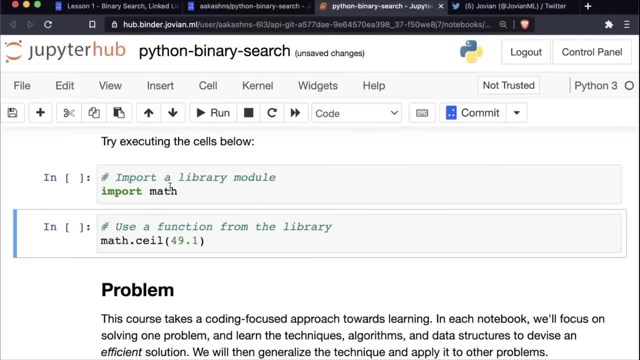 Yeah, The function is gone and you can see that the numbers here go away. So now you can execute the code line by line yourself and see the output, discover the output. And then one other thing you can do, if you want to hide the UI a little bit, is to toggle. 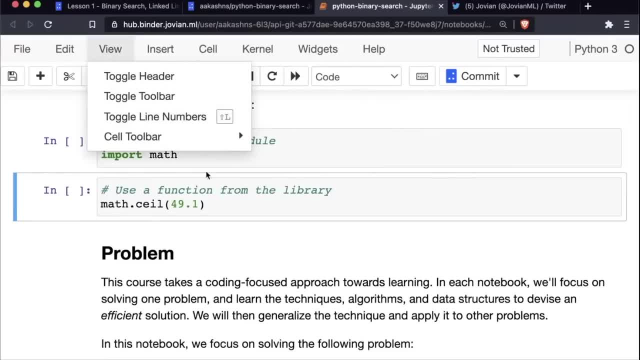 the header and also toggle the toolbar. Now you might need the toolbar for the run button, but there's a tip here: Instead of pressing the run button, you can use shift plus enter. So if you press shift plus enter, that will execute. 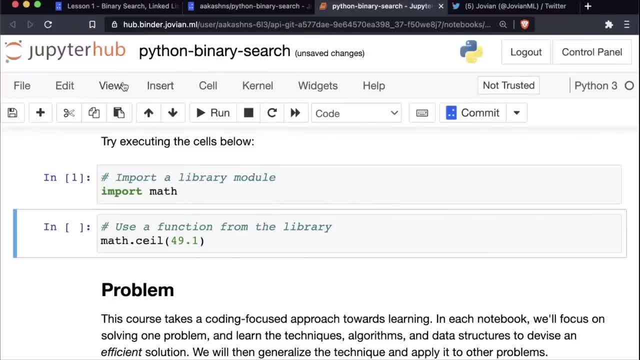 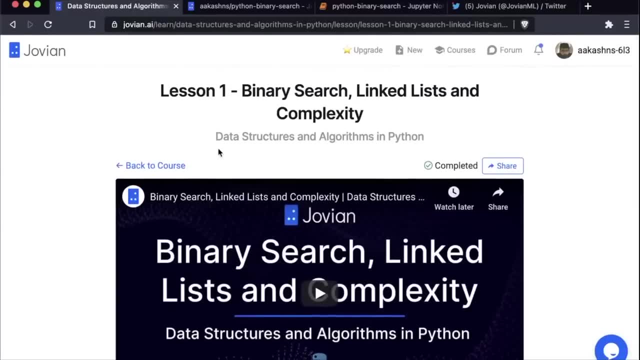 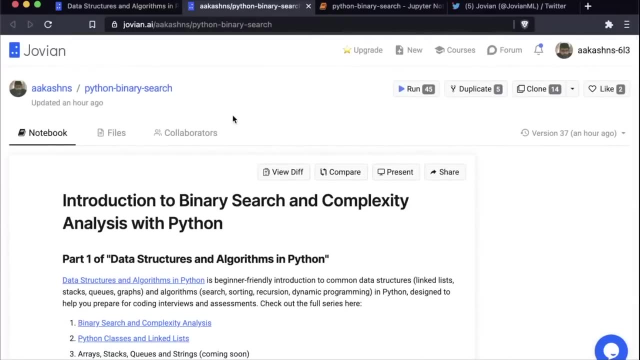 A cell And that's a pretty handy shortcut. So once again you go on the lesson page. on the lesson page you will find a link to the notebook called linear and binary search. on the linear and binary search You can read the explanations, but you can't run them. to run the code. 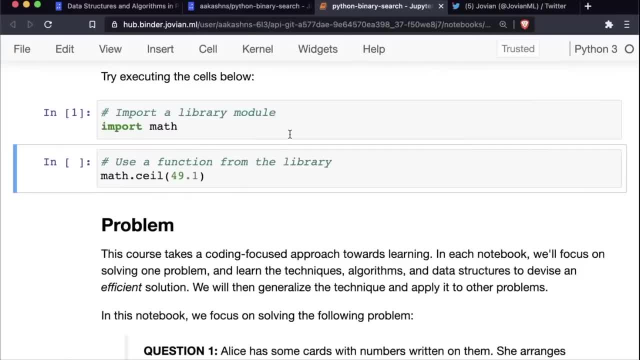 You need to click run and then select run on binder, and clicking run on binder will set up a cloud machine for you and all the code That you see here will get executed on the cloud, So you do not need to set up anything on your computer. 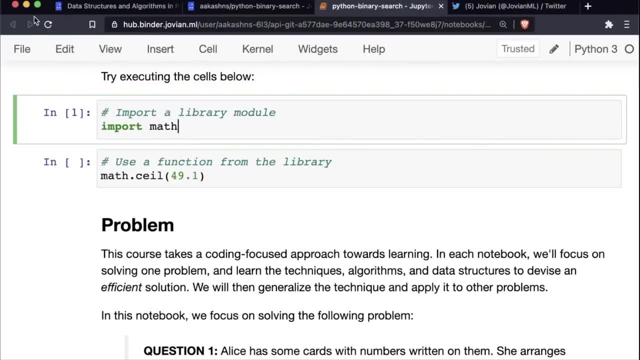 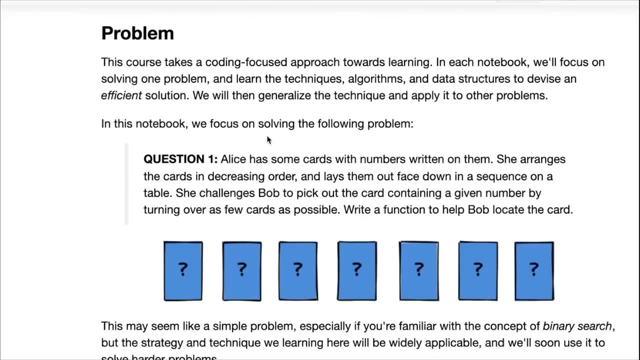 You do not need to download anything. We've done all that for you, So let's get started then. This course takes a coding focused approach towards learning, and in each notebook or each tutorial, we will focus on solving one problem and then learn the techniques algorithms. 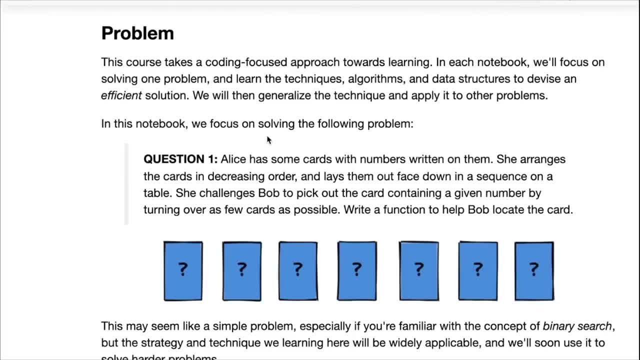 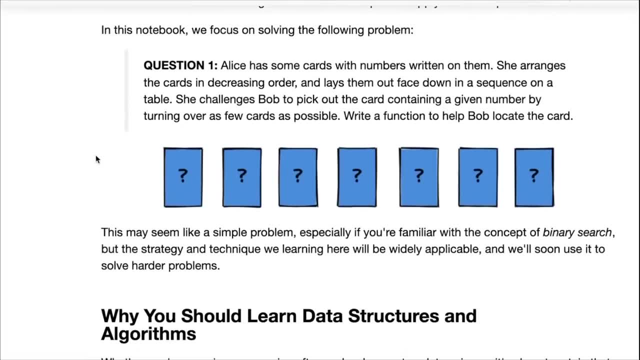 and data structures to device an efficient solution for that specific problem. We will then generalize the technique and apply it to other problems. So in this specific tutorial, we will focus on solving this problem, and here's the problem we're solving, and this is a typical problem that you will come across in a coding challenge. 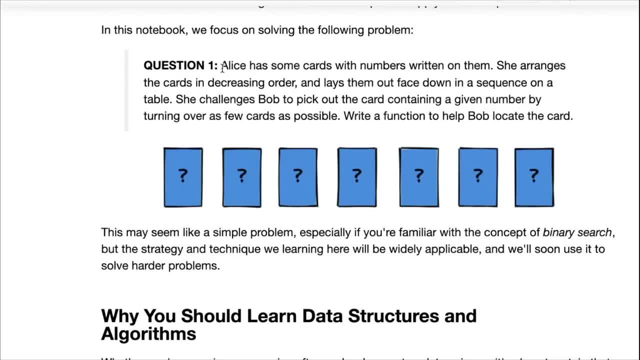 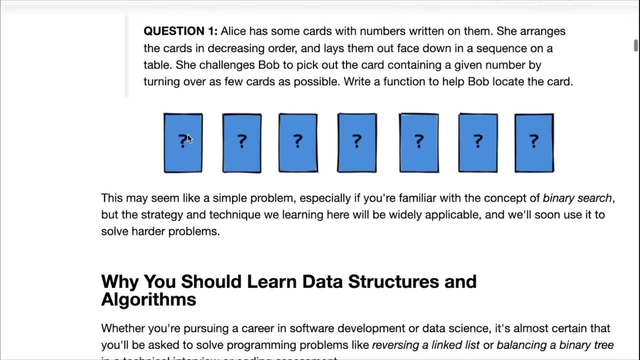 or a coding interview. So here's how the problem goes. Alice has some cards with numbers written on them, and then she arranges the cards in decreasing order and lays them out face down in a sequence on a table. So this is what it looks like. 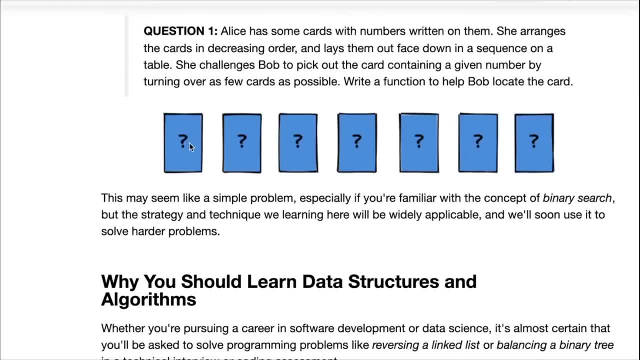 These are cards. Each of these cards has a number below it And the numbers are in decreasing Order. She challenges Bob to pick out the card containing a given number. For example, she could say: Bob, I want you to pick out the number seven by turning over. 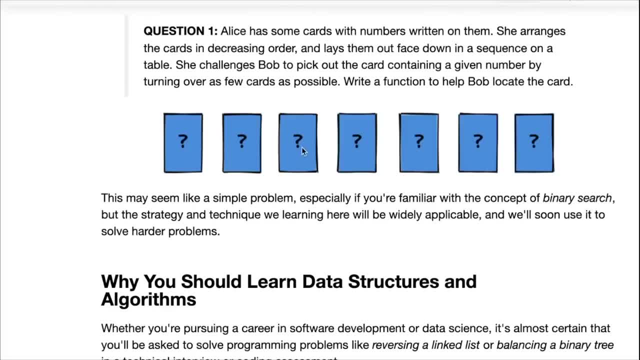 as few cards as possible. So this is a puzzle that's given to us and we're not told how many cards Alice has. So you need to write a function to help Bob locate the card, So Alice can put down any number of cards and the target number that Bob has to pick. 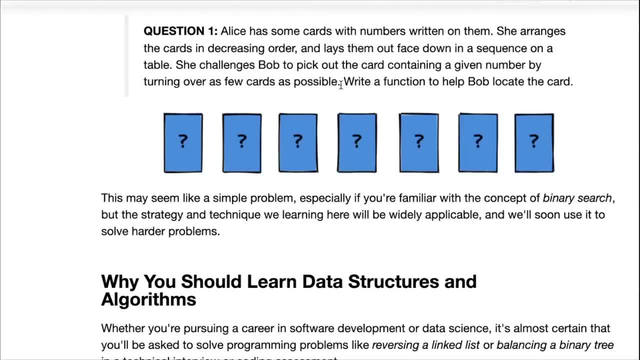 out could be anything. So we have to tell Bob Not a space, Not the solution for a specific problem, but a general strategy that he can use to turn over as few cards as possible. So, for instance, look at these seven cards and maybe put some imaginary, imaginary numbers. 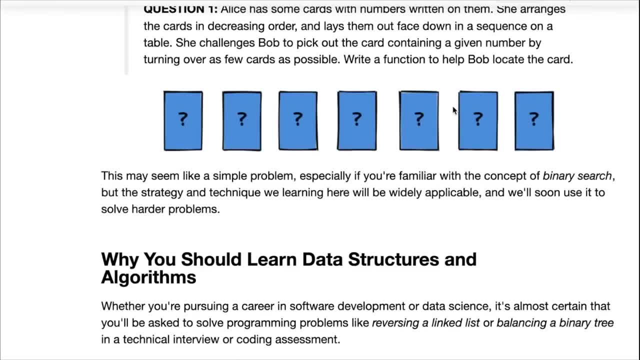 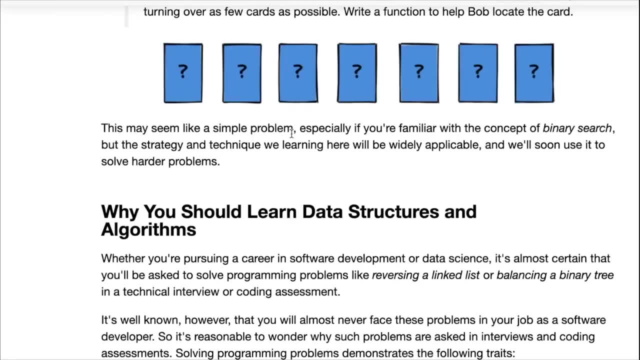 before them, below them, and try to figure out a strategy. try to start thinking about the problem, And this may seem like a simple problem, especially if you're familiar with the concept of binary search, but the strategy and technique that we're learning here will be widely applicable. 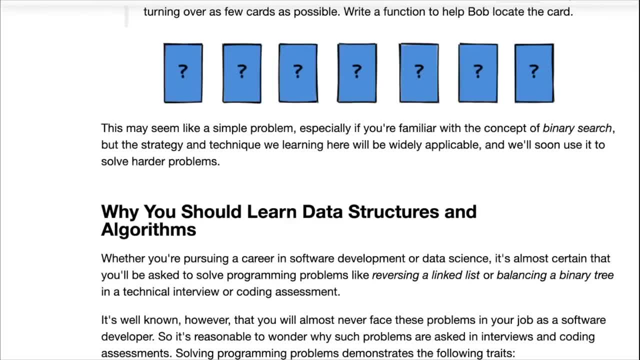 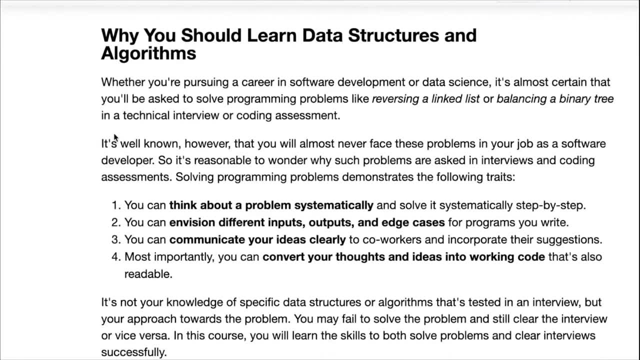 And we will soon use it to solve Harder problems. Now, before, while you think about the problem and before we start solving it, I just want to talk about why you should learn data structures and algorithms, and whether you're pursuing a career in software development or data science, it's almost certain that you will be asked. 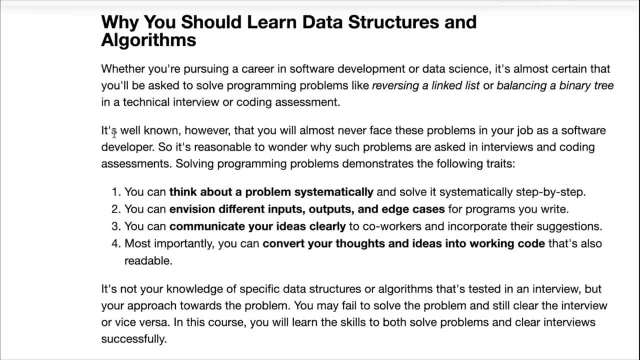 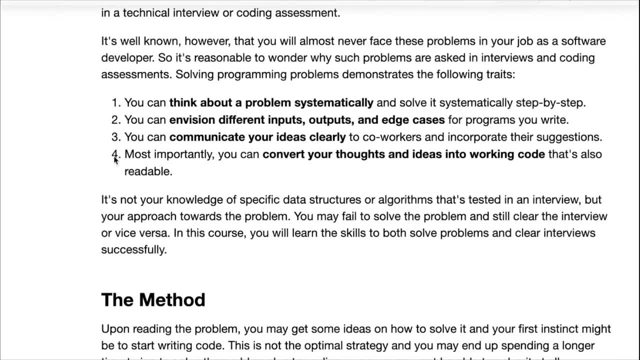 programming problems like reversing a leg list or balancing a binary tree in a technical interview or coding assessment. Now, it's well known that you never face these problems in your job as a software developer, So it's okay to wonder why such problems are asked in interviews. 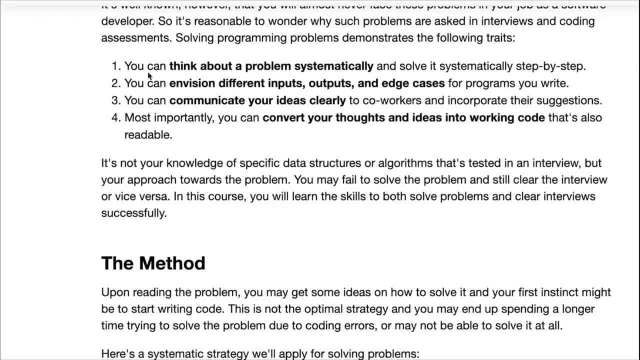 Okay, And they're asked because they demonstrate the following traits, And these are very important traits for a programmer. Number one is that you can think about a problem systematically and then solve it systematically- step-by-step too. And the number two is that you can envision the different inputs and outputs in edge cases. 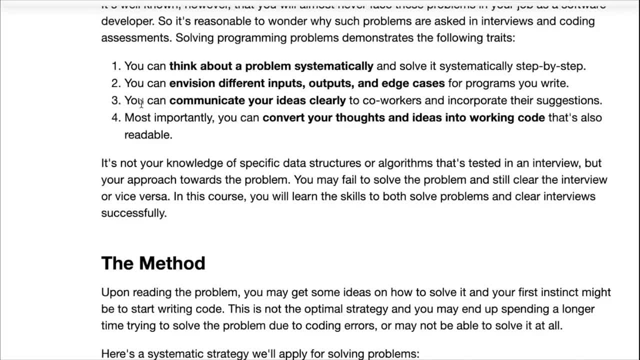 for your problem Because programs, when you put them out in the wild as part of software, can encounter any kind of inputs And, as you have thousands or millions of users, you will encounter any and every possibility, And often this has many security implications. 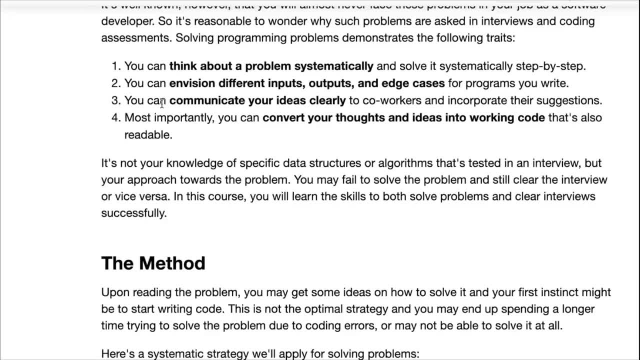 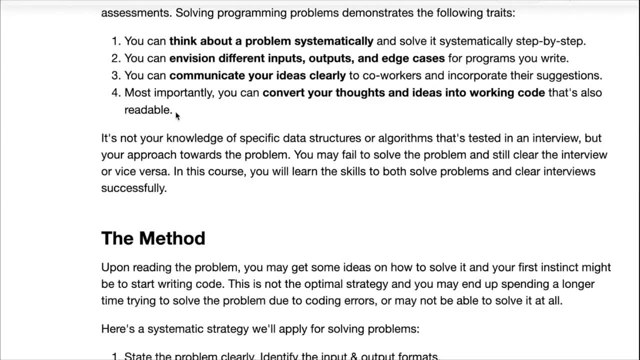 It can take down the server, It can take down your application or you can have a loss of data or loss of property. You can communicate your ideas clearly to coworkers- That's a very important part of problem solving- And, most importantly, you can convert your thoughts and ideas into working code. 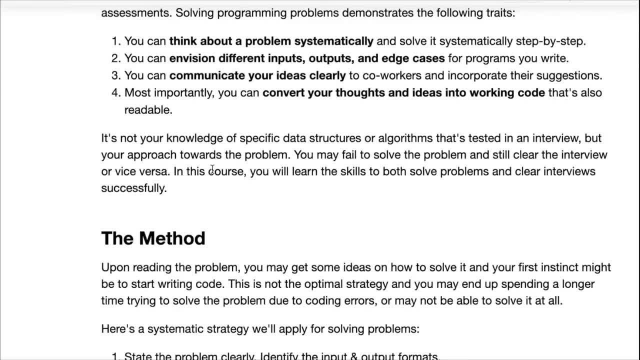 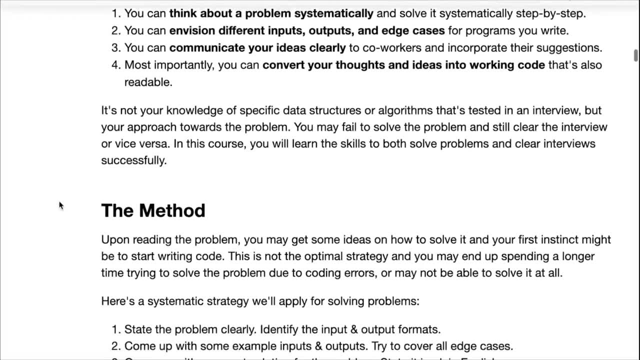 And the code should also be readable to other people. So it's not really the knowledge of specific data structures or algorithms that's tested in an interview, but it is your approach towards the problem. So you may fail to solve the problem, but you may still clear the interview or vice. 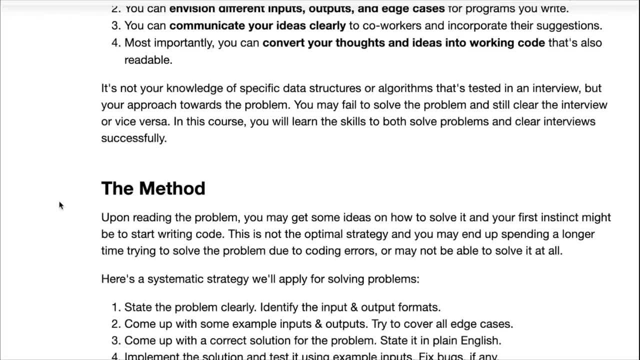 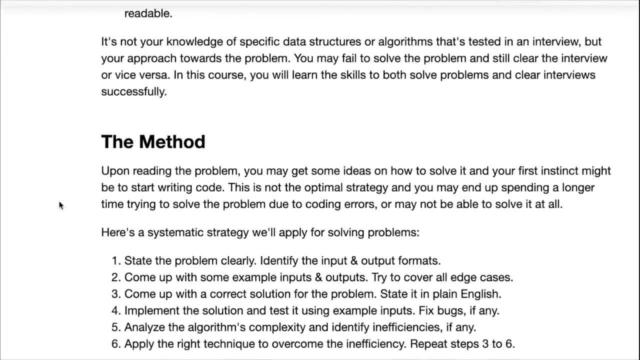 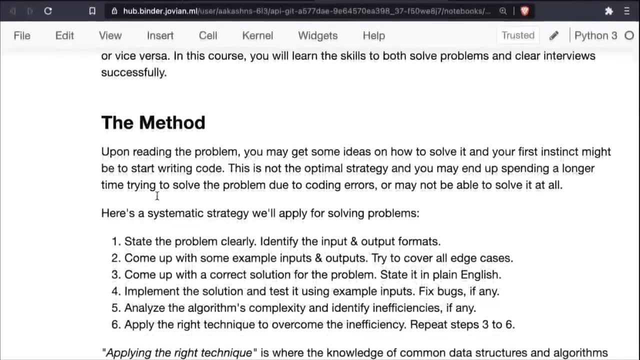 versa: You may solve the problem and still not clear the interview. So in this course, we will focus on the skills to both solve the problem and to clear interview successfully. So that's why you need to learn data structures and algorithms. So, coming back to the problem at hand now, you've read the problem and you may have been 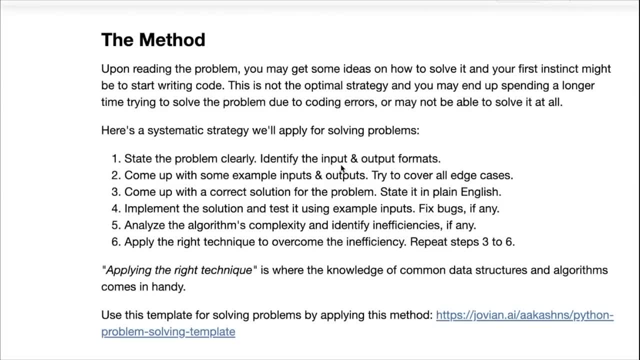 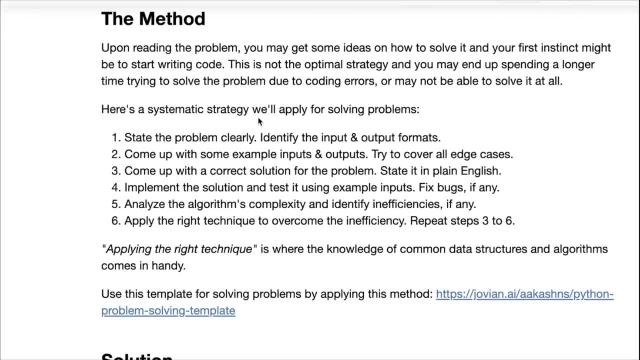 thinking about it, You may have some ideas on how to solve it, And your first instinct might be to just start writing the code for it. but that is not the optimal strategy And you may actually end up spending a longer time to solve the problem due to coding errors. 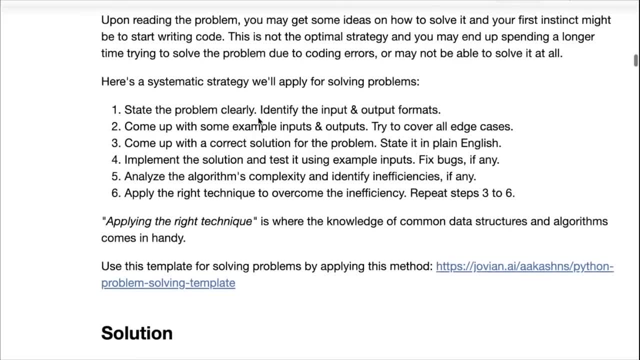 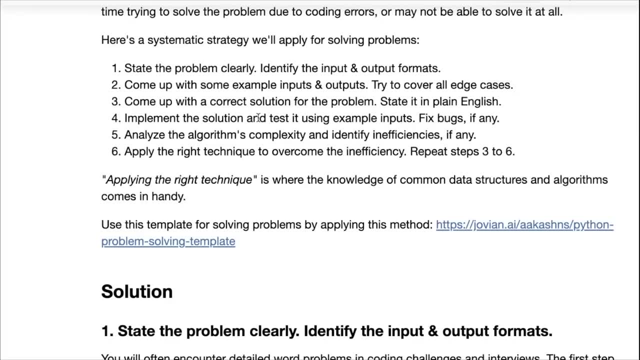 or you may not be able to solve the problem at all. So what we are going to cover here is a systematic strategy that you should apply in interviews or encoding problems, on encoding assessments or, in general, whenever you're faced with a problem like this. 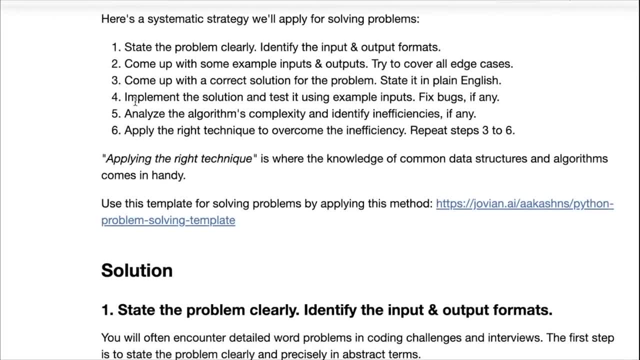 So here's the strategy that we will apply. Okay, Step one: state the problem clearly, identify the input and output formats. Step two: come up with some example inputs and outputs and try to cover all the edge cases. Step three: come up with a correct solution for the problem. 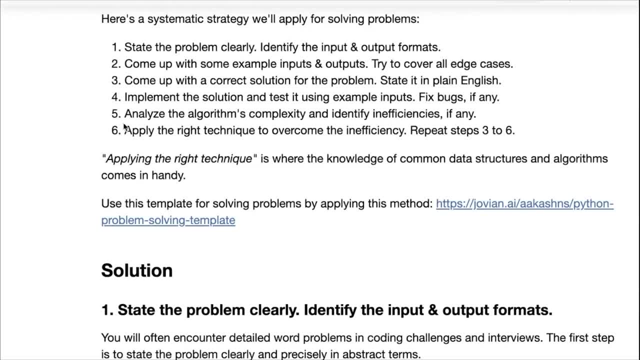 It can be as simple as possible and stated in plain English. Step four- and this is a step that is optional Sometimes- implement the solution and test it using example inputs and then fix any bugs in your in your first solution. And step five: analyze the algorithms complexity and identify any inefficiencies. 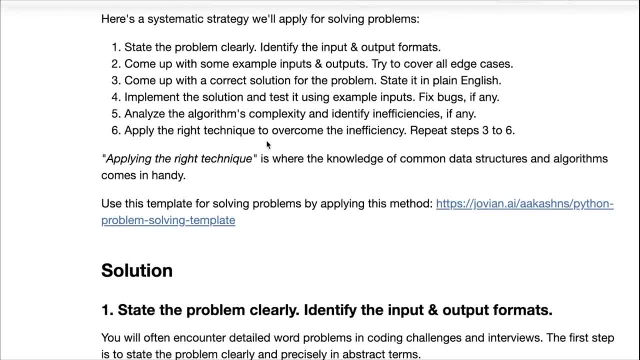 And finally, step six: apply the right technique to overcome the inefficiency and then go back to step three, which is come up with a new, correct solution which is also efficient. Then implement the solution and analyze the algorithms complexity. So this is the technique that we will apply over and over for the course of six weeks. 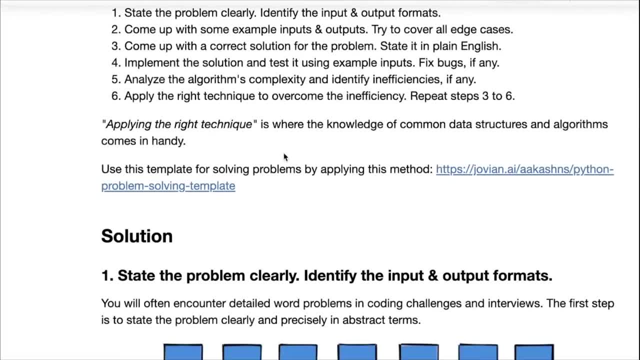 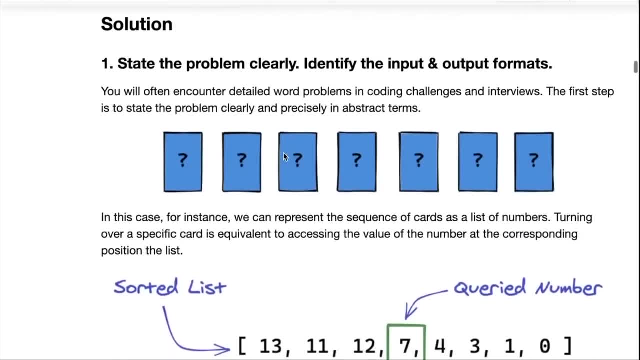 to many different problems, and applying the right technique is where the knowledge of common data structures And algorithms comes in handy. So this is the method we'll be using. So let's jump into the solution. Step one: state the problem clearly. Now you will often encounter detailed word problems and coding challenges and interviews. 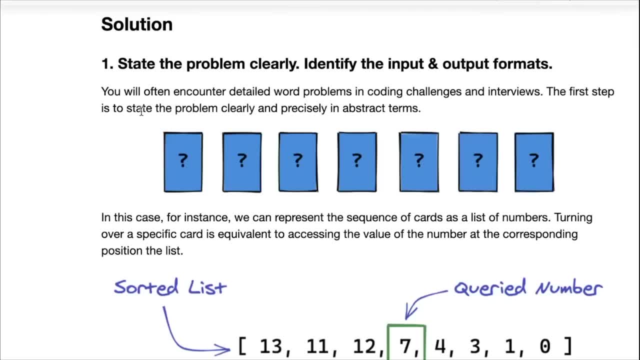 They will go on for paragraphs and paragraphs. For instance, here we're talking about Alice having a deck of cards and then shuffling them, putting them out on a table, talking to Bob, et cetera, et cetera, et cetera. 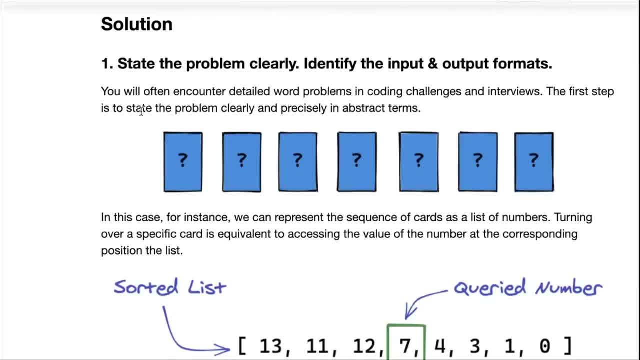 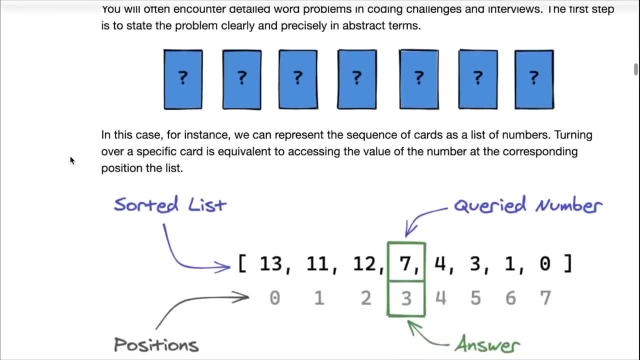 The first step is to state the problem clearly and precisely in abstract terms, because computers don't understand People, computers don't understand cards, computers understand numbers, So for in this case, we can represent the sequence of cards as a list of numbers. 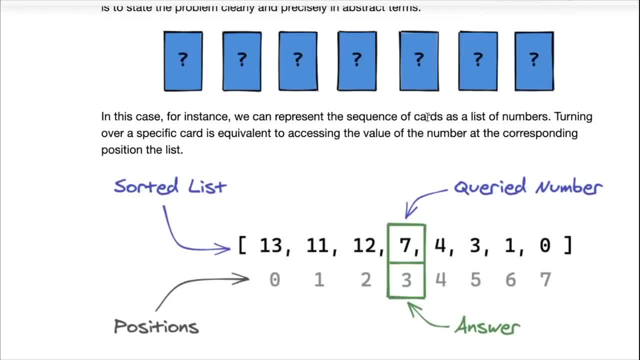 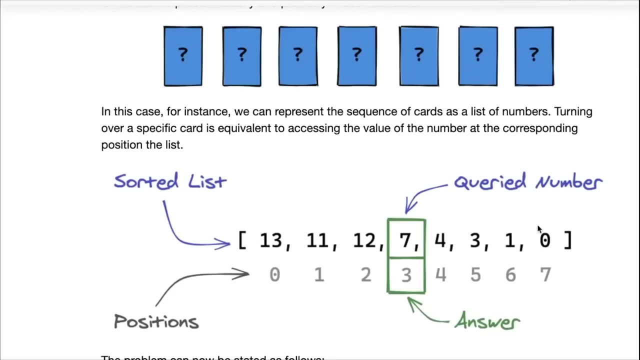 So a list is a basic data structure and Python and the turning over of a specific card is equivalent to the accessing of the value of the number at a certain position in the list. For instance, if we think of this set of cards being represented by this list, you can see. 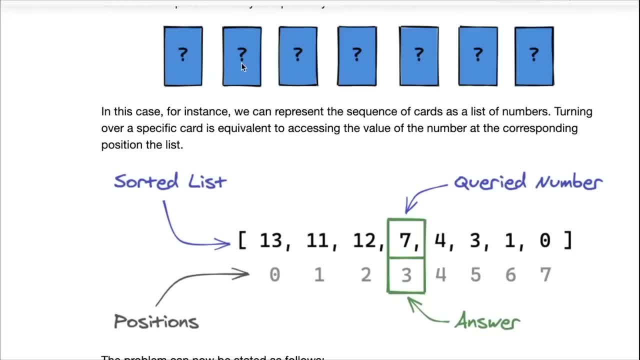 here that this list is sorted in decreasing order, Then turning over a certain card is equivalent to accessing that specific element from the list. So turning over card number two or, as we say in computer science, card number one, because this is card number zero. 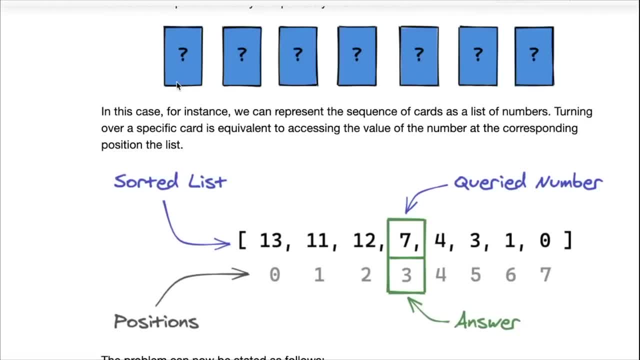 And this is one thing that you might want to get into your head as well- that whenever you're counting, always start counting from zero, Otherwise you may run into many off by one errors. So this is position zero and this is position one. 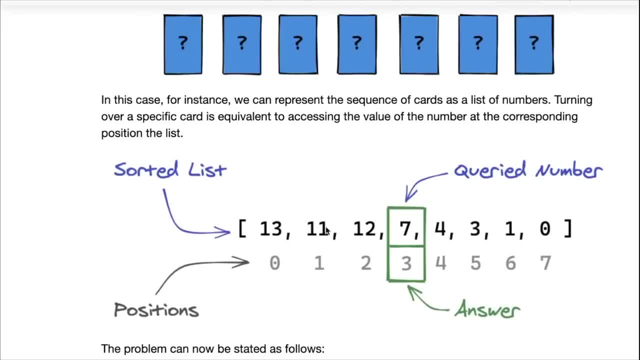 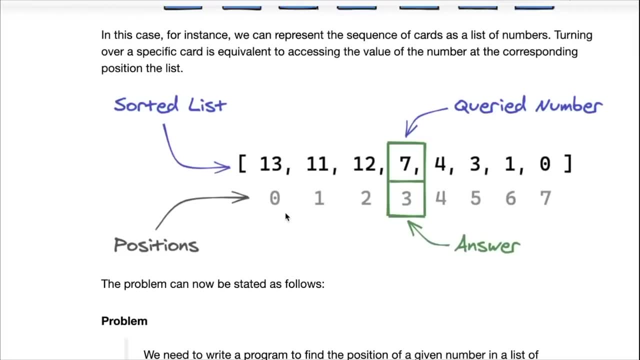 So if you turn over the card at position one, it is as good as accessing an element from a given list, Which, in this case, will turn out to be 11.. So these are the positions in the list, starting from zero, And now what we have to figure out is: how many elements do we need to access? 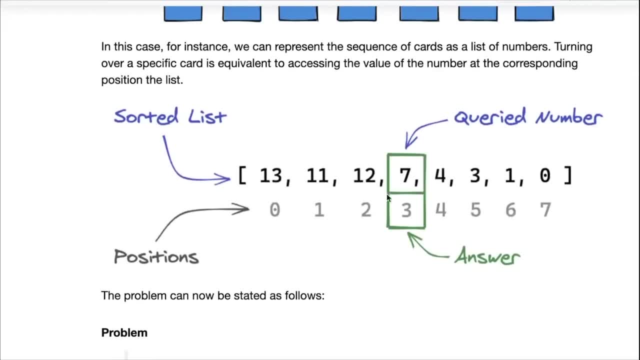 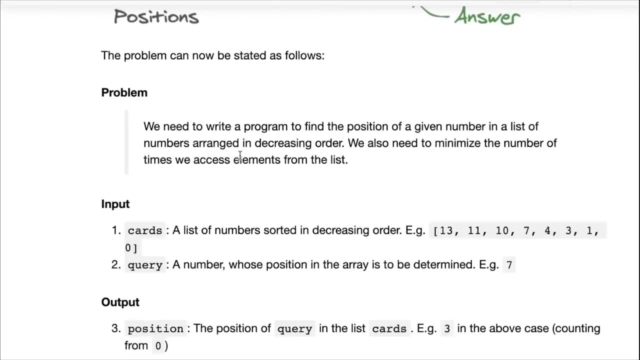 So we need to access the minimum number of elements to get to a particular element, right? So the problem can now be stated as follows: We need to write a program to find the position of a given number in a list arranged in decreasing order. 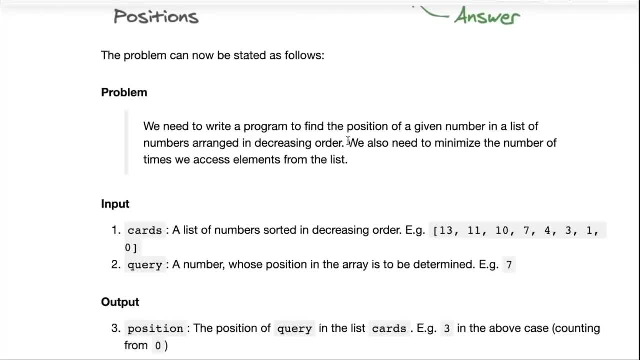 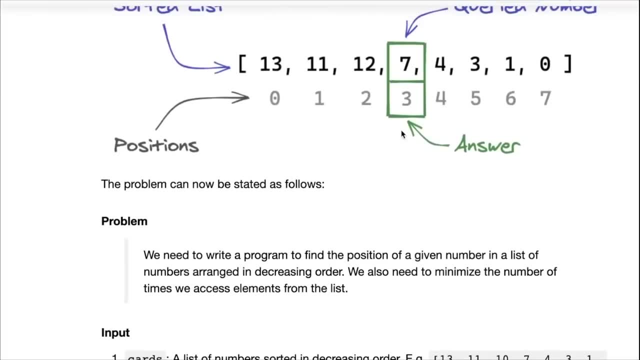 We also need to minimize the number of times we access the elements From a list. So we're finding the position of the given number, seven, and the position in this case is three, And we want to minimize the number of times we access elements from the list. 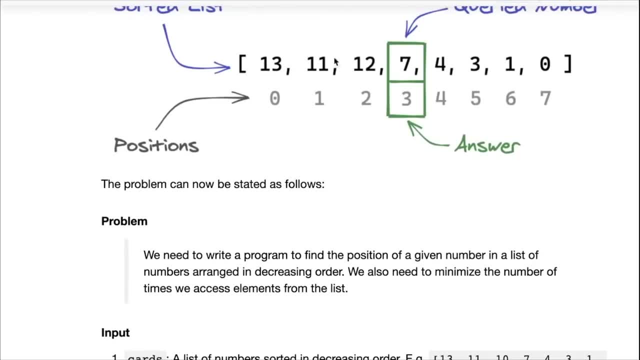 So if we go in this direction, for example, we would need to access 13,, 11,, 12, and finally we discover seven. we come from this end. we may discover seven, six, five, four And finally we may discover seven. 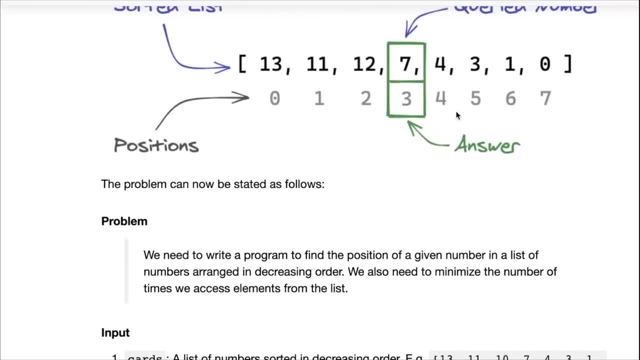 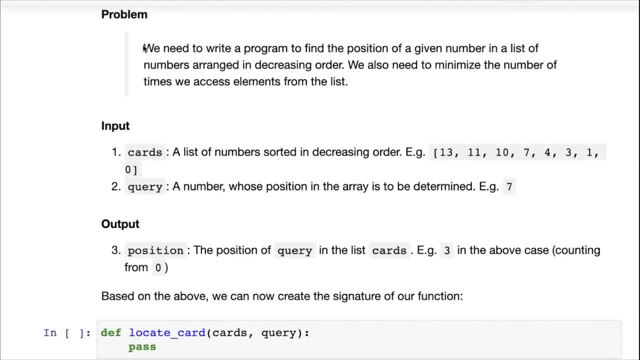 So definitely, coming from the left is better than coming from the right, But is that the best? That's what we're solving Now. Let's find the problem, And what you should do is you should try to write down the problem in your own words. 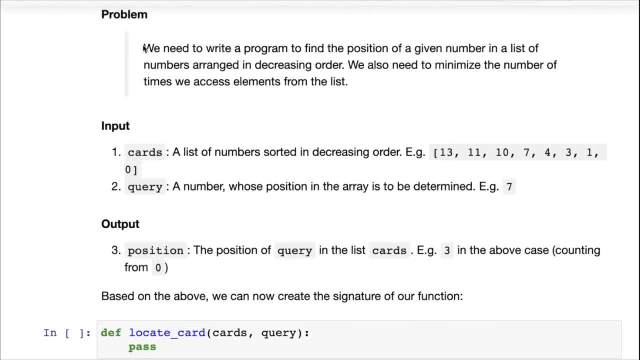 And primarily this is for you to make it clear to yourself. either speak it out loud to the interviewer or write it down in your own words, as short as make it as short as as long as possible, so that you clearly understand what's in it and then come up with the inputs and 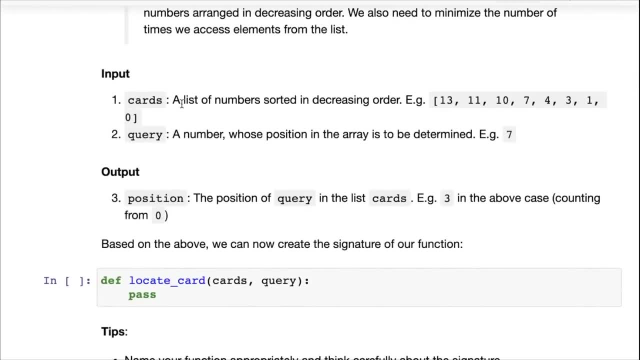 the outputs. So there are two inputs here. There's the input cards, which is a list of numbers sorted in decreasing order, And then the second input is a query, which is a number whose position And the array is to be determined. 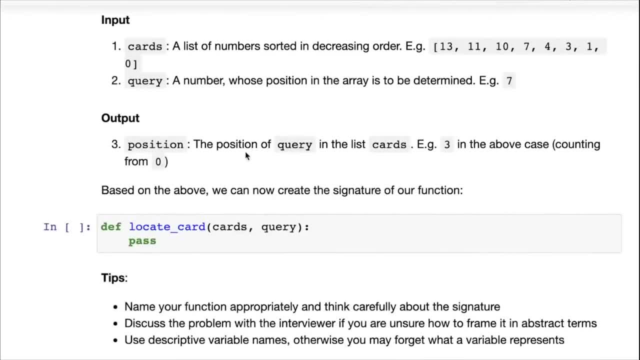 And there is one output, which is position, And the position is simply the position of query in the list of cards. For example, seven is at position three, counting from zero of course. And as soon as you've written the input and output out, you can now write what is called. 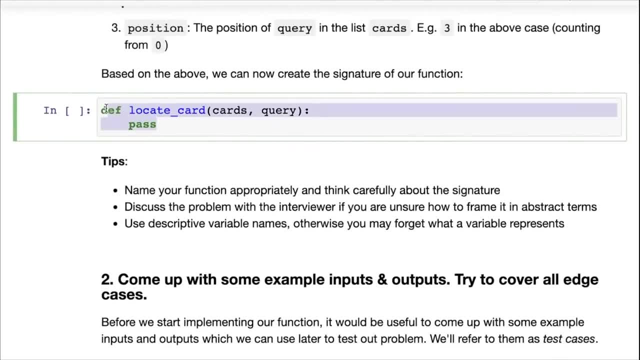 the signature of our function, which is a structure of our function without any actual code inside it. So now we can call it def- locate card with cards and query- and the single statement inside it called pass, Because a function in Python cannot have an empty body. 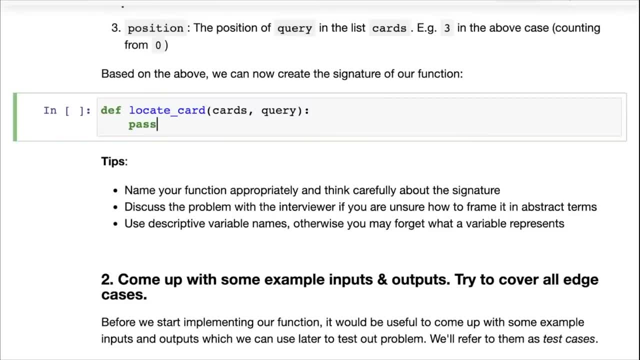 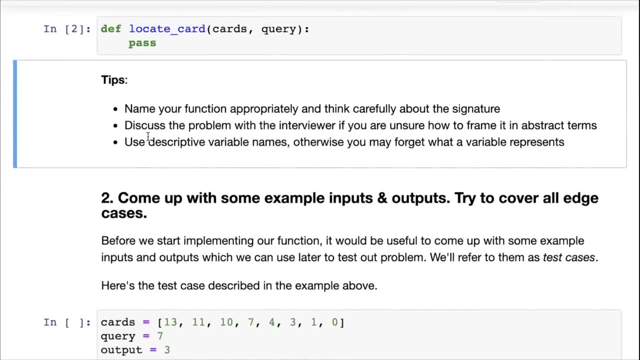 You need to put in at least one statement. So you always put in the past statement first, because it doesn't do anything. There you go. So now we have framed our problem in abstract terms and now we have a function signature to work with. 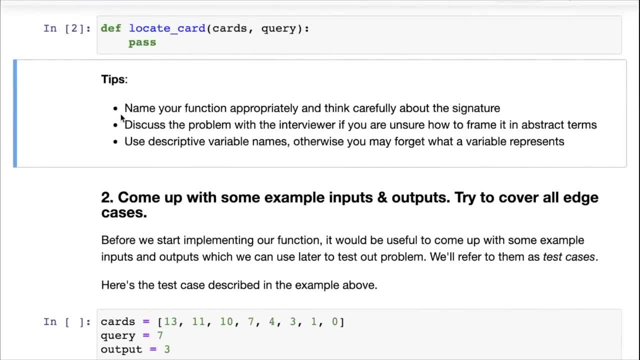 Now a couple of tips here. This is something that interviewers specifically will look for, but also encoding assessments, because your code is also shared with the company, So you may want to name it, Name your functions properly and think carefully about the signature. 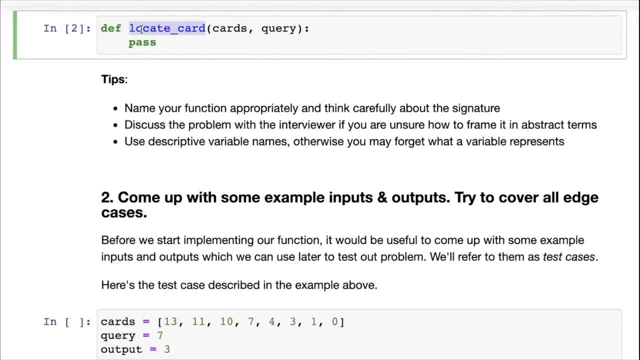 For example, here you should not call your function F1 or funk one or F or something like that. It's better to call it locate card, because that's what it is doing, And the similar thing is true for variable names as well. 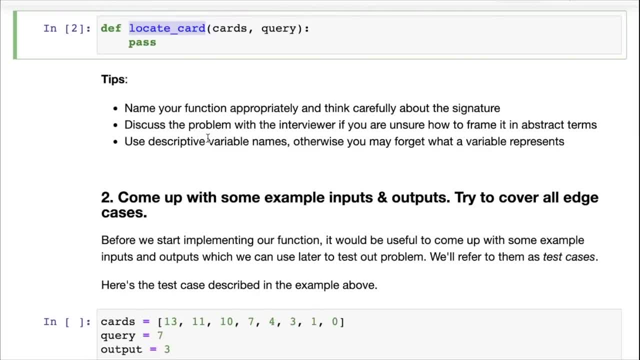 Use descriptive variable names: One because it's good for coding practice and second because, as you work on the problem, you may lose track of what a variable represents, For example, if you call this a and you call this B. now, Many minutes down the line, talking about the problem, writing different lines of code, 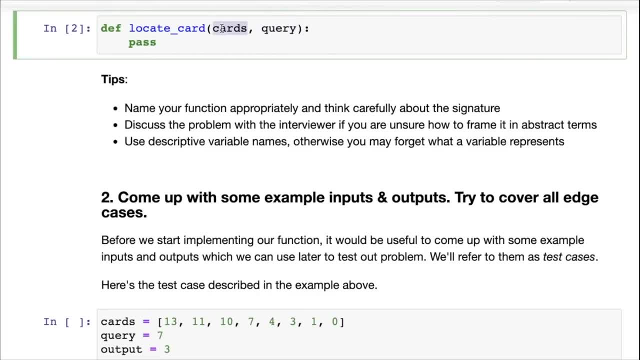 you may forget what a and B represent, So please call them what they represent, even if it can get a little long. And finally, if you're unable to come up with a function signature, if you're unable to come up with a simple description, then discuss the problem with the interviewer. 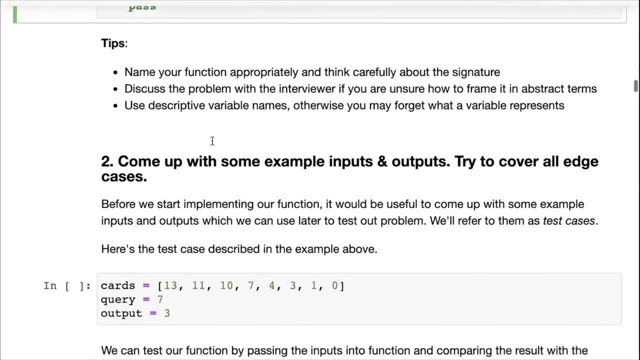 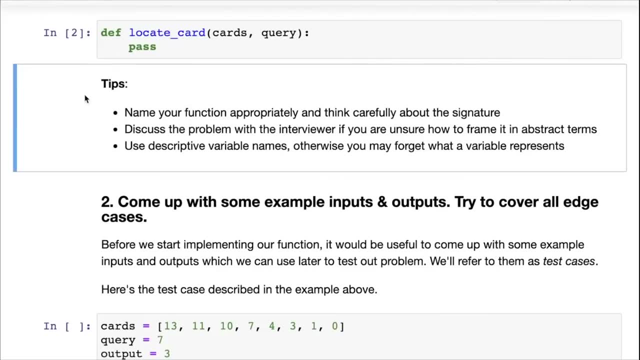 If you're unsure how to frame it in abstract terms, So keep that in mind. And this is really the first and most important step, which is stating the clarifying the problem statement and stating it clearly. Do not start coding before you have done this. 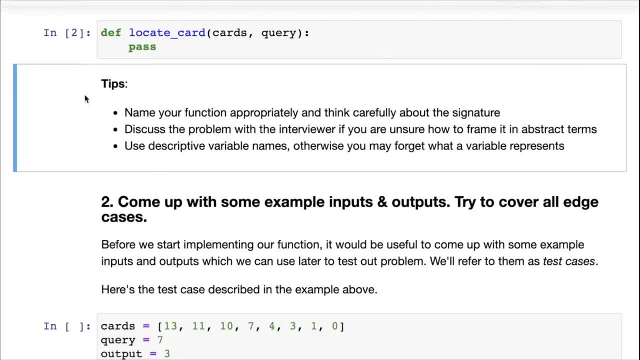 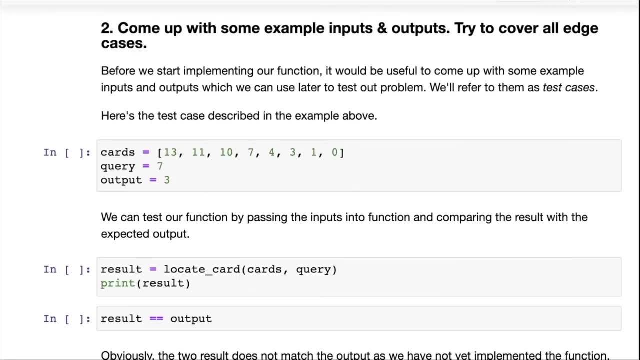 Otherwise, you may get halfway into the code and realize that you have not understood the problem at all. So step two: now we will come up with some examples, some example inputs and outputs, and our goal will be to cover all the edge cases. 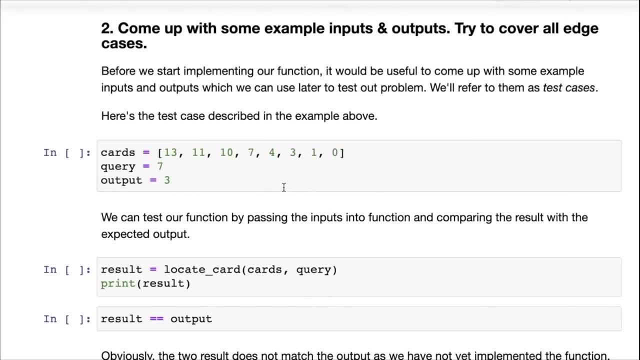 So, before we start implementing a function, we want to have some examples so that, once we implemented, the first thing we'll want to know is: is it correct? And in general, the answer is no, because coding, especially when you're getting started? 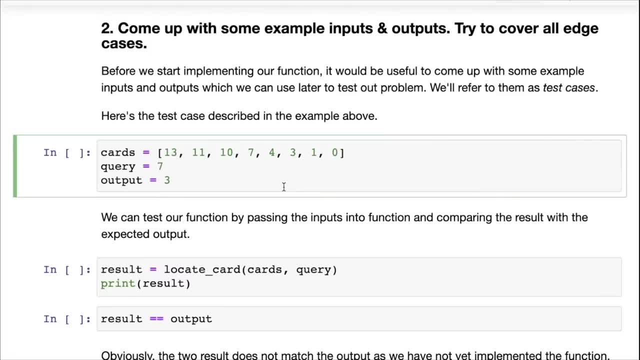 is hard because you have to think about many different scenarios. So an, and especially especially, interviews or coding, assessments are also stressful situations, So you may not be able to focus and think about all the different things that you need to keep in mind. 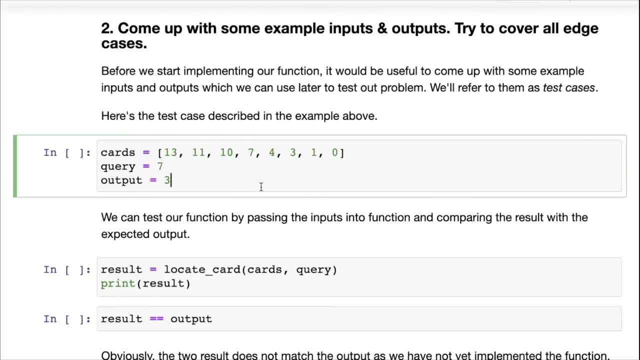 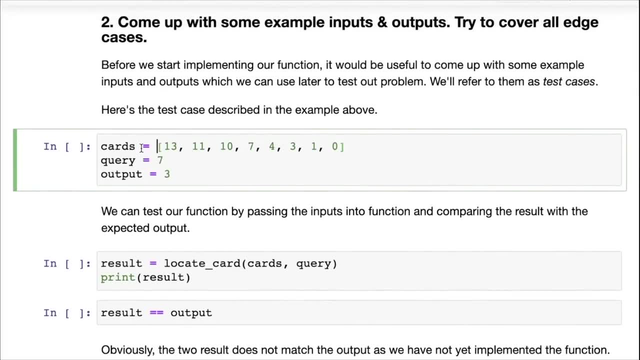 So simplest way to reduce the risk of going wrong is to use a test cases. So here's one test case that we came up with: No, The. what we've done is we've taken the information that we had listed above in the inputs and 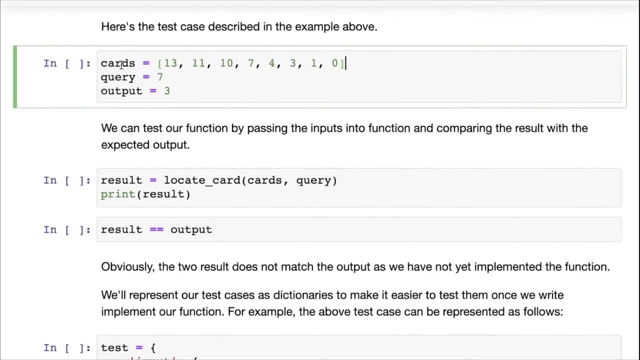 outputs and we've written it in as code. So now we have a variable called cards, which is a list of cards, a list of numbers. Then we have a query which has the value seven and then we have the output which: 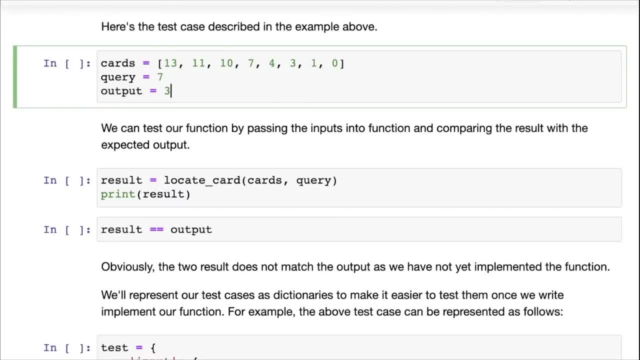 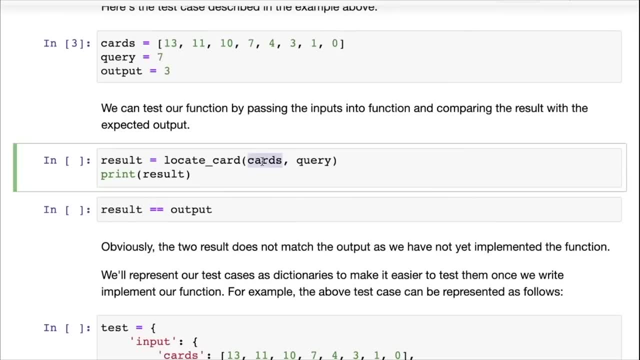 has the value three. So the expected output from the function is three, And once you have a test case, you can test your function at any point. anything you want to test, you can simply pass the input- for example cards and query- into the locate card. 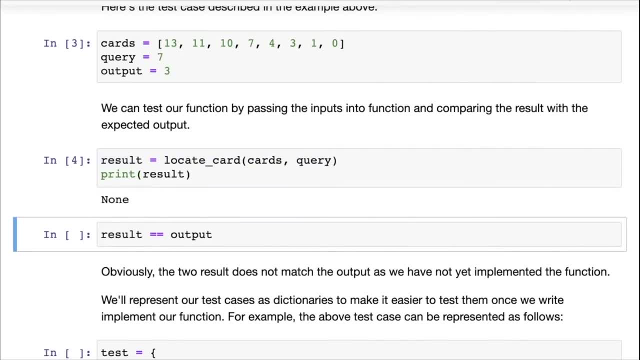 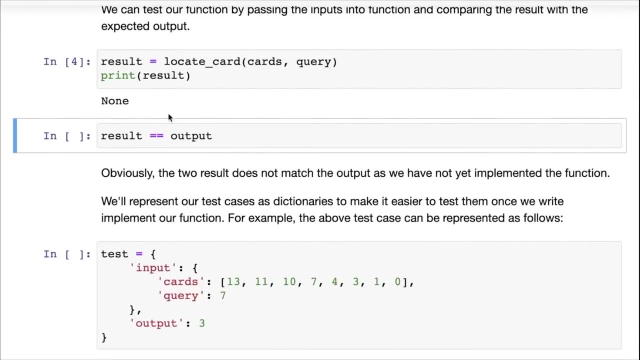 function and get back a result, And you can see here. right now, because there's nothing inside the function, the result you get back is none. but later you will start getting back a proper result from your function And what you can then do is you can compare the result with the output of the test case. 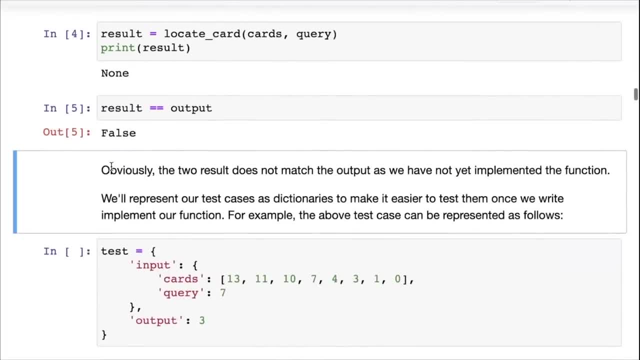 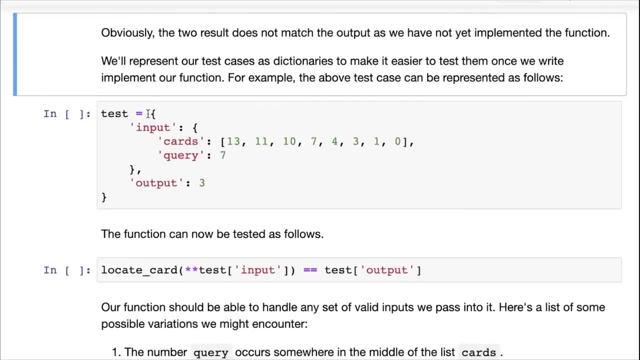 So in this case, when we compare them, obviously the output is three. The result is none. We get back false. Now, one thing we will do in this course to make testing easier, because we will be testing our algorithms again And again as we keep. 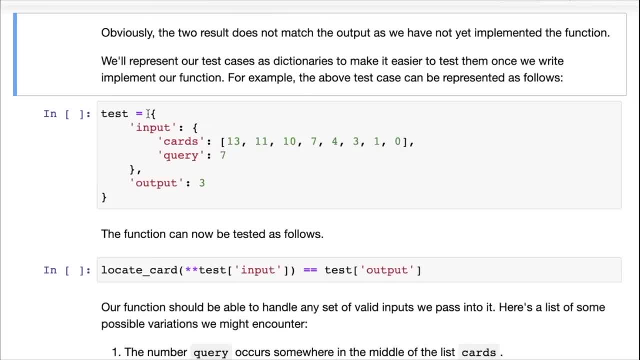 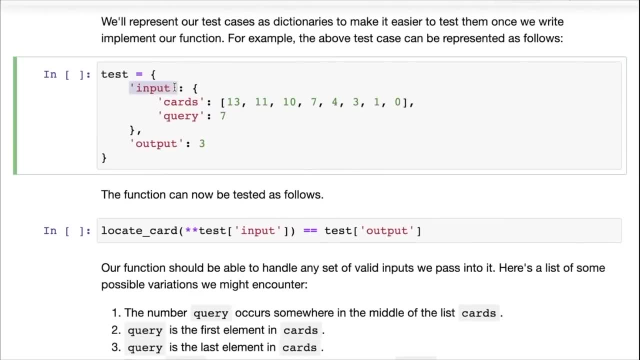 Improving them is that we will represent our test cases as dictionaries. So here, for example, this: this test case will be represented, or every test case will be represented as a dictionary containing two keys, input and output, And the input will contain one key for each argument to the function. 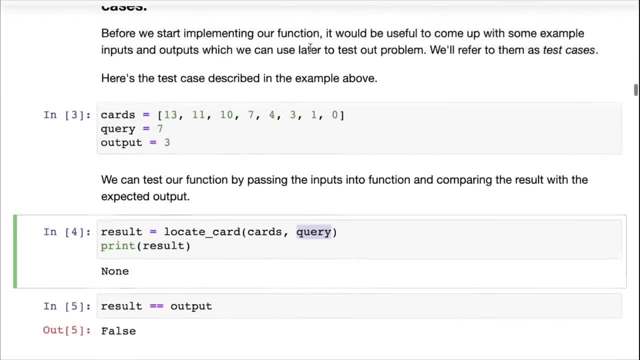 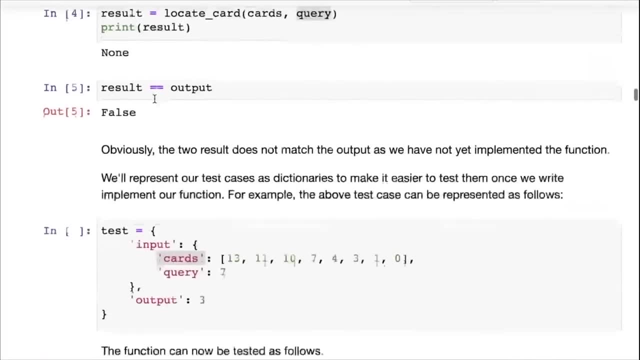 So if your functional arguments are called cards and query in the function signature- and that's why we wrote down a function signature first, so that we don't get confused- here- So if your functional arguments are called cards and query, then we can take one one. 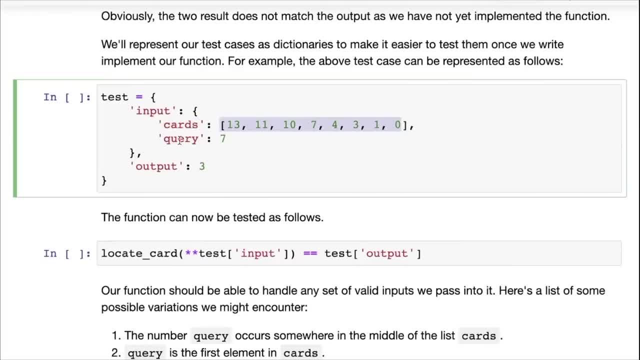 key called cards and put the value of cards there. One key called query: put the value of query there And then in the output we simply contain, we simply put the output that we expect from the function, And now you can test this function like this: 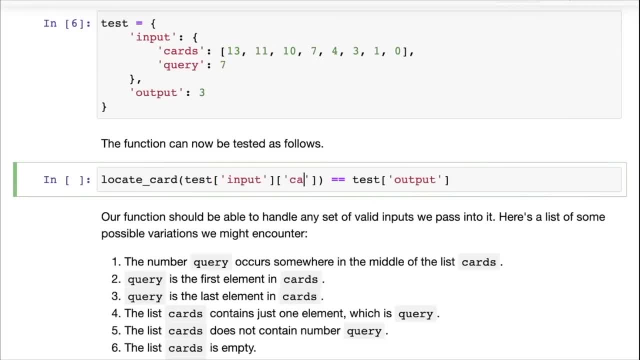 So how you might want to test it first is maybe by actually passing values like this, So you have test input cards and then test input query. Okay, But there's a trick here, whenever you have a dictionary. So here we have a dictionary with two keys and we want to pass these two keys as two. 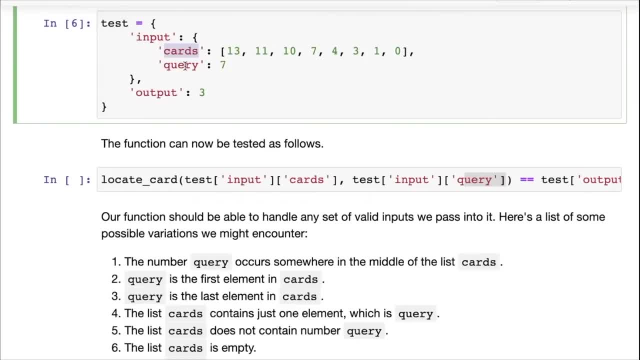 arguments to a function. So we want to pass cards as the cards argument to the function locate card and query as a query argument to locate cards. What you can do is you can simply put the dictionary itself and just write star star. Now if you write star star, what Python does is it takes the keys from this dictionary. 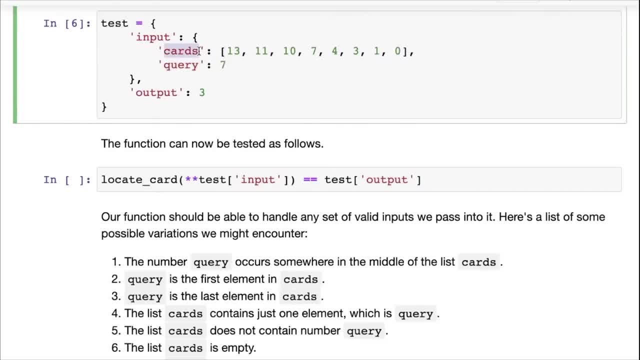 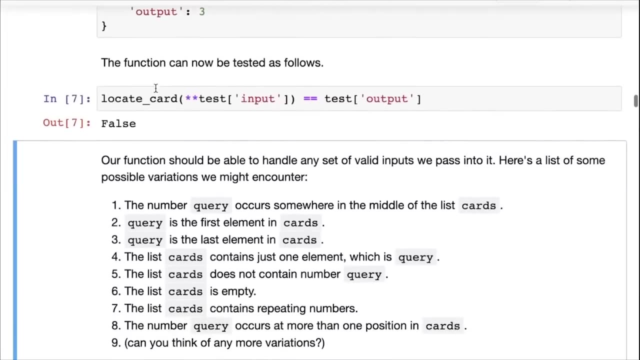 and the values are then used as arguments for Parameters with these names. So there we are now calling locate card on test input and we can compare it with test output and you can see that we get back false. So that's one test case for us. 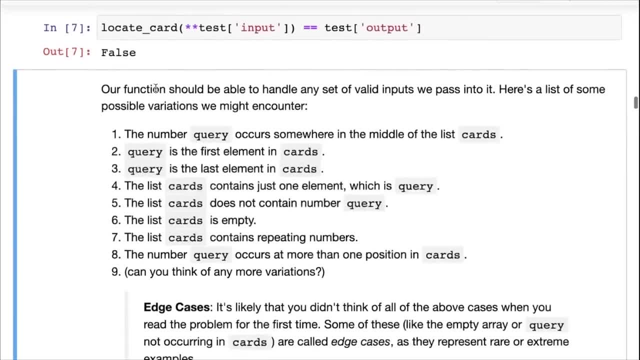 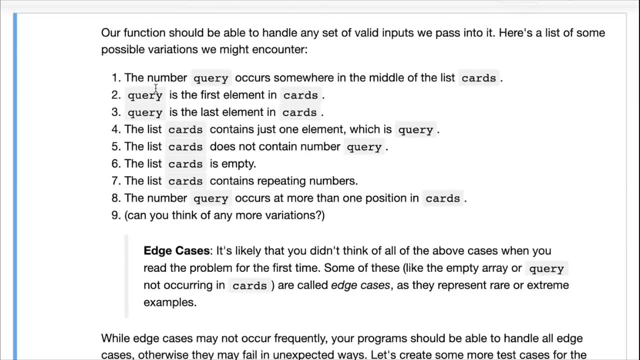 But is that enough? Is that enough for you to now start writing code? Probably not, because, out in the wild, your function should be able to handle any number of any set of valid inputs that we pass into it, And here are some possible variations that we might encounter. 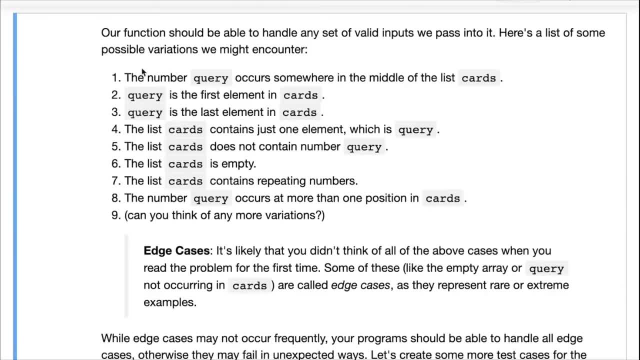 Okay, And it really helps to list them. In fact, while I was writing these variations, I realized that there are many cases that I had not thought of. So even after coding for 12, 15 years almost, I still find it really useful to list out. 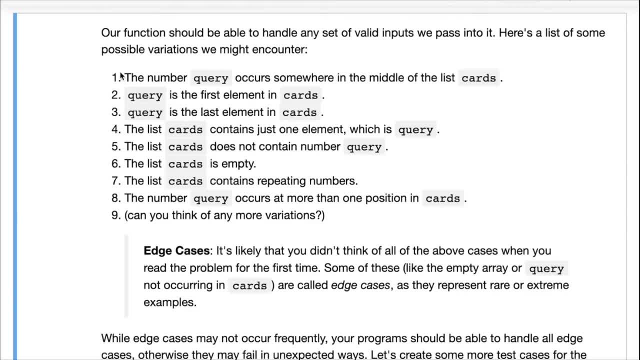 all the scenarios that we can find our input in. So the simplest scenario is that the query occurs somewhere in the middle on the list of cards. This is what you imagine when you read the question. This is what is called the general case, But then there are some special scenarios. 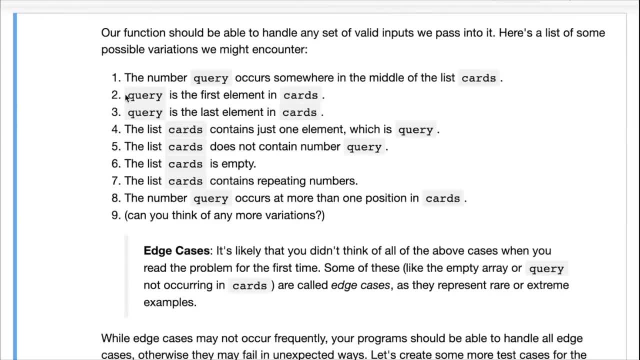 As well. What if the query is the first element in cards? And what if the query is the last element in cards? What if the list cards contains just one element, which is the query itself? or- and this is something that I had not thought of- 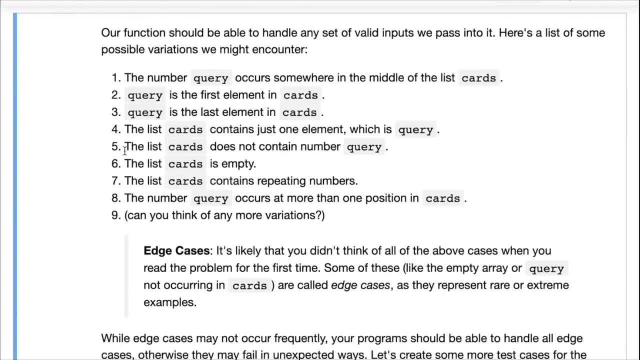 What if the list cards does not even contain the number query? What if Alice is bluffing? So what should be Bob's strategy then to figure out that the number does not exist? What if the list of cards is empty? And what if the list contains repeating numbers? 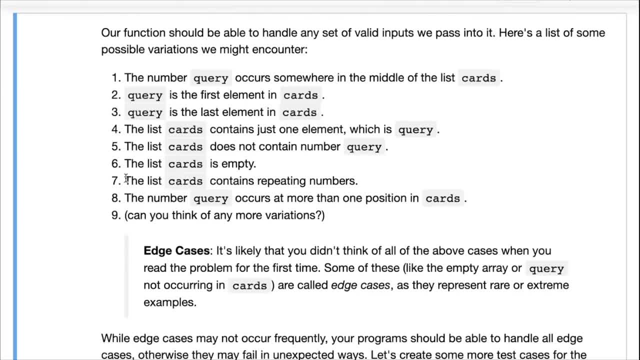 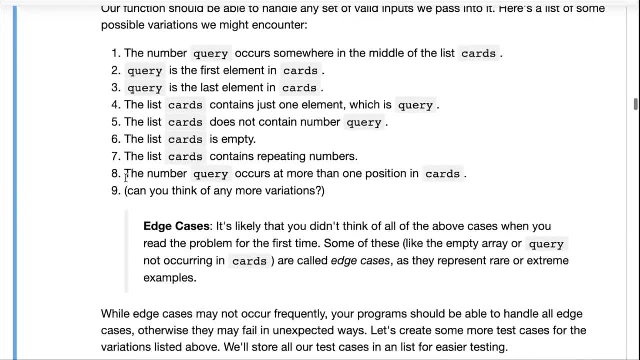 This is again another interesting thing that may not come to mind, because we said a list of numbers and we did not specify that the numbers are unique, So the list can contain repeating numbers. And finally, what if the number, the query itself, occurs more in more than one position? 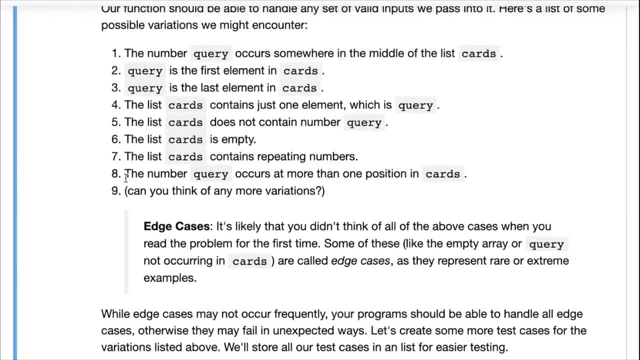 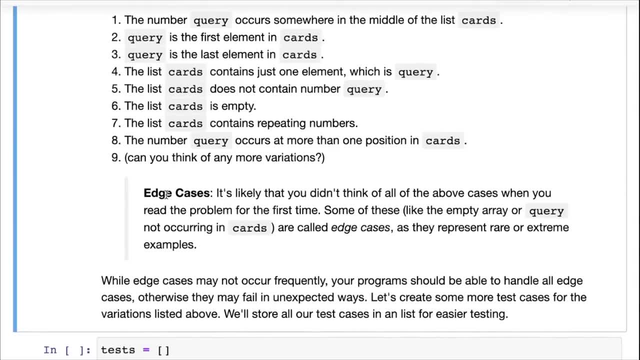 in cards. So those are eight cases that I could think of, And to see if you can think of any more variations. and it's likely that when you first heard the problem you did not think of all these cases, because you often tend to just focus on one. 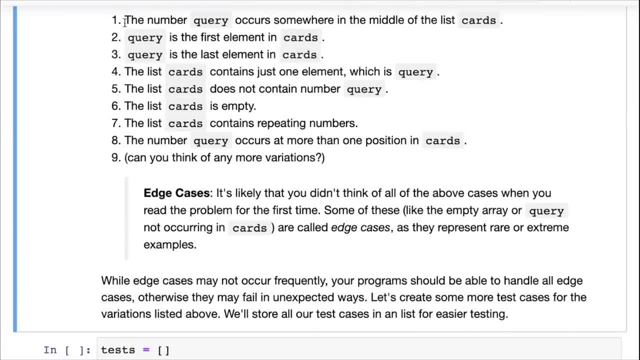 generic case. It's hard to hold too many cases in mind And that's why it helps to list them down, actually write them down in a coding interview or in a coding assessment or an interview. You may want to put this in comments. 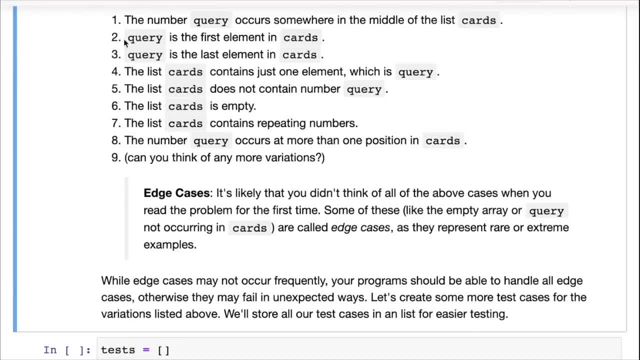 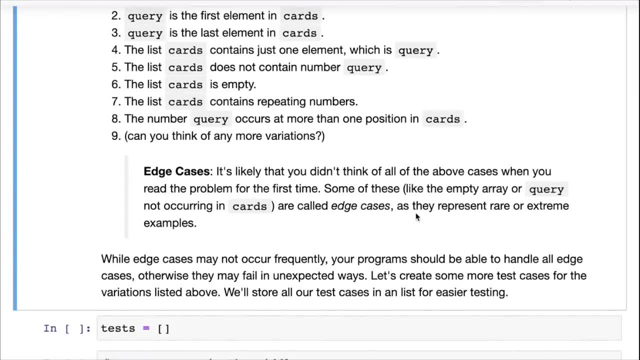 If you have a page coding page, you can just create a comments and list out all the test cases And some of these, especially things like the empty array or query not occurring in a cards. These are all edge cases because they represent rare or extreme examples. 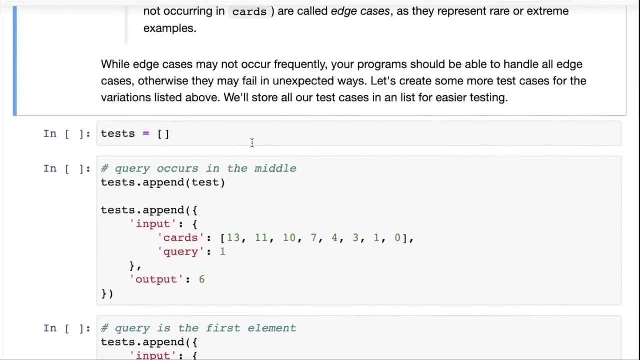 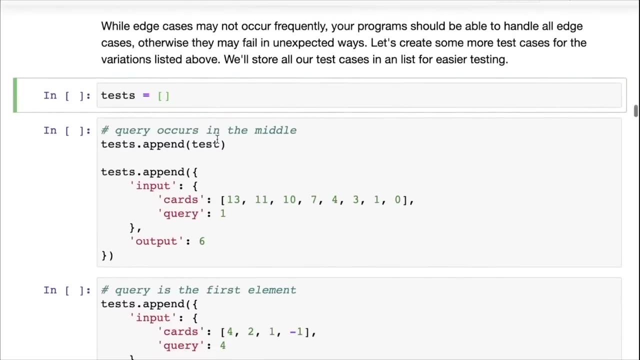 And while edge cases may not occur very frequently, your program should be able to handle edge cases. Otherwise they may fail in unexpected ways or somebody with the with malintentions can use the edge cases to hack your software. So let's create some more test cases for the variations that we've listed and we'll store. 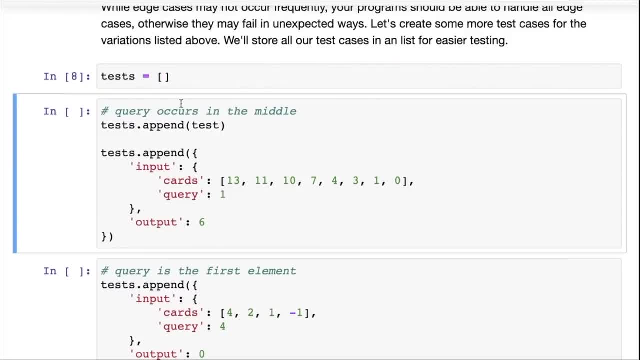 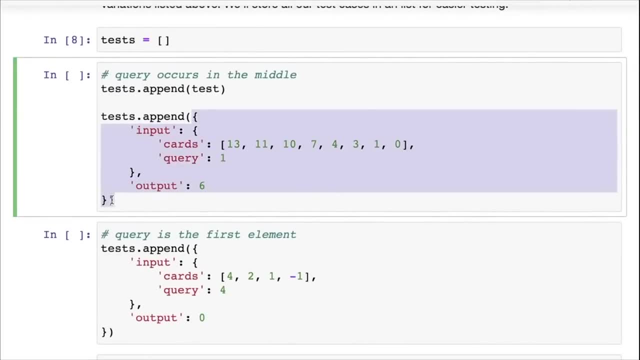 all our test cases in a list for easier testing. So here we are creating a list called tests, and this time we will create all our test cases in the format that we discussed, which is a dictionary format, and we will keep appending them to our list. 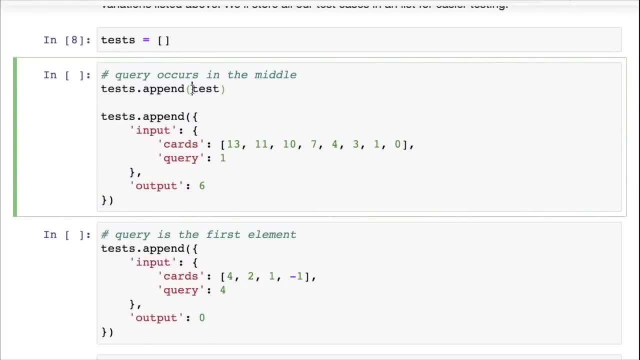 Now, if you do not understand lists and dictionaries and appending, then you can go back and review some of the basic material on Python which is linked at the top of this notebook. So first we take the one test case that we already have. We put that and we take maybe one more example of the query occurring somewhere in the middle. 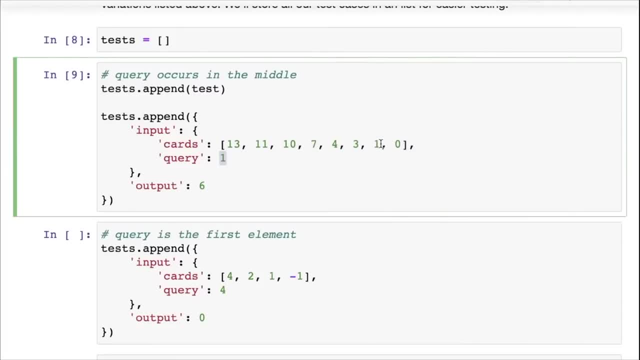 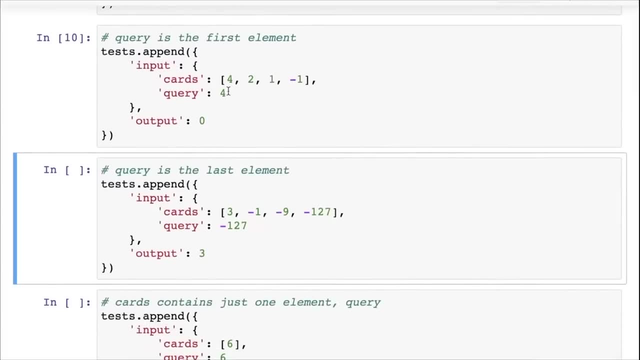 So here you can see, this is the cards list, And then the query. one occurs somewhere in the middle, although it's closer to one end. Then here's one case where the query is the first element four and the output- obviously the output expected is zero. 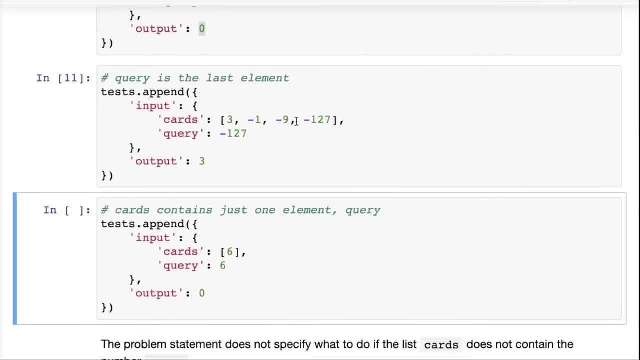 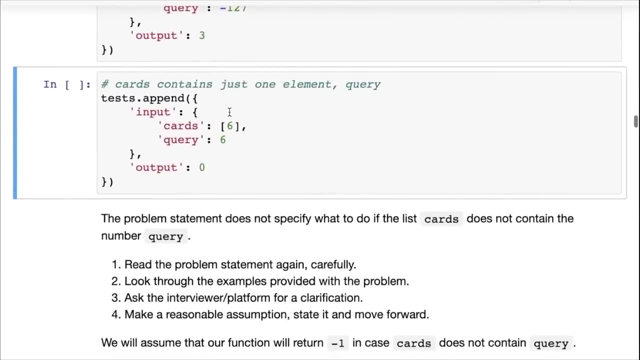 Here's one case where the query is the last element minus one, 27.. And this is another thing. The numbers could be negative as well, Something you may want to keep in mind. Here's another one. The weather card contains the cards contains just one element, the query itself. 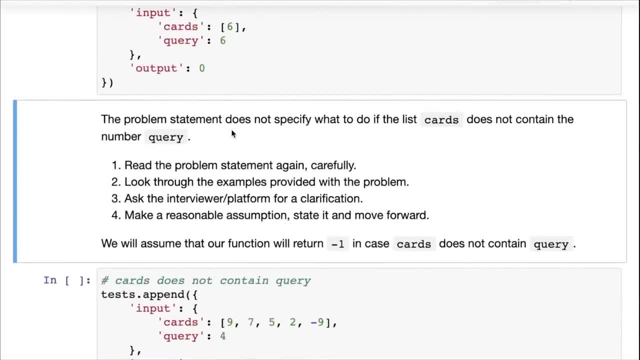 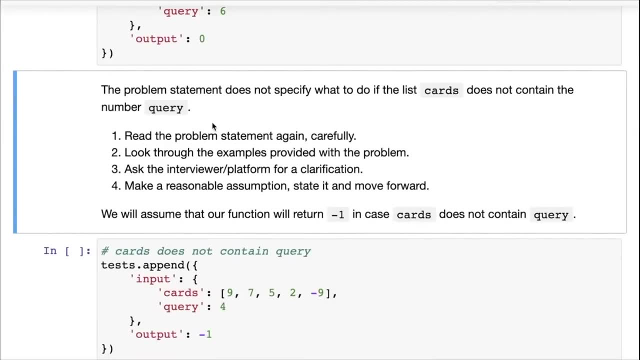 Now, The problem does not state what to do if the list cards does not contain the number query, And you may often face these questions where it may not be clear what to do in a certain situation or if a certain situation can occur, And when you have questions like this, this is a process you should follow. 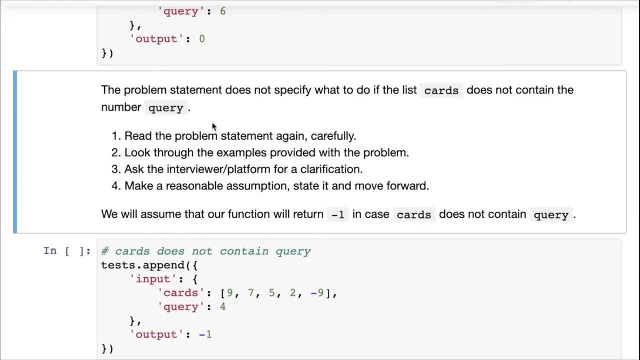 Step one, read the problem statement carefully or ask the interview to repeat the question. So read the problem statement carefully And you may. you will often find hints, And sometimes these hints are just single number, single words Somewhere. Often you will also find some examples, provided with the problem. 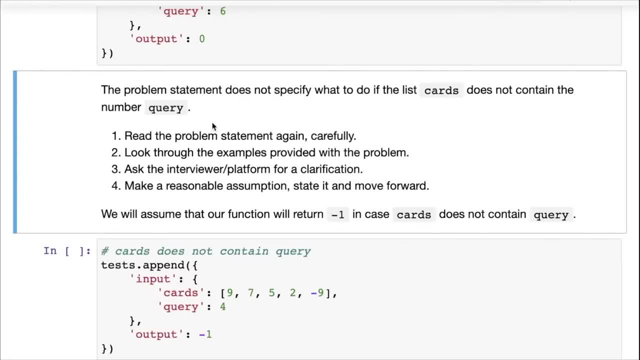 You will also find. if you scroll down to the bottom, you will find some conditions. You will find limits on what the numbers can be, whether they can be integers or can be decimals, whether they can be negative or positive. So it's important to read the problem carefully before you start coding and look through the 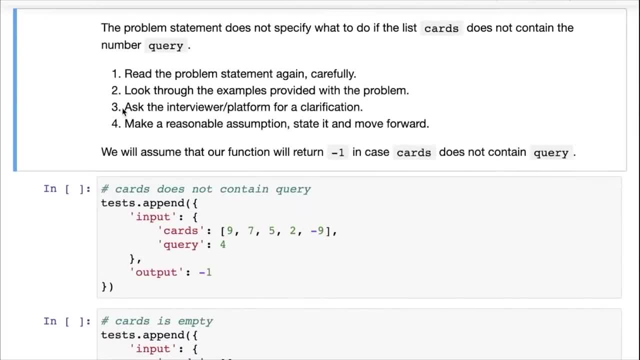 examples and then ask the interviewer or maybe post a question on the platform for a clarification. Often it happens that interviewers, because they take so many interviews, they may forget to specify Certain detail, and or they might expect you to ask the question because you should. 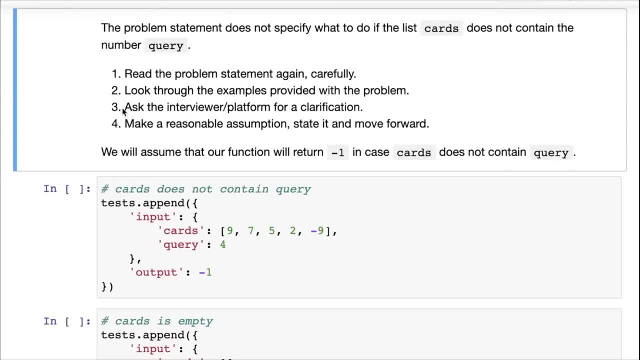 not be coding with an insufficient requirement. So to clarify the specifications of the problem is very important. So if you have any doubt, ask the interviewer. even if you are somewhat sure about it but just want to verify, it's a good idea to ask. 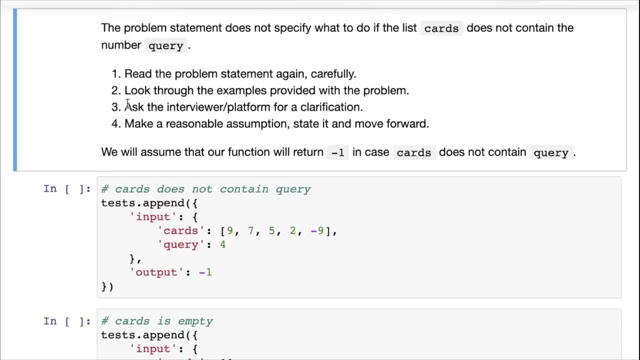 Then finally, if you are done with all of these and you still do not have a solution, then you just make a reasonable assumption stated and move forward. Okay, So we will assume that our function will return minus one in case cards does not contain query. 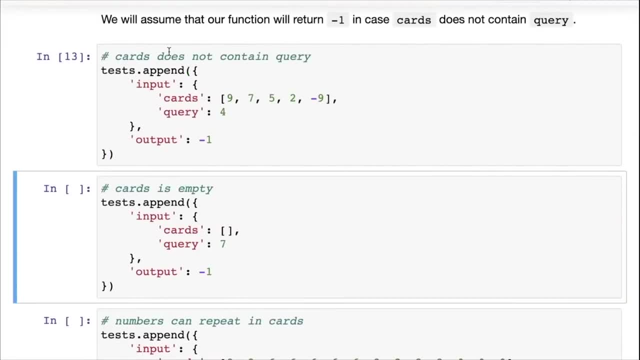 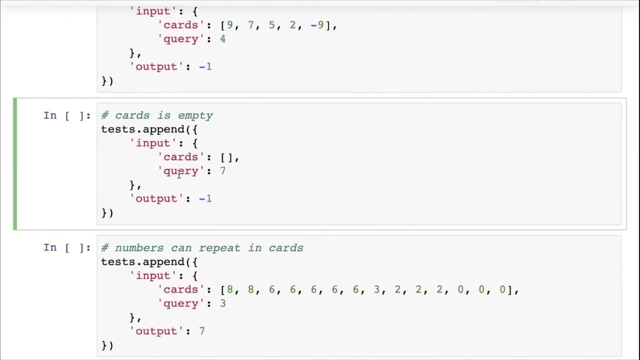 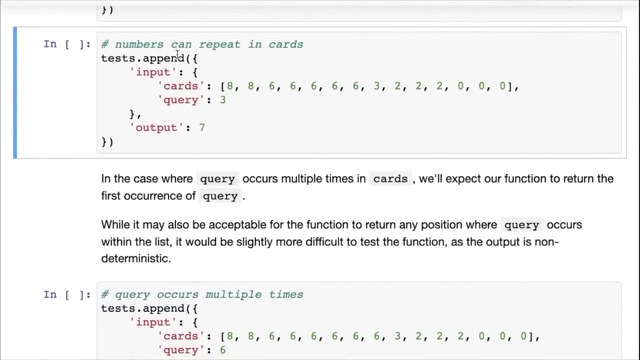 So if cards does not contain query, then we return. we expect the function to return minus one. Now here's one other case where the cards are is empty and obviously then it does not contain the query as well. And finally, there's one last case, which is the number itself can repeat in cards. 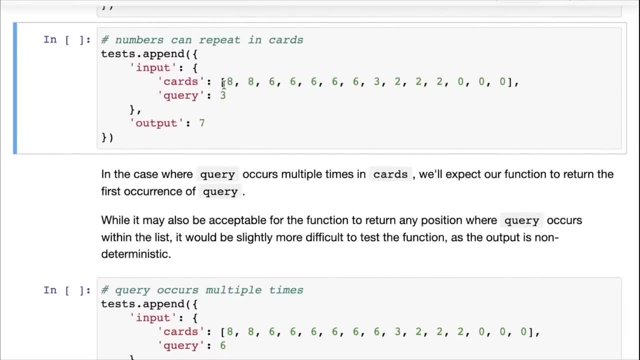 Numbers can repeat in cards And then the query itself can repeat. So here the query does not repeat, three does not repeat, but the numbers on the in the cards that I do repeat. And the last case is when the query itself repeats. 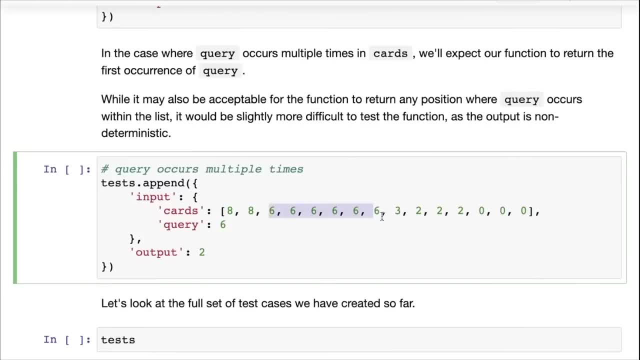 So you can see here in cards the query occurs many times. Once again, it is not specified what to do here, And sometimes it may be okay. Sometimes the problem statement may just say that return any one position. but more likely than not, what you will want to do is you may want to make it more deterministic. 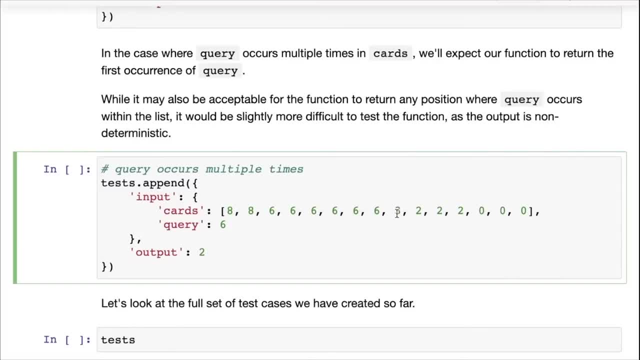 Okay, And that will also make it easy for you to test the function. So what we can say? we can impose this additional restriction that we will expect our function to return the first occurrence of query, And that will make it easier for us to test. 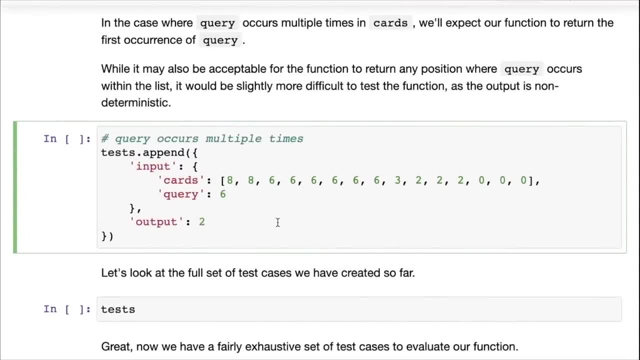 So that when we, when we're testing a problem, we we know that if we're getting a failure, it's not because of multiple possible answers, but it's because of some issue in our code. Right, So you want to get good feedback from failures. 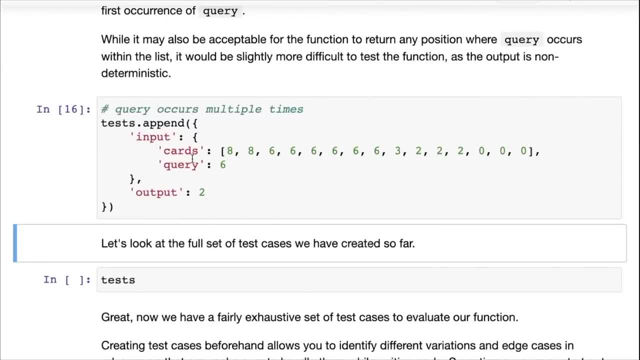 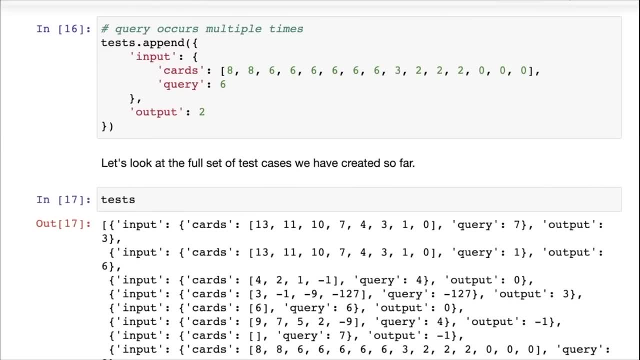 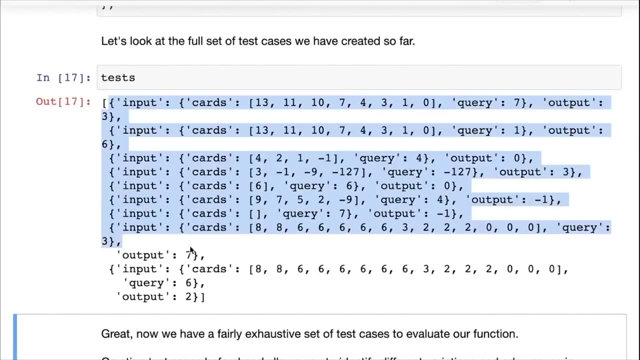 And that's why You want your tests to be deterministic. So here is the final test, and now we can see the full list of test cases. So now we can see the list of test cases here. So you have about eight or 10 test cases here. 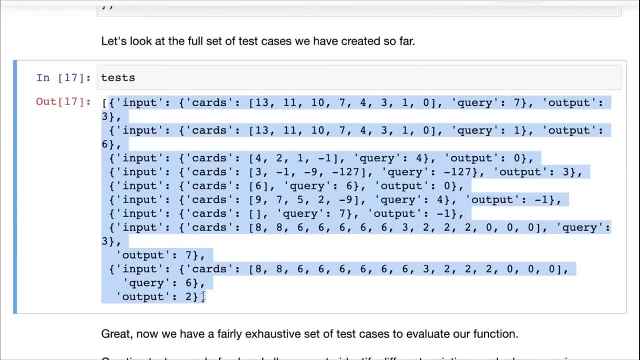 You may not need to create this many test cases in an interview or a coding assessment, depending on how much time you have, but you should create at least a few. at least cover the three or four edge cases. A good number to aim for would be five. 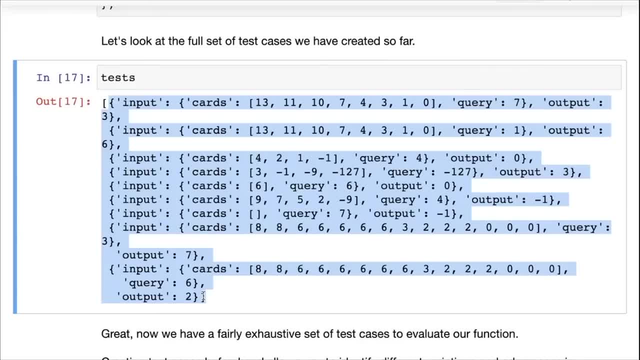 And this will not only help you in the coding interview, help you solve the problem. This will also be appreciated by the interviewer because it shows that you're thinking about the problem. So definitely take a minute or two Now. we've spent 10, 15 minutes talking about this, but once you start applying this technique, 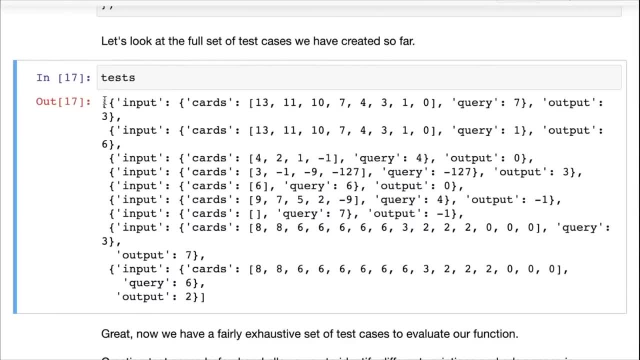 over and over, you will see that you will start creating test cases in seconds. So as soon as you read the problem and you stayed the problem, Fine. Find the input format, find the output format, write a function signature and write the test. 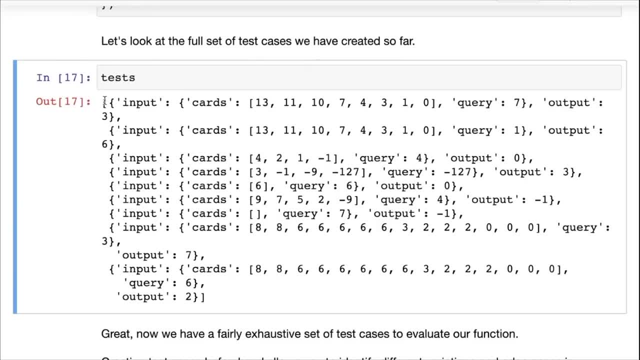 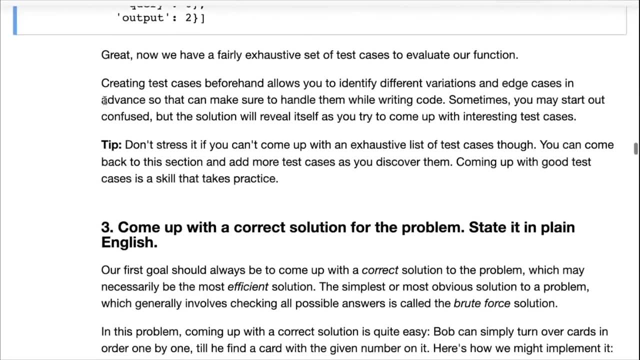 Then you will start working on tests, The ideas will automatically start coming to you And within maybe two or three minutes you will be done with both, all two, both of these steps. So great. We now have a fairly exhaustive set of test cases and creating test cases beforehand. 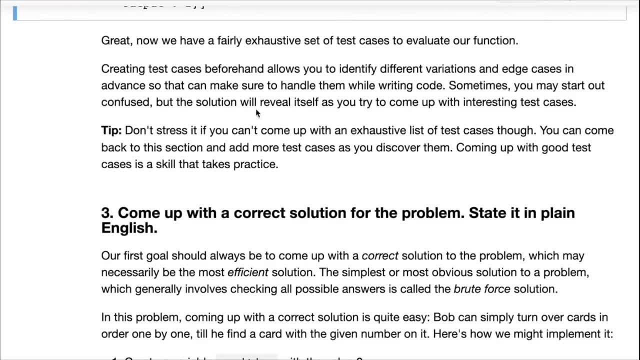 allows you to identify different variations and edge cases, And sometimes it may happen that you may have no clue how to work on the problem. You may feel completely confused, but if you simply start writing multiple test cases and start looking at them, like literally just staring at the test cases, the question 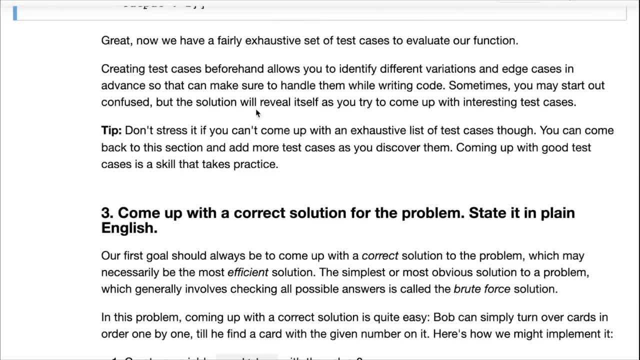 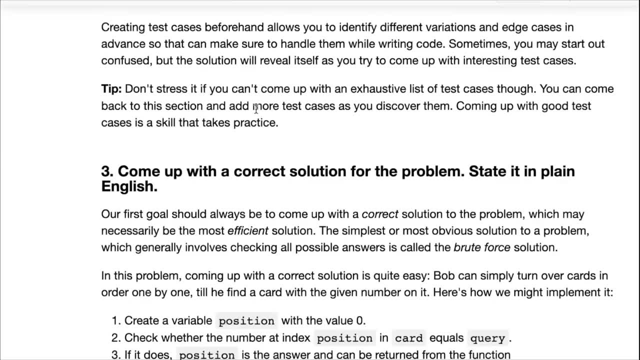 and the answer, the solution will reveal itself to you. So don't underestimate the power of writing things down and don't stress it. Don't stress out If you can't come up with an exhaustive list of test cases, because this takes time. it's. 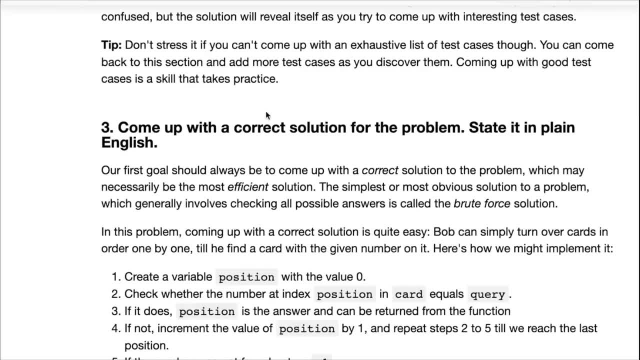 a skill that you cultivate with time. So what you can do is you can list out, maybe, the test cases that come to your mind right now and put them in a single place and keep coming back Whenever a new test case comes to mind, while coding or while discussing or while analyzing. 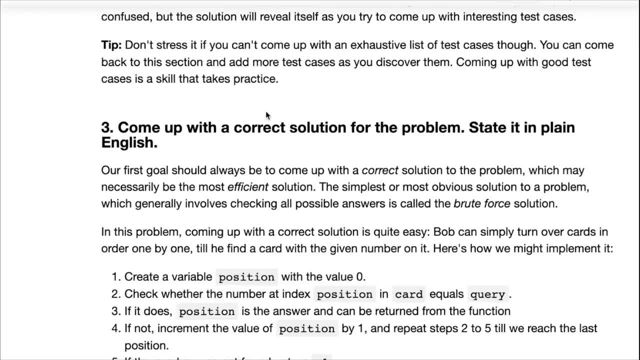 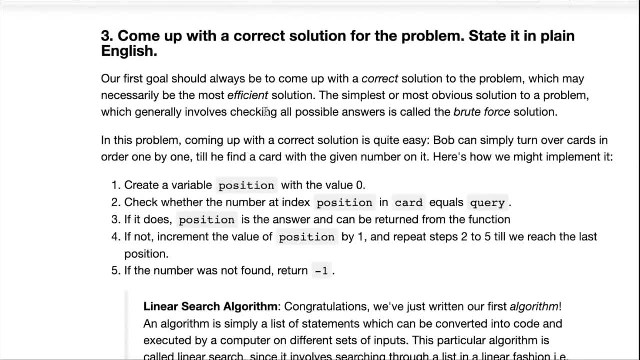 you can just come back to the same place and write down the test case. The important thing is that you have a single place where you're listing all test cases. So we've written our test cases now and now we can come up with the correct solution. 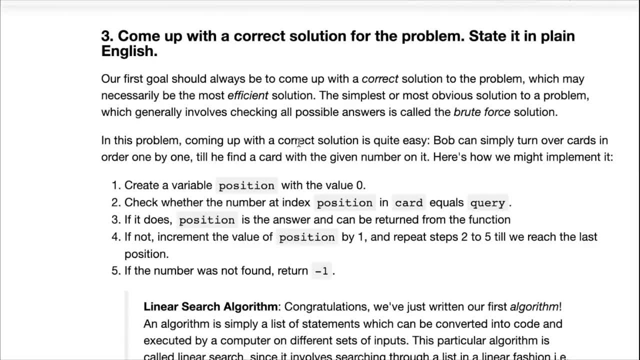 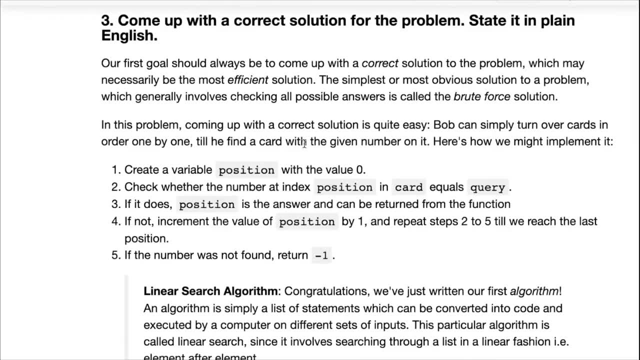 And how do you come up with the correct solution? Not by writing code, but first stating it in plain English. So your first goal And Okay. By correct we do not mean the best or the most efficient solution. First we want to solve the problem. 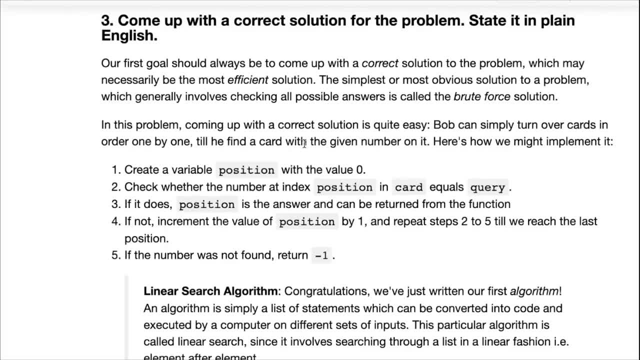 We want to figure out where the particular number lies in the list and not to minimize, because that's solving two problems at once And sometimes that can get tricky. So first aim for correctness, then aim for efficiency, and the simplest or the most obvious solution, which almost always exists and is almost always very easy to see, involves checking. 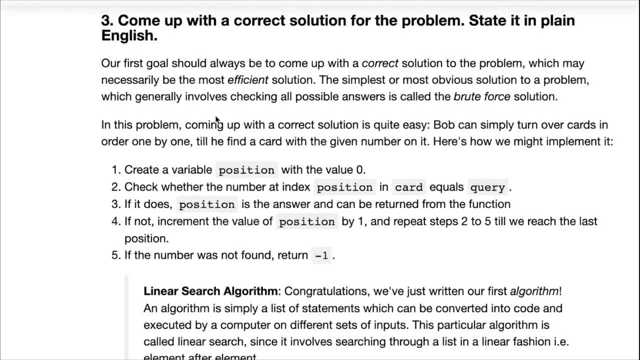 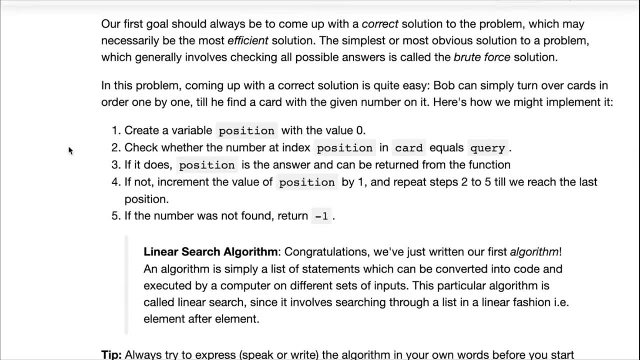 all the possible possible answers, And this is also called the brute force solution. So in this problem, coming up with a brute force solution is quite easy. Bob can simply turn over the cards in order, one by one, till he finds the card with the. 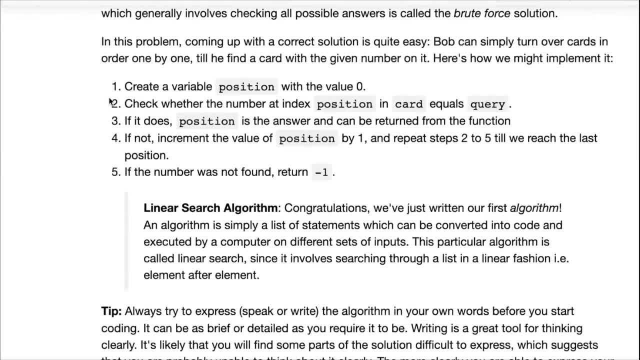 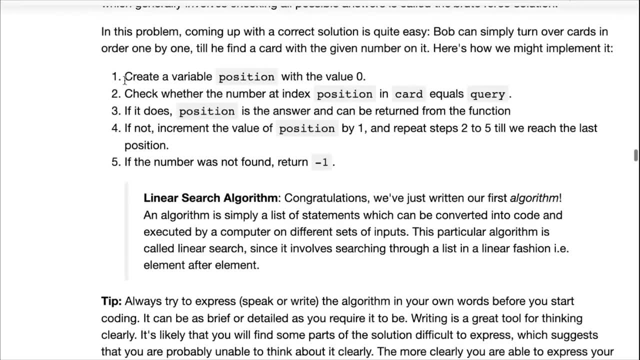 given number on it. So this is what, this is how it might work if we want to implement it in code, And this is where writing it in your own words becomes important. So we create a variable called position inside a function with the value zero. then we check. 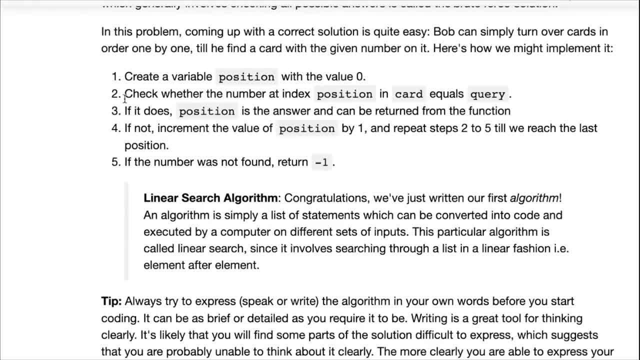 that. Let the index position in the card list equals query or not. Now, if it does, since we're starting from the beginning- if it does, then position is the answer and we can return it from our function. But if it doesn't, then we simply increment the value of position by one and then we repeat. 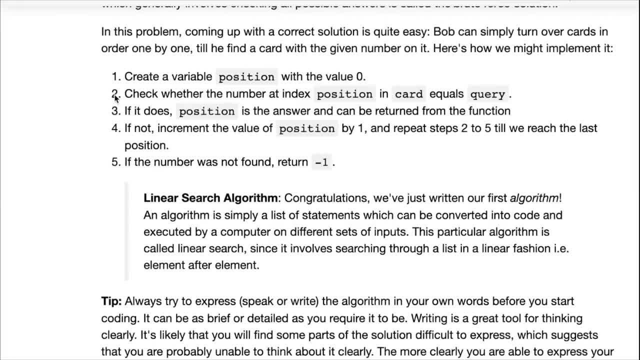 the steps. So we go back to step two and then we check whether the number at the index position on in cards equals query And once again, if it does, we return position. If not, we increment the position once again and repeat. 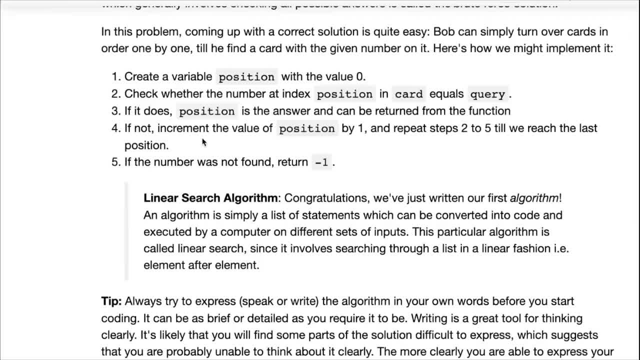 And we repeat that till we reach the last position. And if the number was not found, we return minus one. So it's a simple four, five step description. Doesn't take very long. You can either say it out loud to the interviewer. 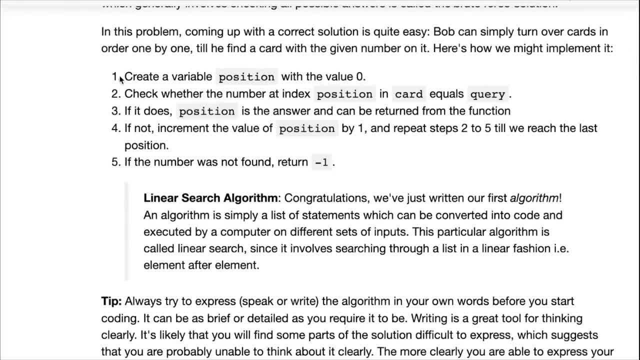 They will also appreciate it, that they will know, you know. you may know that you know the brute force solution and you may not say it because it seems too simple or obvious, but the interview does. the interviewer doesn't know that. 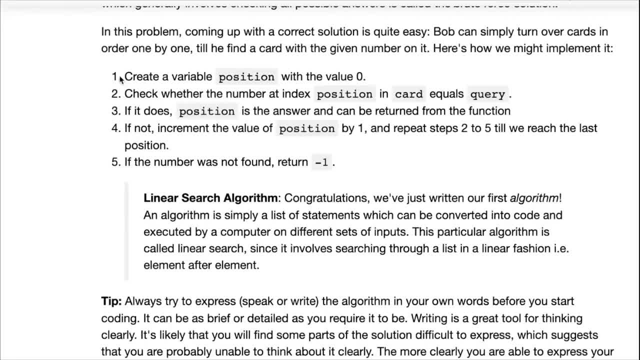 So it's important to state the brute force solution. You may say that I The solution is fairly straightforward and it goes like this: steps one, two, three, four just take 30 seconds, But at the very least it informs the interviewer that you're able to think of some solution. 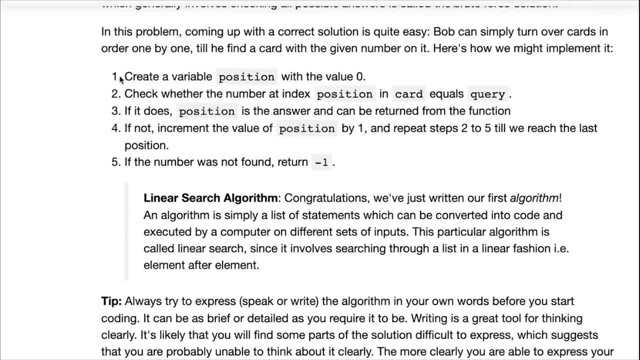 And it happens very often- I've seen it in interviews- where 30, 40 minutes have passed out of 45 minutes and not a single solution has been proposed so far, even though many lines of code have been written. So it's important to state your solution. 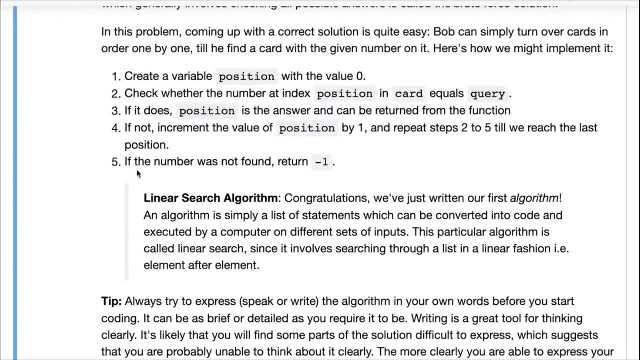 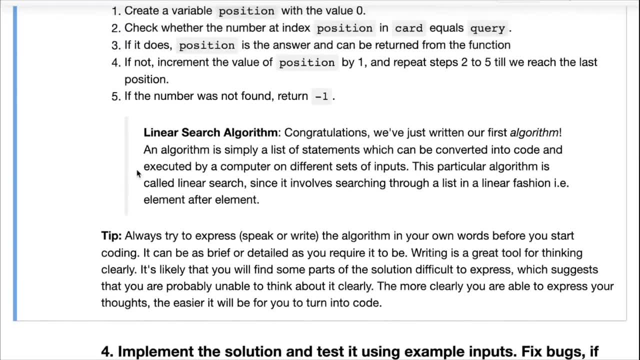 And if you state your solution, the interviewer will also help you and correct you as you go forward. Right, It's a narrative experience, It is a discussion, So use that. And if you are in a coding assessment, you may just want to write out a few comments. 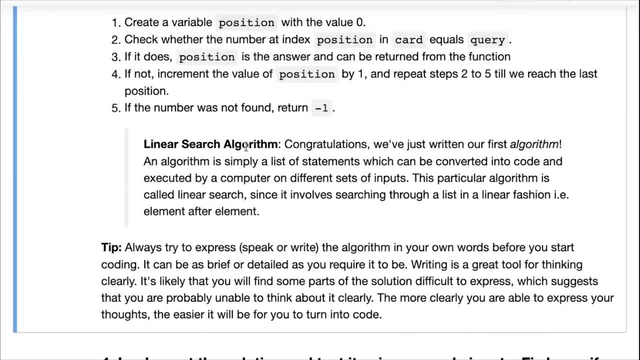 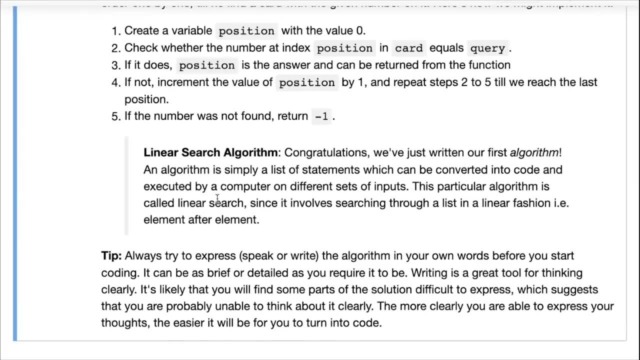 And what we've implemented- implemented here is congratulations- is just our first algorithm. And then algorithm is simply a list of statements, a list of steps that can be converted into code and executed by a computer on different sets of inputs. So this particular algorithm, 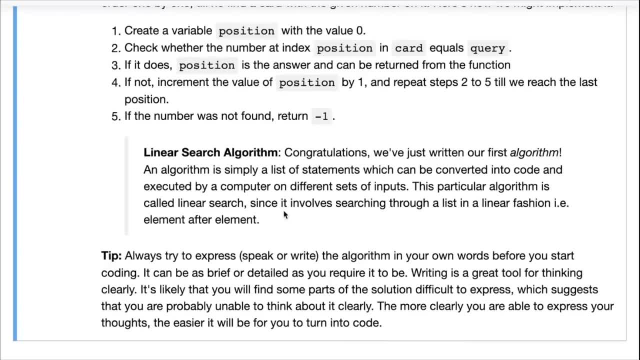 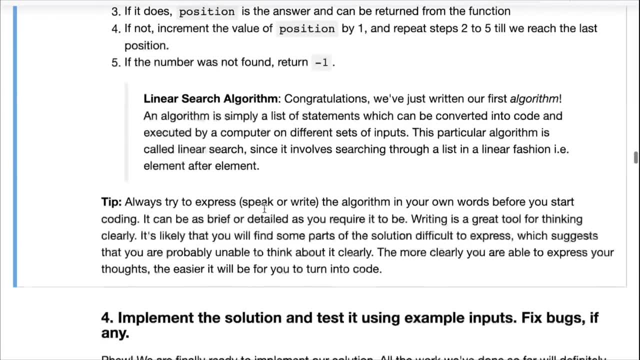 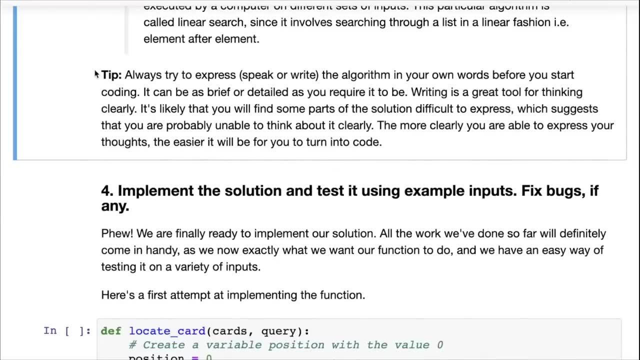 Is called a linear search because it involves searching through a list in a linear fashion, element by element. So now we're ready to implement the solution. and just a quick tip: as I've already said, always try to express the algorithm in your own words, and it can be as brief or as detailed. 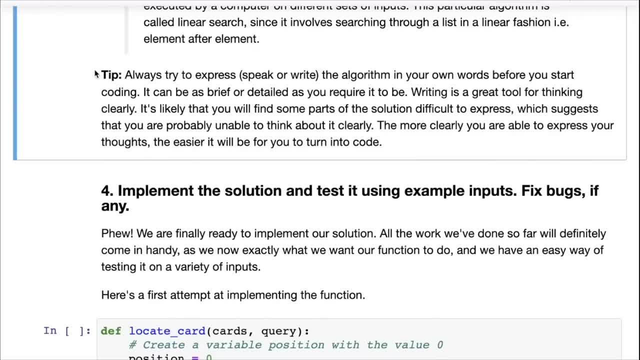 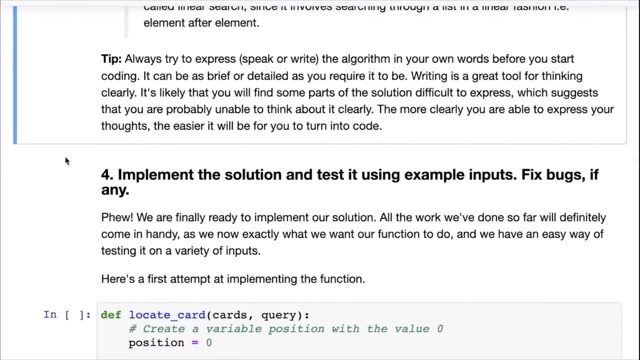 as you like, And don't underestimate the power of writing. Writing can be a great tool for thinking. It's likely that you will find that some part of the solution is difficult for you to express And that simply suggests that you are probably unable to think about that part clearly. 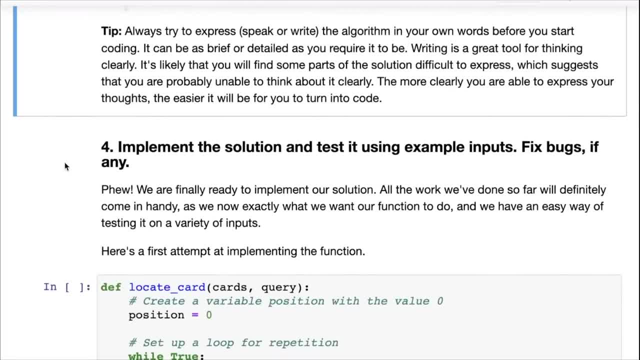 So the most more clearly you're able to express your thoughts, the easier it will be for you to turn it into code, and you will not have to come up with a strategy while you're writing the code, So you can focus on coding and focus on avoiding errors. 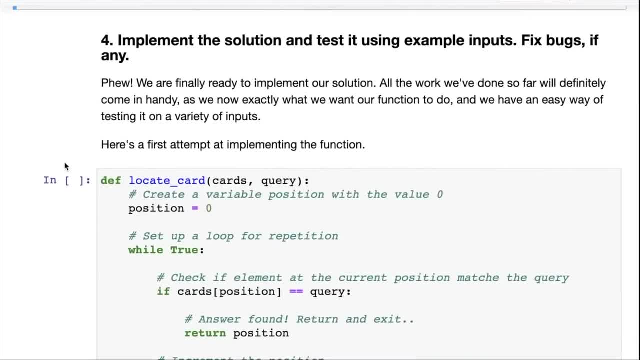 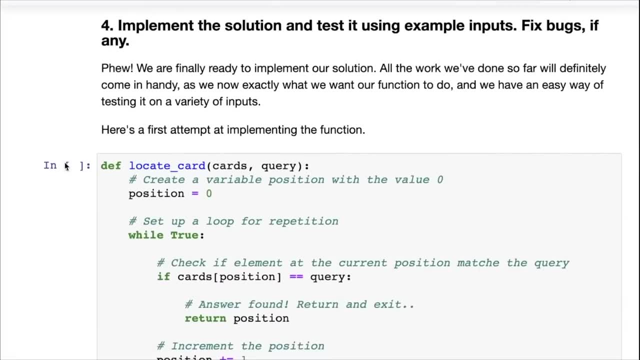 And that brings us to the next step: implement the solution And then test it using the example input. So now you can see how everything comes together. We've already know what the function signature looks like, what the inputs look like. We already have some test cases, and through the test cases we've also identified what 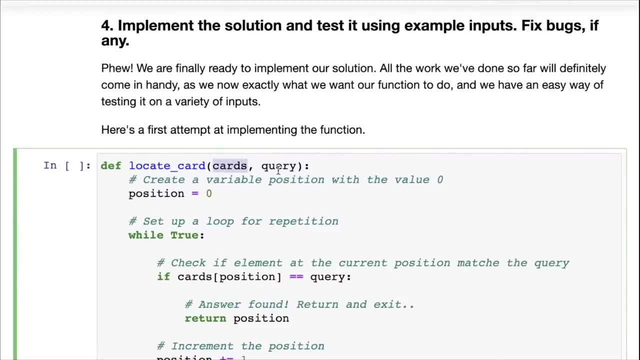 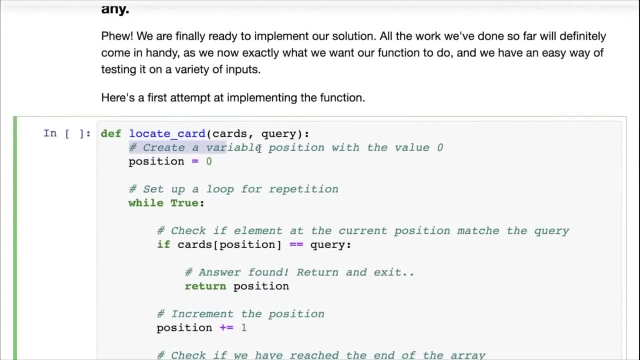 are the different edge cases we need to handle, And we've already written out a description, a rough description, of what the algorithm looks like And, in fact, what you can do is you can simply write out comments within your function as the English description. 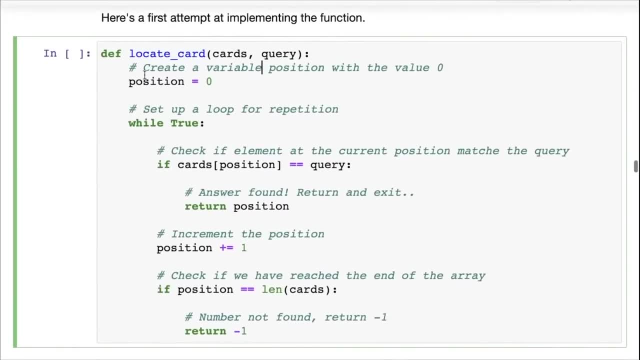 Then you simply need to fill out code for those comments. So, for instance, here are What are the five steps that we had just written down: create a variable position with the value zero. set up a loop. check if the element is matches the query. 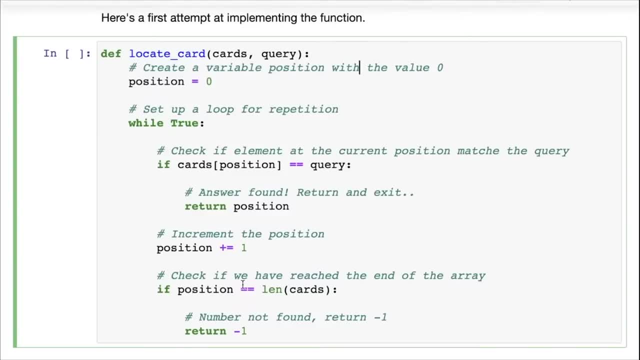 If yes, the answer is found. If not, increment the position and then go back and then check if you've reached the end of the area. If you have, then we return minus one. So then the code now is pretty straightforward. Now we create the position variable zero. 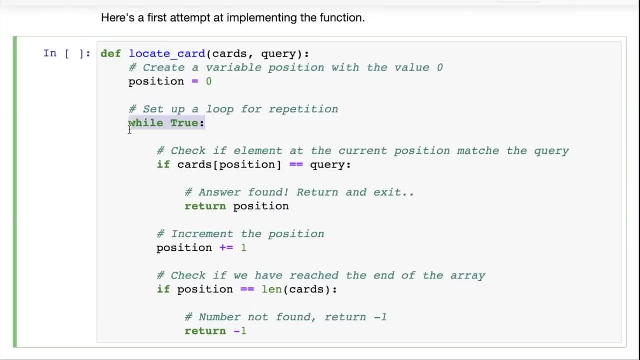 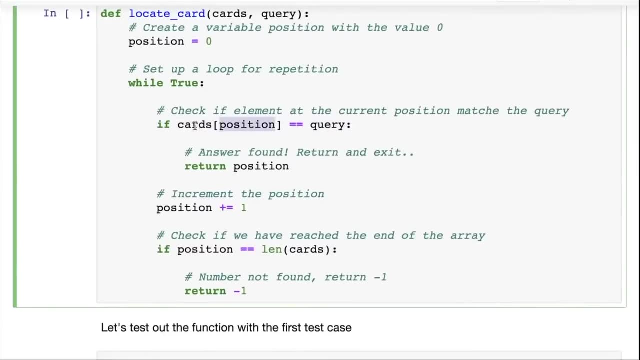 We set while true. So while true kicks off a loop and we just want to kick a first. set up a loop and then we can break out of it when we need to. Then we check if the element at the value position matches the query. 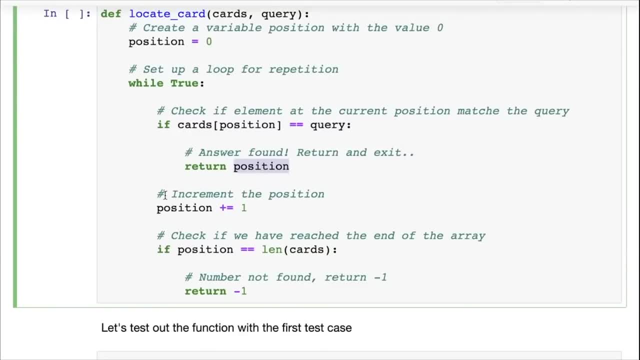 If it does, we return the position. if it doesn't, So. if it doesn't, then this: we come to this part. If it does, then we send the function exits and none of this code gets executed. But if it doesn't, then we increment the position and then we check if we have reached the end. 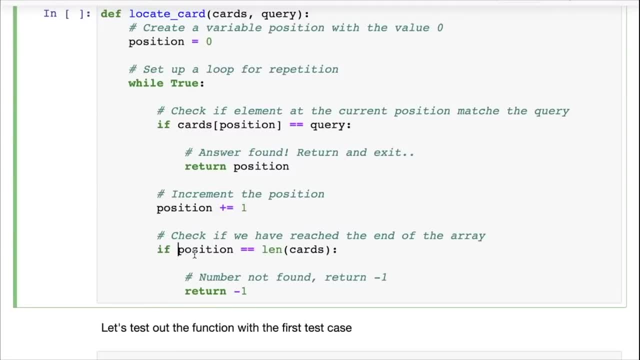 Now, if you have the each the end, obviously we don't want to continue, So we can simply return minus one and exit the loop and exit the function itself. But if it, if you have not reached the end, then we go back to the top of the loop and 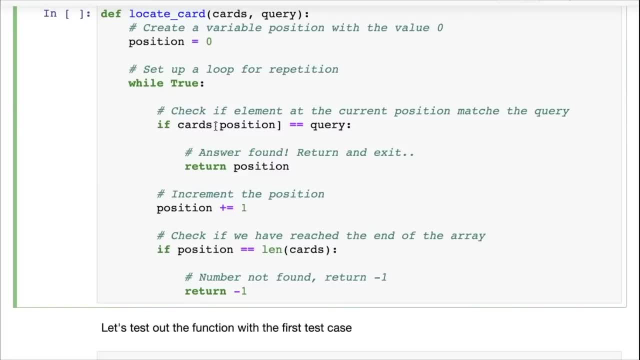 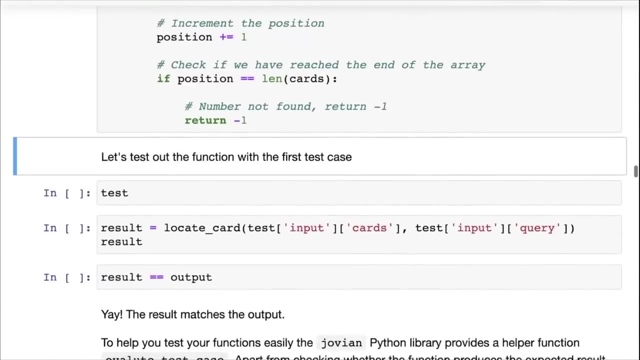 now position starts out with value one. So we check value zero. one, two, three, so on up to the end of the area. Simple enough, Great. So now we have our first function, and let's test our function with the first test case. 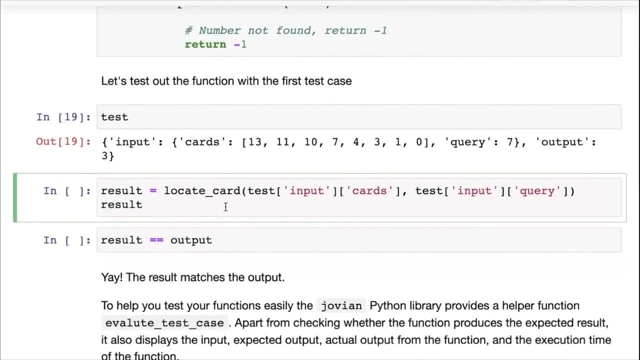 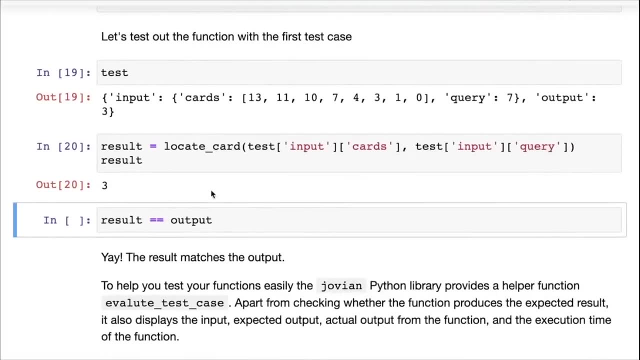 So here's our test case once again, and we can simply call locate card with the test input and the test, the cards and the query, And this is a result, Right, And you can already see that the result matches the output, And that's why, when we compare them, we get the value too. 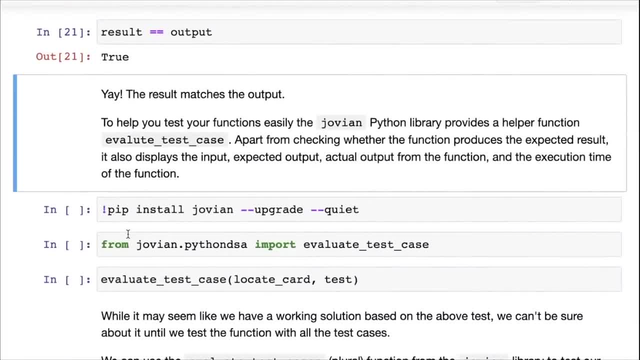 So, yeah, the results match the output, And because this is something that you should be doing very often in this course, we have put together a small function for you within the Jovian Python library. So the Jovian platform also offers a Python helper library. that is, that contains some 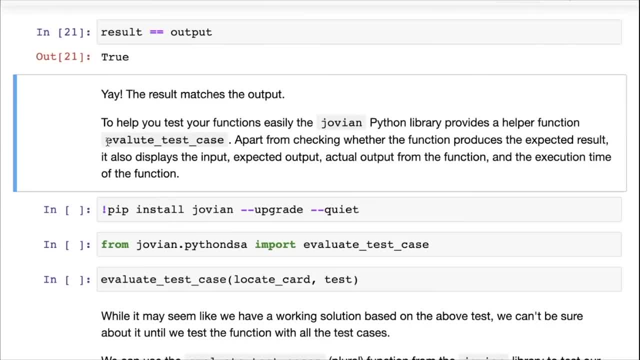 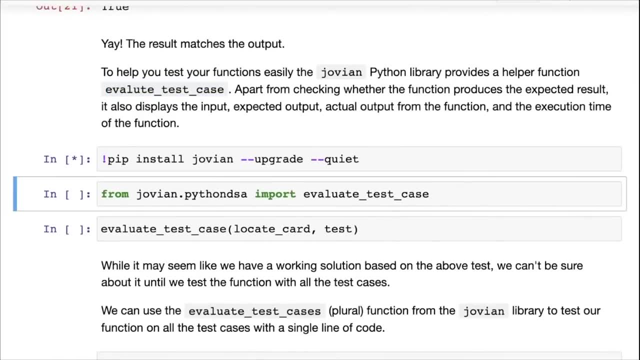 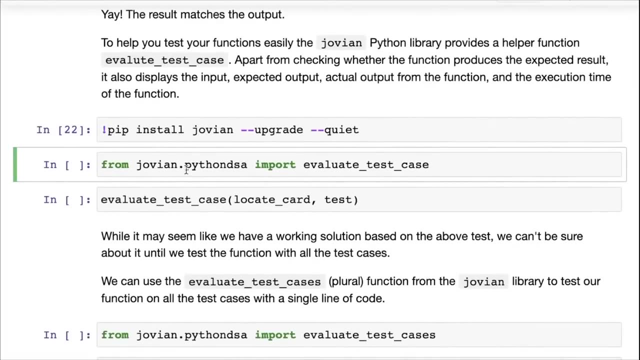 utility functions. So we've put together a small function for you called evaluate test case, and you can write it on your own as well, But you can use this library version. So let's install the library. We will install the Jovian library using pip. install Jovian minus minus upgrade. 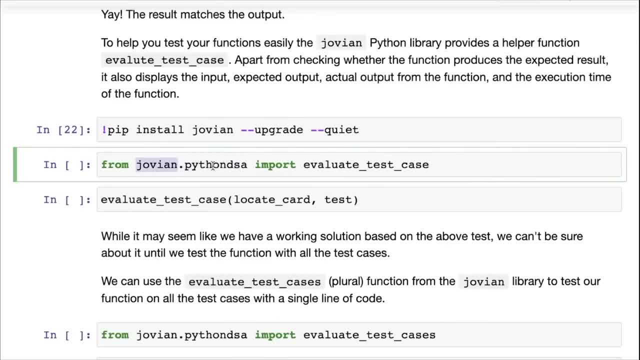 And then from Jovian dot Python DSA. So Jovian is the name of the library And then inside the Jovian library, since we have many courses, the Python DSA course. the utilities for this course are present inside the Python DSA module. 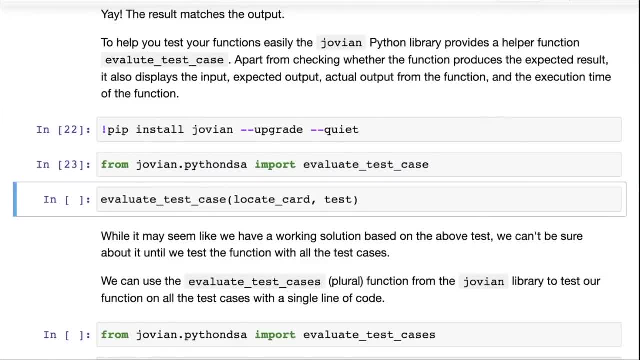 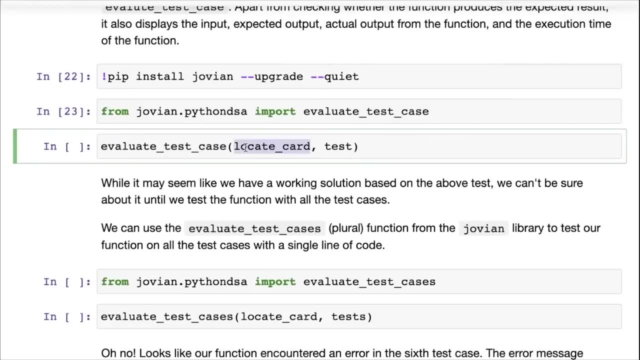 From that module we import the function evaluate test case And finally we can call evaluate test case. Okay, So we can give it the function that we want to test. So we're going to test the locate card function and the test case. the test case needs to. 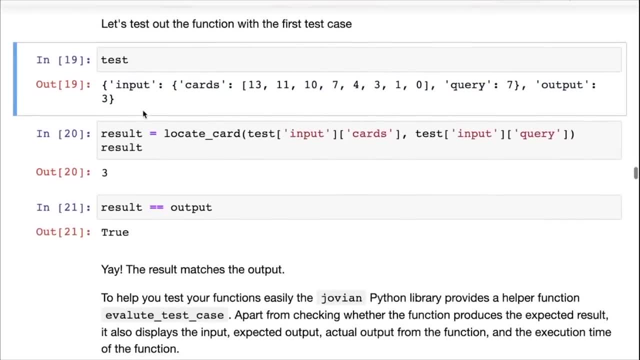 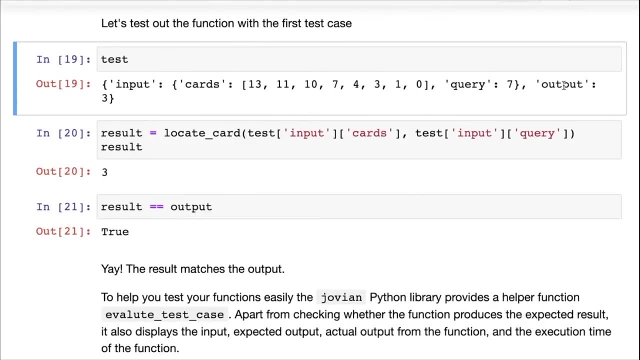 be defined in this format. So all it is going to do is it is going to pick out the input, pass it into the function, get the output, compare that output with the expected output and also print some information for you to see. 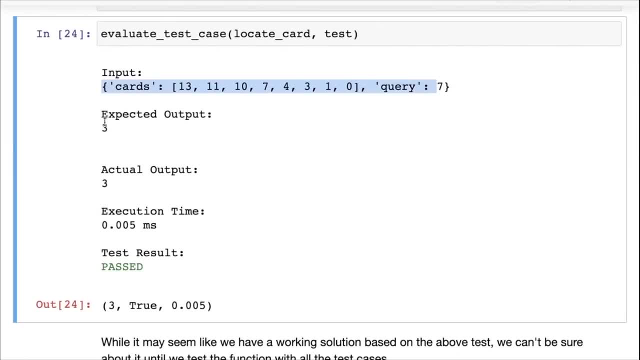 So here's what it does: It prints out the input, It prints out the expected output, It prints out the actual output, It prints the execution time- And this is something that will become important later- and tells you whether the test has passed or not. 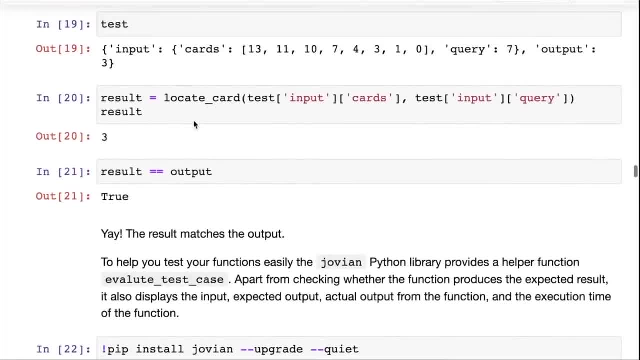 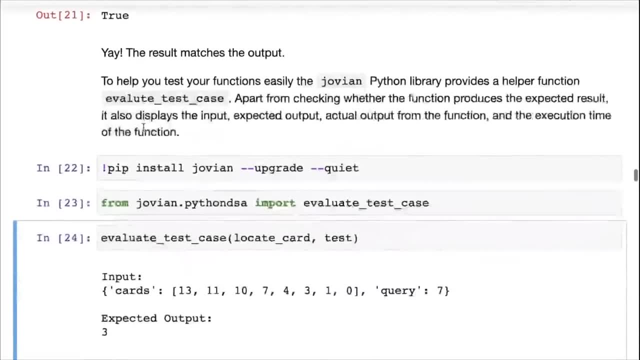 So it's nice to have this, you know, because so we don't have to look through the output and input and compare them. especially when you are in a situation where you need to think fast, it's helpful to create a small function that can just print pass or fail for a test. 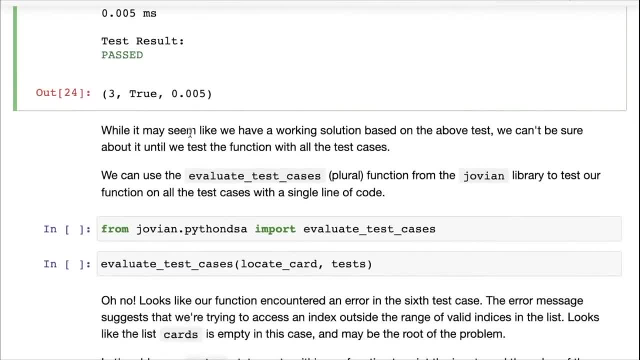 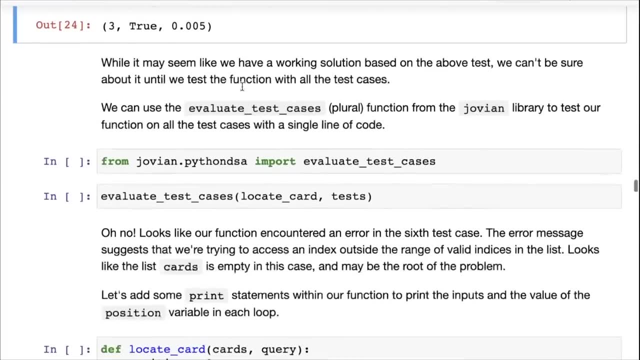 case. So now, while it may seem like we have a working solution because our test cases passed, we can't be sure about it until we test the function with all the test cases. So for doing that we can use the evaluate test cases function. 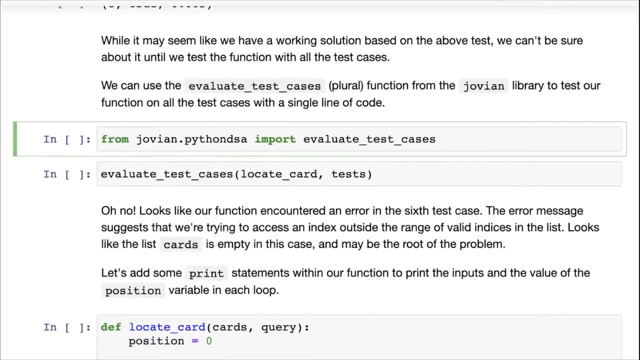 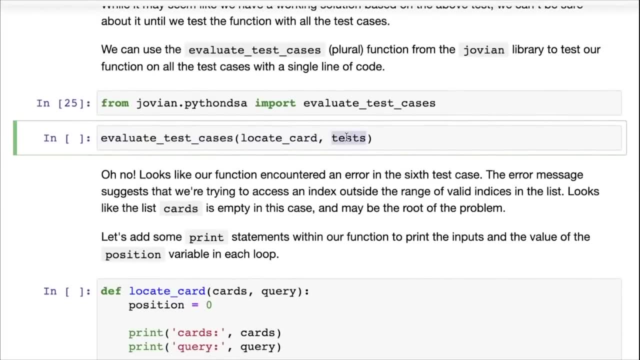 So just as you have a value test case, you have evaluate test cases also part of the Jovian library and you can call evaluate test cases with the same function, locate card And this time pass it a list of test cases. Each of the test cases is a dictionary. 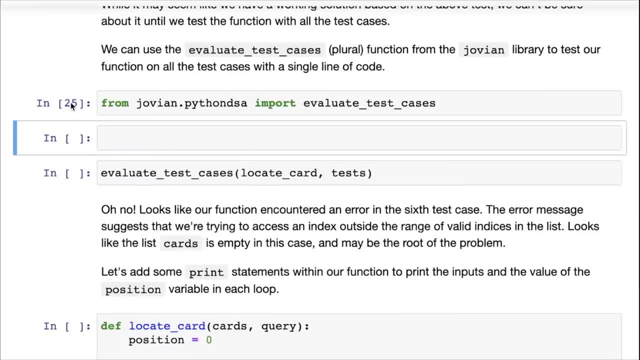 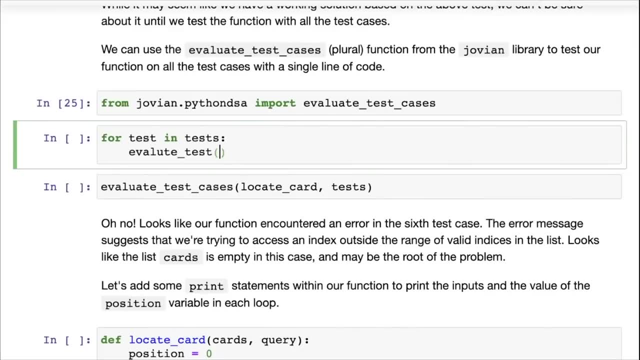 Again, you don't have to use this function. You can simply put things into a loop So you can always just do for test int And then simply call evaluate test with locate card and test, or you can even just directly call locate card with the test inputs. 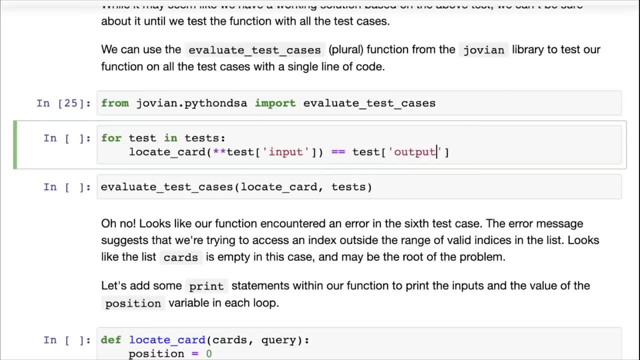 and the test out and compare the output with the test output, right, So you can do this as well and you can simply print that. So here's a simple way to do this, What we are doing here, but what we'll do is we'll use the evaluate test cases function. 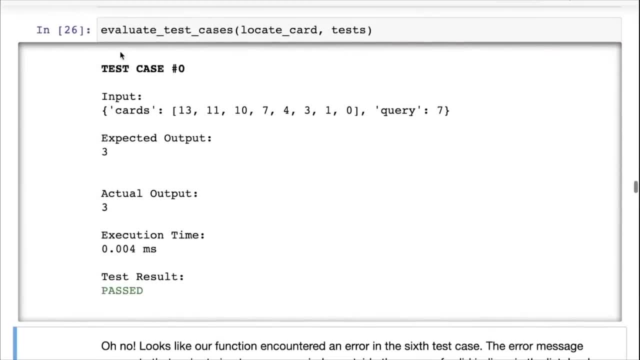 because it prints out a lot of useful information for us. So now you can see that it prints out case case by case. Now, test case zero. we have input, expected output, actual output. The case had test cases passed. That's what we saw it. 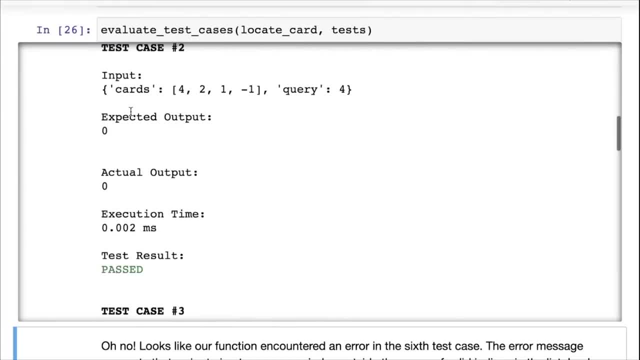 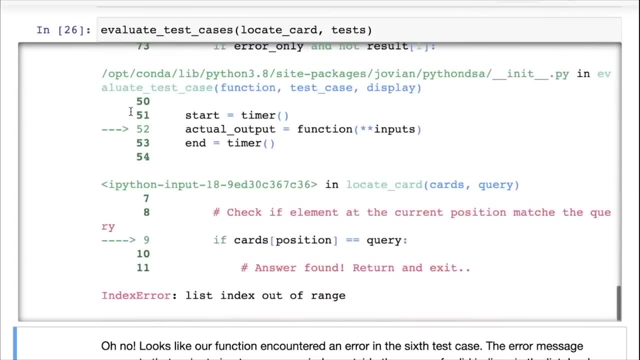 In fact, it's the same test We just did. test case one passes as well. Test case two passes. test case three, four, five, six, Okay, All of them are fine. Okay, So now we can see that we have a different error. 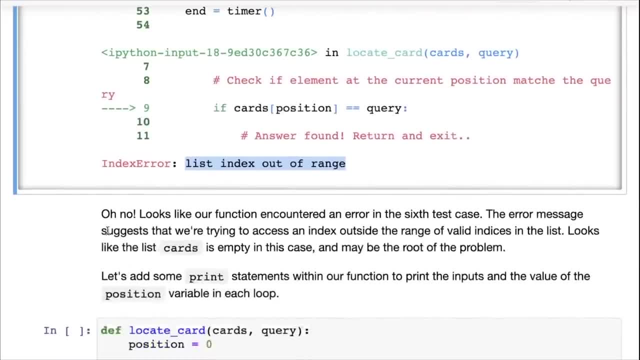 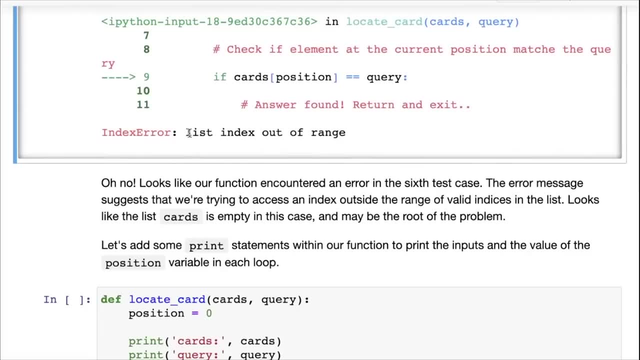 So here's the error. It says list index out of range. So that's okay. It's perfectly all right for your functions to encounter an error. So the first thing, the most important thing, is not to panic. In fact, it's a good thing that we know exactly where the function is failing. 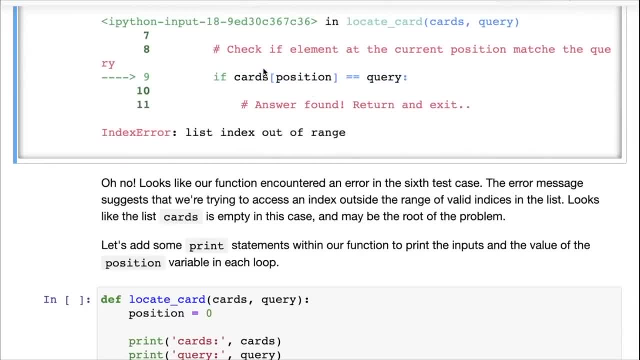 If you look back here you can see what the issue is and then we'll see how to fix the error. But one, one good strategy to approach this is to keep in mind that there will always be bugs in your code, And approach writing code not with the assumption that your code will be correct, but go with. 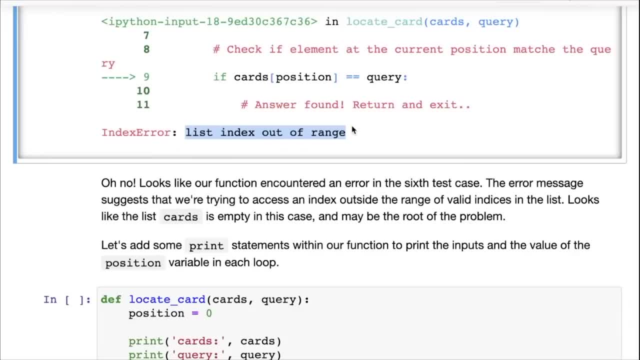 the default assumption that your code will be wrong, that there will be issues. What that lets you do is: one, you do not feel demotivated or you do not panic when you see an error, And second, you then tend to be a little more careful while actually writing the code. 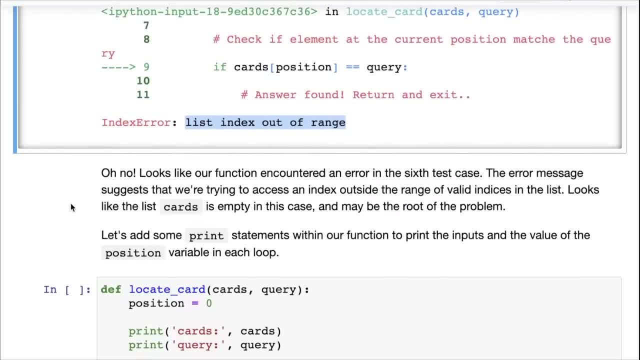 So the way you should be writing code is: every time you write a line of code, you should be asking yourself: how can this line of code go wrong? Or, in this case, how can this line of code go wrong In this particular case, how can cards position equals, equals query in a if statement go wrong? 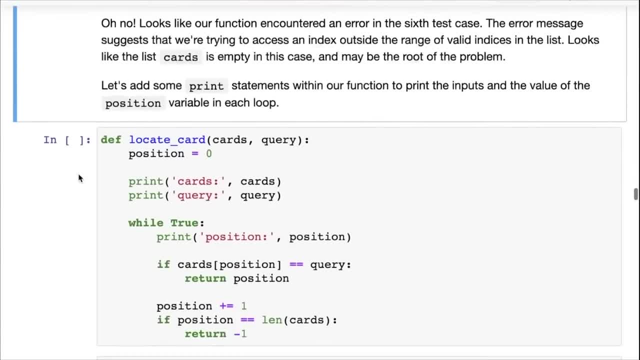 and throw an error And let's look at it. One easy way to check this is to add what is called a logging or what is called printing the information inside a function. So we'll just rewrite a function in in a locate card function. 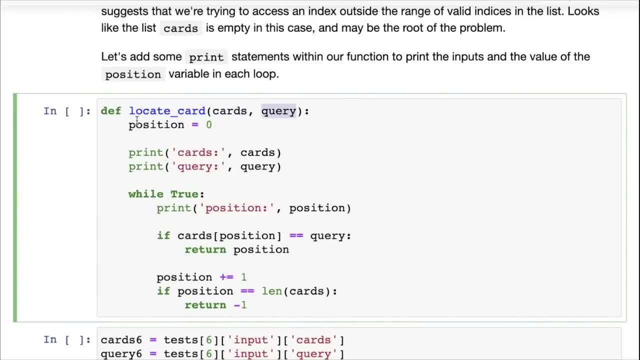 We will put in cards and we will put in query the exact same function that we have. We'll set the position, but before we create the value, we'll simply print the cards in the query. So just for our information, just so that we can see what the function is working through. 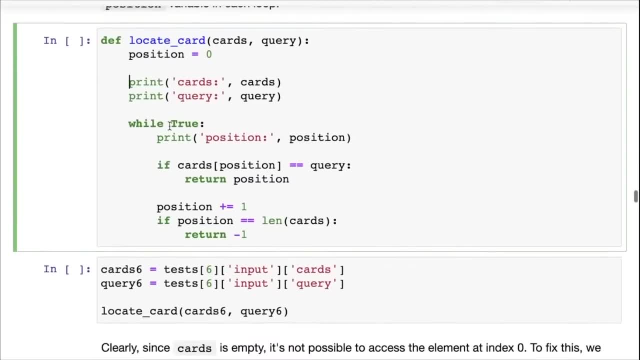 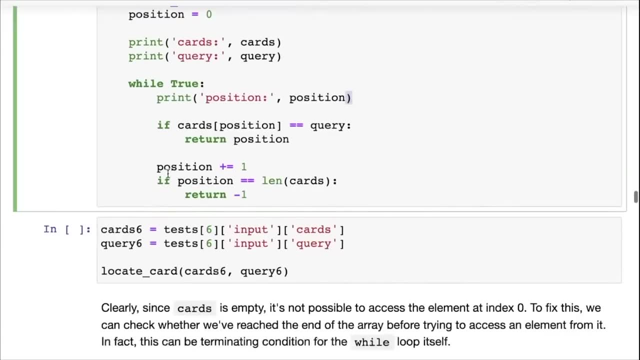 we can get some visibility into the function. We print out cards and query and then, while true, So this is the same loop, at the beginning of the loop we will print out the position that we are tracking. Okay, So let's do that. 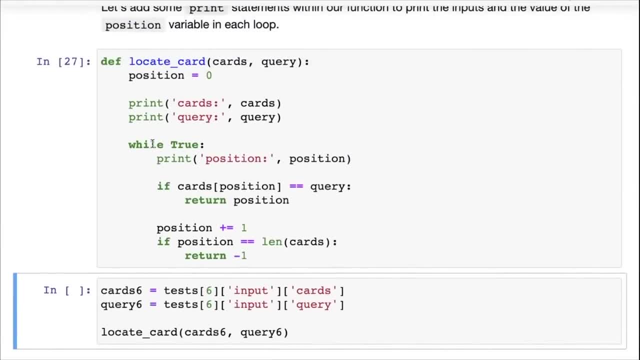 We've simply added some print statements, and this print statement will give us an insight into the inner working of the function. Now, if you do not put in a print statement, then you will have to work it out yourself by reading the code and executing it in your head. 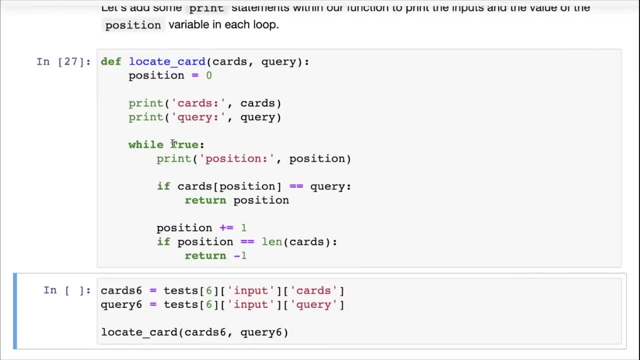 It's always easier to just print all the all the information and then print it nicely. Just say cards and query. You know, we could also have done this without saying cards here, but then that would make it a little harder to read. 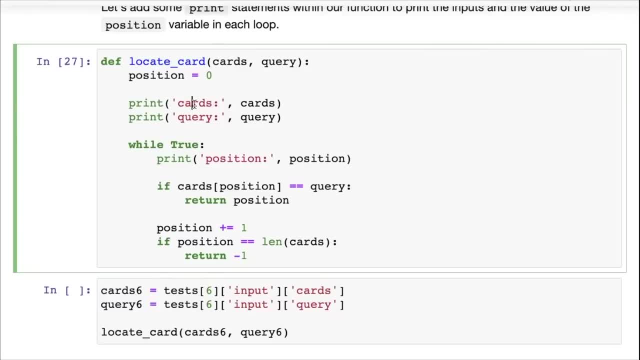 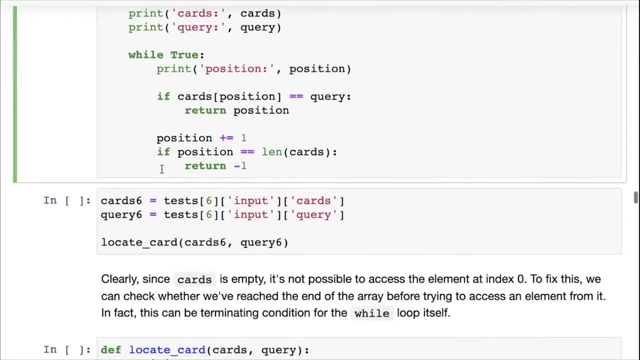 Then that would be more cognitive overload, apart from already dealing with the stress of solving an error, right? So just add nice pretty print statements to make it very obvious what we are printing. So let's see. now let us get the test case out. 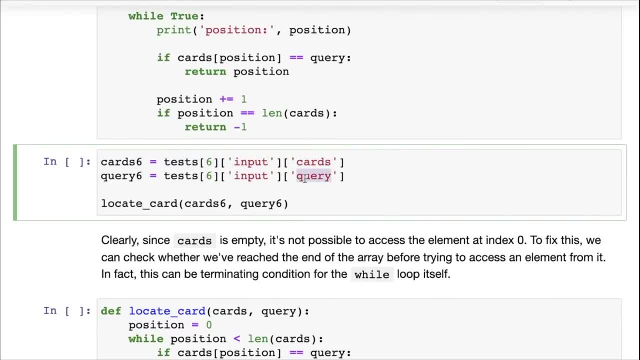 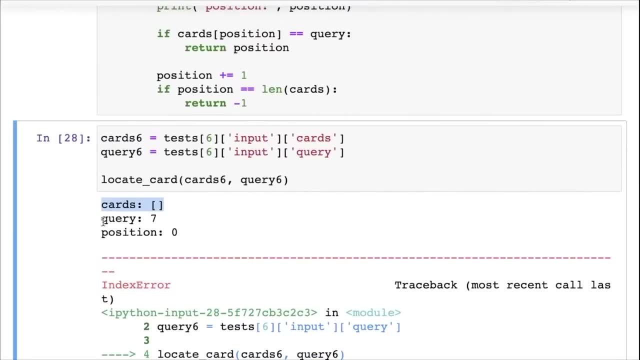 So let's get from test six. get the input, get the cards- Okay, Get the query as well and pass it into locate card. And now we see that initially the cards area is empty and the query seven and the position is zero. 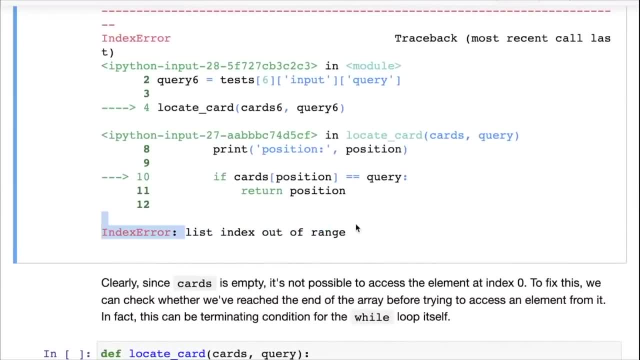 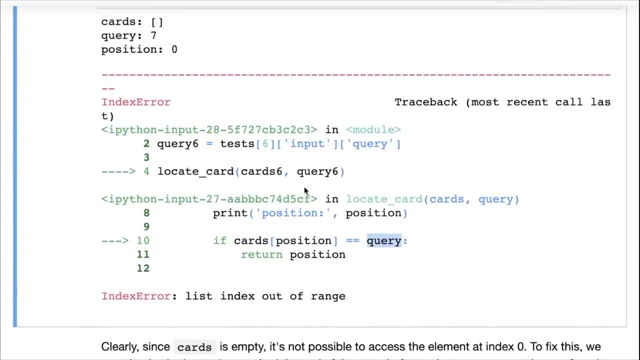 And then we encounter an error. We encounter the error list index out of range on the line cards: position equals, equals query. And now at this point it should be fairly obvious what the issue is. The issue, obviously, is that we have an empty list, and empty list has no elements. but we're 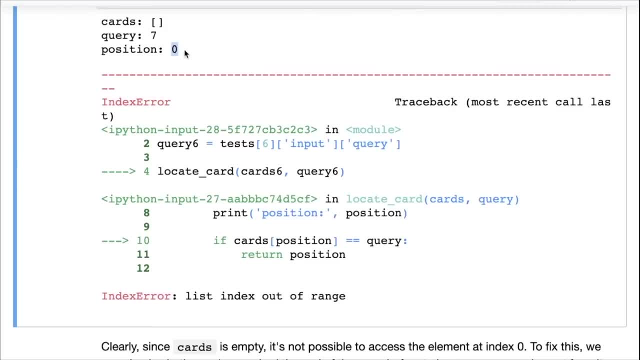 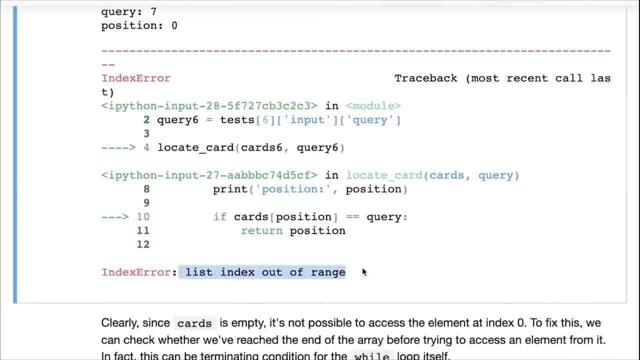 trying to access The position zero, which is, in normal human conversation, the first element of a list. but there is no first element to access And that is why we get the error list index out of range. So this is very important. 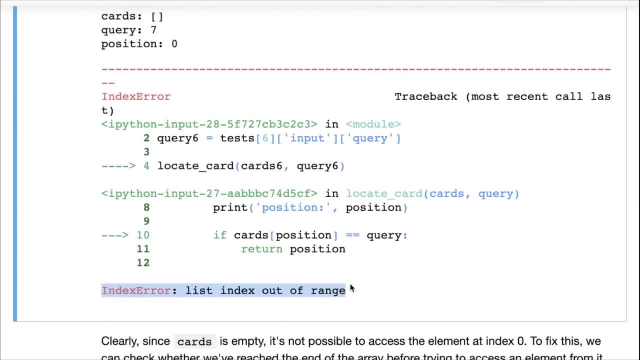 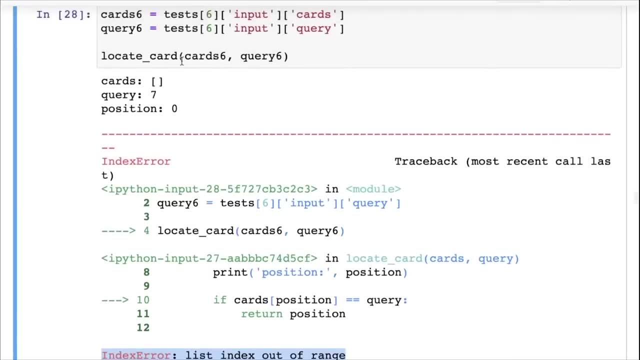 Whenever you get an error, do not try to start looking at the code first. just try to understand the error first And if you're unable to understand the error, just add some print statements. There are tools like debuggers that people use, but I personally, in 15 years, haven't. 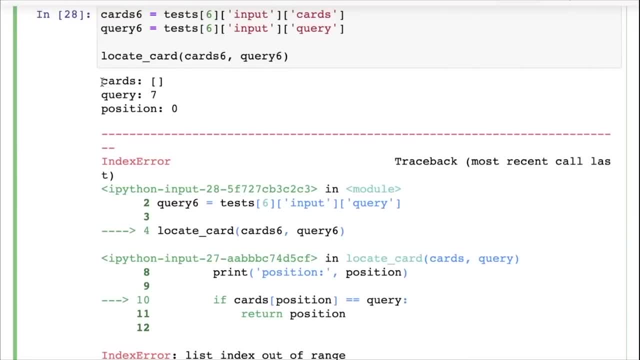 used a debugger. I maybe use it. I've used it a couple of times, but I don't know how to use it. Print statements are really simple. You just put them in, chuck them into the function wherever you need them, as many. 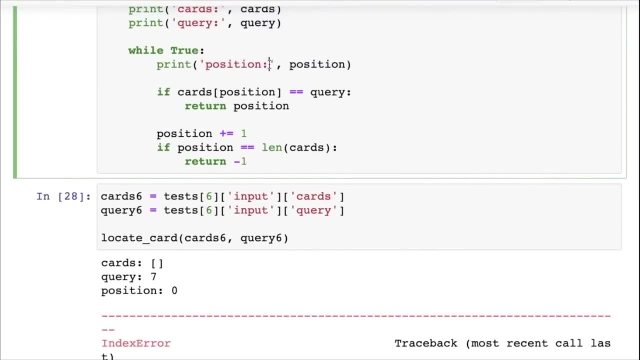 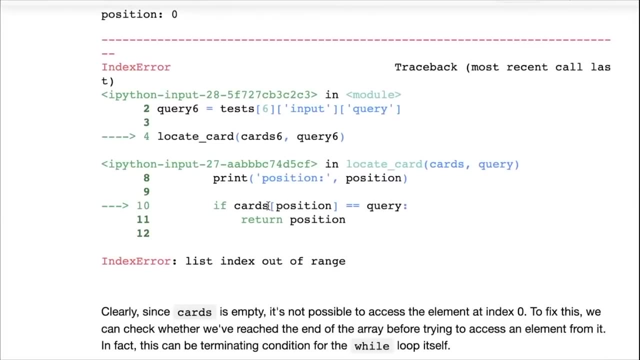 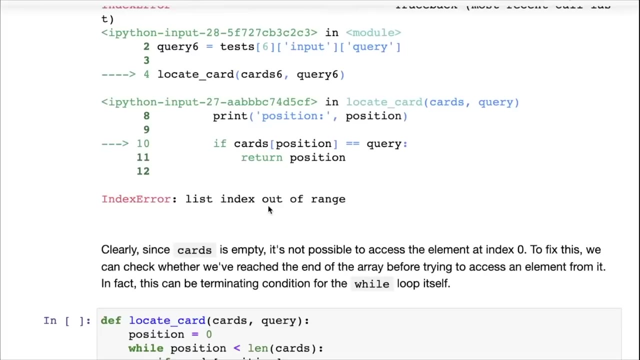 print statements as you need, with nice, clear messages. make it very obvious And that will almost certainly solve the issue for you. So the cards area is empty. We cannot access position zero. So what's the solution here? The solution, obviously, is that before we access anything from a list, we need to make sure. 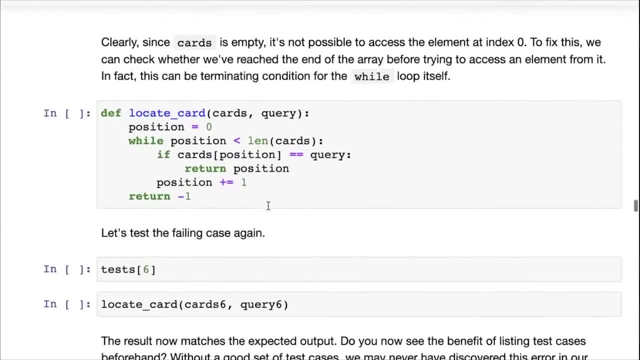 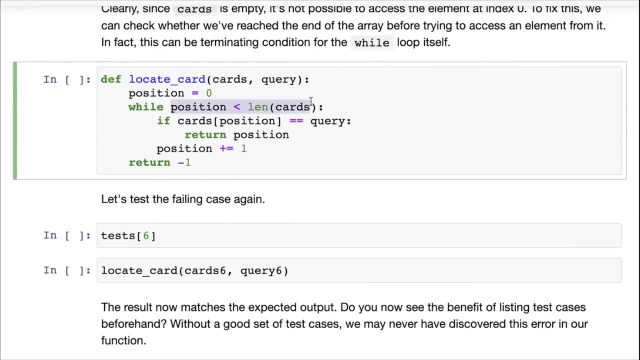 that we can access that list, And this is the way to do it. So now we've rewritten our function slightly. We once again start out with position zero, but this time, instead of putting in a while, true, instead of assuming that we can access the zeroth element of the list, we say that: 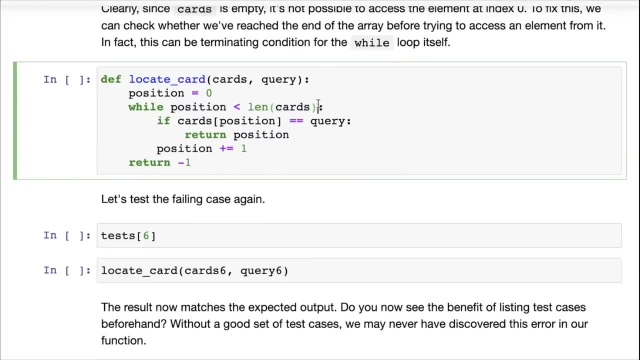 the position should be less than the length of cards. Now if, if you have a cards list of N elements, the indices go from zero to N minus one, or in the case of zero elements, there are no indices to access. So the position? 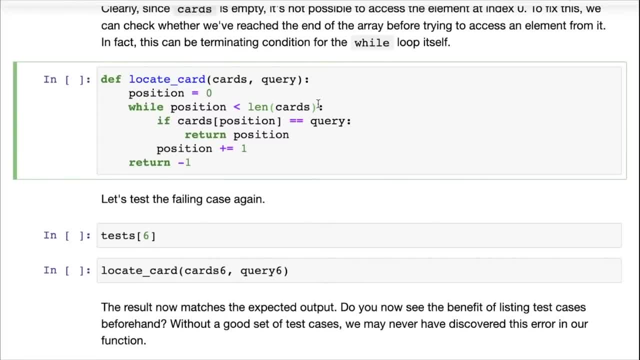 Okay, Less than the length of cards for you to be able to access it, And in this case the length of the cards will be zero. So zero is not less than zero. So the while loop will not run at all and we will directly return minus one. 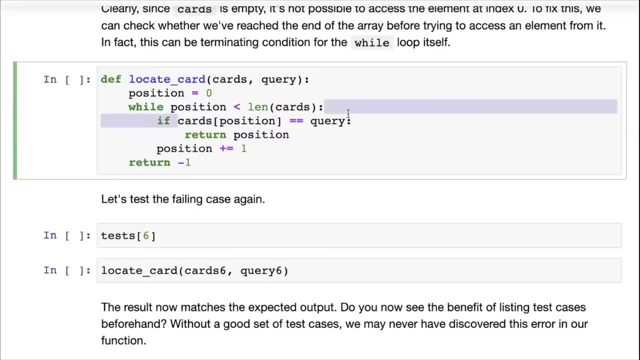 But if the card does have elements, then we can check the element at the value position compared to the query and return the position If it does not. if it does not match the query, we can increment the position. So that was a fairly straightforward fix. 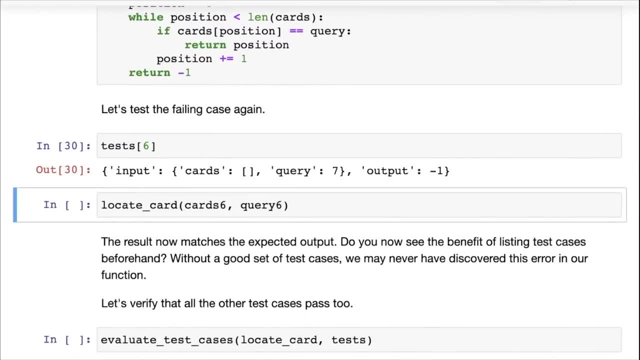 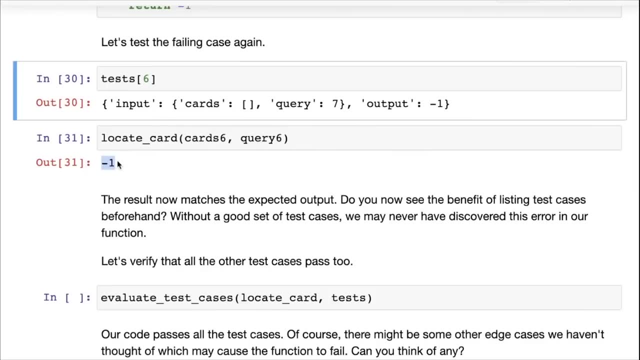 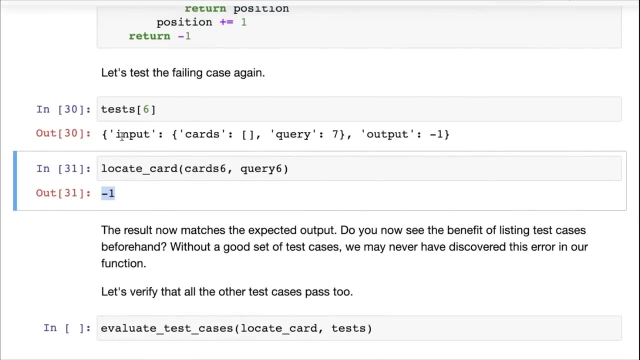 Easy save. So let's test the failing case again. Great, So it looks like the failing case is now passing, because we have output minus one and the expected output matches the actual output of the function minus one. because the query does not exist in the array, which is empty. 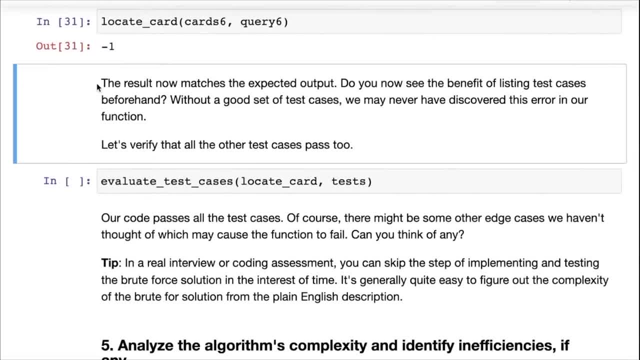 Of course, Now this is not enough. Every time you make a change to the code, you want to go back and test all the test cases, because what ha? what may happen is, while fixing one error, you may introduce another error, And that is where having a good set of test cases is very important. 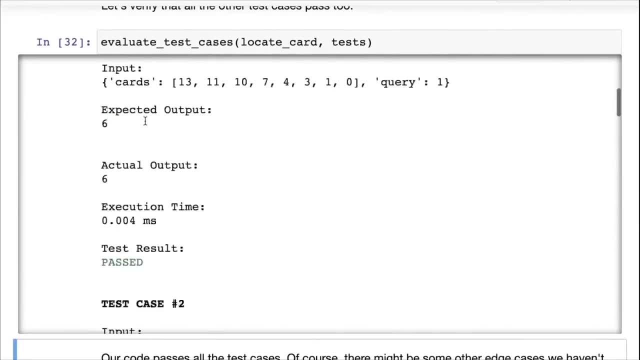 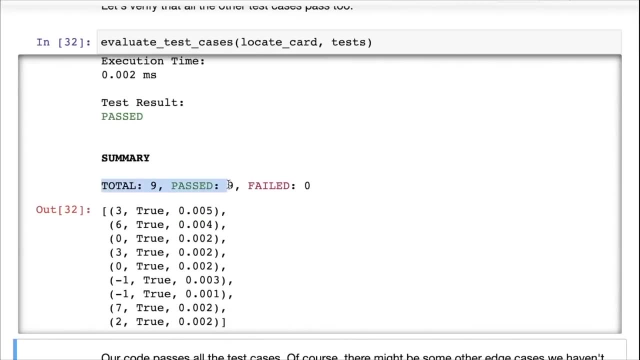 So let's run evaluate test cases Once again. you can see here this time that all the test cases are passing and it's just nice to. it just makes you feel good as well, Makes you feel motivated as well to see that a bunch of test cases are passing. 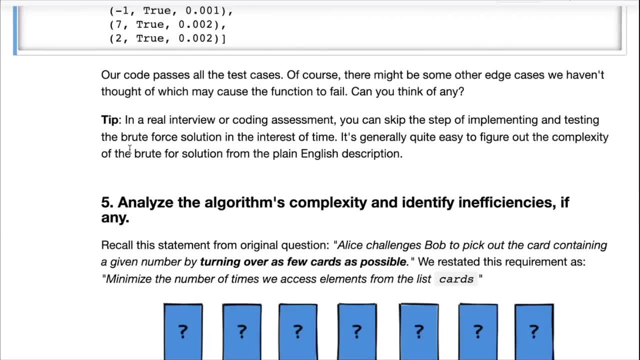 Now in a real coding assessment or a real interview, you can probably skip the step of implementing and testing the brute force solution in the interest of time, Because it may take about five to 10 minutes to implement the solution And then, if you have errors in the solution, it may take some more time to fix those errors. 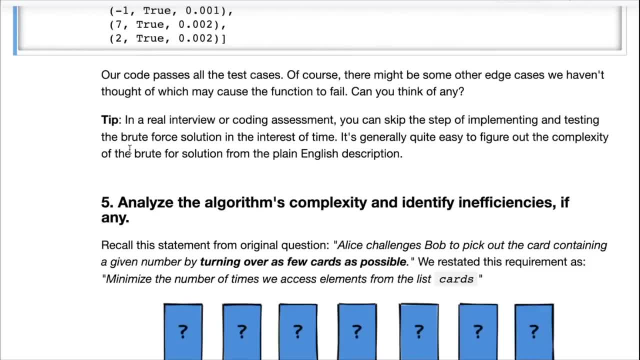 So it's generally quite easy to figure out the complexity- which we'll talk about in second, of the brute force solution from the plain English description, And that is why you should first state it in plain English, which only takes around 20 seconds or so. 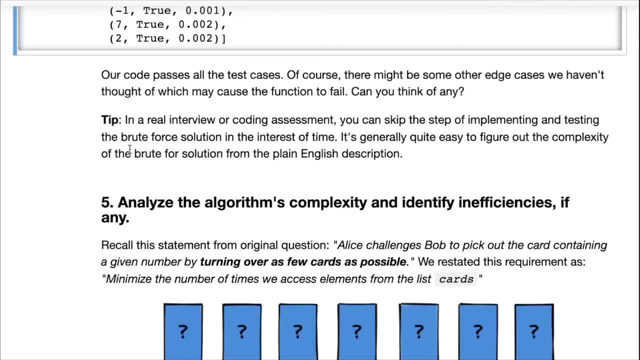 And the computer doesn't throw errors at you for speaking, So you can just state the plain English description. You can do that And move on, talk about the complexity and start optimizing it, But while you're practicing, always, always, implement the brute force solution too. 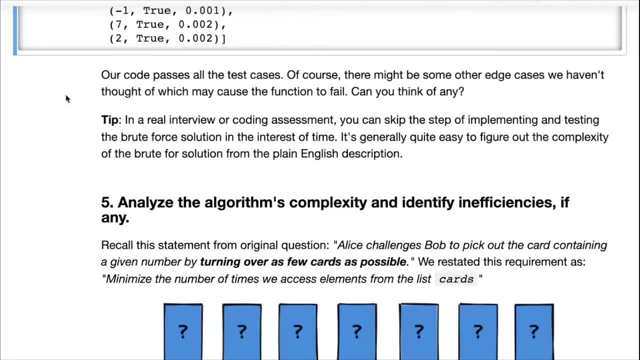 And there's an important reason why you should know how to implement the brute force solution, Because, in case you're not able to figure out the optimal solution to the problem, you can still go back and implement the brute force solution And in a lot of cases that's okay. 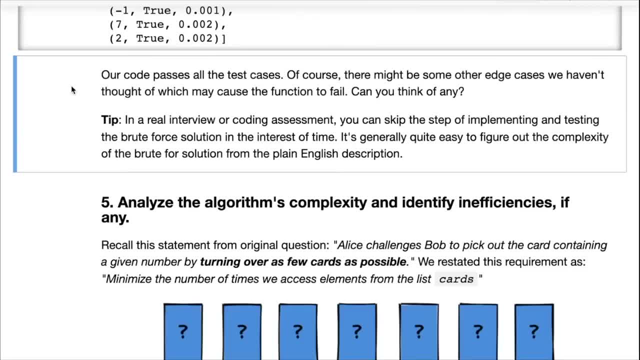 Sometimes interviewers ask hard questions just to push your boundaries a little bit, But if you're unable to figure out the optimal solution, Then they will allow you to implement a brute force solution. So that is why you should state it And that is where you should know how to implement it. 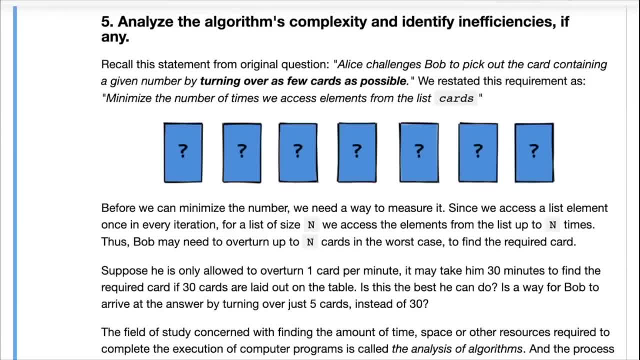 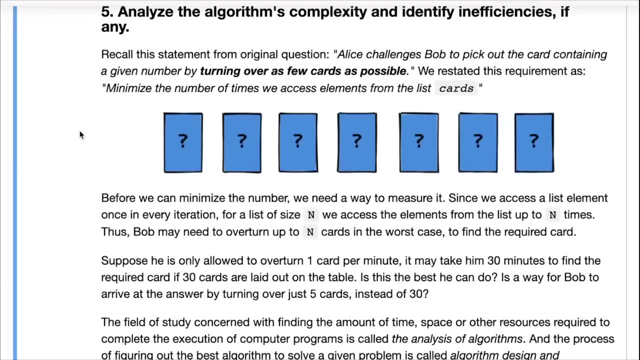 Okay, So we're done with. so we're done now with the implementation of our brute force or simplest solution, And now we need to analyze it, And this is where we'll now learn about what is called the complexity of an algorithm. What does it mean? 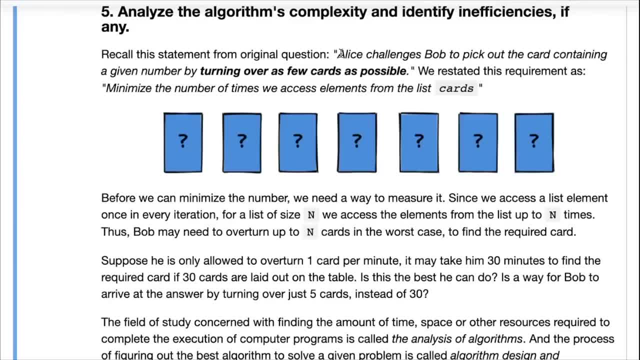 Now. So to answer your question, Alice challenges Bob to pick out the card containing the given number by turning over as few cards as possible. But right now what we're doing is we can say we're simply turning over cards one by one. 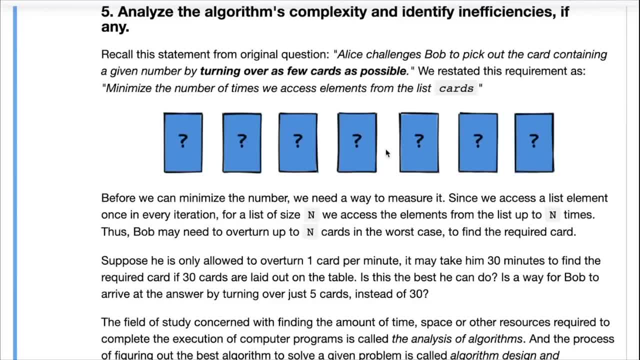 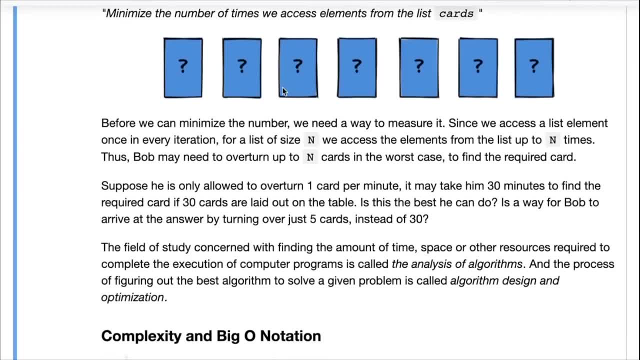 And before we talk about what does it mean to minimize the number of times we turn over cards or the number of times we access elements? we need a way to measure it. And let's think about it. You know it's, it's as simple as just thinking about it, since we access the list element. 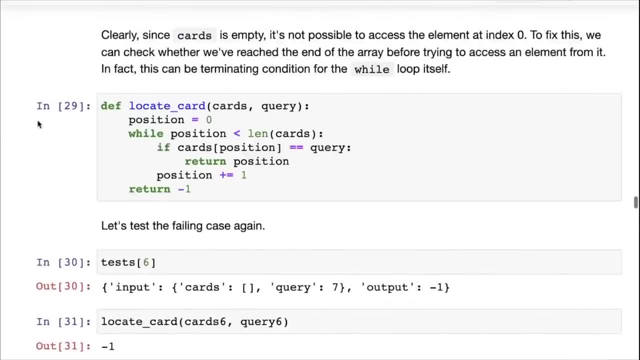 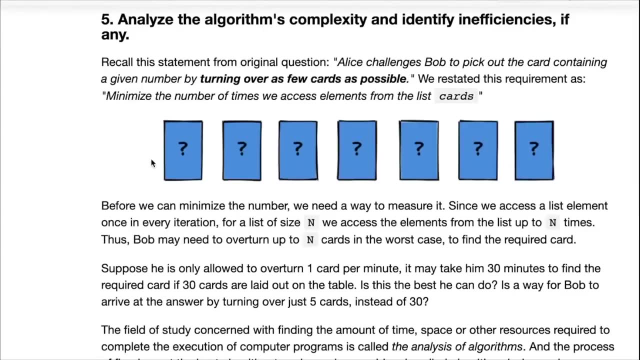 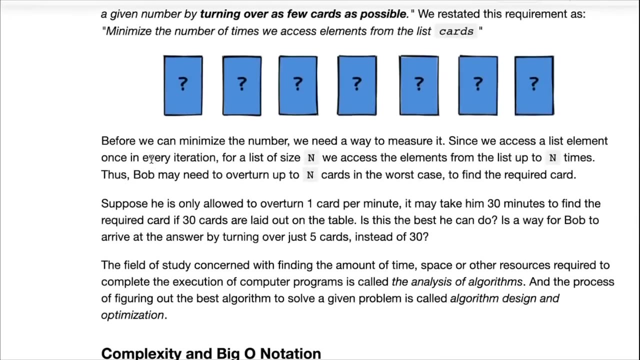 once in every iteration. So here's the code. Our code is pretty straightforward And this is where we are accessing an element from the list. So, since we access the element, since we access the element once in every iteration for a list of size, and we access the elements from the list up to end times because we may have 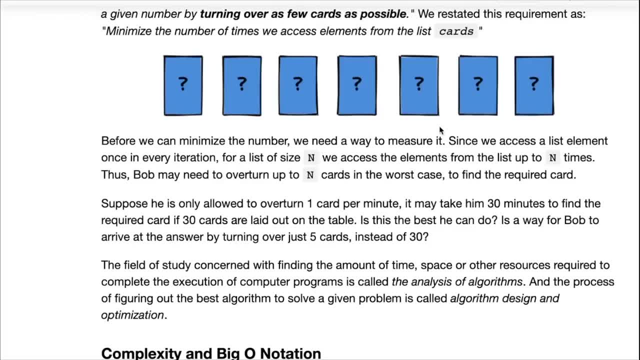 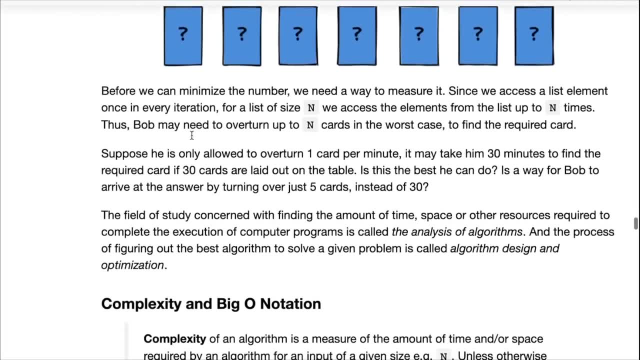 to access this element, and then this element, and this element, and so on. So Bob may need to overturn up to N cards in the worst case to find the required card. Okay, Now let's introduce an additional condition that suppose Bob is only allowed to overturn. 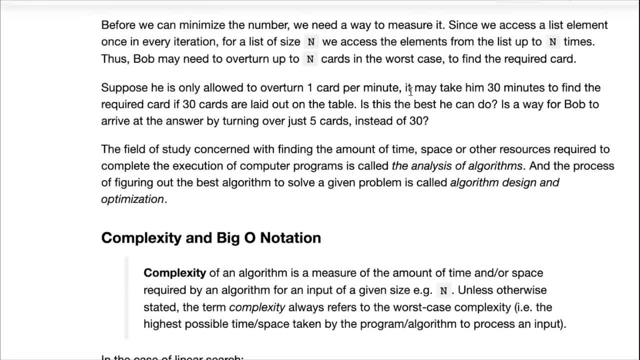 one card per minute. So that means it may take him 30 minutes to find the required card, in the worst case, If 30 cards are laid out on the table Now. is this really the best he can do, Or is there a way for Bob to arrive at the answer by turning over just five cards and 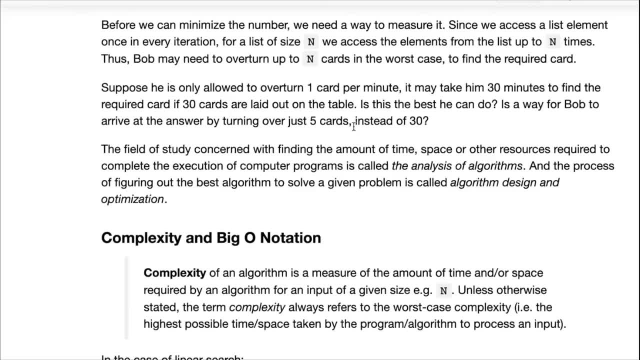 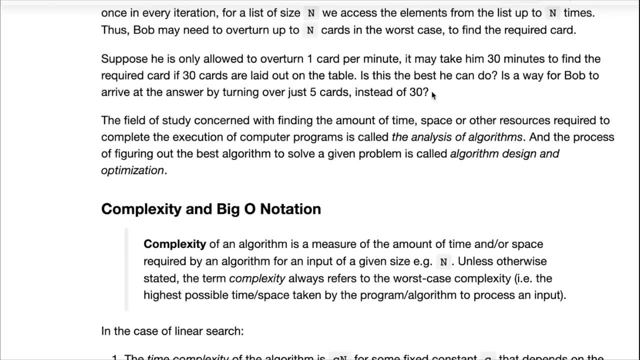 save 25 minutes instead of turning over all 30, and this field of study- and, by the way, Bob in this case is representative- A computer does and a computer takes some amount of finite time to perform each instruction, So each array access actually takes some time, although it's so fast that we do not see it. 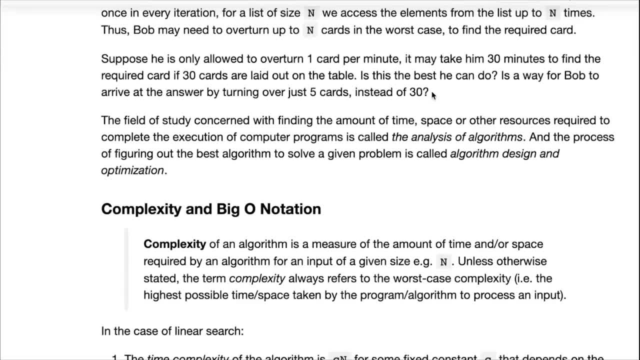 especially for small inputs. but this is something that will become increasingly important as we go week over week, where we will see that we will start to see the limits of how long it takes computers to solve certain problems. So the field of study concerned with finding the amount of time or the amount of space, 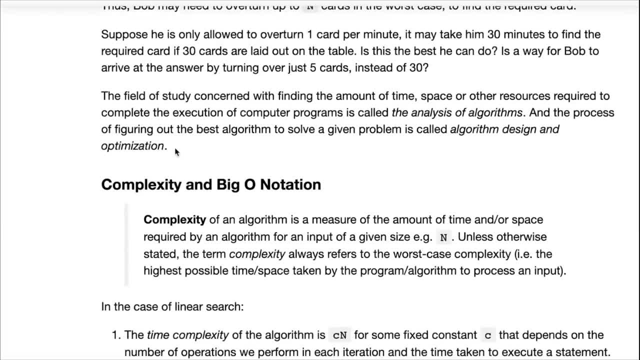 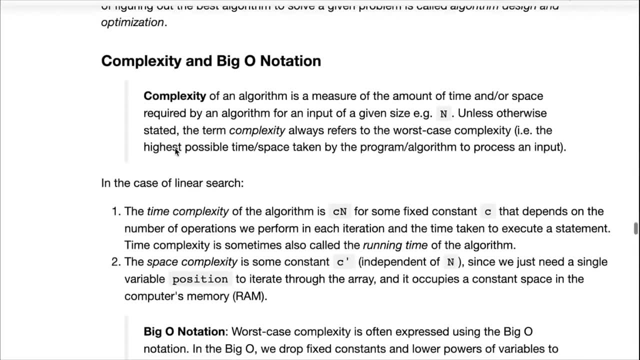 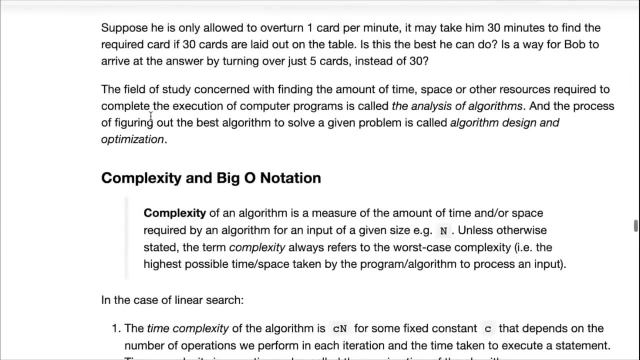 or the amount of other resources required To complete the execution of a program, is called the analysis of algorithms, And the process of figuring out the best algorithm to solve a problem is called algorithm design. And that is what we are doing here. We are actually doing the analysis of algorithms right now and algorithm design next. 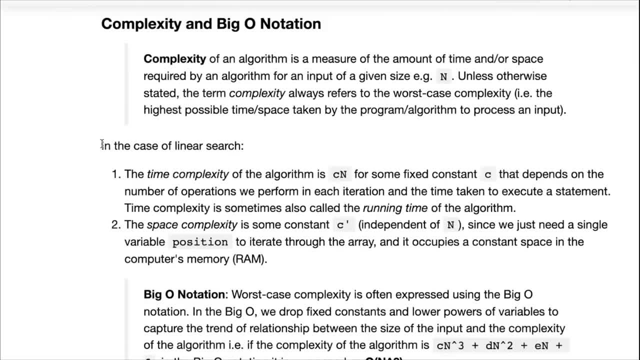 So there are a couple of terms we need to understand, and then we'll go back to writing code. Uh, first thing is complexity And the second thing is the bigger notation, And both of these are terms that you will hear very frequently. 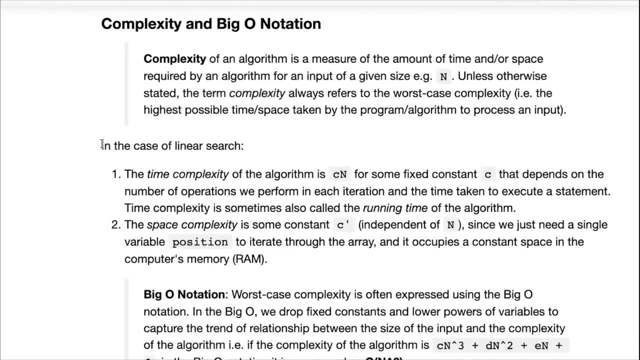 In When you're talking about data structures and algorithms, when you're talking about coding, interviews, assessments. So these are terms that you need to understand and they're fairly simple terms, although the term itself is complexity, but all it means is that the complexity of an algorithm. 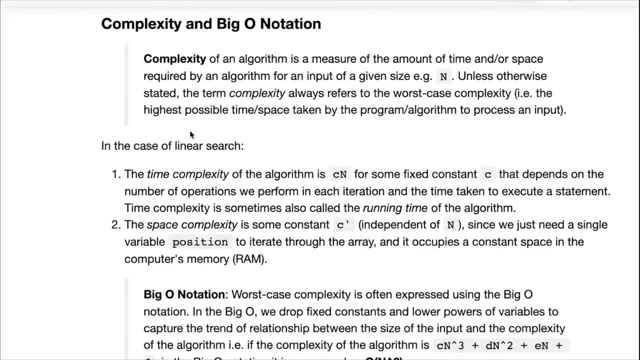 is simply a measure, some some measure of the amount of time or space required by an algorithm to process an input of a given size. example, If you have a list of size N And then the complexity is the amount of time required or the amount of space required. on. 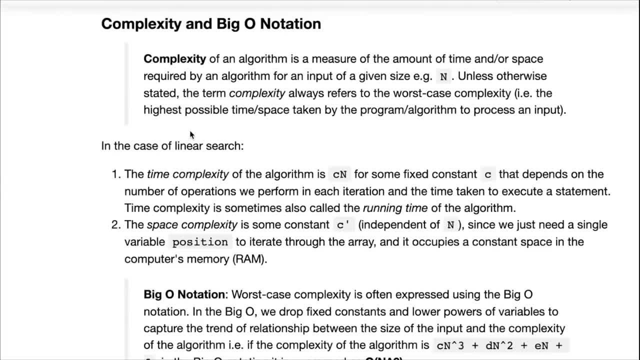 the Ram to process an input of that size. Now, unless otherwise stated, the term complexity always refers to worst case complexity. So it's possible that the Bob turns over the first card and that is the answer. But we always talk about what is the longest or the highest possible time or space. that 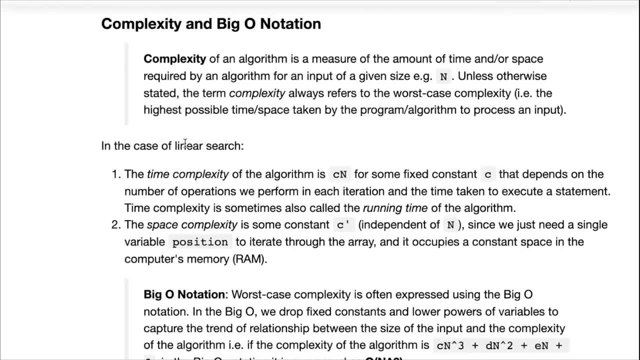 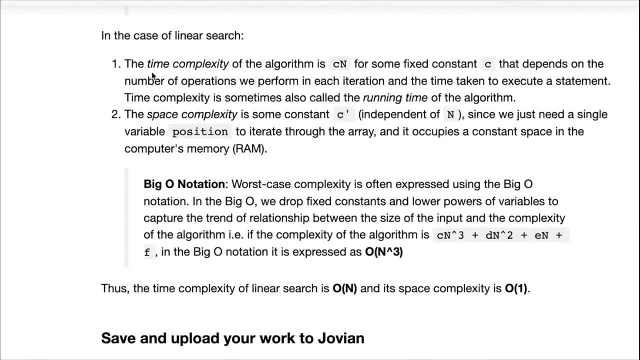 may be taken by the program to process an input right. So we need to design our programs keeping the worst case in mind. Okay, Now, in case of a linear search, which is what we've implemented just now, the time complexity of the algorithm is some constant C times N, assuming N is the size of the list. 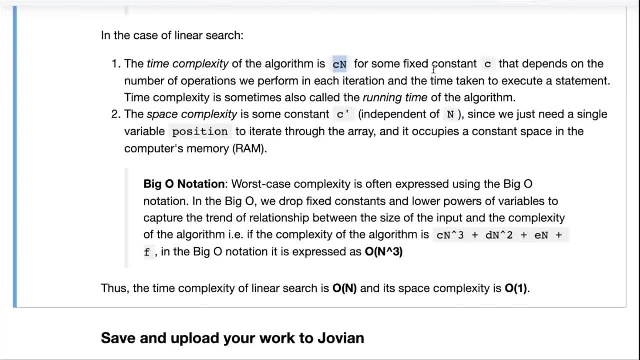 N is the number of cards, right? So now this constant C obviously depends on the number of operations that we perform in each iteration. So in each loop, for example, we have four to five statements, and then the time taken to execute a statement on your specific hardware. 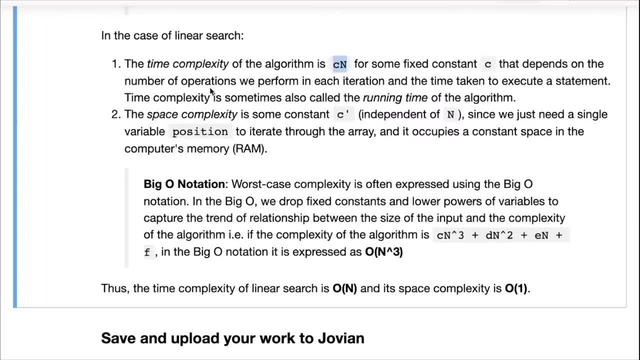 Now, if you have a two gigahertz computer, that may be twice as fast. There's a one gigahertz computer. If you're running it on a phone, it may be different. So the C captures all of these things. 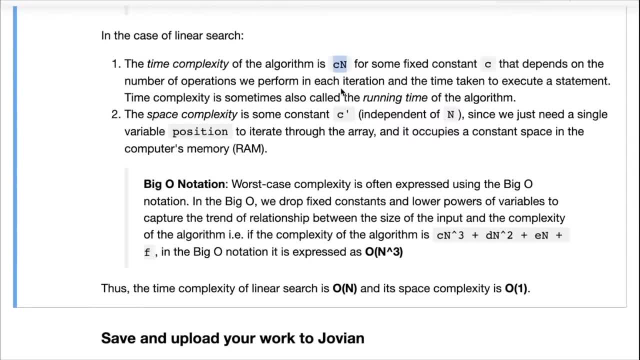 So information about the number of specific operations that we perform in each iteration and information about the actual hardware that you're running on. So C N is the time complexity and N is the size of the input. So in some sense, what we understand from this is that the time complexity is proportional. 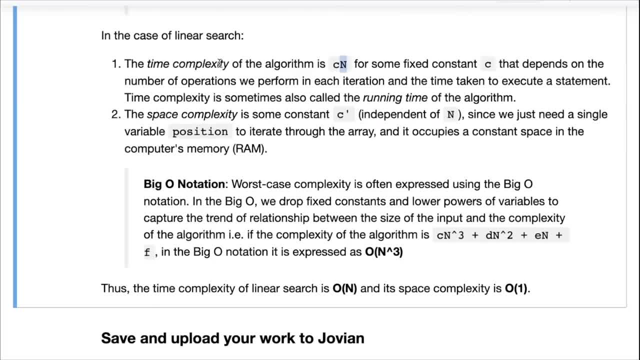 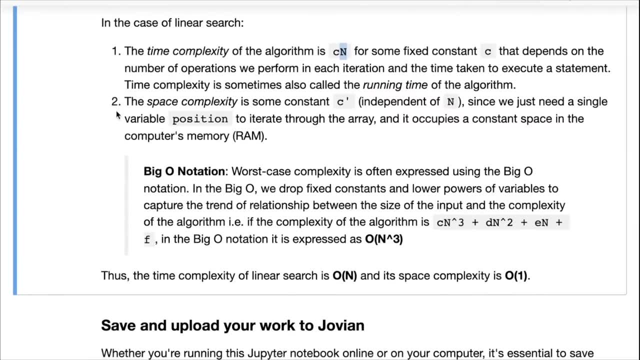 to the size of the input And that's the important part here. The constant, you know it doesn't change as you change the input. The constant doesn't really change Now. similarly, the space complexity. now, since we are already given an area, the additional. 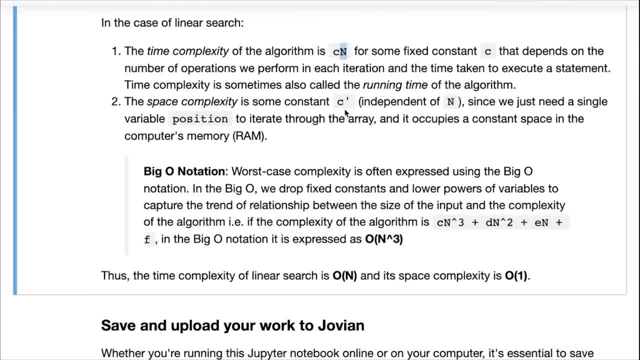 space that our linear search requires is simply a single constant when we are calling it C prime or C dash, and it is independent of N. So no matter how many, no matter how large a list is given to you, and the list is already. 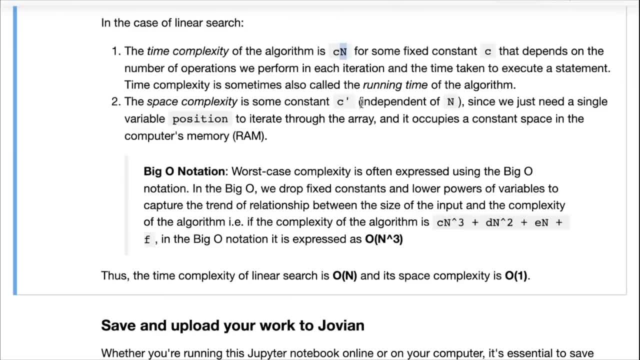 present in memory. we just need to allocate one new variable called position, And that variable is used to iterate through the area and it occupies a constant space in the computer Memory because we keep go on updating the variable right. So the space complexity is C or constant. 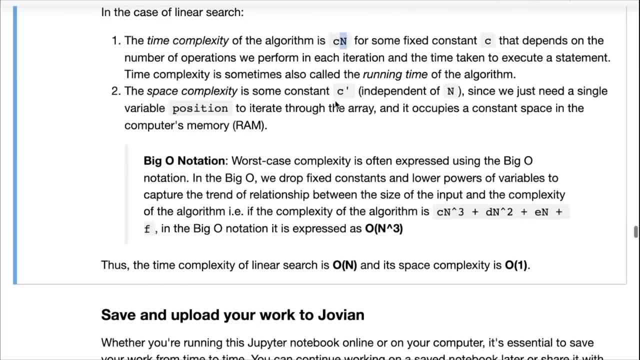 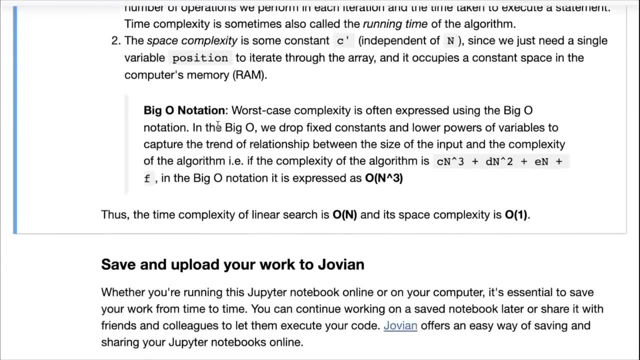 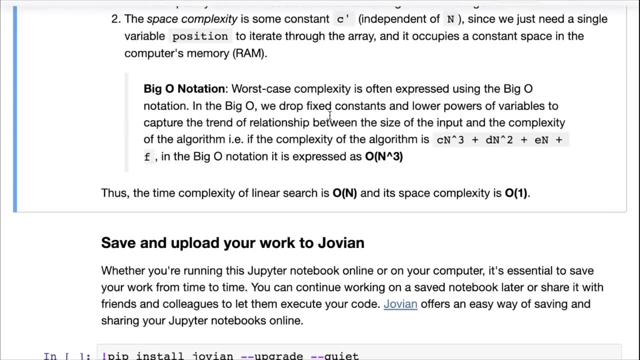 It is independent of N. Now, what we do normally is to represent the worst case complexity. We often use the big O notation and in the bigger notation what we do is we drop any fixed constants and we lower the powers of the. and we drop any fixed constants and we 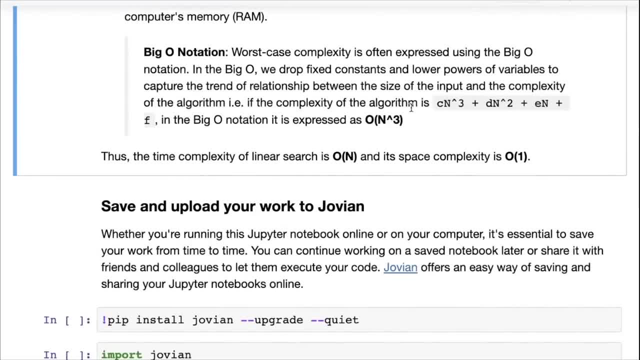 drop any lower powers of variables. So the idea, The idea here, is to capture just the trend, just the trend of the relationship between the size of the input and the complexity of the algorithm. For example, if the time complexity of an algorithm is some, some constant times, N cube. 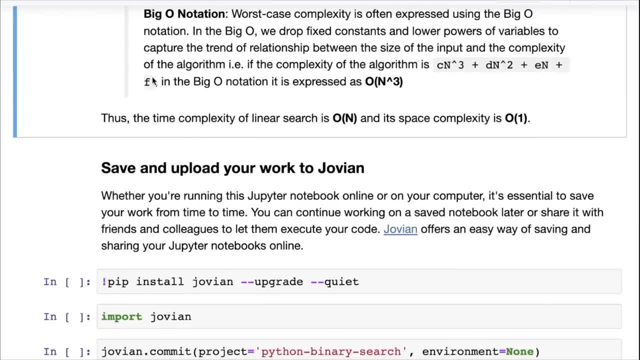 plus some constant times N square plus some constant time N plus some constant, where N is the size of the input. in the bigger notation we simply say that it is order of N cube, which is that in the long run in the, if you just study the trend, it the trend will be. 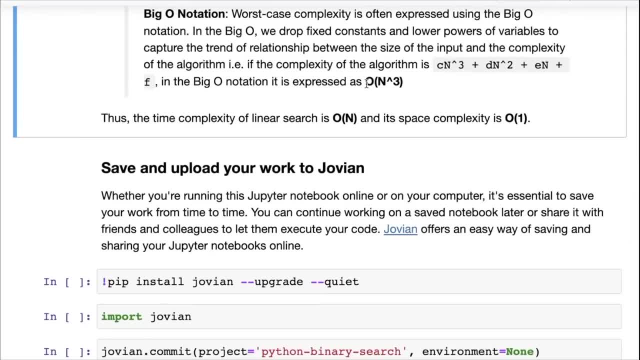 some Something which looks a little bit like the N cube function, and it may be offset by a constant or such. So, putting it this way, the time complexity of linear search is ordering because we just dropped the constant C and the space complexity is order one. 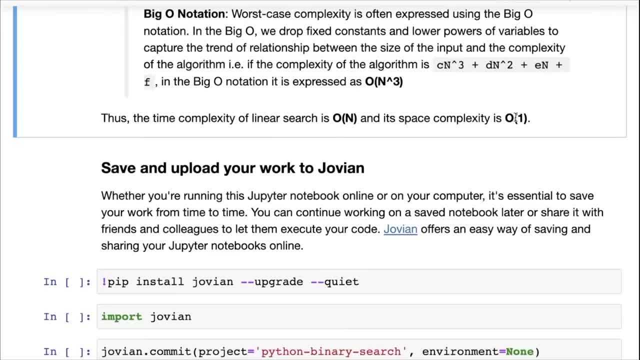 So we again drop the constant C prime and we'll see why it's okay to drop the constant. Sometimes you may find that, okay, we're not exactly doing any iterations, but we're doing N minus one iteration, So we dropped the minus one. 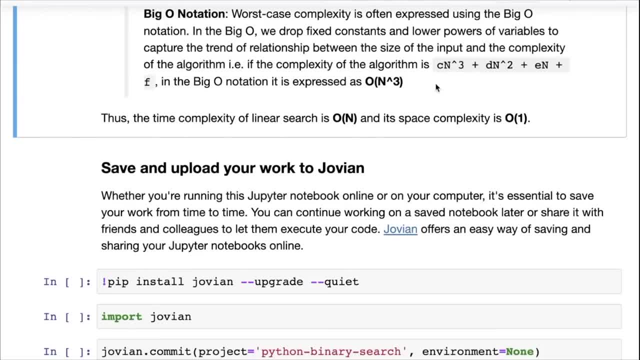 Sometimes you will find that we are just doing N by two iterations and that's simply half of N. So we dropped the half and you might wonder that okay, that that might take twice or three times the amount of time. how, why are we dropping that constant? 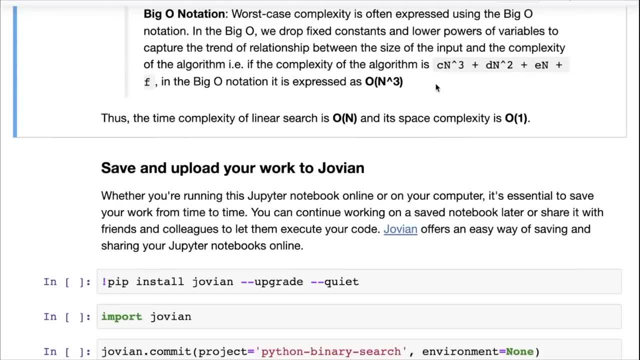 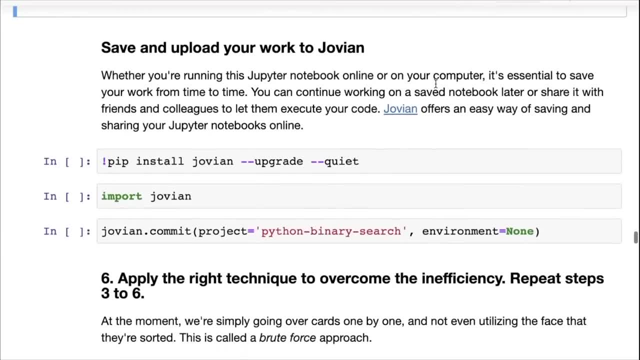 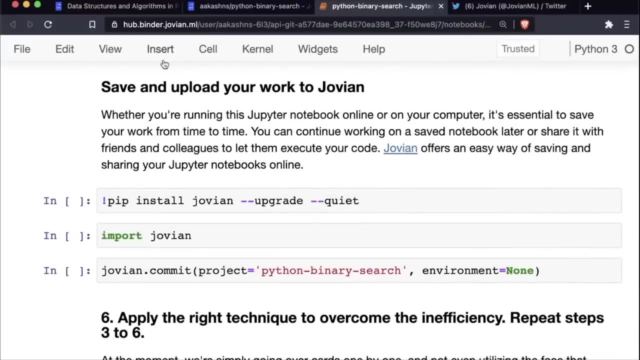 Because that's probably an important thing to keep in mind. but we'll see. we'll see soon as we implement our efficient solution to the problem. So, before we move forward, before we optimize the algorithm, we are just going to save our work, because this notebook, as I mentioned to you, is 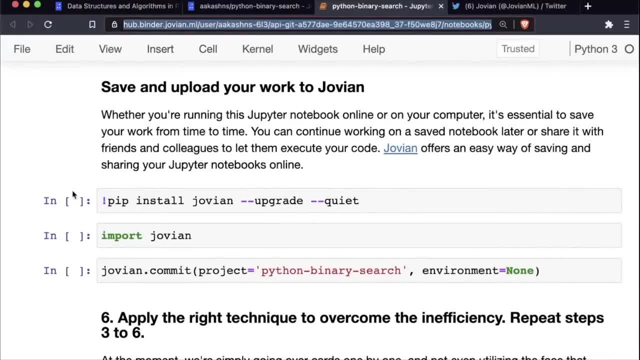 Running on an online platform. we've set up everything for you. You've not had to install anything, but because thousands of people are using this, using this platform, this will shut down. This will not keep running forever, And what you need to do is you need to save your work from time to time. 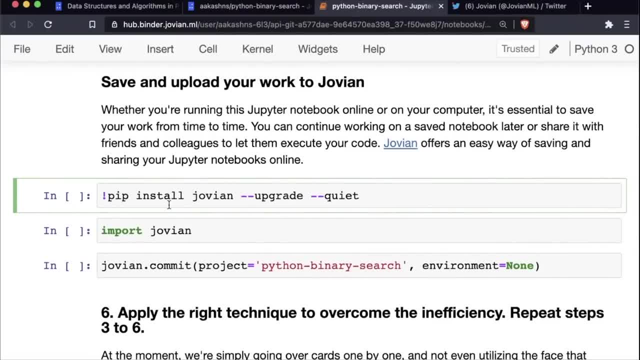 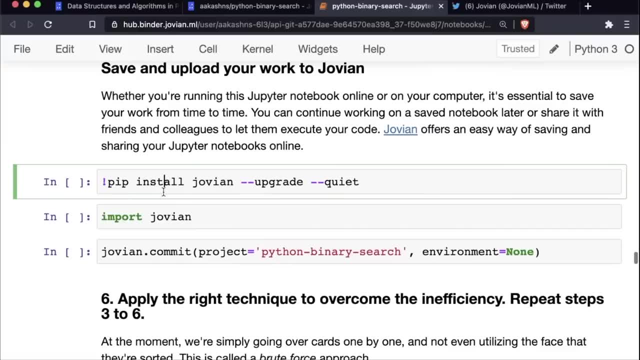 And here is how you can save your work and then pick it up. Everything happens on the Jovian platform. There's no need to download anything, although you could download it if you want, but there's no need to download anything. So all you need to do is use the Jovian library. 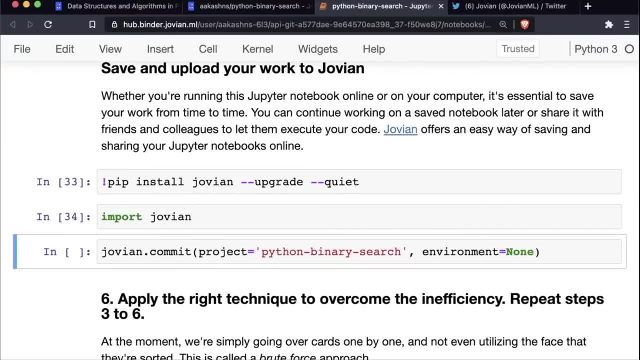 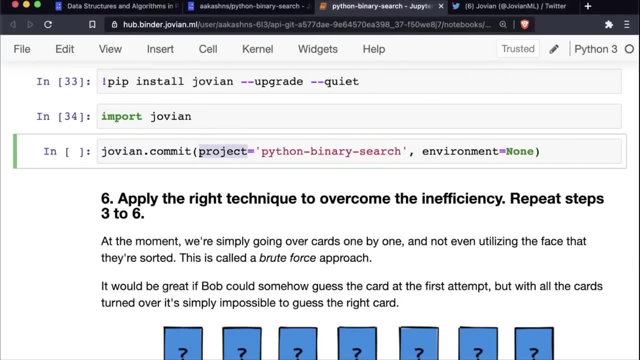 Once again we've done that. Okay, We've got another helpful function for you. So you say, import Jovian and then run Jovian dot commit. So you run Jovian dot commit and then give it a project name, the project name by which. 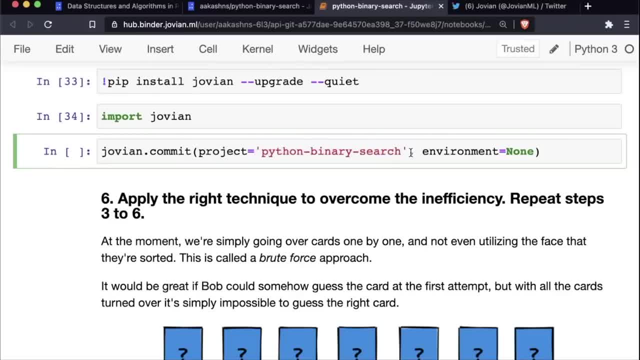 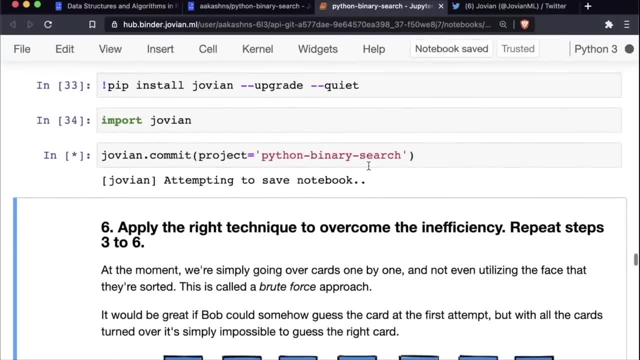 you want to identify this specific notebook- And then there are some other arguments- is not too important, So you can even skip this, and that should be perfectly fine. So now, when you run Jovian dot commit, we will capture a snapshot of your notebook from. 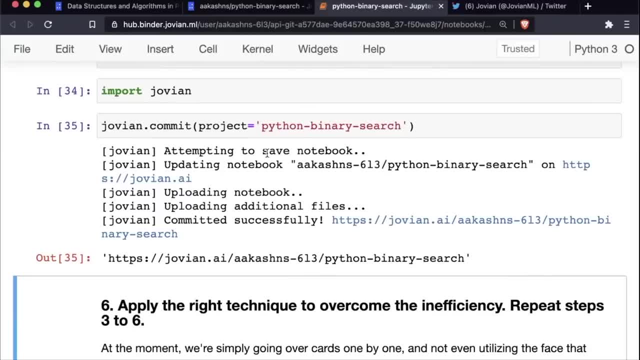 this online platform Or wherever it is running, even if you're running it on your own computer. we will capture a snapshot of your notebook from your computer, wherever it's running, and we will upload it and give you a link where you can access it. 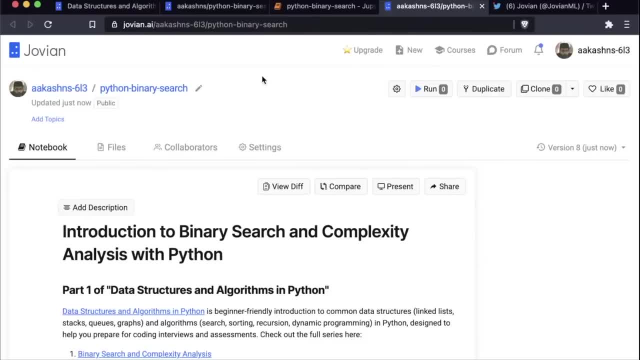 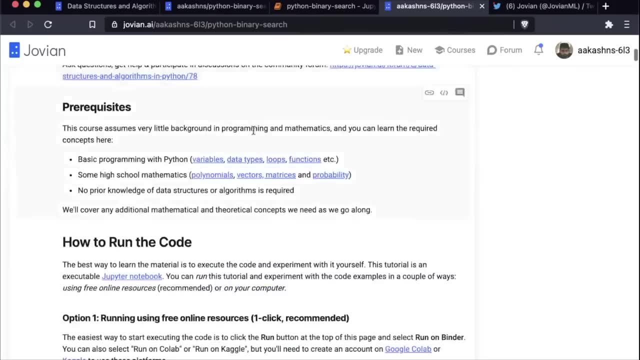 So let's open up this link here. So now you will be able to see this page called Python binary search and it will be on your profile And you can see, you can scroll down and see that it contains all the explanations and it contains all the code. 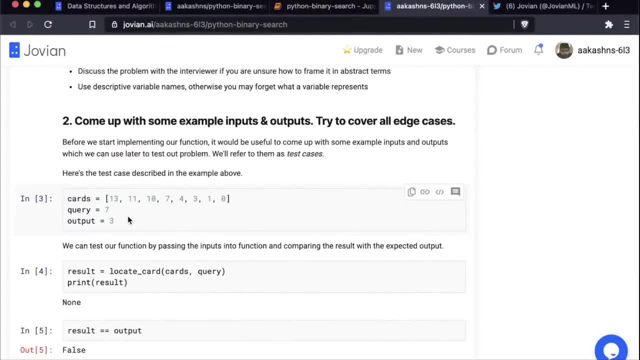 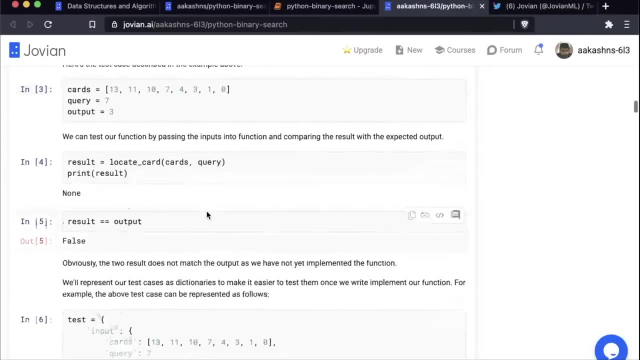 So this is a read only version of the Jupiter notebook. So the read only Version of the Jupiter notebook obviously does not require us to keep servers running so that you can run this code And when, when you need to run it, you know your work is saved, to whatever extent you. 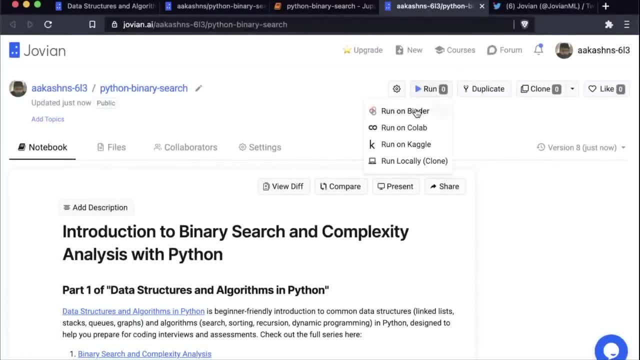 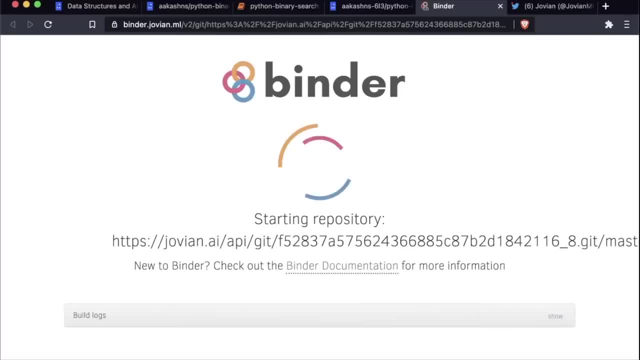 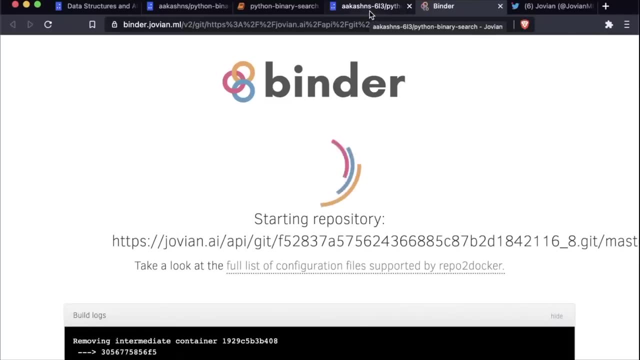 have executed things And now, when you need to run it, you simply click run and then click run on binder once again. Okay, So that is how you resume your work. So what this will do is this will set up a new machine for you, and on the new machine, 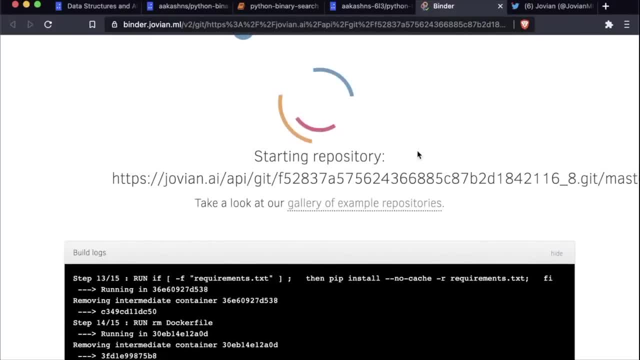 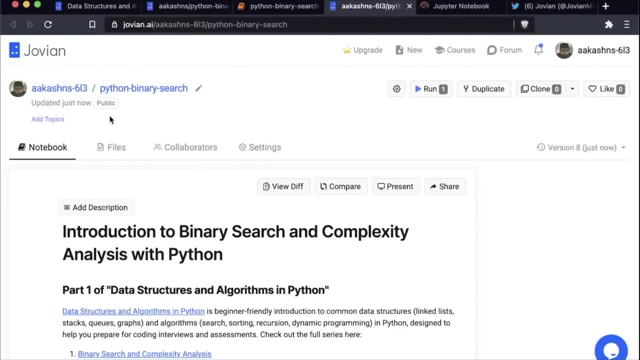 it will post the Jupiter notebook, Okay, And it will start up the machine for you, open up the Jupiter notebook and you will be able to start running the code, and not just you. Now you can make them notebooks public or you can keep them private. 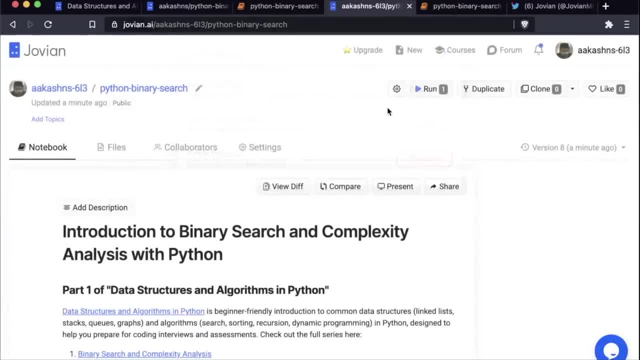 You have multiple viewership options, so your public and private- not just you but anybody else, So you can take this link and tweet it out. If there's an interesting problem that you worked on you want to tweet it out, You can just share this link online and anybody will be able to read through your solution. 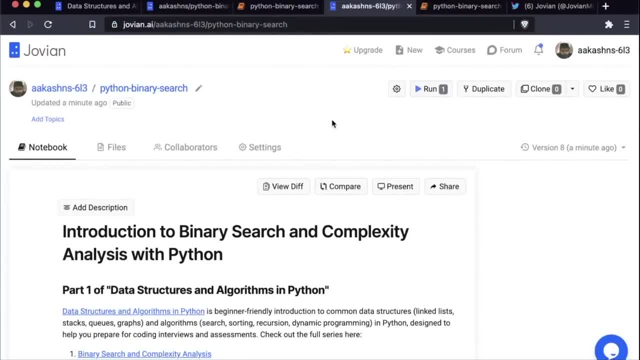 and they can run it as well, Right? In fact, the notebook that I've shared, Shared with you, is hosted on my profile. So Jovian is not just a platform for you to learn, It's also a platform for you to build a repository of projects. 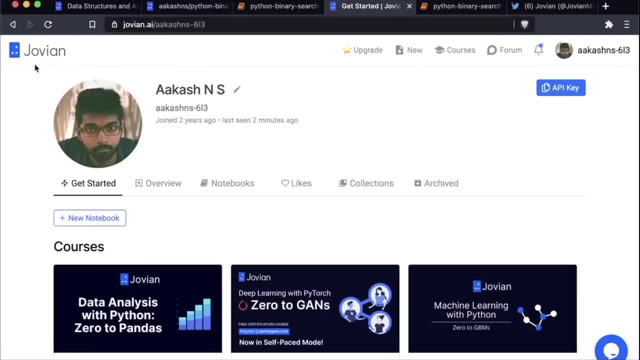 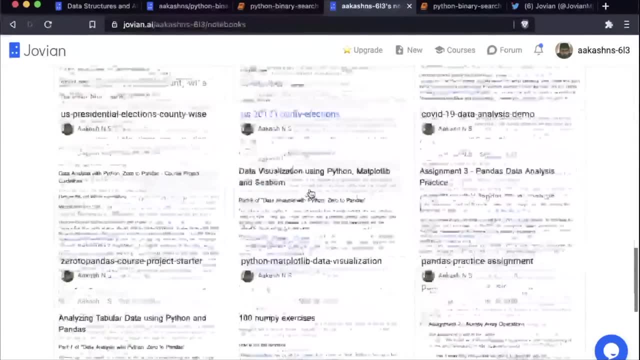 Now, if you go back to your profile, you click on your profile or click on the Jovian logo, and you can see here that you will find a notebook step And in the notebooks tab you will find all the notebooks that you have worked on in the 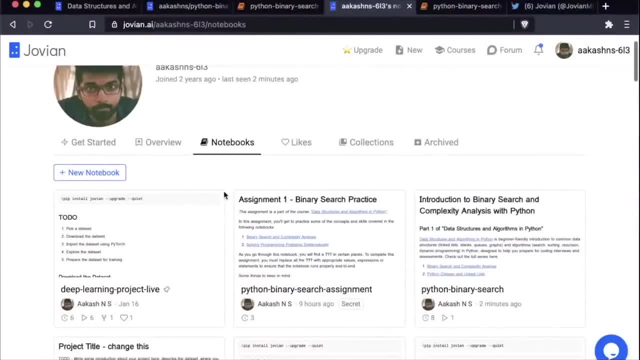 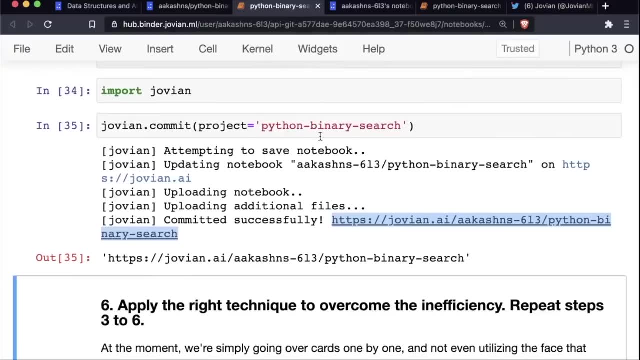 past. Okay. So anything that you've committed using Jovian dot commit, you will be able to resume working on it. So that's, that's how you Save your work and keep saving your work. from time to time, All you need to do is run Jovian dot commit. 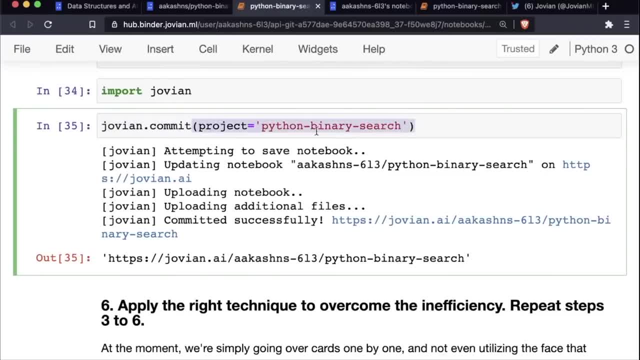 You do not even need to put in this project argument. This is just something if you want to actually give your project a name. otherwise the name will be picked automatically. So just keep running Jovian dot commit from time to time, especially if you're leaving. 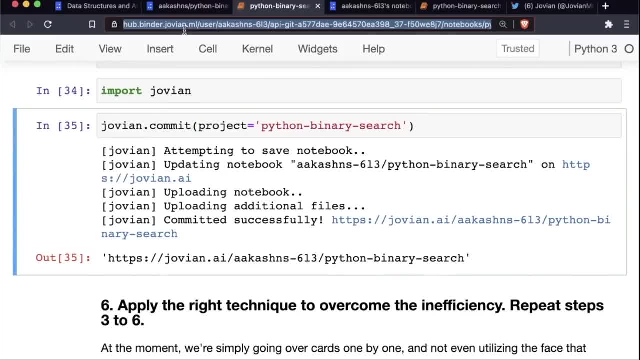 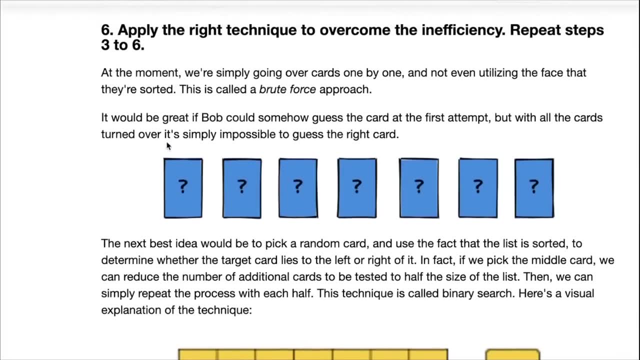 your computer for half an hour or so then and your computer get goes to sleep, Then the server will shut down and you may lose your work. Coming back to our problem, We've just implemented linear search and we understood that it has the complexity of order. 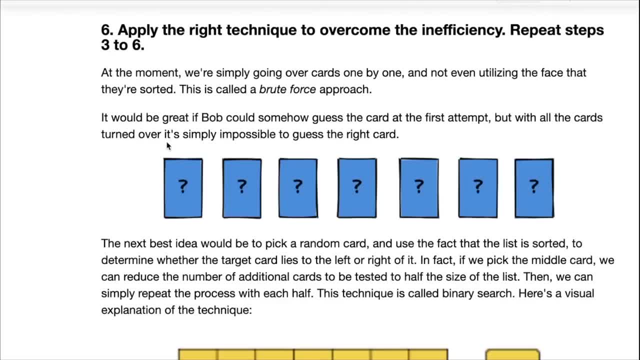 in which is, and that's why it's called linear. It runs in a linear time is another expression that is used. It is also called linear because we are going through the array step by step. Now the next step is to apply the right technique to overcome this efficiency. 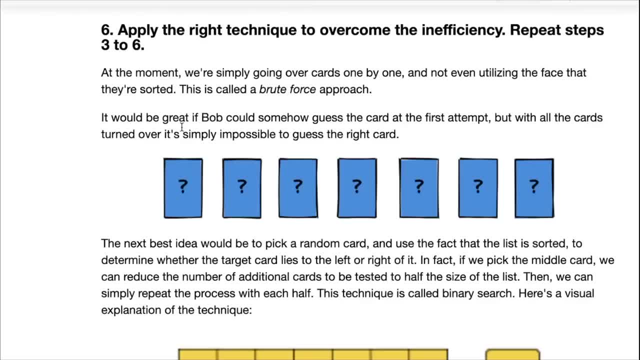 Now, of course, we've not learned any techniques yet, but we can probably figure it out if we think about it, And maybe this is something that occurred to you right at the beginning, And the idea that occurred to you is something that we will now implement. 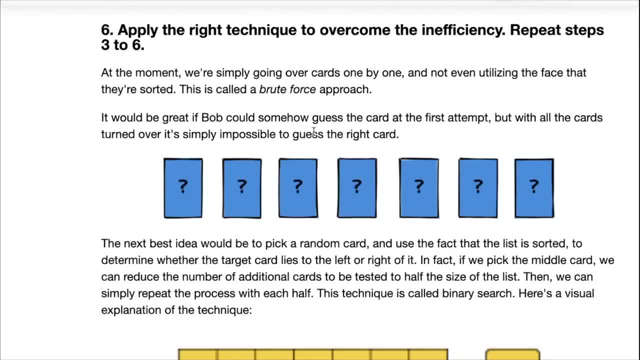 So at the moment, we are simply going over the cards one by one and not even utilizing the fact that they're sorted, And that's why our approach is pretty poor and we're basically checking everything. So it's not a great solution, but it would be great if somehow this would be the this. 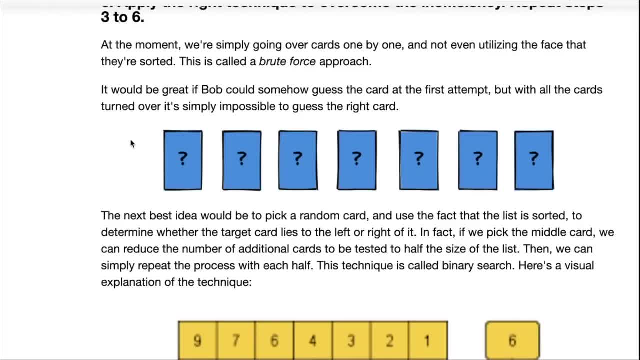 would be the best case If somehow Bob realized somehow Bob could guess the card at the first attempt. that would be perfect. Then that would be an order one, That would be a constant time solution. But with all the cards turned over it's simply impossible to guess the right card. 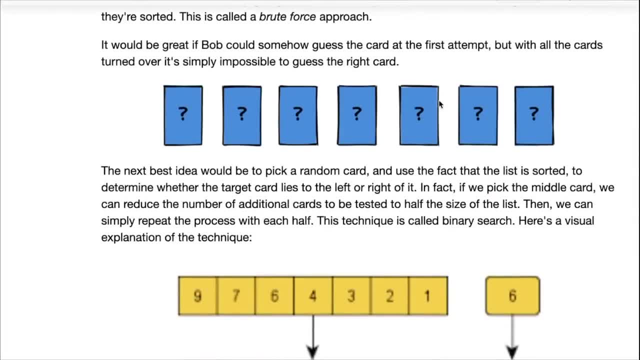 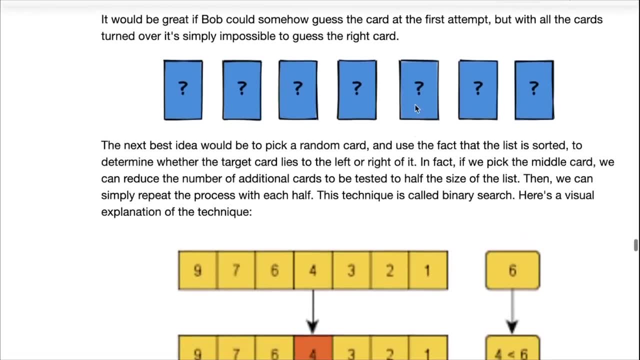 Now the next best idea is to maybe pick a random card. So maybe let's say Bob picks this card and this card turns out to be a nine. Now Bob can use the fact that the cards are in sorted order. So if this card turns out to be nine, that means all of these cards have numbers greater. 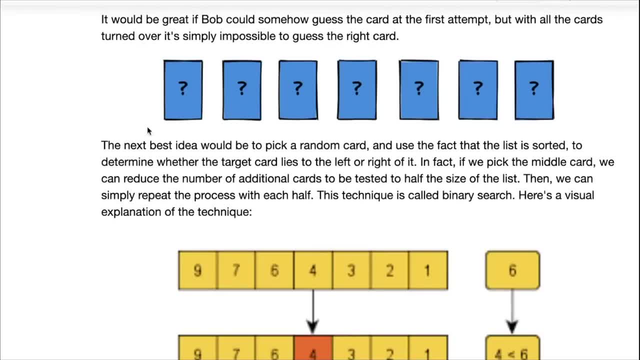 than nine and the target card is seven. So the target card cannot lie in this region. So The target card has to lie in this region And just by picking a random card rather than picking the first card, Bob has eliminated four out of seven cards to be checked right. 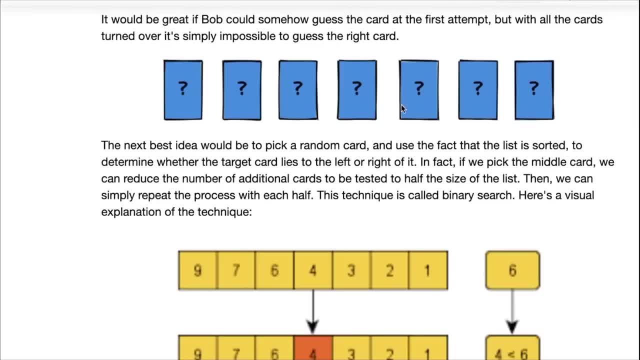 So with one check, Bob has eliminated a total of five cards: one, two, three, four, five, And of course, if this number turns out to be seven, perfect great guess. But even if it doesn't, we've still eliminated quite a few. 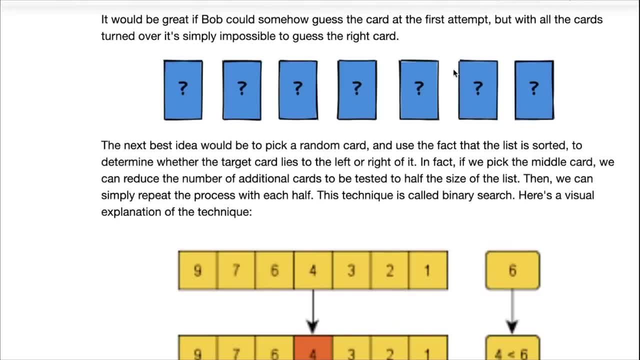 If this number turns out to be less than seven, we've still eliminated three cards. So that's the basic idea here: That we Pick something not from the edges, but somewhere in the middle. Now, what is the best place to pick something in the middle? 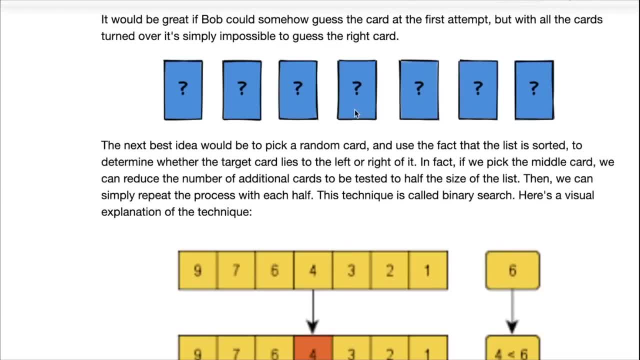 Now, obviously, when we are picking a card, we do not know whether it is going to be less than or greater than the number that we want, especially when everything is closed. So it's best to just pick the middle card, so that, whichever case turns out, it turns. 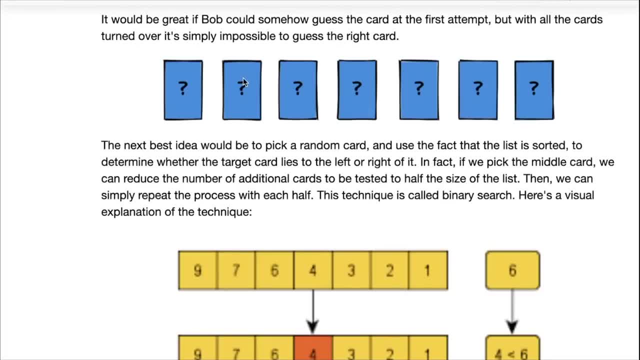 out to be, we're still left with ads. at most three cards to process, right? So if you pick this card and it doesn't turn out to be seven, You either need to look at these three or you need to look at these three. 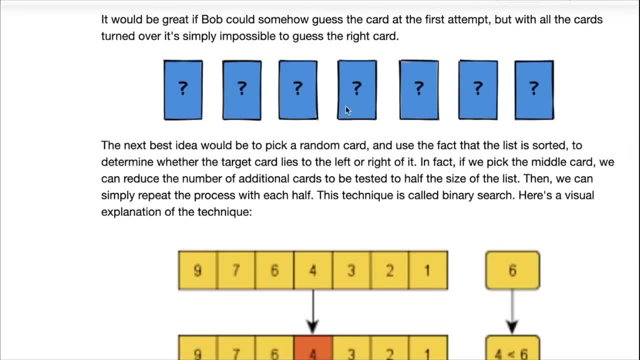 So that is the strategy we'll follow, And this technique is called binary search. And why do it just once? Just keep repeating it. So each time you pick the middle card and you can eliminate half of the area, And this is what the strategy looks like. 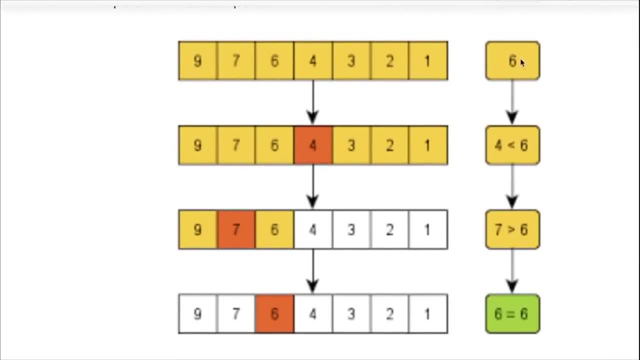 So here we have the area, And in the area where we want to figure out the number six of the slightly different problem, but still decreasing order, we want to figure out the number six, So we access the middle element. Okay, We compare it with six. 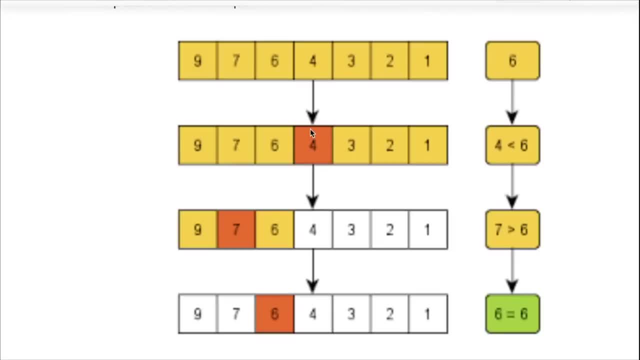 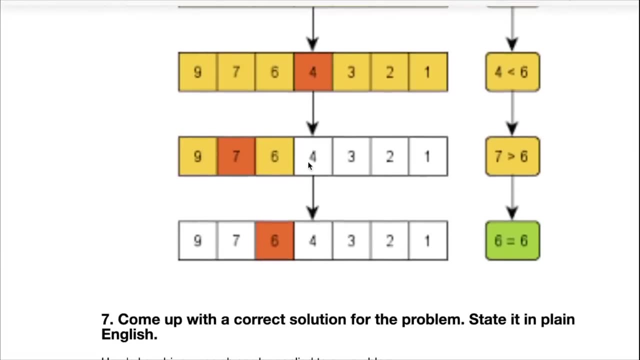 Now it is not six. Okay, It was a bad guess, No problem. But we know that four is less than six. So that means that six lies to the left of four. So we've suddenly eliminated half of the area. We've done one access and eliminated half of it. 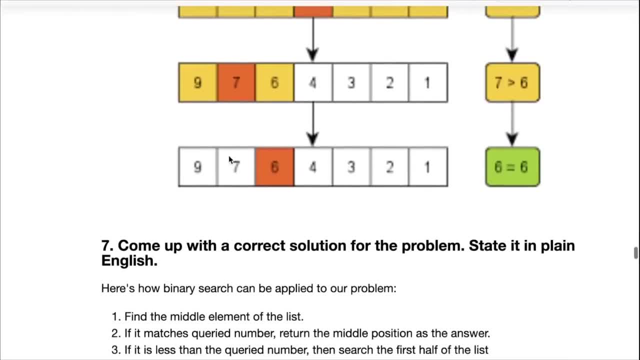 And now we left with three numbers. We pick the middle number. We get seven. seven is greater than six. That means the number lies on the right. Now we're left with just one card. We overturn that last card Or we check that last number. 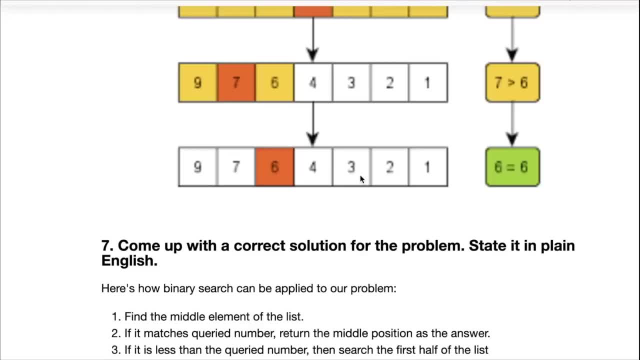 Okay, It is equal to six. Great, If it is not. well, nothing more left to check. All the numbers here are greater than six or less than six, And all the numbers before this are greater than six. So if this number isn't six, then there's no six. 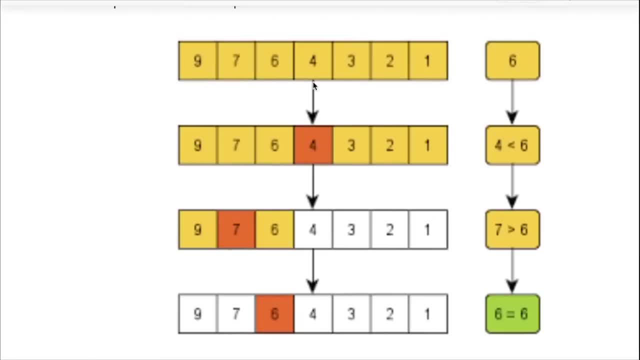 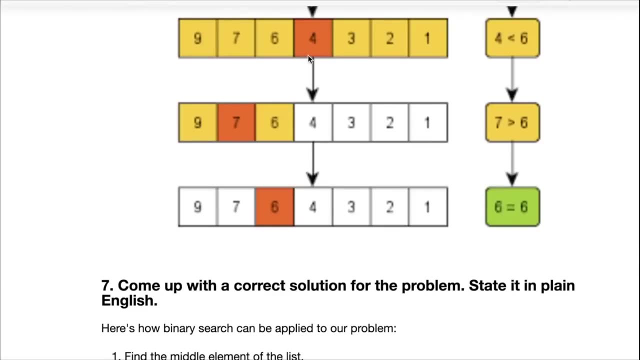 And just like that, for an area of seven elements, we have done just three checks and arrived at the answer. And that was the worst case. right It may, it will never take. you can verify that it will never take more than three checks. 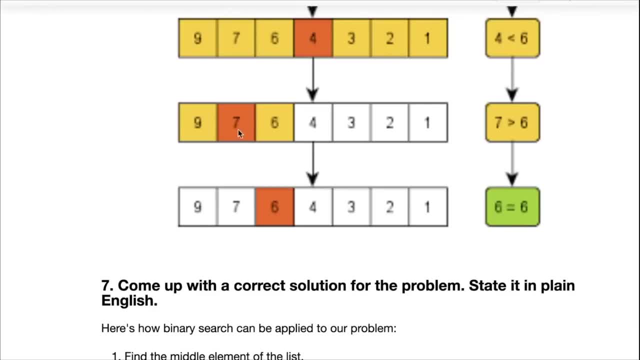 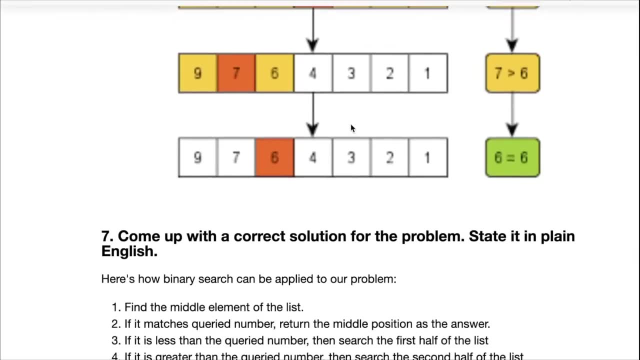 If six comes at this position, we guess it Okay, Immediately. If six comes at this position or this position, we guess it in two checks. And then, if six comes at any of the other positions, we will guess it in three checks. 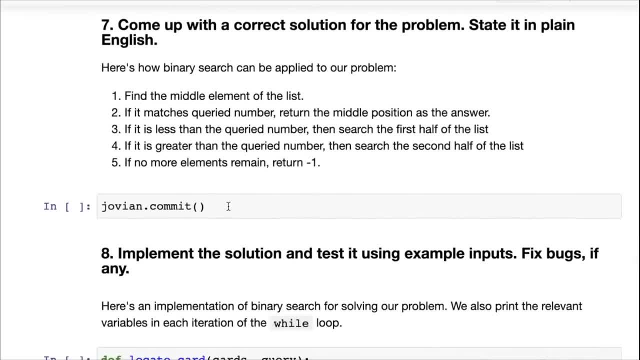 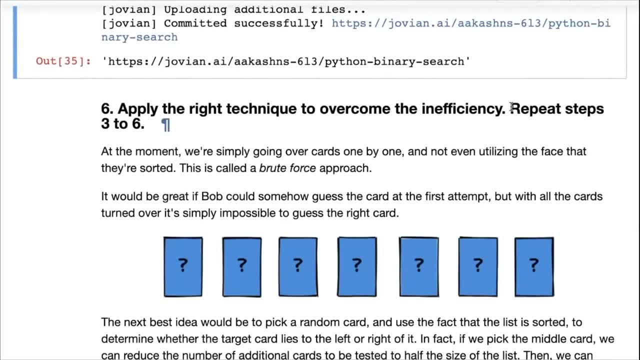 So that's pretty good. And now the idea: if you, if you read this part, it says: apply the right technique to overcome the inefficiency and then repeat the steps three to six. So now we're going to go back to step three, which was come up with a correct solution. 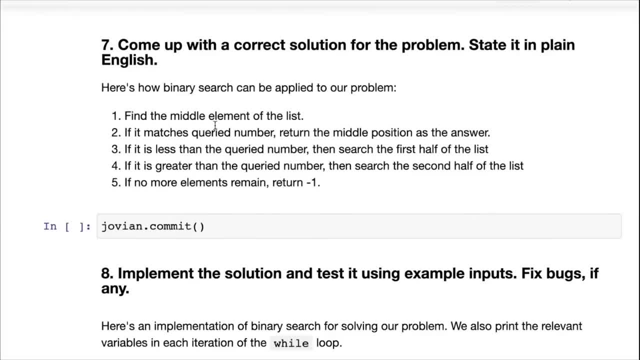 for the problem and stated in plain English: And we have come up with a solution already, We just need to state it. Okay, So here's how this technique called binary search is applied to the problem. It's called binary because, well, we take a left and right decision. 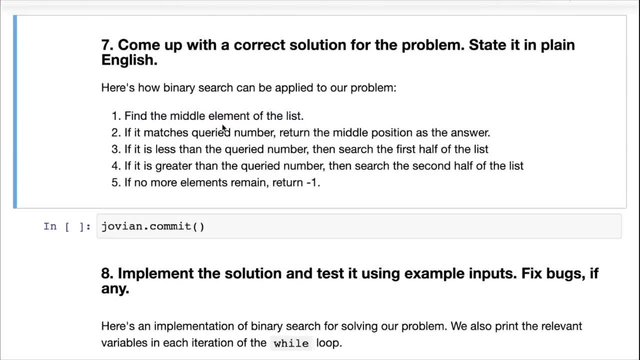 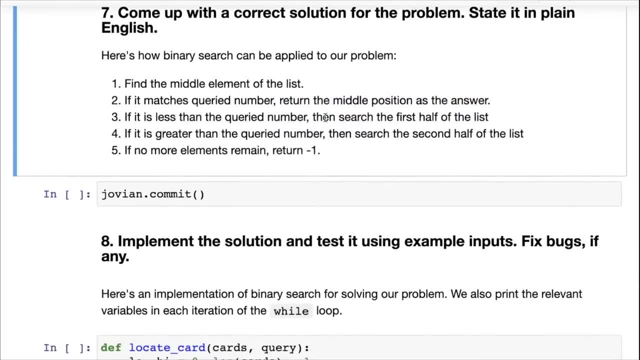 So first we find the middle element of the list. If it matches the query number, then we return the middle position as the answer, And if it is less than the query number, then we searched the first half of the list. And if it's greater than the query number, then we searched the second half of the list. 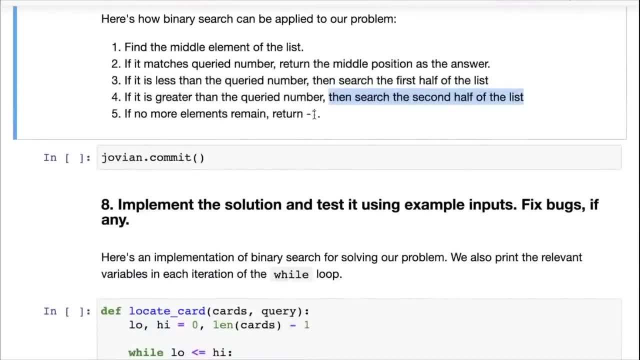 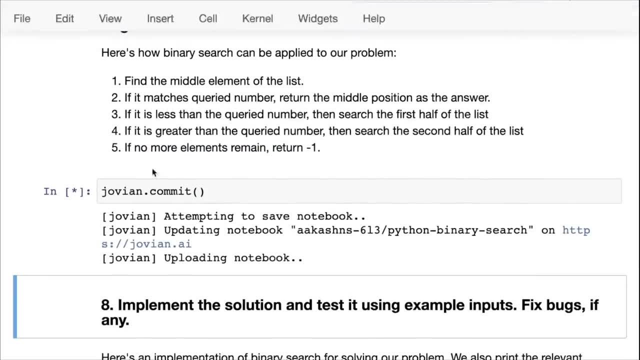 So the exact thing that we saw here, we apply it here. Okay, And finally, if no more elements remain, we simply return minus one. So let's just save our work Now. let's- from this point on, we'll keep saving our work from time to time using Joviancom it. 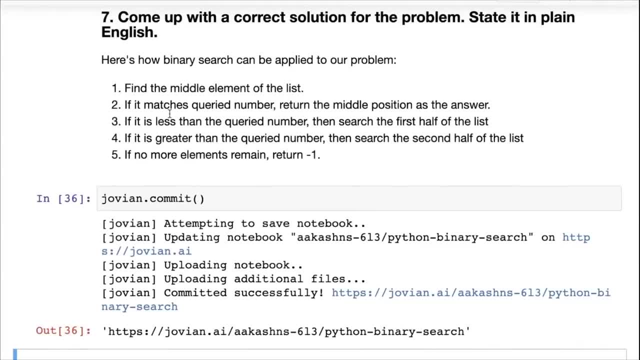 Uh, so now we've come up with the algorithm and you can. again, it's important to write it in your own words. whether you want to write a short description, a paragraph or a step-by-step guide, but write it in your own words and you'll do this in the assignment. 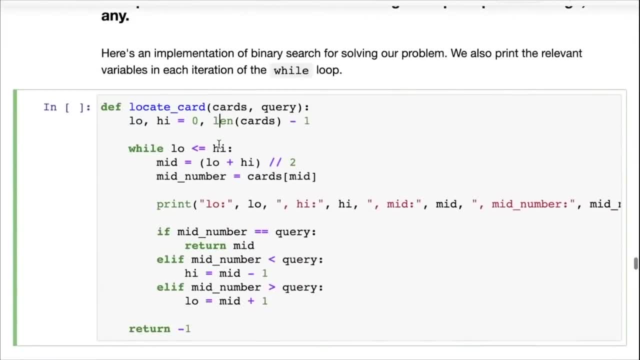 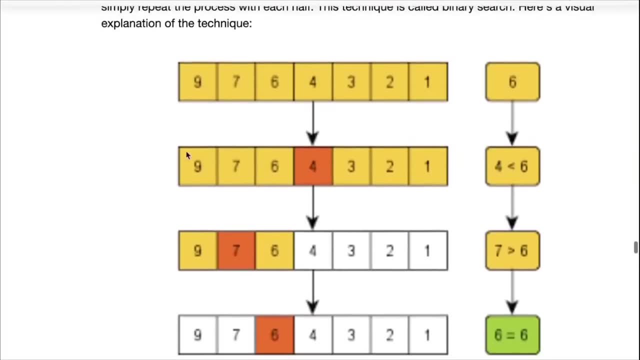 So let's implement the solution now and test it Using the example inputs. So here's the implementation. So what we'll do is we will look at once again, let's go back to this visual representation and we will keep a track of our search space. 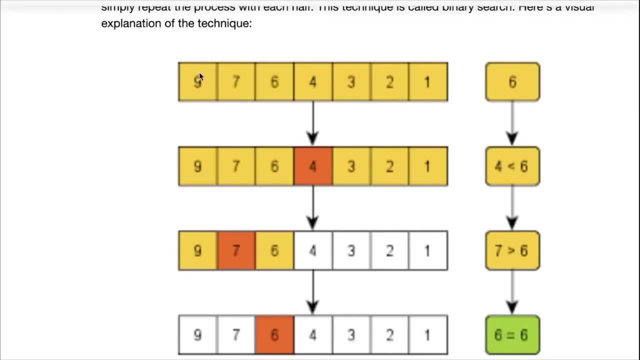 So current, initially our search space is the entire area. So that means we have an area of seven numbers. So our search space goes from position zero to position six and slowly we'll keep reducing our search space over time. So to keep track of the search space we will create two variables: low and high. low. 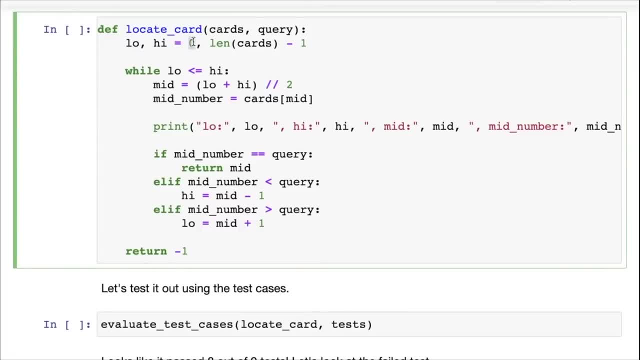 We'll have the value zero, Which is it will point to the first position in the area, and high will have the value pointing to the last position, Last valid position in the area, which is, which is Len cards minus one. So while low, and then the while loop becomes very simple, because as long as we have at least one element in our search space, we can go ahead now to have at least one element in a search space. 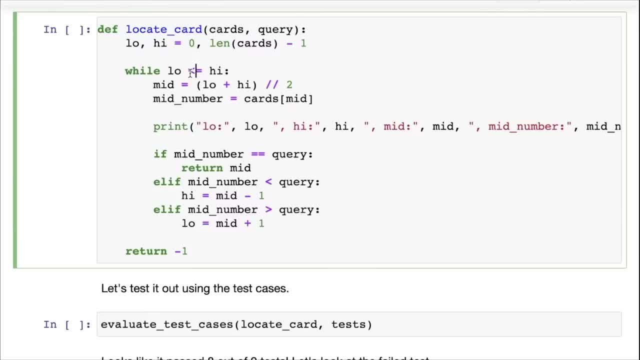 The low value, Which is the starting index, should be less than or equal to the end value, right? So, while low is less than equal to high, because if the starting index is higher than the end index, basically we've exhausted and we've covered the entire list and there's nothing more that we can search for. 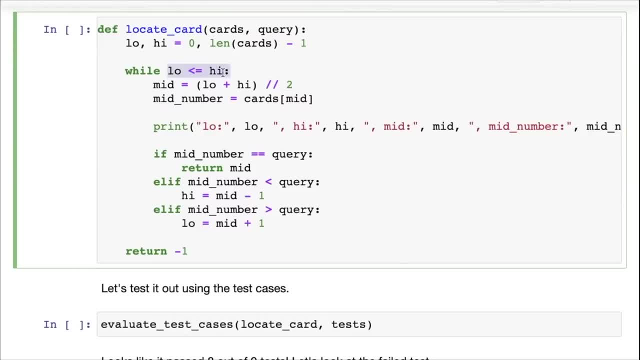 So we should exit at this point. Okay, So now, once we have a, once this condition is satisfied, and it is initially, let's say, you have seven cards, low is zero, cards is a Len card, My One is six, And then you find the middle position. and you can get the middle position by doing low plus high, divided by two. 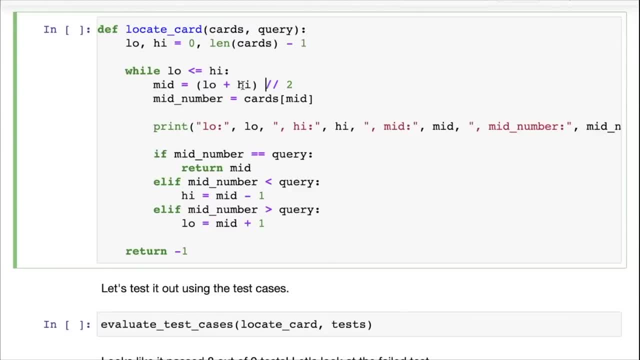 And now let's start applying that strategy here where we say that every time we write a line of code, we should think about how it can go wrong. Now, if you write it like this: low plus high divided by two, and think about how it can go wrong. 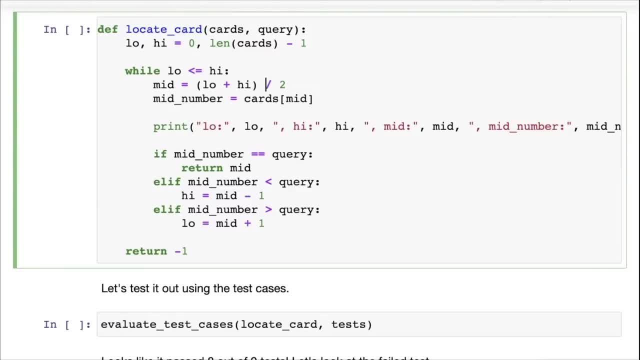 Okay, Low plus high may not be divisible by two, and if low plus high is not divisible by two, you may end up with a decimal number. Now, if you do end up with a decimal number- in fact, The division operator in Python always remains a floating point number- then you cannot use it as an array index, because we want to use this as a position within the area. 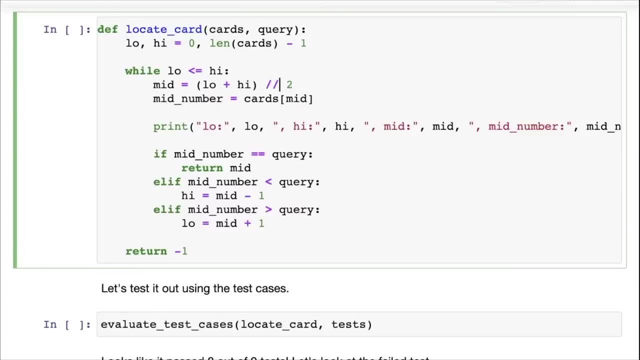 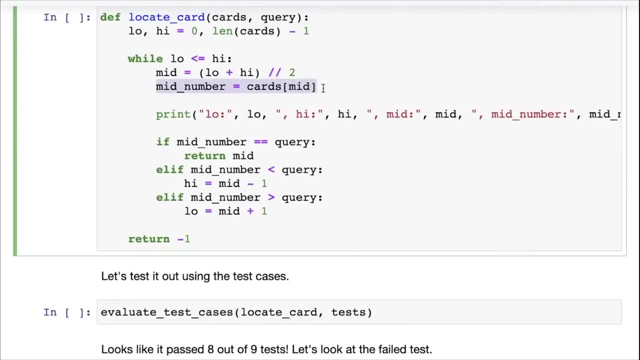 So that's why we need the double slash, which is the, which is the integer division, which simply returns the quotient, So we get the middle position, and then we get the number at the middle position, So we also get cards made, So we access that element from the area. 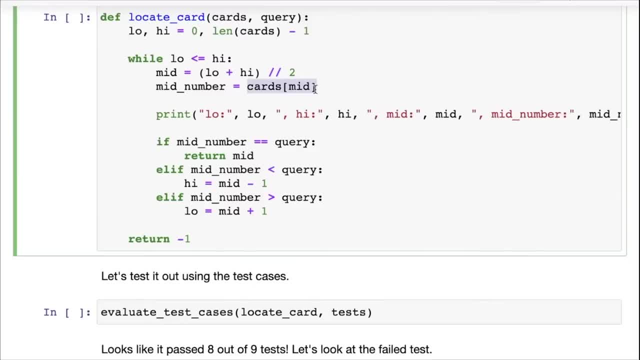 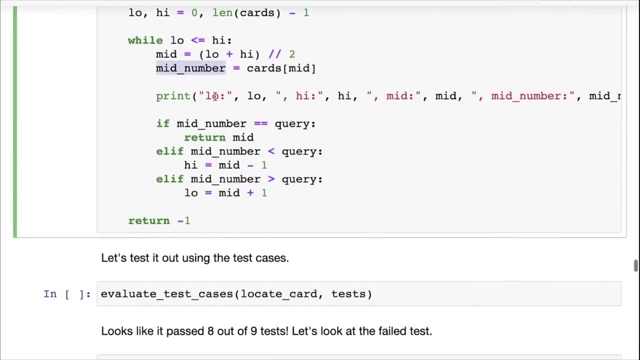 Now, this is where it makes it easy for us to count the number of times we access, because here is One access happening inside the list and there are no other accesses. Then we get the mid number and remember last time we faced an error and we had to add print statements. 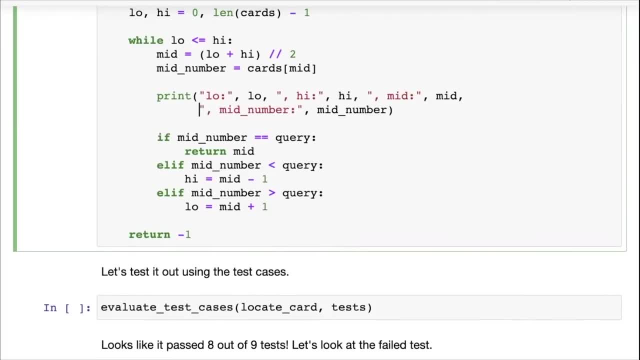 You might as well just add print statements right away. So here's what you can do. We can just print the value of low, the value of high, the value of mid and the value of mid number. What this will do is this will help you check whether the number is working as expected, whether the function is working as expected or not. 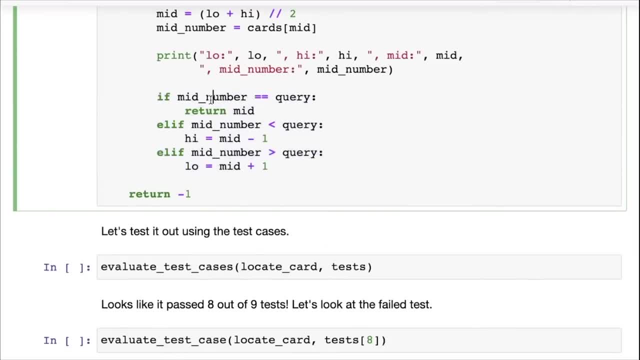 So now here comes The actual check, the meat of the problem. If the middle number matches the query, then we return the middle number. Great, We found it well done. Now, if the middle number is less than the query? I remember the elements are in sorted array and we are looking for the number query. 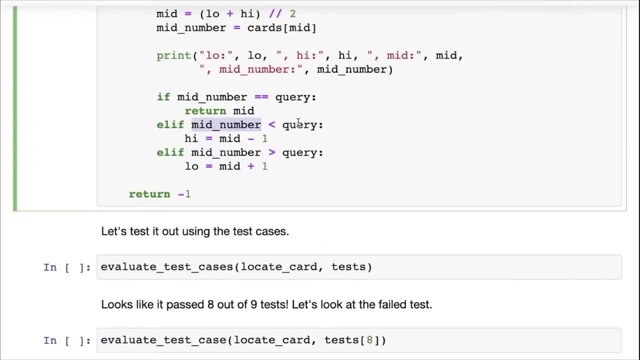 Now the middle number is less than the query, So that means the query probably lies to the left of it, because the query, because the elements are in a decreasing order, Right. So if the query lies to the left of it, so then we need to search with. decrease the search space from the beginning to the position just before the middle number, right. 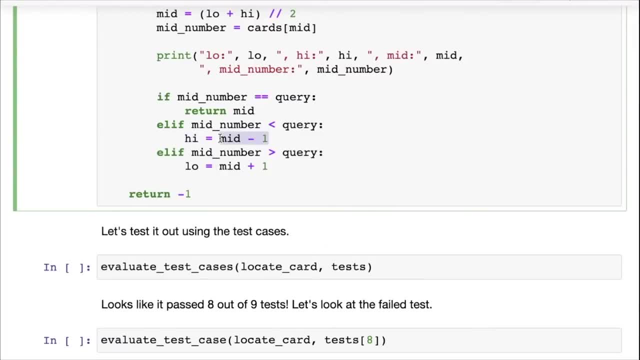 So what we can do is we can simply set high to mid minus one. on the other hand, if mid number is greater than query, So that means because of the decreasing order of the area, the query lies to the right. Now we need to move the starting of the search space to beyond the middle number. 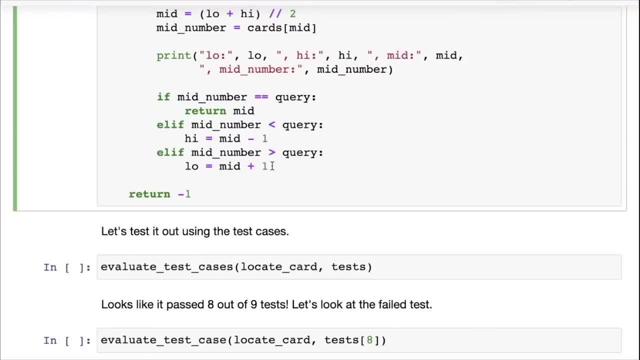 So We simply said low to mid plus one, and that's it. And you can see that we've written a, we've used a if LF, LF loop here, So LF stands for else if in Python. and here the last condition could might as well just have been else, because there are only three possibilities. 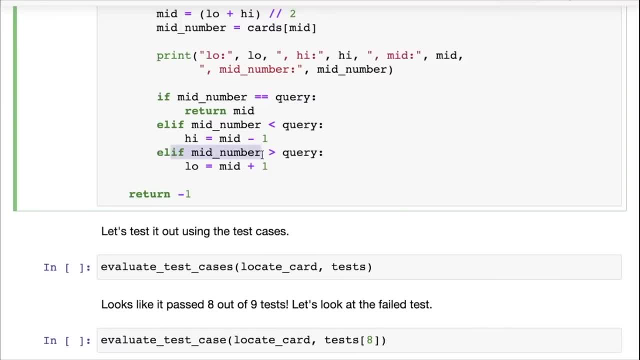 Either they're equal, or mid number is less or it's greater, but sometimes it's nice to list out all possibilities just to make it super clear, and it makes it easy for you, while debugging, fixing issues as well. Okay, So that's our 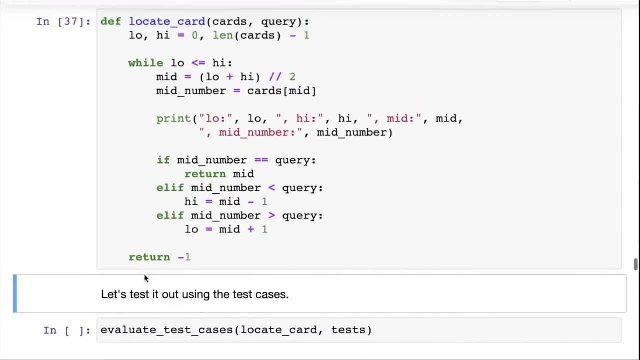 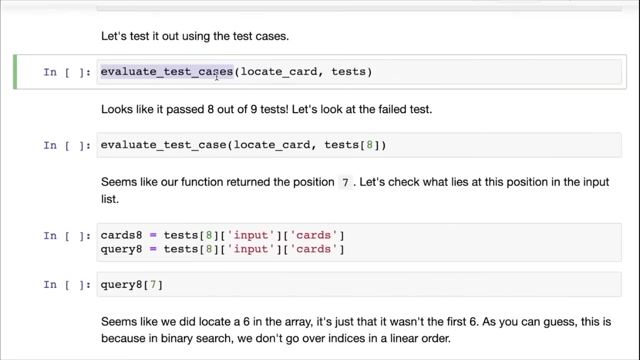 Binary search based algorithm. And finally, when we exit out of the loop, if you have not returned the middle number, if you've not exited the function yet, then we return minus one that the number was not formed. So let's test it out using our test cases, and we have our handy evaluate test cases function here, but you can also test it manually, if you want, by passing individual test cases. but I'll just do this from now on. 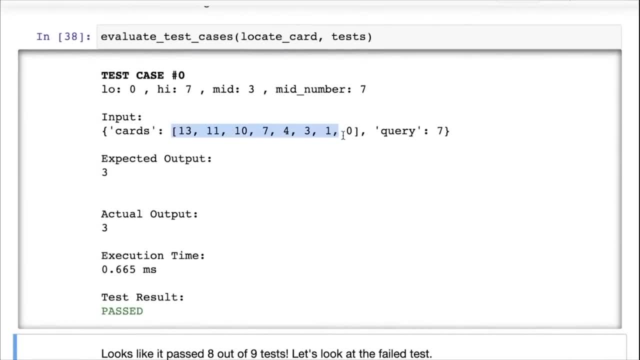 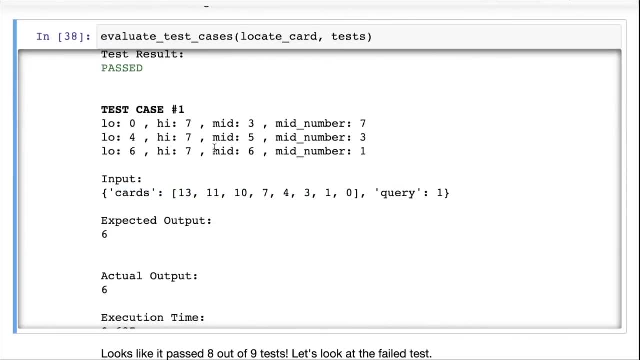 So great. So now we have test case zero: This is the input And this is the query, And it passed. here We have test case one: This is the input and there's a query and it passed. And now, because we have these print statements, we can clearly look into our test cases and actually tell if the if this is tested correctly or not, because now you can see here that we started out with low zero, high seven and a mid mid value of three. 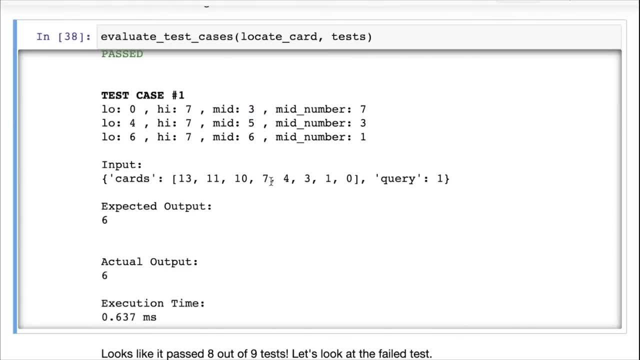 So zero, one, two, three. we, we found the number seven. the query is one, So we need to check this off of the area And that's exactly what we did. We moved low to four And high remain seven. then mid number became three. 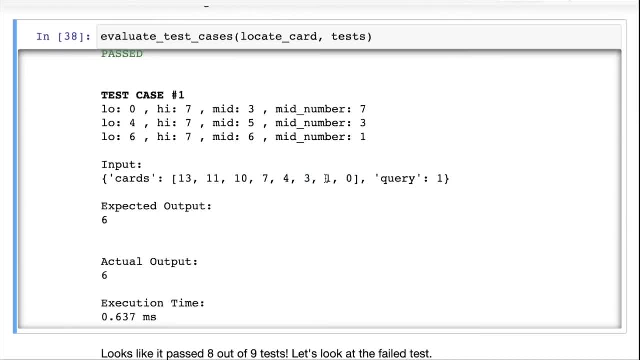 So that means once again, we need to check this off of the area, and then we check this number, and then we found the output. So now you can see exactly how the algorithm works, And this is, in general, what you want as a programmer: you want to have a full understanding of the code that you've written. 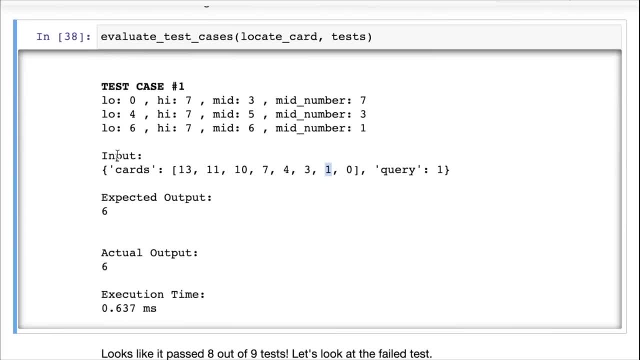 You don't want your code to work- incidentally, You don't want it to. you don't want to be in a position where you are just fixing things, They're trying out different things and somehow At once the code works. you want to be in complete control. 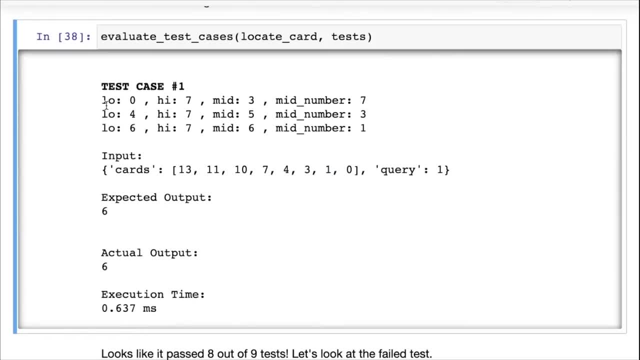 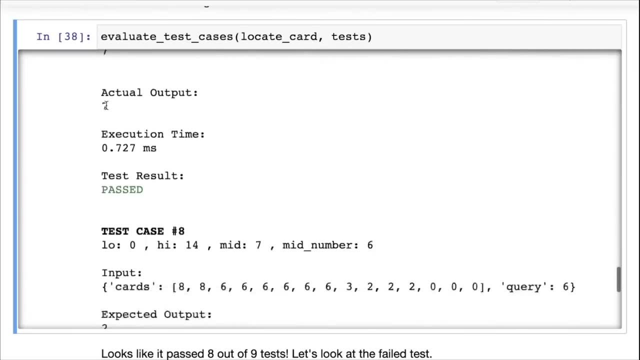 You want to know that these, this is exactly what the code is doing, and if it is failing, why it is failing. So we go to test case two, three, four, five, six. It looks good. It looks like we may have solved everything. 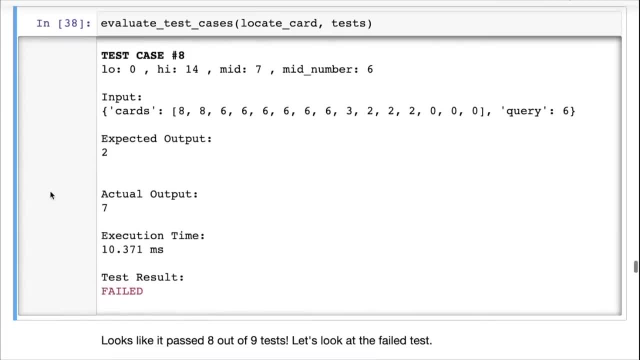 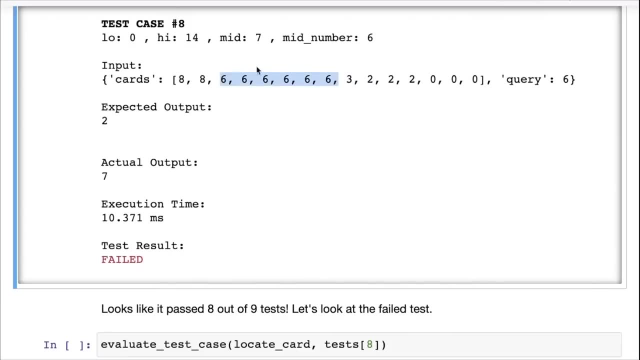 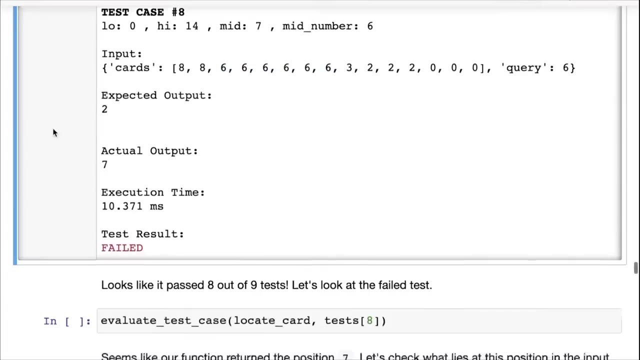 Oh, probably not. So test case eight seems to have failed. So test case eight is this number, this list. and this list contains repeating numbers and not just repeating numbers, but the query itself occurs multiple times. And now, if we look here and maybe let's go go down and evaluate just the test case separately, 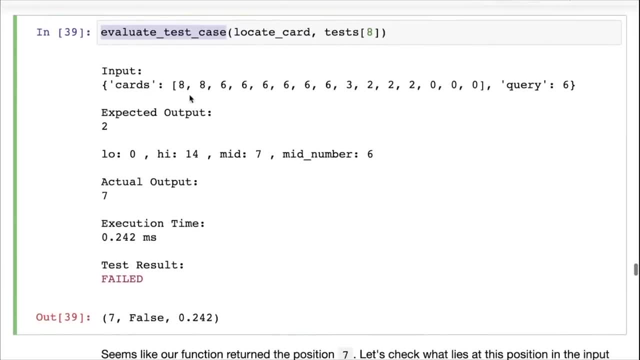 So here we are now using the singular version of the evaluate function. So if you look here you can see you have eight, eight, six, six, a bunch of sixes, then three, two, two, zero, the query six. 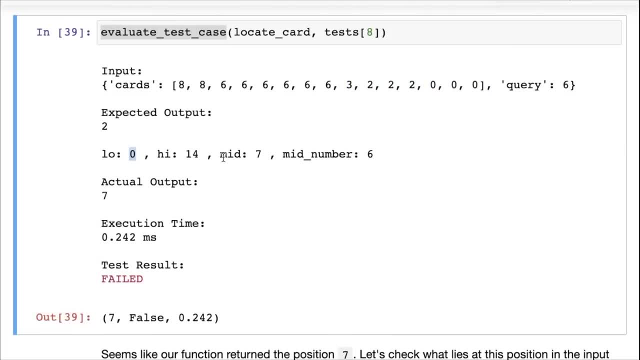 So we start out with a low of zero, higher 14, total of 15 elements. that gives you a middle position of seven and the mid number at that position. So let's count one zero one, two, Three, four, five, six, seven. 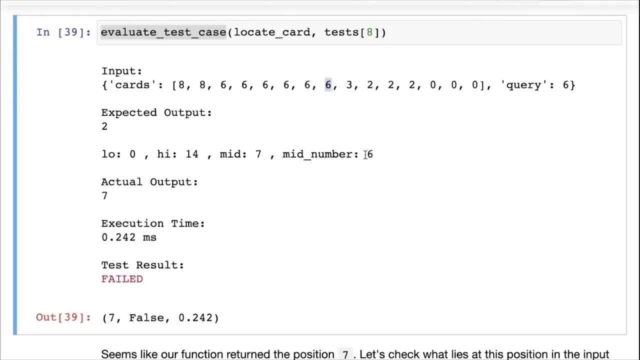 Okay, And the mid number at that position is six. Great A six is also the query, So that's why our function returns seven. But remember that we had decided that our function should return the first position of the number within the area. 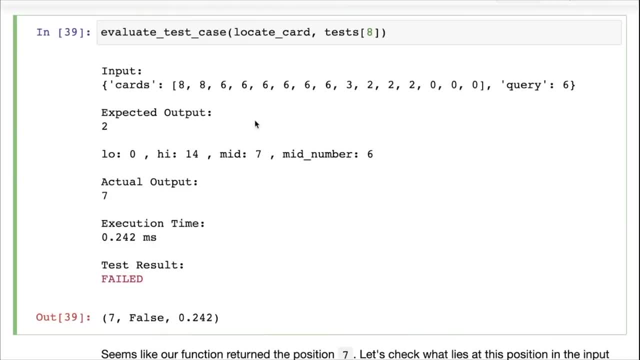 So our function is failing that condition. And why is that happening? Because, unlike linear search, where we start from the left and so we'll always bump into the first position because of the Okay, Decreasing order of elements, So we'll hit, we'll encounter this six before we encountered this six, binary search does not access elements in an order. 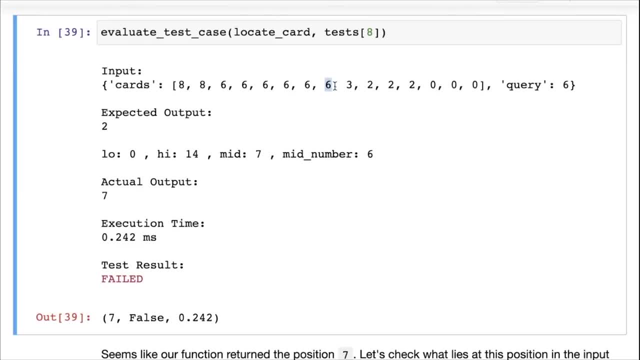 It access elements sort of randomly. There's still a strategy, but it goes left and right And it also depends on the values of specific elements. whether this element is accessed before this element can depend on the value of, let's say, this element, right? 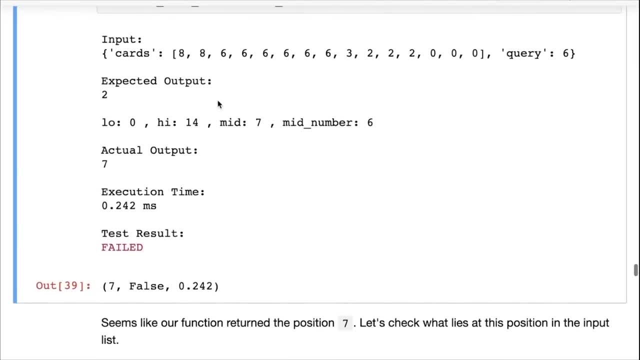 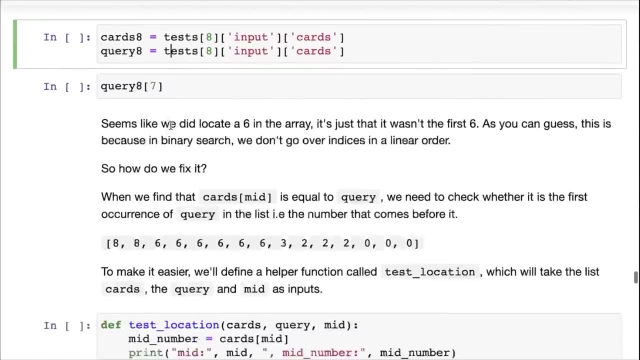 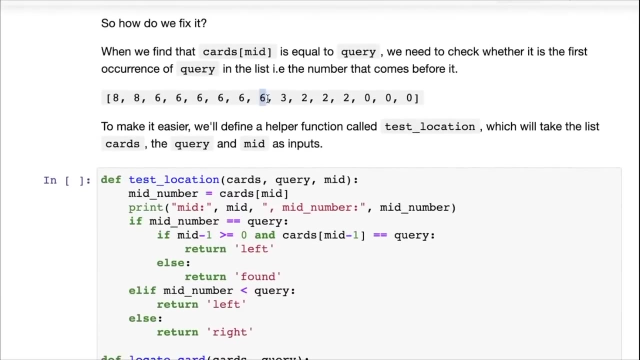 So, as such, it's kind of a pseudo, random kind of order, And so we need An additional condition condition to keep track of it, right? So how do we fix it? So the way to fix it is actually quite simple. When we find that the middle position in a particular range is equal to the query, we simply need to check whether it is the first occurrence of the query in the list or not. 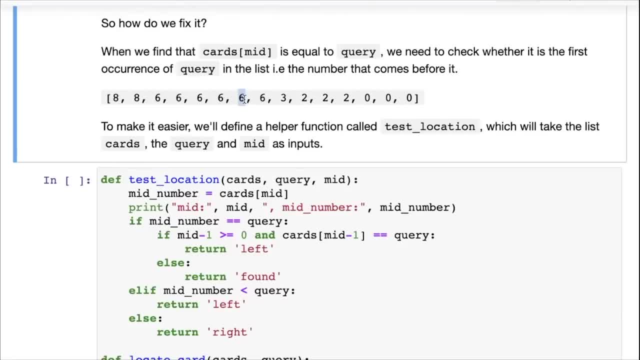 That is, whether the number count that comes before it. is it equal to query or not? If the number that comes Before the middle element is also equal to query, then obviously the middle element is not the first occurrence. So that simply means that we can go back, and because it can occur multiple times before, that simply means that we can go. we can now search the left half. 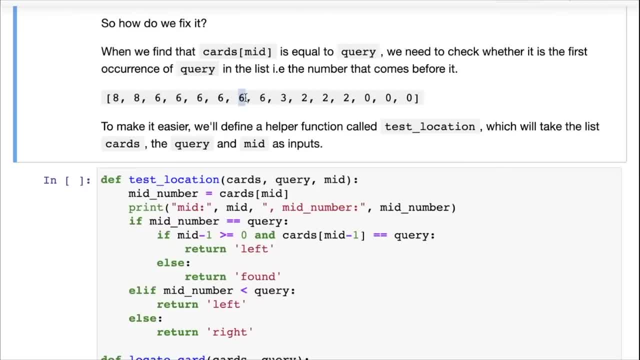 On the other hand, if the middle element, if the number before the middle element is not equal to query- and obviously, because it is a sorted list, it will be greater than query- then all the numbers here are going to be greater than the query. 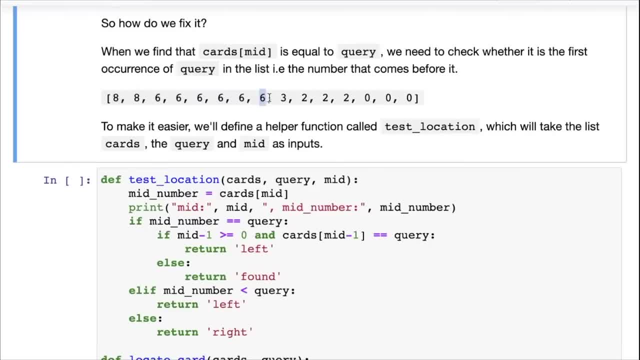 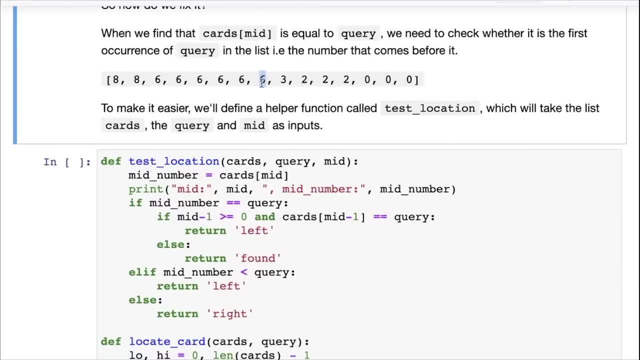 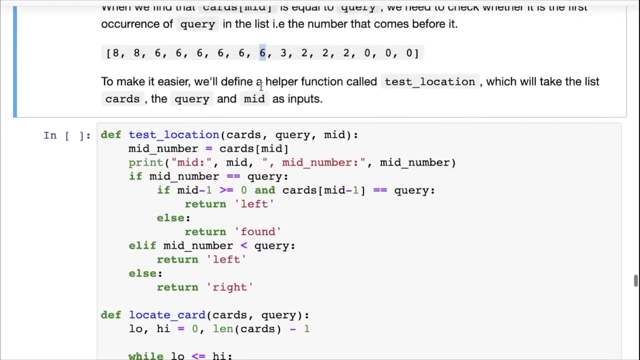 And no the, the, and so this: This must be the first or the only position, Okay, So make sure you understand that this must be the first or the only position where the query occurs. So, once again, to make it easier, what we will do is because there is some logic involved here. what we'll do is we'll define a helper function called test location. 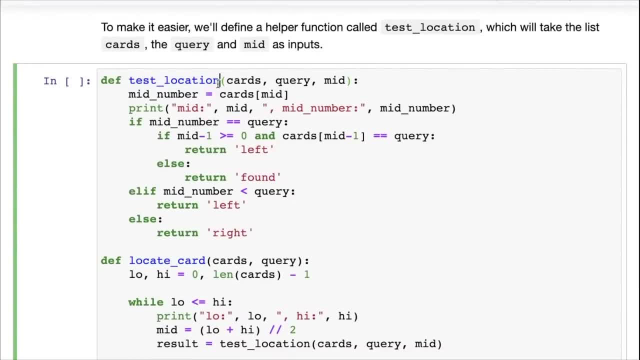 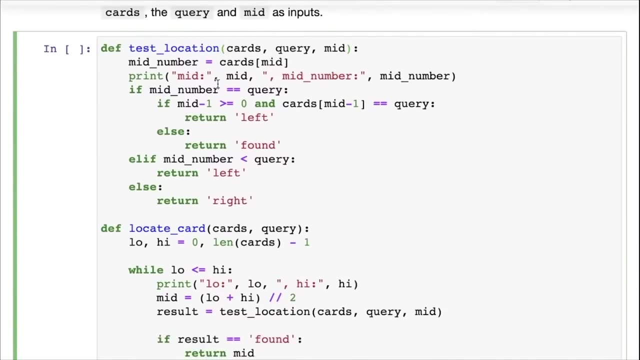 And this is a very helpful thing that you can do every time you find that, okay, you have to. you have to cover these special cases, and your function may start to get slightly longer and slightly more Completed. What you may want to do is create a helper function, and a good rule of thumb is not to have functions that are more than 10 lines of code, or so I try to keep my functions below seven lines of code, because seven, eight lines is 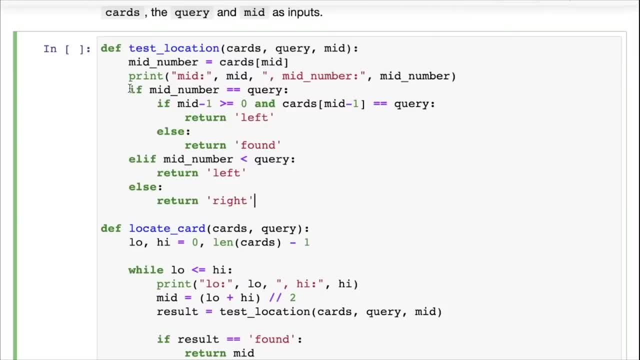 Approximately the amount of information that you can hold in your head at once. So if your function is about seven, eight lines, you can probably take a quick glance and tell what it's doing, identify issues, but anywhere beyond that it's very hard. 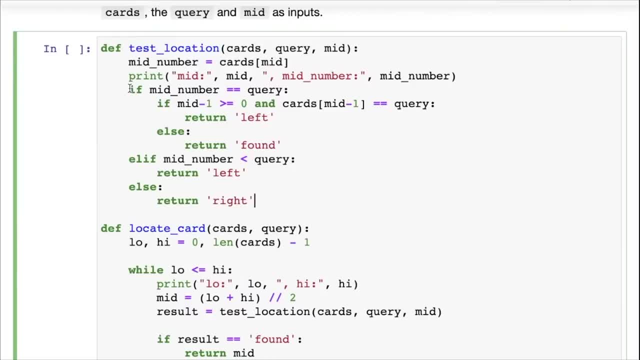 And If you're writing Functions that are going into hundreds of lines, please stop doing that. Please start breaking your code into small functions. There's a. there's a quote by- I forget who it is by, but he's a creator of. I think it's Eric Meyer. 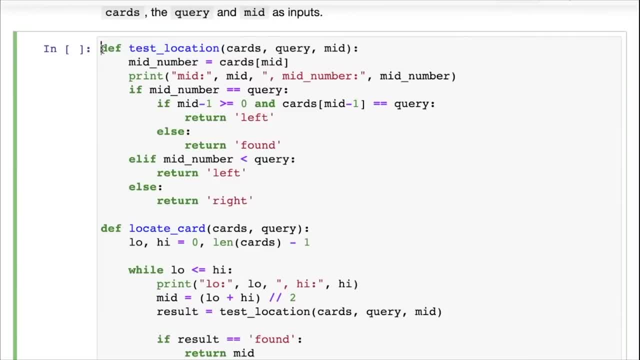 He created the RX library for reactive programming And he said that great programmers write baby code, which is really small bits of code that anybody can understand with a single look. So you should be writing as many functions, as many Small pieces of code, small pieces of logic, as possible. 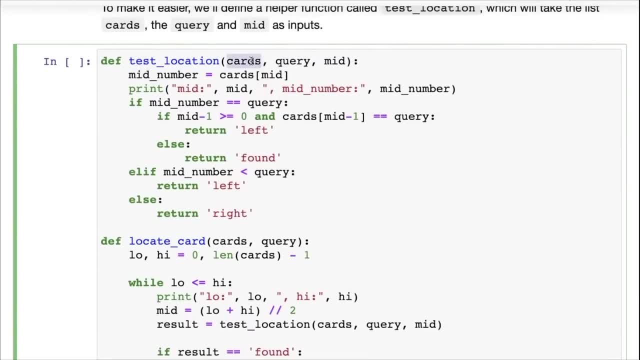 So let's see a test location function. It's purpose is to take the query and then take just a specific position. So forget about binary search for now. just take a specific position and tell if that position is the answer. And how do we do that? 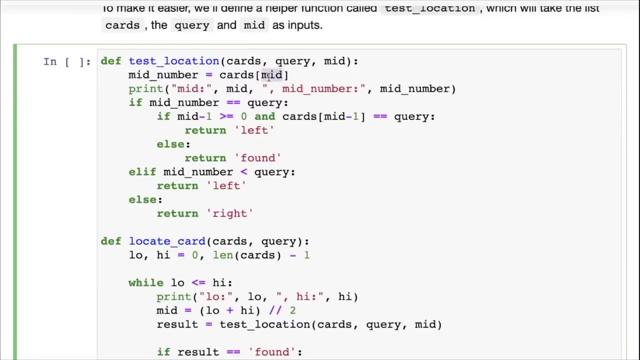 We first get the mid number from the cards, So we get a mid number from cards, So we then we print out mid and we print Out mid number and then we compare the mid number with the query. So this is a special case that we need to handle. 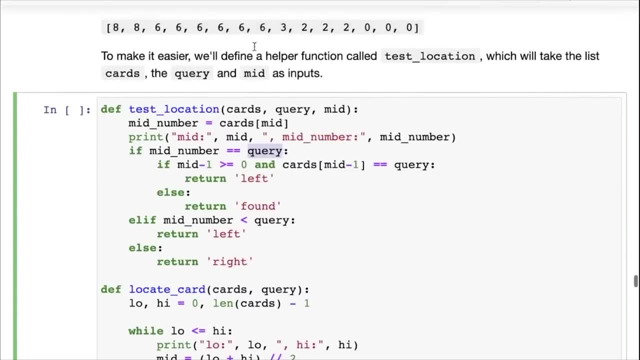 This is where we had the error. Now what we need to check is if the element before the mid number is also equal to query. So if the element before the mid number is also equal to query, then we need to go left. So just to make it super clear what we lose, instead of setting high, low et cetera, we'll simply say that we need to go left. 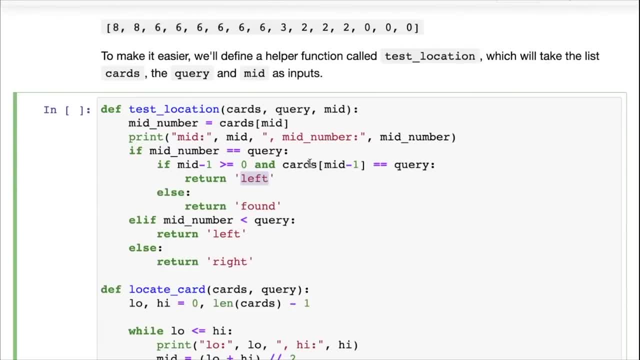 So we'll return the the actual string left. but one thing to keep in mind here, because, once Again, whenever you're accessing an area, you need to make sure that the index is valid. So we simply check that mid minus one should be greater than or equal to zero. 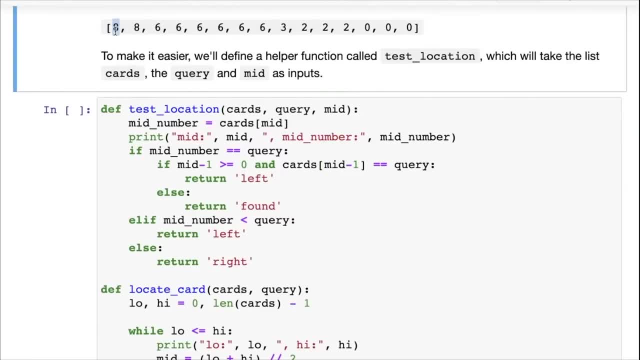 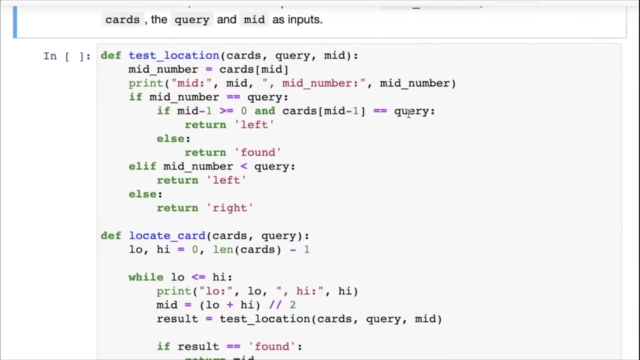 That we made is not this position and which can happen as your search space decreases, For example, if this is your search space, your mid will actually be this position. So if it is equal to the number before the mid number is equal to query, then we return left. 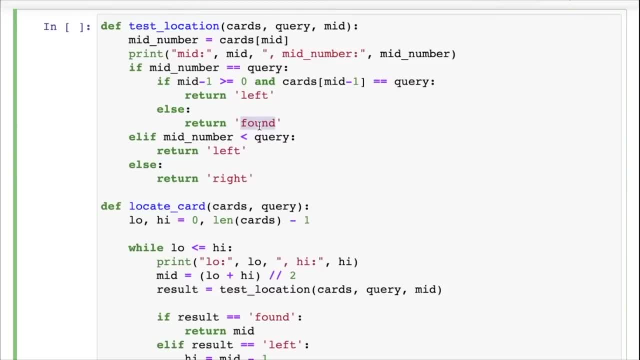 Otherwise we return found once again making it very obvious that we have found the number. So we return phone. else The other case is if the mid number is less than query, that means that the query lies on the left because of the decreasing order of the list. 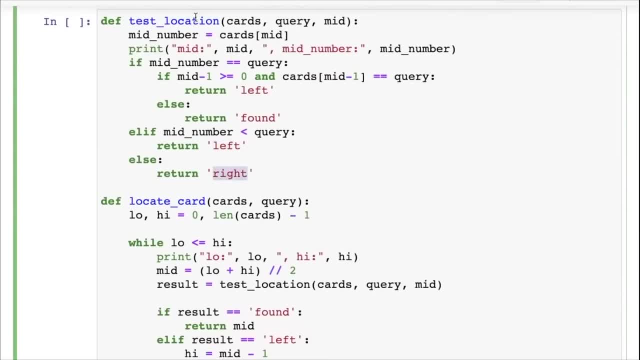 So once again, we need to search on the left, else it returns right. So a test location simply tells us whether we found the solution. or we need to look on the left or we need to look on the right. Now in sometimes you will see programs, especially in C, plus plus Java, return something like minus one, zero and one, and then use that. 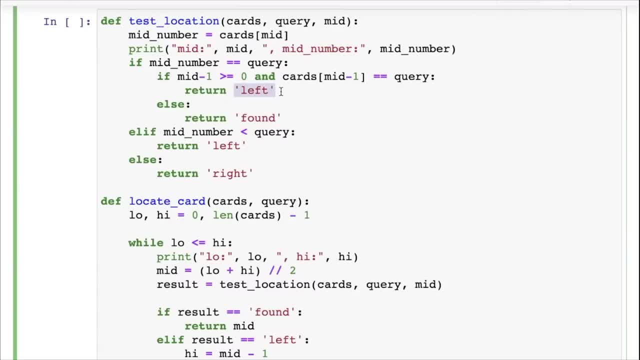 To represent whether you should go left and right, But Python is a high level language and strings are a first-class things are first-class feature of the language. So just use strings because they're really descriptive. They make your code readable. Somebody else reading your code will be able to understand. 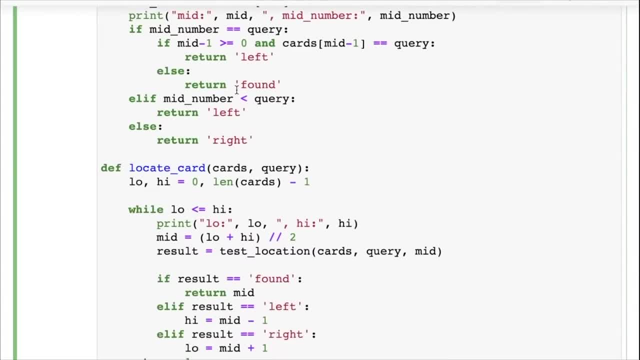 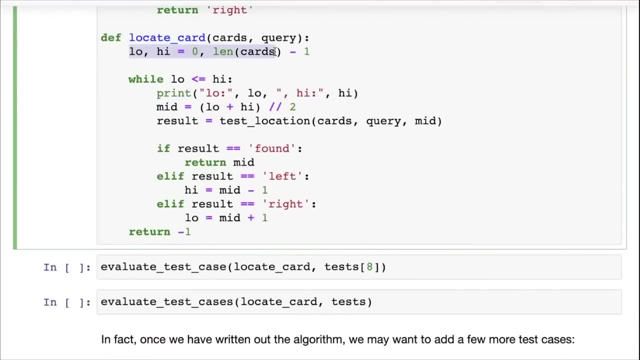 Now, if you're looking at minus one plus one, et cetera, that is going to be difficult for people to understand. So now we can now simplify a locate card function Once again. we have our low high land cards minus one, a zero, and land card minus one. 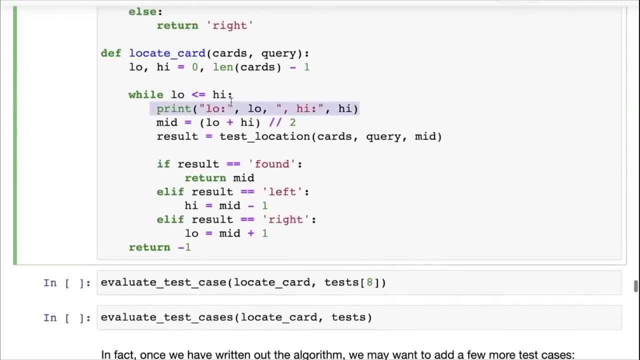 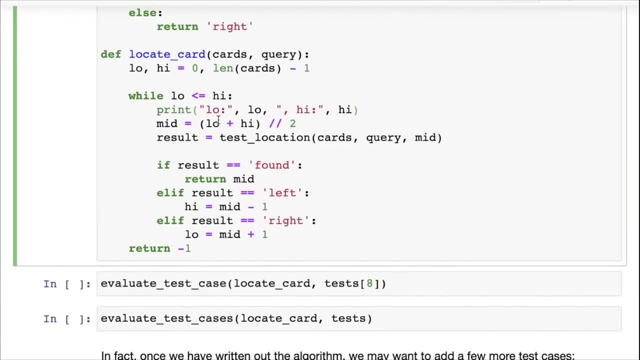 The while loop is the same And we print low and high As well. So we are printing low and high inside the locate card function And then we are printing mid and mid number inside the test location function, wherever is the right place to print something you printed. 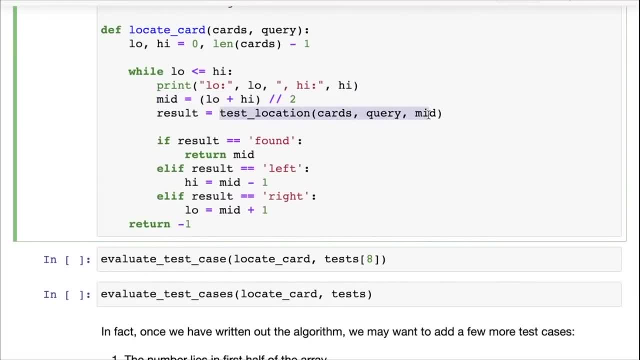 Then we get the mid position and now we simply call it test location. So we are testing if mid is the answer And if it is not the answer, should we go left or should we go right Now? that makes it really simple, because now we get this result and we check this result. 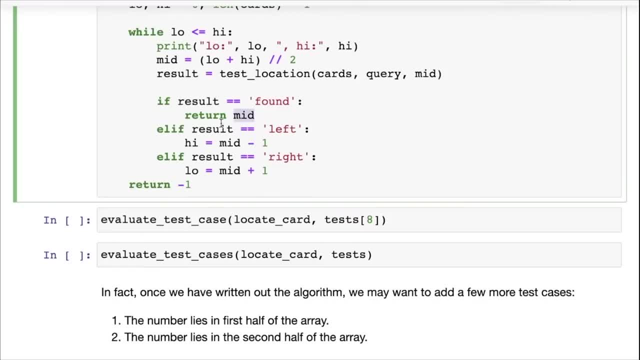 And if it says found, then we return mid. That's the answer. If it says left, then we return mid minus one, or then we simply move high to mid minus one, And if it returns right, then we simply set low to mid plus one. 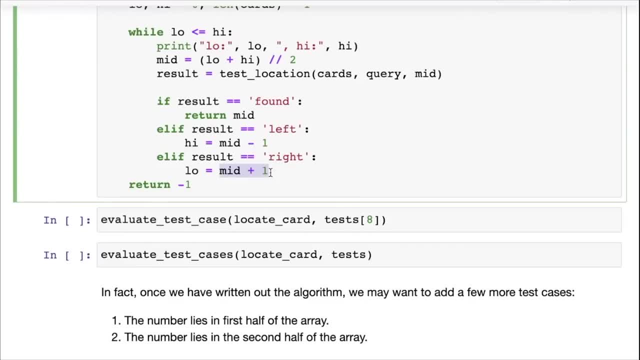 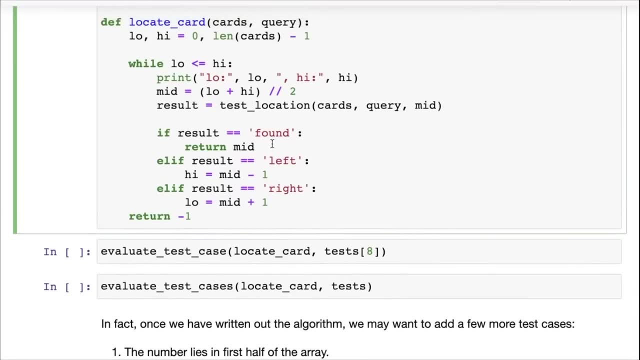 So we are simply changing the start position of the search space to after the middle element, And here we are changing the end position of the search space to before the middle element, right? So this makes it extremely obvious and it's really hard to go wrong when you write code like this, especially. 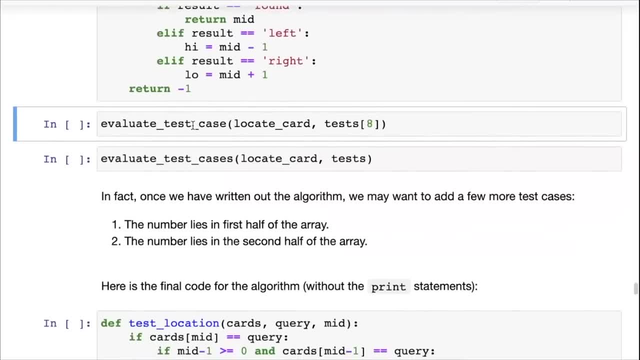 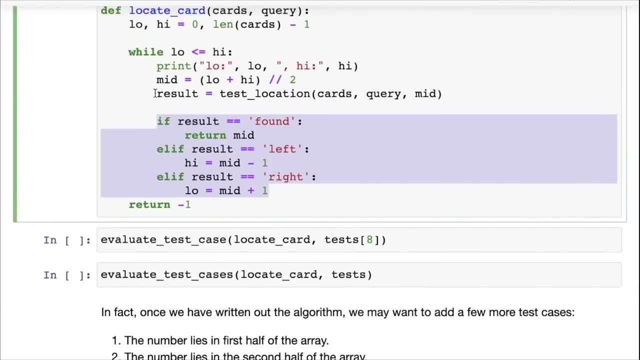 So when you have a binary search problems especially tricky because they always have certain These special cases that you need to handle And if you start handling them within this if loop. so now you have a while loop inside which you have an if loop, inside which you have another, another if statement, and it can get pretty tricky and difficult to debug. 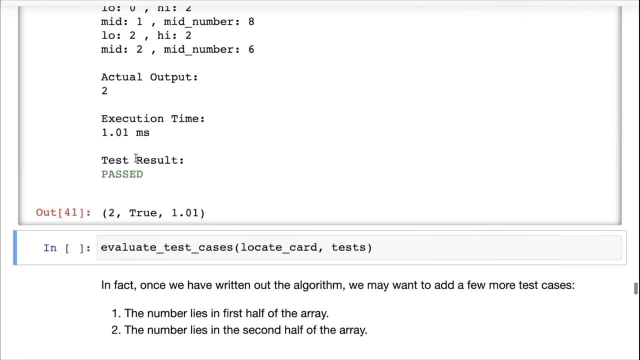 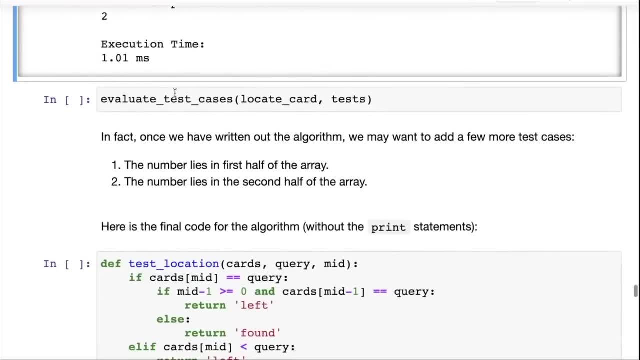 So let's evaluate that test case. And it looks like that test case has passed this time perfectly. You can go through the logs here to verify it. Let's evaluate the test case, all the test cases as well. We should do this every time we change the function. 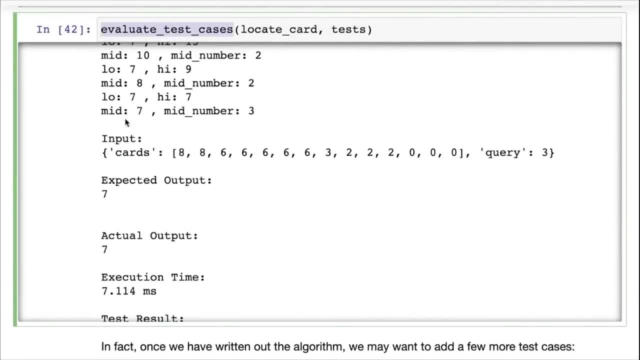 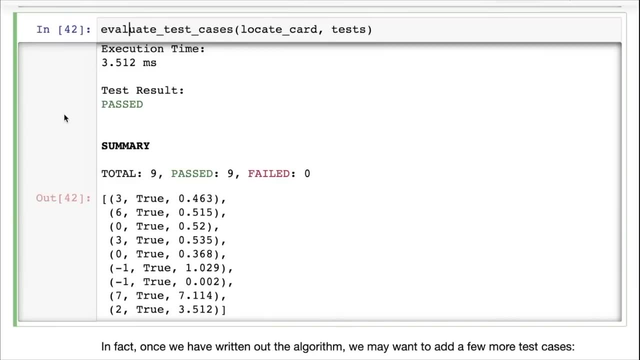 And that is why it's helpful to have a function where you can, every time you make a change, you can just run the test And, on a coding platform like elite code or hacker rank, you will be given some test cases, although those test cases will not be visible to you. 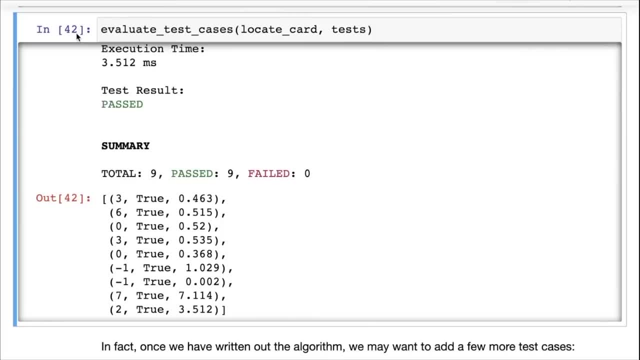 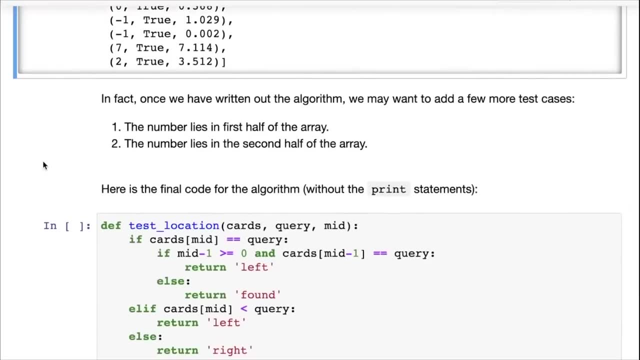 So you can submit your solution, but you may not get an actual result. you may not get to know what the test case was or where your answer was wrong, And that's where you may want to create your own test cases If you're getting a lot of errors. 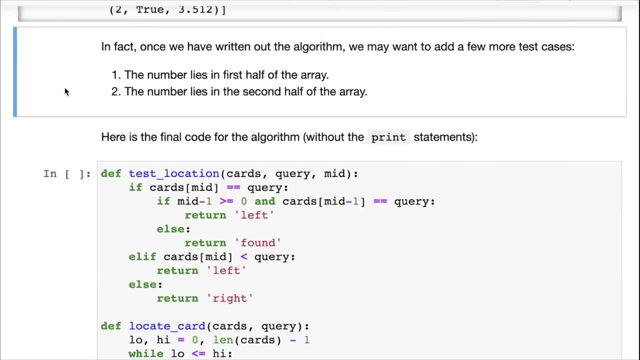 And, in fact, once you've written out The algorithm, you may realize that, okay, maybe you need to add more test cases. What if the number lies in the first half of the area? What are the number lies in the second half of the year. 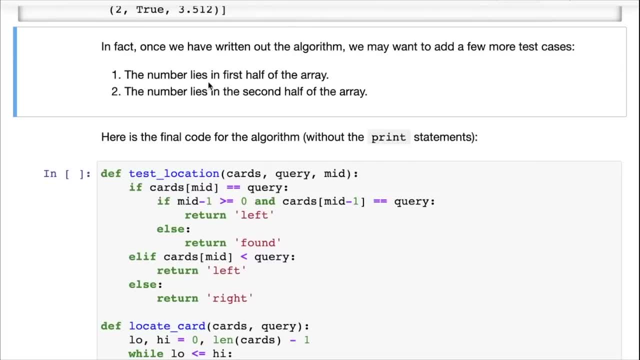 So this was not an important factor when we were not thinking about binary search. but now that we're thinking in this direction of splitting the array into half, we may want to add some test cases where the number lies exactly in the middle, in the left, in the right, 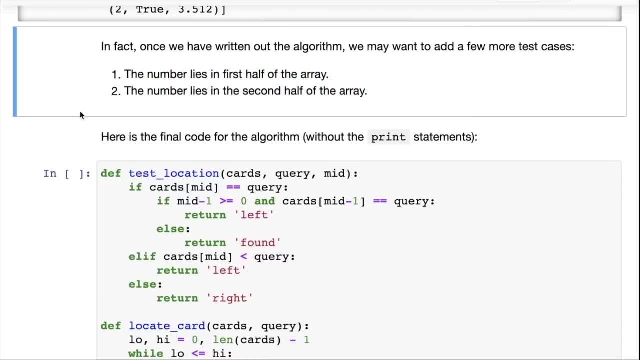 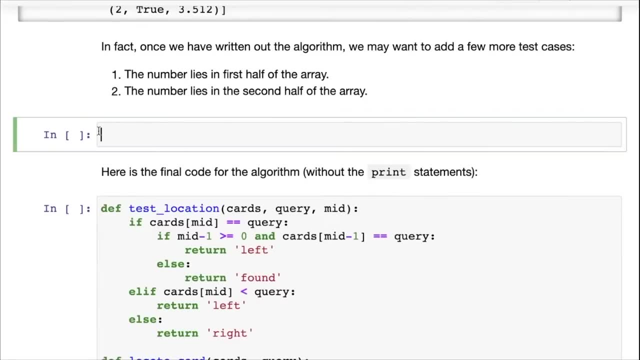 And the simplest way to do that is now: go back to the tests area So you can open a. you can create a new cell here by pressing the character B. So if you click outside and press a character B, you can create a new cell and then you can simply do tests, dot append and then write your test case. 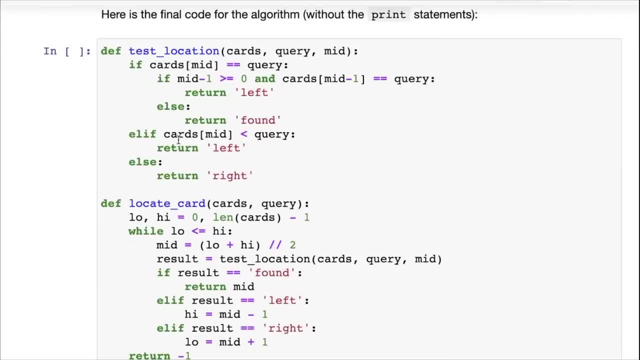 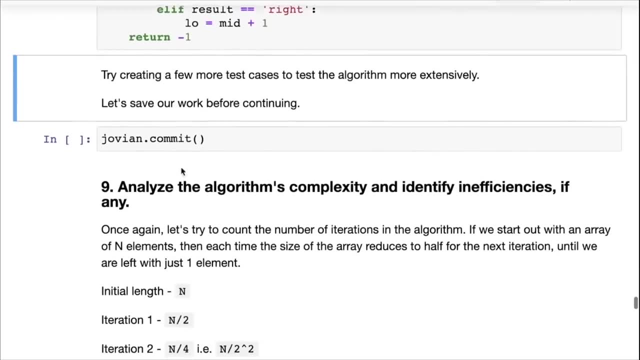 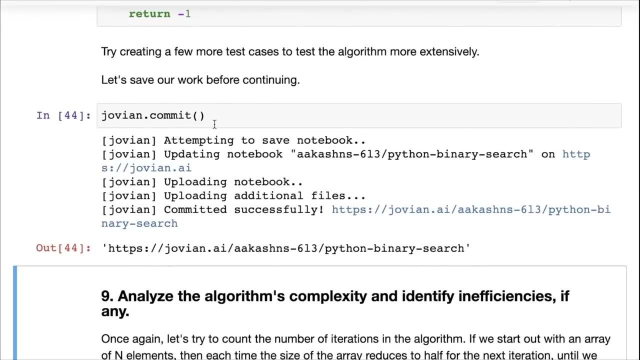 So here is the final code for the algorithm without, without the print statements. So we have test location and then we have locate card and try creating a few more test cases to test your algorithm more extensively. And once again, at every step, we are going to save our work by running job incom. 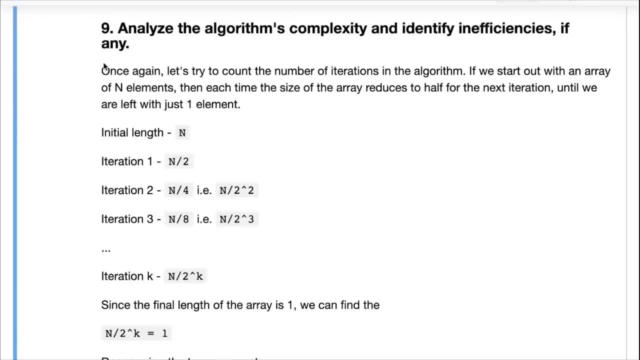 So now we're down to analyze The algorithms, complexity and identifying inefficiencies. if there are any. now you may have just read online. you can actually look it up, say, just search for complexity of binary search and you will read and you will find an answer. but- and you may even just say that in interviews, but it's always nice to just come up with that answer- from first principles- 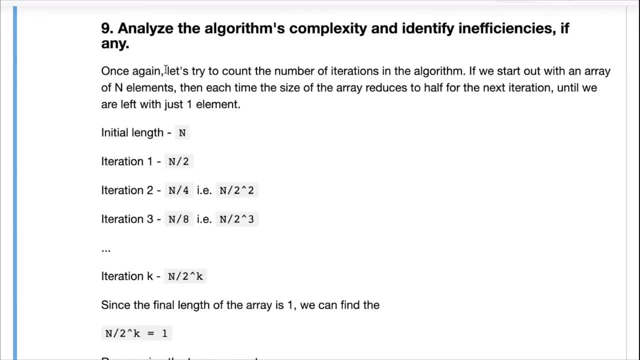 It's always nice, especially in an interview, If you can talk through it, if you can talk through why it is ordered, why it is whatever it is, and we'll see what that is. So now let's once again try to count the number of iterations in the algorithm, because we need to minimize the number of times we access elements from the area. 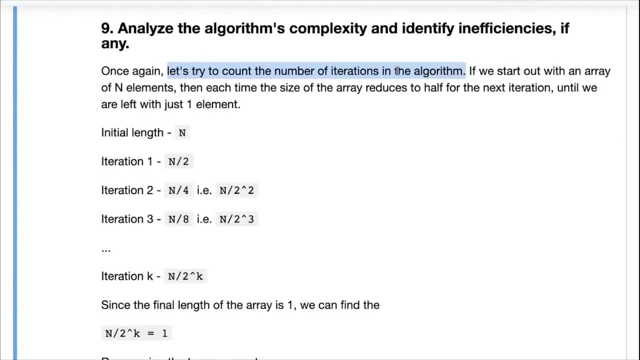 And to do that we know that in each iteration we are accessing the element just once and then we are comparing it. So we're doing a bunch of other operations, but in each iteration we're accessing one element. So we need to count just the number of iterations, the number of times the while loop was executed. 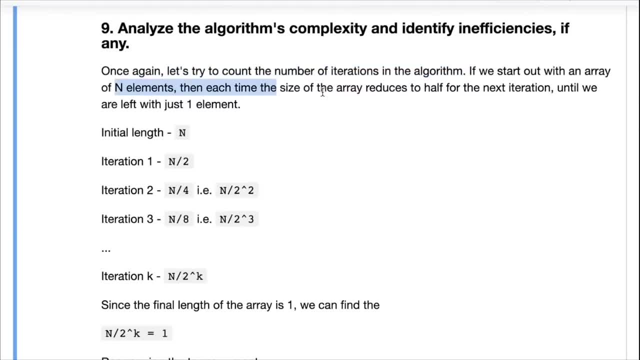 Now, if we start out with an area of N elements, then each time, Each time, the size of the area reduces to half for the next iteration. Now, that's roughly true, because when you come, when you check the middle element and then you decide whether to go left or right, it's actually probably N by two minus one. 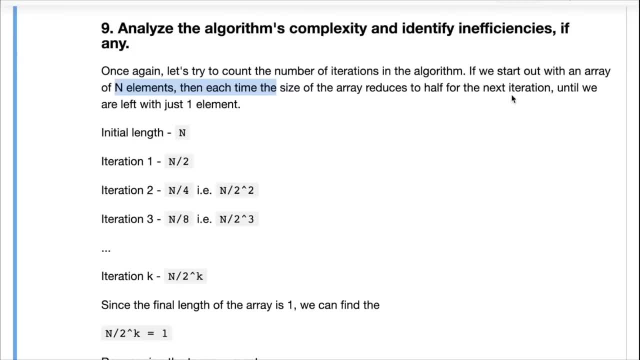 If N is, if N is even or if N is odd, it is the floor of N by two. But again, with algorithms with complexities, we are generally weren't interested in studying the trend, so we can ignore that small part in the calculation. 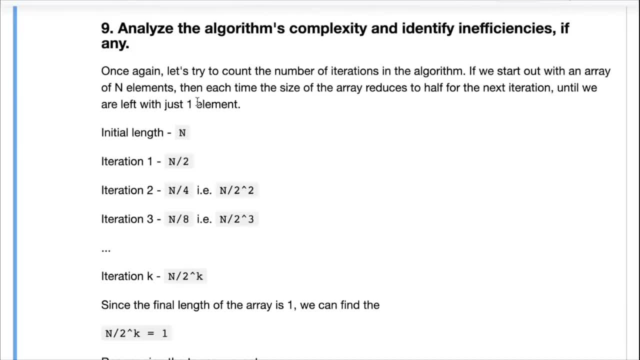 So let's say the important part is that even if it's okay to overestimate a little bit, but try not to underestimate. So after the first iteration we may be left with a search space of size N by two. It may be slightly less than that, but it's okay to overestimate. 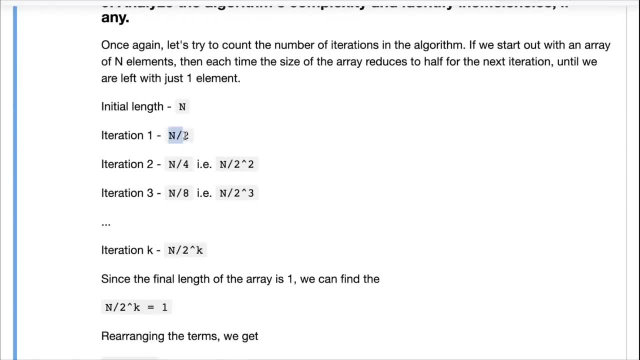 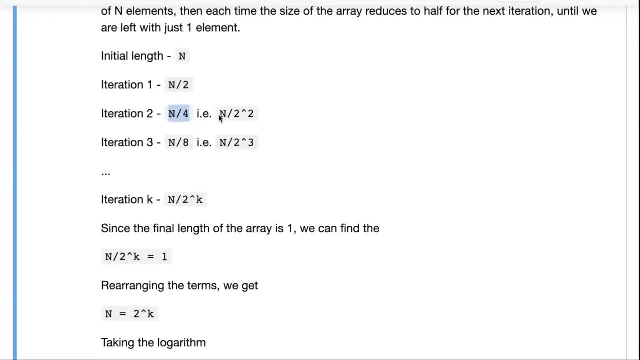 So we have N. so we after N we have after the first iteration we are left with a search space of N by two. Then we split it into half again, So next time we may be left with a search space of N by four, which is N divided by two square. 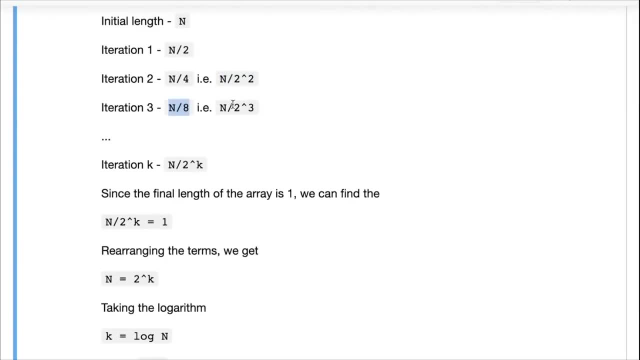 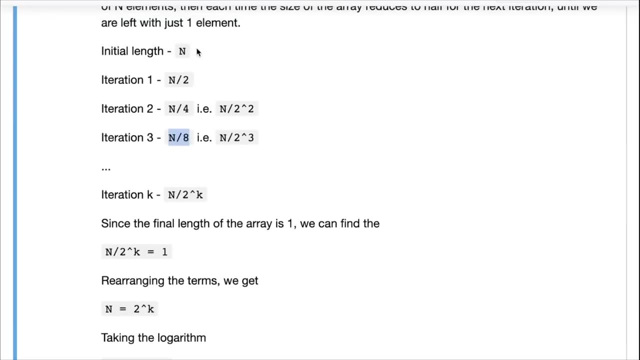 And then then we may be left. We may be left with N by eight, and it's possible that at any of these iterations we may just exit because we may have found the right number. but what we always try to analyze is the worst case: complexity of an algorithm. 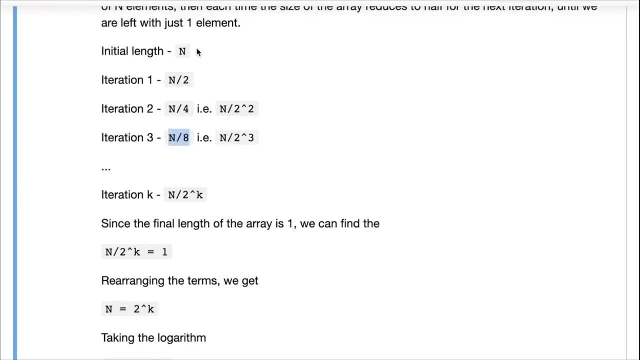 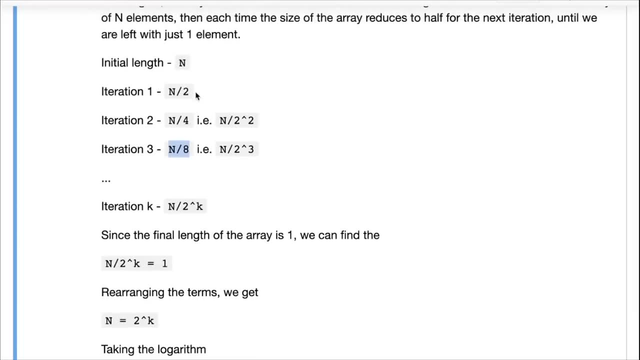 What is the longest possible amount of time or the largest amount of space it can take. So right now we are talking about time, because we are counting iterations and each iteration takes some time. So N by eight after iteration three, that's two to the power three. 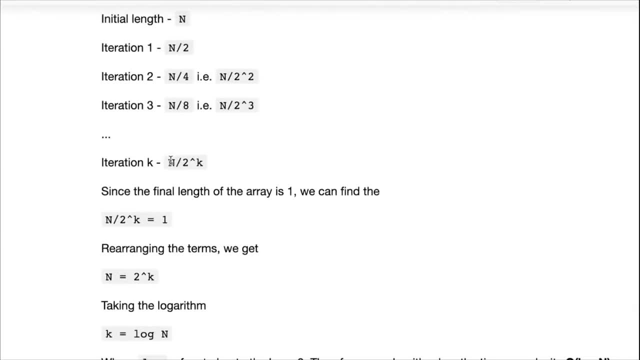 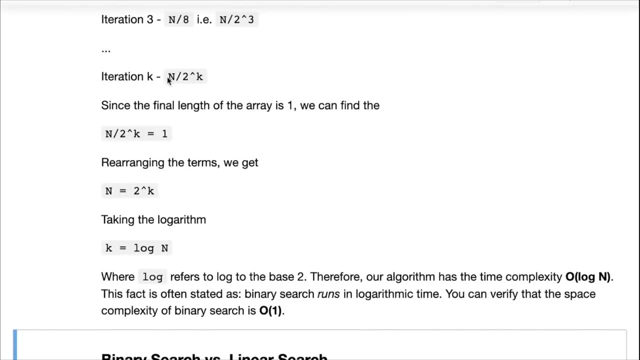 And I think then you can start to see the trend here that after the Kth iteration you will end up with N divided by two to the power K elements. Now, when does the iteration stop? So the final iteration is on an area of length one, and that is when we access that last element and check whether, after all this checking, the last element is equal to the index or not. 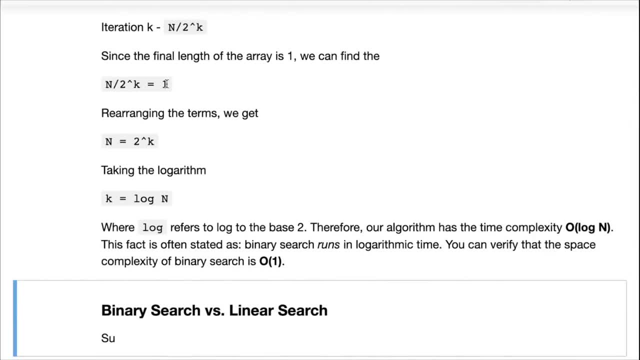 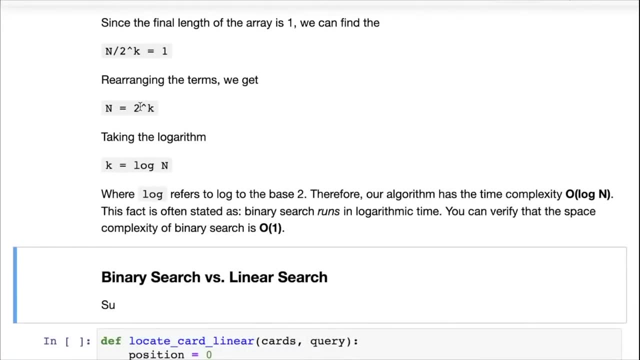 So we can do N divided by two to the par key And if he said that to one, we can rearrange the terms and we get back N equals two to the par key. So After the K iteration, if you want to be left with one element, then that means N divided by two to the K should be equal to one or N should be two to the key. 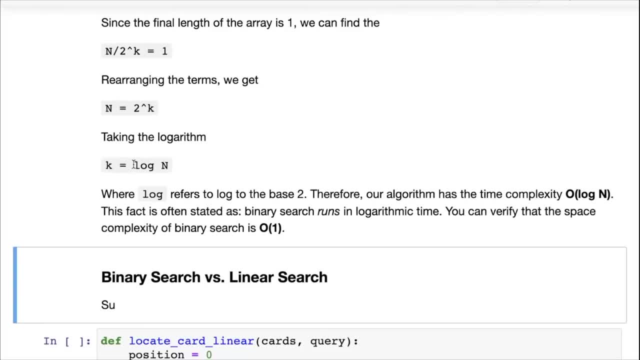 Or in other words K should be equal to log, log N. remember logarithms, and here obviously log refers to log, to the base too. But what I will argue is that you can change the base of the logarithm and that will simply add a constant. 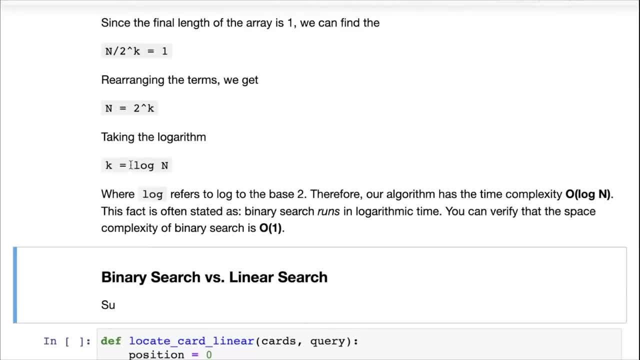 So that will simply, if you're taking the natural log, then that will simply add a constant here. And remember, when we talk about Time complexity we ignore constants. So we can just generally say that our algorithm, binary search, has the time complexity of order of log N. 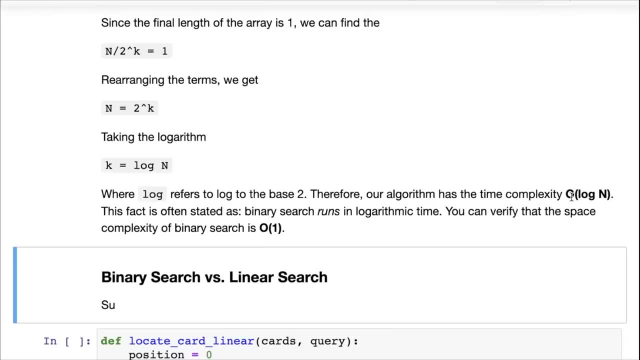 That means, as the input grows, the amount of time taken by binary search is proportional to the logarithm of the number of elements in the list passed to it, or the amount of time taken is logarithm to the size of the initial search space. 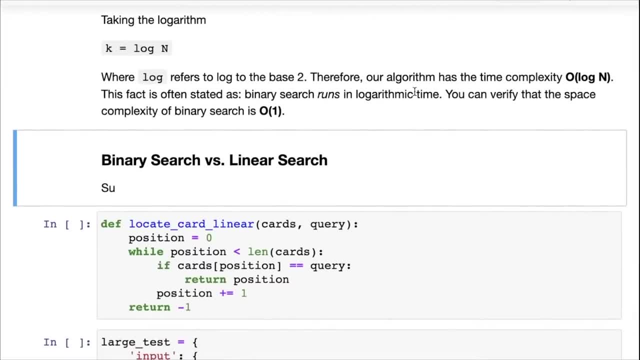 And you can verify this. You can verify That the space complex, or you can. you can check this out by simply writing it out as well. You can take some examples. Let's say you take a card list of size 10 and then walk through it- the worst case- and count how many iterations you have and compare if that is close to log in or not. 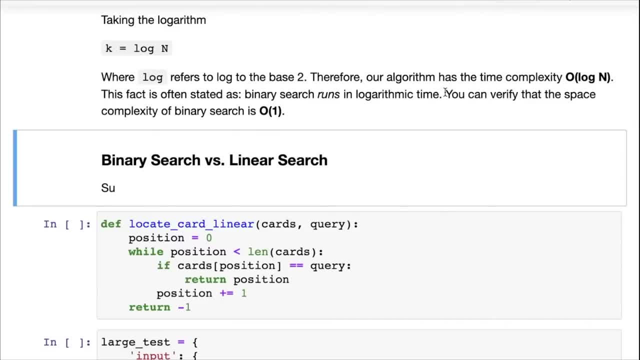 And then, as an exercise, you can verify that the space complexity of binary searches order one. can you, you can try posting in the YouTube comments or in the YouTube live chat how the space complexity of binary searches order one. Well, let that steam. 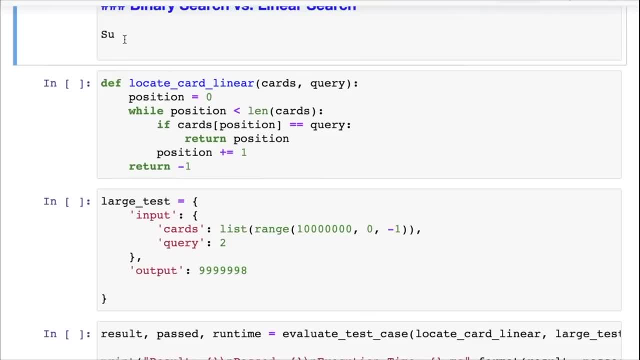 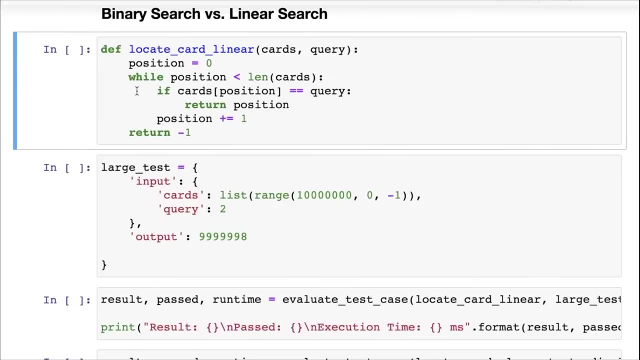 So let's now compare linear search with binary search. How are the two different? And what we'll do is we will create a large test case, because you start to see the benefits of the difference between the order and algorithm and the order log in algorithm only when you have larger test cases, because small test cases, everything runs instantly. 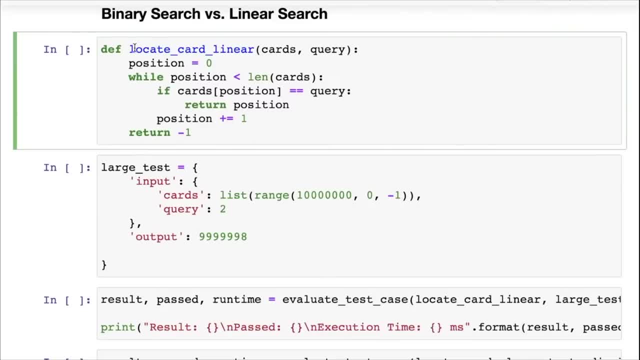 So it's not really that much of a hassle. secure, We have a locate Card linear- and this is the linear version of the algorithm, where we simply go through each of the cards one by one, and then we have a really large test case here. 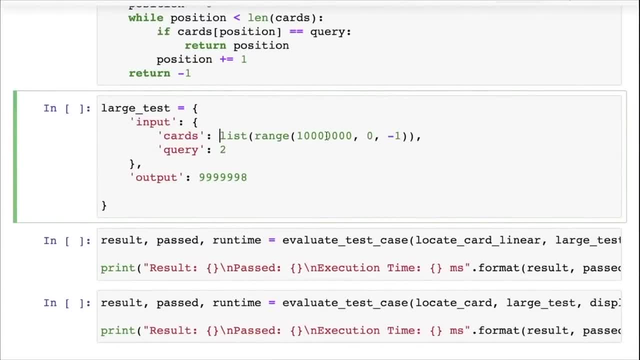 So we have the input and then we have the cards, which goes in the range. Okay, Let's see. So that's one, two, three, So that's thousand, another three, that's million. So we have 10 million elements here. 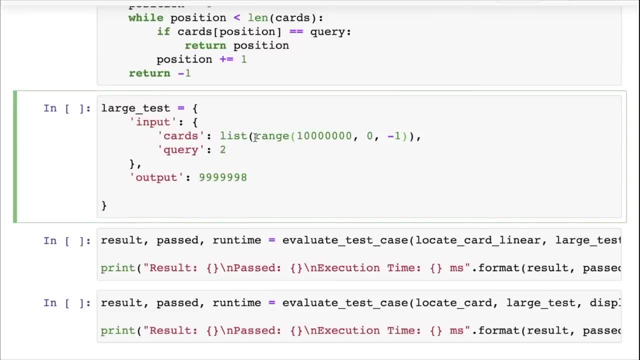 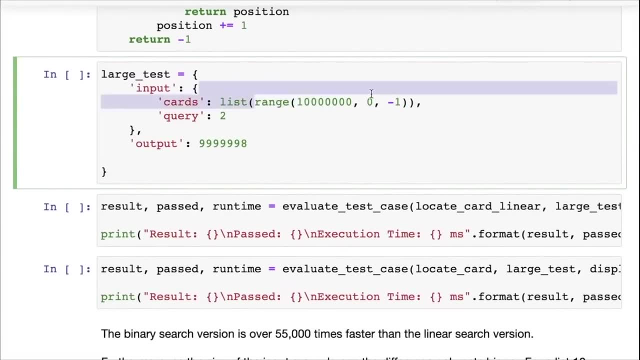 So we have 10 million elements And We are looking at, so we are actually creating a range here, So we are using a function in Python, So we're creating a list of numbers going down from 10 million all the way to one. 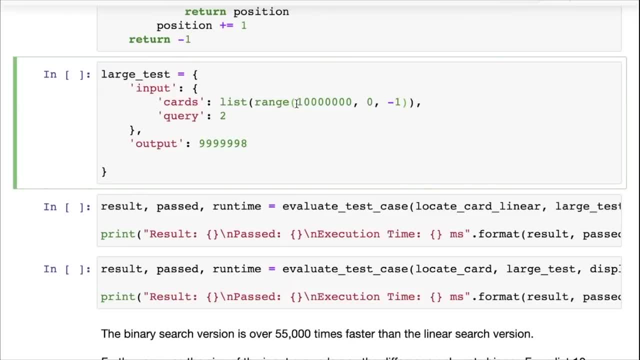 So a decreasing list, going from 10 million to one, and this is how you create it and you can check it out. And in this list we are looking for the number two, which occurs at the very end. So we are sort of creating this is as we will see. if you want to really analyze it, this is going to be a worst case scenario, both for linear search and for binary search. 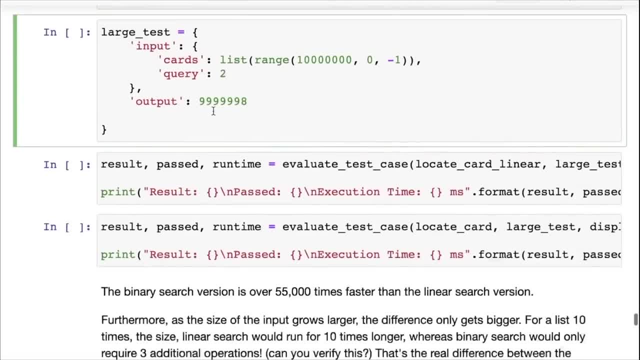 Approximately worst case. So the query is two And then the output is: this is the output that we expect, obviously, because zero to nine, nine, nine, nine, nine, nine, nine is are the array indices, And the last element is one. 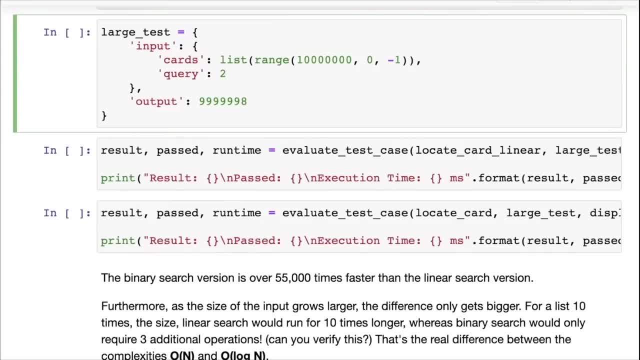 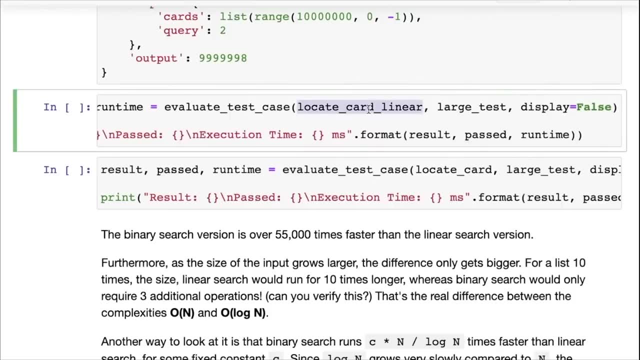 So the element just before is two. So this is the expected output. Great. So now we have this large test, Let us call evaluate test case and let us pass a check. The linear search pass in the last test. And Because 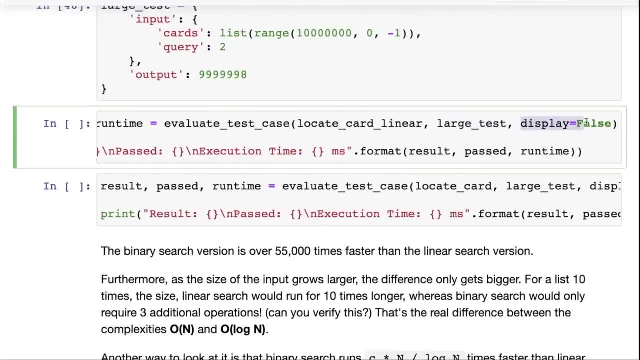 This is a huge list. We may want to turn off the display of the output. We may not want to actually see the input being displayed, So we can simply turn off the display by passing. display equals false and we can just get back the result from the evaluate test case function. 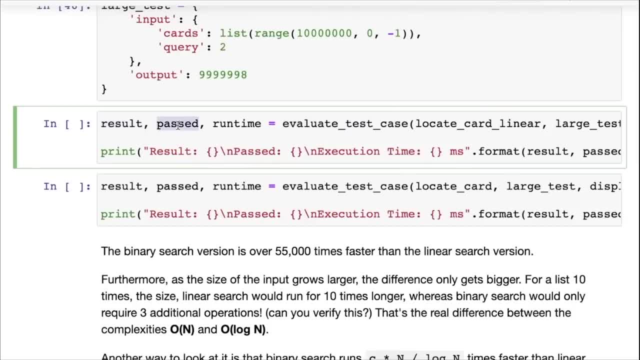 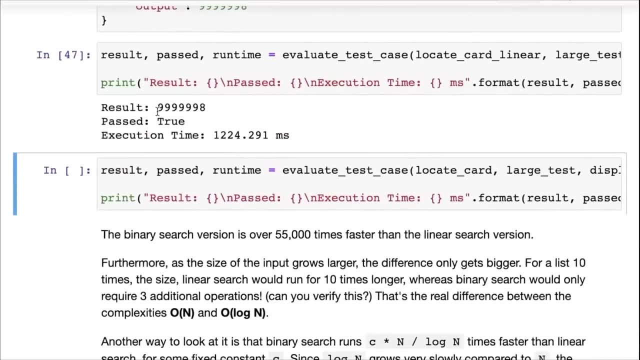 So the result will give the output, the actual output of the function, whether the test passed and the running time of the algorithm. So it takes a second. So it looks like the test did pass, our algorithm is correct, So That's great. 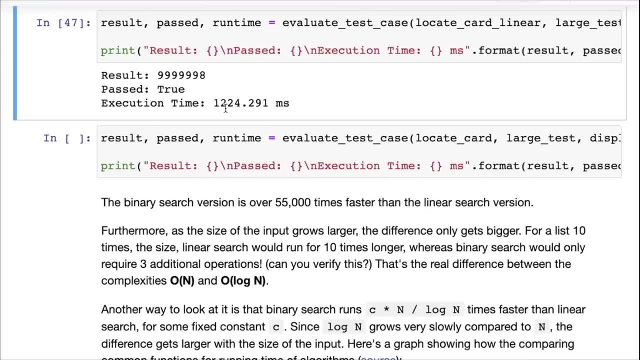 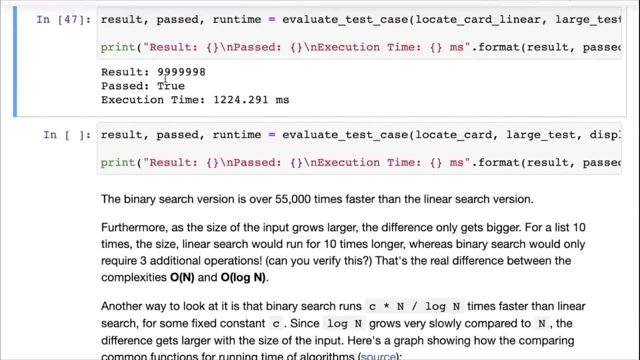 And it took one to two, 4.2, nine, one milliseconds or about 1.2 seconds to answer it. And you can probably tell why: because it, because this is the result. So it probably took nine, nine, nine, nine, nine, nine, eight iterations. 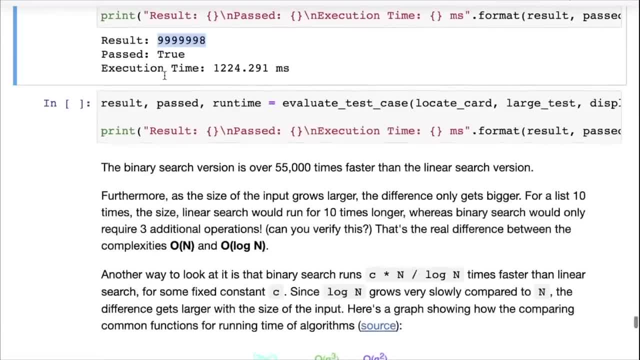 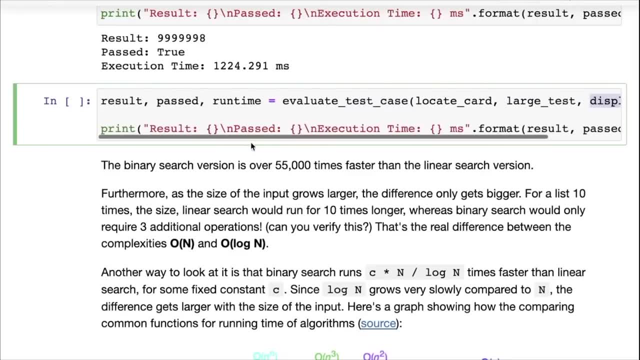 So it had to go through all the elements to get to the very end. On the other hand, when we talk about binary search- so now we are passing in the binary search version once again, turning display to false, And we are displaying the output- 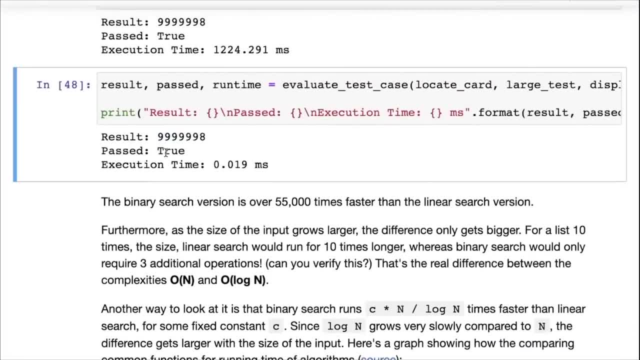 Okay, So this time the result is the same- the tested pass- but the execution time is 0.019 milliseconds. So that's 55,000 times faster than the linear search version, And in fact you can tell how many elements we actually had to access. 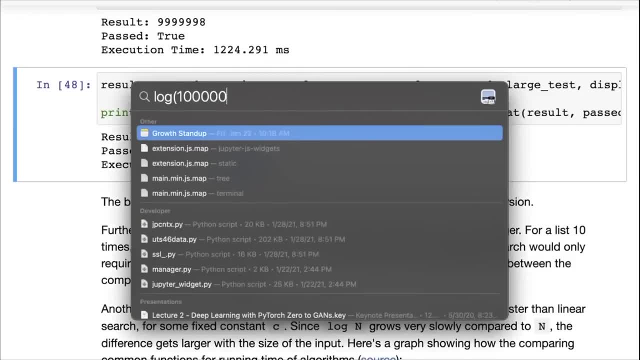 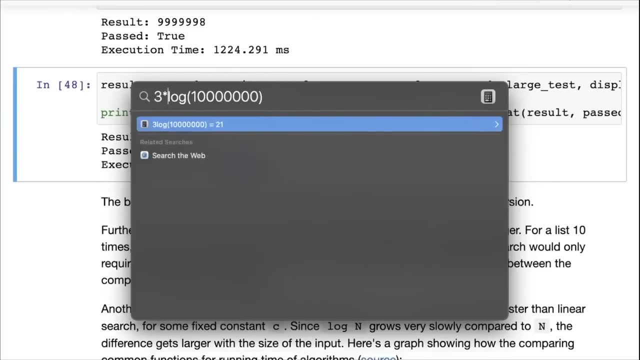 So if we just check log of, so log of this number is about seven and maybe know if we, if you're checking log two, we can Maybe, Maybe check something like this. So not more than 20 elements had to be accessed. 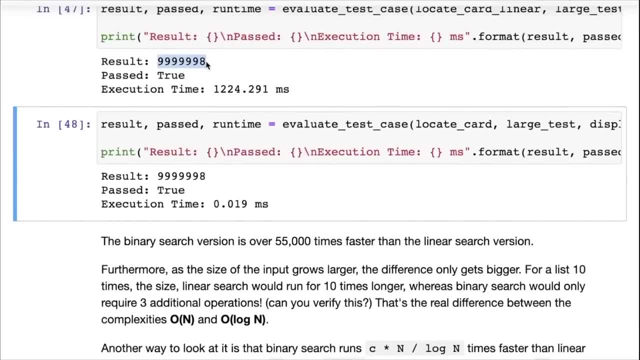 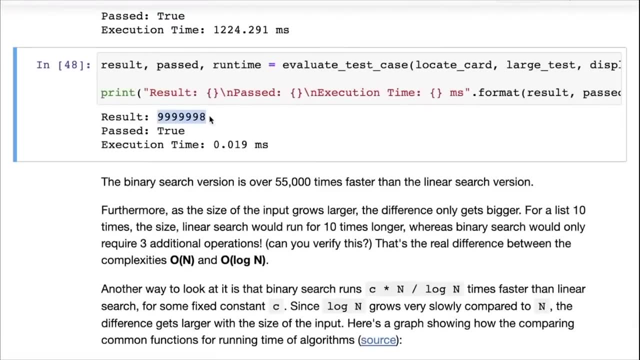 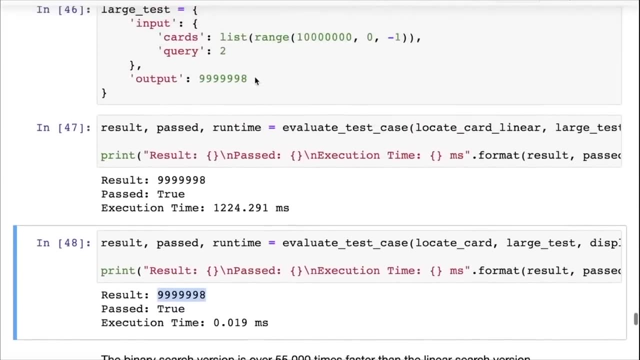 So where we linear search needed to access about 10 million elements, my research was able to get to the answer with just about 20 checks, So that's a lot of time saved and you can increase the size of the array by a factor of 10, and increase this by a factor of 10 as well. 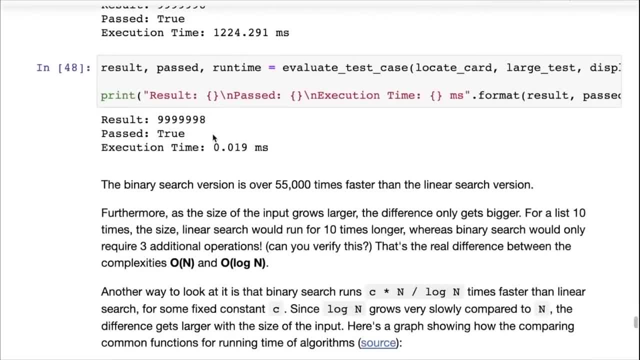 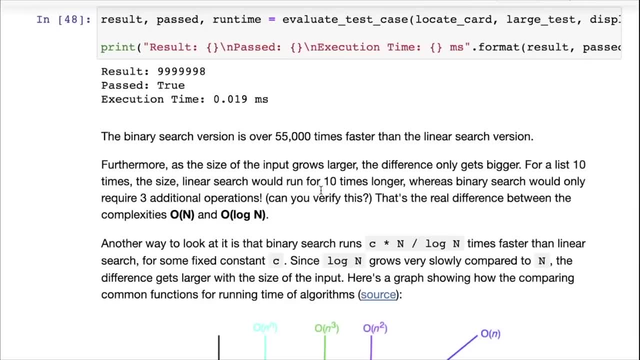 And then you will see far bigger difference where, For a 10. 10 times larger array, linear search would run for 10 times longer, Whereas binary search would only require three additional operations. So the linear search would go from 10 million operations to a hundred million operations. 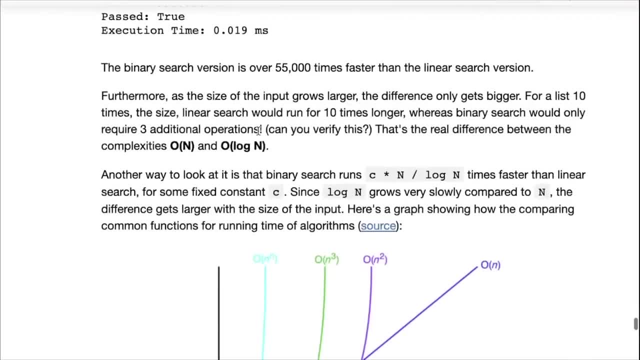 Binary search would go from 20 operations to 23,, and that is the real difference between the complexities order in an order login And as the size of, as the size of the areas grows bigger. another way to look at it is that if you just divide the complexities, binary search runs. 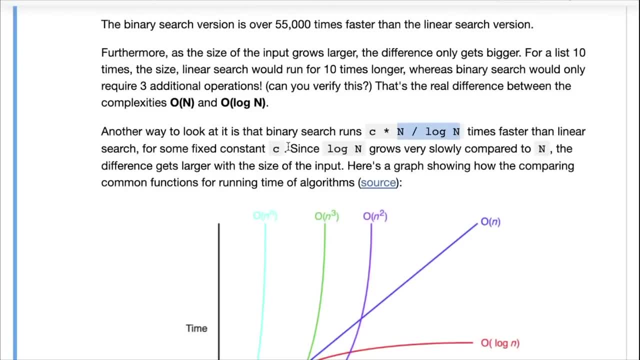 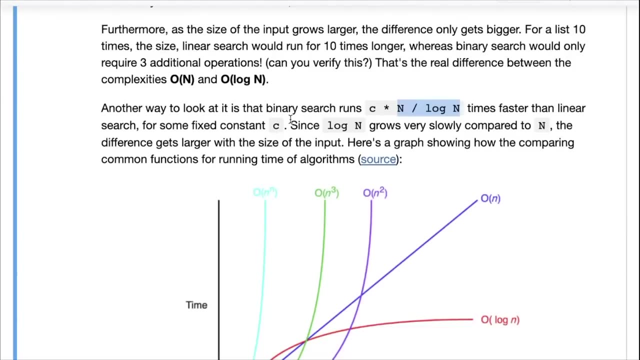 And by log in times faster than linear search for some fixed constant. because there's always some constants involved and as the size of the input grows larger, the difference only gets bigger- the difference in performance. And that is what algorithm analysis of algorithms and optimization of algorithms is all about. 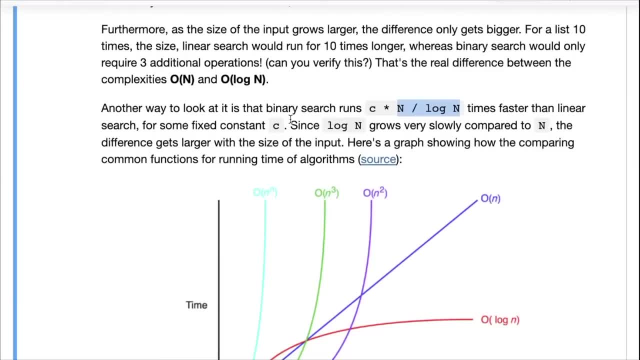 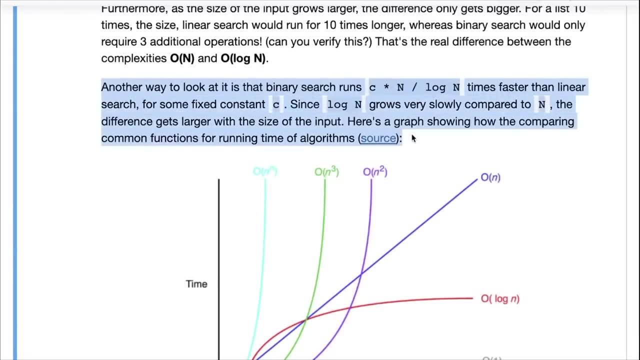 It's about overcoming the limitations of computers by devising clever techniques to solve problems, And it's something that you can actually apply in real life as well. in a lot of cases, there are a lot of things that you may see a brute force solution to, but if you just apply your mind, you may find a more optimal solution, a more easy way or a more lazy way to do it with less work. 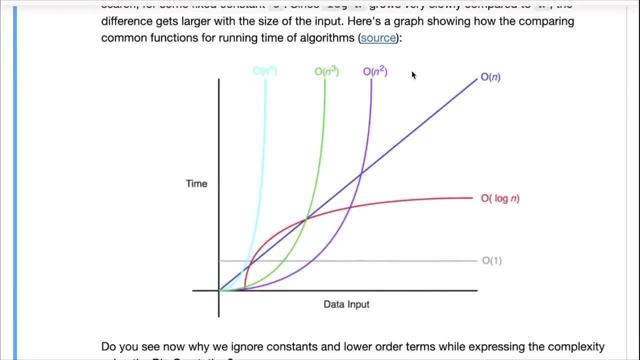 So think about that, And here is a graph showing how the comp, how you can compare common functions, how the, how the running times of common Functions vary. So we will look at all kinds of functions. We will look at constant time functions, order one. for example, accessing an element from an array is order one. 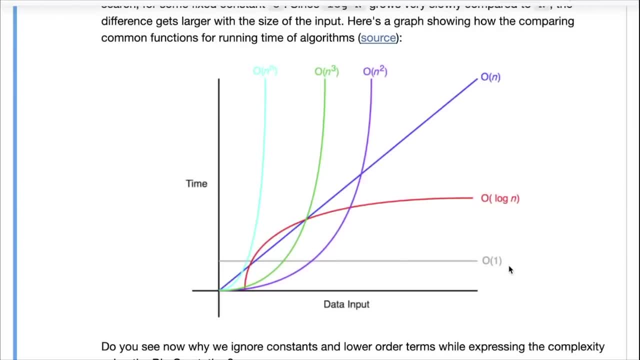 So, even if you have an element of 10 million, a list of 10 million elements, you can access the last element in constant time. On the other hand, we've looked at binary search, which has, which is order, login, And we've also looked at linear search, which is ordering. 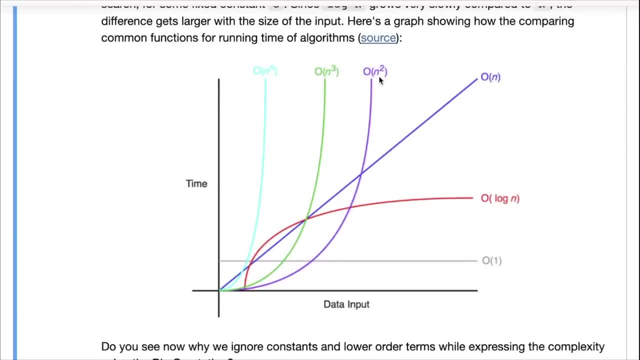 Now in the future we will look at other techniques which have complexities of N, square and cube, N to the power And Far, far higher, and somewhere in between there is a very nice special type of complexity called N login, which is rather nice. 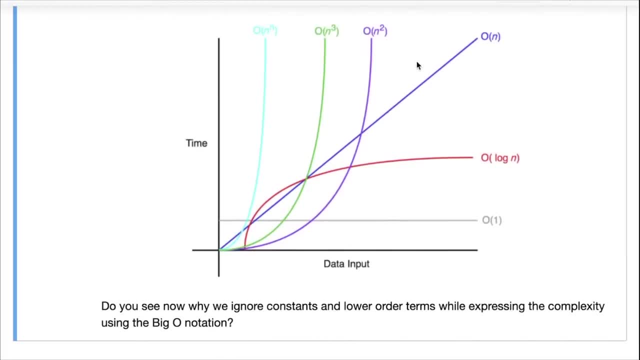 So we'll talk about that as well. And login. in fact, a lot of questions in coding assessments and coding interviews tend to be taking algorithms, which would be, which would have N square complexity in in a brute force approach, and optimizing them either to order N or to order N login. 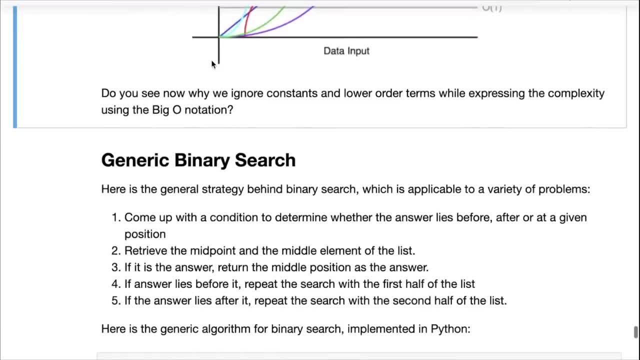 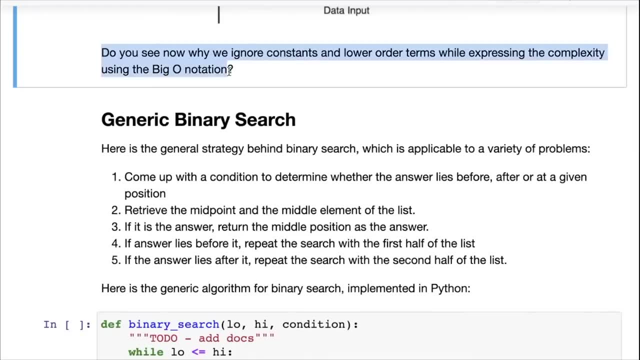 So we'll, we'll discuss all of this. So don't worry if this doesn't make sense just yet. but I hope you see now why we ignore constants and lower order terms while expressing the complexity of the big O notation. So we've covered binary search, but we've seen it in the context of a problem. 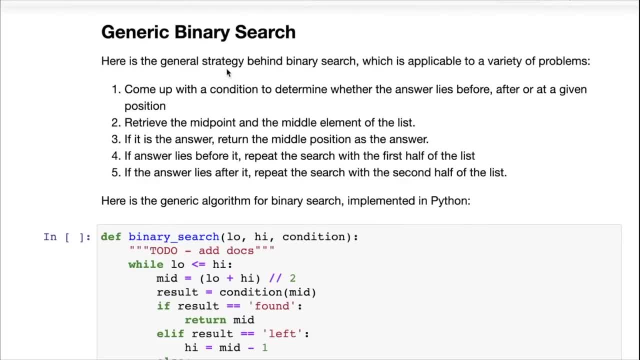 And now we can step away one more step and abstract it out further and identify the general strategy behind binary search. And this general strategy is actually applicable to a wide variety of problems. And this is what you want to Keep doing as a programmer: you need to abstract away, peel away the layers of specific problems, specific details, and find the general technique, find. 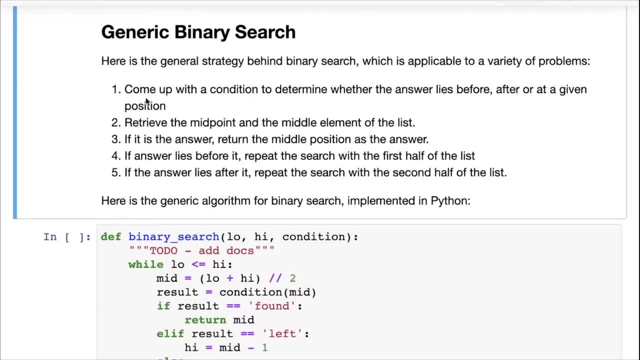 the general strategy and then encode that using your functions and programs. So here's the general strategy. come up with a condition to determine whether the answer lies before, after or at a given position. So we are assuming here that we have some kind of a range and we have to identify a position within a range. 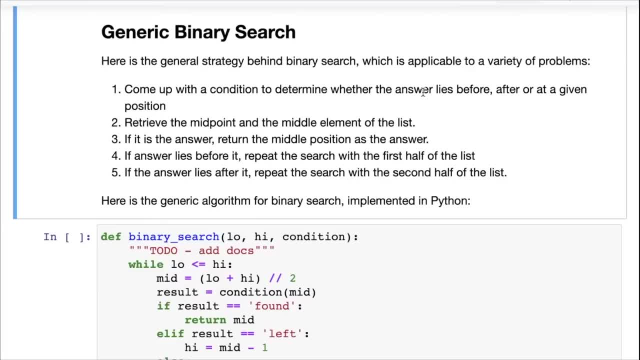 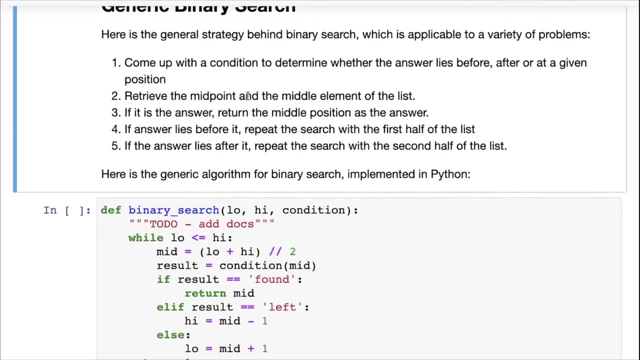 Or maybe an element within that range. but we can access elements using the position. So come up with a condition, that that first tells you whether, given a position, the answer lies at or before or after that position. Once you have that condition, first retrieve the midpoint and the middle element of the list. 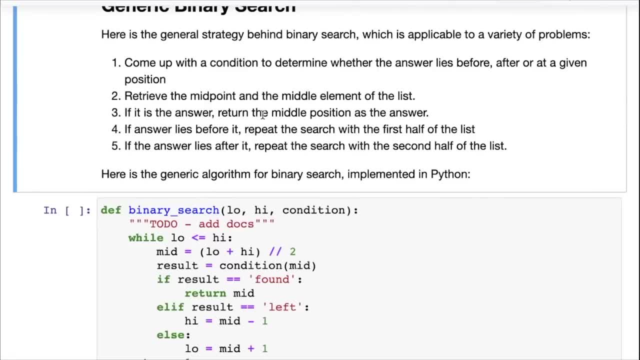 Now, if the middle element of the midpoint is the answer, then return the middle position. That is the answer, you're done. If the answer lies before it, repeat the search. So repeat The process with the first half of the list or the first half of the search space. 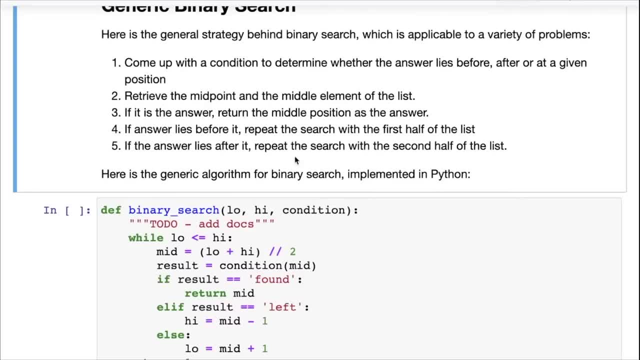 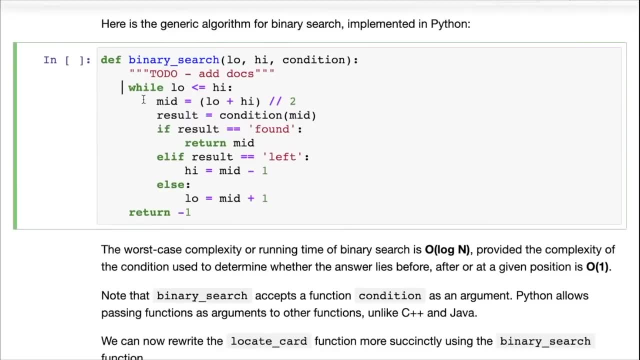 And if the answer lies after it, repeat the search with the second half of the search space. So here is the generic algorithm for binary search implemented in Python, And you can see a classic detailed documentation here. So while so here you have, the binary search is going to take a search space low and 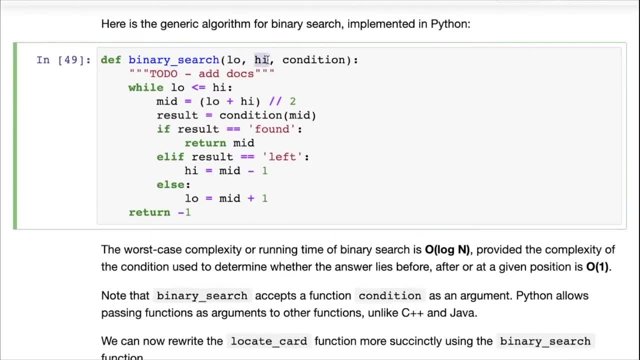 high. So low is going to be zero and high is going to be. well, we will pass in maybe the final. we will pass in maybe the final position, the final index of the area, but writing it this way rather than passing: passing an array also allows you to use binary search for problems that are not based on array. 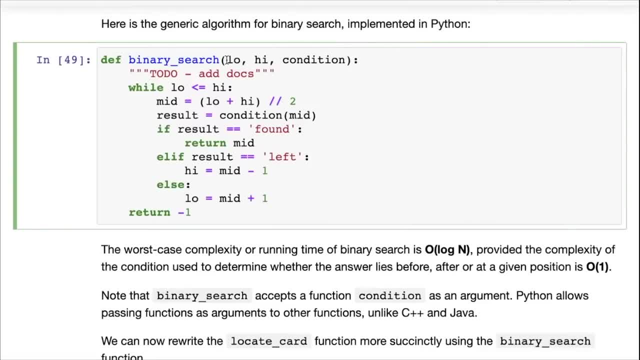 Sometimes these could just be numbers. For example, if I ask you to find a number between 1 million and 10 million, that is a perfect square- Then you can use binary search to do that. Then it takes a condition. So what it does is it starts a loop. 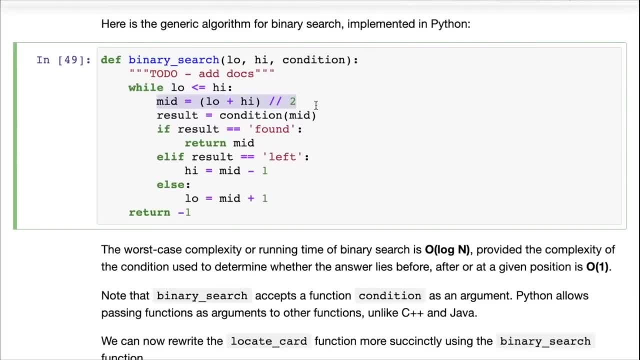 So while low less than equals high, we get the midpoint. So low plus high divided by two, that gives us a midpoint. Then remember earlier we had this condition: test location. So our condition simply is supposed to take the middle position and identify If the middle position is the answer or we need to go left or right. 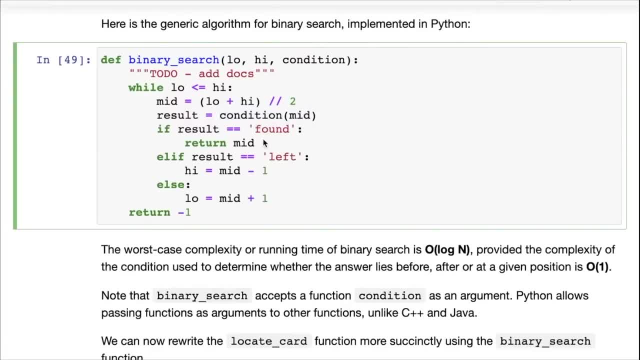 So the condition should return either found, left or right. So if the condition returns for found, we return the midpoint as the answer. If the condition returns left, we return the high, we move to the left side. So, which is we take the end of the search space and set it to before the midpoint. 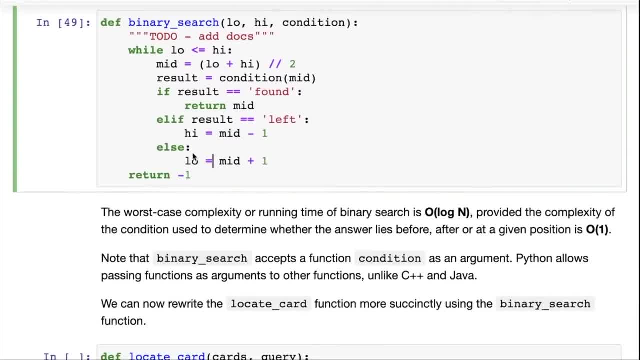 So we set high equal to mid minus one, And if the condition returns right, which is the else case here, we set low to mid plus one. So we Take the start point of the search space and move it off to the element. 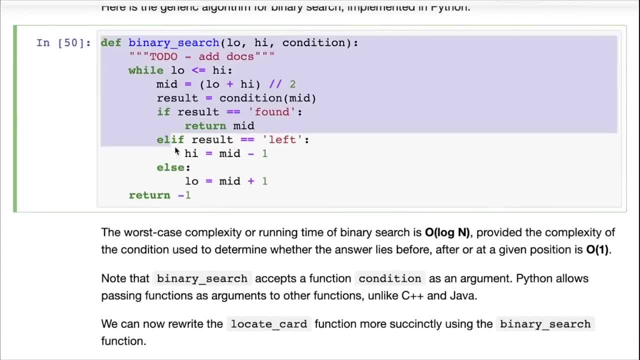 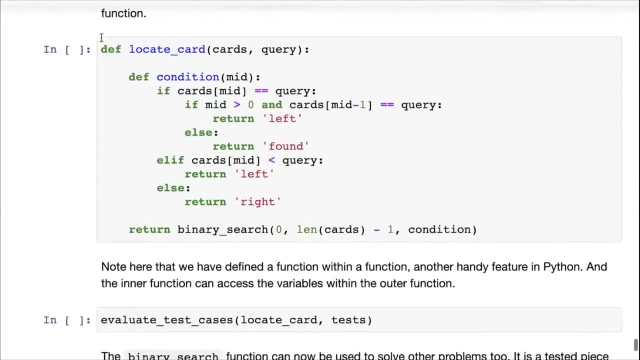 Then we return minus one. So that's a binary, generic, binary searching algorithm, And if you start using this, what will happen is: now, this is a tested piece of code And in fact, we can see it here. No, now we can rewrite locate card and locate card can be: uh, we're passing in cards and we're passing in the query and we need to write a condition. 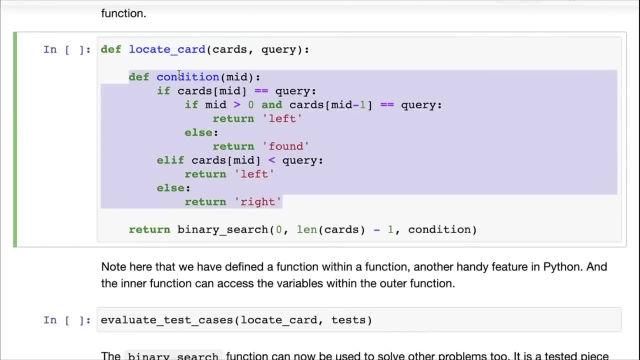 And here we're using a very interesting feature of Python. We are writing a function inside a function, So this is called function closure, and it's a very handy feature. So now we can simply write condition inside locate card, And what that does is: 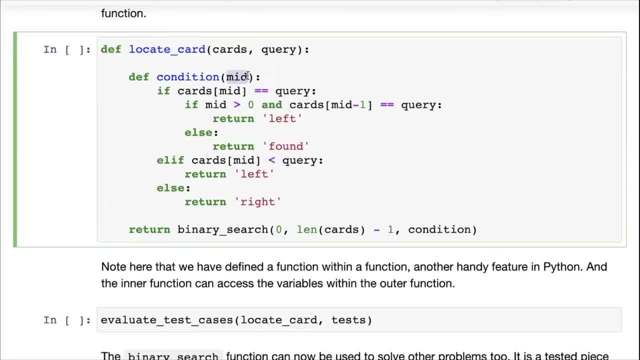 Conduct binary search is going to pass the middle value, the middle position. but condition can also access cards and query. So which is because it lies inside locate. So what we do inside condition is okay, We check them, We get the middle element, cards made. 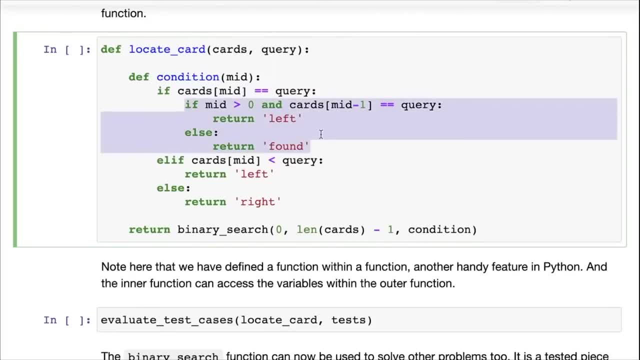 If cards made is equal to query, then here we have that check. We check whether it is the first occurrence of query or can query occur before it. If query occurs before it, we return, left as we return found, And then these are the original conditions that we already had. 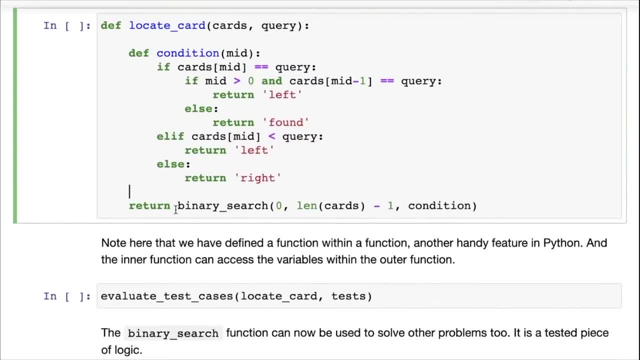 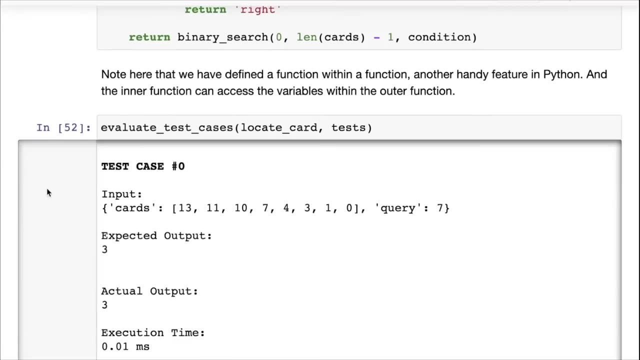 So you can verify this by going back and checking. but the important part here is now: the while loop has gone away. Now we can simply call binary search with zero land cards minus one, So the start index, the end index and the condition, and we can evaluate the test cases and you can see that the well test cases are correct. 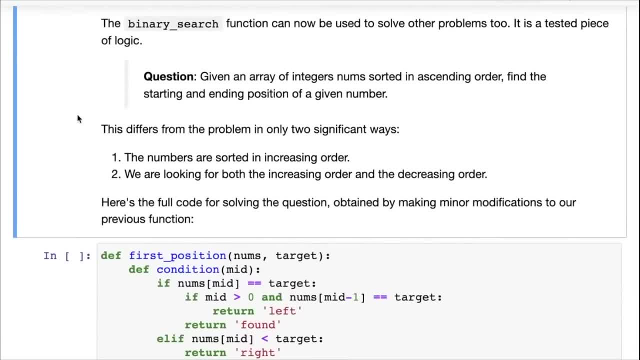 And now you can use this Binary search function, because we have not tested it with one problem. You can use this exact same function to solve other problems too. In some sense it is a tested piece of logic. So here's what we'll do. 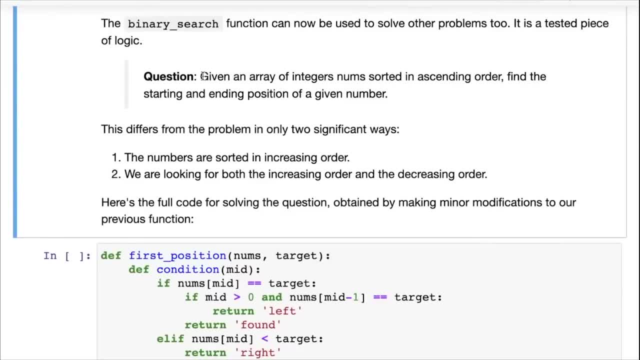 We'll take a quick question and we will implement it. Now we've spent what one and a half hour talking about a particular problem, but let's spend maybe two minutes talking about a new problem and solving it. So here's a slightly related question. given an area of integers sorted in increasing order, find the start. 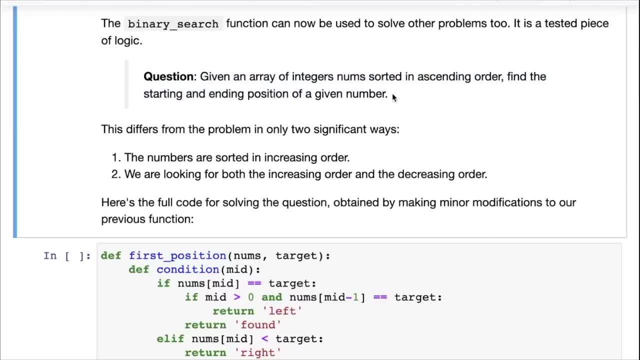 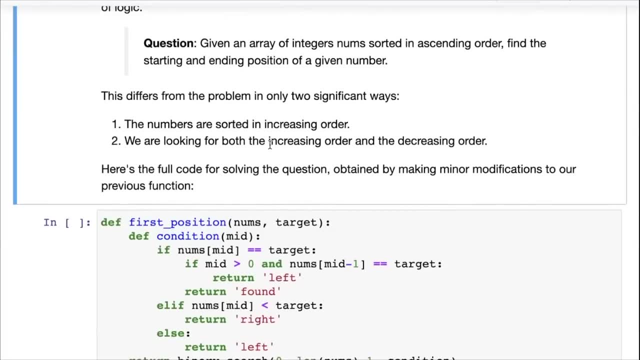 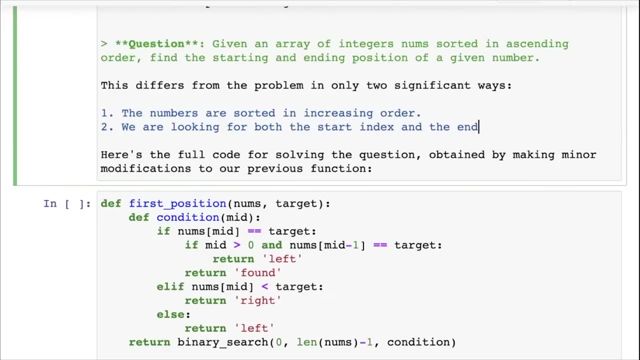 And ending position of a given number. So once again you have a sorted area. this time they're increasing. The only difference is now, apart from the fact that they are sorted in increasing order, the other difference is that we are looking for both the start index and the end index. 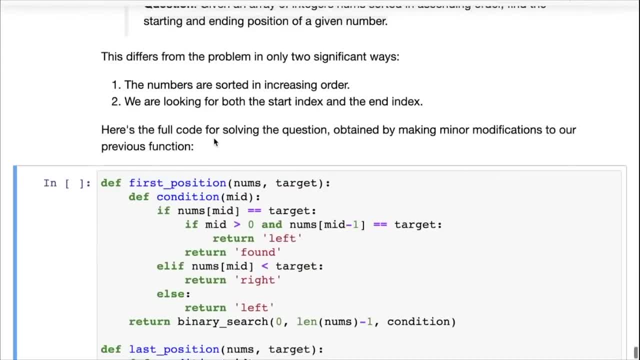 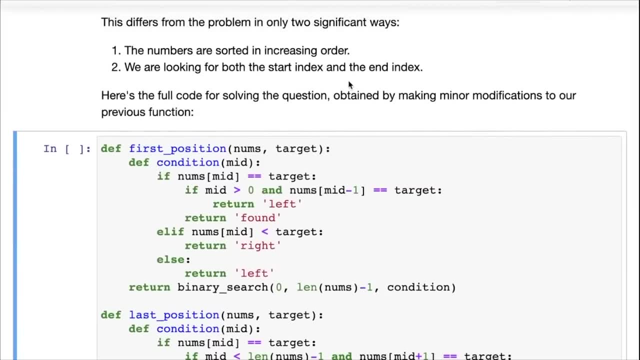 So we're looking for both the start index and the end index of a particular number, because the number can repeat, like we saw one example, and there's a very simple Way to solve this. A simple strategy is: do binary search once to find the first position. 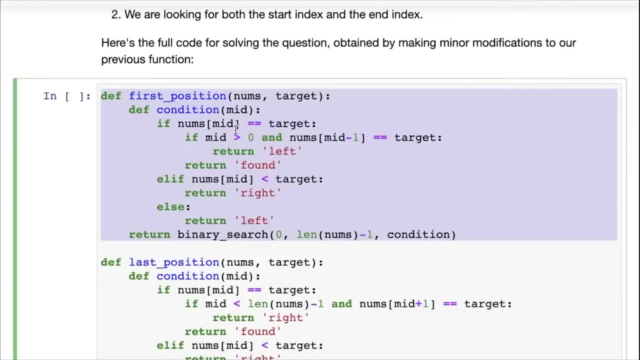 And that's what this function does. I let you read through it. The only changes here are this variable- This has changed this order, because now the now the elements are in increasing order, and then the second change and there's no other change here. 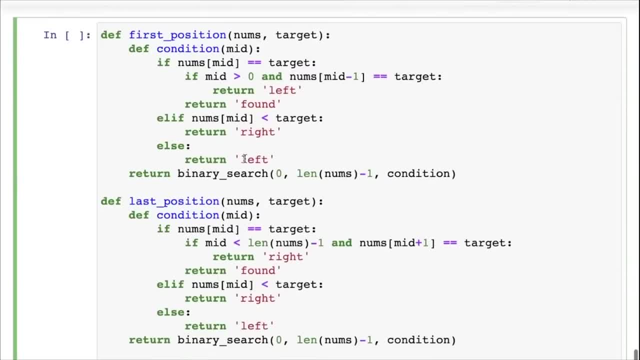 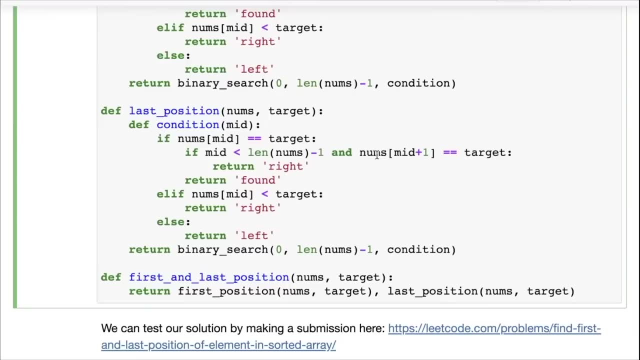 So that there's just one change here And then there is another function called last position. here, instead of checking The left, we are checking the right. So instead of checking mid minus one, we are checking mid plus one, And if mid plus one equals a target, we go to the right. 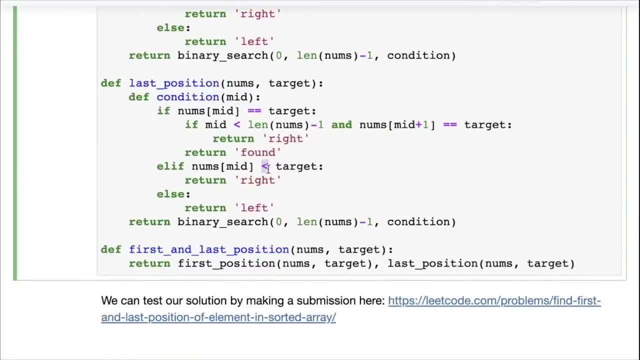 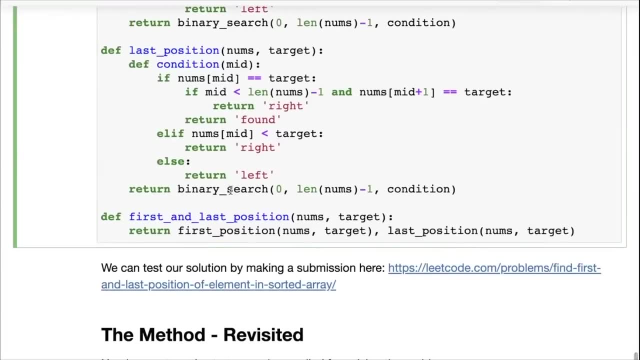 And of course we have the same change here in this code, because instead of decreasing we have increasing order right. So now we write two position, Now we write two functions: first position, last position, and then first and last position is simply getting the first position once. 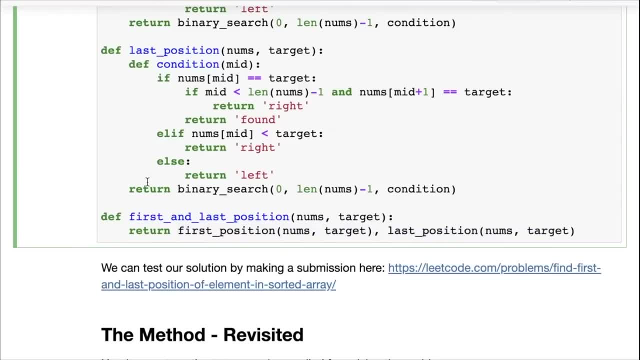 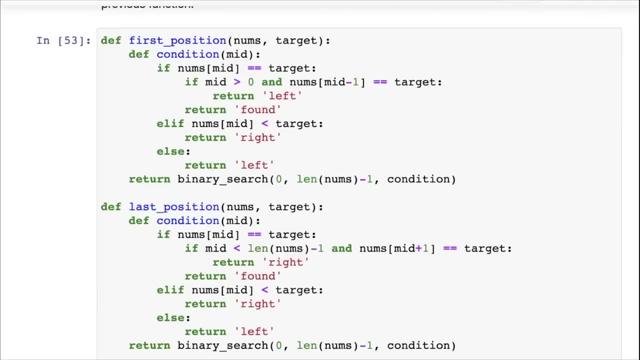 So that's one binary search and getting the last position once. that's two binary searches and that's not bad. No, the complexity is still order login. Two times login or two times some constant times login, when you express it in the bigger notation, is still login. 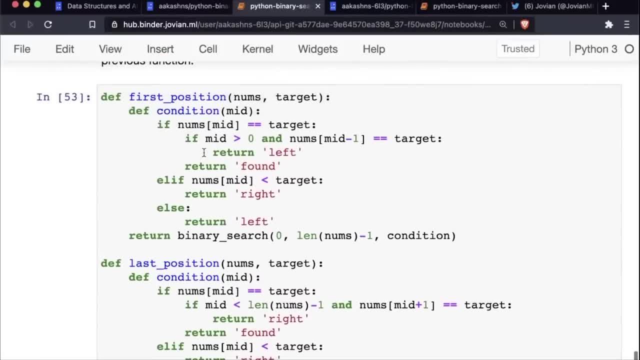 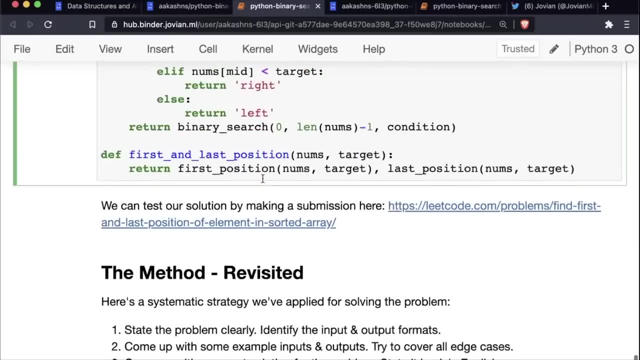 So that's okay And that was quick We are. we were able to reuse most of the code that we have written and that's a benefit- benefit of making generic functions like binary search And in fact, we can test a solution by making a submission here. 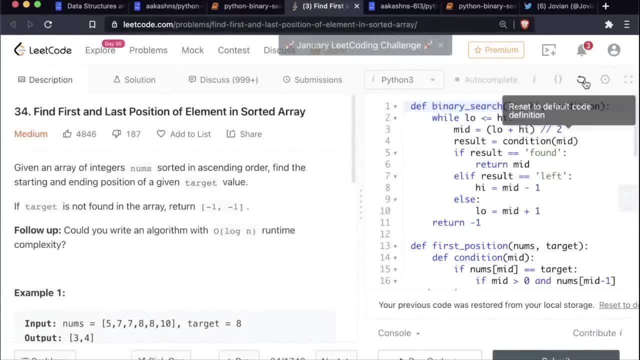 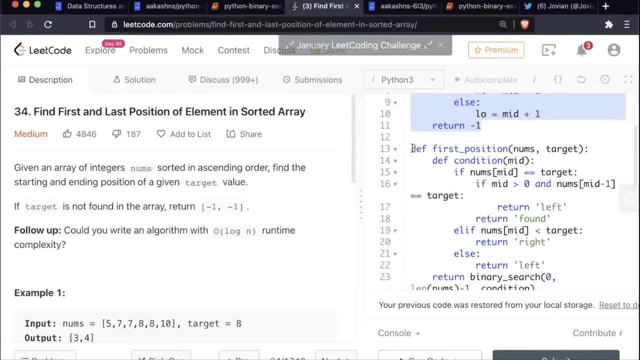 So let's go to lead codecom. Let us hear. what I've done is. I have already copied over the binary search: The first position function, the first position function and the last position function. So, by the way, lead code is a great platform for practicing. 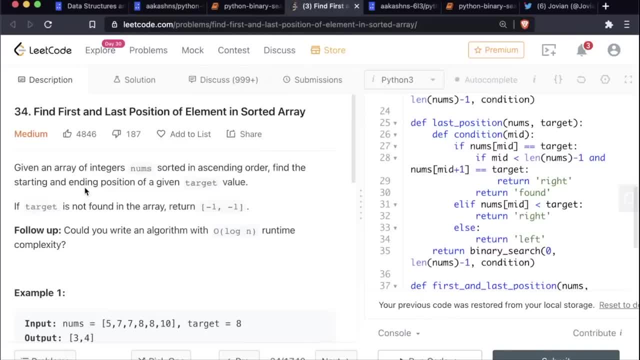 So you can go to lead codecom, sign up with any account and you will find a lot of problems, especially on the in the problems tab, And here you can see that this is exactly the problem that we have been solving just now. 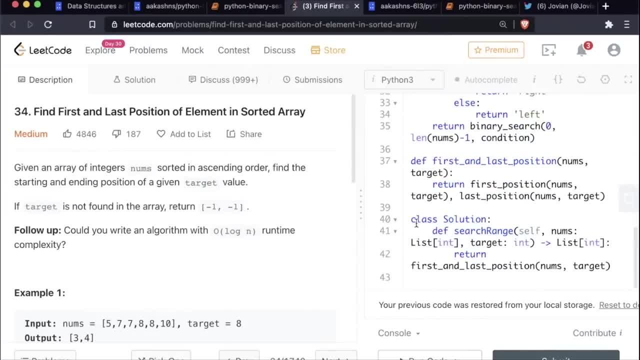 So we've just posted the code here by research: first position, last position, first and last position And lead code. It requires you to write this class called solution Give you beforehand and inside the solution you need to define a function called search range where we are simply calling our first and last position here. 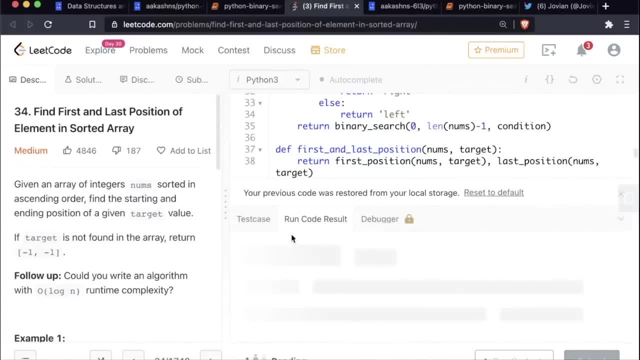 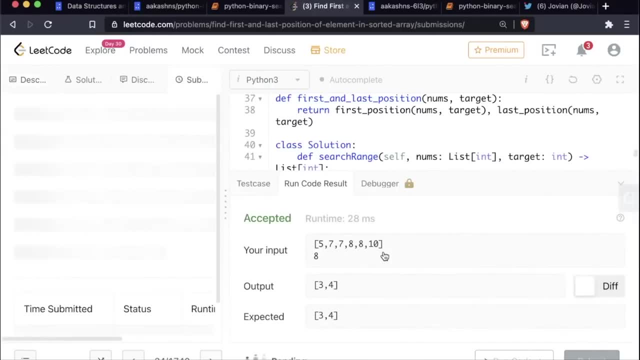 I'll let you see, And we simply we can test this code with a test case. So you can pass a test case here and test it out, Great. Or we can simply submit it And here you can see that the problem was submitted successfully and it tells you things like how much runtime it used. 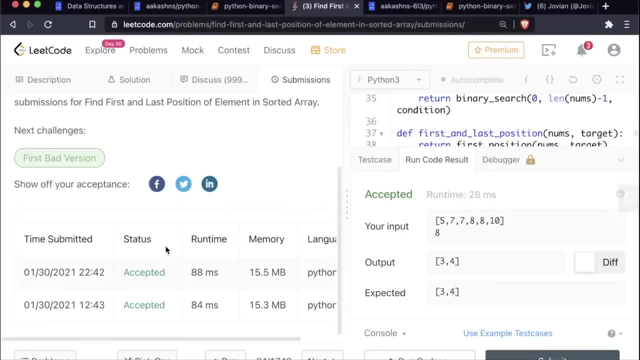 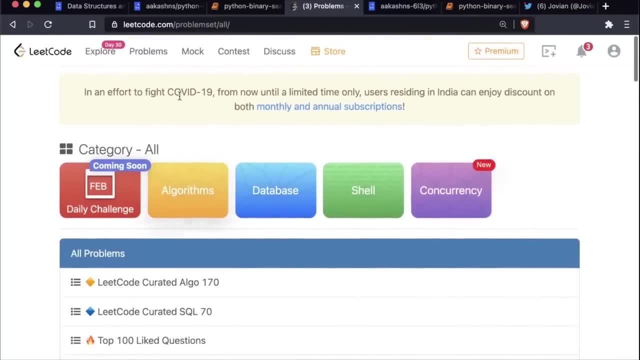 What was the memory it used? And your and our solution was accepted right. So check out leadcodecom, go to the problem section and you can see all the different problems that they have. You can also explore and you have different problems that come up every day. 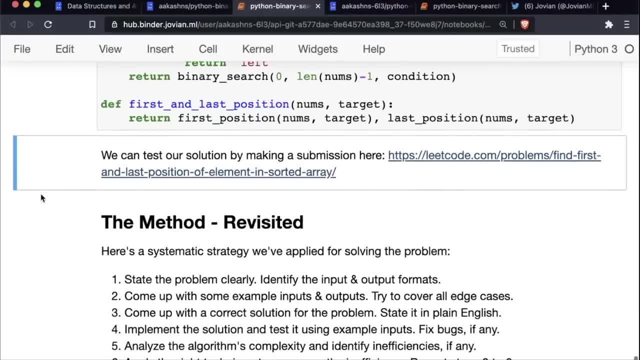 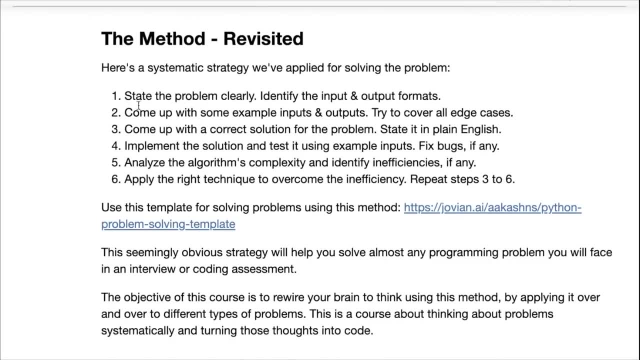 It's a great place to practice. So that's binary search for you, But I just want to revisit the method once again. So this is the systematic strategy that we've applied for solving the problem. We stayed the problem clearly and we identify the input and the output formats. 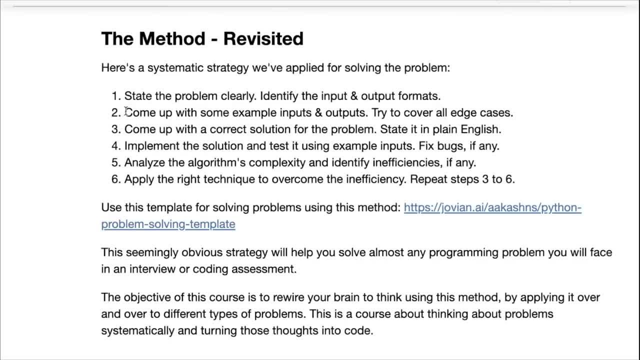 This. this shows that you've understood the problem. You know what the solution will look like. then come up with some example inputs and outputs and try to cover all the edge cases. So this shows that you are envisioning what are the different inputs that can come in before you write code. 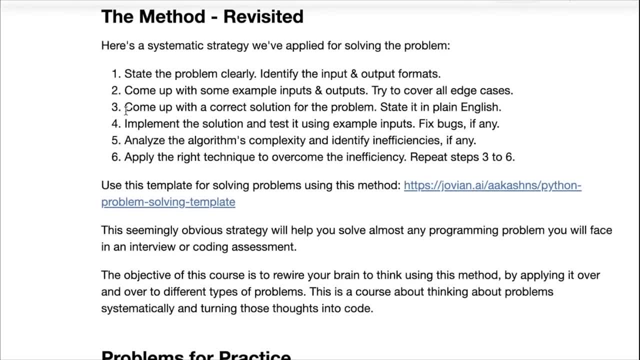 Then you come up with the correct solution- not necessarily the most efficient one- and state it in plain English. Now, when you try to state it, you will have to clarify it, and that will help you clarify your own thoughts and then you can analyze the 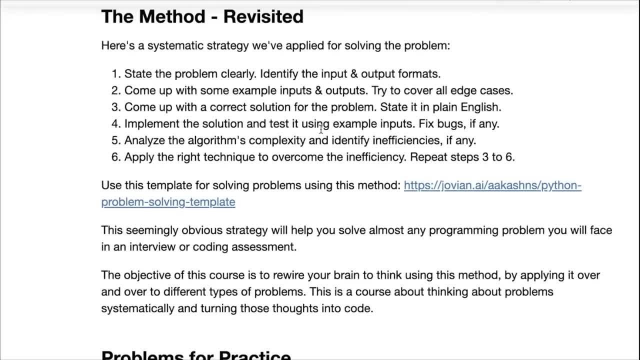 Algorithms, complexity and you can implement the solution and tested using example inputs. So this is the basic solution. now in interviews and in coding assessments maybe you know very there's a time limit. You may not want to implement a brute force, a brute force solution, because then you may get stuck in fixing issues with the brute force and you can directly jump ahead to step five. 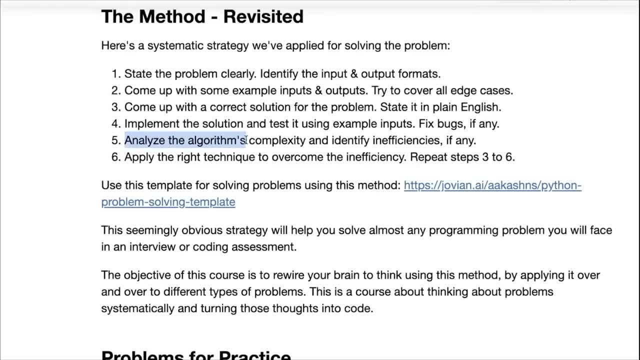 But while you're practicing, always implement brute force. then, step five, analyze the algorithms, complexity, And most of the time, it is simply a matter of counting the number of iterations, How much, Many times a while loop, or maybe a loop within a loop, is getting executed, and identifying efficiencies. 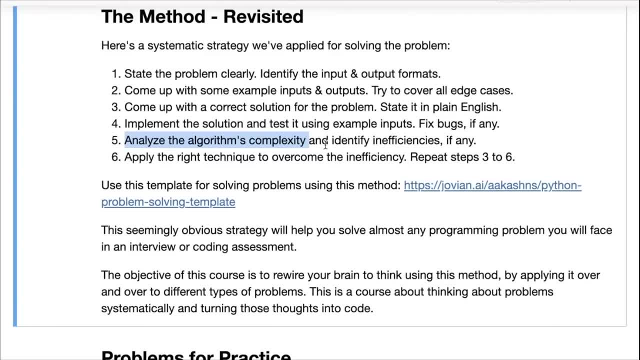 And if it is a brute force solution, it's generally quite easy to see the inefficiency. For example, in this case the inefficiency was that we know that the array is sorted, that anything we do will be better than going line by line, right. 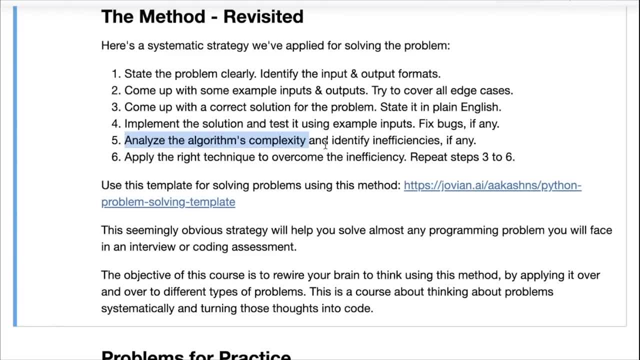 We could pick a random element and that would help us eliminate a good chunk of the area. So that is the inefficiency- and then apply the right technique And we are learning The techniques. So we've learned binary search today and then we are going to learn a lot more techniques that are asked in interviews. 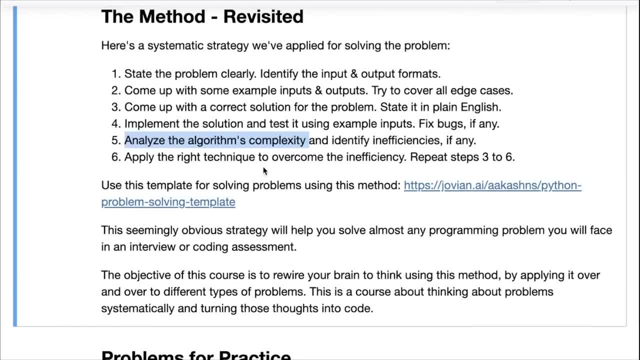 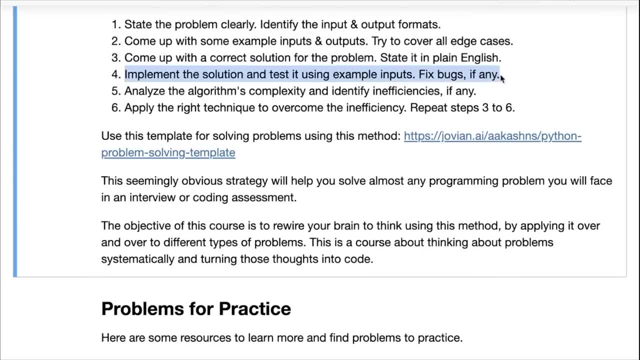 So apply the right technique to overcome the inefficiency and repeat steps three to six, which is, go back and come up with the correct solution with the optimized technique. implement the solution and test it using some example inputs and then analyze that. algorithms complexity. 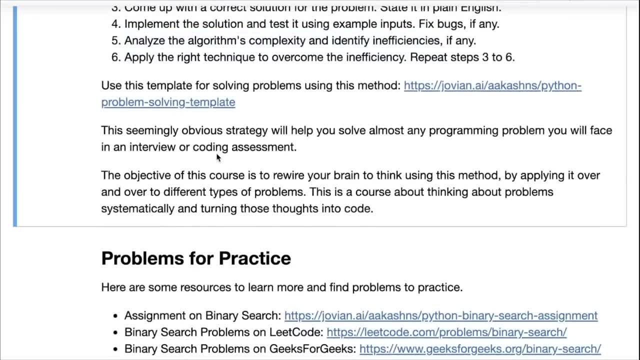 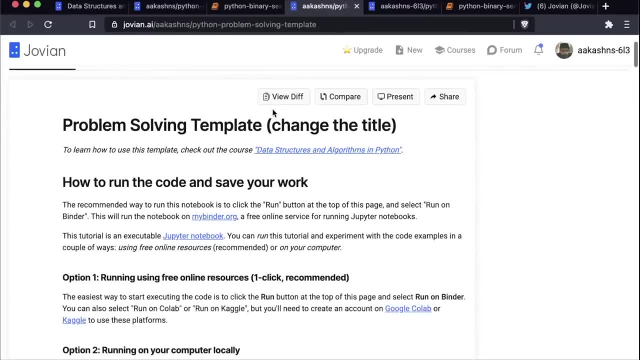 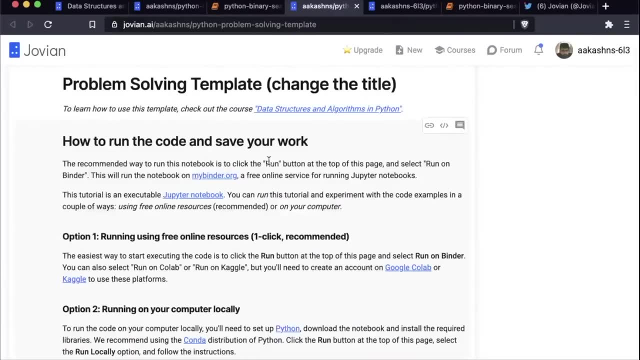 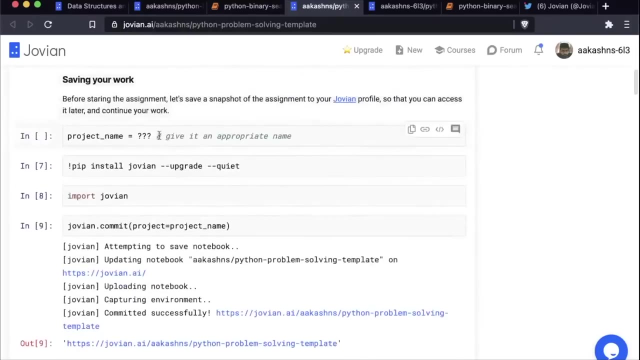 And identify any inefficiencies. So what we've done for you is we have created a template So you can see this Python pro problem solving template. and how you can use this template is to simply run it. So you run the code, you run this template and then, when you run the template inside it, you will see this question mark in a bunch of places. 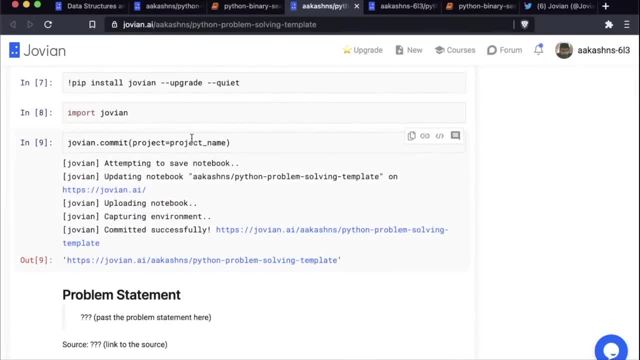 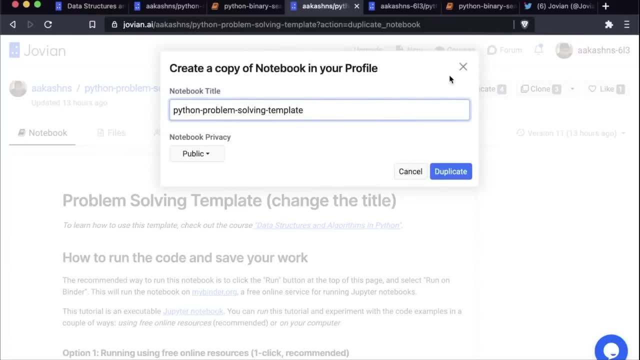 So you can give it a nice project name and you can commit it to your profile. One way you can save a copy over this template to your profile is by clicking the duplicate button. If you click the duplicate button, you can copy it in your profile and you don't have to look for it. 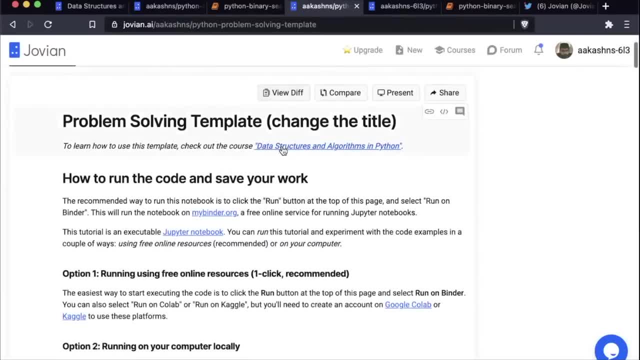 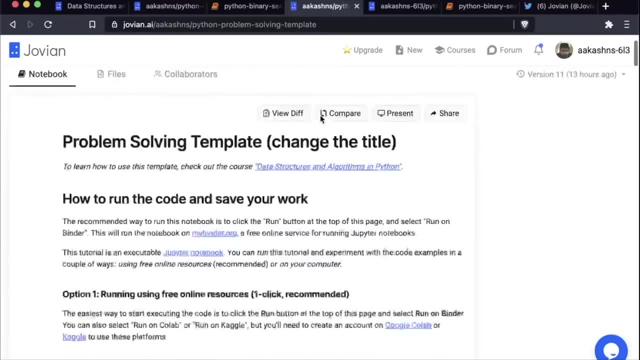 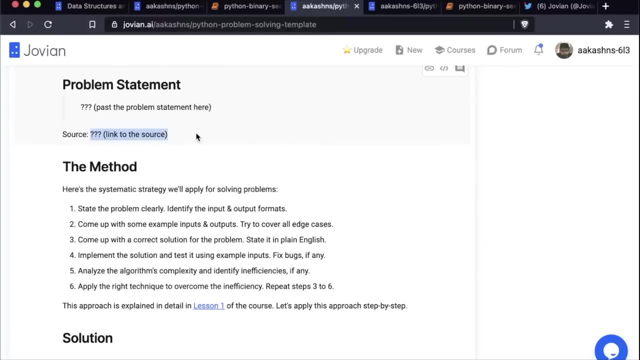 You can just save it, You can just find it on your Jovian profile. But anyway, once you have it copied, you can click the run button and then click run on binder and run run the template. Then you go down. once you run it and you can copy over a problem statement. you can copy over a link to the problem so that when you need to make a submission you can go back and refer. 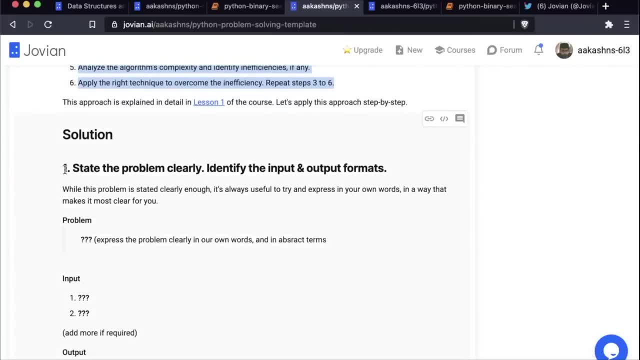 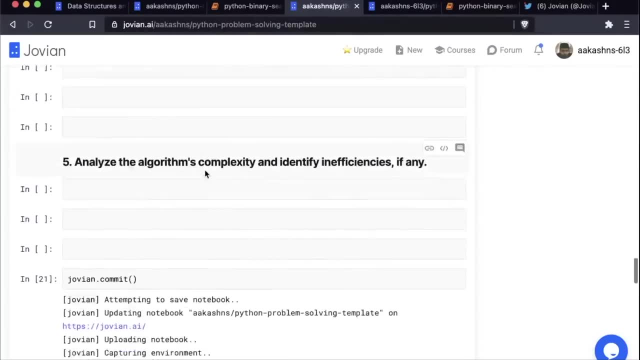 And then here the method is summarized for you, And here we have created sections for you So you can simply start filling out this method. So, step one, step two, step three, Step four, step five. So whenever you're faced with a difficult problem, just use this template. 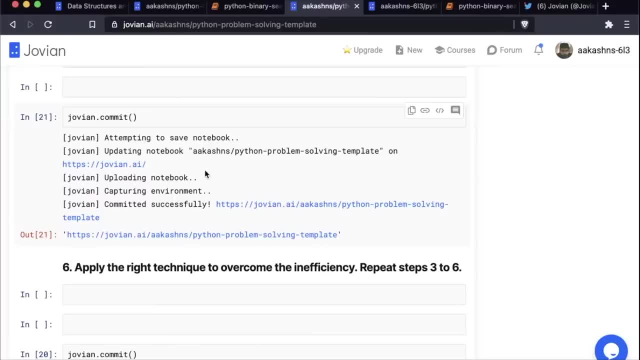 And I guarantee it One: if you work through this course, you will be able to solve a majority of the problems that you come across And, specifically, even if you are able to follow maybe about 30 to 40% of this course, you will easily be able to solve most questions that are asked in interviews, because questions asked in interviews are fairly simple in terms of the data structures or algorithms they test, but the intention that is more. 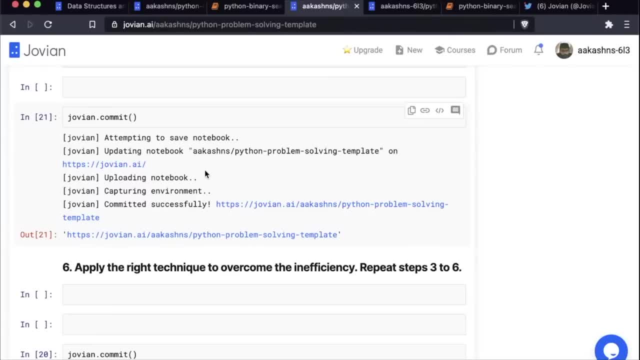 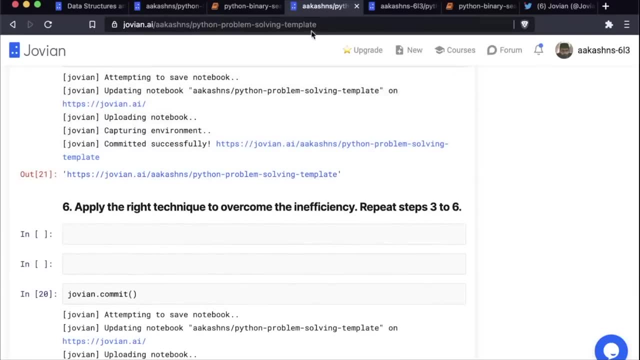 To test your approach. look at the quality of your code and see how clearly you're expressing yourself Right. And this is what is exactly what this method teaches you to do now. to encourage you to do this, to encourage you to try it out. 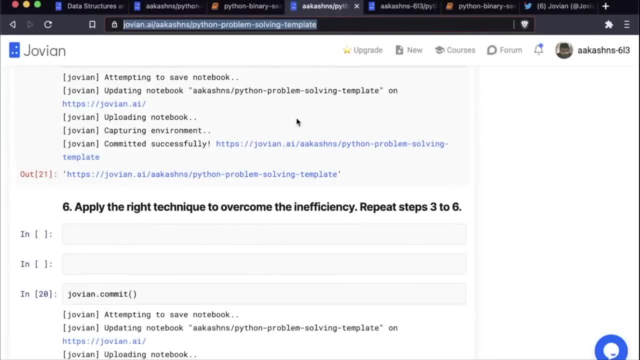 And you can take problems from places like lead code, um code, chef code, forces. There are a few links listed here. You can see practice problems. There are a bunch of links listed here. So that was today's lesson. for the next lesson, 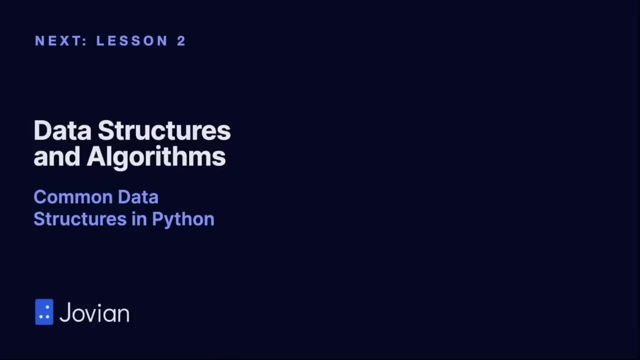 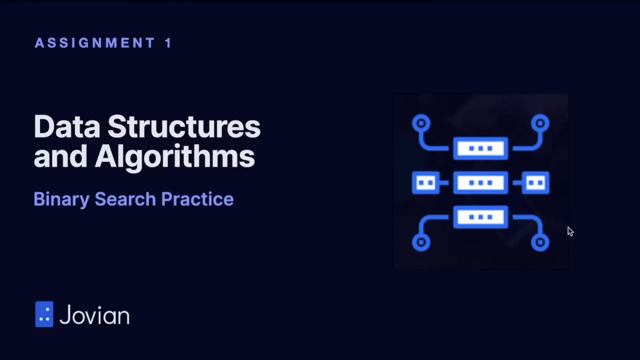 Common data structures in Python. So this is data structures and algorithms in Python and online certification course brought to you by Jovian. Thank you, Hello, and welcome to data structures and algorithms in Python. This is an online certification course being offered by Jovian. 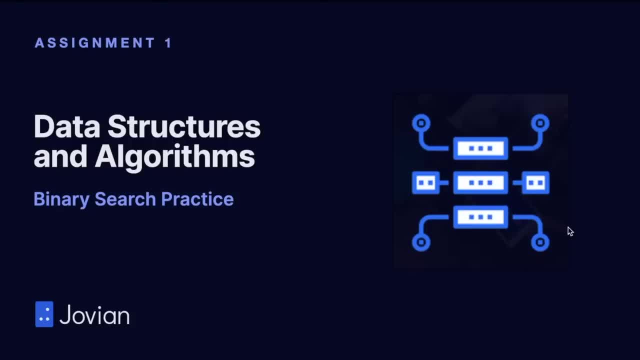 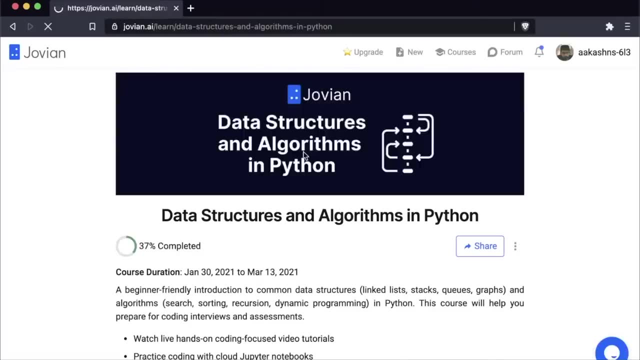 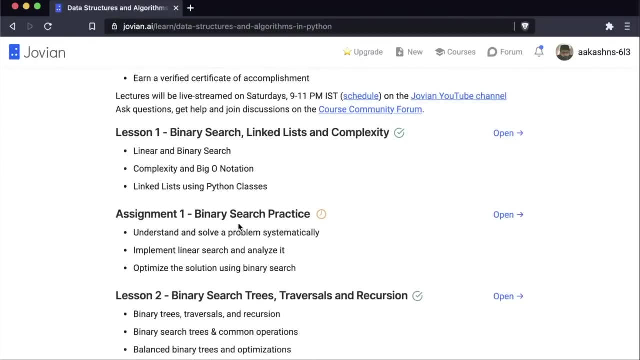 Today we're looking at assignment one, binary search practice. So let's get started. First thing we'll do is go to the course website, python DSAcom. On the course website You can enroll for the course and view all the previous lectures and assignments for assignment one. 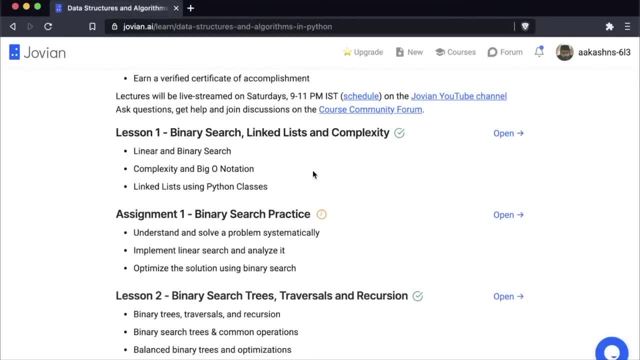 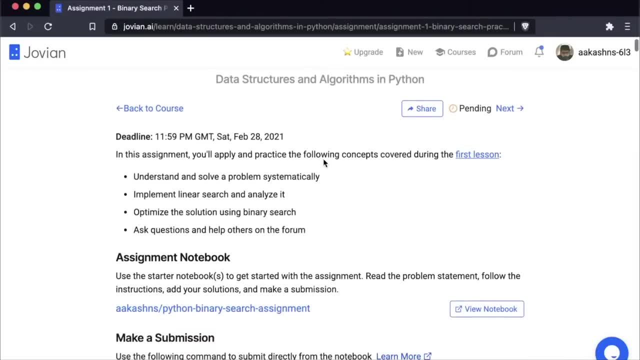 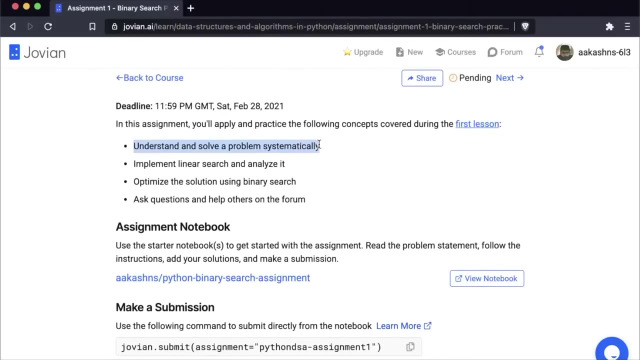 You may want to review the video and notebook for lesson one. Let's open up assignment one. It's called binary search practice. Now, in this assignment you will apply and practice the concepts that we covered in the first lesson, So you will understand and solve a system, solve a problem systematically, implement linear search and analyze it and optimize. 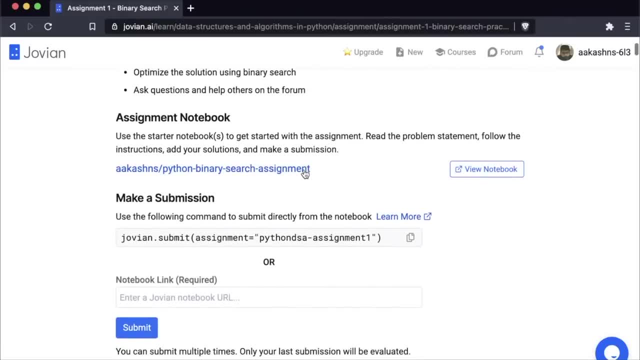 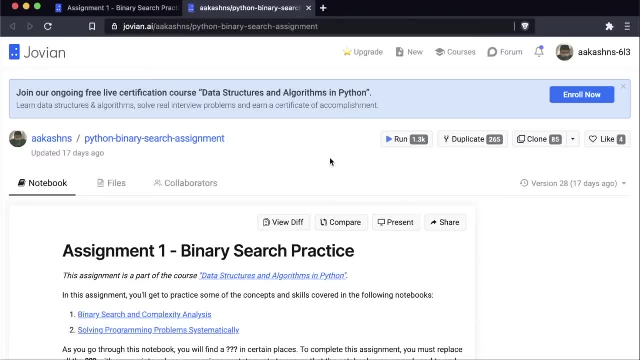 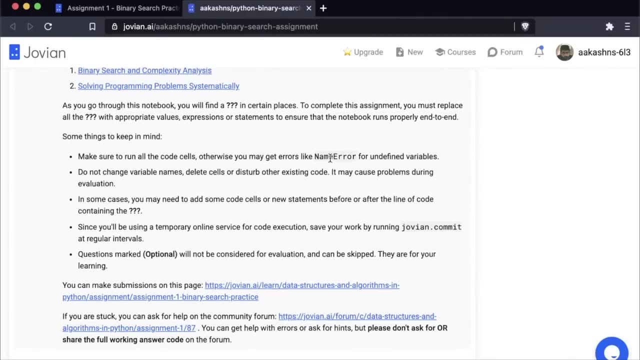 You will get a solution using binary search and ask questions and help others on the forum. Let's open up the starter notebook for the assignment, which contains that problem statement and other information. Now, this is a notebook you're looking at, hosted on Jovian. 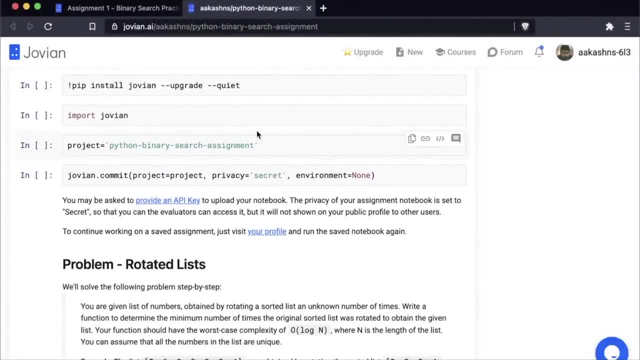 You can see some description here and if you scroll down below, you can also see some code, and you will need to execute this notebook, modify the code within it and record a new version which you can then submit, which you can then submit. 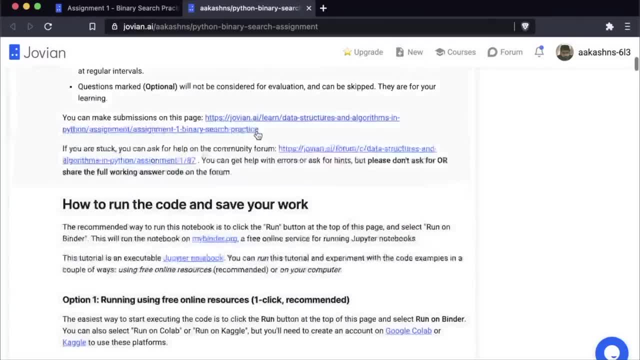 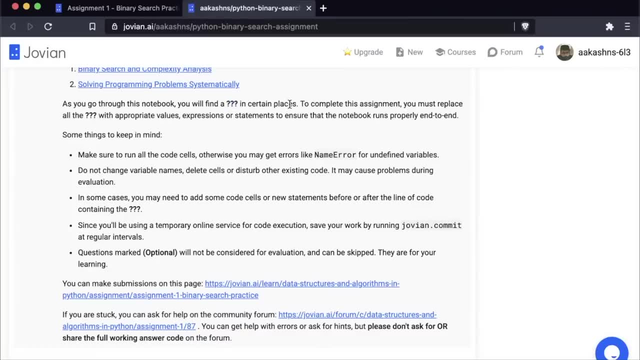 which you can then submit to see your score. So let's start reading through it. As you go through the notebook, you will find three question marks in certain places. to complete the assignment, You have to replace the question marks with appropriate values, expressions. 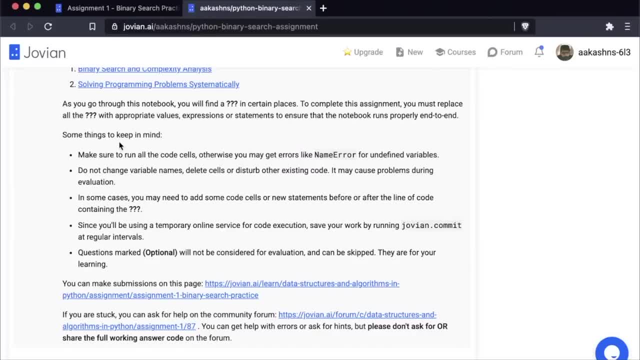 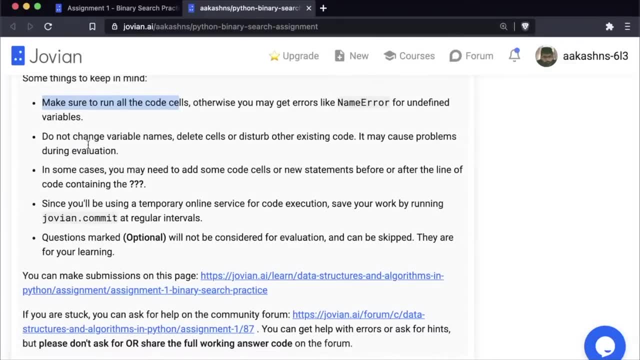 or statements to ensure that the notebook runs properly end to end. Now keep in mind that you need to run all the cells, Otherwise you may get errors like name error or undefined variables. You should not be changing any variable names or deleting any cells or disturb any existing code. 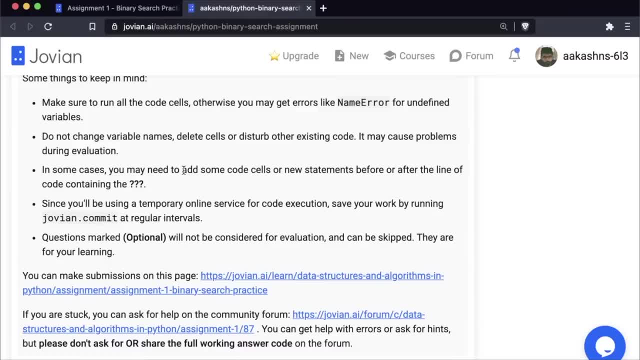 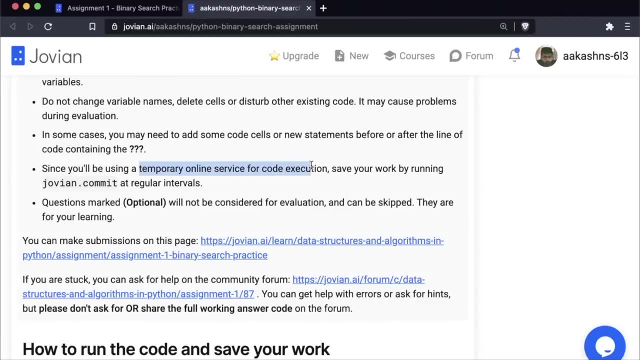 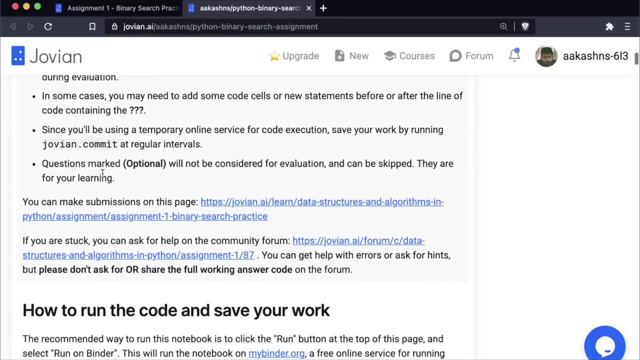 You can add new code cells or new statements, but do not redefine or do not change some of the existing variables. You will be using a temporary online service for code execution and we'll see how to use it in a moment. So keep saving your work by running joviancom at regular intervals. 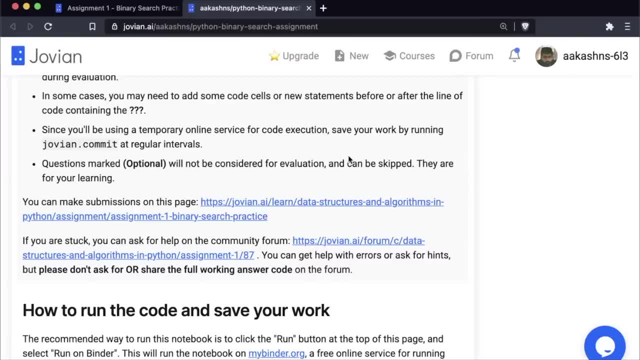 And then the question marks- optional- will not be considered for evaluation, Although we recommend doing them. they are for your learning, but you can make a submission before you do it, Or you have solved the optional questions Now you can make a submission back on the assignment notebook. 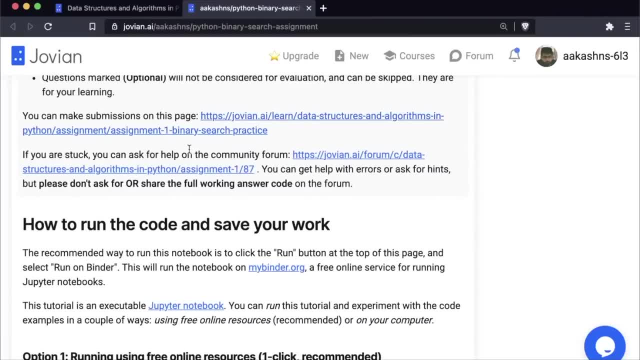 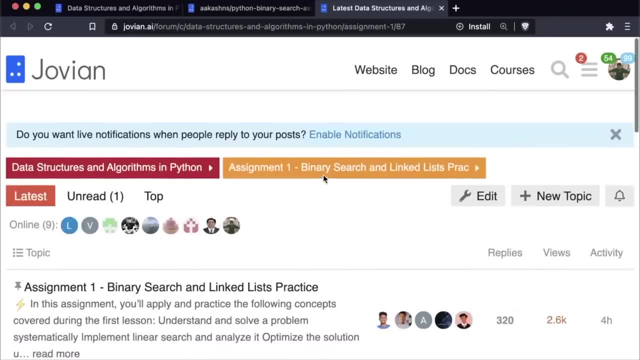 page and we'll see how to do that. And if you're stuck, you can ask for help on the community forum. It's listed here and we'll see how to do that as well. Now, one final thing I want to mention is you can get help. 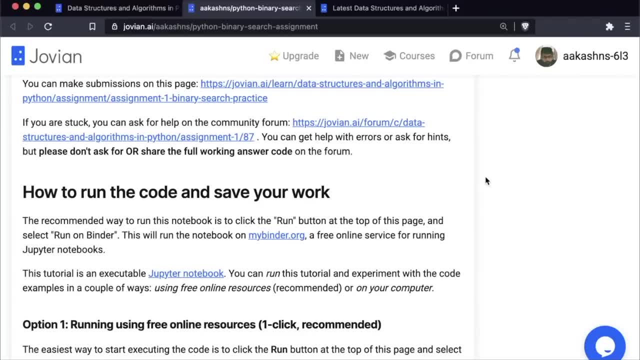 with errors or ask for hints. You can even share your code and errors that you are getting in the code, but please don't ask or share the full working answer code on the forum. This is so that everybody has the opportunity to work through the problem. statement on. 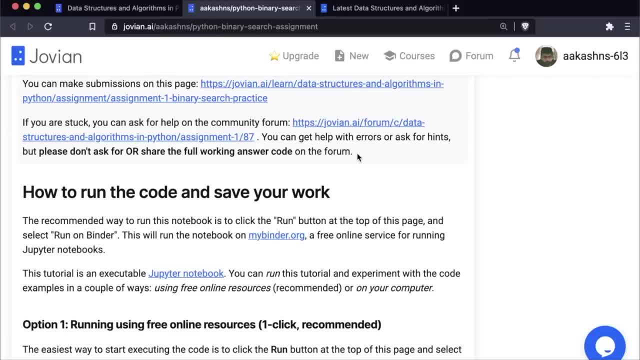 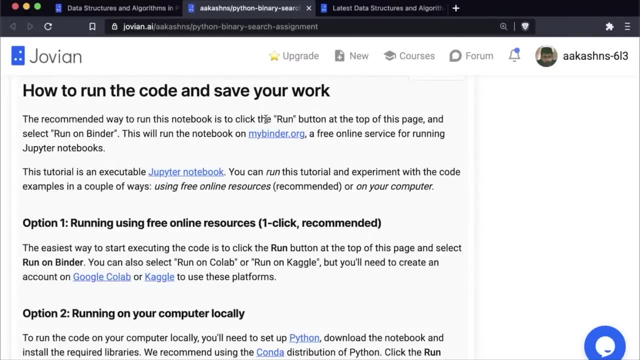 their own, make mistakes, learn from their own mistakes and arrive at the right solution. Now, how do you run this code? The recommended way to run this code is by clicking the run button at the top of the page and selecting run on binder, but you can also run it using some other options, like. 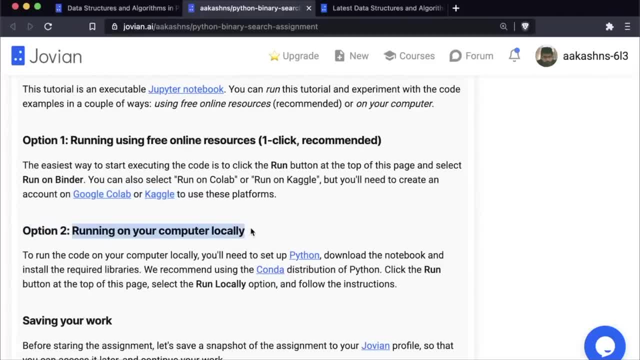 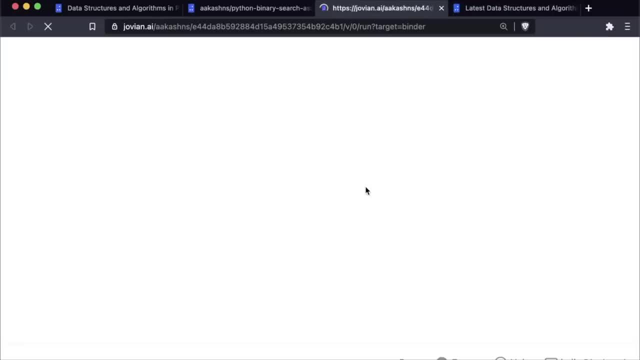 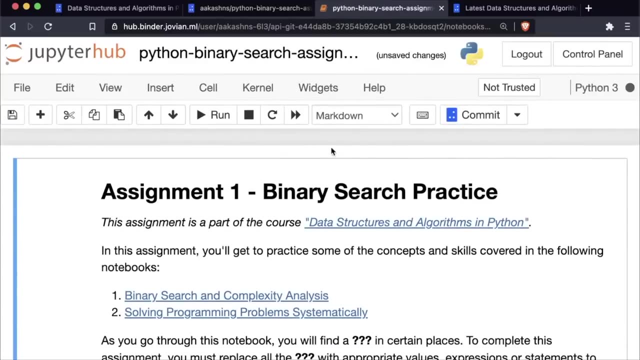 Google Colab or Kaggle, or you can run it on your computer. You tell locally. So we're going to use the recommended method run on binder. Now we have the notebook running in front of us. The first thing I like to do is go to kernel and click restart and clear output so that we can 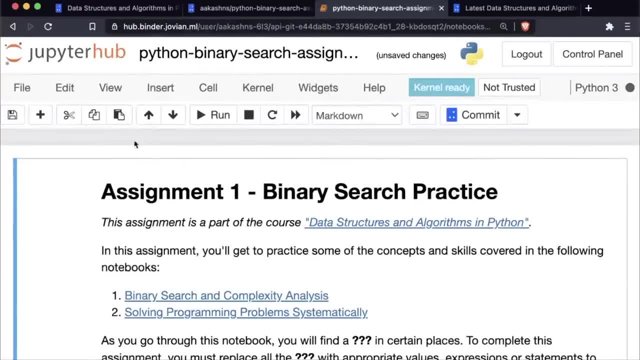 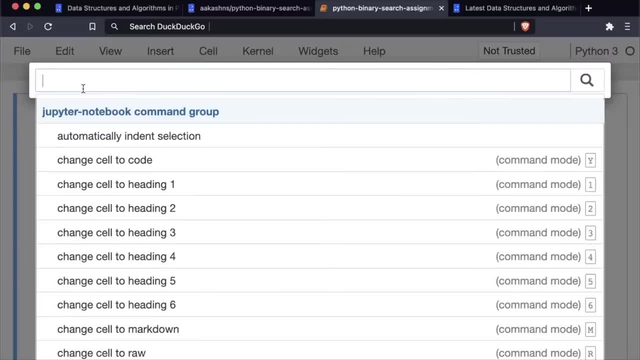 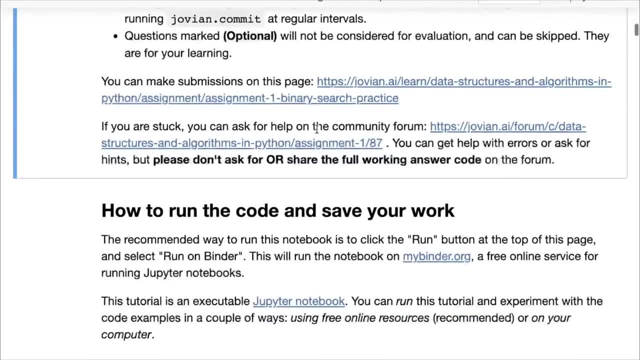 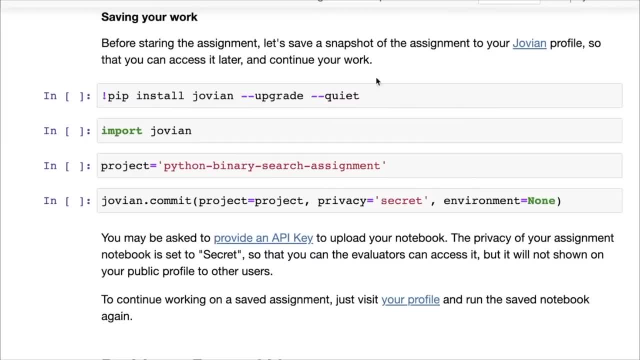 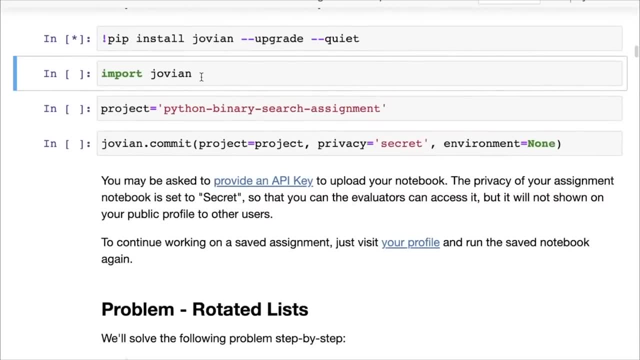 And before starting the assignment, let's save a snapshot of the assignment to our Jovian profile so that we can access it later and continue our work. I'm going to run pip- install Jovian. This is going to install the Jovian library, then run import. 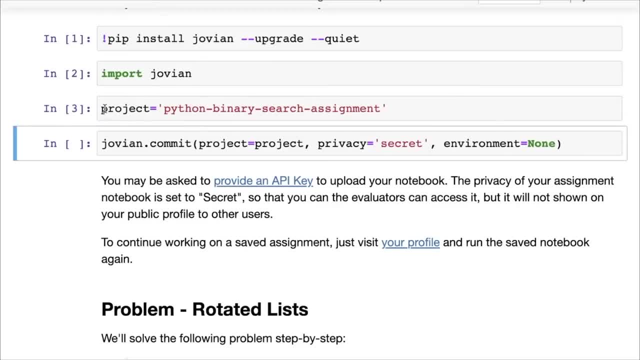 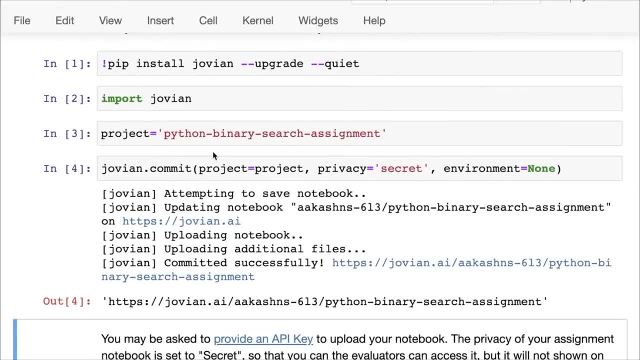 Jovian to import the library and set a project name- here I'm just calling it binary search assignment- and run Jovian dot commit. Now you've taken a starter notebook which was hosted on my profile and then you've run it on binder. but as soon as you run Jovian dot commit, a copy of 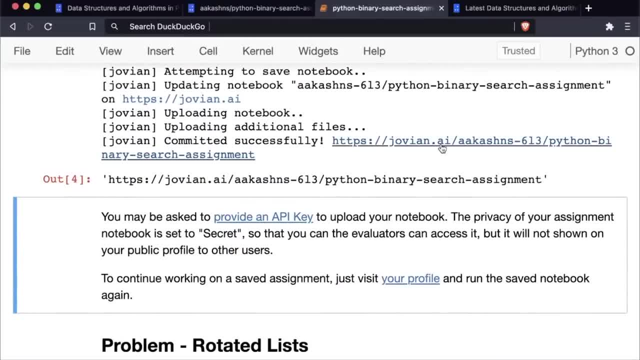 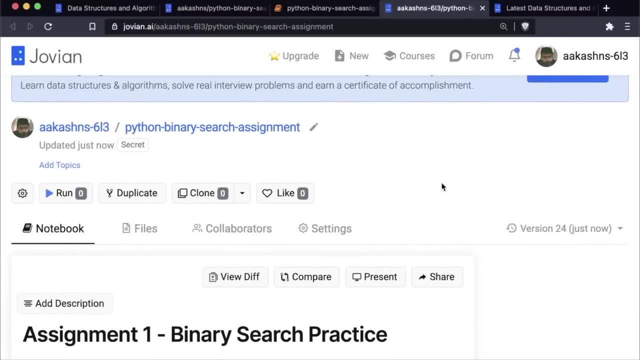 the starter notebook gets saved to your profile. so what you will see here is a link to a notebook hosted on your Jovian profile. let's open it up here and see. So now this is your personal copy of the assignment notebook. Any changes that you make here and run Jovian dot commit. 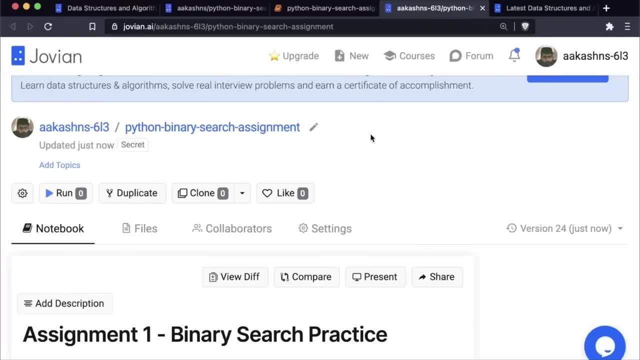 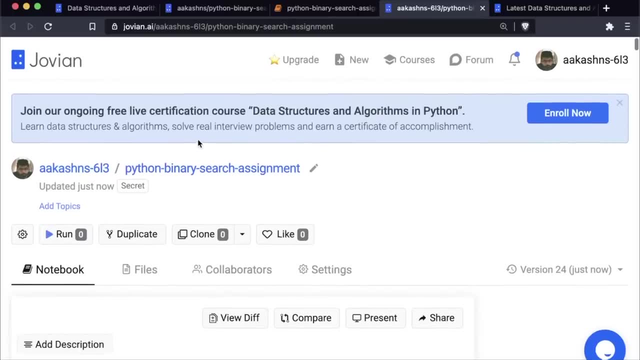 will get added to your profile. So if you want to come back and continue your work, then you do not have to go back to the original starter notebook, which contains all blanks. rather, you can come back to your profile. and you can come to your profile simply by opening. 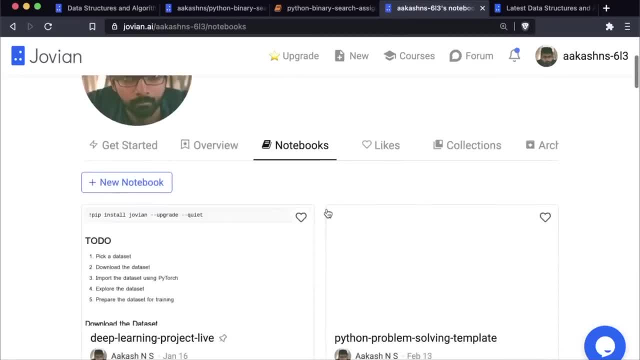 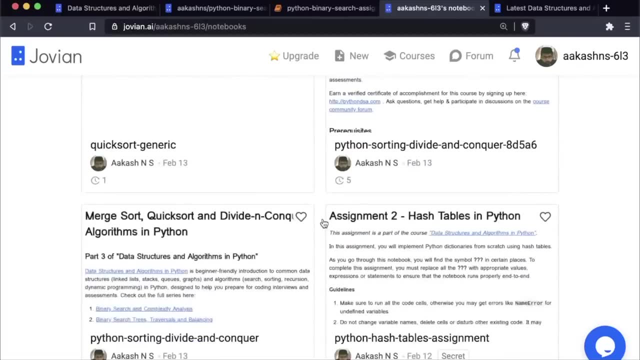 Jovian dot AI and on your profile you can go to the notebooks tab and on the notebooks tab you will be able to find, As you can see here, you will be able to find the binary search assignment here. There you go. 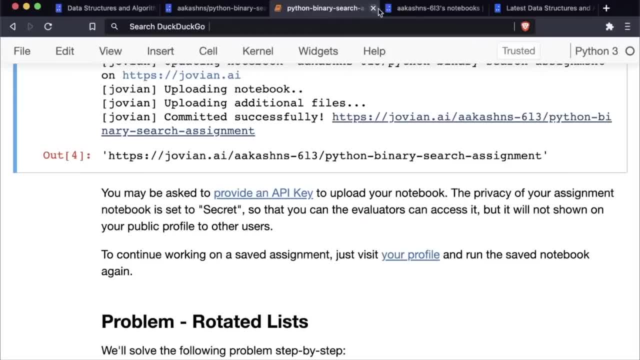 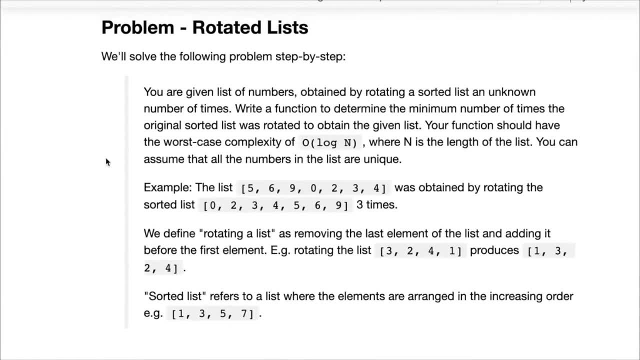 This is the binary search assignment that we just created, and you can open it and run it on binder to continue your work. So, moving along, this is the problem we are looking at here. You are given a list of numbers obtained by rotating a sorted. 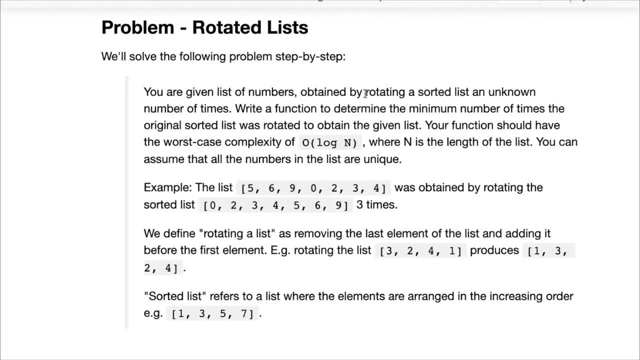 list and unknown number of times. Okay, So we have two new terms here- Rotating, A sorted list- And don't worry if you don't know what that means. Normally, if you see any new terms in a problem, they will be explained. 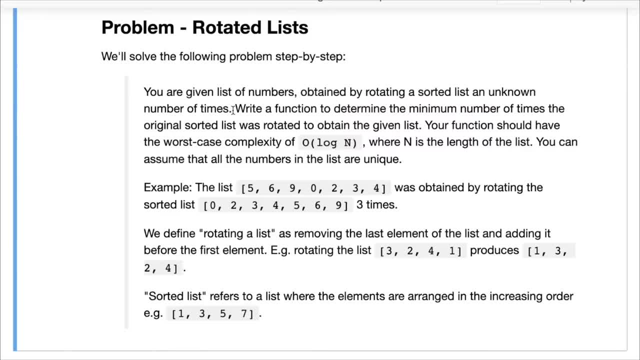 somewhere within the problem itself. For instance, here you can see that there's a definition. We defined rotating a list as removing the last element of the list and adding it before the first element. For instance, rotating the number a list- three, two, four, one- leads to removal of. 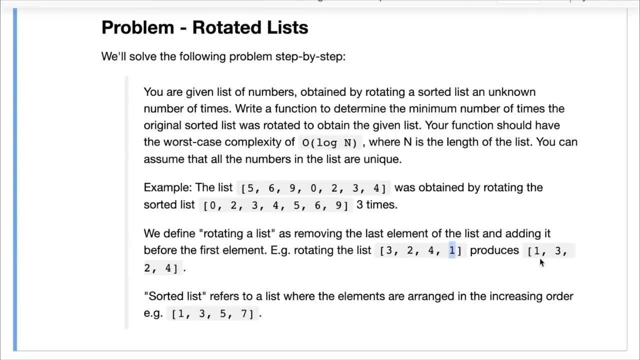 the last number and then placing it at the very beginning. So you end up with the list one, three, two, four. This is a new operation that we are defining. This is not something standard, but you will find that a lot of problems will define new. 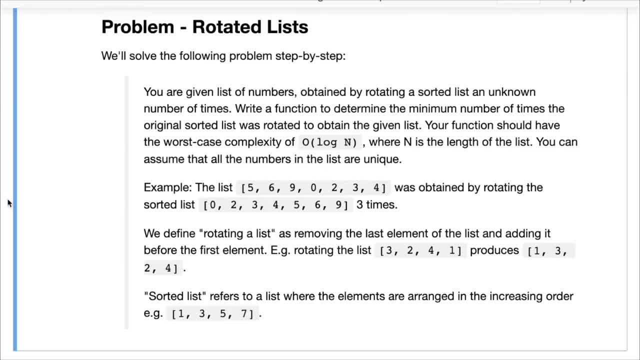 terms or new operations so that they it becomes easier for you to understand the problem. So that's rotating a list. Now. rotating a list once produces one, three, two, four. Now if you rotate that list again, the resulting list one more time, then you will end up with 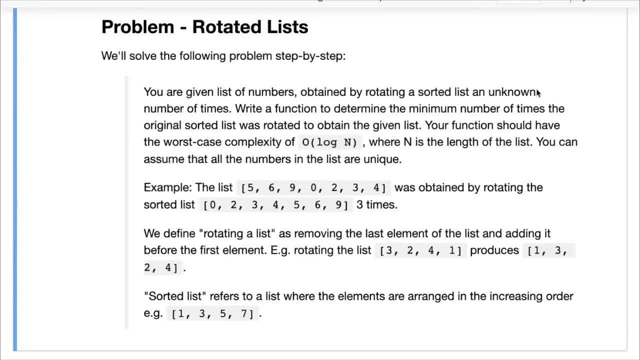 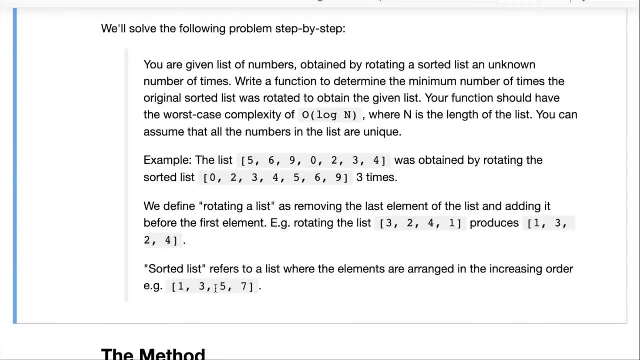 four, one, three, two and so on. And then the other term is sorted. So sorted refers to a list where the elements are arranged in increasing order. In this case we have numbers, and the numbers one, three, five, seven are increased arranged. 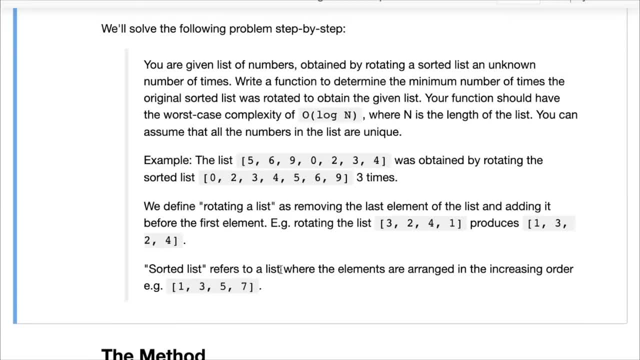 in increasing order, So this is a sorted list. but if this was three, two, four, one, well, that's not. the numbers are not arranged in increasing order, So that's not a sorted list. So you are given a list of numbers obtain, obtain by rotating a sorted list and unknown. 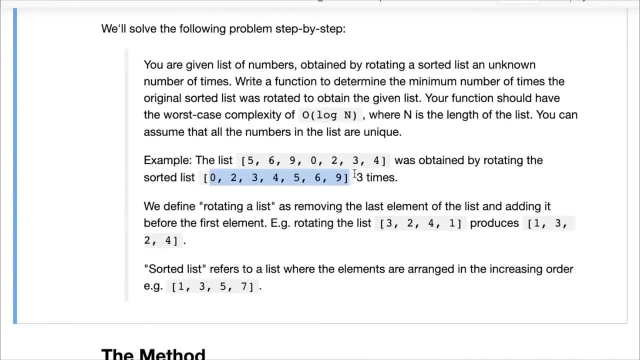 number of times. for instance, this sorted List- zero, two, three, four, five, six, nine- is rotated a certain number of times And you can verify that if you rotate this three times you end up with the list five, six. 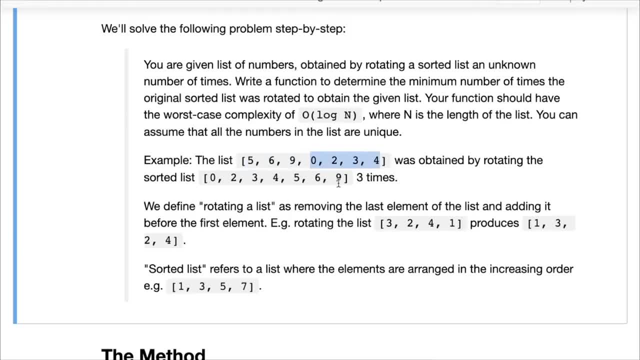 nine zero, two, three, four. right, You can see that first nine comes to the beginning, then six come to comes to the beginning And then five comes to the beginning. So you need to write a function and you're given just this, the list, you're not given the original. 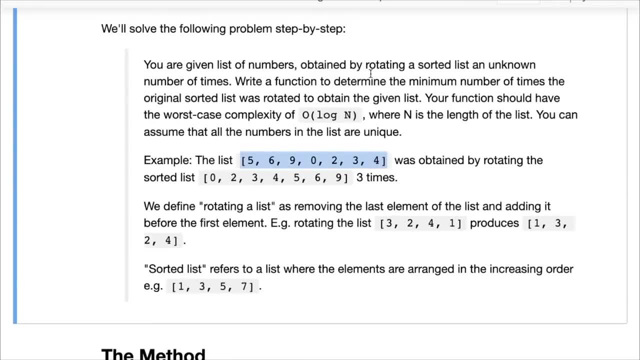 sorted list. You're given the list obtained by rotating some sorted list and unknown number of times. Now you need to write a function to determine the minimum number of times the original sorted list was rotated to obtain the given list. Your function should have the worst case complexity of order, log n, where n is the length of the. 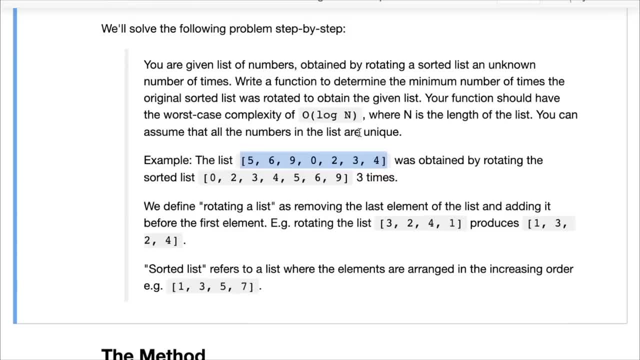 list And you can assume that all the numbers in the list are unique. Okay, So three parts. write a function to determine the minimum number of times you need to rotate the original sorted list In this. in this case, it is three. 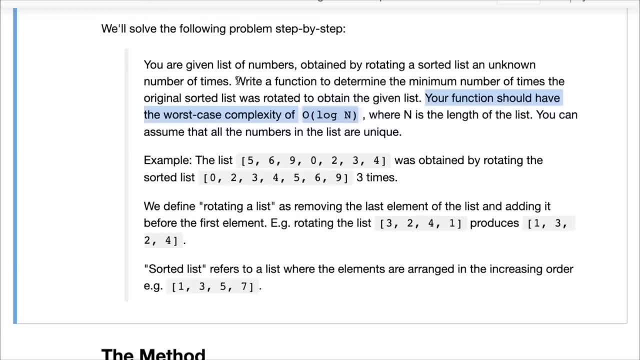 The function should have the worst case complexity of log n. So this determines correctness, Determines efficiency. and then this is some additional information to help you that you can assume all the numbers in the list are unique. If this was not mentioned, you would also have to handle the case where your list does not. 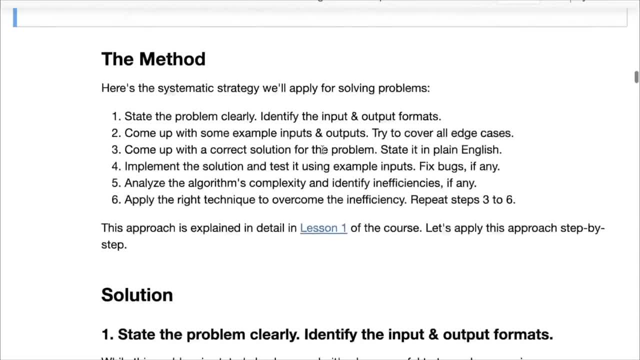 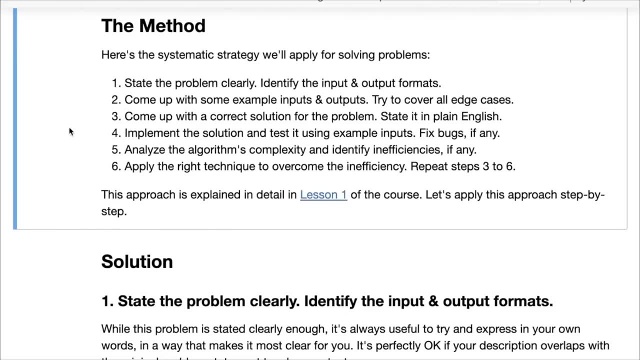 contain unique numbers. Now we will apply the method that we have been applying all throughout this course for solving the problems. Number one: state the problem clearly, identify the input and output format. Number two: come up with some example inputs and outputs and try to cover all the edge cases. 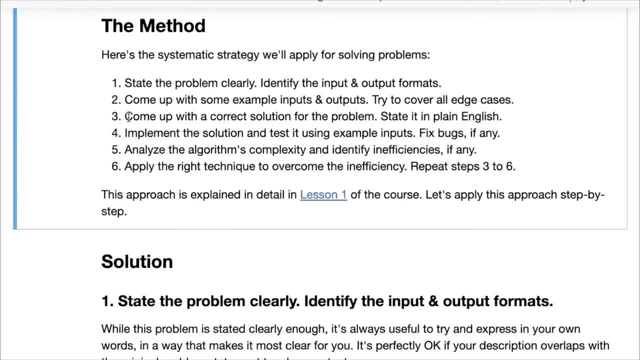 Number three: come up with a correct solution for the problem and stated in plain English. Number four: implement the solution and tested using some example inputs and having test cases And then implementing a solution allows you to test them using the example inputs and fix any. 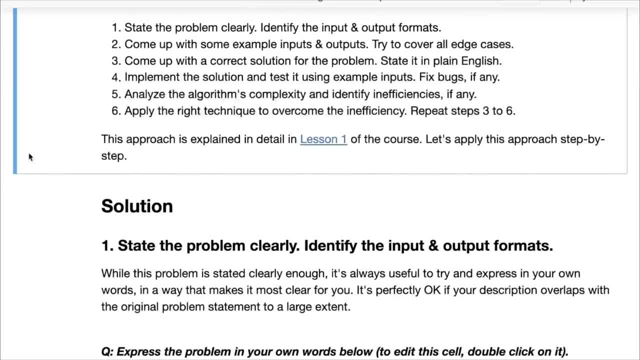 bugs. That's why it's very important to have some test cases. Number five: analyze the algorithms complexity and identify any inefficiency. And number six: apply the right technique to overcome the inefficiency. And then you go back and repeat steps three to six. come up with the correct solution, implement the. 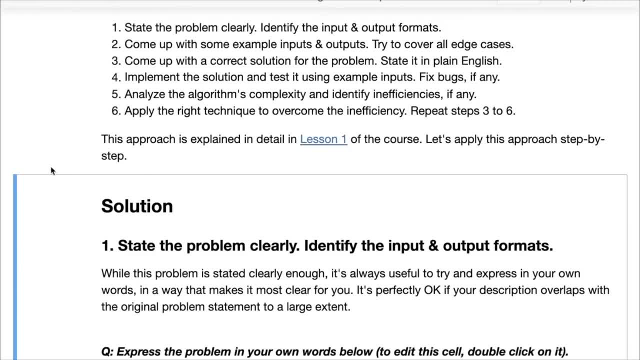 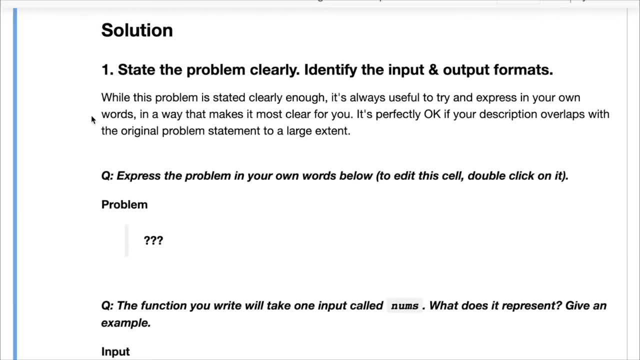 solution and tested and analyze the algorithms. complexity, And you can review lesson one for a detailed explanation of this method. Now let's apply it step by step. The first step is to state the problem clearly and identify the input and output formats. Now, while it is stated clearly enough, it always helps to express it in your own. 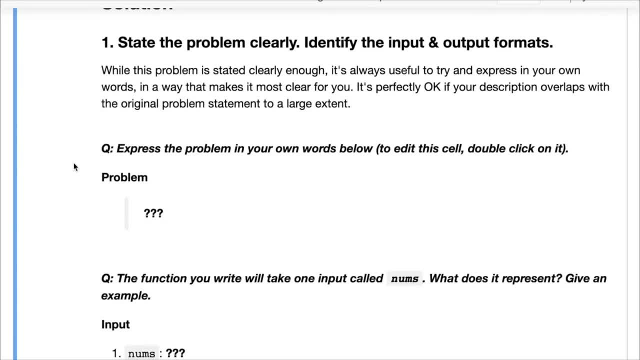 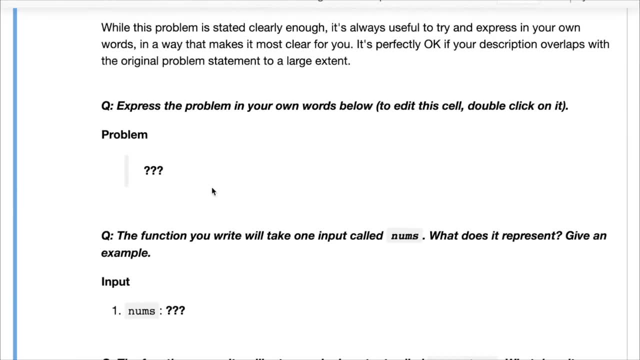 words in the way that it makes it most clear for you, And this is something that you can keep returning to, rather than the original problem statement, because this is something that you will understand better, And it's okay if your problem overlaps with the original problem statement, but do try to. 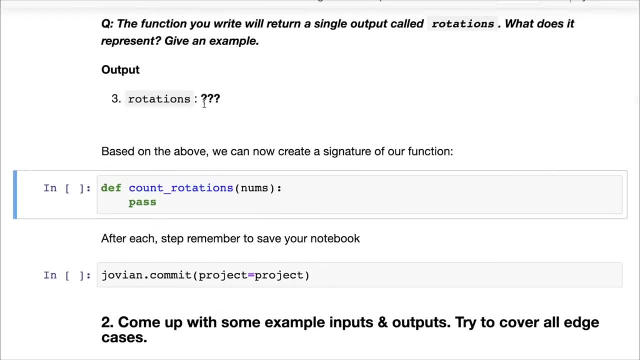 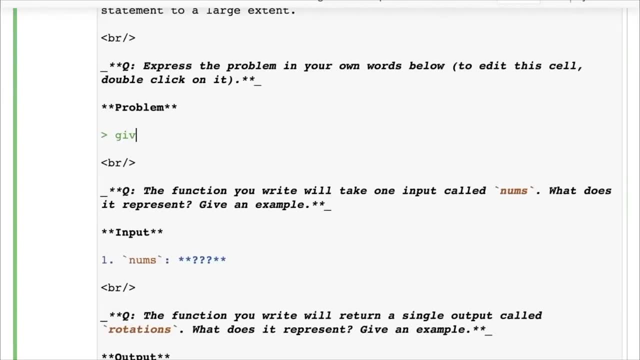 express it in your own words. So in this case, what I've just done is I have double-clicked here. Once you double-click, you can now edit this text cell and now we can start writing. a problem? So, let's say, given a rotated list. 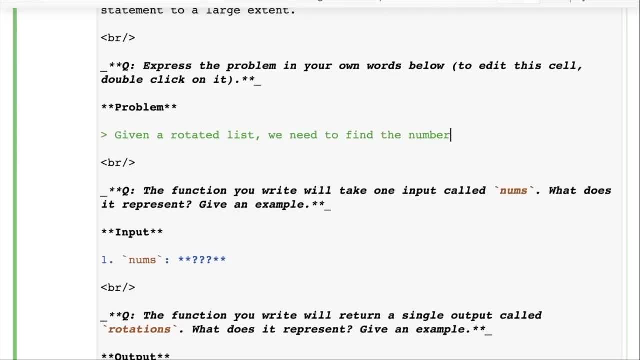 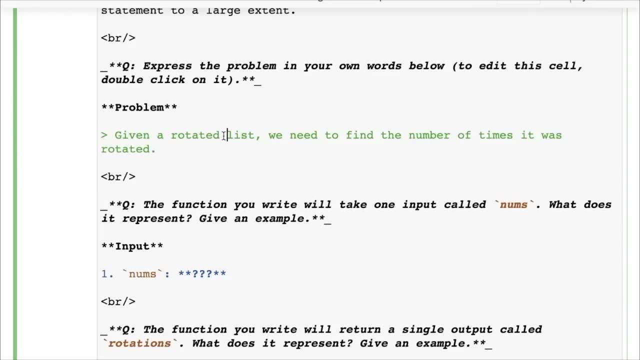 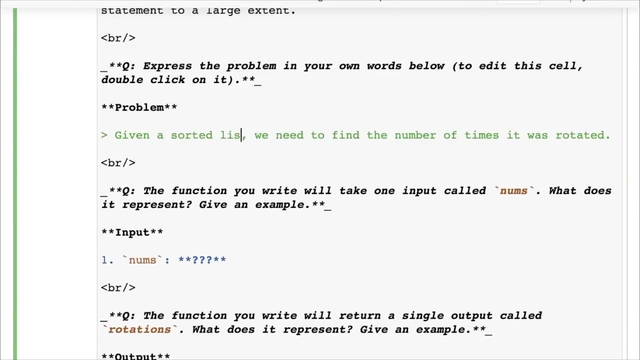 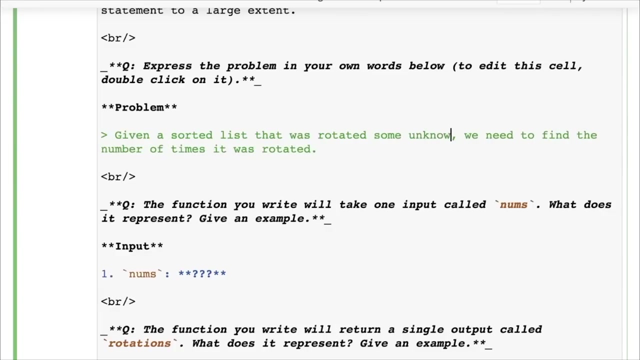 Okay, Okay, We need to find the number of times it was rotated, and, okay, I think what I've probably missed here is that it is a sorted list. So, given a sorted list that was rotated some unknown number of times, We need to find the number of times it was rotated, right? 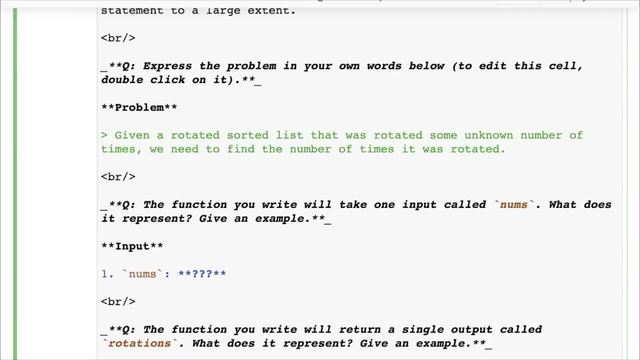 Maybe I'm just going to say given a rotated sorted list because technically the input is not a sorted list, It's a rotated sorted list. So, given a rotated sorted list that was rotated an unknown number of times, we need to find a number of times it was rotated. 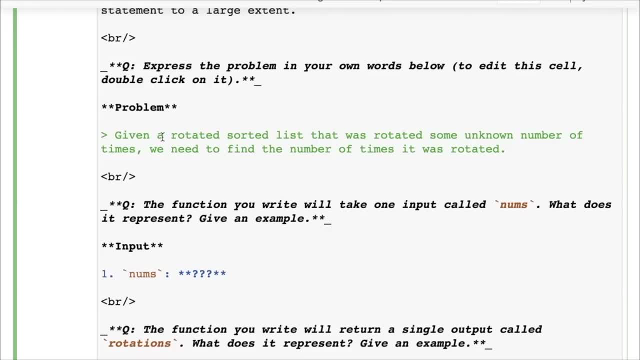 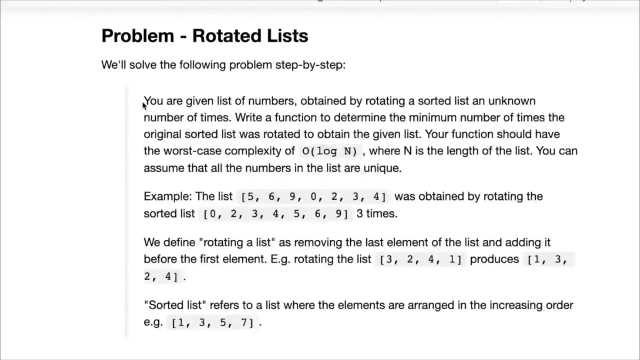 But doing this exercise helps you determine if you've understood the problem correctly, and you may often find that, okay, there's a certain detail in the problem that you missed. Okay, But at this point I'm happy with my description and you will see that it is matching the description to a large extent, but it's. 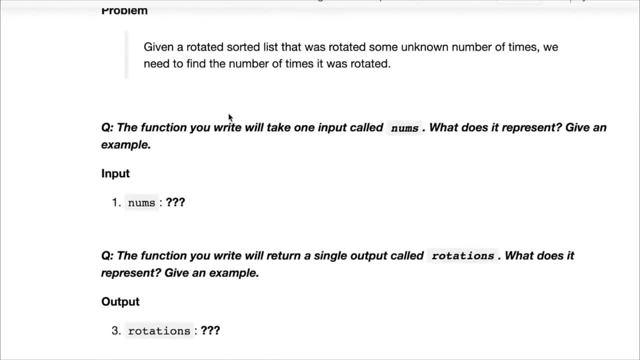 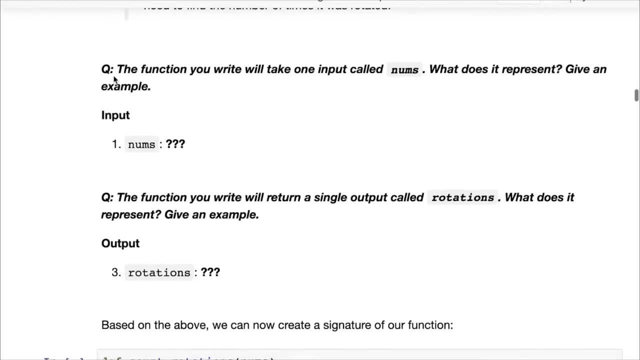 something that I understand better. So I'll just refer to this from this point. Now. I'm assuming here that I know what rotation and sorted means, Otherwise I could also include those. Then here's a question: The function will. you will write: we'll take one input called nums. 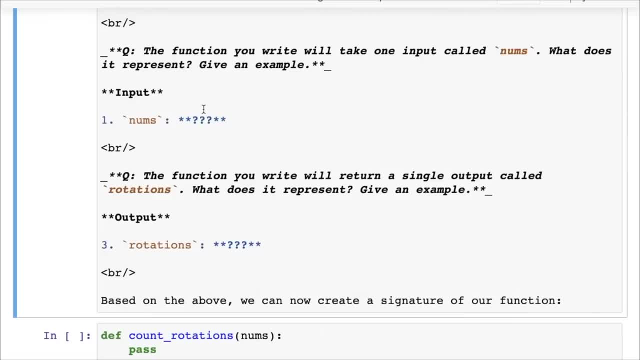 What does it represent? What does it represent and give an example? Okay, So once again we double click on this and one input is nums. So this is a sorted, rotated list And let's give an example here. Let's say we take the sorted list three, five, six, seven, nine. 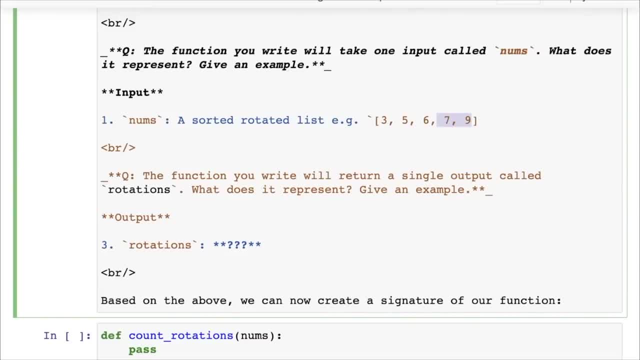 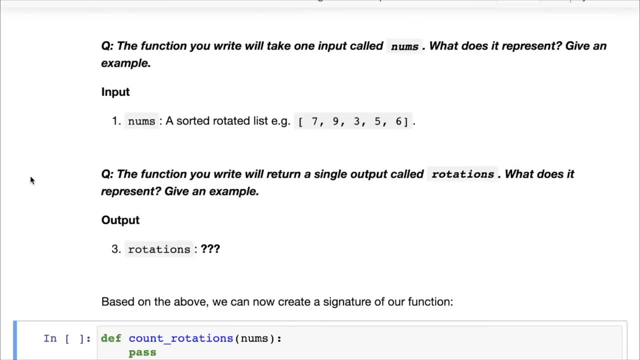 And then we rotate it a few times. Let's say, we rotate it a couple of times, So we ended up with this sorted, rotated list. That's our input. So we've answered the question here Now. the first question was to express the problem in your own words. 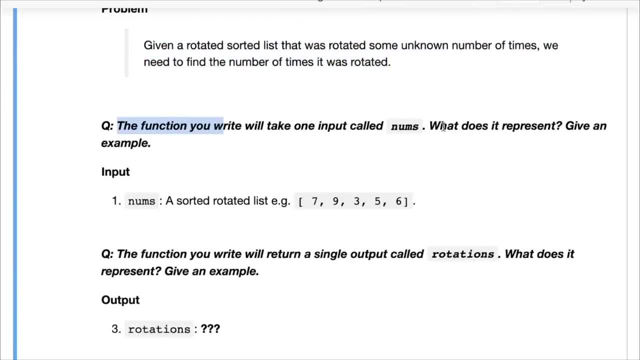 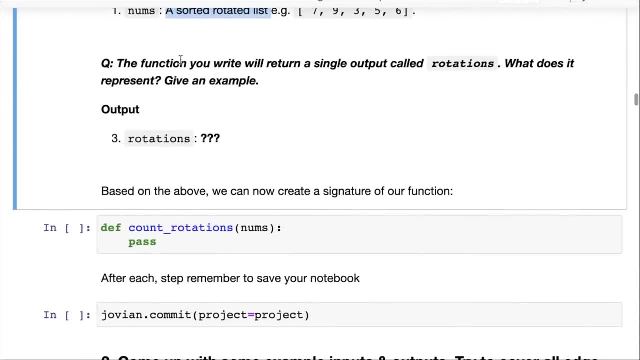 This is the solution. The second question was: what does the input nums represent? Give an example. It represents a sorted rotated list: seven, nine, three, five, six. The third question is the function you will write. It will return a single output called rotations. 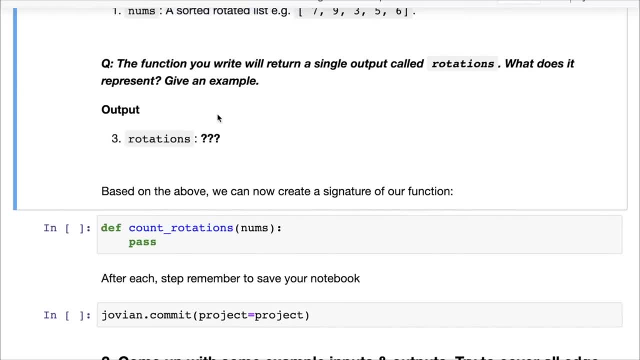 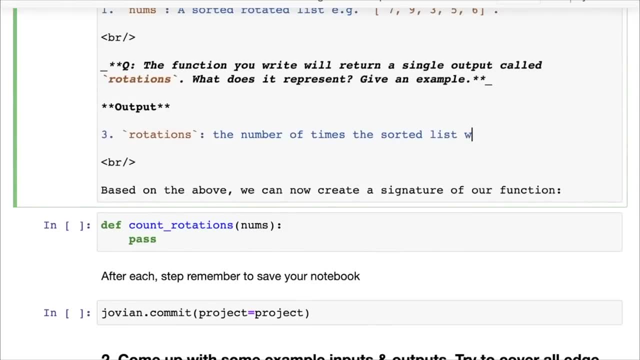 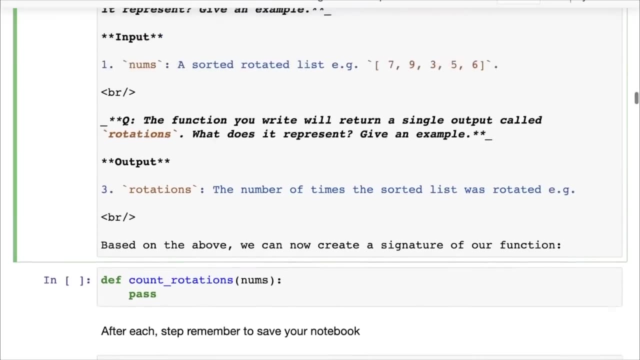 What does that represent? Well, you have to write a function that identifies how many times the list was rotated. So this is the number of times the sorted list was rotated, Okay, And in this case, the example that we have is that this sorted list was rotated twice. 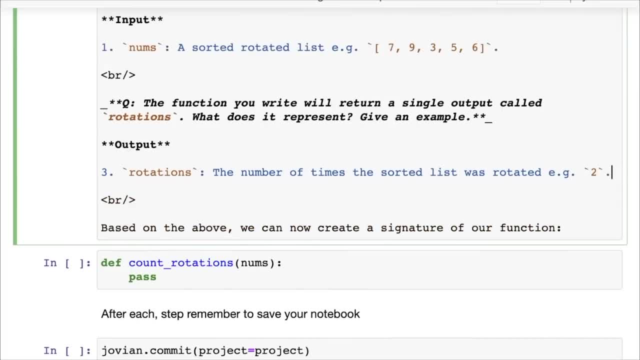 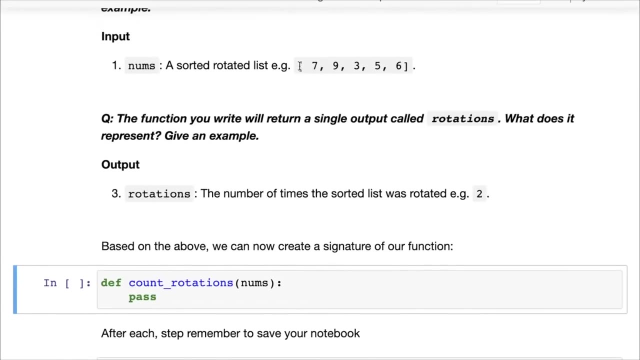 Three, five, six, seven, nine was rotated two times, So you mentioned two here. You can see these back quotes that I'm using here. This is next to the number one on your keyboard or below the escape key. What these backwards let you do is they let you express text as code within Markdown. 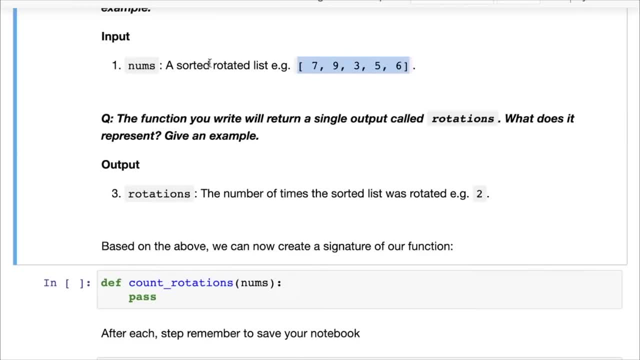 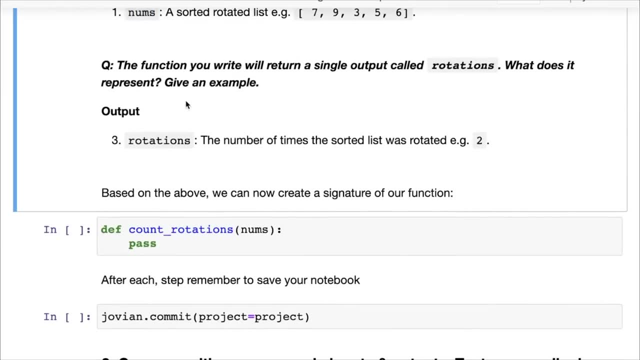 You can see that they have a gray background and they have a different font. This looks a lot more like cool. Same as here true for nums. So you can use Markdown and its features to your advantage to organize your descriptions and your text better. 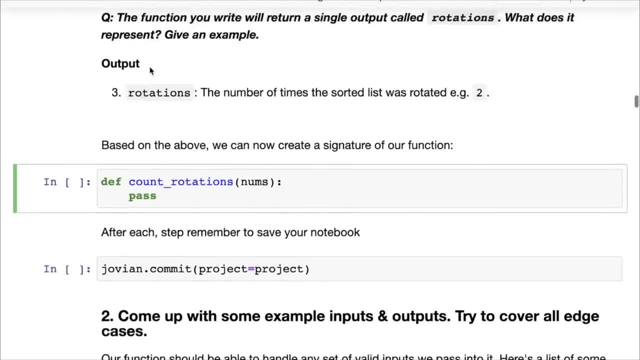 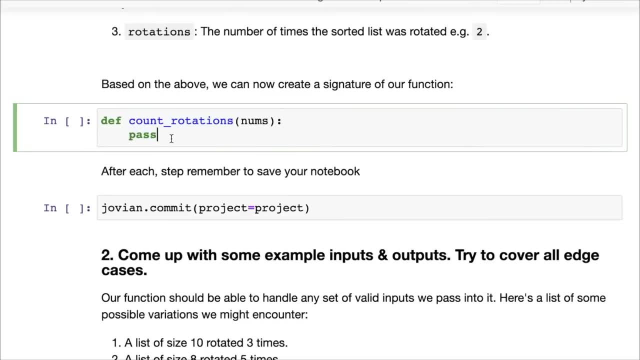 Okay, So now, based on the above, we can now create a signature of our functions. We have a function called counts rotations. It takes a number, list of numbers and it returns. Well, right now we're just putting pass in here, but we know that it's going to. 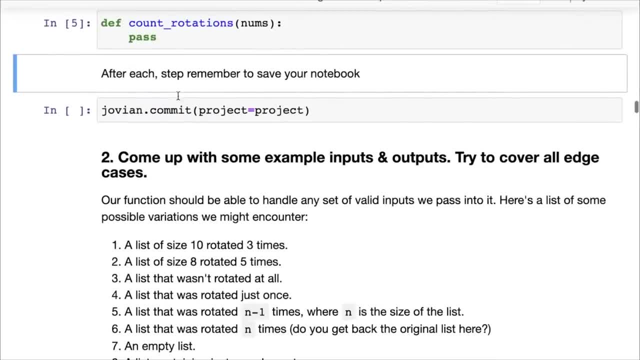 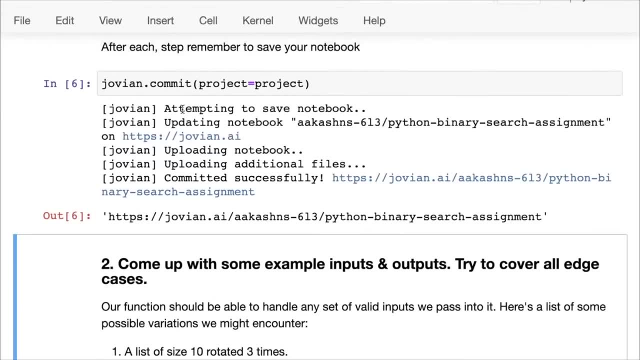 return on single number rotations. Now, after each step, remember to save your notebook. So we are going to just run joviancommit. And now, if you leave your computer, you do not have to be worried that your work may be lost. 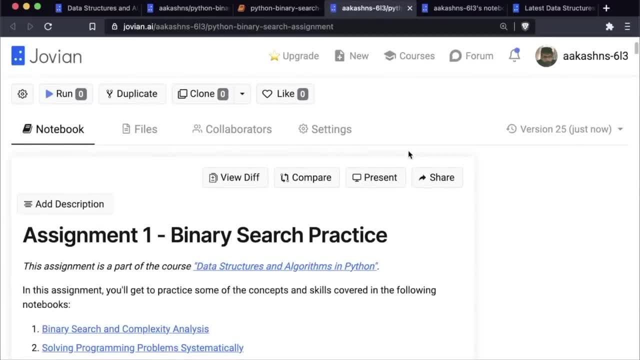 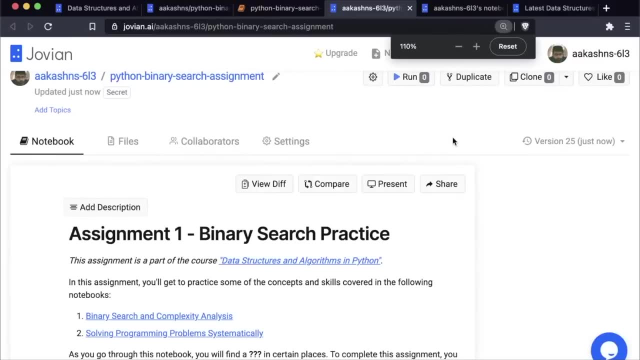 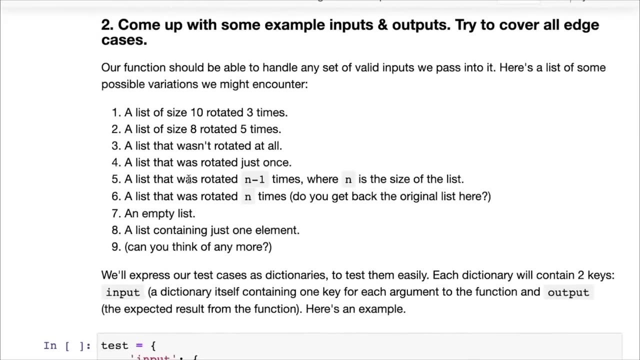 So you can go in here and you can open up this notebook from your Jovian profile and press run at any point to run this notebook. Now step two is to come up with some example inputs and outputs and try to cover all the edge cases, and our function should be able to handle any set of valid inputs. 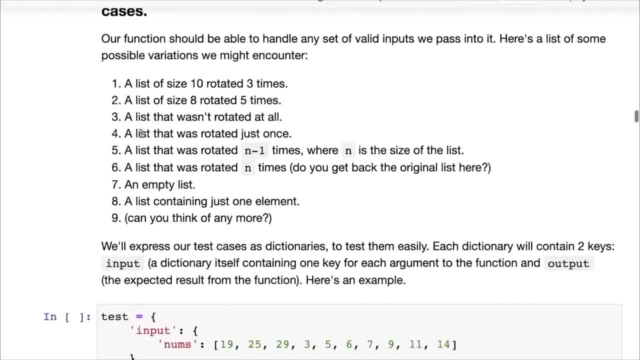 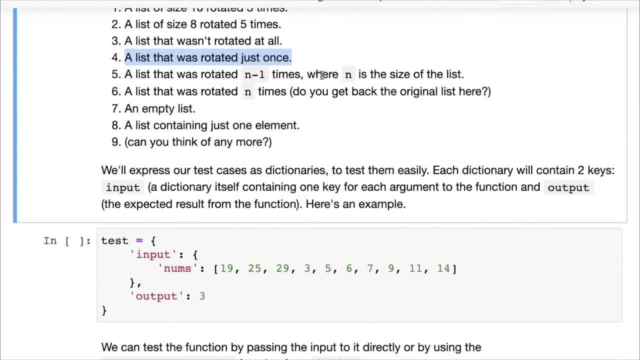 So here is some variations that you can encounter: A list of size 10, rotated three times. a list of size eight, rotated five times. So these are two generic examples. And then a list that wasn't rotated at all, A list that was rotated just once, a list that was rotated N minus one times, where 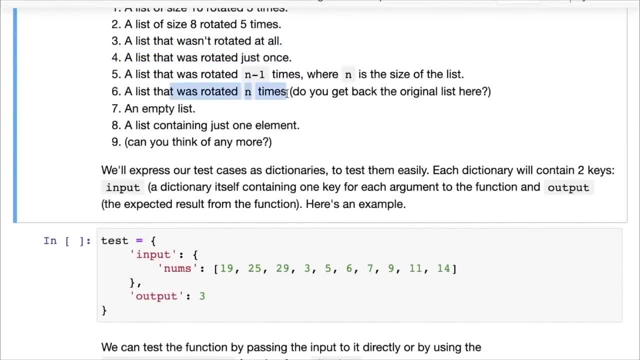 N is the size of the list, a list that was rotated N times. And what do you mean by rotating the list N times? Well, let's see an empty list and a list containing just one element, And if you can think of more test cases, 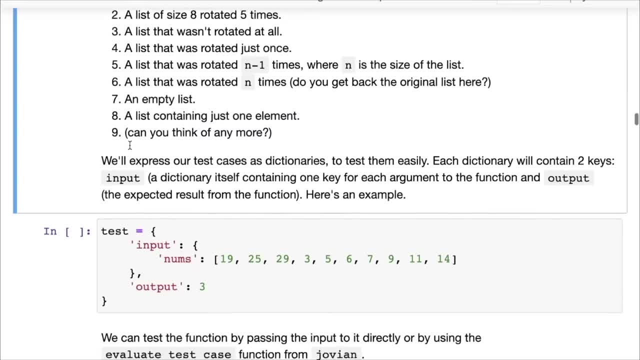 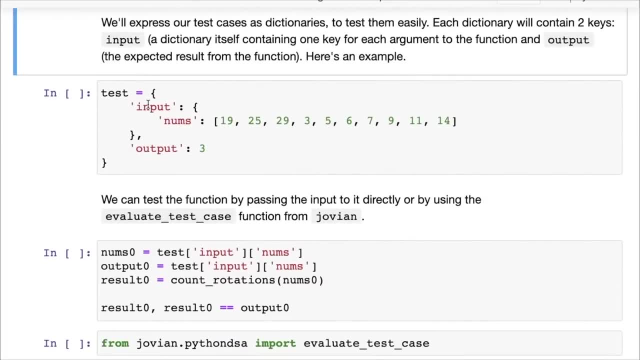 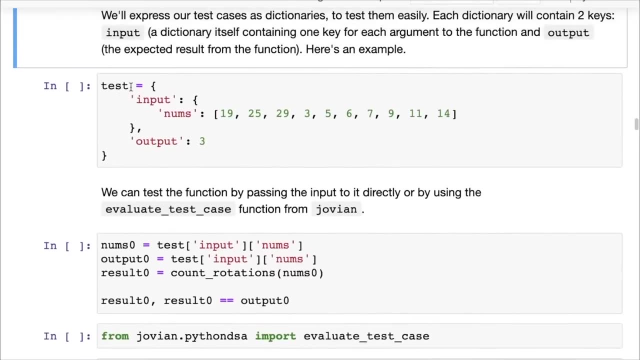 You should definitely add more test cases here, And what we'll do is we will express our test cases as dictionaries. So this will help us organize the test cases and test them all at once more easily using helper functions. So you can see here that we've organized one test case here and we've 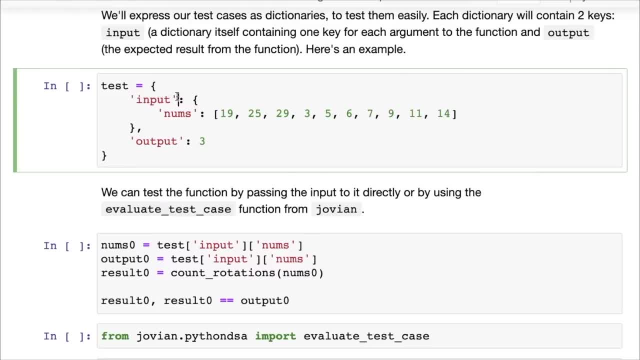 expressed the test case as a dictionary. So here we have the input to the test case, that is the input key, And then we have the output to the test case. Now, because A function Can take many arguments, The input itself is going to be a dictionary. 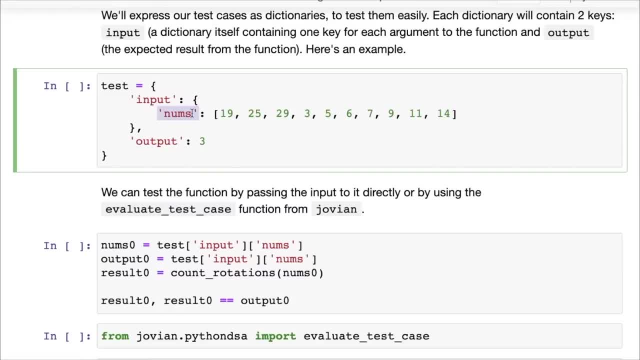 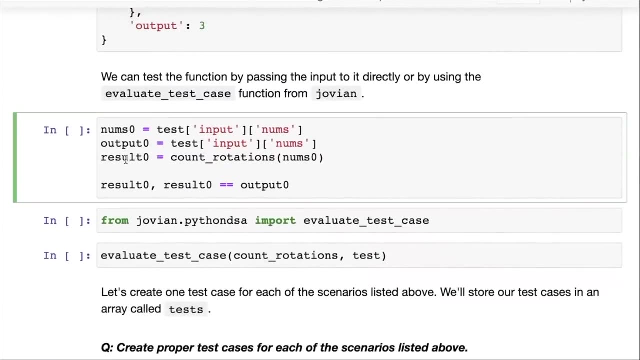 And then for each argument. in this case there's just one, So we just call it nums. We have the input here and this is the size of the output. Okay, So let's create this test case and let us then, if you want, to fetch the. 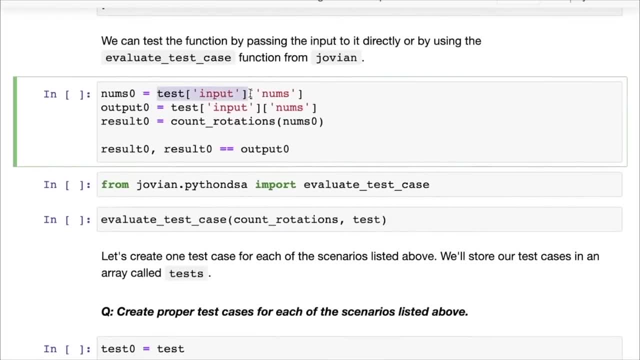 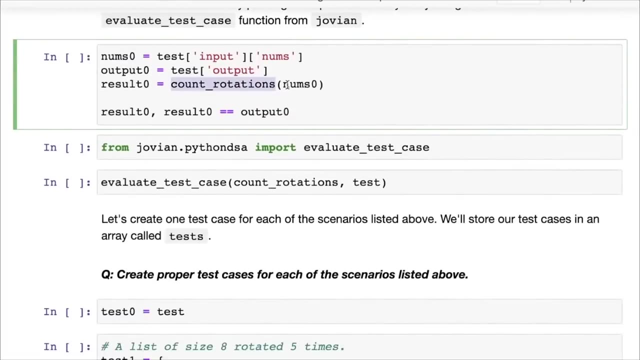 actual input and output out of it. So here we can fetch best input Nums. that's going to give us the nums. We can use test input. The output should be best outputs. This seems to be an edit and the result is: count rotations num zero. 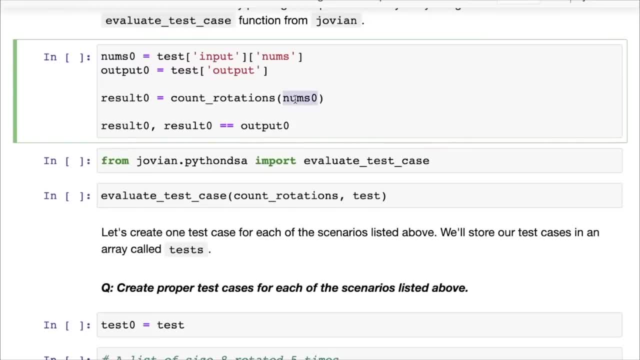 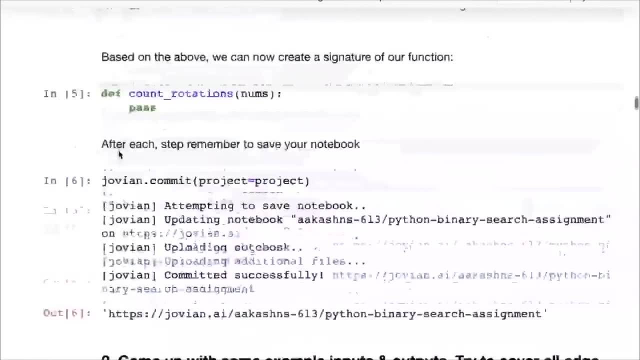 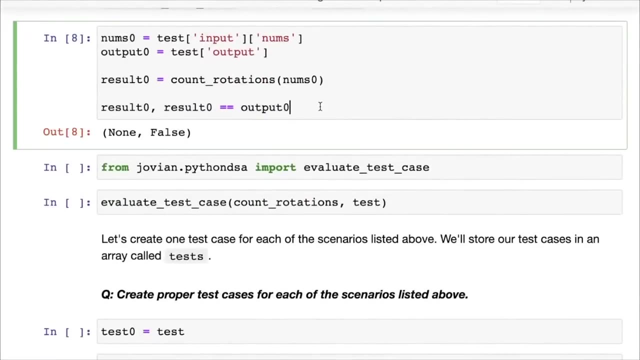 Okay. So this is the actual result obtained by passing the test case into count rotations, And you can see that the result we get back is none, because right now we do not have any code. We just as pass inside, Okay, And the result and the output are not equal, because the output is the 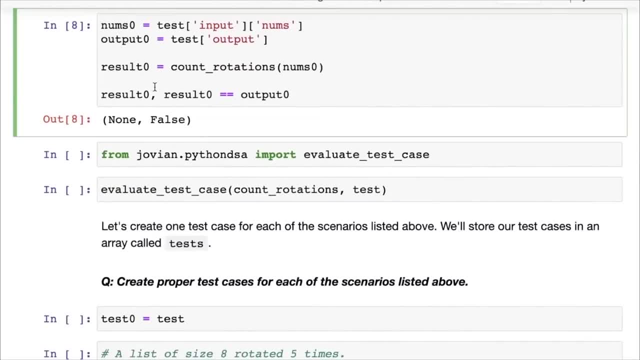 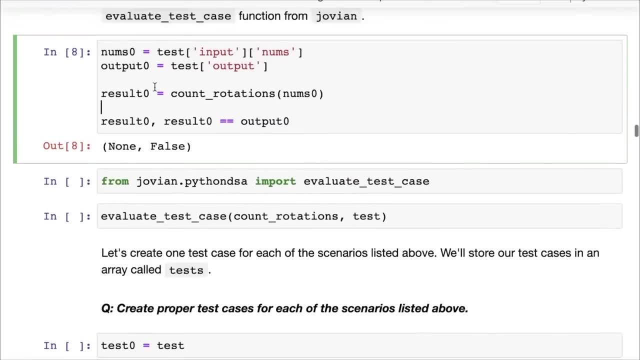 number three, but the result is none. So that's okay. Our test case is failing right now because we have not yet implemented the function, But as soon as we implemented, we expect to see the test case passing. now, to help you avoid all of this work, we have given you a function called evaluate test case. 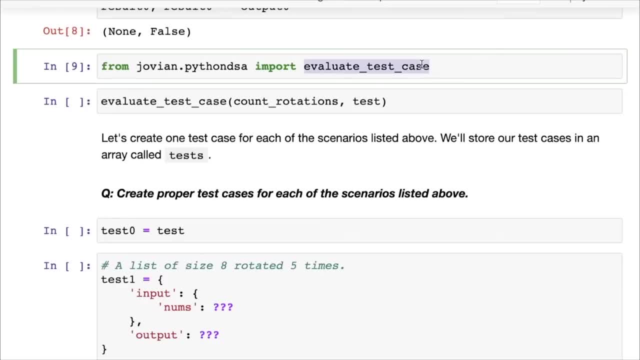 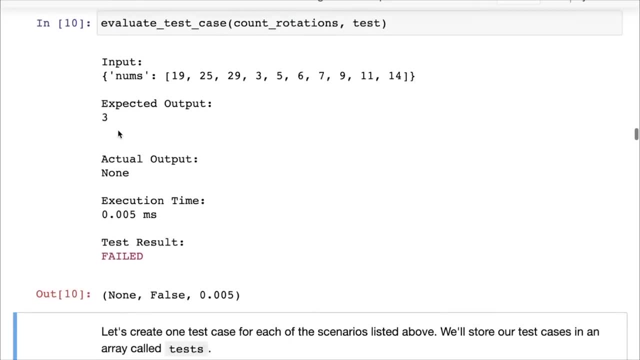 So from Jovian or Python DSA you can just import evaluate test case and then call evaluate test case with the function you want to test And the actual test case and you can see here it prints the out input that was passed in the expected. 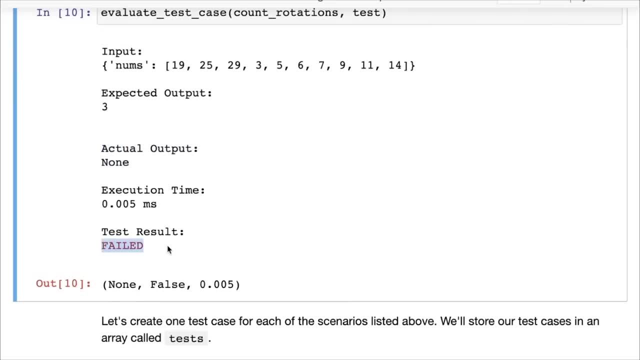 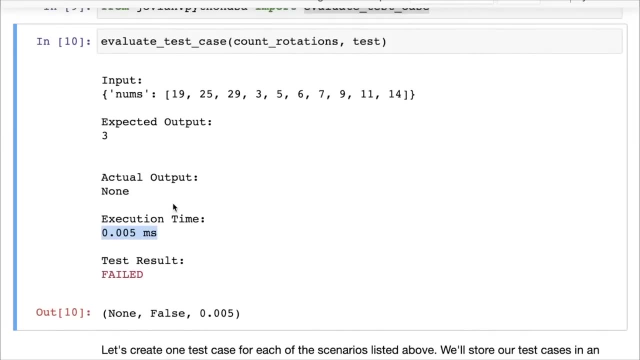 output: the actual output that was obtained and the test result. in this case, a test result was failed, And the execution time is also printed here, If you just want to evaluate if a certain implementation is faster than another. so now your job is to 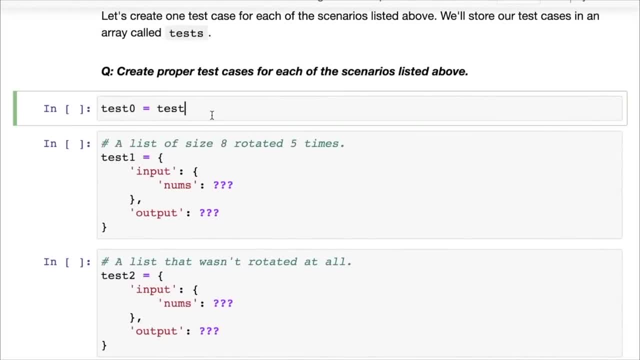 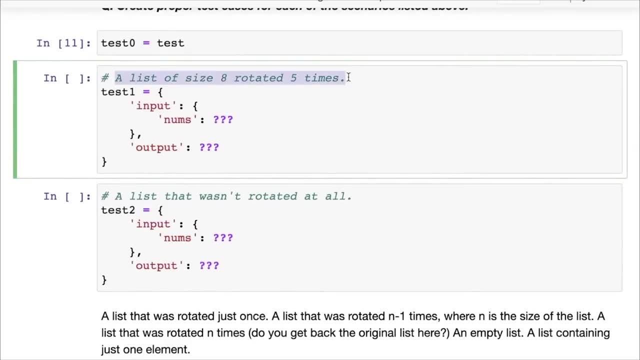 create test cases for each of the scenarios listed above. So here is test zero. That is same as The original test case that we had created. here is test one: a size, a list of size: eight rotated five times. I will let you create this, but it will look something like this: 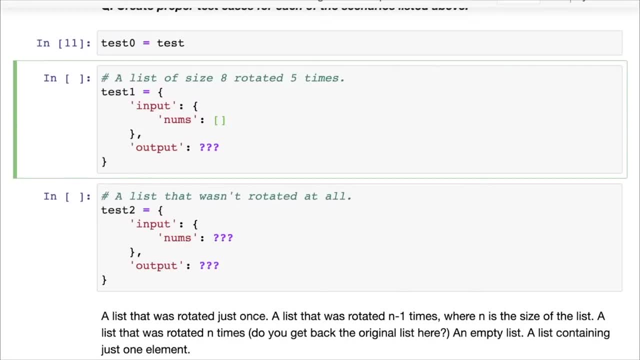 You will open up, you'll replace the three question marks with, let's say, a list of size eight. So one, two, three, four, five, six, seven, eight, And you can imagine that this was rotated five times. 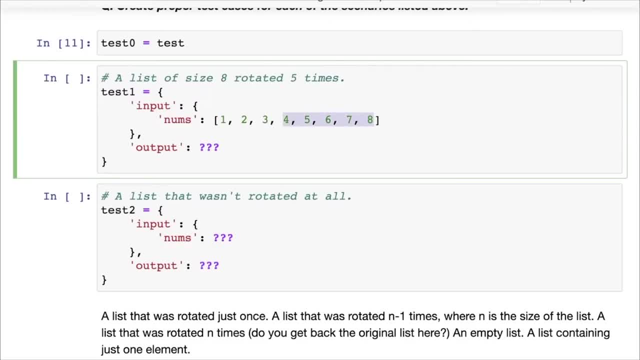 Then one, two, three, four, five or five of these numbers will then move to the first position And you get this as the input numbers and the output. Well, it was rotated five times, So I think you can guess that the output here should be five. 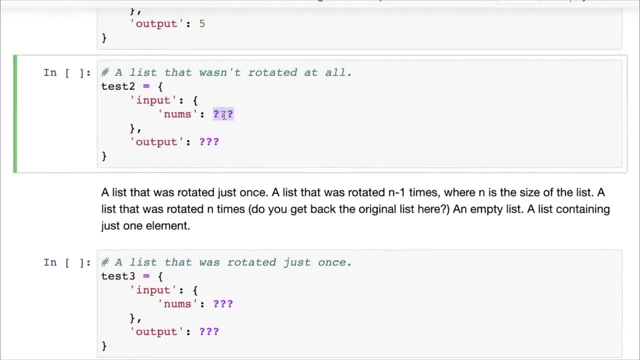 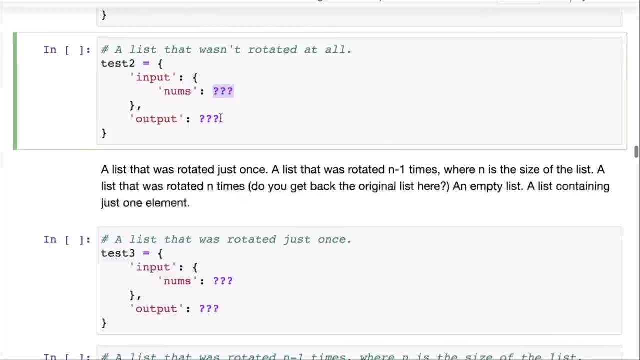 Now here is a list that wasn't rotated at all. What should be the output here? I'm sure you can guess that the output here should be zero, So I let you fill this out. Here is a list that was rotated just once. 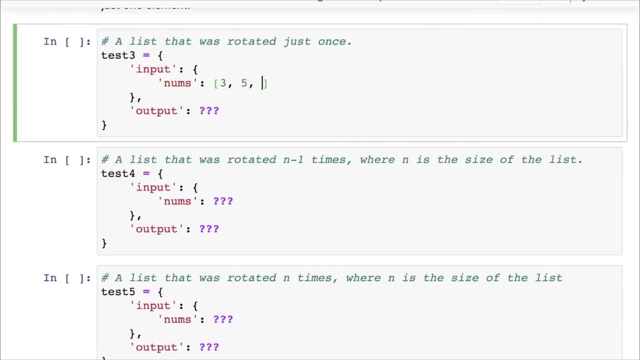 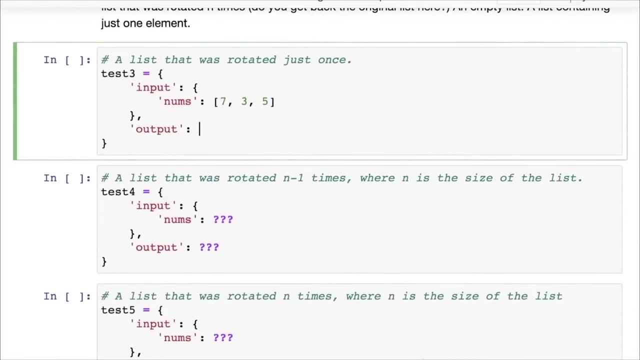 So let's try, Let's fill, Not this one. So this, this list, rotated once, would give us seven, three, five. There you go, A list that was rotated N minus one times, where N is the size of the list. 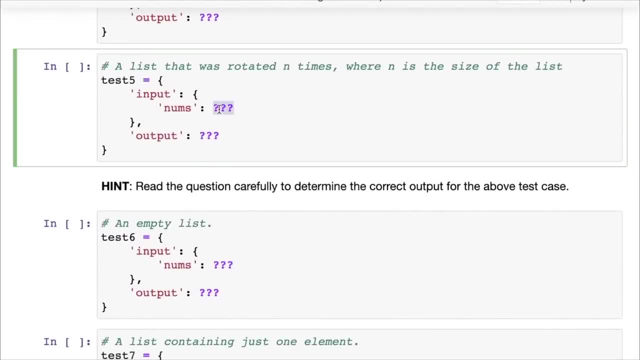 Okay, I'll let you do that. A list that was rotated N times, where N is the size of the list. Okay, What does that look like? So you take this list and then you first put 10 in the first position and then you put nine in the first position. 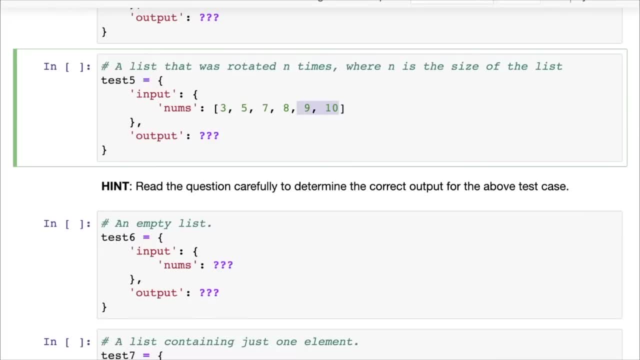 So nine, 10 comes to the beginning and three, five, seven, eight comes after it. Then you move eight to the first position, Then you move seven, Then you move five, Then you move three. If you, if you move all of these back to the first position, you end up with the same list. 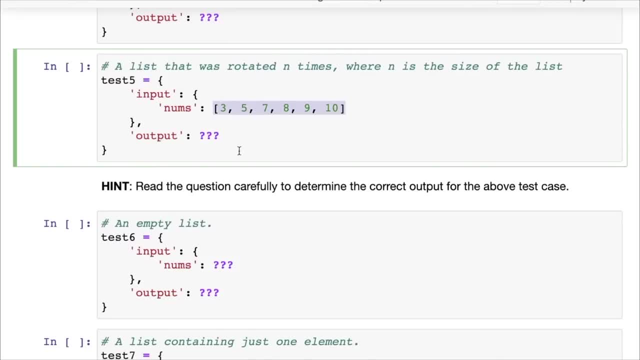 So you've rotated it N times. Now what should be the output in this case? There are about six numbers here, So is the output six? I don't know. I'm not so sure because remember the question. the original question says: 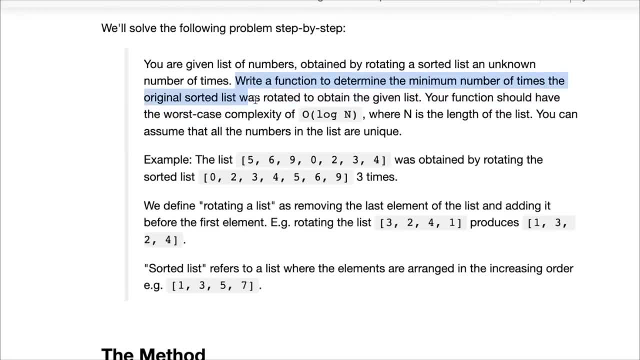 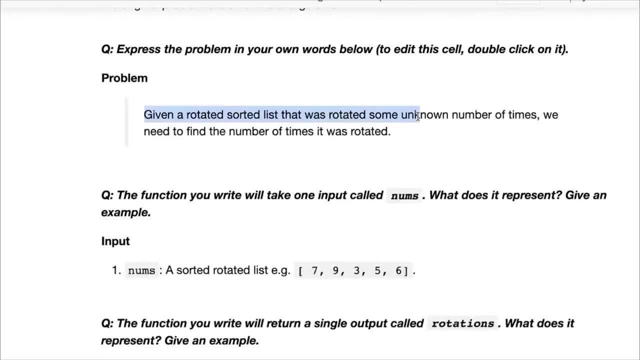 write a function to determine the minimum number of times. the original sorted list was rotated to obtain the given list, So it has to be the minimum number of times. We may want to just go back and change this. We need to find, not the number of times. 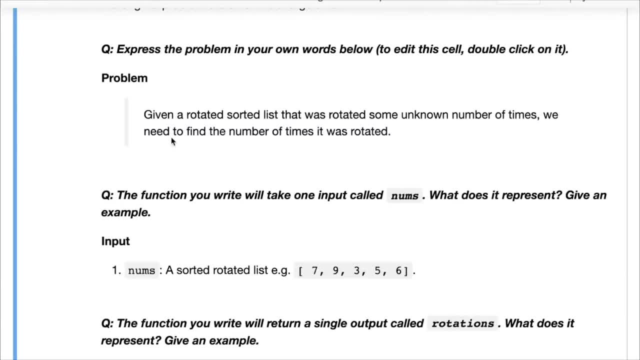 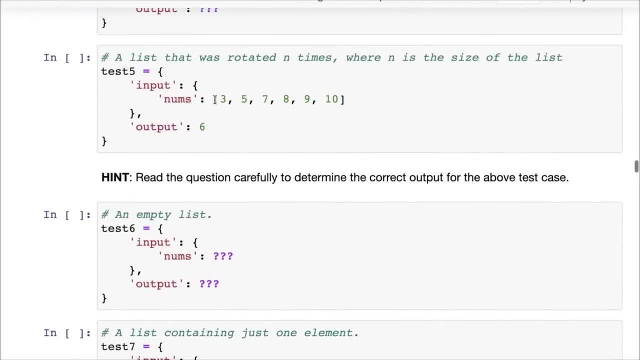 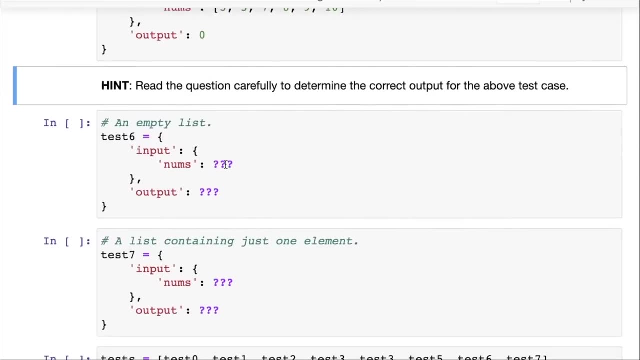 It Was rotated, but the minimum number of times it was rotated or it needs to be rotated right. So, coming back here, the output should be not six but zero, So keep that in mind. Then here's an empty list. 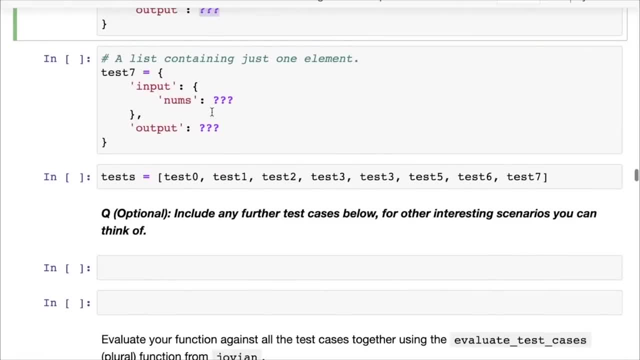 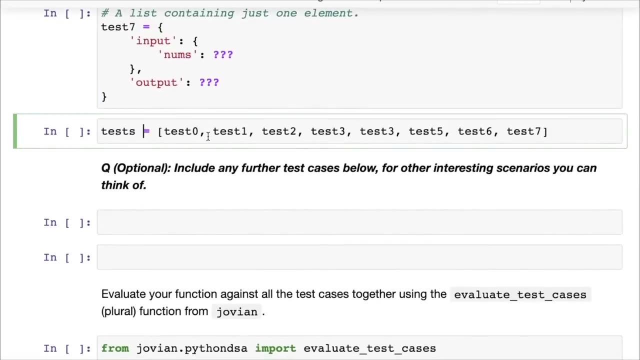 I let you figure out what should be the nums and the output here, And here is a list containing just one element. Once again should be pretty straightforward. Can you rotate a list With one element? I let you decide, and then we are taking all the tests and putting them into a single list. 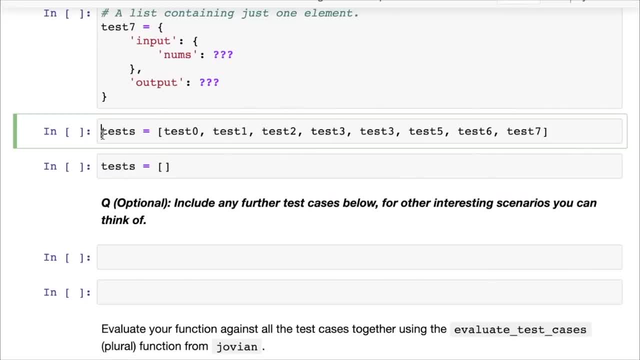 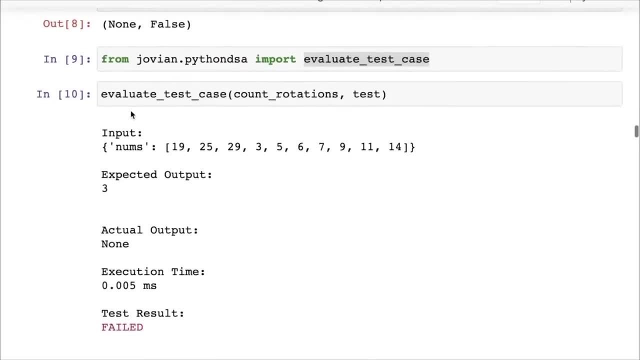 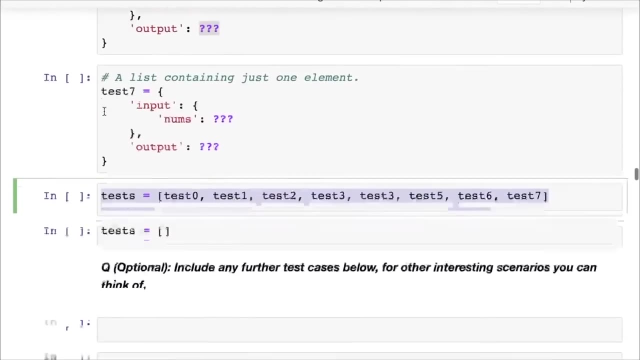 Now, since I have not defined all the tests, I am not going to use this definition, which contains all the tests, but I'm just going to pick the number of tests that I have defined. So we have defined here: test zero, test one, test three, test five. 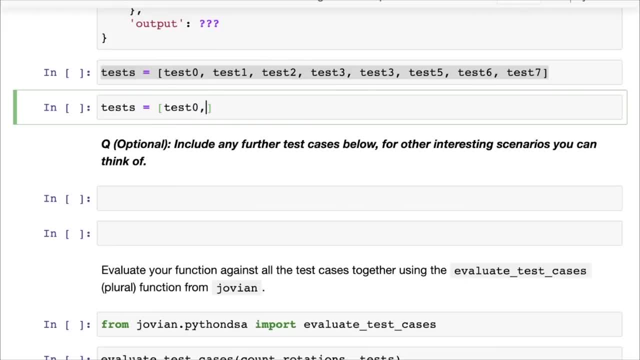 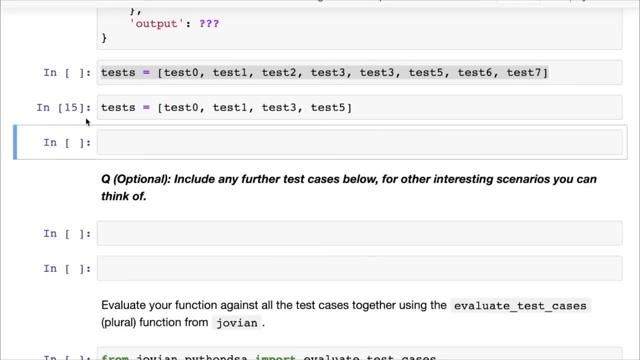 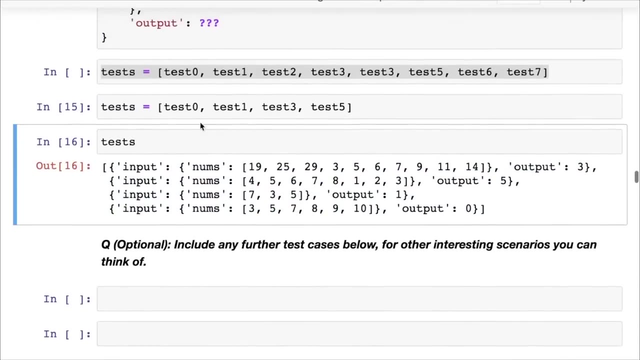 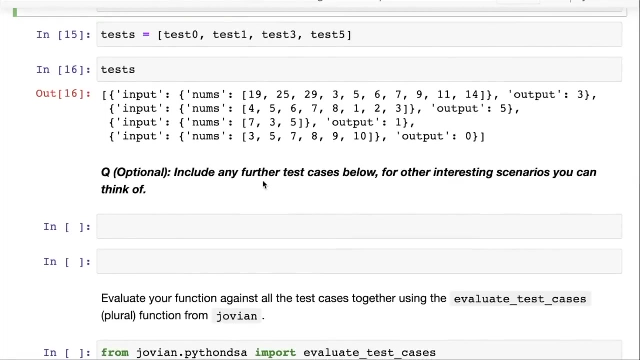 I'm just going to put in, And that's the full set of tests that we have. You definitely need to fill out all the test cases And if you can think of some other cases that you should be testing, and you should include those test cases here as well. 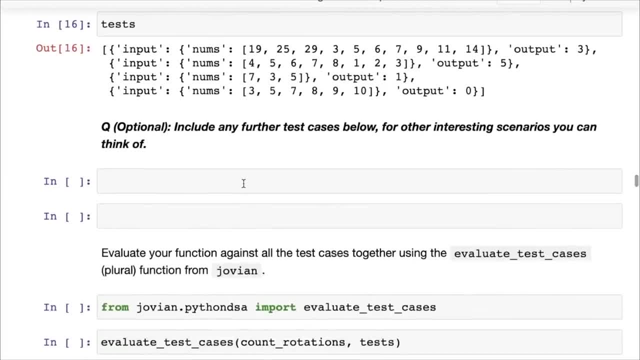 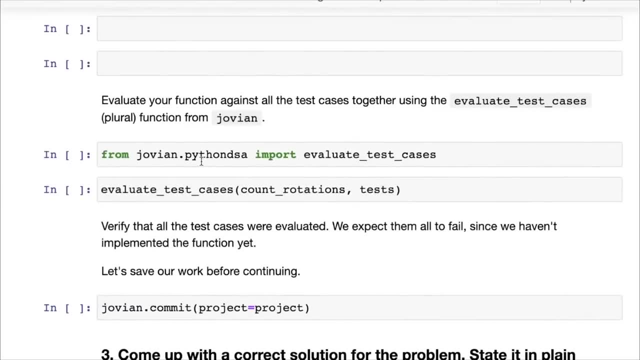 Okay, Now to evaluate your function against all the test cases together, you can use the evaluate test cases helper function from Jovian. So there are two functions: evaluate test case works with a single test case and evaluate test cases works with a list of test cases. 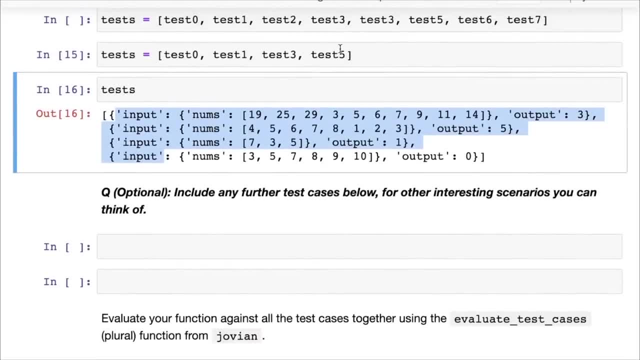 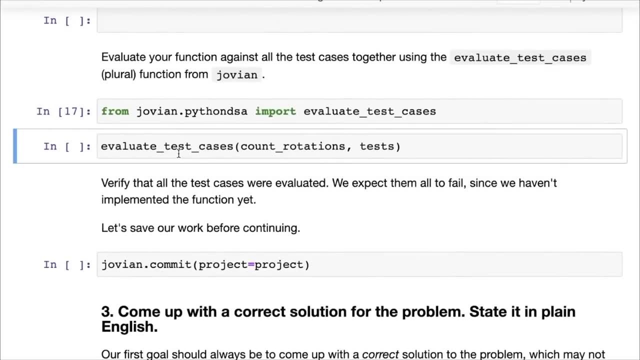 So we have a list of test cases here. I have four, but you should have about eight at least, And a few more if you've created them, So we can import from Jovianpython DSA evaluate test cases and then invoke evaluate test cases with the count rotations function. 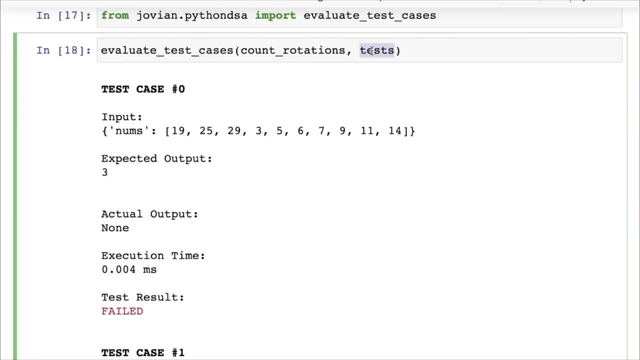 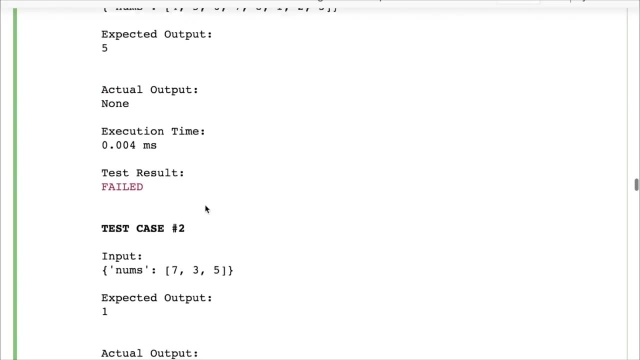 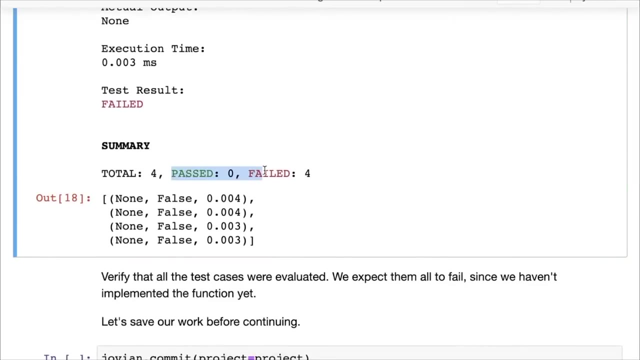 Still we don't have any logic in the function. So we all the test cases should pass and the list of test cases we've created. So you can see test cases: zero fails, one fails, two fails, three fails. So out of the four test cases, none of them have passed. 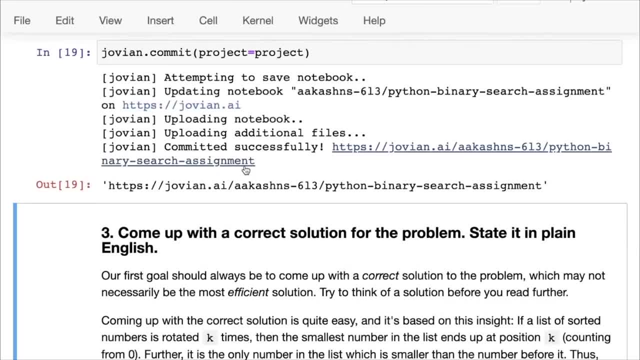 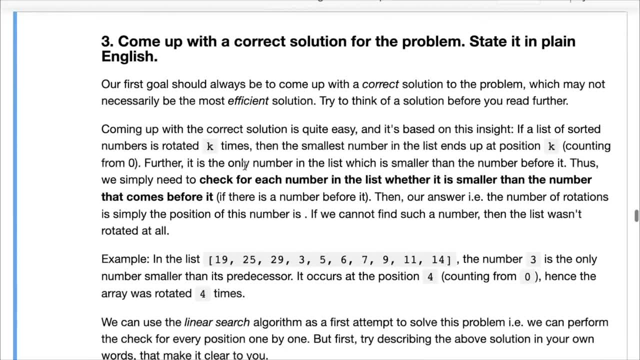 No problem, We have completed step two, which is to create some test cases, And we'll know, once we've defined a function, whether the function definition is correct. Now the next step is to come up with a correct solution for the problem and stated in plain English. 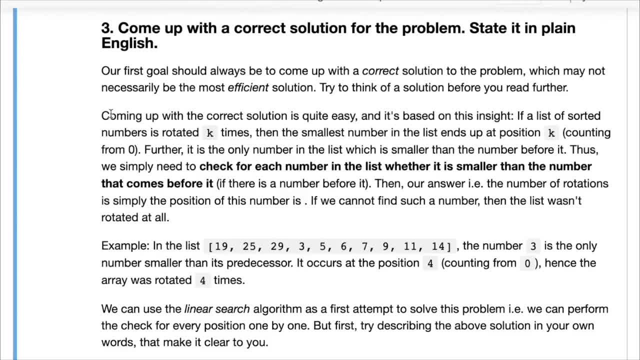 And there's a hint here for you already, coming up with the correct solution is quite easy, And it's based on this simple insight. If a list of sorted numbers is rotated K times, so you keep rotating it step by step, moving the last number. 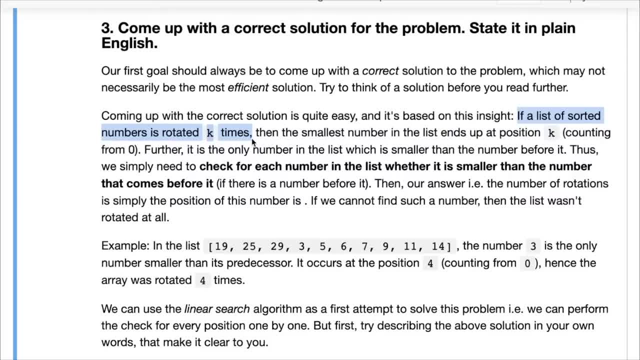 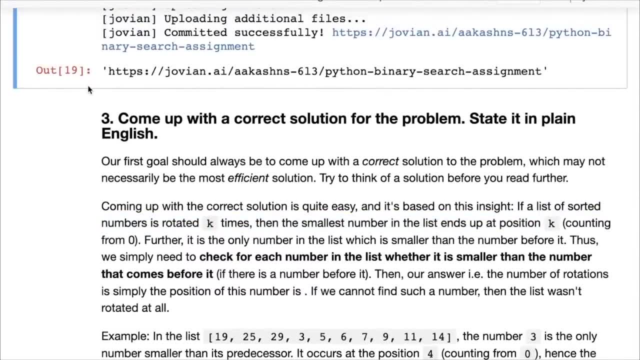 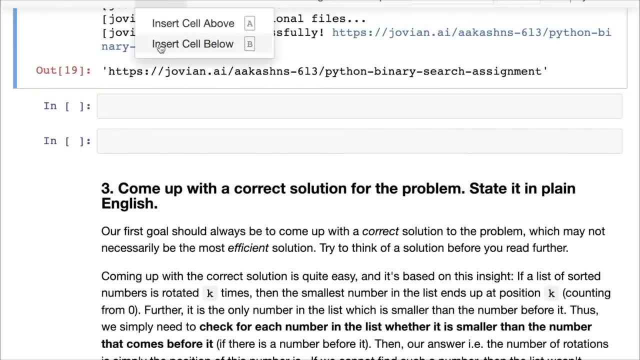 To the first position. then the smallest number in the list ends up at position K And you can verify this. It's very simple to do this. Whenever you have a doubt, just create a new cell. By the way, you can create a new cell by clicking on the left side of a cell and clicking insert cell below. 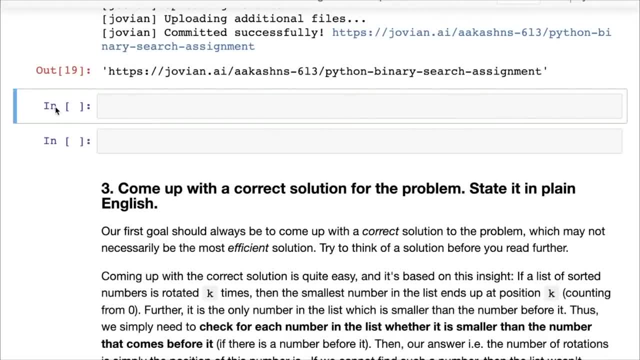 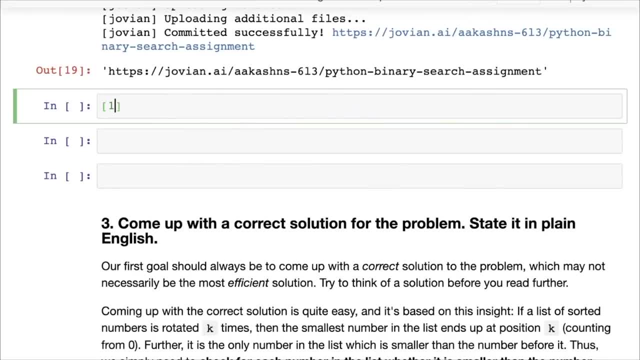 Or if you're in a code cell, just click here near the prompt and press the B character And that adds a new cell below. So let's take the list 1,, 3,, 5,, 7,, 5,, 6,, 7, and let's rotate it K times. 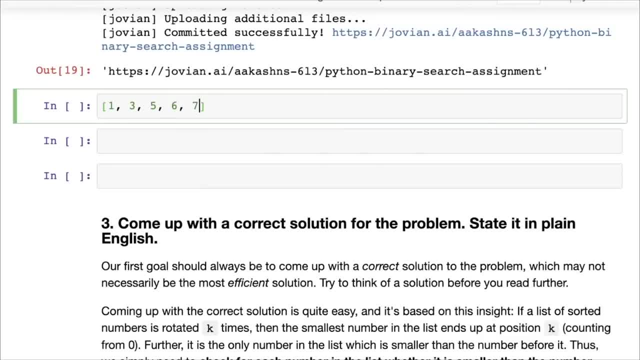 Let's try with: K equals two. So if you said K equal to two, then you're going to take two of these numbers from the very end and move them to the beginning. So that means zero comes at position six, comes at position zero, seven comes at position one and the starting element in the sorted list now comes at position two. 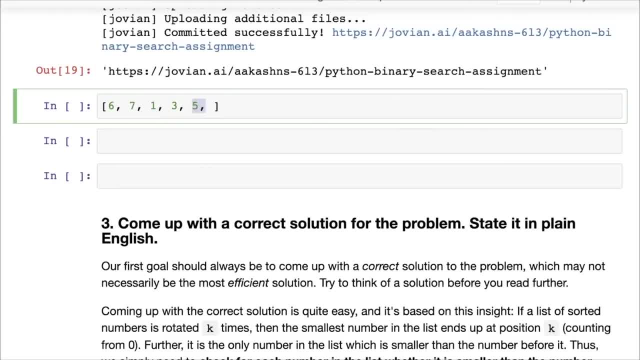 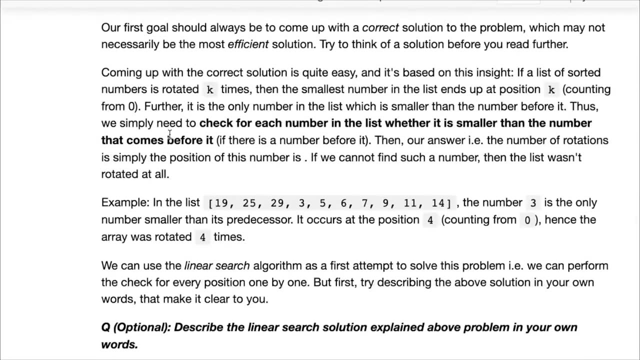 That's interesting. Let's move the third element as well. Okay, So now we've moved three elements or rotated the list three times, and the smallest element ends up at position three. So it seems to hold true and you can verify this now with a larger list, smaller list, empty list and all the test cases that you have. 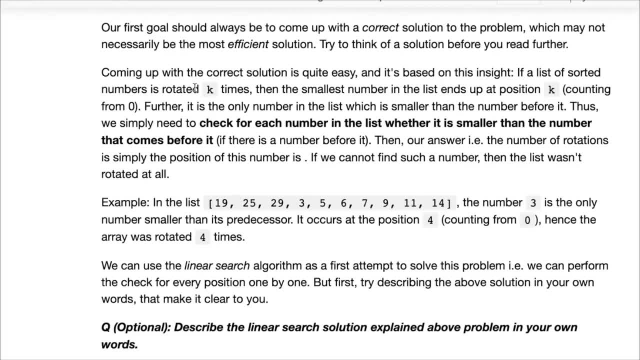 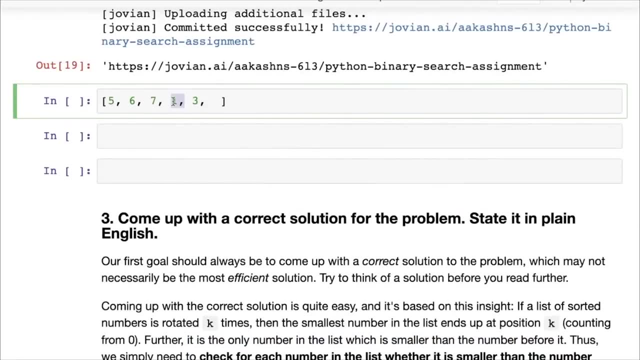 And if a list was sorted K times, sorted list was rotated K times, then the smallest number in the list ends up at position K, counting from zero, Whether it is the only number in the list which is smaller than the number before it, And you can see this once again- the smallest number is at position three and all of these numbers are higher than the numbers that come before them, except the number one which is smaller than seven. 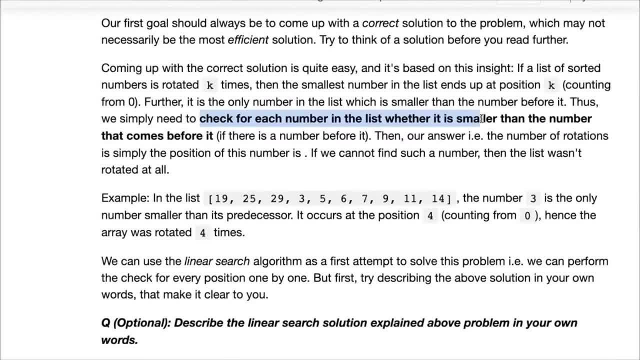 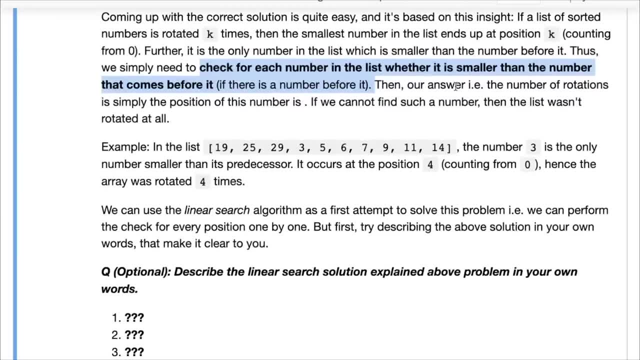 So we simply need to check for each number in the list whether it is smaller than the number that comes before it. If there is a number before it, Then our answer is simply: which is the number of rotations? is simply the position of this number right? 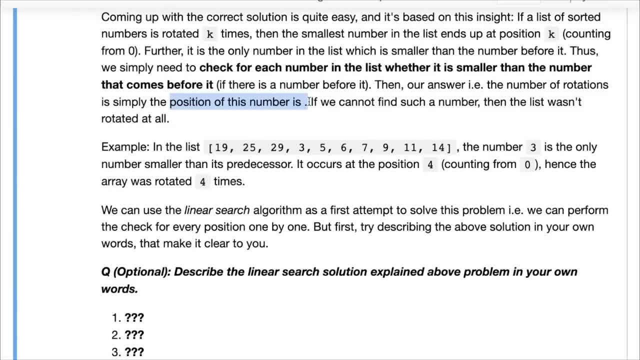 So if you can find the position of the number which is smaller than the number that comes before it, the position of the number is also equal to the number of times the sorted list was rotated, And if we cannot find such a number, then the list wasn't rotated at all. 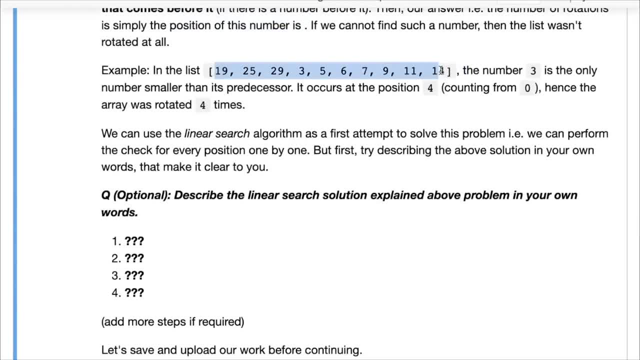 And that's it. You can see here, in this list, now, applying this logic, three is the number, the smallest number. And not only that, three is the only number which is lower than the number that precedes it, the predecessor, which is 29.. 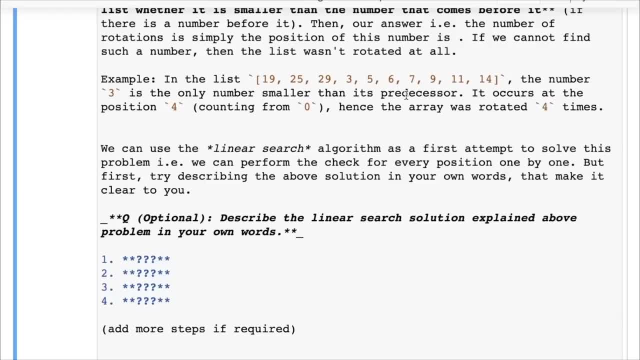 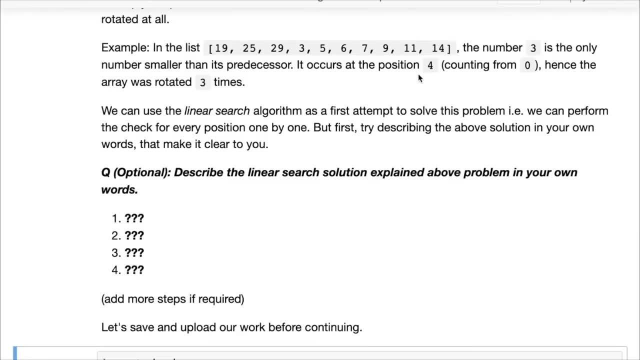 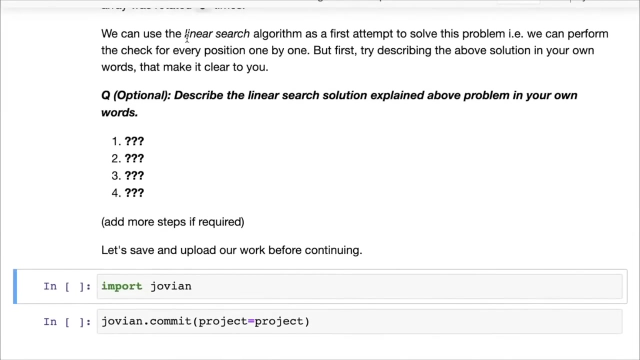 And since three occurs at position four, well, actually three occurs at position three. zero, one, two, three- The list was rotated exactly three times. Now We can use the linear search algorithm as a first attempt to solve this problem. 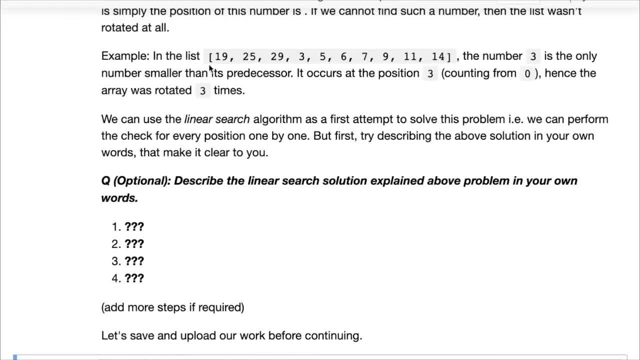 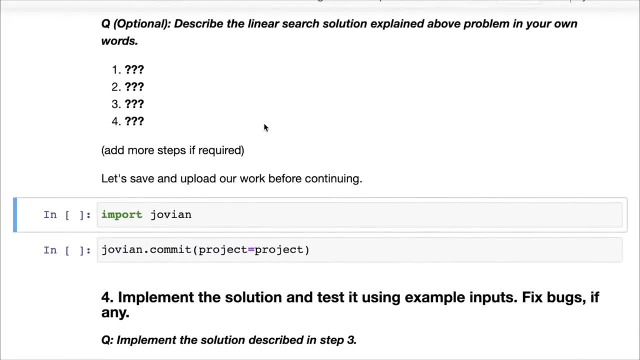 And the linear search simply involves working through this list, walking through this list from the left to the right. So now the task for you is to describe the linear search solution in your own words, and please write it in your own words, but here's how I'm going to write it. 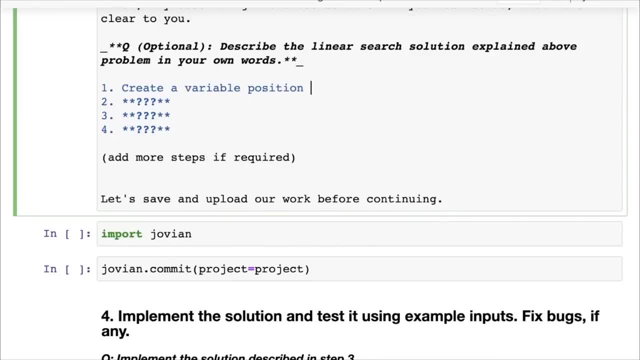 Let's say, create a variable position with value zero. So this is the Position for tracking this. for tracking the position, then look at the number at the given position and not only look at it but compare the number at the- let's say, the current position to the number before it. now, if you're starting position with the value zero, maybe 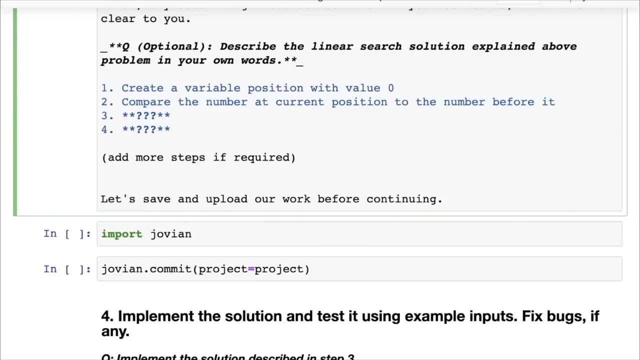 We may not. there's no number before it, So we may not be able to compare it with something. We may even just start with the value one. That's all right. If the number is Smaller than it's breed is Cesar, then return position, because position is the answer. 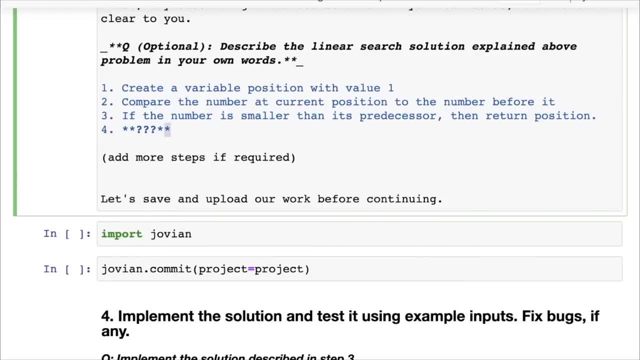 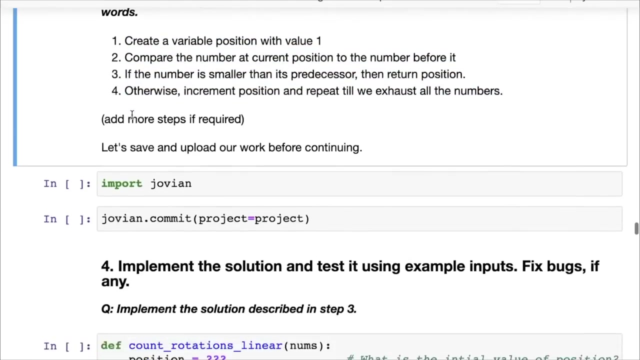 We found the number that is smaller than its predecessor. There's only one such number. Otherwise, increment position and repeat till we exhaust all the numbers. Okay, Simple, You can add more steps. If your Description of the algorithm requires more steps, that's perfectly. 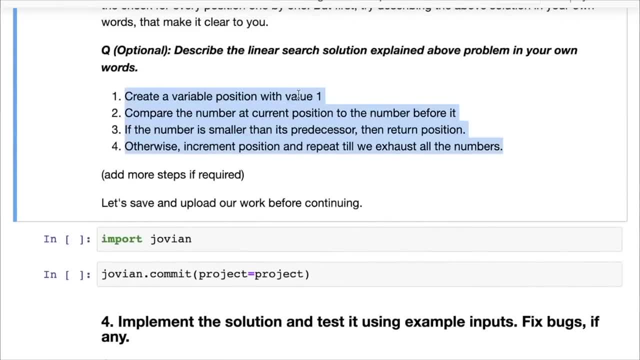 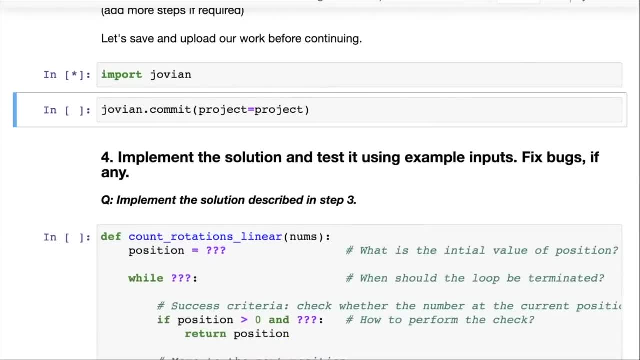 All right, we have a very clear description of the solution Now we're starting with. the position is one, not zero, because we also want to track the previous position. Now we import Jovian here and commit our project once again and keep saving your. 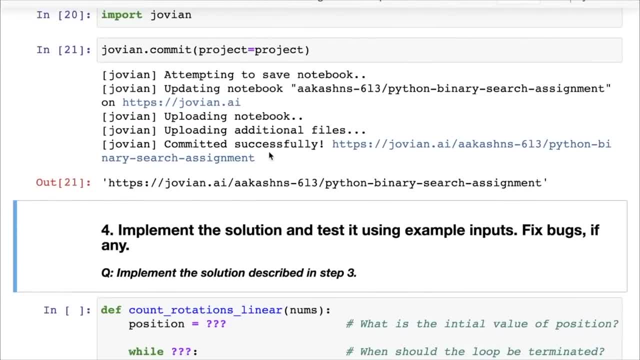 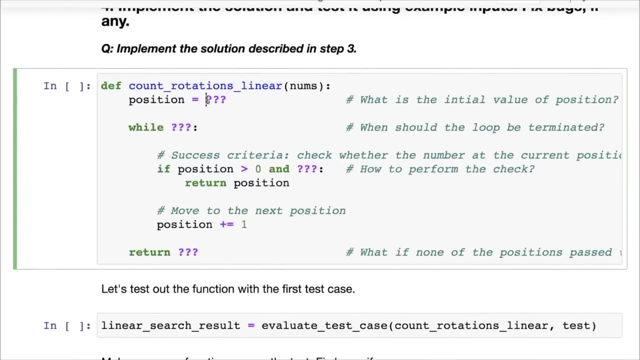 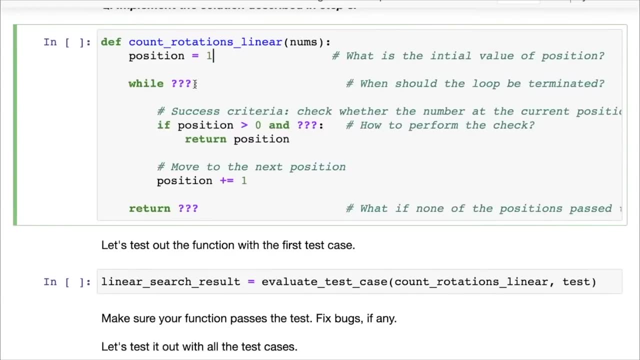 work after every step so that you can continue your work. So now we're talking about implementing the solution and testing it. So let's implement the solution. We said that we want to start with position. We want to start with position one, and while, when should the loop be terminated? 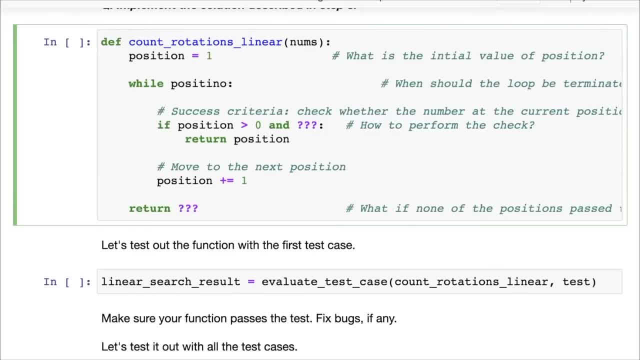 Well, while position is less than the len of nums, I guess that's fair. And then, what is the success criteria? So we have: if position greater than zero and nums of position less than nums of position minus one, Okay, So that's a success criteria here. 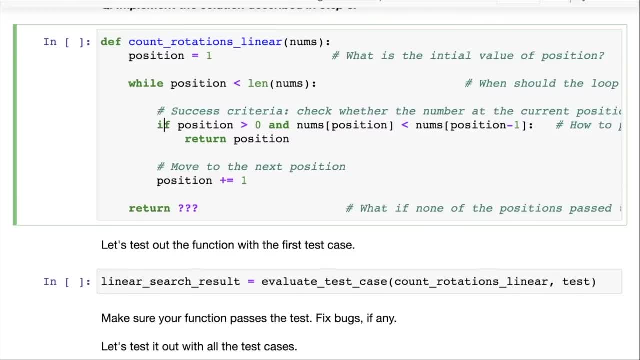 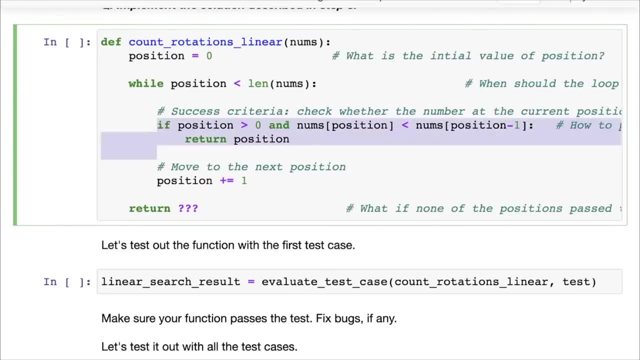 We can start position at zero as well, And all that will happen is this: condition will get skipped and position will get incremented. And this is a good practice, because whenever you iterate over the list, you normally just want to start with zero, just to avoid any confusion later. 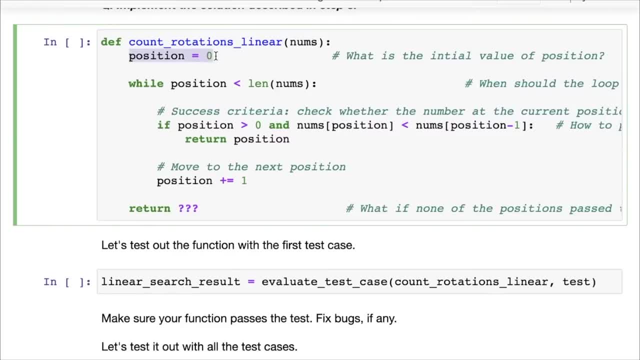 When you're reading the code that did you intend to write zero here, or one, et cetera, et cetera? So just put in position equals zero here and simply skip the check here, or simply skip this comparison if position is not valid right. 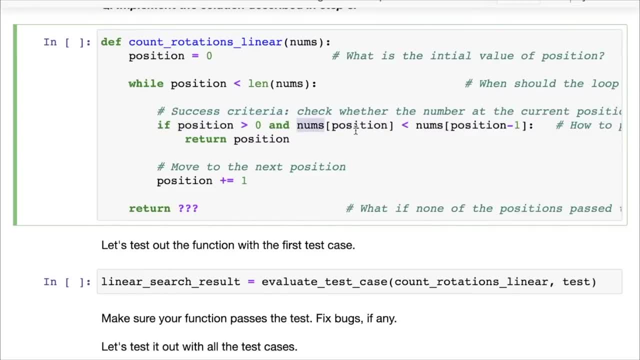 So whenever you're accessing an element from inside a list or inside a dictionary, you always want to make sure that that index or that key is valid. Okay, Here we are making sure that the key position minus one is valid by checking position greater than zero. 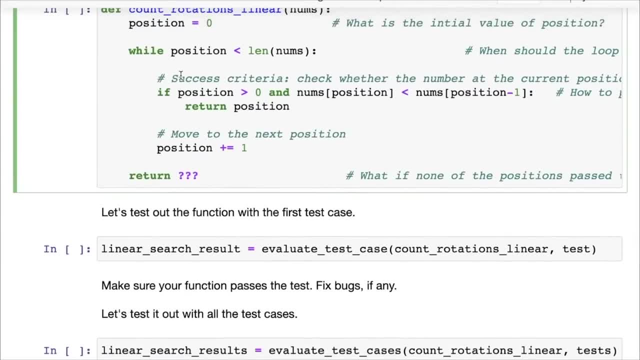 In any case, we now have the logic And, finally, we are saying that if the number at position is less than the number that comes before it, then we return that and that's just going to. if it's not, then it's going to increment the position and it's going to check. 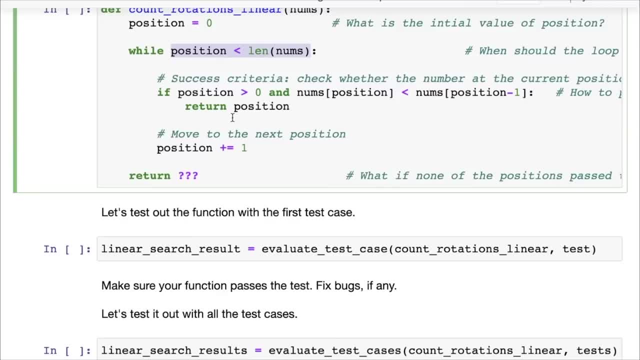 again, and again, and again, till we run out of numbers. Now, if you've exhausted the entire list, then it follows that there were no rotations or they were end rotations, exactly. in either case, the number we return should be zero. Okay. 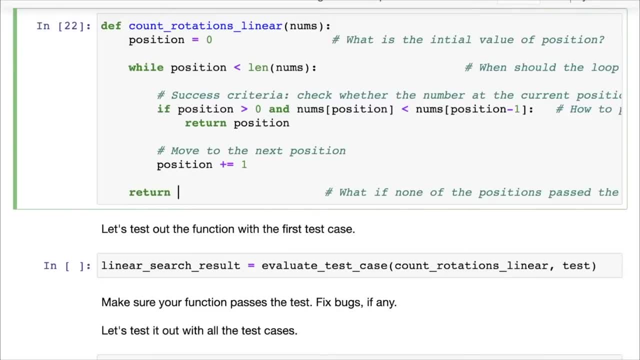 So keep this in mind. The sum: you may have the doubt: should you be returning minus one here or should you be returning zero here? Well, the question does specify clearly that you are given a sorted, rotated list and you have to find the number of times it was rotated. 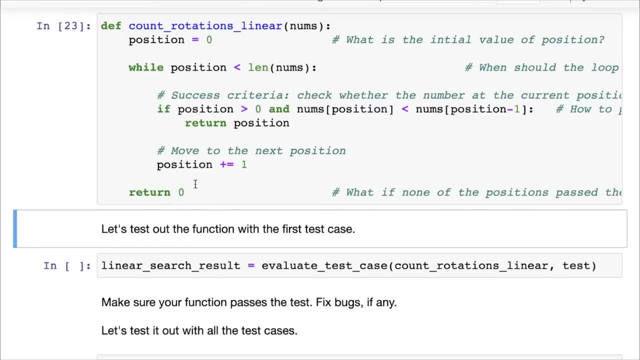 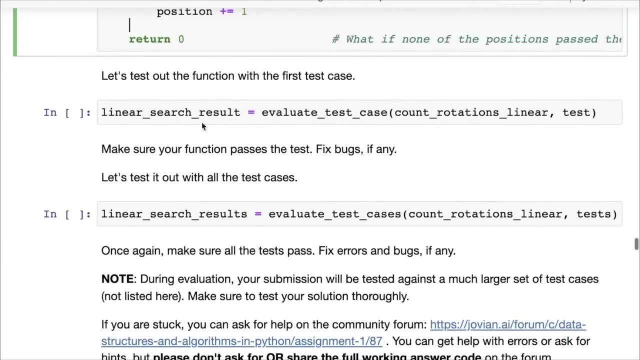 Now, obviously minus one rotations are not possible, So minus one would not be a valid return value from your function, And this is the reason we write test cases too. Now let's evaluate. So let's call evaluate test case for a single test case on count rotations linear. 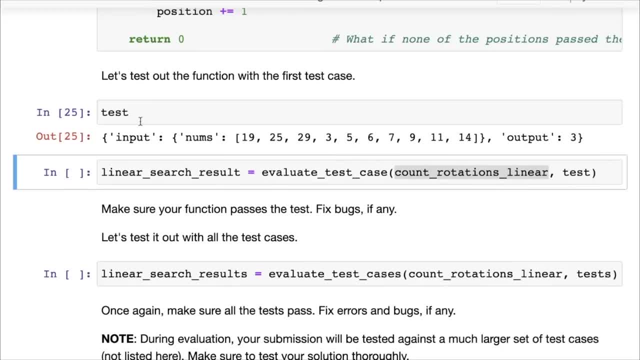 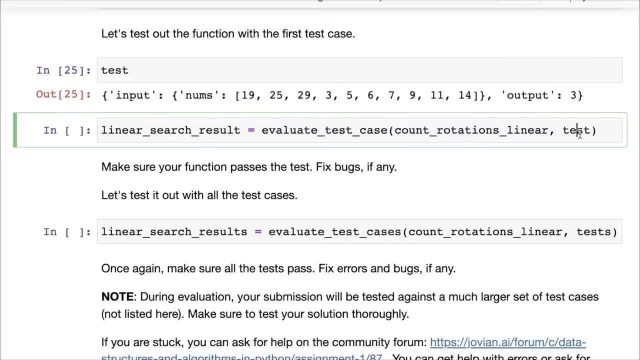 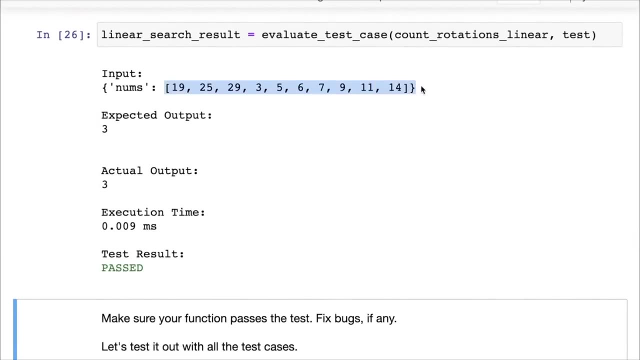 and let's see what the test case is. This is the test case here and this is the output. we call evaluate test case with count rotations, linear and test, and that gives us a linear search result. You can see here. this was the number, the list of numbers. 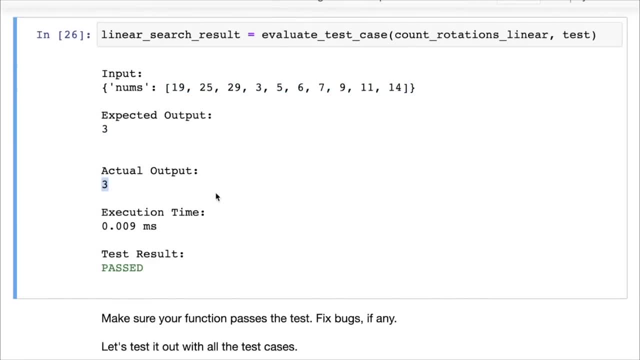 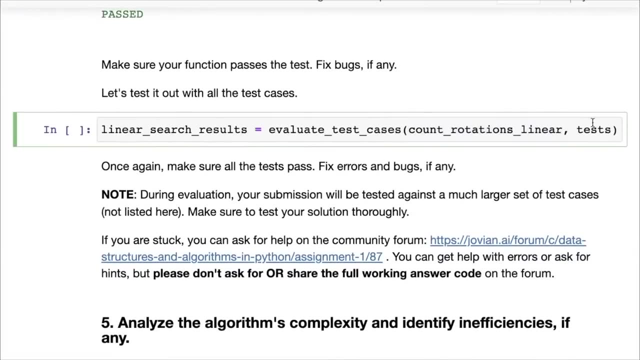 This was the expected output and this was the actual output, So great Our function seems to have passed the test case. Now we can evaluate all the test cases by calling count rotations linear on all the test cases together and give. that gives us a whole list of test results: test case zero and. 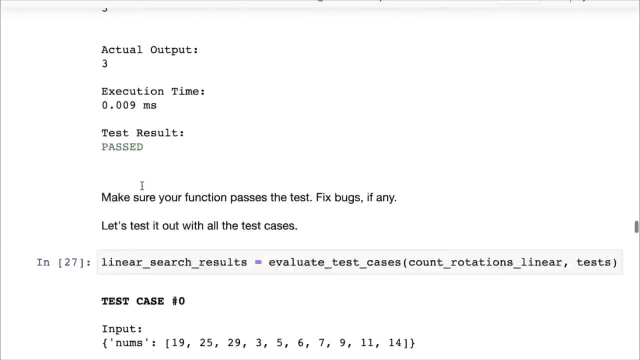 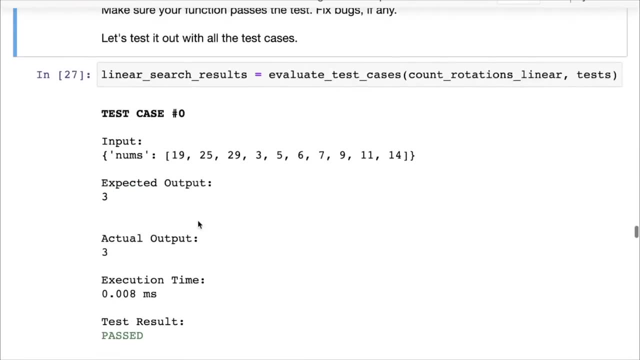 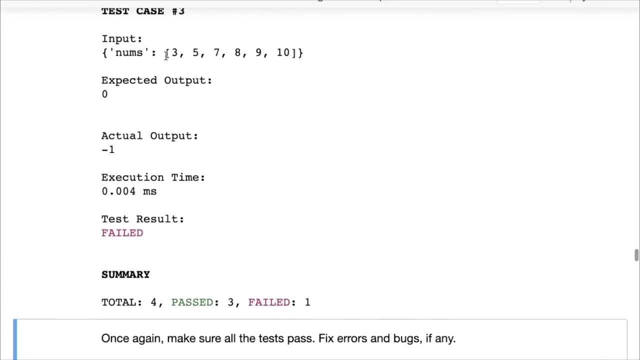 one and two and three. all of them have passed. Now, if you had put in minus one here, you would see that one of the test cases would fail, which is the case where the list wasn't rotated at all or was rotated end times. 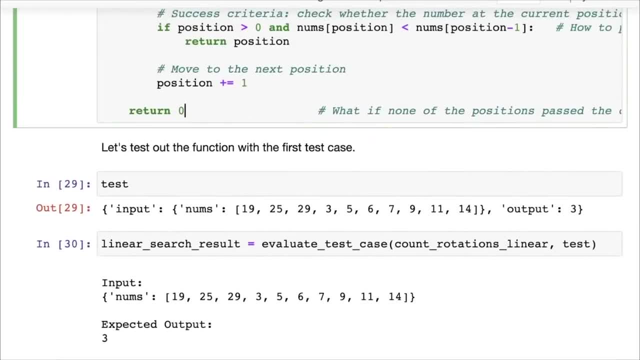 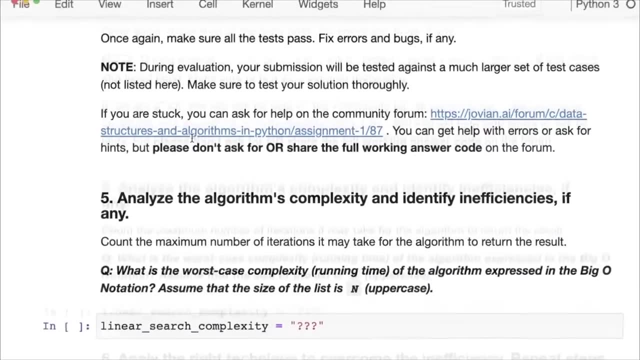 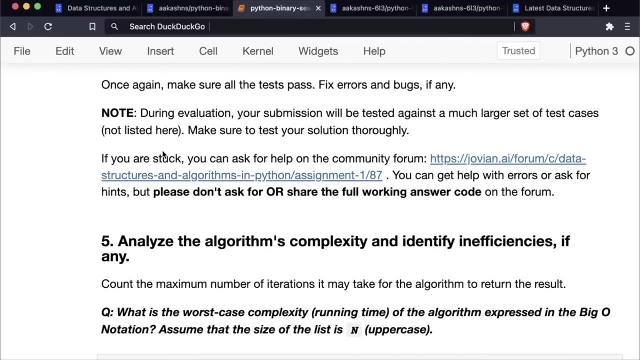 So that should tell you that the answer here should be zero. So that's our linear search algorithm, And at this point you may face issues, You may feel stuck, You may not be able to figure out how to write the code, and that's perfectly all right. 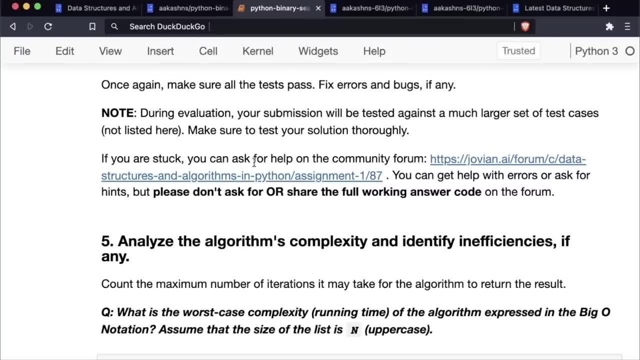 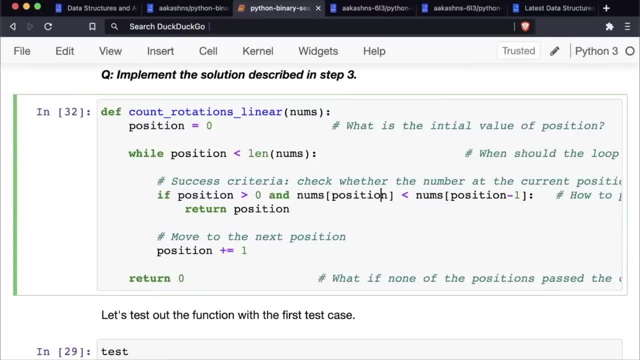 That's part of learning. You may face errors, You may face exceptions. For instance, if you did not have this check here- position greater than zero, or maybe what you had here was some other condition, like position less than equals, position plus one. 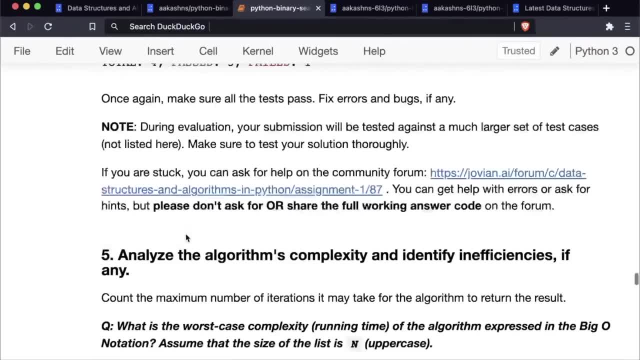 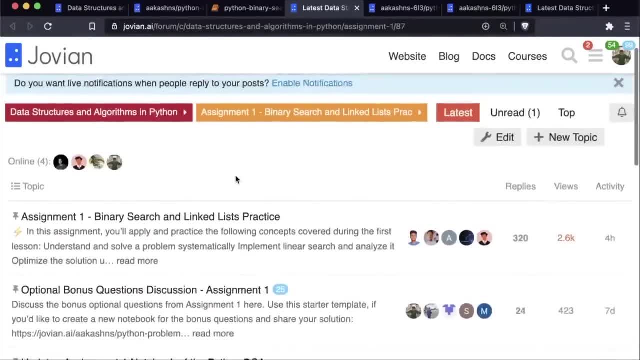 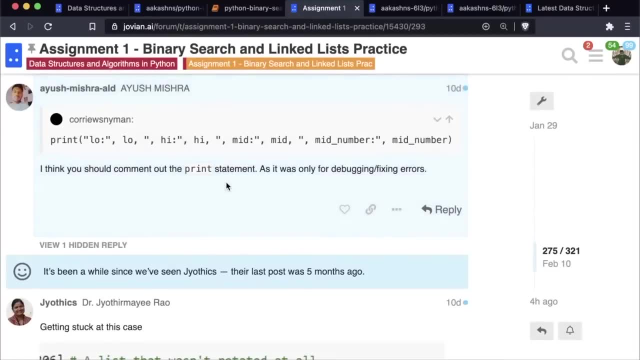 And that's okay. Then you can go to the forum and post your issue. So let's open up the forum here. This is the Forum discussion for assignment one, and you can go into the original topic here, which is a longer discussion. 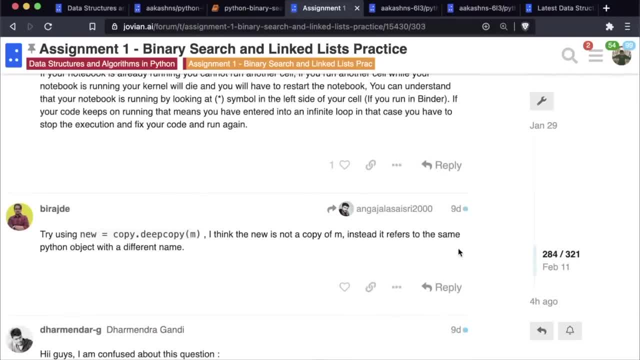 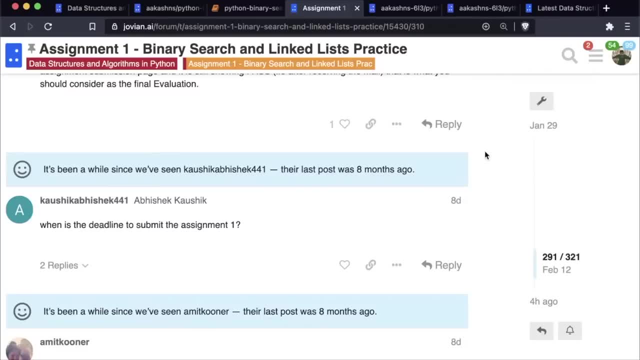 So this is where everybody's posting small issues. So you can see that there's about 321 messages that have been posted. You can start looking through this forum. You can start reading through some of the posts. You can even search if you press control F, and you can even search for questions here. 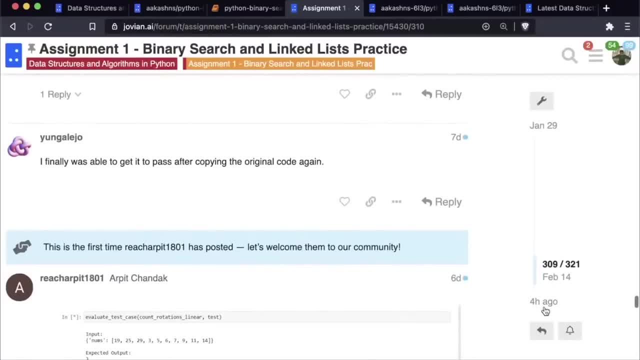 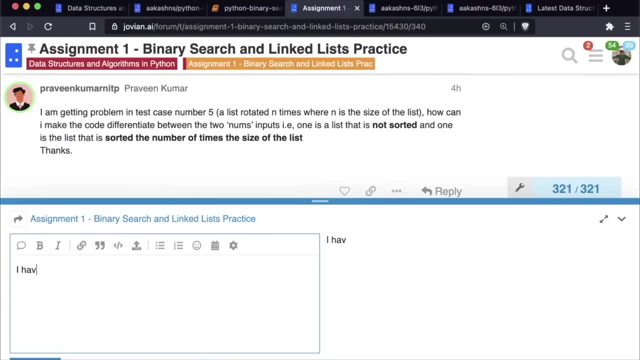 Now, if you want to post your own question, scroll down to the Very end, or you can just click this button here and click reply Okay And mention your question here. I have a an issue. Should I return minus one or zero? in the case the list has not been rotated. 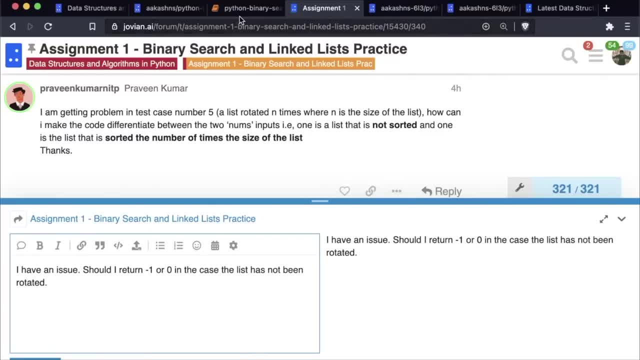 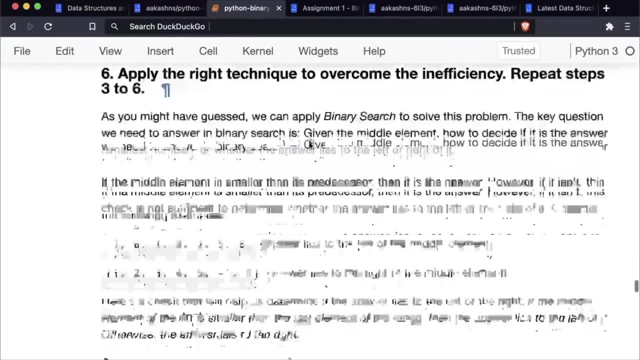 Okay, Maybe that's, And if you want, if you have code that's not working or there's an error, you can also include a screenshot of your code, or I'll show you another trick You can actually include. let's say, you commit your notebook. 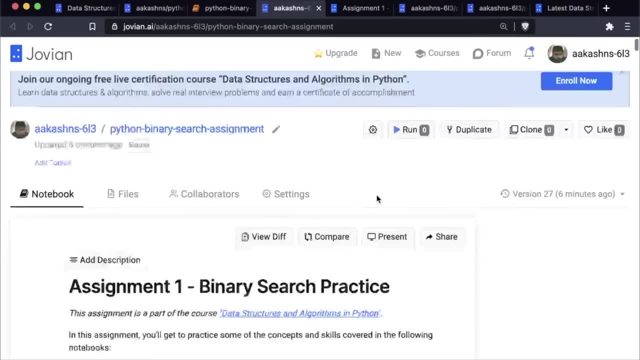 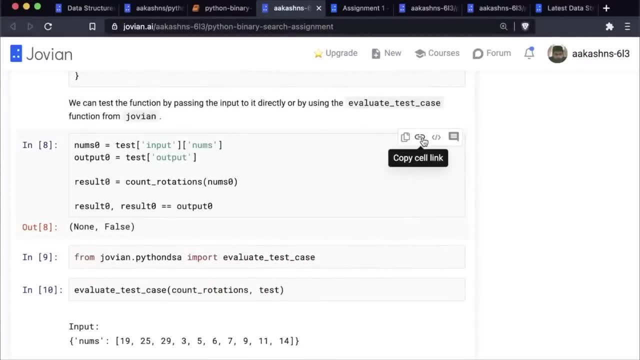 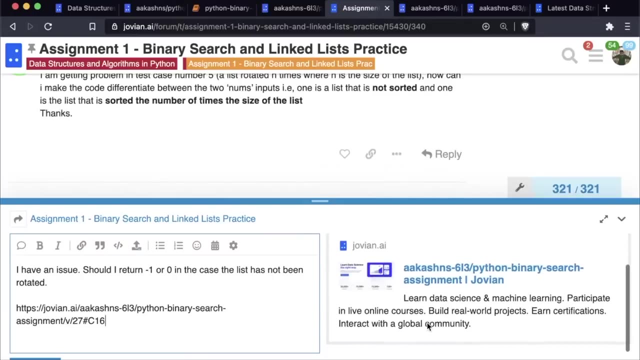 So let me come up here. I've committed my notebook And if you have a particular line of code that you want to share, you can actually click copy cell link and paste it here, So that will give a link to the entire cell. 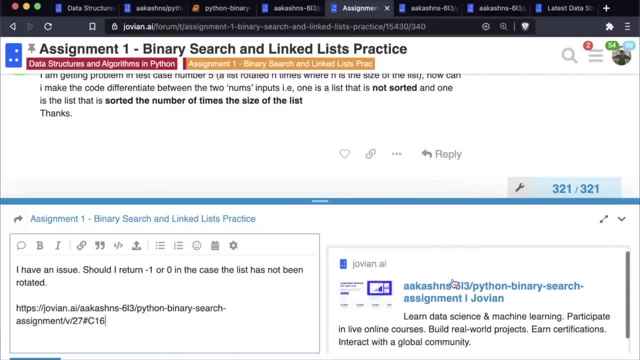 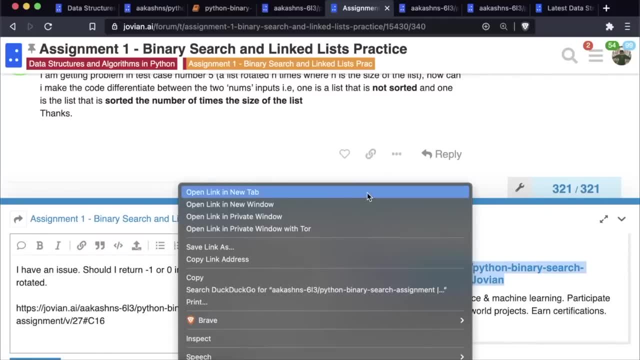 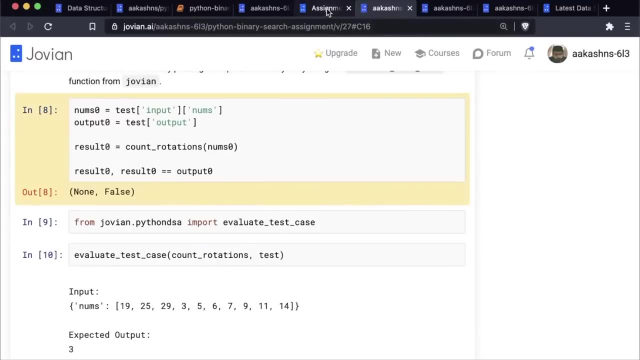 And if somebody clicks on the link, then they can view that specific cell Of the notebook directly. Let's see, You can see here that it brings us directly to this specific cell. There's another option. You can even click on embed cell. 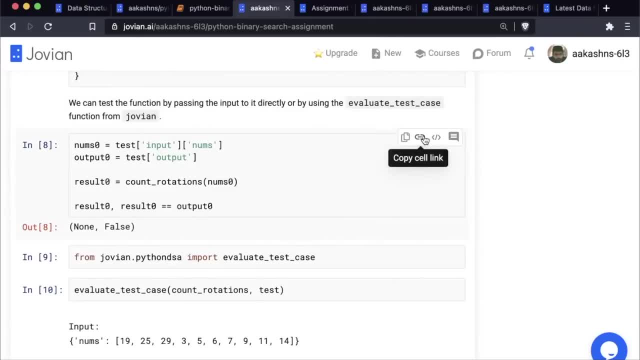 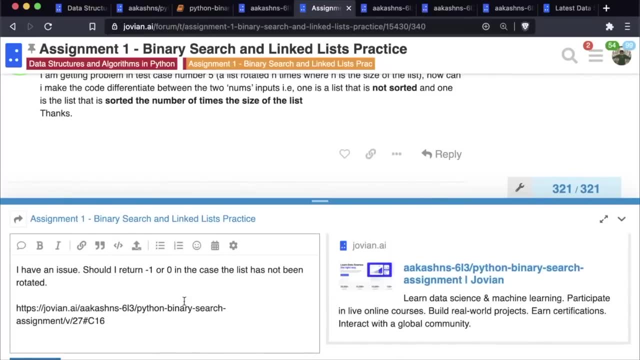 Okay, For embed. for secret notebooks we do not allow embedding but copying the selling should work And then click reply and your question will be posted and somebody will reply to your question. Just come back to the forum in a few hours or maybe the next day, and you should see an answer. 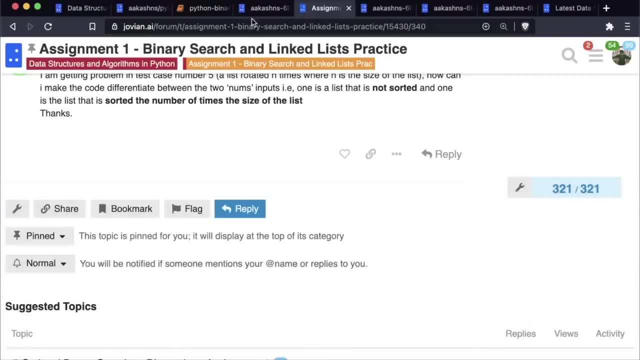 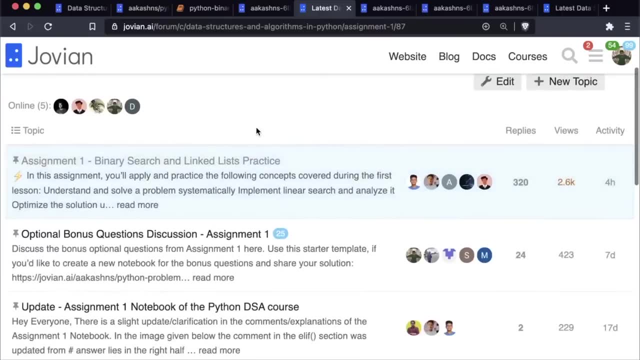 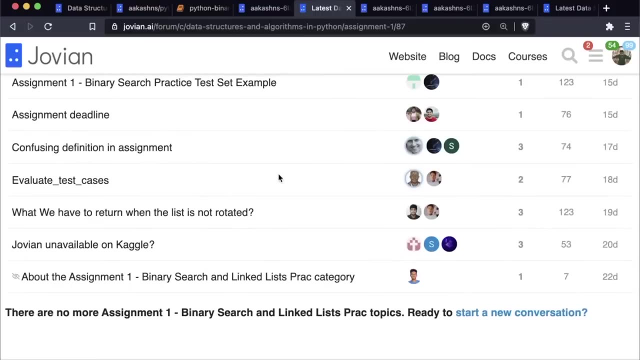 You will also receive an email. So that's the discussion topic. You can also go back to the topic here, the category here, and create a new question. You can see that, if you want to start your own thread, if you think your question deserves. 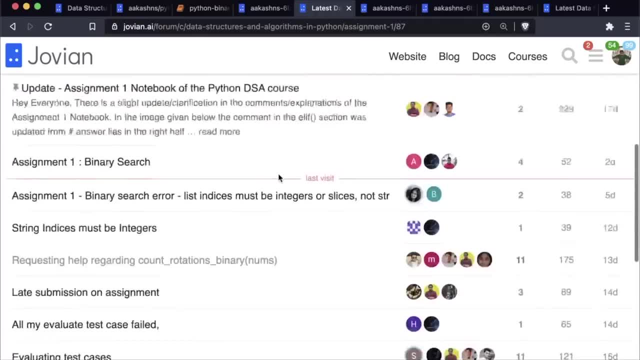 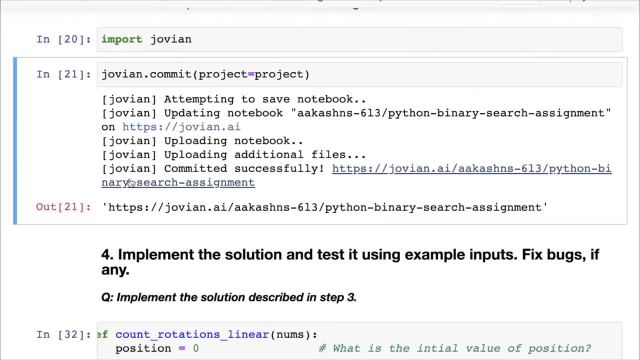 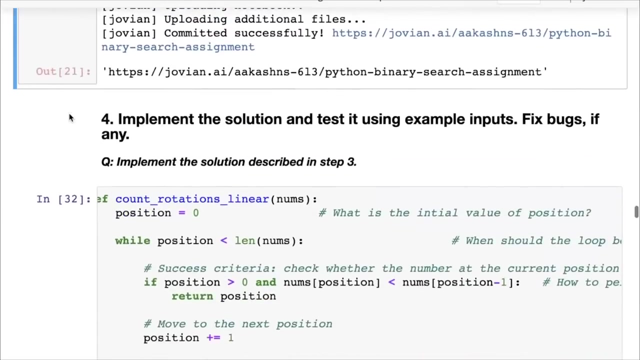 A deeper discussion where multiple people can reply. you can also create a new thread by clicking new topic. Okay, So keep this in mind and do make use of the forum. What we've seen is people who are active on the forum are at least four to five times more likely to complete the course and on the certificate of accomplishment and continue working on these topics after the course as well. 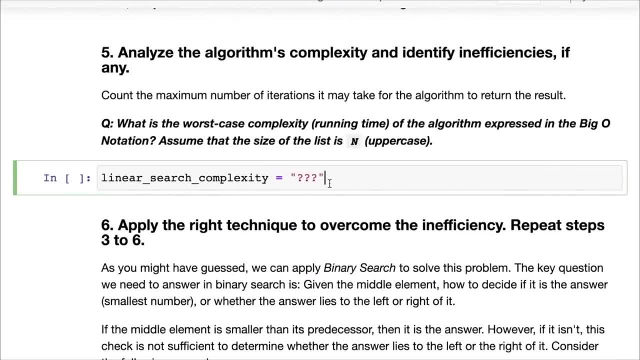 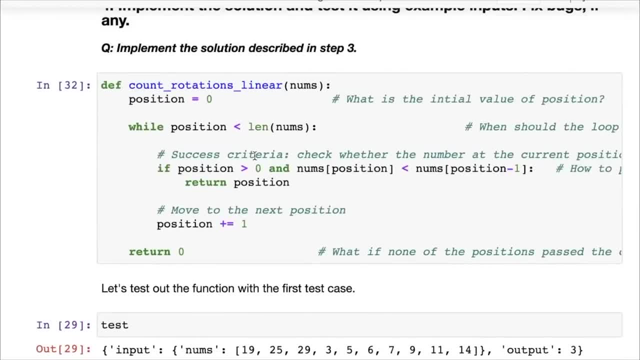 Okay. So the next step is to analyze the algorithms, complexity And the way to do this- if you've seen less than one- is to simply count the number of iterations, the number of executions of the while loop. Now, if you have a list of numbers of size N, then you can see here that this is the key loop here. while position less than the number. length of numbers. 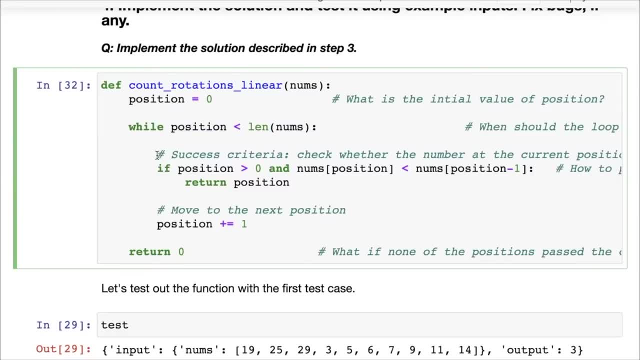 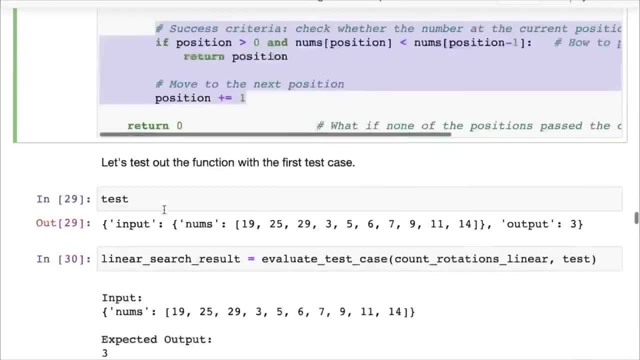 So then there will be N loops or N iterations, And then inside it each item. We're performing certain comparisons and returning things. So all of these are in effect constant time, And based on this you can probably tell that the complexity of linear search is ordered of N. 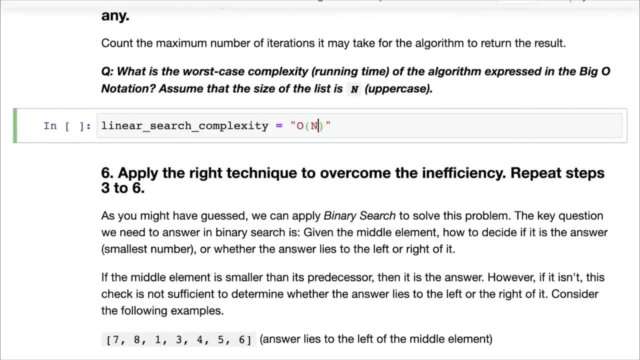 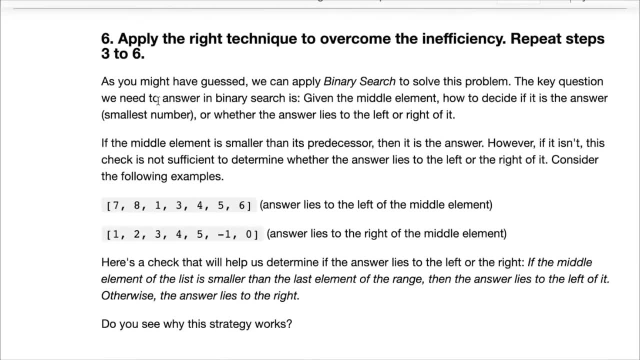 So you can just put in a big O and in the big O notation this will be ordered in. So that's the first part of the assignment linear search. Now the next step is to apply the right technique to overcome the inefficiency. and that's where you can now. you can now read through the rest of the. 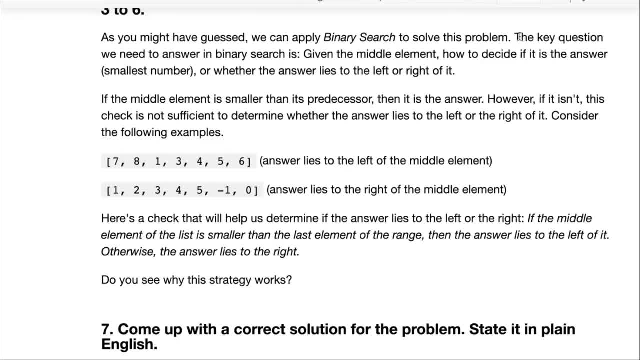 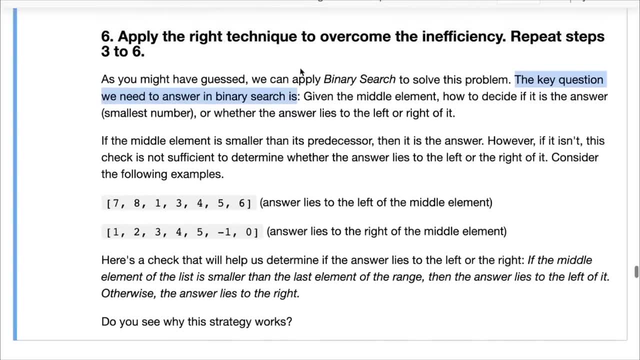 Assignment. Now, the idea here is this: binary search is a technique we'll apply And the key question we need to answer: in binary searches, given the middle element, can you decide if it is the answer, which means if it is, let's say, the smallest number in the list, or whether the answer lies to the left or the right of it? 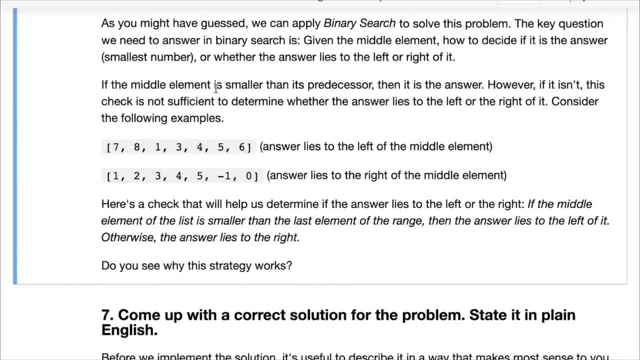 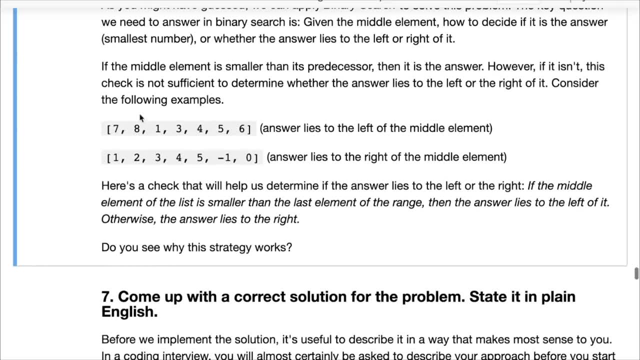 Okay, So given the middle, given if the middle element is smaller than its predecessor, Then it is the answer. We already know that, because there's only one number in the list that is smaller than its predecessor. So you can see here, for example, now, if the middle element was one, which it's not, but suppose that the middle element was one and you can see that one is smaller than eight. 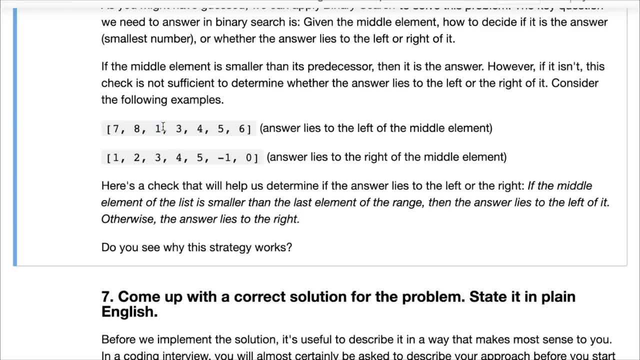 Then we know that one is the answer. So the position of the middle element is the answer. However, if it isn't, then we need a way to determine whether the answer lies to the left of the middle element or to the right of it, and consider these. 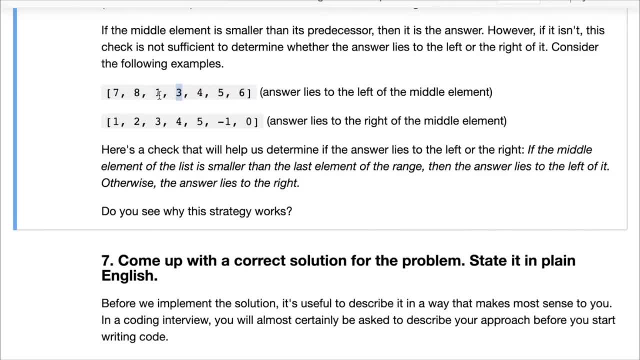 Examples. So here you can see that the middle element is three and the answer is the position two. So in this case the answer or the smallest element lies to the left. On the other hand, in this case you can see, the middle element is four and the smallest element, minus one, lies to the right of it. 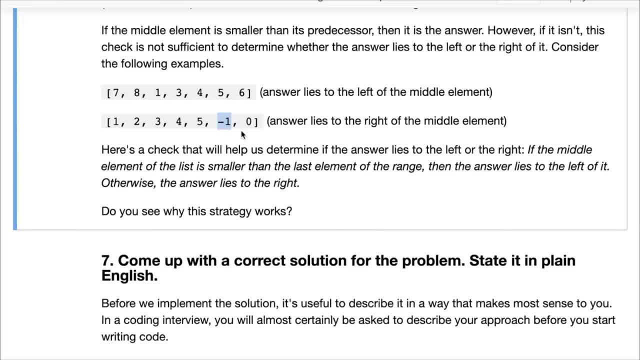 So now you need to apply your mind and think of a check that will help you determine if the middle element, given the middle element, If the answer lies to the left or the right, of it right And we're looking for the smallest element. 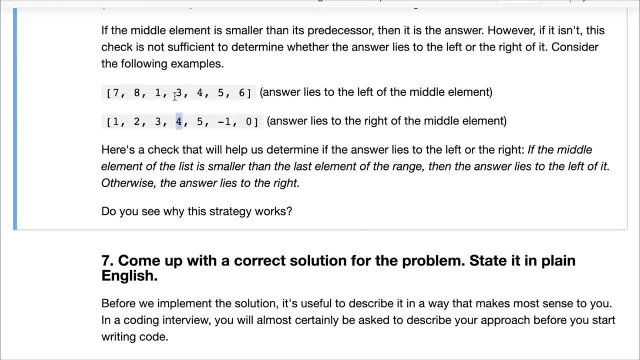 Remember the logic here. if you just spend a couple of minutes, you will come up with this quite easily. If the middle element of the list is smaller than the last last element of the list, okay, Or the last element of the teams that we're currently looking at. 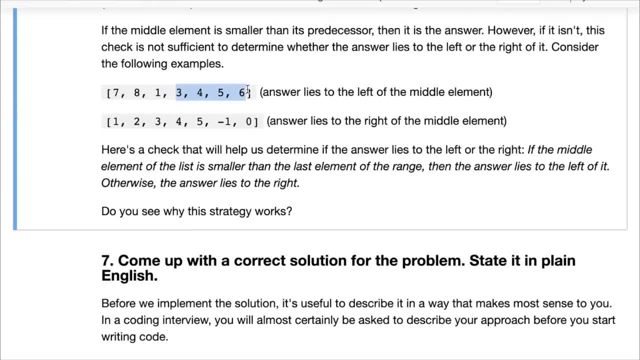 That means that all the numbers here are in increasing order, So then the answer lies to the left of it. On the other hand, if the Middle element of the list is larger than the last element of the range, That means that, because we know that the list is a rotated sorted list, 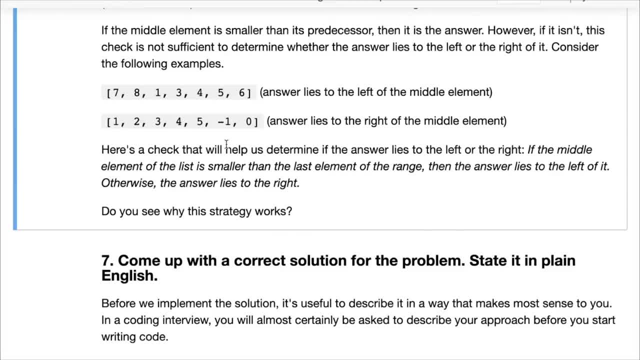 So that means that the numbers increase up to a point and then there's a decrease and then they continue increasing. That's the only way in which the final element can be smaller. So that means the answer lies to the right of it. So that's the logic here for binary search. 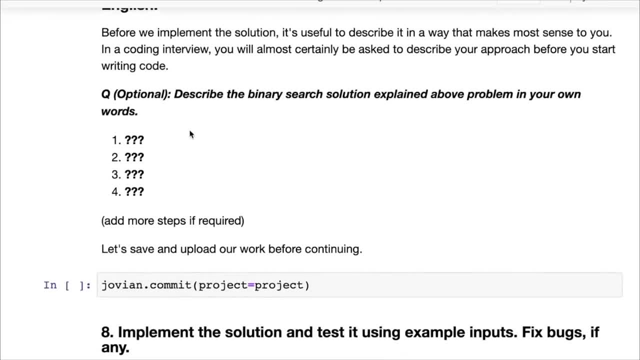 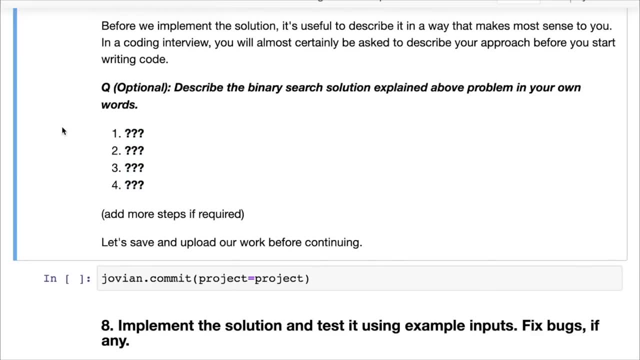 And now what you have To do is describe the binary search solution in your own words. So here, once again, you have these four or five lines. It's very important that you do this, because if you cannot express it, then coding it is also going to be difficult for you. 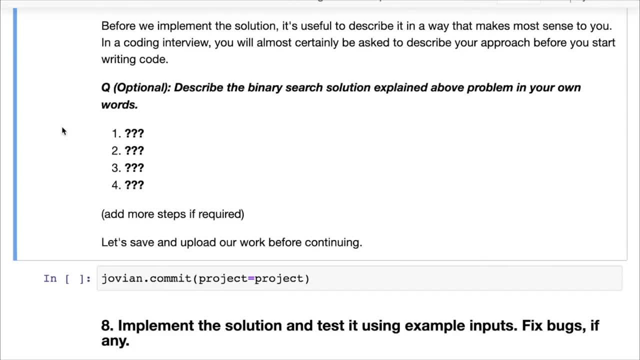 So always do this exercise of expressing the solution in your own words When you're practicing, when you're solving a coding challenge or something, even in an interview. it's also very important, Because the first thing you need to do is to communicate to the interviewer your thought. 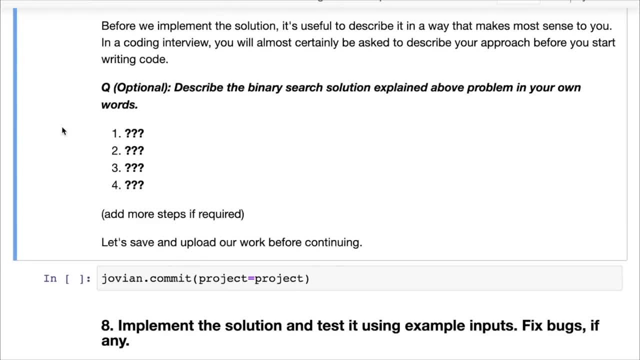 Process and how you're thinking about the problem. So the first thing you need to do is describe a simple solution in your in simple words, and then they may or may not ask you to code that solution, And then the next thing is to identify the complexity or identify the inefficiency. 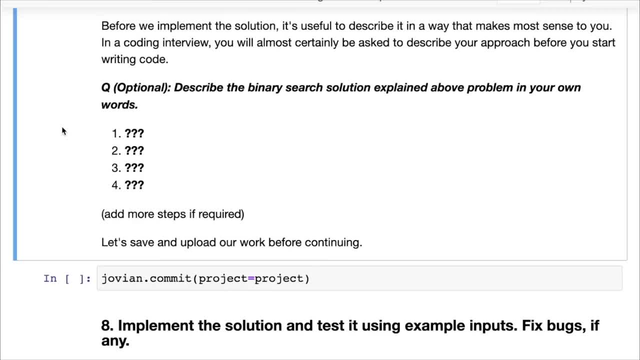 Then the next step for you is to describe the optimal solution, or the binary search solution, in your own words. Okay, Now, if you don't describe the solution in your own words and you start writing the code, they may not be able to follow your code. 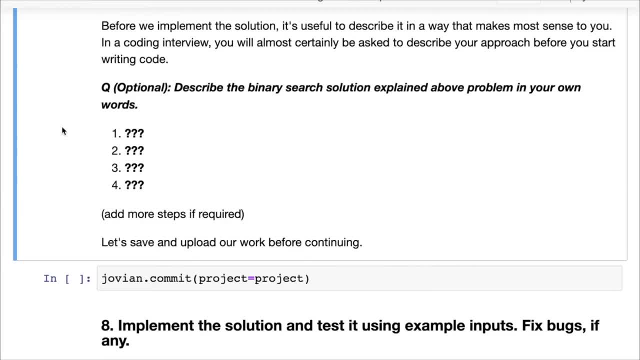 So even if you've written mostly correct code, maybe with one or two edge cases wrong, they may still have a feeling that you don't know what you're writing. But if you explain the solution clearly to them, they will know that now you understand the solution and they will be able to follow the code as you write it and they will be able to pick up mistakes or errors and help you with the errors. 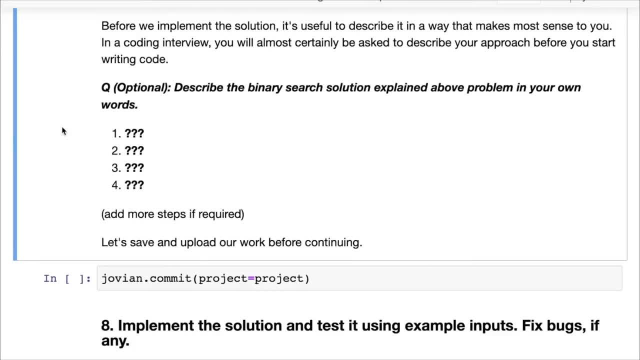 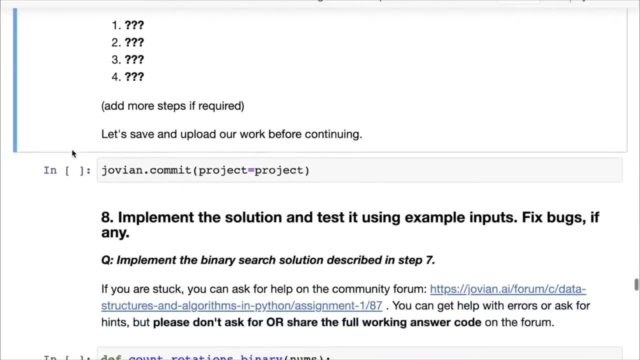 One secret is that interviews are always open to helping you, unless you make them really confused. So keep that in mind and describe the solution in your words. Once you do that, you can commit. Now the next step is to implement the solution. 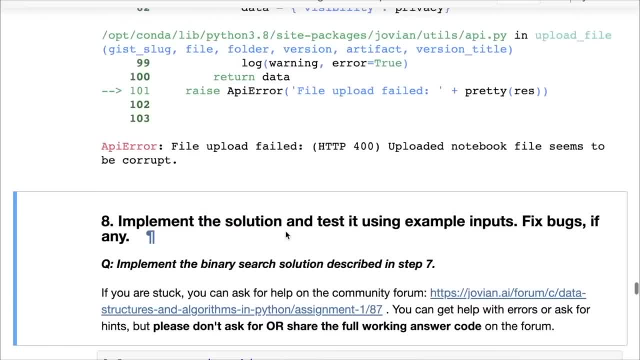 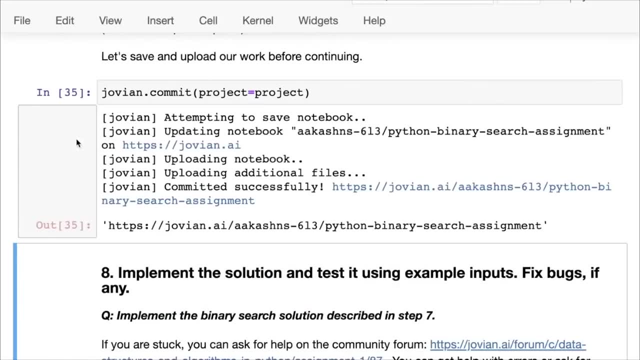 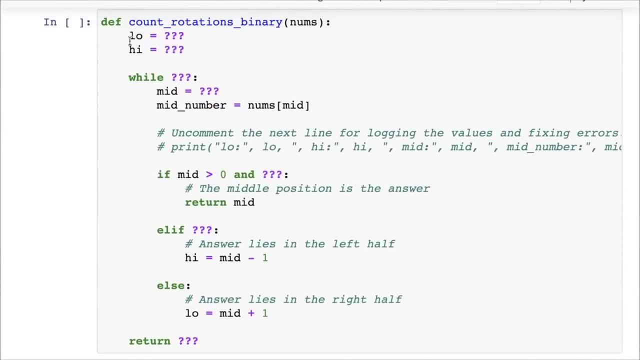 Now the implement the binary search solution as described in the previous step. Let's run this again. Yeah, So then you run count rotations, define the Function count rotations binary. Now you may want to review lesson one here on how to start it out. 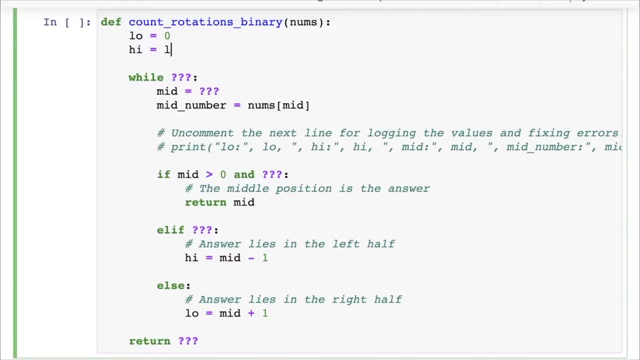 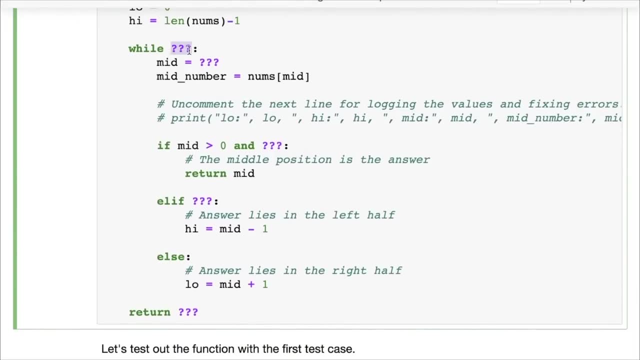 And you'll see that low starts out at zero and high starts out at Len nums minus one, and I will not solve the rest of this. but there is a certain condition here between low and high. So in binary search we are starting with the entire list as the range. 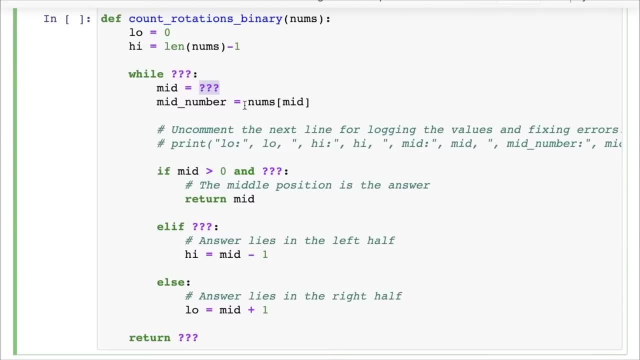 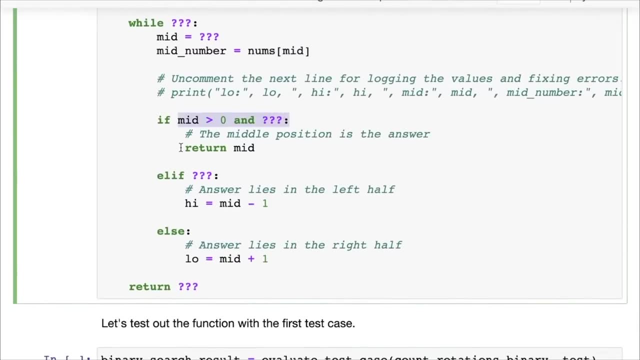 Then we are looking at the mid number. So we're getting the first, the mid position, and we look at the number at the mid position. Then we check if the middle position is the answer. So if the middle position is the answer, we return the middle position. 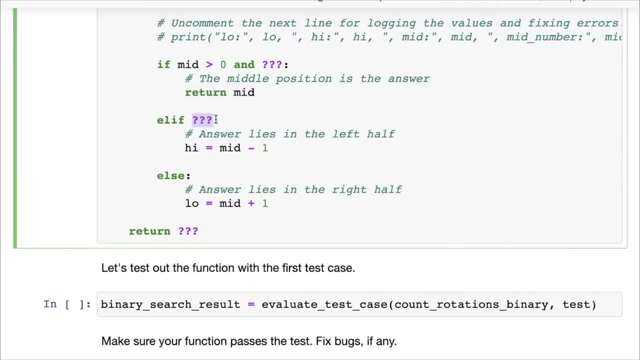 Then we check if the answer lies in the left half. So here's a condition where you decide if the answer lies in the left half And we, once we, if the condition holds true, all we do is we change the high switch. 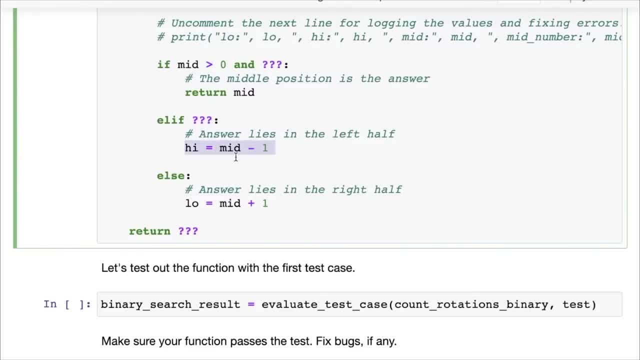 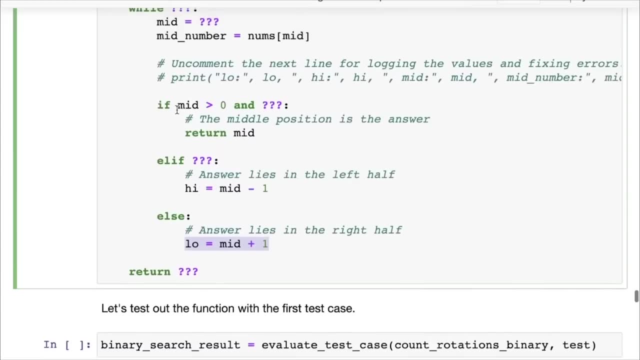 We change the end point of the range to mid minus one And then we check if the answer lies in the right half. In that case we changed the starting point of the range to mid plus one and the Y, And then the loop repeats. 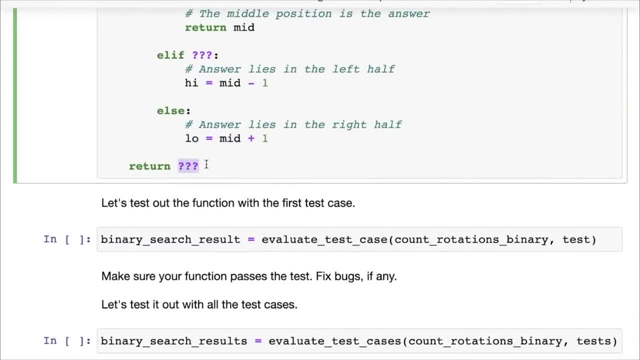 Okay, So that's the general logic of binary search, And one thing you have to keep in mind is, if none of the elements satisfy the criteria that you have, what is the answer? And this is a very important condition. This is where it is very easy to go wrong. 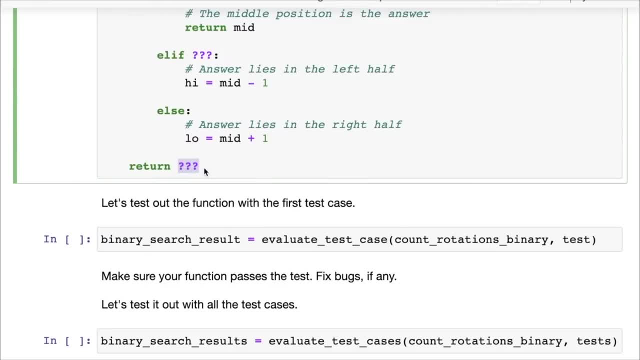 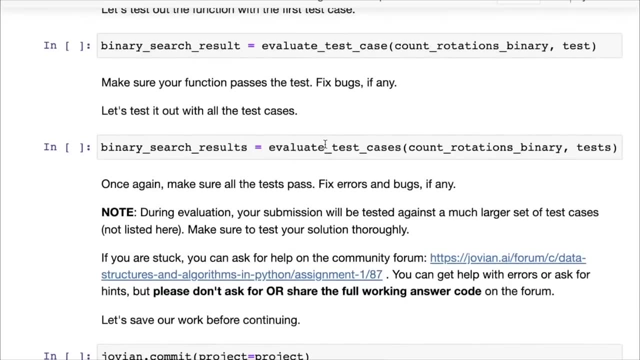 It was also called the edge case or the trivial case. So you should handle and think about this carefully, Okay, And then, once you've done that, you can evaluate the test case and you can a single test case You're going to evaluate. 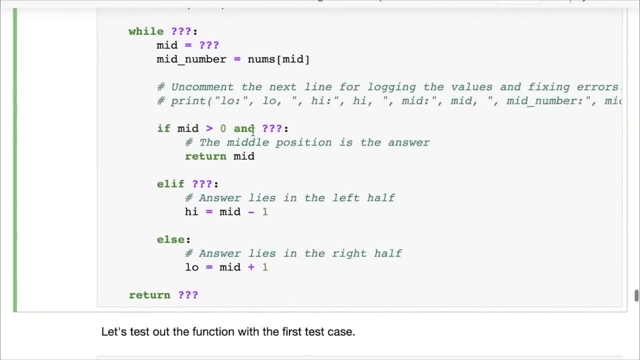 Okay, Okay Now, if your test cases are failing, you may want to enable this print statement inside by uncommenting it, but make sure to comment it out at the end once again, and the print statement will help you see what the low, high and mid points were. 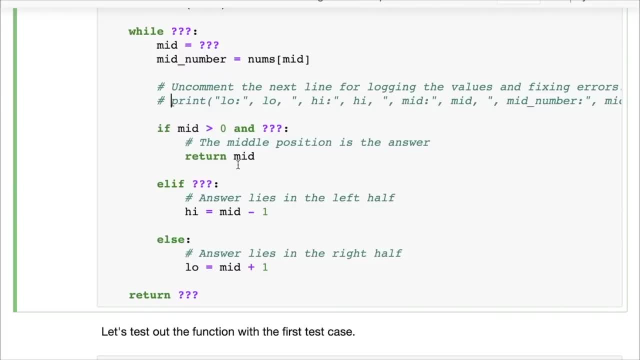 Now you may want to then take a pen and paper, look at an example that is failing and see if the printed numbers match what you expect to see. debugging your function is a very important skill, So keep that in mind And use a debugging technique like this by adding print statements and working out the same problem side by side on paper to fix your issues. 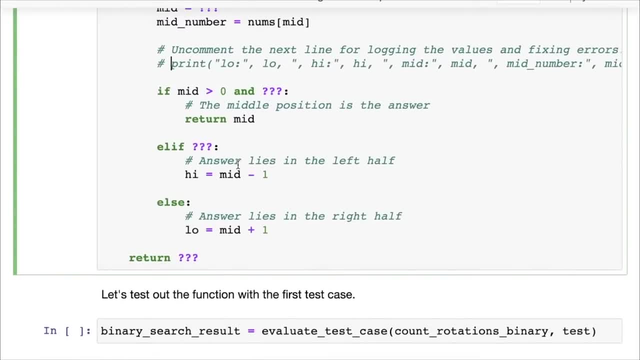 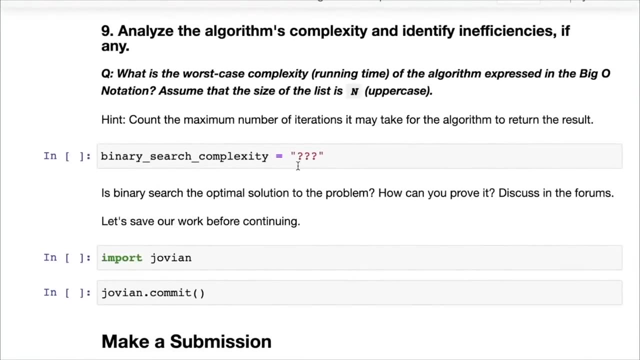 Otherwise, you may feel lost if you're not able to look into the internal workings of the function. Next, you have to analyze the algorithms, complexity and identify inefficiencies. This should be straightforward enough. We've already looked at the complexity of binary search, but all you need to do is make 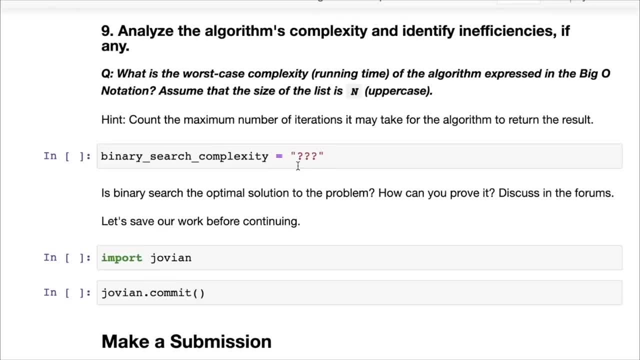 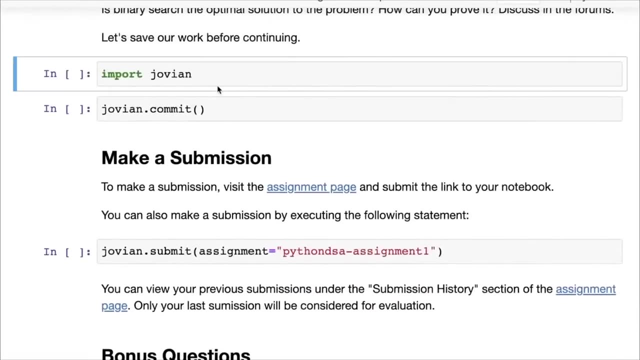 Make sure that what you're doing within the algorithm matches the analysis that we've done earlier. So the problem size reduces by half each time and then we are doing constant work in each step before solving a problem of half the size. So that should roughly give you an answer. and keep committing your work. 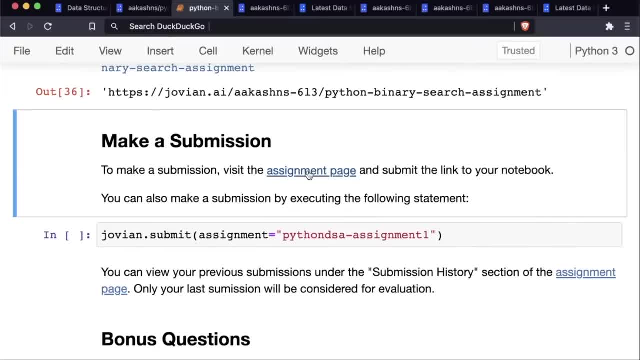 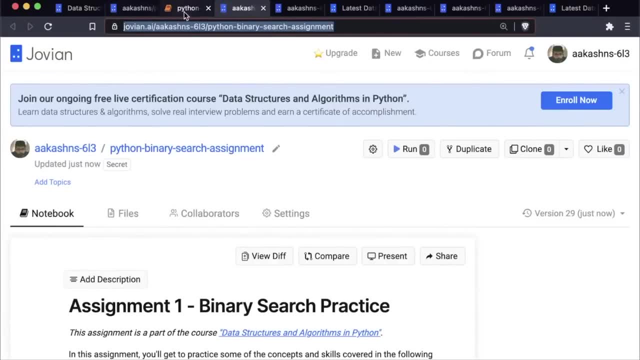 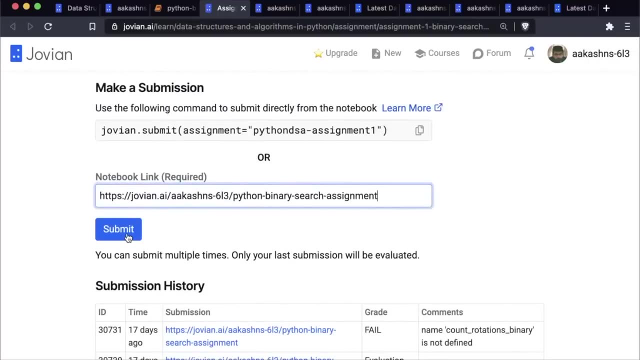 Now, finally, to make a submission. you have two options Now. one option is to take this link, So your notebook has been committed here And you can come to the Assignment page. Let's open up the assignment page, binary search practice. come down here and paste this link here and click submit. 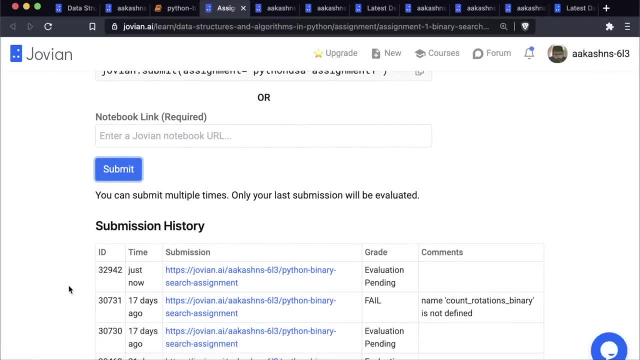 Now, once you click submit, the assignment will be submitted and it will go into automated evaluation. So in about a couple of minutes- maybe up to an hour depending on the queue of submissions from Definitely different participants- you will receive a grade over email. 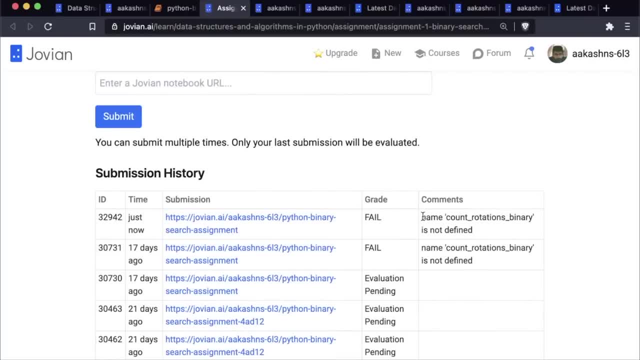 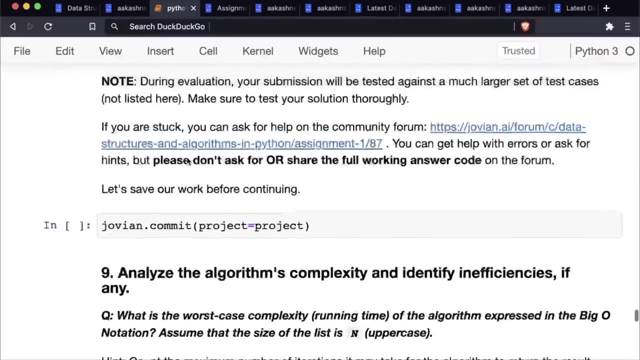 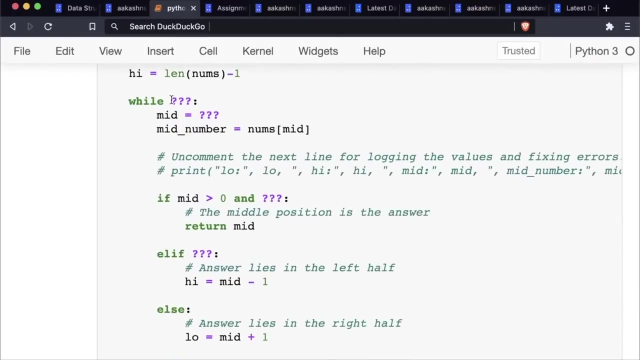 Let's just refresh the page And it seems like there was an issue here. The issue was that count rotations binary was not defined, So it's possible that this happened- Count rotations binary did not get defined- because there are a bunch of question marks here, So we may need to then fix the issue and then come back. 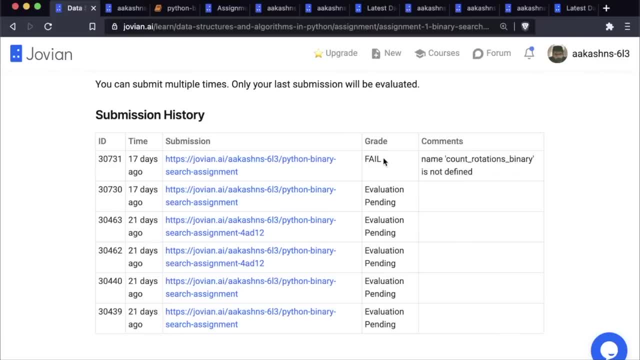 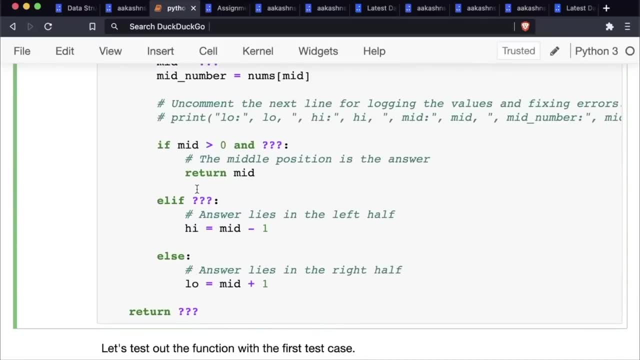 And make a submission once again. Okay, So I have received fail grade. I will go back and I will fix the issue and then come back. Okay, Now, it's very important for you. That's why- to have good a set. 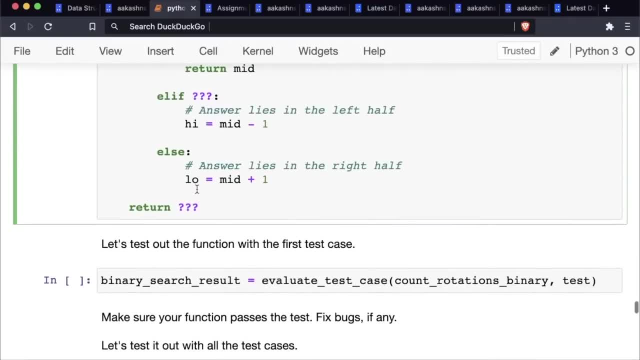 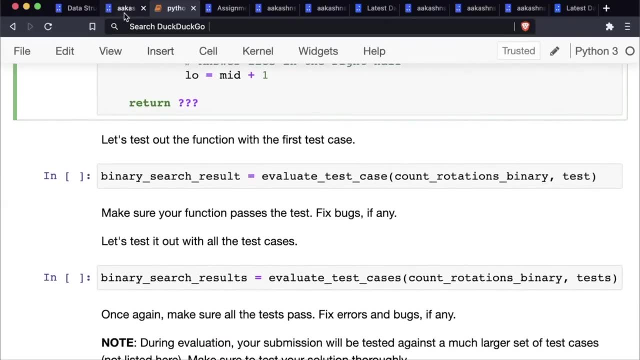 good set of test cases for you to test your function so that when you submit it or when you get an error, you can maybe look at your functions performance on the test cases and fix anything that needs to be fixed and add new test Cases If you need to. 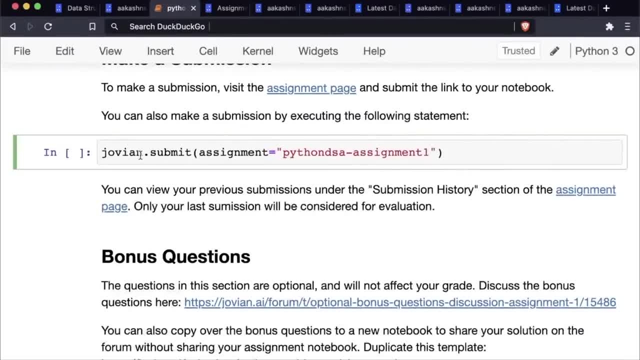 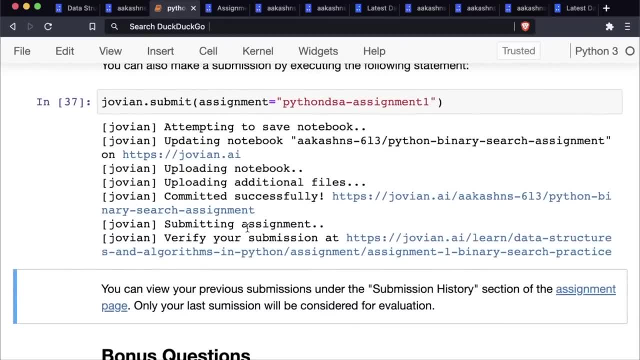 The one other way you can submit is by simply running the code by German dot. submit assignment equals Python DSA hyphen, assignment one. The code is mentioned here. You can see here that the submission was made and you can verify your submission on this page. Okay So. 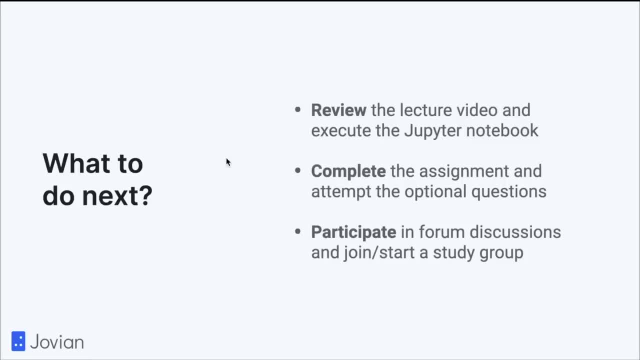 that's assignment one. So what should you do next? Review the lecture video, if you need to, and execute the Jupiter notebook You may need to keep. you may want to keep the Jupiter notebook running side-by-side as you're working on the assignment. 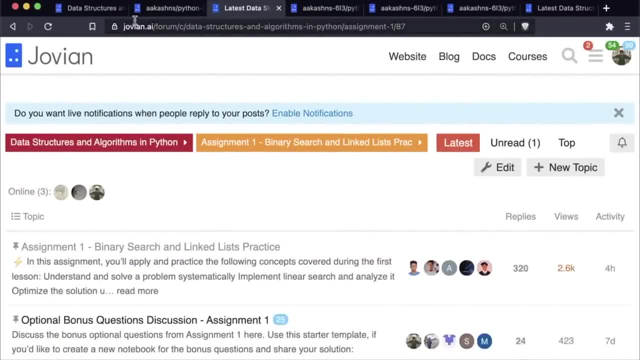 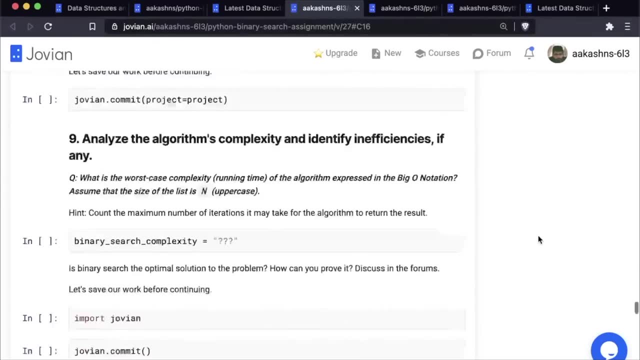 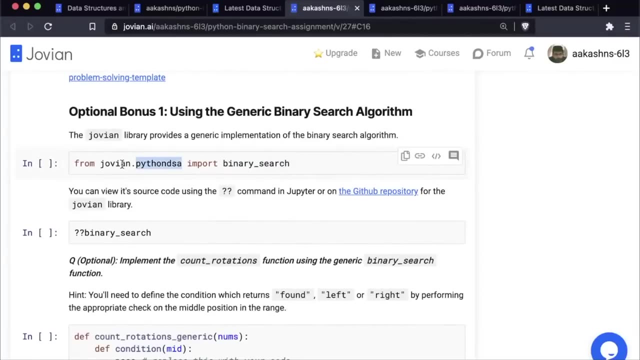 then complete the assignment and even attempt the optional questions. If you scroll down here on the assignment notebook, you will find that there are some optional questions for you. Here's one bonus question: Use the generic binary search algorithm. So inside the Python DSA module in Jovian. 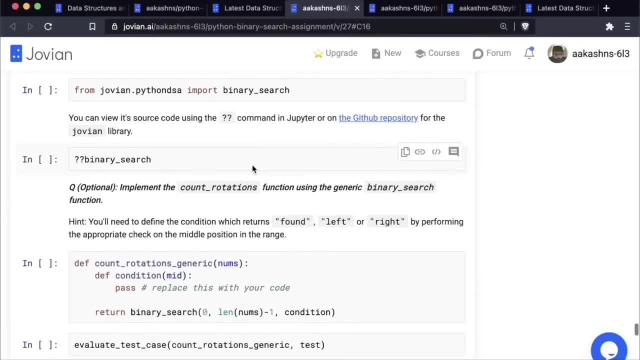 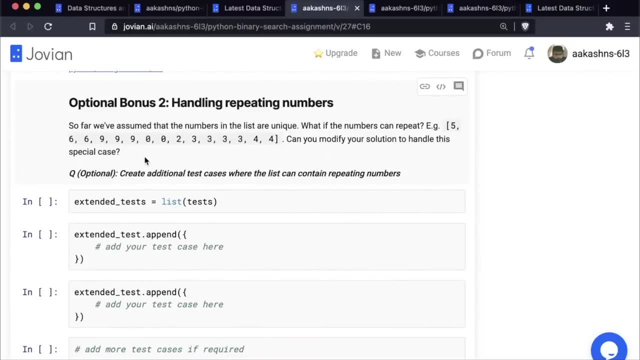 there is a function called binary search. You can use the Generic binary search example. Then here's an optional bonus question to handle repeating numbers. We did see that you can assume that there are no repeating numbers in the list, but here's one list with repeating numbers. 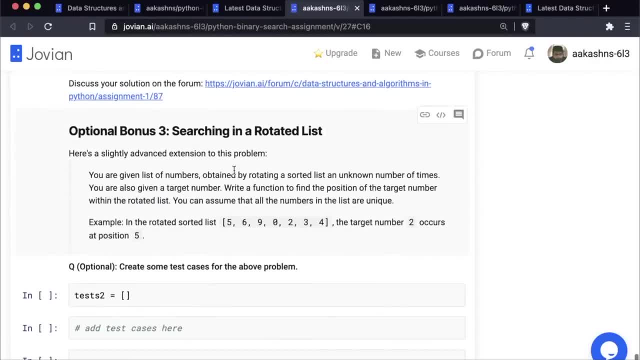 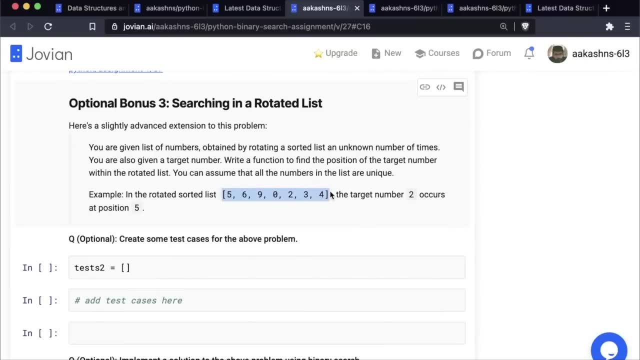 Can you modify your solution to handle the special case? And then here's an optional bonus. question three about searching in a rotated list. So you're given a rotated list. Now, instead of finding the number of times it was rotated, you're, you're. 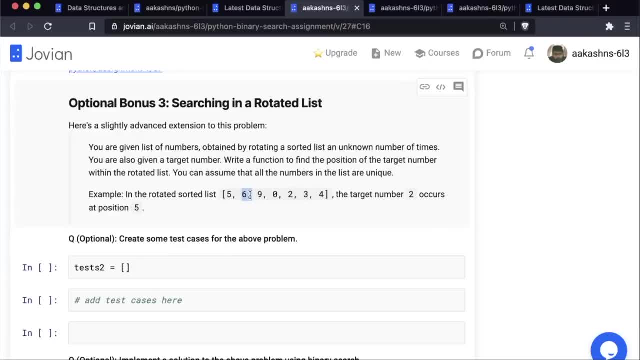 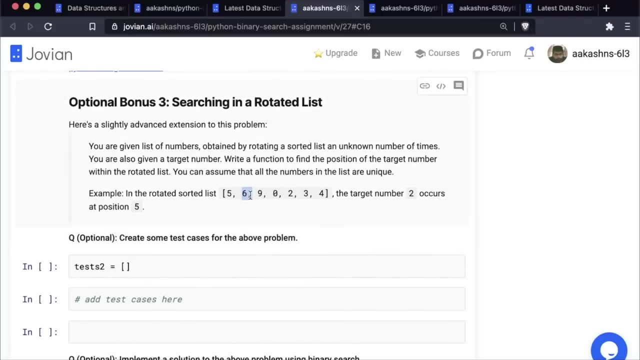 trying to find the position of a certain number, For instance the position of six. can you apply binary search and modify your previous solution slightly to search within the rotated list and find the position of a given number? Okay, Now here's a hint. 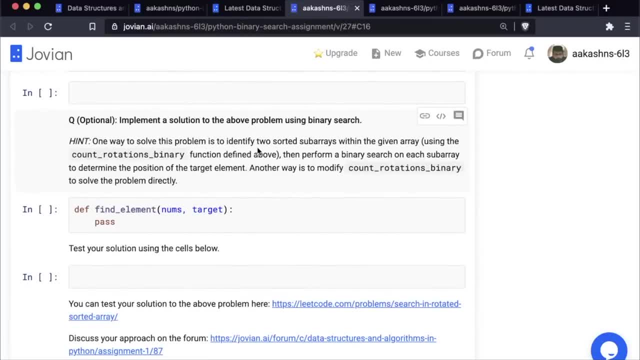 You can simply identify two sorted sub-arrays within the given array and perform a binary search on each sub-array using the. to identify the two sorted sub-arrays You can use the count rotations binary function. So that's one potential solution. Another way is to modify the count rotations binary function to solve the problem directly. 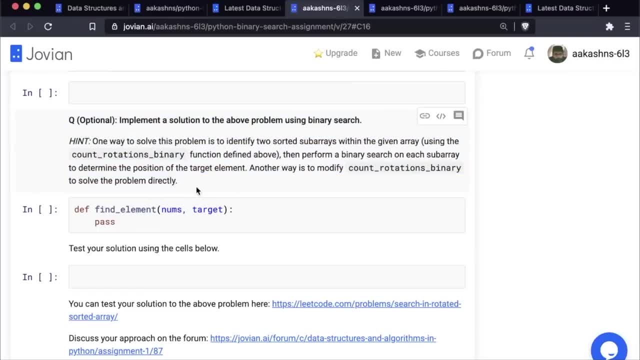 So it's a very interesting problem to solve, And if you found the assignment easy, then you should definitely solve these bonus questions. And if you can solve this question by yourself without taking additional help, then you can solve pretty much any problem related to binary search that may be asked. 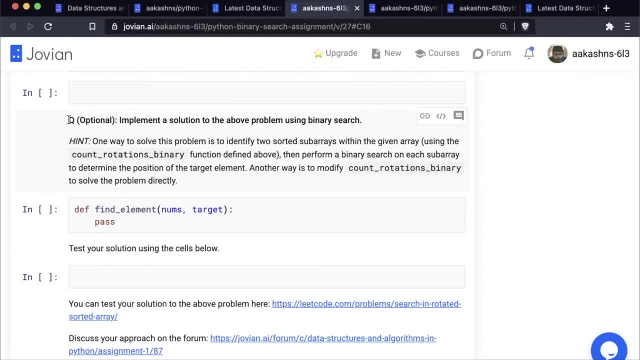 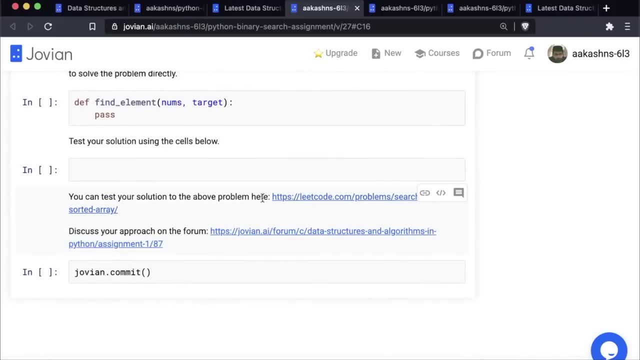 in an interview, because most of the questions are some variations of something like this, And this is pretty much the hardest problem you may get asked. You can also test your solution by making a submission on lead code, And this is only for the final optional question. 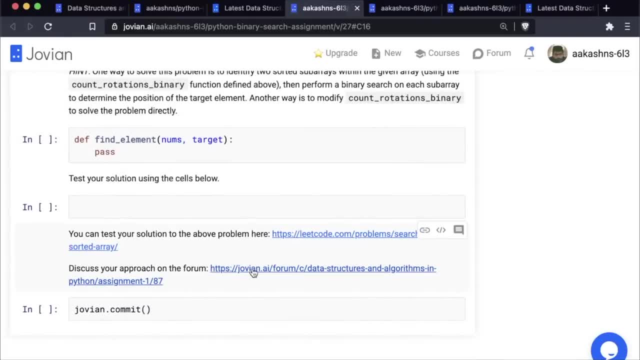 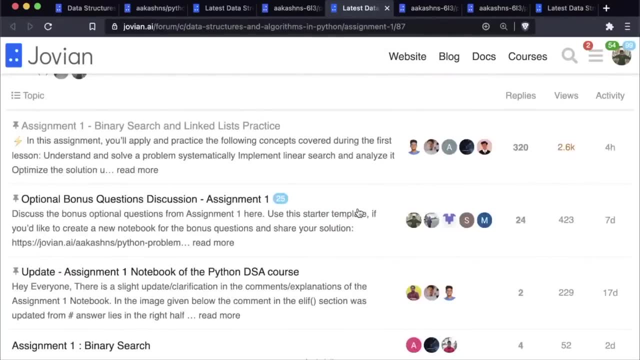 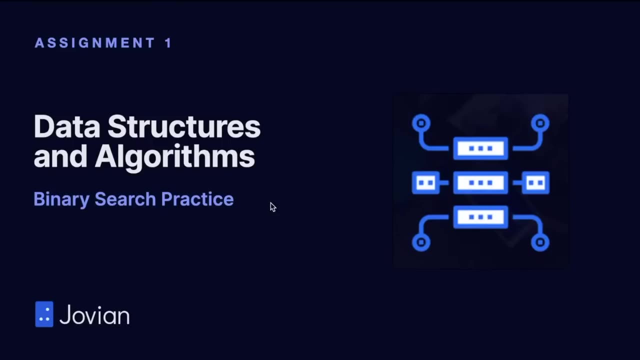 And there's a thread on the forum where you can discuss the bonus questions separately as well. So do make use of the forum thread too. Here it is optional bonus questions discussion. So that was assignment. one of data structures and algorithms is called binary search practice. 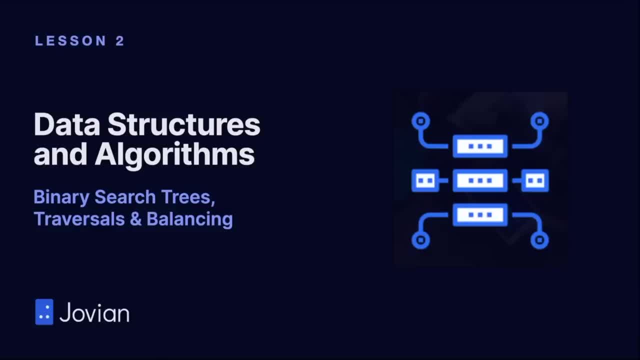 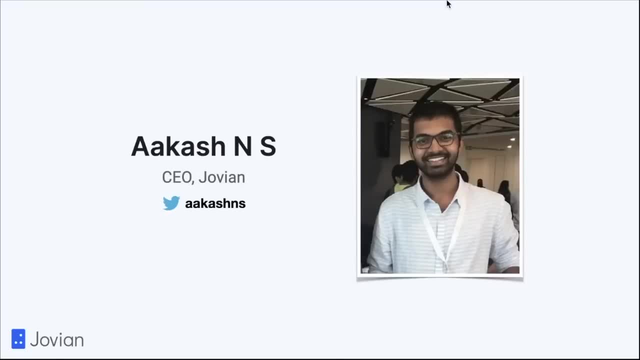 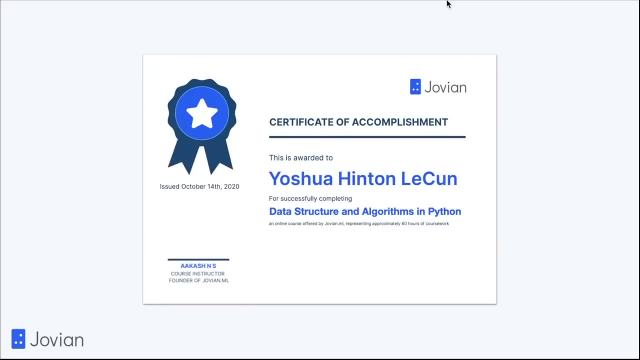 Hello and welcome to data structures and algorithms in Python. This is an online certification course by Jovian. My name is Akash and I am the CEO and co-founder of Jovian. You can earn a certificate of accomplishment for this course by completing four weekly assignments and doing a course project. 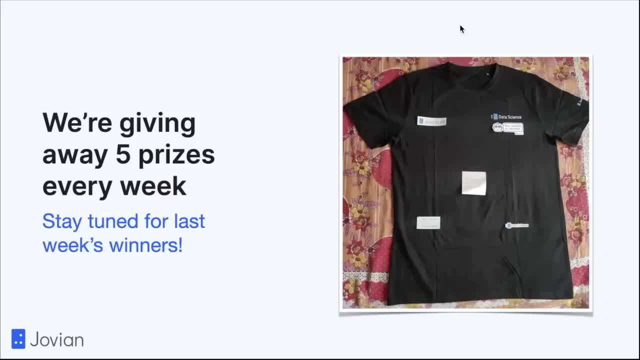 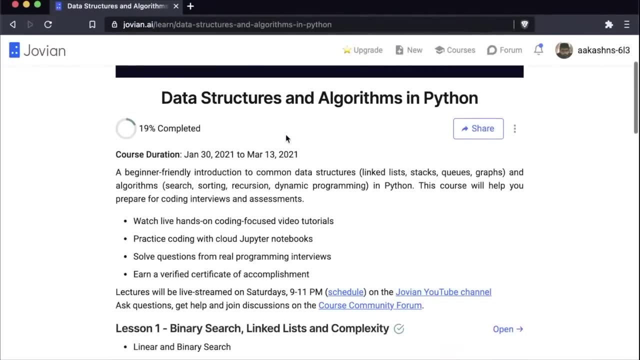 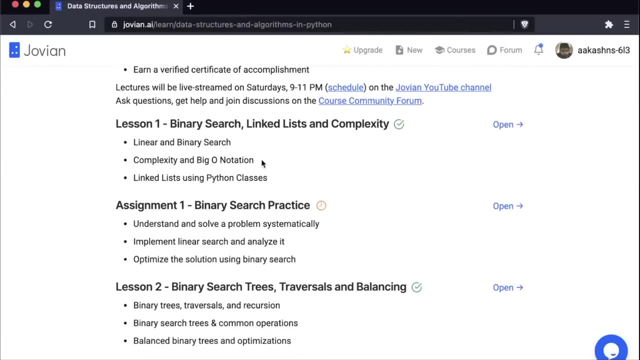 Today we are on lesson two of six. Now, if you open up pythondsacom, you'll end up on this course website, where you will be able to find all the information for the course. You can view the previous lessons, which is lesson one, and you can also work on the previous assignment, which is assignment one. 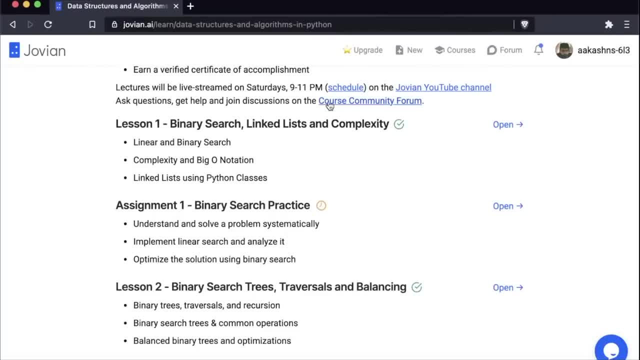 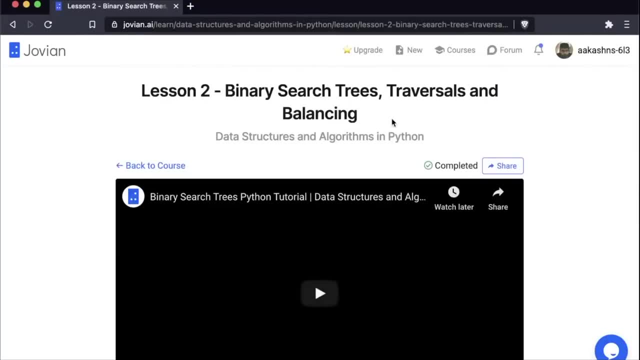 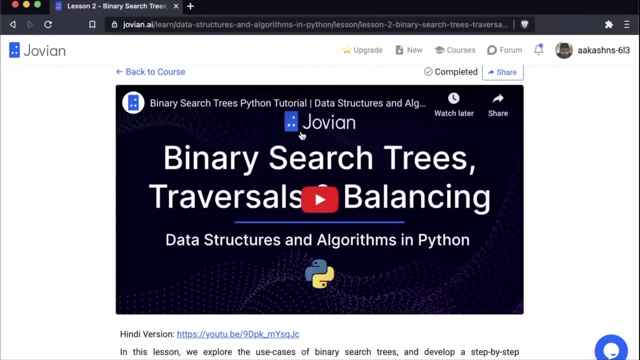 And you can also check out the course community forum where you you can get help and have discussions. So let's open up lesson two. This is the lesson page. here You will be able to see the video For this lesson. you can watch live or you can watch a recording here, and you can also see a version of this video lecture in Hindi. 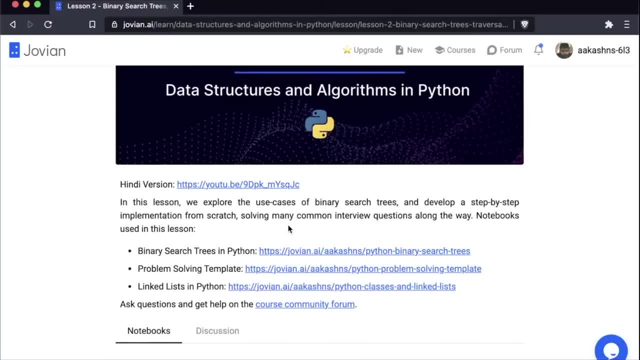 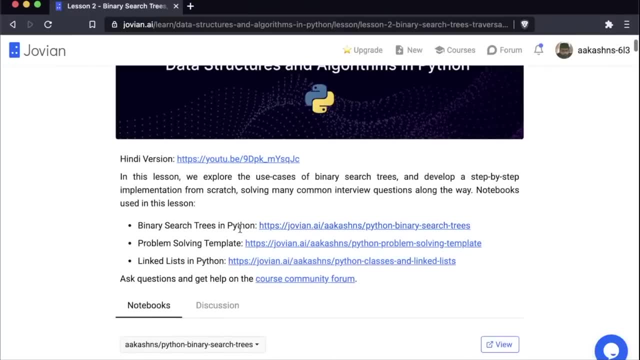 And in this lesson we'll explore the use cases of binary search trees and develop a step-by-step implementation from scratch, solving many common interview questions along the way. So here is the code that we are going to use in this lesson. All the different notebooks containing the code are listed here. 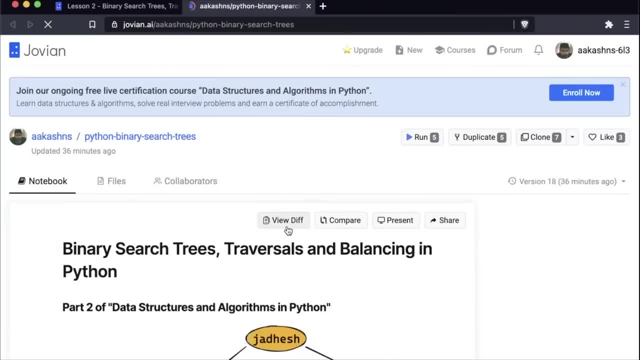 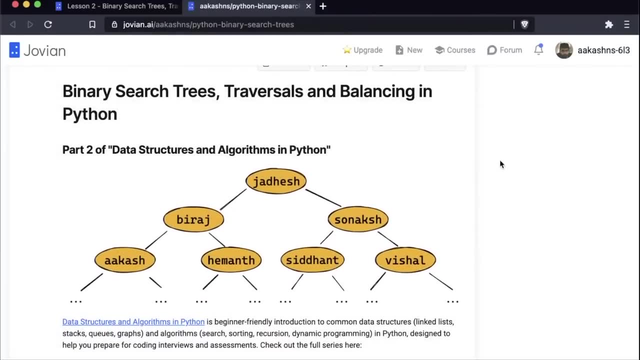 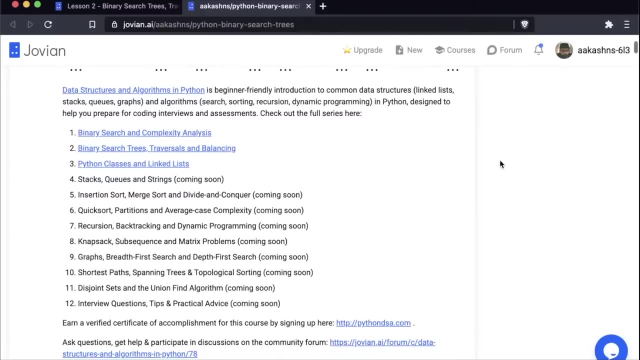 And let's open up the first one. So here you can see all the explanations and the code for this lesson. This is binary search, trees, traversals and balancing in Python, And this is the second notebook in the course. You can check out the first notebook in lesson one. 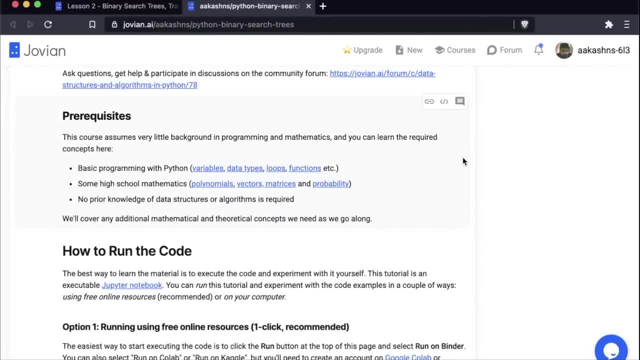 And if you're just joining us, this is a beginner friendly course and you do not need a lot of background in programming. with a little bit of Understanding of Python and a little bit of high school mathematics, You should be able to follow along just fine. 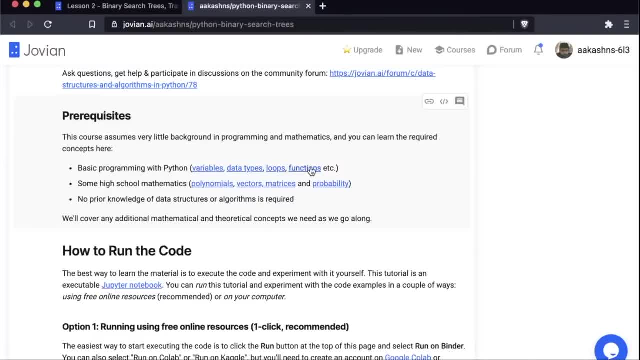 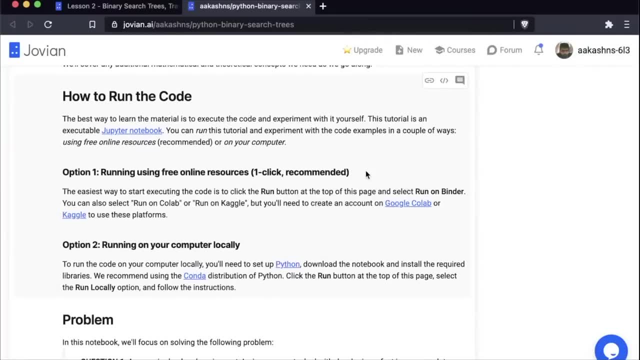 If you do not know these, then you can follow these tutorials to learn the prerequisites in just about an hour or two. Now, the best way to learn the material that we're covering in this course is to actually run the code and experiment with it yourself. 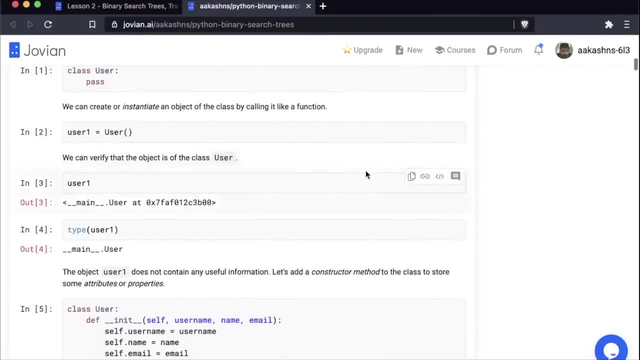 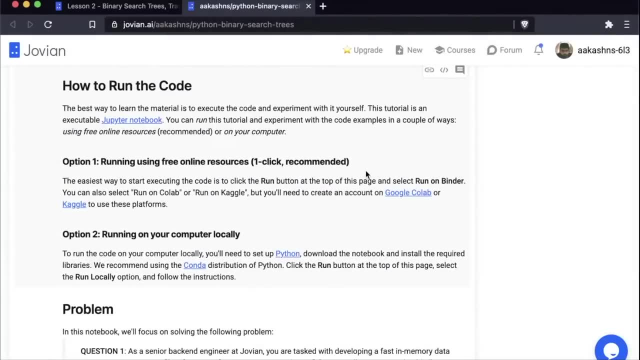 So to run the code- and you can see here, if we scroll down you can see that there is some code here on this page as well- Not to Run the code, You have two options. You can either run it using an online programming platform or you can run it on your computer locally. 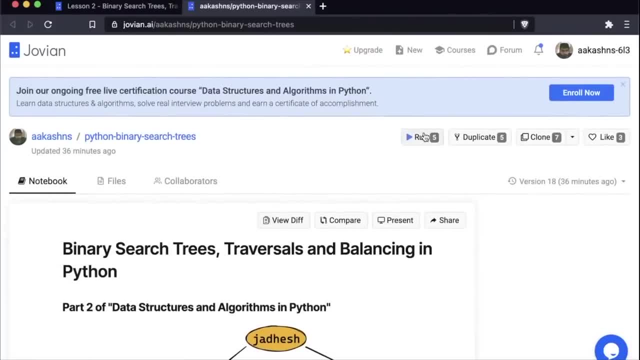 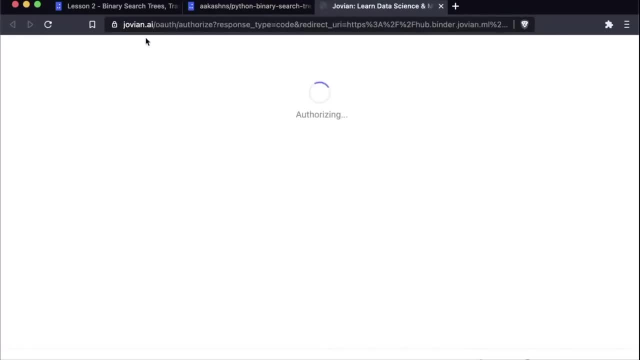 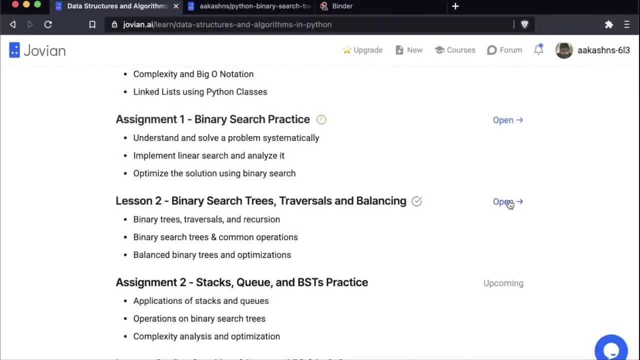 So to run this code, we will scroll up and click on the run button and then click run on binder And this is going to start executing the code that we were just looking at. So once again, you can go on the course page. python dsacom. open up lesson two. 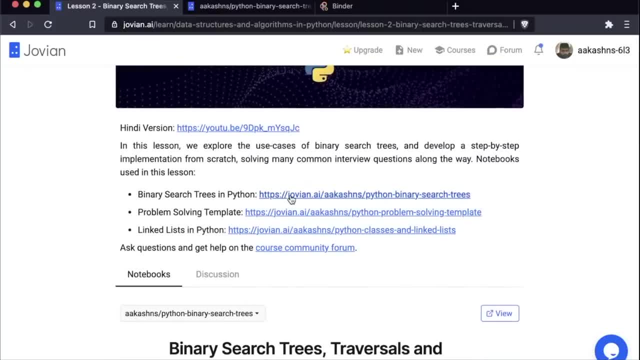 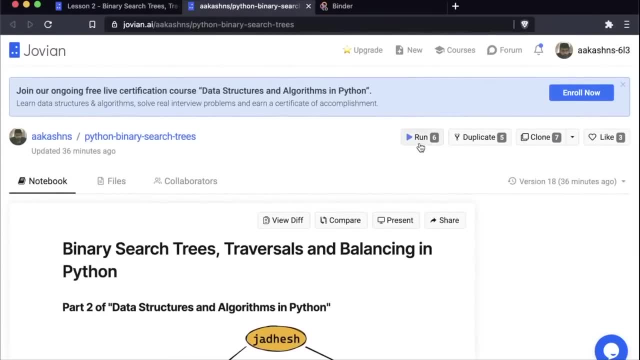 And You can watch the video there. and on lesson two, you can open up the link to the code where you can read the code and the explanations here. And if you want to run the code, just click the run button and that will execute the code for you. 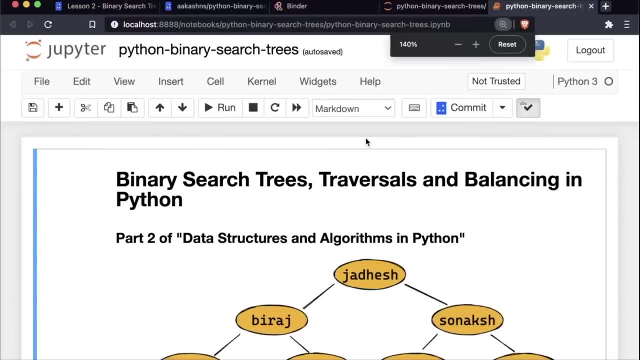 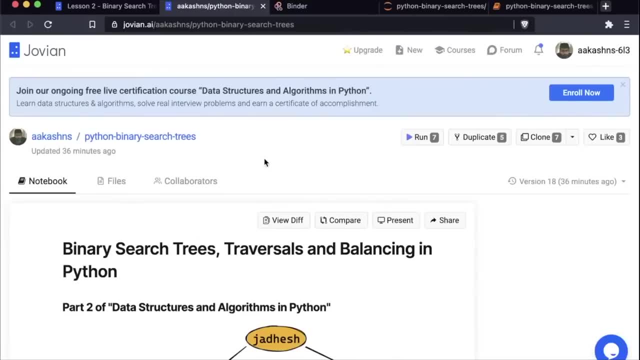 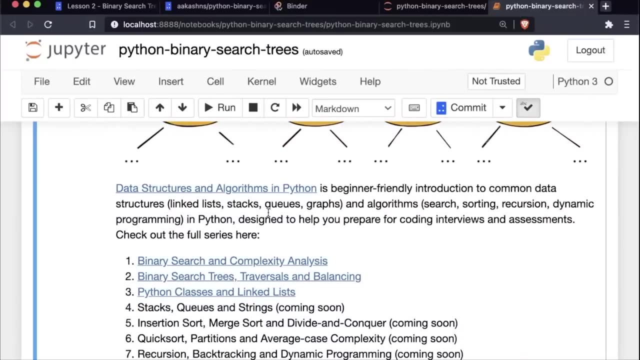 So once you click the run button on binder, you should be able to see an interface like this. This is the Jupiter notebook interface: the same explanations that we were seeing on the lesson page. You can see here the same explanation And now available here. but the difference is you can now edit these explanations and you can go down and you can actually run some of the code in this tutorial. 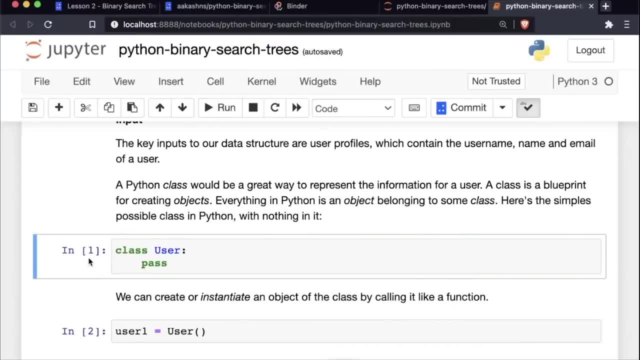 You can see here that you have a run button And when you click the run button, that is going to run the code in this particular cell, And this is a Jupiter notebook made up of cells. Now we'll do a couple of things here. 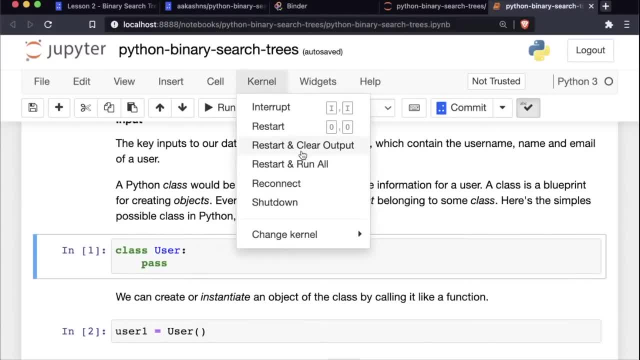 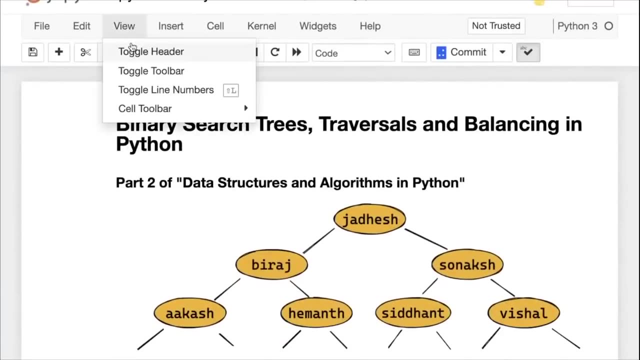 The first thing we'll do is we click on kernel and click on restart and clear output. What this will do is this will clear all the outputs of the code cells so that we can execute them ourselves. And then I'm just going to zoom in here and hide the interface so that we can look at the explanations and the code. 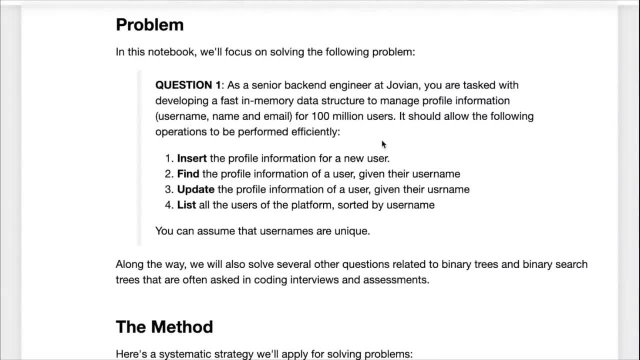 So finally, we have some running code and in this notebook we will focus on solving this specific problem, And this is a common question. A question of this sort can be asked in interviews, So this is an interview question, but along the way we will also learn how to build. 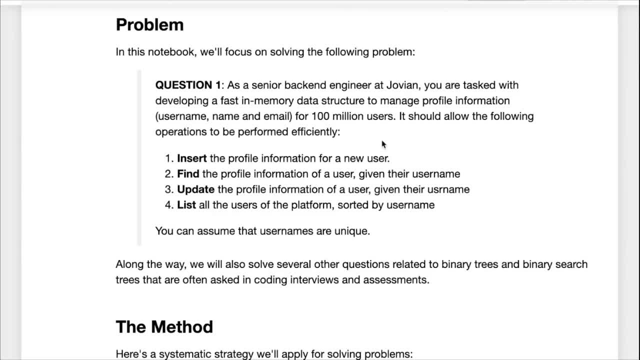 Bye, Binary trees and binary search trees and how to apply them to several other questions. So here's the question. As a senior backend engineer at Jovian, you are tasked with developing a fast in memory data structure to manage profile information, which is username, name and email, for a hundred million users. 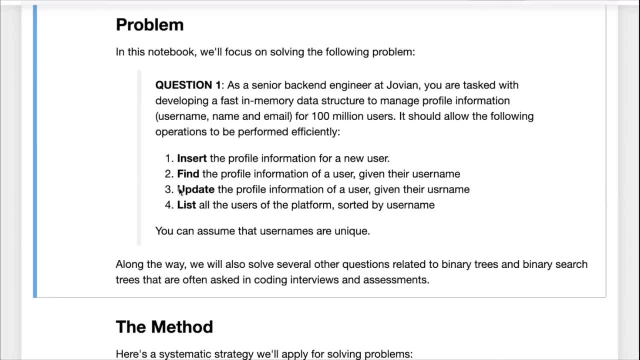 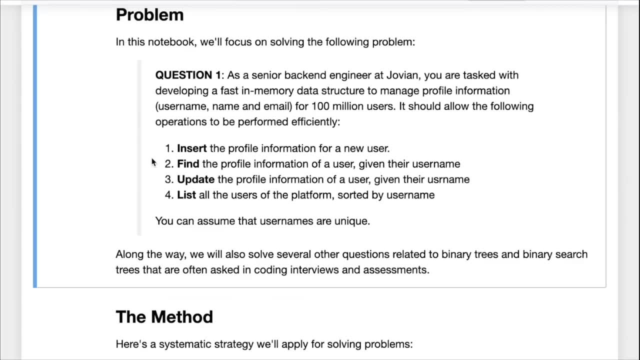 It should allow the following operations to be performed efficiently: You should be able to insert the profile information for a new user, find the profile information for a user, given their username, and then update the profile information of a user, Once again Given the username, and list all the users of the platform sorted by username, and you can assume here that usernames are unique. 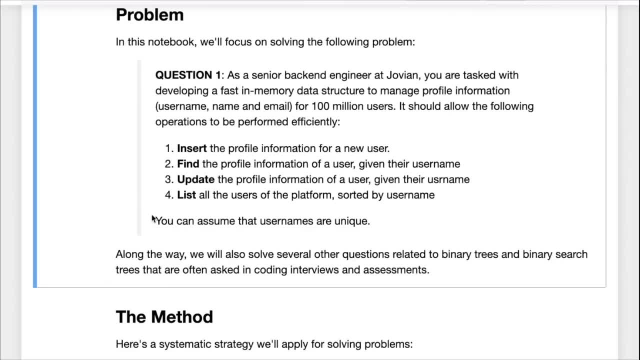 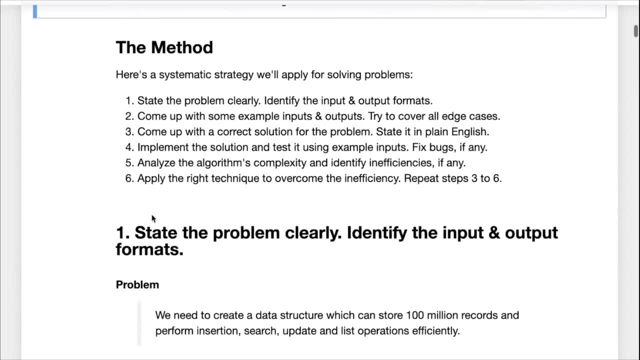 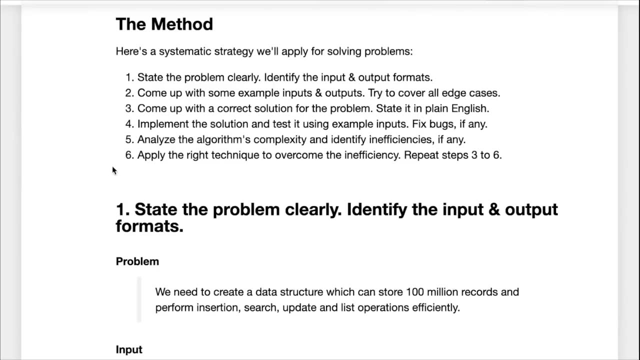 So this is a very realistic problem that you might face if you're working at a company where you have a lot of users. So let's see how we solve this problem Now. here's a systematic strategy that we'll apply for solving problems not just here, but throughout this course. this first step is state the problem clearly and in action. 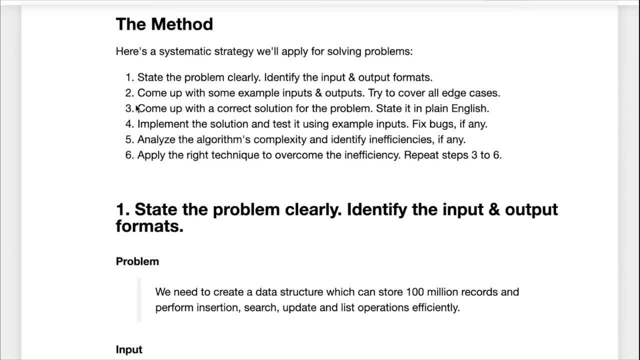 In abstract terms and then identify the input and output formats, then come up with some example inputs and outputs to test any future implementations and try to cover all the edge cases and then come up with a simple, correct solution for the problem. It doesn't have to be efficient. 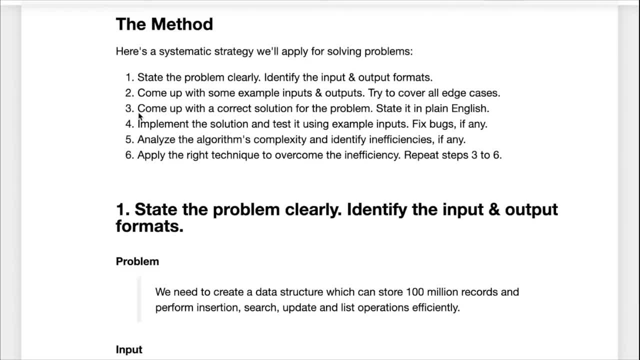 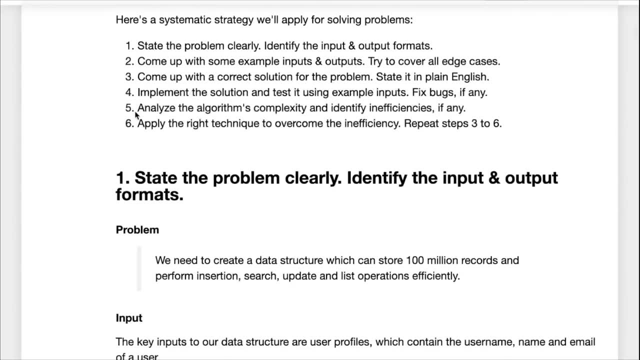 It just has to be correct and stated in plain English- and then implement the solution and test it using some example: inputs, fix bugs if you face any, and finally analyze the algorithms, complexity And identify inefficiencies, if any. Now, once you identify inefficiencies, then we apply the right technique, and that's where data structures and algorithms comes into picture. 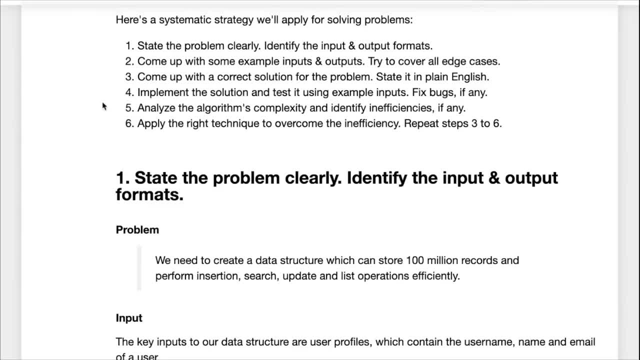 So we apply the right technique to overcome the inefficiency and then we go back to step three. So come up with a new, correct solution which is also efficient, stated in plain English, implement it and then analyze the complexity. Now, if you follow this process, you should be able to solve any programming problem or interview question. 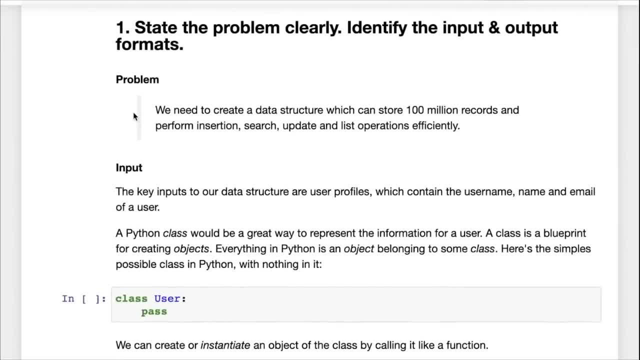 So, step one: we state the problem clearly and we identify the input and output formats. Now we can reduce the problem to a very simple single line statement. We need to create a data structure which can efficiently store a hundred million records, and we should be able to perform insertion, search, update and list operations, all of them as efficient as possible. 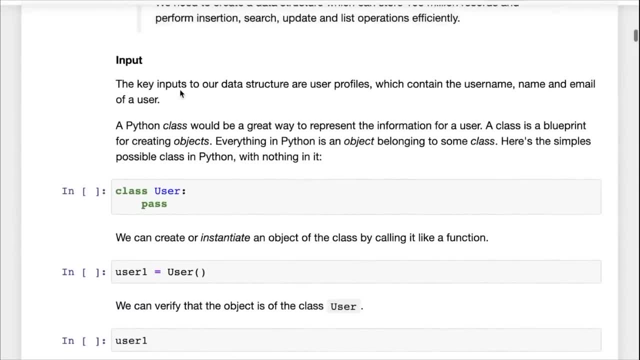 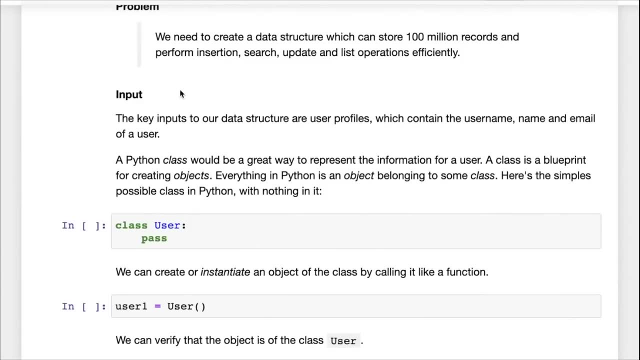 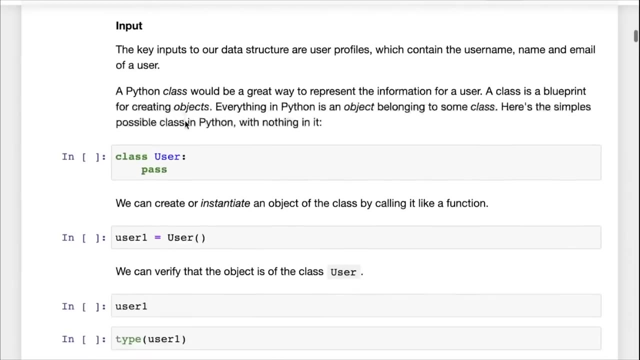 Now the input, the key input to our data structure: the list. The solution that we are building is going to be user profiles, which contains user name, name and email of a user. Now, before we come up with a solution, we need a way to represent user profiles, and a Python class would be a great way to represent the information for a user. 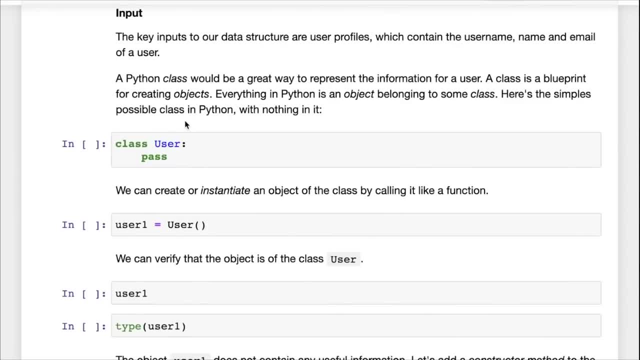 So you may have heard of the term object oriented programming, and that is what we're going to look at now. If you're not familiar with the class, it's very simple: A class is simply a blueprint for creating objects. And what's an object? 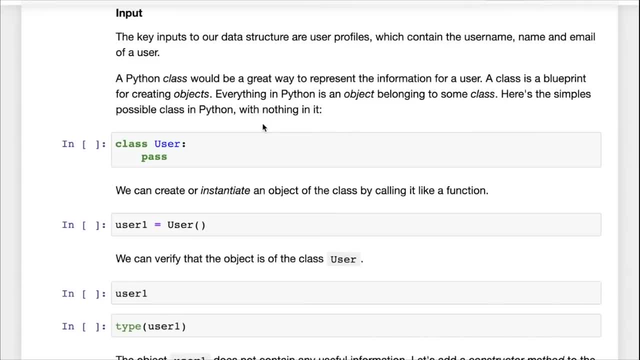 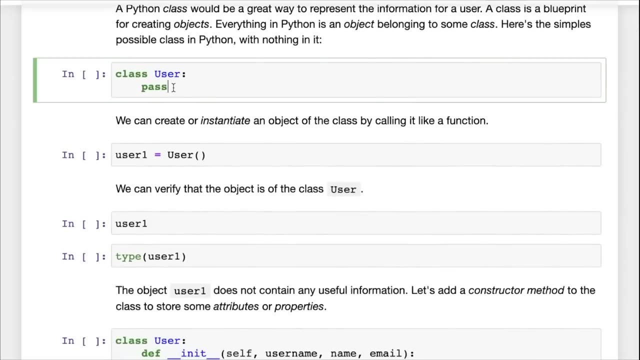 Well, everything in Python is an object, whether you're looking at a number, a dictionary, a list, anything. and you can create your own custom objects with custom properties and custom methods by creating your own custom classes. So here's the simplest possible class in Python with nothing inside it. we are creating a class user. 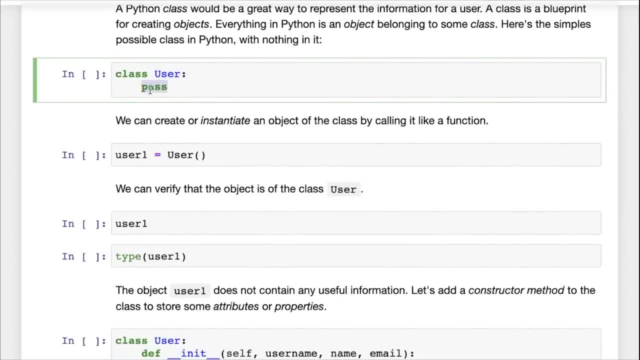 So this is how you declare a class and then when putting nothing inside it. So whenever you put nothing inside a function or a class or anything you can put, you need to put the past statement, because Python cannot accept empty blocks of code. 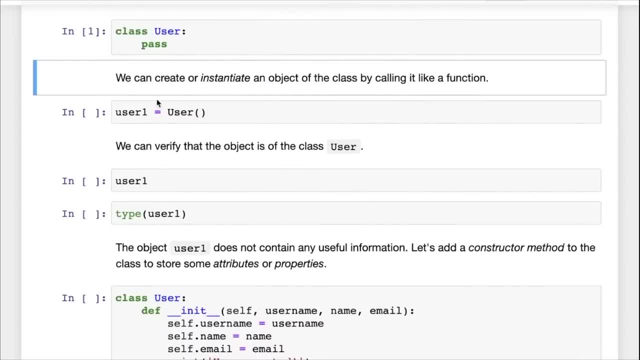 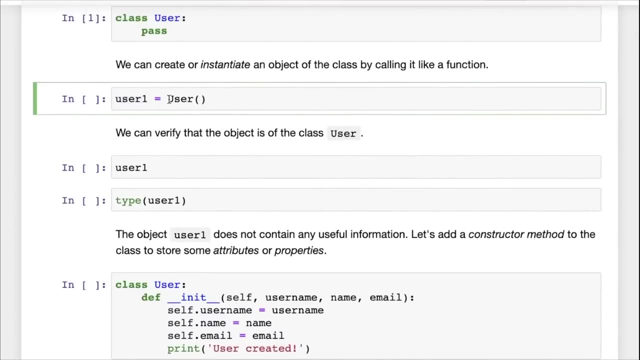 So here we are creating a class which does not have anything inside it, And we can create an object- or it's often called instantiation- which is creating an instance of a class, instantiate an object of the class by calling it like a function. So we say user, one is user. 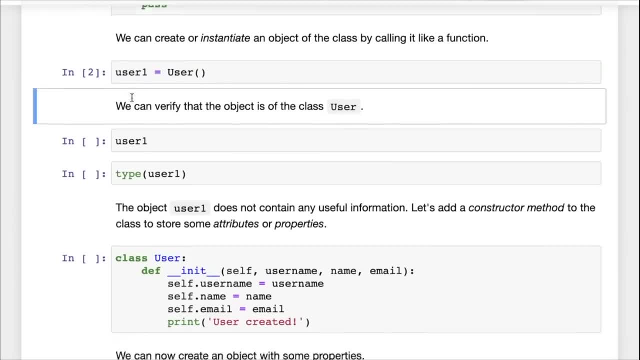 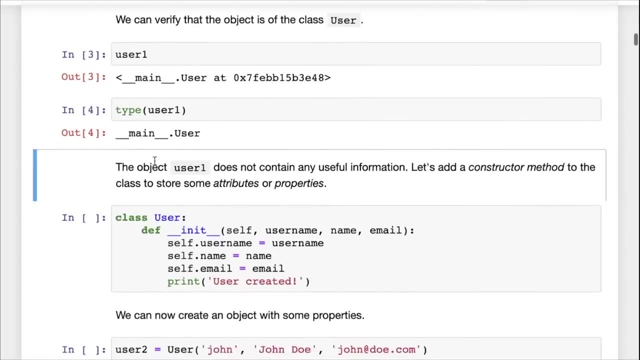 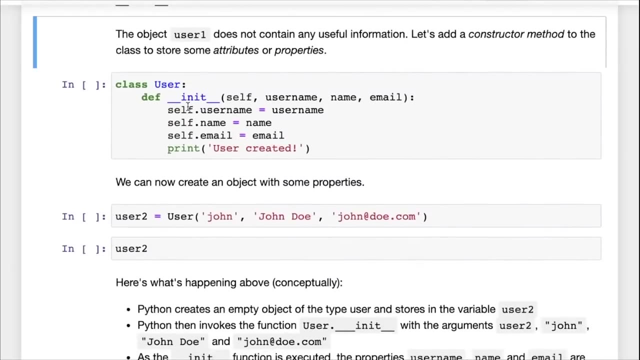 So this creates an object and the variable user one points to that object. Now we can verify that the object is The class user by simply printing it or by checking its type user one and type user one are both user. Now the object user one does not contain any useful information. 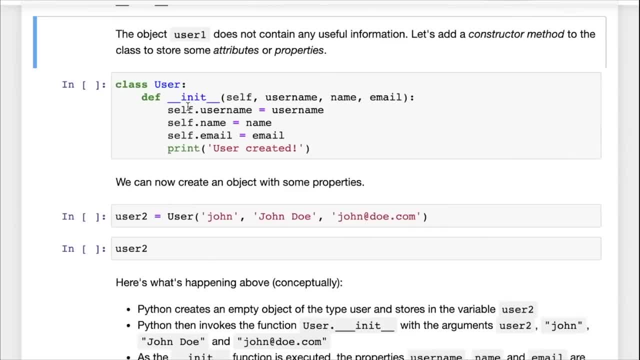 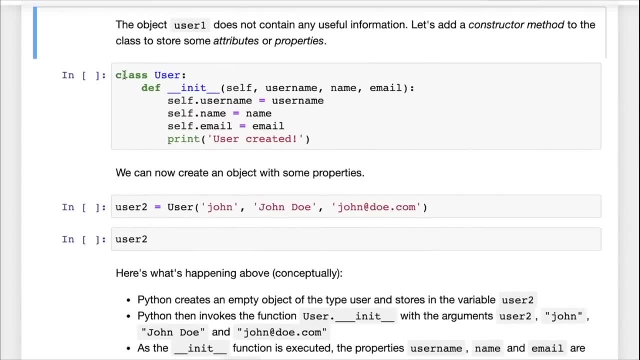 So let's add what's called a constructor method. So constructor method is used to construct an object to store some attributes and properties. So now we're defining the class user once again, but inside it we are defining this function, And you can see that this function is inside the 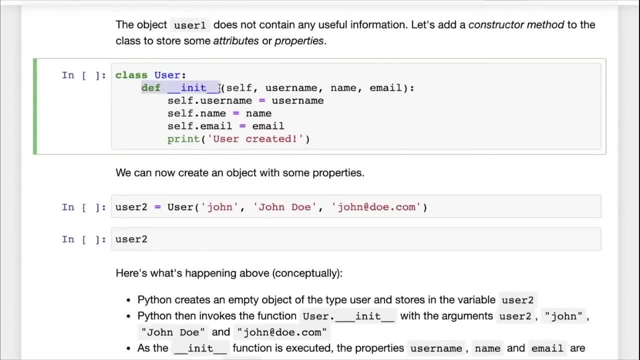 Class, because there is some indentation here. So we define this function underscore, underscore in it, and it takes four arguments. Now, the first argument is a special argument called self, and we'll talk about this. And then we have three arguments: username, name and email. 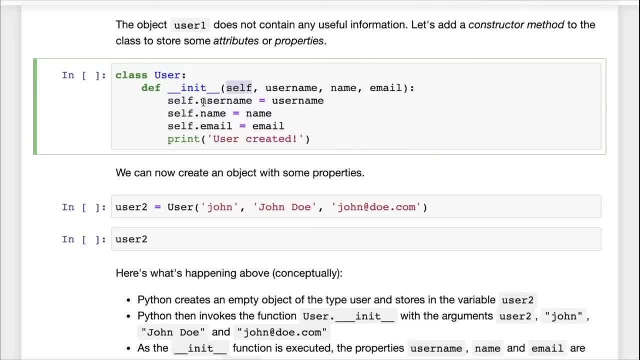 And inside in it what we're doing is we're setting self dot username, So we're setting a property on self to username, We are setting a property on self to name and we're setting a property on self to email And finally we're printing user create. 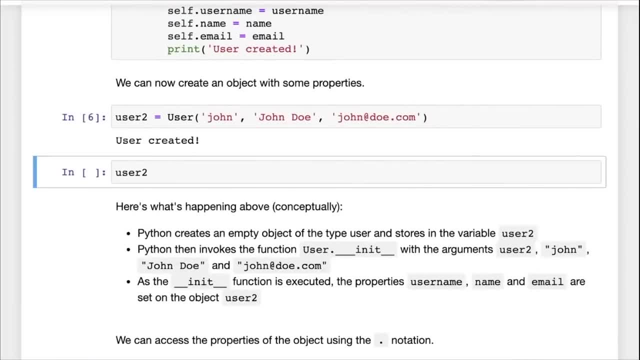 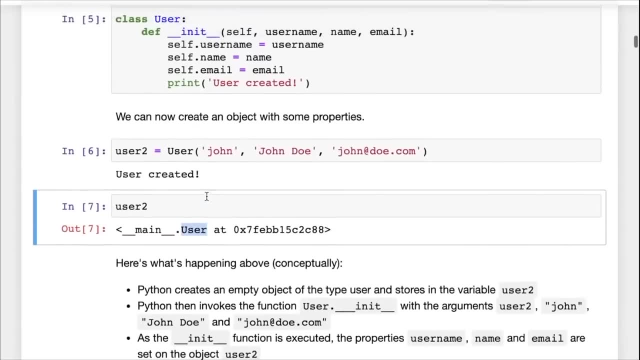 So let's see, let's create another user, user two, And you can see that user two is also an object of the class user. Now here's what happening conceptually When we do this. the first thing that happens is when you invoke this function, when you 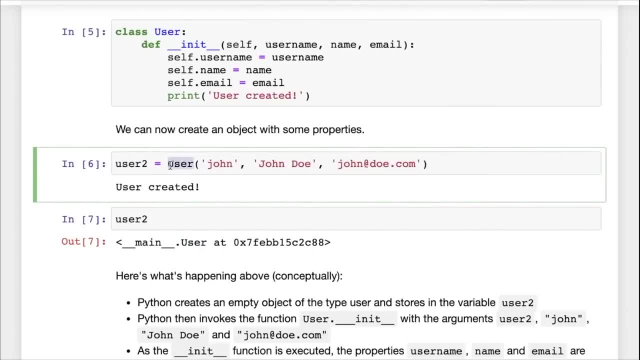 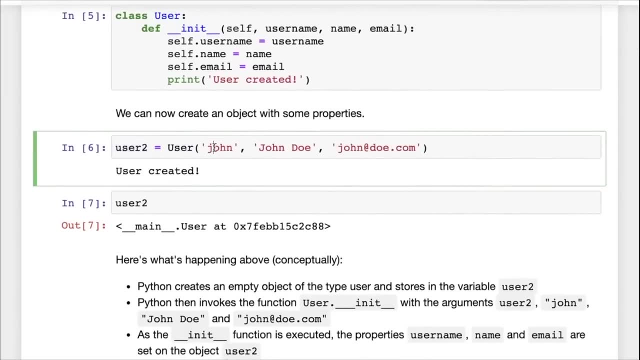 invoke user as a function. Python first creates an empty object of the class user and then stores it in the variable user two, and then Python invokes the init function And to the init function it passes user. to the object that was just created as self and then the other. 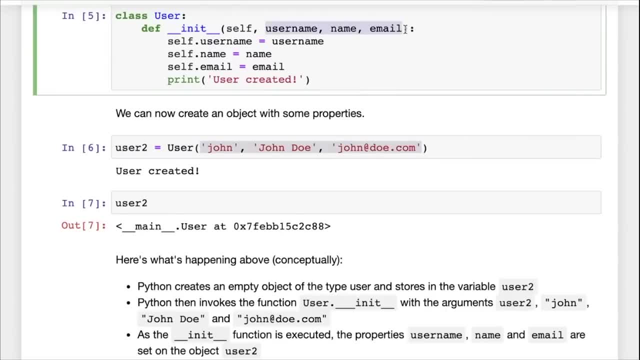 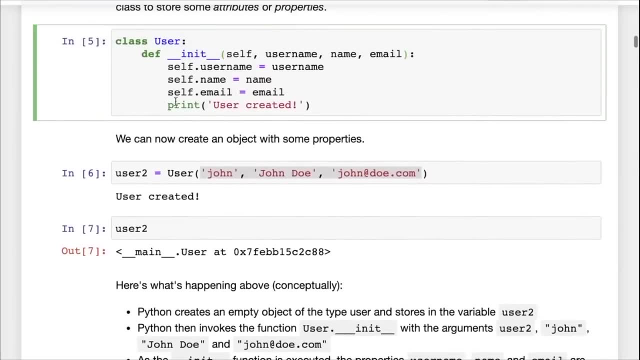 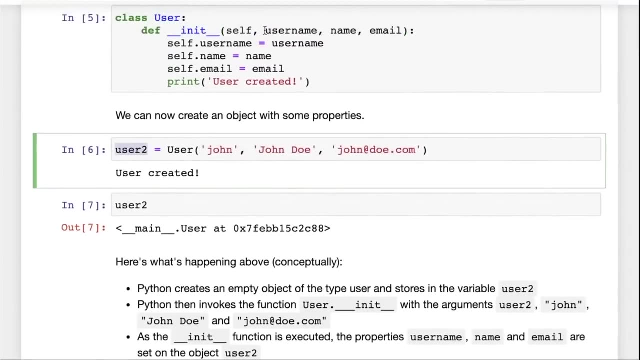 arguments that were passed while creating the object as the rest of the arguments. So you can imagine that we are basically doing. you're basically calling user dot underscore, underscore in it the function, with user two, an empty object, and these arguments, John John. 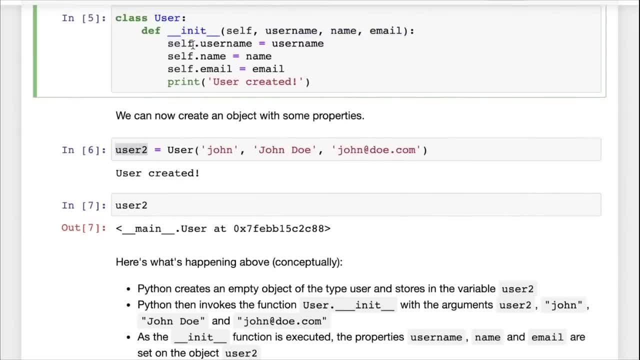 do and John docom, And then inside the unit Function we simply set these properties on user two. So now we get: user two dot username is John, user two dot name is John do and user two dot email is John do. John at docom. 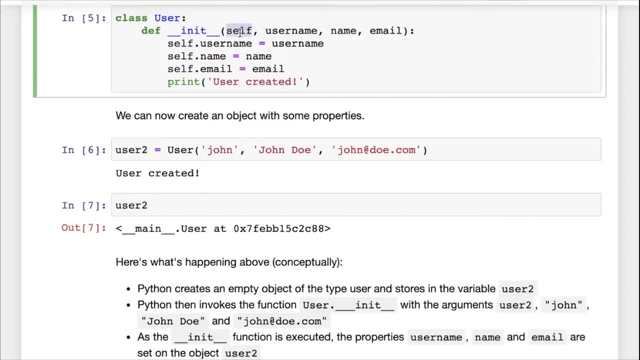 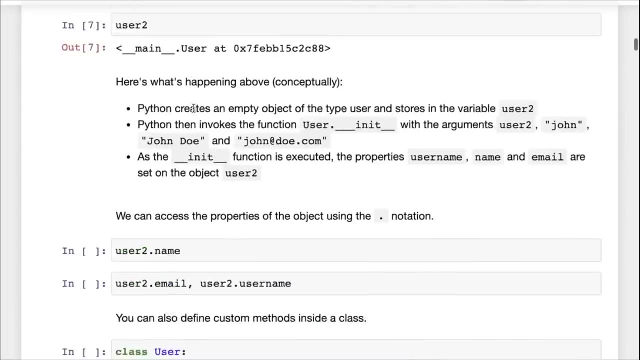 So that's basically how classes work in Python. Then that's why you always have this additional, extra argument in all class methods, which will refer to the object that finally gets created. Okay, So Once user two is Created with the values John, John do and John docom, 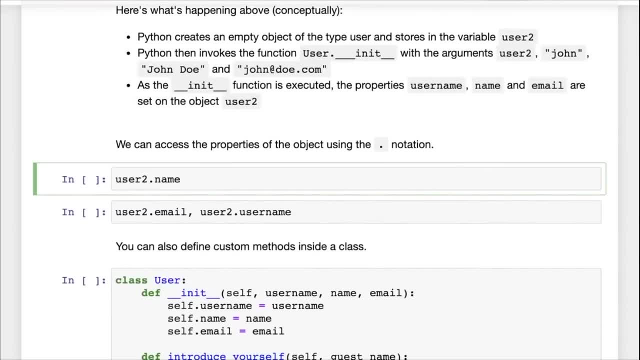 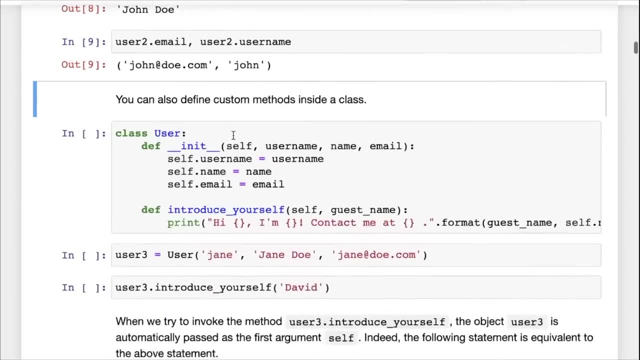 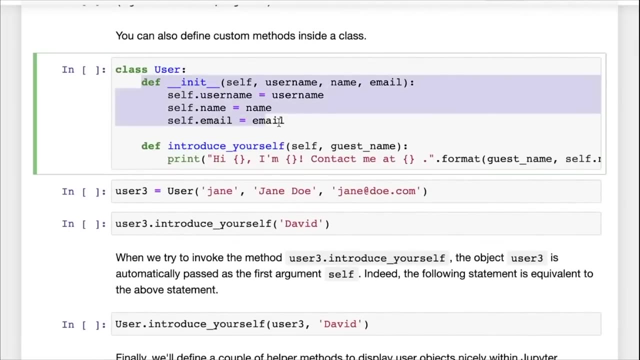 You can check that user two dot name is John do and user two dot email is John at docom and user two dot username is John. Now you can also define some custom methods inside a class. So obviously we had the init method, but here we are also defining another method called introduce yourself. 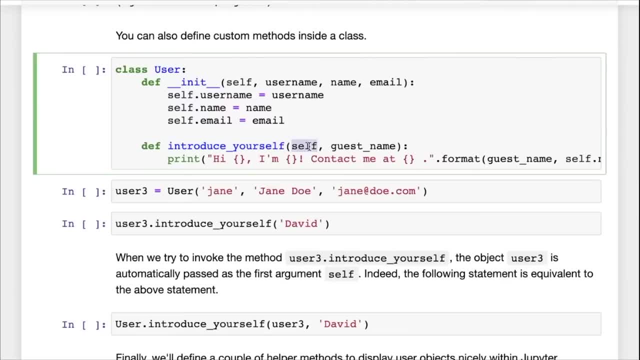 Now introduce yourself. uh, takes again two arguments. The first argument Is self, which will refer to the actual object that gets created later. And then we have a guest name and we basically say: hi, guest name, I am such and such. contact me at such and such. 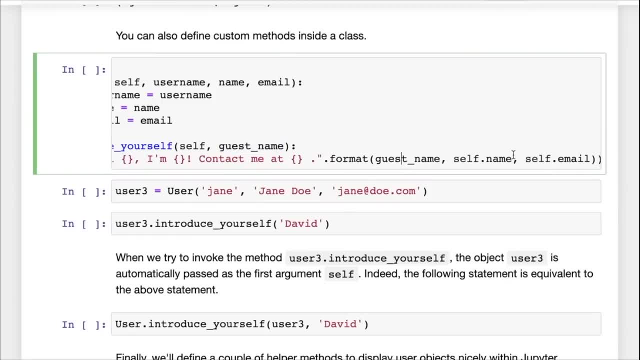 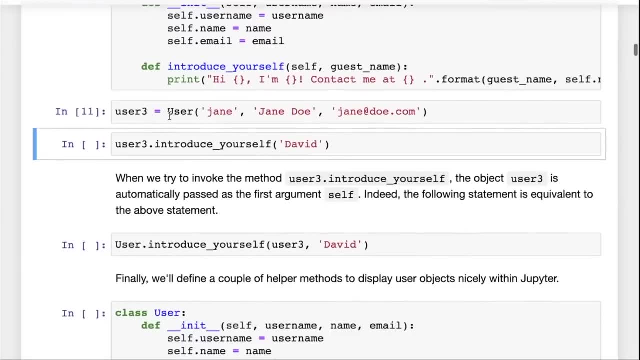 So these blanks are filled in using the guest name, self dot name and self dot email. Okay, So that's how you define a method in a class. So here we have, uh, another user. we're creating Jane and Jane do at, Jane at docom. 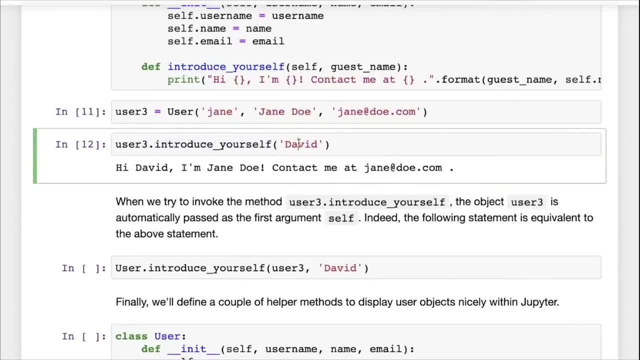 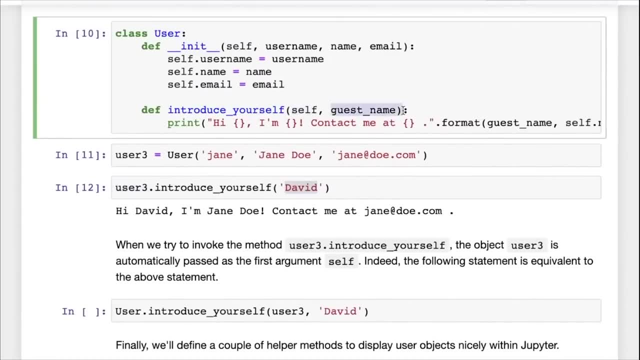 And you can see here that when we Call, introduce yourself with David. So user three, which is Jane, becomes self and then David becomes guest name, And that's why we get: hi, David, I am Jane. do contact me at Jane at docom. 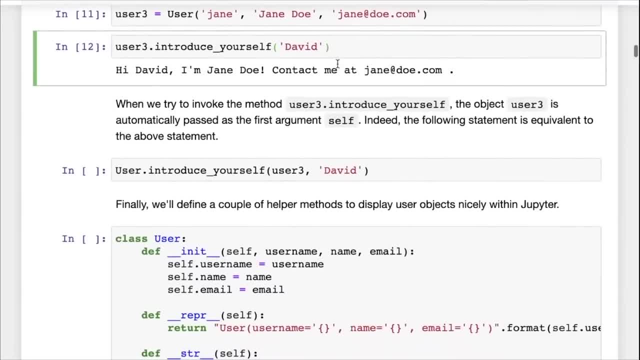 So that's a quick refresher on classes in Python. Now there's a lot more to classes, but the simplest thing you need to know is how to define a class, how to create a constructor um which is underscore underscore in it, how to set some properties. 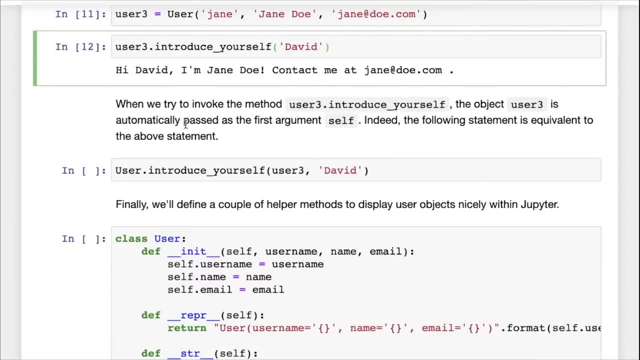 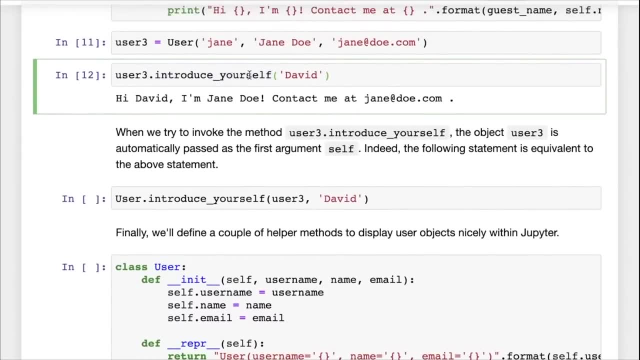 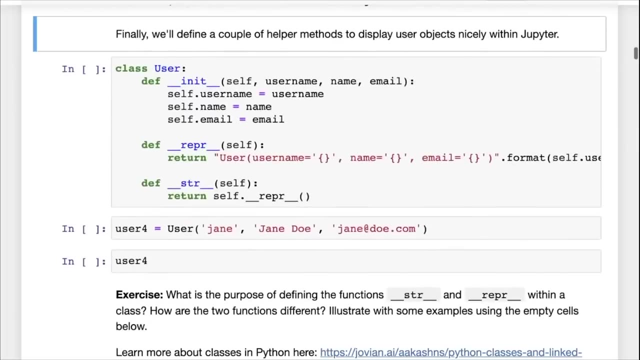 Like we said, the property Name, email and username and, finally, how to define methods. Like we defined the method introduce yourself. and that's all we will need today, So we won't need much more than that. And one final thing that we're doing with our class is we're defining two other special functions underscore. 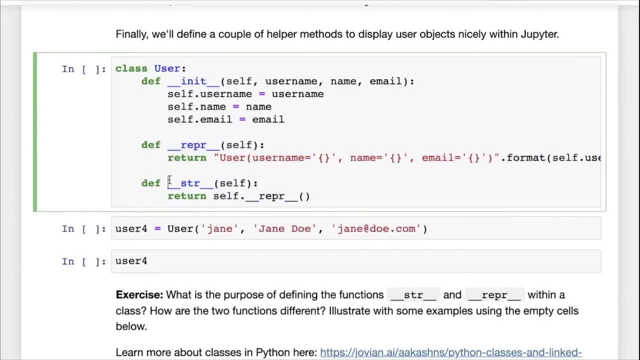 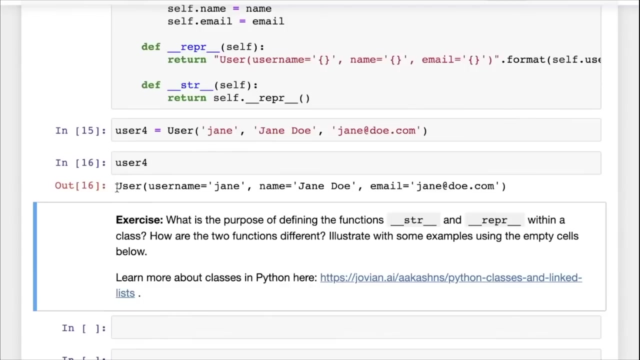 underscore our EPR rapper and underscore underscore STR. So now these two functions. these two functions are used to create a string representation of the object And you can see here, once we create an object, user four now, and if we try to print user four, you can see that user four is now printed like this: 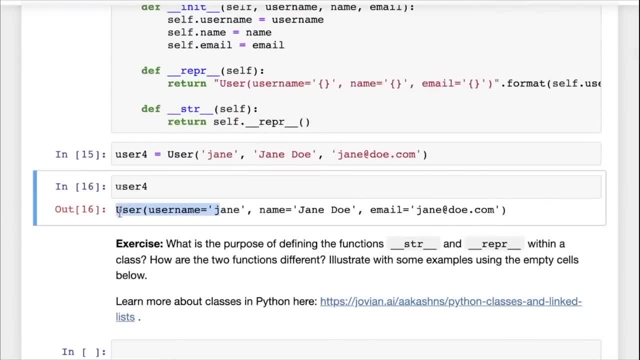 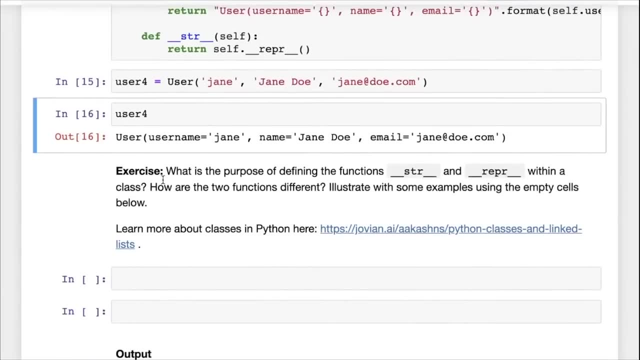 So user three was not printed. I mean, user three was a printed just as a user. but with user four we have all this information printed here As well. So now here's an exercise for you, which also brings us to the first quiz of the day. 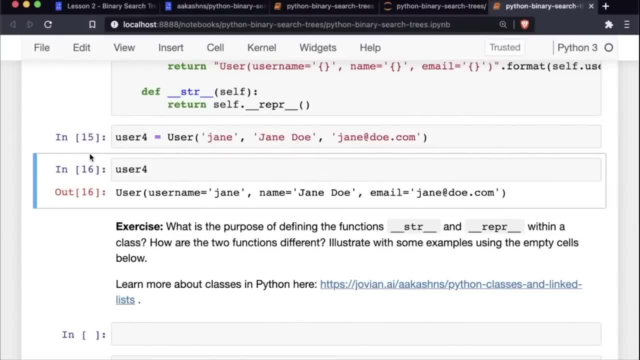 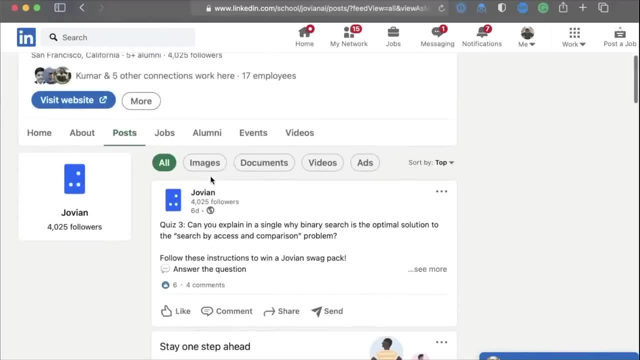 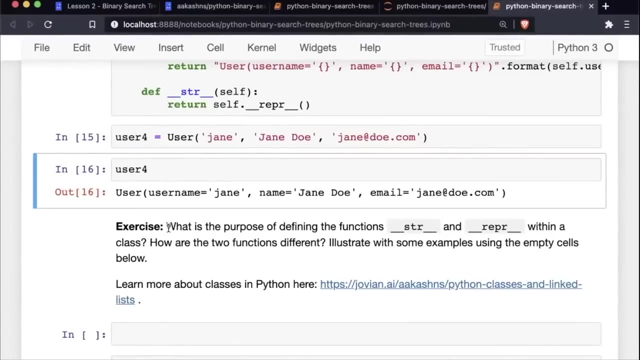 Now we are going to do three quizzes in this video and you can answer these quizzes on LinkedIn. So go to our LinkedIn profile. If you see the posts, you will see a new post here which will give you a question. And the question is: what is the purpose of defining the functions STR and rapper within a class? 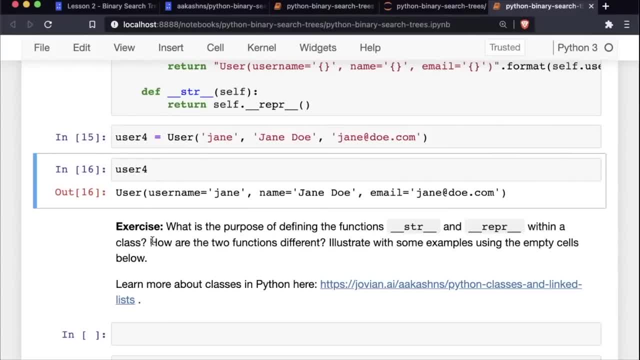 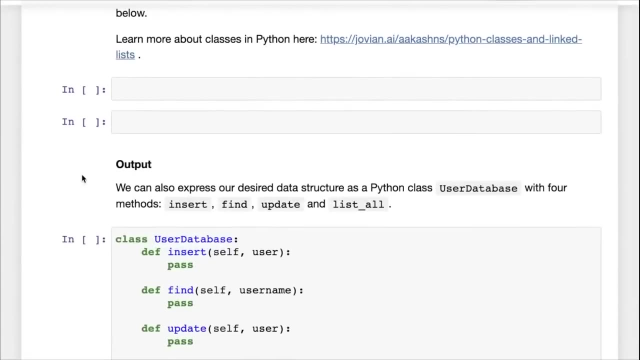 And how These two functions different. now leave a comment with your answer and we will pick the right answer. One right answer And one lucky winner will get a swag back from us. So that was the input we have. We now have a way to represent users by creating classes. 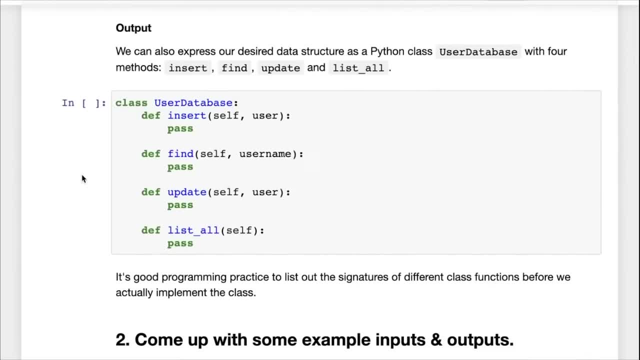 And then the output that we want, the final output that you want to create for our problem, is a data structure. So a data structure is, once again, something that We can Define using a class. So we can define, we can expect our final output to be a class called user database, which has four methods: insert, find, update and list all. 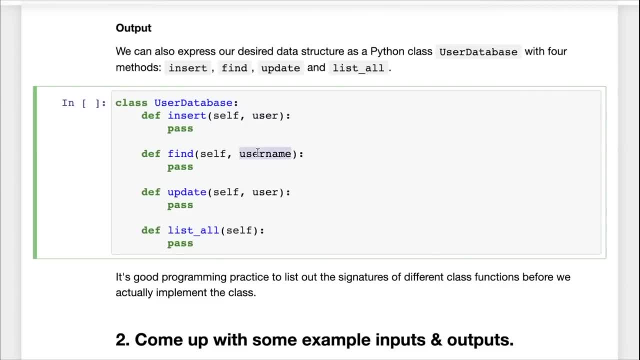 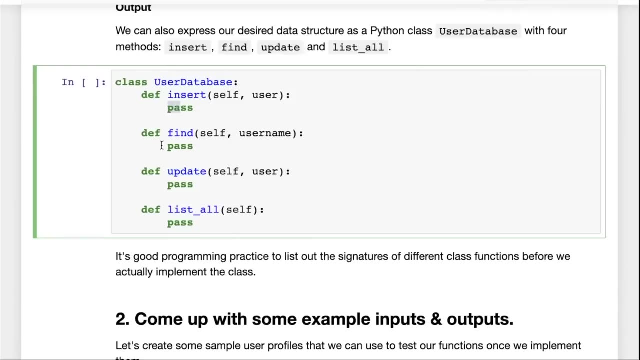 And insert: takes a user and inserts it into the database. Find takes a username and returns the user. update takes a user and updates the data for that user. And finally, list all returns a list of the users. So this is what the class will look like, and we have not implemented it yet. 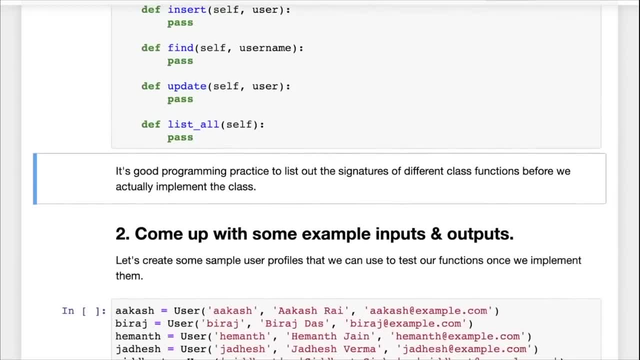 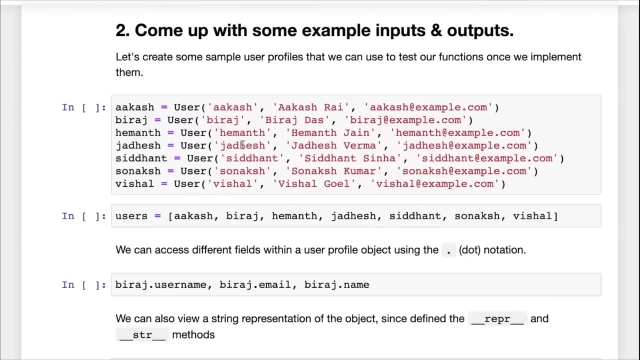 But we now have an interface, So now the next step is to come up with some example inputs and outputs. So let's create some sample user profiles that we can use to test our functions once we implement them. So we're going to create these seven user profiles, and you can see that we're creating these seven user profiles with the username, name and an email and storing them in these variables using the user class that we have just defined earlier. 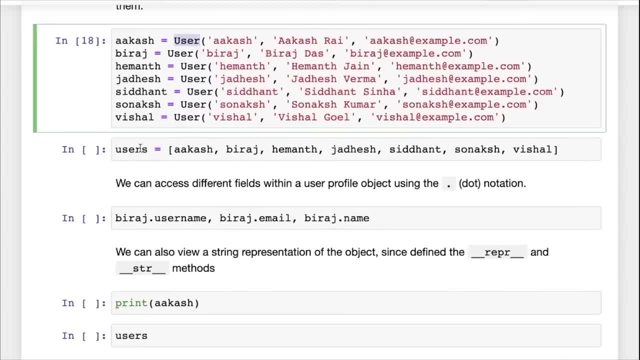 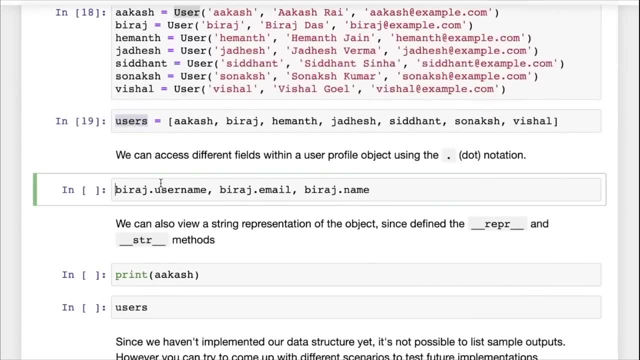 And we're also going to store the user profile. So we're going to do that. Okay, We're also going to store the list of users in this variable called users And, as you can see, we can access different fields within a user profile using the dot notation. 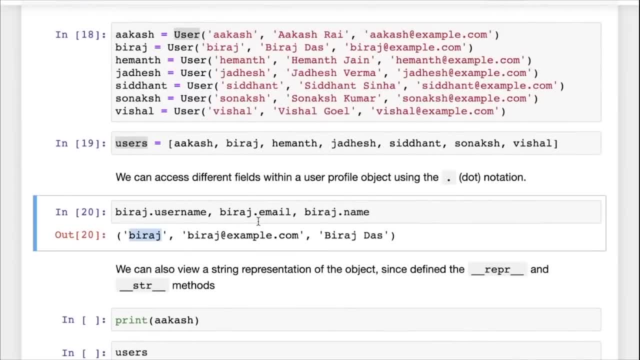 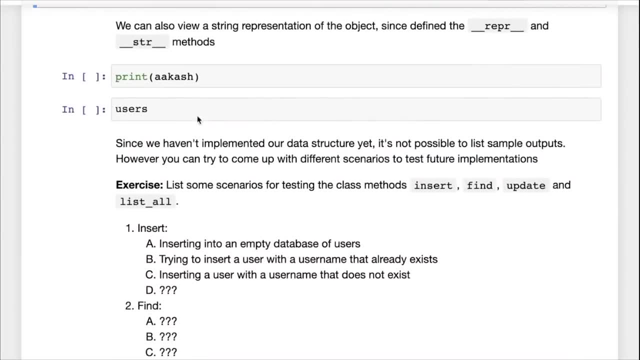 So you can check: barrageusername is barrage and barrageemail is barrageexamplecom and barragename is barragetas. Now you can also view a string representation of the user, as we have seen. So if we print the user, you can see some information about the user. 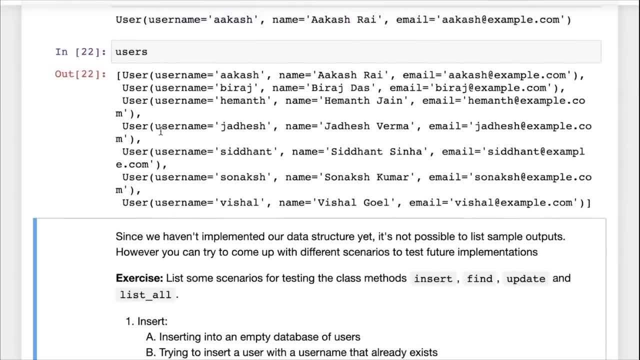 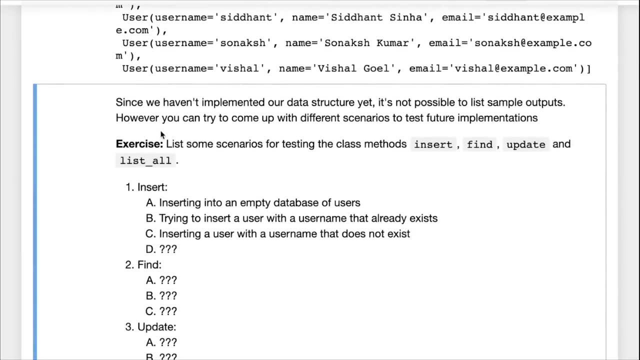 And here is the full list Of users that we have created. So it's always a good idea to set up some input data, set up some test inputs that you can use to test with your implementation later on. And since we haven't implemented our data structure yet, it's not possible to list any sample outputs, but you can try to come up with some different scenarios to test any future implementations. 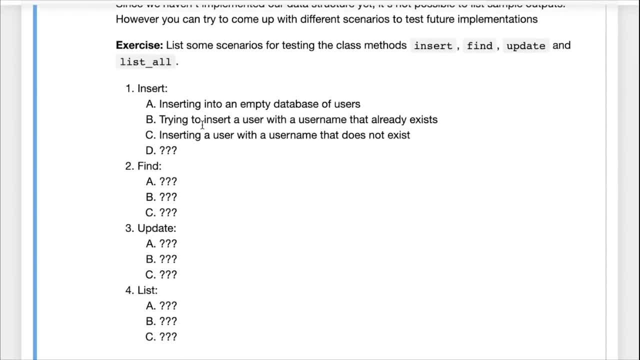 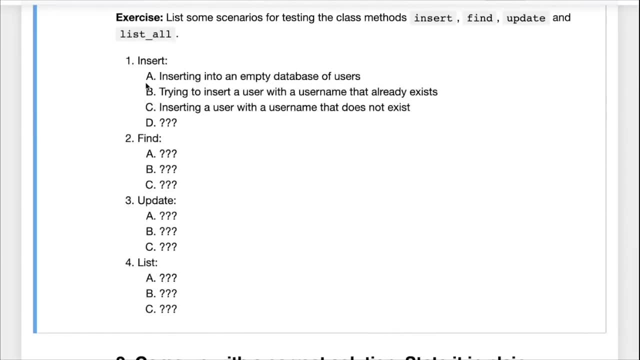 So let's let's list some scenarios for testing the methods of our user database class. So the methods are: insert, find, Update and list all. And for inserting, you may want to test that you're inserting a user into an empty database of users. 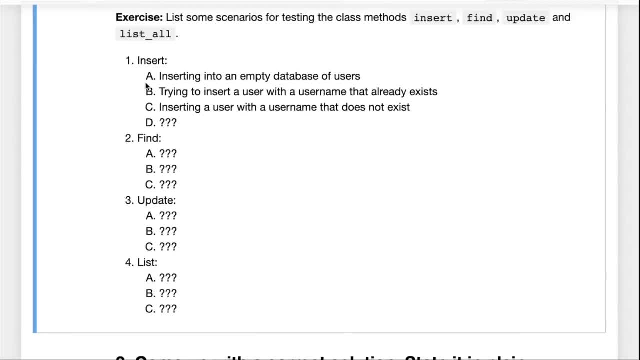 So that's what's called an edge case. And then the general case is to insert a user into the database, assuming that the user already does not exist. Then another edge case is trying to insert a user with a username that already exists, right. 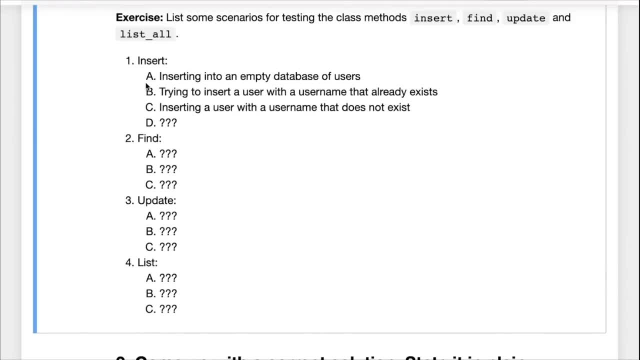 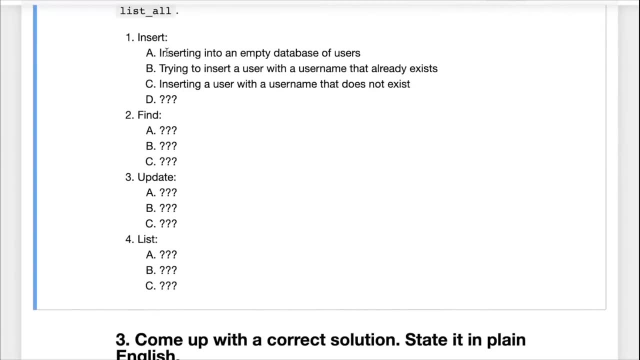 So these are all the different ways in which we can use the insert function, and there can be some more. So here's an exercise for you. Try coming up With all the different scenarios in which you would like to test the different functions: insert, find, update and list. 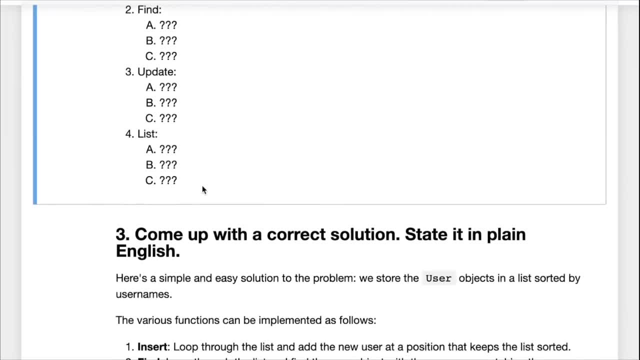 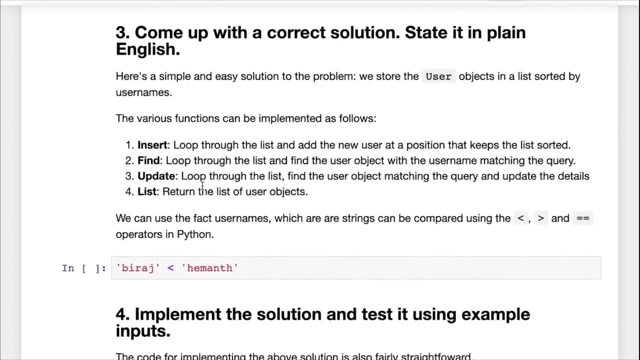 So that complete step two. Now we have some sample inputs and then we have some scenarios in which you we are going to finally test our function. So the next step is to come up with a simple, correct solution and then state it in plain English. 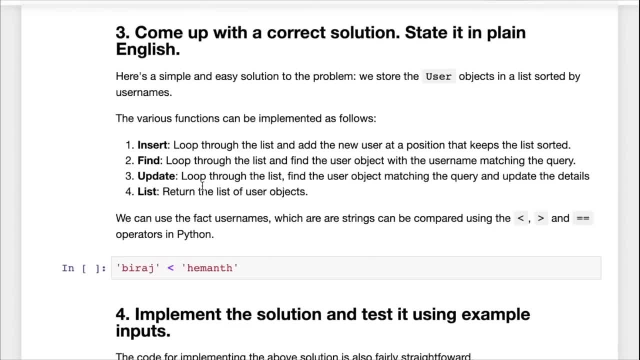 Now here's a simple and easy solution to the problem. We simply store the user objects in a list sorted by usernames. That's simple enough, And suppose we do that. So inside our data structure we have a list which simply contains a bunch of user objects. 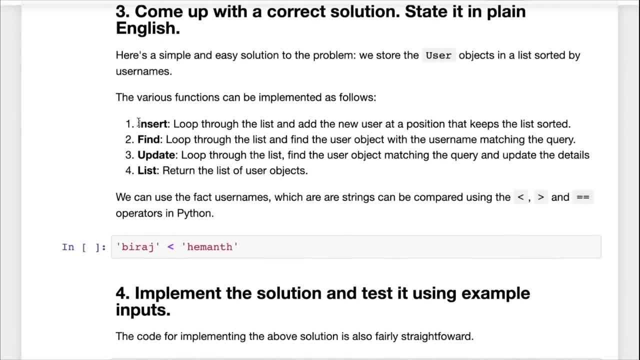 Then the various functions can be implemented like this. So you have the insert function. the insert function simply requires looping through the list and then adding the new user at a position that keeps the list sorted. So, for instance, if you have the users 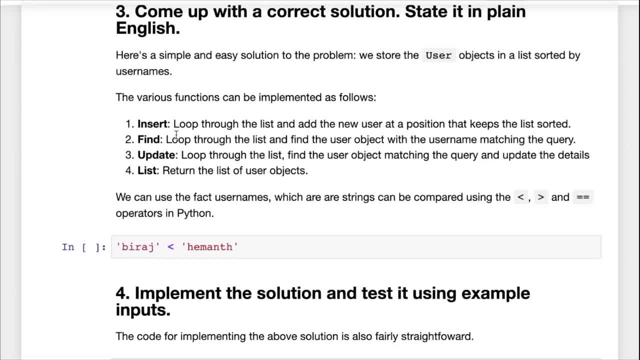 Akash, Hemant and Siddhant already, and then you're inserting the user Biraj. Then you can tell that Bharat should go between Akash and Hemant in alphabetical order. So that's how you insert a new user and maintain the sorted property of the list. 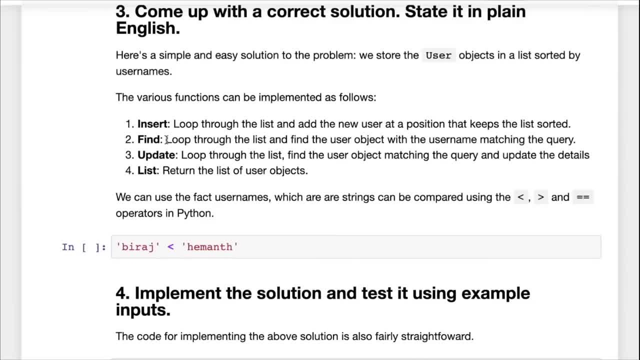 Then to find a user, we simply loop through the list and then find the user object with the username matching the query. So that's you. If you're looking for him, For instance, you start from the beginning. you go through Akash. 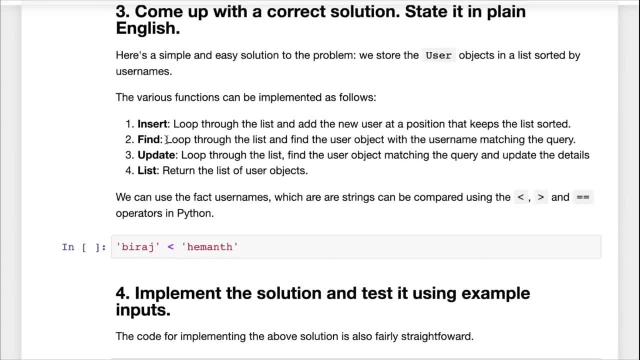 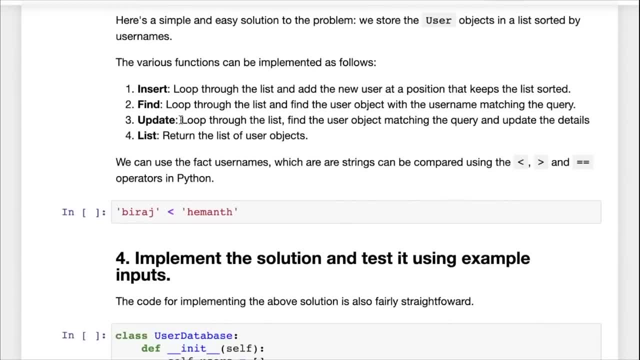 Paraj and finally hit Haman, and then you can retrieve the user object associated with Haman And then you have update. now updating is very simple as well. It's similar to find. So you find the user object matching the query and then update the. 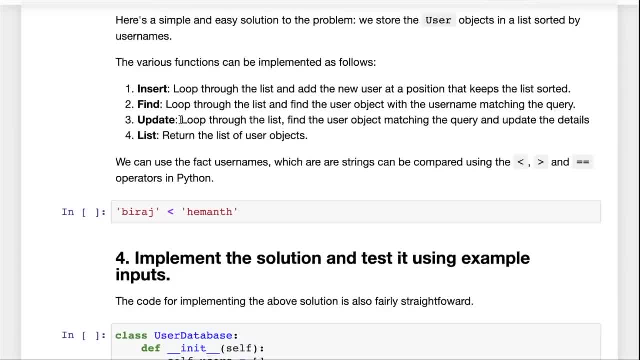 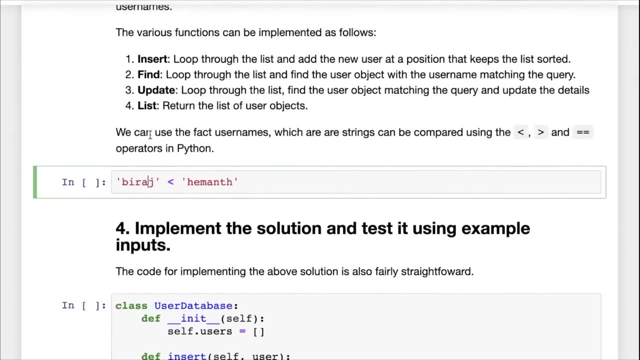 details of that user object. And then, finally, because our internal representation is already a list of user objects sorted by usernames, So we can simply return that list when we want to list the users. So that's a plain English description and it's always a good idea to describe. 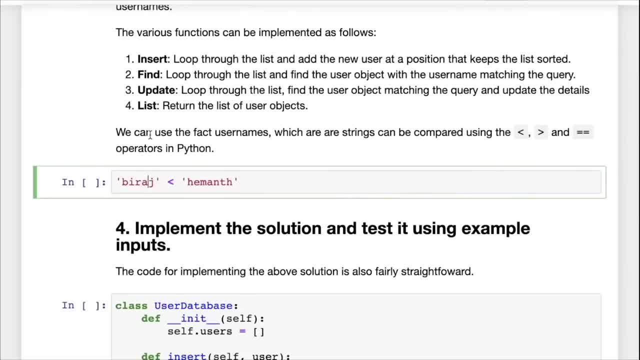 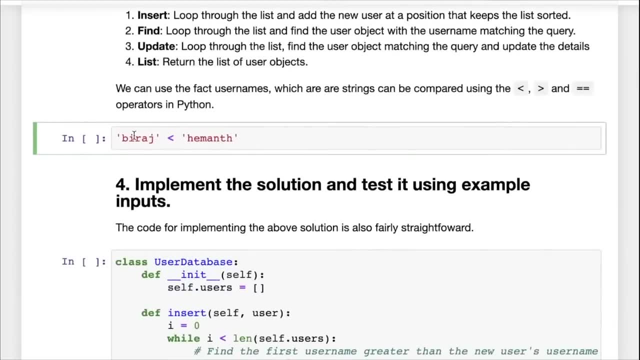 your solution in plain English so that you can clarify any doubts you have. And even during interviews, it's a good idea to have a conversation with the interviewer before you actually implement the solution. And now, one fact that we can use to help us understand the solution is that 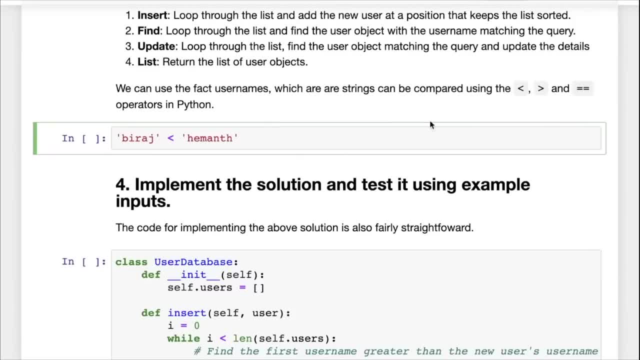 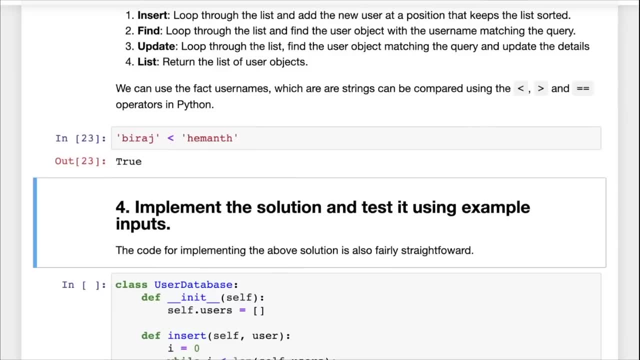 there are a few things Is that usernames, which are strings, can be compared using the less than, greater than or equal to operators, So we can compare strings just like numbers in Python. So that'll make it easy for us to implement these functions. 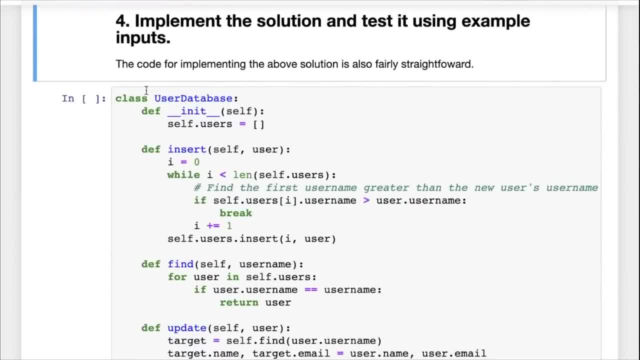 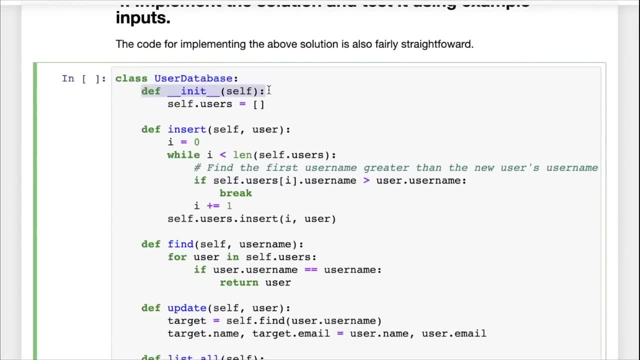 And that brings us to the implementation, and the code for implementing These is also fairly straightforward. So now we have the user database class. We are actually implementing this class, And here you see that we have a constructor and the constructor does not take any. 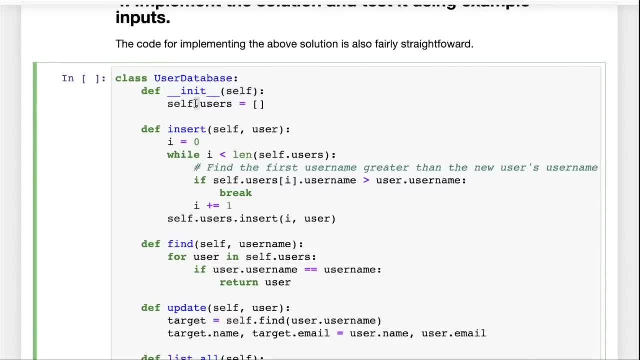 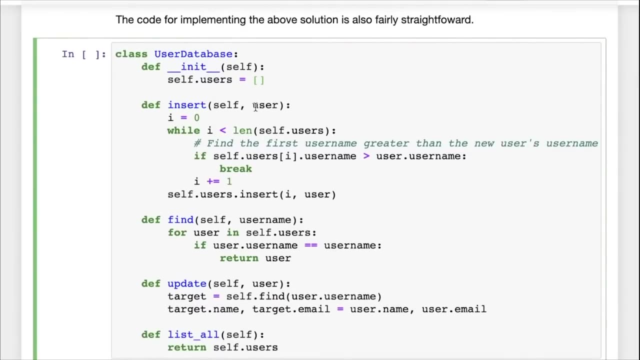 additional arguments apart From self, And all we do is inside self. we set a property dot users and that property dot users is set to an empty list. Then we come to insertion. So now assume that we already have some users in our user database. 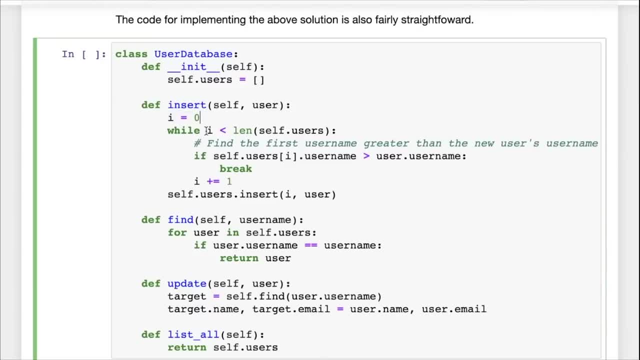 So we start out with a pointer set to zero and we go through all the valid positions in the users list, So which is from zero to N minus one if there are N users, and then we find the first user name greater than The new users usernames. 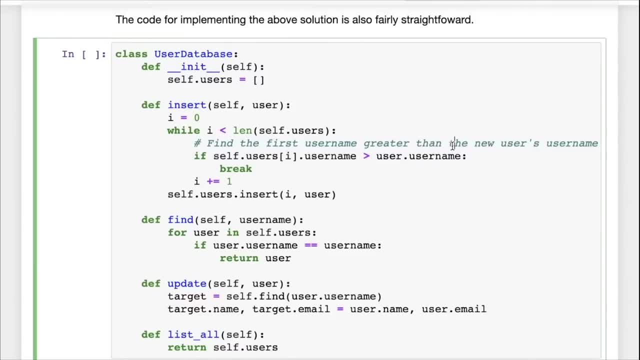 So, for instance, if you're inserting uh, Hey, month, then you go through Akash and barrage and then finally you realize that the next value is probably said hunt. So you want to insert him and before sit on right. So you want the first username that's greater than the new users username and you check this property. 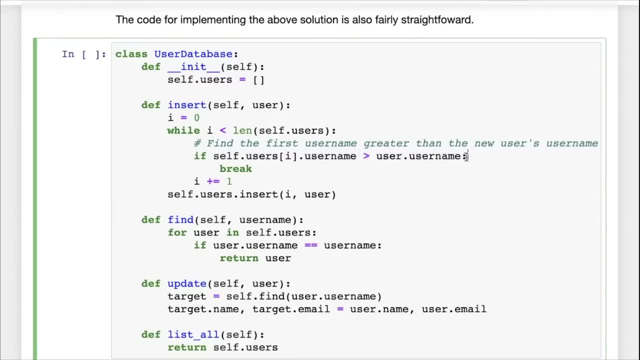 And as soon as you find the next, that the next user is greater than the, the user that needs to be inserted, We break out And then we insert that user at that position. Okay, So this is the insertion. You can just four or five lines of code. 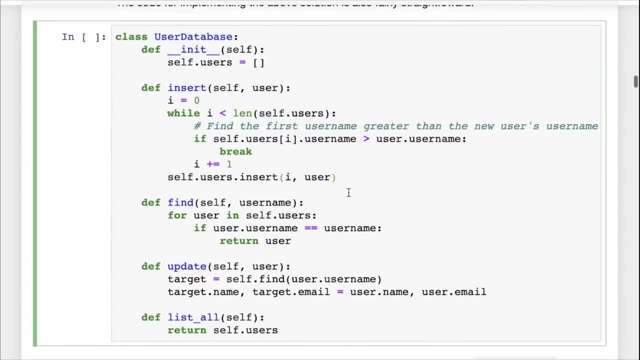 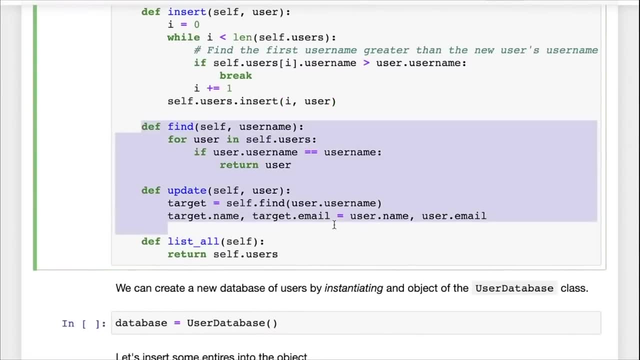 So you can work through this code. try to read this code line by line and see how it works Now. similarly, you have the fine function, the update function and the list function. They're all pretty straightforward. There's really not much here. 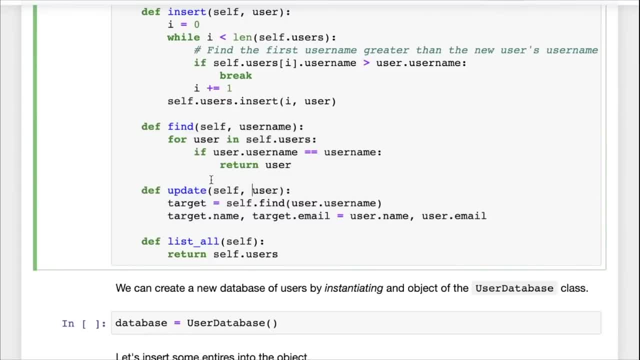 So this is an exercise for you, because this is also the brute force of the simple implementation. So this is an exercise for you to go through each of these functions and try it out And use the interactive nature of Jupiter to experiment and add print statements inside each of the functions. 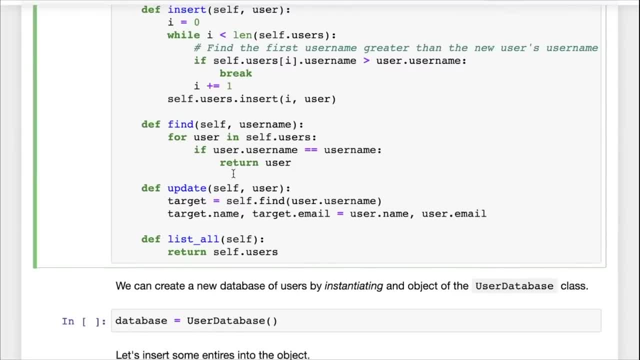 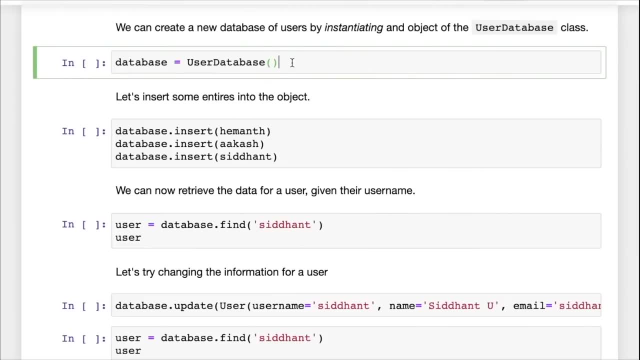 If you need, inside each of the loops, if you need more visibility into what's happening, Okay, Uh, but what we will do is we will try and test this implementation out, And the first thing we do is instantiating a new database of users using the user database class. 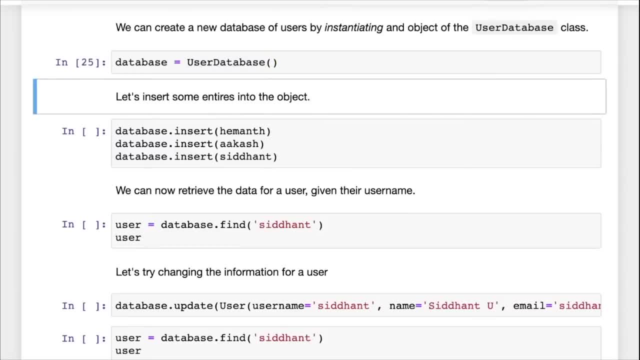 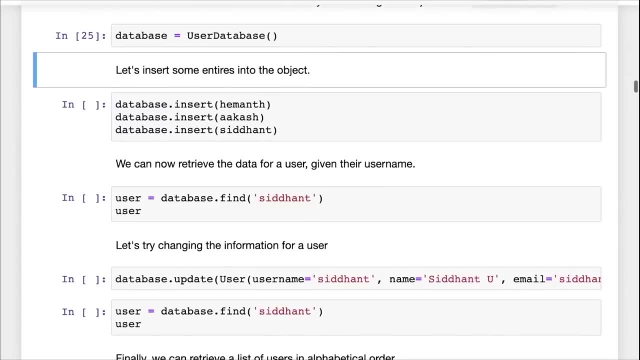 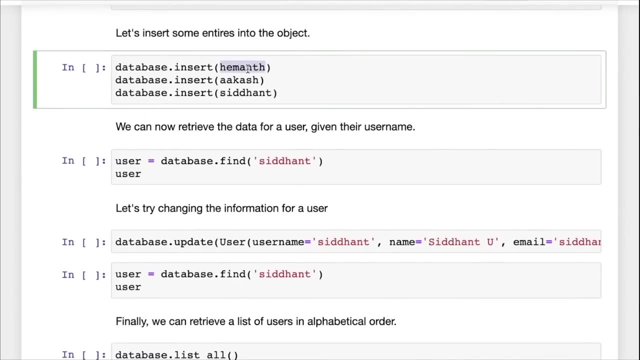 So here we say user database, and that gives us a database, Okay, Of users. And now let's insert some entries into this database So we can now insert. for instance, we can insert the value Hey man, Akash and Siddhant. 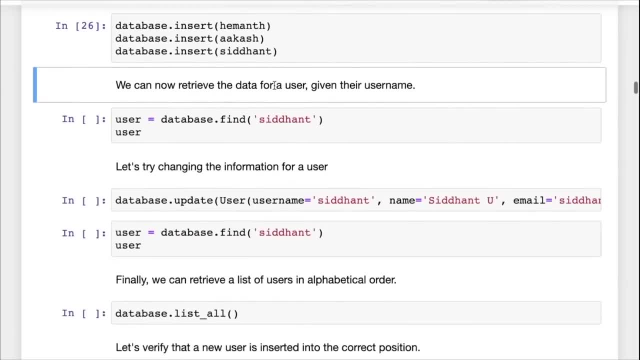 So here we have inserted three values into the database and now we can retrieve the data for a given user, given their username, using the find method. So now we say database dot find, So Done, That returns a user and we can check the value of user. 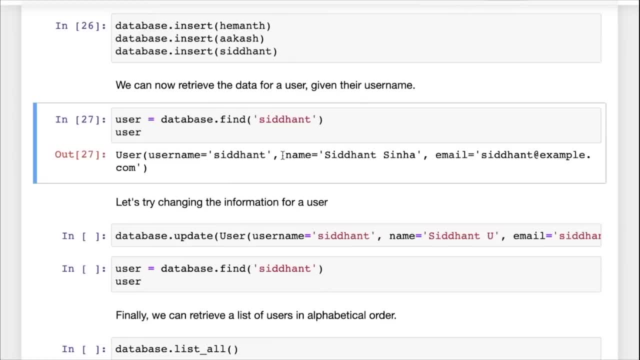 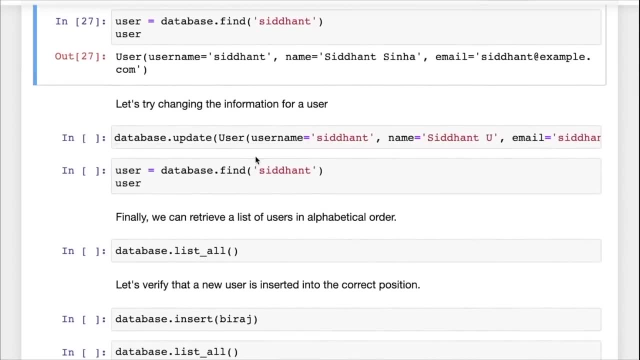 And you can see that now we have retrieved the data for Siddhant, which is username Siddhant, name Siddhant Sinha and email Siddhant at examplecom. Now let's try changing the information for a user. So to change the information we can call database dot update and then simply pass in a new user object. 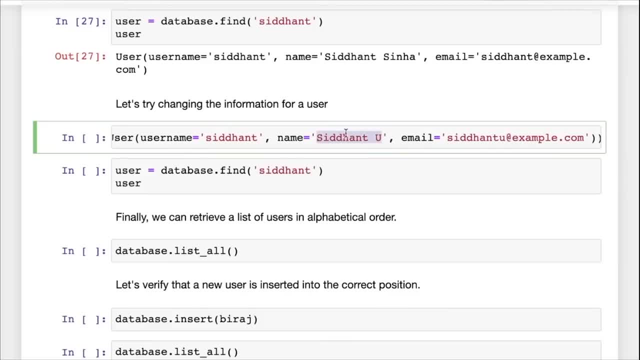 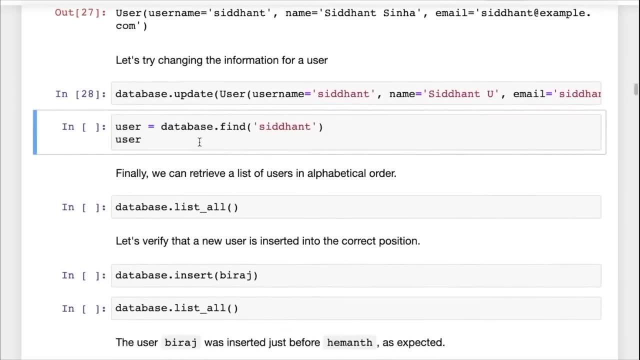 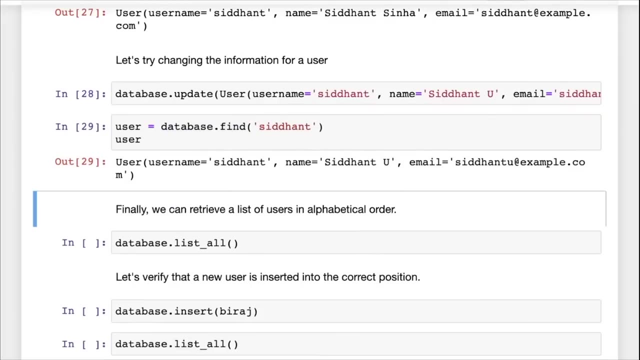 So let's say we want to change the information from Siddhant Sinha to Siddhant U. So this is how we do it: We call database dot update And now if we find the information once again, now if you can't find, called database dot find. once again we get back a user object and this time with the updated information. 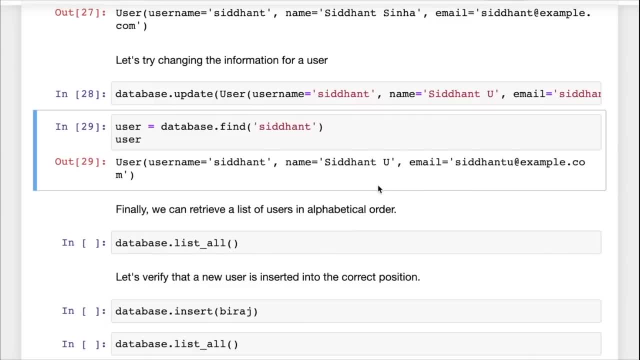 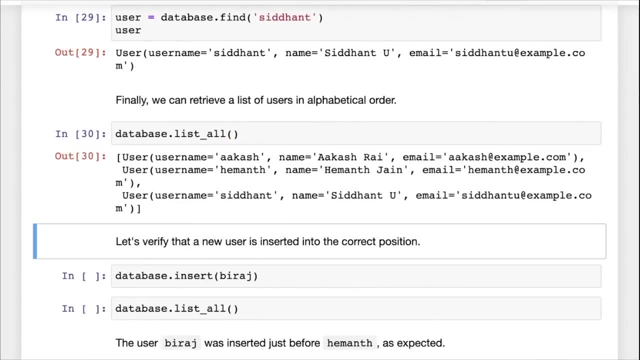 So we have created the database, We have inserted some values into it and then we have retrieved values out of it And we've also updated them. And finally, we can retrieve a list of the users in alphabetical order. Okay, Okay. 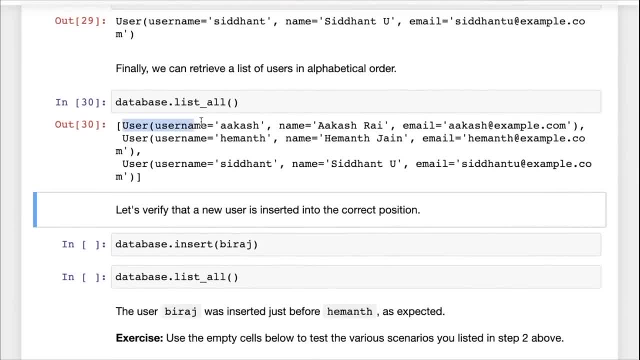 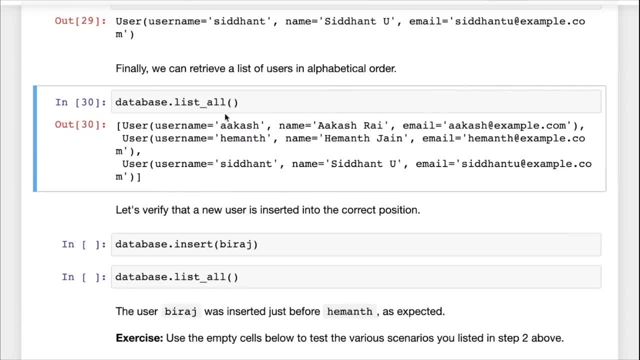 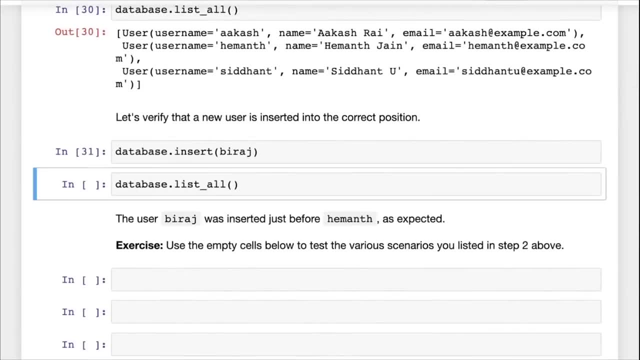 We have the username himant And we have Siddhant. These are the three values that were inserted and they are all in alphabetical order of username. Now if we insert a new user- let's say let we insert barrage- We can make sure that barrage is inserted into the right position. 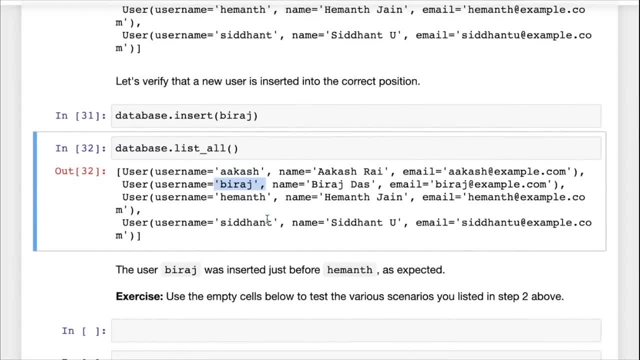 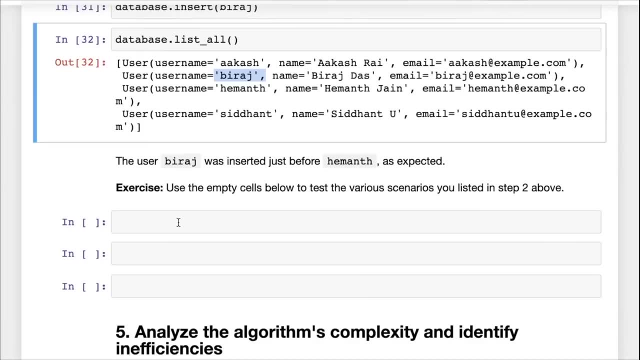 Okay, So that's how we use the data structure that we just created, And you can use the empty cells here to try out the various scenarios when you run the notebook. So just to recap, we created a simple class inside which we are storing a list of users in sorted order of usernames. 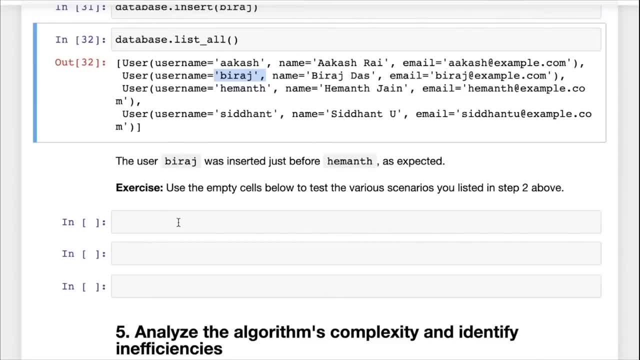 And then insertion is pretty easy. We simply loop through, find the right position and insert any new values. Finding values is very easy as well If we simply loop through and keep comparing and updating values is simply a matter of finding them and then updating that specific value. and listing is simple because we can simply return the internal list. 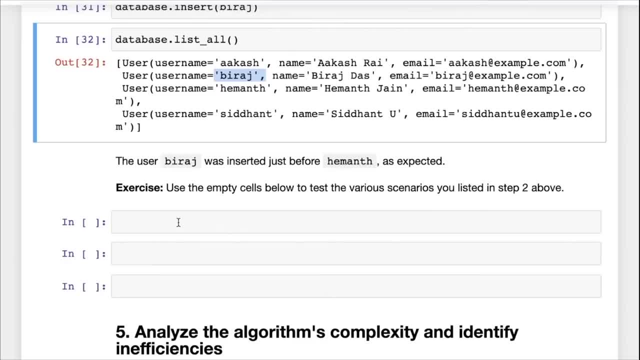 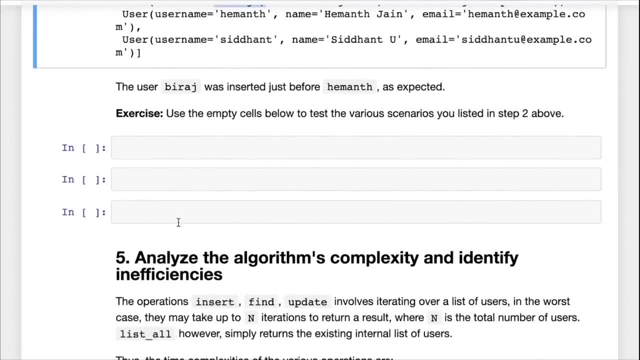 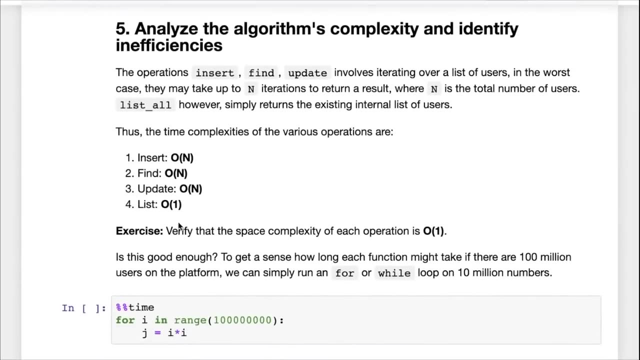 representation that we're already storing in the sorted order of usernames. So that's the simplest solution, or one of the simplest solutions. There can be even simpler solutions, maybe. So the next step now is to analyze the algorithms complexity and identify any inefficiencies. 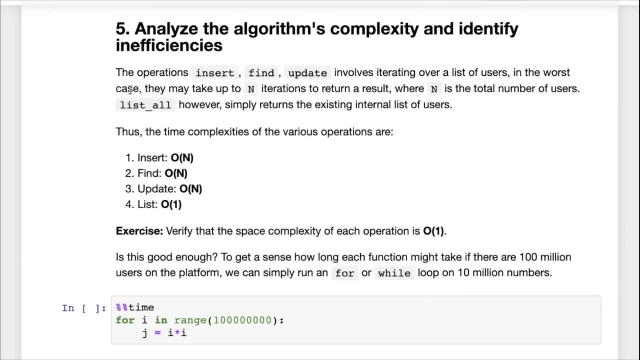 So typically in an interview setting, you may not want to implement the simplest solution, So you can actually skip step four. You know, when you've described what the simplest solution is in English, in plain English, which was step three, you can directly jump to analyzing its complexity and then move on to optimization and implementing the optimized version. 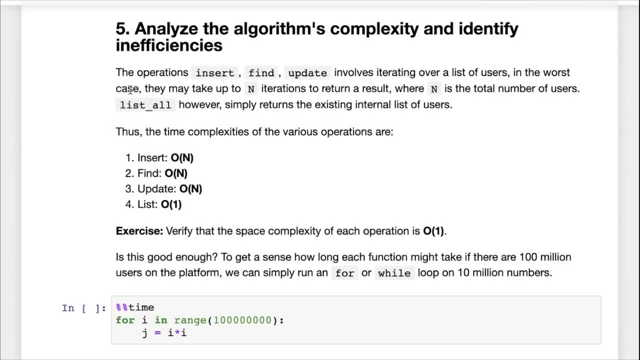 But when you are practicing or when you're learning, it's always a good idea to implement even the brute force solutions. So let's analyze the complexity. the operations insert, find, update involve iterating over the list of users And in the worst case they may take up to N iterations to return a result where N is a total number of users. 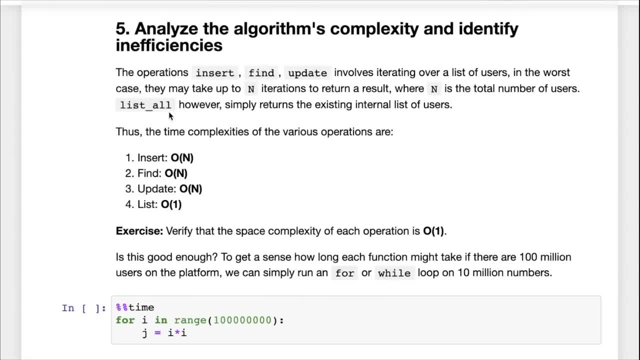 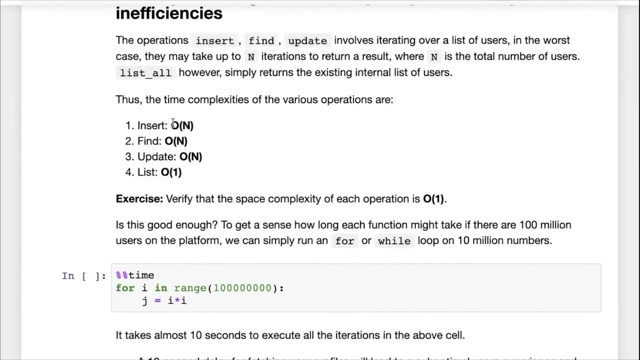 Now the list all function is slightly different because it simply returns an existing list. So the list all function does not take linear time, It takes constant time. Now, based on this information, it's very easy to check, to guess the time complexities of the various operations. insert, find and update. have a order N. 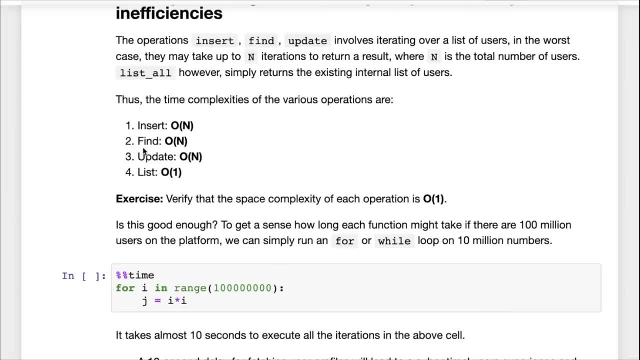 This is the worst case. time. complexity, which means they can take up to N iterations. However, the list function has an order one. complexity, which means it, irrespective of how many users you have in your database, it returns the list in the same amount of time. 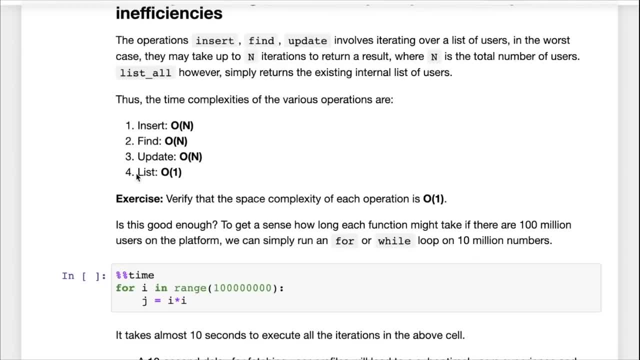 Now, if you want to display the list or if you want to iterate, or the list, that may take you additional effort, but getting the list itself is a constant time operation. Okay, Okay, Thanks, Bye, Bye, Bye, Bye. 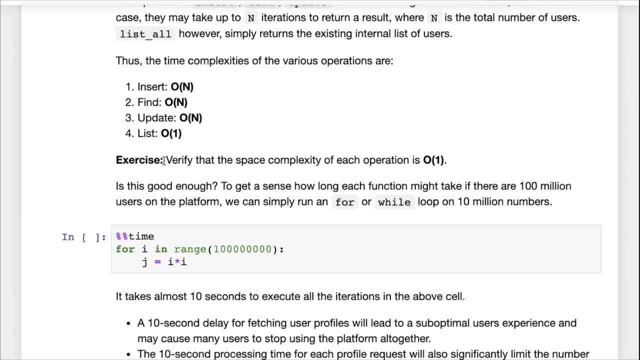 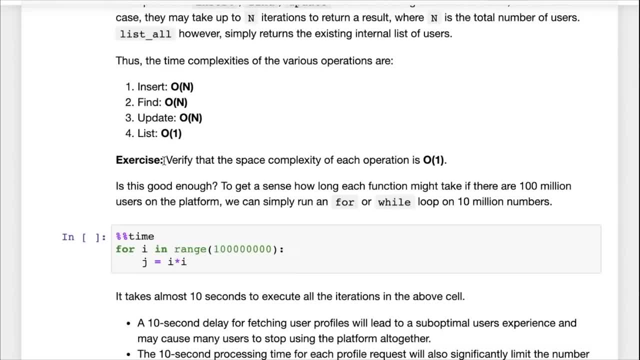 watch lesson one where we talk about analysis of algorithms, complexities and the big O notation, what we're calling order of N, the big O notation. all of these explained in a lot more detail so you can go back to lesson one and check it out. 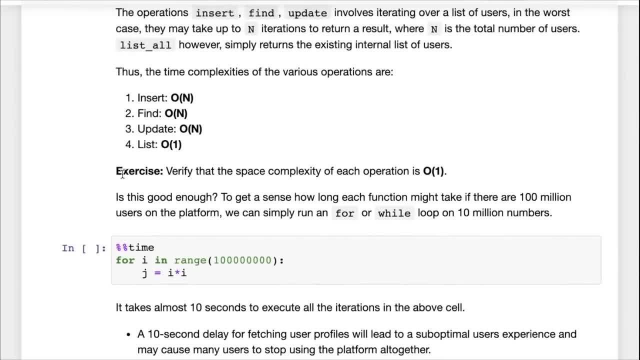 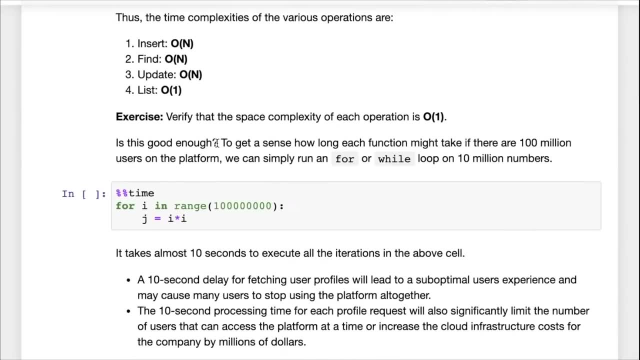 Now we've created a simple solution, and our first question might be to wonder if this is good enough and to get a sense of how long each function might take if there are a hundred million number users on the platform. let's create a while loop. 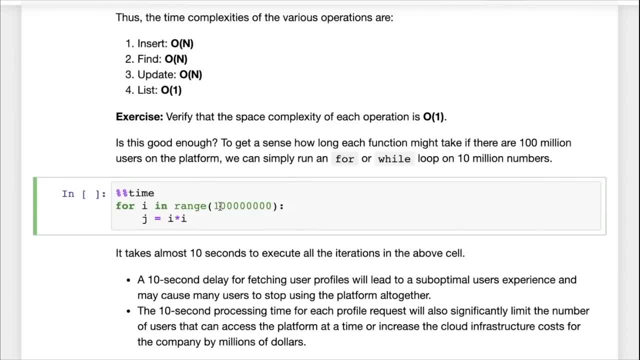 Let's create a for loop and let's run it for. let's see how many this is 1,, 2,, 3,, 4,, 5,, 6,, 7,, 8.. So let's run it for 10 million, a hundred million numbers. 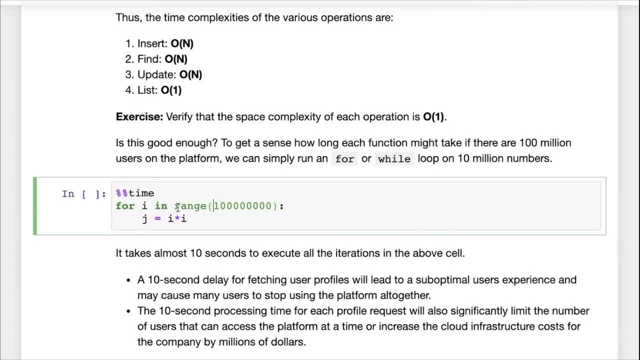 So here we have a number of numbers. Let's run it for 10 million. We are creating a range of a hundred million numbers and we're running a for loop which iterates over the entire range, And we're simply performing a simple operation which we're not really using. 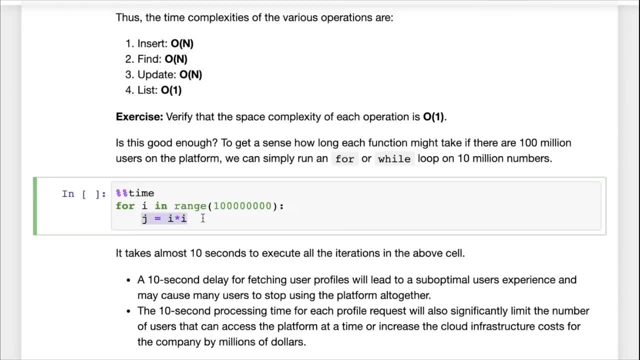 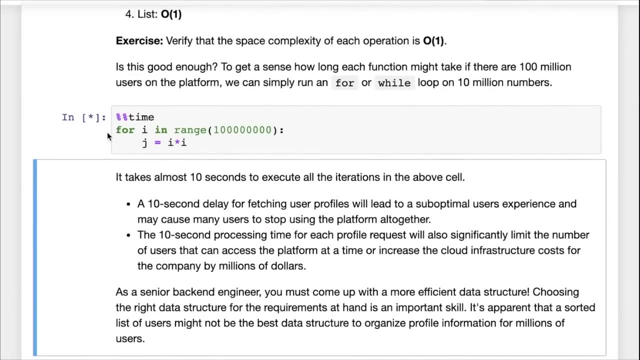 We just we're just multiplying the number by itself to simulate what might happen if we have our database of a hundred million users And we're trying to access, find a user. Now what is the worst case scenario here? And let's run this and you can already see that it is taking a while for a hundred. 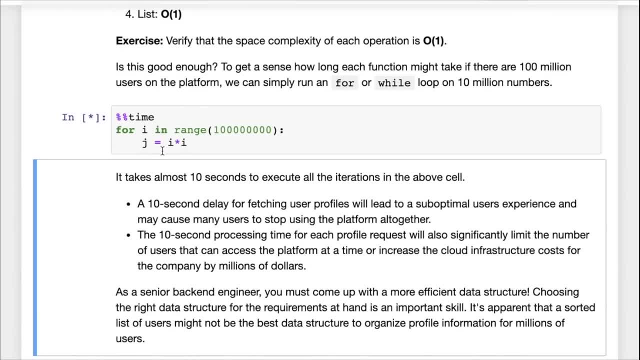 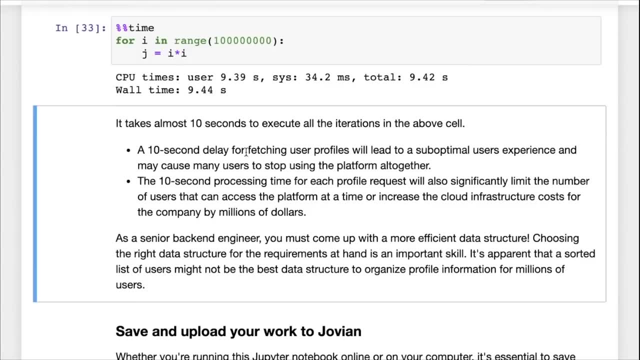 million users. The loop takes about 10 seconds to complete. here It took about 9.45, and a 10 second delay for fetching user profiles will definitely lead to a suboptimal user experience And that may cause users to stop using the platform altogether. 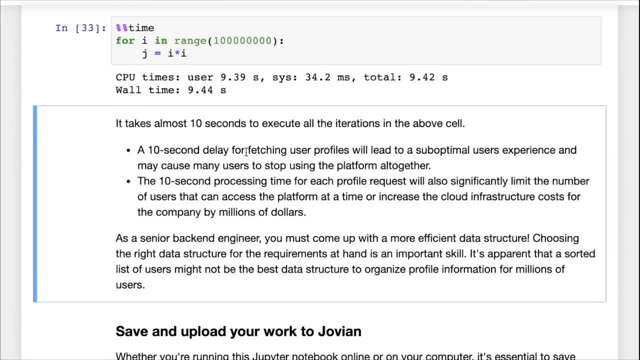 Now imagine you came to jovenai and it took 10 or 15 seconds to load your profile and then maybe even longer to load the other information and display it. You would not be happy with the experience. And then a 10 second processing time for each user, for each request, each profile. 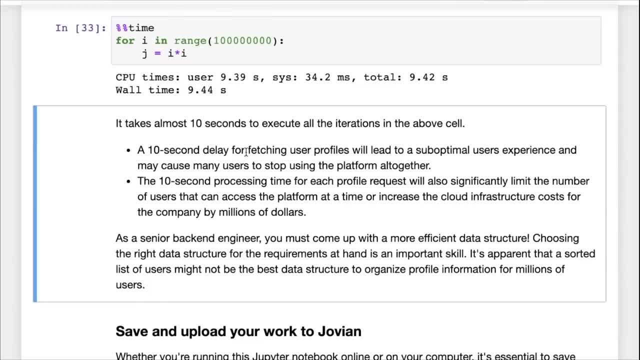 request will also significantly limit the number of users that can access the platform at a time, because if you're running the backend server on one computer which has eight cores, then each core will be busy for 10 seconds Each time a user tries to access the platform. 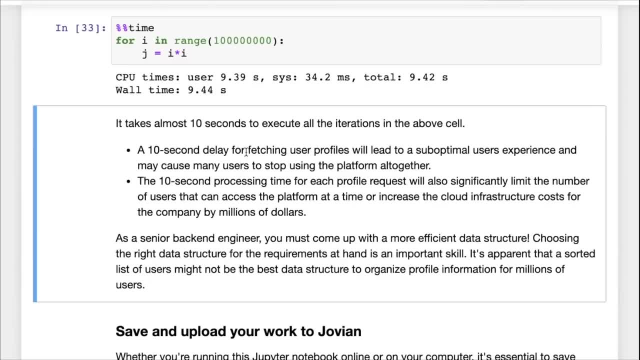 So you can only serve about eight users in 10 seconds time. Now that's pretty bad. That could significantly Limit the number of users. Uh, you will have a significant outage if a lot of users come to the platform or on the other. 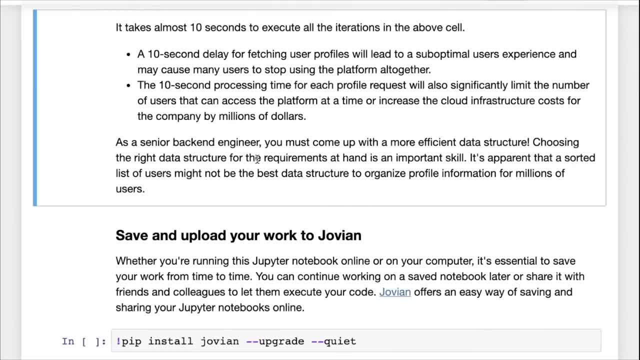 hand, you may have to increase the cloud infrastructure, add more servers, add bigger hardware, more course, more ramp, and that could increase the cloud infrastructure costs for your company by millions of dollars. So, as a senior backend engineer, you must come up with a more efficient data structure. 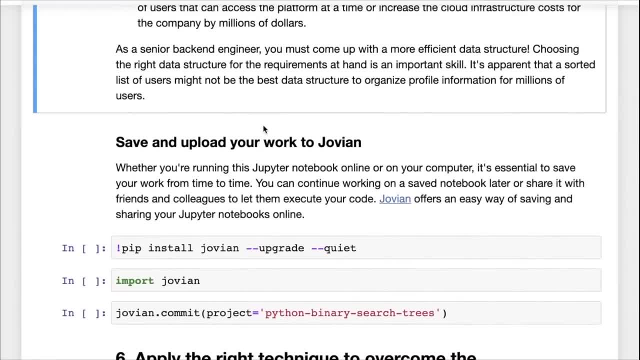 And this is why choosing the right data structure for the requirements at hand is a very important skill. Now We can clearly see that using a sorted list of users may not be the best data structure to organize a profile information, So let's see what better we can do here. 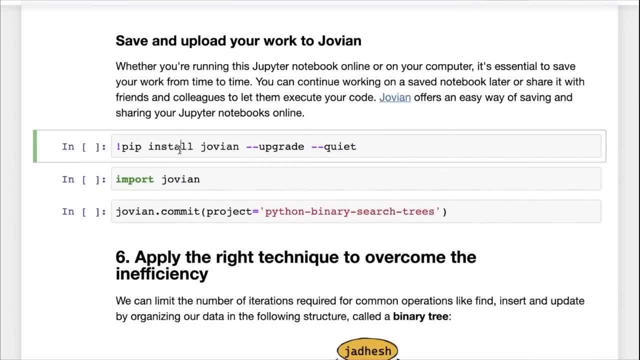 And before we do that, let's save our work. So remember that this notebook, we were running it on an online platform called binder, and binder can shut down at any moment because it is a free service. So what you want to do is run pip install. 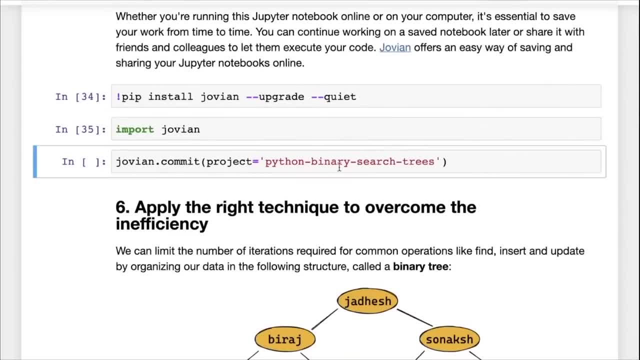 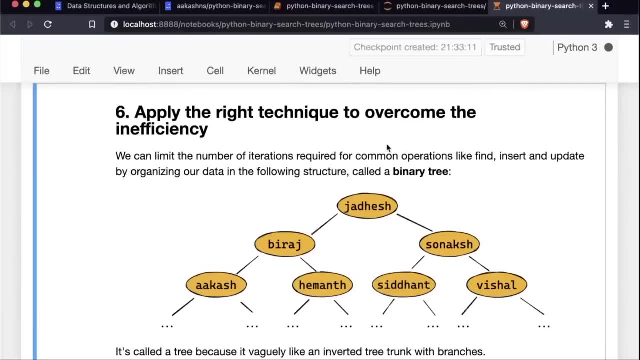 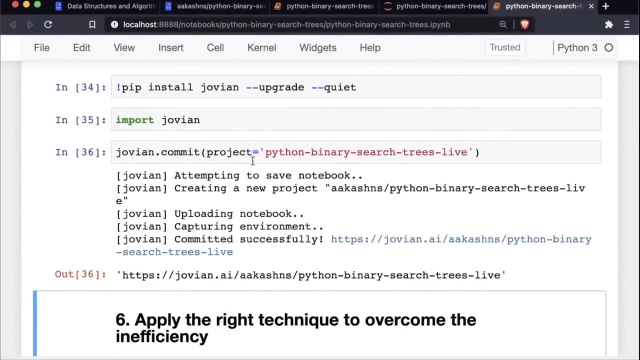 Jovian and then import the Jovian library and you can then run Joviancom it. now, when you run Jovian dot commit, what this does is this: captures a snapshot of your Jupiter notebook, whether you're running it on binder or you're running it on your own local computer, and it saves the snapshot of. 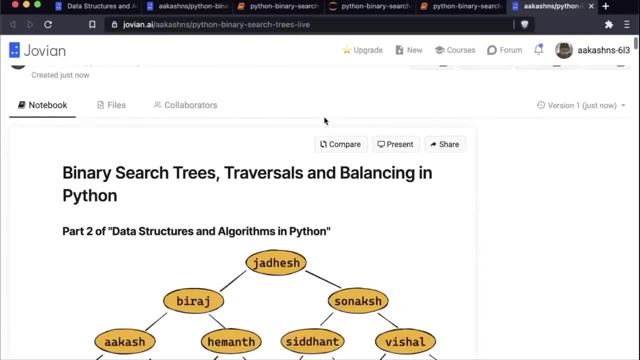 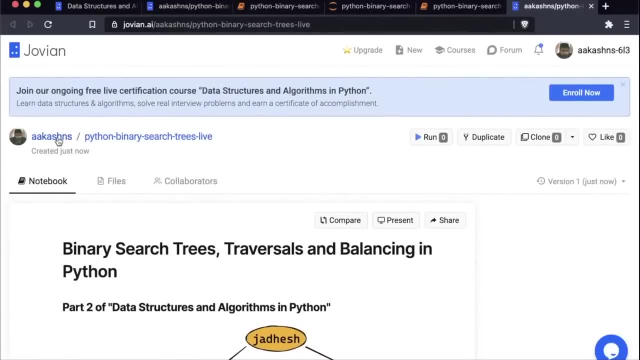 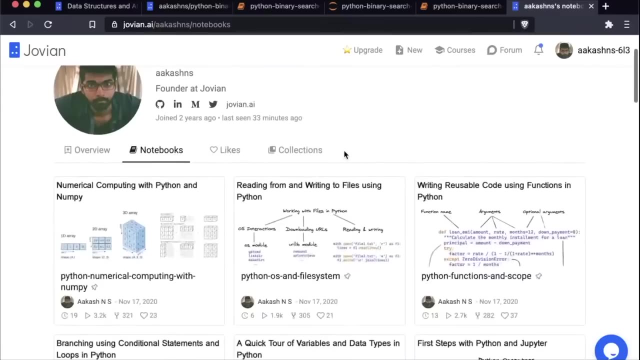 this Jupiter notebook on your Jovian profile. So here you can see now on my Jovian profile I have this notebook and I can go back on my profile and view the other notebooks that I've created in the past. So your Jovian profile becomes a collection of all the Jupiter notebooks that you're working on. 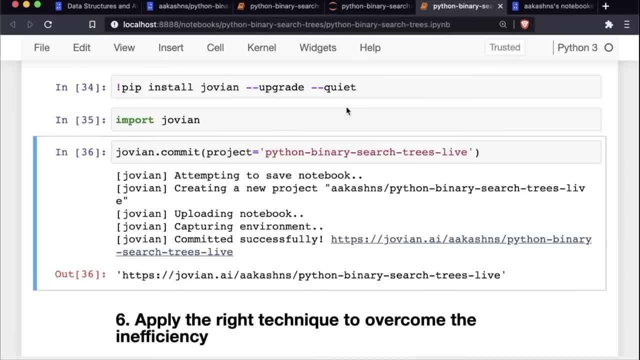 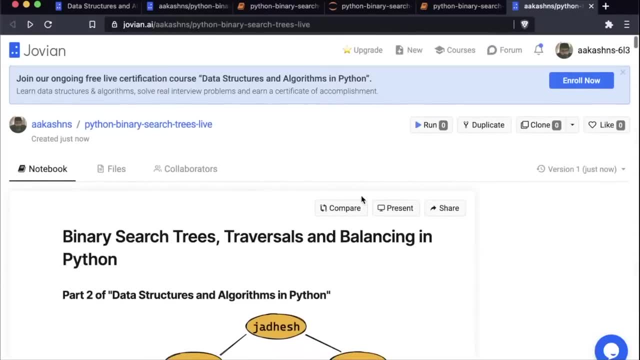 So always, just, it takes just a couple of lines: import Jovian and run Joviancom. It's always run Joviancom it inside your notebooks And if you want to resume any work that you were doing then all you need to do is click on the run button and then click run on binder once again. 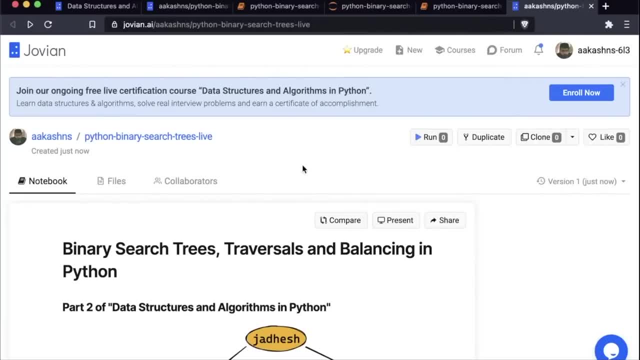 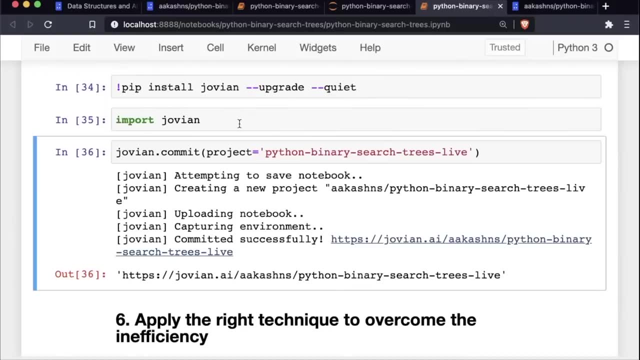 And then you can start executing the code within the Jupiter notebook once again. Right. So remember that binder is a free service, so it will shut down If, after about 10 minutes of inactivity- which is if your computer goes to sleep or you change your tab- just keep running Joviancom, it from time to time. 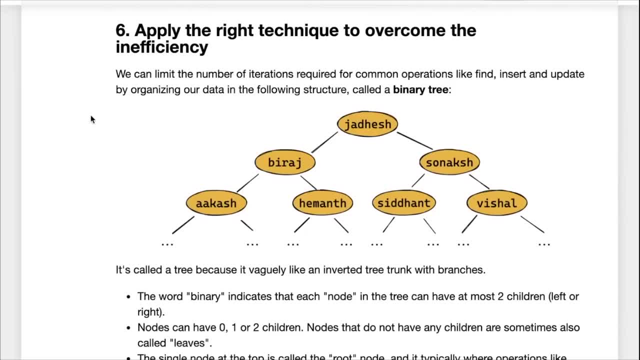 So now we have a simple implementation and we've analyzed it and determined that it is not efficient. It is inefficient. So now we need to apply the right technique to overcome the inefficiency And we can limit The number of iterations required for common operations like find, insert and update, by ditching the linear structure that we had earlier and organizing our data in a more tree, like structure. 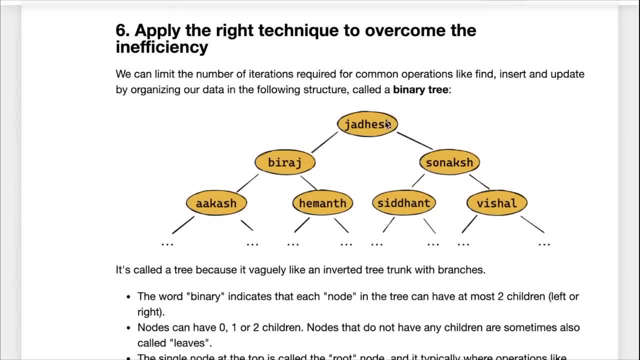 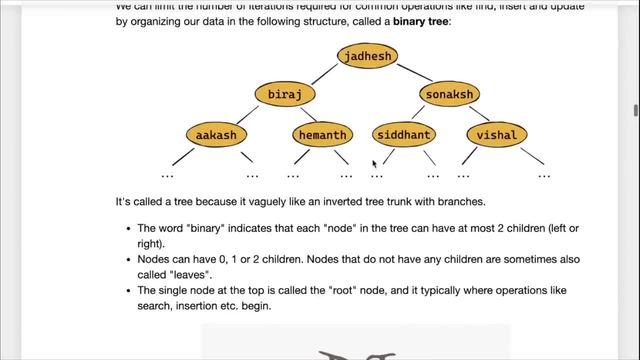 So this is a structure that we'll use for our data And we will call this a binary tree. Now, this is called a tree because it vaguely resembles an inverted tree trunk with branches, So you can think of this as the root, So this has the root, and then you can see each of these are like branches. 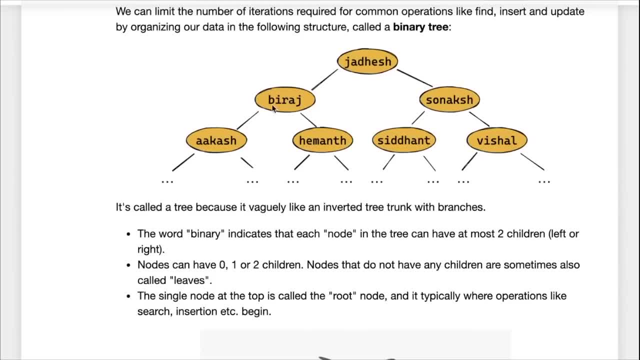 And then there are nodes, where branches then split into multiple branches, So these are called nodes. And finally, at the end you will have individual nodes which do not have any more branches, And those are called leaves. So these are some terms that are used. 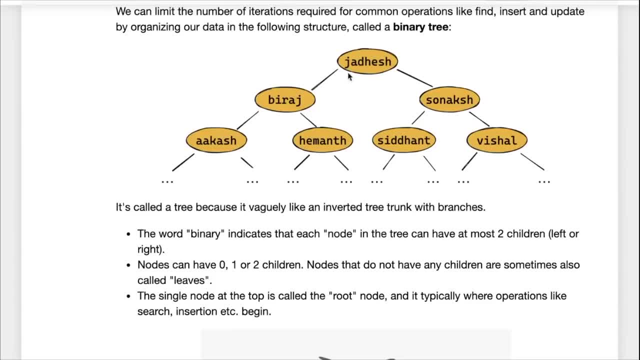 The tree represents the entire structure. The top node is called the root and each, each element in the tree is called a node. The top node is called a root And then the bottom most nodes which do not have any Subtree. 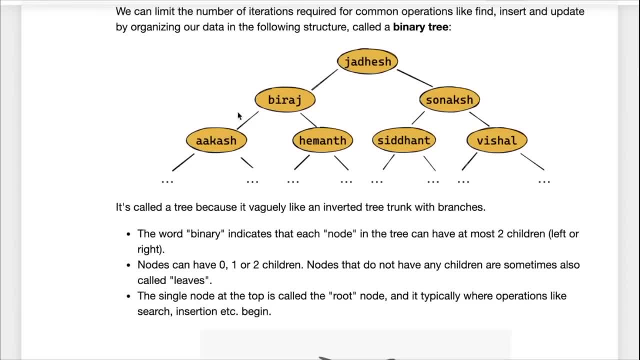 Or what are called children which do not have any children, are called leaves right. So the root node has two children and then each node there with can have zero, one or two children. So it's not necessary to have exactly two children, but up to two children is what. 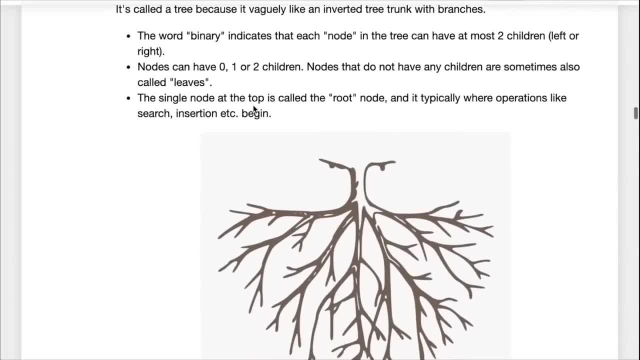 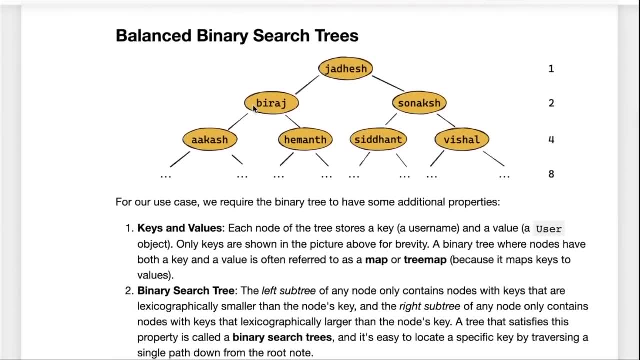 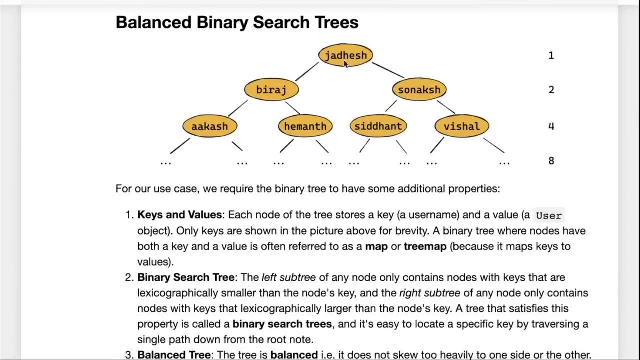 determines a binary tree, So that's a binary tree, but the binary tree that we need will have some additional properties, which was what will make it efficient for our Purposes. So you can see, one thing you can observe here is that the root node seems also seems to be: 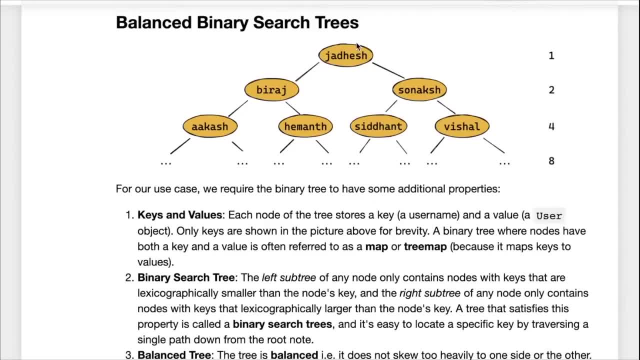 the central value. If you sort the keys in increasing order, So what you will notice is on the left we have uh keys which have which lie before Jadesh, and on the ride we have keys which like after Jadesh. 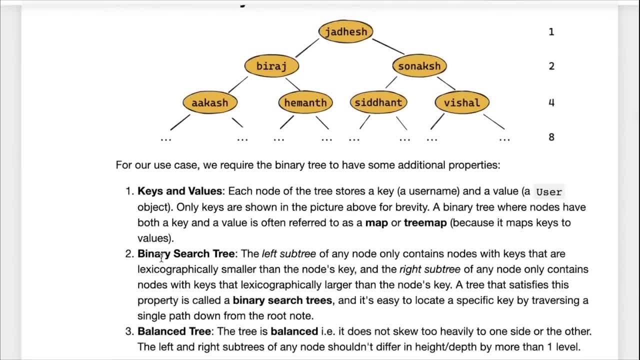 So that's one thing, And that is actually the second property listed here- that the left subtree of any node consists only of nodes which have keys that are lexical graphically smaller than the nodes key right. So the key for this node is barrage, and that is lexical graphically smaller than Jadesh. 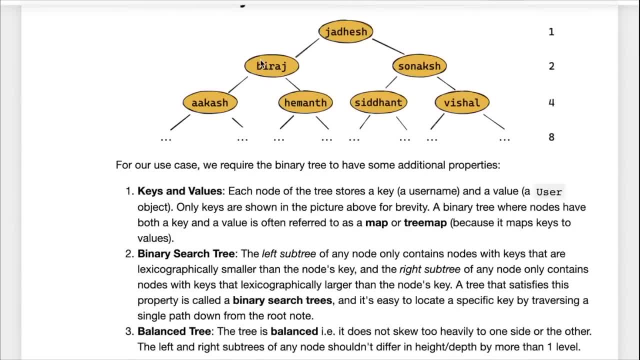 And similarly Hemant and Akash are all smaller than Jadesh. And then this property holds at every node. So at every node, if you check Sonak, you can see that Sedan is less than Sonak and Vishal, which 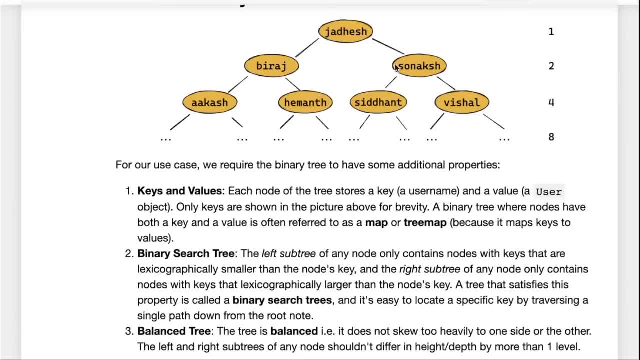 comes to the right, is a more than Sonak, and then Sonak, Sedan and Vishal- all three are greater than Jadesh right. So when a binary tree satisfies this property, it is called a binary search tree. So that's what we're looking at here. 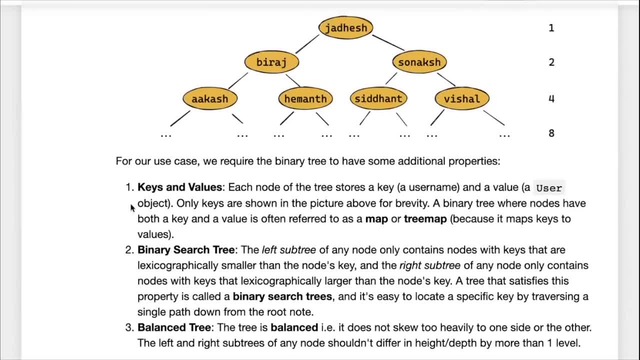 This is a binary search tree, So that's the first property that we need. The second property is that our nodes will have both keys and values. Now, sometimes you can create binary nodes, binary trees, with just keys. Each node will have a single number or a string inside it and you can call it the key or value, or 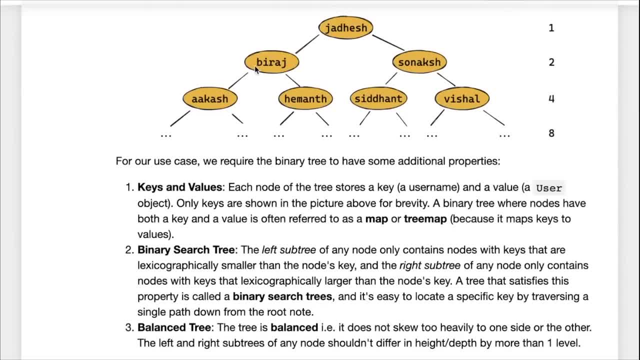 element or whatever you wish. But what we want is we want The keys to be usernames so that we can compare the keys easily. but along with each node we also want to associate a value, which is the actual user object. So if you're looking for him on, let's say we started the root node. we see that Jadesh is the. 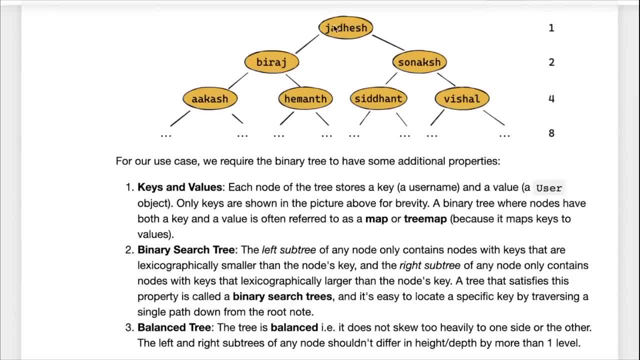 root node And since it is a binary search tree, we know that Hemant lies to the left. Then we reach barrage. We know that Hemant will lie to the right of barrage, So we go right, We reach Hemant and then we access the value stored at Hemant, which is the user details for him. 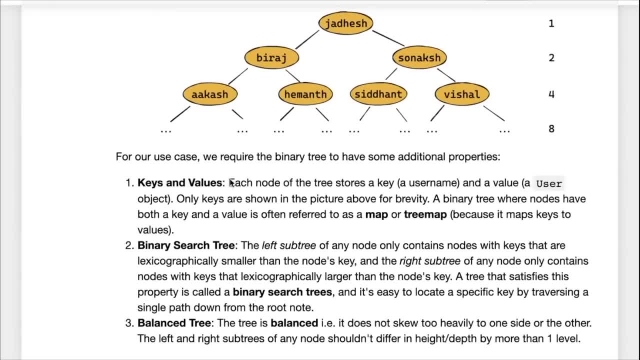 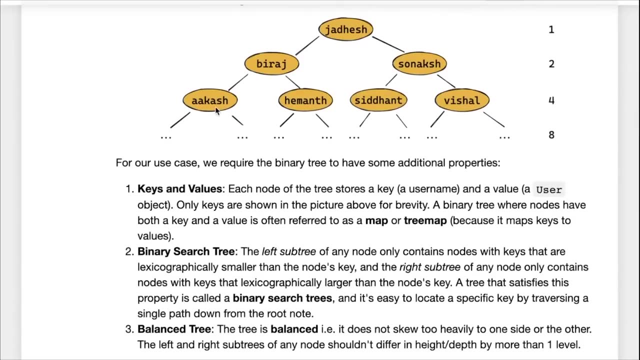 Hemant right. So we need both keys and values in a binary tree, And this is what is called a tree map, or a map in many languages. And then, finally, this tree that we will create, this data structure that we will create, it will be balanced. 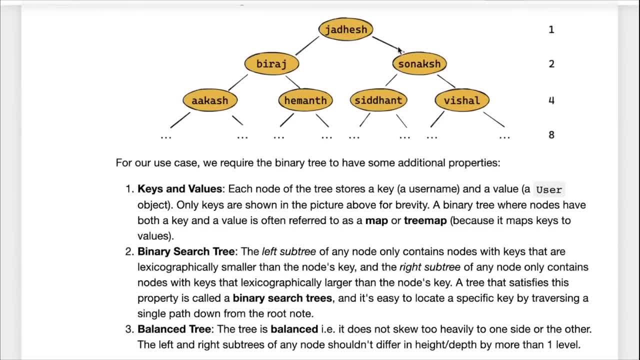 So here what we're looking at is each node has two children left and right, but it is also possible to have an unbalanced tree where you only have one child on each on, on, on maybe one of the sites. So we will require it to be balanced, which means that it does not skew too heavily in one direction. 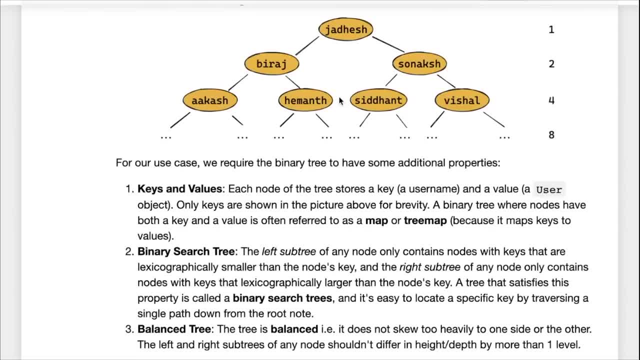 And we'll talk about what balancing means, And we'll talk about how to check if a tree is balanced, on how to keep a tree balanced. Okay, So we'll go over all of these things step-by-step, but these are some of the properties that we want. our final data: 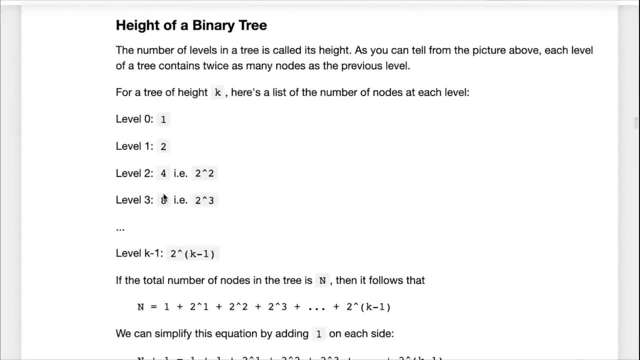 structure to have. Okay, So one important property of a tree, of a binary tree, is the height. Okay, In fact, if you start counting, you can say this is level zero, where you have one node, and this is level two, or this is. 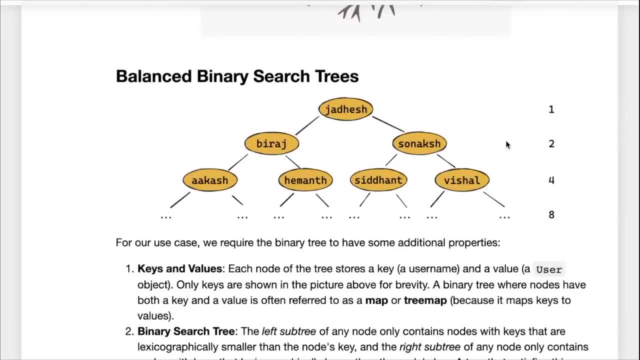 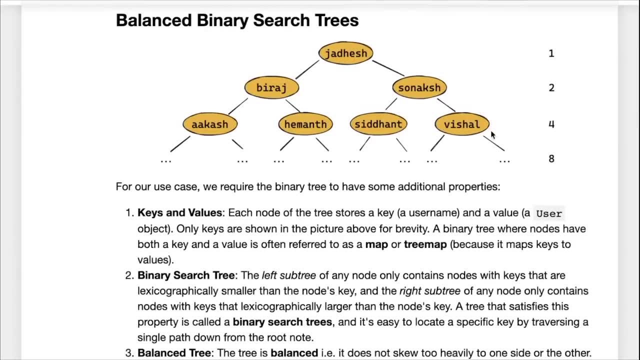 level one, where you have two nodes: the left and right, the left and right child of the root node, And then this is level three, level two, where you have four nodes: the left and right child of the first node on level one and the left and right child of the second node on level one. 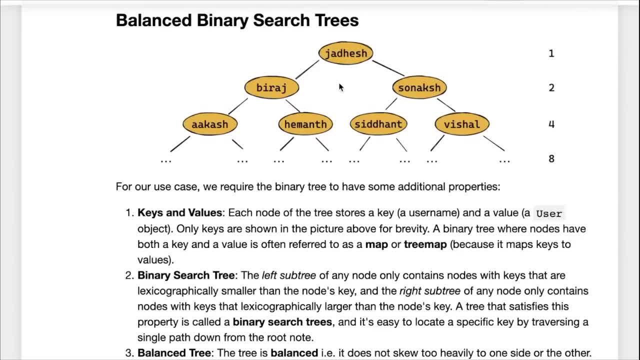 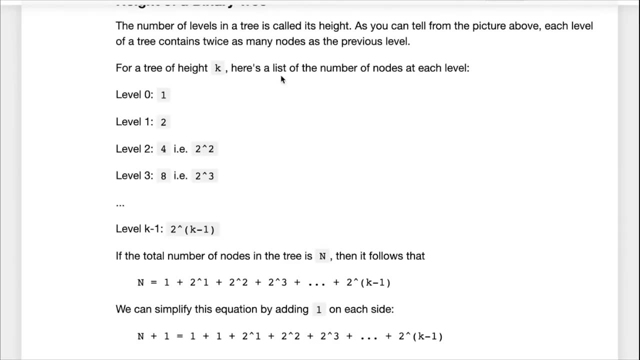 Right. So you can see that the number of Nodes in each level in a balance Binary tree is double of the number of nodes of the previous level. So if you have a tree of height key or which, which means a tree which has exactly K levels, then here's the list of the 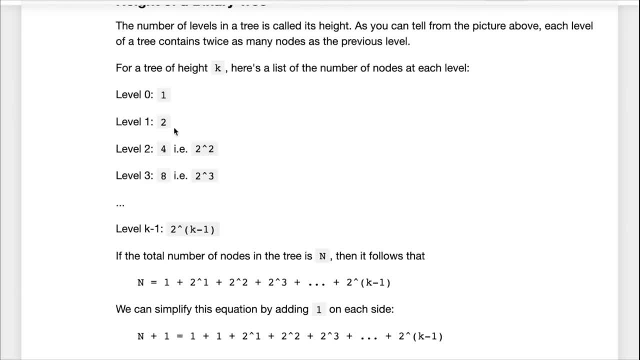 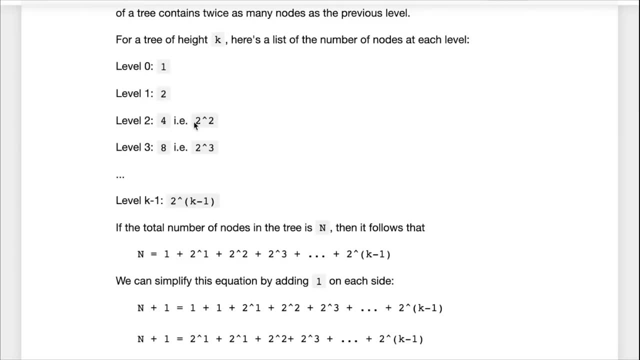 number of nodes at each level. Now, level zero will have one node, The root node. level one will have two nodes: its children. level two will have four nodes, their children. So that's four nodes is two times two or two to the power two. level three: 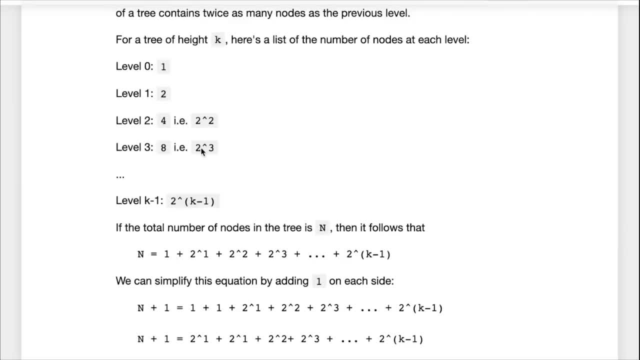 We'll have eight nodes, Two nodes for each of these four nodes, So that's two to the power three And similarly, if you keep going down level K minus one, the final level will have two to the power of K minus one nodes. 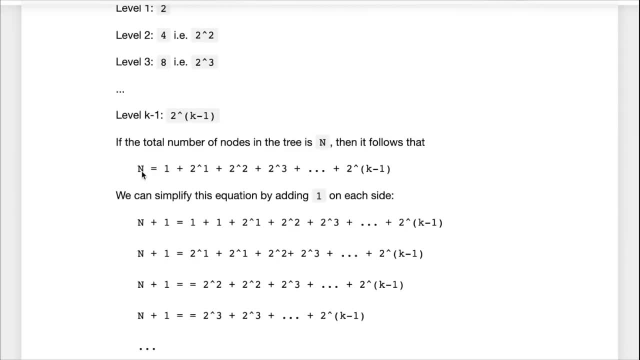 So that if the total number of nodes in the tree is N, then it follows that N is one plus two plus two, square plus two, cube plus so on, plus two to K minus one. Okay, So what we're trying to determine here is what is the relationship between the height of the tree and the total number of nodes in the tree? 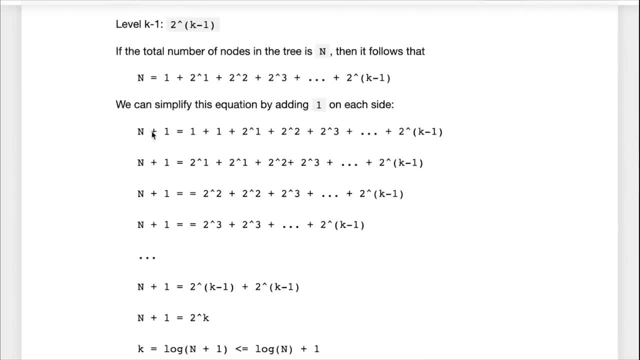 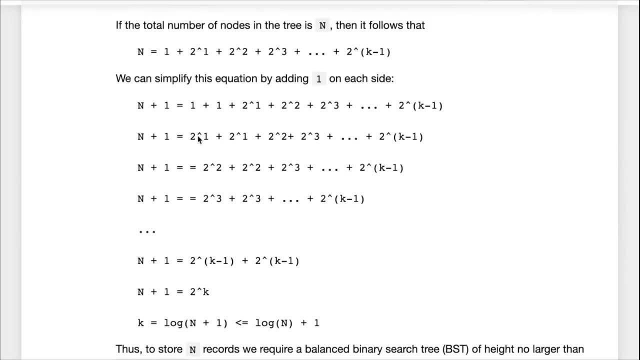 And This is the relationship and we can simplify it a bit If we add one to each side. you can see here that this side we get N plus one And this side we get one plus one, which gets simplified as two or two to the power one. 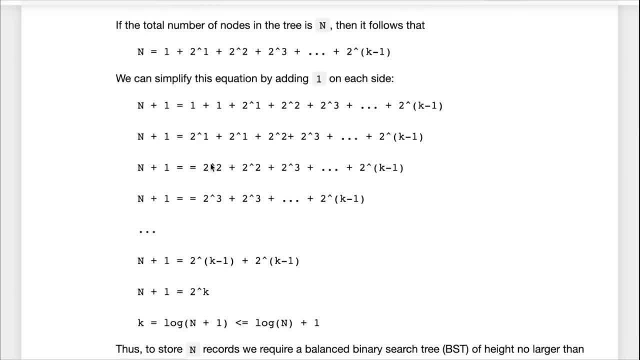 And then we can add two to the power, one with two to the power one, And that gets simplified as two to the power of two. Then we can add two to the power of two and two to the power of two, And that gets simplified to two to the power of three. 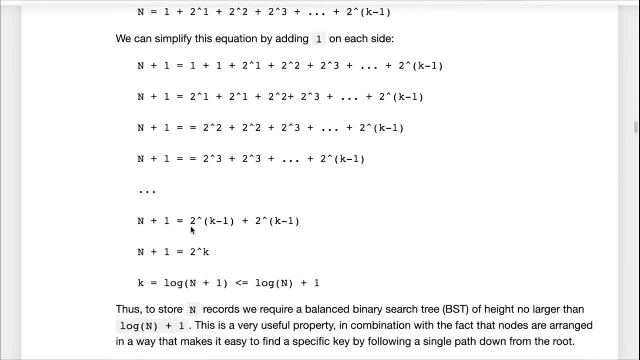 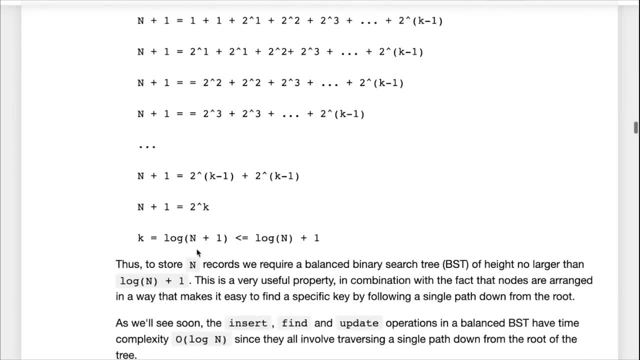 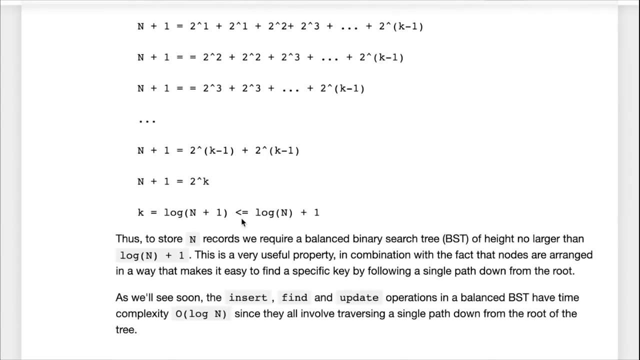 And we can keep performing this reduction, We can keep adding these together till we finally end with two to the power K minus one, plus two to the power K minus one, which is simply two to the power of K. So what that gives us is that K- the height of the tree, is log of N plus one, which is approximately, or in almost every case, less than log N plus one. 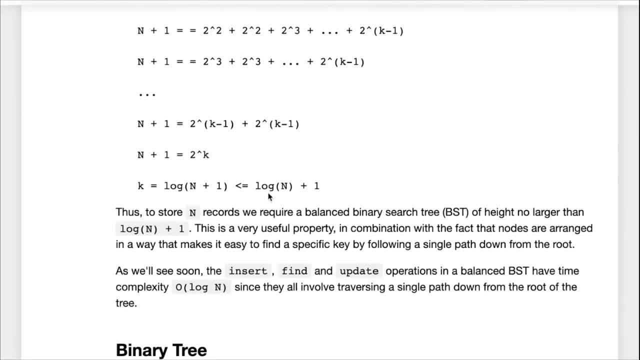 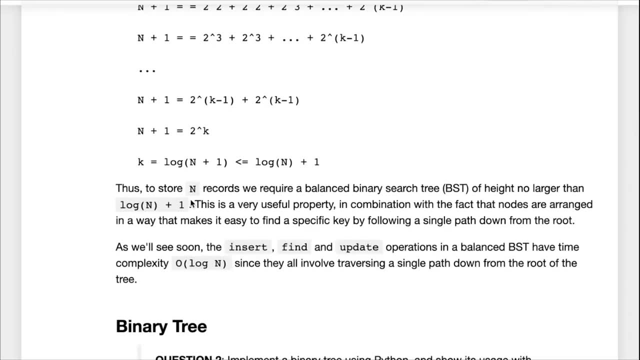 So that's a a bit of an approximation we're doing here, but it is uh. the height of the tree is less than log N plus one. So to store N records we require a balanced binary search tree of height no larger than log N plus one. 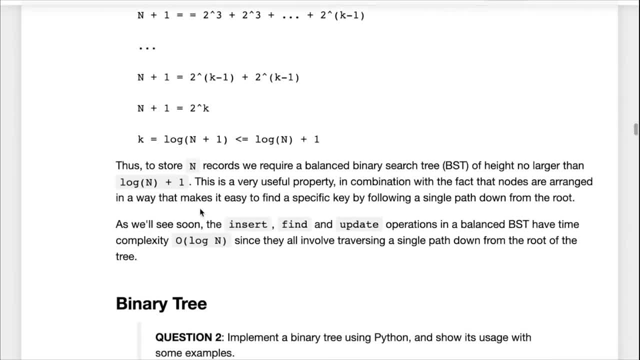 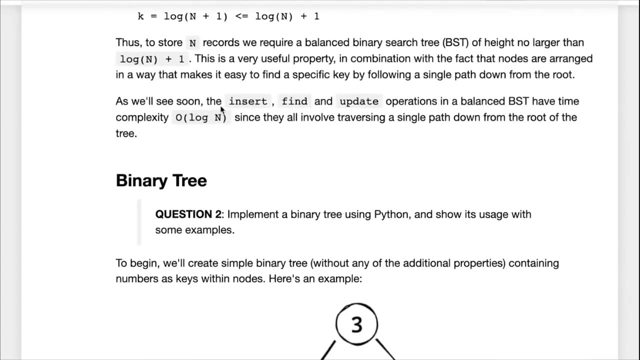 Now, this is a very useful property, in combination With the fact that no nodes are arranged in a way that it makes it easy to find a specific key simply by following a path down from the root, the binary search tree property, And we'll see soon, by the end of this lesson, that the insert find an update. operations in a balanced binary search tree have complexity. order of login. 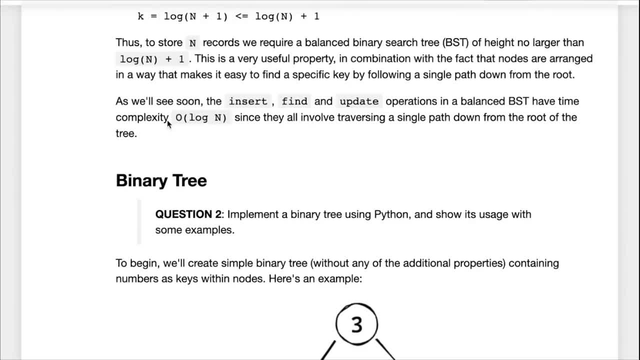 So in our original implementation, our brute force implementation, they had order N and this time we've reduced the complexity to order login and that is far better, And we'll see how that happens. Okay, So that's a quick introduction to binary search trees. 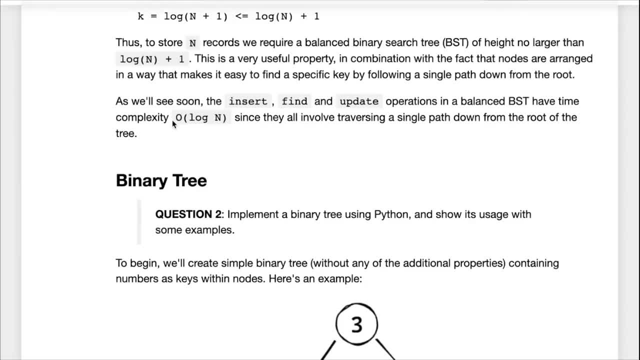 We have. we've had enough theory. Now let's get into some implementation. but before that we have the second question. Now, binary trees are very commonly used as data structures for a variety of different, in a variety of different languages. For instance, Java, C plus plus, Python, Java and C plus plus have this concept of a map which is represented using a binary tree. 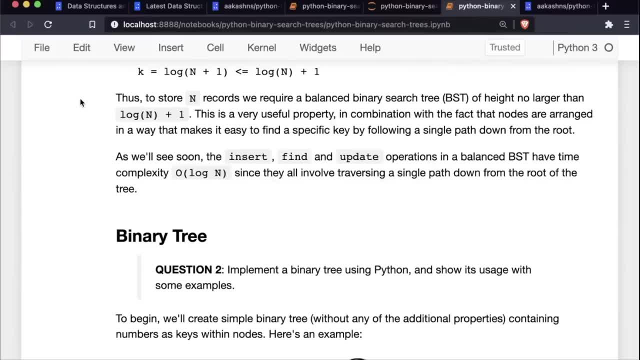 And it is also used in file systems. So binary trees are also used in file systems to store indexes of files. So when you browse your file system or when you search for a specific file, it is a binary tree that is used to look up the file and find the location of the file. 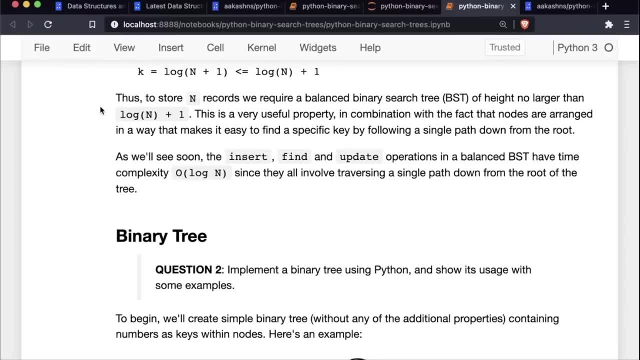 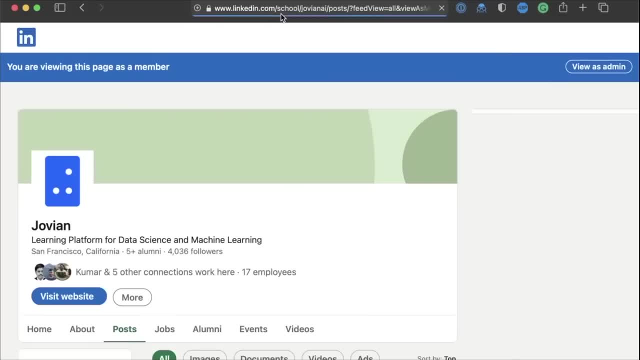 Now that's where that brings us to our second question of today. Now you can, you can find the second question on our LinkedIn profile. So once again, go to linkedincom- slash school, slash Jovian AI- and you will find the second question here. 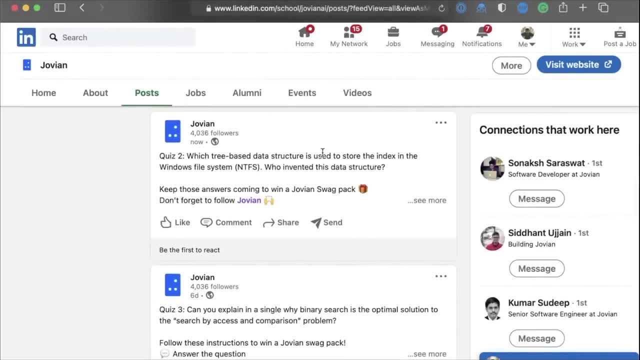 The second question is which tree based data structure is used to store the index in the windows file system and who invented the state of structure? So, like this question, follow us And comment with your answer and you can stand a chance to win a swag pack, right? 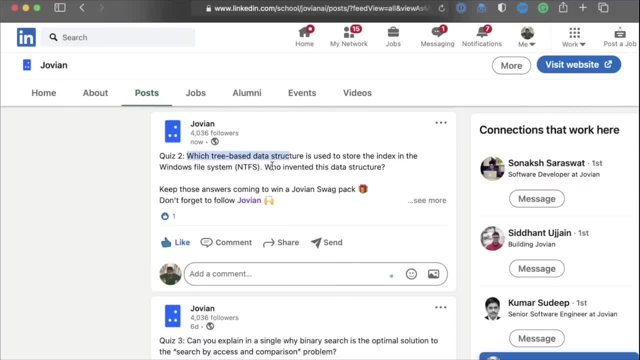 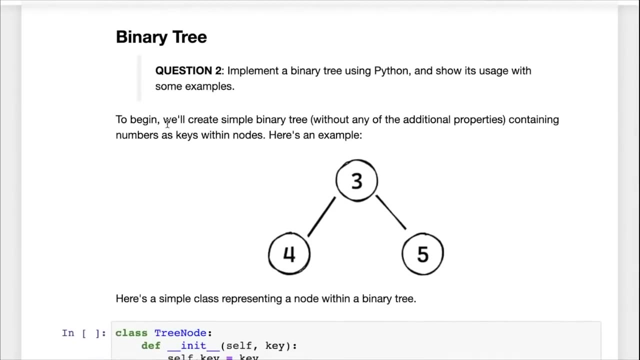 So, if we repeat the question, which tree based data structure is used to store the index in the windows file system, also known as NTFS, and who invented this data structure? Okay, So let's get to the implementation of binary trees, And here's a very common interview question that you might get. 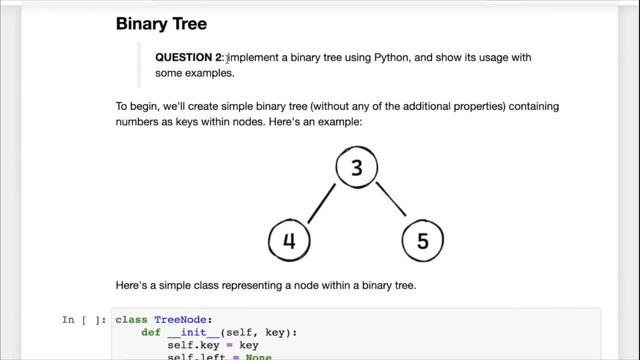 Implement a binary tree Using Python and then show its usage with some examples. So what we'll do as we implement binary trees and binary search trees is to also cover many common interview questions. In fact, we'll cover exactly 15.. So that's a quite a few. 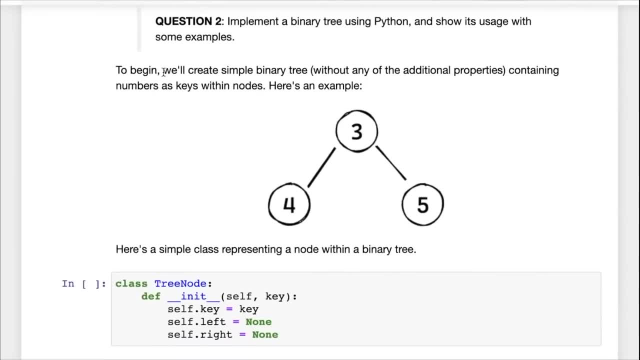 And the first one is to implement a binary tree and to begin, we'll create a very simple binary tree, So we will not have any of the special properties like key value pairs and binary search tree and balancing, rather, and we'll also use numbers as keys within. 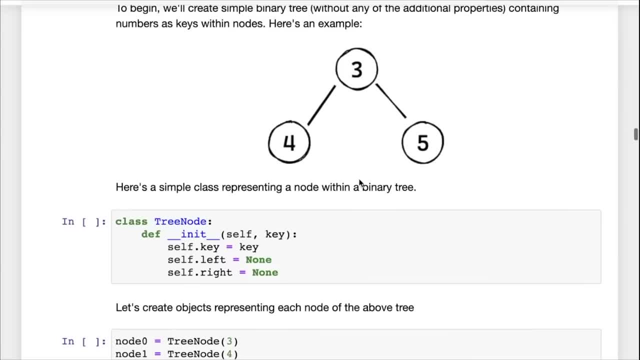 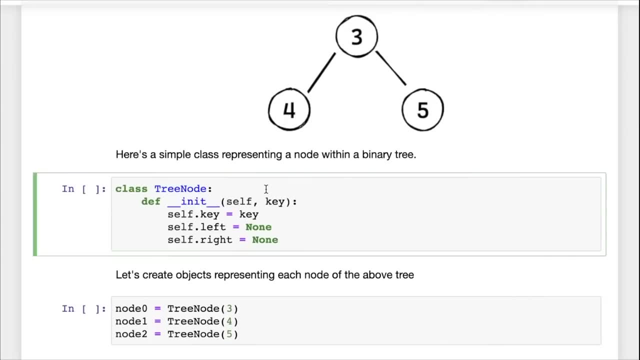 Our nodes because they're simpler to work with. So here is an example: binary tree. So we have a root node and then we have a left child in right child And here's a simple class representing this, representing a single node within the tree. 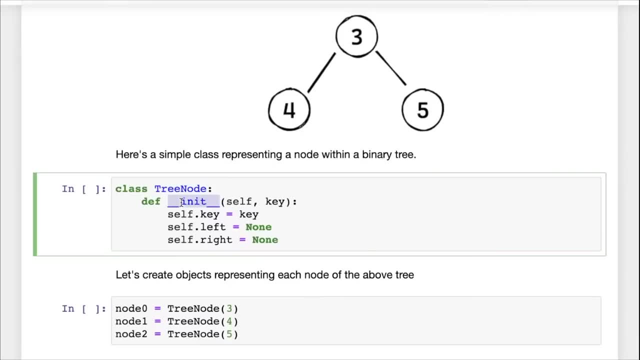 So we're calling this class tree node and it has a constructor function. It simply takes a key and it sets self dot key to key. It also has a couple of other properties- self dot left and self dot right- which are initially set to none. 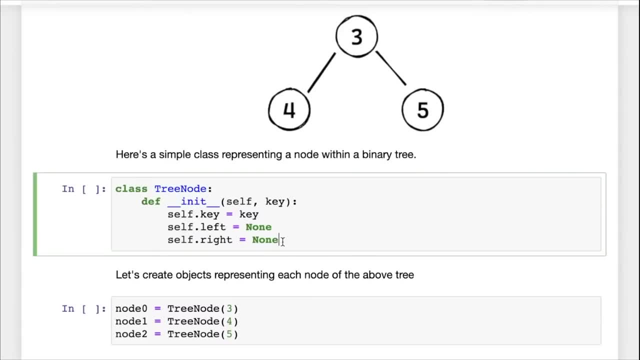 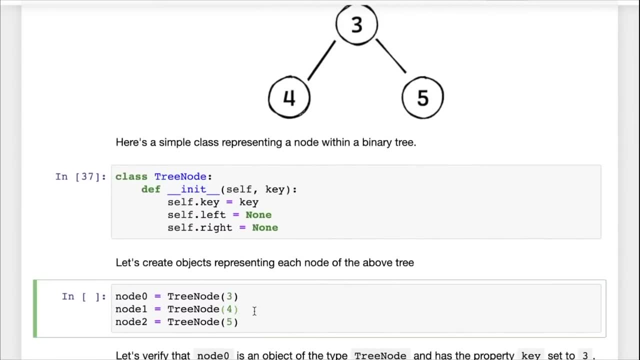 So each node, when it's created Exactly, Exists independently of other nodes. And now let's create nodes representing each of these nodes. So we have node zero, We're calling it, We're calling tree node with the value three. Then we have node one and node two. 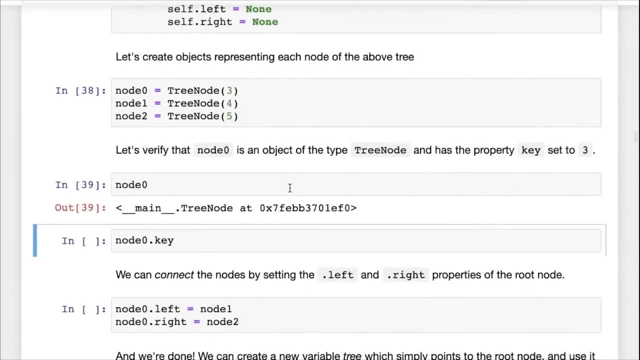 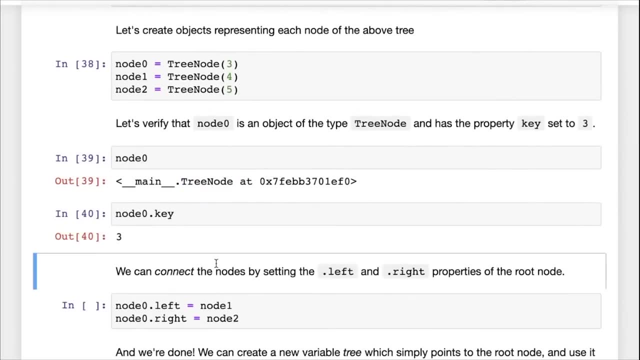 So there you go. Now we've created the nodes and we can verify that it is of the type tree node You can see here. and if we check the key of node zero, you can see that it has a value three. And we can now connect the nodes by setting the dot left and dot right. 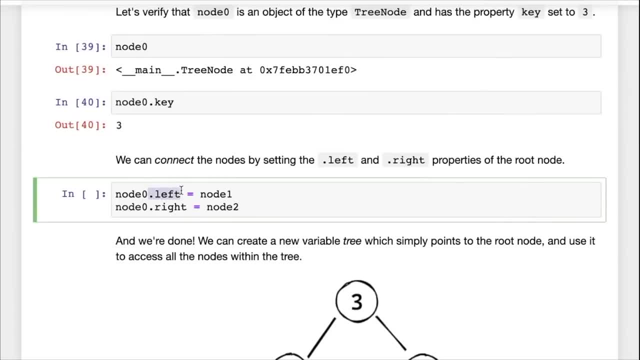 Properties of the root node. So if you go to node zero and set dot left to node one, so now we've connected node zero to node one. And similarly, if we set node zero, dot right to node two, now we've connected node zero and node two and that's it. 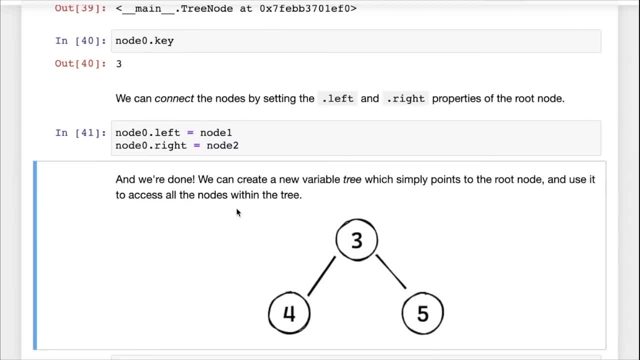 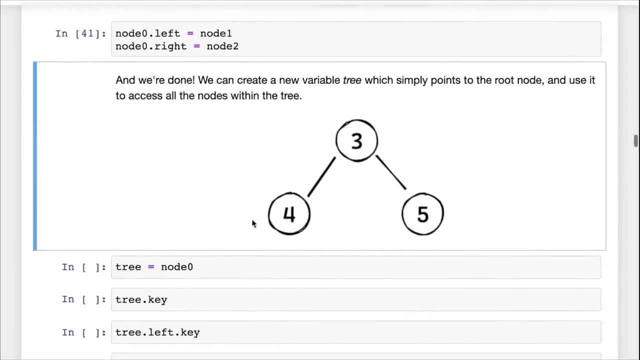 We're done. So now we have three nodes and then we've connected each of those nodes And we may also just want to track which is the root node, So we can create a new variable called tree and simply pointed to node zero. 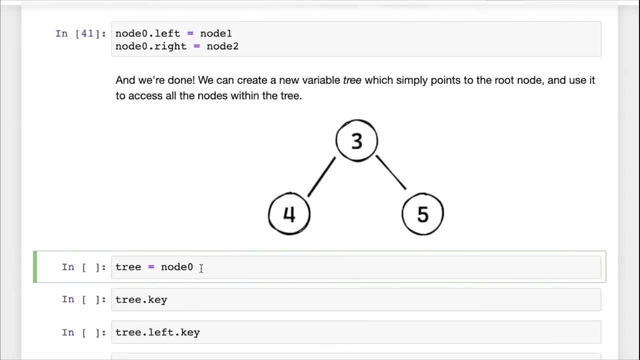 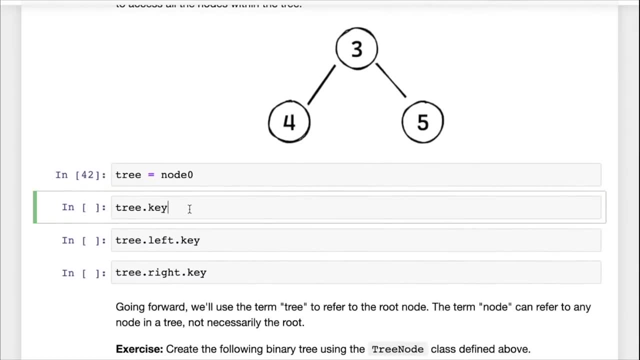 So three points to the root node of the Tree, And then the root node is connected to its children and the children will be connected to their children and so on. So you can check here that if we check three dot key we get three. 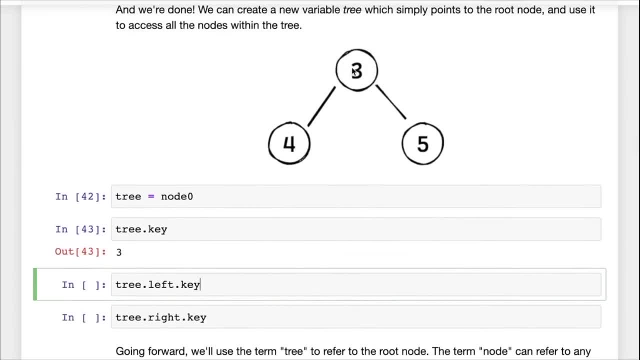 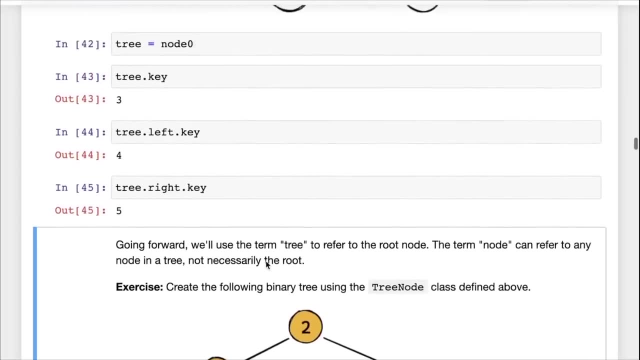 And if you check three dot left dot key, so three is a root node. It has a value Three. three dot left is this node, So it should have the value of four and three dot right dot key should have the value of five. 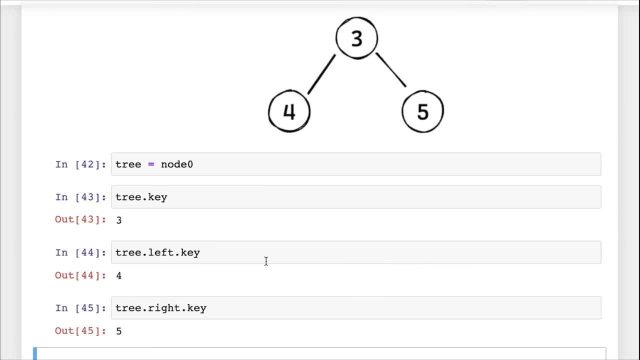 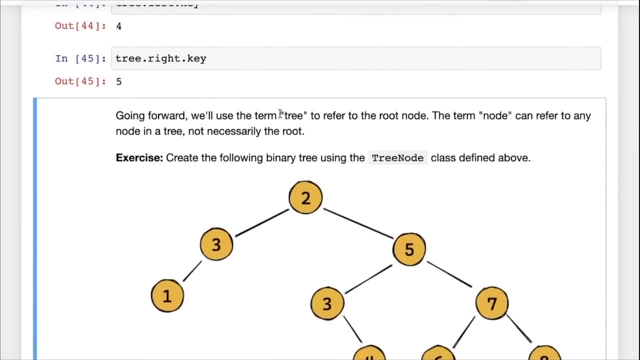 Okay, So pretty straightforward And that's pretty much the answer to the question. Implement a binary tree and Now, going forward, we will use the term tree to refer the new root node, to refer to the root node, and the term node can be used to refer to any node in a tree, not necessarily just the root. 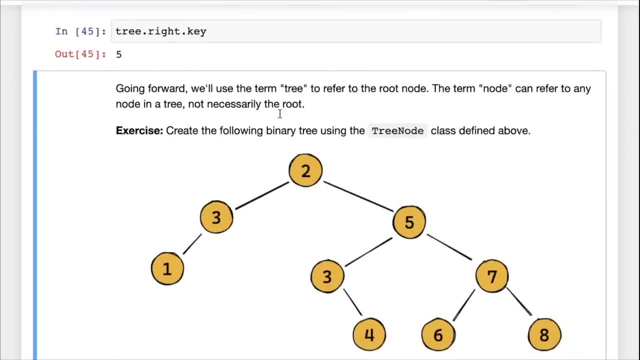 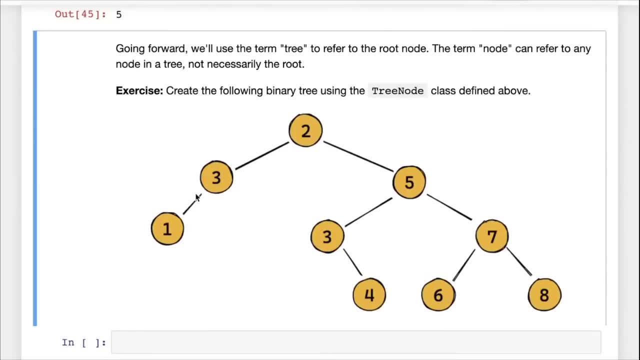 Okay, So here's an exercise for you. Try to create this binary tree. So now you have a root node here and then you have a left child and right child, And then this left child has another left child but does not have a right child. 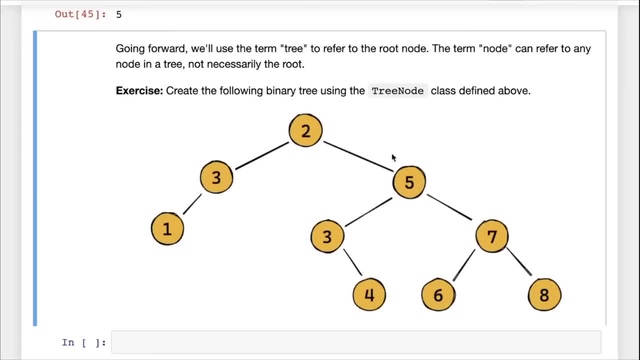 Similarly, here you have another right child and then it has a left child, So you can use this as a reference. Okay, Okay, Okay, Okay. So you have a left child which does not have a left child, but has a right child. 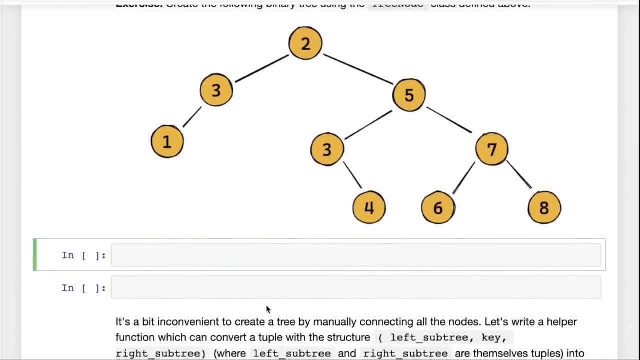 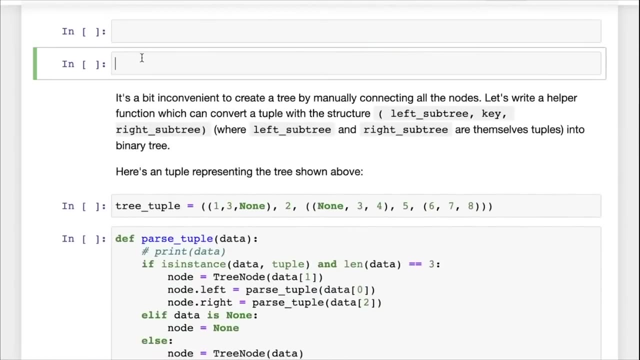 Okay, So there's a slightly more complicated tree structure- and try to use these cells, These empty cells that are given here, to replicate this tree structure and then try to view the different levels of that tree manually. Okay, Now, please do that, because that's a great exercise in understanding how the structure works and how to connect the nodes, but it's a bit inconvenient to create a tree by manually connecting all the nodes. 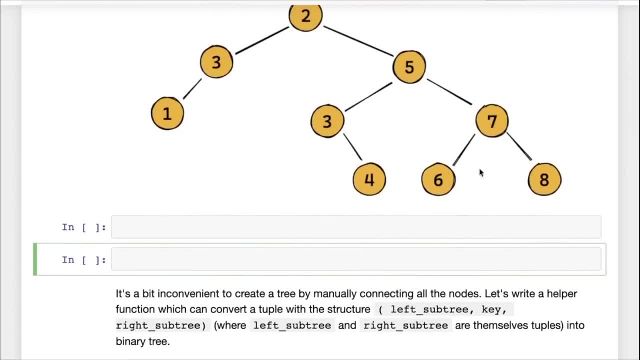 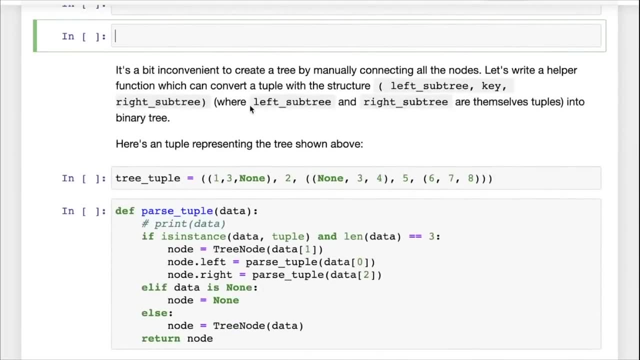 In fact, here you may have to make a total of one, two, three, Four, five, six, seven, eight, nine connections, right? So what we can do is we can write a helper function which can convert a tuple, and the tuple will have this kind of a structure. 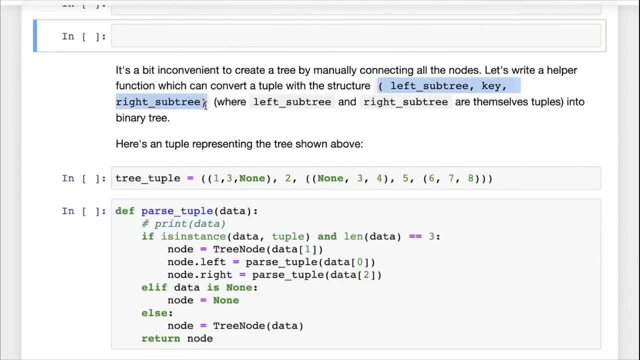 So a tuple is simply is kind of like a list, except that it is represented with these around brackets of parenthesis. So a tuple will have this kind of a structure. It will have three elements and then the middle element will represent the value or the key within the root node. 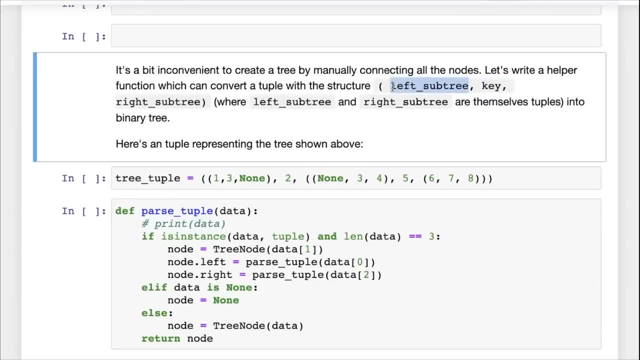 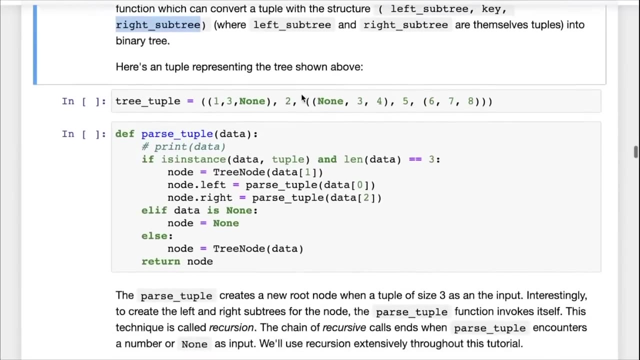 So the first element will itself also be either a tuple- if the left child is is an entire subtree- or if it is a single number, then it will be just a number, and then the right element will represent the right subtree. Okay, So here's an example. 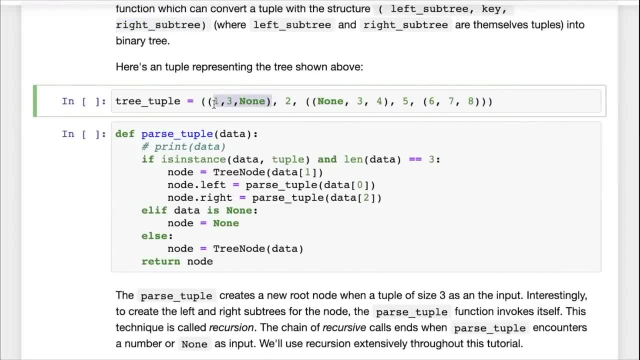 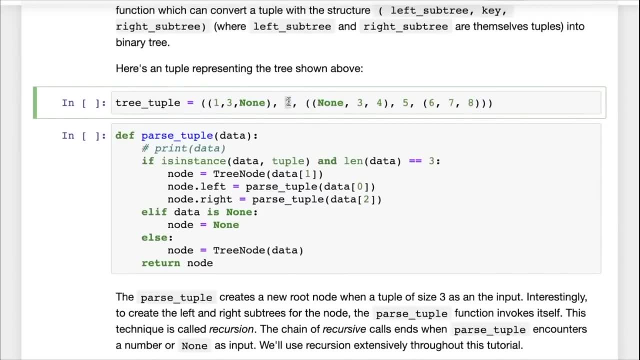 Here is one tree tuple. Now, if you see this tree tuple, it has three elements. This is the first element, This is the second element And then this is the third element. So this first element Two Represents the root node. 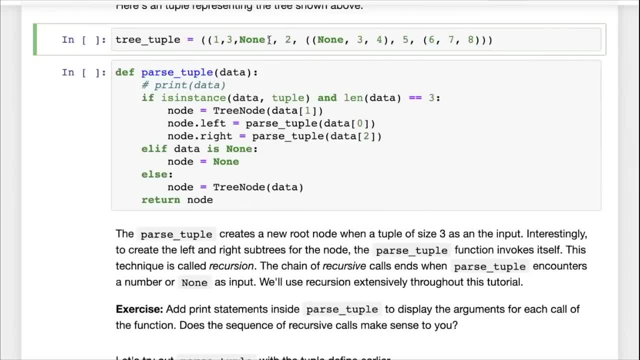 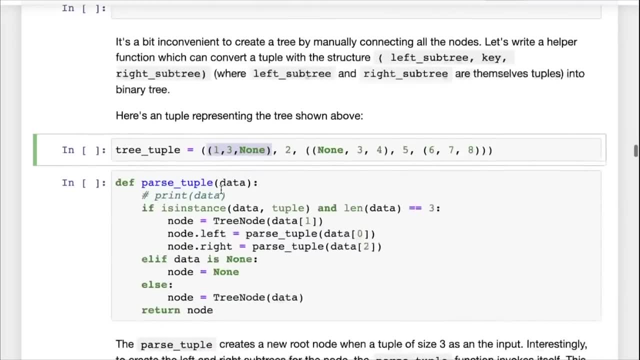 And then this: uh, so the second element two represents the root node. this first element or element at position zero represents this subtree. So you can see here that in this subtree, if you look at just that subtree of that tree, three is the root in that subtree. 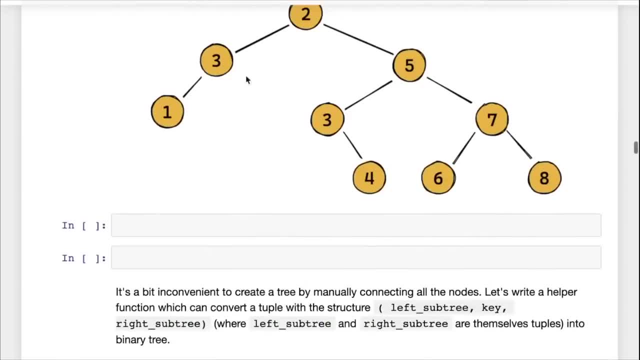 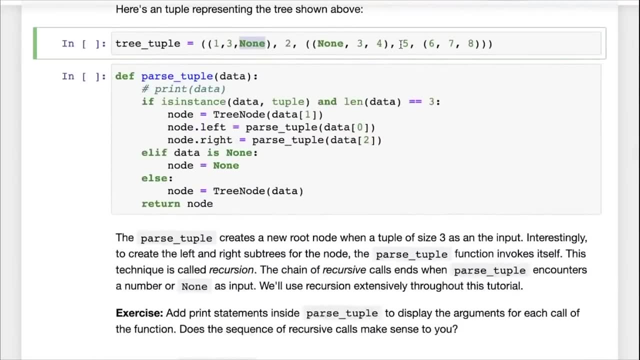 And then one is the left child and there is no right child. So that's what this represent. And then for this subtree where five is a root node, and then you have two Other subtrees that's represented here. So five is the root node, and then you have a subtree here and a subtree here. 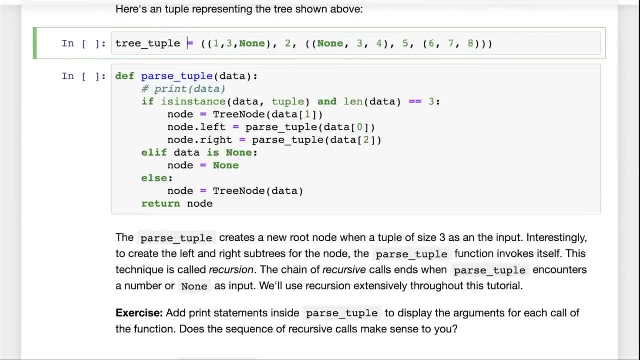 So this is a very easy way. It is a. this is a convenient way for us to represent a binary tree And what we can do is we can define a function, parse tuple, and this past tuple function can take a tuple like this and then convert it into a tree like structure of link nodes using the tree node data structure using the tree node class that we have defined above. 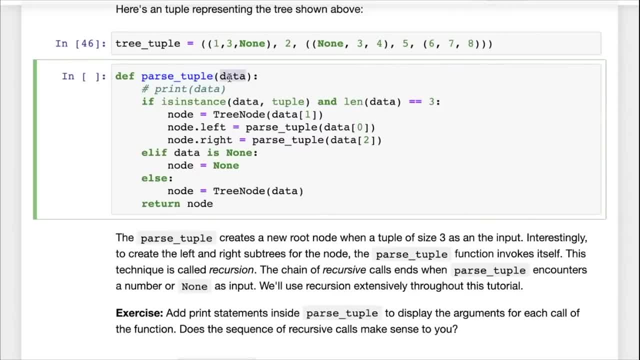 So we call the past tuple function with some data, for instance this tuple, and the past tuple first checks if data is of the type tuple and it has a length three. If these two things hold true, then first we create a node. 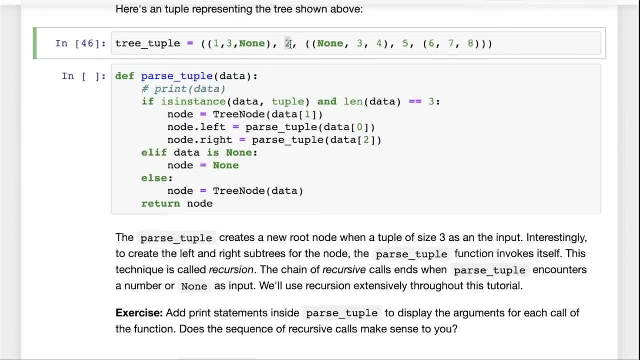 We create a node with data one. So in this case we create a node with two as the key, and then we set the left and the right subtrees of the node. Okay, And then we're doing something very interesting here. We are calling the past tuple function once again. 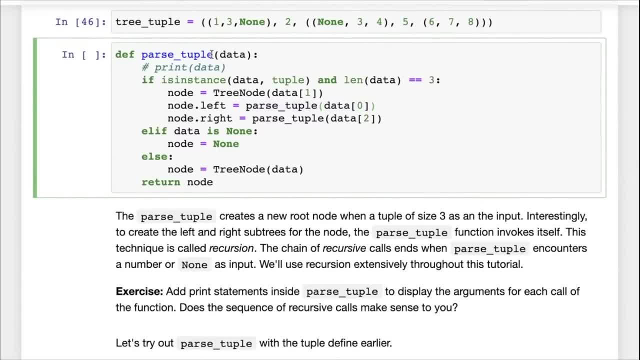 So we call past tuple this time. So this is called a recursion. when a function calls itself inside it, That's called regression. So we call past tuple with the first element, which itself is a tuple, right? So once again, that it calls another invocation to past tuple. 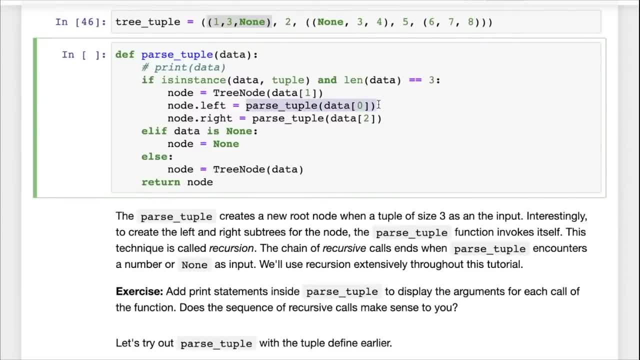 And for a moment let's assume that that returns the proper subtree, the proper node. So we said that node which which Got created, to node dot left, And similarly we create the right subtree using these values. And then we said that node to node dot right. 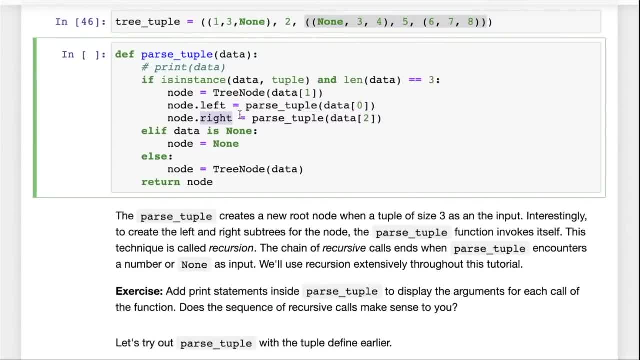 Okay. Now you might wonder in the function we're calling itself. So when will this stop? Can't it go on forever? And that's where you have to track the actual function calls. So when we call past tuple with the entire tuple first, it calls past tuple with this. 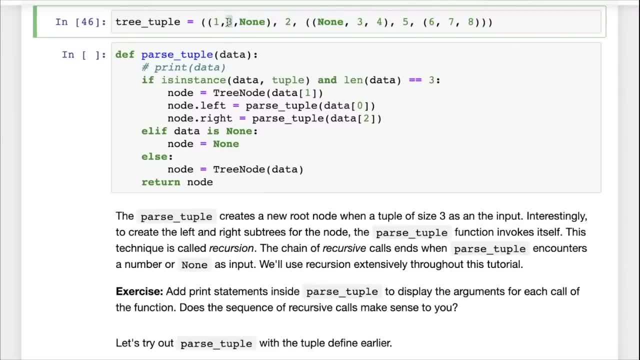 And when you call past tuple with this Uh, then you can see that three is used to create a node and then past tuple is called with one. So when past tuple is called with one, this condition no longer holds true. And we also check the next condition, which is if the data, if one is none and one is not known, 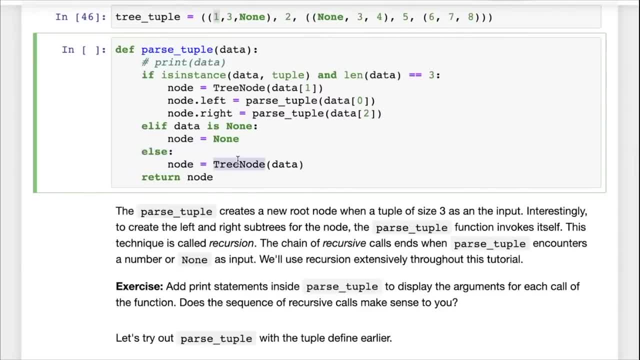 So this condition does not hold true. So we fall into the else condition and we simply create a node. right. So we just create a node, and this time we are not calling past tuple once again, right. So this is called a Dominating condition of the recursive function. 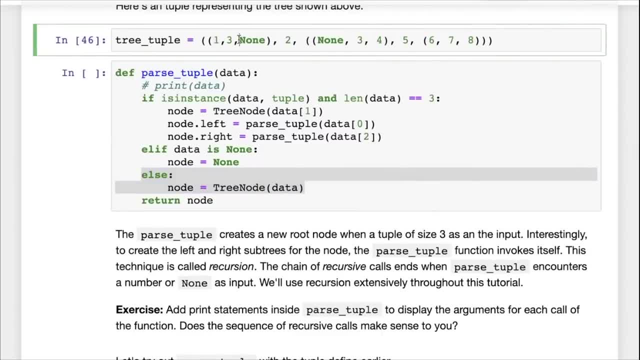 And similarly, once we get back the result from one, then we call past tuple with the value none. Once again, this condition is not entered and this condition matches. So we set node equal to none and then we return the node. 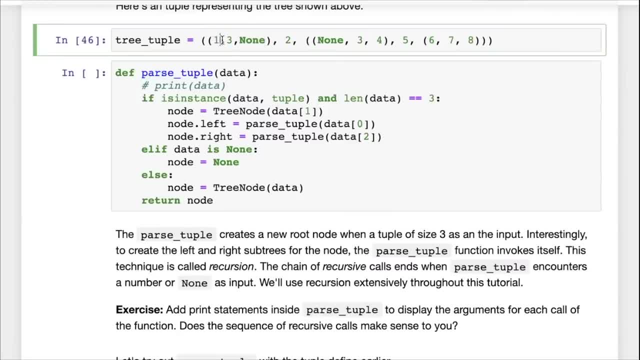 Okay. So when we reach either a leaf node, which is either a single number, or we reach the value none, That is when we stop invoking the function recursively and then the function returns, and that's how the entire tree gets gets. 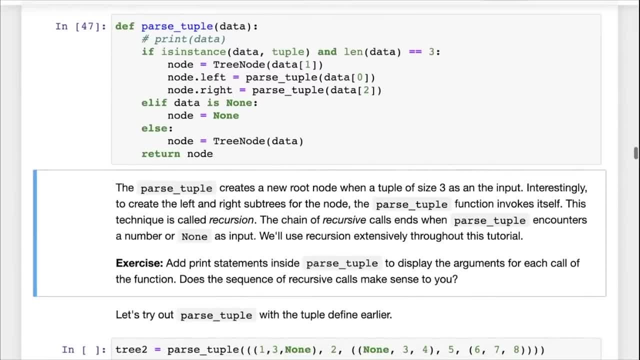 converted. So this is a very powerful idea in programming, the idea of recursion, the idea of functions calling themselves, and it can seem unintuitive and confusing at first. So one thing you can do is you can add a print statement here inside this function, to see how it works, to see how the different calls are going. 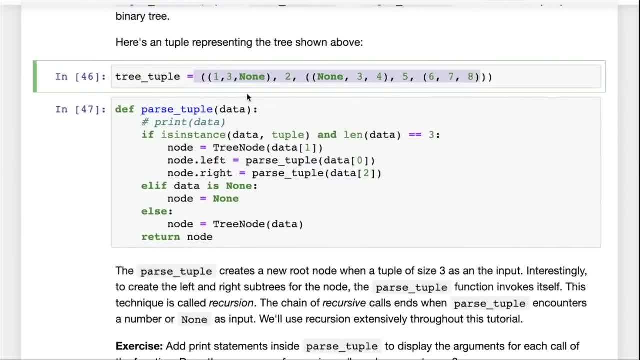 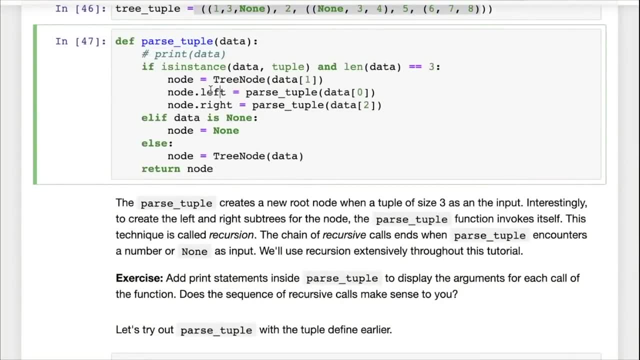 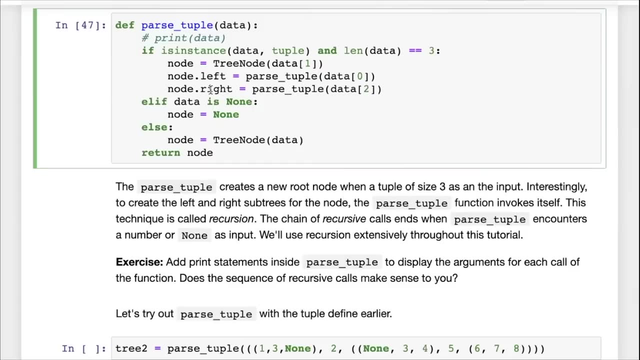 So when you call past tuple with the entire tuple, what are the internal calls that are made? and and study how the result comes out. maybe try it on pen and paper, But it's a very important technique for you to learn. you will be asked or you will find applications of recursions in many places throughout your programming or data science career. 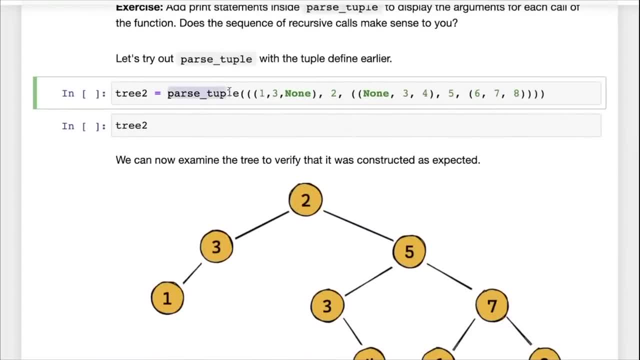 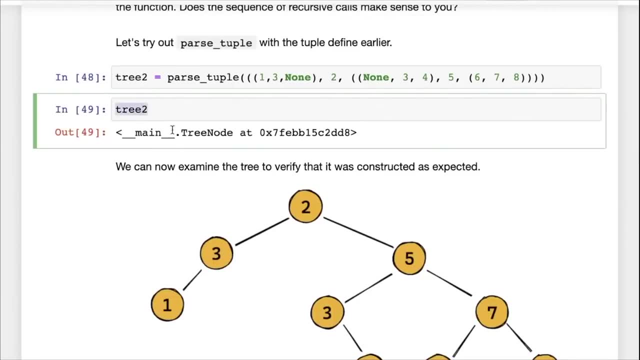 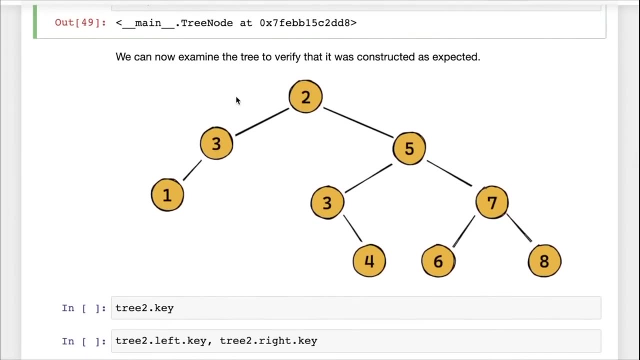 So to learn it. so let's now call past tuple, with this tuple as an input, and let's see: okay, so that returned a tree. and then that tree is of the type tree node. That's great. And now let's examine the tree to verify that it was constructed as expected. 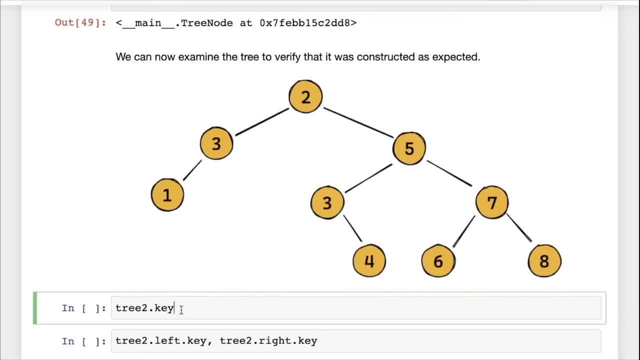 So now we check three, two dot key. So three, two dot key should be pointing to the root node which has the key two. and then let's check the level one. So that was level zero. Let's check level one. 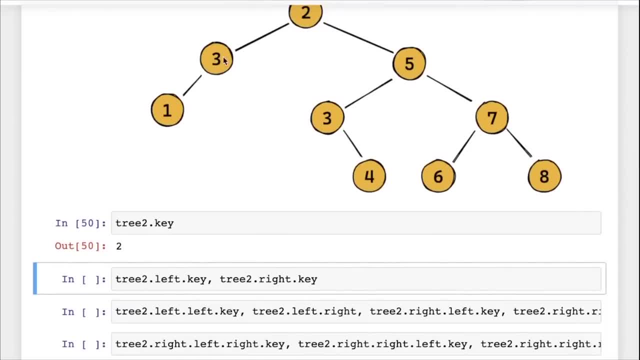 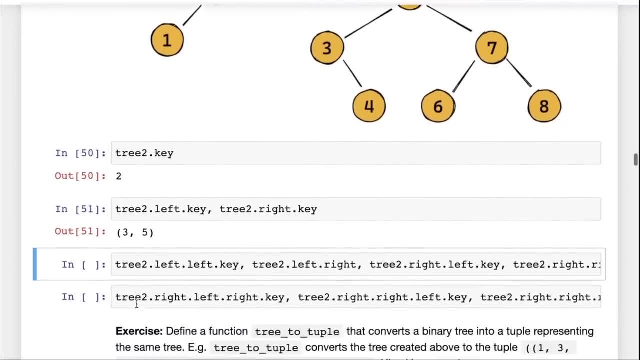 So let's check three, two dot left dot key and three, two dot right, dot key. You can see, here we get the values three and five. Let's check the next level. on this level We have three, two dot left, dot left, and then we have three, two dot left, dot right, but there's no value there. 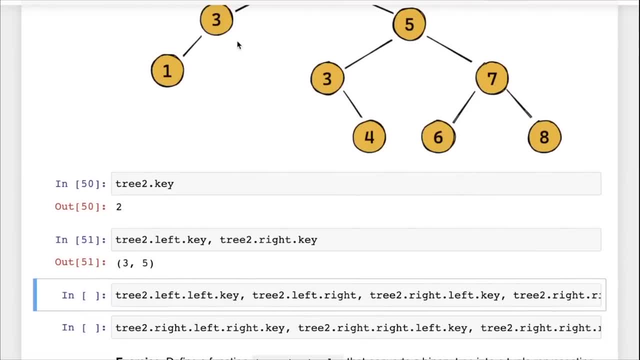 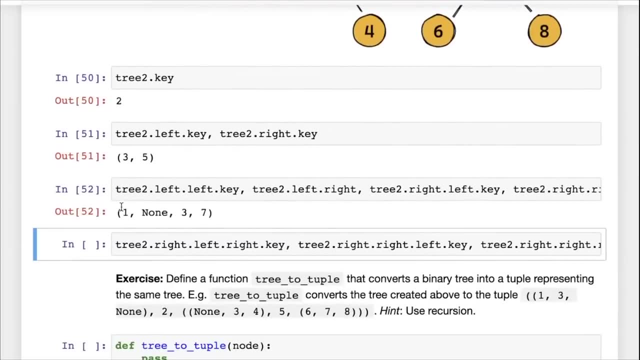 So we can see that we have three two dot left, dot right. So Okay, Can't really check for a key here. then we have three two dot right, dot left and three two dot right, dot right. So you can see that three two dot left, dot left, dot key is one, but three two dot left, dot right is none, because there is no child here. 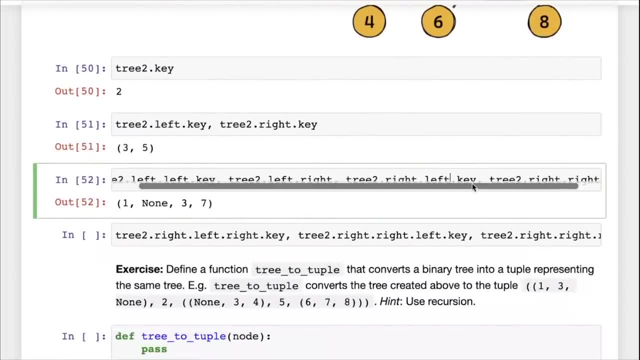 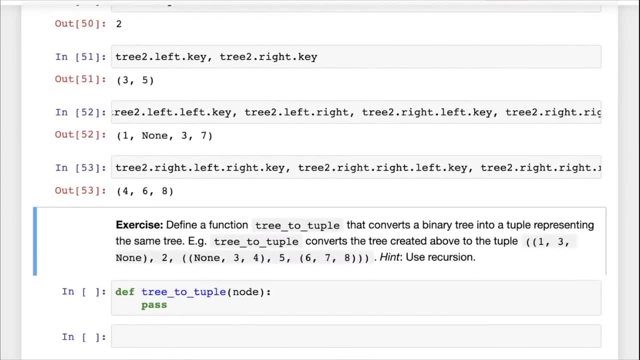 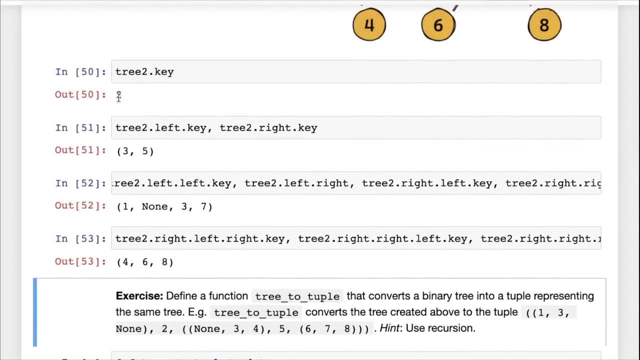 No right child. Then we have left dot key and right dot key and that gives you three and a seven. And similarly you can now check level four, level three, as well. So here are all the levels of the tree. So it looks like the tree was constructed properly and you can see the power of recursion at play here, that the recursive function can now construct trees of any levels. 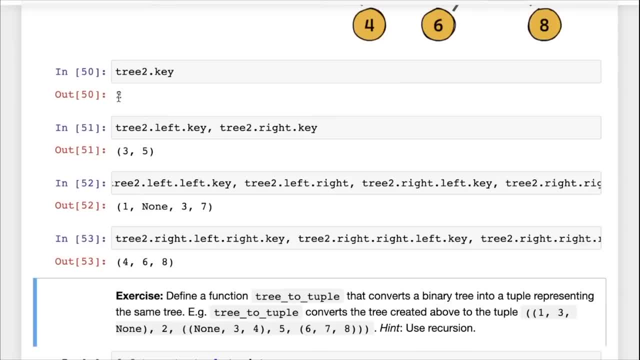 Now you can create tuples within tuples within tuples And as long as they have the right structure, as long as you have this three element structure, whether left element represents a left subtree, the right element represents a light right subtree, in the middle element represents the current node. 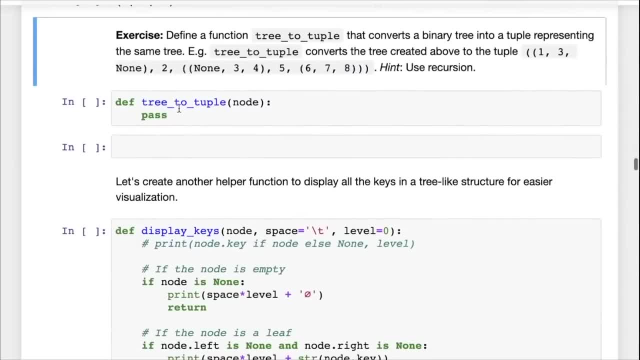 You can construct a tree of any size. So now here's an exercise for you. we've defined a function to convert a tuple into a tree. define a function now to convert a tree back to a tuple. So if you have a binary tree can work. return a tuple representing the same tree. 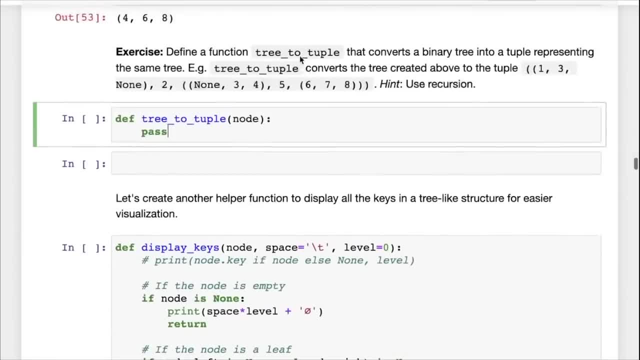 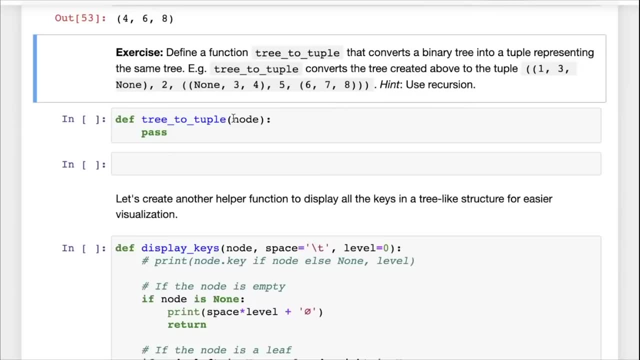 For instance, for the three graded above three, two calling three to tuple should return this original tuple which is used to create the tree. And here's a hint on how to do this: use recursion. So do fill this Out and see if you can figure out how to do this. 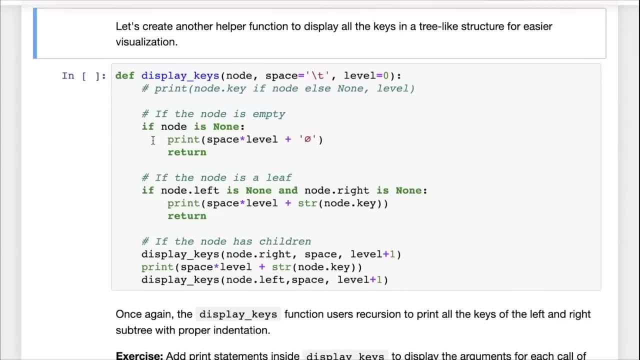 So now we have defined a class for a binary tree and we also have a way for creating a binary tree from a tuple. So now let's create another helper function to display all the keys of the tree in a tree like structure, for easier visualization. 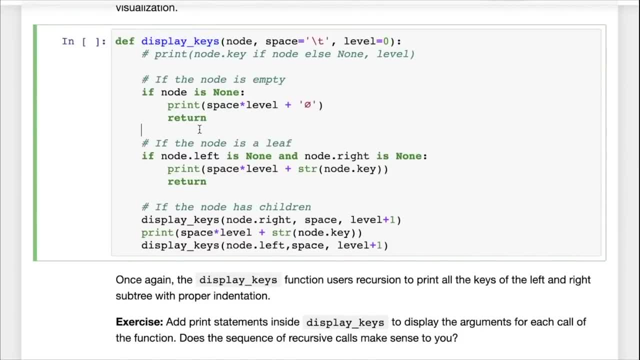 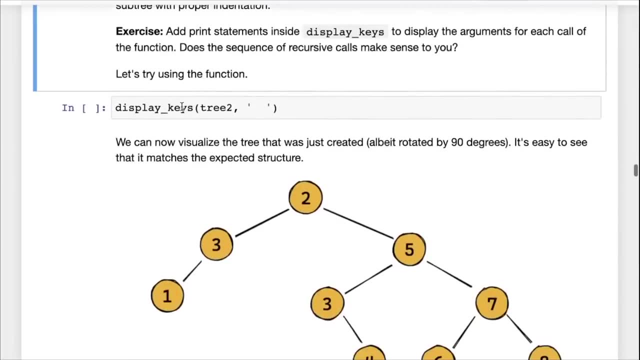 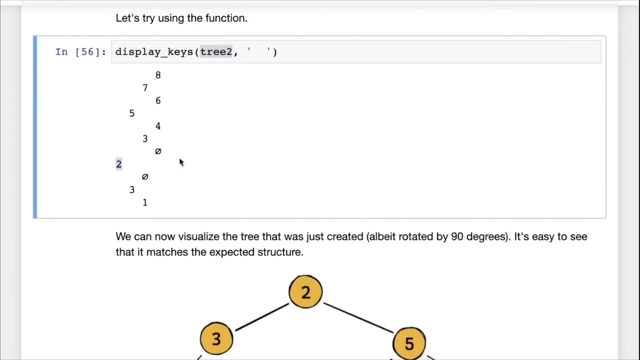 So here we'll just use, we'll call this function display keys, and we'll not get into the code for this because it's, once again, it's a pretty straightforward, but there are a few conditions We need to handle. but here's what it will give us. when we call display keys on a tree, then we'll, then we'll get this kind of a representation of a tree. 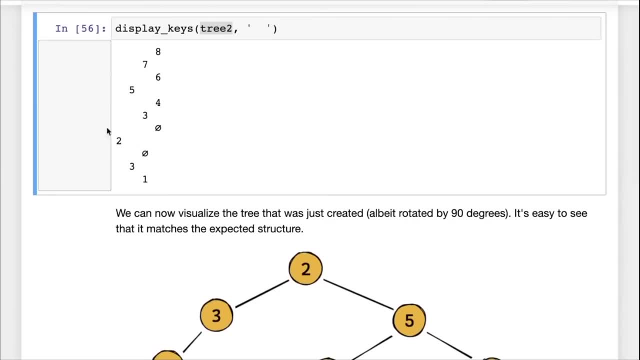 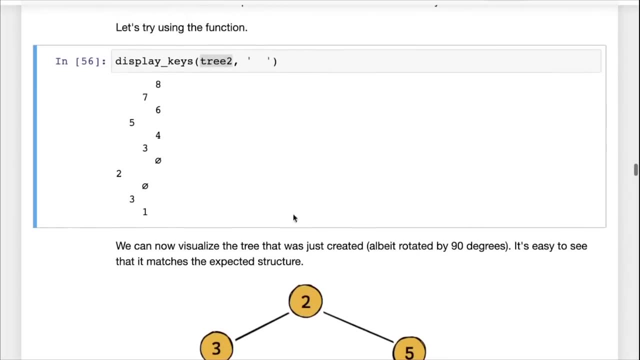 And you can see that this is not exactly the same representation as this. You will have to take this representation and then mentally rotated by 90 degrees in the clockwise direction to get a representation like this. but you can see roughly that the root node is two and then it has a left child three and it has a right child five, then three. 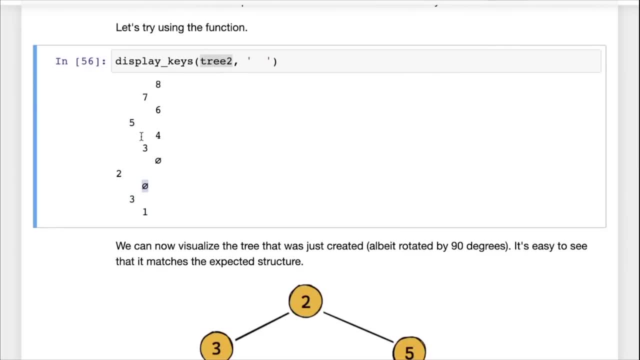 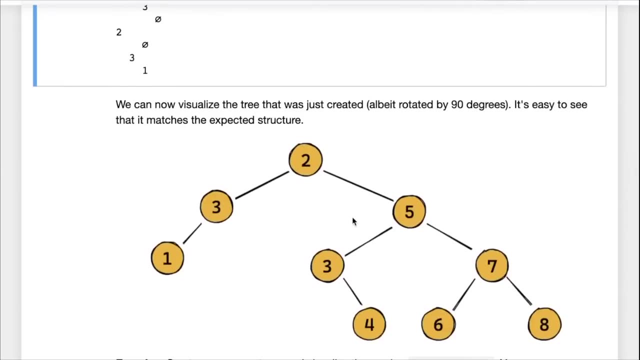 Again, it has a left child, one, And there is no right child. Now five has a left child, three and three has no left child and three has the right child, four and so on. So the exact same structure has been replicated here for us to view visually. 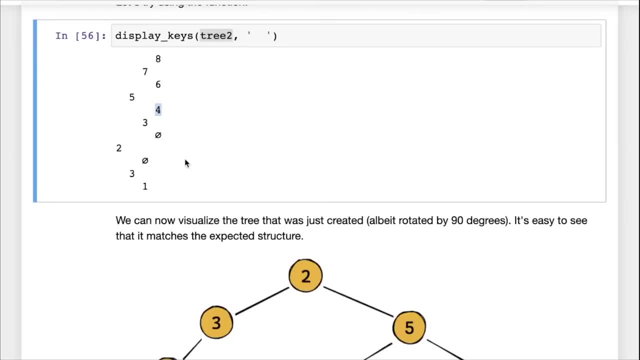 Well, this is a very useful thing. We're spending all this time here or talking about how to create trees and how to visualize trees, because the easier you make it for yourself to create trees, the more likely you are to test. the easier it is for you to test different scenarios out. 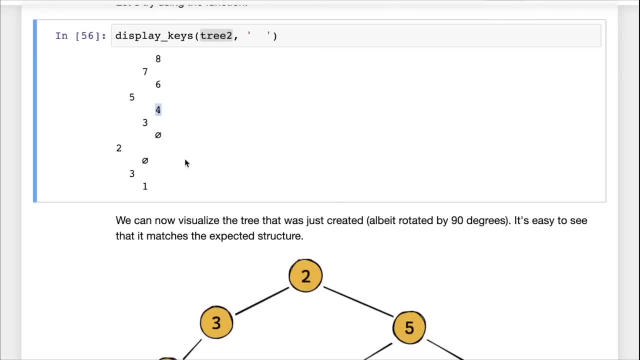 So always spend A little bit of time coming up with good string representations for any data structure. You create something that helps you visualize them and an easy way to create these data structures. Okay, So now we have a way to visualize the tree as well. 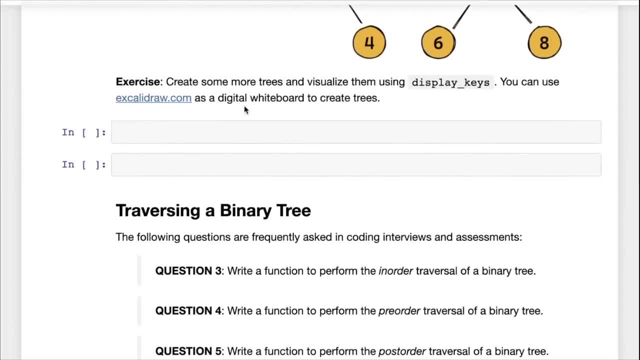 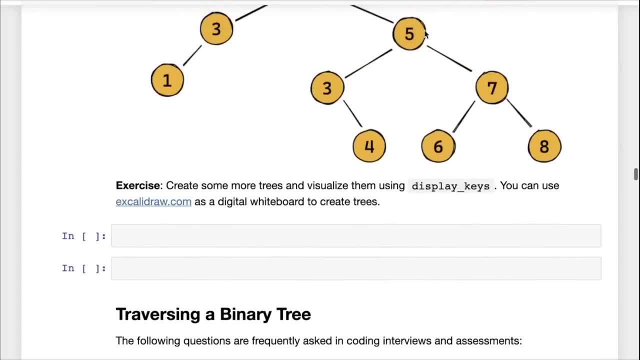 That's great. Now here's an exercise for you. Try to create some more trees and visualize them using display keys, and you can use this tool, Excaliburcom, and that's where, how. that's how these diagrams were created as a digital whiteboard. 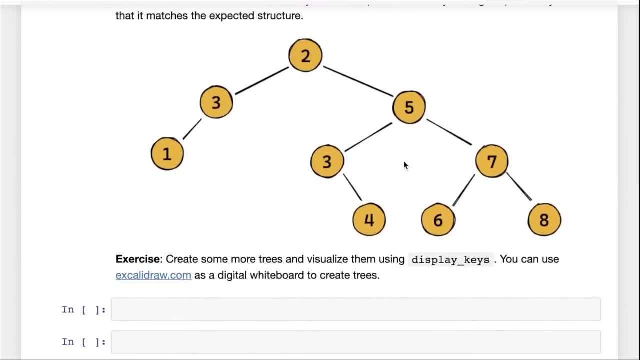 So you can create some Trees. You can create trees like this and then try to create, come up with tuples for those trees, Try to create those trees using the parts tuple function and finally try to display them. Okay, So experiment with it and see, explore what are all the different tree structures that you can create. 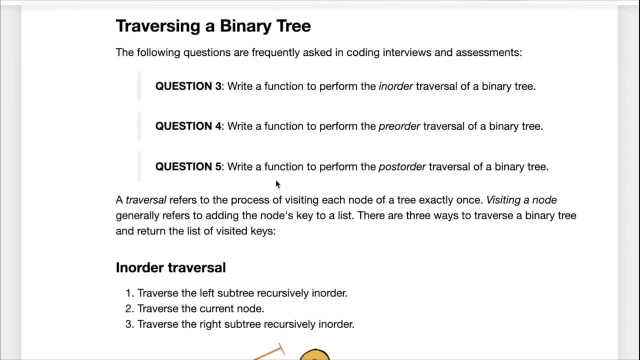 Now the next one of the frequently asked questions in interviews is to traverse a binary tree. Binary tree traversals are very common, So you may face one of these three questions right: A function To perform the in-order traversal of a binary tree, or write a function to perform the pre-order traversal of a binary tree, or write a function to perform the post-order traversal of a binary tree? 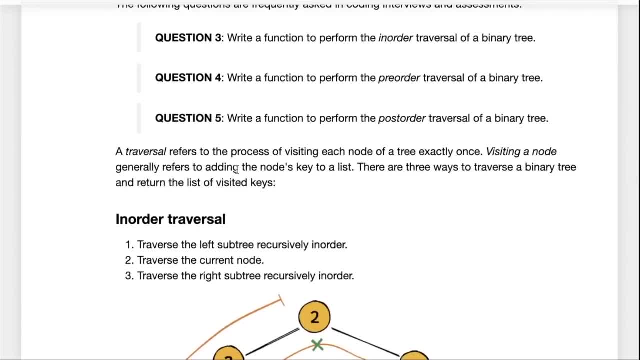 What do you mean by a traversal? A traversal refers to the process of visiting each node of a tree exactly once. Now, what do you mean by visiting? by visiting It could mean any operation, but generally it refers to either printing the key or the value at the node, or adding the nodes key to a list. 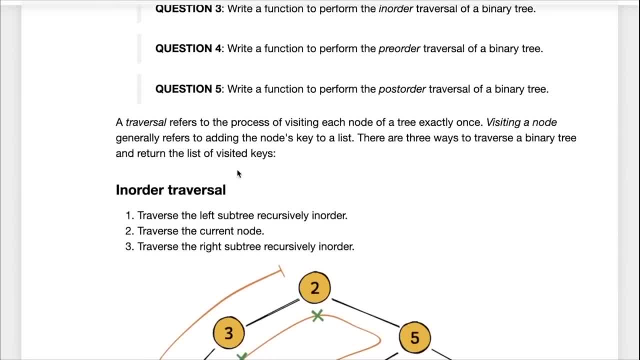 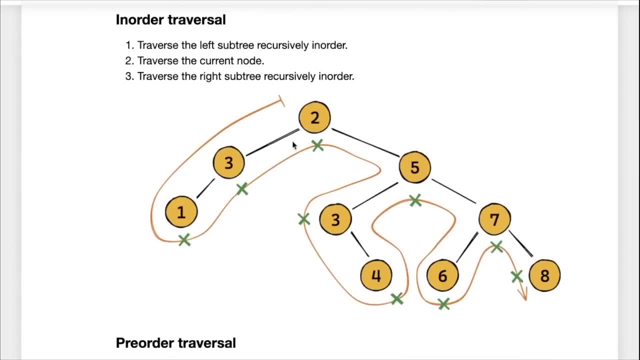 And then there are three ways to traverse a binary tree and return a list of visited keys. So the first one is called in-order traversal and the in-order traversal. Now, traversal is defined recursively because binary trees have this recursive structure. So you will see that almost all the functions that we write will have some sort of a recursive structure. 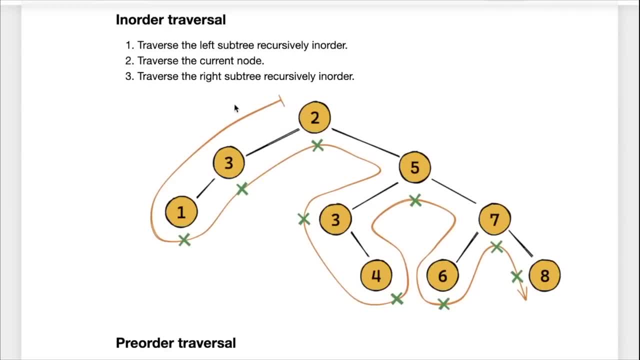 So in-order traversal involves first traversing the left subtree recursively in order- Okay- Then traversing the current node and then traversing the right subtree recursively in order. So what does that mean? Well, we start out with this tree and we're we're traversing it in doing an in-order traversal. 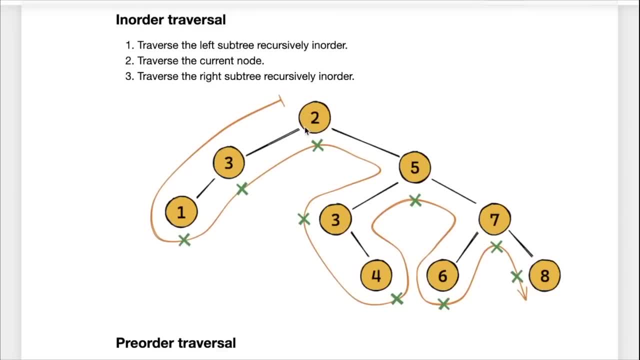 So we try, we look at the root node and then we realize that there it has a left child, So it has a left subtree. So we do not visit it yet, which means we do not print it or we do not add it to our list yet. 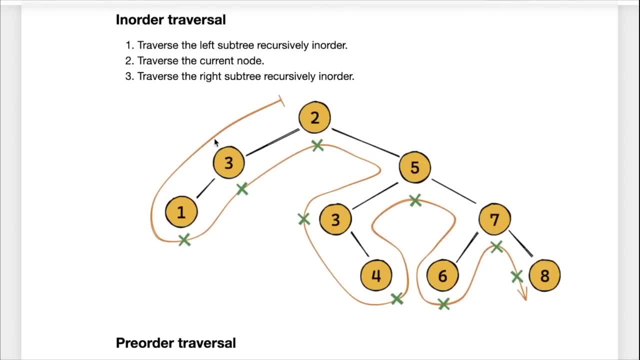 Rather we follow the, we follow the path on the left side and then we come across three And then we realize that, okay, three also has a left child, so we don't visit it yet. So then we go down to one, we go down to one, and now it does not have a left child or a right child. 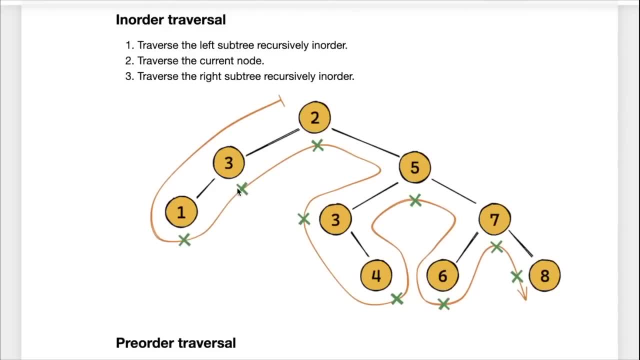 So we can visit one. then we go to three, and now we so we visited the left subtree of three, So now we can visit three, And then the next step is to visit the right subtree of three. but of course three does not have a right child. 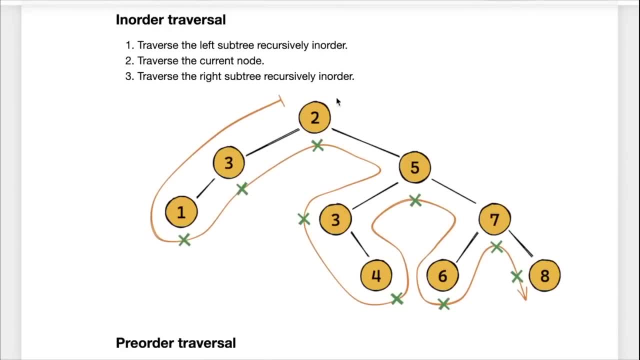 So there is no right subtree to visit, So we can move back up to Two. So now we visited the left subtree of two, So now we can visit two. So we print one, three, two, And now, once we've visited two, we can now visit the right subtree of two. 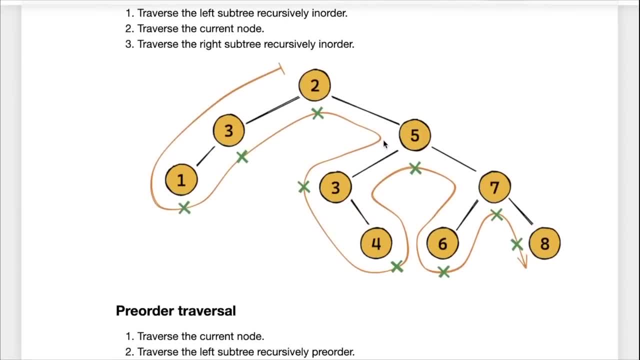 So to visit the right subtree, we go to five. Once again we realize that five has a left subtree, So we go to three. now, three doesn't have a left subtree, So we can visit three. then we visit four, Then now, since we visited the left subtree of five, we can now visit five, and similarly we then visit six. 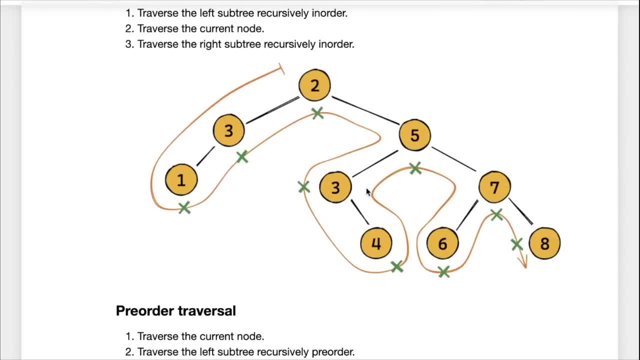 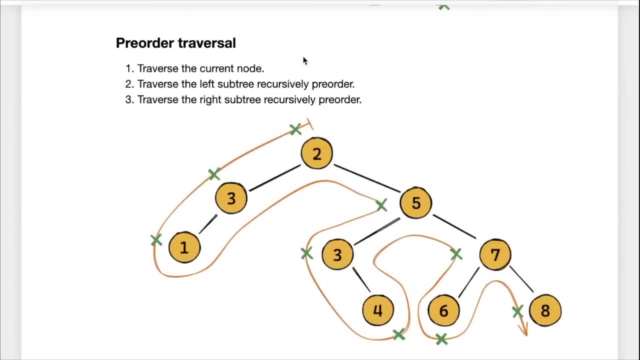 seven and eight. Okay, So that's the in order traversal of the tree. And then there is another traversal, called pre-order traversal, which is slightly different, where you traverse the current note first. So here we start out at two and we say that, okay, we're going to visit two first. 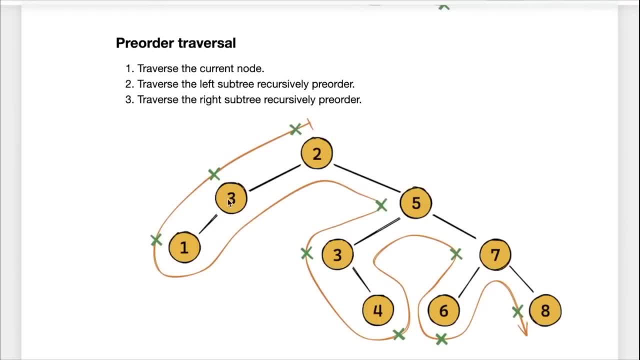 So we visit two, or print it or add it to a list. Then we traverse the left subtree and then we traverse the right subtree. So we go, we visit three and one, and then we come to the right side. We visit five and three. 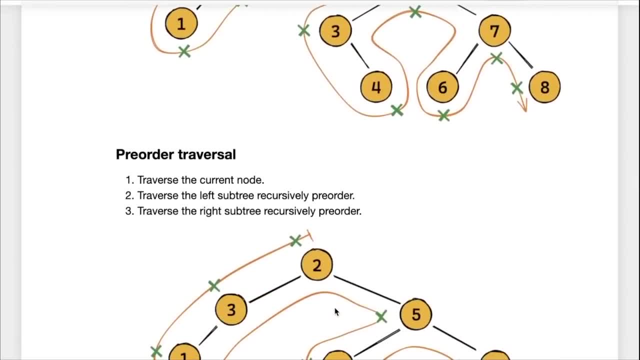 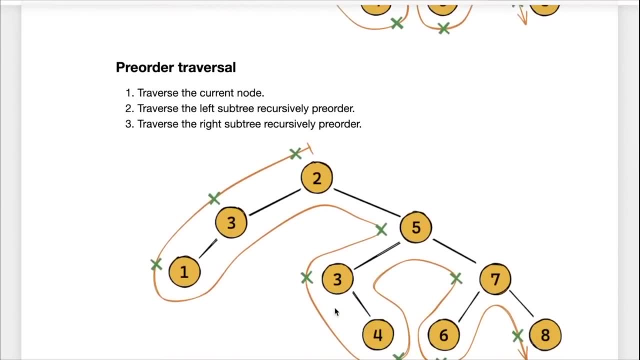 So you can compare these two diagrams and see how- in order and pre-order traversal- Okay, All are different. Now, these are very important for you to for you to understand, because they are great examples of different functions which have very similar implementations. but there are just one or two things you will need to change. 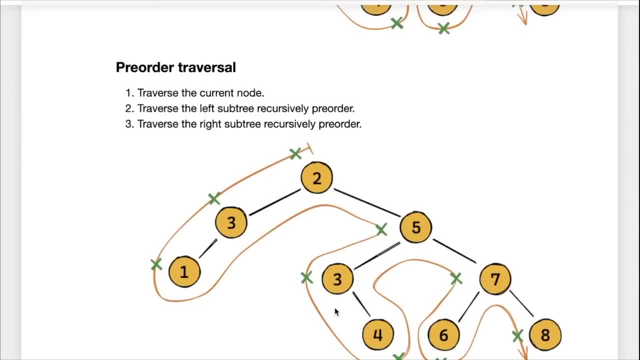 Uh, and these are recursive as well, So do understand the subtle difference between them. And second, they are very commonly asked in interviews. You will most likely face some coding assignment or an interview where you will be asked to perform a traversal of. 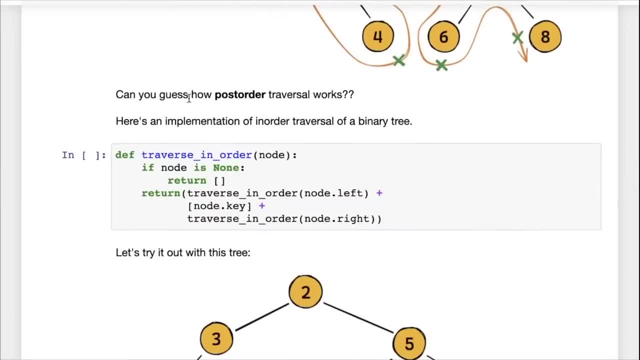 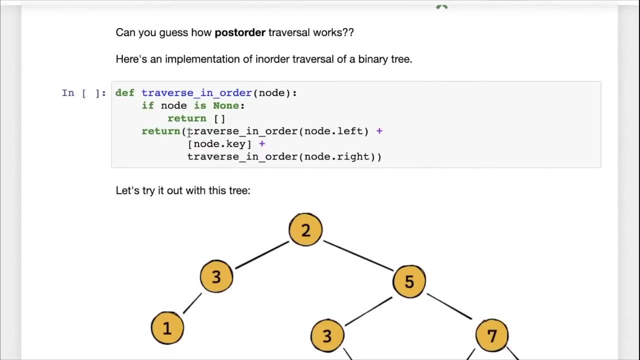 A binary tree, And then finally, there's another order called, another traversal, called the post-order traversal, And I let you guess how it works. You can also look it up. and here's an odd implementation of in order traversal. Now it may seem a little complicated, but it's actually pretty straightforward. 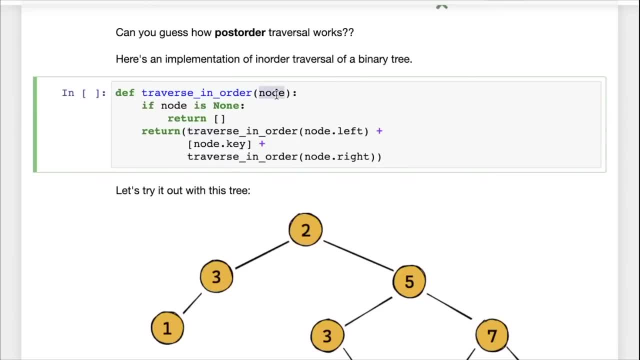 So let's look at it here. What we do is, given a node, we first try was the nodes left subtree. Then we create so that should return a list, a list of all The keys, and then we create a list with just the nodes key. 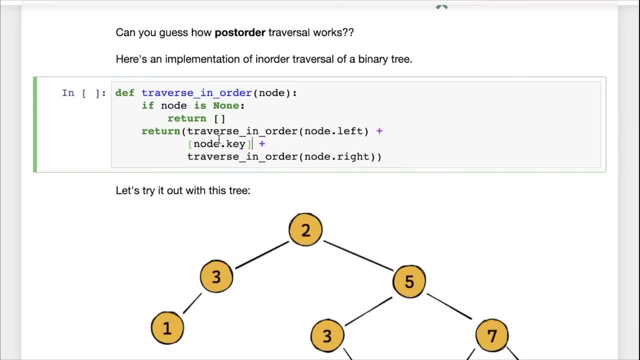 So we get the list of keys from the left subtree in with the inorder traversal, Then we get add to it the current nodes key and then we call it reverse in order with the right subtree And that recursively keeps adding these keys each one and the end condition. 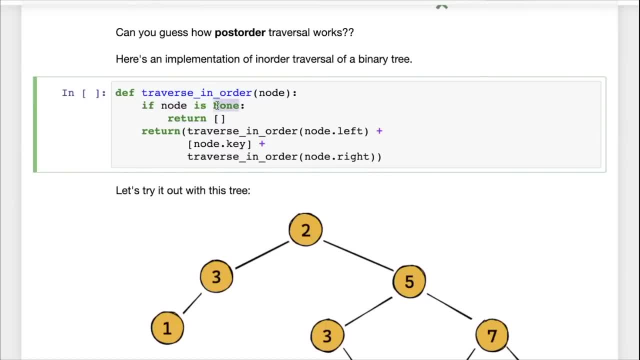 So the terminating condition for the recursion is when we hit none. So when we hit a node which does not exist- so that means we come there from a parent which does not have a left Or right child- then we return the empty array. 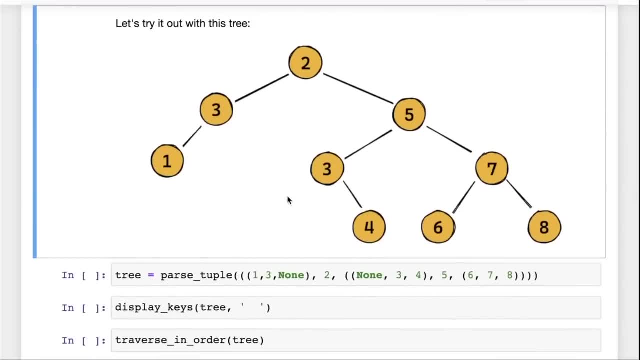 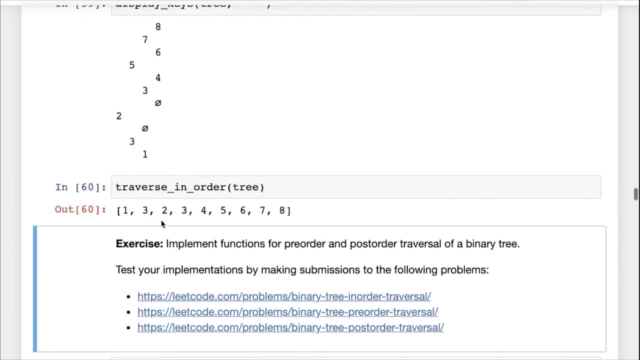 Okay, So let's try it out with this tree. So this is the tree we have and we just saw it's traversal. Now, if we traverse the tree in order, we get the values 1,, 3,, 2,, 3,, 4,, 5,, 6,, 7,, 8, and we can verify here. 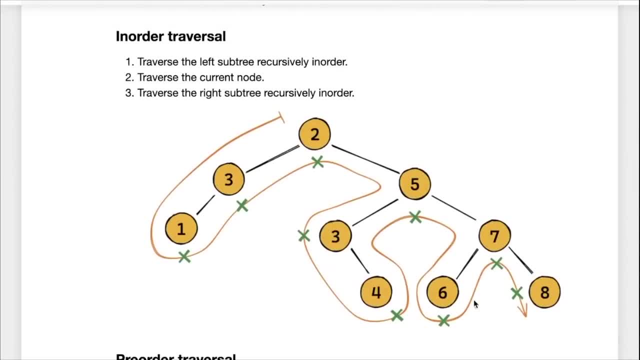 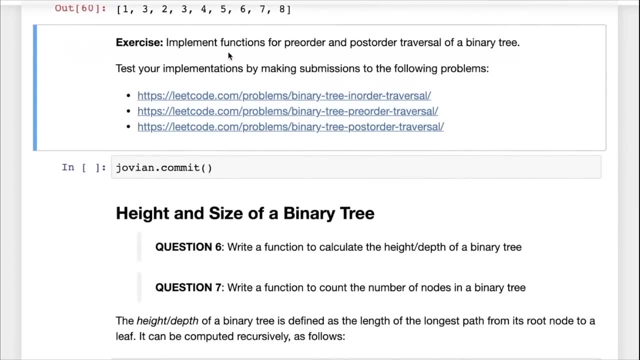 We have 1,, 3,, 2,, 3,, 4,, 5,, 6,, 7,, 8.. So that was the inorder traversal of a tree. Now the exercise for you is to print The pre-order and post-order traversal of the binary tree and you can test. 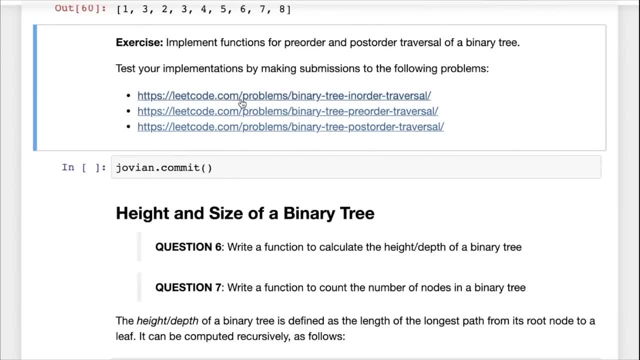 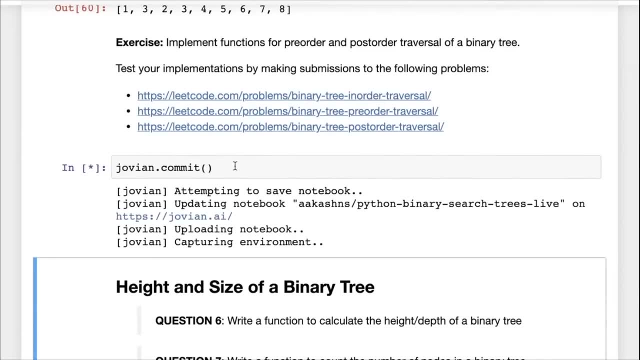 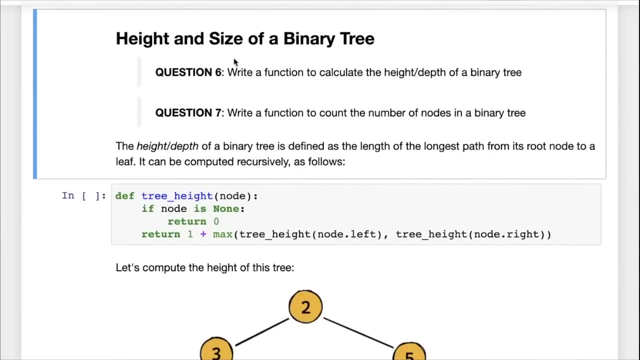 your implementations by making submissions to these problems on leadcodecom. Okay, So that was our discussion about traversals. Another thing that you may get asked commonly is writing functions to calculate the height or the depth of a binary tree and then writing a function. 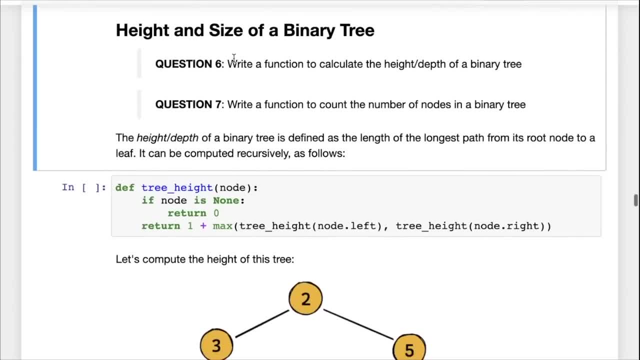 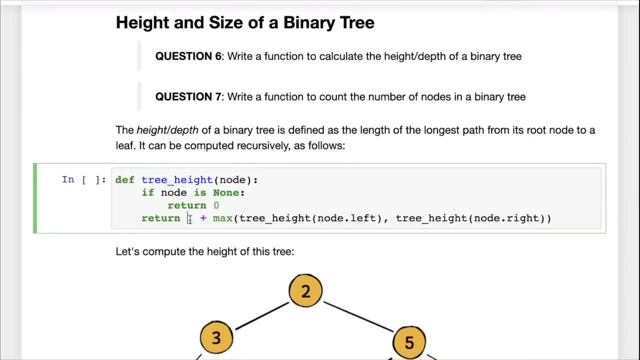 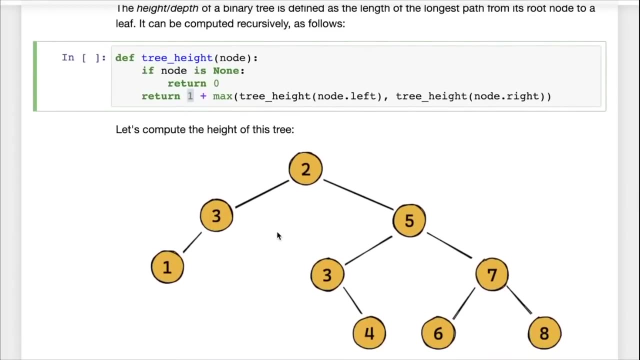 to count the number of nodes in a binary tree. Once again, these can be expressed recursively as well. Now, The height of a tree given a node is simply one plus maximum of the height of the right subtree or the left subtree. The height of retreat is defined as defined as the longest path. 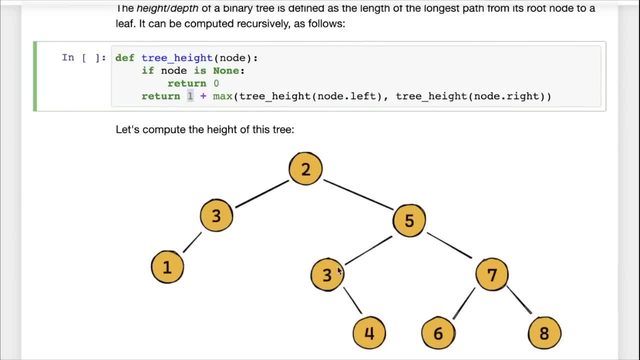 from a root node to a leaf. So you can see that the longest path from a root node of the to the leaf is of length four. so two, five, three and four. And the way to do get the longest length of the longest path is by checking the. 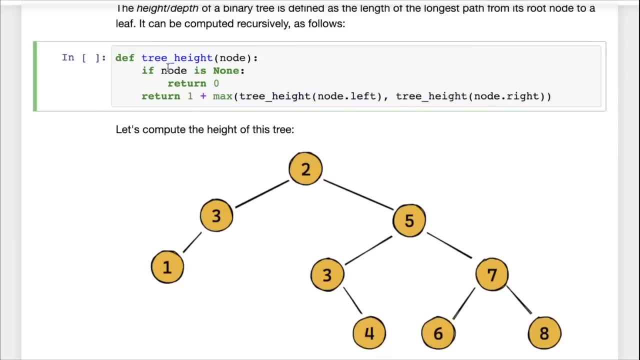 max of the left height, right Height, and then adding one to it. And of course the terminating condition here also is: if you hit a node that does not exist, you return zero. So that's how you get the height of a tree. 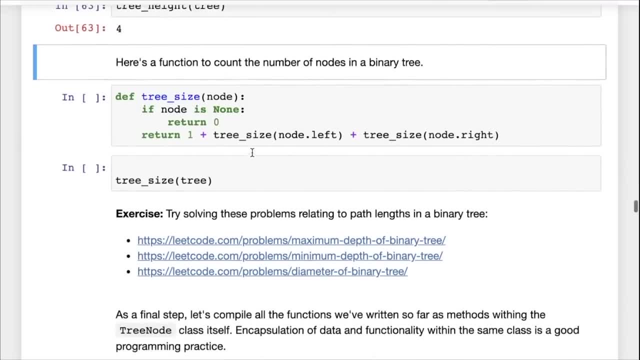 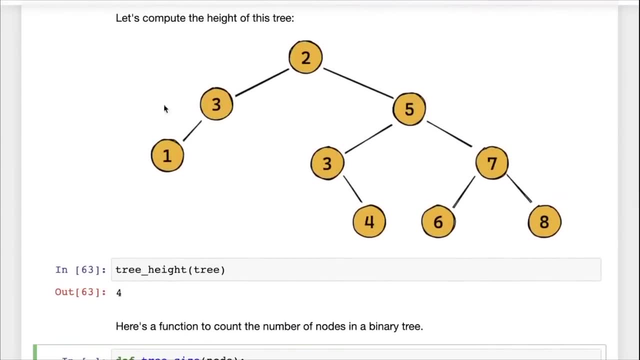 And you can check that the height of a three is four. Then here's another function to count the number of nodes in a tree. Once again, really simple. All you do is this time, instead of checking the maximum, we simply get the size of the left subtree, get the size of the right subtree, add them. 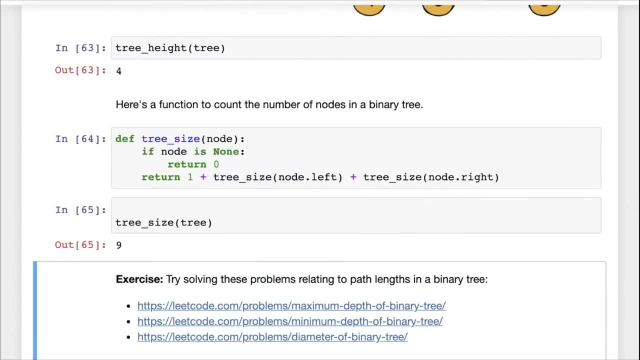 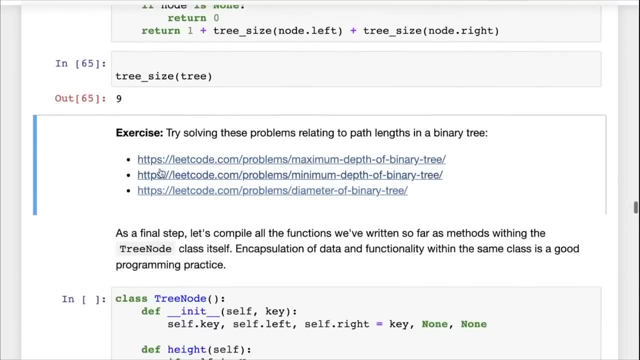 and add one to it. So here you can see that there are nine elements in the street: three, six and nine. So we get three size of three as nine. Now here are a few more questions relating to the path lens in a binary tree. 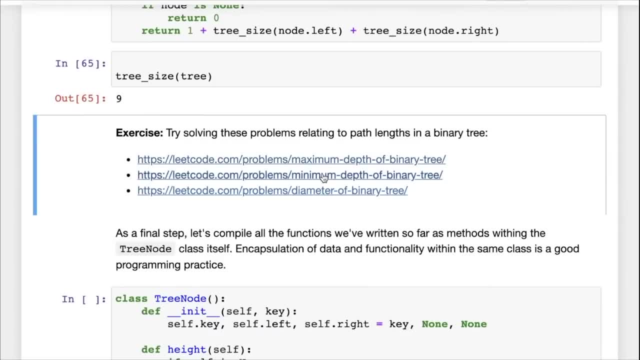 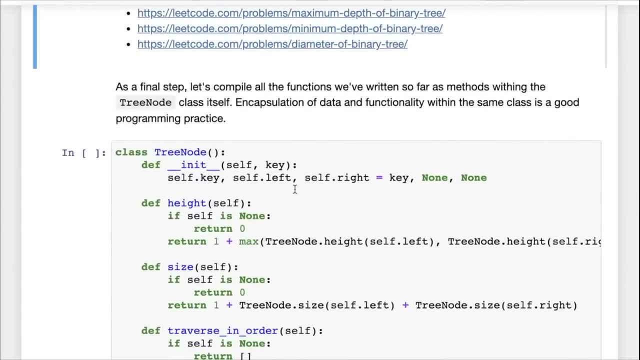 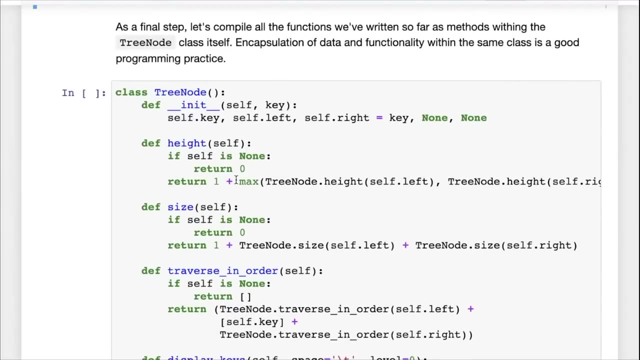 So you can just check. There's a concept of maximum depth and minimum depth, And then there's also the concept of a diameter. So you can try out both of these. now, as a final step, what we can do is we can compile all the functions we've written, all the methods, uh, as methods within the tree node. 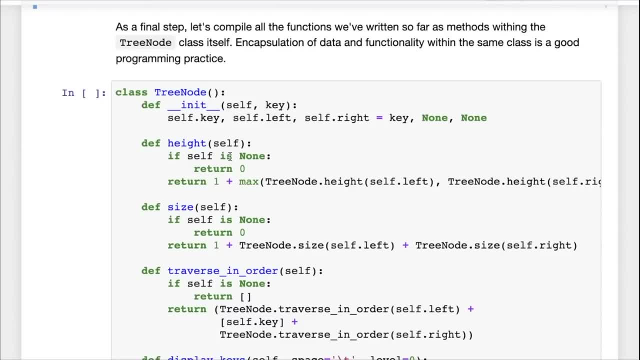 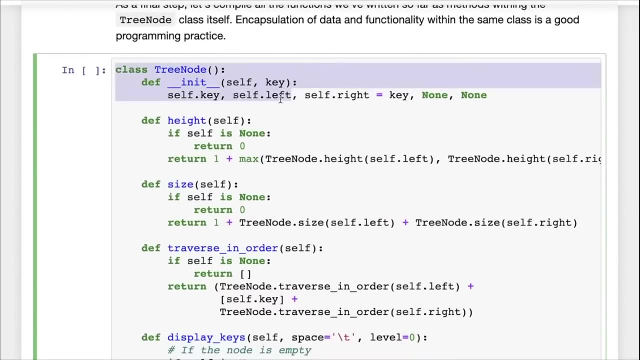 Class itself, And this technique is called encapsulation, where we are encapsulating the data as well as the functionality related with the data or the data structure within the same class, And this is a really good programming practice. So as you write more code, try to think about how you can create these classes with, not just 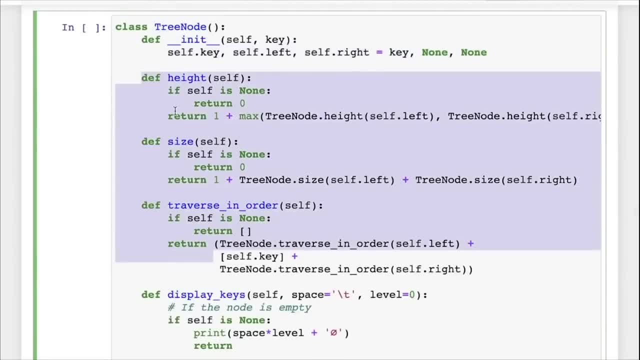 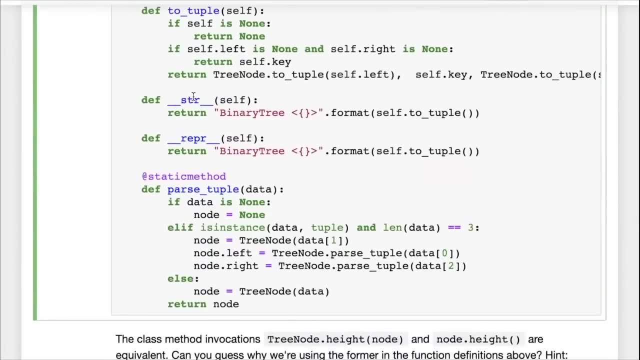 the information inside them, but also with the relevant methods inside them. Okay, So we've now added the methods- height, size, traverse in order, display keys to tuple- and we've also added These methods- STR and rapper, and remember quiz one, or you can go on LinkedIn and post an answer to what. 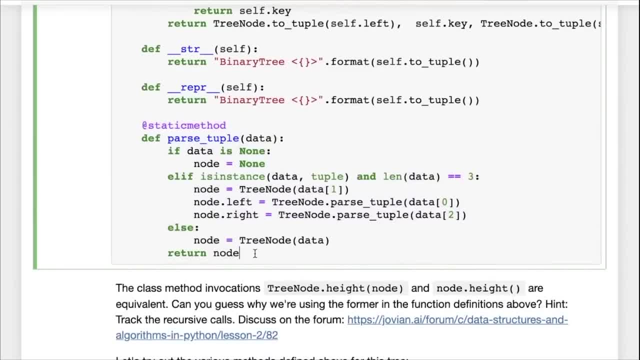 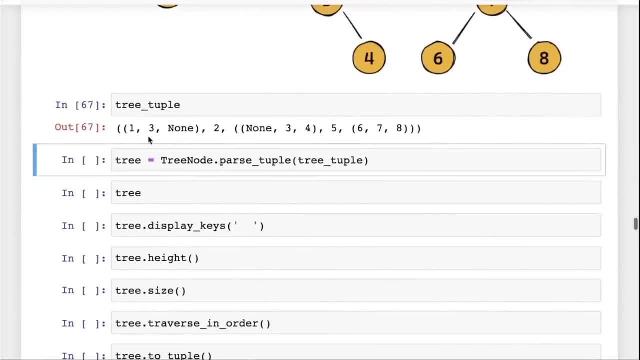 these functions do and finally, pass tuple as well. So all of these functions are now added within the class and you can try it out here. So, for instance, here we have a tree tuple and we can call tree node dot pass tuple to convert this tree. 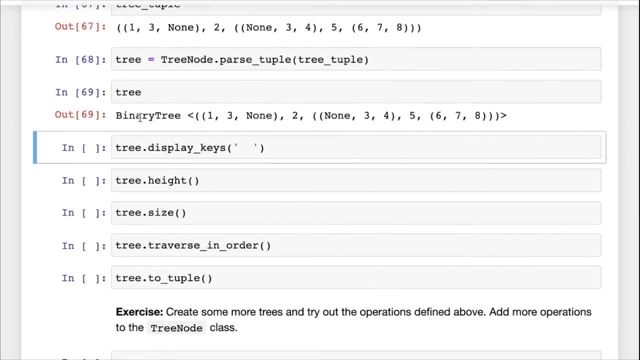 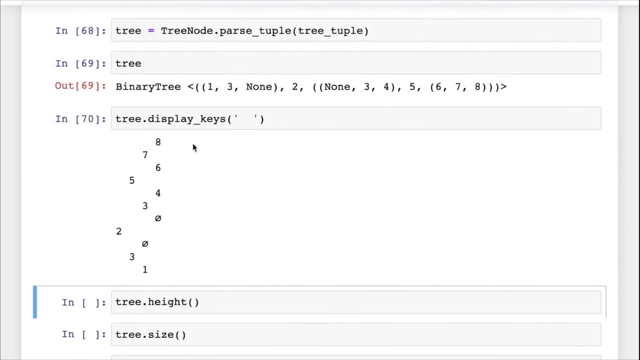 tuple into a tree. So you can see that now we are also representing the binary tree itself using this tuple like representation. but we can also Display it in this hierarchical structure using display keys. Then we can check the height using tree dot height. 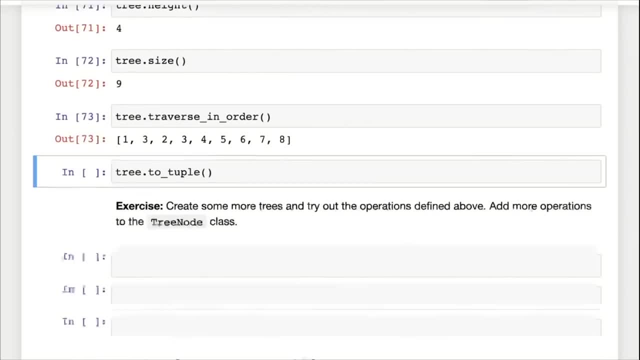 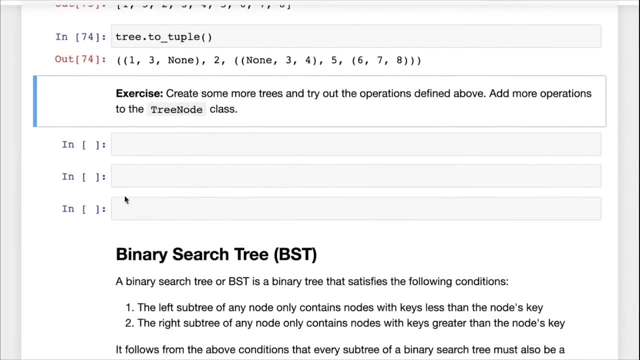 We can check the size using tree dot size and we can traverse the tree in order using traverse in order, And we can convert the tree to a tuple using tree dot two tuple. So do create some more trees and try out the operations that we've just defined, and try all. 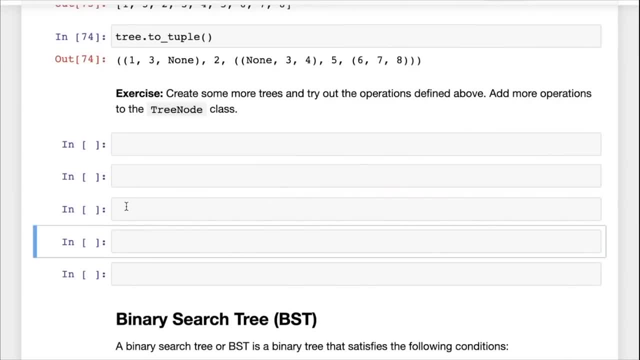 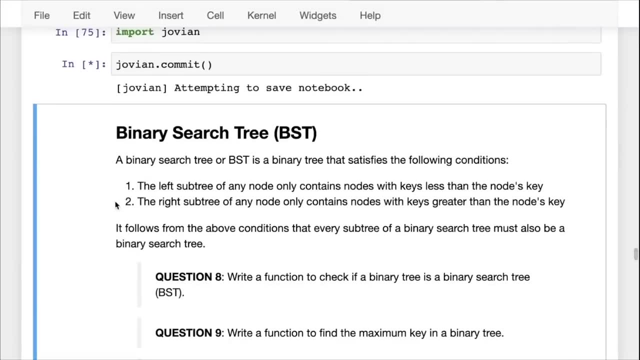 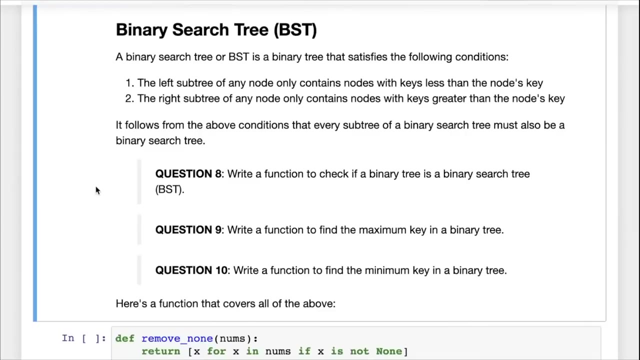 You can also try adding more operations to the tree node class, And before continuing we can Just save our work. So I'm just going to import Jovian and run Jovian dot commit. So that concludes our discussion on binary trees. 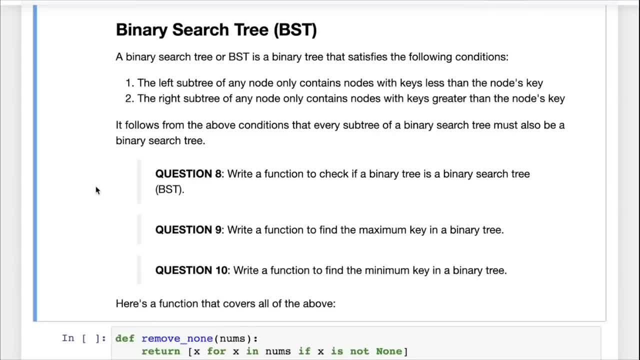 Next, let's talk about binary search trees. Now, a binary search tree, or a BST, is a binary tree that satisfies these two conditions: The left subtree of any node should only contain nodes With keys less than the current nodes key, and then the right subtree of any node should only contain nodes with keys greater than the current nodes key. 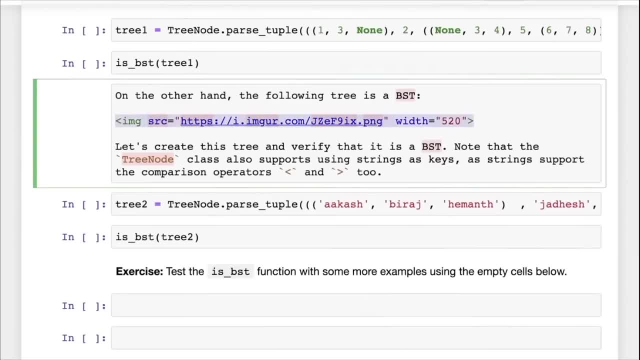 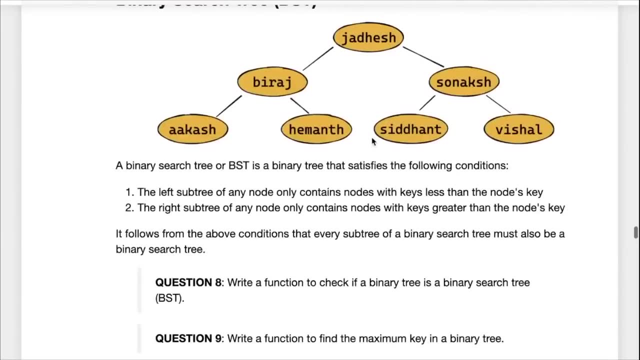 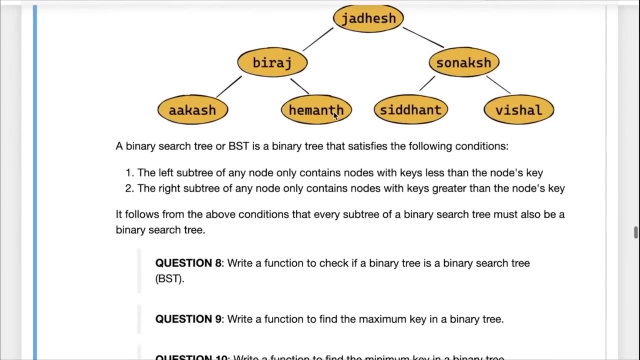 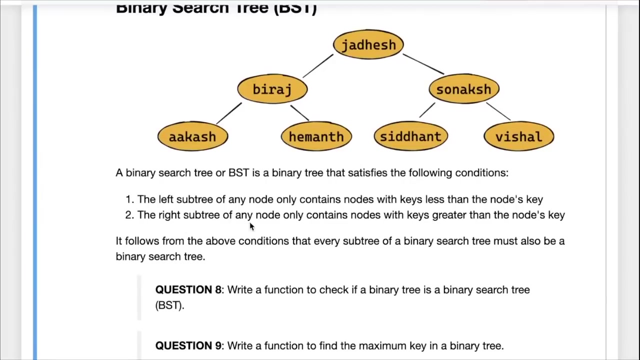 And we can see that this is- let's just copy this over So we can see that this node, this tree here is actually a binary search tree and you can verify that these two properties hold for each of these nodes. And it should follow from these two conditions that every subtree of a binary search tree must also be a binary search tree. 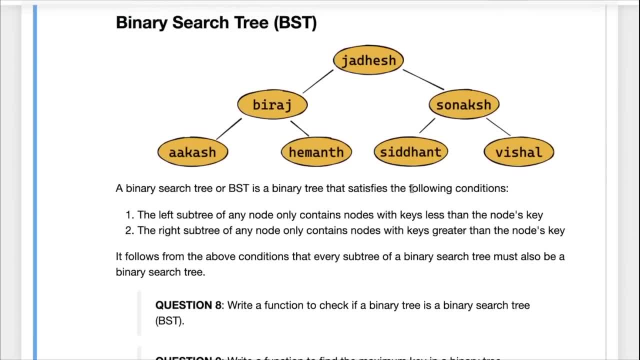 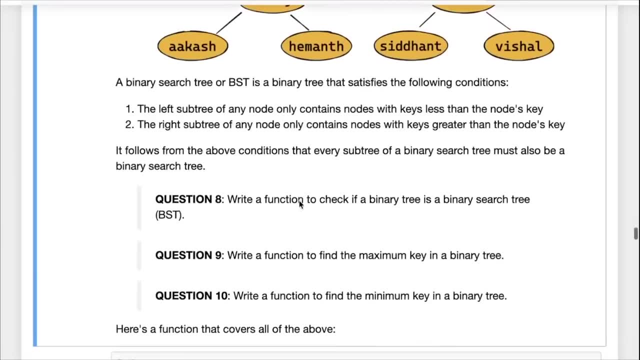 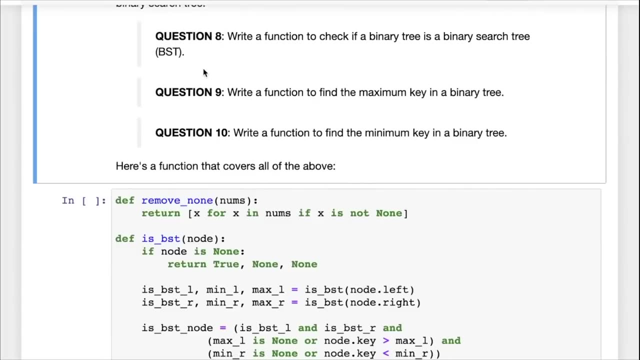 So I can, I'll let you verify that- that if you pick up any subtree inside, so you pick up any node and you see the tree under that node, you will see that it is a binary search tree. So here are some questions that are often asked relating to binary trees and binary search trees, and we've lumped them together because we'll answer them with a single function. 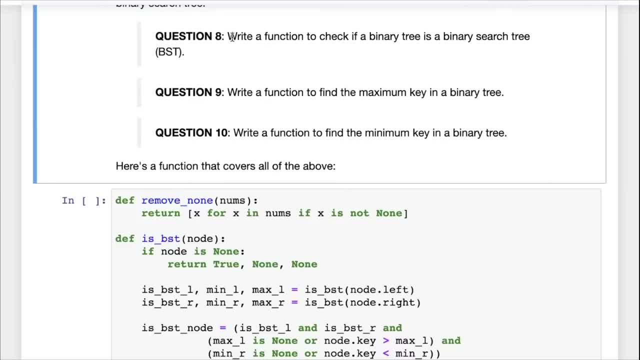 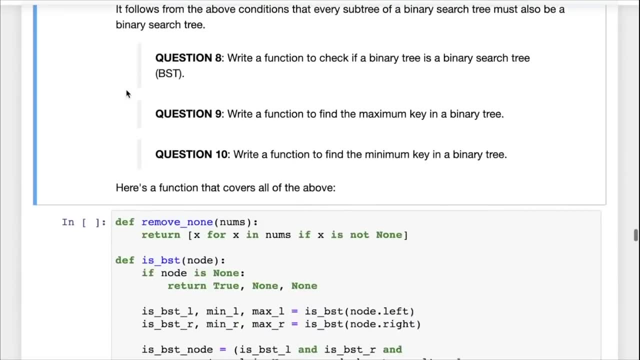 So he's a function that you might Be expected to write. So write a function to check if a binary tree is a binary search tree, which means ensure that these two conditions hold. And second, write a function to find the maximum key in a binary tree. 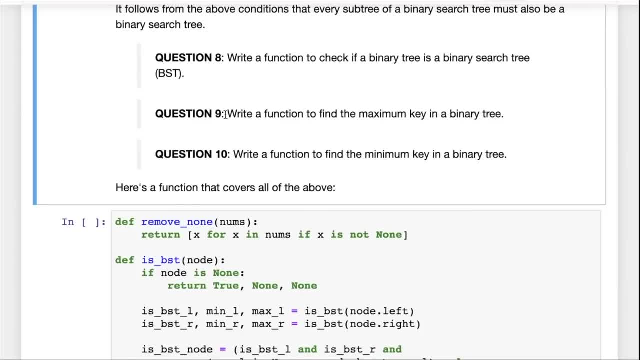 So this could be a generic question: finding the maximum key. And here's another question that you might face: write a function to find the minimum key in a binary tree. So what we will do is we'll answer. we'll answer all of these questions together. 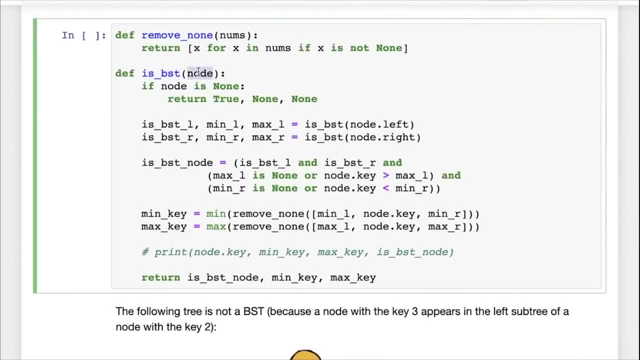 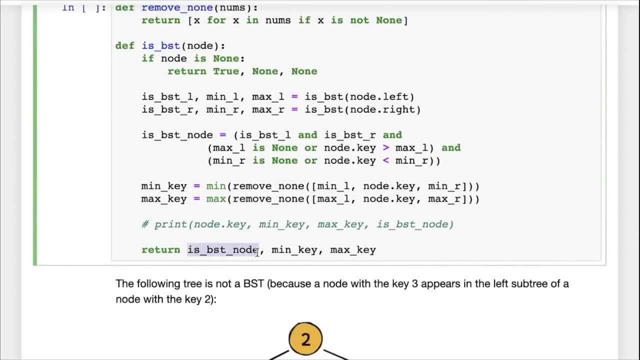 Okay With a single function called is BST. So is BST. takes a node and then is BST returns three things. So if you look at the return value, it returns whether the node and the tree under that node is a BST. So here. so this is going to be the value determining. it's going to be either true or false, telling us whether the tree under that node, with that node as root, is that a BST. it also returns the minimum key from that. 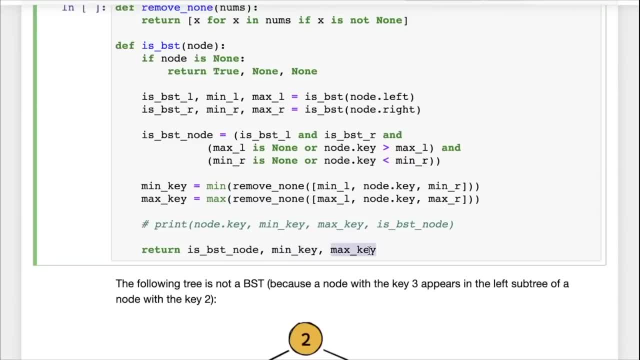 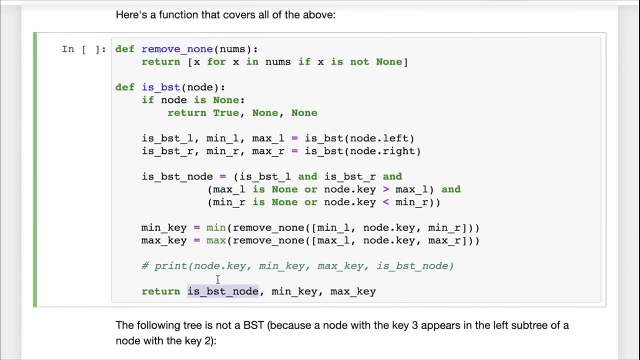 End Entire tree And it also returns the maximum key from that entire tree. Now why are these two useful? We'll see in just a moment. So the way we calculate is BST node is by actually looking at the left subtree and the right subtree recursively. 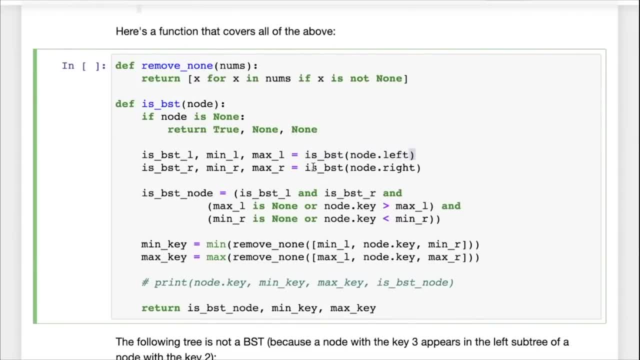 So we call is BST on the left subtree of the node and we call is BST on the right subtree of the node. So we get back three values, which is: is the left subtree of binary search tree. is the right subtree binary search Tree. 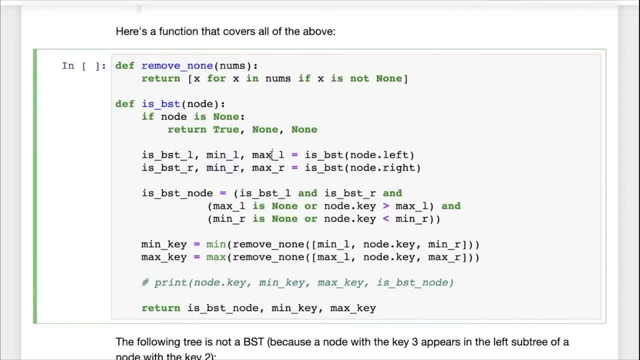 The minimum key in the left subtree, the minimum key in the right subtree and then the maximum key in the left subtree and the maximum key in the right subtree. So now what we can do is we can say is is BST node, So is the entire tree of binary search tree. 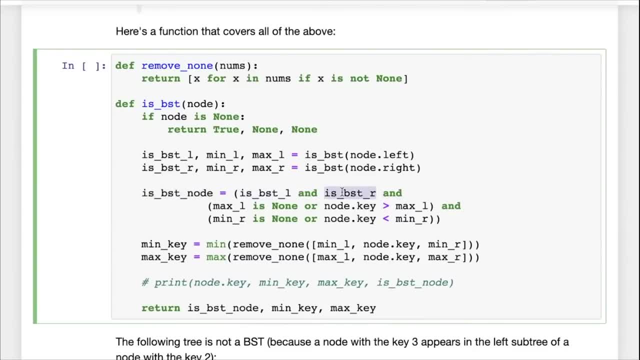 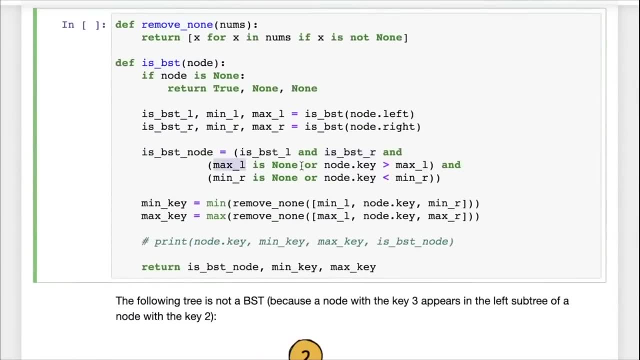 Well, if the left subtree is a binary search tree and the right subtree is a binary search tree, and then we verify these two properties, which is the maximum key in the left subtree is either none, which means that there is no left Sub. 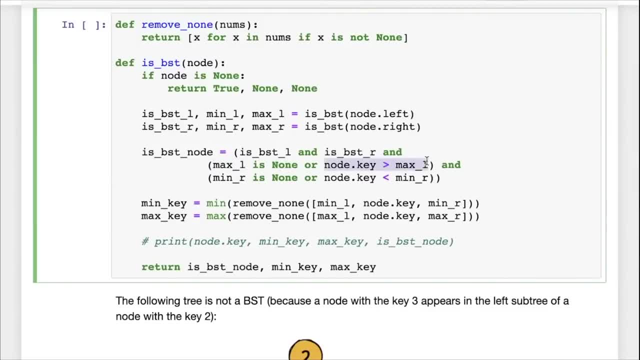 sub tree or the current nodes key is greater than the maximum key And the minimum key in the right sub tree. the smallest key in the right sub tree is either none, which means that there is no right sub tree, or the minimum key in the right sub tree is greater than the current nodes key, so that this 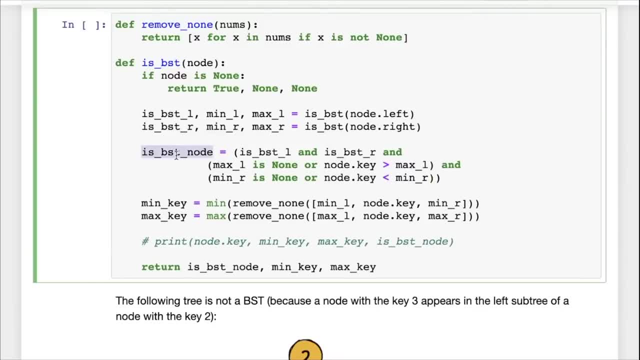 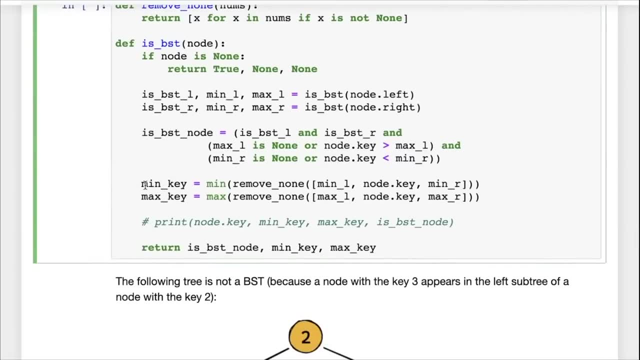 was condition one and condition two, And that tells us whether this entire tree is now a binary search tree. And then, finally, we can also calculate the minimum key and maximum key simply by computing the minimum of the left minimum node dot key and right minimum. 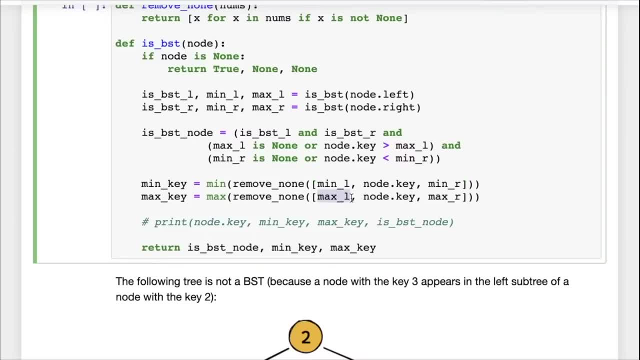 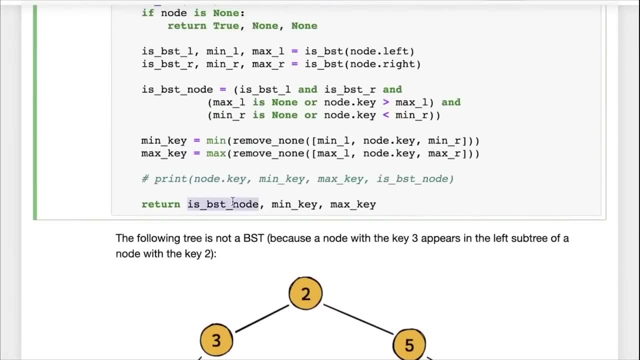 And the maximum can be calculated by checking the maximum of the left maximum node dot key and right maximum. Okay, So what we return from the is BST function is whether that a node and the tree represented rooted at that node is a binary search tree, and then the minimum. 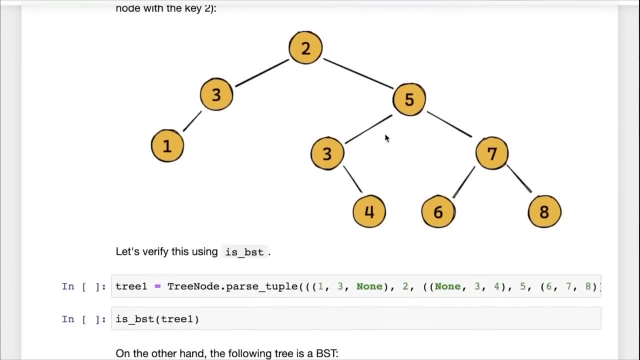 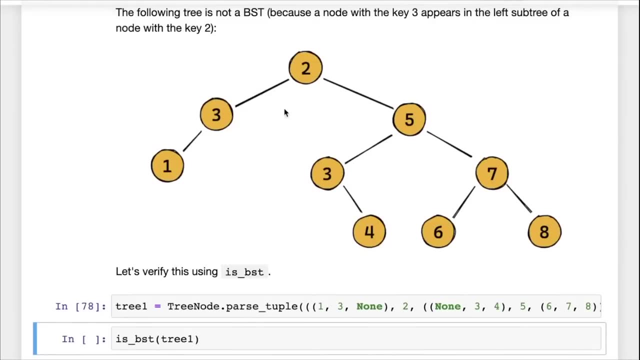 and maximum key out of it. So if we look at the BST function- This tree right here, let's verify whether this is a BST And well before we check we can probably tell that it's not, because you can see that three appears as a left sub child of two, but three the key is greater than two. 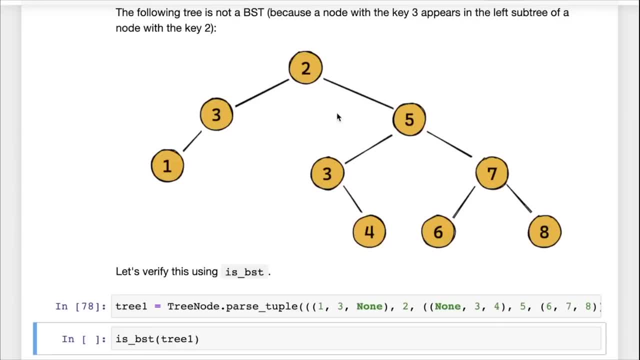 And that's a problem. So this is a violation of the property elsewhere. This property satisfied. You can check any other node here and you will find that the left sub tree is always Smaller than the right than the node and the right sub trees larger than the node. 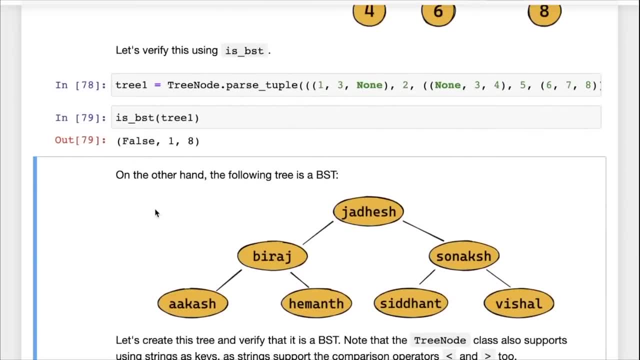 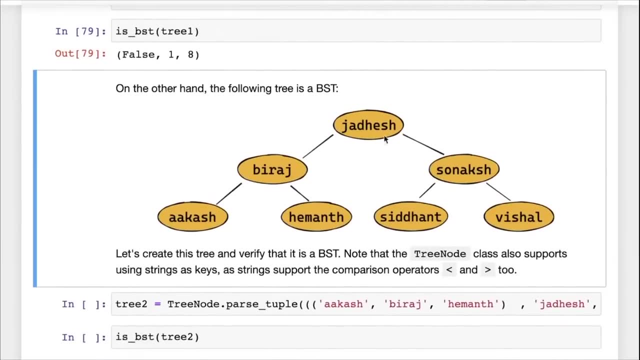 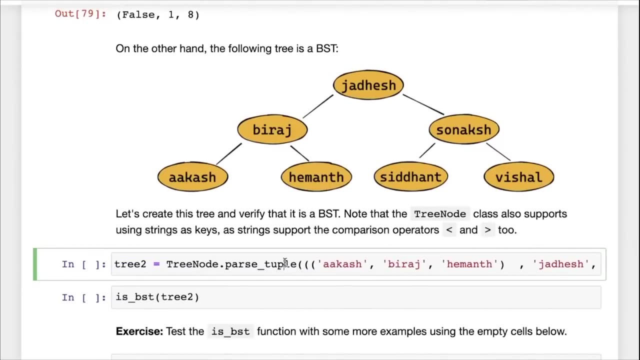 So let's check: is BST tree one? It's not, so that's false. Now, on the other hand, this tree is a BST. This is the tree that we've been looking at all this while. So, once again, we can create this using tree node dot, parsed tuple, and note that. 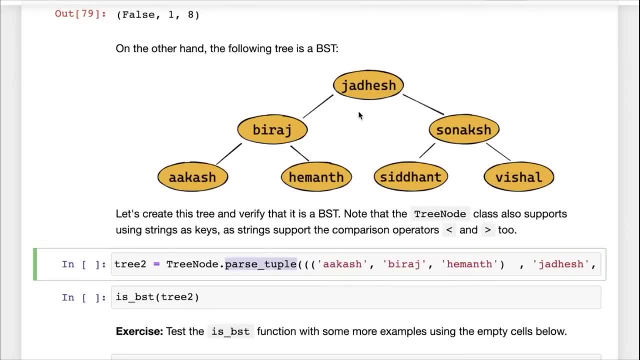 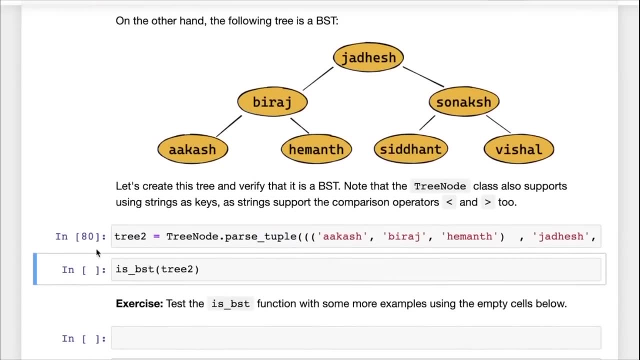 the keys can. the way we've implemented three node keys can not only be numbers, but they can also be strings, So we don't need to change anything here. And that creates three, two And we can even display three, two surface to do three: two dot display keys. 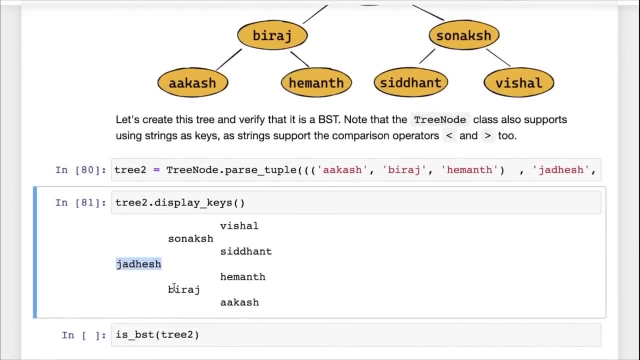 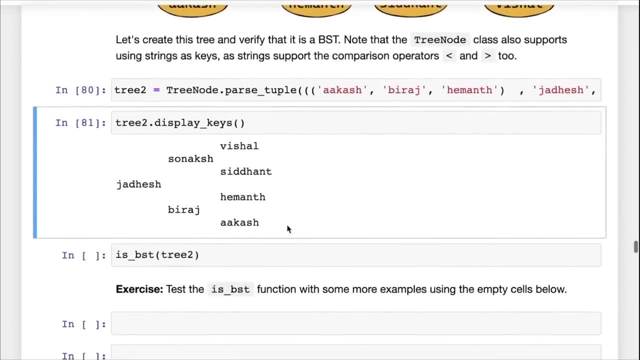 You can see that it has the structure where is at the center, And then on the left you have barrage. on the right You have so much barrage and so much. Then you have Akash, Hemant, Siddhant and Vishal, and this is a BST. 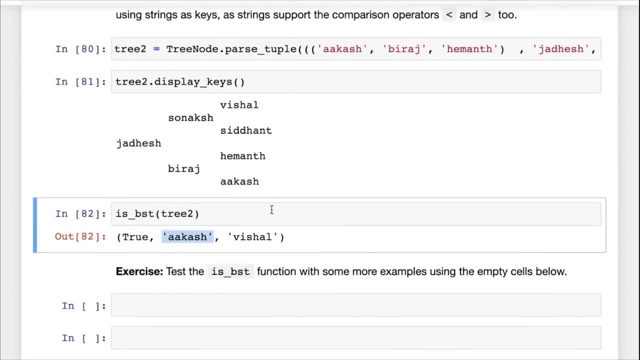 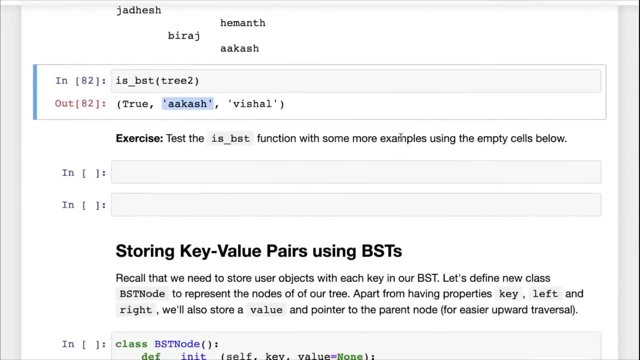 So you get back through here and the smallest value here is Akash and the highest value is Vishal, As you can verify in alphabetical order. So that's pretty handy. Now we have a way to check if a binary tree is a binary search tree. 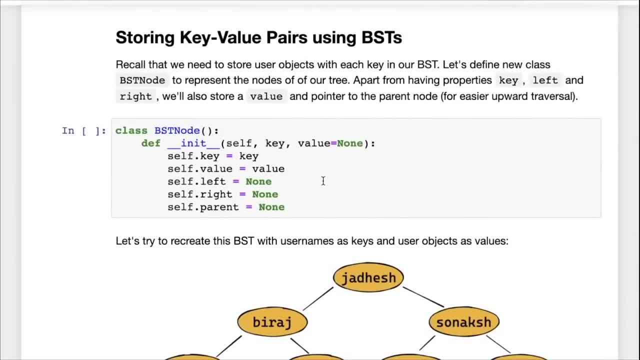 And this is again a very common interview question that you might face. next, Remember that we need to store not just keys, but also user objects within each key, with each key within our BST. So what we do is we'll define a new class called BST node, to represent the notes of our binary search tree and BST. 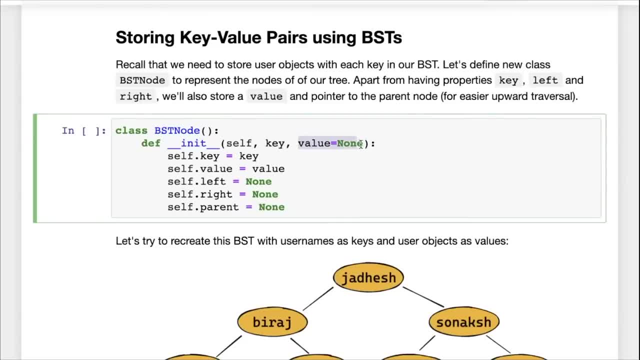 BST node will not only have the key, but in the constructor it can also accept a value, and this is optional. So we will set the key and we set the value. We will also set the left and right. apart from this, we also set another property called parent, and the parent will point to the parent nodes. 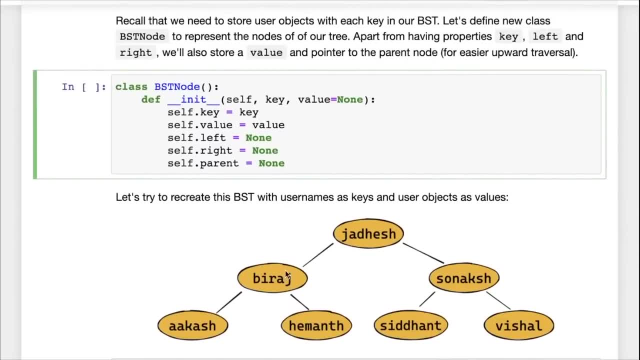 So, for instance, if this node is a left subtree of this route, then the parent of barrage will point to Jadesh and this will be useful for upward traversal. Now if you're given a pointer to a node and you have to go back and find the root of the tree, 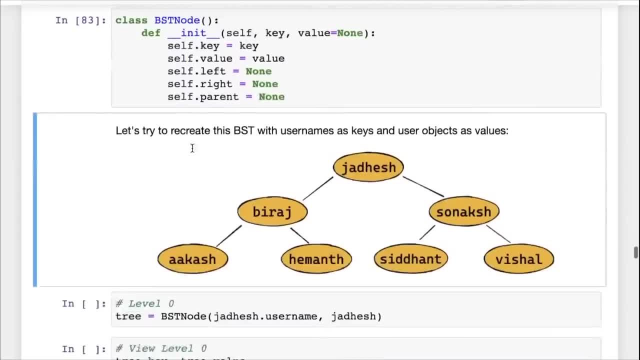 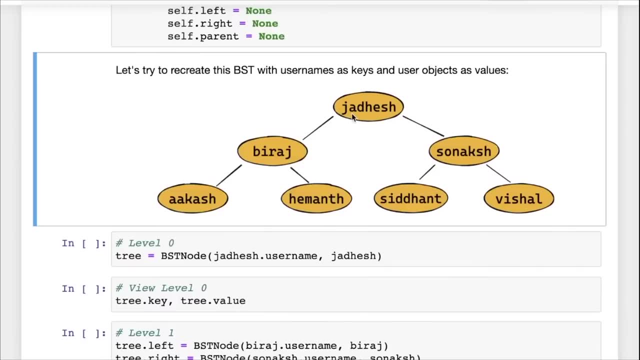 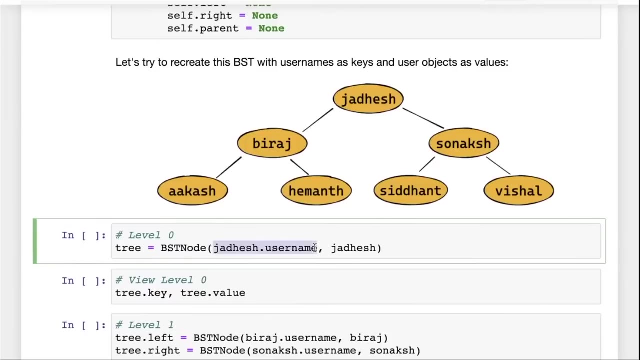 The parent will be helpful there. So this is our BST node, And let's try to recreate this BST right here with usernames as keys and user objects as values. So first we create level zero. So level zero, we create BST node. Now the key is Jadesh or username, which will be just the string Jadesh. 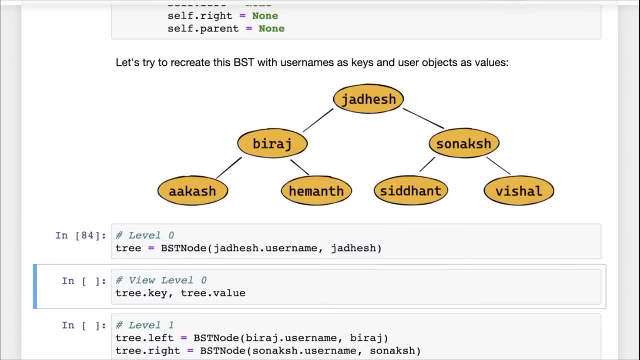 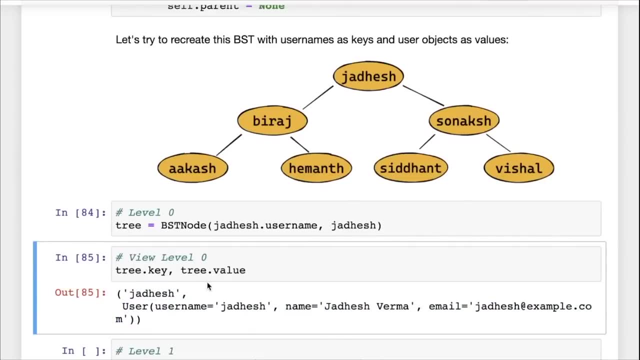 And then the value will be the Jadesh user object. So we've created that and we can check its key and value. You can see that Jadesh is the key And then the user object Is the value let's create. let's create level one. 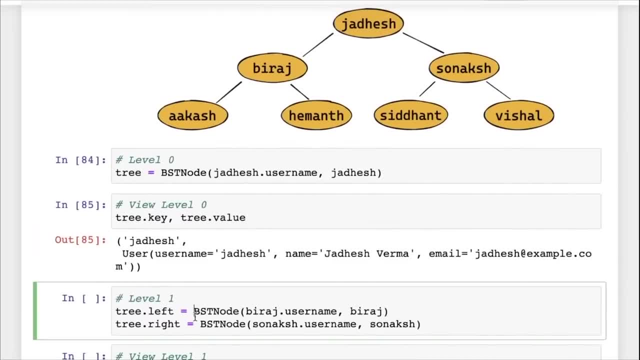 Now level one is we said tree dot left to BST node, barrage, not username and barrage. Now one other thing that we should do here is, once we set it, we should say tree dot left, dot parent to tree, And similarly we said tree dot right. 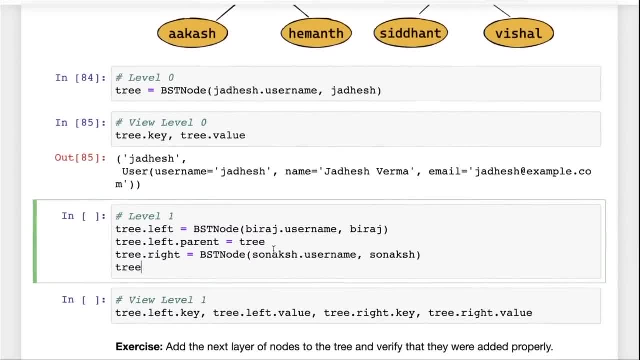 It's not tree dot Right Is Sonox. So we said BST node with Sonox dot username as the key And Sonox is the value, And then we can set tree dot right dot parent as tree. And now can you can view these values. 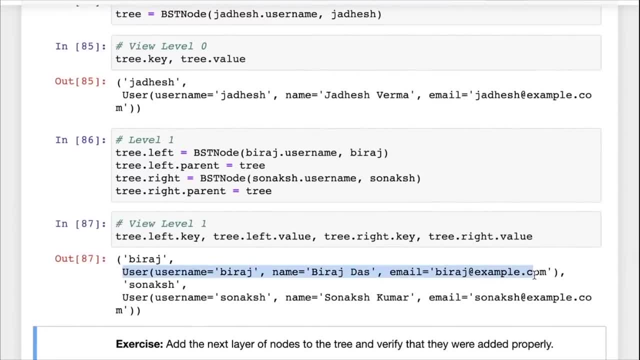 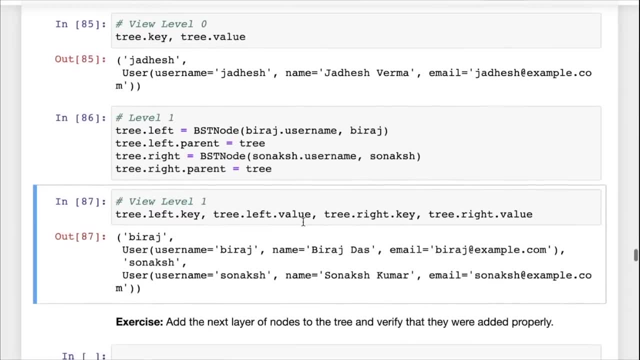 So now you can see that we've inserted barrage and the username barrage. We've inserted Sonox and the user Sonox here as keys and values respectively. Now the exercise for you to is then: try to add the next level of keys and values and then 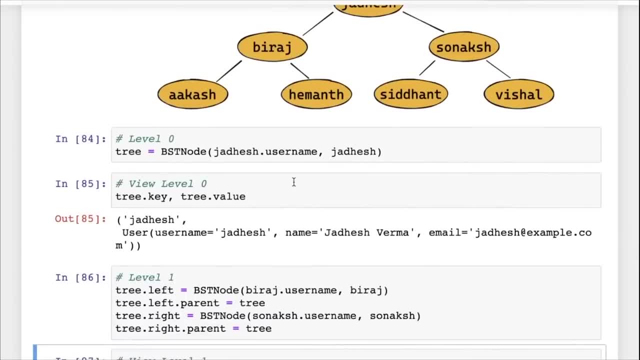 verify that they were inserted properly. but you can see now that we now have a way to represent the data- the both both the usernames and the user objects- in a binary search tree, So we're getting pretty close to the data structure that we want to create. 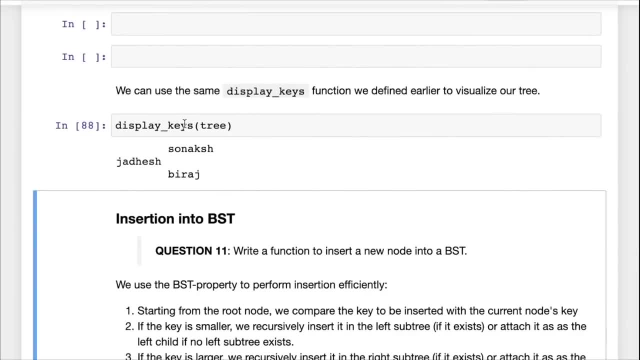 Once again, we can display the keys of the tree by calling the display keys function. Now, this is also rather nice. There's a good thing about Python that, because Python functions are dynamic, because you do not need to specify the types of the objects while defining the function- the same display keys function can be used both with. 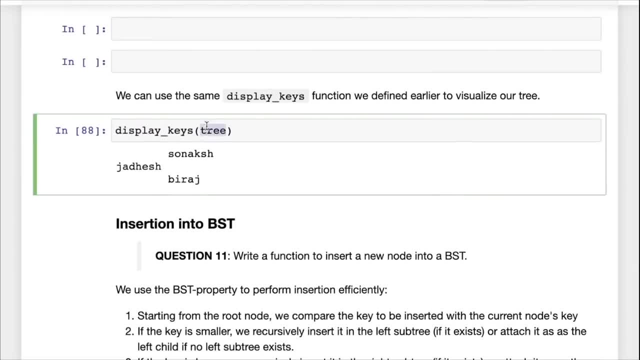 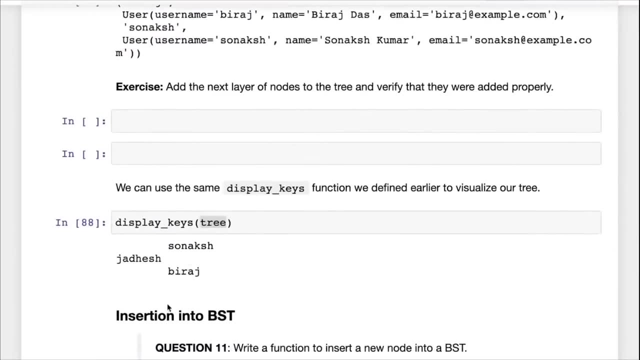 Python tree node and BST node classes. So all it requires is that the object of your class should have a property dot key for it to be able to display the keys in this visual setting, And the same is true with most of the other functions that we've defined. 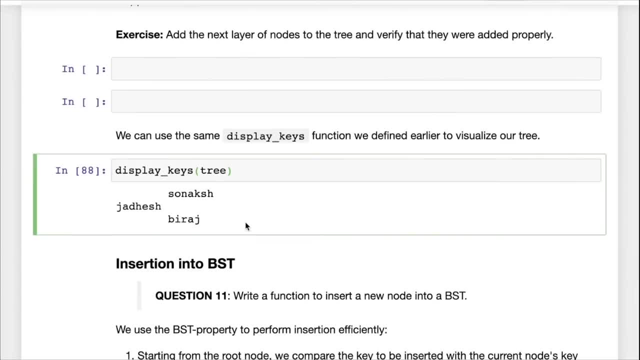 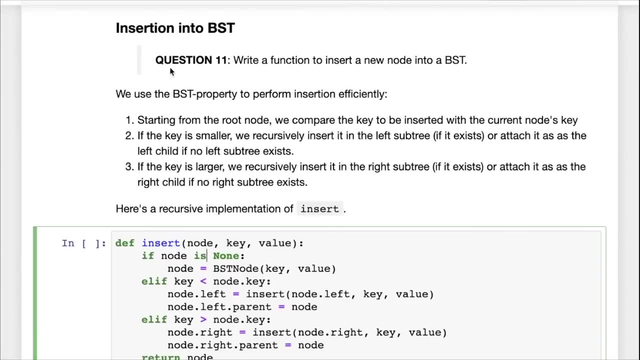 In fact, any function we've defined for tree node will also work for BST node. Okay, So, moving right along, now we have a way to construct a BST, but it It's a bit inconvenient to insert values manually, because what we're doing so far is we are manually. 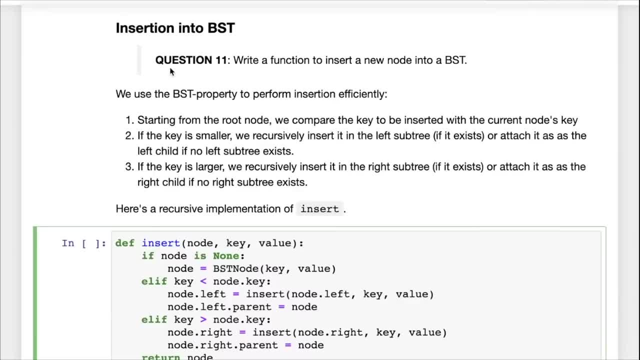 checking whether we should insert a value in the left or the right. rather, there should be a way to do it automatically. We should be able to call a function insert- And here's this is a common question as well- right- A function to insert a new node into a binary search tree. 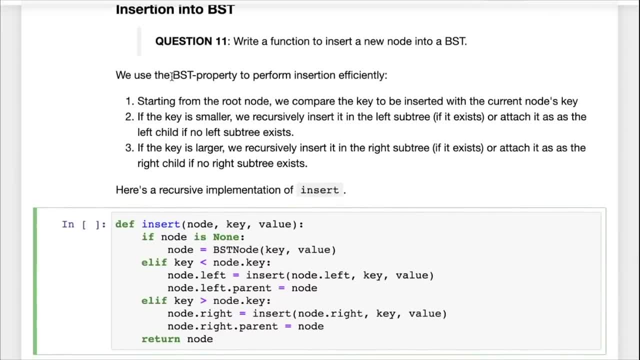 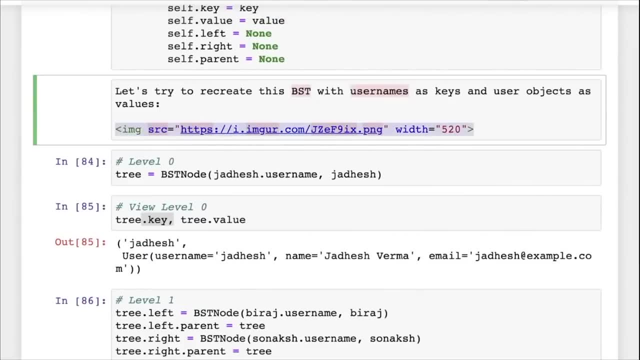 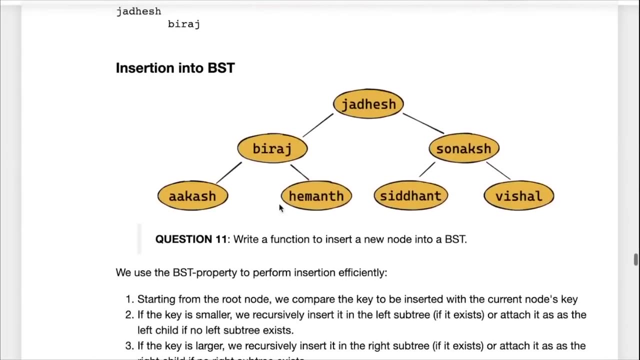 So we'll use the BST property to perform insertion efficiently. Once again, let's grab a copy of this tree here so that we can think about. I did easily, Okay. So now we have this tree and let's say we want to insert a new user with. 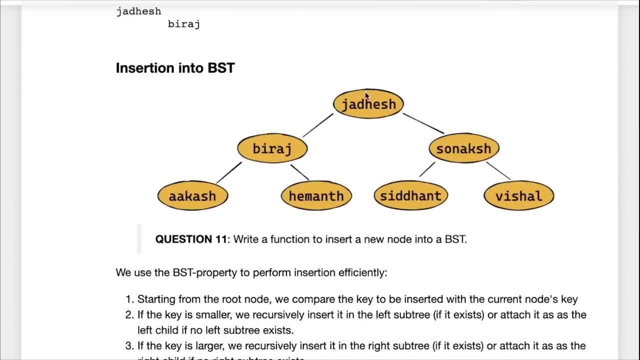 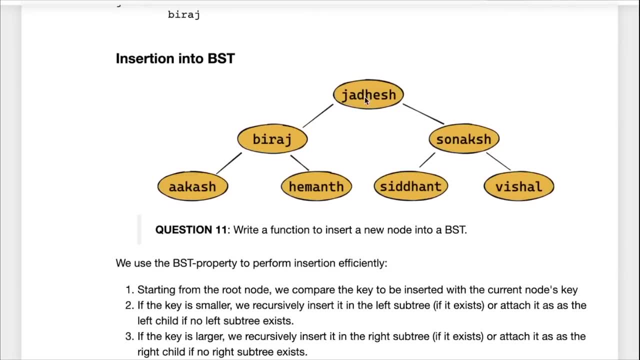 the username Tanya into this tree. So first we started the route and then we compare the key to be inserted with the current nodes- T keys. The current node is the route. So we compare Tanya with Jadesh and we see that Tanya is greater than. 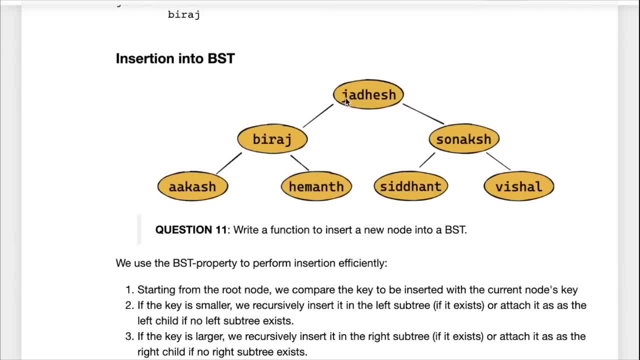 Jadesh, because T comes after J. So obviously Tanya should not be inserted into the Let Subtree. rather, Tanya should be inserted into the right subtree. So if the key is smaller, we recursively inserted into the right- left subtree. 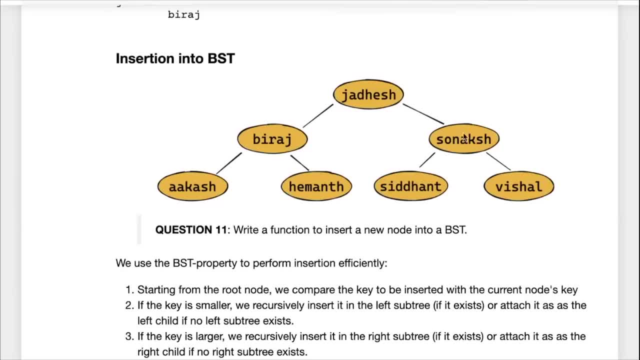 And if the key is larger, we recursively inserted into the right subtree. So then we encounter Sonox Tanya is also greater than Sonox. T is greater than ST comes after S. So once again we call, recursively call, insert on this subtree. 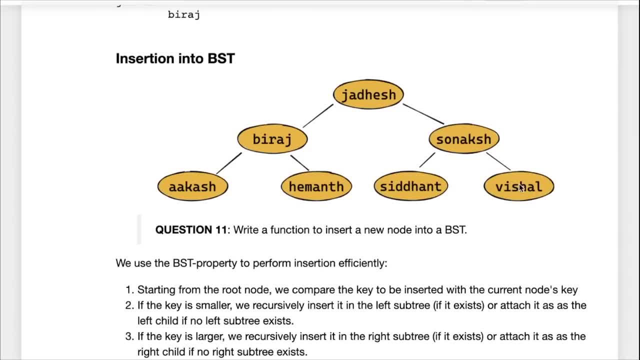 that subtree rooted at Vishal. This time we noticed that Tanya is smaller than Vishal, So T is less than V. So then We need to Recursively insert in the left subtree. but there is no left subtree here, And this is the point at which we can create a new node and attach. 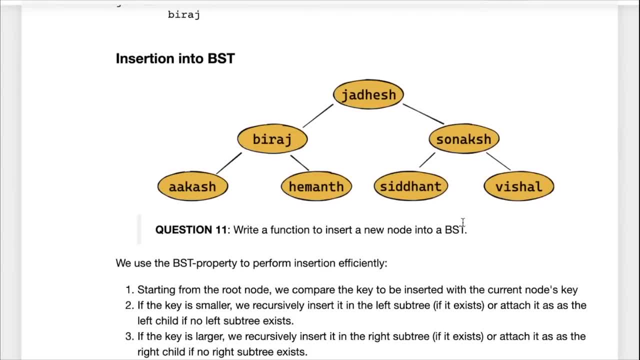 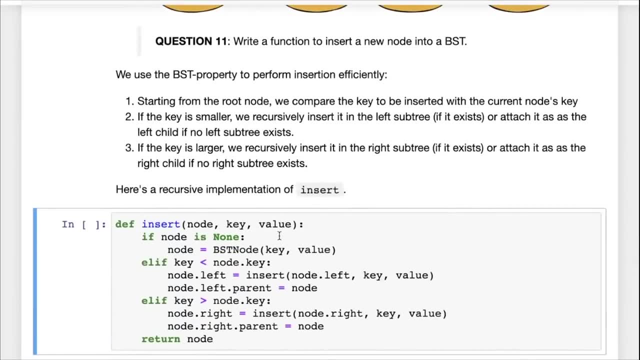 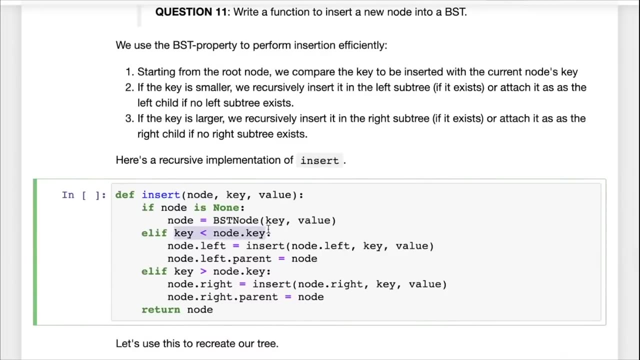 it as the left child of Vishal. So you can see that the note Tanya will get added here at this position in the tree. So here is a recursive implementation of insert, exactly what we just discussed. First we check if the key is less than the current nodes key. 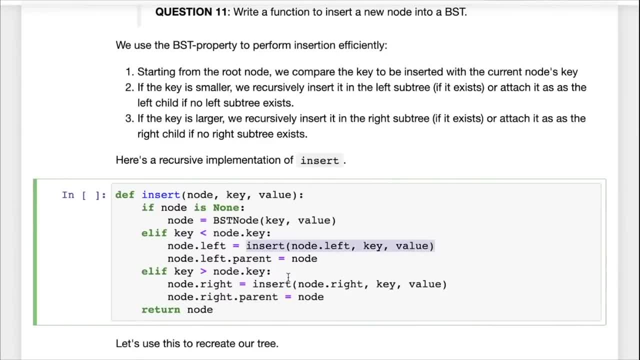 And if that is the case, then we insert it into the left subtree. Then we check if the key is greater than the current nodes key And if that is the case, we inserted into the right subtree. and the ending condition is that if the node is none, which means we've hit a position where 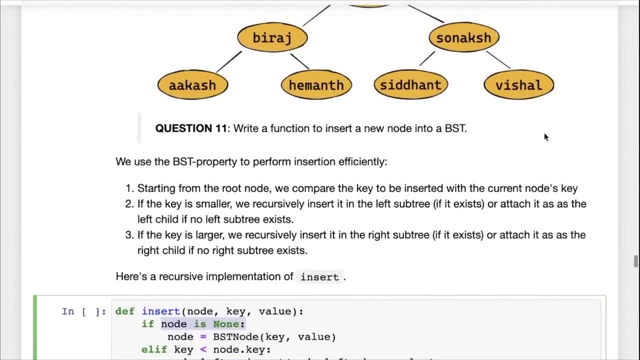 we do not have a left subtree and we need to go left, or we do not have a right subtree and we need to go right. Then we create a new node. So we create new node node equal to BST node, and then we return the node. 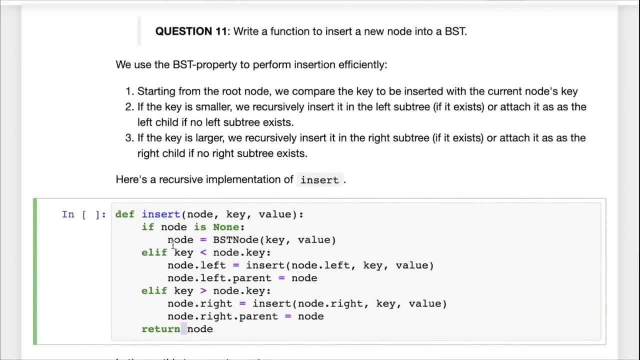 So we return the node. And this is an interesting thing that we're doing here. We are returning The root node back from insert. So when we called insert with no dot left, we get back the pointer to the left subtree So we can set it back to more dot left and we can also set the parent. 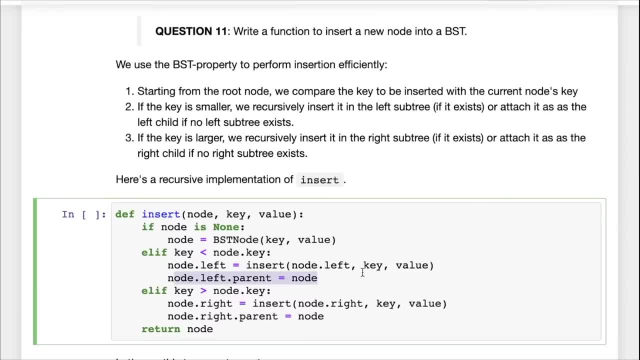 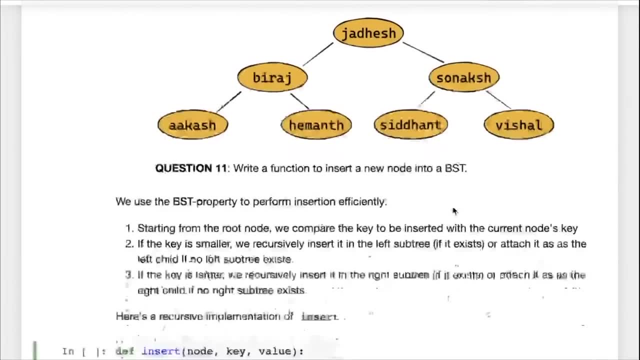 of the left subtree to node. Okay, So this is just updating the parent, So just study this function carefully and see how it works. It does exactly what we just talked about and it finally returns a pointer to the to the tree once again. 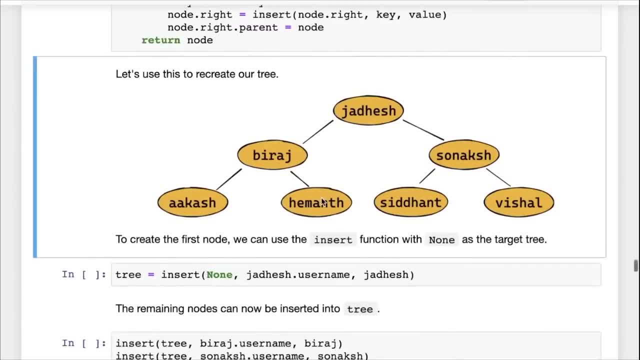 So let's use this to recreate the tree that we had here. Now to create the first node, we can call the insert function with none. So initially we don't have a tree to begin with, So we just called insert with none. And remember that insert after performing an insertion returns the pointer to the tree. 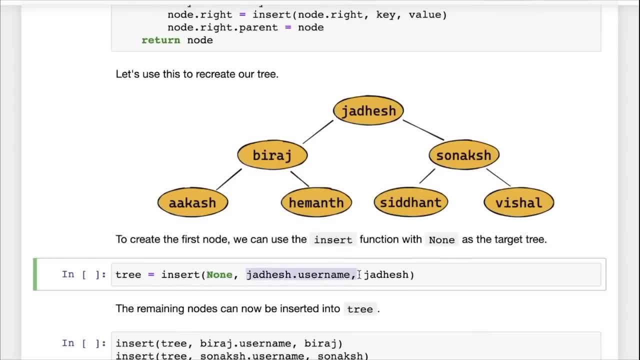 So we call insert with none and we want to insert the value Jadesh dot username And we want to insert the. we want to insert the key Jadesh short username with the value Jadesh. So that gives us The tree. and now the tree has one element. 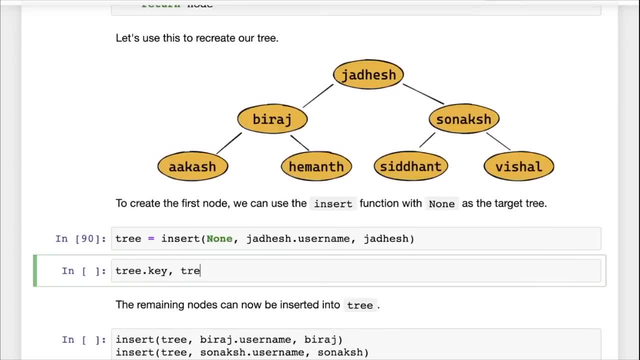 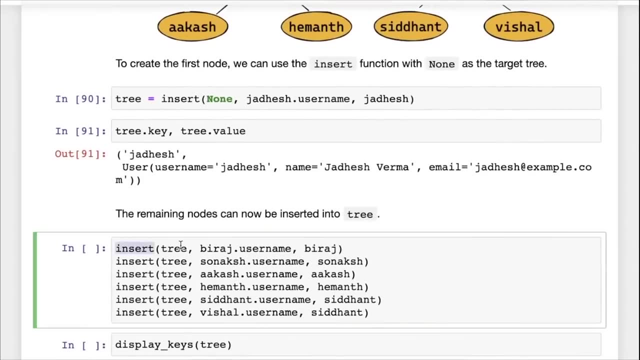 You can see tree dot key and tree dot value. And now the remaining nodes can just be inserted into trees. So now we call insert with tree and call it with barrage, dot username and barrage. Then we call it with Sonar, start username and Sonar should username and Akash, and this way: 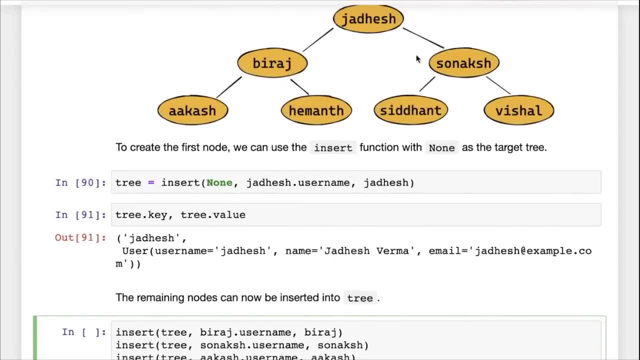 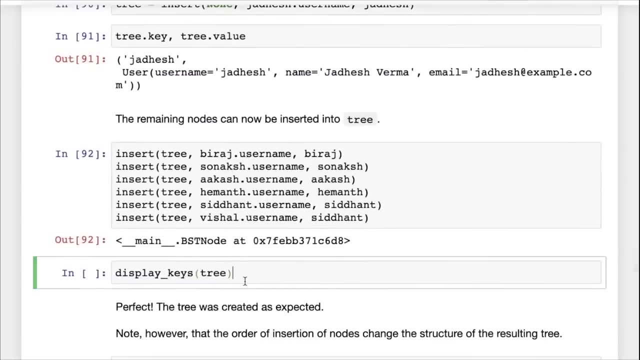 So we're adding barrage, Then we're adding Sonar, Then we're adding Akash, Hey man, So don't wish all And see that we are not specifying exactly where these nodes need to be inserted. Uh, but you can see that once these nodes are inserted, then they are inserted in the right places. 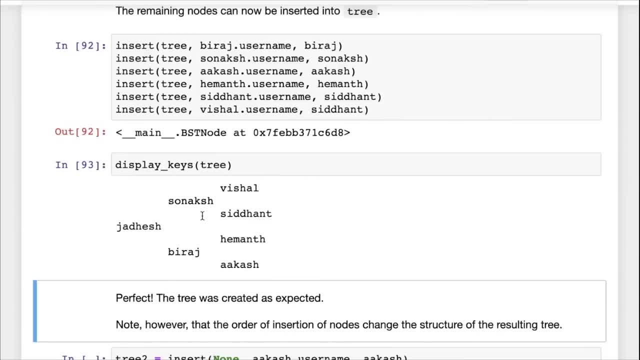 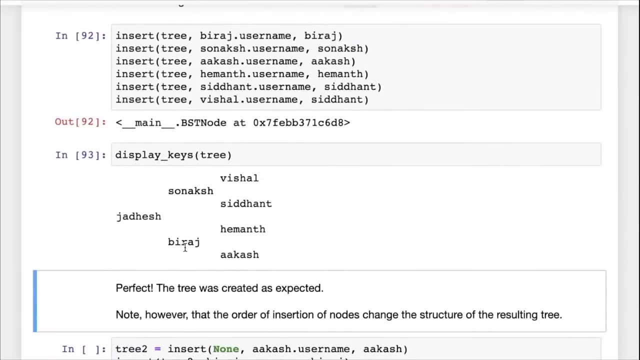 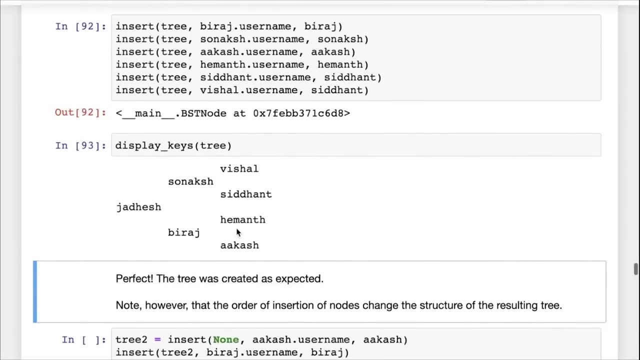 So Jadesh, you can see that the binary search tree properties preserved here And also we've exactly replicated the tree structure that we had here. So the left subchild of Jadesh is barrage and the right child is Sonar, for barrage, The left child is Akash and the right child is human, and so on. 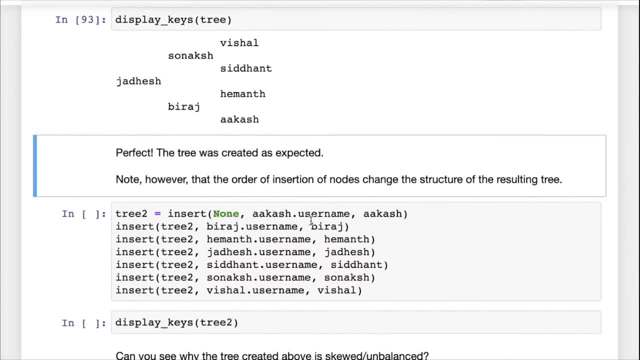 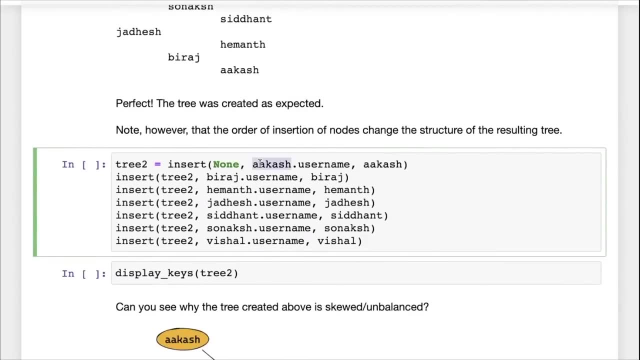 Now note, However, that the order of insertion of nodes can change the structure of the resulting tree. So, for instance, if we insert all the nodes in the increasing order of username. So for example, here we are inserting Akash Paraj, Heman, Jadesh, Siddhant, Sonak Vishal. 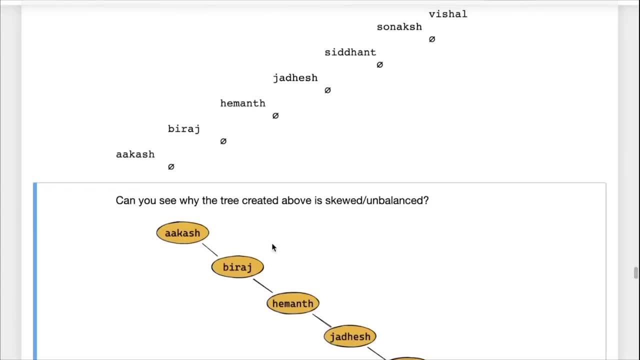 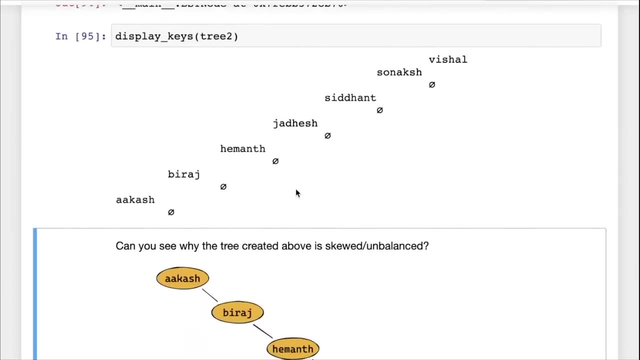 So this is the lexicographic increasing order And we try to display that tree. This is what we end up with. So we end up with an unbalanced or a very skewed tree, and you can see why it was created as a skewed or unbalanced tree. 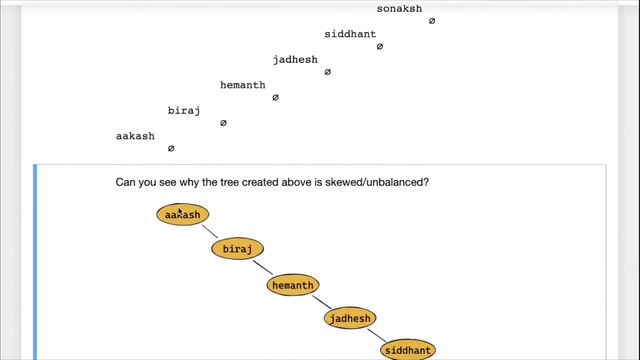 Well, let's look at it So: we started with Akash, So we have a single node, and then, when we try to insert barrage, we realize that we need to go right, So we insert barrage here, then we try to insert Heman. 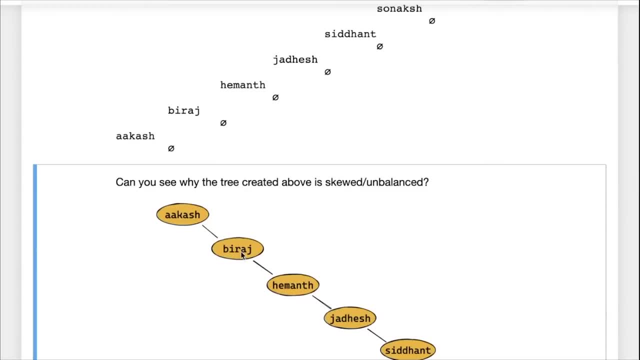 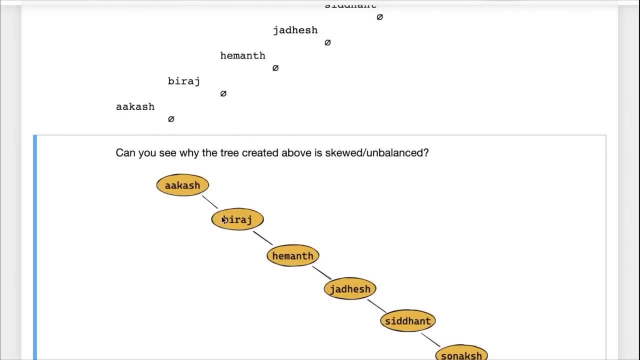 Then we realize that we need to go right from Akash and right from barrage and go to Heman, And then we keep going this way. So how you set up the root node and how you set up each subtree and the order in which you insert the nodes is very important. 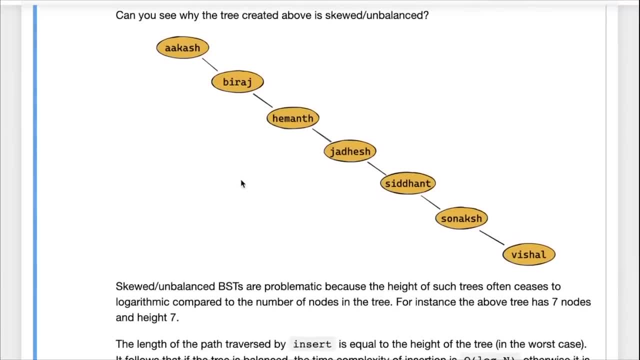 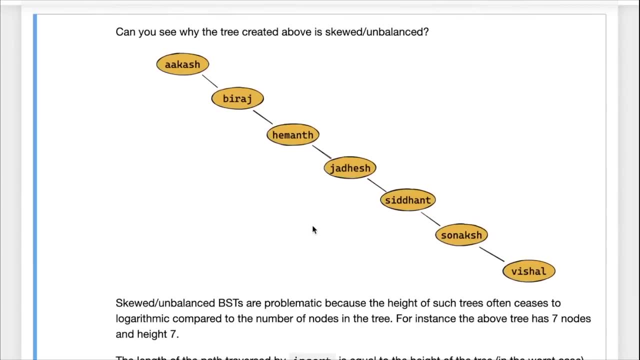 And that can create a huge skew within the tree. now skewed or unbalanced trees are problematic because the Height of such such trees is no longer logarithmic compared to the number of nodes in the tree right. So earlier we had deduced that in a balanced tree, if containing N nodes, the height is log N or log N plus one. 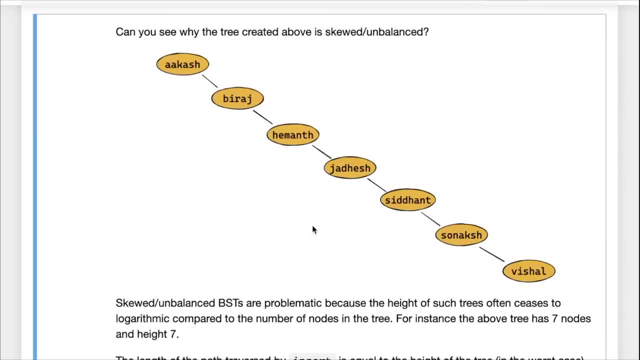 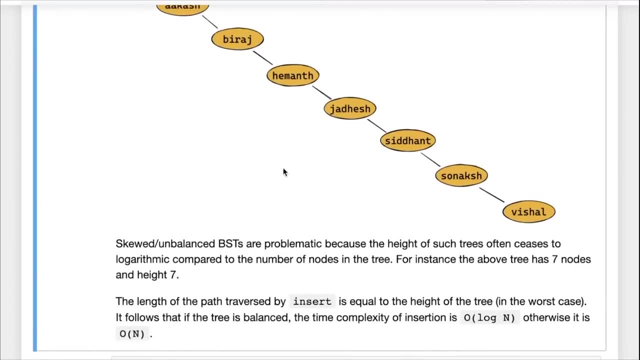 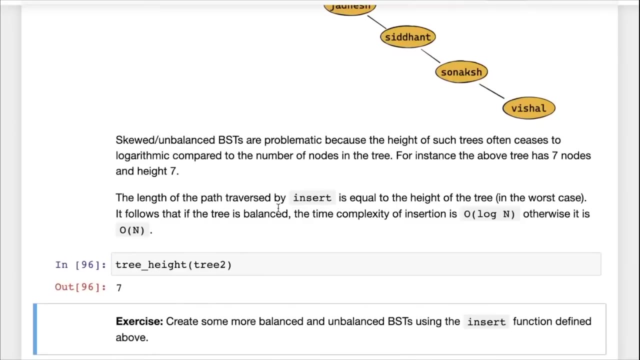 And that makes the operations like insert, update and find very efficient. But here, where you have a very skewed tree, the height can actually match the number of nodes. For instance, this tree has seven nodes and it has the height seven. And in these skewed trees, once again, you may get back the fact that insertion, finding and update can be ordered in, because you may have to traverse the entire height of the tree, which is equal to the number of nodes of the tree. 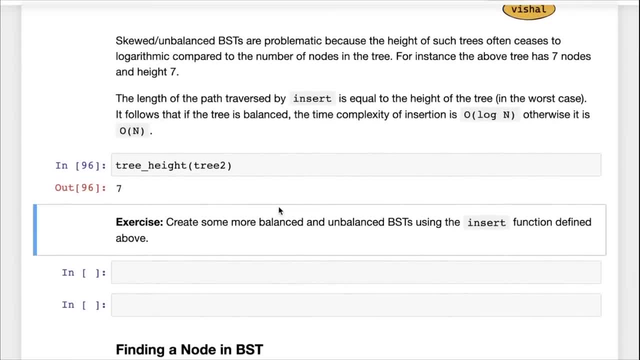 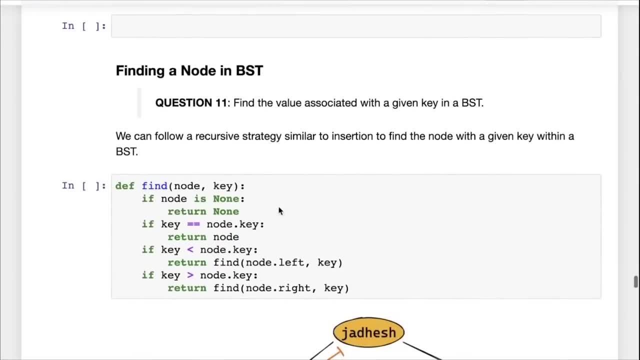 And that may once again defeat the purpose of using a binary search tree in the first place. So maintaining the balance of a binary search tree is very important and we'll see how to do that. So we've seen how to insert a node. 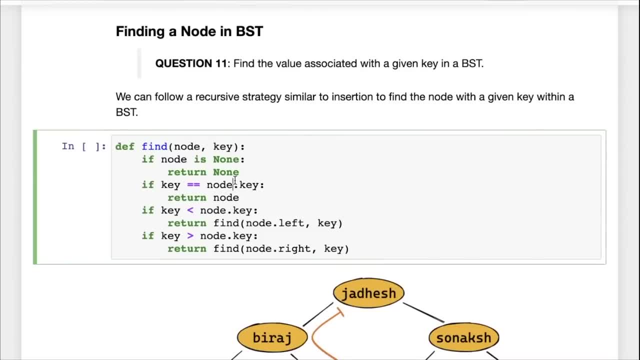 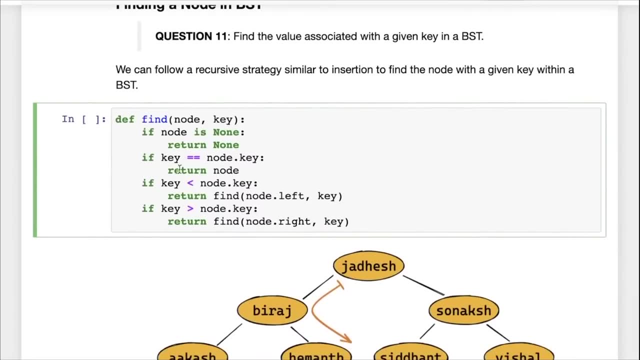 Now the next thing is to find the value associated with a given key in a binary search tree. So once again we can follow a recursive strategy here, similar to insertion. So we check, we start from the top. Let's say we want to find the key. 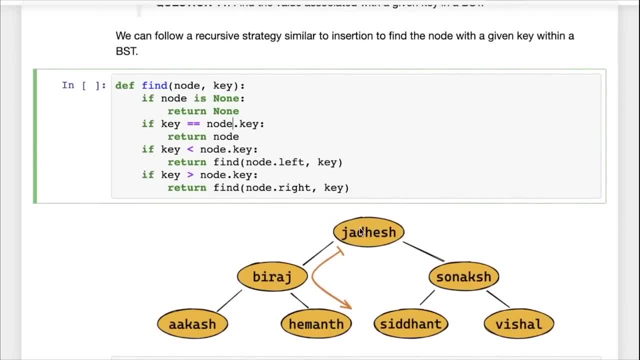 Hey man, we start from the top and we compare it with the root node. Now here, if it matches the root node, we can simply return this node. If it does not, then we check whether we need to go left or right. 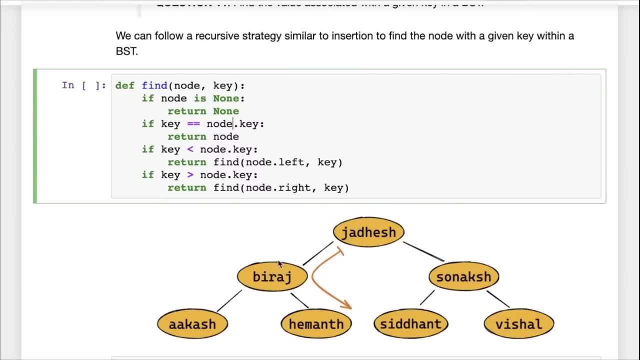 Since he month comes before Jadesh, we need to go left. Then we encounter a barrage and here we realize that we need to go right And finally we encounter him and we return. Another option is that we have a value- Let's sit Tanya- which does not exist here. 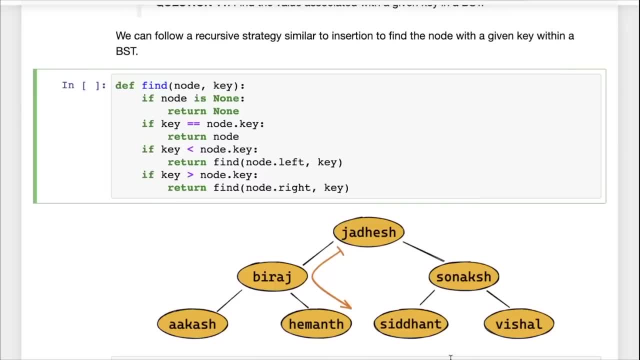 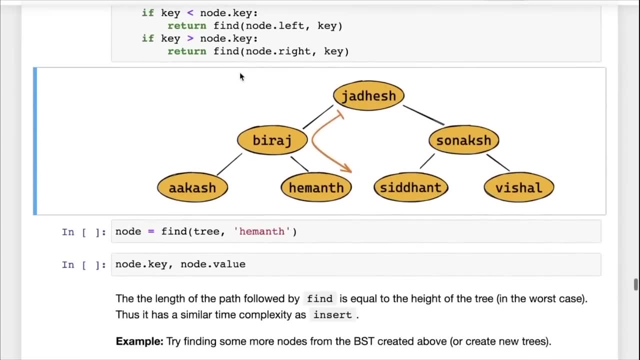 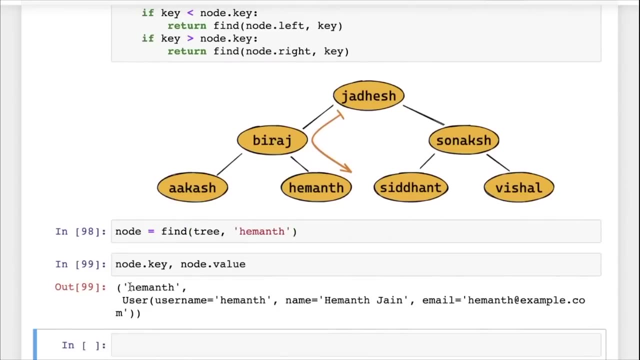 So if we try to search that we may go in this kind of a direction and we end up at an empty place. So in that case we simply return none. So you either find a node and return it or you return none. So you can see here that if we call it fine tree with him and we get back the details for him and 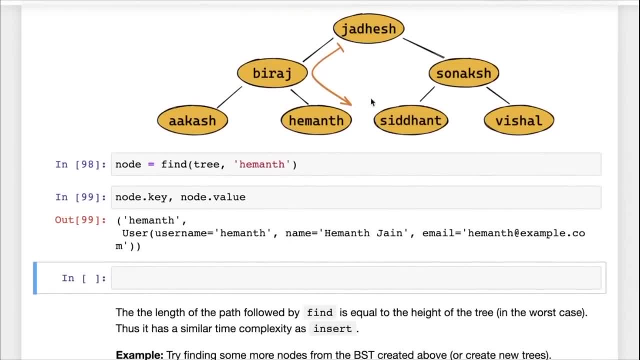 we get the value And, very interestingly, because there's a balance tree, we only had to take two steps and not go through the entire tree And in the worst case, you can check that any path from the route to any leaf in a balanced tree will only be two steps long. 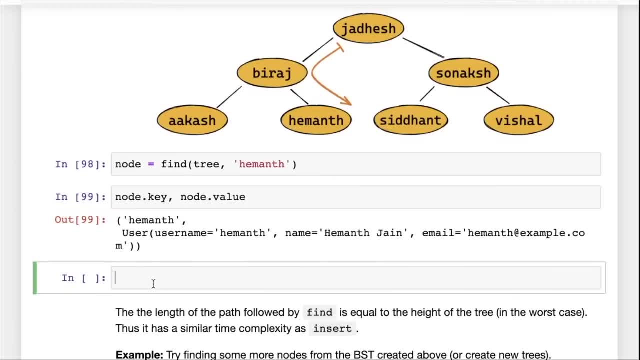 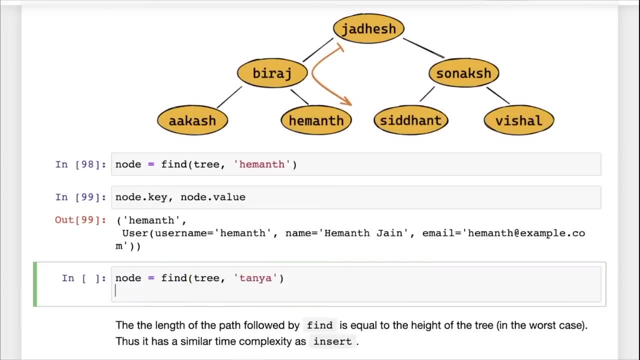 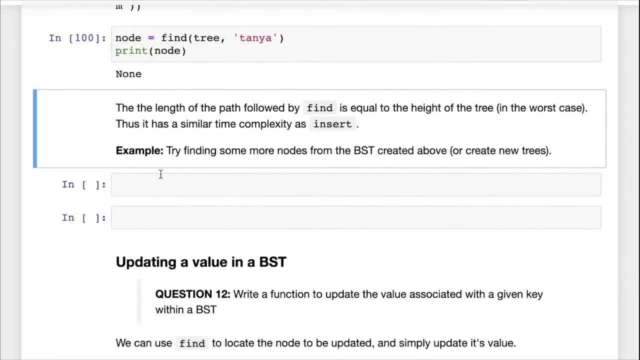 And that's what makes it so convenient. Now, on the other hand, if we try to find the key Tanya, You can see that it's not far to try creating larger BSTs and try finding some more nodes. It's important to experiment with these operations once they're defined, because now it's simply a matter of calling the function. 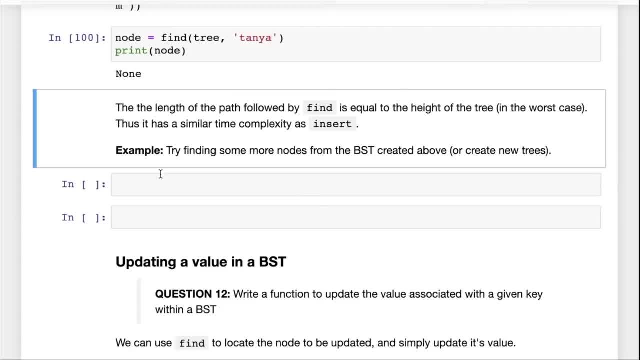 We've written the code for it, So experiment with it. try creating larger trees with multiple levels and dozens of, maybe hundreds, of nodes. Try generating some fake data, putting it into the trees and see how trees build up, And that'll give you a feel for how binary search trees. 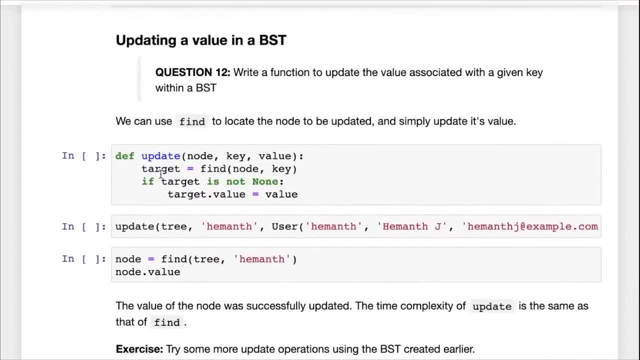 Work. next, Let's talk about updating a value in a BST. Now, updating a value is fairly simple. We already have a way of finding a node. So if you want to update a node, let's say we want to update the node Hema, the key, Hemanth. 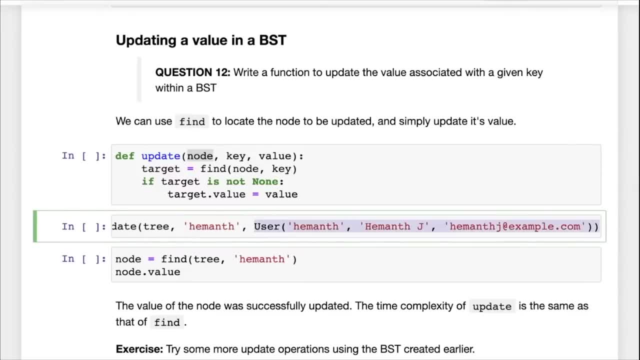 And here we want to update it. We want to update it to this value, which is the new value of the user Hemanth, and we're changing the name and we're changing the email here. So we first find the node And if the node is not none, then we simply change the value at that node. 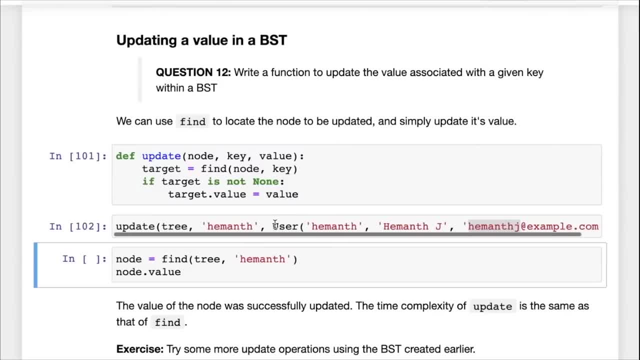 It's as simple as that And we, what we're also seeing is we are reusing the fine function here and this is a good practice to always incorporate into your programs, into your functions. Whenever you find yourself copy pasting some code and maybe changing one or two things here and there, think about whether you can extract that piece of code into a function and then reuse that function. 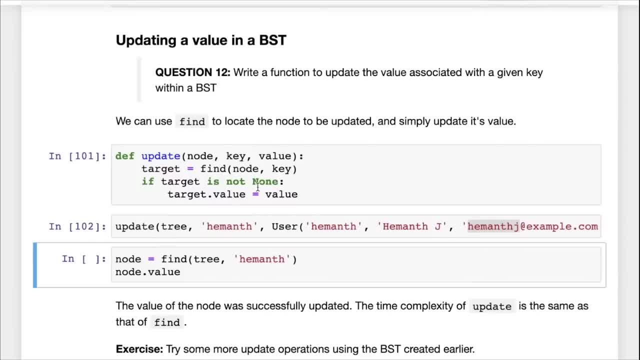 So always try to make your code more and more generic. The less code you write, the less there are the chances for errors, the easier it is to understand and the smaller your functions become. So write small, reusable, generic functions whenever you can. 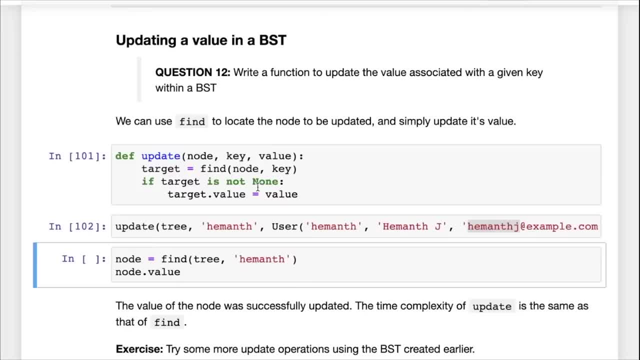 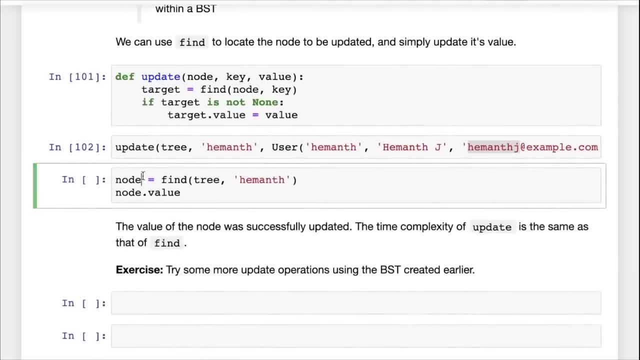 And this is a principle called the DRY principle, or the DRY principle, which stands for: don't repeat yourself whenever you're writing programs, So in update, we're not repeating ourselves by using the find function to find the right node and simply updating it by setting its value. 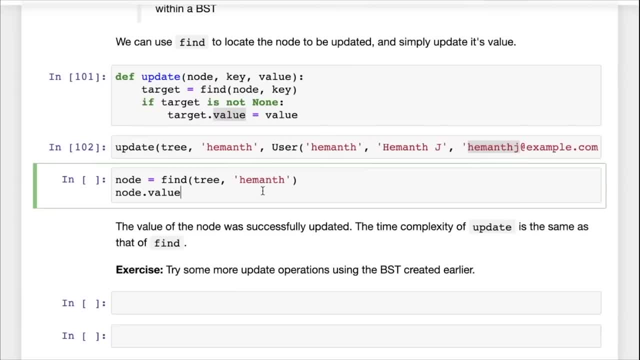 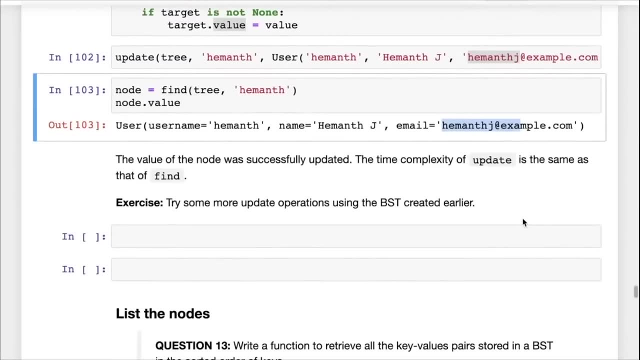 So let's update a month here to the new value and you can see that now we have the updated data here. So we have payment J and human J at examplecom. Now the value of the node was successfully updated and you can edit and you can easily check that. the time complexity of update is same as that of fine. 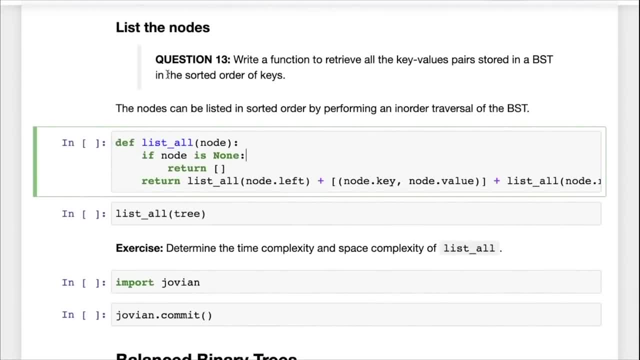 Now, finally, we have the last operation that was required, And this was to write a function to retrieve all the key value pairs stored in a binary search tree in the sorted order of keys. This is a question that you might face once again, and this is simply the inorder traversal. 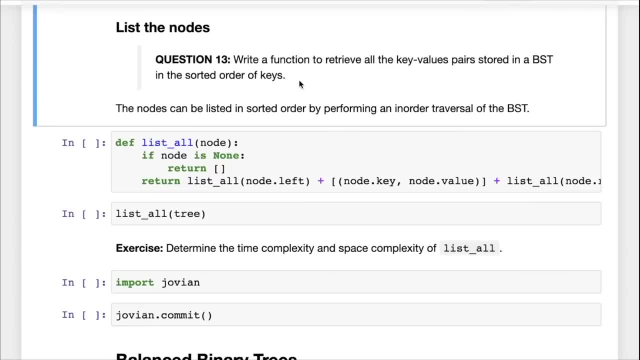 It's a different way of stating the inorder traversal. Now, what you will have to figure out or reason about is why the inorder traversal of a binary search tree produces a sorted array of our- Sorry, Sorted- list of keys. Think about it. 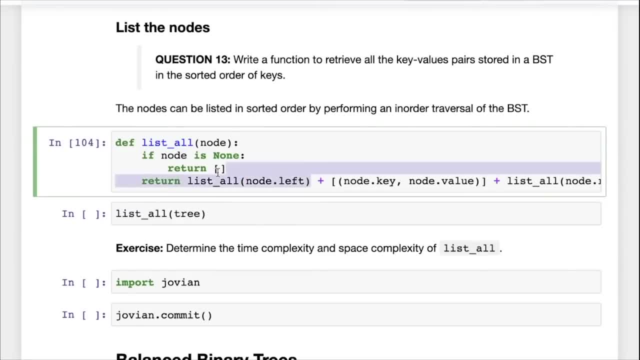 So here's the list all function. All we do here is we call list all on node dot left and then we call list all on node dot right And in between them these give us two areas. So we assume that list all dot, node dot left gives us the list of key value pairs from the left subtree, in sorted order. 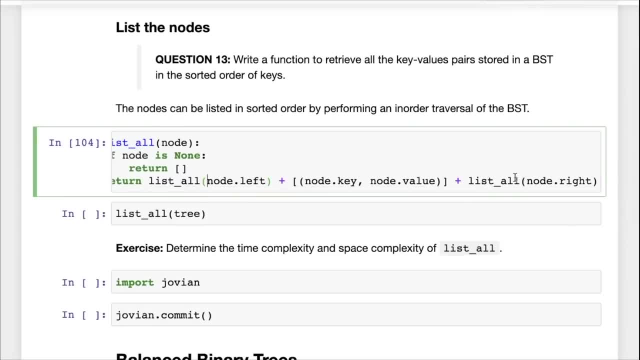 Similarly, here we get the list of key value pairs from the right subtree in sorted order And between them we simply insert This key value pair from the current node and recursively it automatically fills out the entire array. And this is the end condition where we encounter an empty node. 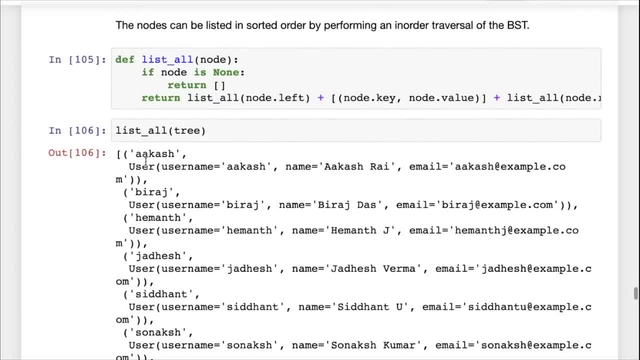 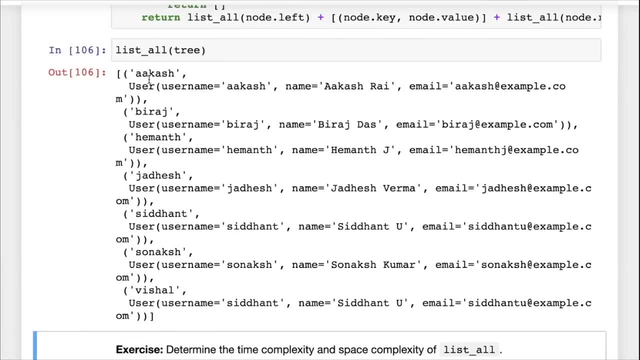 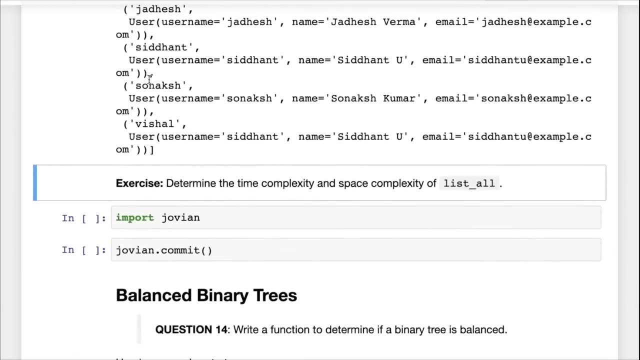 We simply return the empty array. You can see now, when we pass in this tree, we get back the list of users, key value pairs arranged by the sorted order of keys. Now here's an exercise for you: Determine the time, complexity and state. 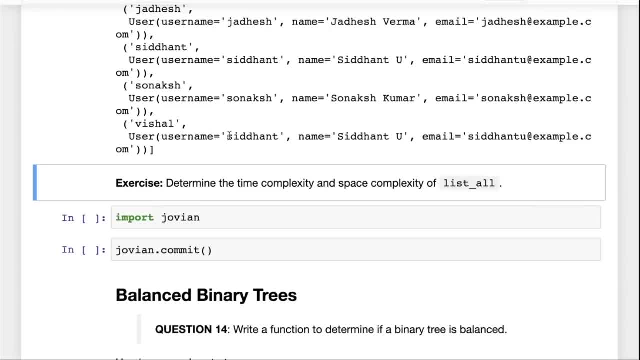 Complete a state, space, complexity of the list, all function. Now you can do this for a balanced tree or an unbalanced tree, and here's a hint: It will not make a difference, but think about it. So, once again, let's save our work. 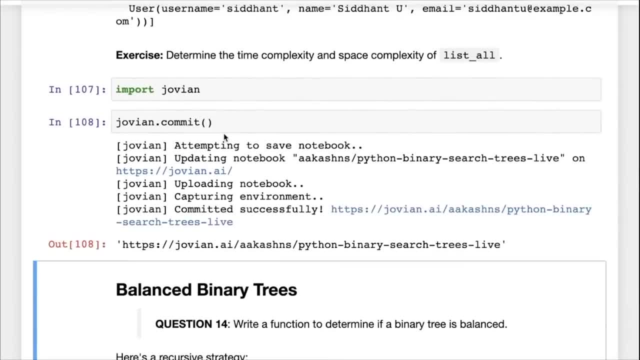 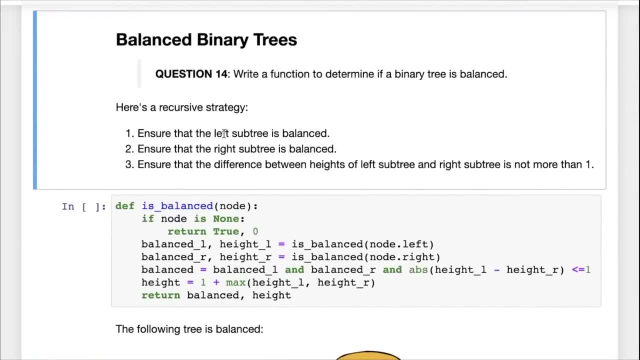 And now we've talked about binary trees and operations on binary trees. Now the next thing is to look at balanced binary trees, And this is once again a very common question that gets asked. write a function to determine if a binary tree is balanced. 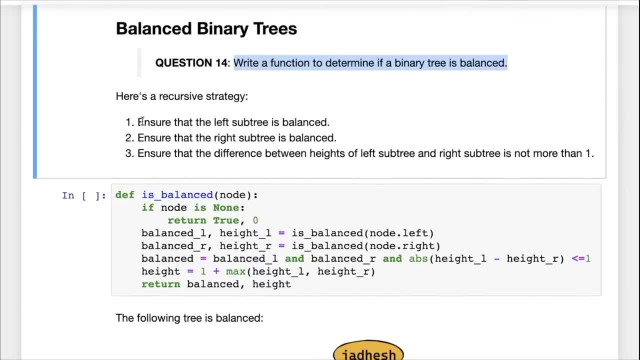 And here's a recursive strategy to do this. In fact, this is really the definition of balanced binary trees: The left subtree should be balanced, The right subtree should be balanced and the difference between the heights of the left and right subtree should not be more than one. 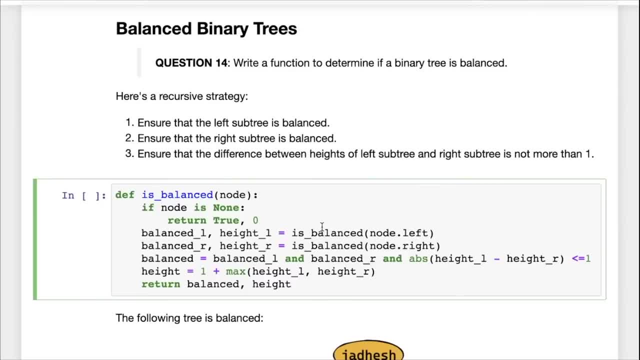 Okay, So this is an important thing. Now, when we're looking for balance, we're not always looking for perfect balance, Because it may not always be possible to create a tree with perfect balance. because to have a perfectly balanced tree, where, for every node, the left subtree and the right subtree of the exact same height, you will have to fill out all the nodes at all the levels. 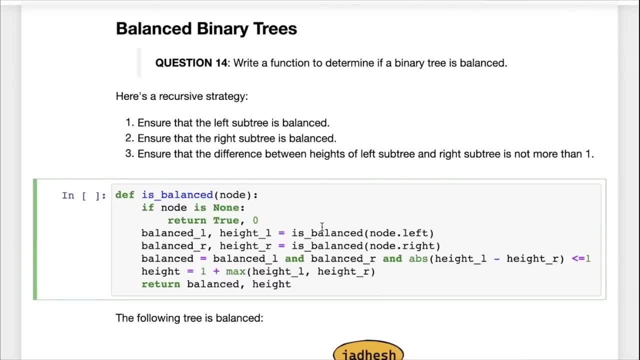 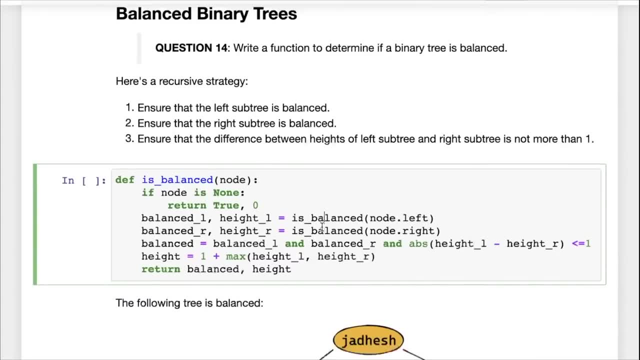 And that can only have. that can only happen for certain numbers. For example, you can have one node, which satisfied this property, or you can have a tree with three nodes which satisfy this property, or you can have a tree with seven nodes which satisfies this property. 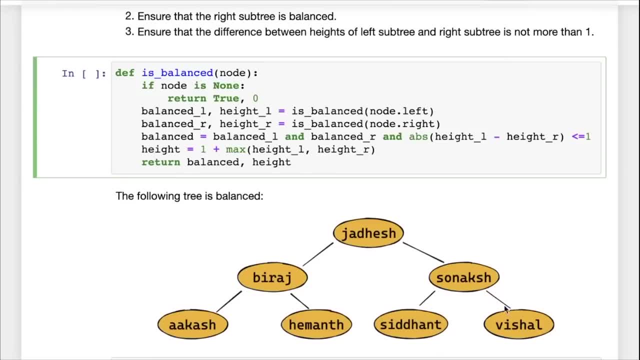 But Yeah, You may not be able to get a tree with six nodes to satisfy that property. For instance, if you remove Vishal here, you will see that the left subtree and right subtree of this node, Sonaksh, will not be of equal height. 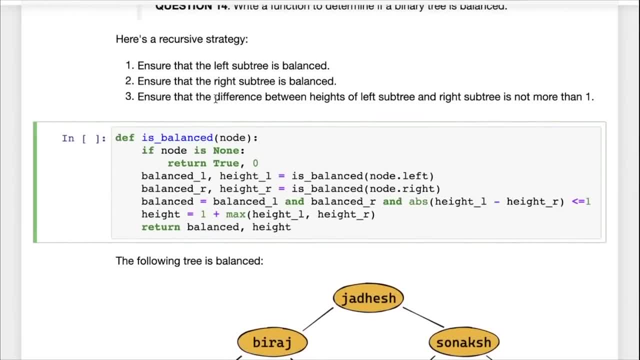 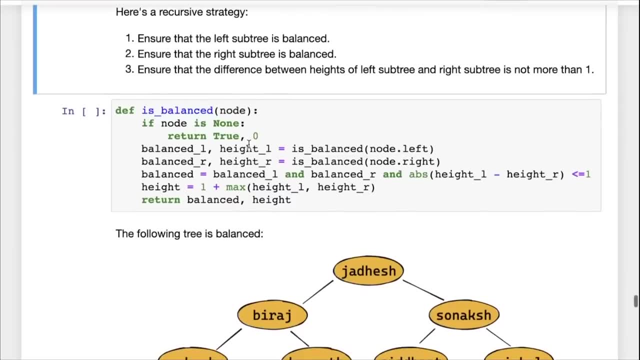 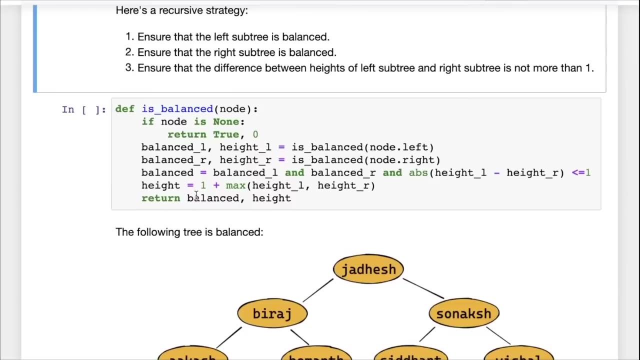 That's why, for balancing, we relax the criteria slightly. We simply need to ensure that the difference between the heights of the left and the right subtree is not more than one. So here's the code for is balanced. once again pretty straightforward. but we will return two things here. 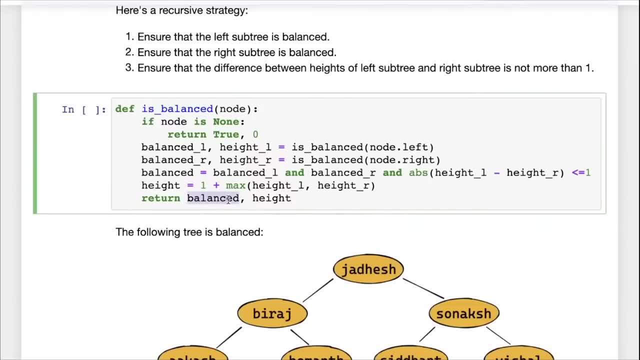 We will. This is balanced will not only return whether the tree, a node is balanced, It will also return the height of the tree which is rooted at that node. So the way we implement it is: first calling is balanced on node dot left and then calling is balanced on node dot right. 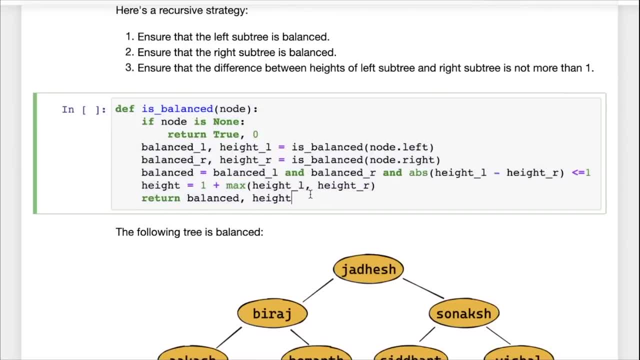 And, by the way, this is exactly how we implement a recursive functions as well. Sometimes we write the recursive functions signature, then we immediately write the return value and then we assume That a recursive call is going to return these values. So a recursive call is balanced. 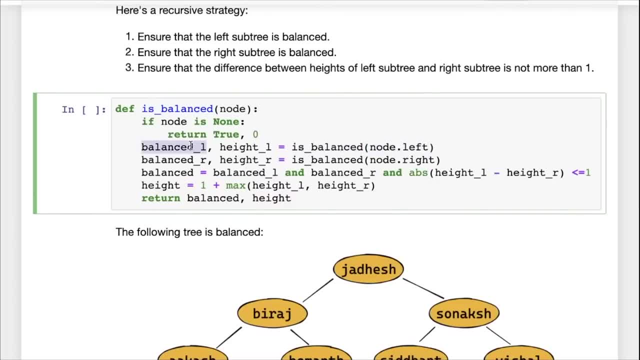 No dot left is going to return whether the left subtree was balanced and the height of the left subtree, And then we assume that is balanced, for no dot right is going to recall- uh is going to return whether the right subtree is balanced and the height of the right subtree, because that's what we return here. 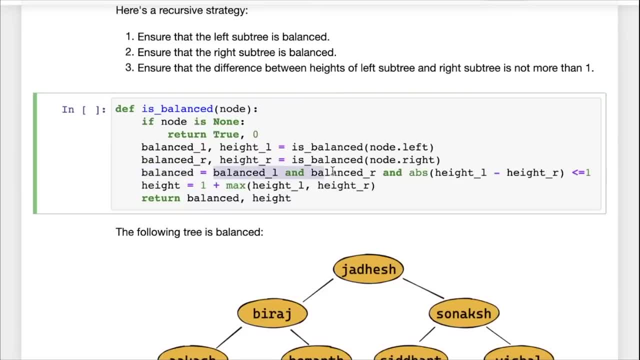 Then the entire tree is balanced. If the left subtree is balanced and the right subtree is balanced and the absolute value of the differences in their height Is less than one, which means the height L minus site R is either minus one zero or one. 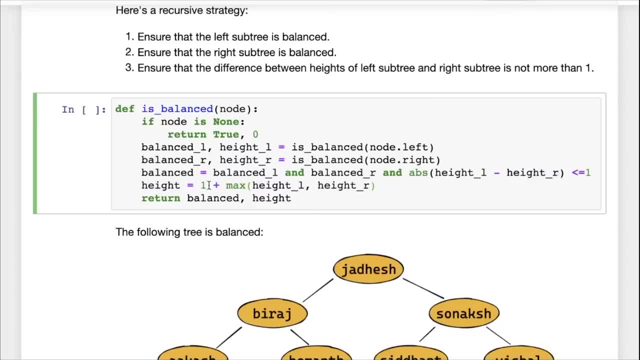 And, finally, we calculate the height of the tree itself, which is simply one plus the maximum of the height of the left subtree and the right subtree, And we return it. So that's how you implement a recursive function, or think recursively. And there's one last thing, which is the end condition, and the end condition. 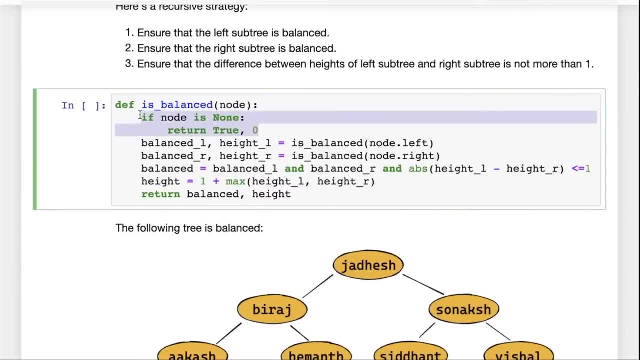 Although it's often the last thing you think about, it's the first thing that you have to put in the end condition is to check whether a node is none, Because, as we call node dot left, You may not have a left subtree, So you may call is balanced with none. 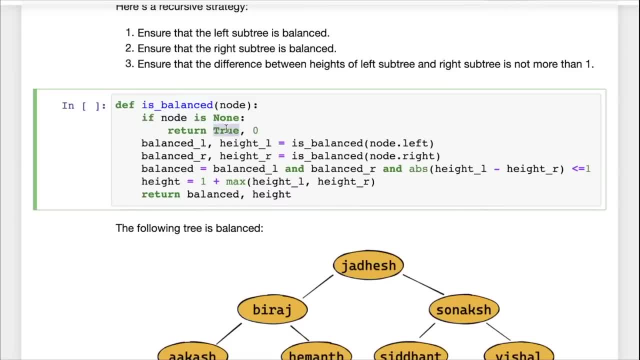 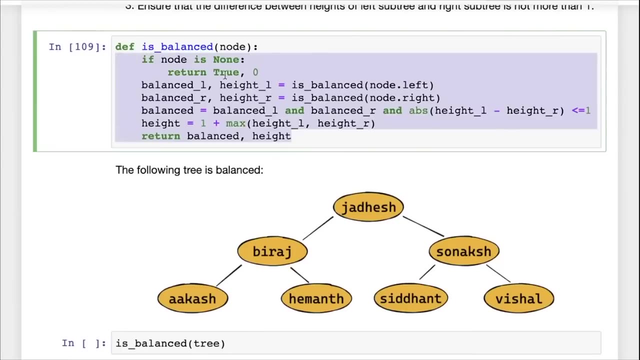 And if the node is none, we simply return true, because an empty tree is balanced by default because there's no imbalance there and it's height is zero. So that's our is balanced function. It's just four or five lines of code, But if you are not able to reason about recursion easily, you may get stuck with this and you may spend an entire 45 minutes trying to write this function. 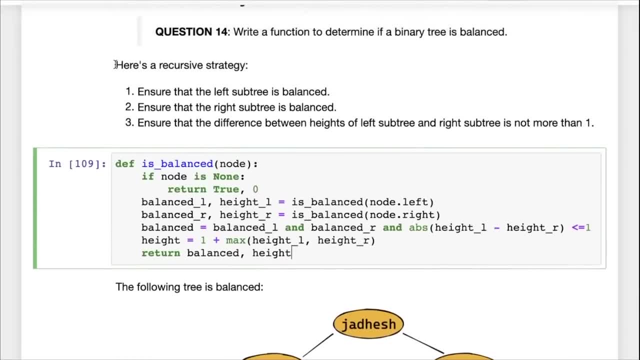 And debug it. So always try to think in recursive terms, And that's why always, it always helps to write down what you want to do in plain English so that you can determine what should be the inputs and outputs to your function. Maybe also have some test cases ready and then start implementing your function and it becomes really easy. 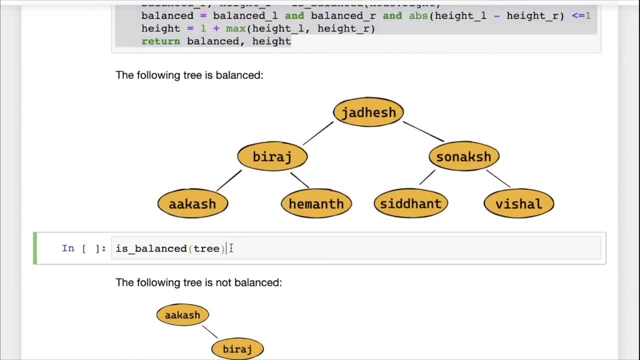 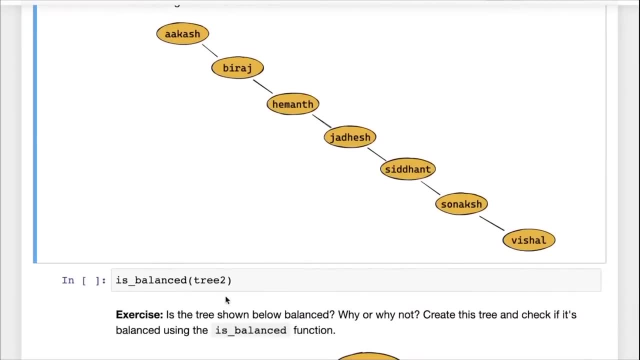 So this tree, for instance, is balanced- here You can check is balanced, You get back through. but this tree here you're looking at this is not balanced. So this Was three too, And if we check is balanced here, you get back false. 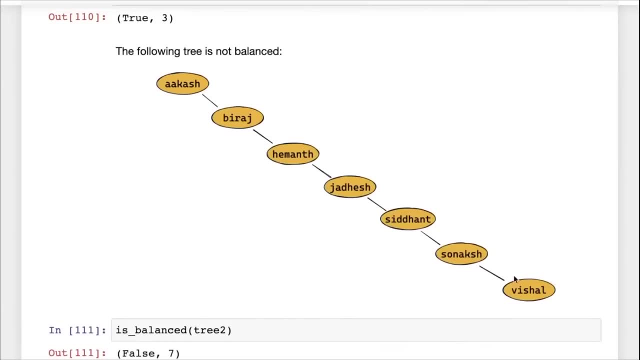 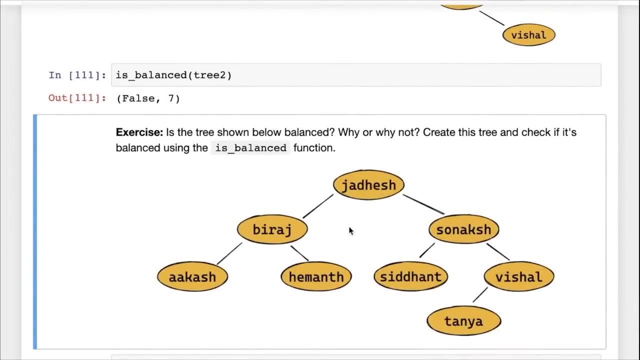 So here you also get the height of the tree, which is three, And here you can get the height of the tree, which is seven. But here's another tree. is this tree, is this tree shown here, balanced? Why, or why not now create this tree and check if it's balanced, using the is balanced function? 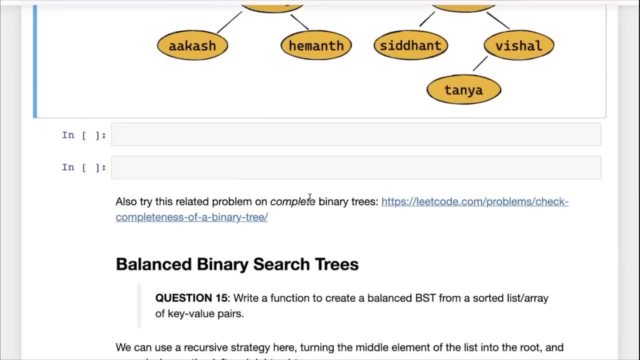 So there's another concept called complete binary trees which is slightly similar to balanced binary trees, but it's a slightly stricter criteria. So you can check out this problem here and you simply need to modify the is balanced. The code for is balanced slightly to get the code for complete binary tree. 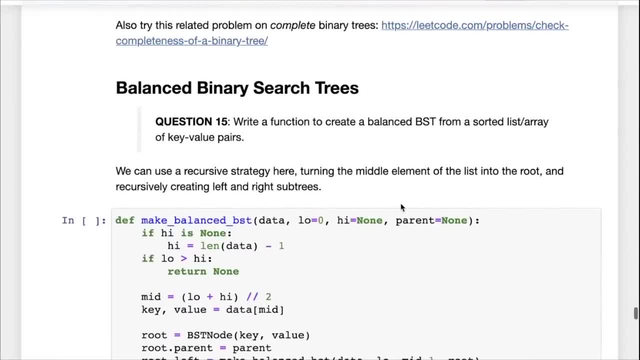 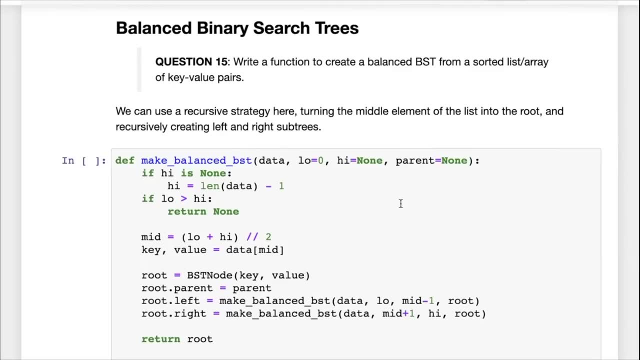 So do check out this problem on leetcodecom. All right, So we've looked at binary search trees and we've looked at balanced binary trees. Now let's bring them both together into balanced Binary search trees. And here's one question that you will face at some point: write a function to create a balanced binary search tree from a sorted list of key value pairs. 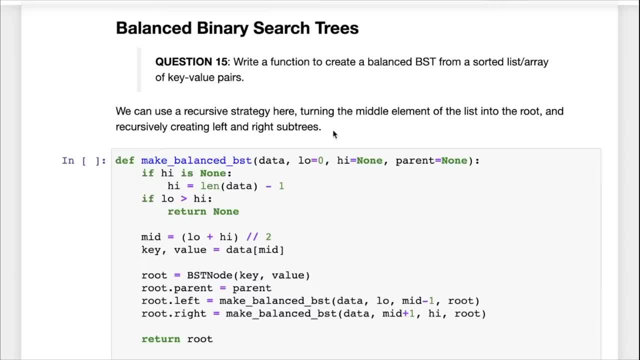 So you have a sorted list of key value pairs. So the key is, for example, could be usernames, The values could be the user objects, and they are sorted by key. and you have a list and you have to create a balanced binary search tree from it. 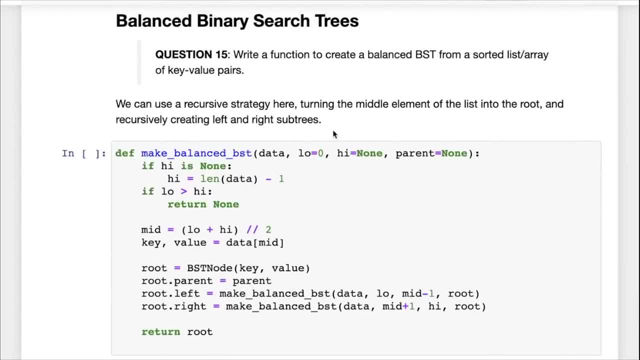 And here's the basic logic, which is somewhat Similar to binary search, which is something that we've covered in lesson one. do check it out. What we can do is we look at the middle element. for instance, if you have a list of 15 elements, then the element at position seven, counting from zero, the element at position seven is the middle element. 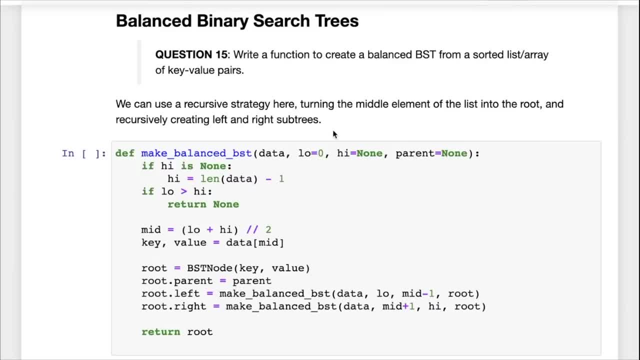 Now we can take the middle element and then create a new binary search tree with the middle element as the root node. Okay, So you take, You make the middle element the root node, and then you take the left half of the list and use that to create a balanced BST and make it the left child of the middle element, the root node. 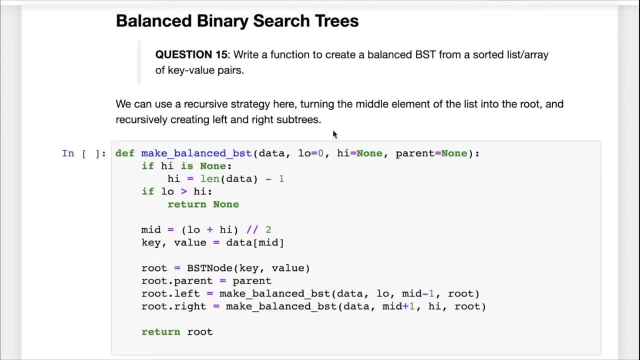 And then you take the right half, which both of the house will have seven elements each. So you take the right half and you create a balanced BST out of it and then make it the right child of the middle element. So that's the idea here. 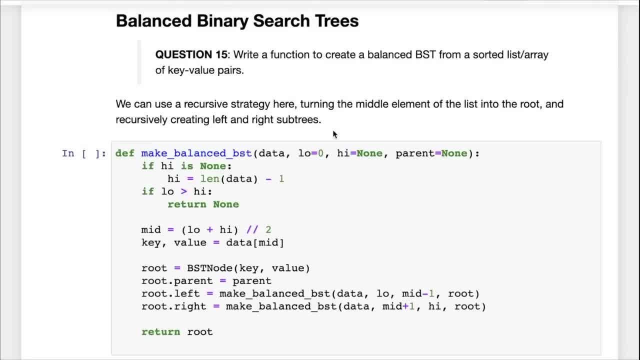 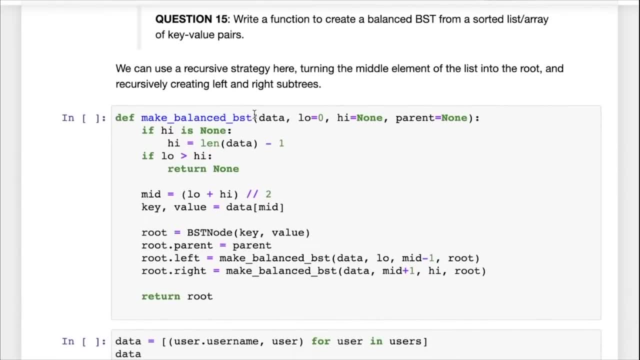 And how do you make a balanced BST for the left or right child, recursion right. So once again, here's a recursive solution: make balanced BST. takes data, which is a list of key value pairs. It takes a low and a high and it also takes a parent. 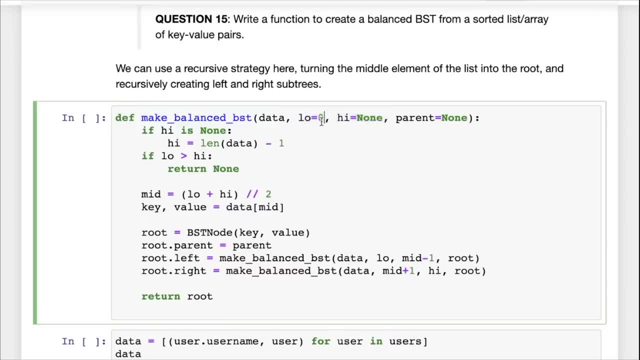 And we look at those now. low is set to zero by default and high by default is set to the last index in the data. So we use that to get the middle index. So, for instance, if low is zero And highest 14, the middle index is seven. 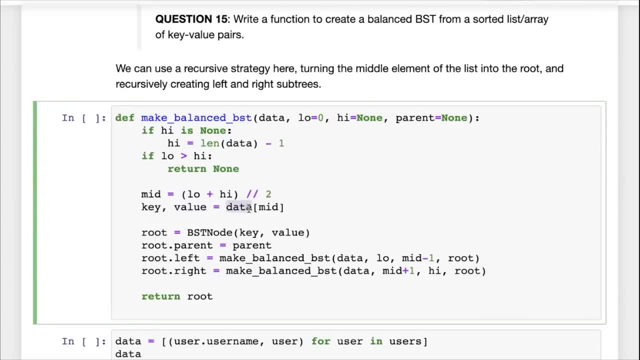 Then we get back the key and the value from the middle index. So we calculate, we find data made and that gives us the key and the value, for example, since the username and the user object, then we create the root node. So we create the root node using BST node and then we call make balanced BST on data, but this time from low to mid minus one, So from the indices zero to six, and make that the left child of the root, And we call it make balanced BST on the right node. 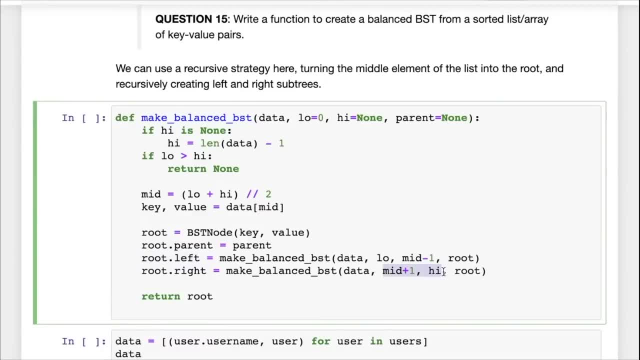 So on the right half, so from mid plus one, so, which is index eight to 14, and we make this the right subtree, and then we return the root, and that's it. That's pretty much it. The only thing that we might need here is the terminating condition when low becomes less than high, which means that we have no more elements to create trees out of. we simply return none. 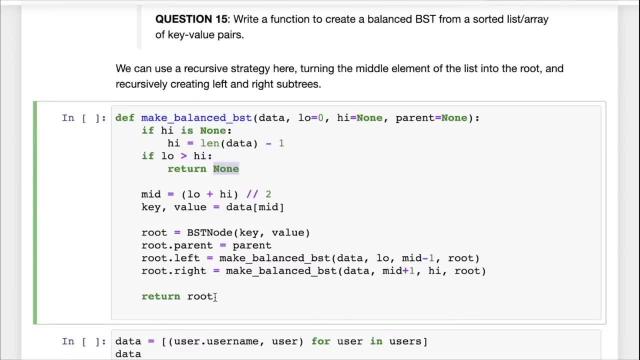 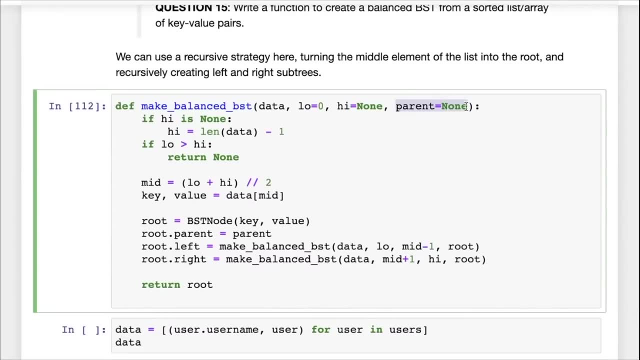 So the left or right subtree for those, for the parents of those nodes, get set to none. So that's your makes balanced BST function. We also have this other thing called parent going around and this I will let you figure out what the parent does here, but this is the basic idea. 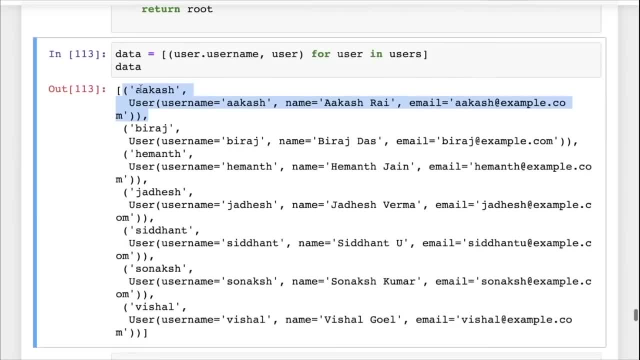 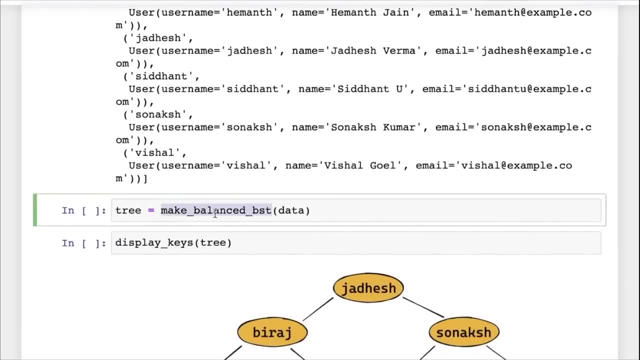 So here is a list of key value pairs. You have a key value pair sorted in increasing, in the increasing or lexicographic order of keys, and we're calling make balanced BST with data And that gives us a tree. and let's view the tree here. 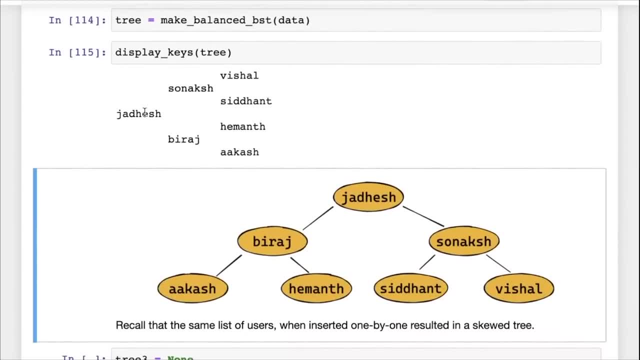 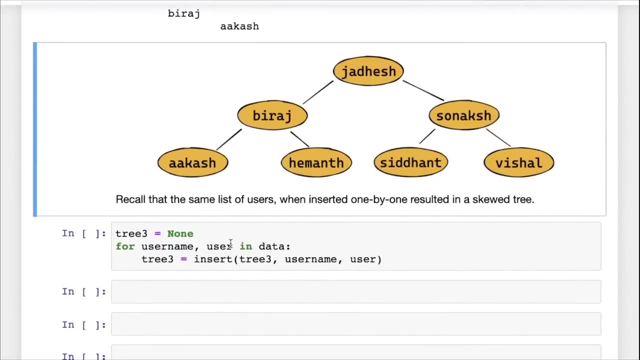 So there you go. Now we've created the tree perfectly as we wanted it. Ja, they should at the center, and we have Barrage Sonak each side and then the appropriate nodes on each side, as the children of those nodes Now recall that the same list of users, when inserted one by one, resulted in a skewed tree. here we are getting the list of users, username and user from data and inserting them. 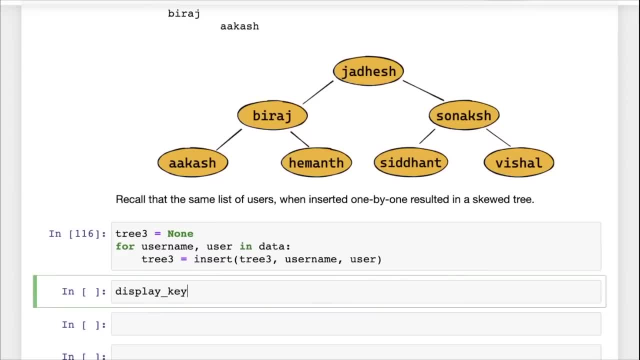 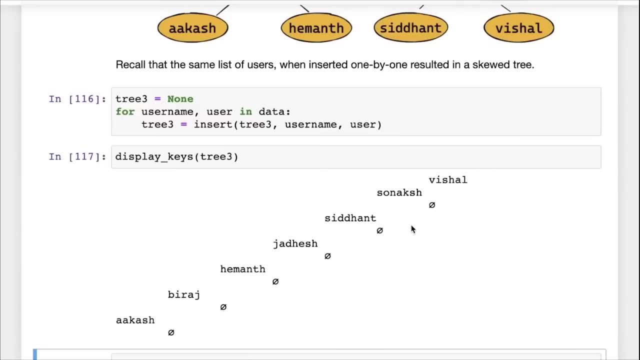 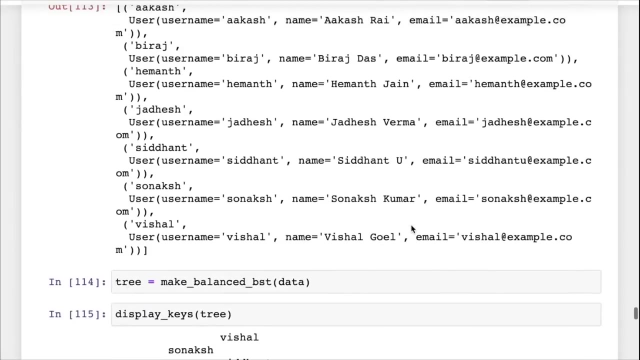 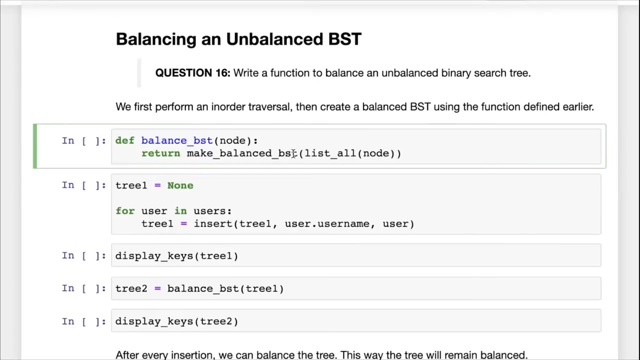 And you can see calling display keys on three. three Returns a skewed tree. Okay, So whenever you have a sorted area and you want to create a balanced BST, the way to do it is to start from the middle out. Now, finally, one other question you may be asked is to balance an unbalanced binary search tree. 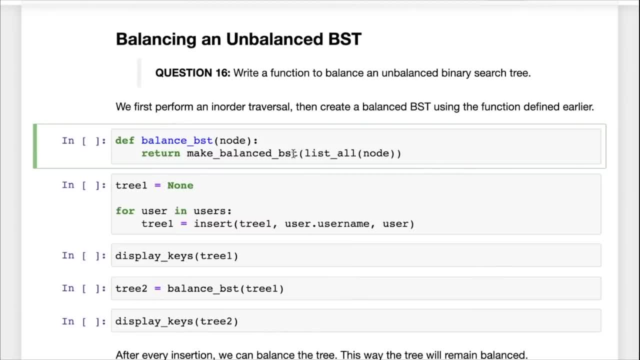 And this is pretty simple at this point- And this is kind of a trick question because it's a very simple question. It's a very simple question, Okay, Because if you were given this question directly, you may not be able to think about what to do. 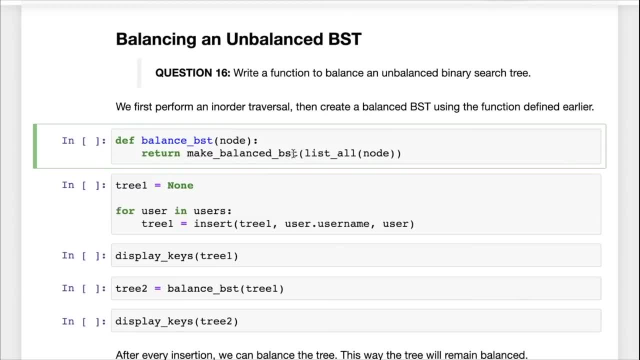 How do you balance an unbalanced binary search tree? But now that we have, we have a way to create a balanced binary search tree from a sorted array of key value pairs, And we have a way to get a sorted array of key value pairs. 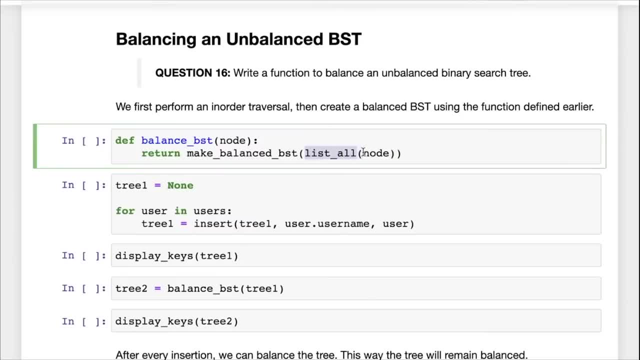 So now it simply becomes calling the sorted array, So calling list, all on the node which is also the inorder traversal, So doing an inorder traversal of the binary search tree which gives us a sorted area of key value pairs and then passing that into the make balanced BST function. 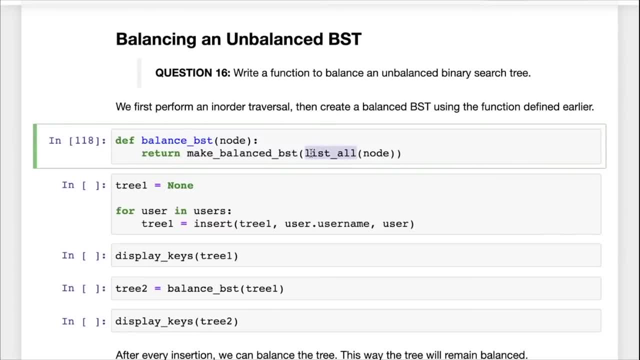 Okay, So that's the trick here. It's a two part question And once again we see the benefit of reusing our functions here. No, we this now balancing. an unbalanced BST now becomes a single line of code. That's very nice. 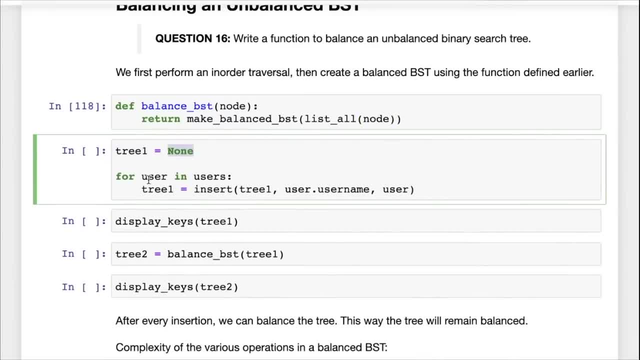 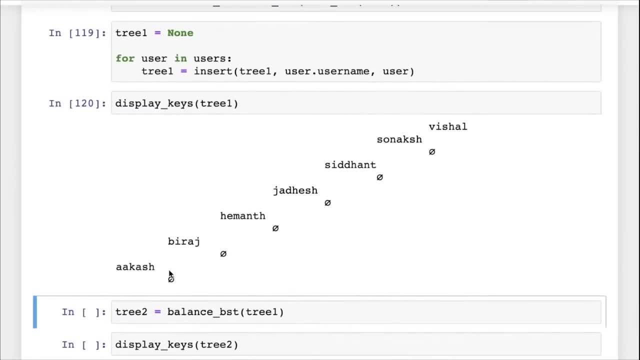 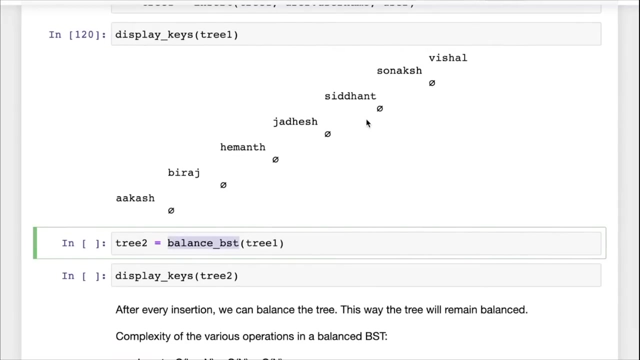 So we created three here with the value none and now we insert into it the values one by one And you can see that that creates a skewed tree, because we are inserting the values in increasing order, electrographic order. So we keep adding right children and we never add a right left child. but then we call the balance BST function, which internally takes this, gets in order traversal. 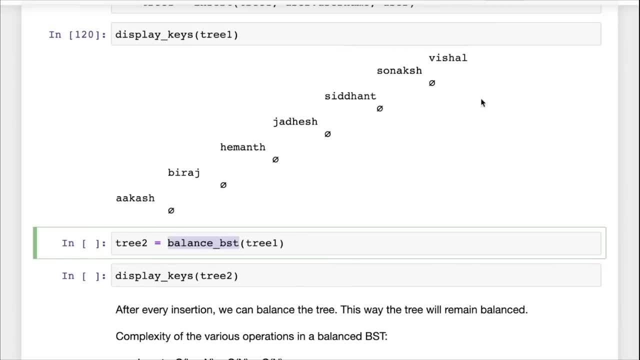 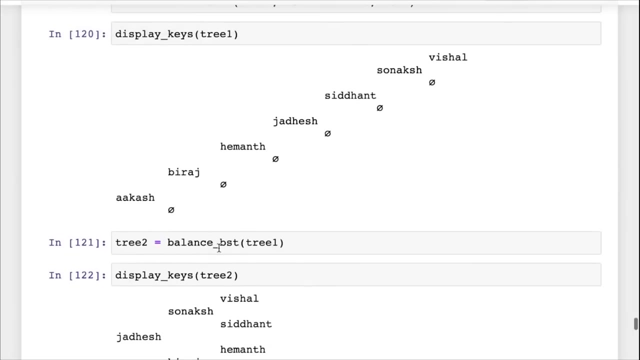 So the inorder traversal lists all the keys and key value pairs and sorted order, And then we call them make balanced BST function which starts from the middle and then creates a balance binary search tree out of it. So there you see, this is how you balance a binary search tree. 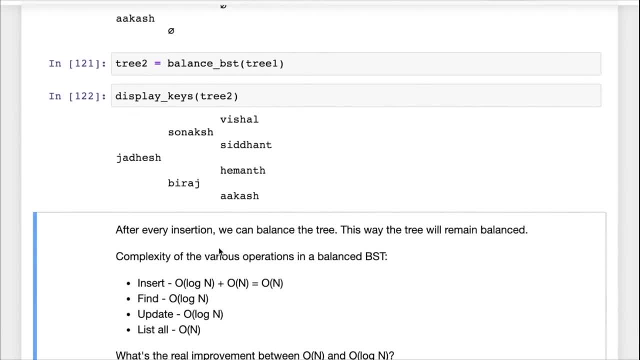 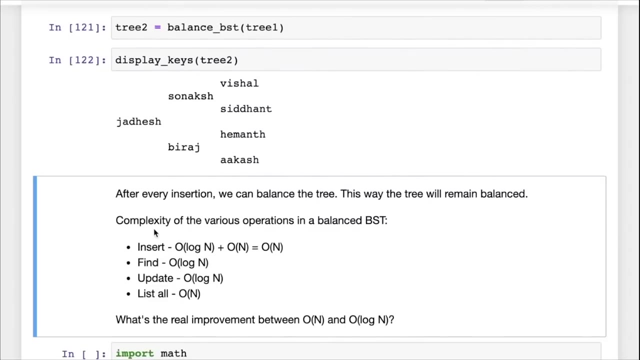 And what we can do now to maintain the balance as we grow our data structure is a simple thing that we can do is to insert, to balance the tree after every insertion, And that brings us to the complexities of the various operations in a balanced BST. 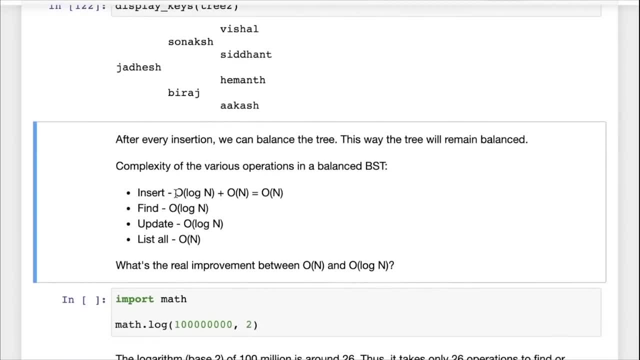 So if we are doing, If you're doing an insertion, that takes order login, because now if a tree is balanced, its height is order login. So for insertion you may have to traverse a path from the root down to a leaf and that path can be of length at maximum equal to the height, which is order login. 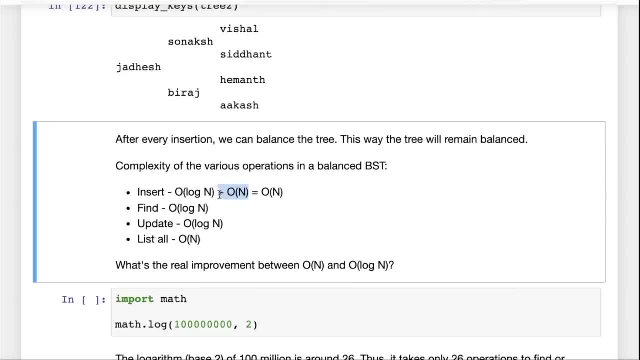 But if we are also doing a balancing with every insertion, then we also have an order and term added here and order and plus order login, because a login becomes much smaller than N as N grows. So order and plus order login is The same as order N. 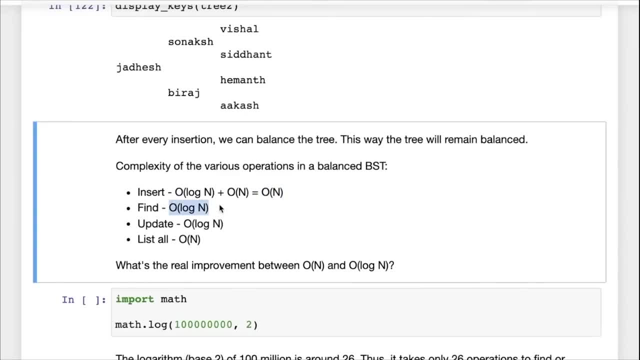 So that makes insertion order in finding a node becomes order login, updating a node becomes order login and you can verify that listing- getting a list of all the nodes- is ordered N. So what's the real improvement between order N and other order login? 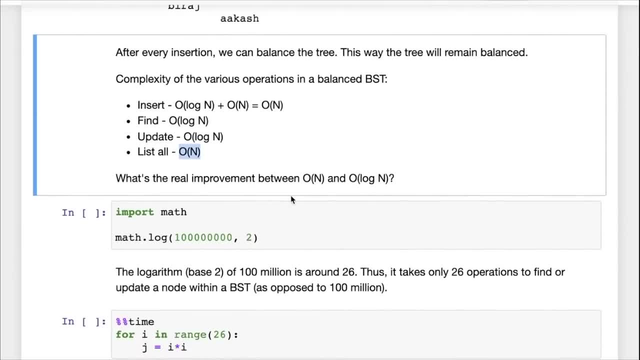 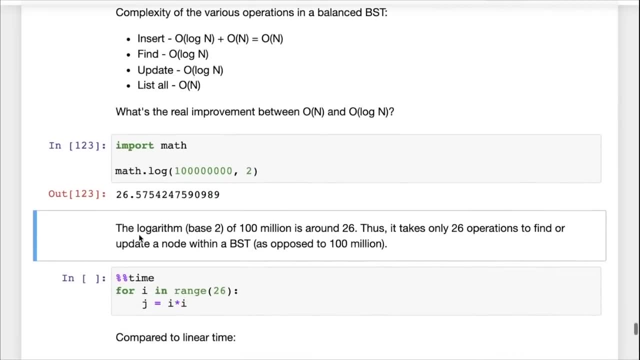 So let's think about it. If you're looking at a hundred million records, then log to the base. two of a hundred million is about 26 or 27.. So it only takes 26 operations to find, To find or update a node within a balanced BST, as opposed to a hundred million operations. 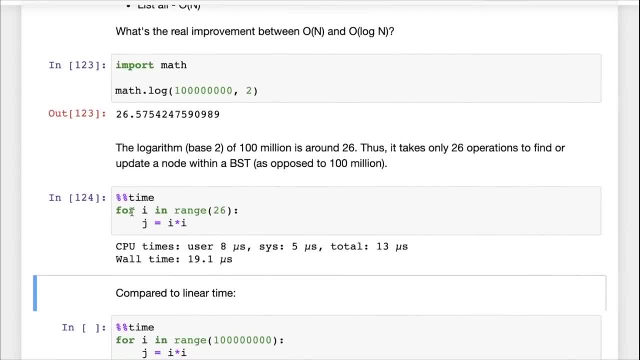 So you can see here a 26 or a loop of size of a length 26, and we're doing some operation inside. It only takes about 19.1 microseconds, That is, one microsecond is 10 to the power minus six seconds. 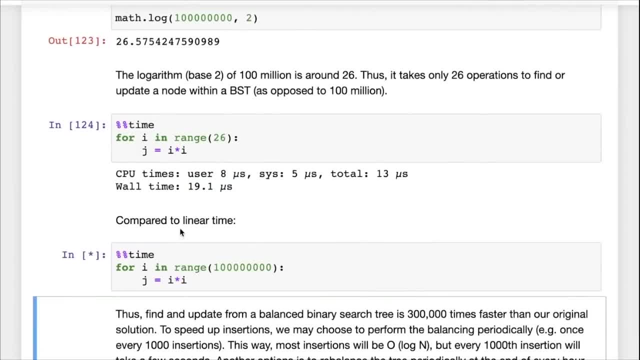 On the other hand, order N involves looping through the entire list, So looping through a hundred million numbers rather than 26. And that Obviously takes far, far longer. And we saw that it took about 10 seconds, right, About 9.98 seconds. 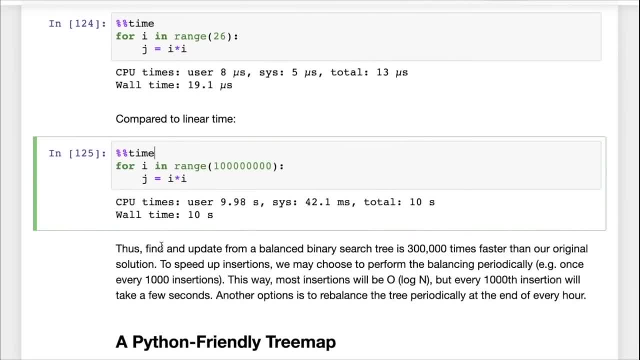 So to find an update, finding and updating a node in a balanced binary search tree is 300,000 times faster than our original solution. And all we've changed here is the data structure, And that's the importance of data structures, because now each user will be able to view their profile in just 19.1.. 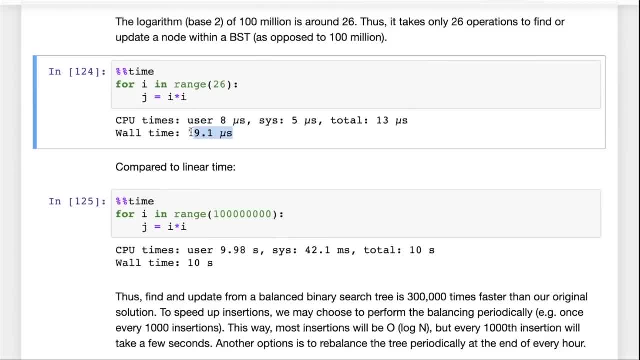 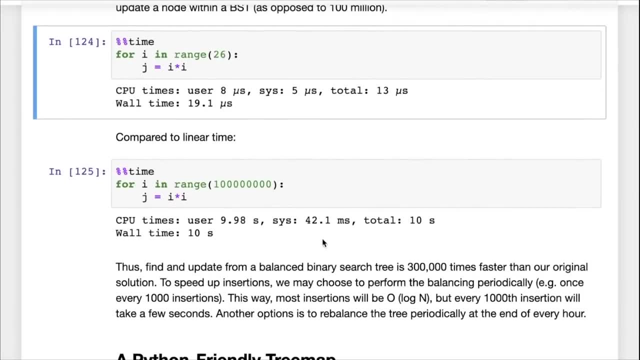 Microseconds. At least that part of the request will take only this long, So the user experience will be better and your CPU will be busy for a shorter time, So you will be able to serve not eight but hundreds of thousands of users every second. 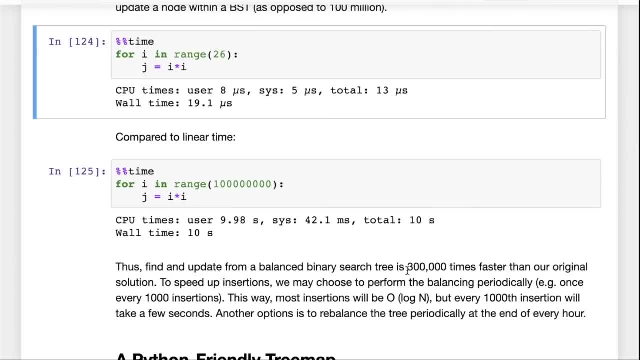 And finally, your hardware cost will also be far lower, because now your CPU is busy for a lesser time, So you do not need to use a very large machine, or you do not need to use too Many machines to support hundreds of millions of users. 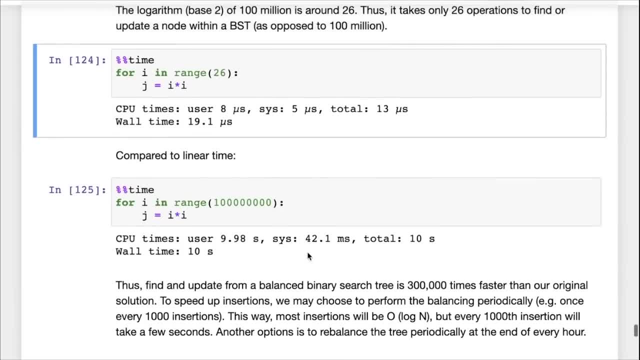 And that is the benefit of choosing the right data structure. Now there's one tip here: How do you speed up insertions? So what we may do is we may choose to perform the balancing periodically instead of at every insertions. For example, we can balance for every hundredth insertion, or every thousandth insertion, or every hundred thousandth insertion, whatever. 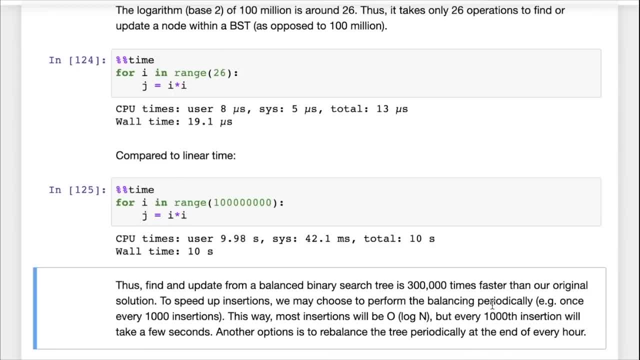 No, that and that's where we have to balance. how often do we need to insert things versus how often Do we need to restore the balance? Another idea is to do the balancing, maybe periodically at the end of every hour. So for a second or two there may be a slight dip in the performance because you may be performing the balancing. but even that, there's a way to do it. 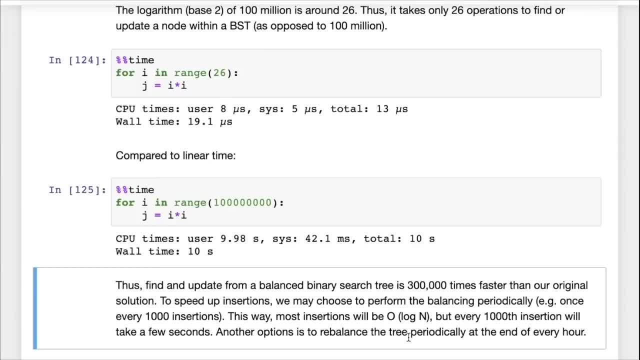 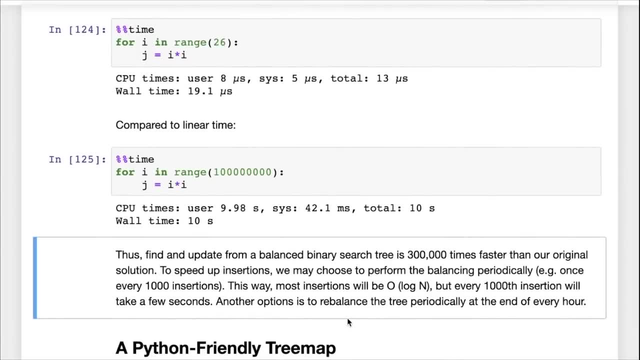 So you can take a copy of the tree and then balance it and then simply replace the pointer to the original tree. So there are many other tricks that you can apply, And in fact there's also an algorithmic trick which brings Insertion and balancing together into an order login operation, which we look at right at the very end. 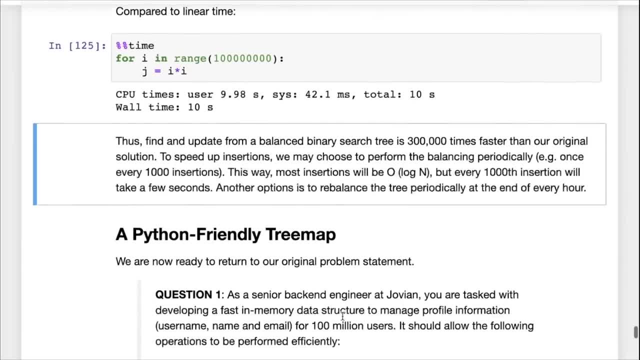 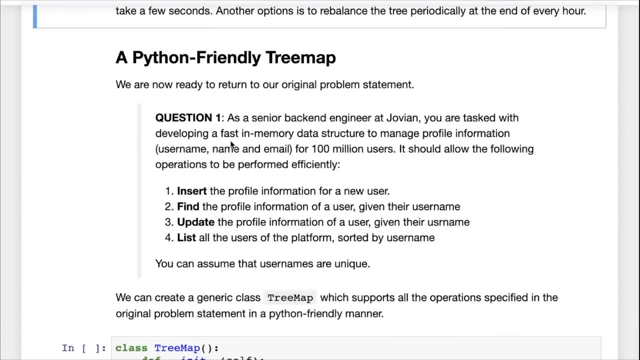 So stay till the end? Uh, but before we do that, let's come back and answer our original problem statement. So remember now, as a senior backend engineer, you are tasked with developing a fast in memory data structure to manage profile information, username, name and email for a hundred million users. 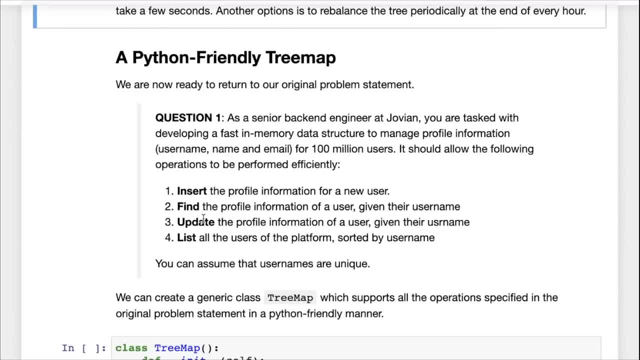 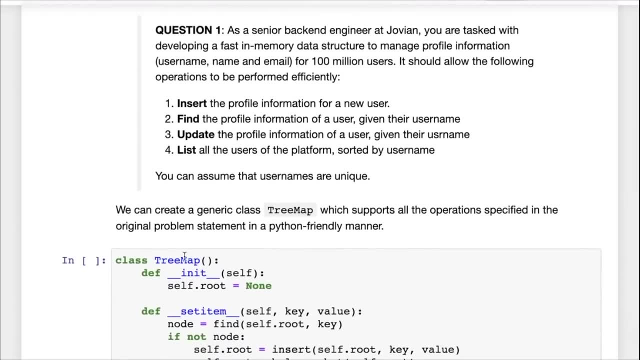 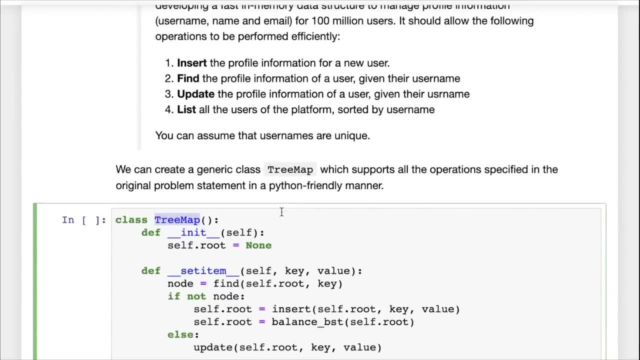 And it should allow insertion, find, update and listing the users by Username all as efficiently As possible. And to answer this question, instead of creating a user database class, we can create a generic class called tree map, because we have been making things more and more generic as we've gone along. 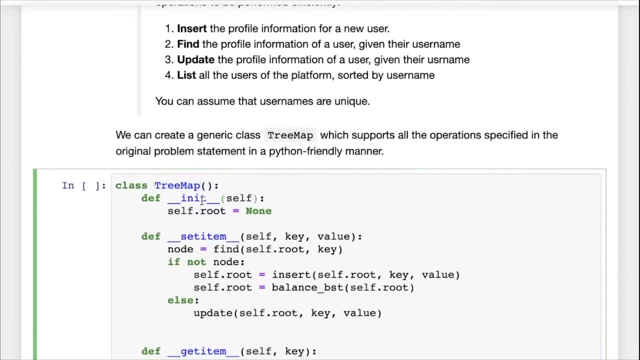 So let's define a function called tree map, which internally stores A binary search tree, a balanced binary search tree, inside it. So when we initialize a tree map, we said self dot, root to none, which means we have not created a tree. 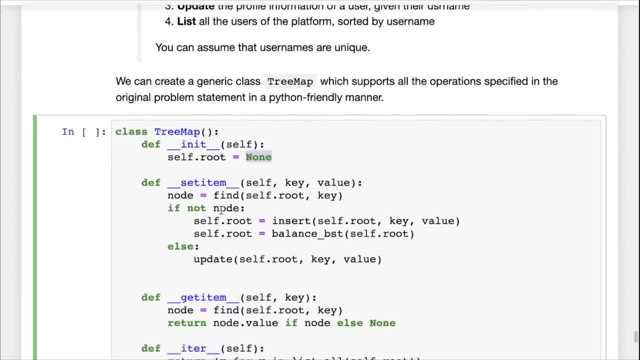 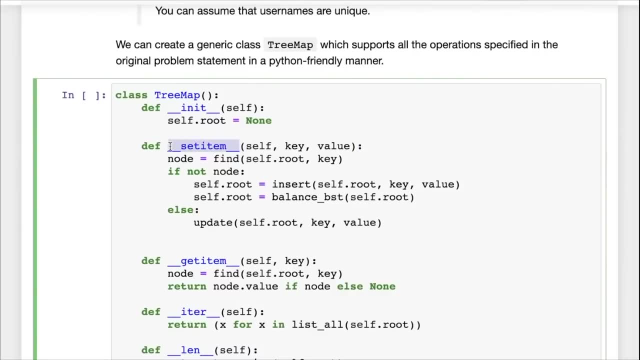 So far. and then, instead of defining functions- insert, update and delete- we are going to use some special functions in Python classes, So we're going to use the function set item. We're going to use the function set item here, and set item is just like insert, except it is a combination of both insert and update. 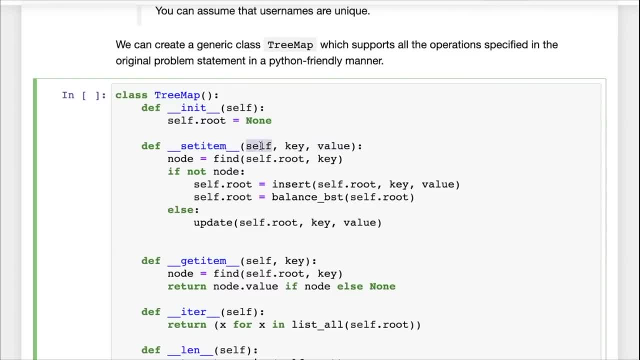 So to set item, we will pass a key and a value And, of course, self will refer to the tree map object itself. So The first thing we do is we get the route which, which is basically the binary search tree that we are storing internally here. 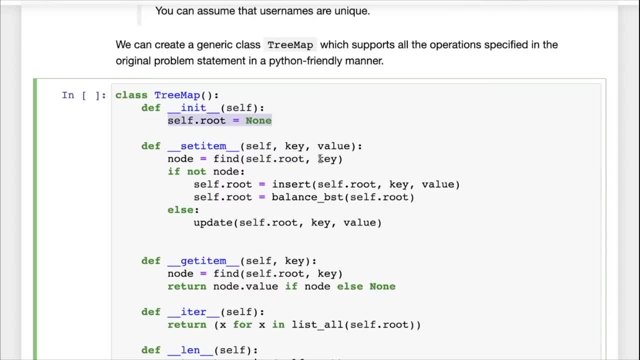 So we get the binary search tree and then we find we look for the key inside the binary search tree. So if the key is found, so if we find the node in our tree, then we come into this else position and then we simply update its value. 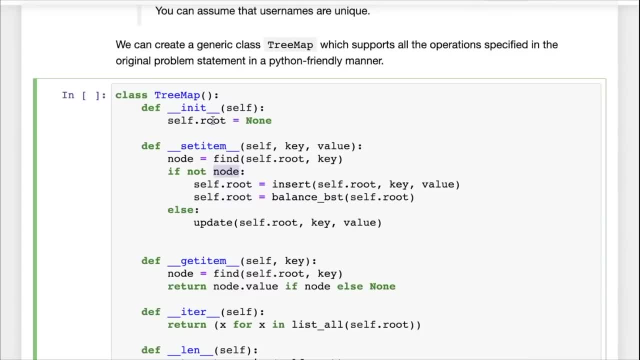 And if we do not find the node? so which is what happens initially, because initially our self dot root is none. So when you call find with none And pass a key, you'll get back none. So then we first set self dot root by inserting the key into the tree. 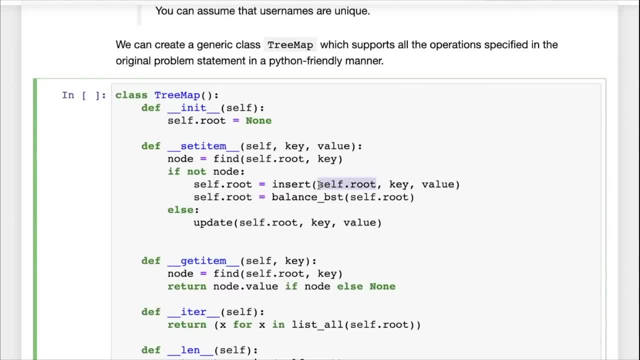 Okay, So if a key exists within our binary search tree, then we update it, And if the key does not exist within a binary search tree, then we insert it into our binary search stream. Okay, So we've combined insert and update into the single operation called set item. 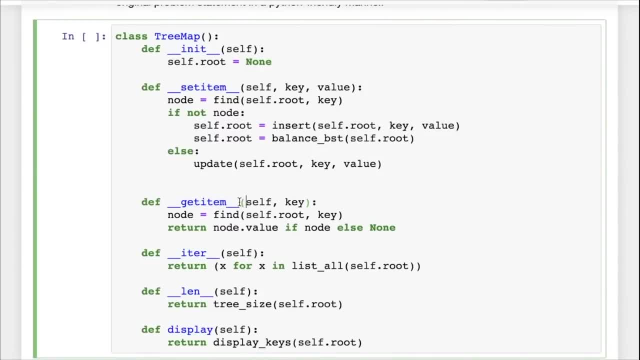 And similarly we define another operation called get item. This is the find operation. All we do here is we find the node inside self dot root using the find function we had defined earlier, And if the node is present, if it is found, then we return the value of the node. 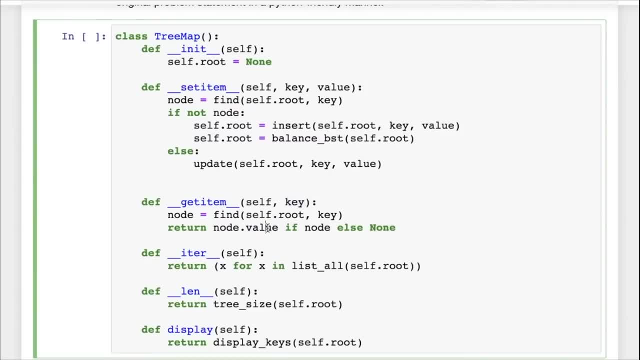 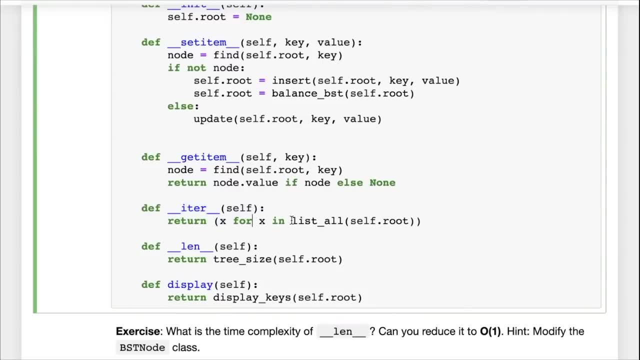 Otherwise we return none. So, given a key, we retrieve the value. And then we have. we defined one last function called iter, and this is the replacement for our list. all function. So what we do is we simply say: we call list. 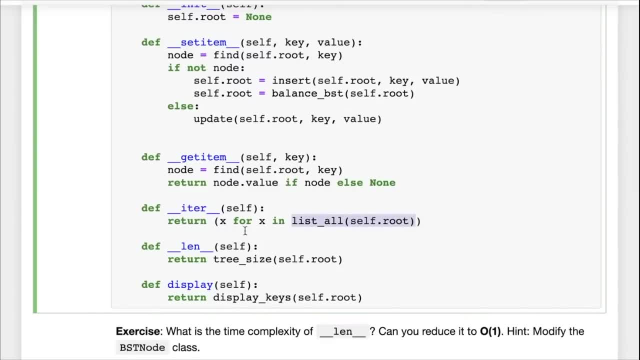 All On self dot root. So that gives us a list of key value pairs. And then we have the special syntax. We say X for X in this list and we put these round brackets around it. So what does round brackets around it does is that this creates a generator out of it. 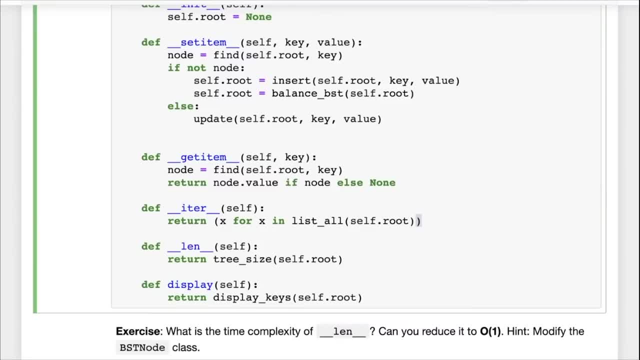 So now this is no longer list, but this is a generator, and a generator is something that you can use within a for loop, So the iter function will allow our class to be Used directly within a for loop, And we'll see the example in just a second. 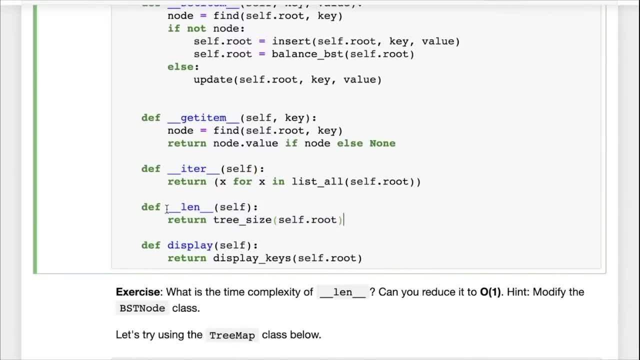 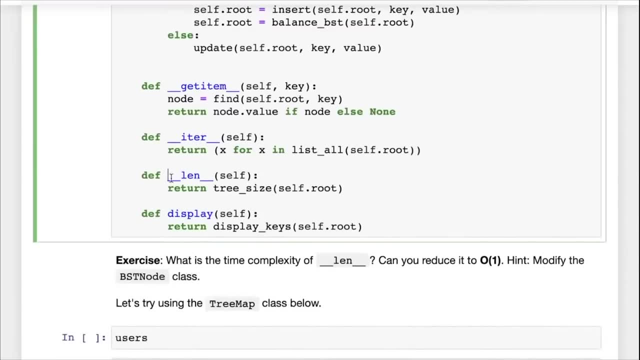 And finally we have another function called underscore, underscore, Len. So remember there are double underscores here. So there's double underscore- set item double underscore. double underscore, get item- double underscore. Similarly double underscore Len- double underscore. here We simply return the size of the self dot root. 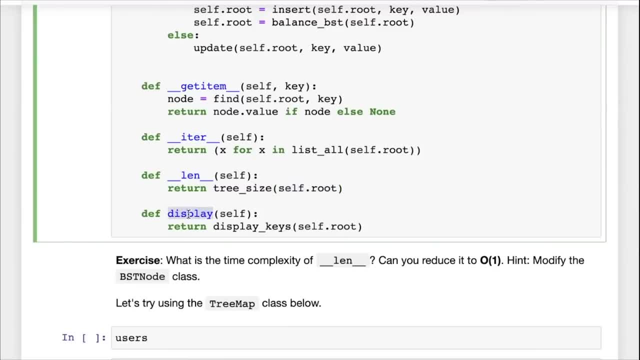 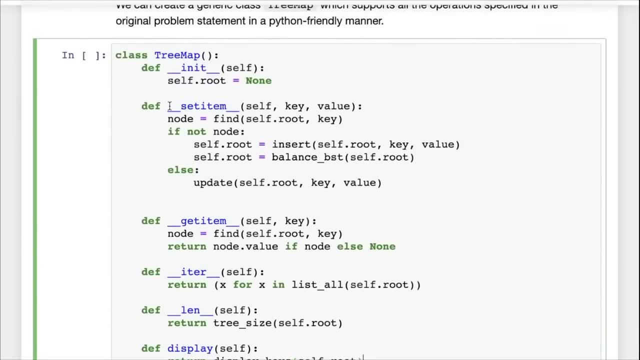 So here we simply return the size of the binary tree, And then we have this function called display. This is going to simply display the keys. Okay, So now we've defined the stream up Structure and it has all of these funny looking methods. 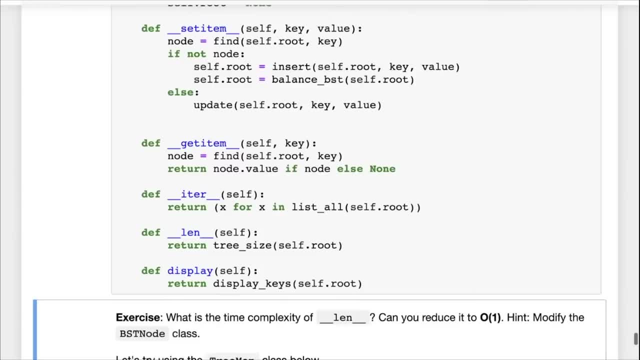 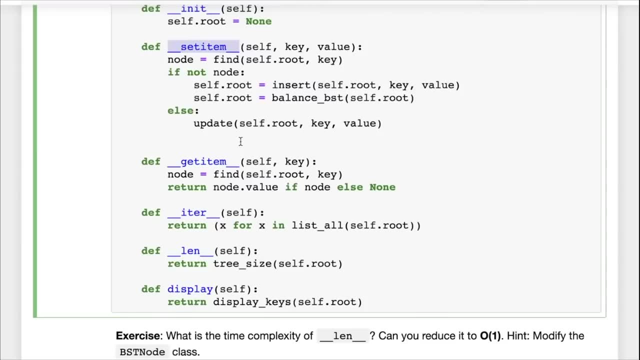 Like we know in it. but what about all of these? but we'll see what these do in just a moment And we know what the what the functionality is. but you may be wondering why we've defined them like this. So the reason is these are special methods that are treated specially in Python. 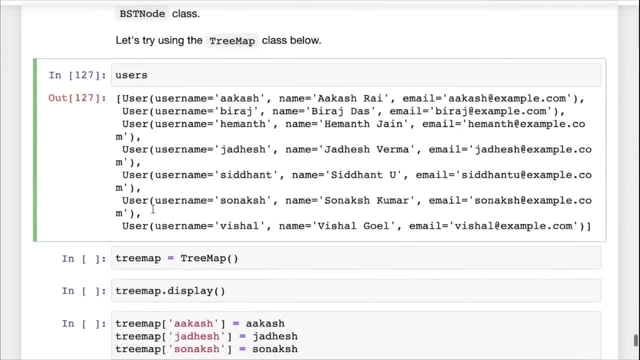 So here's how you can use them. Let's first get a list of users that we'll later insert into a tree. Let's get a tree map So we instantiate the tree Map Function but the tree Mac class, and that gives us a new tree map inside it. 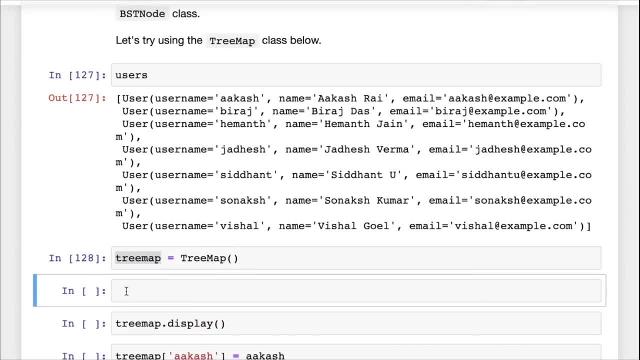 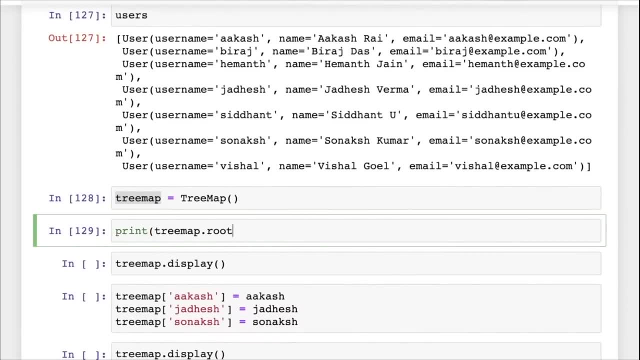 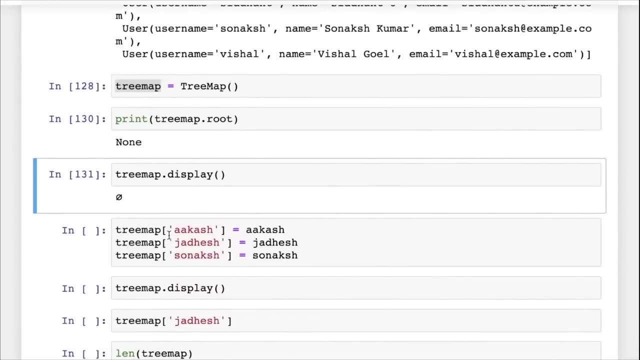 There is no binary tree, You can check. if you check tree map dot root, you will see that it is none. There's no value here And if we try to display it, you can see that this tree map is empty. then to insert, instead of calling tree map dot insert. or instead of calling tree map dot. 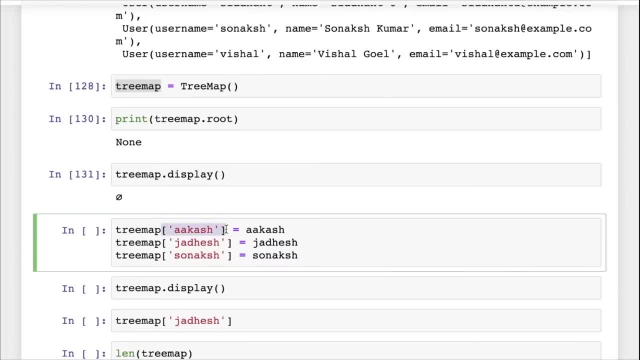 underscore- underscore- set item. we can use this Indexing notation, So we open these square brackets and we put in the key that we want to insert. So, if we want to, against the key, insert against the key Akash, which is the string. if you want to insert the value Akash, then we simply say: tree of Akash is Akash and similarly, tree of a certain key, with the indexing notation set to this right. 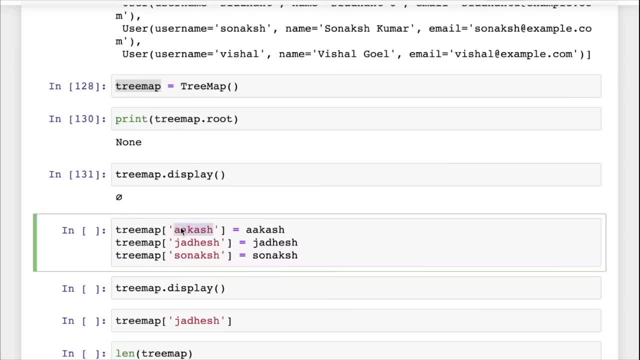 So this is going to first look for the key as we have defined in set item. If it finds the key, then it is going to update the value for them, The key. if it does not find the key, then it is going to insert that key value pair as a new node into our tree. 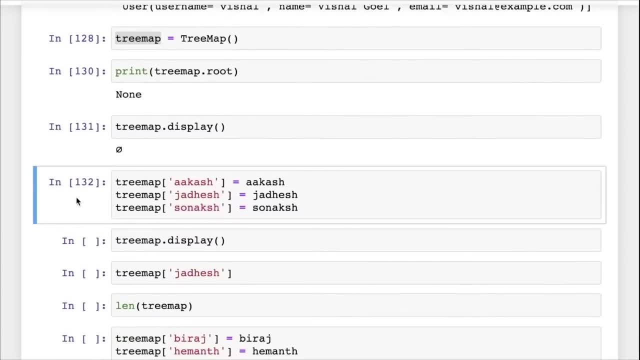 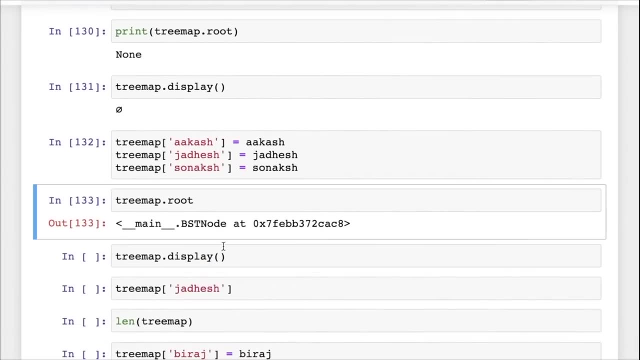 So let's check it out now And let's see here: If we now check tree map dot root, you will see that now it is a BST node And if we try to display it, you can see that now it has a structure. 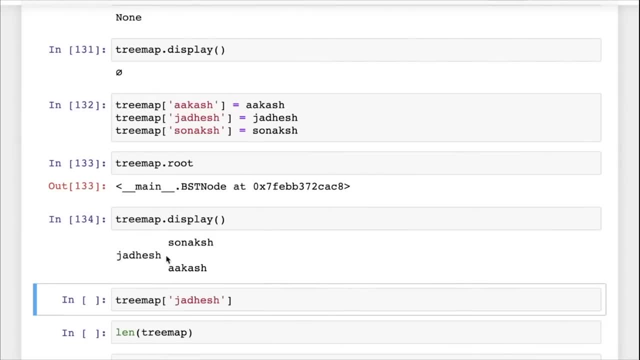 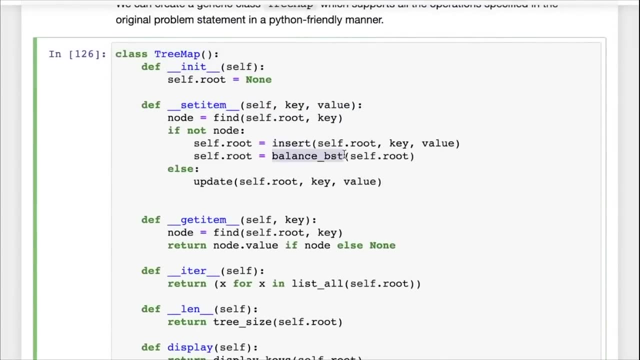 Jadish, So not an Akash. also note that this is a balanced tree And if you go back here to set item, you will notice that Whenever we insert right after this, we also balance the tree. and now you can change the logic here so that we do the balancing not after every insertion. 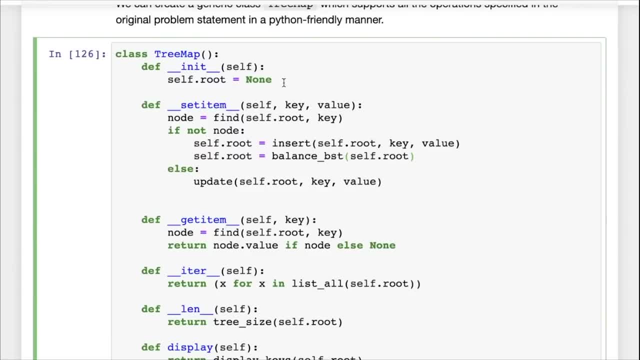 but maybe after every a hundred insertions. So you may need to track somewhere What is the current number of, what is the current insertion counter And when it gets to a hundred, only then do the balancing and then set the counter back to zero. 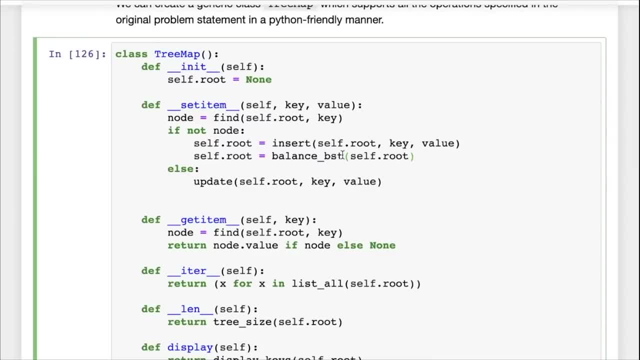 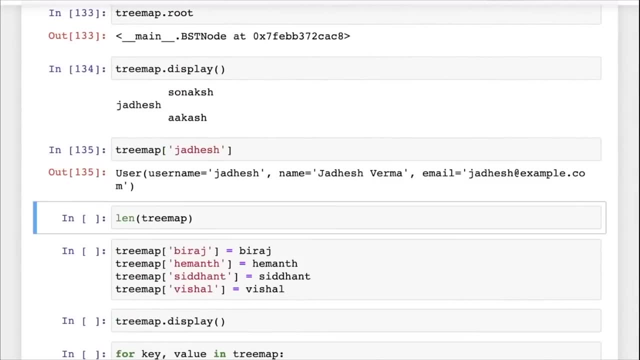 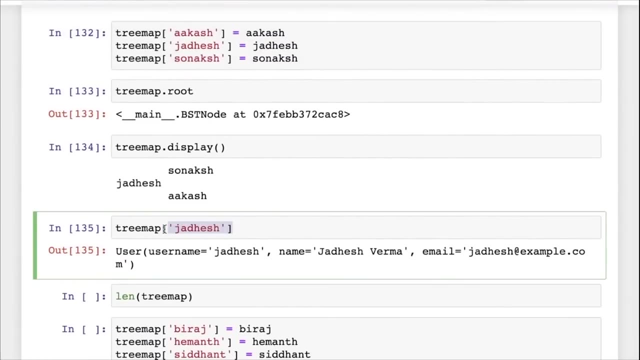 So that's an exercise for you: perform the insertion or perform the balancing at only at certain intervals. And here's a way to retrieve an element. So the retrieving element is also now really simple. You just call tree map with Jadish as the index. 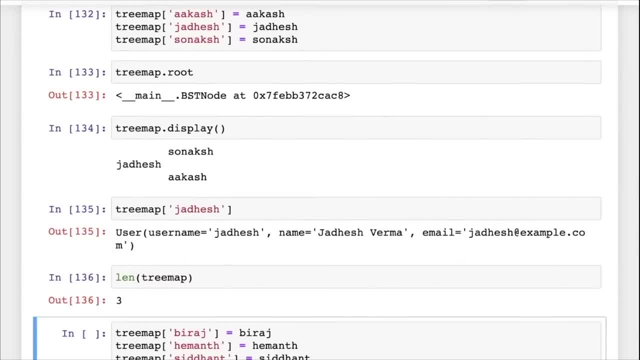 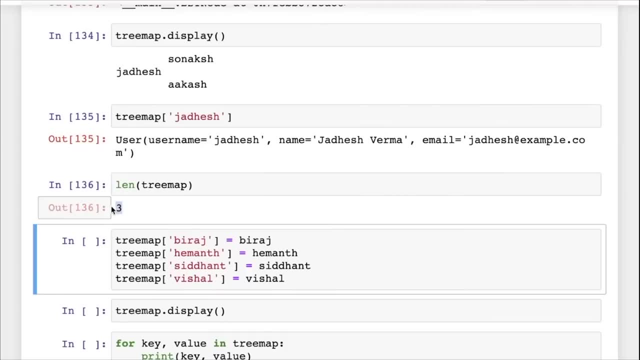 And that gives you the value if it is found, And if it is not found, it simply returns none. now, because we have defined the function: underscore, underscore, Len, underscore, underscore. So you can see, here that has the value three, because that now we can use it with. 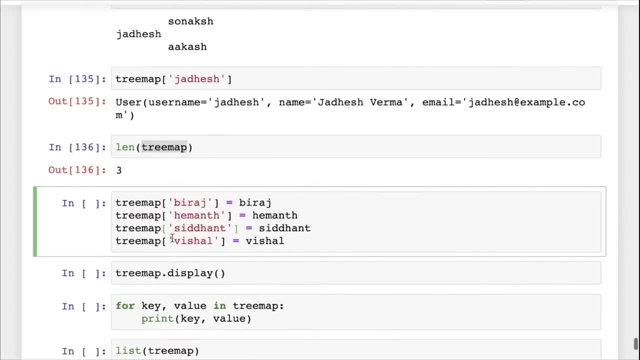 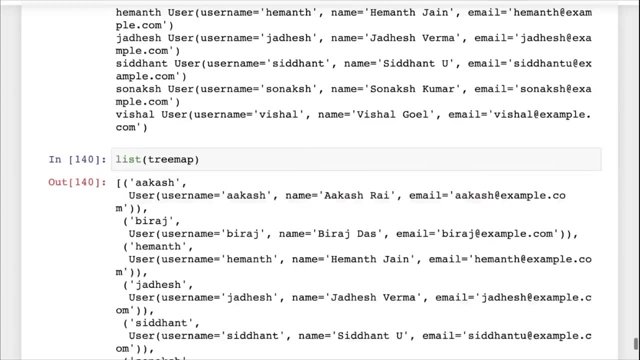 the Len function, which is used for lists and dictionaries, and let's add a few more things And let's set the values and let's see here, So you can see, all this works exactly as expected. Now we're able to set values. 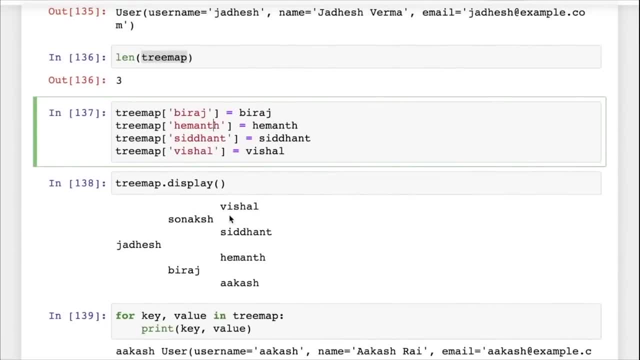 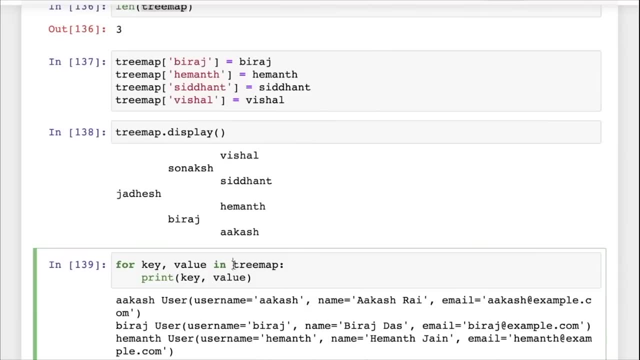 We're able to update values, We're able to display the tree. It is remaining balanced And remember I mentioned that you can use this in a for loop, So you can now put the tree map directly into a for loop And what this will do is because we have defined the underscore, underscore iter. 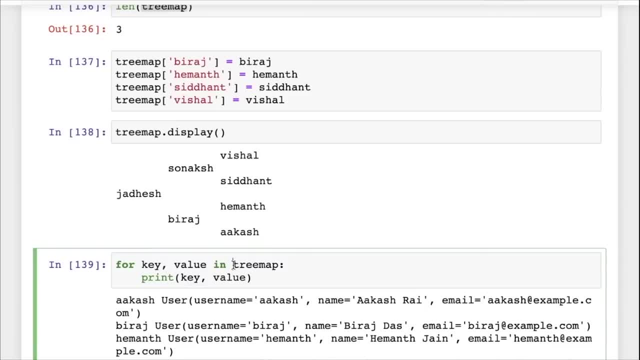 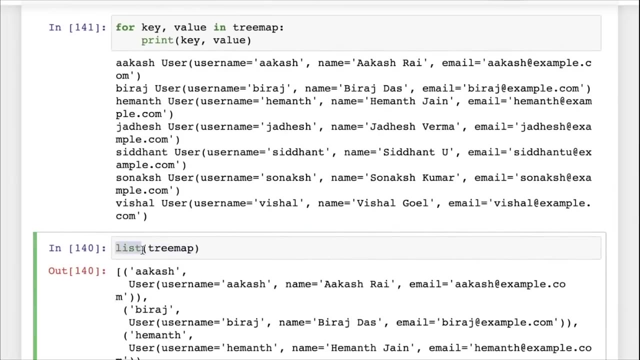 function, and the iter function returns a generator. So now You can use this In a for loop and you get back the key value pairs from the list- all function that was used inside iter. you can print the keys and the values And, in fact, if you want to convert it to a list, all you need to do is pass it into the list. 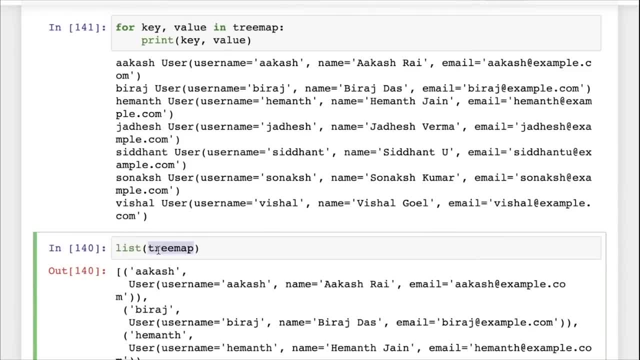 And, once again, because this is a generator, because this is an iterable, this is now an iterable class and you've defined that the way to iterate over this class is to get elements out of the key value pair list. So when you call list, you get back this list of key value pairs. 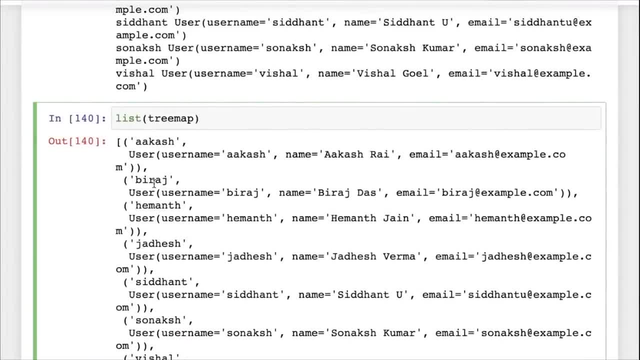 Okay, So now we've made it a very Python friendly class. you know, instantiating It is very easy. We simply create a new tree map. Adding values is very easy. We simply use the indexing notation. Removing elements is very easy. 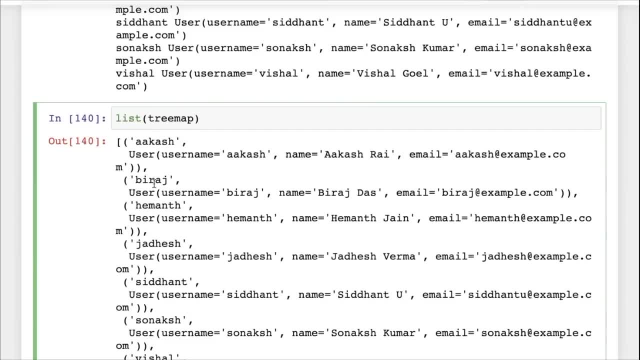 I will not. removing a finding elements is very easy. We simply use the indexing notation. Updating elements is the same as inserting. We can also check the size of the tree quite easily using the land function. And then we can also use iterate over the keys- iterate over all the users in a for loop- quite easily. 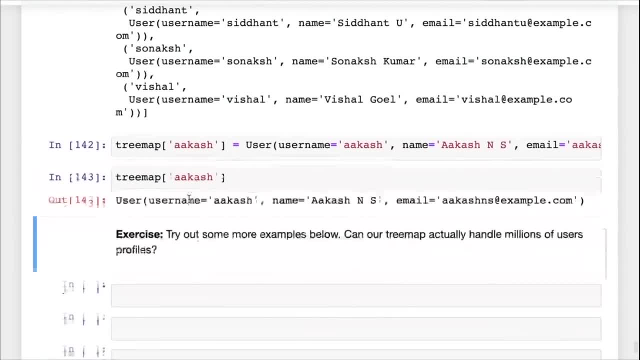 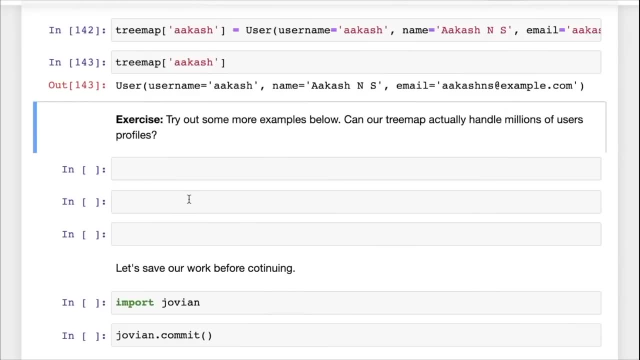 And we can also update values. As you see here, values have been updated. Now the. the purpose of doing this is to make it easier for other people to use this data structure. Now, as a senior backend engineer, you may have designed this data structure and you may have implemented binary. 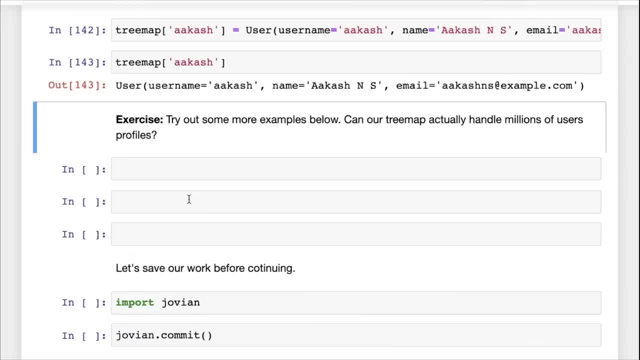 search trees inside it. but it's not important for other people on the team or other people using your data structure to know what the internal Implement. What's important for them is to be able to use it easily. So that's why I always think carefully about the interface or the API of your functions or of your modules or of your classes. 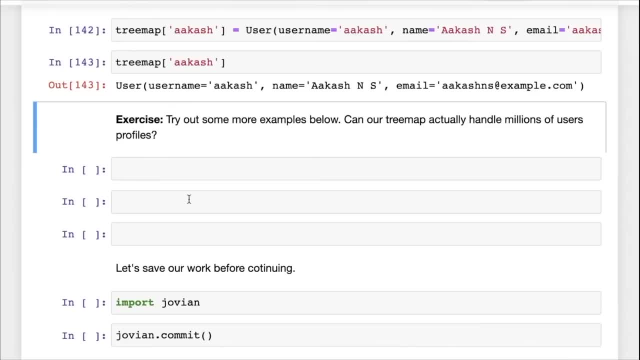 Try to make them as Python friendly as possible. This was something that will be appreciated. that will be appreciated in interviews and by coworkers. So make them Python friendly so that when people want to use something you've created, it is extremely intuitive and they do not need to. 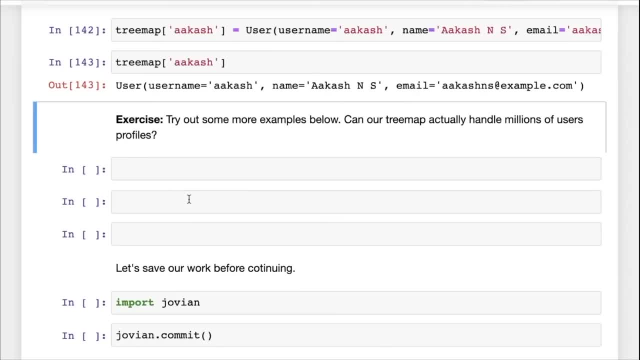 really understand the understanding Of the underlying details. for instance, I could be using this class and I could have no idea that it is a binary search tree. All I know is how to insert and how to get a value out of it, And I know that it is super efficient because you have designed it and I don't don't need to worry about the internal details. 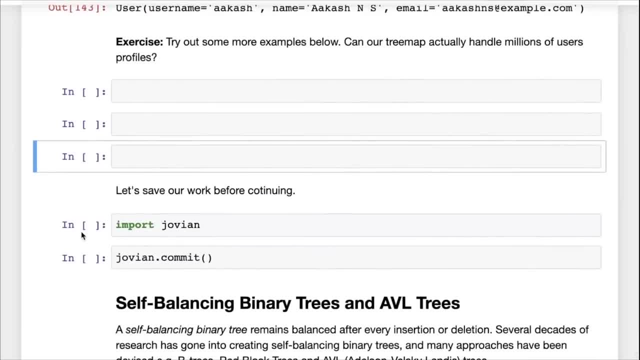 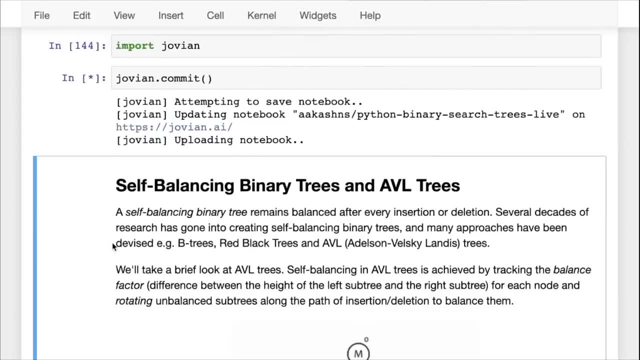 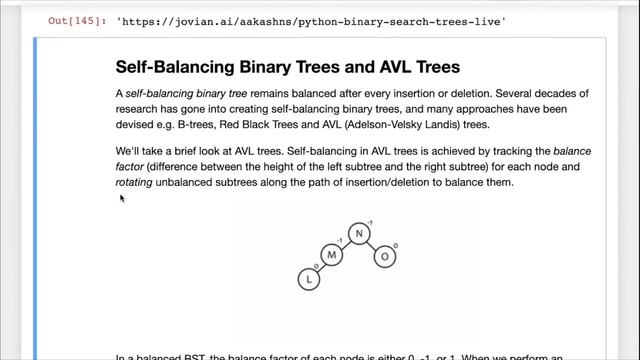 So encapsulation and a good API is a very important skill to have to cultivate, So do that as you work on programming problems. Now, once again, let's save our work before committing. Uh, now, I did tell you that There is a way to create self balancing binary trees, and a self balancing binary tree remains balanced after every insertion or deletion. 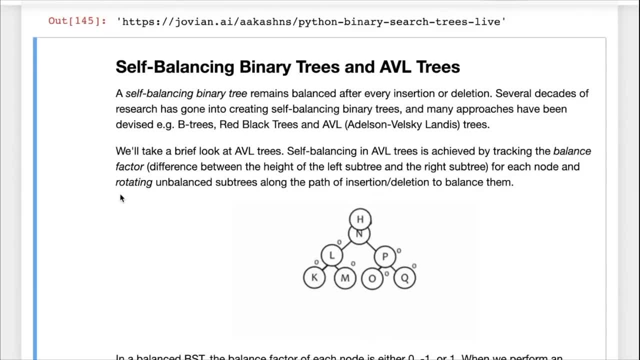 And in fact several decades of research has gone into creating self-balancing binary trees, and not just binary trees, but other trees as well which are not binary in nature, And many approaches have been devised, for instance red black trees, AVL trees and B trees. 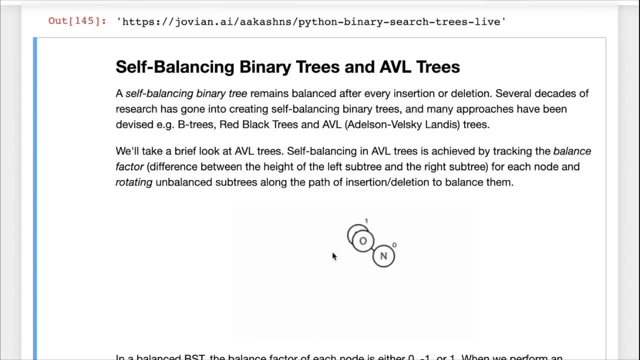 So here's an example. This is an avian tree, So here, whenever a node goes Out of balance, we rotate the tree, and you can see visually what we're doing here Now. whenever you see that there is an imbalance in the tree, we rotate it. 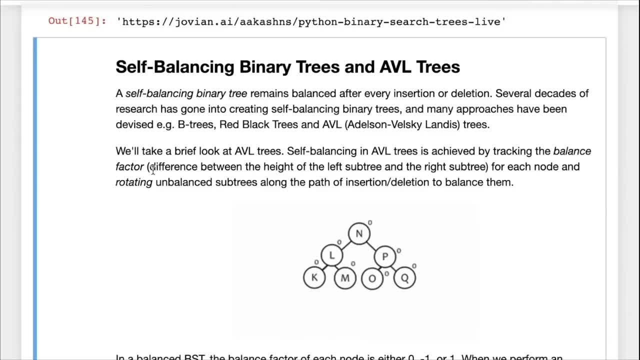 And how do you do this? We do this by tracking the balance factor, which is the difference between the height of the left subtree and the right subtree for each node, and then rotating unbalanced subtrees along the path of insertion or deletion to balance them. 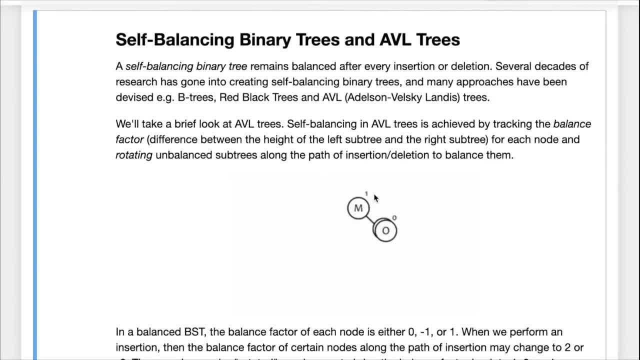 So you can see, the balance factor is zero right now. The balance factor becomes one and the balance factor It becomes two. Then we rotate it to set the balance factor back And then the balance factor here becomes minus two. So here we do a right rotation here. 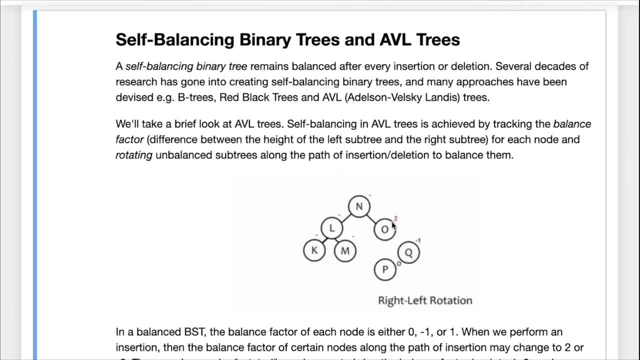 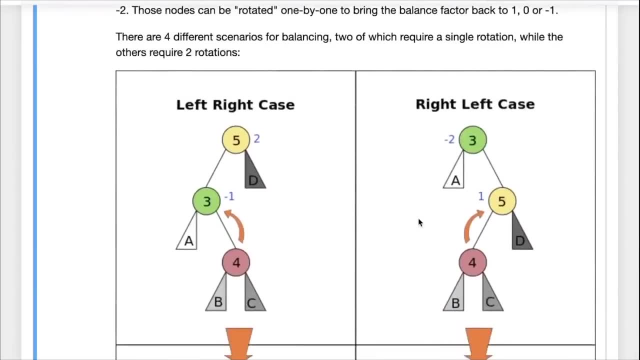 The balance factor becomes minus two here and minus one here. So here we do two rotations. So there are four cases in total. There's the left right case, the right left case, the left left case in the right right case. all four cases were demonstrated here as well. 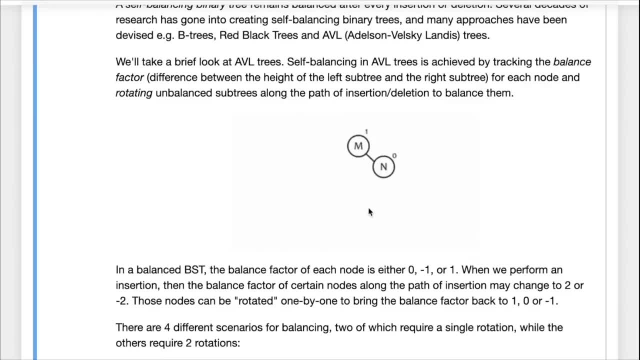 And then you may need to do this rotation not just once, but you may need to do this multiple Times along the path of insertion. So when you insert a node and that node creates an imbalance, then you need to walk backwards. So you need to keep going from parent to parent and keep rotating nodes whenever you need to rebalance them, based on the updated balance factor of each node. 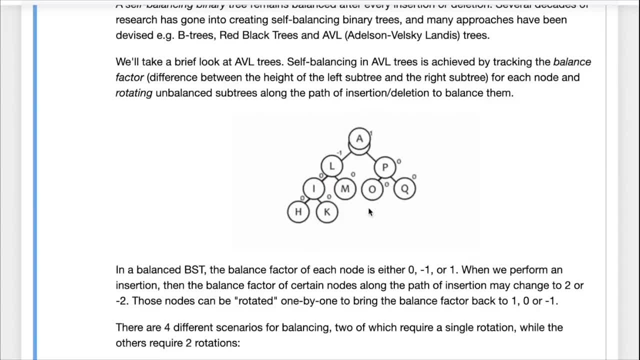 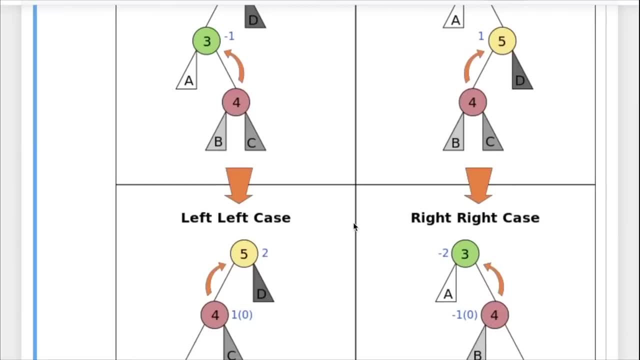 So it seems a little complicated, but it's actually not. It's just that there are multiple cases to handle, So you will need to write a couple of helper functions. You'll need to write a function, Left rotate, which Rotates node left while still preserving the binary search deep property. 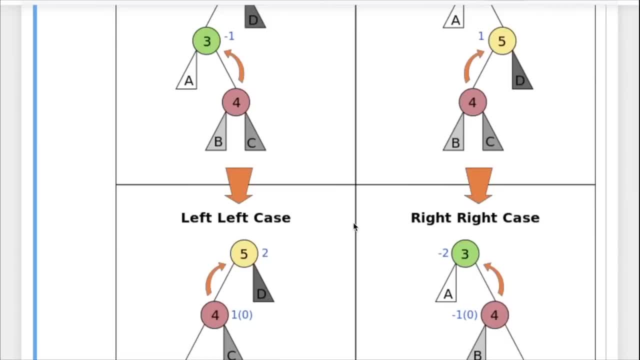 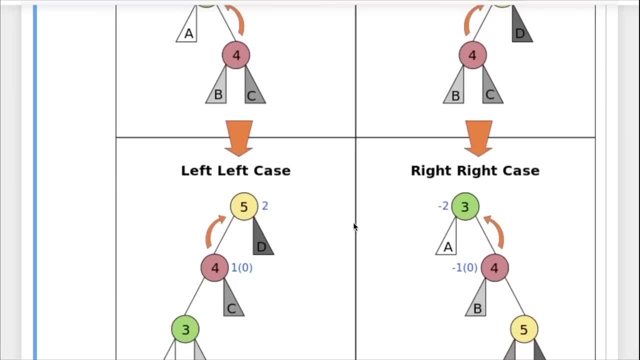 You will need to write a function right Rotate which rotates the function which rotates it to the right while preserving the BSD property, And then, in the insertion, you will also need to perform the rotation at the right places and you will need to track the balance factor inside each node. 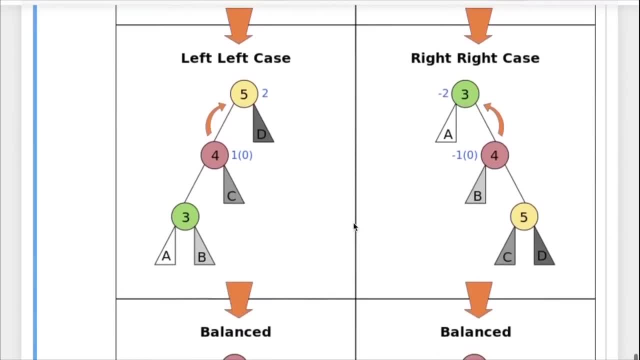 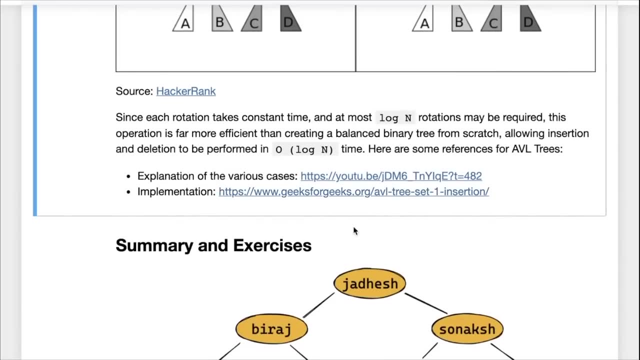 So there are a few things to work out here. and, don't worry, You will normally not be asked to implement an avian tree within within an interview or within a coding assessment, So you do not really need to Learn the implementation, but it's nevertheless a very interesting data structure to study. 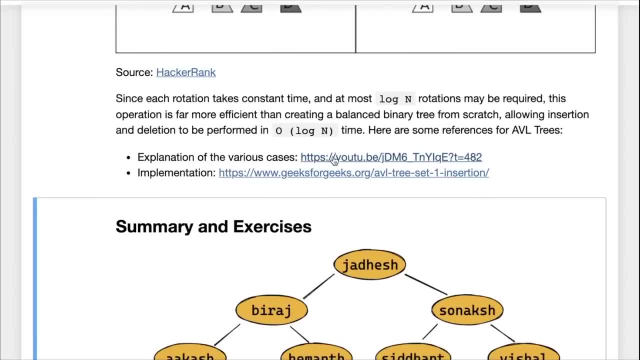 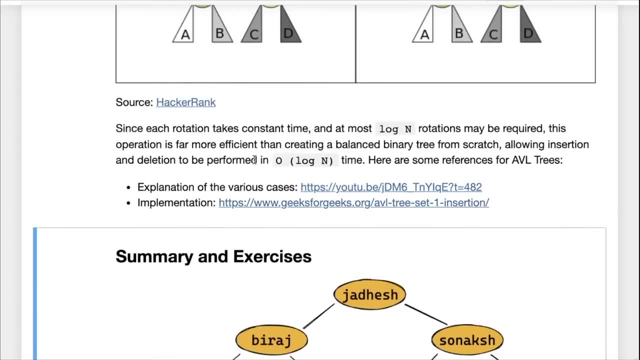 And here are a couple of resources you can check out. So you can check out this YouTube video, which explains it very wonderfully, And you can check out this implementation on geeks for geeksorg And the important thing for us to take away here and which is something that you may be asked, if not the implementation but just the complexity. 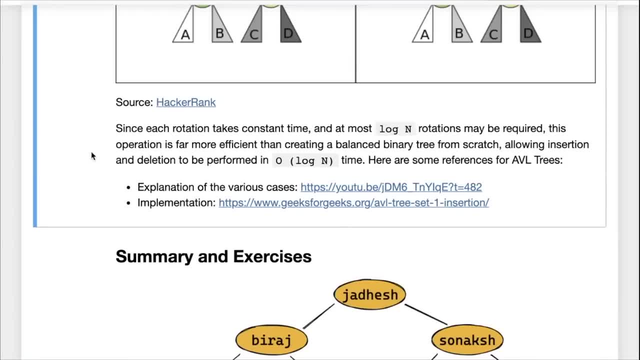 The important thing is that each rotation takes constant time and at most log and rotations may be required, Because If you are starting with a balanced tree and you're inserting a new node, then you may traverse a path of height at most, of length, at most login. 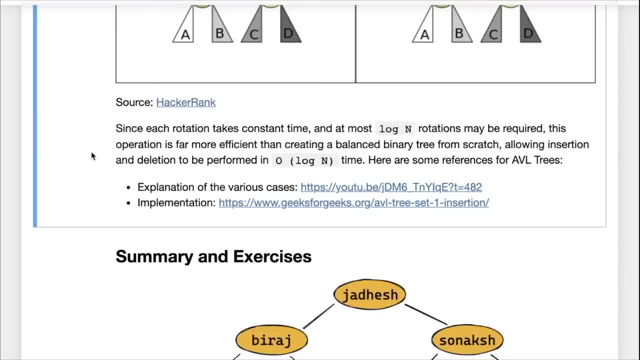 So you may need to perform, at most login rotations, maybe twice of that. So what that means is, in order login time, you will be able to insert and maintain the balanced property of a binary tree right, So you do not need to recreate the entire tree again. 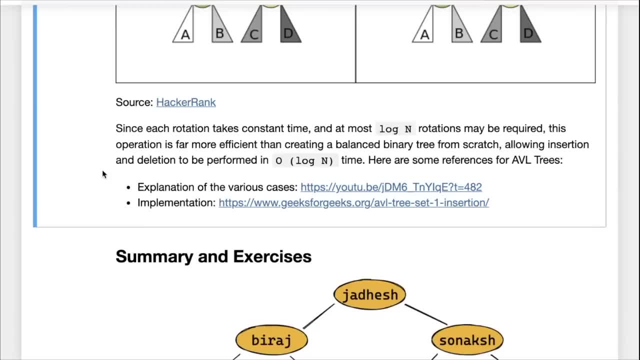 And that makes your tree very efficient, because now, when you're working with a hundred million records, Insert Will also take 20 steps, and finding will also take 20 steps, and updating would also take 20 steps, and all of these will work in microseconds. 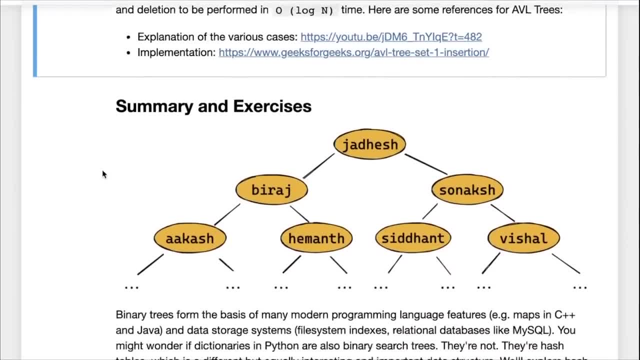 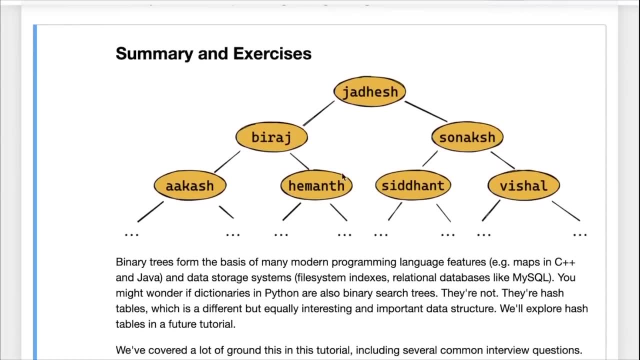 So that makes your data structure very efficient. And with that we conclude our discussion of binary search trees. So here's a quick summary. We we looked at this problem of creating a data structure which allows efficient storage, retrieval and updation also. 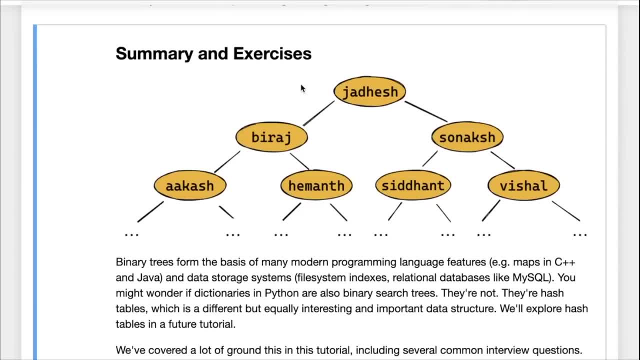 Efficient iteration in a sorted order. We first started out with a list of sorted list of values, sorted by the keys, And we realized that that was probably not the right idea because we are working with really large number of records. Then we created this binary tree structure. 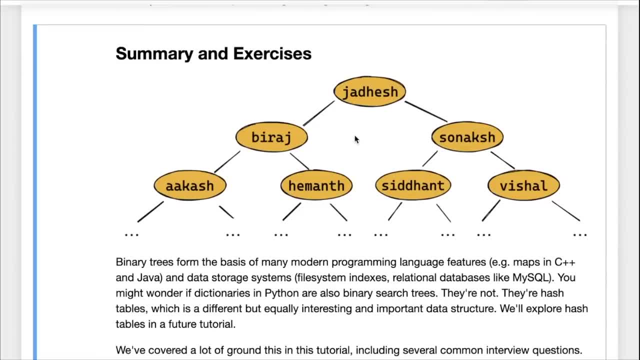 So we looked at binary trees, We looked at how to create them, We looked at easy ways to visualize them, easy ways to create them from tuples. We looked at how to calculate their heights, their sizes, how to traverse them in. In order- pre-order, post-order. 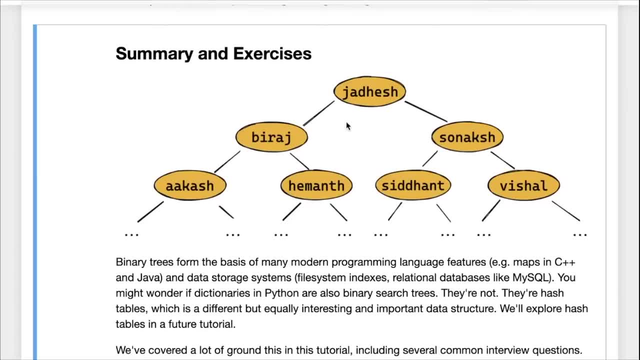 We then looked at binary search trees, which have this property that the left subtree has keys that are smaller than the root nodes keys And the right subtrees keys are larger than the root nodes keys And that property holds at every subtree And that makes it really easy to find, to locate a specific element or find the position to insert an element. 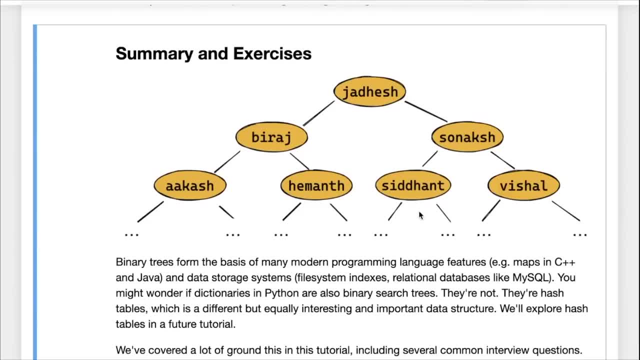 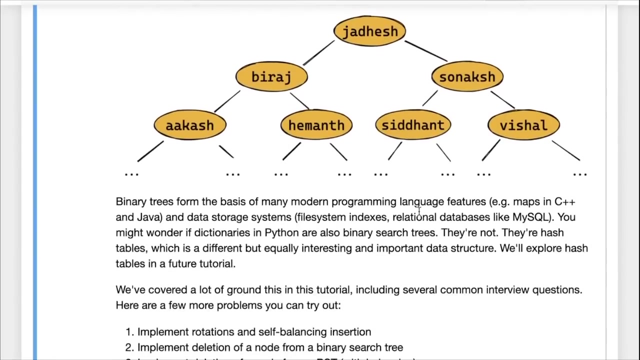 So we created binary search trees. We created the operations Insert, update, find and list, All in a binary search tree. We also determined ways to check if a binary tree is a binary search tree or not. Then we talked about balancing and we saw how to create balanced binary search trees. and binary search trees form the basis of many modern programming languages. language features. 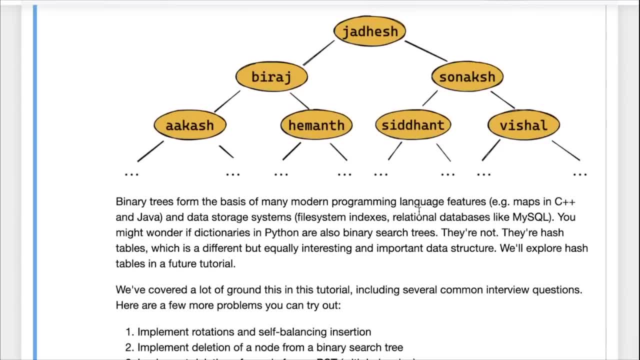 For instance, maps and C plus plus in Java are binary search trees, and data storage systems like file system indexes or relational databases also use something called B trees, which is an extension of binary search trees. So it's very important to know about binary search trees. 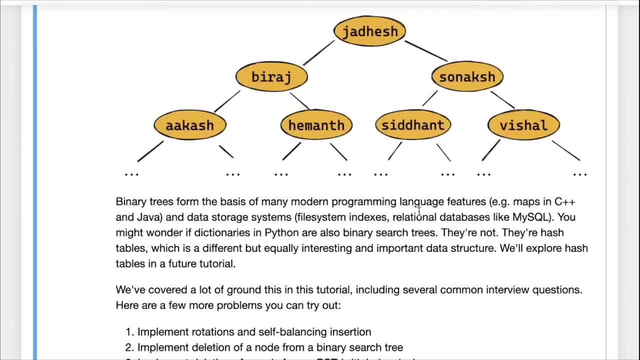 Even if you may not ever need to implement them, you may be asked about them And in many cases, you may need to pick a binary search tree as a data structure for a problem, Like we did in this case. Now you may wonder if dictionaries in Python are also binary search trees. 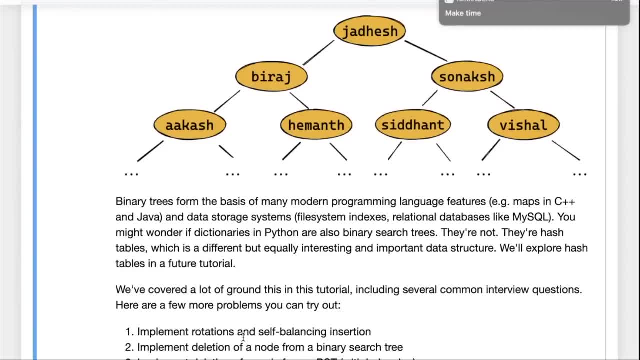 Well, they're not. dictionaries in Python are not Binary search trees. So we'll soon release an assignment that you can find on the lesson page and you will work on hash tables in the assignment. And here are some more problems that you can try out. 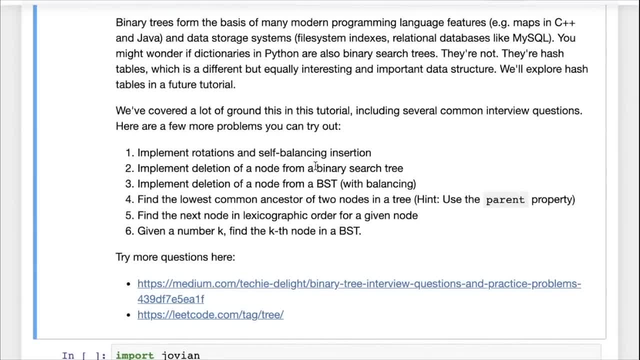 So you can try to implement rotations and self balancing insertion. You can try to implement the deletion of a node in a binary search tree. That's slightly more complicated, because what do you do if you have to delete a node that has both left and right subtree? you can try deletion with balancing. 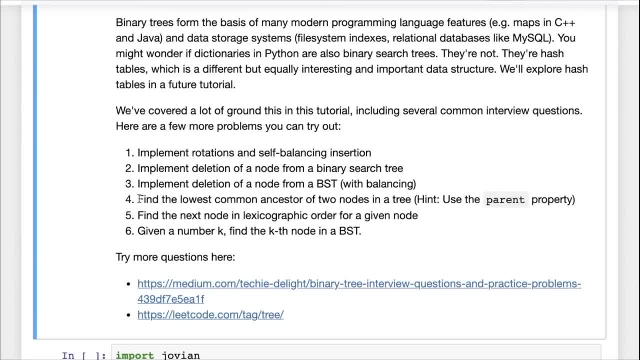 Yeah, Yeah, Yeah, Yeah, Yeah, Yeah, Yeah. If you really are up for a challenge, here are a couple more. finding the lowest common ancestor of two nodes in a tree, So the common node which is as common parent of both nodes. here you can use a parent property. finding the next node in lexicographic order: 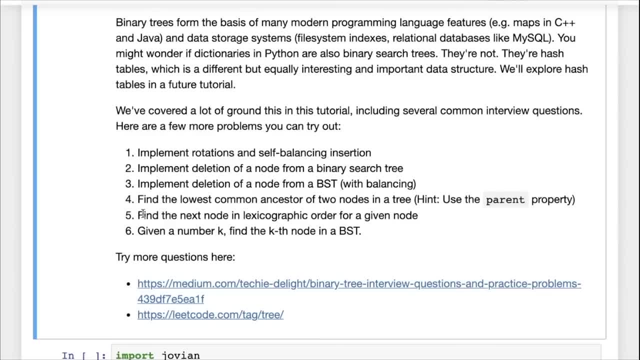 So, given a node, how do you find the next node? What's its complexity? or given a number K, how do you find a K node in a binary search tree? So to do this you will have to employ some clever tricks. And then there are a couple more resources here. 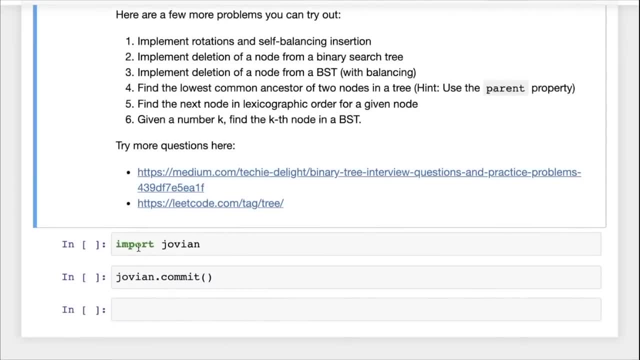 You can open up these and find more questions. The important thing to take away is that almost all of these will involve some form of recursion, So you will either work with the left subtree or the right subtree, or both, And some of them may also require you to store additional information within the node. 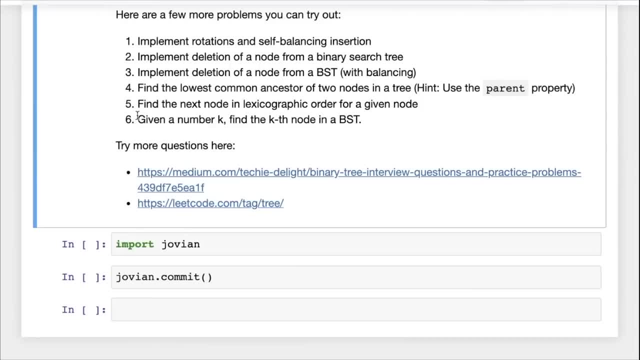 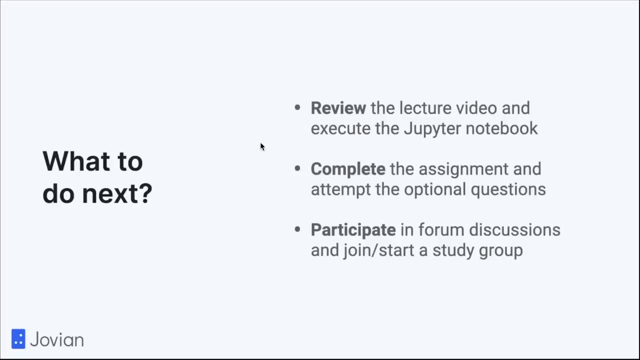 For instance, for uh, for this one, uh, the given a number, K, find the K node. this may require you to store the size of each balanced binary search tree in each. So what to do next? you should review the lecture video and execute the Jupiter notebook. experiment with the code yourself, then complete the assignment. 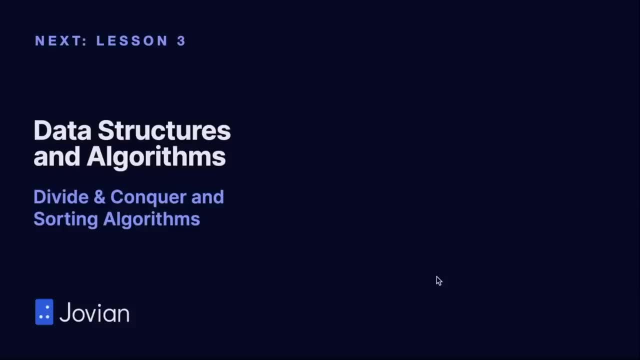 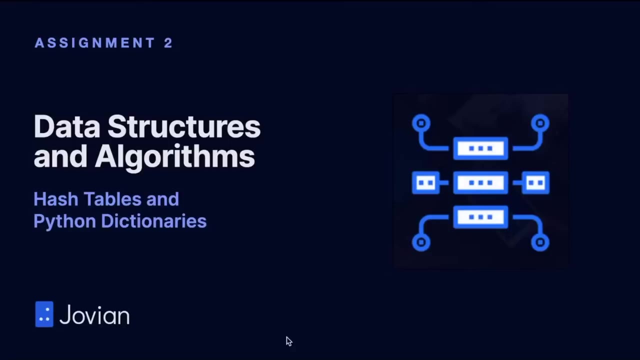 Hopefully the next lesson is called divide and conquer and sorting algorithms. This is data structures and algorithms in Python, and I will see you next time. Thank you And goodbye. Let's look at assignment two of data structures and algorithms in Python, The topic: 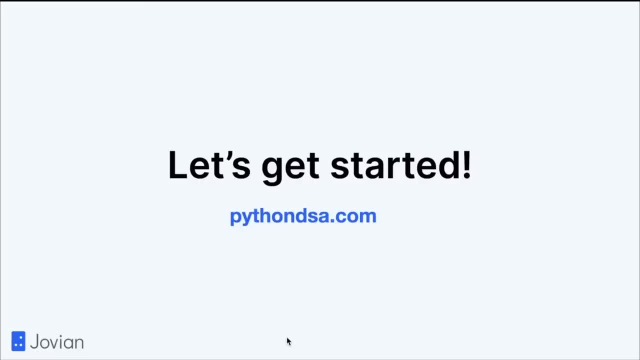 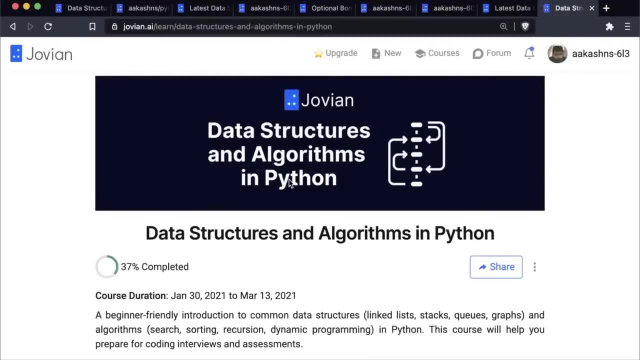 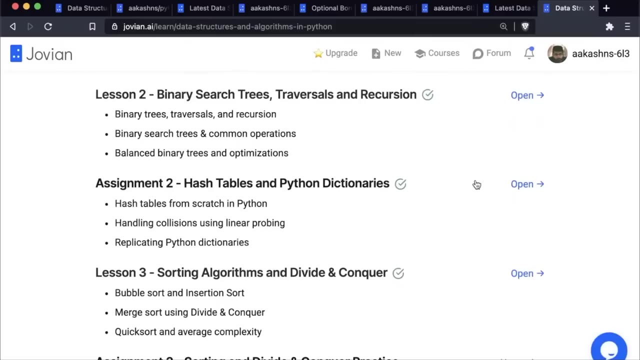 Of the assignment is hash tables and Python dictionaries. Let's get started. The first thing we'll do is go to the course website, python, DSAcom, And on the course website you can find all the lessons and previous assignments. We are looking at assignment two. 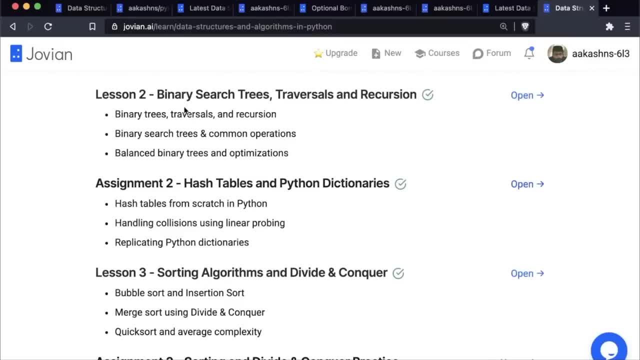 So you may want to open that up. and assignment two is based on or inspired from some of the topics discussed in lesson two, So you may also want to watch lesson two and complete the notebook before You work On assignment two. let's open it up. 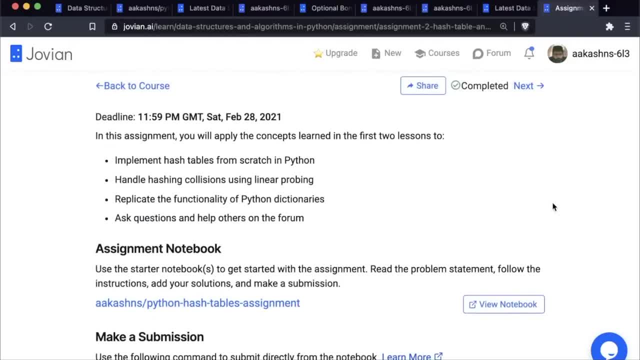 Now in this assignment you will apply some of the concepts learned in the first two lessons to implement a hash table from scratch in Python. That's very interesting. You will, and hash tables are a very important data structure. They present in pretty much every programming language and are a common topic discussed and asked in coding interviews. 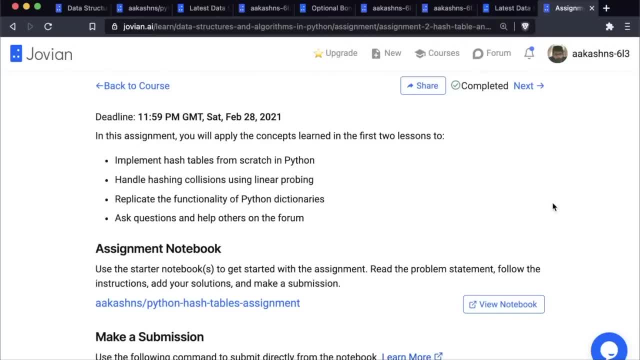 So we'll see how to implement them from scratch. And one of the central problems in hash tables is called collisions. So we'll see How to handle hashing collisions using linear probing, And we will also replicate the functionality of Python dictionary, So Python dictionaries are actually implemented using hash tables. 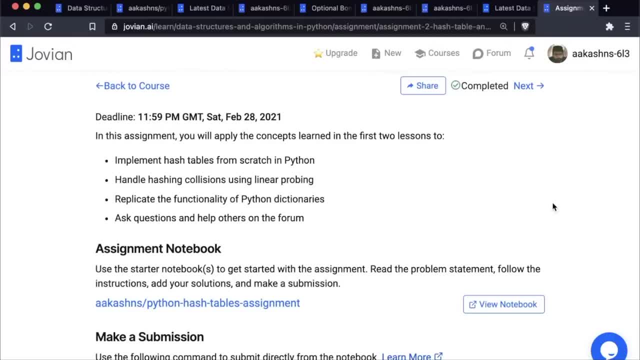 So we'll see how to replicate the way Python dictionaries are created and used and modified and the way we access keys and iterate over keys and set values and change values and so on. So we'll pretty much re-implement The Python dictionary. Now we have an assignment starter notebook here so we can click on view notebook to open up the notebook. 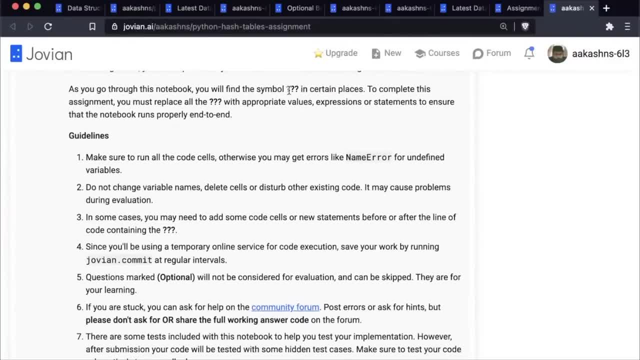 Once again, this is a Jupiter notebook And as you walk through the notebook, you will find question marks in certain places. to complete the assignment, You have to replace all the question marks with appropriate values, expressions or statements to ensure that your notebook runs properly end to end. 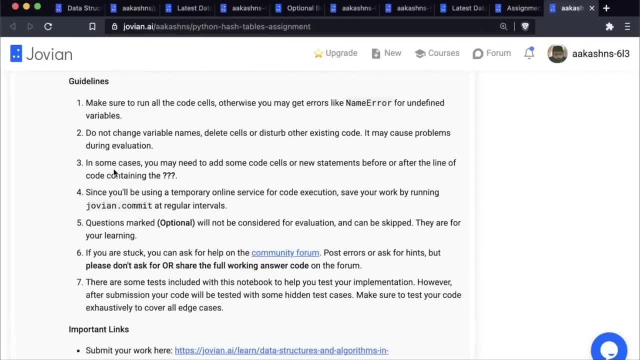 Okay, So make sure that you run all the code cells. Do not change any variable names And in some cases you may need to add code cells or new statements. And, since you'll be using a temporary online service for code execution, keep saving your work by running joviancommit at regular intervals. 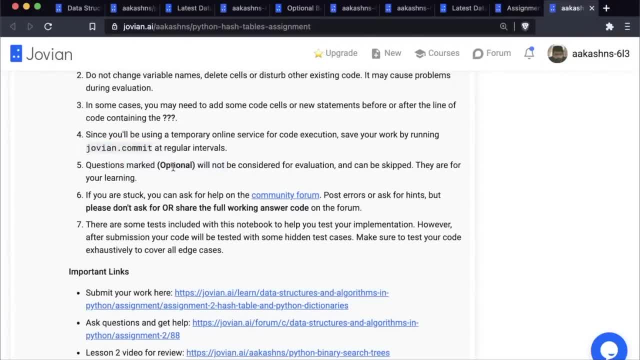 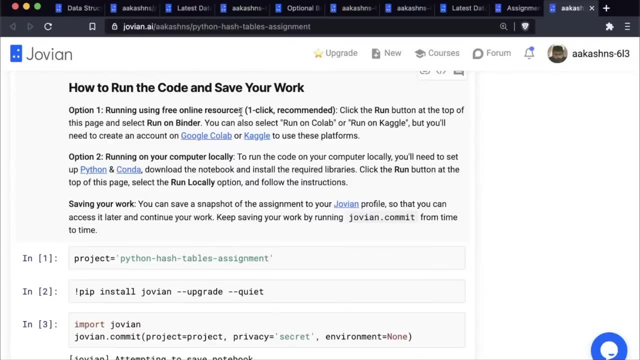 There are some optional questions. They are not considered for evaluation, but they are for your learning. Okay, So let's run the code. Other recommended way to run the code is using free online resources, binders specifically, but you can also run it on your computer locally. 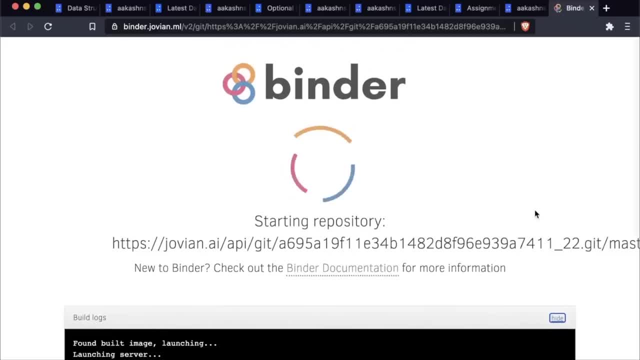 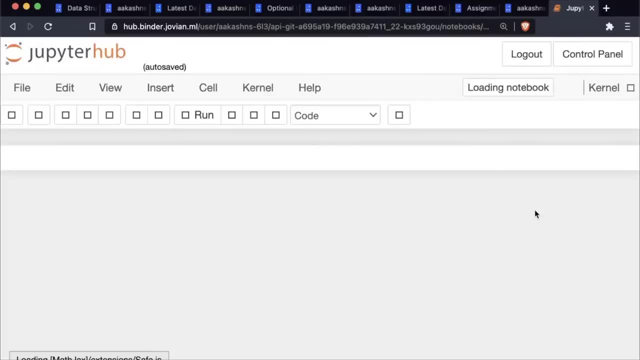 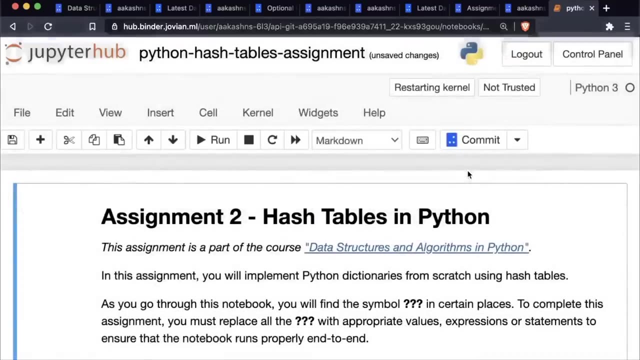 So we're going to click run and click run On binder. Once again. this may take a few minutes sometimes depending on the current traffic on the platform that we have it. Now we have the Jupiter notebook running. The first thing I like to do is click colonel and restart and clear output so that we can execute all the code cells and see their outputs from scratch. 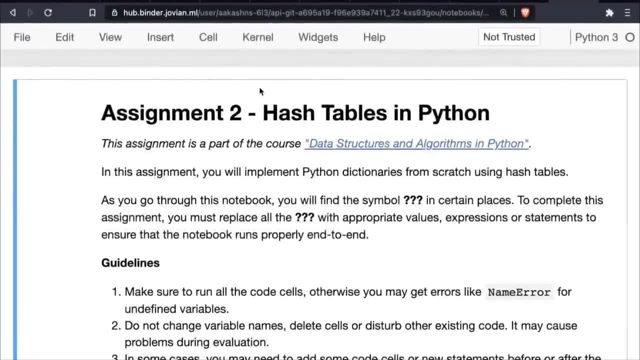 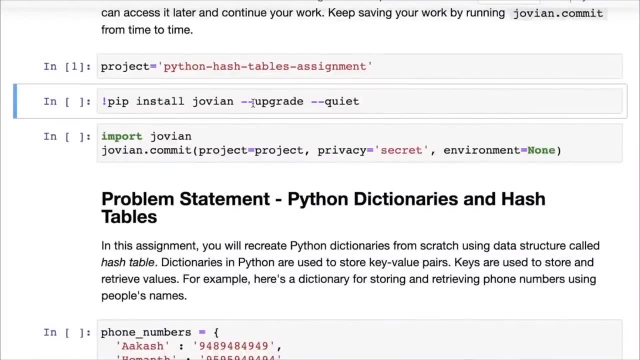 Most are going to hide the header and the toolbar and zoom in here a little bit so we can see things a little better. The first thing we will do Is set a project name, import the Jovian library and run joviancommit. 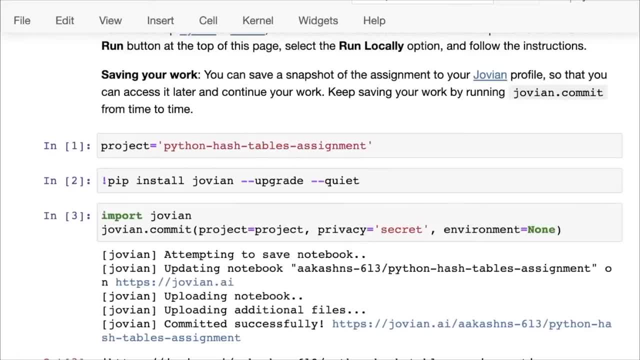 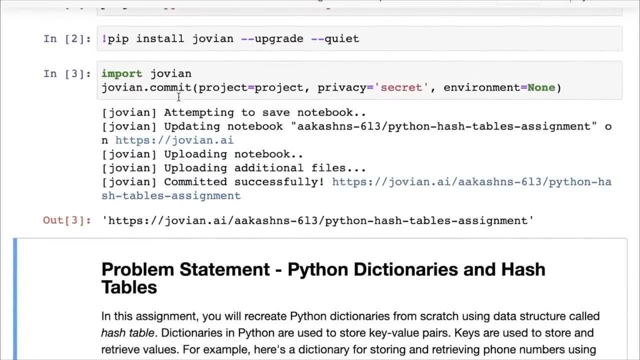 This will allow you to save a snapshot of your work to your Jovian profile. So now you have a copy of the assignment starter notebook. any modifications that you make every time you're on Joviancommit will get saved to your personal copy. 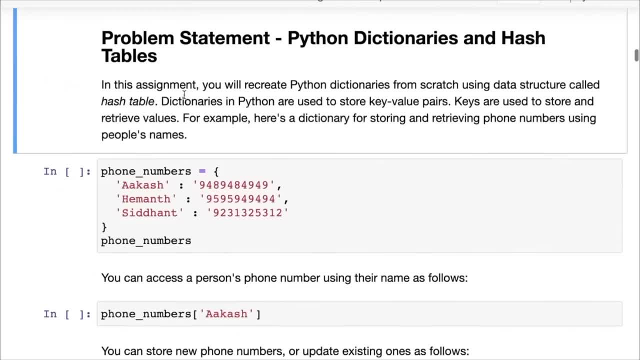 And it is this personal copy that you will submit at the very end. So let's talk about the problem statement. in this assignment, you will recreate Python dictionaries from scratch using a data structure called hash tables, and dictionaries in Python are used to store key value pairs. 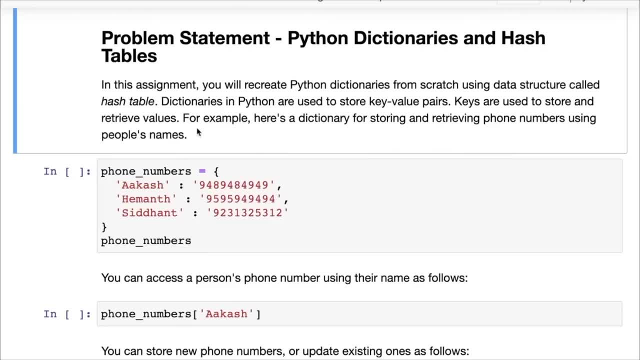 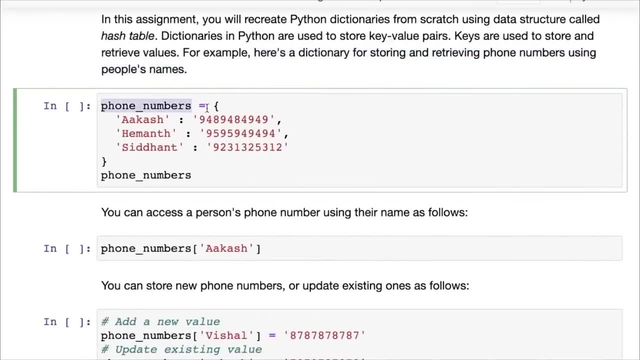 So keys are store, used to store entity values, And here's an example. here's a dictionary for storing and retrieving phone numbers using people's names. So we have a dictionary called phone numbers, and the way you create a dictionary is using this special character, the brace, or the curly bracket as it's called. 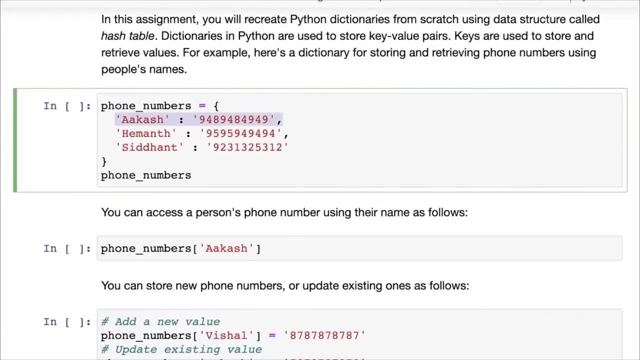 And then in a dictionary you have these key value pair. So this is one key value pair where you have a key. The key in this case is a string, Akash- and here you have a colon, and then here you have a value. 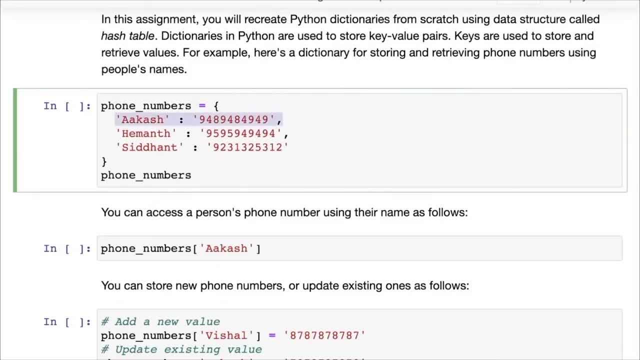 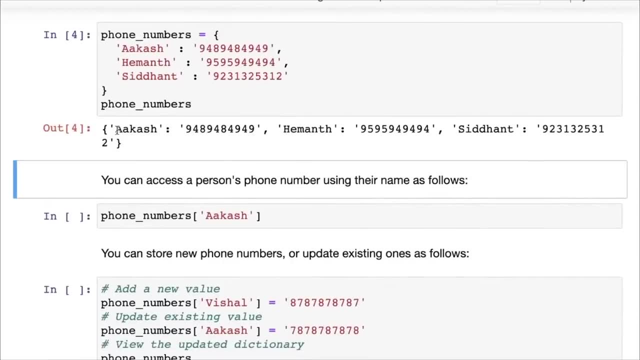 The value in this case is a phone number. So that's how you create a key value pair and comma separated key value pairs is what you need to create a dictionary You can see. once the dictionary is created, it is displayed in the exact same way. 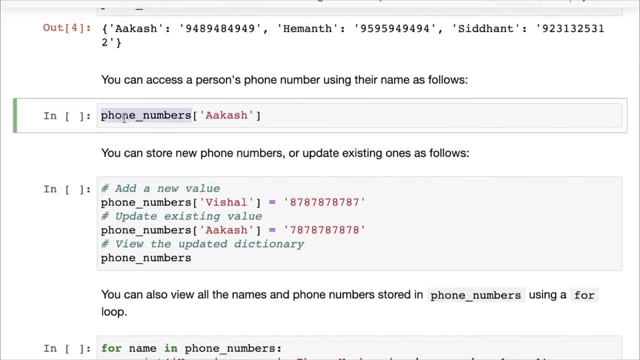 And then you can access a person's phone number using their name. So if you have the variable phone numbers and we use the indexing notation- So this is The square bracket- and we pass in a key here, we get back their name. and you may wonder what happens if the key is not present. 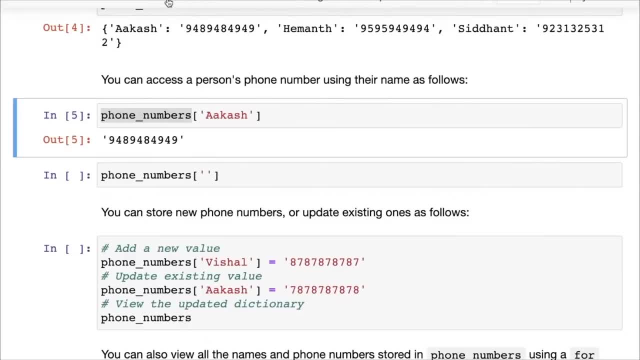 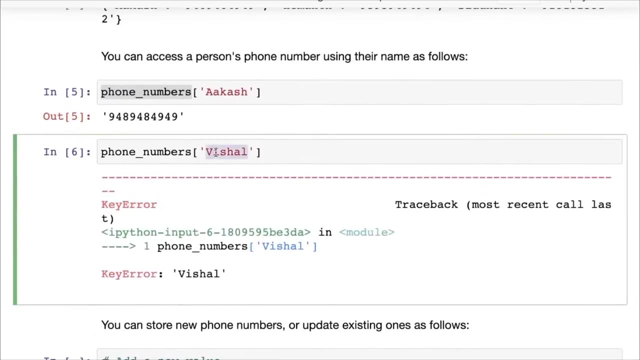 The great thing about Jupiter is you can insert a new cell like. you can just click insert cell below, or you can use a keyboard shortcut B, as I just did, and check- maybe let's check the key, Vishal, Okay- And you get back a key error and you may also wonder what happens if. is it case sensitive? 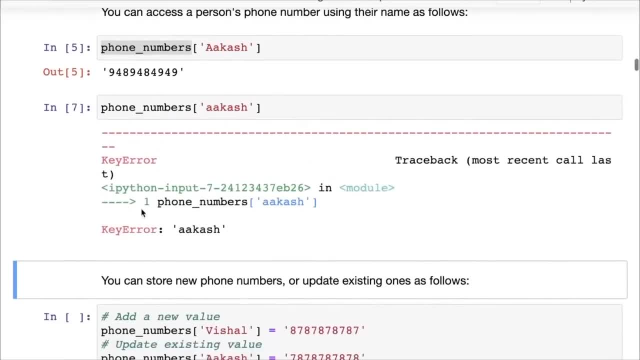 Does that matter. You can check It very easily. So a lot of the questions that you might get, a lot of the questions that you may want to even ask on the forum or look up online, can be resolved simply by creating a new cell and typing out some code. 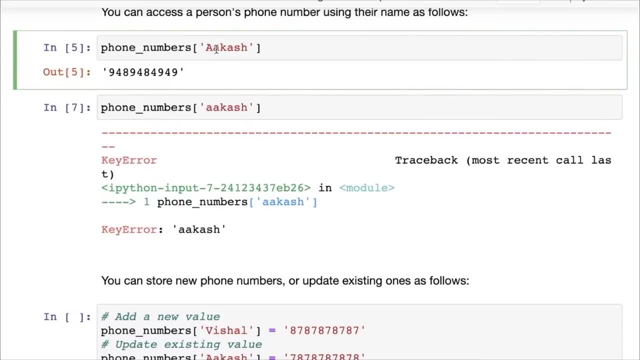 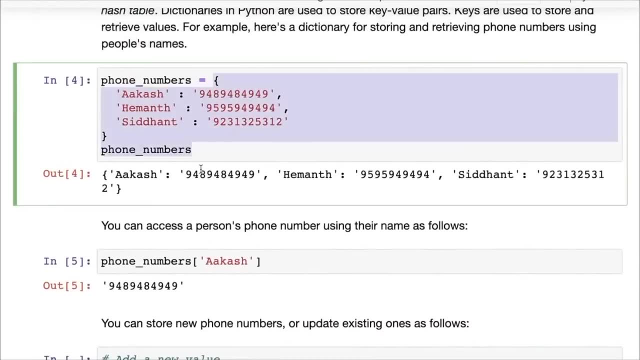 Like what happens if questions can all be answered by writing some code. So now let's add some new phone numbers. So this is how you create an initial set of phone numbers, This is how you access a phone number and this is how you add new values. 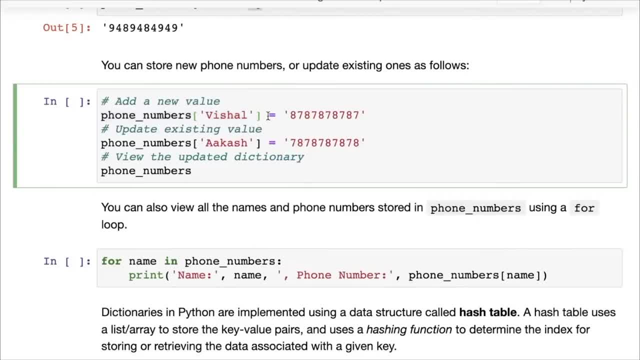 So adding new values is like accessing them, But instead of accessing it you put an equal to and then you actually set the value here. So we can add a new value here- the phone number for Vishal- and we can also update an existing value in a dictionary simply by accessing that value and putting an equal to and putting in a new value there. 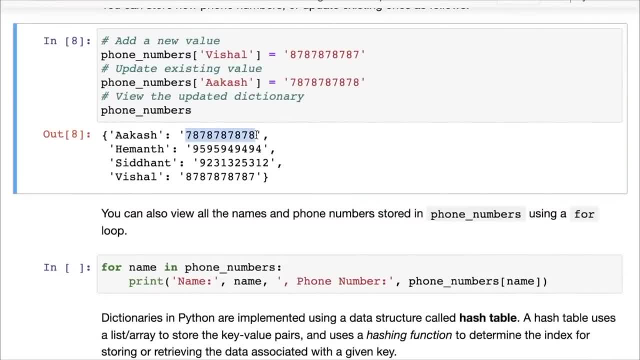 You can see now that the dictionary is updated to contain the new phone number 7, 8, 7, 8, and not the original phone number 9, 4, 8, 9, 4, 8.. 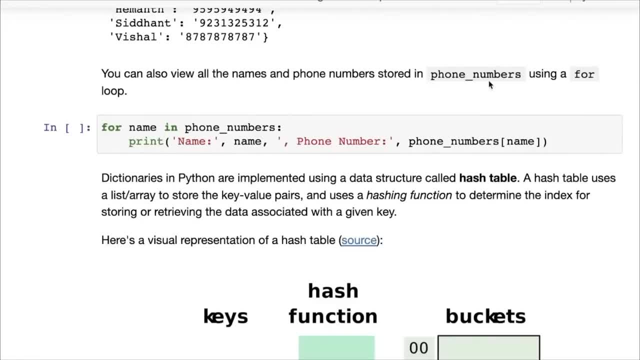 You can also view all the names and phone numbers stored in the Phone number dictionary using a loop So you can say for for name in phone numbers. So when you put a dictionary into a for loop you get back a key within each loop. 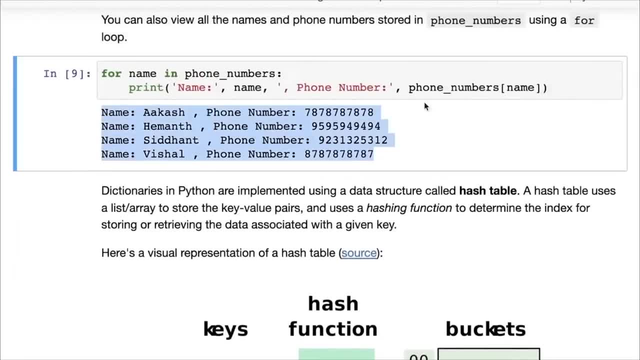 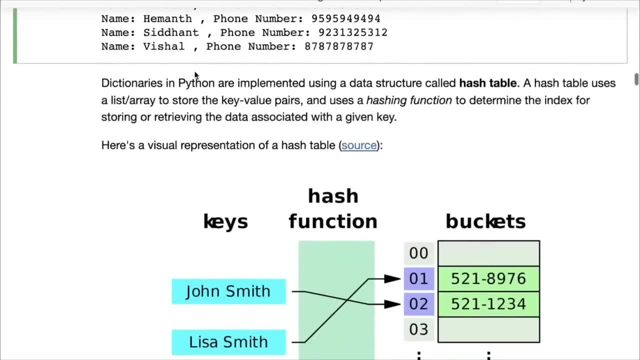 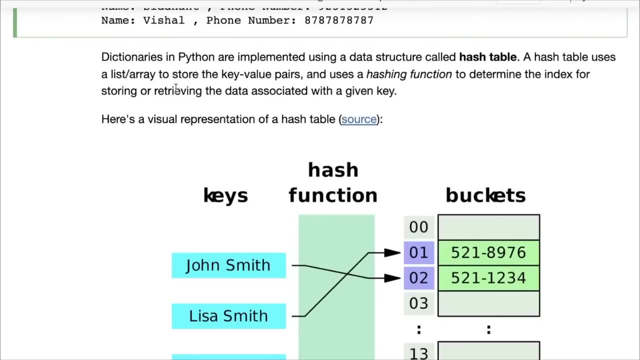 You can see here that the name and the phone number is displayed for you using the print statement. So those are some things that you can do within a dictionary, and dictionaries in Python are implemented using a data structure called a hash table, and a hash table uses a list or an. 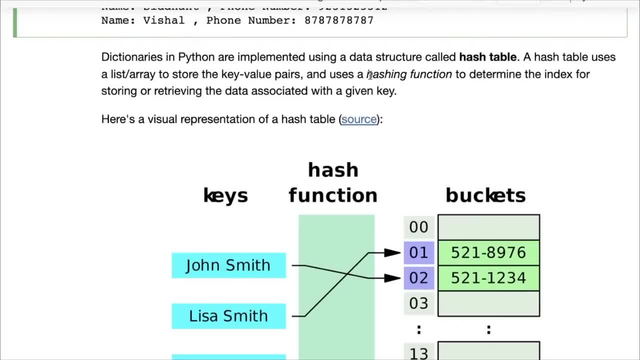 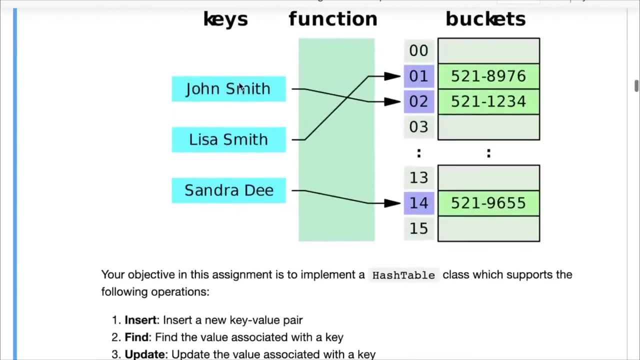 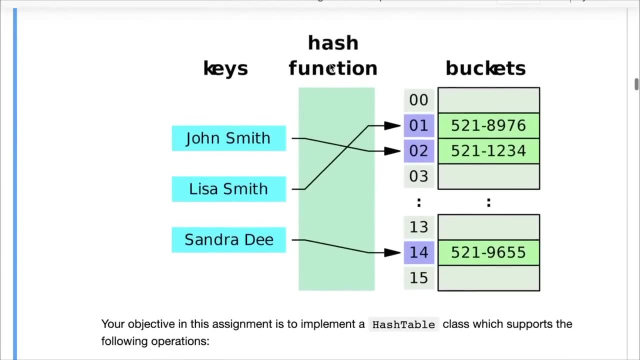 array to store key value pairs And uses a hashing function to determine the index for storing or retrieving the data associated with a given key. So here's what it looks like. here You have the key, John Smith, and you have a function called hash, and the function hash takes any key and it returns an index within the list. 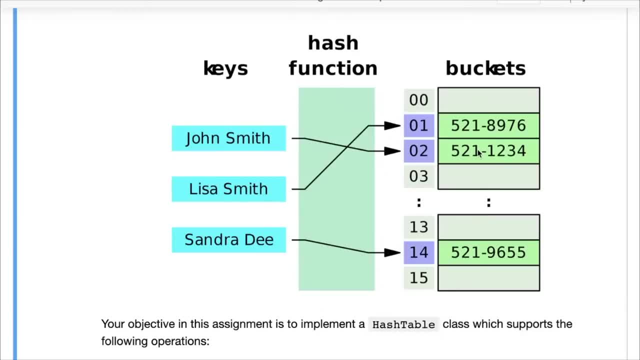 So why do we use a hashing function? Well, one approach, as we've discussed in lesson two, is we can store Okay Key value pairs in a list and we can simply search through the list each time we want to look up the value for a key. but that is inefficient because that requires looking through potentially all the keys before we get to the key that we want, or maybe half of the keys. 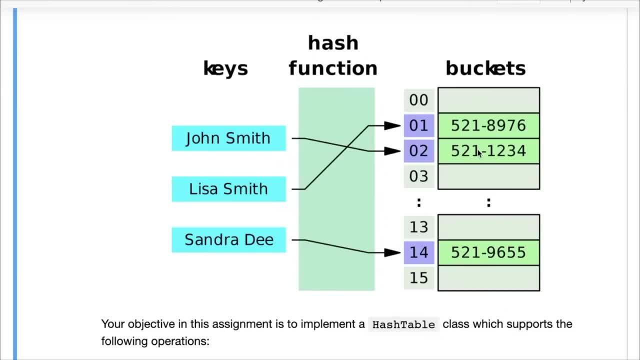 So that makes it an order N operation. If N is the size of the list, that's pretty inefficient. We want something faster and a hash function actually operates in constant time. So hash simply takes the key And it converts a key into a number. 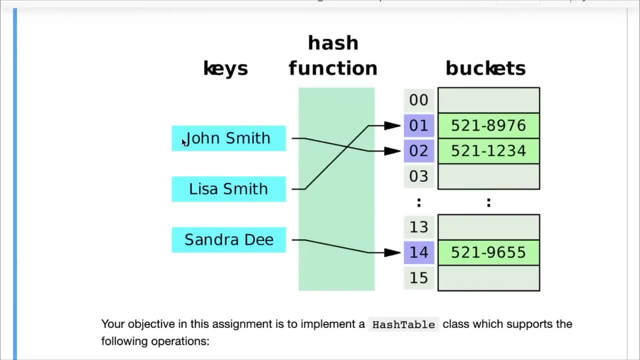 So in that sense, it gives you the index of the specific key value pair in constant time rather than ordering, And that is what makes hash table So efficient, right? So hash function does not require looping through the list. It simply takes a key, gives you the index and you can simply then get the key value pair or the value from that index. 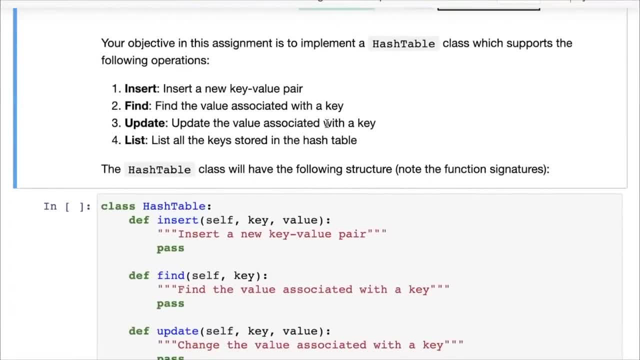 Now, your objective in this assignment is to implement a hash table class Which supports these operations and insert operation, a way to insert a new key value pair. a find operation to find the value associated with a given key. and update operation to update the value associated with a given key, and then list operation to list all the keys stored in the hash table. 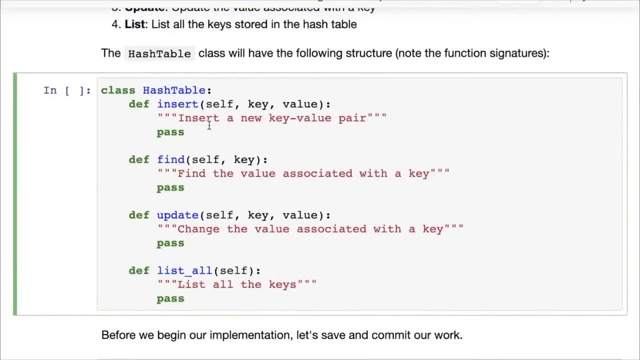 And here's where we are going to use Python classes. And there's a brief introduction to Python classes in lesson two of this course. So do check out lesson two If you want a refreshing on Python classes. we have the class hash table and inside the class hash table you have a bunch of methods. 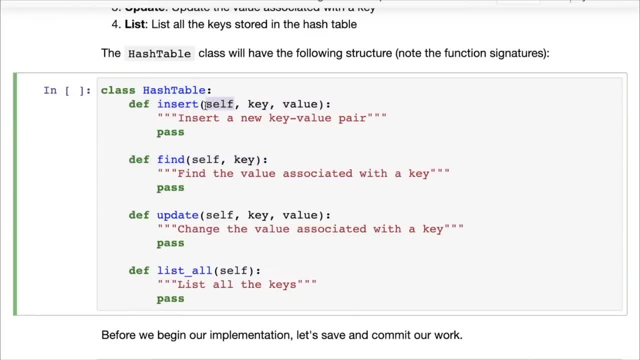 Now the insert method, apart from taking the self argument- and remember that the self argument is- refers to the object of the class that will be created. So this is equivalent to the this variable in Java or C plus. but these are the actual arguments. 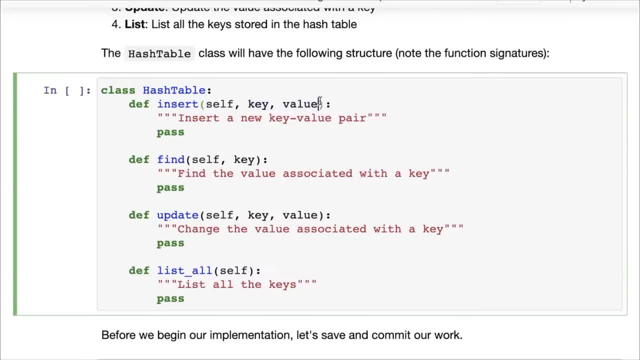 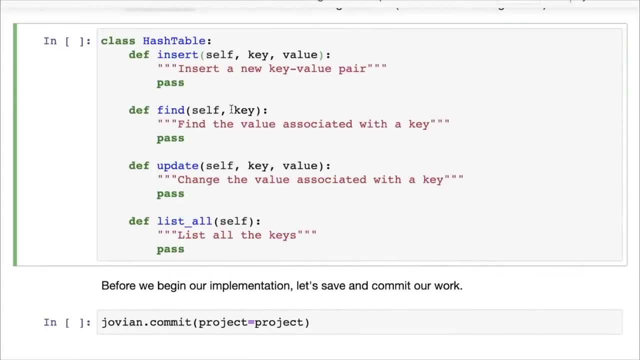 Of the method. the actual arguments are key and value. So the insert function or the insert method will take key and value. Then the find method will take a key. The update method will take a key and value once again. So the fine method takes a key and your job is to return the value. 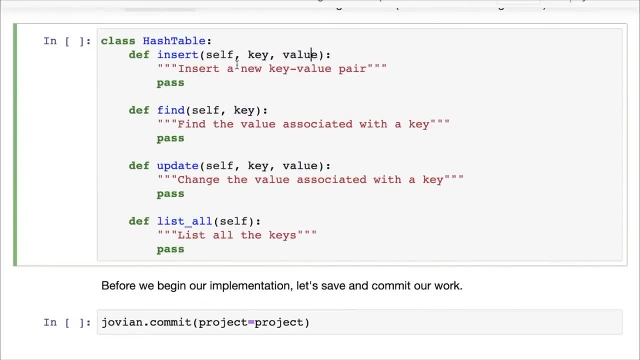 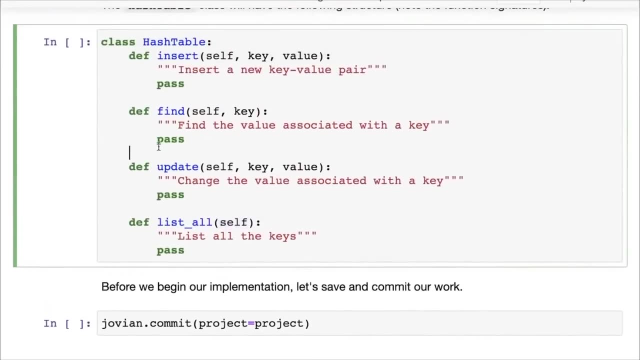 Insert method takes a key and value and you insert the key value pair into the hash table. Then you have the list all method which is used to list all the keys from the table. before we begin our Implementation, Let's just save and commit our work. 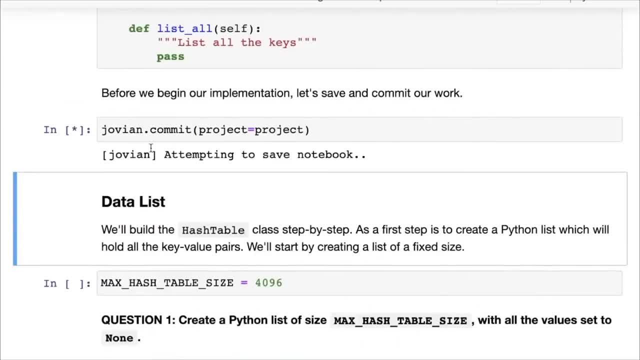 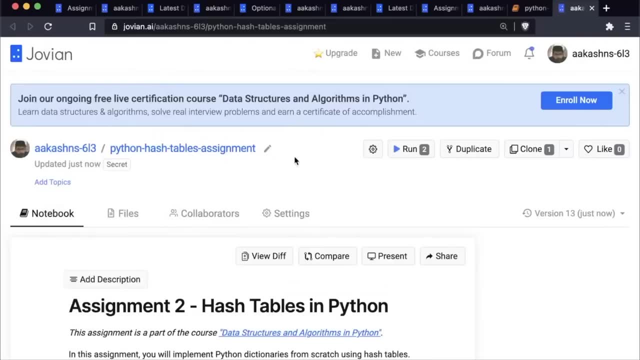 So we're running Jovian dot commit here. Let's just run that once again. there we go. The notebook has now been committed, So what you can do is you can come back to this particular page and you can find this from your profile, and then you can click run to continue your work based on the modifications that you've already made. 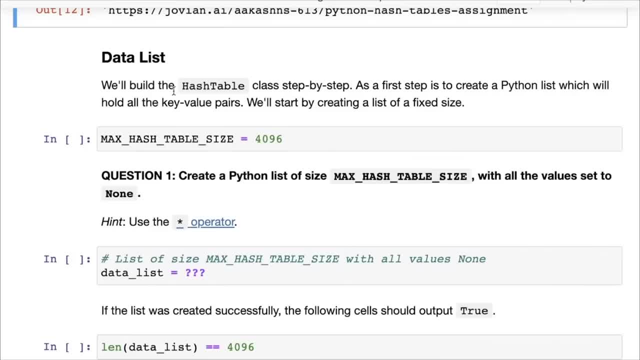 Okay, So we build a hash table class step by step, And the first step Is to create a Python list Which will All the key value pairs. Now remember that a hash table internally uses a list to store the key value pairs and we will create a list of a fixed size. 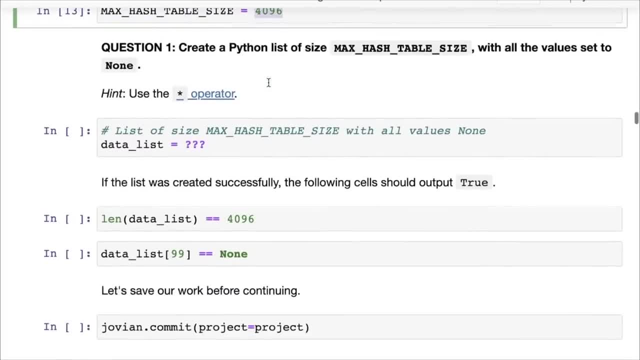 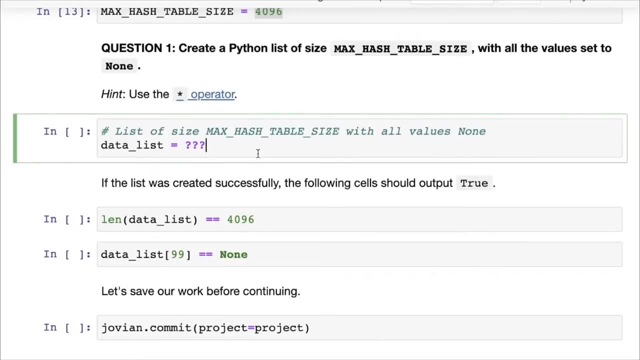 So we'll set this variable max hash table size of size four zero nine six initially, And we are going to create a Python list of the size. How do you create a Python list of the size And we want all the values to be set to none? 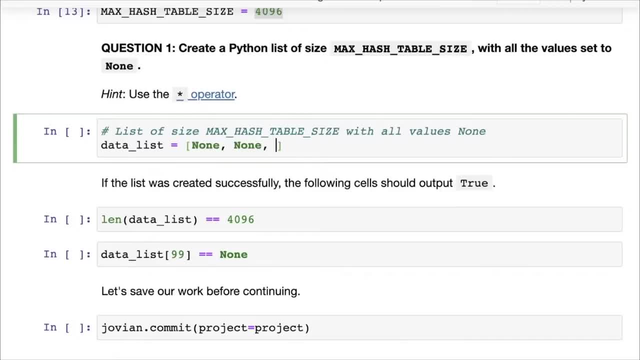 So this is the way to do it. You can, of course, you can start typing none, and that would take a long time, Or you can use a simple technique: just put in none times four, zero, nine, six, and there's one of the great things about Python. 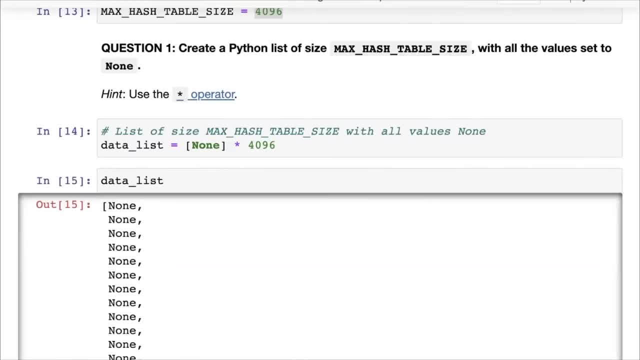 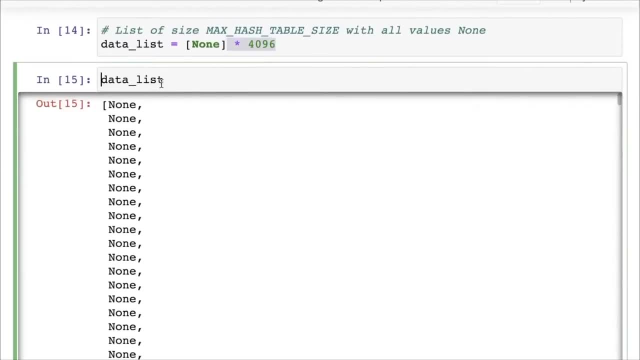 It is such an expressive language that creating a list of 4,000 elements simply requires this single expression. here You can check that. here You can even check the length of the data list. Now, if the list was created successfully, here are some test cases. 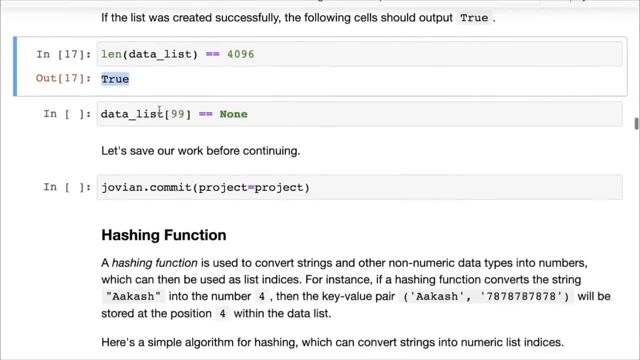 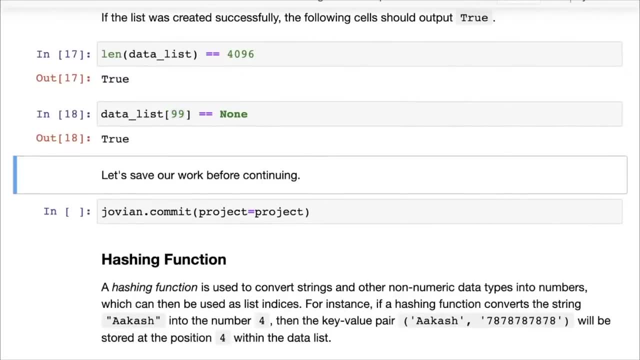 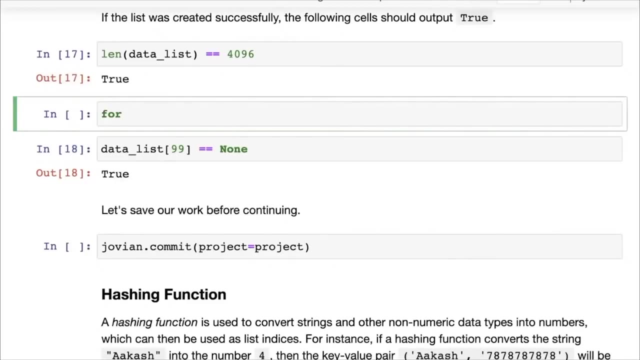 Here is one check that the length of the list is four zero nine six. Here's another check and we're simply picking a random value from the list 99, and just checking if that is equal to none. but if you really want to have a a short, short test here, what you should be doing is you should be checking for item in data list. item equals none. 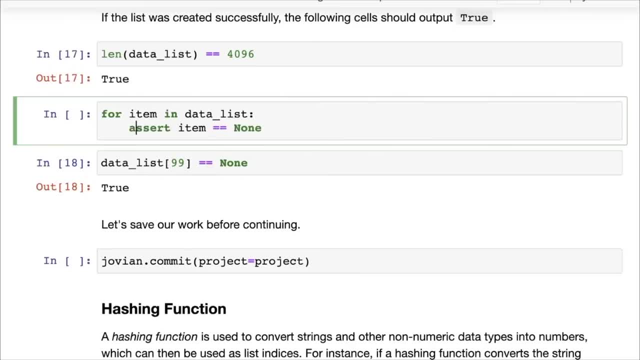 Okay, And here's a trick you can do. You can write a word called assert, and what assert does is: if this comparison Is true, then it does nothing. It lets your code proceed as usual, but if at any point this comparison becomes false, then it throws an error. 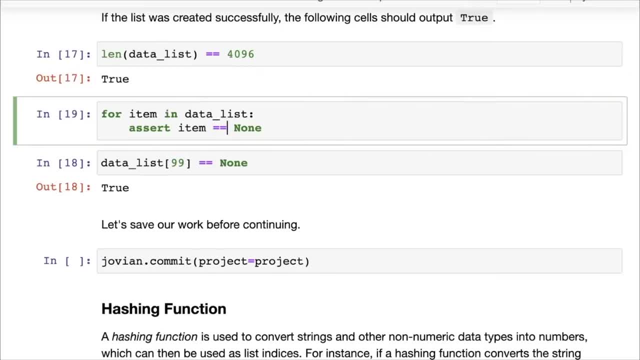 So let's see here, you can see here there was no error. So that means it worked fine. but if this comparison was wrong, so let's say if item, if he had here, we wanted the items to be equal to seven. if you put it and and he tells us does not contain the item seven at certain position, then you will get in. 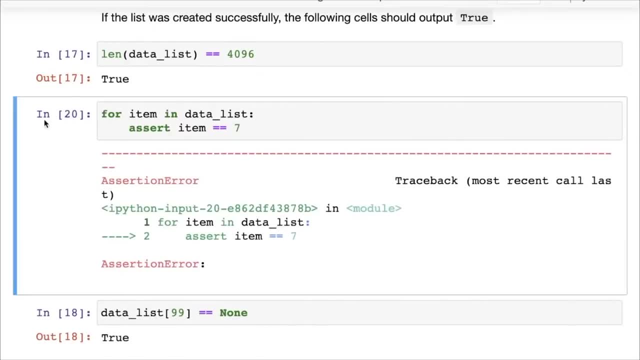 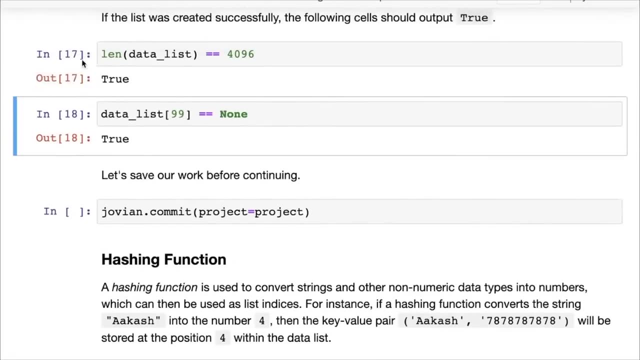 Assertion error here. Okay, This is how you can create your own test cases by putting in assert. But the idea here is that, whatever you try to do, make sure that you're adding some more test cases and not just depending on the test cases that are given here. 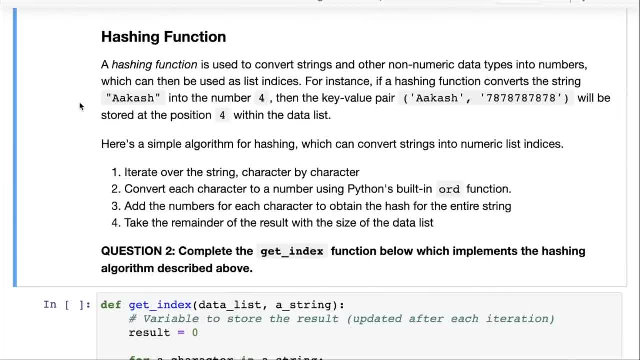 These are simply to guide you in the right direction. Okay, So next up, we have a list. Now we need a way to store or insert key value pairs into a list. That's where the hashing function comes into picture. The hashing. 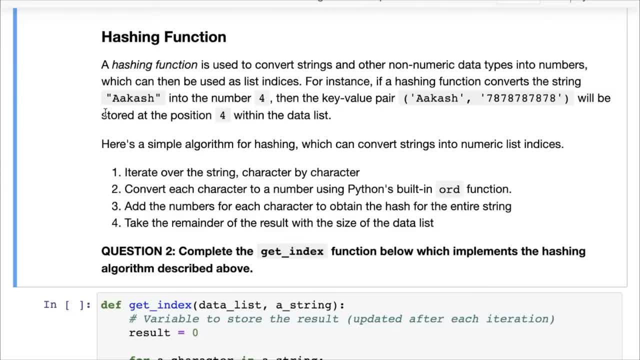 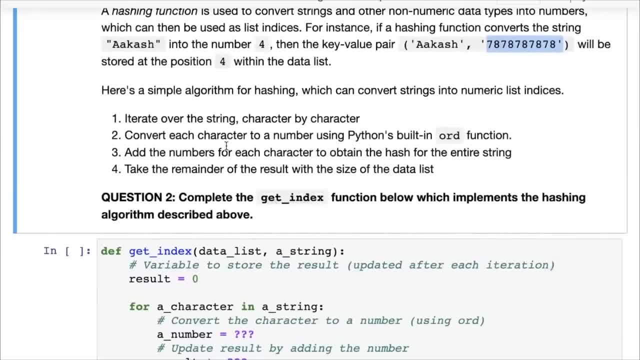 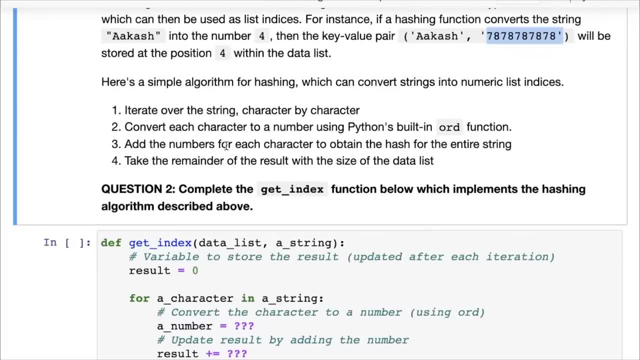 And here's a simple algorithm for hashing which can convert strings into numeric list indices, and a hashing algorithm does not have a single definition. You can come up with a hashing algorithm, And in fact, coming up with a good hashing algorithm is an area of research in itself. 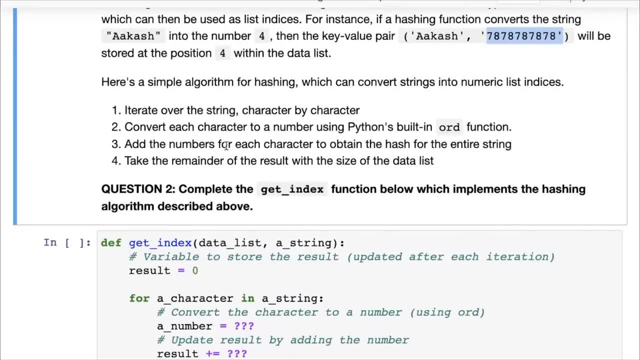 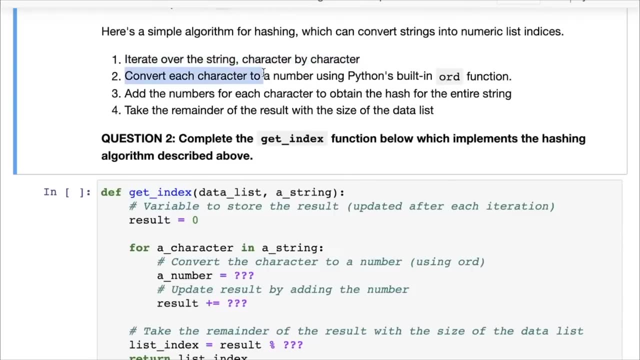 Now, of course, Python dictionaries use hashing. that is inbuilt into Python and that's a fairly optimized hashing algorithm. That's probably the result of several years of research. but here's one very simple technique: We iterate over the string character by character, and then we convert each character into a number using Python. 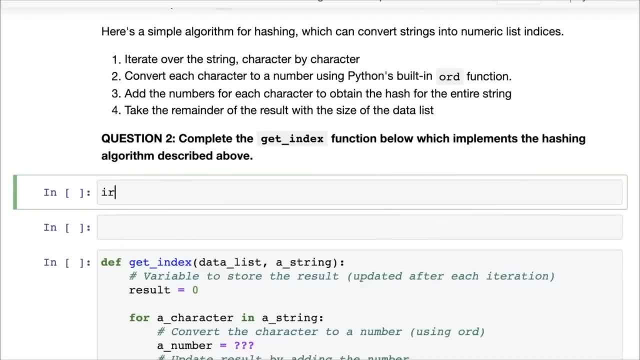 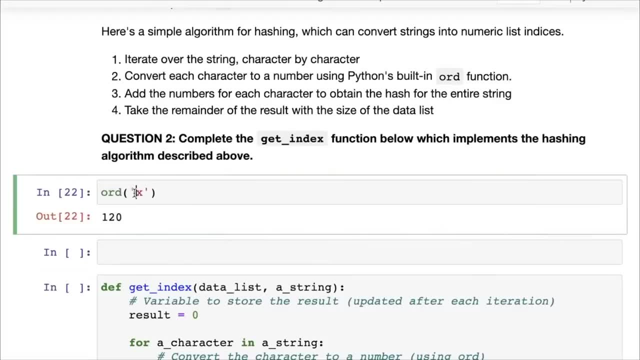 Now, Python is built in ORD function And you can see here that if you call ORD on a character X, you'll get back a number. It already gives you a way of converting characters into numbers, but not entire strings. That's why we need to iterate over the string character by character. 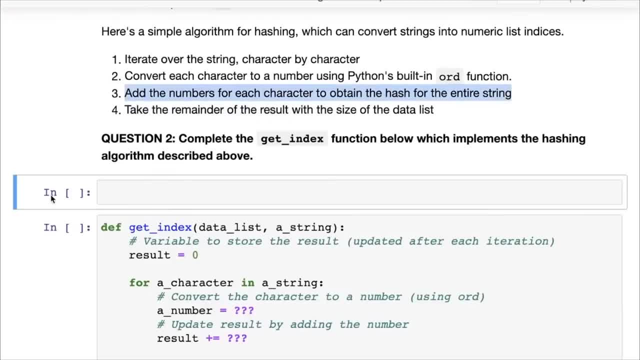 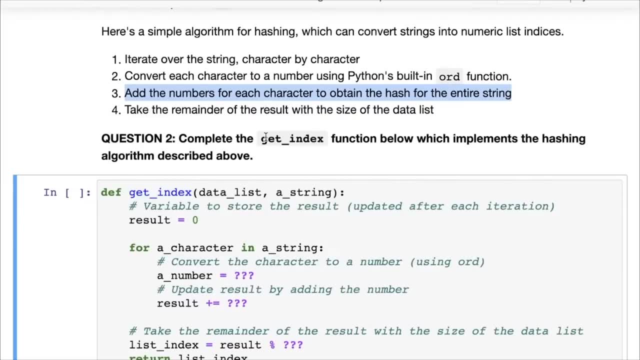 Then we simply add the numbers for each character to obtain the hash for the entire string. It's a very simple technique. We just keep: if you have the number Hello, We take the odd for hello. The odds for either. odds for L. 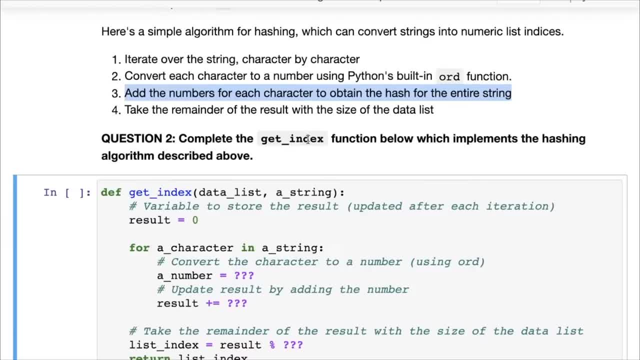 L and the odd for O and add them together. And since we want that number, the final result, to be an index or a position within the list, so we take the remainder of the result with the size of the data list. So it's possible that once you add the numbers together you may end up with a. 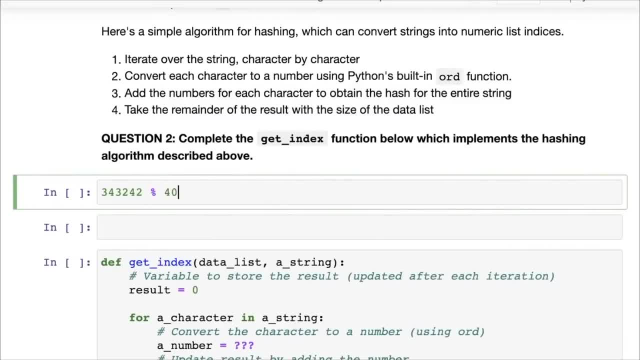 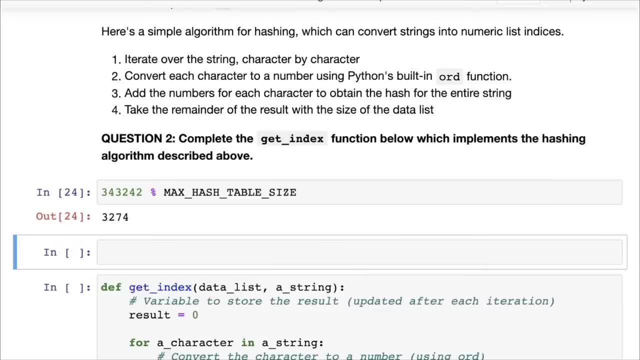 pretty big number. but if you take the remainder with four zero nine six or the max hash table size variable, you get back a number that is smaller than four zero nine six. so you can use just that remain as the index. So let's first define a function called get index. 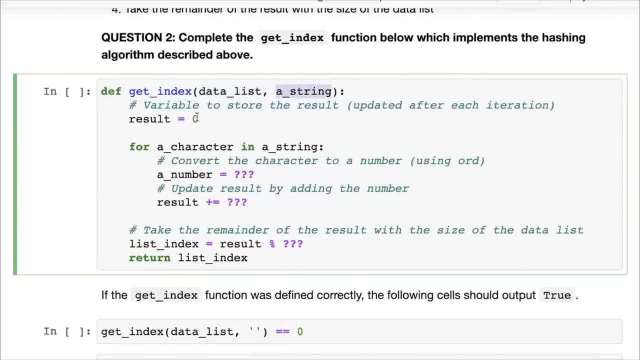 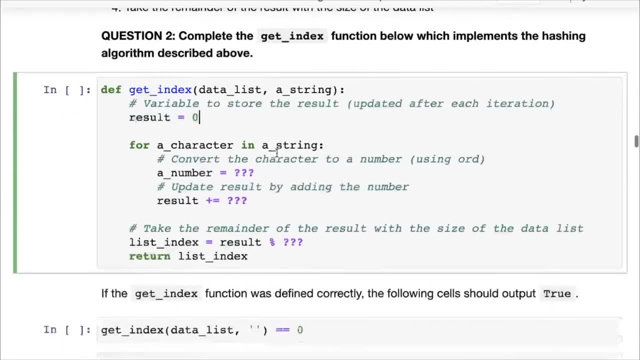 All it does is it takes the data list and it takes a string and it returns. it applies this hashing algorithm to return an index for that string, for that key. So for a character in a string, We need to convert the character to a number. 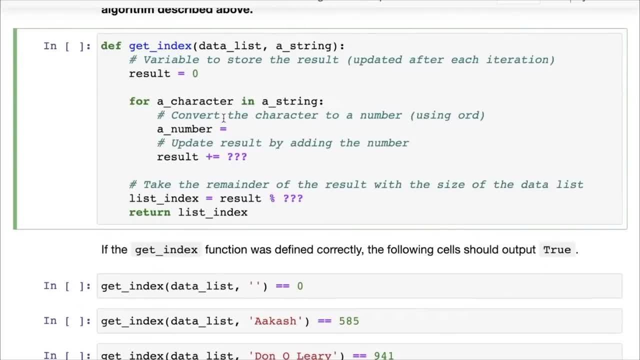 So we convert the character from the string into a number by calling a body on a character, Great. Then we update the result by adding the number. So we say result plus equals a number, pretty straightforward. And that repeats for all the characters in the string. 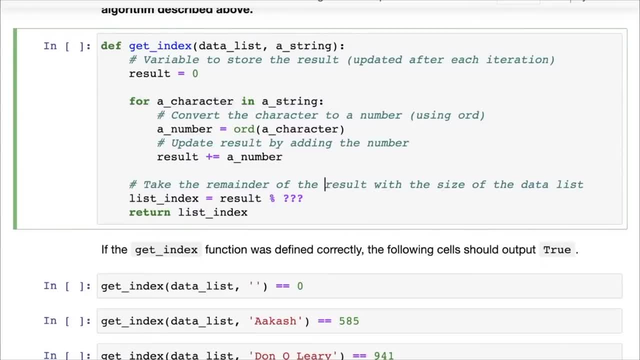 And then we get back the final result. Now, that result may be longer than the actual size of the list, And this is where we were there. We may then want to check the size of the list. Okay, Now remember there's one. no, I could also have probably written max hash table size here. 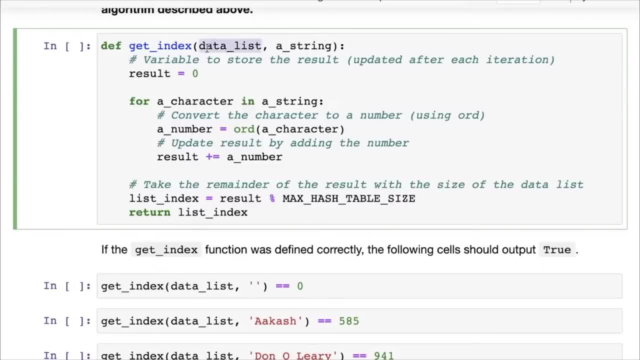 but that would be wrong, Isn't it? Because we are passing in a data list here We are passing in a data list, And although we have so far created it in data list of size four zero nine six, your function should ideally be you looking at the size of the data list that you have. 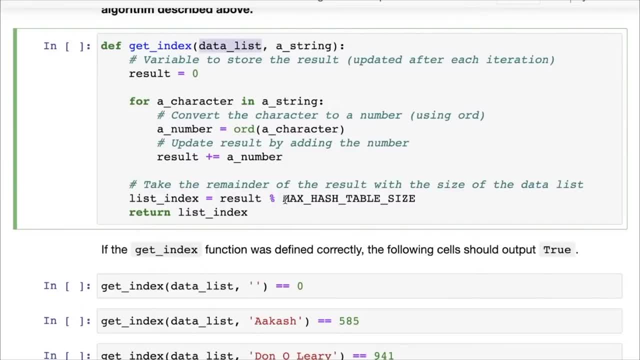 And not any global variables. So keep that in mind, And the right thing you should check here is land data list, And what this will allow is now: this will allow your function to work with data lists of different sizes, not just the standard size- four, zero, nine, six- that we have defined above. 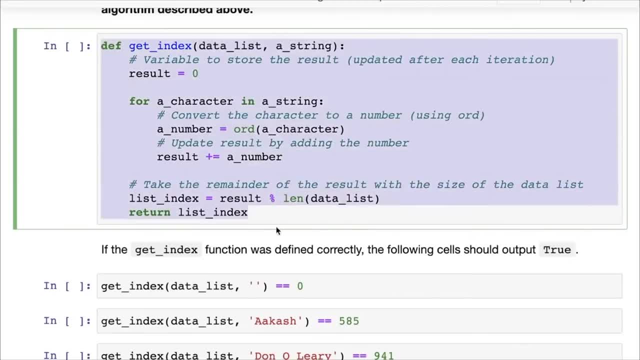 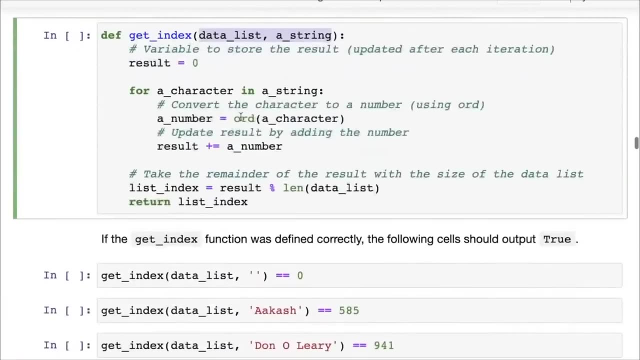 Okay, Very important thing: Always make sure that your functions use the arguments that are passed into them, that they are generic, that they can work with any input And not just a particular input. that have been that has been defined earlier. Okay. 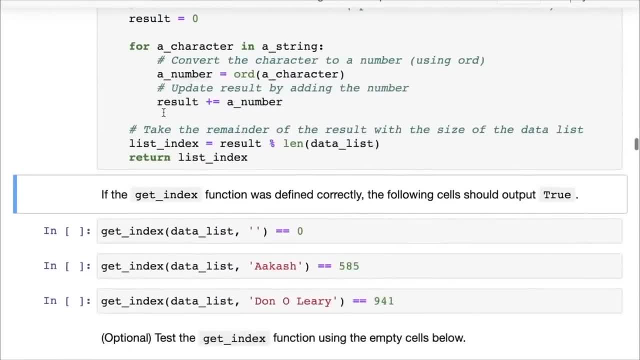 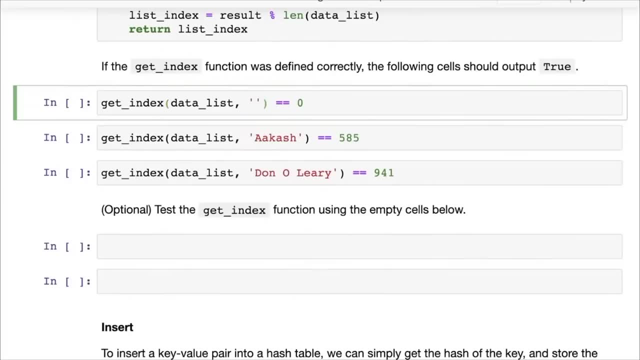 So there you go. Now you have. this is a function, get index that has been defined. And here are some tests. Now, if you pass in the data list and you pass in the empty string because there are no characters, the result is likely to be zero. 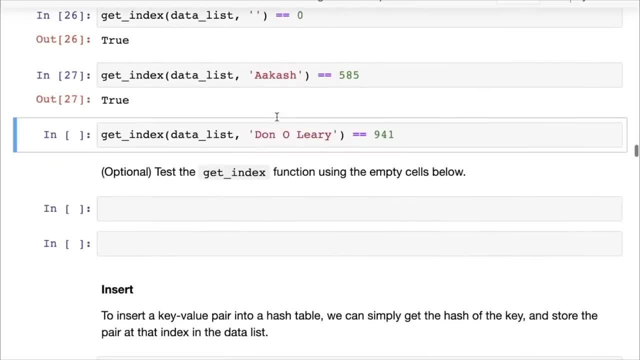 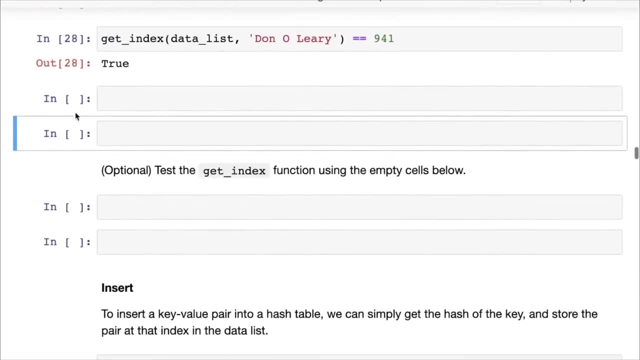 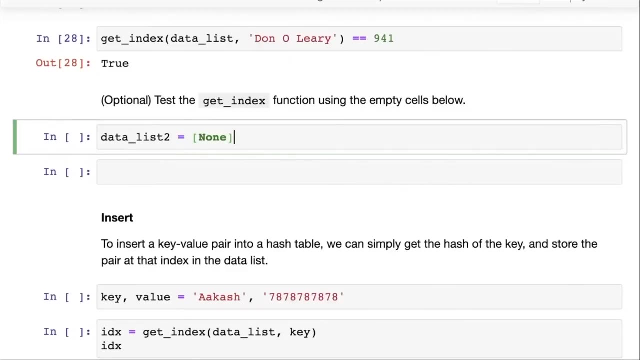 Great. Here's another one. The result here is five: 85.. Here's another one. The result here is nine: 41.. Great. Now This is where you should be testing your function with some custom test cases. I'm going to create a new data list too, and this is going to have the size none times 48.. 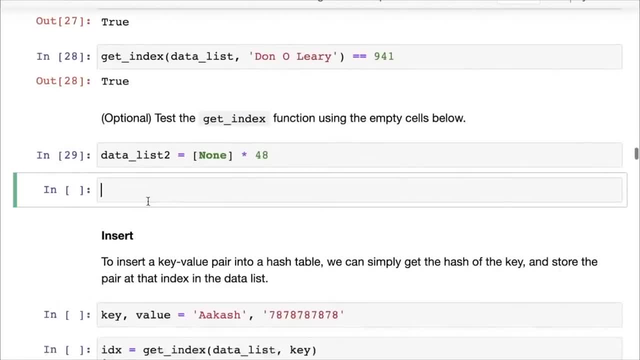 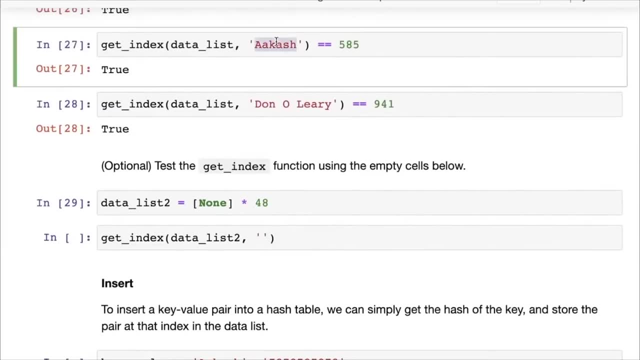 So there's only going to have the size 48 and I should be testing get index with this data list as well. So let's say we're looking at the key Akash, Now we know that. let's see, we can actually test this out here. 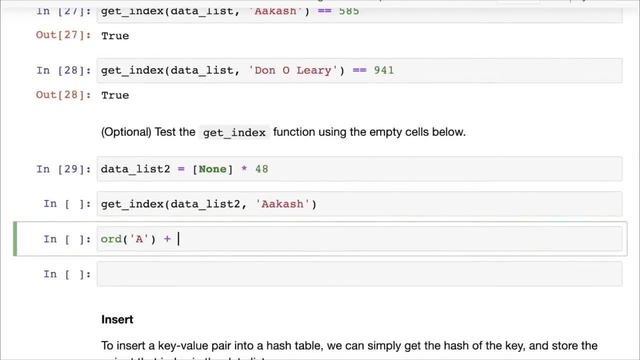 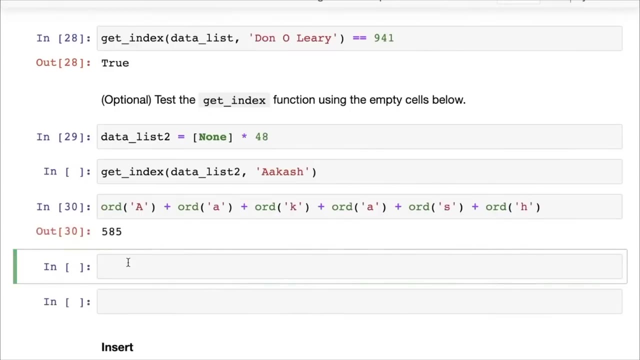 What happens If you add ORD of a plus ORD of a plus K, a, S and H, that number is five, 85.. But since the size of the list is 48, what we should be getting back as the result is 48 divided by 585.. 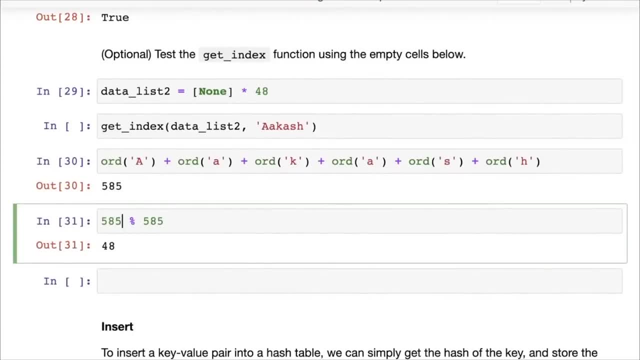 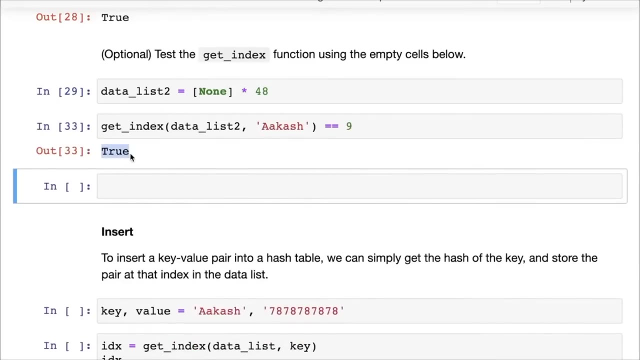 So we should be getting, oh sorry, five, 85 and it's remainder with 48.. We should be getting back the number nine. This should be equal to nine. Okay, So let's check that if this is equal to nine, and indeed this is equal to nine. 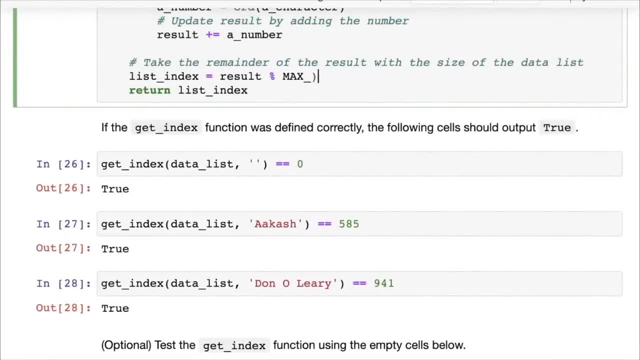 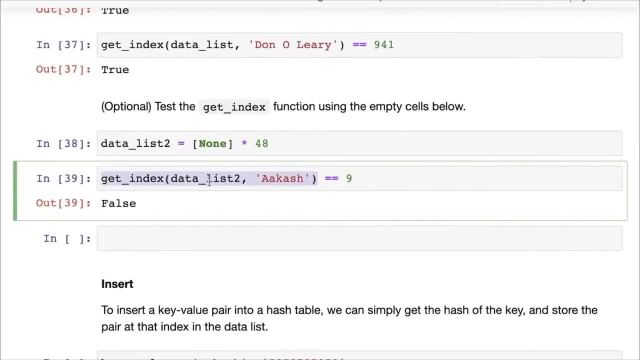 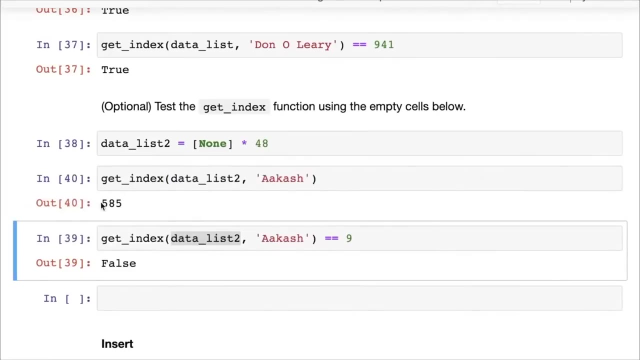 On the other hand, if we had max hash table size, you will see here that since we are not taking into consideration the actual size of the list that was passed into the function, we are getting back the value five, 85. Because we are taking the remainder with four zero nine six. 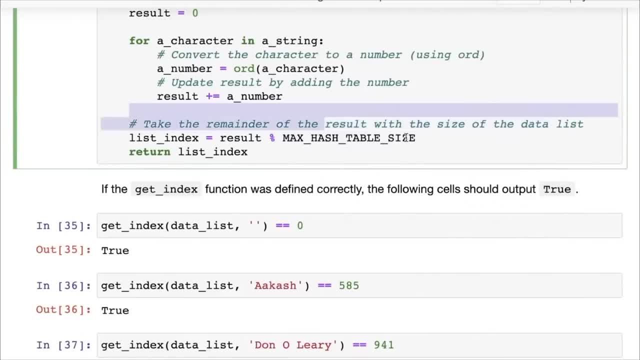 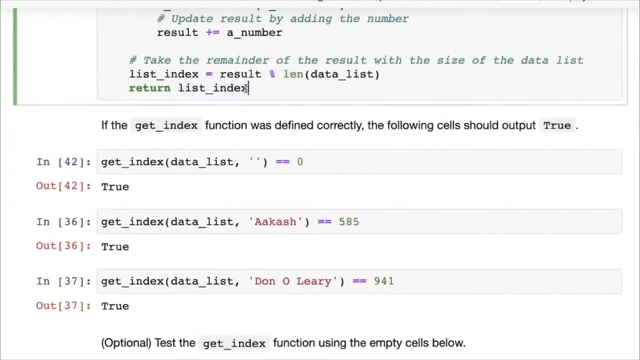 Okay, So remember to take the result remainder with the size of the data list that was passed in. So this is one of the several gotchas in this assignment, And they're there for a reason, because this is something that you need to keep in mind: a function which only uses its arguments and does not depend on any external global variables or constants. 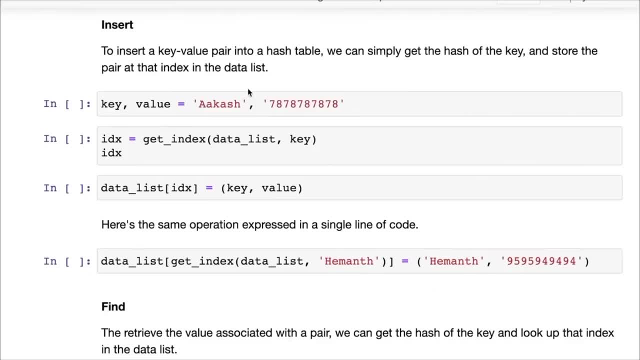 And things like that Is called a pure function. of course, a pure function also does not modify any external global variables, So it simply takes some arguments and returns the result irrespective of anything else outside. So now we can do: insert a key value pair into hash table. 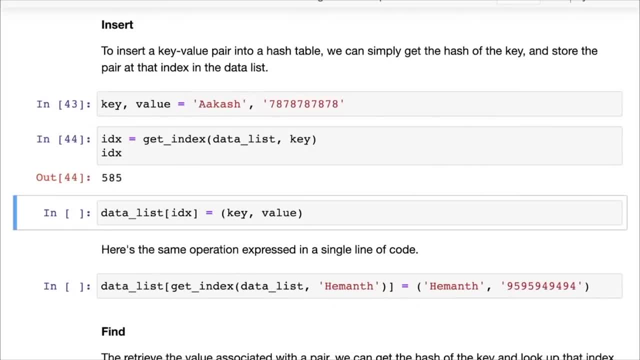 We can simply get a hash of the key. So here we have a key value pair and we simply get a hash of the key. by calling get, index or data list and key, We get back the index five, 85. And then, And then inside the data list at the given index, we can simply set the key value pair as the elements stored at that index. 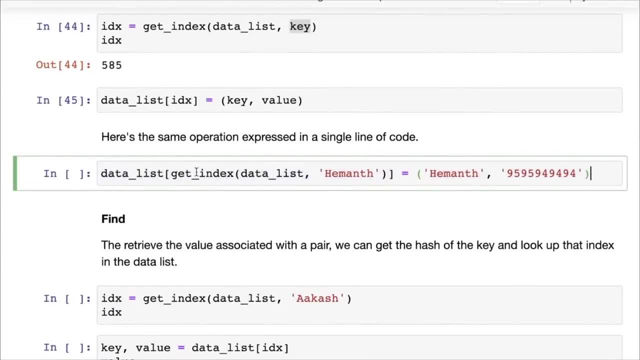 And the same operation can be expressed in a single line of code. So here we're calling get index or data list and he month, and that's going to give us an index and we're going to then invoke a set at that particular index within data list, the, the element he month. 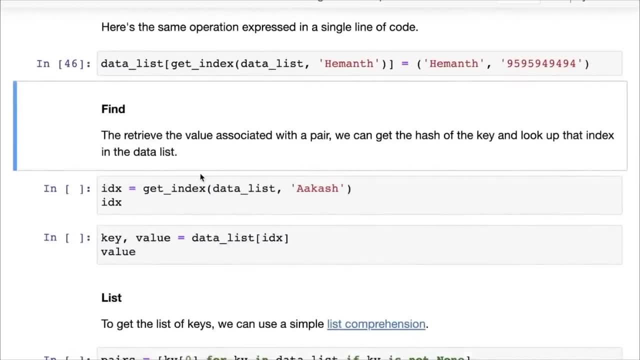 so we can use the index from him on his phone number, retrieve or find the element associated with the pair. So now to retrieve or find the element associated with the pair, we can simply get a hash of the element, the value associated with the key. 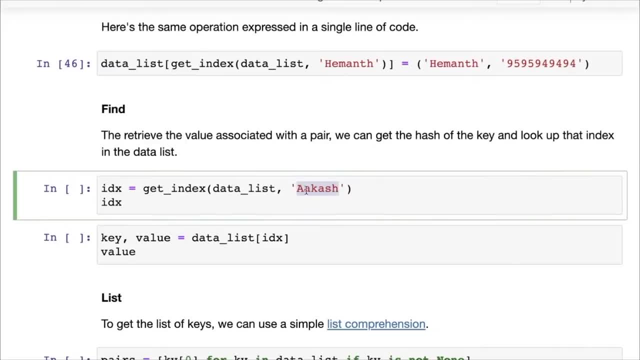 We can simply get a hash of the key and look up that index within the data list. But here we have the key Akash and we have the data list and we call get index. So we get the index of the key Akash And that gives us the index here. 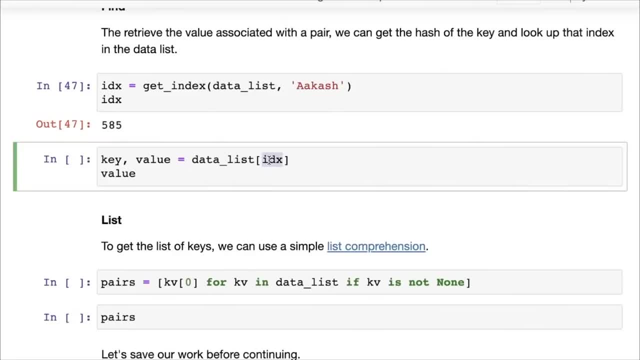 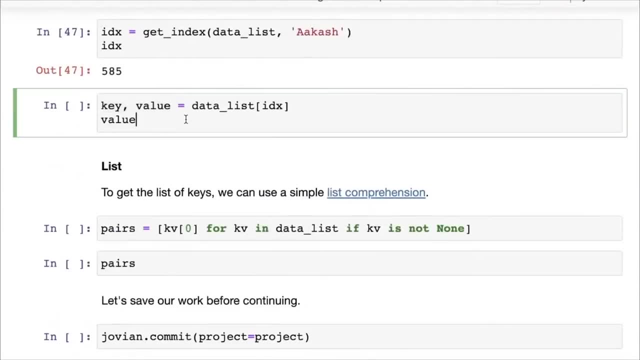 And we can then call data list and pass in the position IDX And that should give us a key value pair. Remember that we stored a key value pair at the given index, So we should get back that value here. So now we know how to store a value. 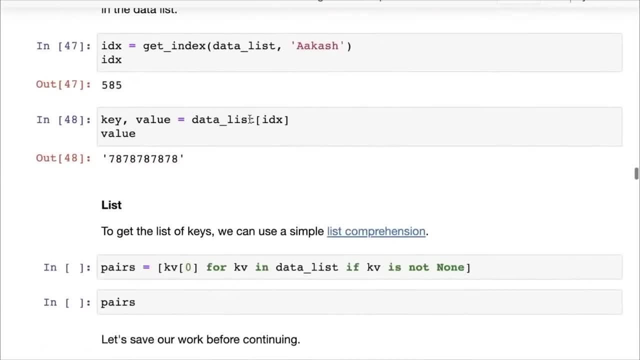 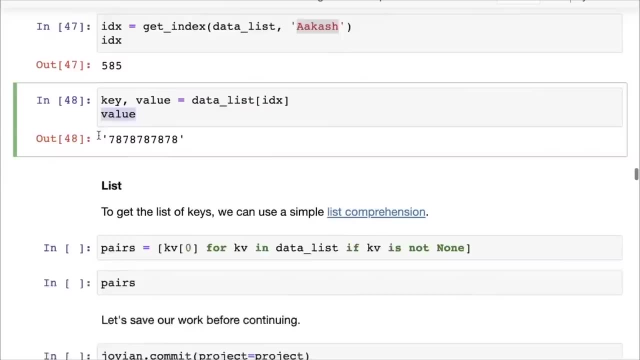 You get its hash for the key and you store the key value pair and how to retrieve a value. So you get a hash for the key and then you retrieve the key value pair And from there you can get the value. You can also list the keys. 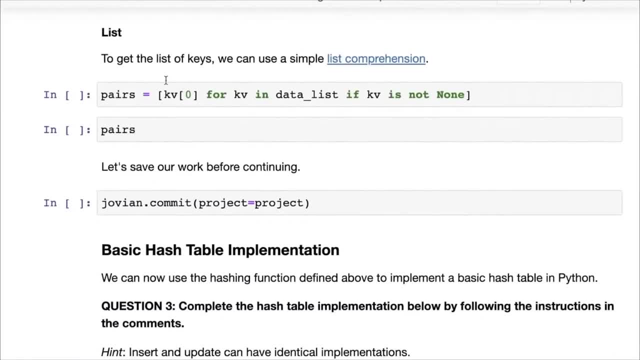 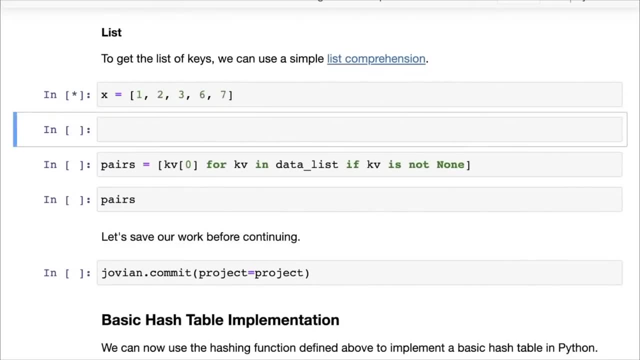 To list the keys. here is some special code we're using. So let's see this is called list comprehension and let's take a quick look at list comprehension. So list comprehension works like this: If you create a list Y from a list X, let's say, 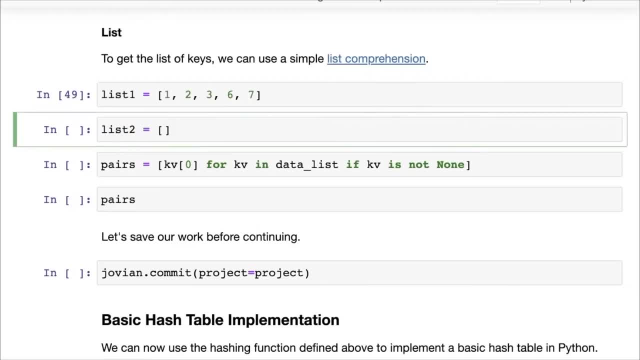 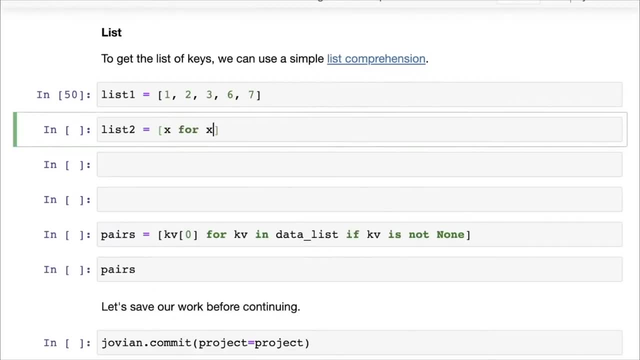 let's call this list one and list two. Good variable names always help. So if you have a list one and you write this X for X in list one, what does that do? that for X in list one fetches elements one by one from the. 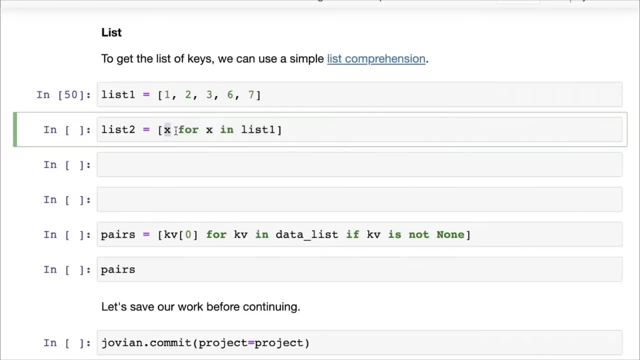 list And then here you can specify what to do with the numbers that were fetched. So right now I'm not doing anything. I'm simply returning that number And then I'm putting the entire thing into a list. What this does is this creates a new list, So you can see. 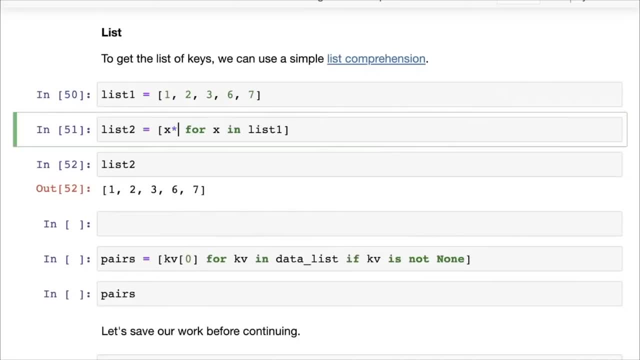 this is a copy of the original list. What I could do is I could write X times two for X in list one, And now I would end up with a list Which in which each element is the double of that particular element. I could also do X times X If I wanted. 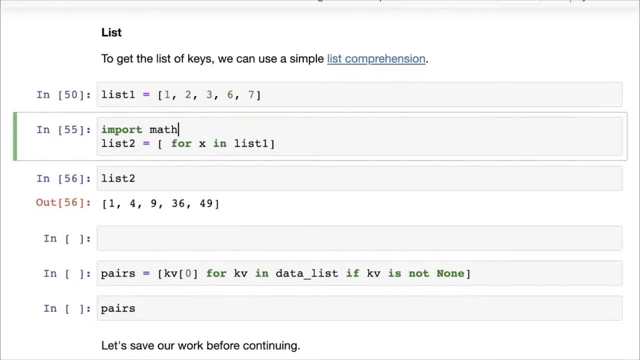 I could also call a function on it. Let's see what function we can call here. Let's maybe put in some numbers here: 1.3,, 2.4,, 3.2.. So we could put maybe the function math dot round. 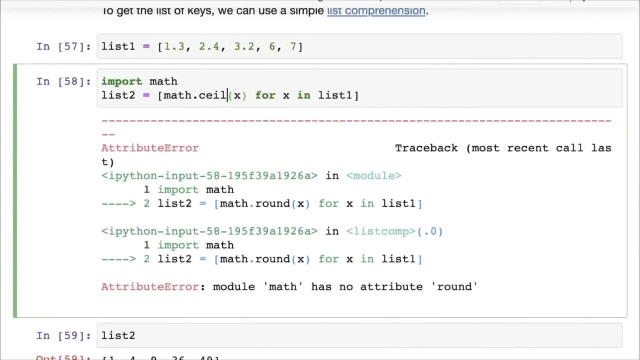 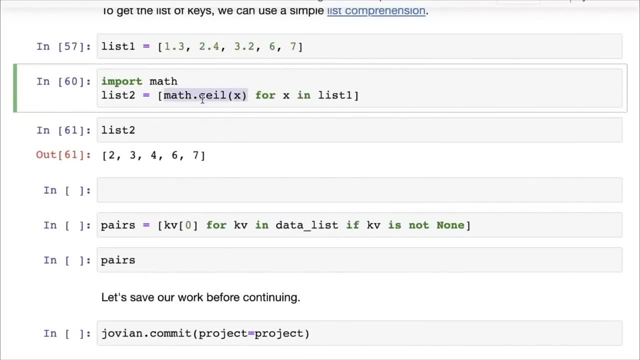 X. oh sorry, math dot seal. This is going to give us a ceiling. The 1.3 becomes two, 2.4 becomes three, So you can do any operation with each element of the list And once you put that in a bracket and you have this for here. 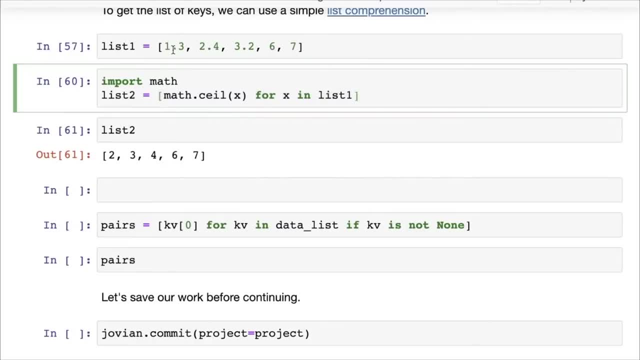 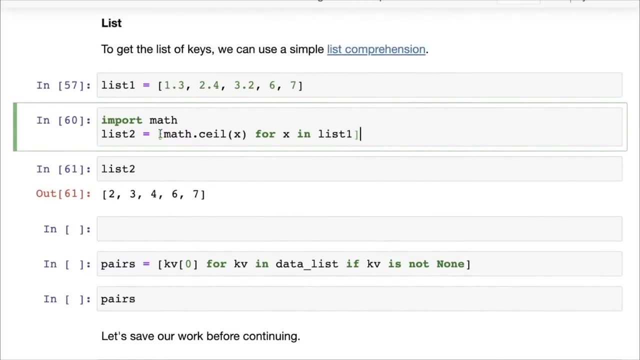 that's going to apply that same operation to the entire list, And this is called list comprehension in Python. It's a very powerful way to express complex operations on lists and dictionaries. And there's one final thing in list operations, which is the if condition. 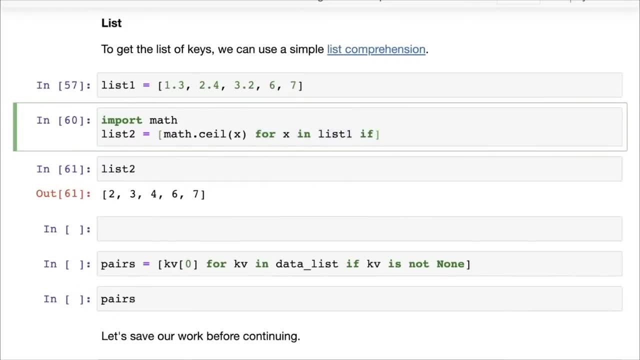 So remember, X in list one can be followed by an if condition, and the if condition can once again apply on X. So if X is greater than three, let's say we put this condition, then what happens is we choose only those numbers from list one. 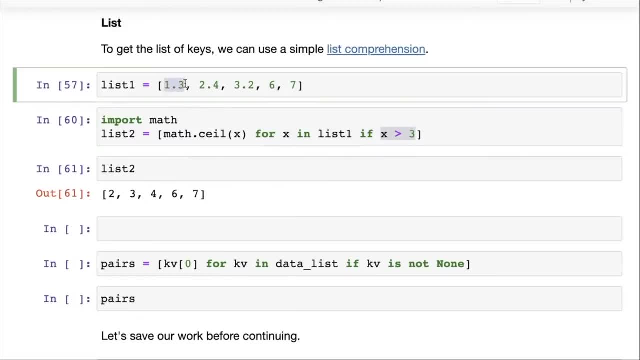 which satisfy this condition: X greater than three. So that means we would skip 1.3,, we would skip 2.4,, we would get 3.2,, we would get six, we would get seven and we would apply math dot seal to them. And that's how we get back four, six. 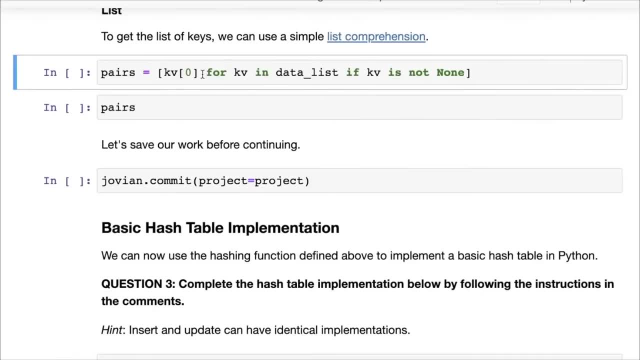 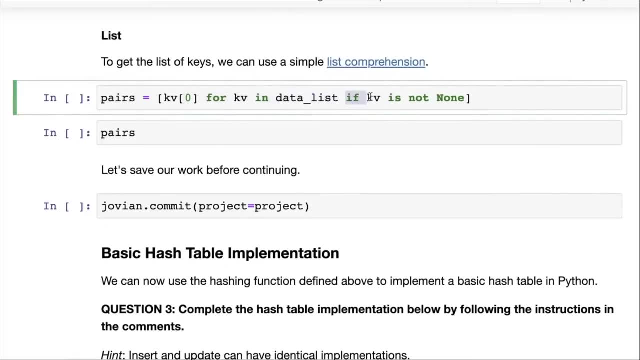 seven. So that's list comprehension in a nutshell. So to get a list of keys, all we can do is four key value pairs in data list. If the key value pair is not none, remember that we have a lot of none values and it's a huge list. 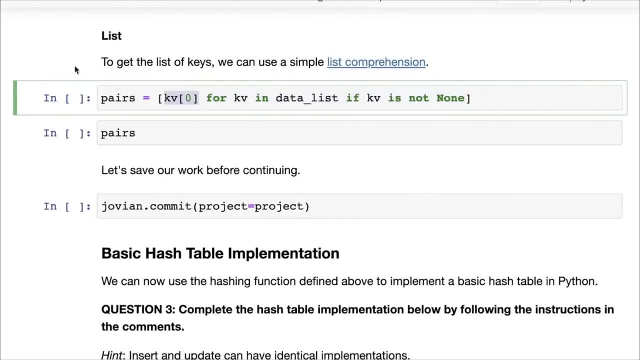 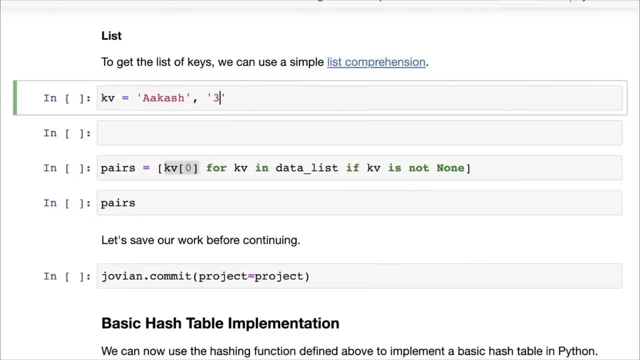 If the key value pair is not none, then we simply return KV zero. So remember, if you have a key value pair, if you have, like, a key value pair, that's Akash and a phone number, And you can also put- because these are tuples, you can also put a round bracket here, if you want. 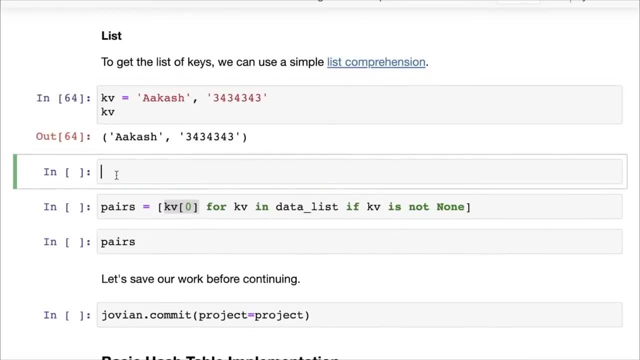 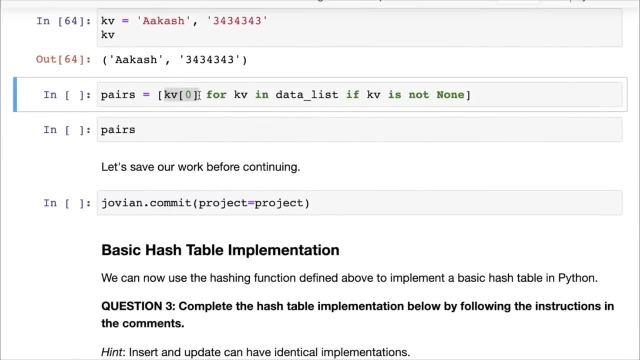 but even without it, it's the same thing. That's a key value pair. So KV zero is going to give you the key and KV one is going to give you the value. So we simply get the key for those key value pairs in data. 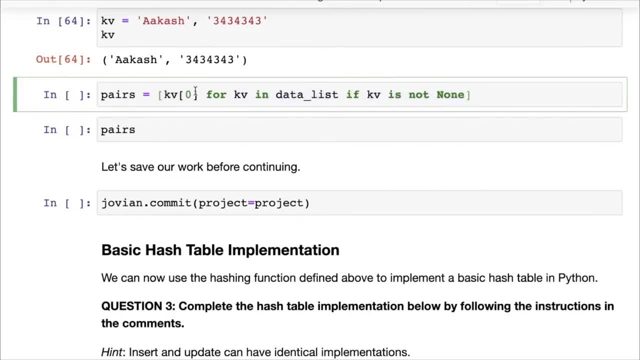 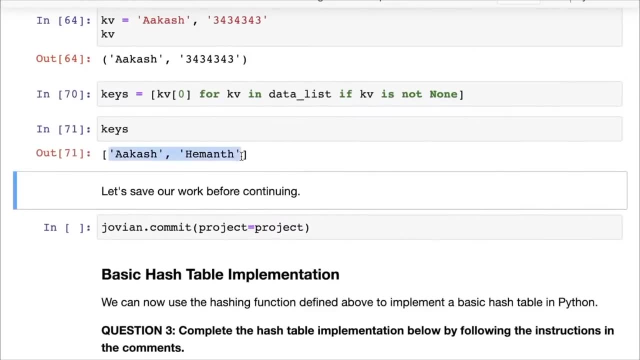 list where the element at that position of the key value pair is not none, And that should not be called pairs. That should probably be called keys. You can see that the keys are Akash and Hemant. So that's how we can now use the get index function. 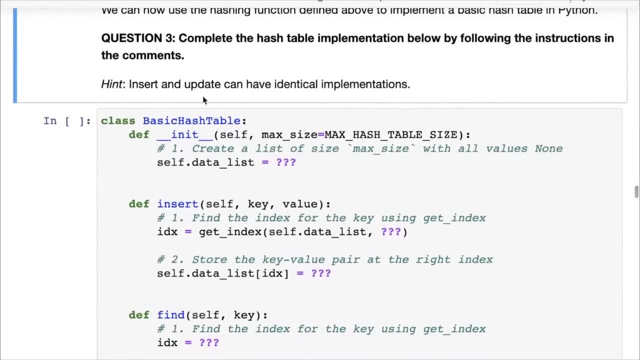 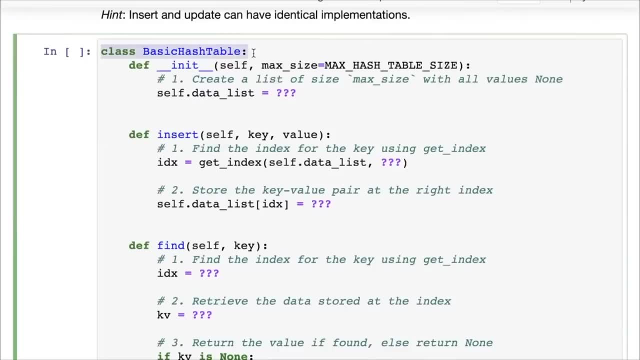 And the next step for you is to complete the hash table implementation here by following the instructions given in the comments. So now you have this basic hash table class and in this class you have a constructor. Now the constructor takes the object, self or this, and the self is going to point to the actual object or the actual. 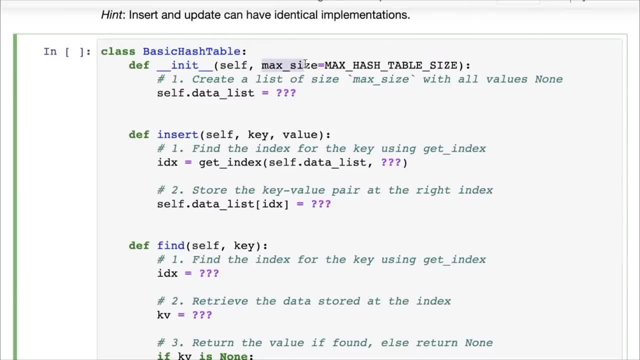 hash table that gets created using the class And then it takes a maximum size. What are we doing here? We want to make our hash table configurable. We don't always want to have four zero nine six elements in our internal list, If we may need a hash table that can store more values. 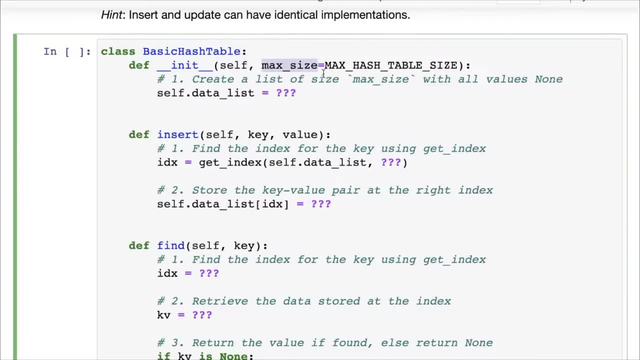 or we may need a hash table that can only store fewer values, So we are going to set a default value for it, which is the max hash table size. So if you do not provide this argument by default, it will create a list of size four, zero, nine, six. 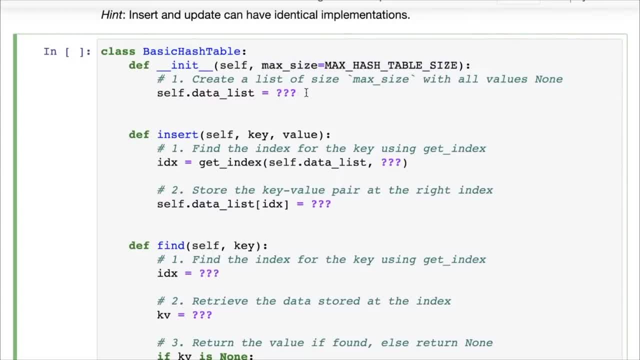 but we also want the option to specify a maximum size. Now you need to create a list of size, max size, with all the values set to none. Now you may be tempted to do this, but that won't be wrong. Remember that always use the arguments to a function. 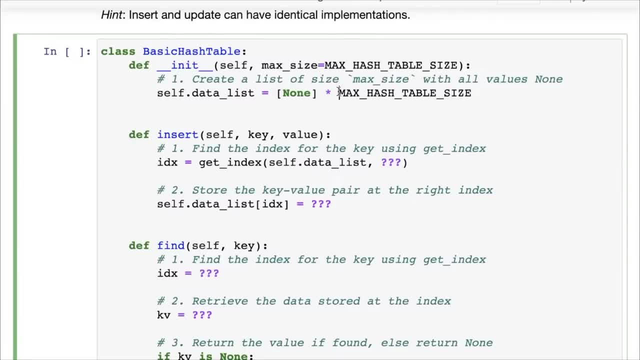 try not to depend on an external value or external constant, So this would be wrong. You may also be tempted to do this. data list self dot data list equals data list that we've already created. This would could also be wrong, not just because you're not using the max size, but also. 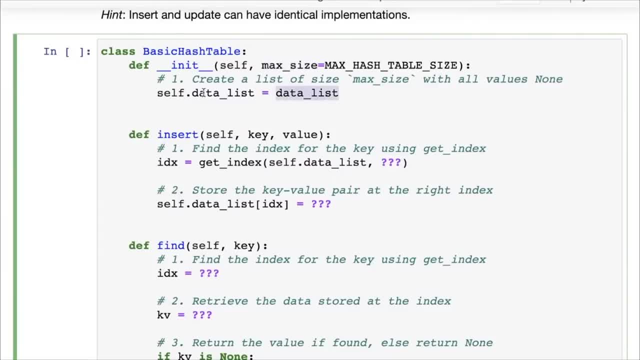 because now you're tying this class implementation to a global variable, And that global variable is a list which can be modified. So if you all the objects of this class, any number of hash tables that you create using this class, will all use the same data list. 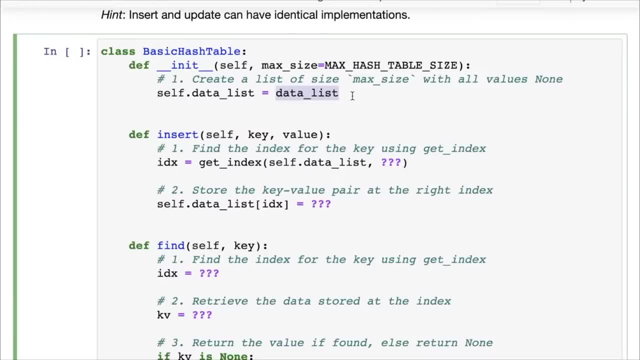 And that's not what you want. Each hash table that you create- maybe you have a hash table for phone numbers, You have a hash table for addresses, You have a hash table for something else- Each of them should have their own internal data list. 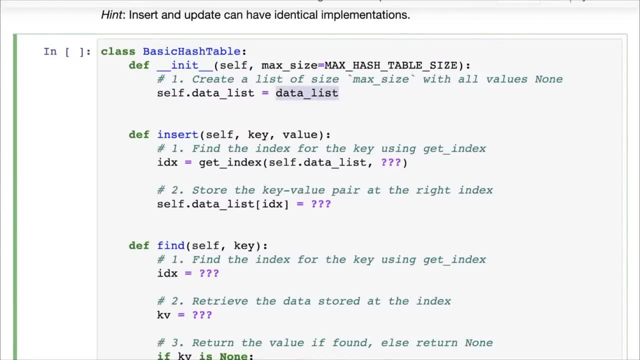 And this is not going to create a copy of that original list, is simply going to point to the original list. So what do you want to do? is you want to do none and you want to multiply it with max size? There you go. This is the correct way to do this. 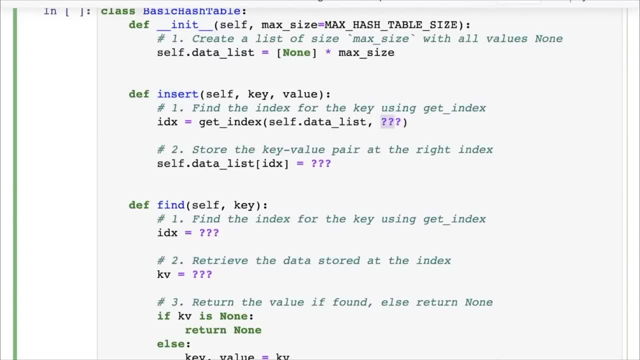 Now we're looking at insert here. now to insert: we did see that. to get the index all you need to do is You need to pass the key. and remember: here you need to pass not data list but self dot data list, right? 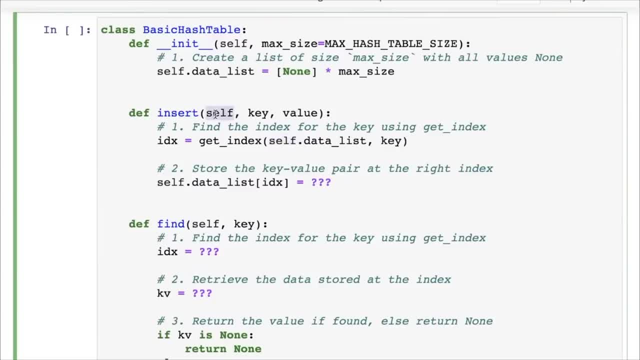 Because now we want to use the data list that is stored inside this specific object of the class. We do not want to use the global data list, And this is something that is an mistake that we often make Initially. I've still make this mistake where I have certain global variables. 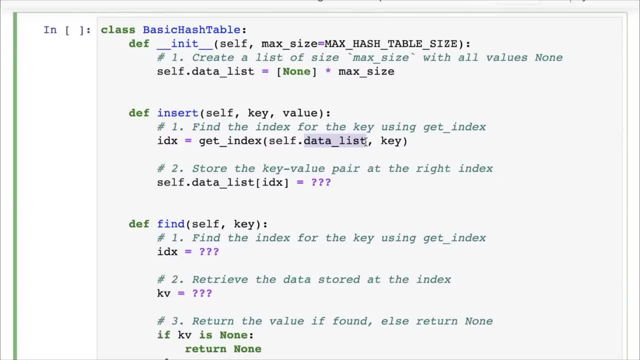 defined and I'm using those global variables inside my class. Why doing that? Anything that you want to put inside our class object, you need to put inside self, like we've done here, and then to access it, you need to use self dot to access that specific property or element, or even method. 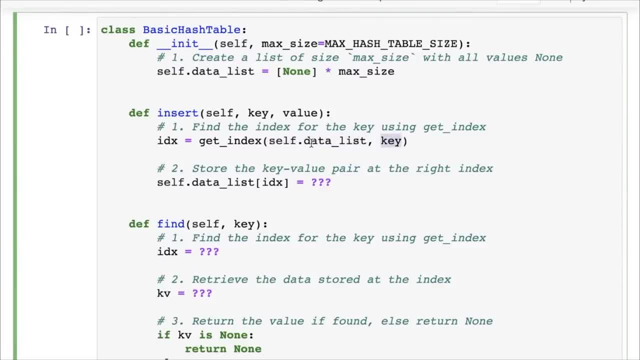 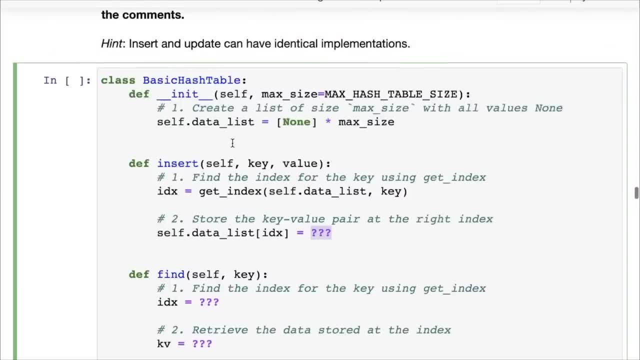 So now we have self dot data list and we pass in the key and the data list into get index and that gives us the index. Now the get index function was defined earlier. We've seen it already. Now we want to store the index inside the list. 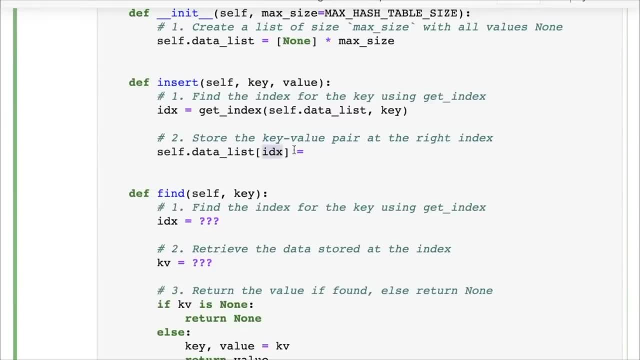 So We call self dot data list IDX and we want to store the key value pair there. So we can simply put in key comma value here. If you wish, you can also put in the brackets, but they're not necessary, And that's going to insert the key value pair. 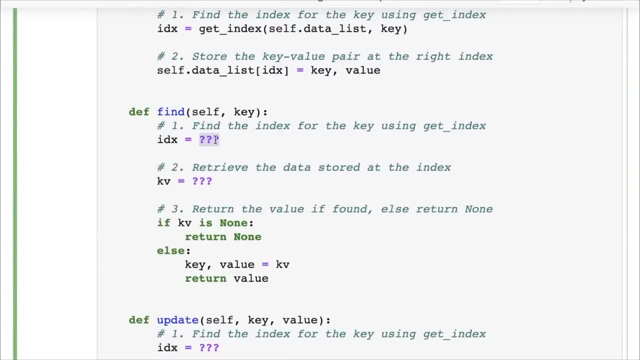 Now how do we find the value associated with a given peak key? First we get the index for the key. So we call get index on self dot data list and key. Then we retrieve the data stored at the Index. So this would be simply self dot data list of IDX. 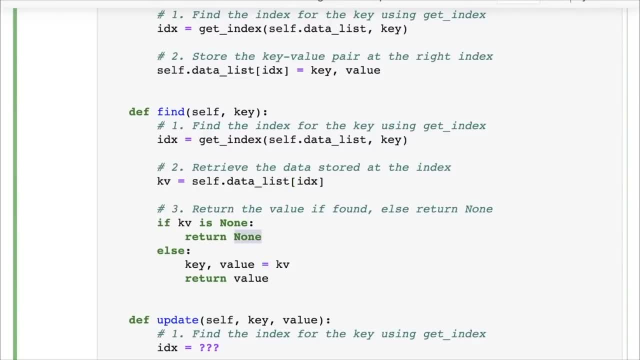 And then if the key value pair is not none, if the key value pair is none, well, there's nothing at that index, We can return none. Another option would be to also maybe raise an index error and with a message: et cetera, et cetera. but return on is good enough for now. 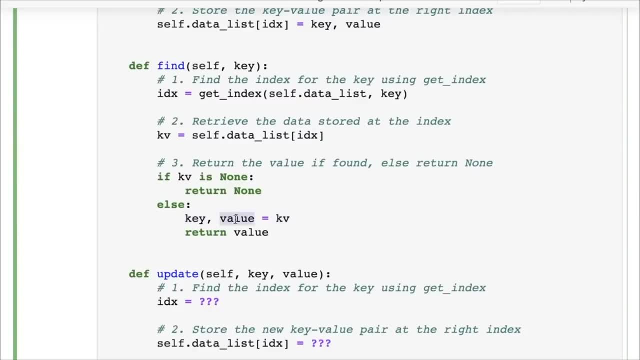 Then, if not From the key value pair, we get back the key and the value and then we return the value. Keep that in mind. If you simply return this, you would get an error, You would get an exception that may go unexplained. 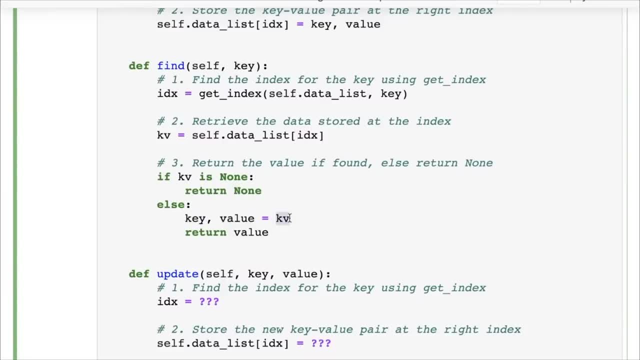 So whenever you are destructuring or you're trying to get two values out of a tuple, make sure that the tuple is not none, especially in this case, because we're starting with a list of nuns in a place where we're supposed to be storing key value pairs. 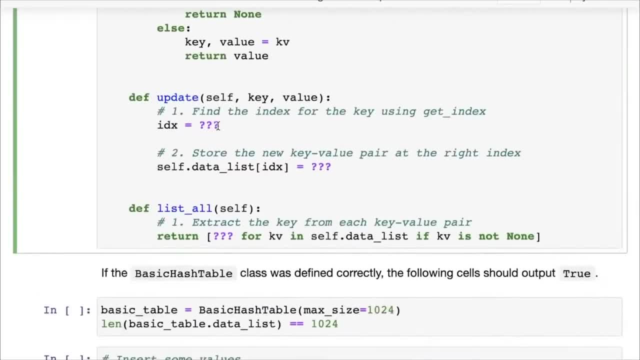 So that's fine. Now update is Going to be pretty much identical to insert. I don't see any difference here. So we can simply say: get index or self dot data, list and key, And then now we simply store the key value pair inside it. 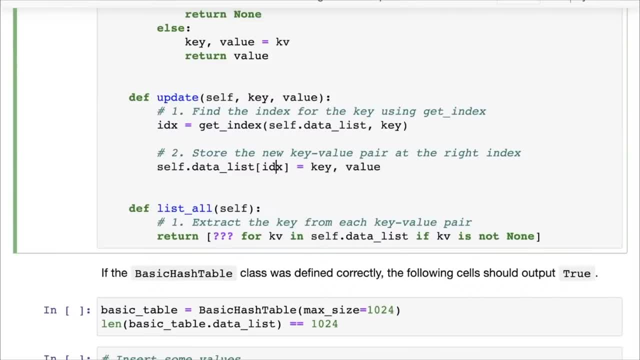 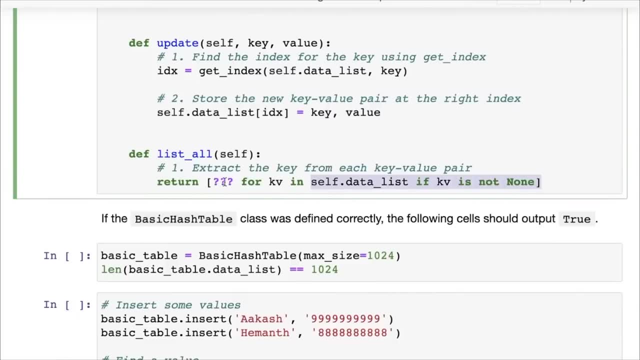 So we can simply store the key comma value inside self dot data list IDX. Then for list, all again straightforward: self dot FKB is not none, So get all the Key value pairs that are not empty And then we simply get KB. zero is going to give us the key from KB, so that there it is here. 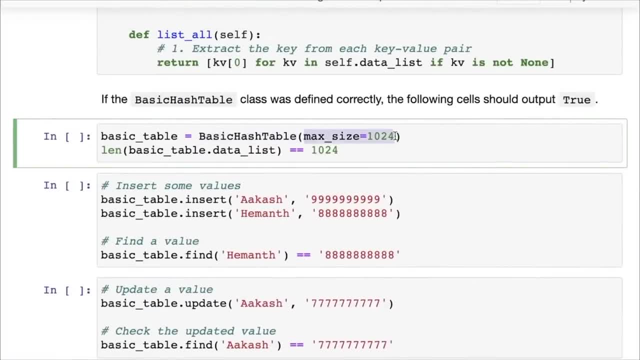 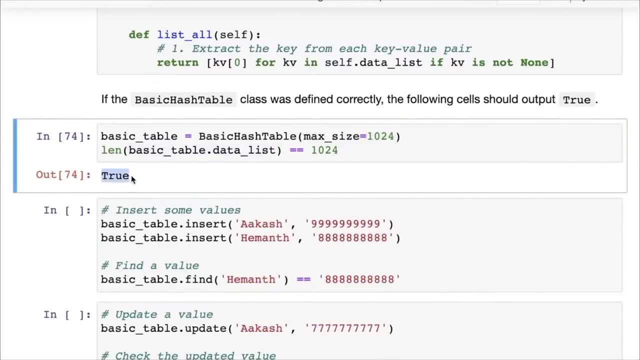 You can see already that we are creating a basic hash table of max size: one zero, two, four. So the first thing that we can verify is that the length of the basic of the data list is one zero, two, four. Then you go, then you insert some values here. 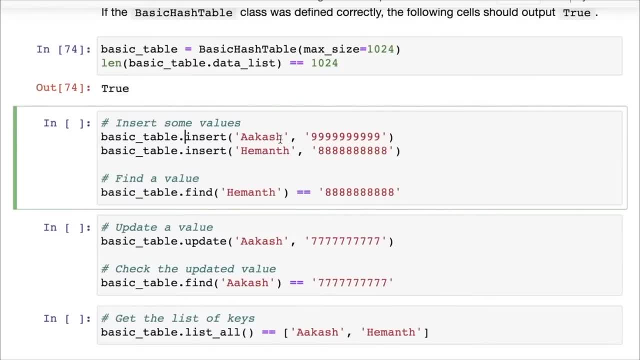 So we insert the value Akash, we insert the key value pairs. So we insert the value nine, nine, nine, nine for Akash. So this is one key value pair. We are inserting a month and eight, eight, eight, eight. 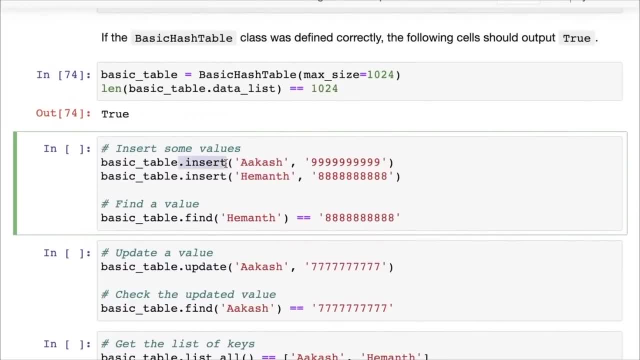 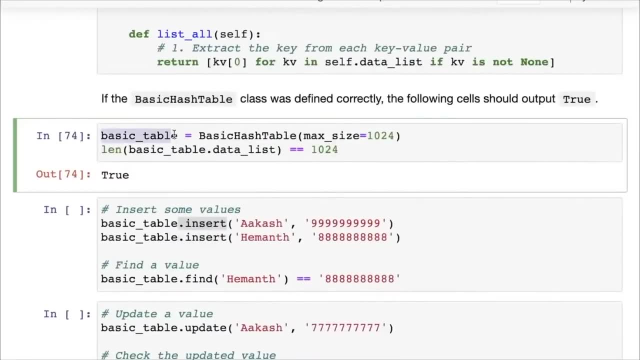 And what this will do is when you call basic table dot insert, it will call this insert function And self will now point to the basic table that we have just created because we're calling insert on that specific basic table. So self will point to the basic table. 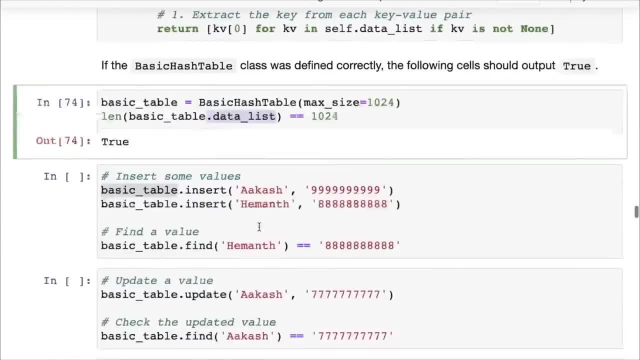 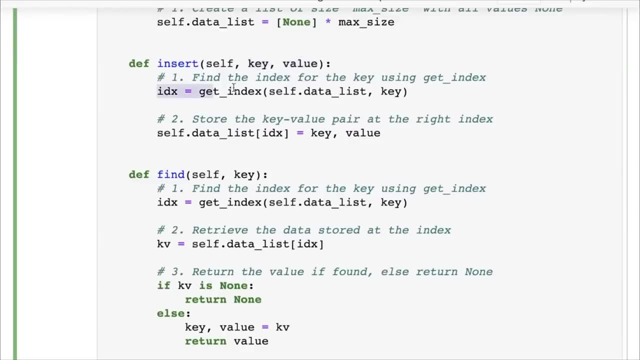 So self dot data list will become basic table dot data. Okay, Data list and then the remaining arguments: Akash and nine, nine, nine, nine. we'll get passed in as the key and the value. So this code will execute. 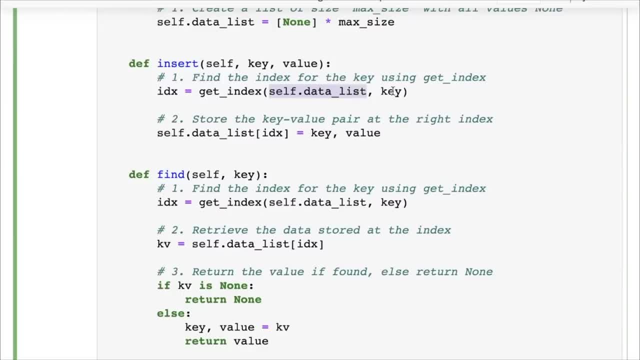 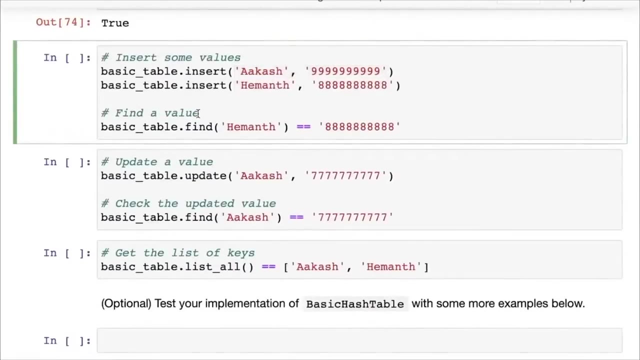 We will get the index within self dot data list for the key Akash And then within self dot data list or basic table dot data list. In this case, at the given index that we just computed, we will store the key value pair, which is Akash, and the phone number, and that's how it will work. 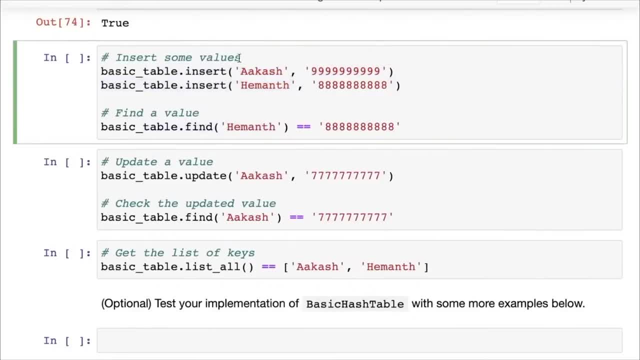 So we're inserting some values and then we are finding a. So when, once we insert the two values and then we find a value that should give us the value eight, eight, eight, eight, you may want to then maybe modify this test case to also include the test for the other value that we inserted. 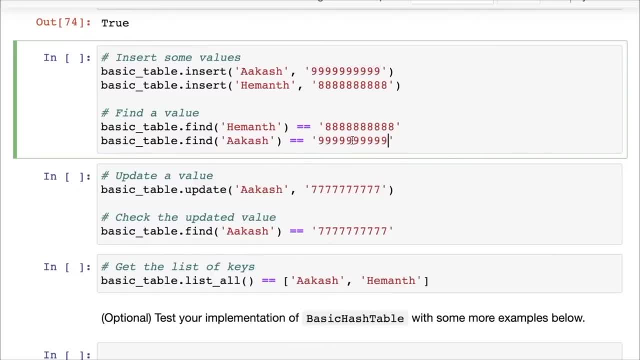 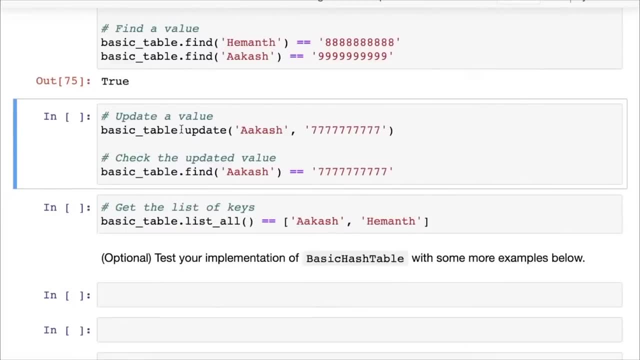 So feel free to modify the test cases or add new test cases so that we're checking not just one value but both the values. next Let's see how we, if we can update a value. So we call basic table dot update and we said seven, seven, seven, seven. 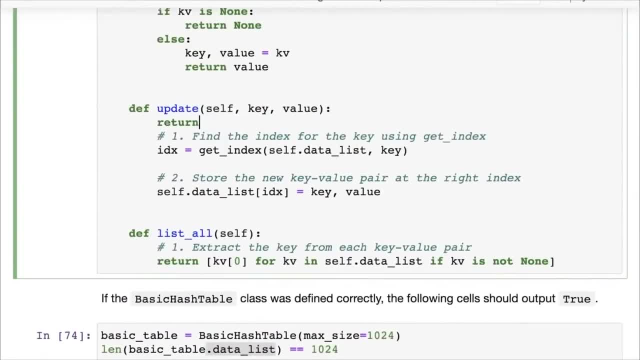 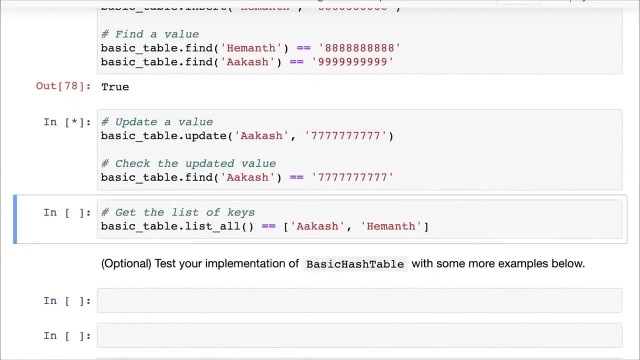 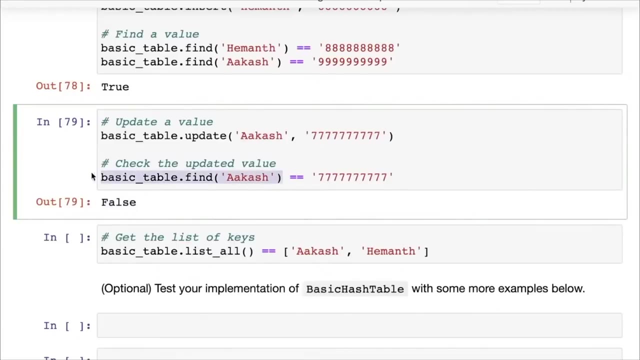 Now suppose you're not implemented update here. That's for a moment Return. Suppose you're not implemented update here, Then if you called update you would get false here because the value did not get updated. and you can check that by simply checking basic table dot find Akash. 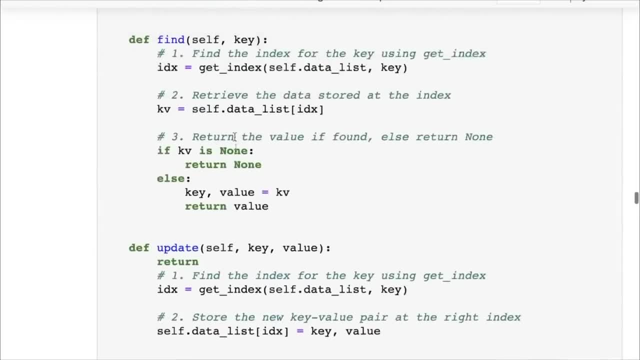 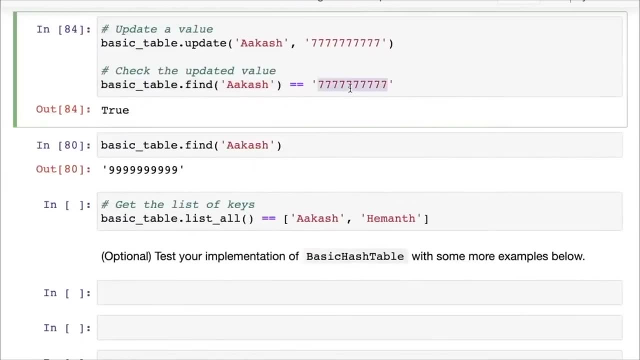 You can see that it still has a value nine, nine, nine, nine. That's how test cases are helpful. Let's remove the return. Okay, So now the value seems To have been updated. Just fine. Then let's get a list of all the keys, and the list of keys should match true. 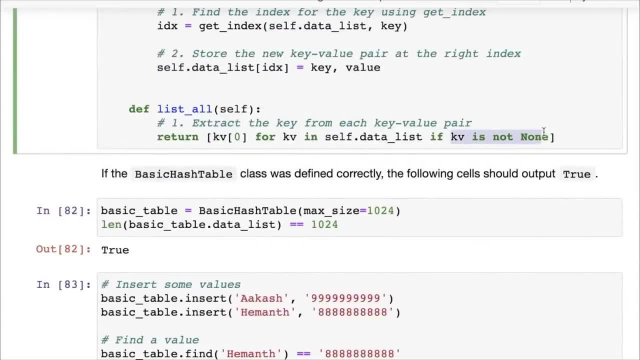 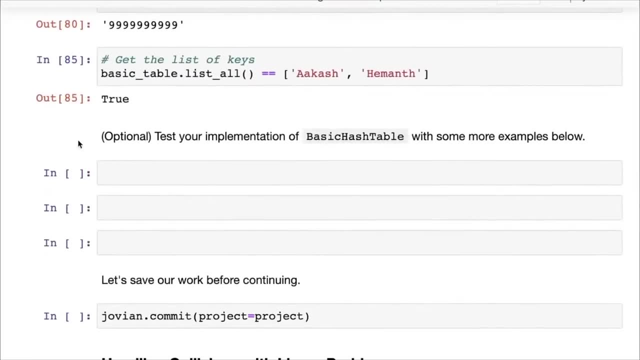 Once again, if we did not have this- KV is not none- then we would get back not just the ski value pair, but we would get back all the nuns, and we don't want that. So these were some test cases, but you need to down, create more test cases and test them out to make sure that your implementation is correct. 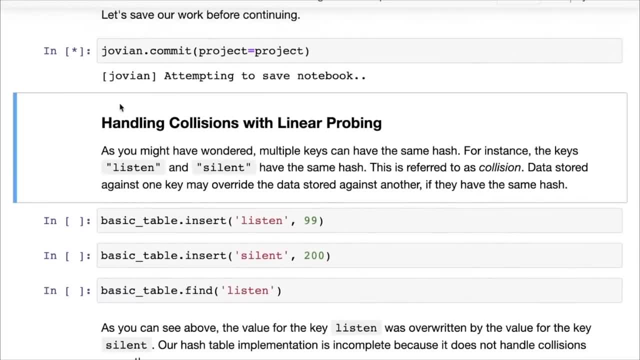 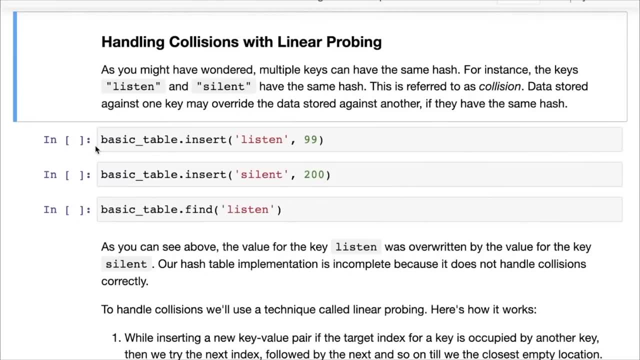 Now, once you've done that, you would want to run Joviancom it Now. the next step- and this is something that you may have thought about while working through the assignment- is that how do you ensure that different keys do not point to the same index? because we're doing all these things where we're converting each character into a number and then adding up the characters. 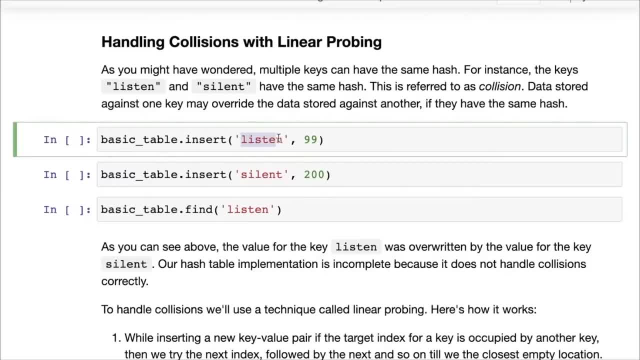 Now, obviously, if you have words which have the same characters but in different orders, now obviously are different keys, but they do not have, they have the same hash. Listen and silent have exactly the same keys, exactly the same hash. 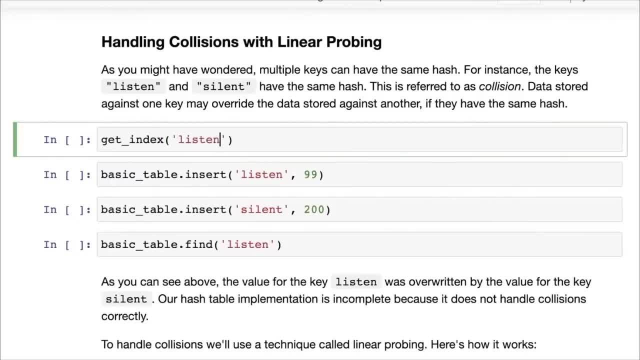 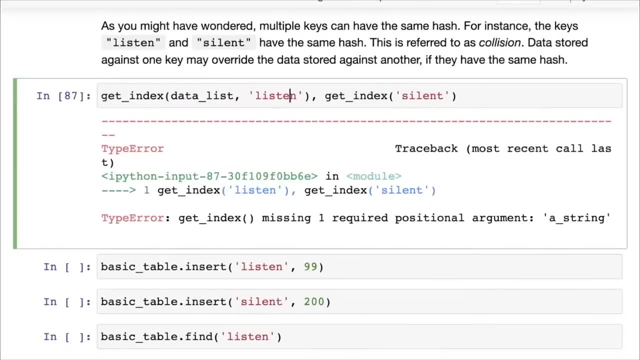 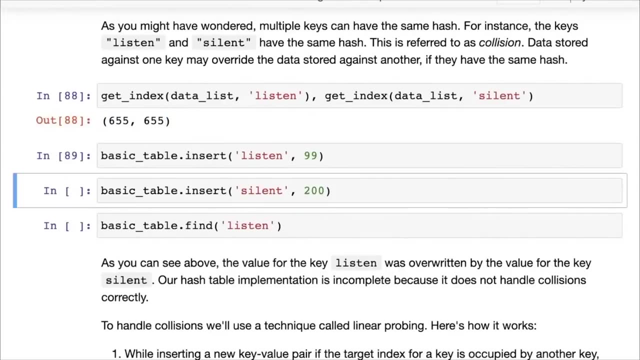 So, for instance, you can check, get index listen and get index silent. Okay, We also need a data list. Let's put in a data list here. Both of them have the hash 655.. That means if you insert a value at with the key listen and then you insert a value with the key silent, 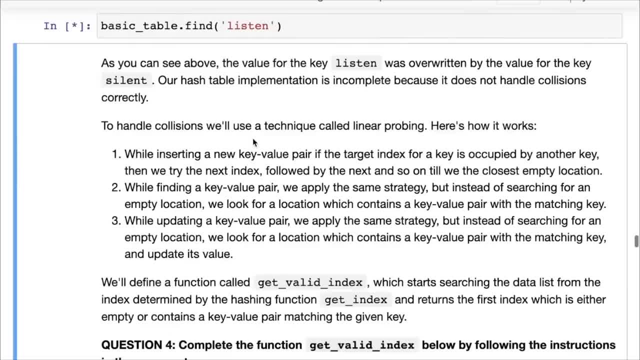 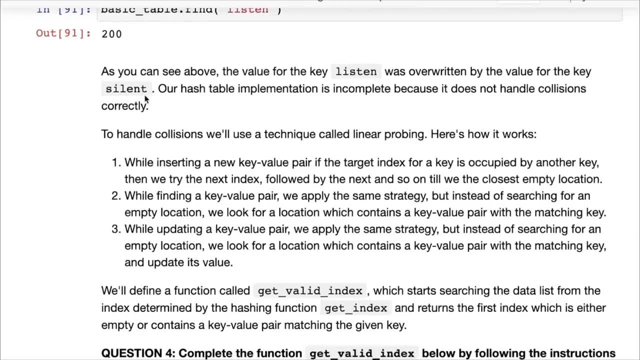 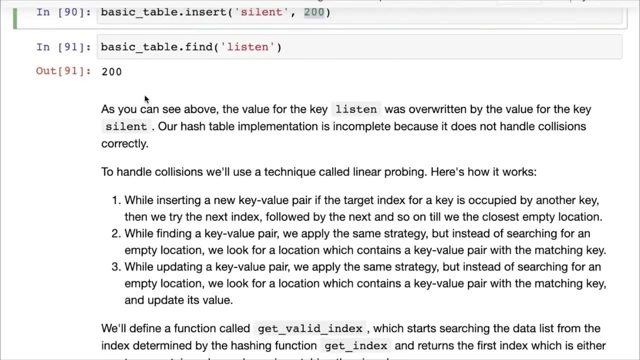 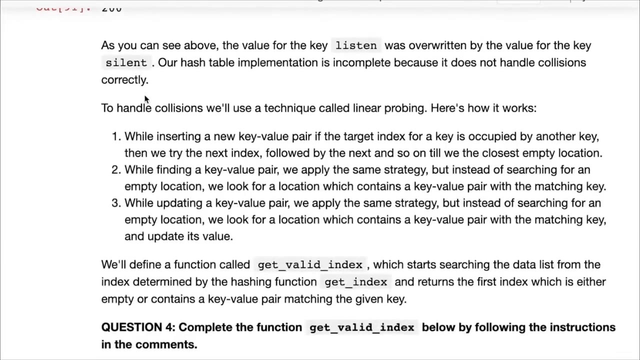 The data at this position will get overwritten. So when you try basic table dot, fine, listen- you will get the value associated with silent, and that's bad And this is called collisions. This is called a collision because here the two keys are colliding in some sense, because the leading to the same hash and any hash table that you implement is ultimately going to have collisions, because the number of strings or the number of keys is possibly infinite. 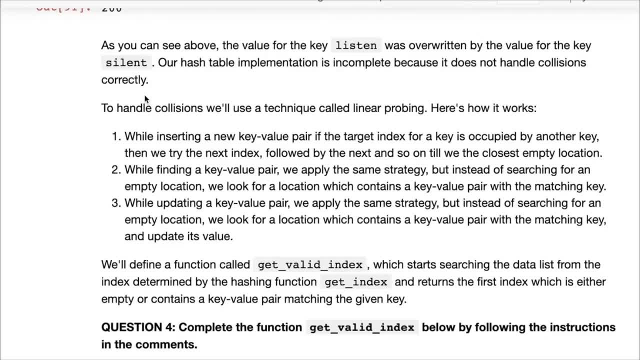 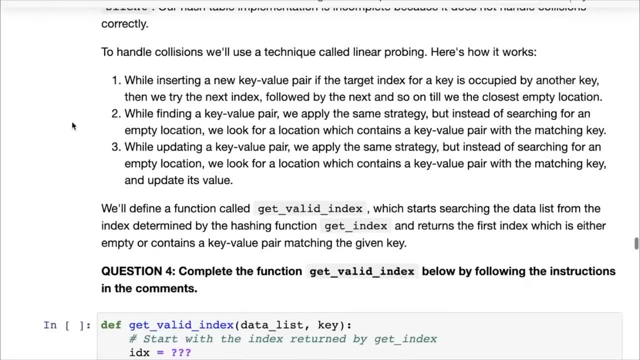 But you have a limited number of positions or indices in your table. So our hash table implementation is incomplete because there can be data loss and it does not handle collisions And there are multiple techniques to handle collisions And we the technique we will use in this assignment is called linear probing. 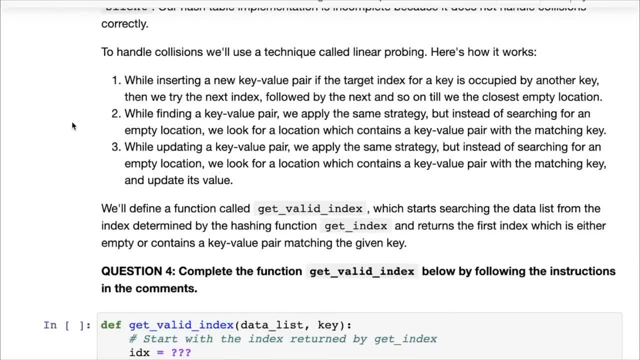 And here's how it works. while inserting a new key value pair, If the target index for key is occupied by another key, then we simply try the next index, And if the next Index is also occupied by another key, We try the next, and then, if we try the next, and then we try the next, then we find the closest empty location. 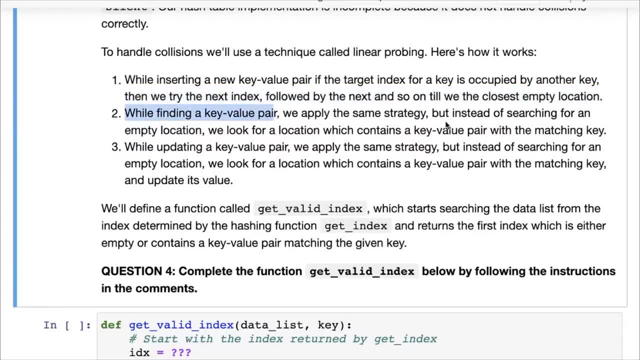 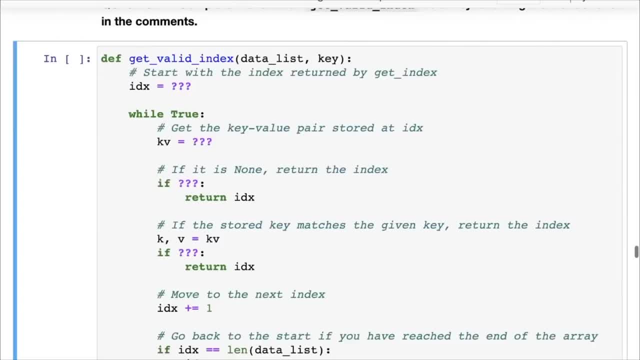 And then, while finding a key value pair, we apply the same strategy, but it's searching for an empty location. This time, we search for a location which contains the key value pair with the matching key. We get the hash of the key that we want to find. 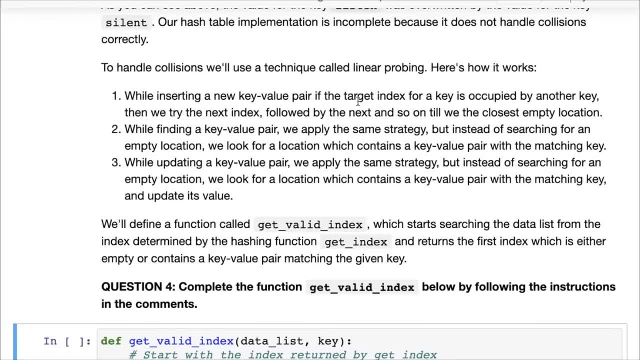 And then we check if that position is occupied by another key, not the same key, Then we try the next index, and then we try the next index, Then we try the next index till we find a position which is occupied by a key value pair for the same key. 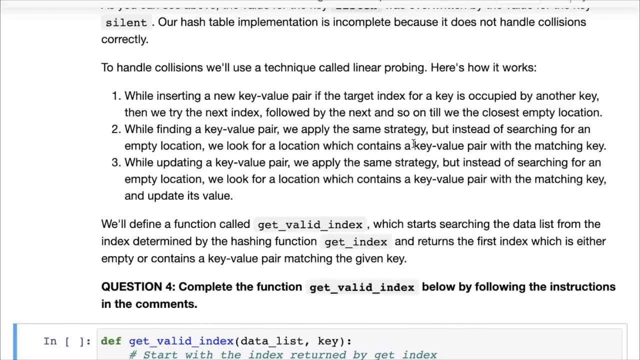 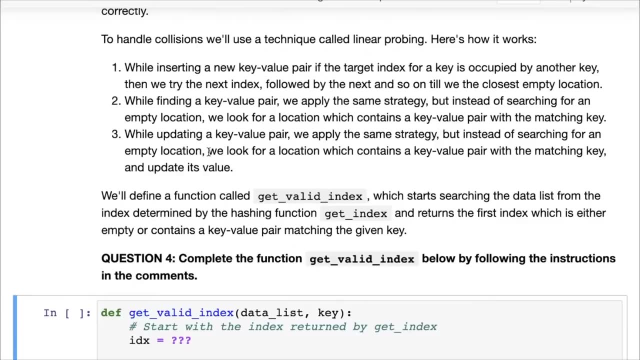 And if we find an empty position, that means the key does not exist, because if it did exist, then it should have been somewhere in that string of searches that we just come. that we just did now by updating the key value pair. Again, we apply the same strategy, but instead of searching for an empty location, we look for a location which contains a key. 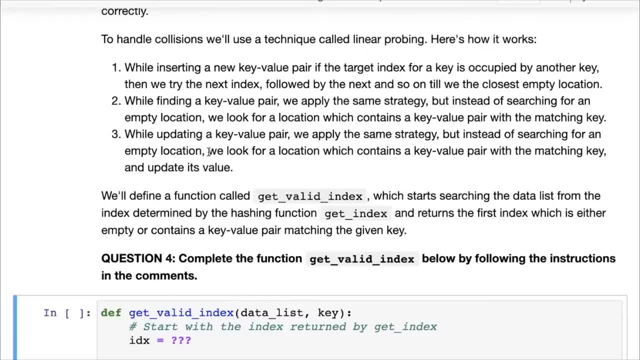 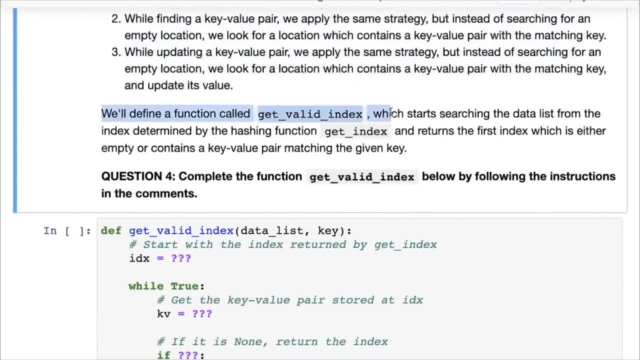 value pair with the matching key and update its value. So that's how you handle collisions in a hash table. And to handle collisions we will define a function called get valid index which first gets the hash using get index and then start searching the data list and returns the first index which is either empty or contains a key value pair matching the. 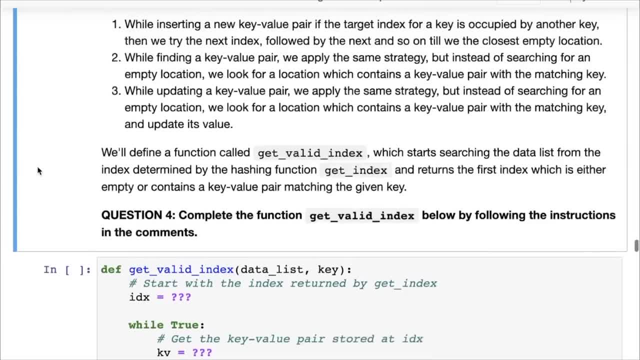 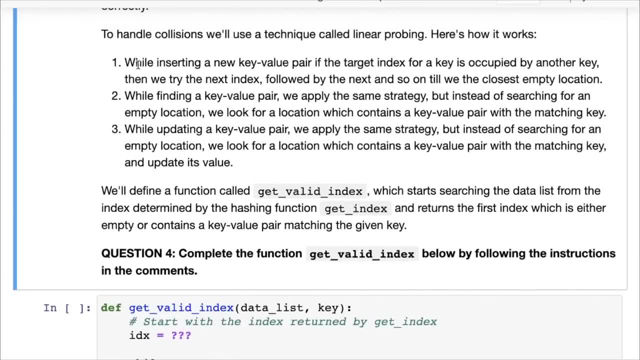 given key. So we are now addressing two requirements in one shot with the get valid index function for insertion. we are looking for an empty position For find an update. we're looking for a position which is occupied by a, by the given key value, by the given key value pair. okay, or? 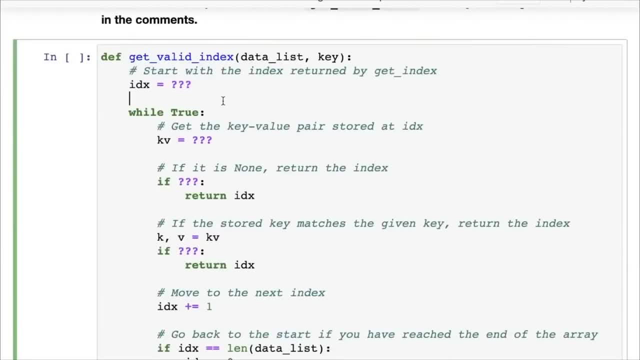 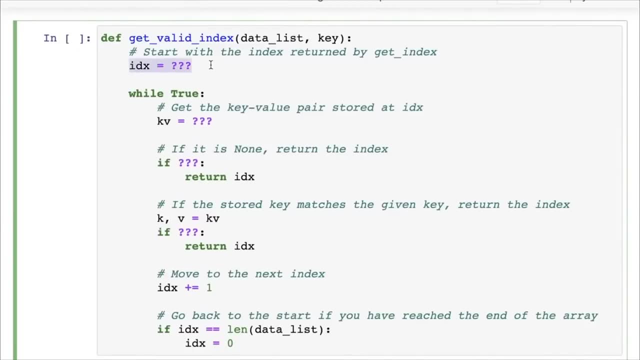 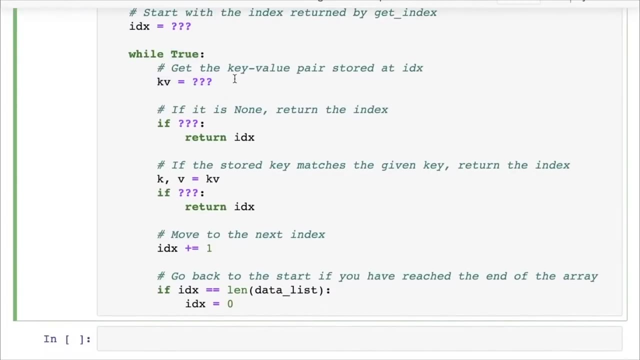 the given key specifically. So here's the get valid index function And I will let you work through this, So you will start with the index returned by get index. then, while true, because we don't know how long we may need to iterate- get the key value pair stored at the index. 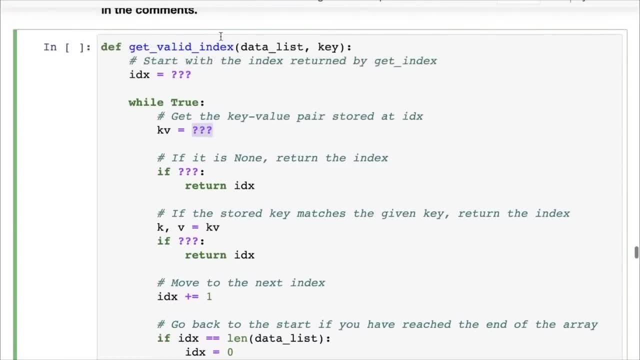 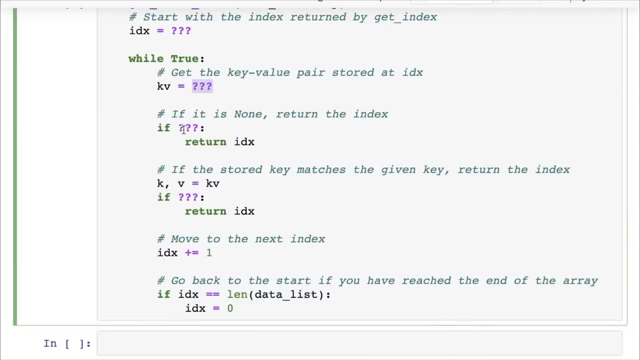 This is where you may have to. It's simply a question of putting the index into a data list, getting the key value pair. Now, if the key value pair is none, which means that there is nothing at that index, it is empty. 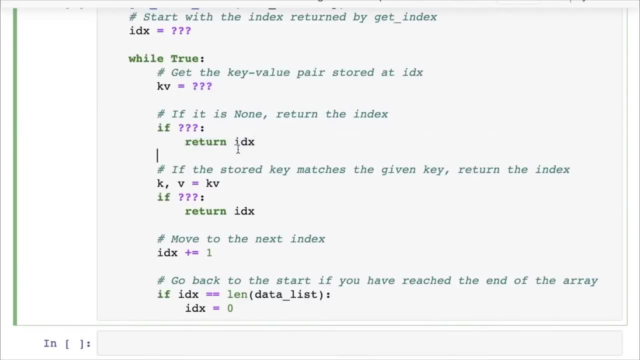 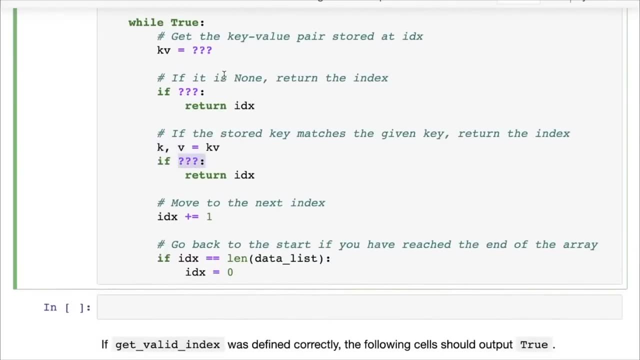 That's great, We're done. You can simply return the index, On the other hand, if it does have values, so then we get the key and value out of it. If the key matches the key that we want to store, great. 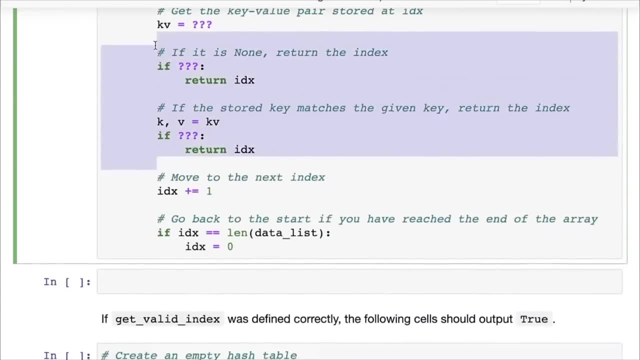 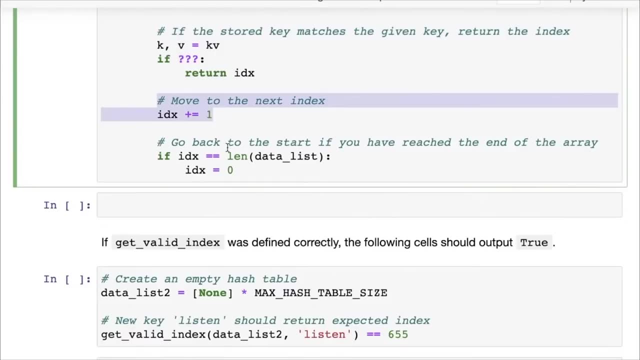 Then we can return the index once again. if neither of these hold true, we move the index to the next position. But as we move to the next position, it's possible that we may run out of indices or the index may become equal to the. 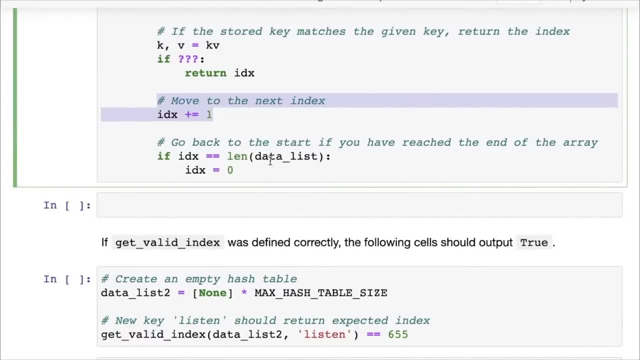 length of the data list. So then we wrap around and go back to the zero position. So this is an important part where we go around. So now our list is in some sense circular, where we can keep looping around it so that if we have something that needs to be. 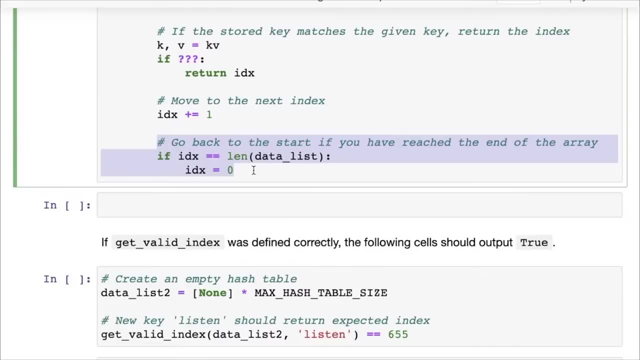 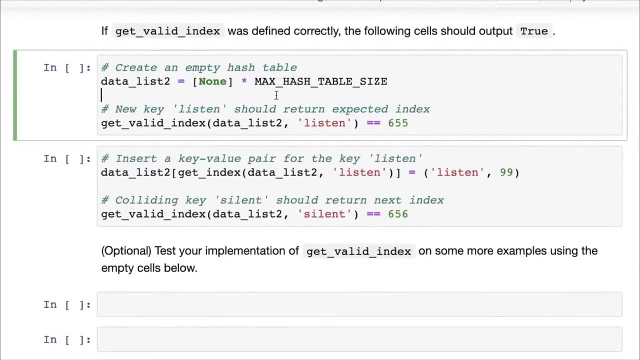 stored at the last position, but the last version is occupied. then we move back to the zero position and so on, And then you can check it. Get Valid index was defined correctly, And if it was, then these cells should output true. 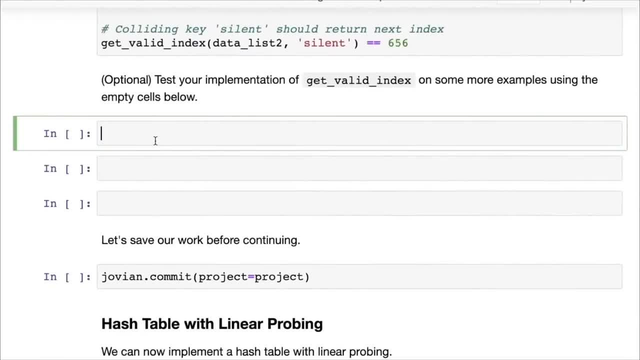 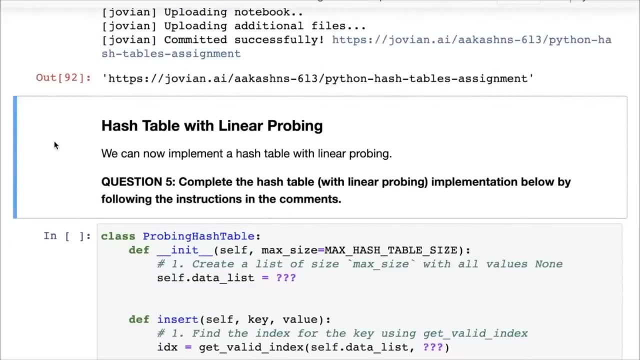 Once again, these are just some sample test cases, So you should include some more of your own test cases here And then finally, once you're done, just save your work. Now the next step is to incorporate linear probing into your hash table. 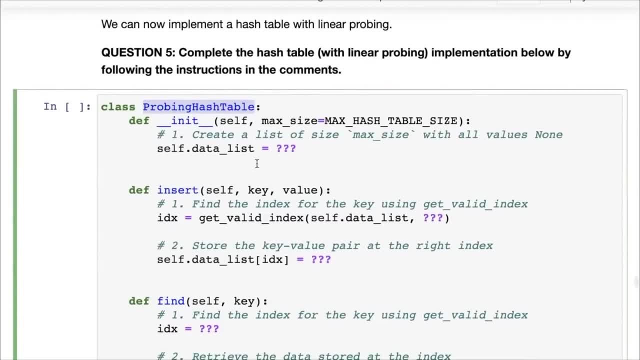 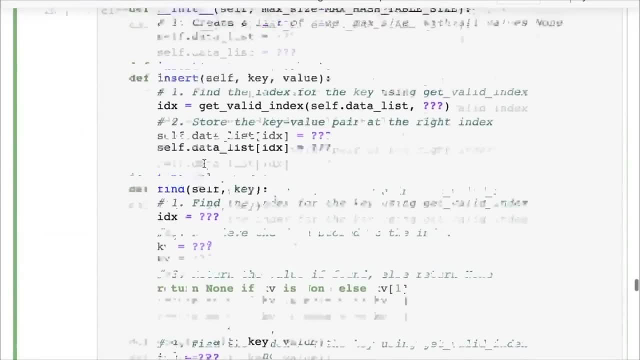 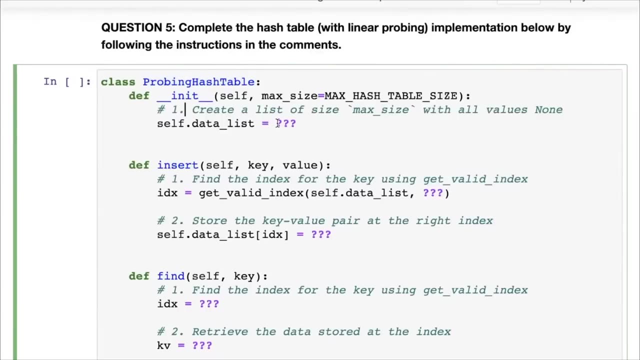 So here's a new class called probing hash table. here You need to use not get index, but get valid index. It has pretty similar code. So I let you work this out. Be aware not to simply copy paste code and you will run into issues if you copy paste code. 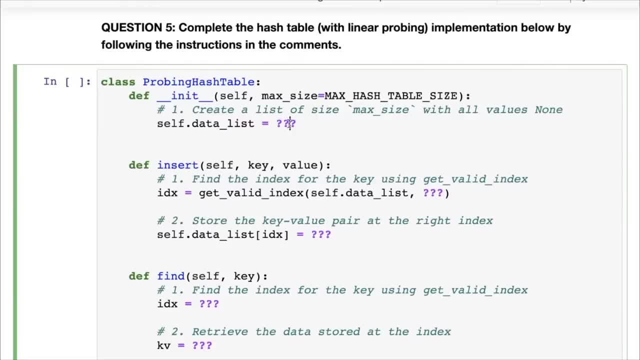 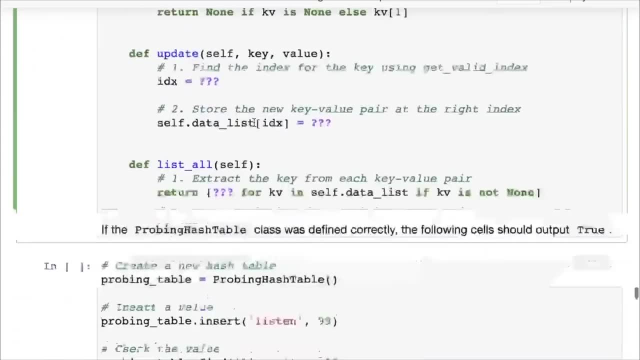 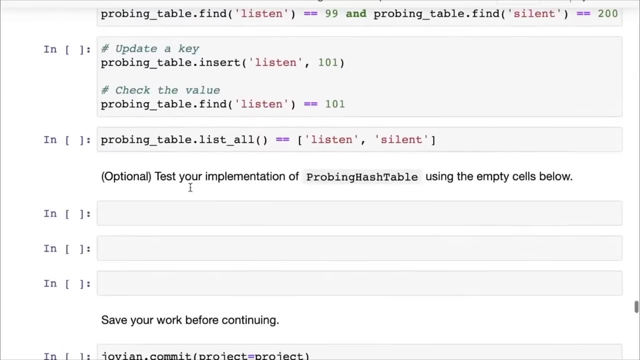 So always make sure that you are writing the code yourself and carefully writing each word or each variable and each method and each argument of the code. Then there are some test cases here for you to test the probing hash table Once again. you can try it out with some examples and see if it works fine, specifically here: 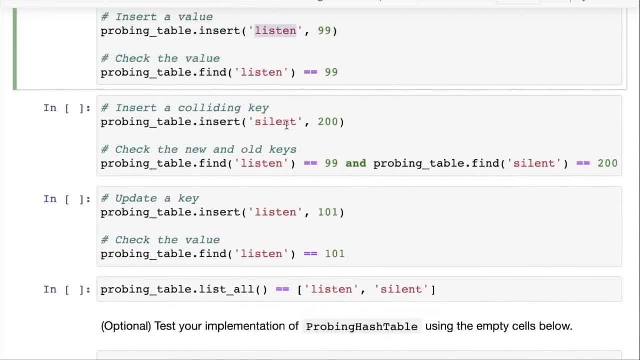 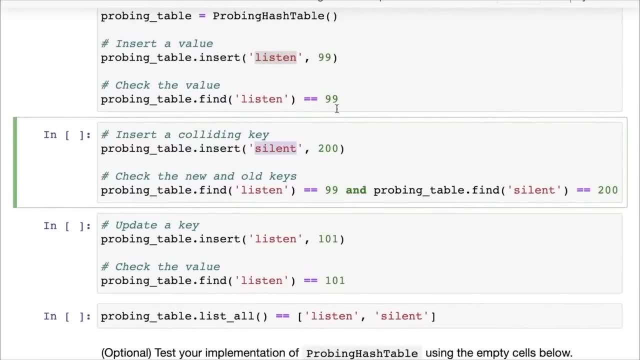 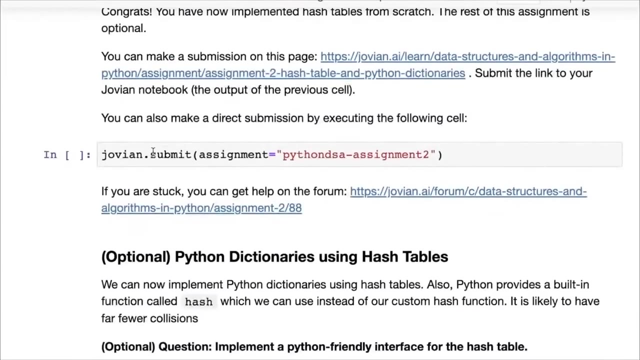 We are taking the same example- listen and silent- both of which in basic hash table would have the same key, but in probing hash table would have different- will have the same position, but in probing hash table will have different positions, And that's it. at this point you're done with the assignment. 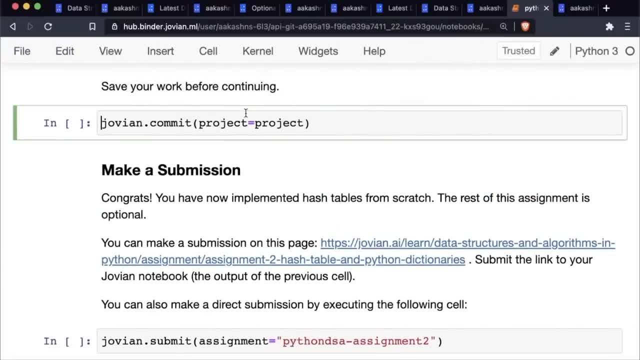 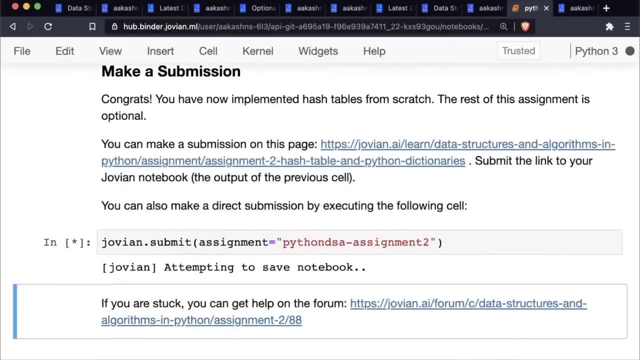 So you can make a submission. If you have run Jovian dot commit, you can take this link and make a submission on the assignment page, or the other option for you Is to simply run Jovian dot submit by 10 DSA. assignment two. 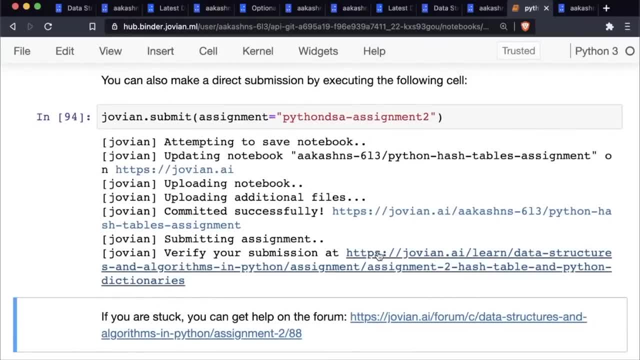 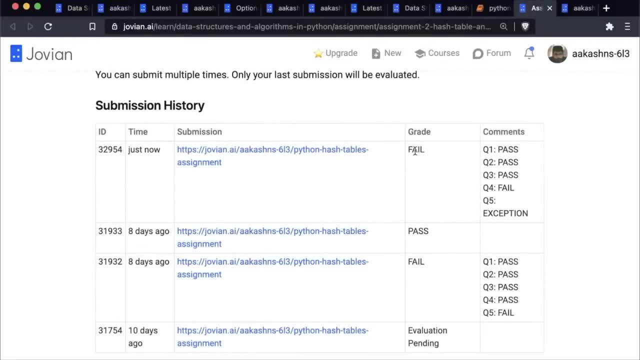 And once you make a submission it will be evaluated automatically. So let's click through here So it will be evaluated automatically. And if you scroll down here, you will see that you will get a great- and not just great, but you will also get comments for each question. 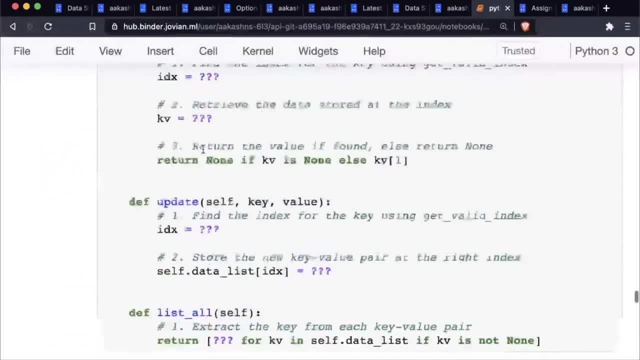 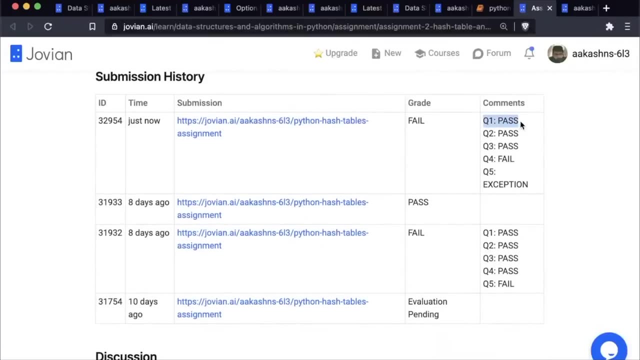 So if you see here there are question numbers, here You can see that there's question five, question four and so on. So it seems like we, since we implemented The get index function, since we implemented the data list correctly, question one was a pass. 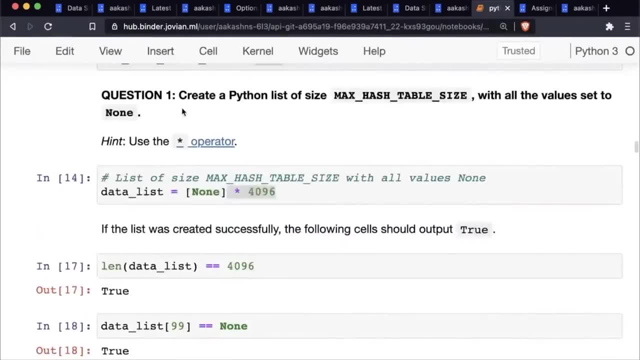 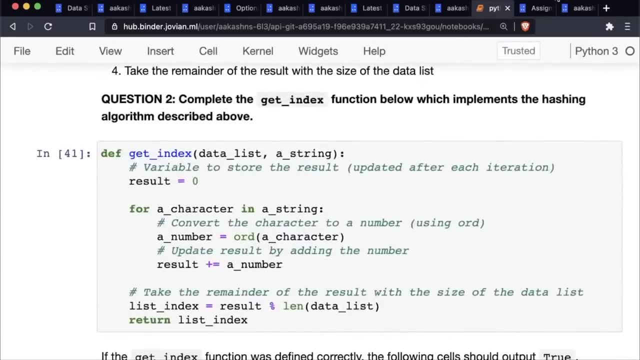 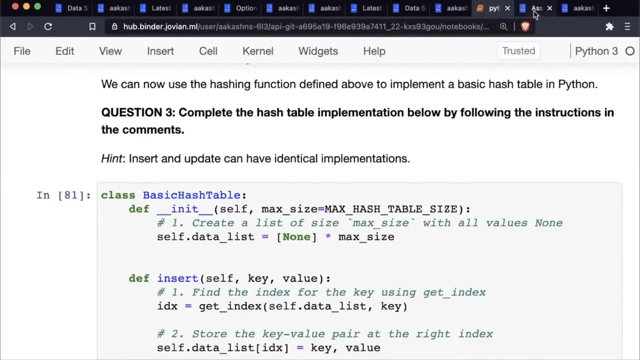 Let's see what question one was very quickly. Question one: create a Python list of size max table- hash size. question two was a pass, So question two was the get index function. Question three was a pass, So question three was complete: the hash table implementation. 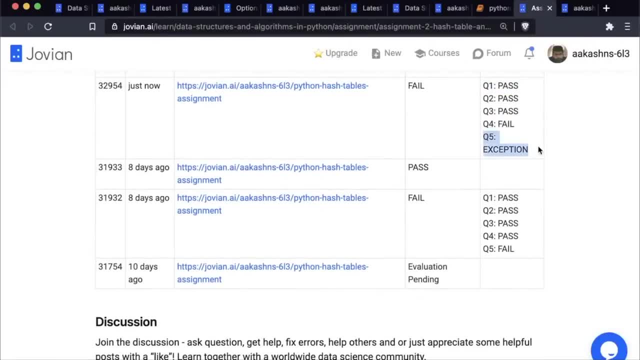 Question four was a field- get valid index. We've not defined it yet. And question five led to an exception, obviously because we have Some Code which will not execute, because we have some blanks that need to be filled in. So keep that. use this as feedback. 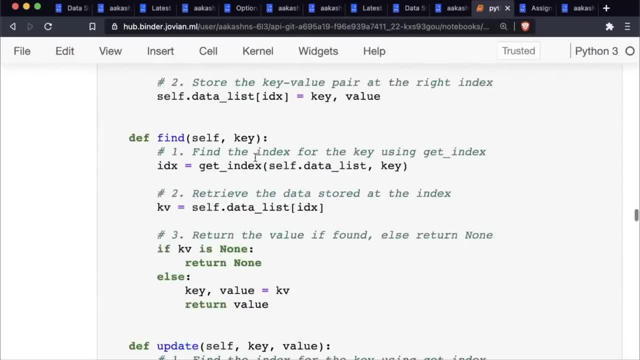 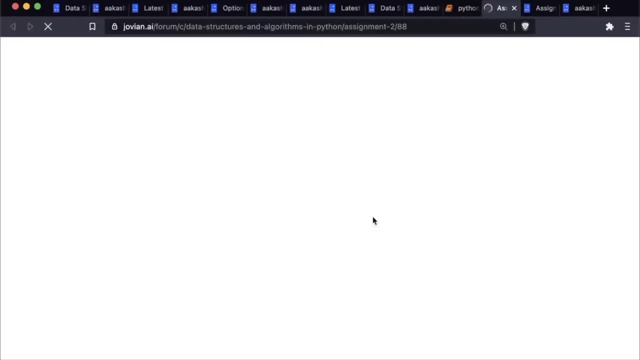 You will know exactly what to fix. And if you are stuck at any point, you know what to do. You can go to the forum. So let's see the forum here. This is the forum subcategory for assignment two. You can create a new topic here. 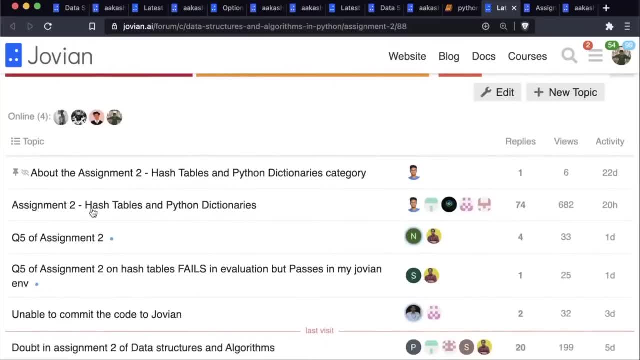 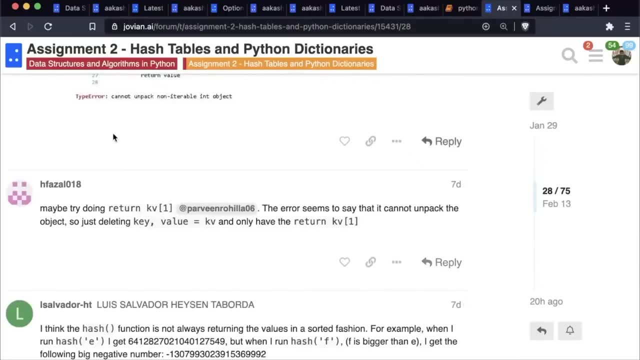 If you want to have a longer discussion, or you can simply go to the main topic- assignment to hash tables- And you can ask a question here. There are already a lot of discussions going on here, So it's possible that your question may already have been answered. 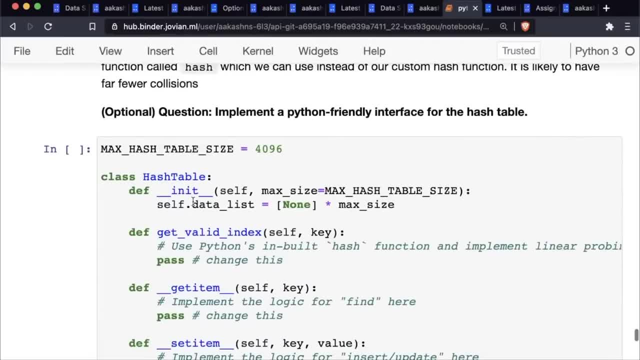 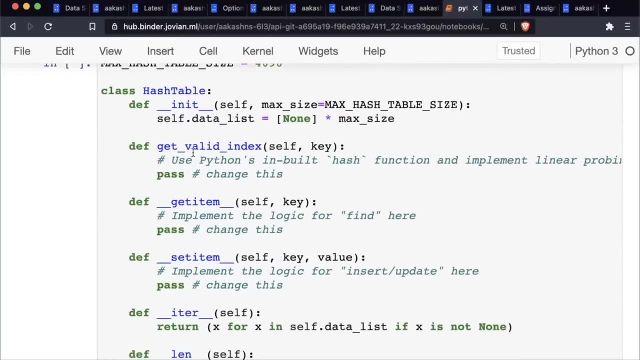 And after this there are also some optional questions. Now here, the option question is for you to implement a Python friendly interface for the hash table. So instead of defining functions, insert, update and find you will define the functions. get item, set item. 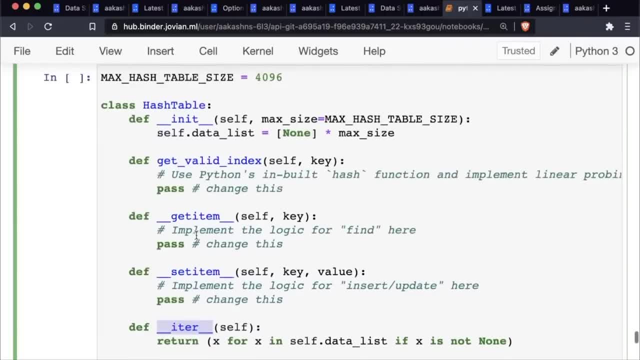 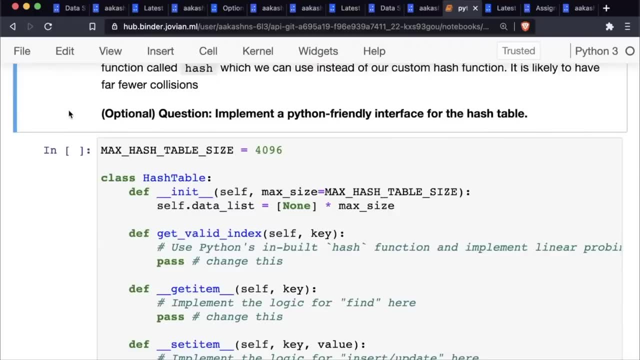 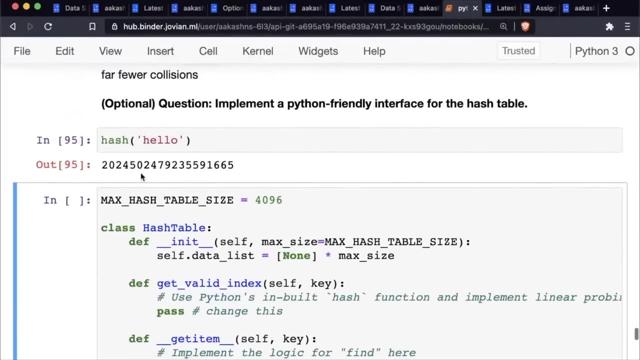 And instead of list all, you will define the function ETA. And also, instead of using the hash function, instead of using the custom hash function that we have defined, you will define a. you will use a function that's inbuilt into Python called hash, and it takes any string or any object and it returns a number for it. 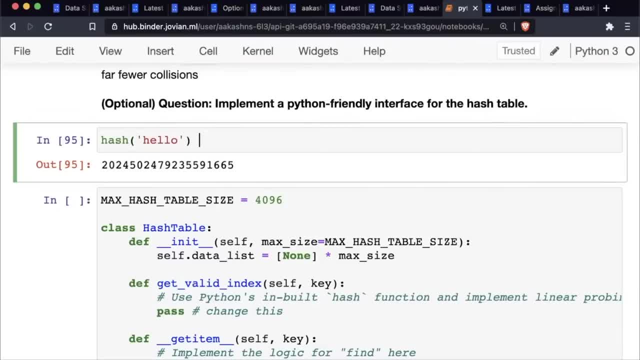 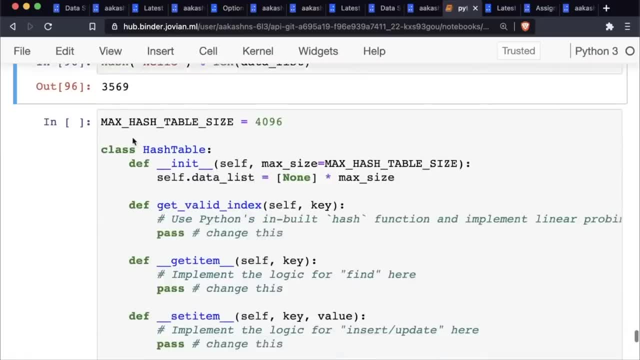 Now, since hash does not accept a list, so you will have to take the remainder manually. So in this case, for example, you've taken the remainder and gotten back the number three, five, six, nine, So you define a hash table here. 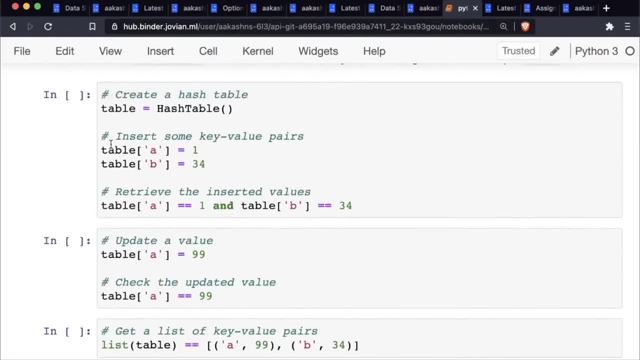 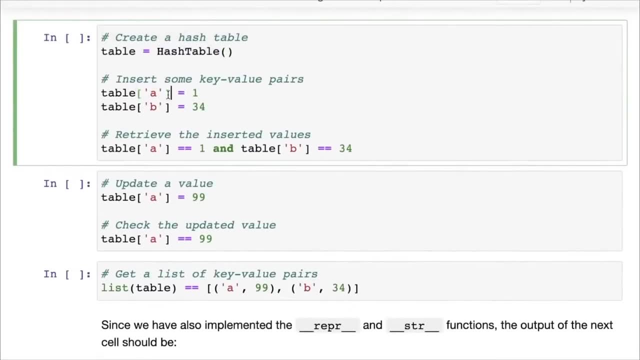 And once you have done that, you will be able to use it just like a Python dictionary. You will be able to use it exactly like this: You create a hash table and then to insert a value, you use the indexing notation and insert the value to retrieve a value. 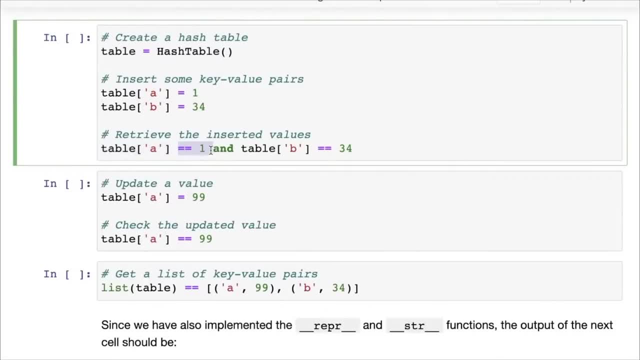 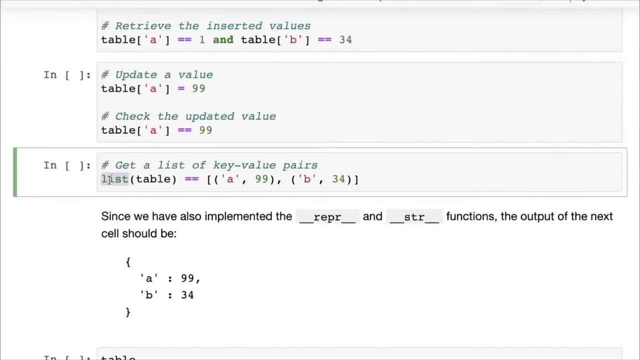 You use the indexing notation to get the value back, And here you can compare it with a number. to update a value, You simply use the indexing notation again, and to get a list of values you simply call the list function. or you can also use it within a for loop. 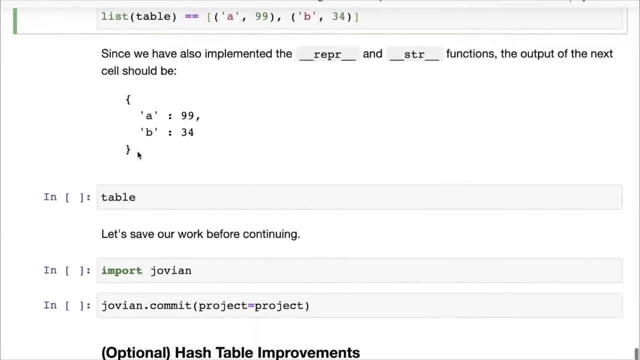 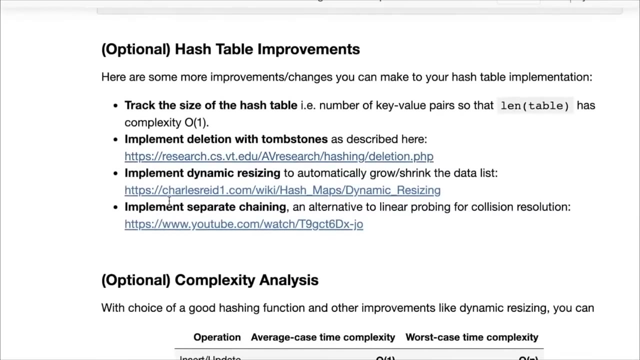 And we've also defined a function called wrapper and STR. What that will do is that will let Python print a representation like this When you simply run a cell which just contains the name of this variable. that's one, And then there are a bunch of improvements that you can try to hash tables. 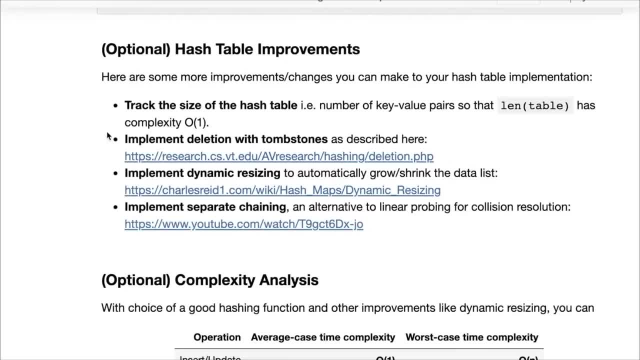 This is a great exercise If you want to improve your Python programming skills and also understand how hash tables work. if you can complete these four exercises, there's pretty much no question related to hash tables that you cannot answer. You will know everything about them. 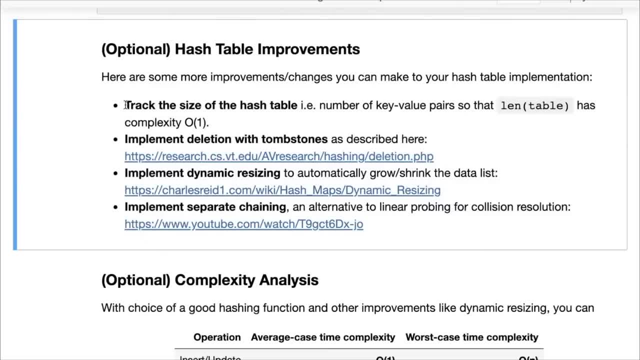 And each of these exercises may take another 30 minutes to 45 minutes, but it's completely worth the time. Maybe spend a set aside a few hours on the weekend to work on these optional exercises. Now here's one: how to track the size of the hash table instead of having to loop through the entire table to get the number of key value pairs. 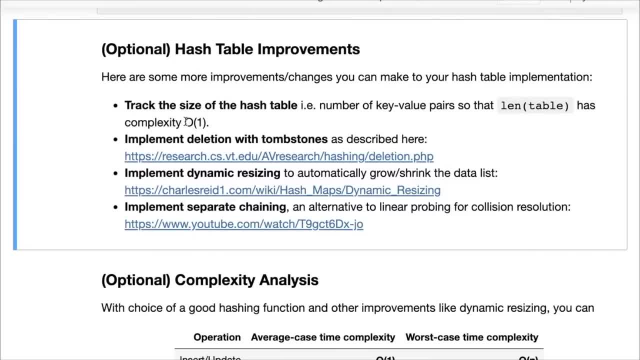 Can you store the length somewhere so that you can track it And Size order? one Here's one: to implement deletion. So to implement deletion, you have a topic called technique, called tombstones that are used. They can use this tombstone technique and implement it, just a little more code. 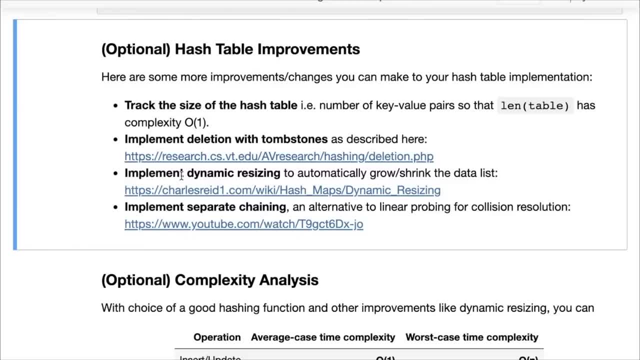 Can you implement dynamic resizing? So, instead of starting out with a hash table of a given size or requiring the user to specify a size, can you, or maybe start with a hash table of, let's say, one 28 elements and then double it as soon as you reach one 28 elements, or maybe even before, to avoid? 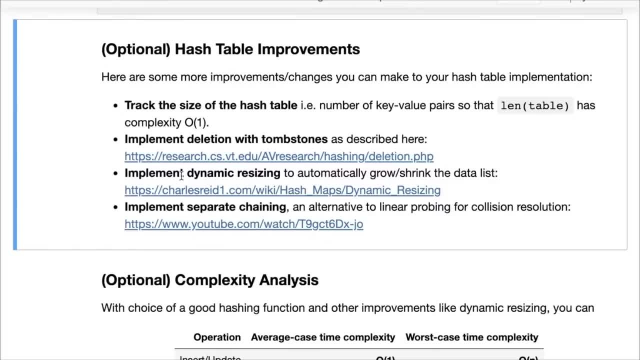 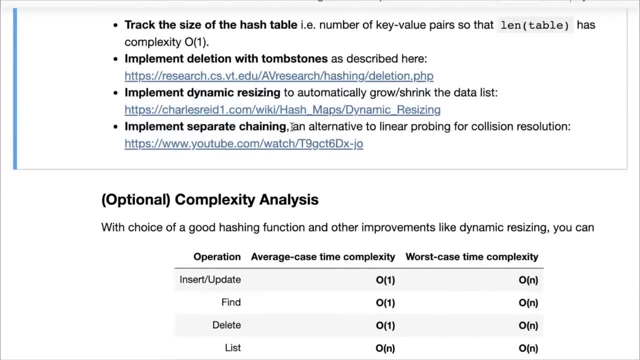 Collisions. You may want to double it as soon as you reach 64 elements, like 50% of the capacity. So dynamic resizing is the technique that allows you to automatically grow and shrink the data list internally. And then the here's another technique for coalition resolution. 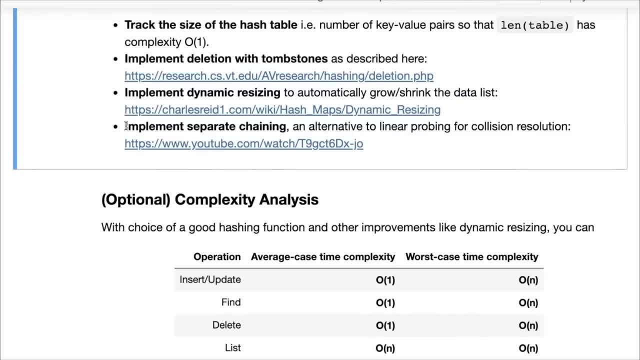 This is called separate chaining. So, instead of going to the next index, what you do is you maintain a linked list at each position and for all the key, for all the keys, you still use that position, but you look through the link list while looking for a key. 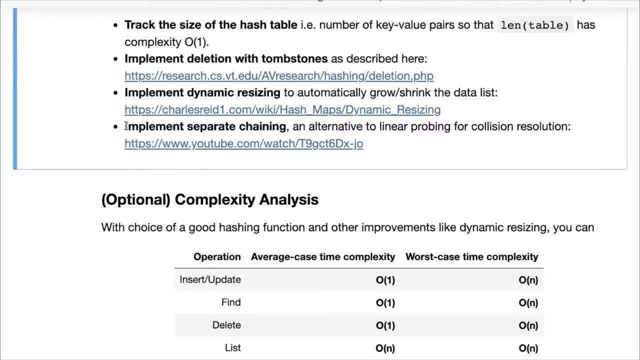 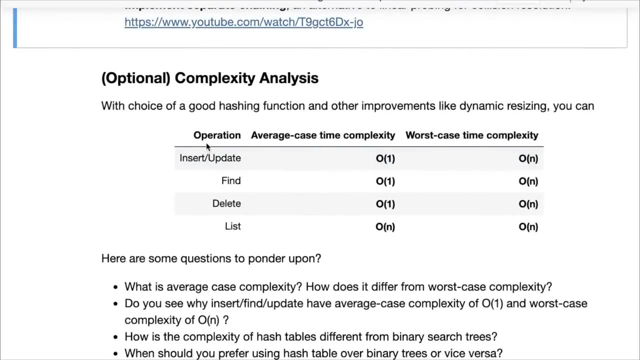 Or you add a new element to the link list for that position, If you're adding a new key there. So here's separate chaining explained in a YouTube video. You can look through that and try to explain it on your own. And one final thing: here is also the complexity analysis. 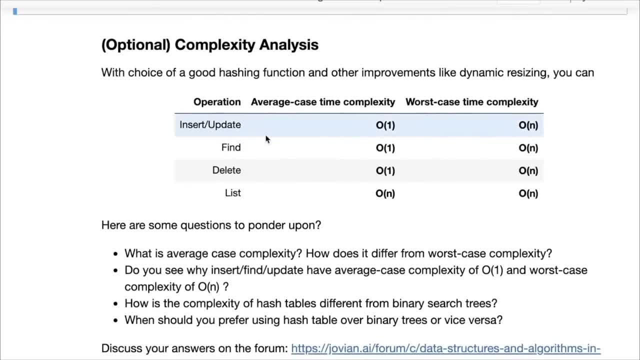 And here's where you talk about average case time complexity. because on average, if you have a good hashing function and you've implemented some improvements like dynamic resizing, then the average Complexity for insert, update, find and delete are order one and list, of course, is still ordering. on the other hand, the worst case time complexity, because there can be collisions- are still ordering. 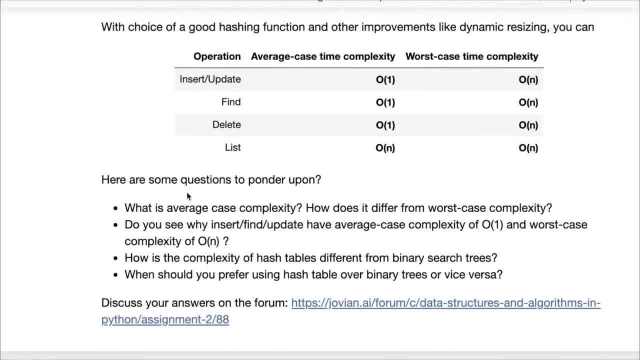 So here's something for you to ponder upon: What is average case complexity and how does it differ from worst case? complexity is also something that is discussed in lesson three of the course, where we talk about quick sort, and you see why. insert, find an update, have an average case. 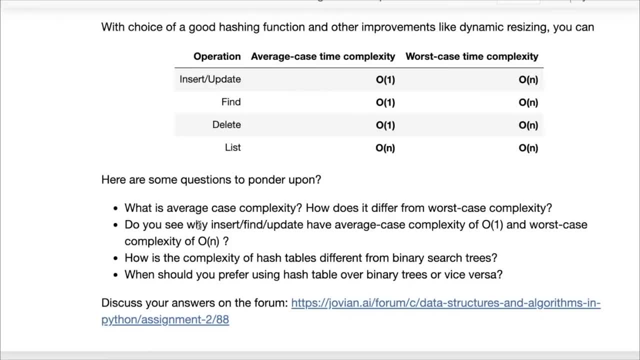 Complexity of order One and, a worst case, complexity of ordering. If not, it is something that you can look up online. try to see if you can search a tutorial and learn why this happens. Then how is the complexity of hash tables different from that of binary search trees? 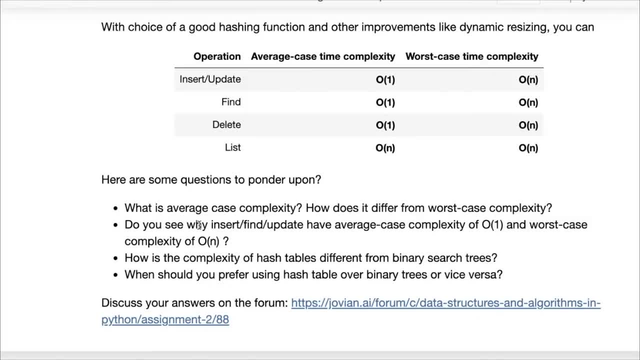 We've discussed binary search trees in a lot of detail in lesson two. Another question becomes: when should you prefer using hash tables And when should you prefer using binary search trees, or vice versa? So all these very interesting questions, And you may get asked some of these questions in interviews as well. 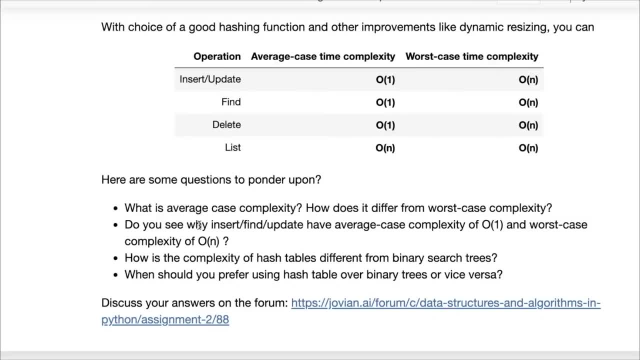 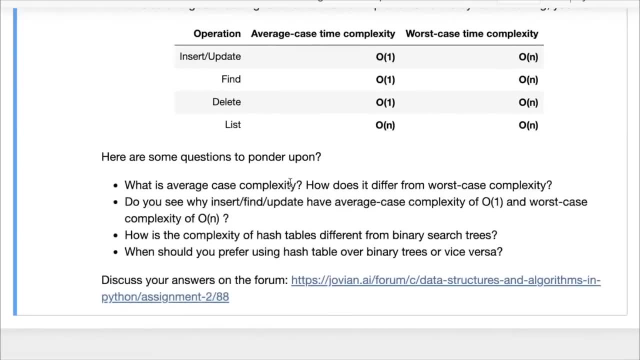 It will help you especially to ponder upon some of these questions. even if you do not end up solving all of these optional questions, do look at the complexity analysis and think about it, And there's a forum thread where you can discuss your thoughts. 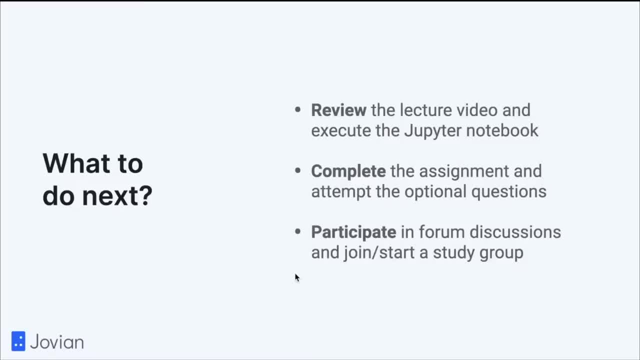 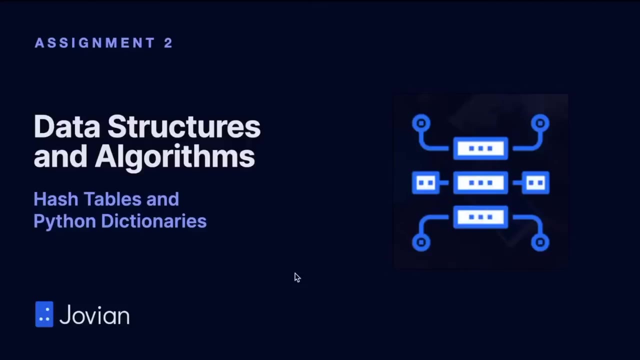 So what do you do next? Review the lecture video, review the assignment walkthrough video and execute the Jupyter notebook, Complete the assignment and attempt the optional questions as well, And do participate in forum discussions. So this was a walkthrough of assignment two of data structures and algorithms in Python. 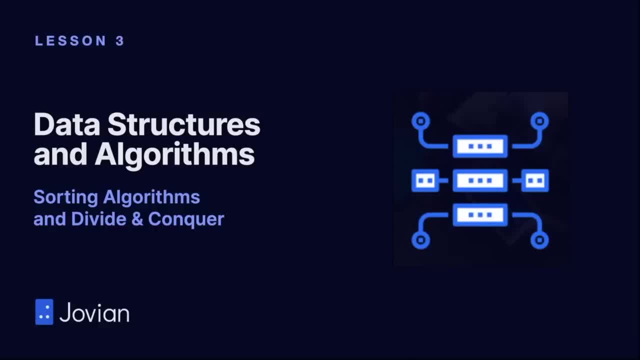 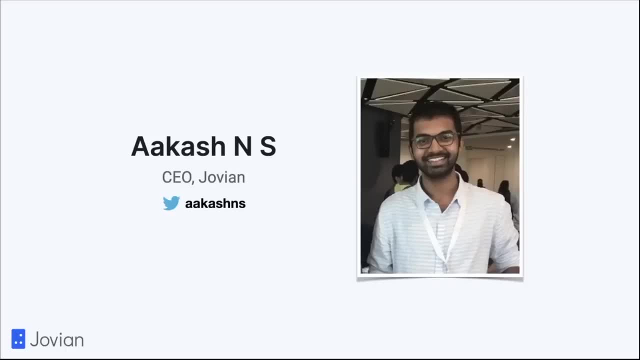 Hello and welcome to data structures and algorithms in Python. This is an online certification course conducted by Jovian, And today we're on lesson three. My name is Akash, I'm the CEO of Jovian and I'm your instructor for the course. 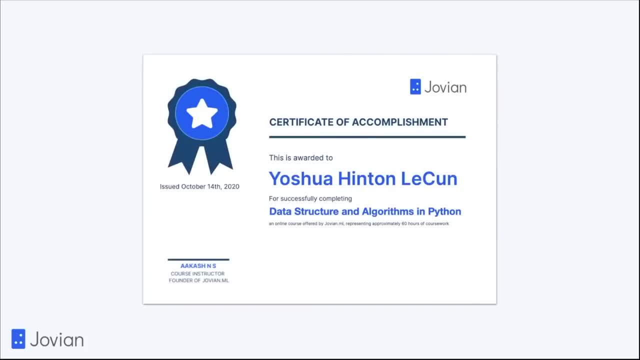 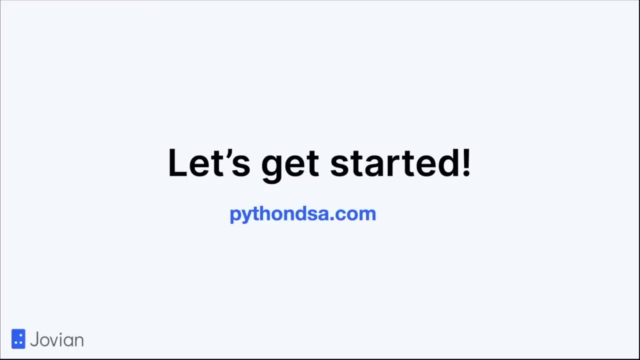 If you follow along with this course and complete four weekly assignments and a course project, you can earn a certificate of accomplishment for this course. So let's get started. The first thing we do is visit the course website, pythondsacom. 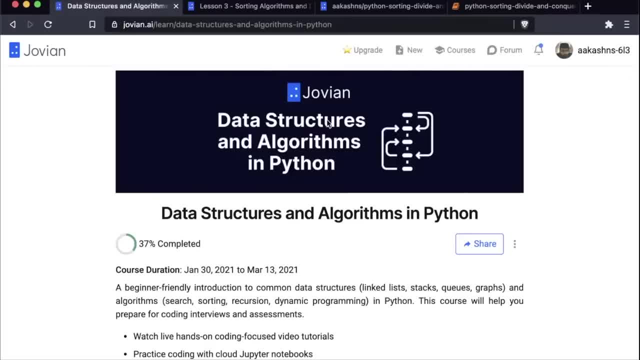 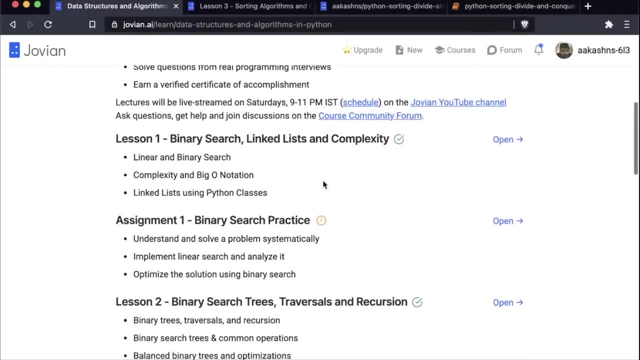 So when you visit pythondsacom, this will bring you to the course website. Here you can find all the information and material for it. For the course, you can check out lessons one and two and assignments one and two, both of which are still open for submission. 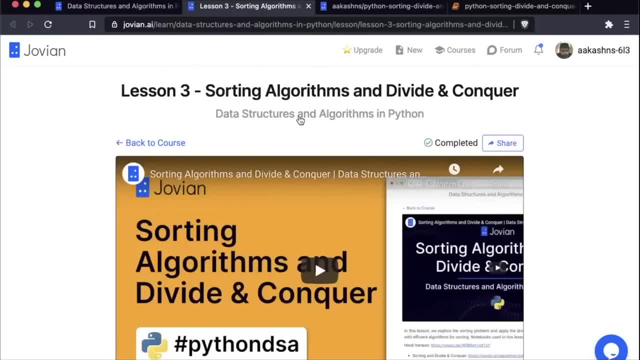 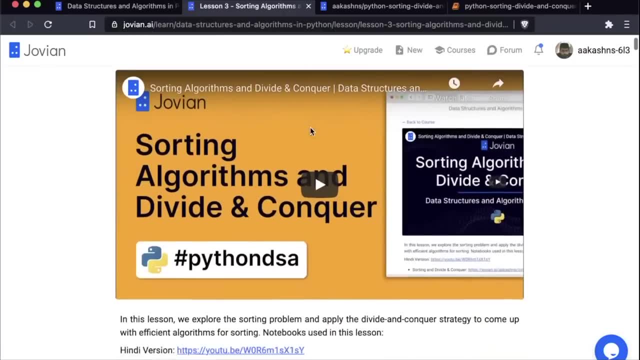 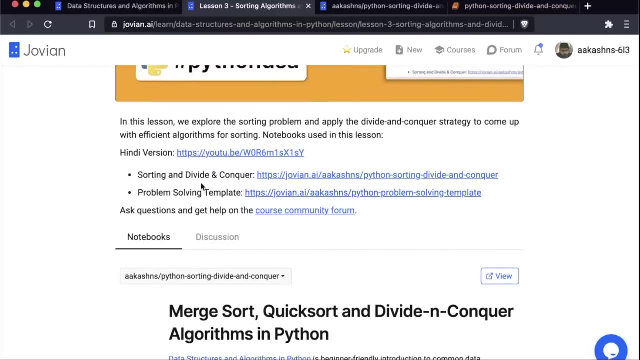 And let's open up lesson three. So the topic today is sorting algorithms and divide and conquer, and you can watch a video recording of the lesson here. You can also catch a version in Hindi. Now the code used for the lesson is provided. 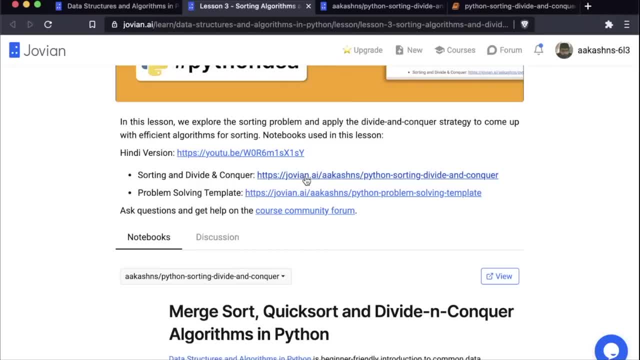 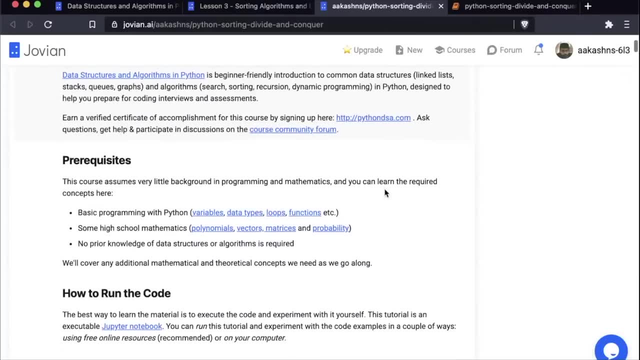 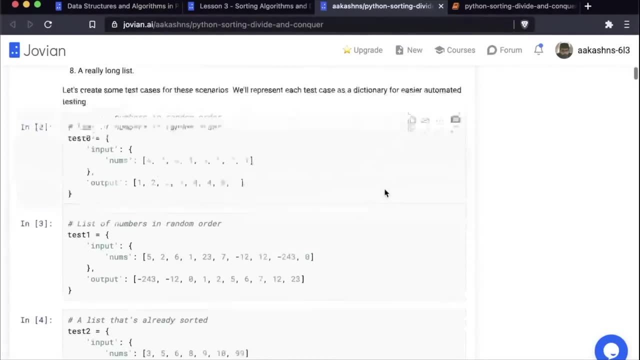 Here. So let's open up this link. sorting and divide and conquer. This is where all the code is present. So here we have it. Now we are looking at the tutorial and the code for this lesson. If you scroll down, you can see that there is some code here. 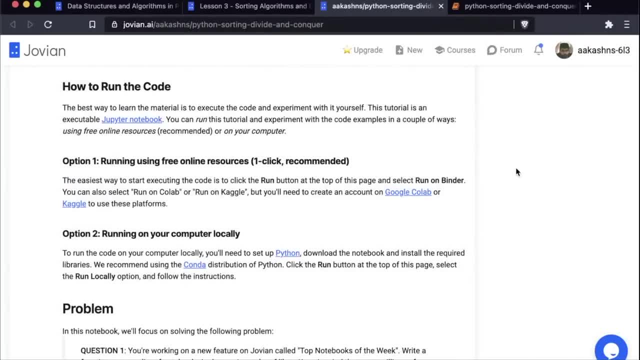 Now to execute this code, you have two options. You can either execute this code online using free online resources, which is what we recommend, or you can download it and run it on your computer locally, And the instructions for both of these are given here. 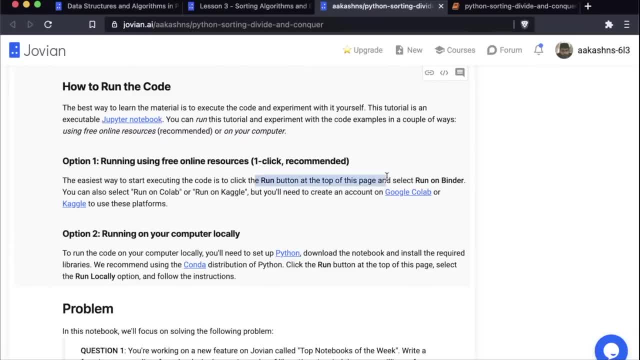 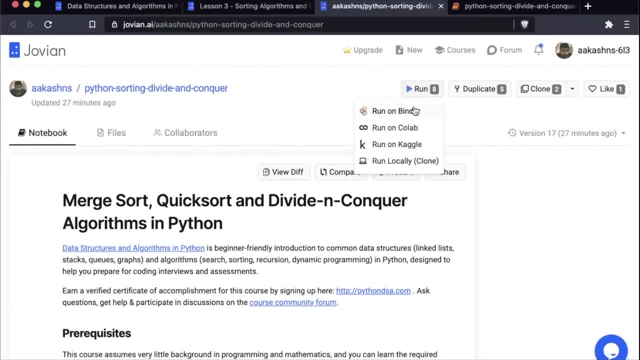 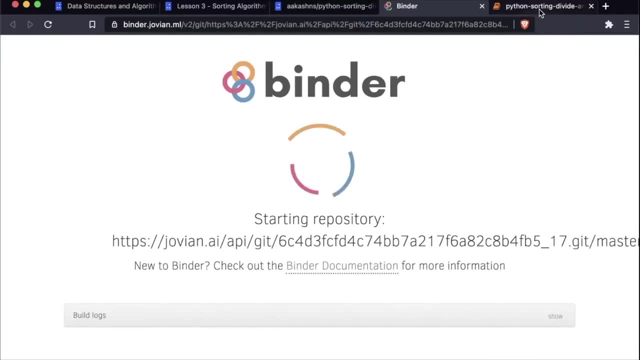 We are going to use the first one, which is to click the run button at the top of this page and select run on binder. So let us scroll up here and let us click the run button and then click run on binder Now. once you do this, it will open up an interface. 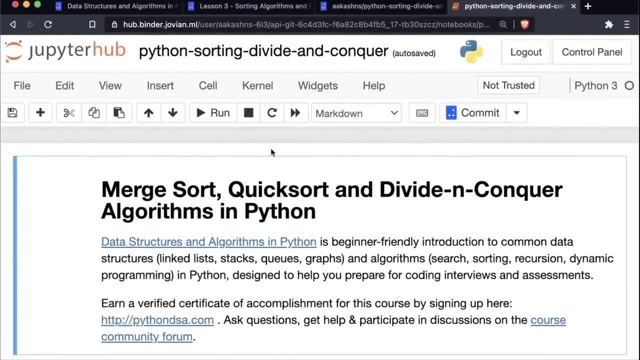 Like this, And what you're looking at here is a Jupiter notebook. So a Jupiter notebook is an interactive programming environment where you can write code, look at the results and you can also write explanations, And we've provided you with a cloud-based Jupiter notebook set up. 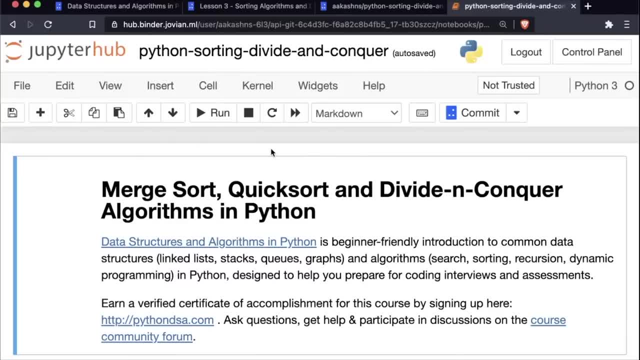 So you don't have to install anything. All the code that you execute here will be running on our cloud, but you can also download it and run it on your own computer by following the instructions. So the first thing we'll do is click on the kernel menu and click restart and clear output to remove any of the outputs from previous executions of the code. 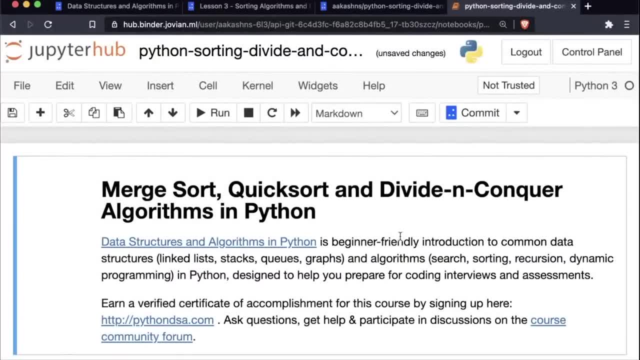 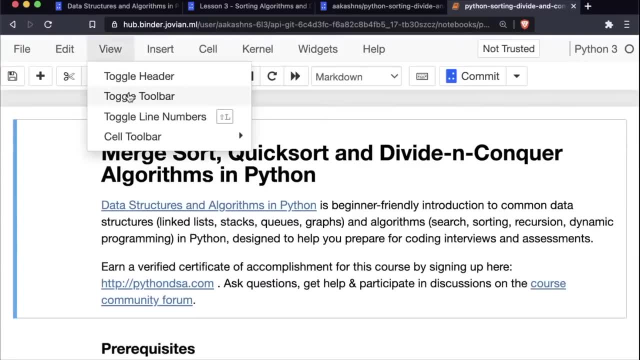 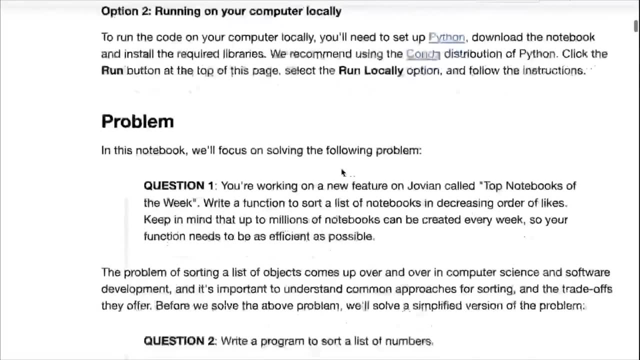 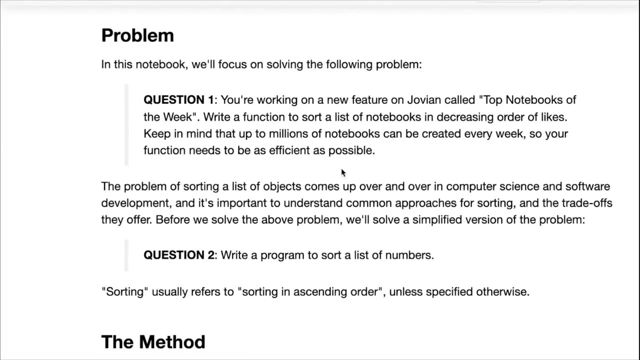 So that we can execute the code and see the outputs fresh for ourselves. Now I'm also going to zoom in a little bit here, so we can look at the code and let's get started. So this is a coding focus and practical course And we're talking about different data structures and algorithms. 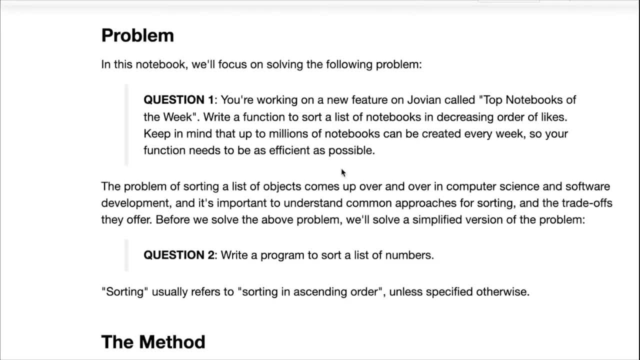 The topic today is sorting algorithms and divide and conquer algorithms in Python. So in every lecture we focus on a specific problem. So in this notebook, in this tutorial, we will focus on this problem which you're looking at here. So let's read the question. 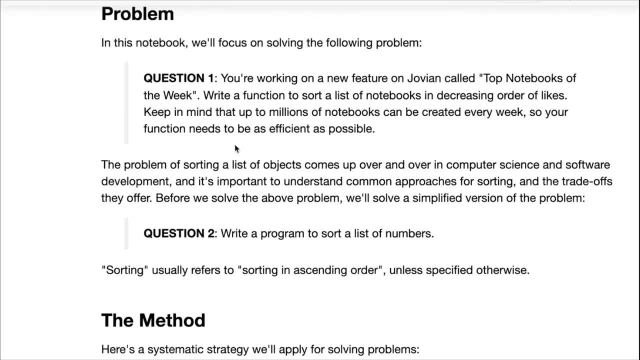 You're working on a new feature on Jovian called top notebooks of the week right, A function to sort a list of notebooks And decreasing order of likes. keep in mind that up to millions of notebooks can be created every week, So your function needs to be as efficient as possible. 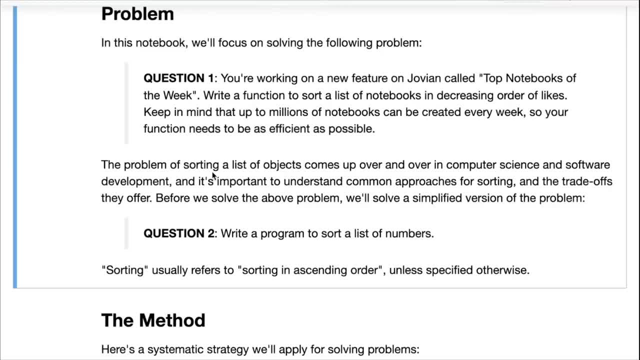 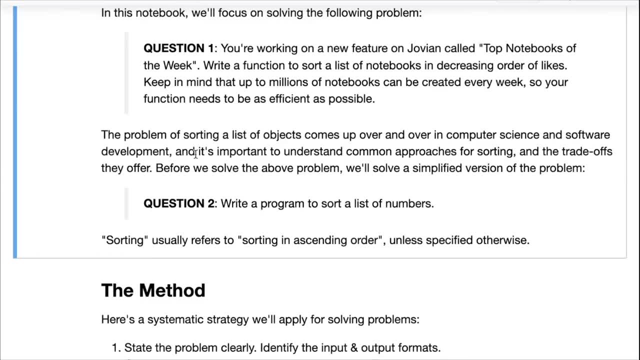 That is the key point here. Now, this is a classical problem in computing, the problem of sorting a list of objects, and it comes up over and over in computer science and software development, And it's important to understand common approaches for sorting how they work, what the trade-offs are between them and how to use them. 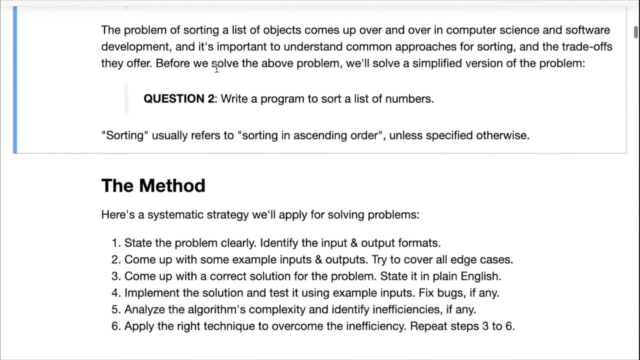 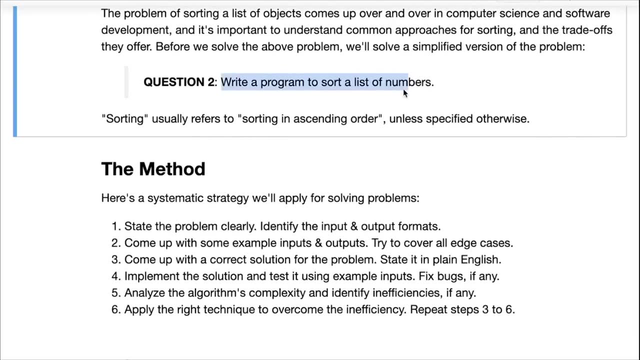 So before we solve this problem, we'll solve a simplified version of the problem. It's quite simple to state: write a program to sort a list of numbers, and sorting usually refers to sorting in ascending order, unless specified otherwise. So that's our question for today: write a program to sort a list of numbers- and we'll expand upon it to answer this original question as well. 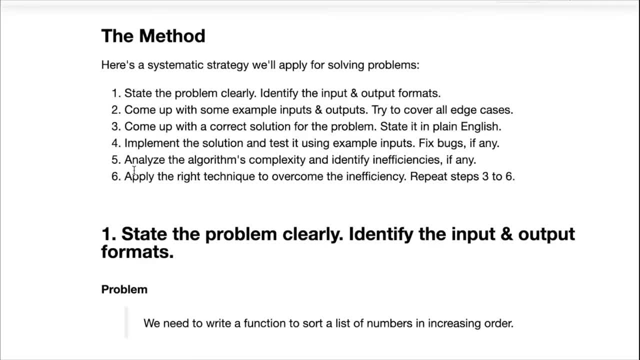 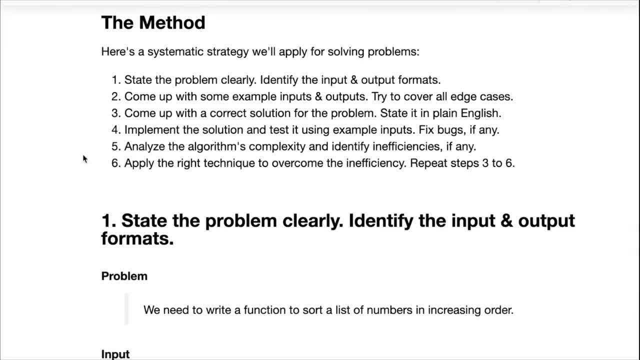 Now, this is the method that we've been following throughout the course, and we will continue to follow a systematic strategy for sorting. So let's start with solving programming problems. Step one: state the problem. clearly identify the input and output formats. 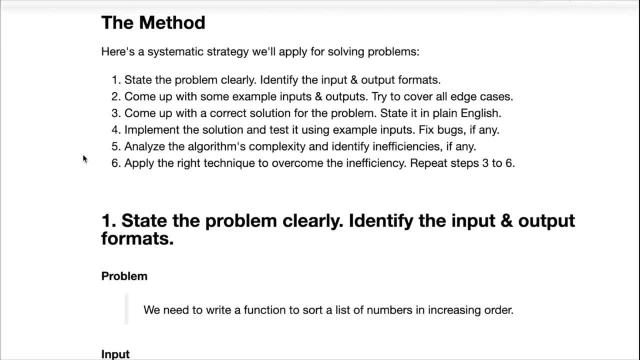 Step two: come up with some example inputs and outputs and try to cover all the edge cases. and step three: come up with a correct solution for the problem, stated in plain English. Step four: implement the solution and test it using example inputs. So this is very important: that you implement the simple solution. 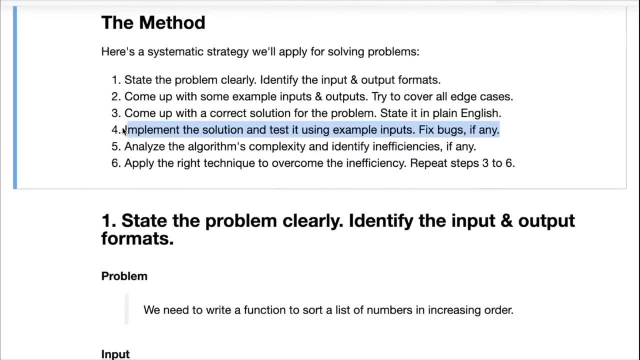 So you just need a correct solution first- not the efficient one- And then you implement it. Then you analyze its complexity, identify inefficiencies, and then you apply the right techniques to overcome the inefficiency. And that is where the knowledge of the right data structures and algorithms comes into picture. 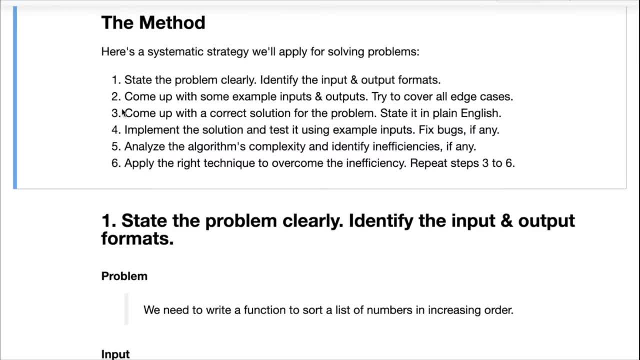 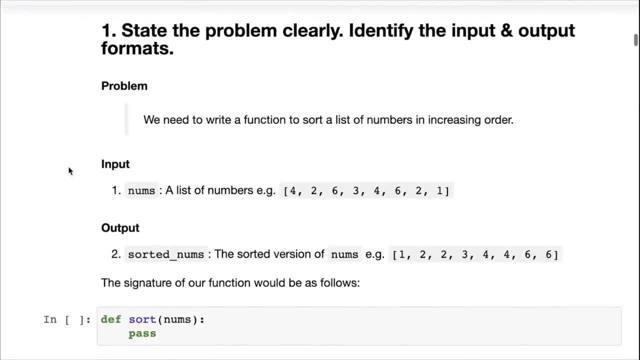 And once you apply the new technique, then you once again state the solution, implement it and analyze its complexity and repeat if necessary. So this is a strategy we'll follow here today as well. So step one: state the problem clearly and identify input and output formats. 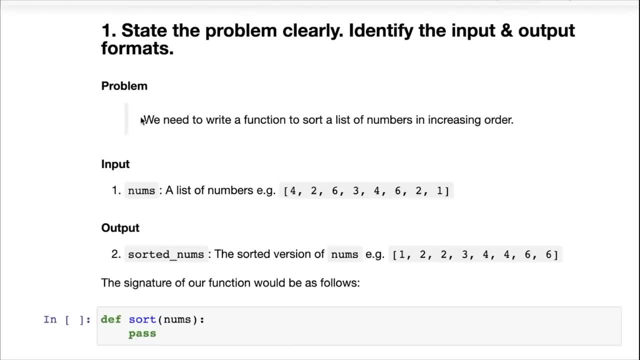 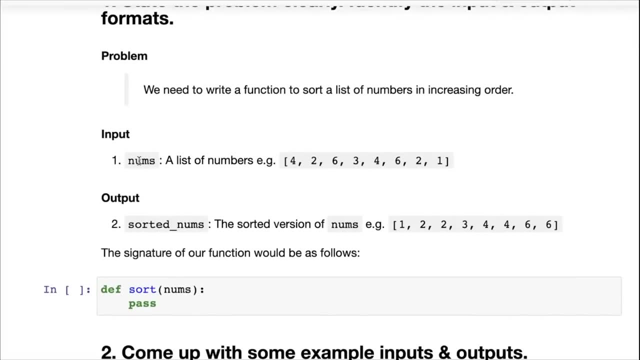 Now the problem is stated clearly enough for us. We need to write a function to sort a list of numbers in ascending or increasing order. Now here's the input. The input is a single argument called nums, and that is a list of numbers. 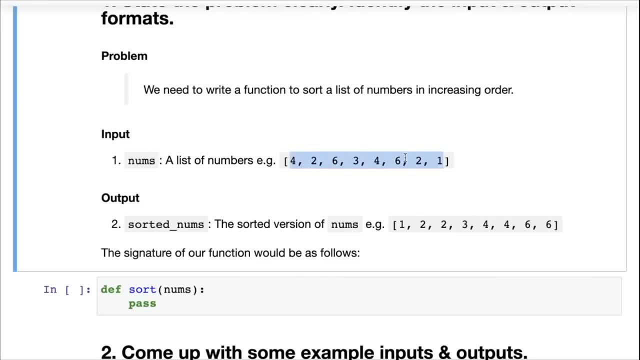 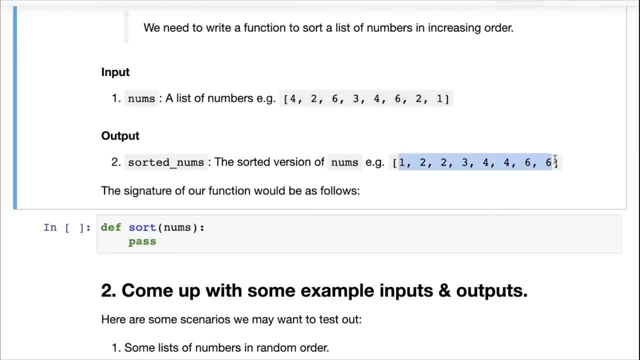 So, for instance, here's a list of numbers. You can see that they're not in any specific order, And then the output is the sorted version of the input. So here is the same list of numbers in sorted order, And based on these two we can now write a signature of our function. 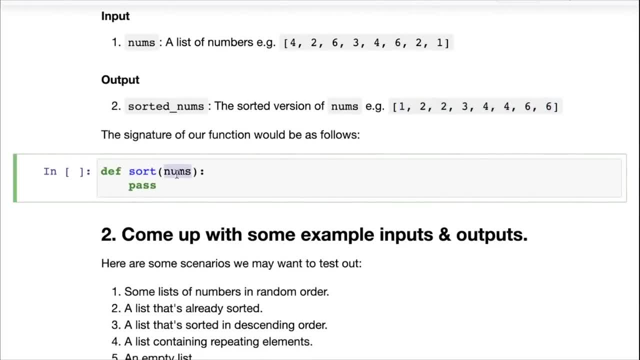 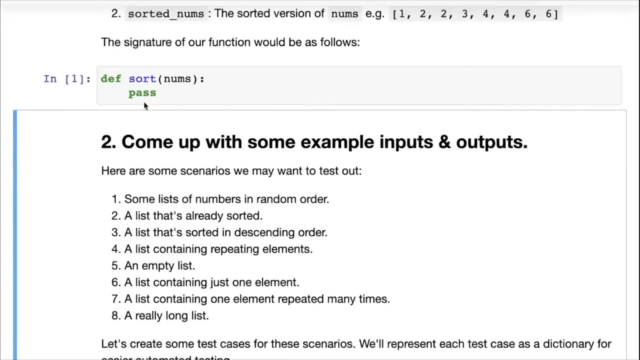 So our function will be called sort Or something else, but it will accept just one input, And right now we've not written any code here, So we just put in pass. Now I'm running this code here using the shift plus enter shortcut, but you can also use the run button on the toolbar. 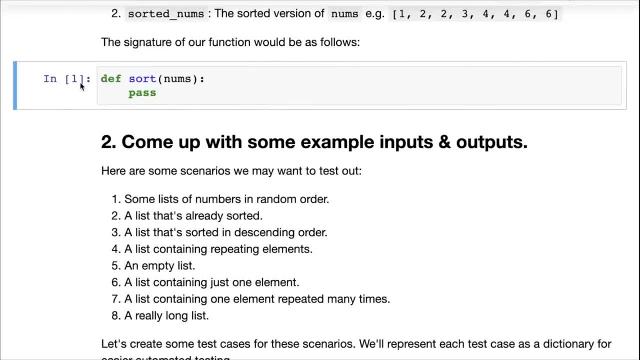 So either run or shift plus enter. And the great thing about Jupyter notebooks is that you can add more code cells anywhere and test anything that you want. For instance, if you want to insert a code cell below, just click the insert cell below. 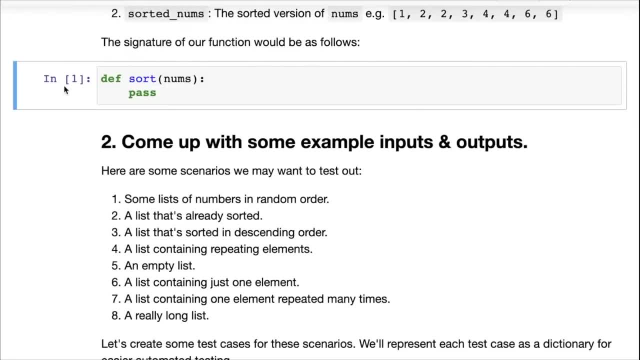 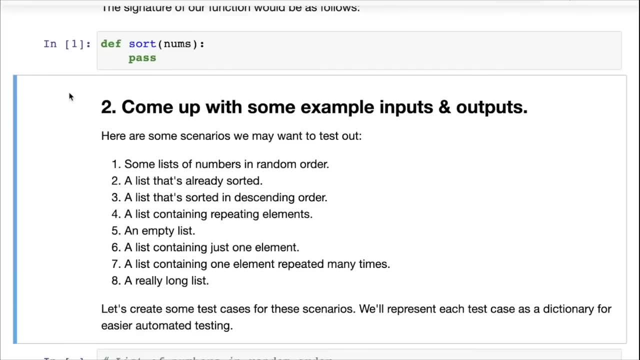 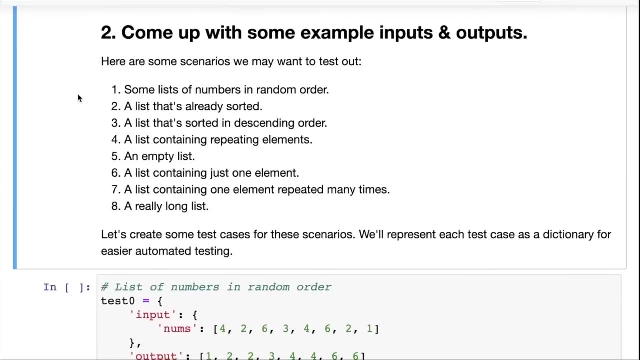 Menu option, or click outside a cell on the left and press the B button, And now you can write some code here and run it. So please feel free to experiment with this notebook as you go along. So step two: come up with some example: inputs and outputs. 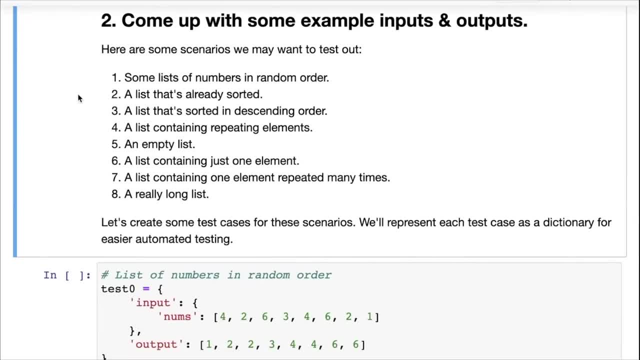 Now, this is very important. You need to think about all the different scenarios in which you may want to test out your function before you put it into production, so that you catch errors early on, And thinking about scenarios will help you identify what are the special cases you need to handle in code. 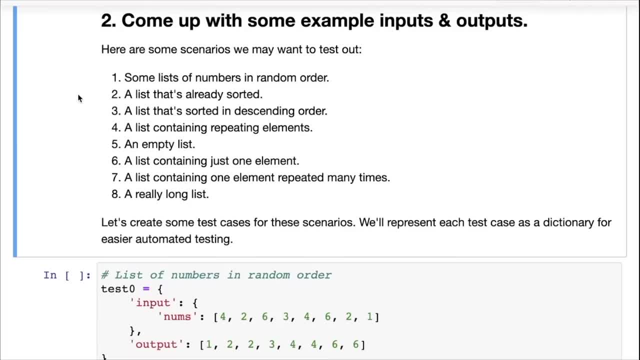 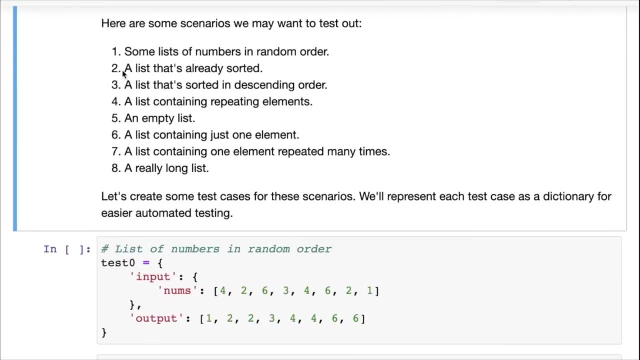 And it's easier to do it right now than while writing your code, because that may lead to bugs. So here are some scenarios that I was able to come up with, and there may be more, so you can continue and increase this list. 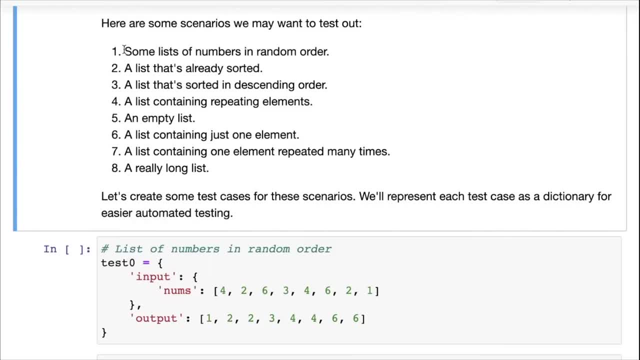 So the first one is some list of numbers in random order, some numbers in any random order, and you can try slightly smaller lists and larger lists, and so on. Second Is a list that's already sorted. We need to ensure that an already sorted list does not become unsorted. 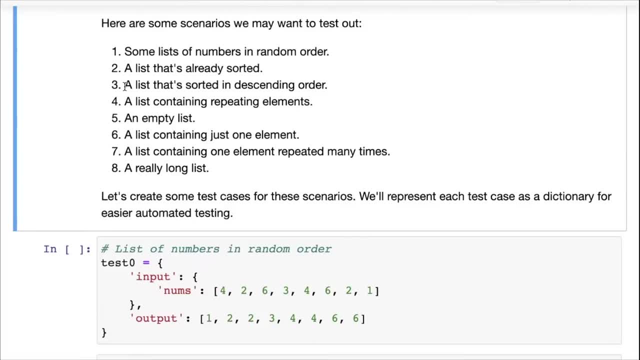 A third is a list that sorted in descending order. We may want to check that, see if we need to handle that case separately somehow. then a list containing repeating elements. This is something you may not have thought of, but the question never said that the number should be unique. 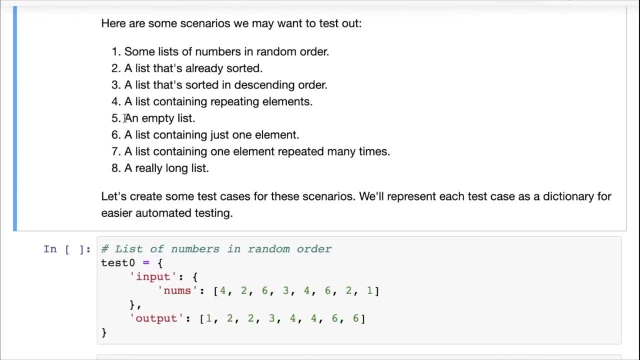 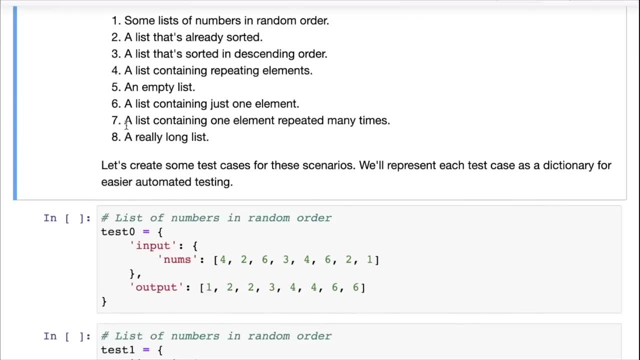 So that could be repeating elements here. An empty list, interesting input. The output is also an empty list, or a list Containing just one element, or a list containing one element repeated many, many times, or even a really long list. This is something that we may want to test, because we want our algorithm to be efficient at the very end. 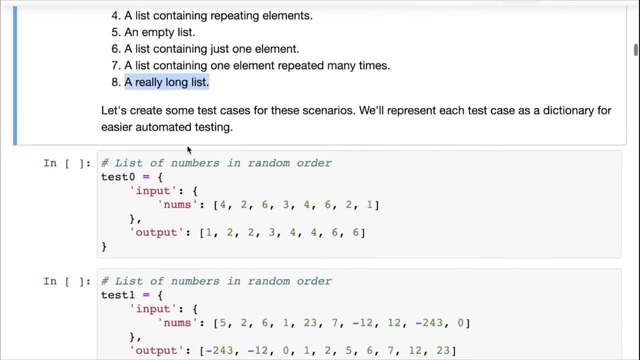 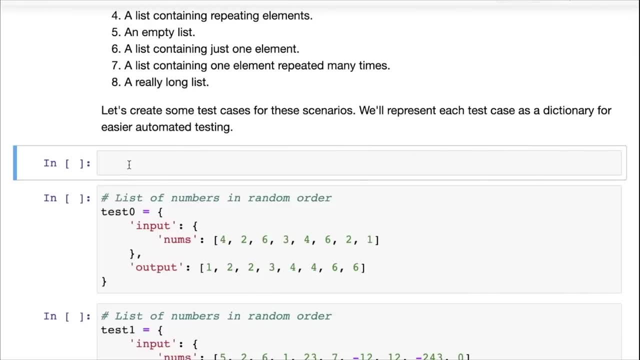 So long list may help us just evaluate the efficiency empirically. So these are the scenarios And what we now need to do is create some test cases for these scenarios. So test cases involve creating an input and an output, For instance. here's an input: 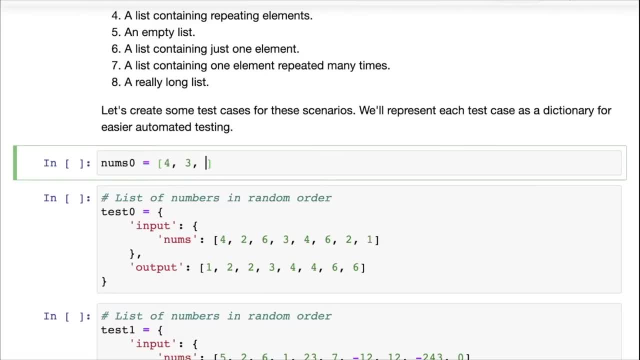 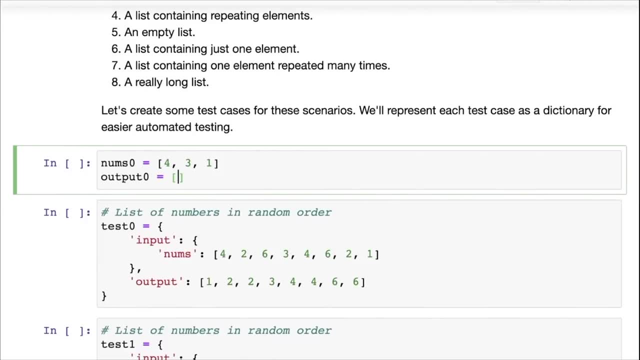 Num zero And this could be the list: four, three, one. and here's the expected output. So let me call it output zero and this would be one, three, four. Now, this is a good way to put to create a test case and you can use it later for testing, but we will put our tests into this particular structure. 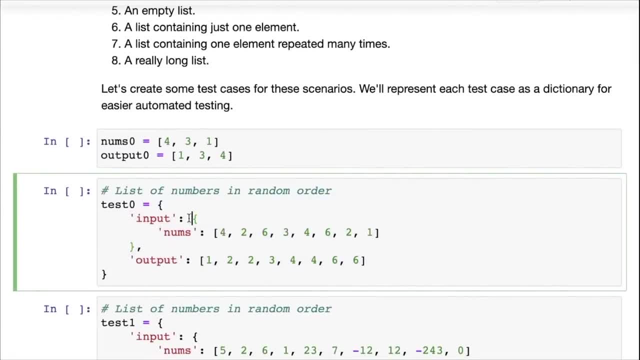 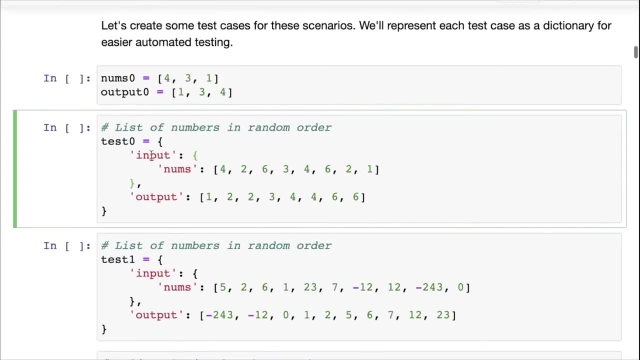 We'll create a dictionary, and creating a dictionary like this will help us automate the testing of all our test cases with a single helper function. So what we're going to do is, for each test case, create a dictionary, and then it will have two keys. 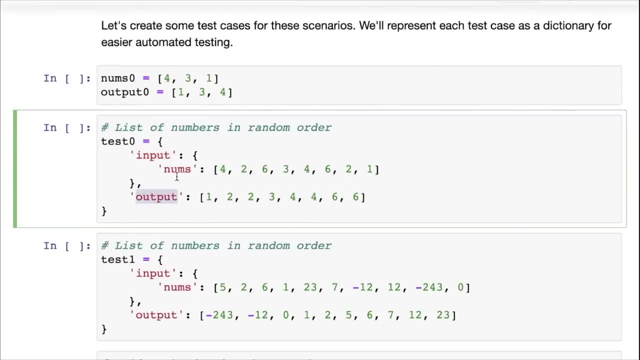 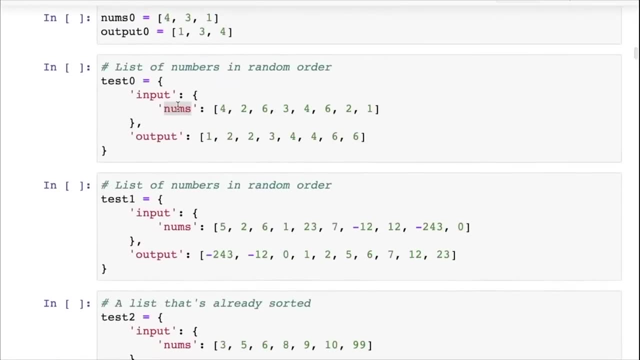 First key is called input And the second key is called output. And in the inputs, for each of the arguments that go into the function- And remember, there's just one argument here- We will have one key, So we will have the key nums and the key nums will have the input value for the test case and the output will simply contain the output. 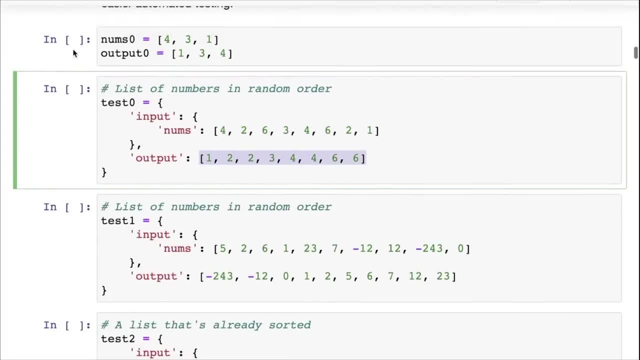 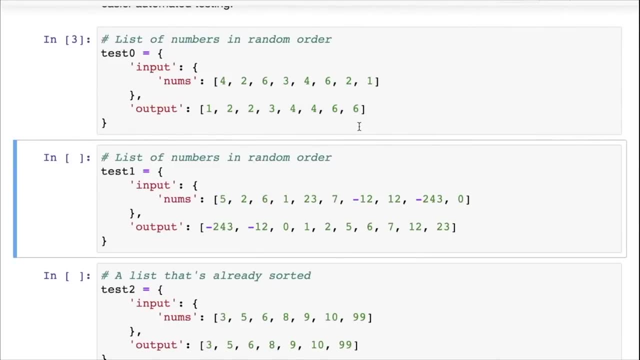 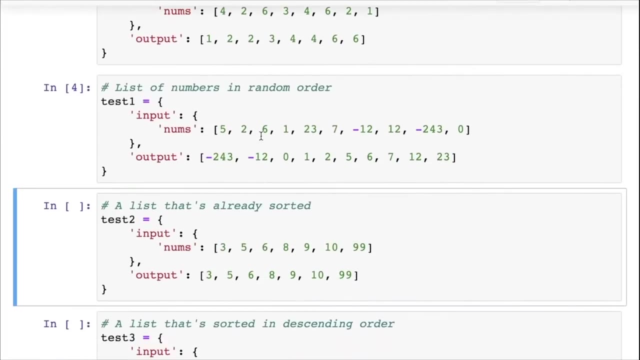 Returned By the function. So that's how we'll set up our test cases. So does our test zero. a list of numbers in random order. Then we have test one. This is also another list of numbers in random order. You can see here no specific order. 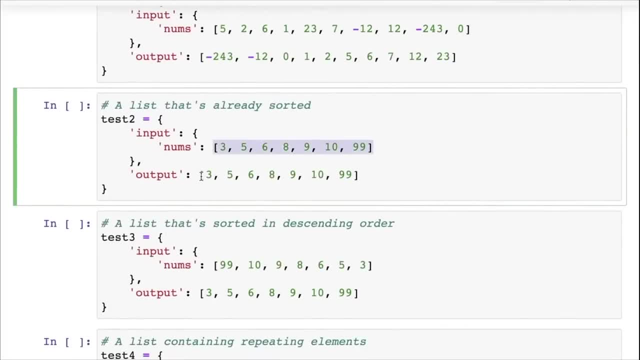 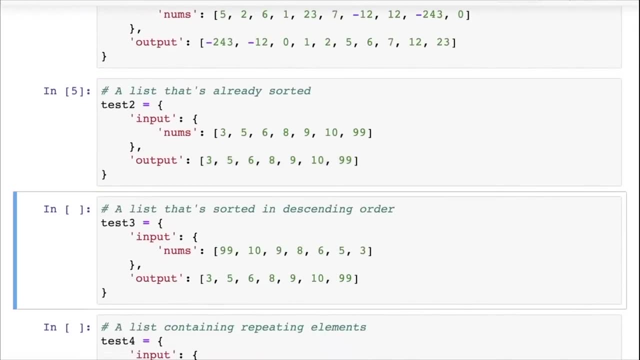 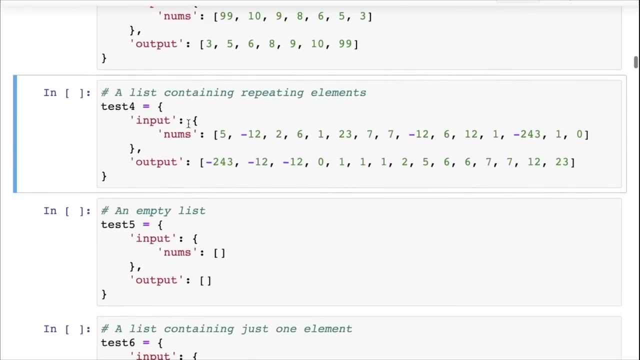 Now we have a list that's already sorted and the output obviously is the same. now for the random ordered list. The output is the same numbers in sorted order. Now we have a list That's sorted in descending order and the output is the same list and increasing order. 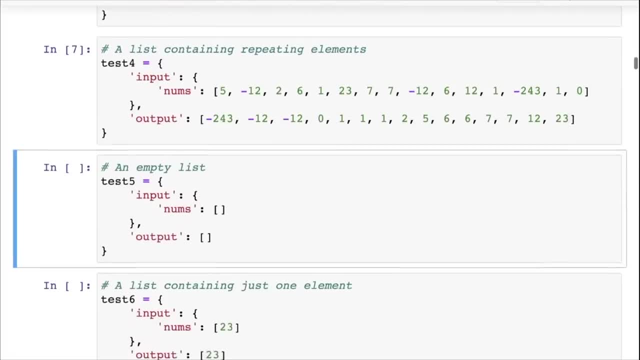 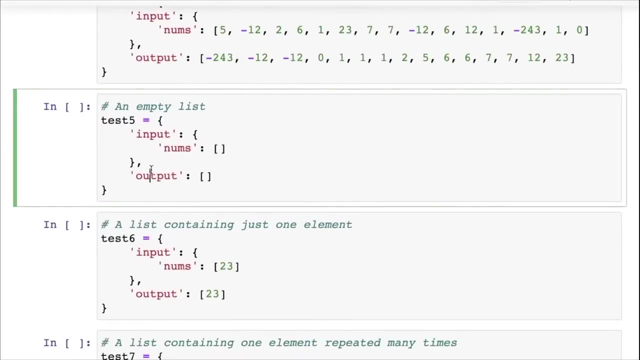 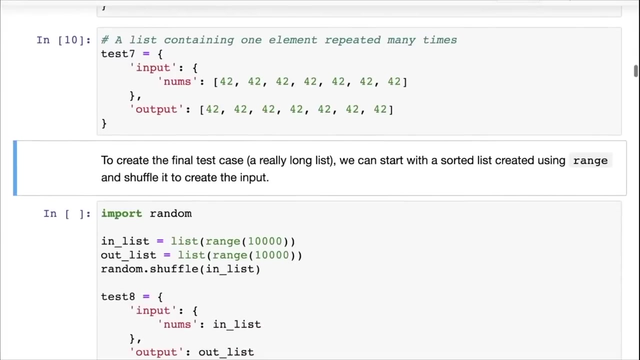 Then we have a list containing repeating elements. You can see that the numbers one, two, six and seven, and even minus 12 repeat here. Here we have the empty list, Here we have a list containing just one element, And here we have a list containing one element repeated many, many times. 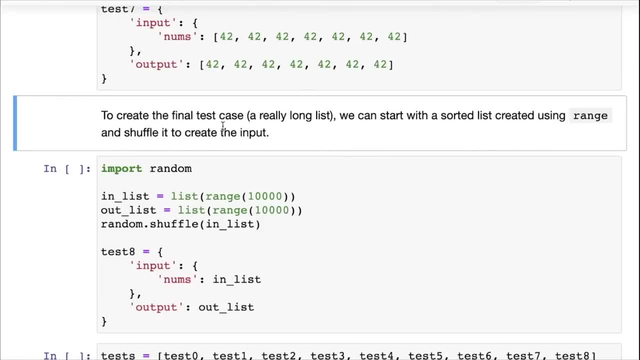 And then the final test case, which was to create a really long list. That's where we can start with a sorted list created using the range function and then shuffle it to create the input. Otherwise, you may spend a lot of time just creating a list and then writing the sorted version of it. 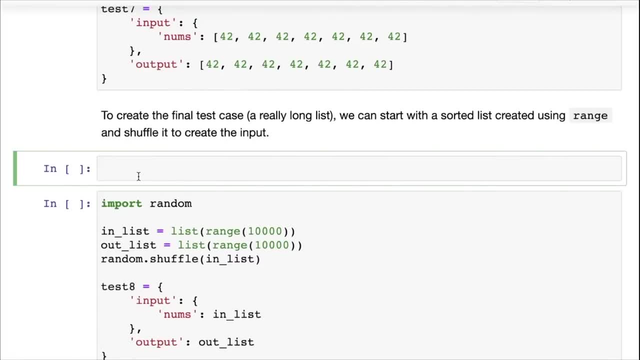 That's too much work. So always use a computer, always use helper functions whenever you can, even to create test cases. So we'll use the range function. Now. the range function takes either a single number or two numbers, So you can have something like this: range two to 10, or just range 10.. 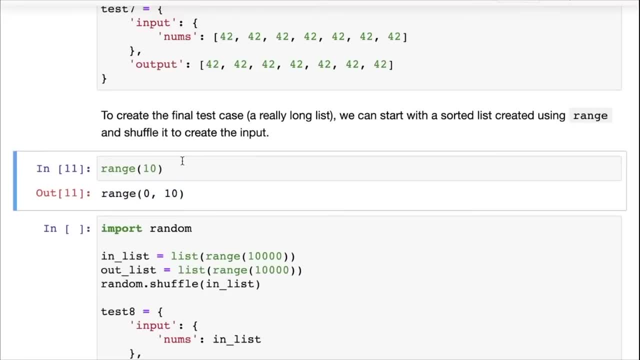 And if you just look at it this way, it just prints range zero to 10.. Now, if you actually want to see what's in it, there are a couple of ways you can do: list range 10, and that gets converted into a list, or you can use it in a for loop. 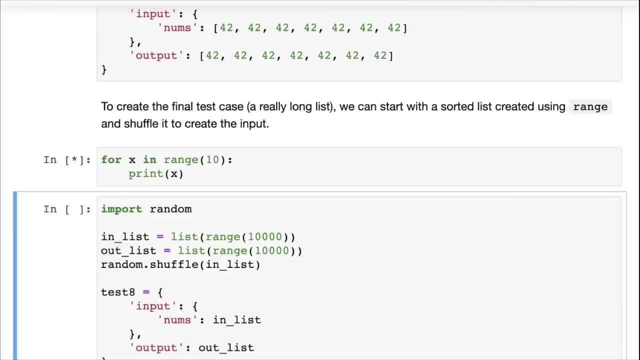 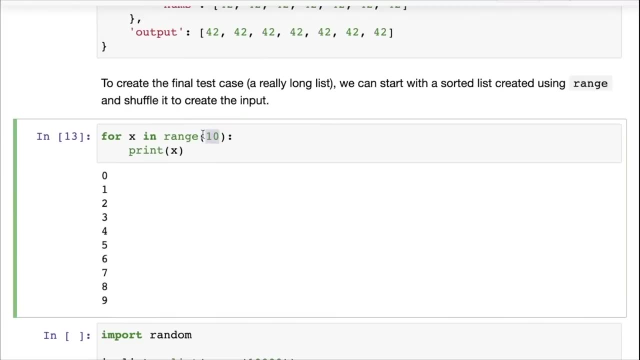 So you can put for X in range 10. print X So you can see that it contains the numbers zero to nine and that's important, that the range does not include the end element of the range. Okay, So just keep that in mind. 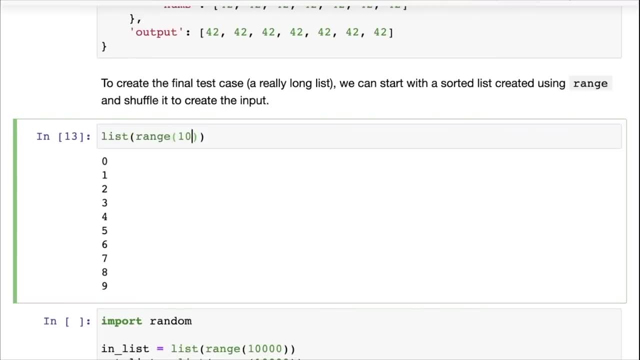 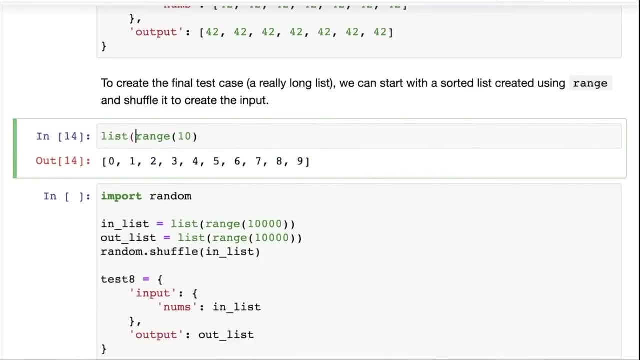 Now what's the difference between a range and a list? A list contains all the 10 numbers together at once, but a range internally simply maintains a counter. So when you use a range in a for loop, it simply starts the counter from zero and increments it up to the starts- the counter from the starting value. 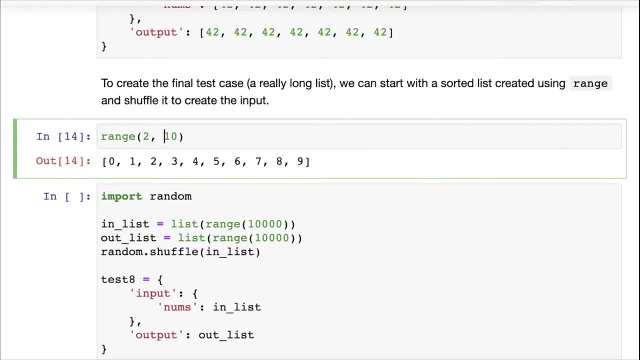 So if it's two to 10, then it starts a counter from two and increases it up to the end value minus one, So it does not use as much space as a list. It simply uses a one Single variable internally, And that's why it's more efficient. in any case, right now we need lists. 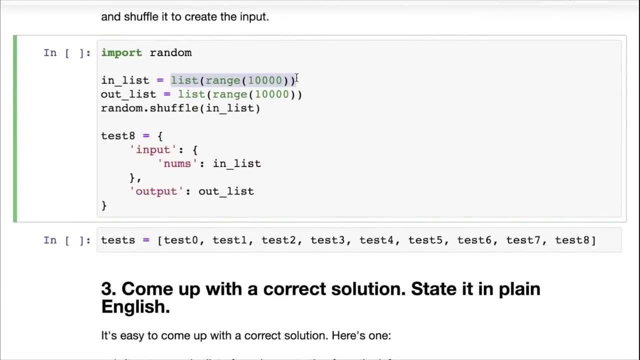 So what we'll do is we will create a list of 10,000 numbers, So zero to nine, 9,999, that is our in list, And then our outlist is also going to be zero to 9,999.. 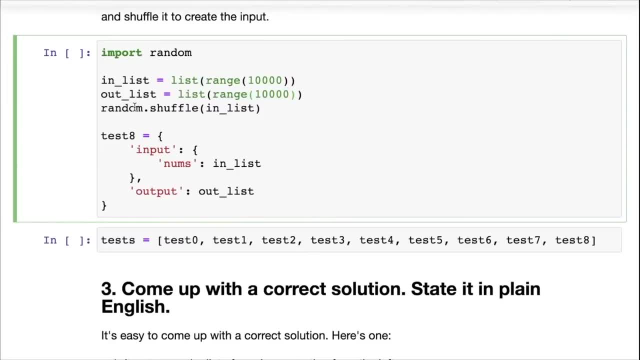 That's our outlist. Both of them are sorted. Now what we do is we shuffle the inner list, So we import the random module from Python and then we call random dot shuffle And we call random dot shuffle on in list and that shuffles the, the first list, the in list. 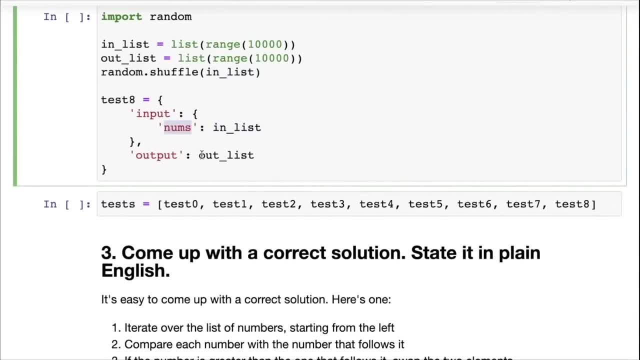 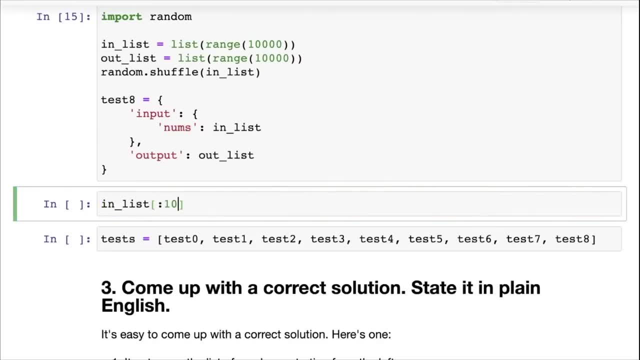 So now we have that as the input nums and then the outlist. the sorted list is the output. Now once again, we can even check that in list is actually shuffled. Maybe by looking at the first 10 elements you can see here that these are all suffered numbers. 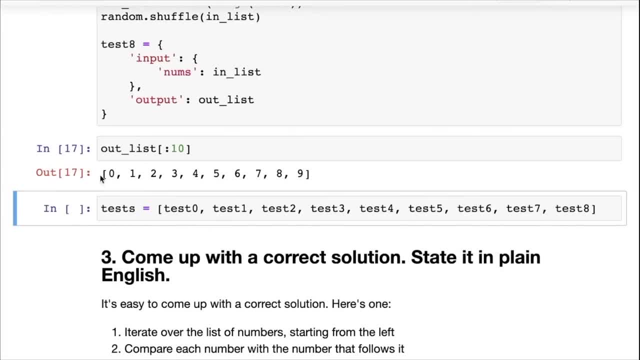 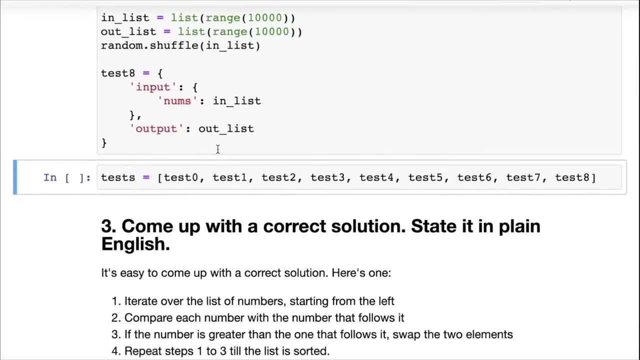 On the other hand, if you check the outlist, you can see that these are all In order. So those are our test cases And it's very important to create good test cases, even in interviews. before you start coding or before you even suggest a solution, you should try and list out your test cases, either verbally to an interviewer in a coding assessment, you may create a block of comments at the top and start listing some test cases at the top, or you can create proper test case dictionaries like this: 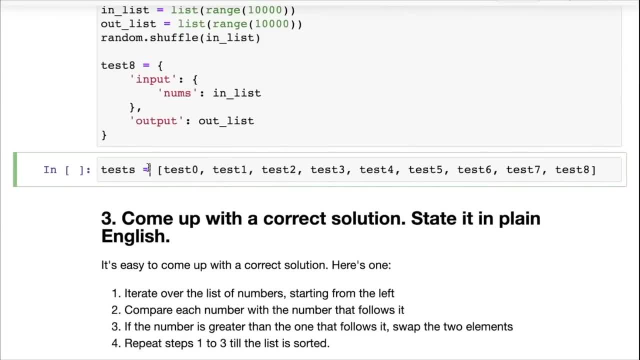 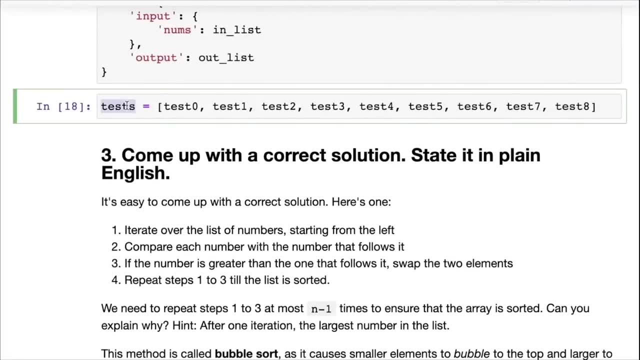 It takes a few minutes, but it's totally worth it, because you can then Test your algorithms very easily. And finally, we'll take all our test cases- test zero to test eight- and put them into a single list called tests Great. 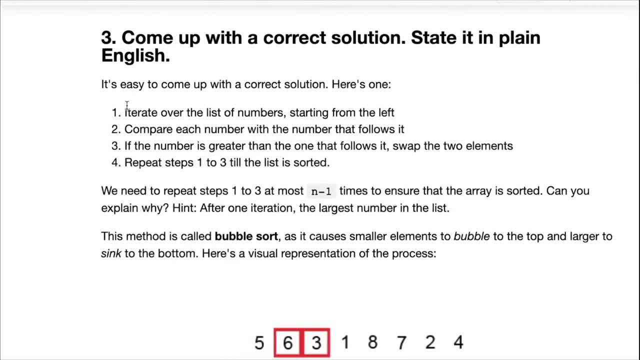 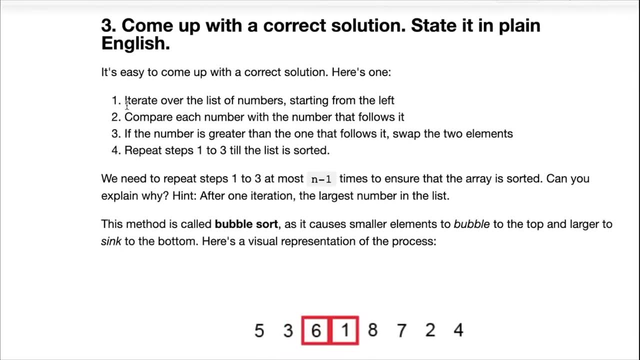 So we've made some good progress so far. Next, let's come up with a simple, correct solution and stated in plain English. and coming up with the correct solution is pretty straightforward. We have a list of numbers, so we iterate over the list. 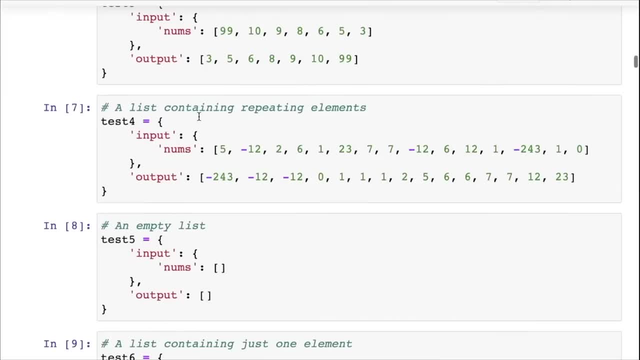 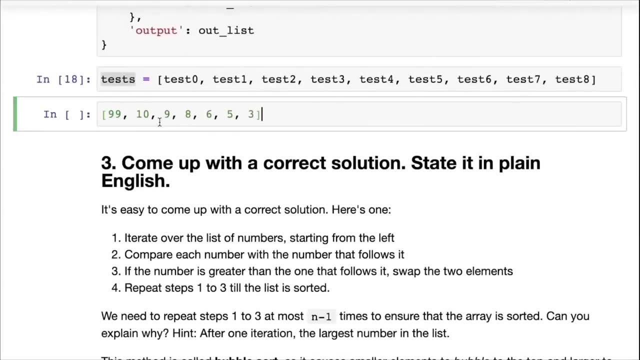 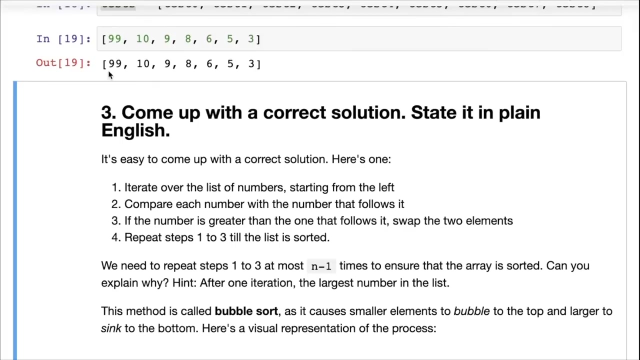 Let's grab a list of numbers So that we have something to look at. Here you go. So we have a list of numbers, So we iterate over the list of numbers, starting from the left, So we start from the very left, and then we compare each number with the number that follows it. 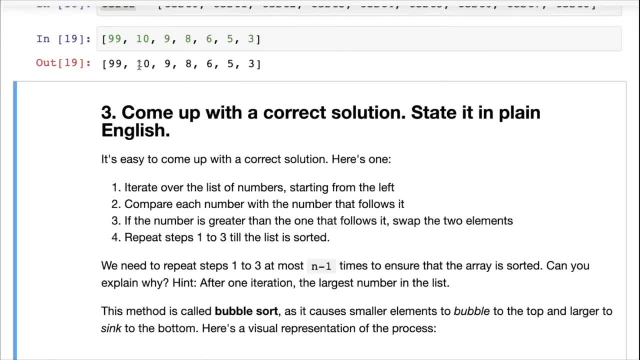 So we compare 99 with 10, and if 99 is greater than 10, then we can say for sure that 99 should appear after 10.. Right, In the final sorted area and the sorted area by default, it means the increasing order of numbers, right. 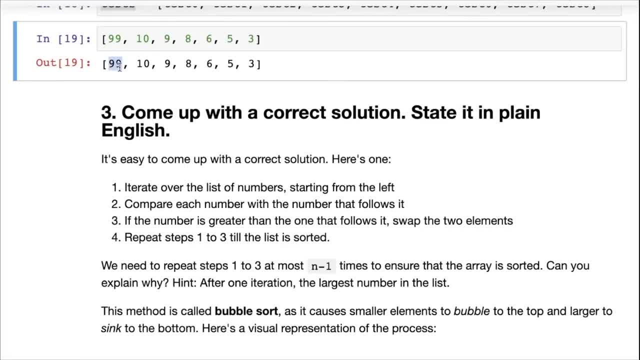 So that's what we're solving first. So what we can do is we can simply swap 99 and 10, because we know that 10 should appear before 99 and 99 should appear after 10.. Now, once we continue the swap, we move to the next position and then we compare 99 with the next element, nine. that turns out to be higher as well. 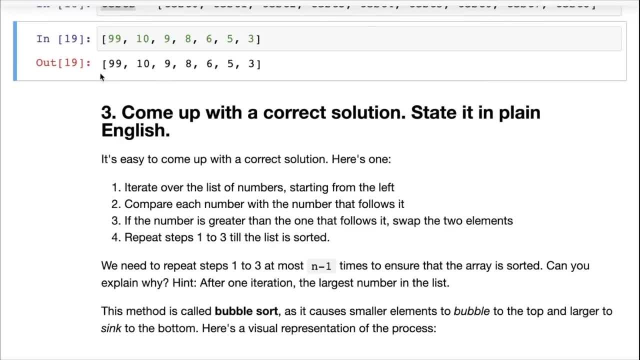 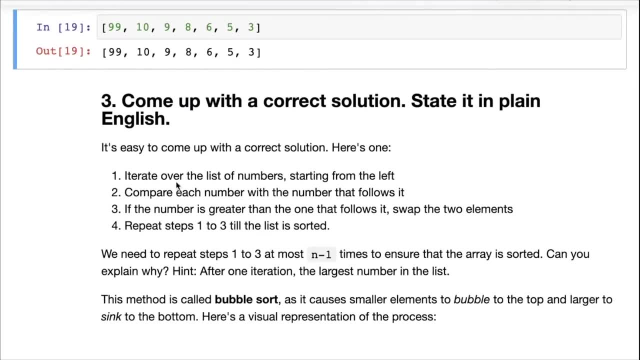 So we swap it and then we keep going. So we iterate over the list and for each element, compare the number with the number that follows it, And if the number is greater than the one that follows it, swap the two elements. Now you do that once. 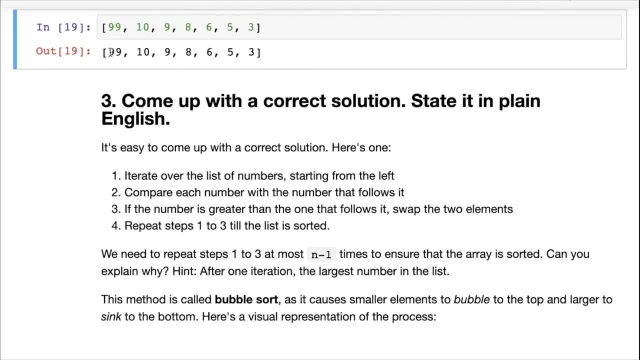 And that alone is probably not enough to compile the entire list, because the entire sorted list, because 99 in this way will end up at the end If you follow the process, but the rest of the list is still not sorted. So we repeat these steps: one, two, three. 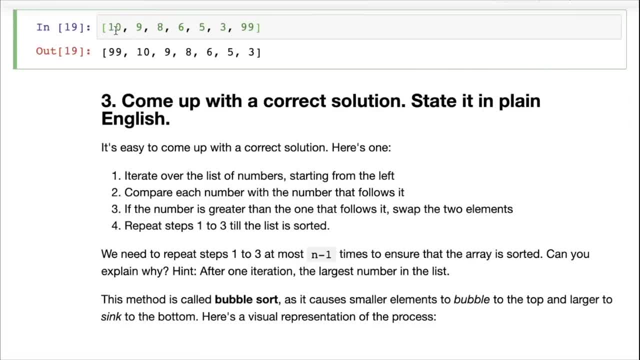 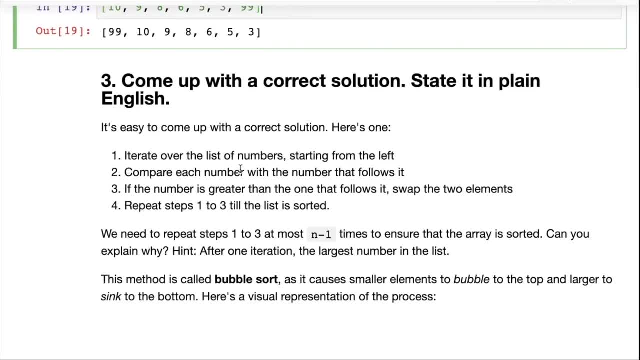 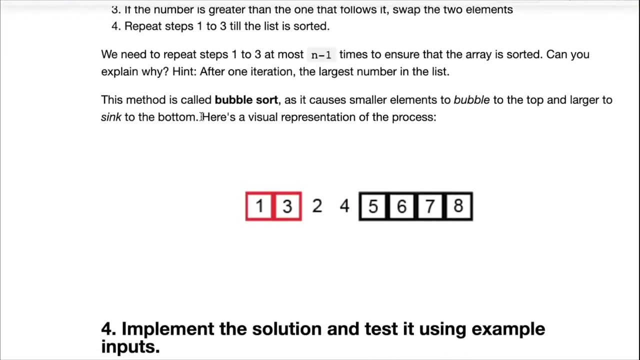 So once again, we start from the left and then we start comparing 10 with nine and then 10 with eight, and so on, and keep swapping elements as we go forward. Now I have a claim here that you may. you will need to repeat the steps one, two, three at most, and minus one times to ensure that the array is sorted. 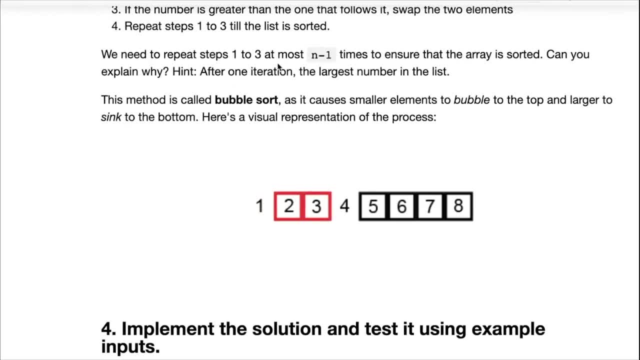 Can you guess why? And here's a hint- after one iteration of the process, you will need to repeat the steps one, two, three at most, and minus one times to ensure that the array is sorted. Can you guess why- And here's a hint- after one iteration of the process, you will need to repeat the steps one, two, three at most, and minus one times to ensure that the array is sorted. 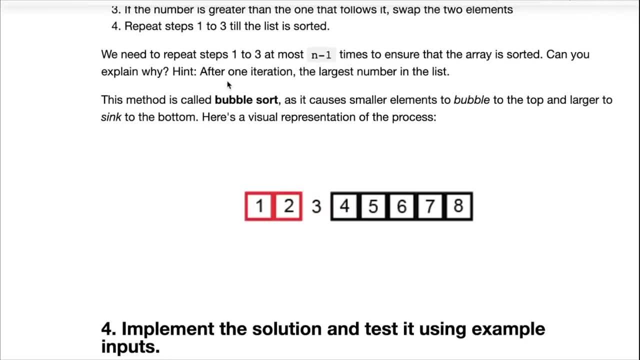 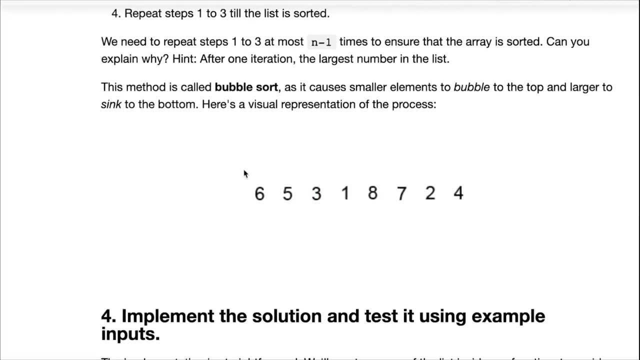 the largest number in the list will reach the very end. so that means that each time you're putting one of the largest numbers at the very end, so you need around end steps. So here's an animation showing the same thing. Here we compare six and five and then we switch them. 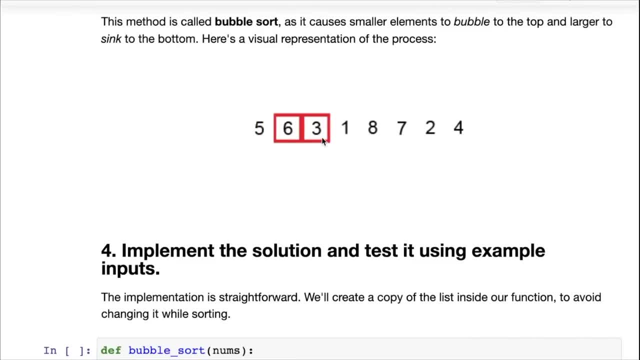 Then we compare six and three and we switch them. Then we compare six and one, and we switched them. Now we compare six and eight, and we don't switch them because they're in order. Next, we compare eight and seven, and we switched them. 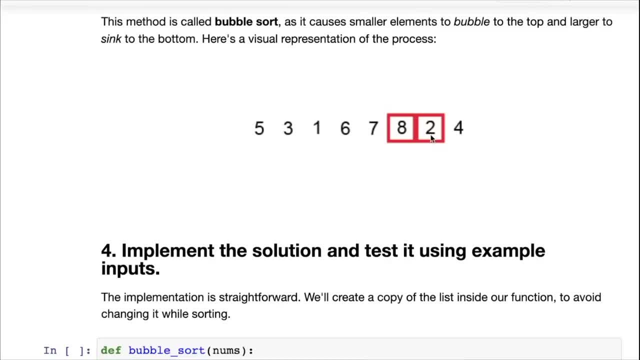 Next, we compare eight and two, and we switched them. And finally we can work: compare eight and four, and we switched them, And in this way the largest number, eight, has reached the very end. So now we can freeze its position and we can start again from the beginning. 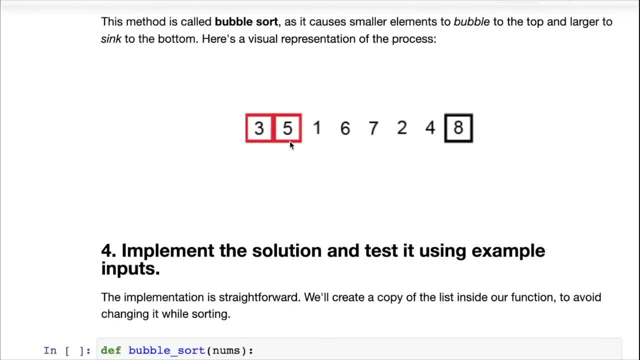 And you can see that this time the next number seven will end up here, And then the next time the number six will end up here, And then next time the number five will end up here, and so on. So in N repetitions of this process of comparison left to right, we will have sorted the area. 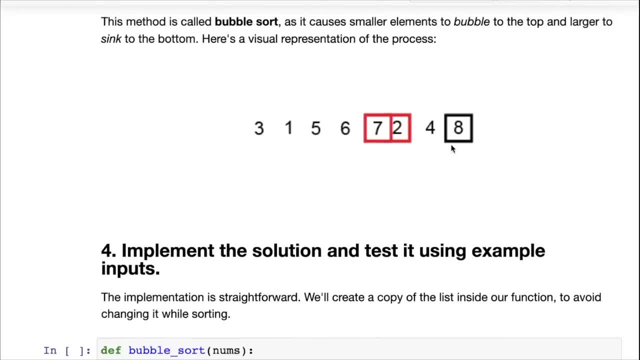 And this approach is called bubble sort because it causes the smaller elements to bubble to the top or to the beginning. You can see that The numbers one- three slowly bubble up to the top and it causes the larger numbers, like eight and seven, to sink to the bottom. 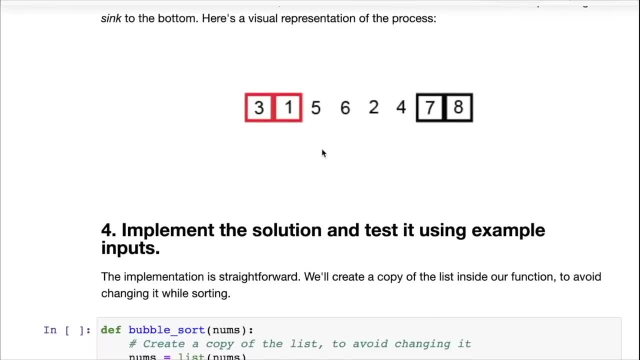 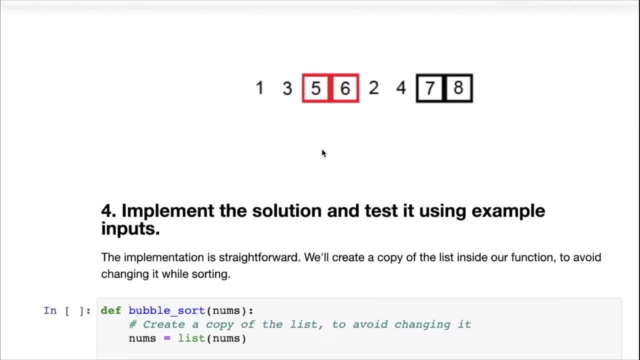 And you can watch this entire animation to get a full sense of how bubble sort works. What will also really help is if you can take an example on paper and work it out on your own, step by step. especially with sorting algorithms, this really helps. 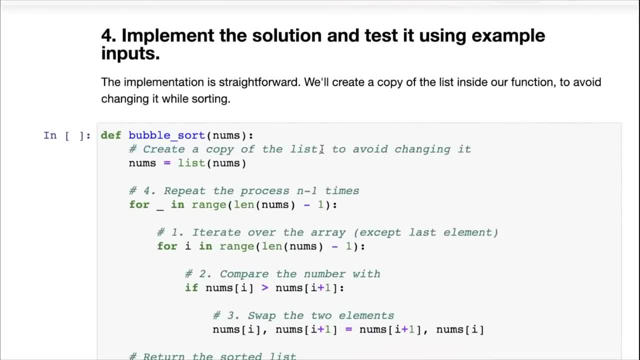 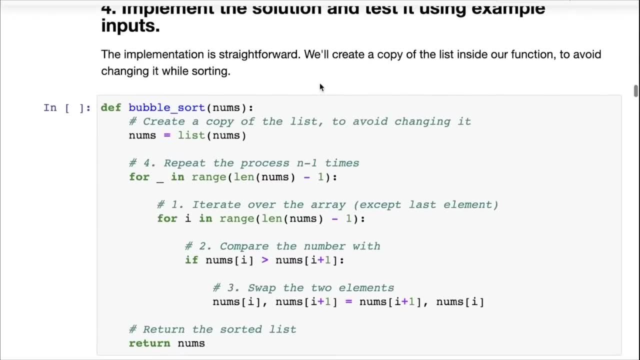 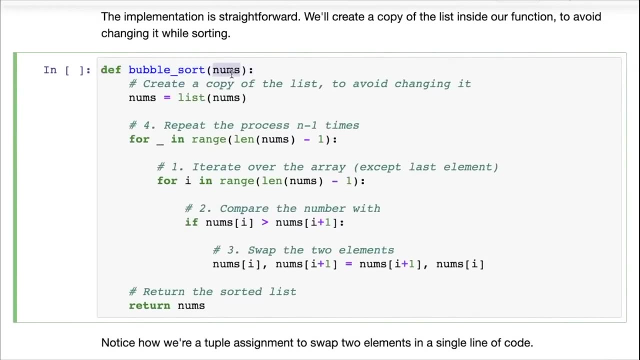 Okay, So now we've come up with a correct solution, Let's implement it and let's test it using an example. Okay, Now the implementation itself is also pretty straightforward. So we have the bubble sort function here. def bubble sort. It takes a list of numbers. 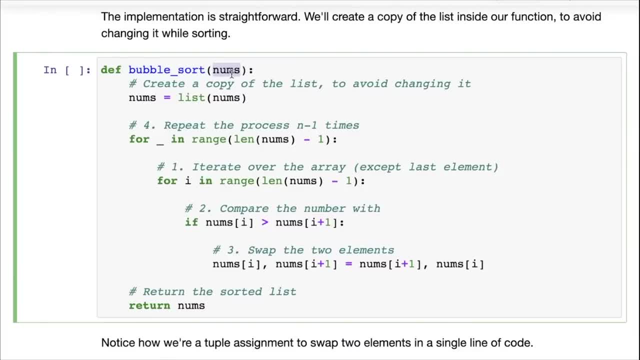 Now we may not want to modify the list of numbers in place, because then our test cases will not be reusable. So just to avoid modifying our test inputs, we're going to create a copy of the list to avoid changing it. and the way to create a copy? simply call the list function with the 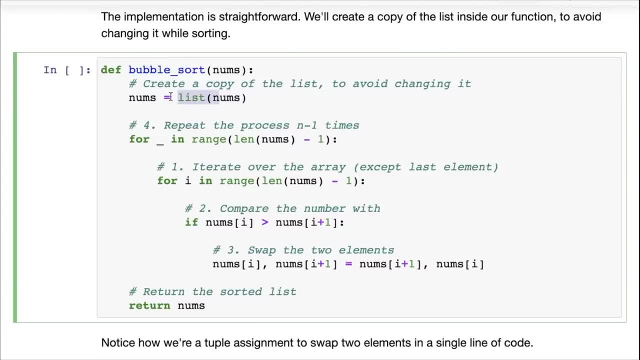 list as input. So now we are set replacing nums with a copy of nums. Now, depending on your particular use case, this may not be necessary. So this is something that you can actually check while you're in a coding assessment or in an interview or talking to an interview. just check with them. 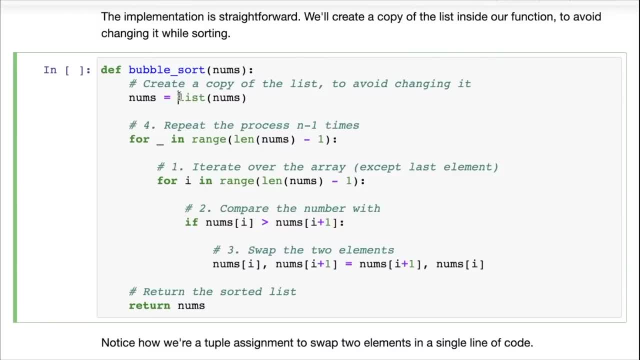 Do they want an edit to be sorted in place or do they want a new array to be created? If they want, if they're okay with sorting it in place, then you probably don't need this, But you may still just want to keep it in. 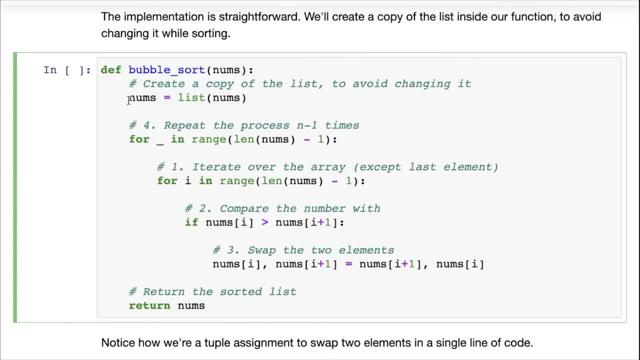 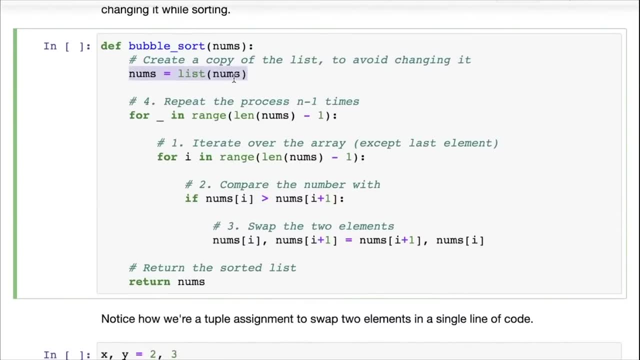 Because otherwise you may end up modifying some of your test cases unintentionally, and that may lead to problems. So always good to create a copy of the input rather than modifying it in place. Okay, So then let's come to steps one, two and three. 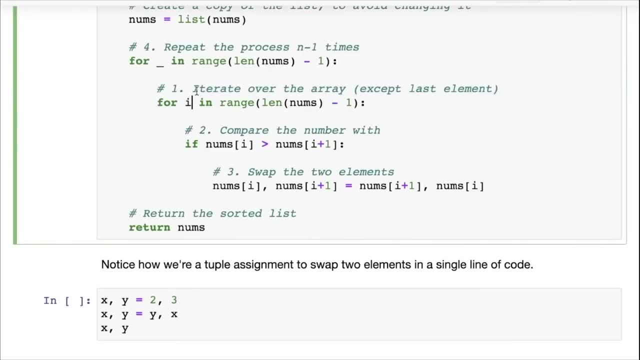 And then we'll see step four, which is the outermost step really. So we iterate over the array, So we go from: we take I and we check the range len nums minus one. So the number of Elements in the array is N and N can be obtained using len nums. 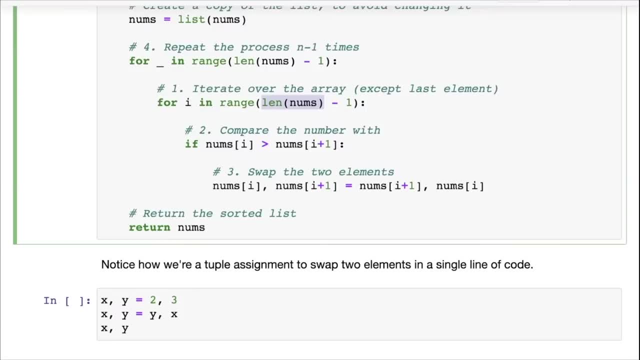 Then we want to go from indices zero to N minus two. So the total number of indices is zero to N minus one. But if you go to the N minus one or the last element, there is no further element to compare it with. Okay, 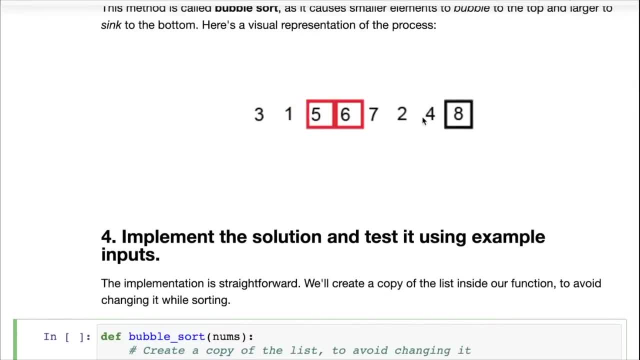 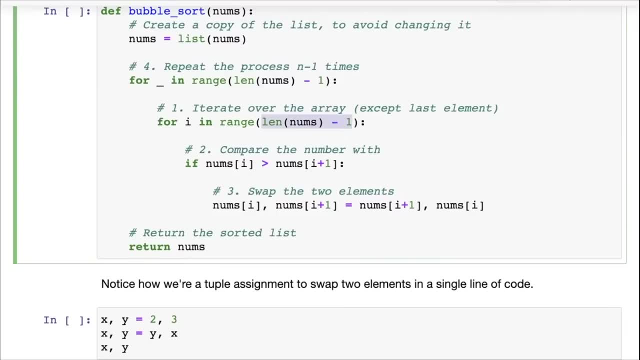 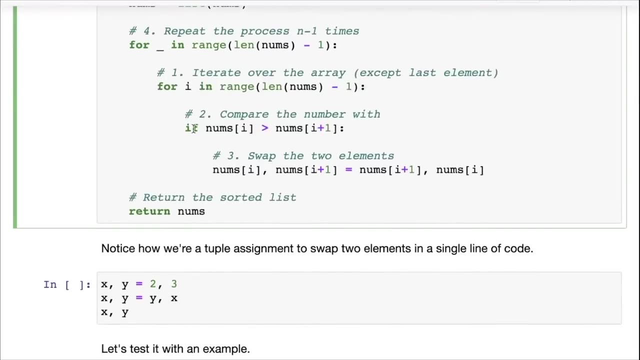 So keep that in mind, that you only want to run this iteration till your pointer comes to this point, not to the last element. And that is why we check if we put I in the range zero to Len nums minus one. So the highest value that it can take is len nums minus two. 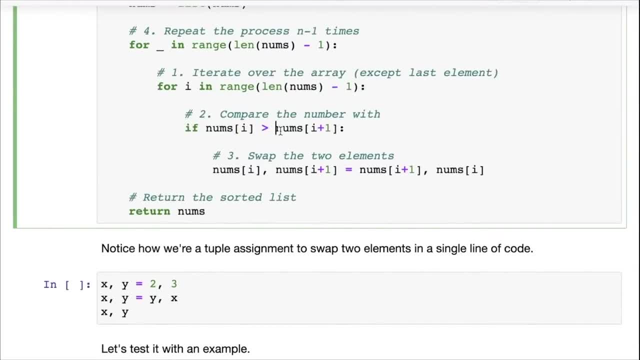 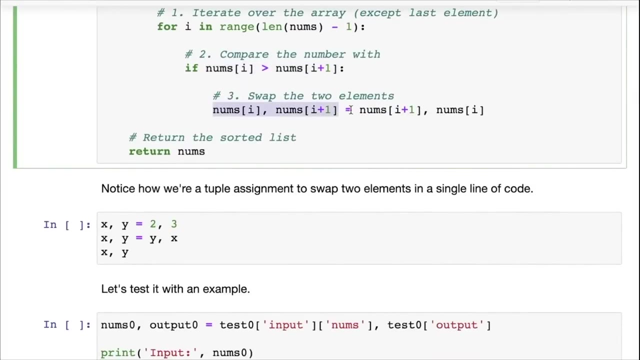 Next we compare nums I with nums I plus one. So we compare the number with the element that comes after it, And if it is greater, so that means these two are out of order. So then we simply swap them. So we set nums I comma, nums I plus one equal to nums I plus one comma, nums I. 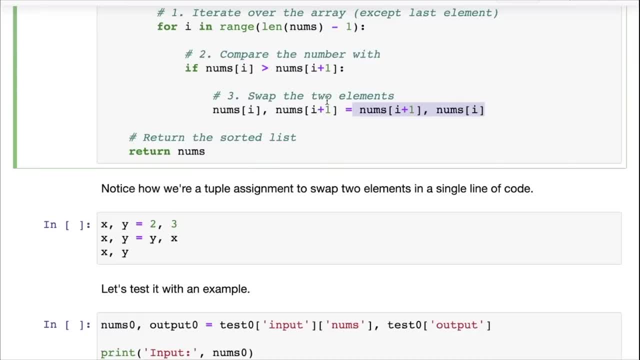 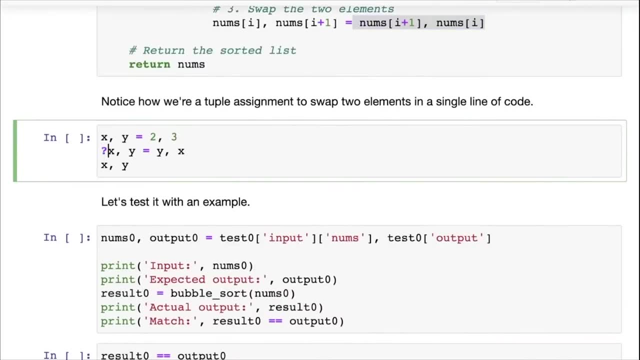 Now This is an interesting way of sorting. in C or C plus plus or Java You would have to write three or four steps to swap numbers. but in Python is really simple. First you say X, Y is. let's say we're missing X comma Y or two comma three. 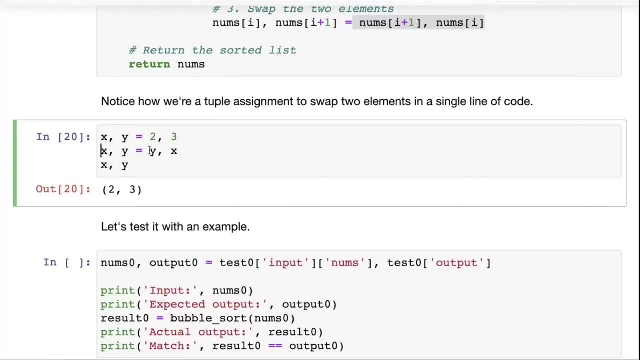 So you can see they have the values two and three, and then we simply write: X, Y equals Y, X. So what happens is the value of Y gets placed into X and the value of X gets placed into Y. It's a single step for swapping two numbers. 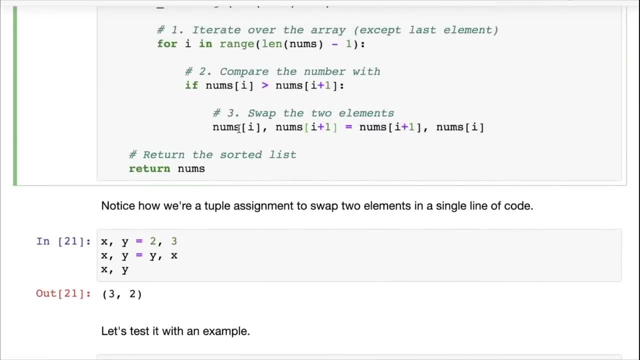 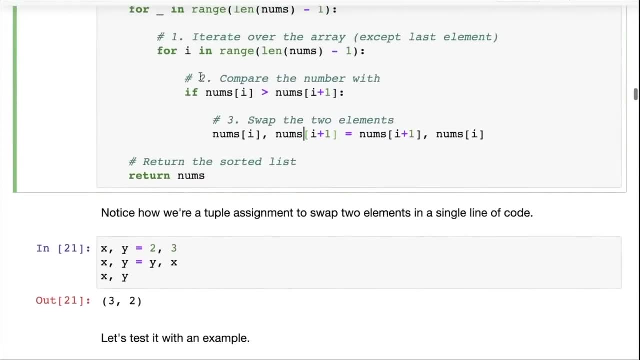 There you go. So we swap the two elements. Exactly what we are showing here, swapping the two elements. Next we repeat this. So now we're doing this from left to the penultimate element, And in this way we have pushed the largest element to the end. 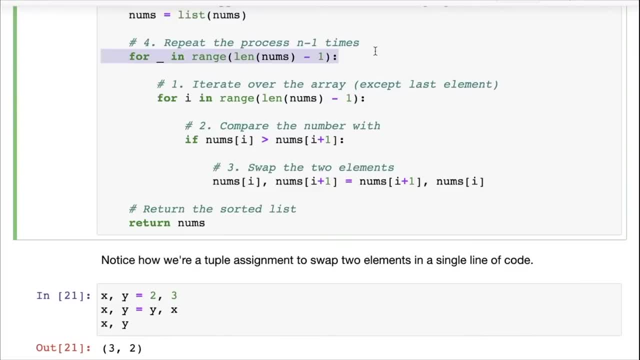 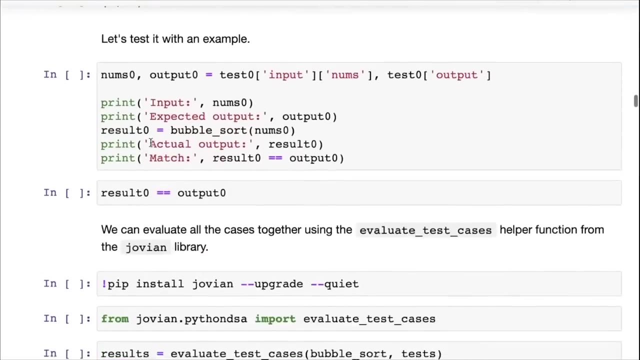 Now we need to repeat this process N minus one times, so that each time we are pushing one of the largest elements to the very end, and in N minus one repetitions of these three steps, we will end up with a sorted list. And finally, we return the sorted list and that's it. 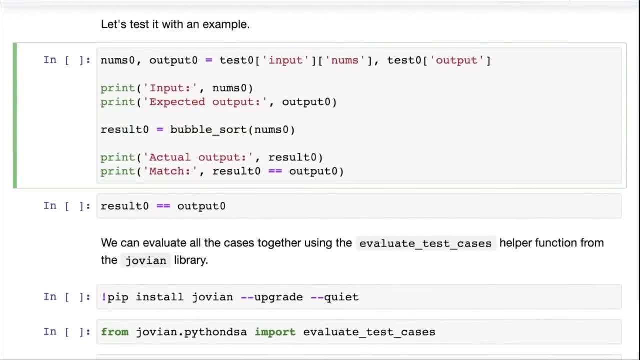 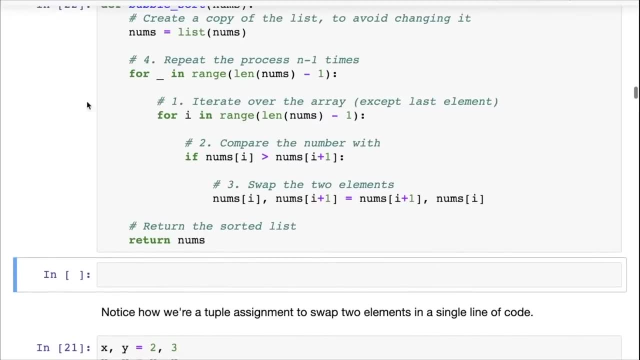 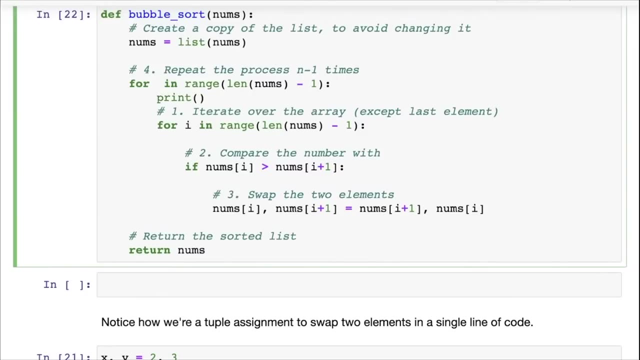 So let's test it out with an example. And, by the way, if some of this doesn't make sense, so a simple way to debug it is to add print statements here, So you can add a print statement and maybe just print this value. 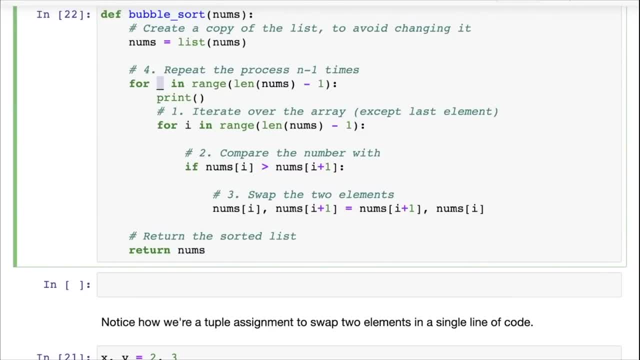 So we've used underscore here because we don't actually use this value. but let's say we wanted to use this value. Then we can print That this is iteration J and then inside it you can print that the value of I is I and 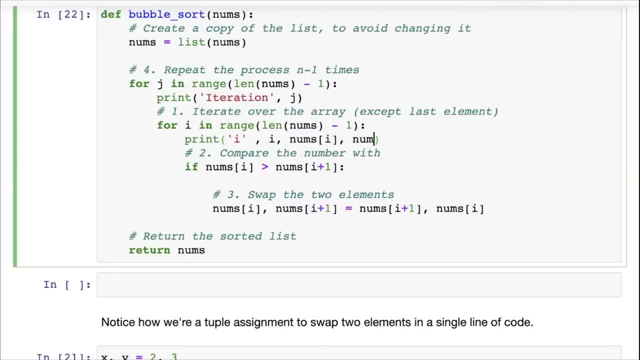 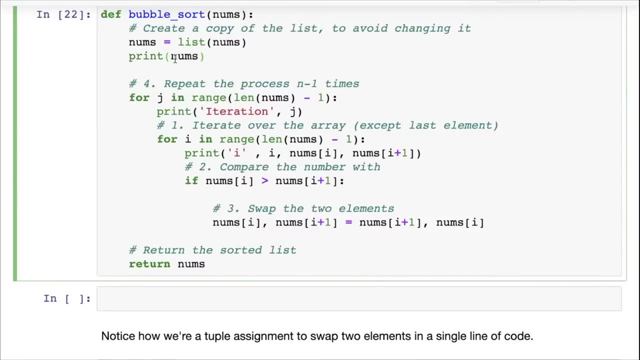 you can also print the value of nums I, and you can also print the value of nums I plus one, and at the very top you can also print nums. Now, if you add all of these print statements and then execute your algorithm now you will be able to see exactly what is happening inside each iteration. 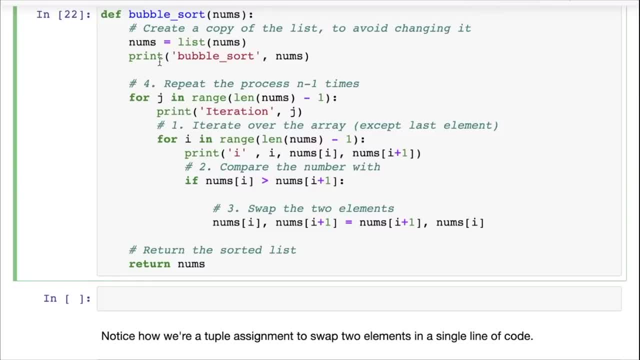 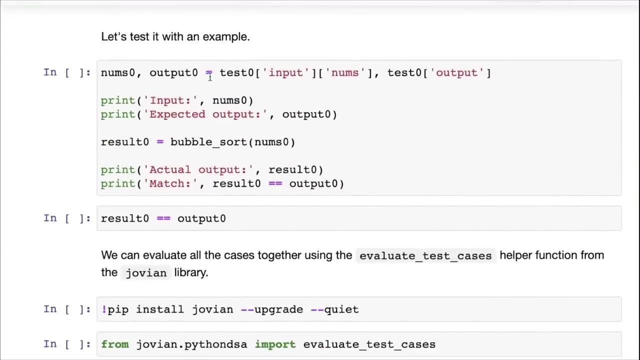 So that's a great way to debug your code If you're facing any issues, and also understand what the code does. but in any case, we won't need these, so I'm just going to comment these. So let's test it out. 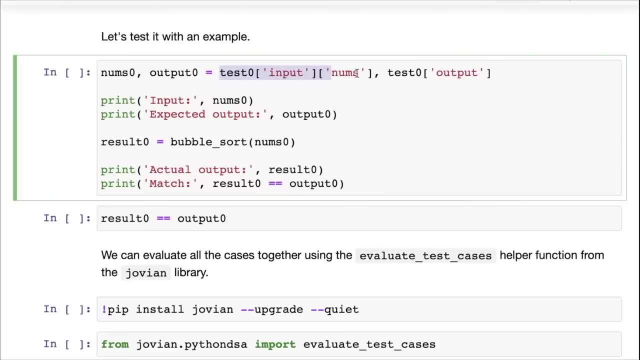 So we get from test zero, we get the nums as input and then we get the output. and we can print the input and the expected output and then finally calculate the result by passing nums zero into bubble, sort Okay, And then printing the actual output and finally whether the two match. 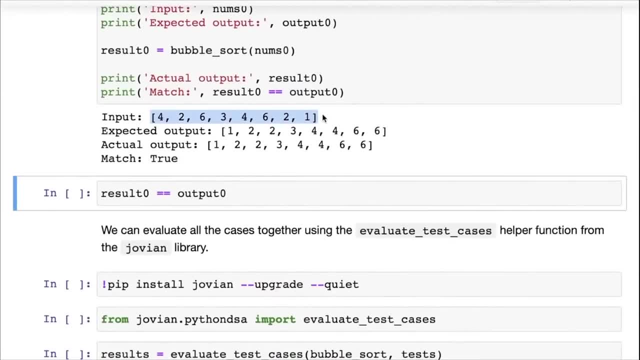 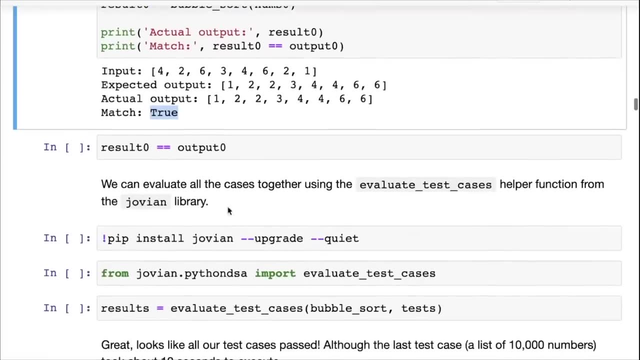 So you can see here now that the input was this unsorted list and then the expected output was the sorted version, and that's what we got. So in fact, there was a perfect match, and that's it. So we implemented our first sorting algorithm. 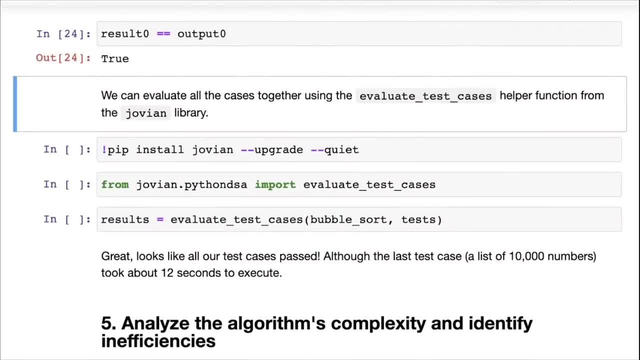 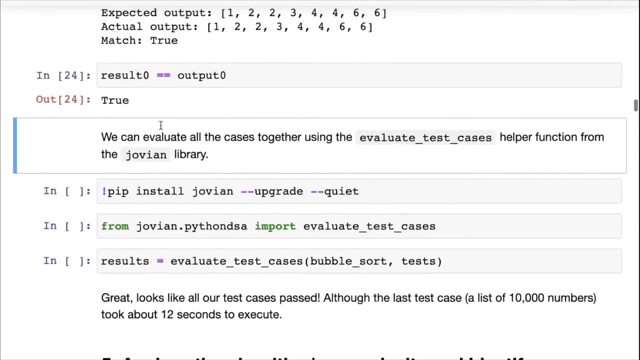 It was pretty straightforward: a few lines of code as an exercise. you can try to implement it. It's from your memory. just write it in plain English first and then try to implement it. It's a good coding practice And we can also evaluate all the test cases that we have. 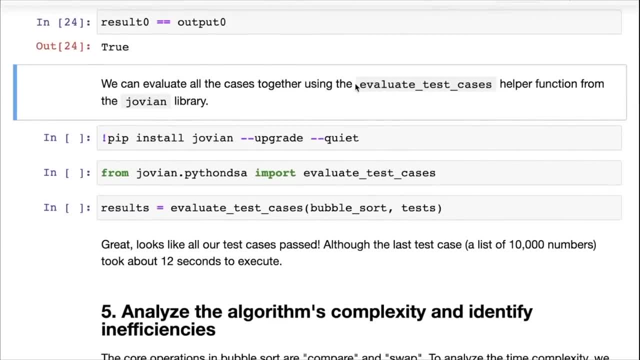 Remember we had created about nine test cases and to help you evaluate the test cases we've given you a helper function called evaluate test cases, which is part of the Jovian library. So we installed the Jovian library here. pip: install Jovian and then from Jovianpythondsa. 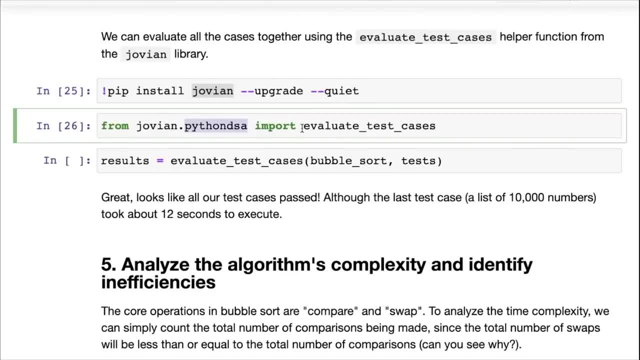 So Python DSA is the name of the course and that's also the module where we have helper functions for this course: import, evaluate test cases. and evaluate test cases simply goes over the list of test cases that you have and it pulls out the inputs and passes. 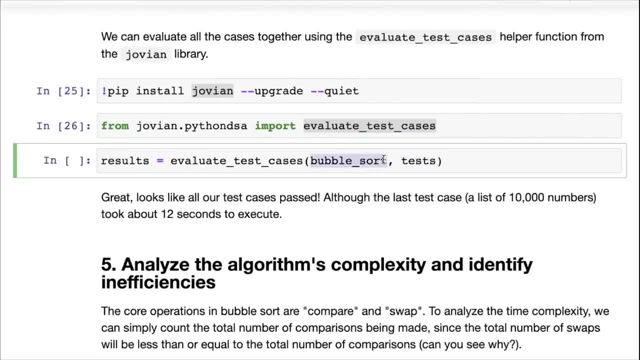 them as arguments to the function provided here, which is bubble sort and then gets the outputs and compares the outputs and also prints the information with like what was the input, What was the expected output and the actual output and whether they match. So let's check it out. 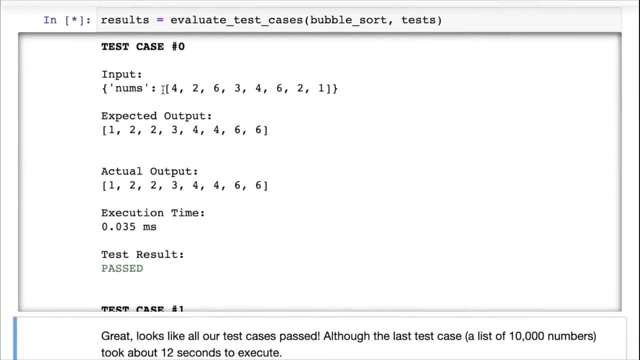 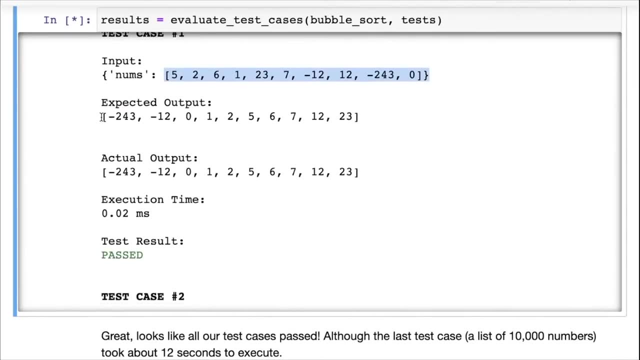 Okay, So you can see here: this was test, case zero and that work, which we just tested out. Here's a larger list including some negative numbers. This worked as well. You can see the test result is passed. Then you have another list here. 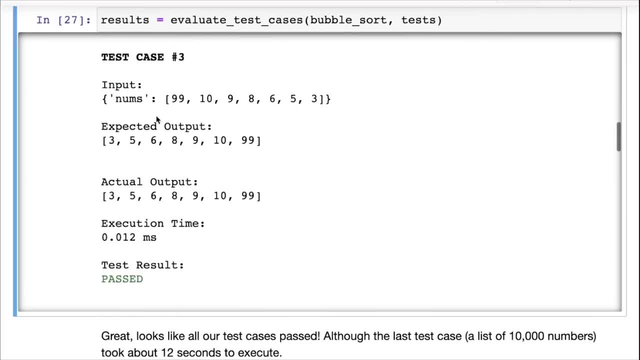 This seems to work fine too. This is already sorted. Here you have one which is sorted in decreasing order. that works. Here you have one with repeating numbers. that works too. The empty list works, Um single element works, and this works too. 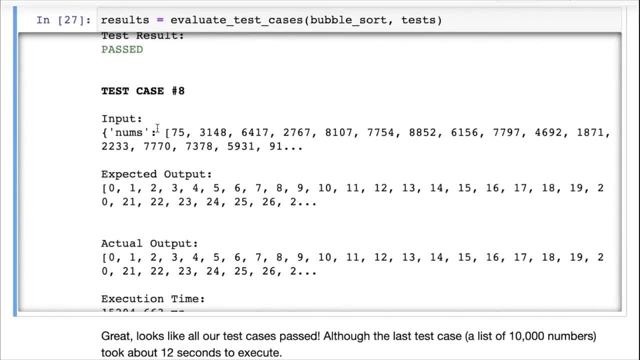 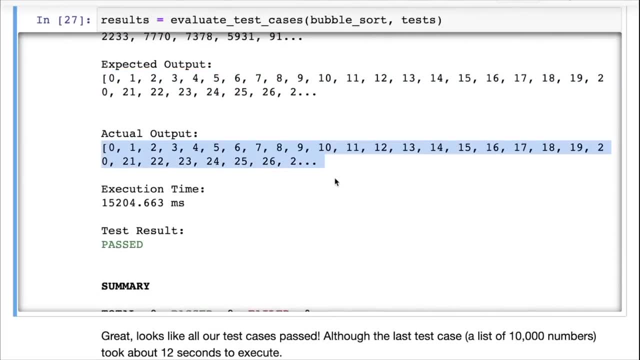 This is the same element repeated over and over. And finally, here is our final test case. This had 10,000 elements, Remember, So you can see that this was the expected output and this was the actual output. So we have successfully sorted 10,000 elements. 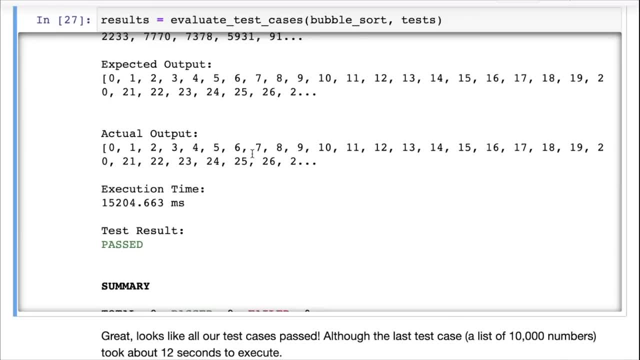 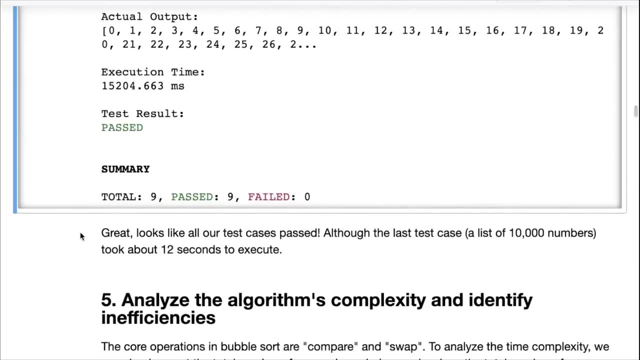 And that's really the power of programming- that, without having to look at any of the numbers, we've just written four or five lines of code and we've sorted 10,000 elements. So all our test cases passed, Although do look here that it took about 15 seconds for the sorting of 10,000 elements. 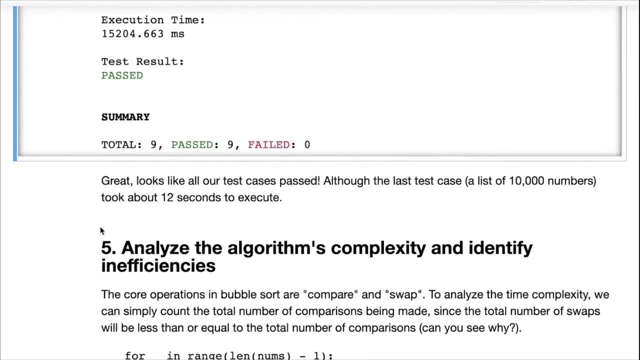 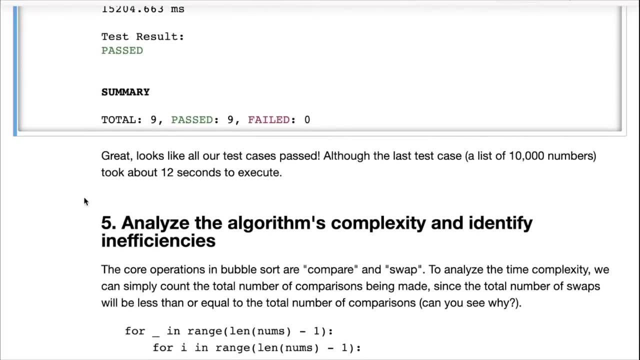 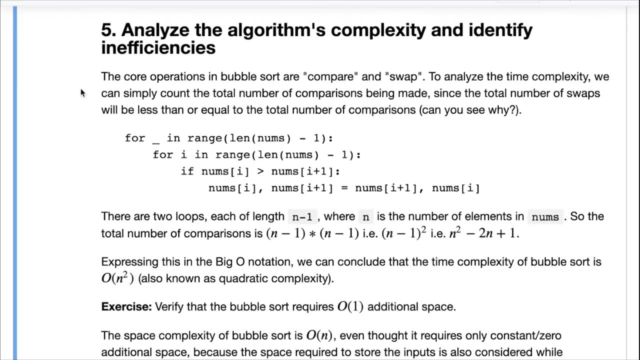 Now, maybe that's not, maybe that's not that bad, but we we are looking at probably millions of notebooks every week at Jovian, So we want there to be a faster sorting algorithm. Okay, So Two, Three, Four. 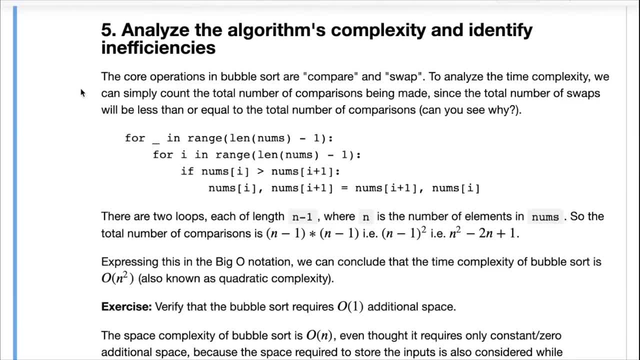 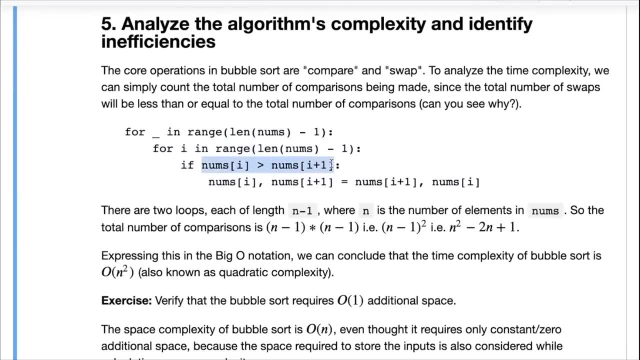 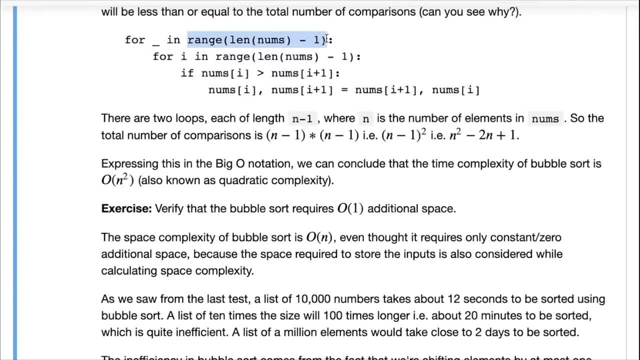 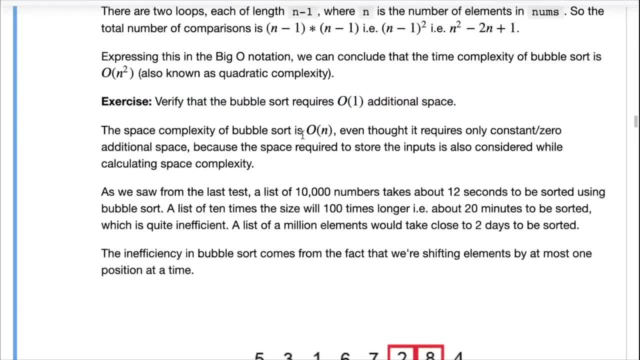 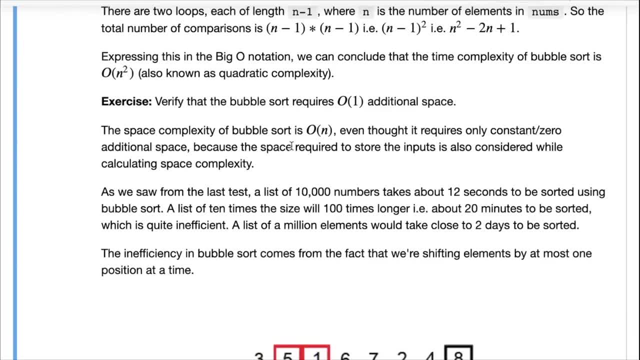 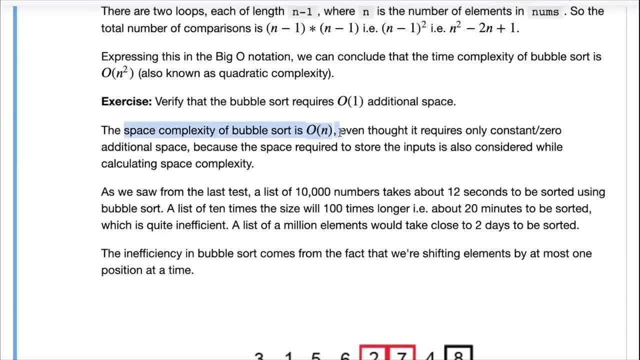 100.. So the overall space complexity is order in, because we need to store the actual input list somewhere, But, on the other hand, the amount of additional space required as order, one which is a constant factor, independent of the size of the list. 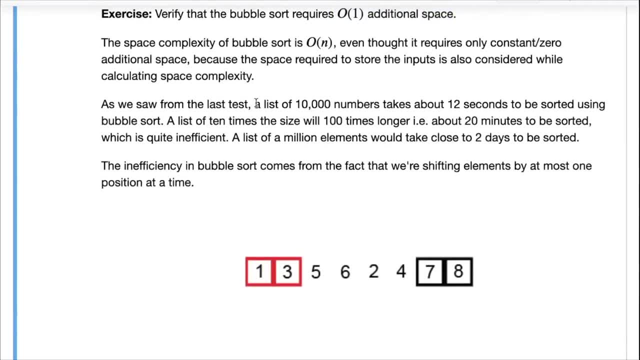 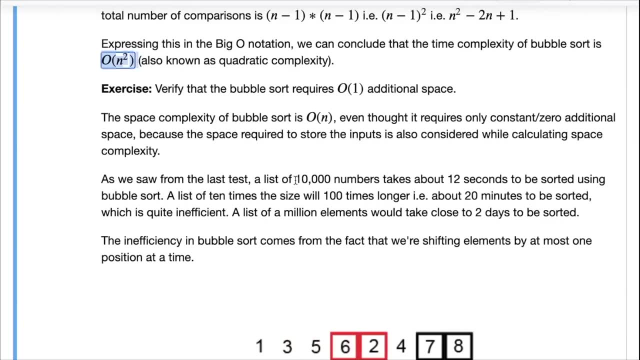 So that's, that's how bubble sort works. Now, analyzing this order, N square complexity and keeping in mind that a list of 10,000 numbers takes about 12 seconds. So if N is 10,000 and N square is multiplied by some constant is about 12. 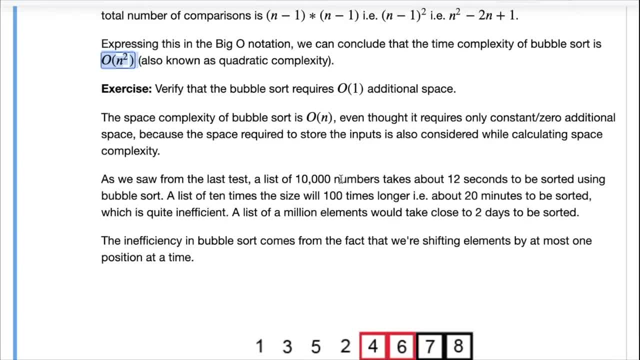 seconds, then if you had a list that was of a hundred thousand elements, so that would be 10 N whole square, or a hundred times the same amount of time that it would take to sort it. So that means it would take about 20 minutes to sort a hundred thousand. 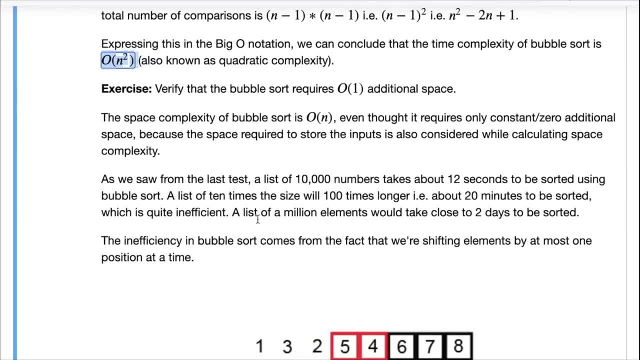 numbers, which is, I would say, is a bit inefficient now, and a list of a million numbers would take close to two days to be sorted In Python. Now if you do it in C plus plus, maybe it might be a four or five times faster. 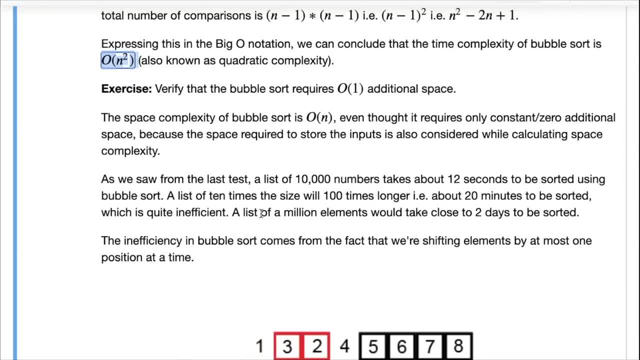 But again, the moment you go from a million to 10 million, that will actually end up taking a year or so, and that's bad, And that is why N square or quadratic complexity is something that we would like to do away with, because it grows very fast. 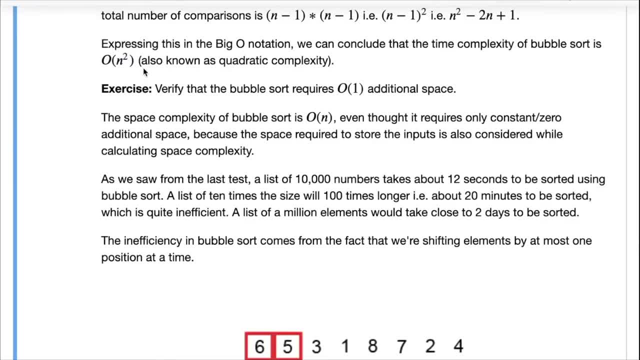 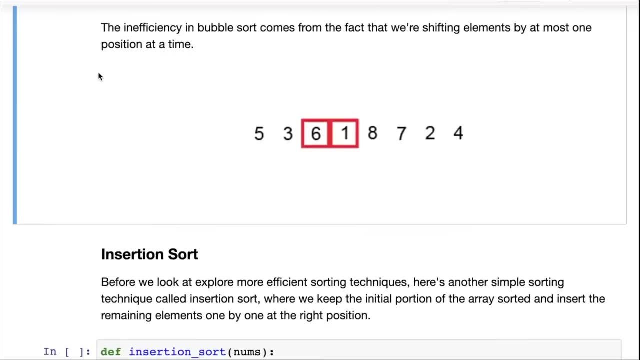 As soon as you hit maybe a 10,000 or a hundred thousand elements, then it starts taking longer, Then a few seconds or a few minutes or a few days, And at that point you can no longer use that particular algorithm. So we need to optimize bubble sort, and the inefficiency in bubble sort comes from the 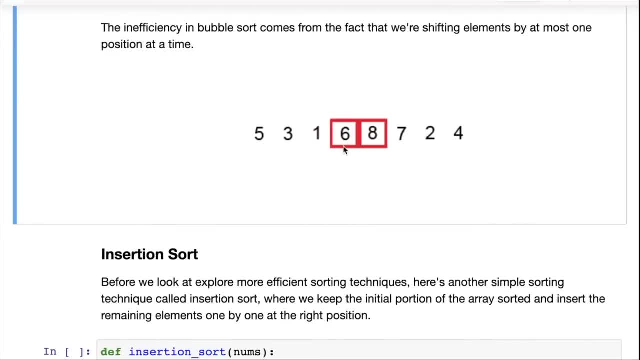 fact that we are shifting elements by at most one position at a time. So each time we go through the list, we capture some information about the list, but we are simply moving one element from left to right, so to speak, and each time 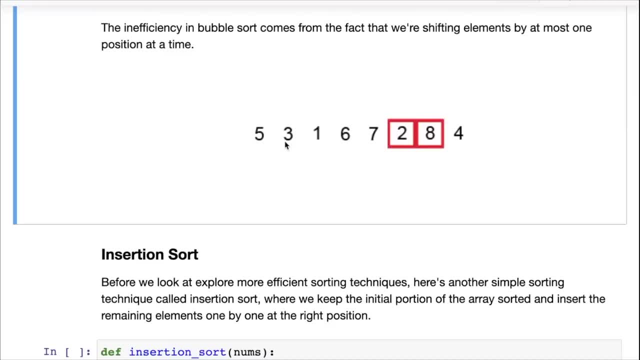 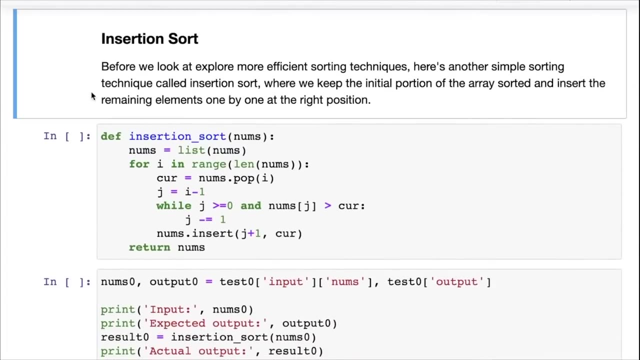 we are just moving It one at a time by doing swaps. rather, it would be nice to just place elements directly, maybe a few positions ahead, And that's where we will look at some optimized algorithms Now. another common algorithm that is used is called insertion sort, and this: 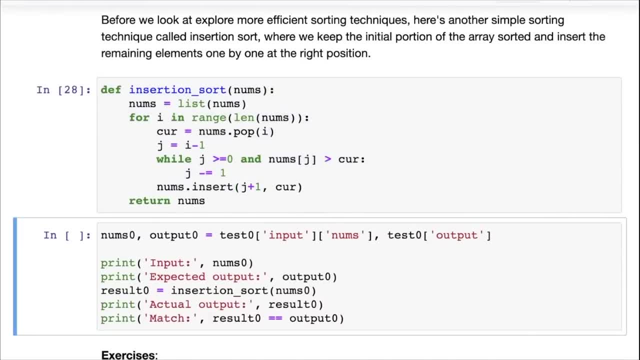 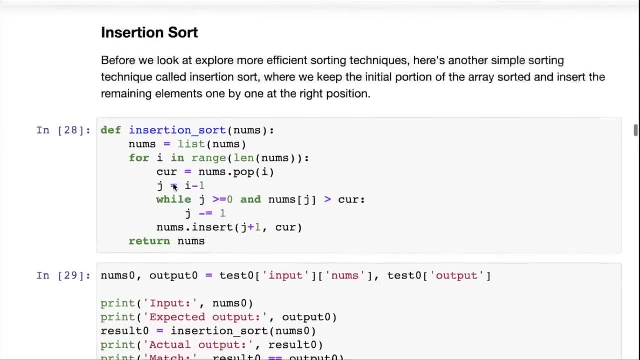 is. here is the code for insertion sort, So you can look through the code for insertion sort here and here is an example. You can see how it works And we'll not look into insertion sort in a lot of detail but roughly, this is how. 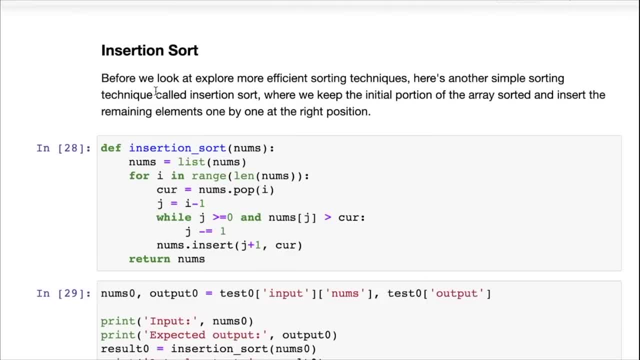 you arrange cards in your hand, which is by starting to move cards around so that at the- maybe on the left edge you have sorted cards, on the right edge you have the unsorted cards and you keep moving the new cards into sorted positions. 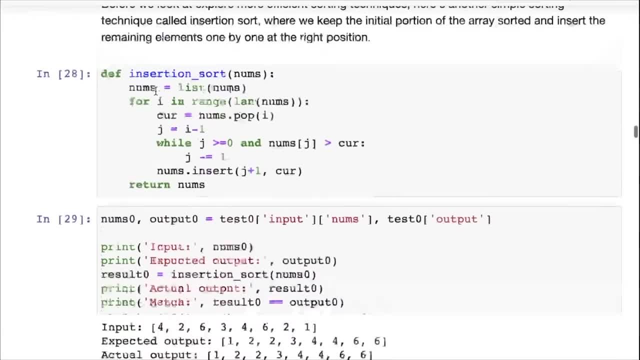 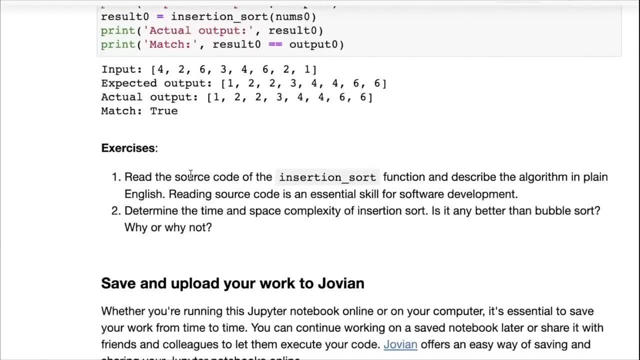 That's how it works. So here's an exercise for you: go through this function, read the source code and then describe how it works. So here's an exercise for you: go through this function, read the source code and then describe the algorithm in plain English. 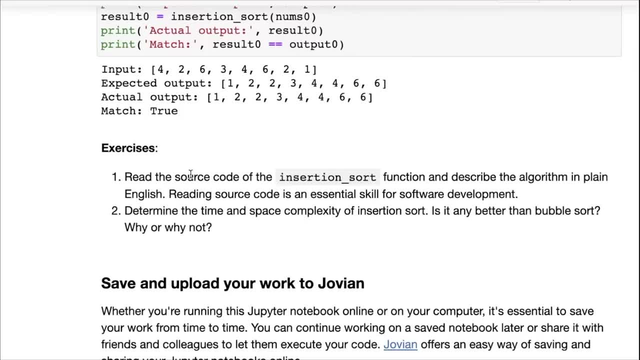 Now reading source code is an essential skill for software development. This is something that you'll have to do in your work, whether you're doing software development or data science. maybe because there are no comments in the code, there is no documentation or the person who has written the code is not. 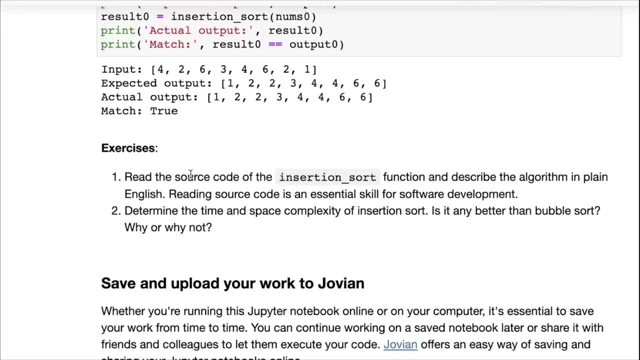 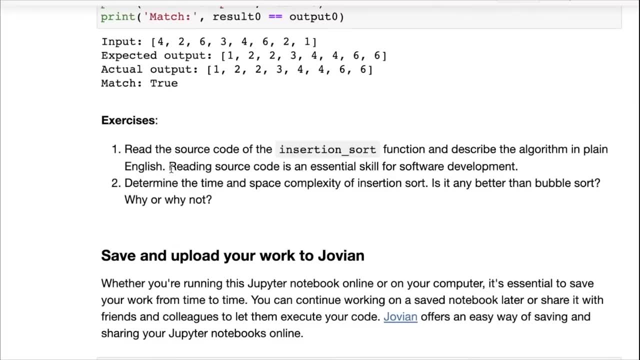 available or has left the company, or this is some open source library. So in all these cases you will have to read and understand code. So read it and then describe: insertion, sort the algorithm in plain English, then look it up online and see if it matches what you've written. 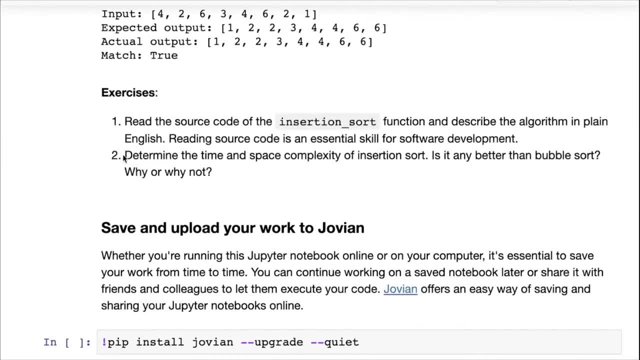 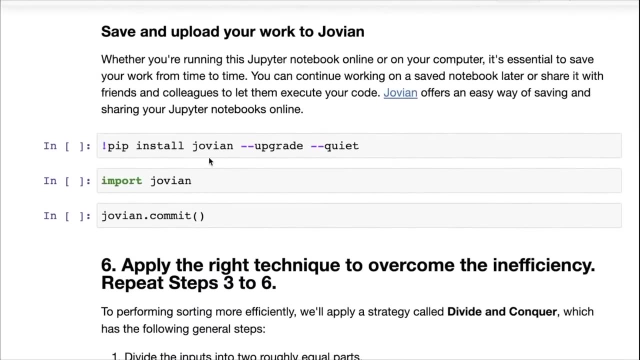 And then second is to also determine the time and space complexity of insertion sort and see if it is any better than bubble sort and explain why or why not. So these are a couple of exercises for you. So that's bubble sort and insertion sort. 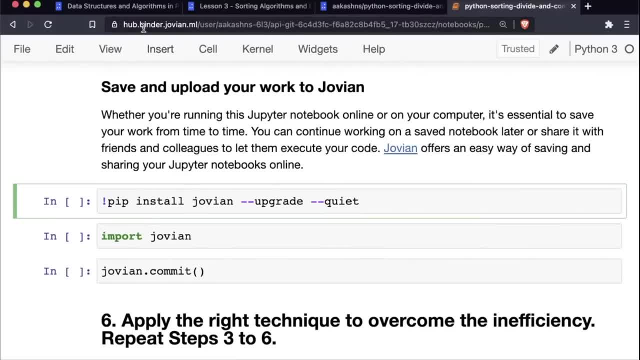 Now, before we continue, I just want to recall you that this is a Jupiter notebook running on an online platform, hubbinderjovianml, And since this is free- Uh, it will shut down after some time- So you want to capture snapshot of your work at regular intervals, and that's. 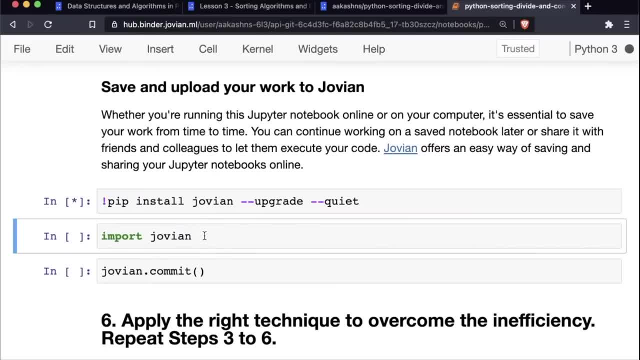 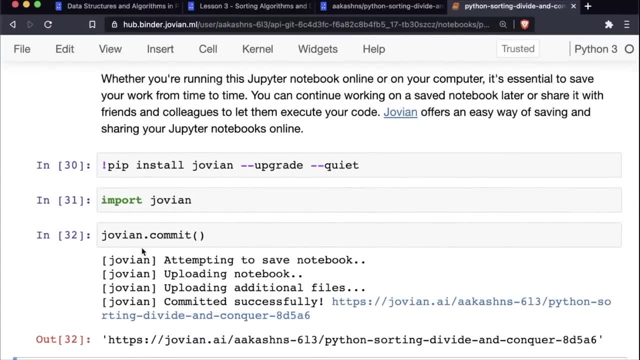 where you can use the Jovian library. So you install the Jovian library using pip, install Jovian, import Jovian and then run Joviancommit. Now, when you run Joviancommit, it captures a snapshot of this Jupiter. 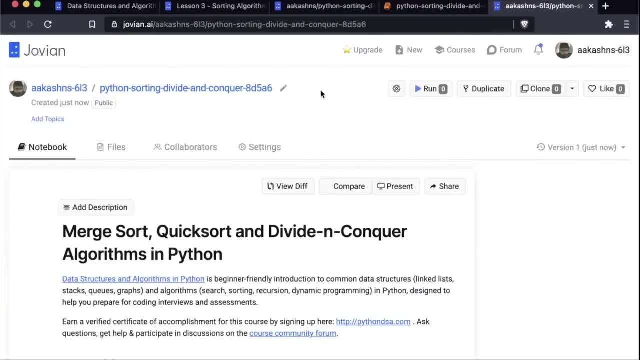 notebook and puts it on your Jovian profile. So now this will be your profile when you run Joviancommit and you will be able to resume your work by clicking the run button on this page anytime And this notebook will go to your profile. 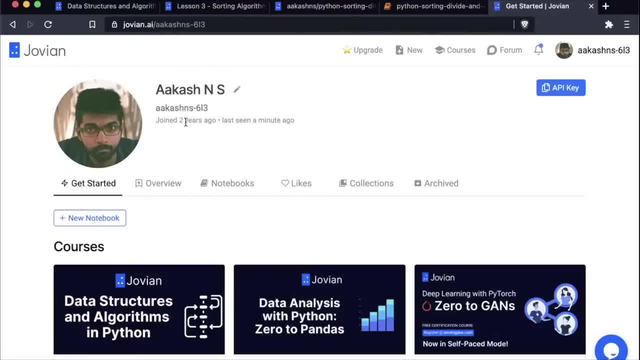 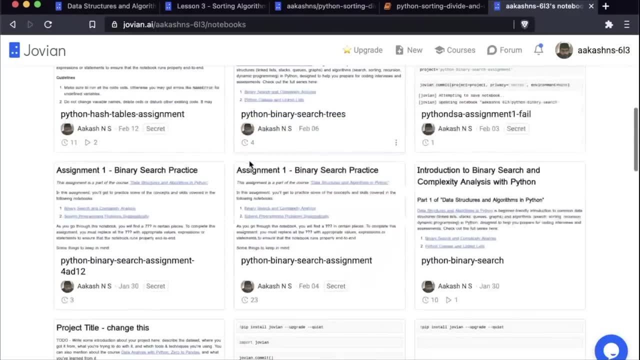 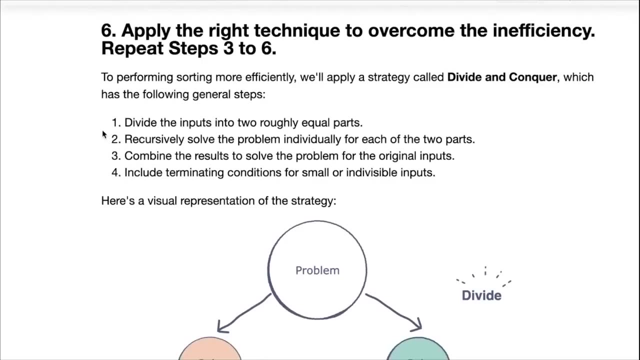 So you can just click on your Jovian profile or just click home here And if you check either the overview or the notebooks tab, you should be able to find your notebook here. Like here you go. Okay, Coming back now we're at step six, where we want to apply the right technique to 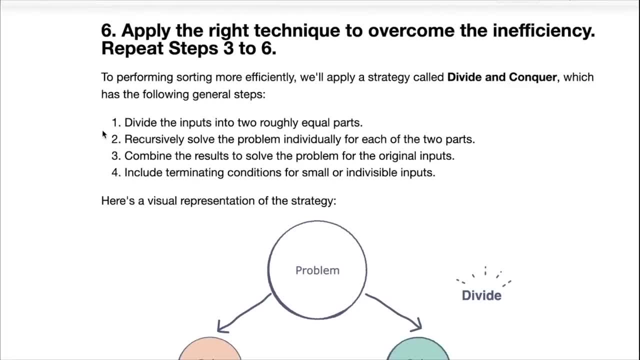 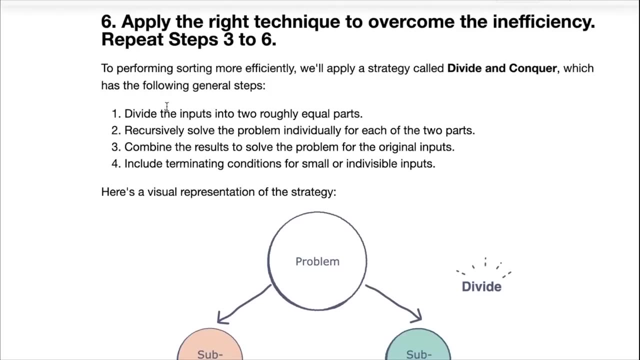 overcome the inefficiency in the algorithm. Now, to perform sorting more efficiently, we will apply a strategy called divide and conquer, And divide and conquer is a very common strategy used across the board for many different kinds of algorithms, And it has this general steps that is applied in different, different 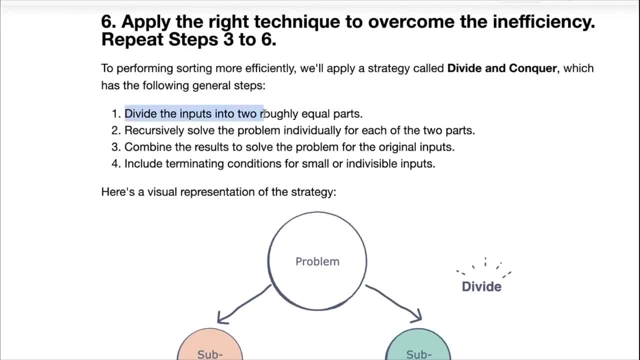 ways across different problems. So step one is to divide the inputs into two roughly equal parts- Okay, They don't have to be exactly equal, but two roughly equal parts- And the idea here is that those two parts can themselves be used as inputs, as sub problems. 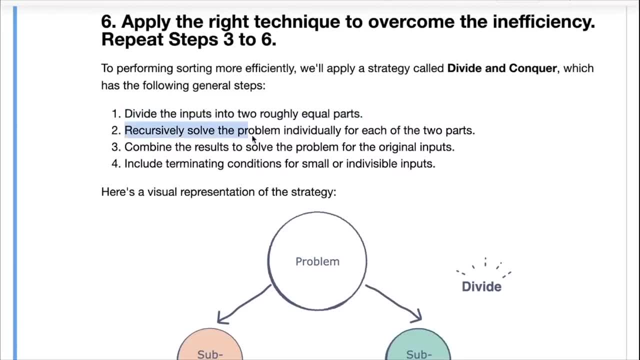 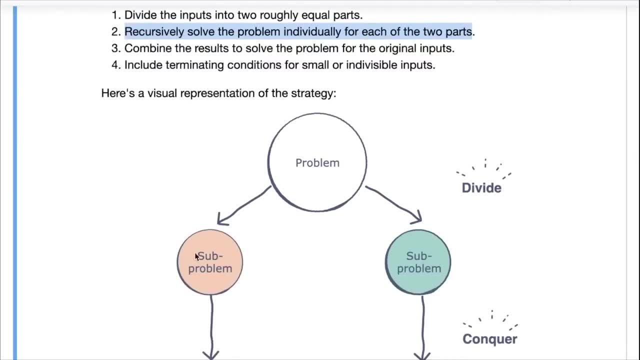 So Then we use recursion, So we recursively solve the problem individually for each of the two parts. So here you have a problem, You've created two sub problems out of it, and then you call the recursion. So the recursive solution itself will use divide and conquer, and then we'll keep going and so on. 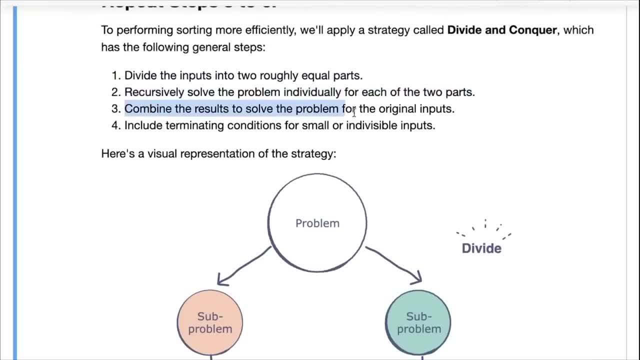 but once it gives you the solution, combine the results to solve the problem for the initial, for the original inputs. Okay, So you have now results of the sub problems and you combine them and you get back the final result, And then the only last thing you need to know is because you're going to keep calling this, keep doing this division recursively. 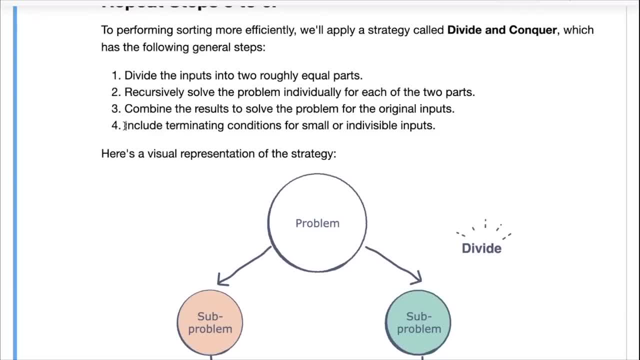 So if you have an input of size a hundred, you will call the same function on inputs of size 50 and 50. Then you will call the same function for each of those 50. You'll call the same function on inputs of size 25 and 25.. 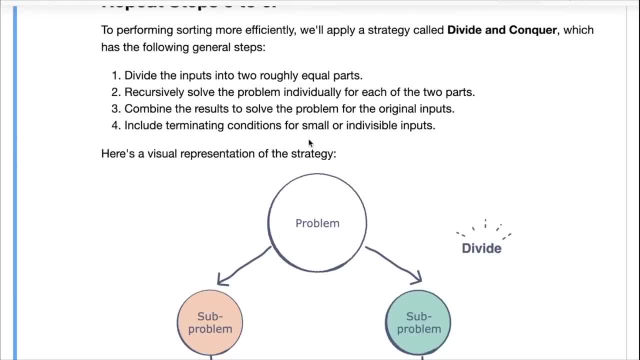 So, each half, and as you keep going, you will eventually end up with small or indivisible inputs, And that is where you can solve the problem directly and include Terminating conditions. So that's where the recursion stops. Okay, So you include dominating conditions for small or indivisible inputs. 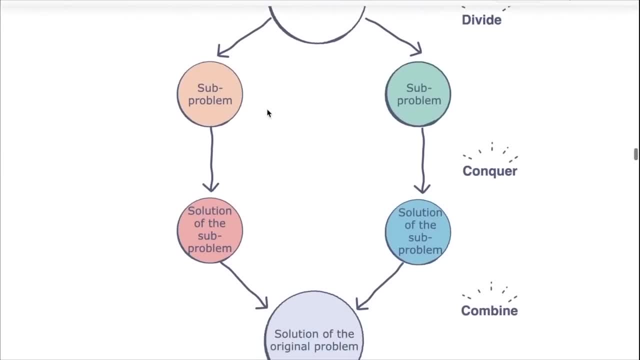 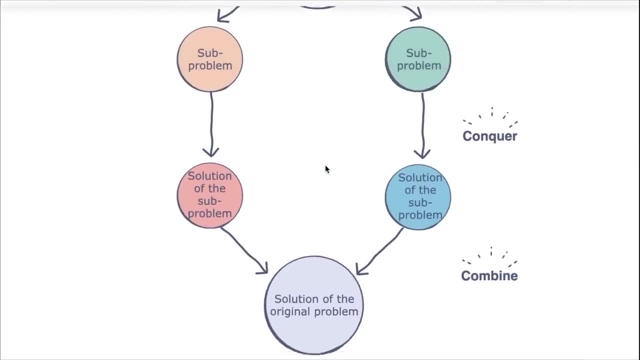 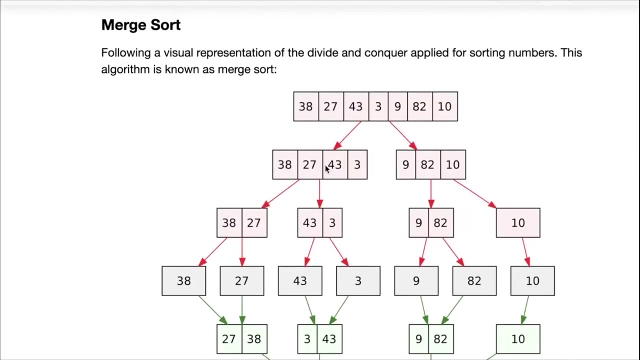 So that's divide and conquer. You take the problem divided into two sub problems, recursively solve the sub problems, get the solutions of the sub problems and then combine them. So you can also call it divide, conquer, combine in some sense And merge. sort is the algorithm. that is the classic application of divide and conquer to the sorting problem. 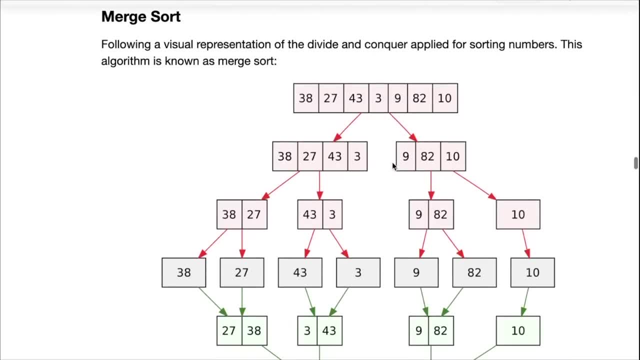 So let's take a look at merge sort by looking at an example, visually. So here we have a list that needs to be sorted in increasing order. So remember step one. divide the problem into two sub problems. So here we have half the list, a little more than half here. 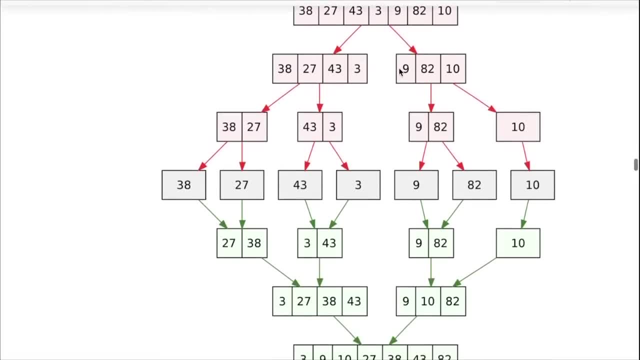 We have another half, So we have split it into four elements and three elements. Then we take, we call recursively, We call the same sorting problem, The same algorithm on these. So we split 38 and 27 into one half and 43 and three into another. here nine, 82 becomes one half and 10 becomes the other. 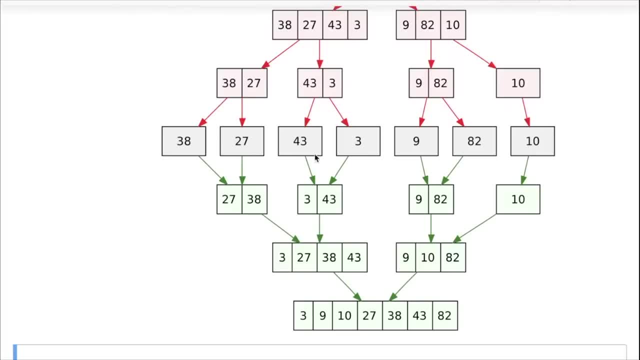 Again, we can split 38 and 27.. We can split 43 and three, nine, 82, 10.. So now we've ended up with single elements, So with recursion, we've ended up at this dominating condition: We can no longer split the list. 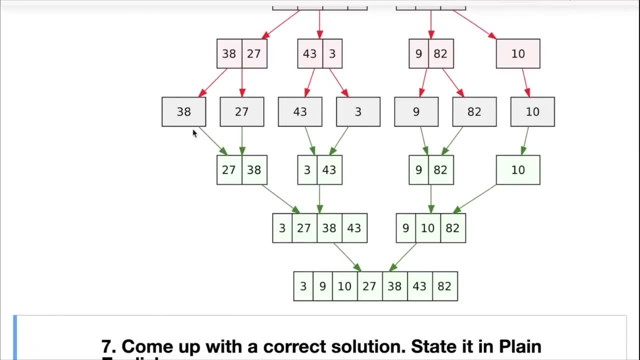 So now we start combining the problems. Now, if you're looking to sort a list with just one element- 38. Well, that list is already sorted, so you can return that. and 27 is already sorted- the single element, So you return that. 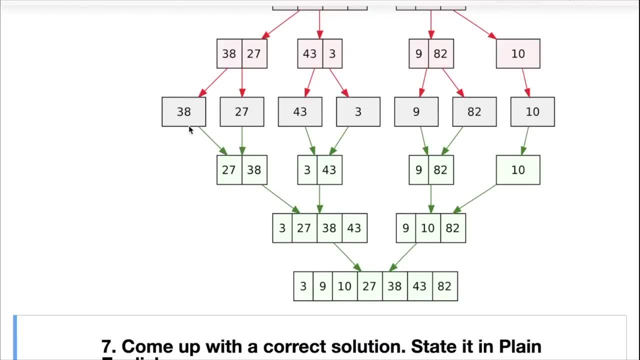 Now we have these two sub lists and we need to combine them. Each has one element, So we can simply compare these two elements and we can tell that 27 comes first and 38 comes second. So that's how you combine these two results to get 27,- 38.. 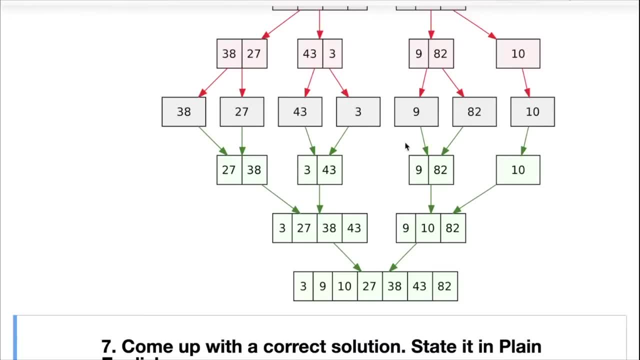 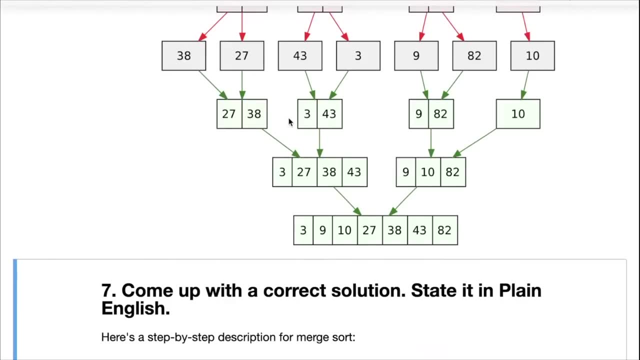 Then, similarly with 43, three, you combine them to get three, 43, and you get nine, 82 and 10. next, You can combine these two Results. So this is where now the combination is important. Okay, We need to look through and we can probably tell that three should come first, and then 27, and then 38 and then 43. 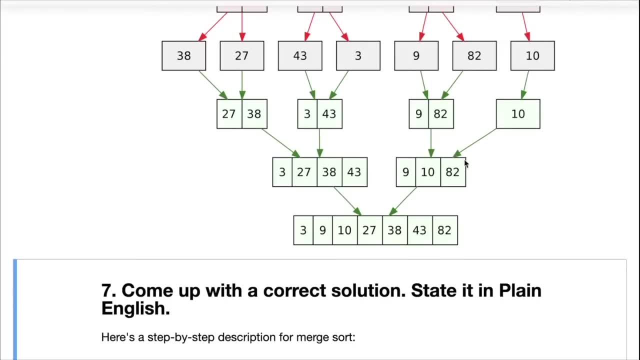 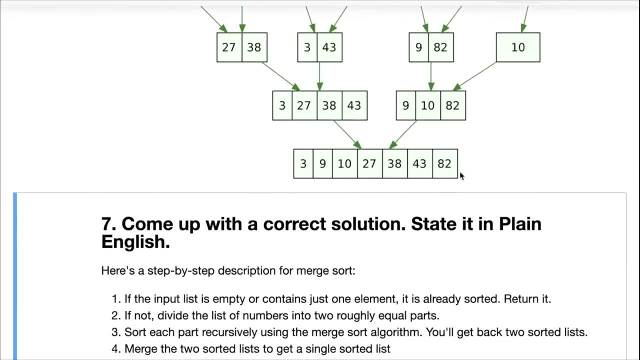 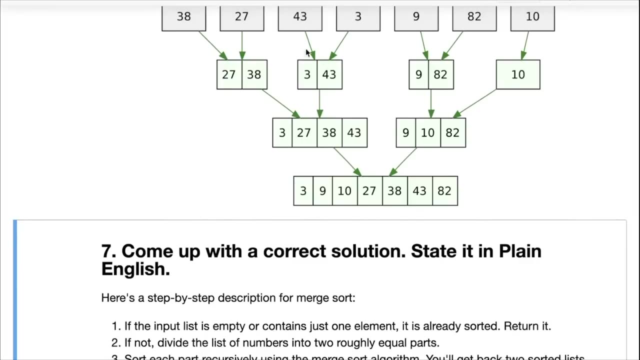 So we've combined them here, And similarly here we've combined nine, 10 and 82, and then we take the final results, these two finalists, and then we combine them back to get the fully sorted list. Okay, And we'll talk about this combination, or what is called the merge operation, in a lot more detail soon. 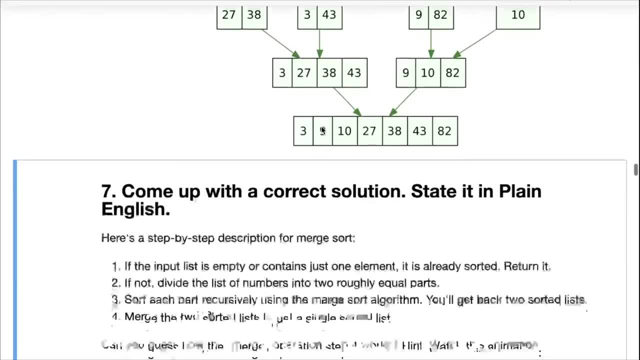 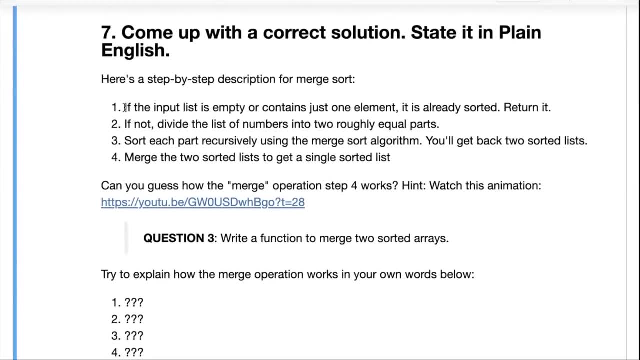 But this is roughly the idea here. You keep splitting it into half and then you combine the halves. So let's now state it in plain English. So first the terminating condition: if the input list is empty or contains just one element, then it is already sorted, or return it. 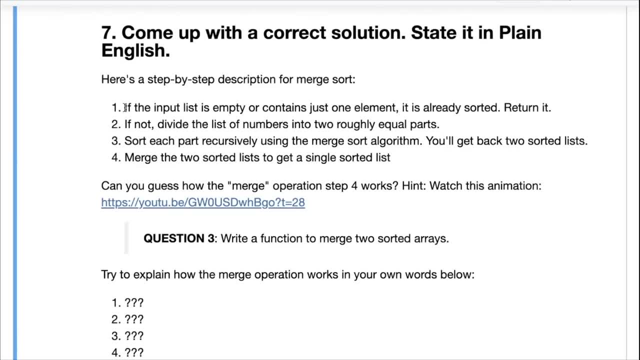 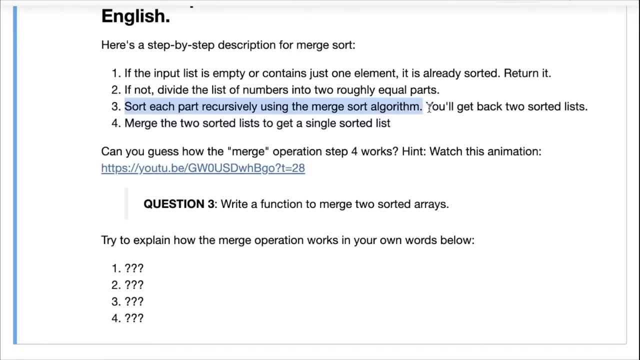 If it is not, divide the list of numbers into two roughly equal parts, then sort each part recursively using the merge sort algorithm And By the power of recursion you will get back to sorted lists. Then merge the two sorted lists to get a single sorted list. 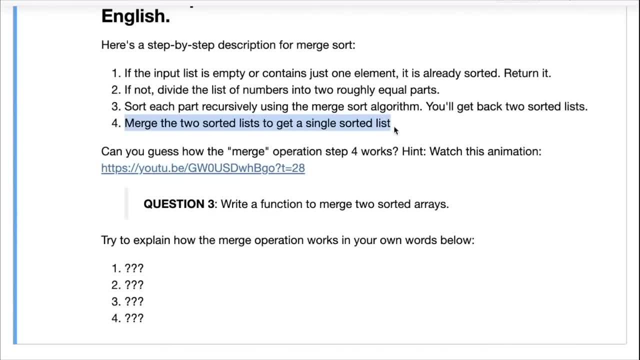 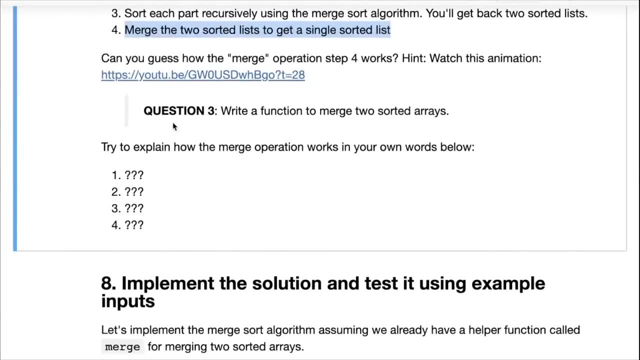 And this is the key operation here And this is why it's called a merge sort, because we are always merging sorted list and making bigger and bigger sorted lists out of them, And the merge operation is something that you may be asked to write in an interview or a coding challenge, apart from the whole merge sort operation itself, 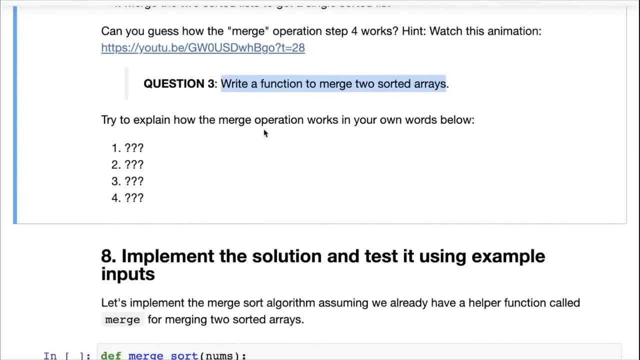 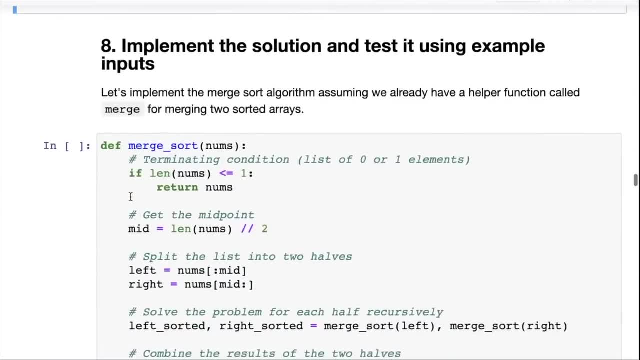 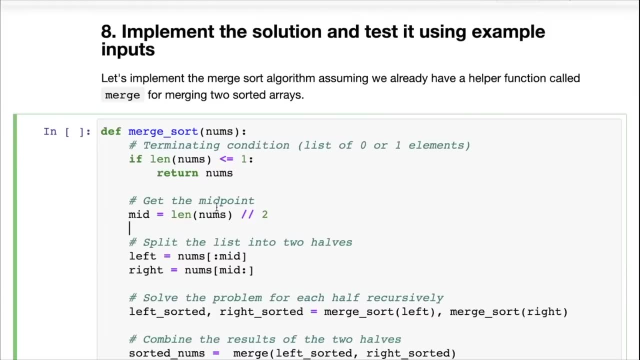 So this is something that you can try to explain yourself. So try to think about how the merge operation might work and explain it in your own words. Here is some space for you, but let's jump into the implementation of merge sort. Now we will implement merge sort, assuming that we already have a helper function called merge. 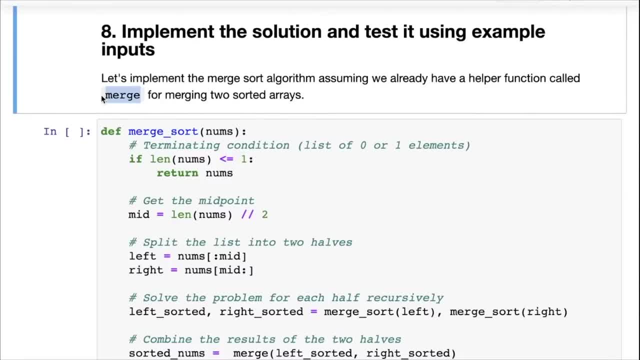 And this is a very useful trick- where your program may need some complicated piece of logic or some logic which you have not figured out. So all you do is assume that you already have the function and write, use it first and then implement it later. 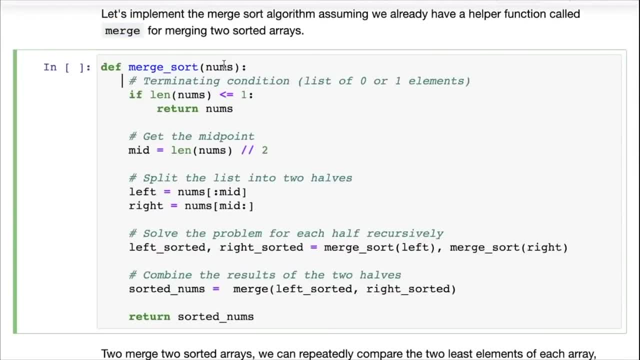 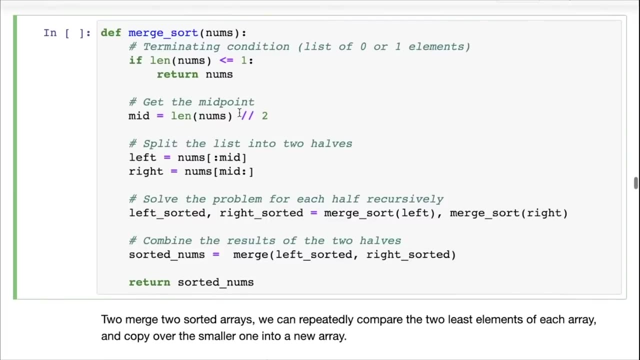 So here's a merge sort algorithm. So now we have the merge sort algorithm and we have numbers here given as an input to merge sort. Now here's the terminating condition: If the length of numbers is less than equal to one, which means if the list is empty or has just one element, return the numbers then. if not, then 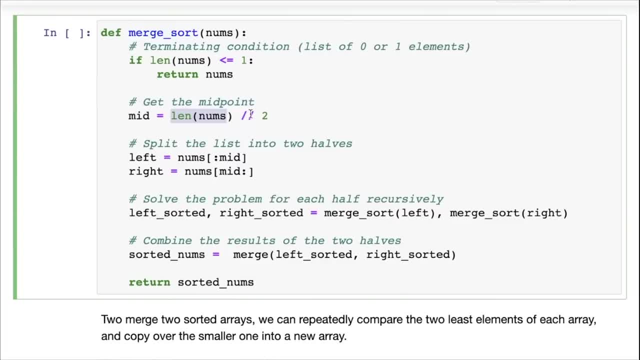 Get the midpoint, So return length of numbers divided by two. And remember using the double slash here, because a single slash would return a decimal and we cannot use a decimal as an index or a position in the list, So that's why we're using the double slash here. 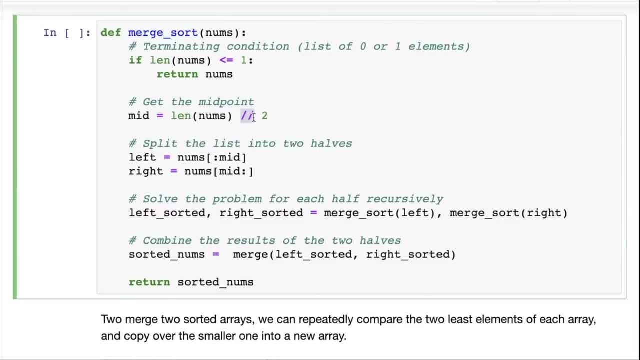 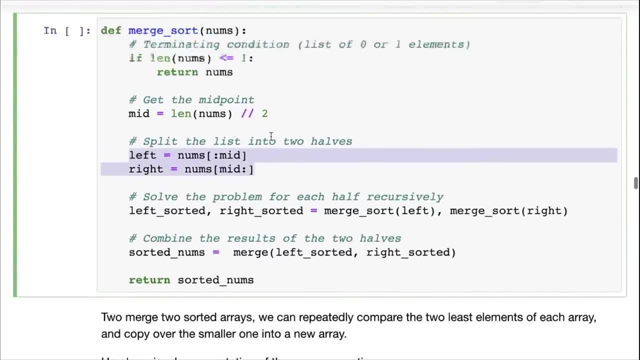 So we take the length of numbers divided by two. So if the size of the list is 10, so we get back five here- then we split the list into two halves And here's some interesting syntax for you, And let's look into what the syntax actually means. 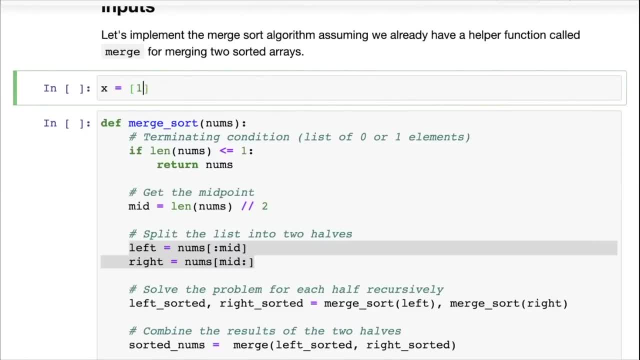 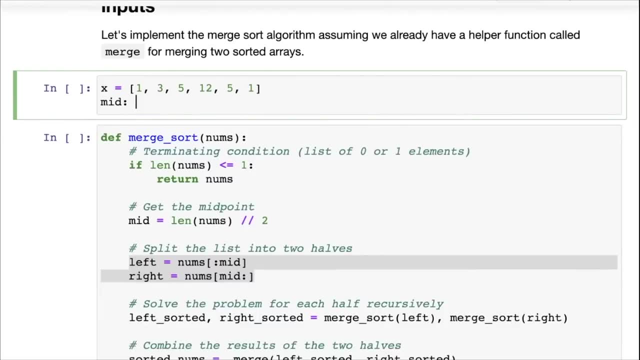 So Okay, Let's say you have a list, So this is a list we have. and let's say, mid has the value. Well, we can check it here: 1,, 2,, 3,, 4,, 5,, 6.. 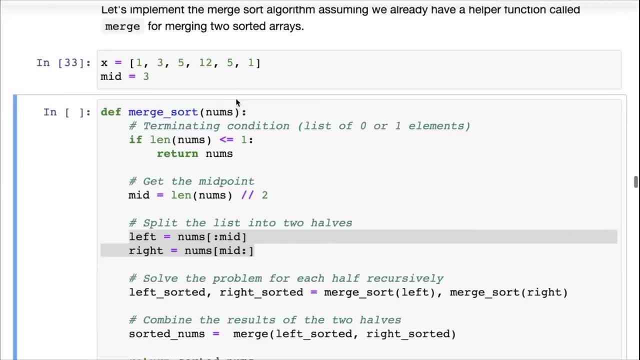 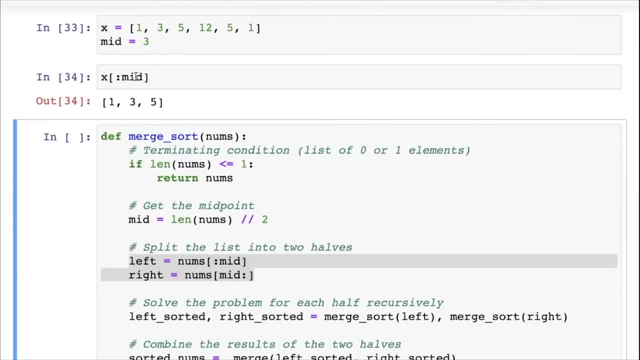 So six elements by two, mid has a value three. Now let's check X of mid. What does that give us? Well, that gives us 1,, 3,, 5.. Well, actually, X of colon made. It means X of zero to mid, and X of zero to mid means all the elements from position zero till before the position made. 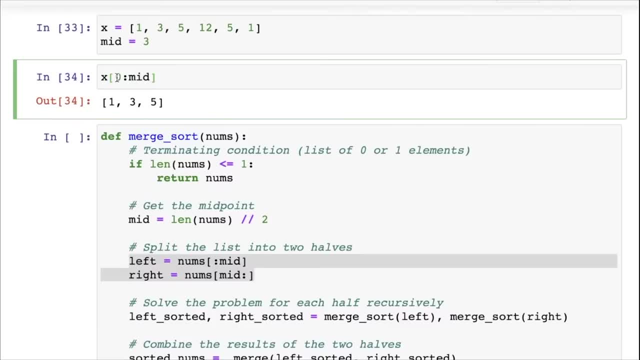 So that's very important. Once again, it's like a range, So you get the indices at position zero, one and two, not at position three. Okay, So that gives us these three elements. Then let's check the other thing, X of mid colon. 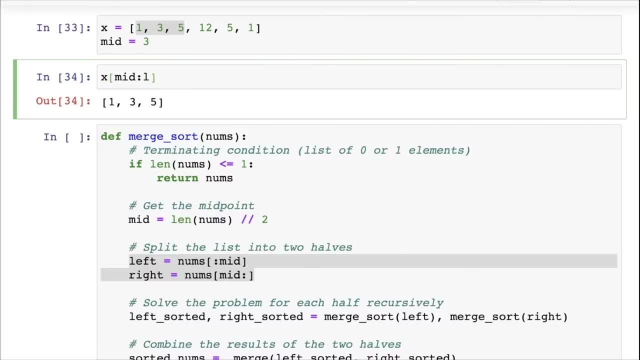 Now, what this gives you is. this gives you the elements Starting from the position made all the way to the end. So you can also write here minus one, or we can also write here Len of X minus one, but or we can just skip it, and 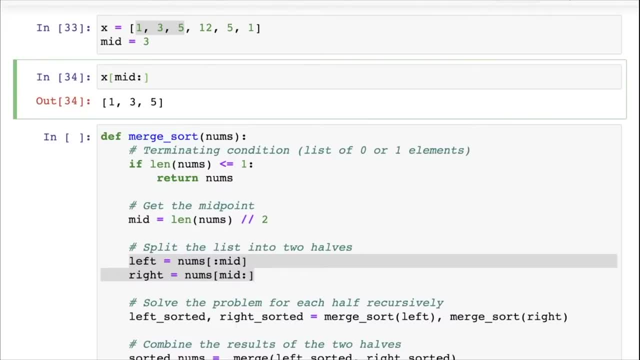 Python will automatically interpret that you want all the elements starting from mid to the end, That is, 12, five and one, So positions three, four and five, and hence to split the list, all we need is to invoke this: 1, 3, 5, and 12, 5, 1.. 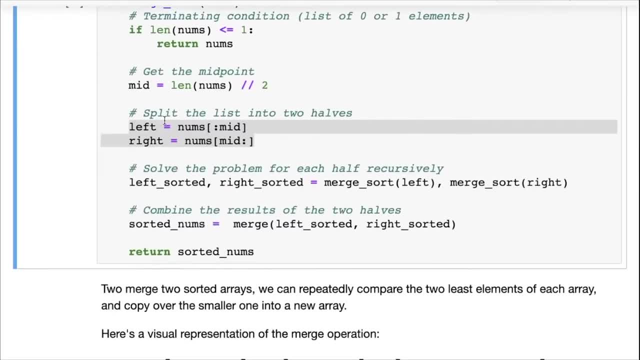 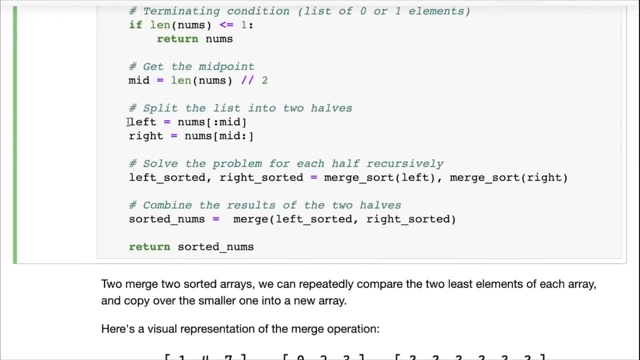 We get back two parts of the list. So this is a nice thing about Jupiter. Whenever you don't understand a line of code, just create a cell above or below and try out a simple example. So now we have the left half, nums zero to mid, and then the right half. 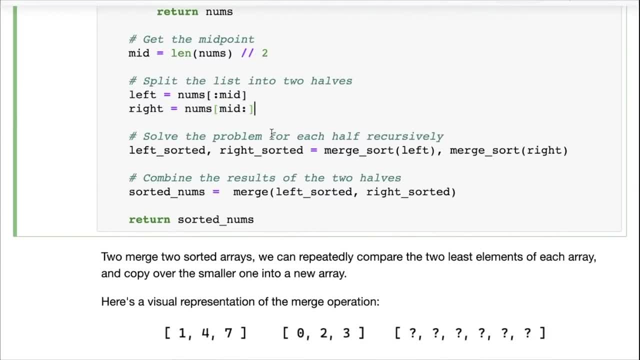 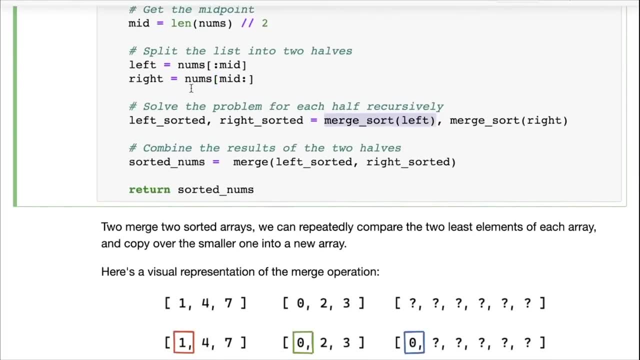 So nums mid colon. Now here's where the magic happens. We call the function recursively, So we call the merge sort function itself, So we call, we call merge sort on left, and that gives us back a list, a sorted list for the left. 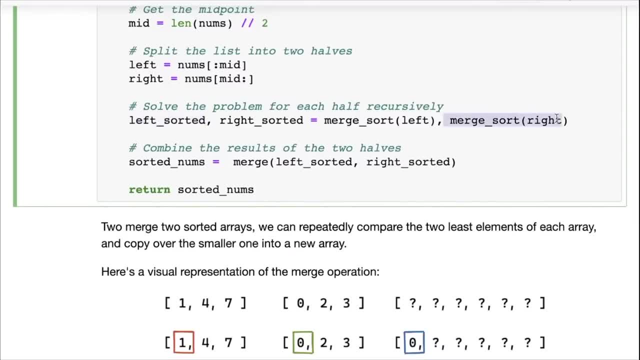 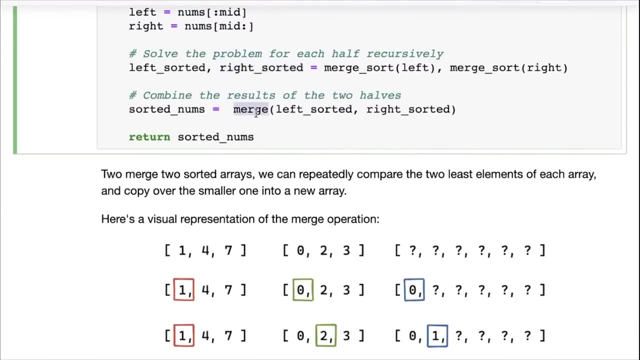 Half called left sorted, And then we call merge sort function right, And that will give us back a sorted list called right sorted, And then we combine the results of the two halves by calling the merge operation. So we now- we are now saying that we want to merge left sorted and right sorted to get back the final sorted numbers. 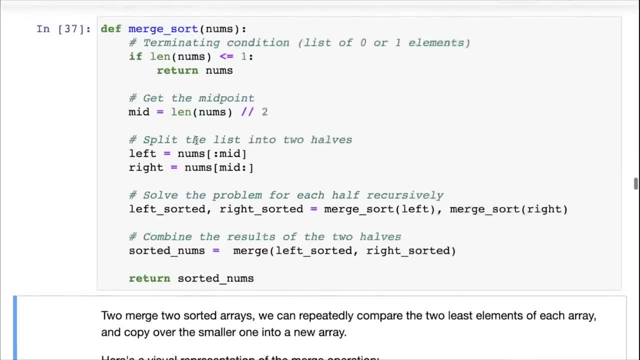 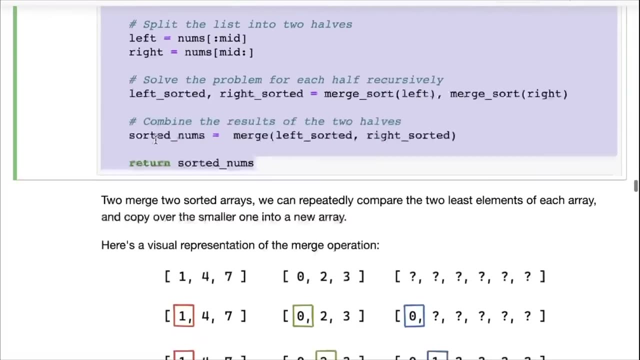 And then we return the sorted numbers. So that's much sort. So, yeah, it's almost seems like magic, but it's pretty small, pretty straightforward, Only Okay, About four or five lines of code If you combine some of these lines. so then let's come to the merge operation, because that seems to be the meat here, right? 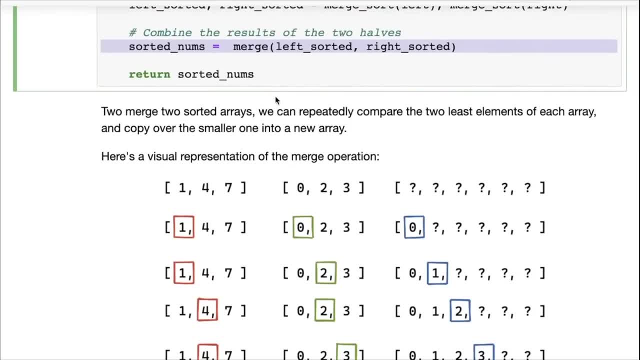 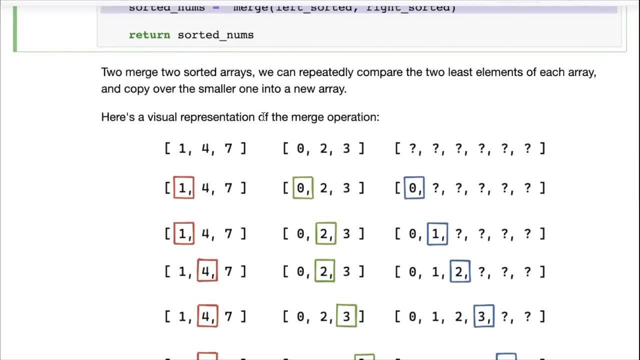 This is the only missing piece. So too much to sorted arrays. What we can do is we can repeatedly compare the two least elements of each area and copy over the smaller one into a new area. So here's what that process might look like. 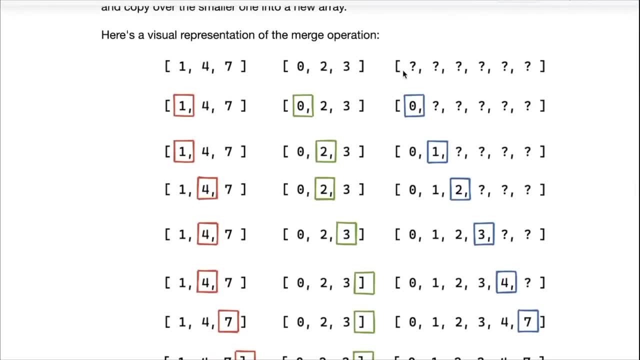 Let's say you have these two parts- one four, seven and zero, two, three- and we want to get this sorted list and notice that these are both already sorted because these are the results of the recursive cost to merge sort. So we keep a pointer on the left on each one. 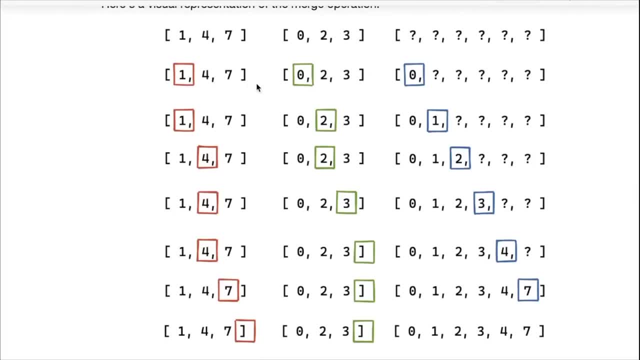 So here we have the pointer at one, Here we have the pointer at zero. We compare the two, We take the smaller one and put it in the list. How do we know we can put it? Because if this is smaller than this, all these numbers are also greater than zero. 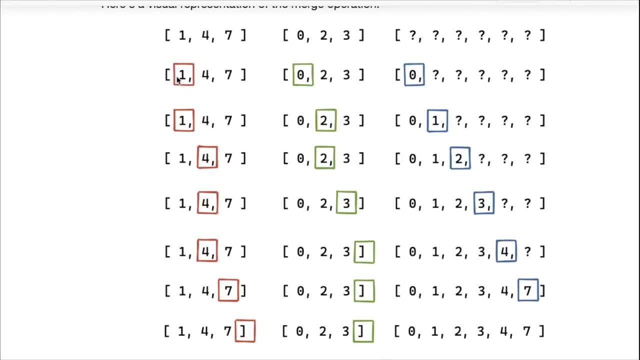 And then, since one is greater than zero and all these numbers are greater than zero or greater than one, so that follows that all the other numbers to the right of one and to the right of zero are greater than zero, and hence zero should come in the first position. 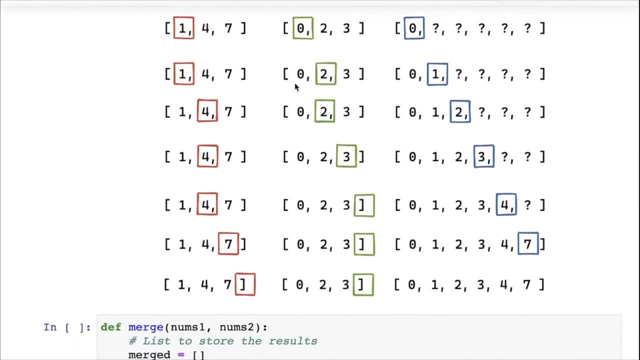 So we put it there and advanced the pointer. Now you can see here, Now we can compare one and two, and this time one is smaller, And you know that all the numbers here are greater than two, So they're also greater than one. 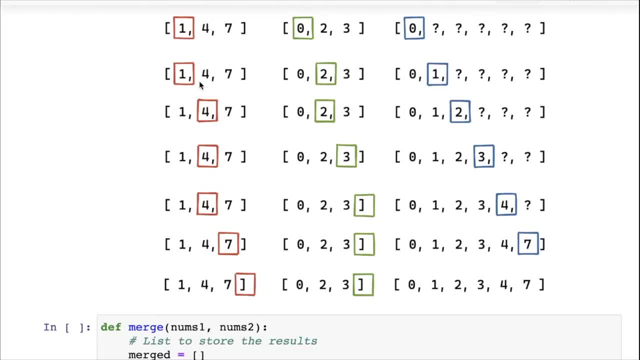 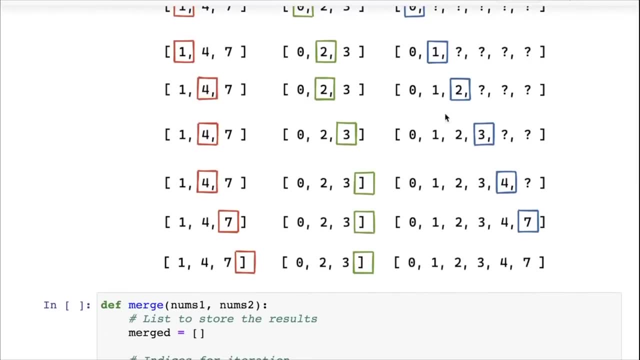 And then all the numbers here are also greater than one. Hence we know that one is now the next largest number, So we can now put in one and advance the pointer and keep going. this time Now you compare two and four, So now you can put in two. 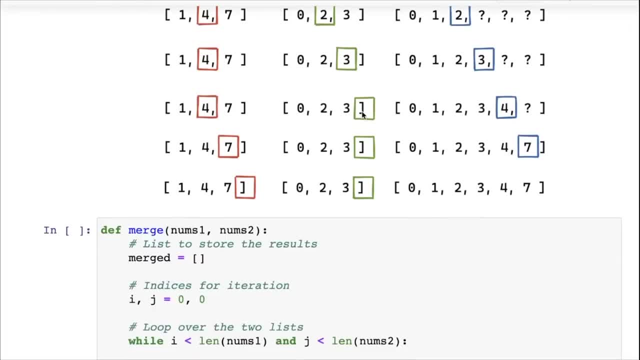 And Advance the pointer. Now you put in three and then advance the pointer And at some point you will exhaust one of the lists. And when you exhaust one of the lists then you can stop comparing and you can simply copy over the remaining elements. 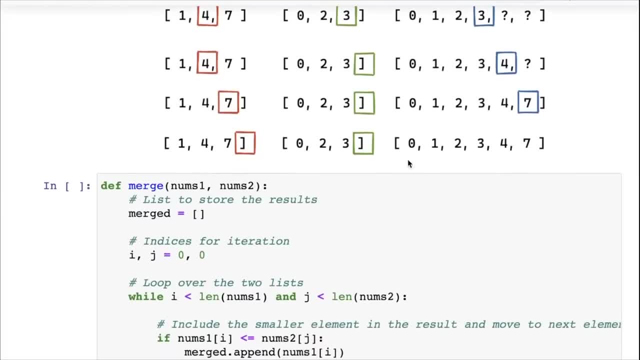 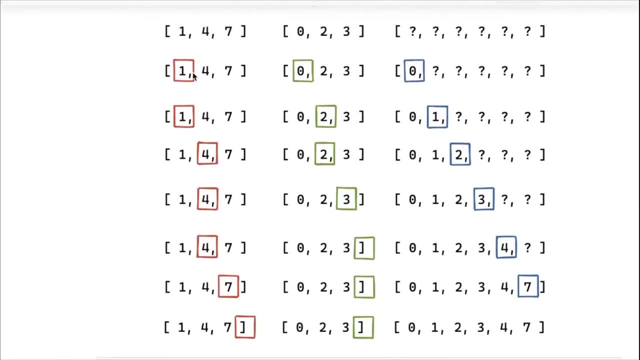 So we can now copy over four and seven and we've exhausted this list and we get back the sorted most areas: 0, 1, 2, 3, 4, 7.. So it's really simple. It involves each step, involves one comparison and incrementing one pointer. 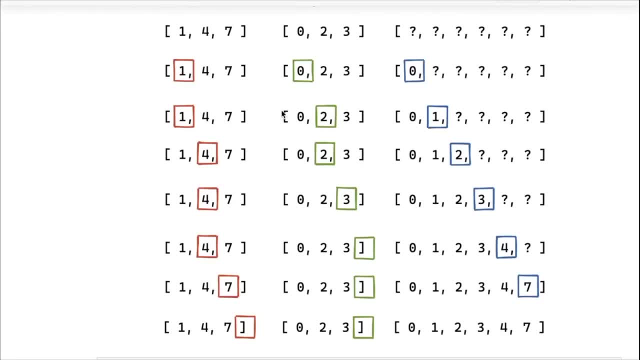 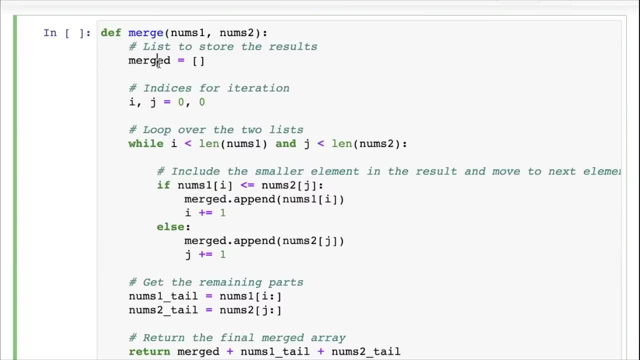 So you're either incrementing this pointer or you're incrementing this pointer, Okay. So let's now define the merge operation and you can see the benefit now of assuming that the function already existed. Now we do not have to worry about the actual sorting and recursion et cetera. 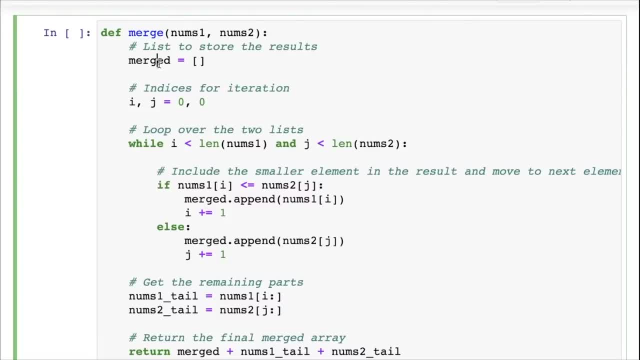 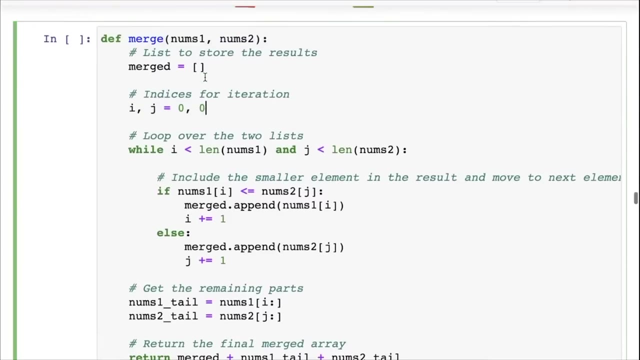 We simply have to worry about merging two sorted arrays. So first we'll create a list to store the results, and we have nums one and nums two, the two left and right lists that we are going to combine. Then we are going to set up two indices or two numbers for iteration. 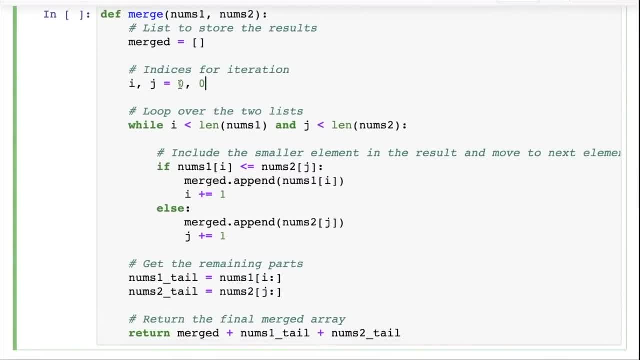 The two pointers on the two lists and we set up each of them at position zero. So each of them are currently at position zero here and we loop over the two lists. So we say: while I less than Len of nums one and while J less than Len of nums two. 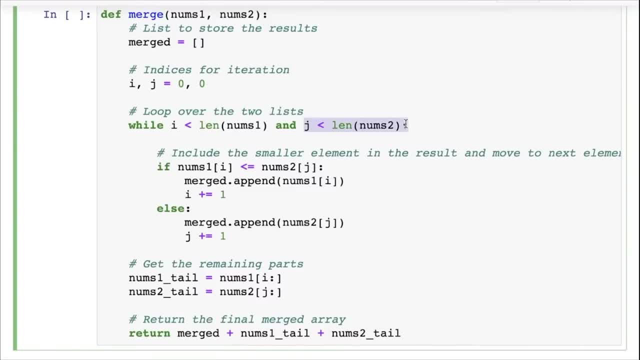 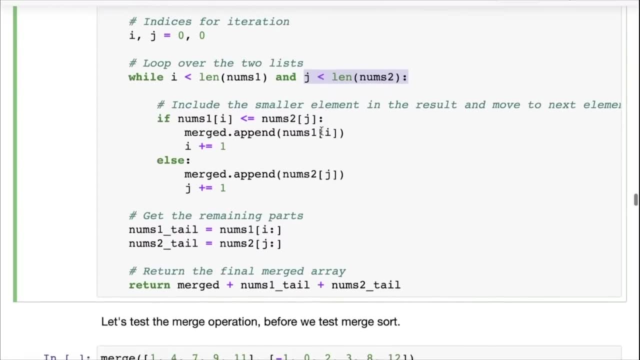 So if you have four elements in the left list, then I can go from zero to three- all four positions. And if you have five elements in the right list, Jay can grow from zero to five, zero to four- all five positions. 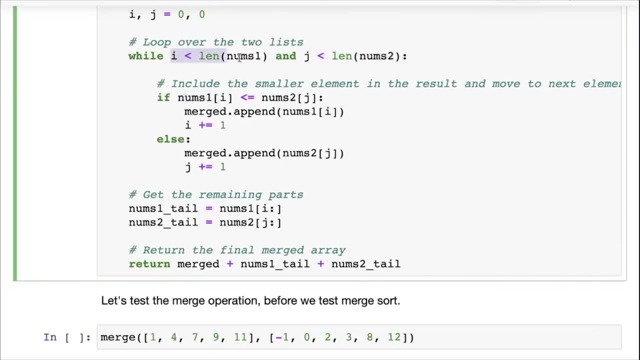 Then we check and we remember. we want to make sure that both of these indices are valid. If any of those have reached the end, then you want to skip and we can simply copy over the remaining list, Right? So, as you see here, as soon as we reach this point, there's no more comparisons to be made. 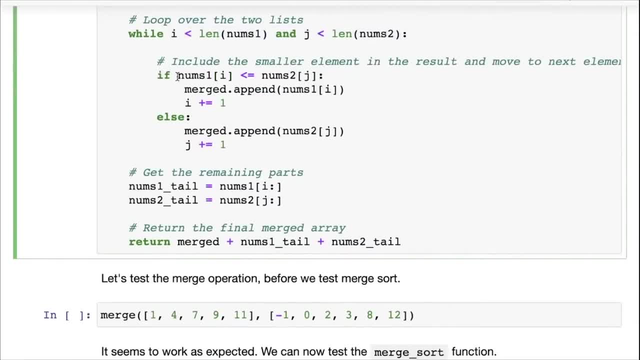 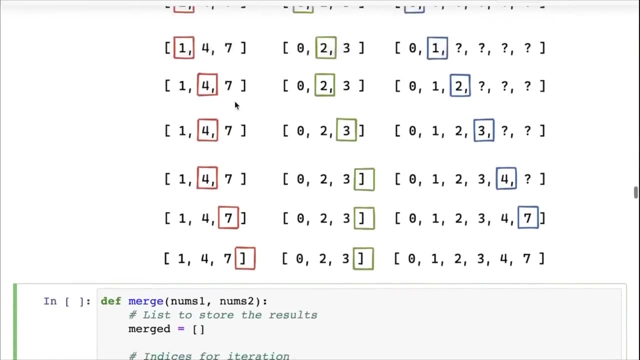 So we can exit the loop. So now we check which one is smaller. So if we, if nums one I, so the left list current element is smaller than nums to J, Then we append to the merge list Noms one I, as we did here, and we increment I. so this is exactly what we've done here. 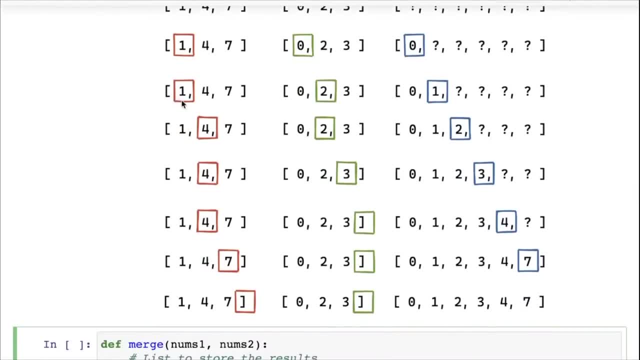 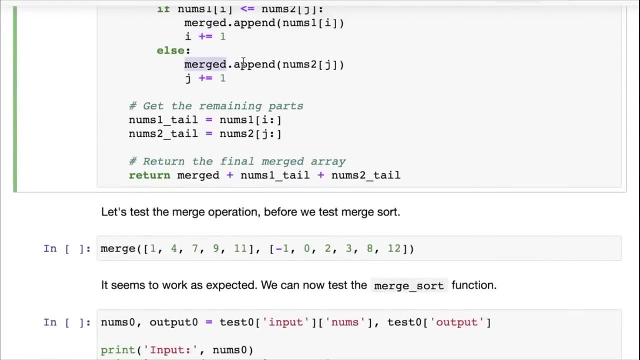 So we put in well, let's say here: So we put in one here and we increment the left pointer. on the other hand, if that's not true, we append the element from the right, So nums- to J, and we increment the right pointer. 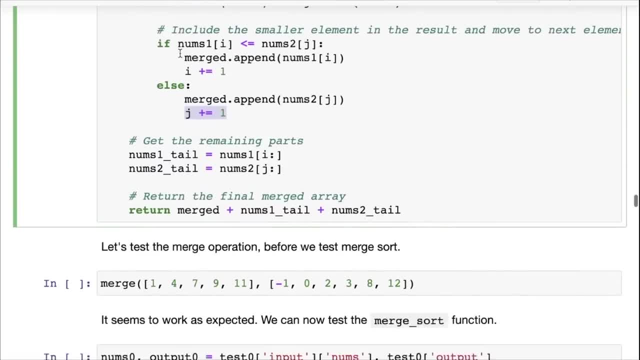 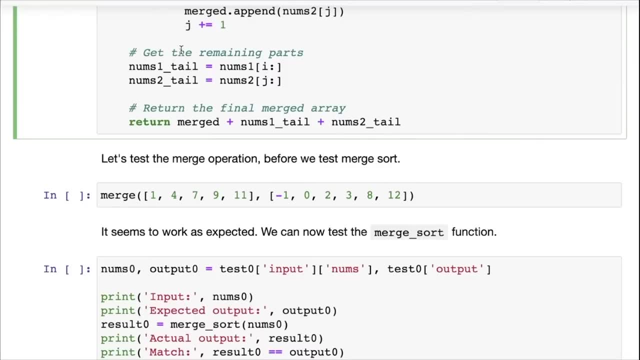 So in each case, in each while loop, we are incrementing one of the pointers and then, when the while loop ends, one of the pointers, One of the lists, would have been exhausted. That's when the while loop ends, so we can get the remaining parts of both the lists. 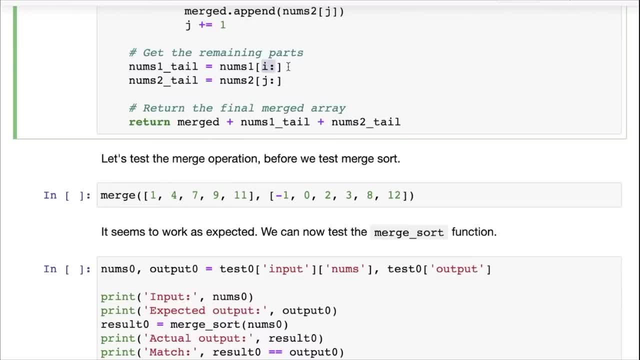 So we can get nums one, I colon. we'll get the remaining elements on the first list. The left list now is to J colon. We'll get the remaining elements from the right list, But remember, since one of them is exhausted, so one of these two is going to be empty right now. 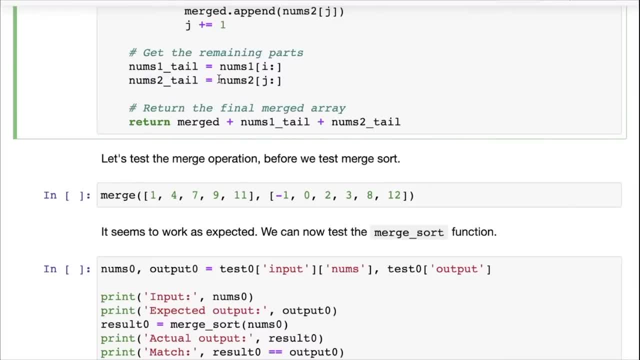 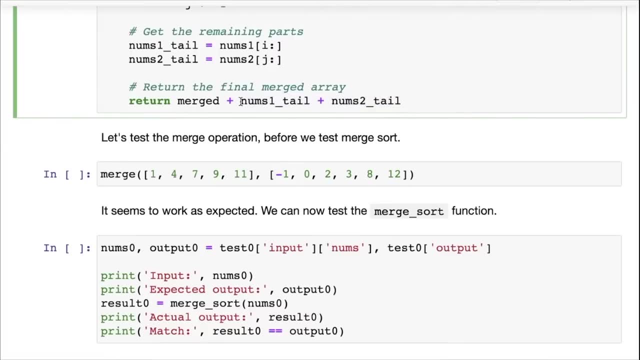 We. we can check which one is empty and simply add the remaining one. but here's a simpler solution: We just add both of them to the most area. So we append Both the lists at the end and this automatically takes care of the empty case. 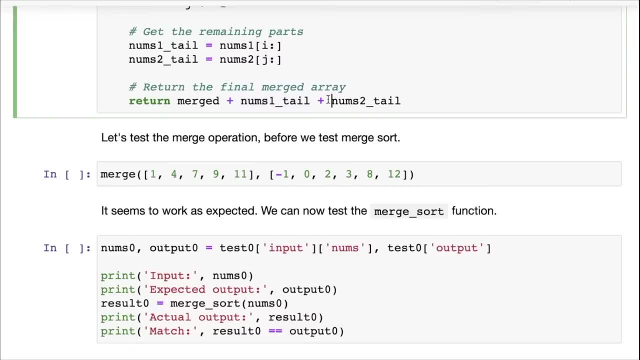 If the left side becomes empty, then this adds nothing to the most area, And this adds the remaining numbers from the right side. If the right side becomes empty, then this adds the remaining numbers from the left left side, and this adds nothing. 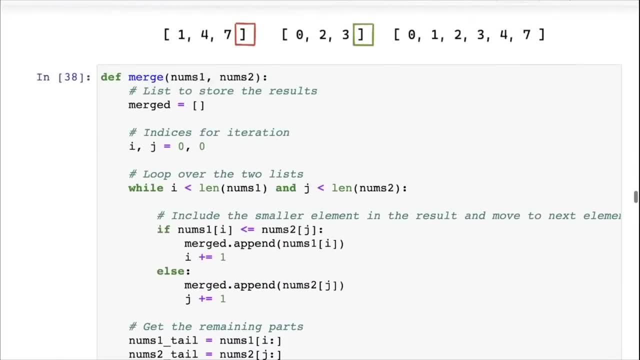 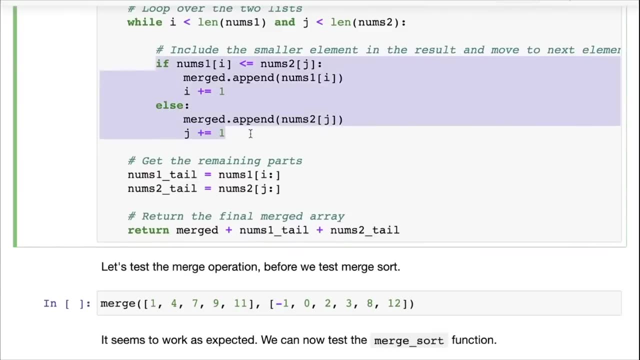 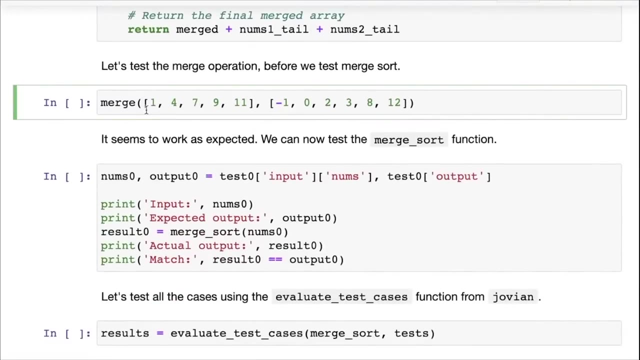 So that's a small trick. So that's the merge operation, Again, not very difficult. If you have any questions, take this out into specific cells and try it out with examples, And you Should see it working. So let's try out the merge operation now. 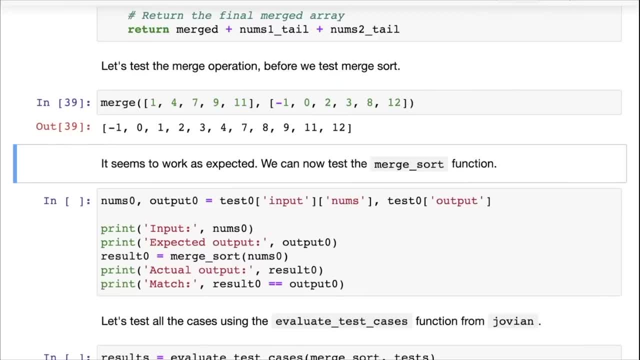 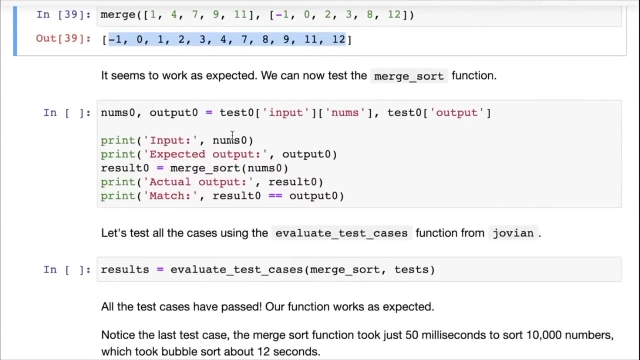 So here we have two sorted lists. You can see here and there you go. You can see that this is now arranged. All these numbers are now arranged in a sorted order. So now we have the merge operation and we have the merge sort operation. 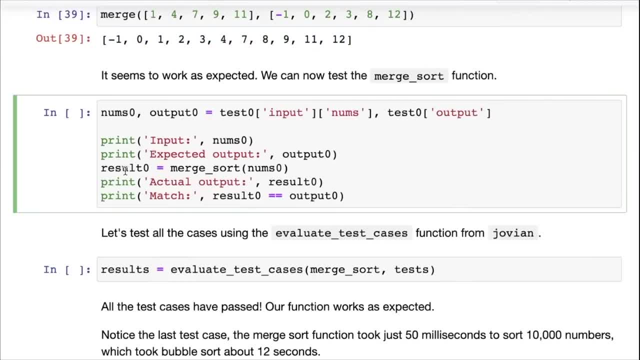 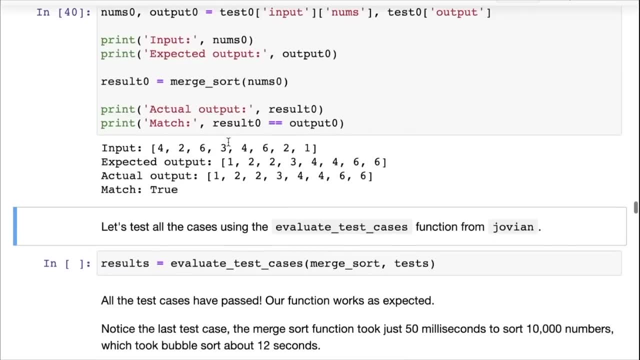 So we can now test out the merge sort function. So we get the first set of inputs and outputs from test zero And you can see here that this is the input and this is the expected output And this was the actual output as well. 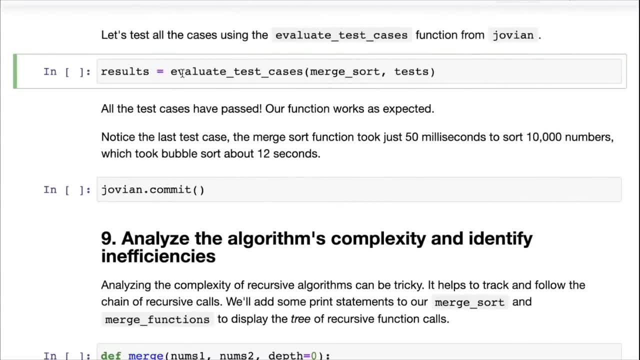 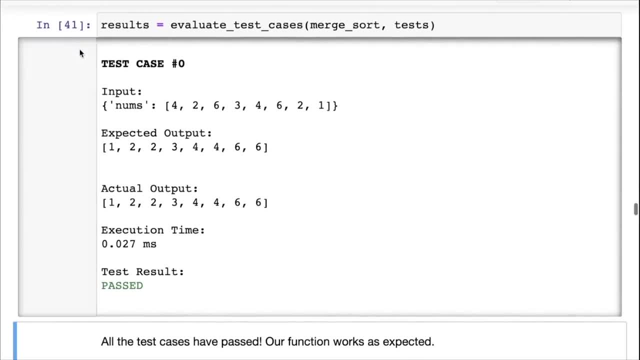 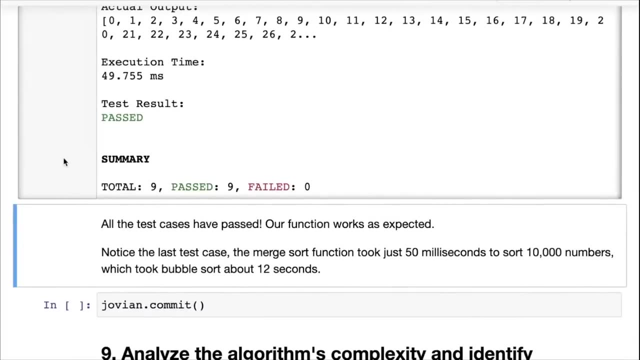 Now let's test all the cases using the evaluate test cases function from Jovian. So here we're simply going to call evaluate test cases on the entire list of test cases And you can see all the test cases seem to be passing. Now, if one of these tests 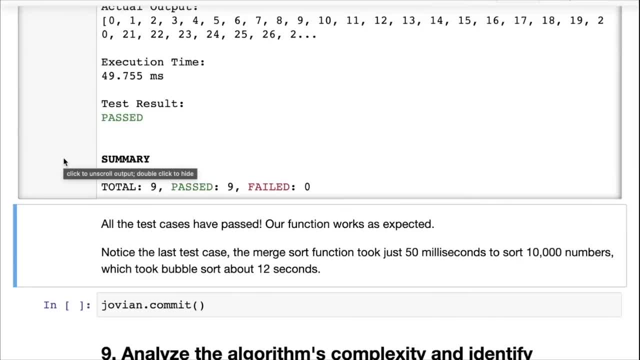 Cases had failed. what you should go do is you should go back and add some print statements inside your merge function, or add some print statements inside your merge sort function. The right places to add the print statements is right after the function definition- right. 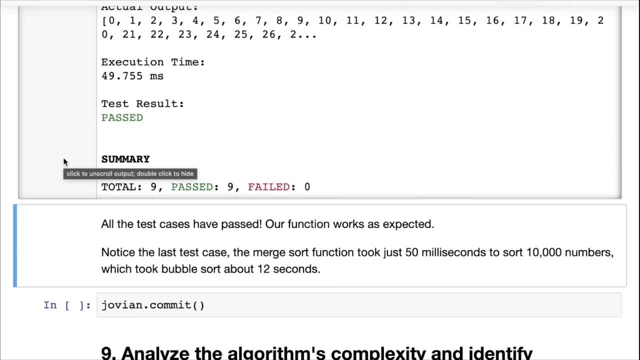 After, in the body of the function, it can be the first statement and then inside each loop. So inside each loop, whatever are the changing parameters, you should print them inside a loop And then, finally, you can also print the return value of the function. 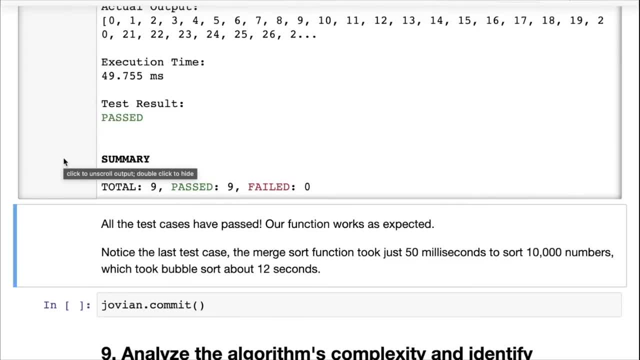 So in this way you can build a full picture of what the what your function is doing, And that makes it much easier to solve issues. So test cases and print functions make it easy to fix errors in code And don't worry if there are errors- there are always errors in code. 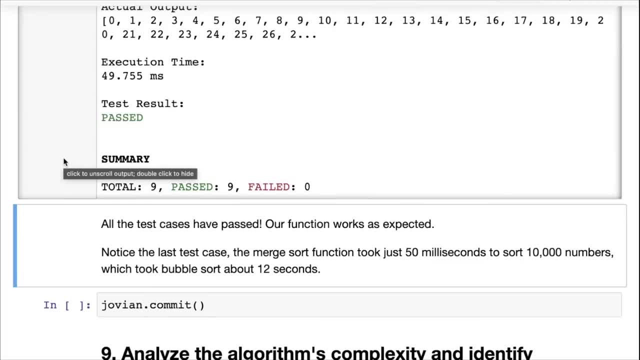 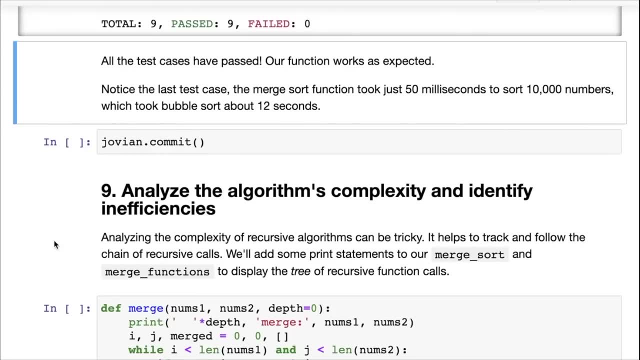 What's important is you should be able to find a way to fix them easily and without test cases or without printing. you may get stuck and you may just keep staring at the code and trying to figure out what exactly went wrong. So please do that. 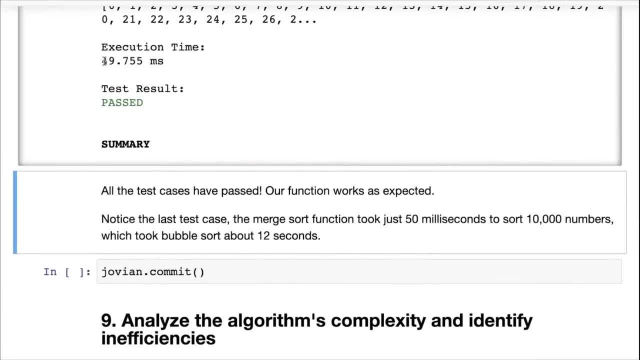 Now, one last thing I want you to notice is The execution took only about 50 milliseconds. On the other hand, remember, bubble sort took about 15 seconds to sort 10,000 numbers, So that's much, much faster right. 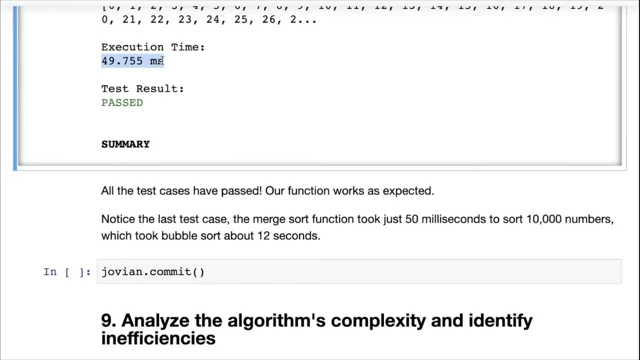 A millisecond is 0.0001, 10 to the bar minus three seconds. So in a second you can probably sort 200 of 200 lists of size 10,000. And that's what makes much sort so much more powerful, and because it is so much more. 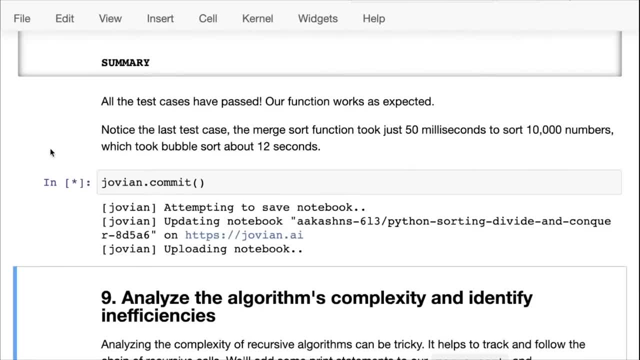 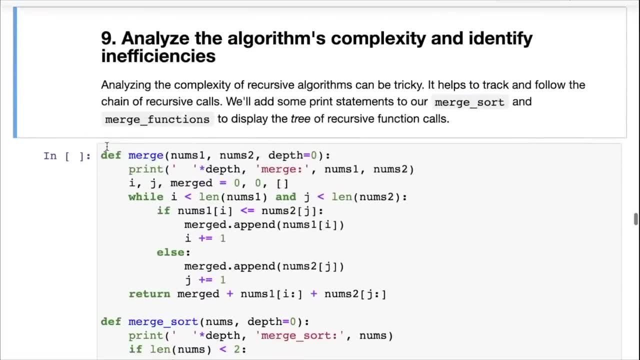 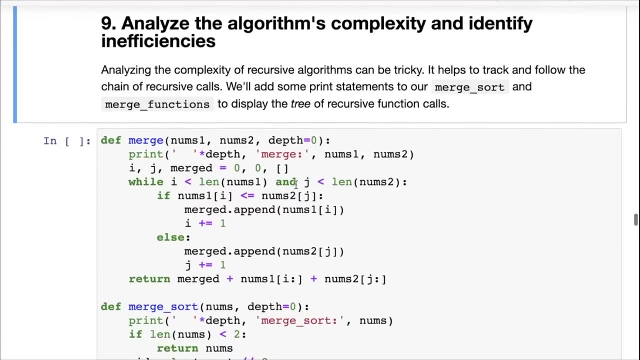 efficient, And as we analyze the complexity, you will learn that much sort is, in fact, more efficient in terms of the bigger notation as well. So let's analyze the algorithms, complexity and identify if there are any inefficiencies. now analyzing recursive algorithms can get tricky, and that's where it helps to track and follow the chain of recursive calls. 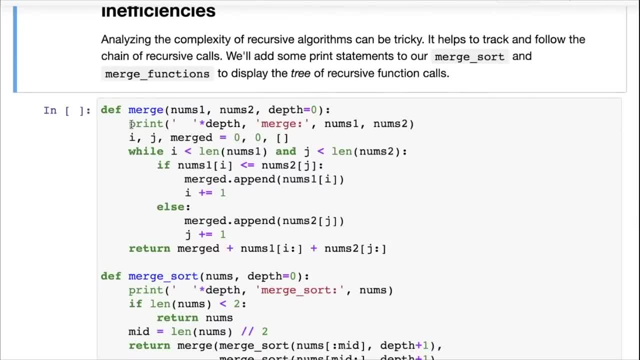 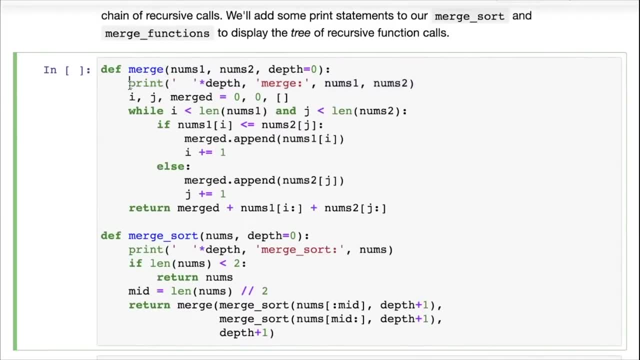 So what we'll do is we will add some print statements to our merge sort function and a merge function, So we'll simply see What the merge sort function was invoked with. Okay, So we'll add a print statement inside merge and we'll add a print statement inside merge sort- both of them. 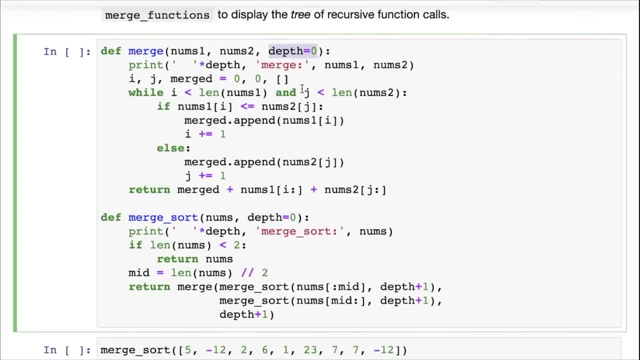 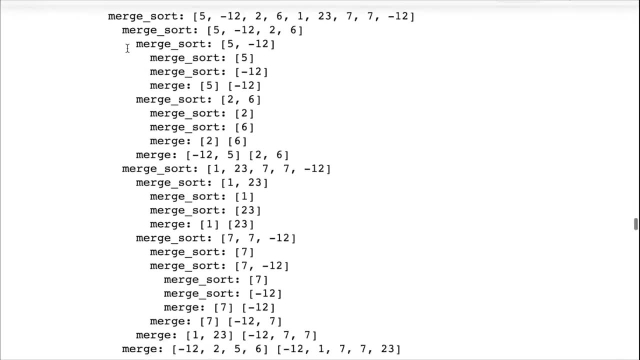 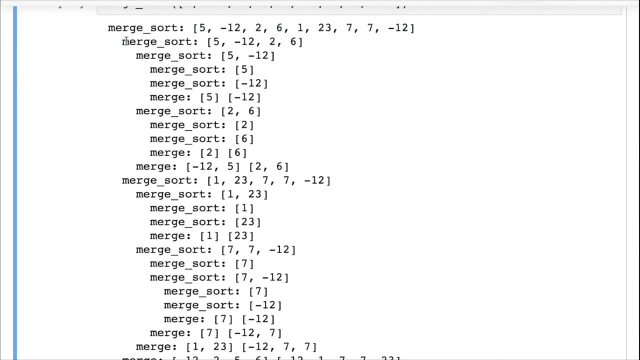 And we are also tracking something called a depth to track the chain or the depth of each recursive call, And you'll see what I mean in just a second. Okay, So this is what it looks like. We called merge sort on this big list of elements unsorted, and that merge sort internally led to two calls of merge sort. 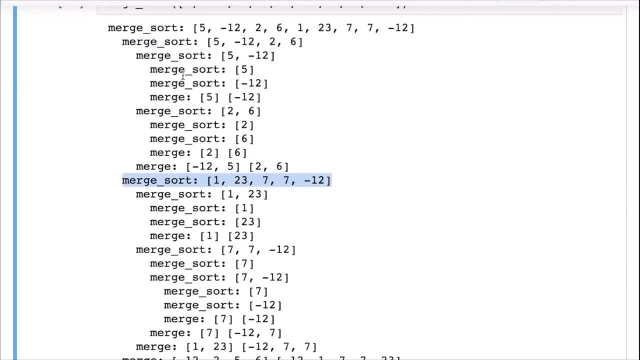 So you can see this one here and this one here. So you have two calls to merge sort, one with the left half of the list and one with the right half of the list, and they're unequal And these two merge sorts finally returned merge lists. 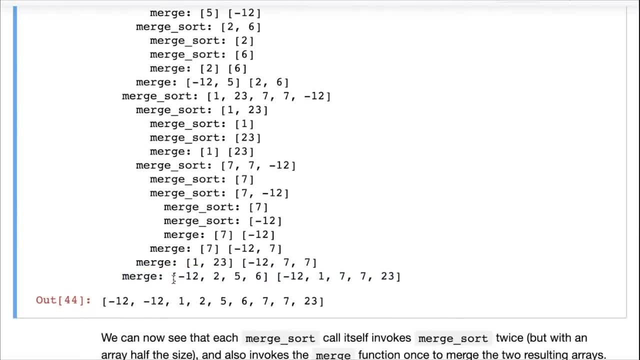 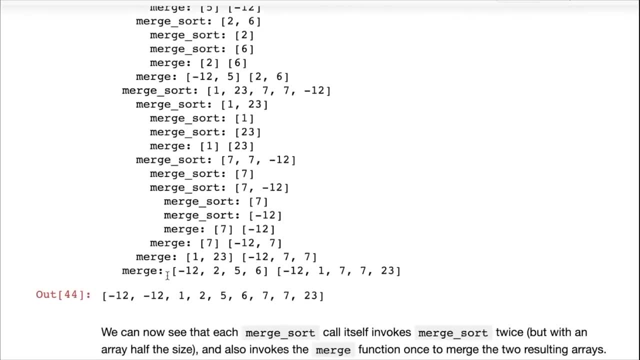 And we finally called a merge operation on the two of them. You can see that this is the merge operation, the final merge operation called here on the two merge sort lists And this merge operation is working with these two sorted lists. Okay, So we can see that each merge sort. 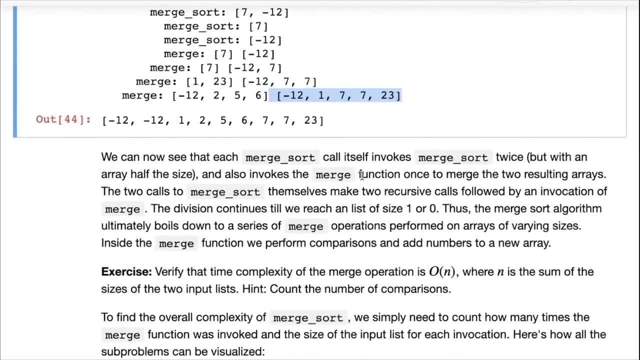 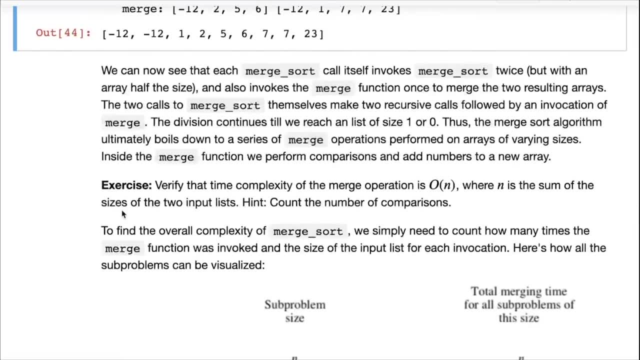 Invokes the itself, invokes merge sort twice, but this time with an area of half the size. you can see, merge sort was invoked with arrays of lists of half the size And it also invokes the merge function once to merge the two resulting areas, the two sorted areas. 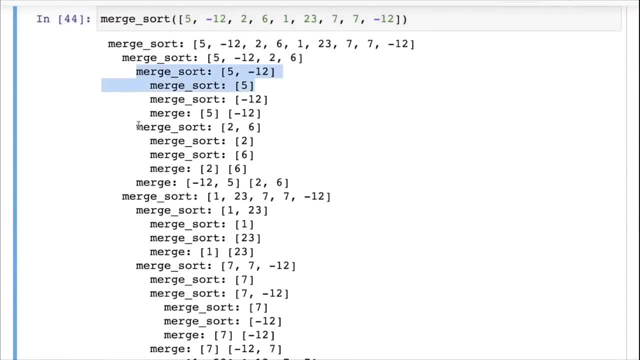 Now the two calls to merge- sort. if you observe closely, they themselves make two more calls to merge sort and one more call to merge. And then those internal calls make two more calls to merge sort and one more call to merge, And so 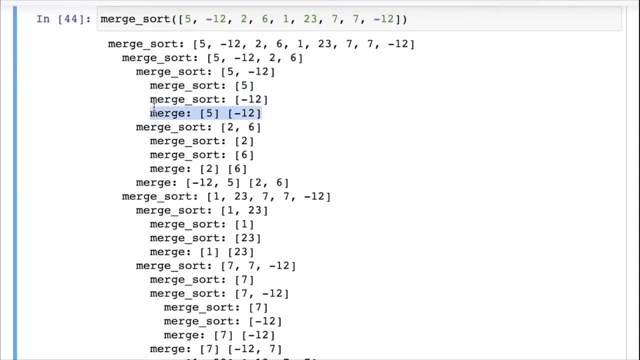 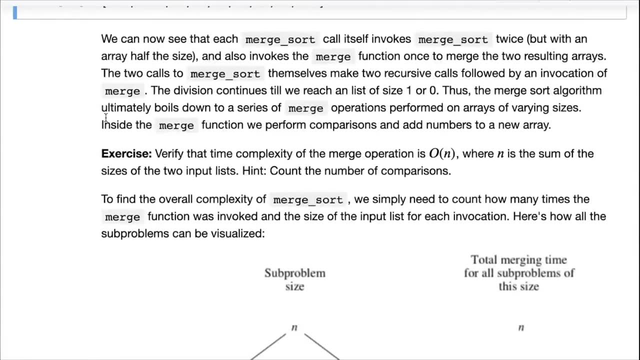 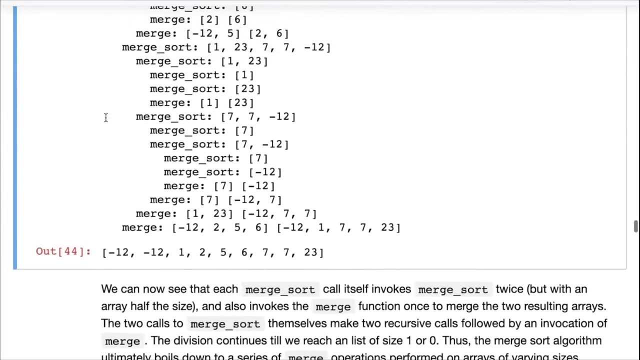 Till we end up with single elements, at which point merge sort simply returns that single element. So the merge sort algorithm ultimately points out to a series of merge operations. You can see here that each merge sort all it's doing is calling merge sort internally and then calling a merge operation. 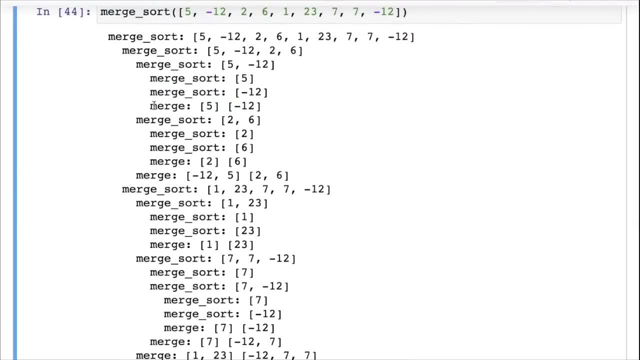 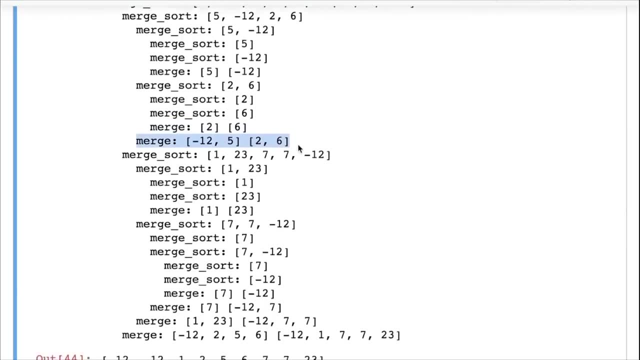 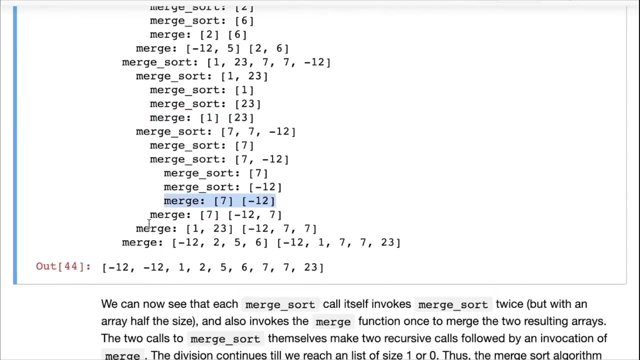 So, ultimately, what we're doing is we are first merging five and minus 12, and then we're merging two and six, And then we're merging minus 12, five and two comma six, and then we're merging one- 23, and we're merging seven minus 12,, and then we're merging seven minus 12, seven, and finally we're merging one, 23 minus 12,, seven, seven, and then finally we are merging the big list, right? 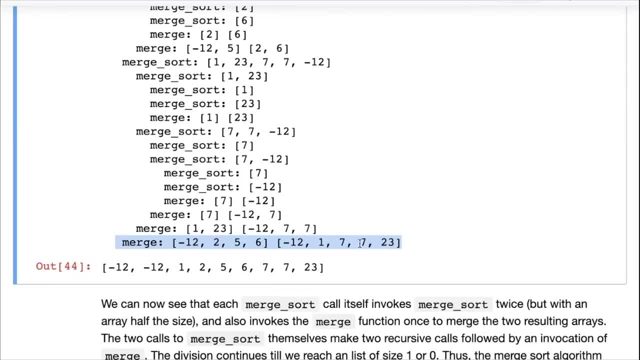 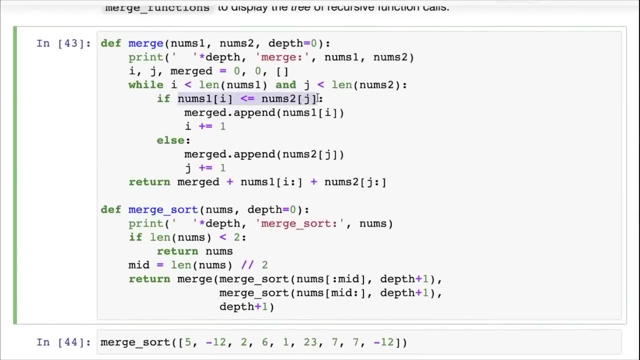 So it's ultimately just a whole bunch of merge operations And if you look inside the merge operation, this is where a comparison is happening And this is where this append Is happening. So Yeah, Step is happening. So we are comparing and appending. 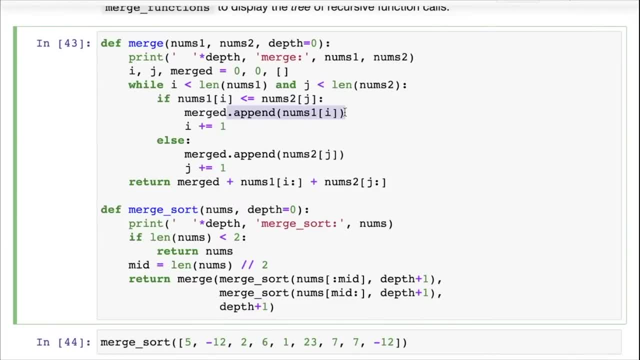 So those are the two key operations here, And with every comparison there is append. So if you simply count the comparisons, once again that's happening. that should be enough to get the time complexity And what is the number of comparisons that's happening? 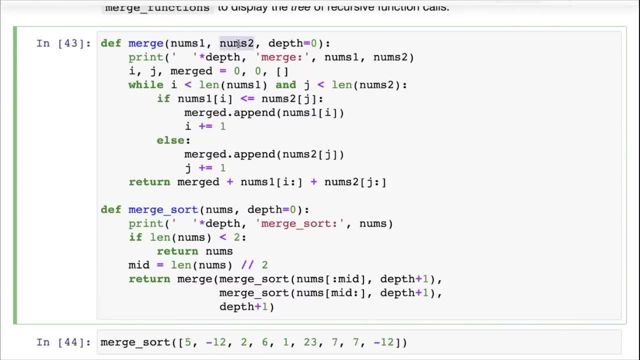 Well, that's straightforward too, If you have two lists, nums one and nums two each, and the total length of the two lists is N. So because the size, the number of iterations is equal to In the, in the worst case it would be equal to the lengths of the two lists combined. 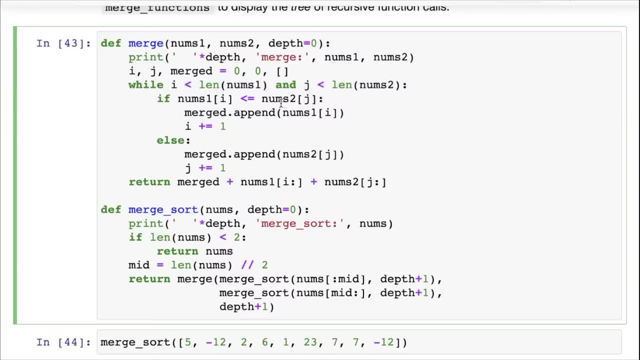 So you may have to first maybe increment I by one, then increment J by one, Then once again increment I by one and J by one. So the total number of iterations here is Len of numbers one plus Len of norms Two right. 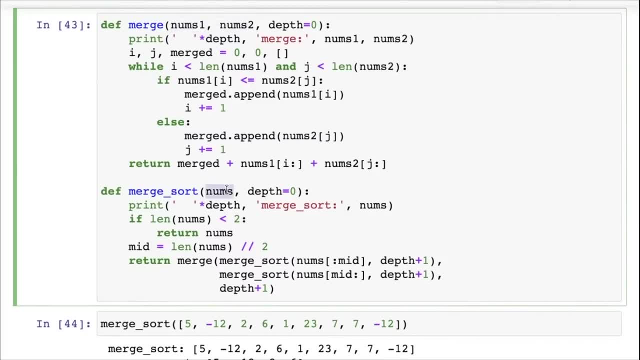 But remember the merge was called. if merge sort was called with a list of size N, then merge was called with a list of size N by two and N by two roughly. So the total list, the total length of numbers, One plus nums. 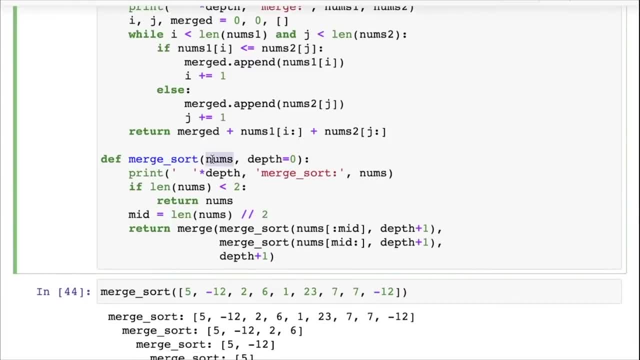 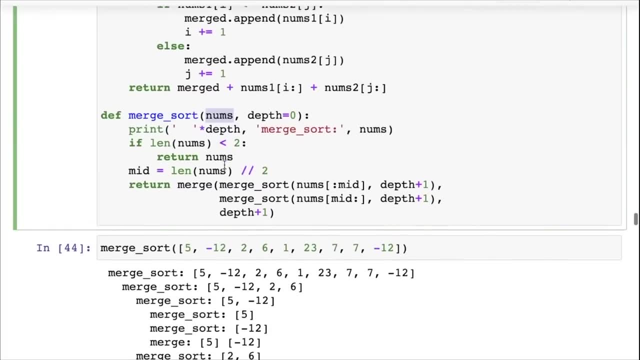 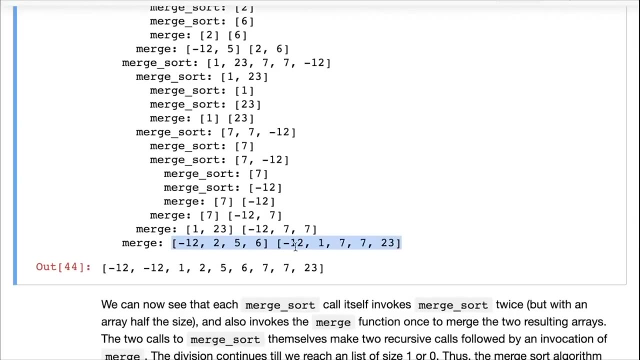 Two is actually the overall length, N. So that's the real trick here: that merge. the merge operation is an order N operation where N is the number of elements, the total number of elements. Okay, So this merge operation takes four plus five, nine comparisons and this merge operation takes five comparisons. 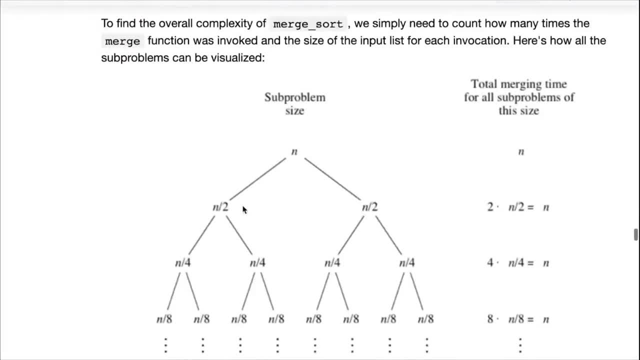 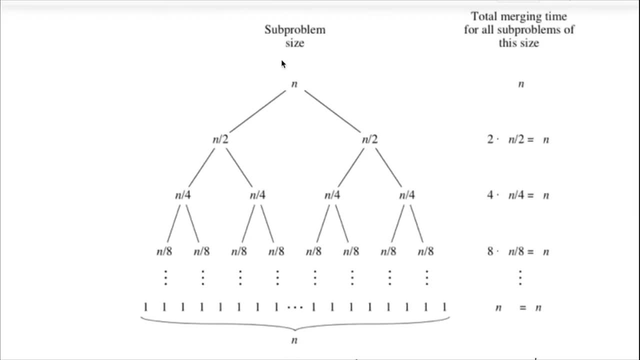 And this merge operation takes three comparisons and so on. Now, this way: Now, if you visualize the Problem now as a tree where we are calling more sort with NL, with N elements and that ends up calling merge sort with N by two elements, 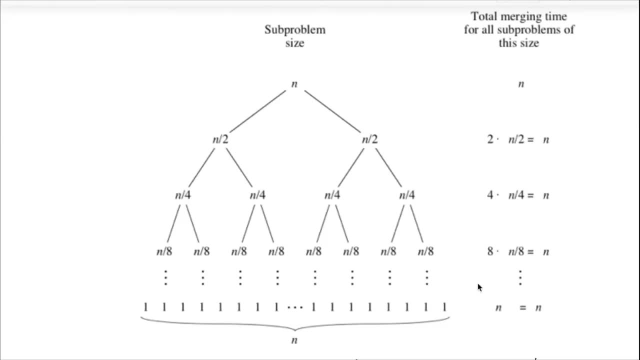 And that ends up calling more sort with N by four elements all the way down And then we start merging. So here, when we get to individual elements, we are calling merge with literally single elements And as we come up here we are calling merge. at this point we are calling merge with elements of size N by eight and N by eight, but we are calling merge eight times. 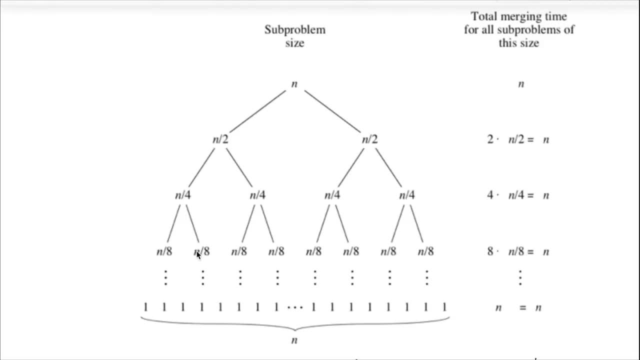 So now each of these sub-problems makes a call to merge and each of these sub-problems has the list size N by eight. So you have eight calls to merge of size N by eight. So the total number of comparisons done is N, and at every stage you can check this at the top level. uh, you are calling merge with N total elements. 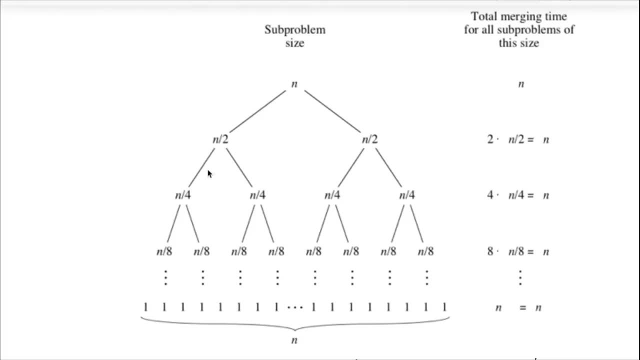 So the total number of comparisons is N. at the second level you're calling merge here once with N by two elements and you're calling merge here once with N by two elements. So the total number of comparisons is two times N by two, that's N. and here you're calling merge with N by four elements, four times. 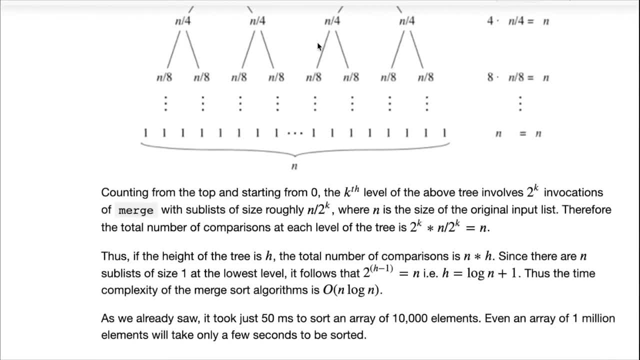 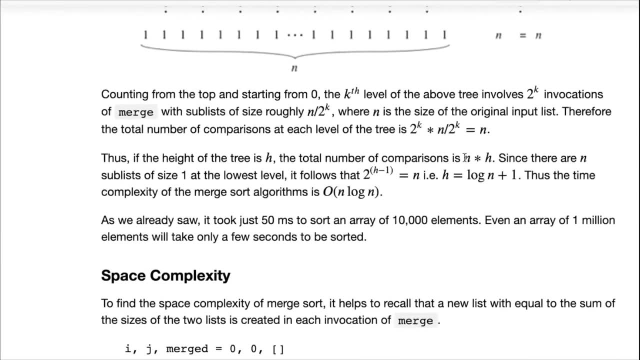 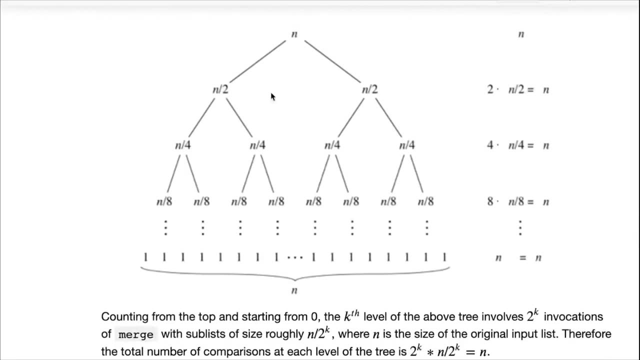 So that's N. So if the height of the tree is edge, then the total number of comparisons is N times edge, right. So on each level you'd require N comparisons for the merge and you call merges at every level for each of these sub-problems. 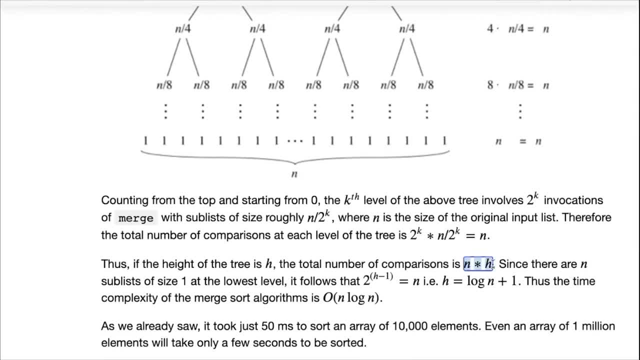 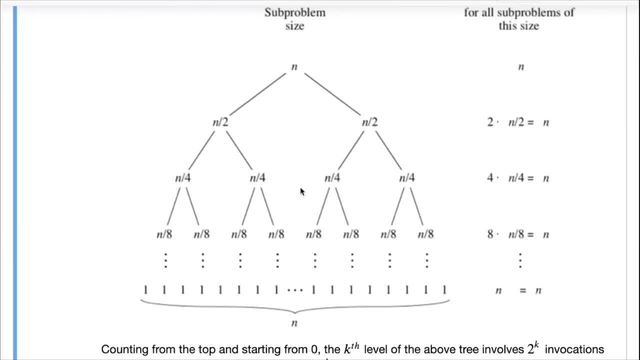 So the height of the tree is so the Okay Total number of comparisons is N times edge. Now how do we get the height of the tree If the height of the tree is edge, and you can see here that as we go down, this is level zero and it has one element. 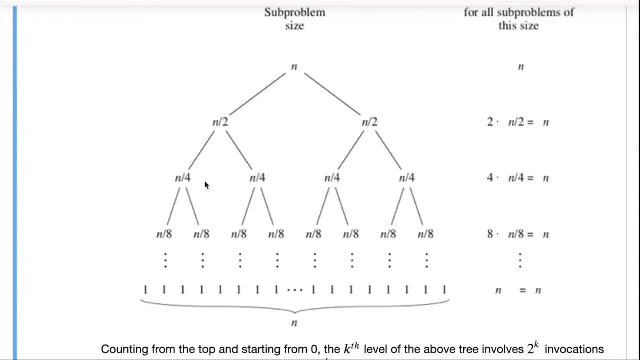 This is level one and it has two elements. This is level two and it has four sub-problems. and this is level three and it has eight sub-problems. So level K has two to the power case of problems. So if you keep going down, this is level H minus one. 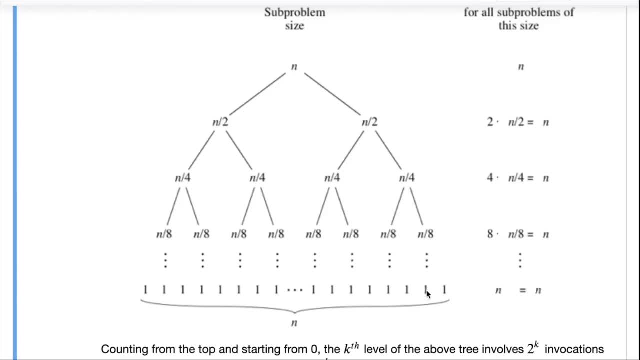 So level H minus one should have two to the H minus one sub-problems. But remember, at the last level we simply, we simply have sub-problems or merge, merge calls with single elements. So that means we have a total of N elements here or N leaf nodes here. 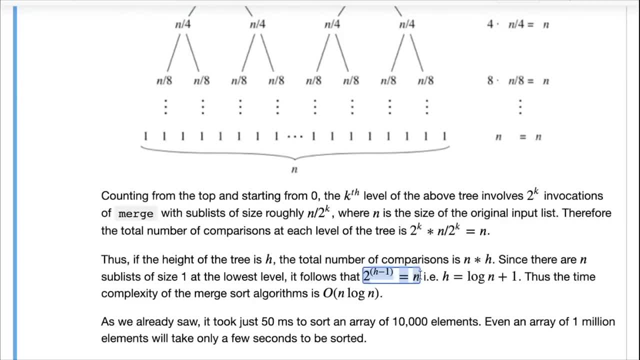 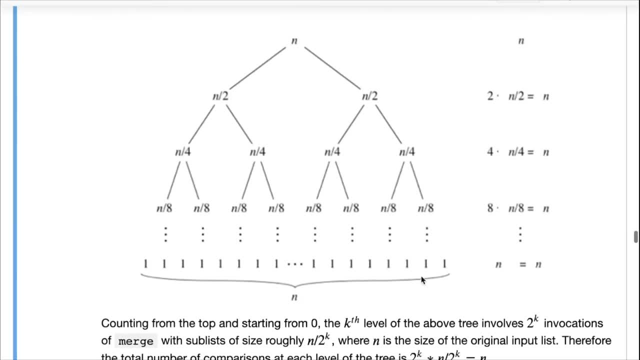 So it follows that two to the power of H minus one is N. Okay, So I'll I'll let you think about that and reason with that. This is something that you may have to work out on pen and paper to get correctly. 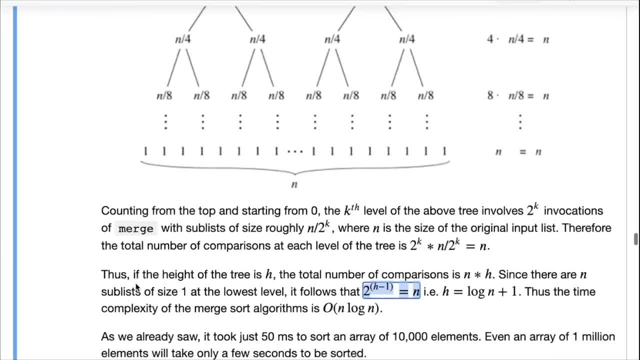 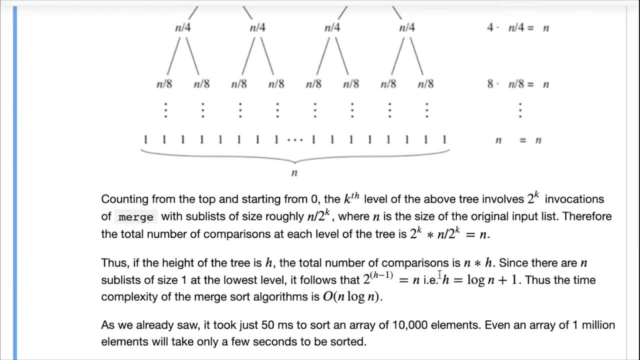 That if the height of the tree is edge, then two to the power, H minus one, is equal to N, because at the bottom most layer you have N leaves in the tree. So it follows that edge is log N plus one. So, since we said that there are N times edge comparisons and H is log N plus one, 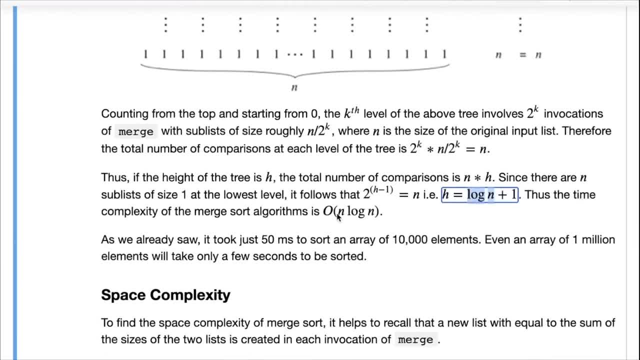 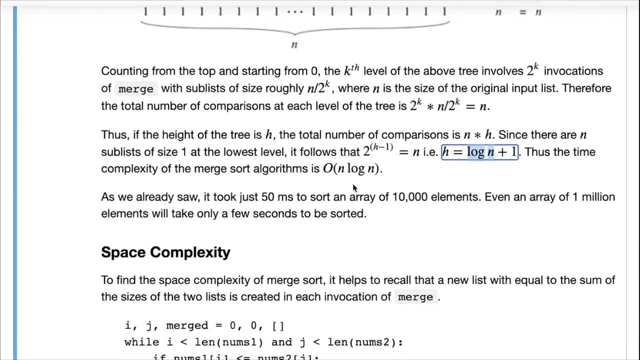 So it follows that the complexity of merge sort is N log N and that's a big improvement from N square. It may not seem like much But it is so. N square for 10,000 is 10,000 times 10,000, but N log N for 10,000 is 10,000 times 12 or 13. log to the base two. 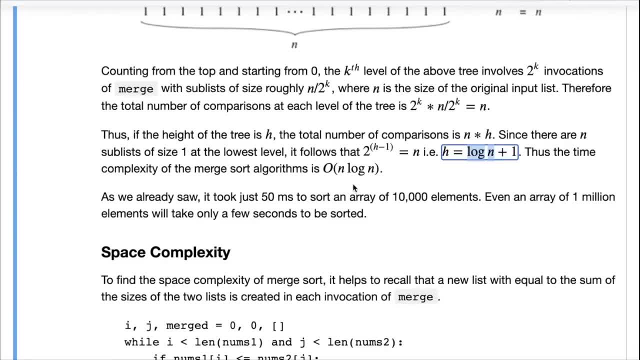 So that's about a few hundred times faster. Now, even for an area of a million elements, it will only take a few seconds to be sorted, and you can verify this by actually creating a list of a million elements. Okay, So the complexity of merge sort is N log N. 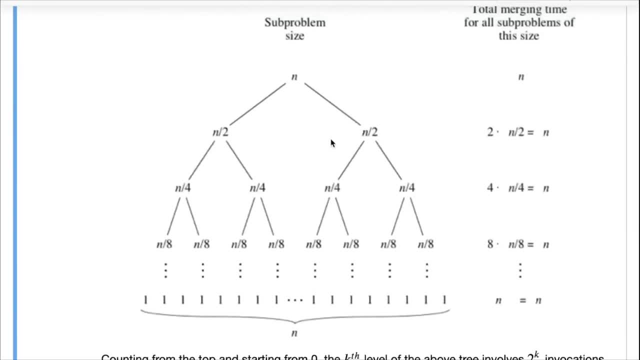 Okay, So the complexity of merge sort is N log N, and you get it by drawing this sub problem tree and realizing that there are. you get a sub problem tree of height, log N or log N plus one, and at each step you perform a merge operation or multiple merge operations totaling to N comparisons. 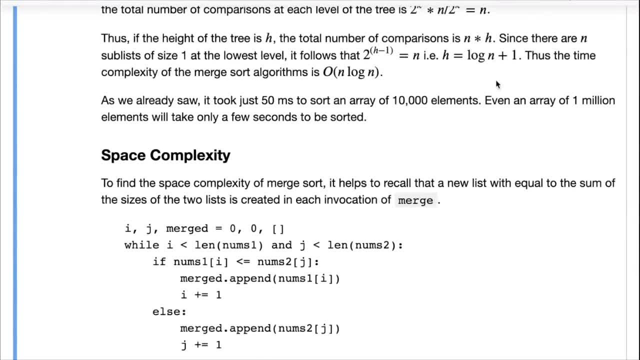 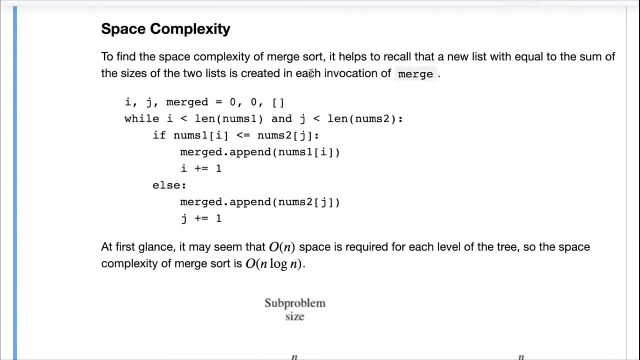 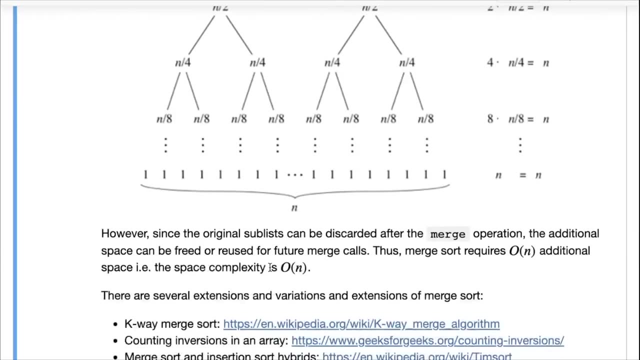 So so N times. log N is the complexity of merge sort. Now here's also a discussion about space complexity, and this is something that I will leave as an exercise for you. So do read through this and see you can reason why the space complexity of merge sort is order N: okay, 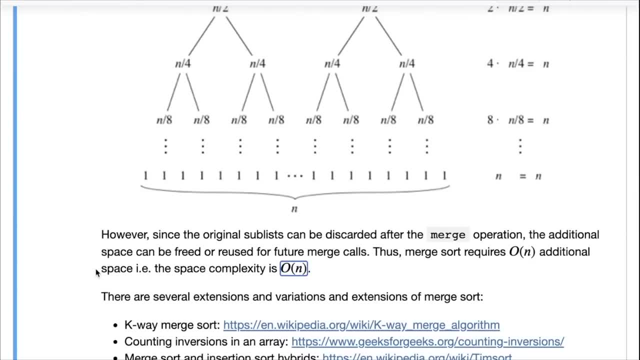 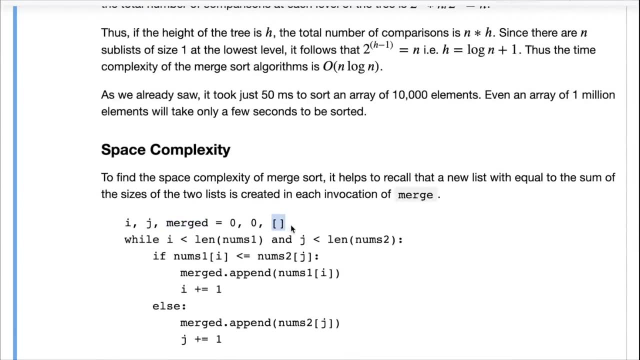 So time complexity is order N, log N and the space complexity is order N. but here's a hint why it's order N. You can see that inside the merge operation we are creating a new list and then we are copying over elements from each of the two lists into the new lists. 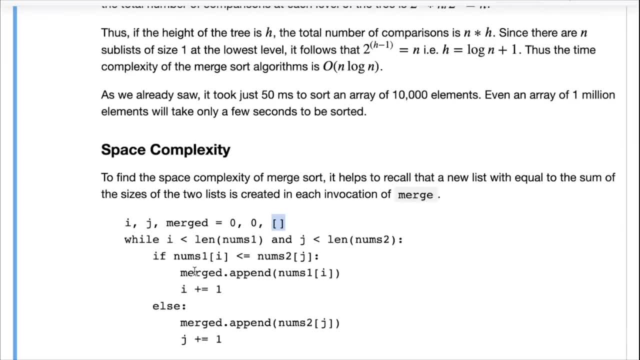 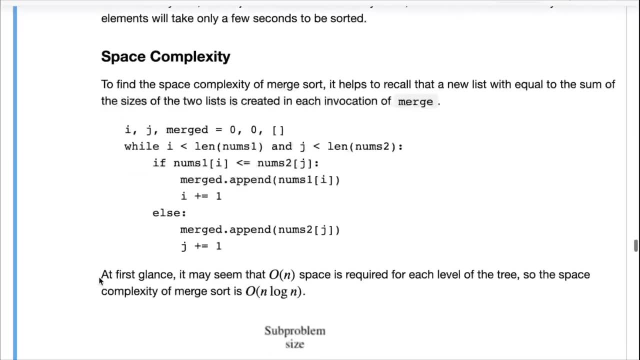 So we are allocating a new list inside merge, And now it's so. now that's no longer constant. That list will have the same size as the size of the problem itself, And hence roughly. that's why the space complexity is order N. 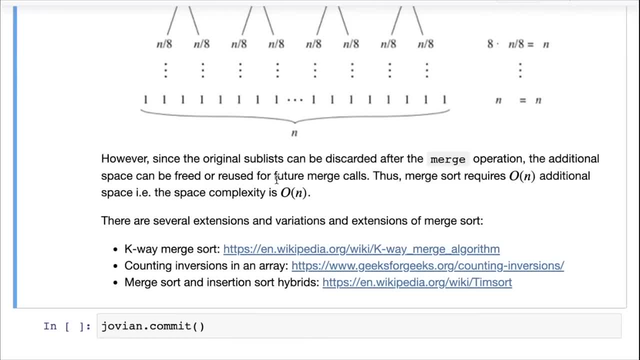 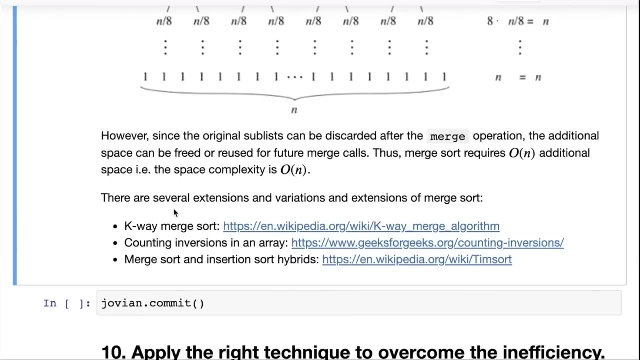 Okay, So with that we conclude our discussion of merge sort. It's a divide and conquer algorithm. You split the list into half recursively, sort both of them, then merge the two sorted lists and the initial condition is one or zero elements. Now there are several extensions and variations of merge sort. 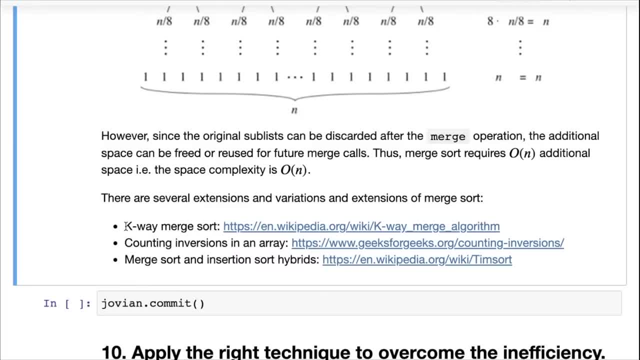 Good The cave. So let's say merge sort, where we split not into two parts but into K parts. then we have the counting inversions problem where we modify, merge, sort a little bit to also find some other info, information about the list. 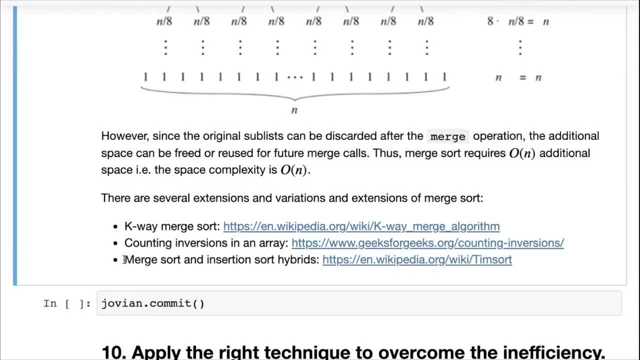 And finally, we have hybrid algorithms which combine merge sort and insertion sort. So what they do is, for smaller lists, they use insertion sort because that's more efficient, And then for bigger lists, they use merge sort, So as they're splitting the list when you get to a small, 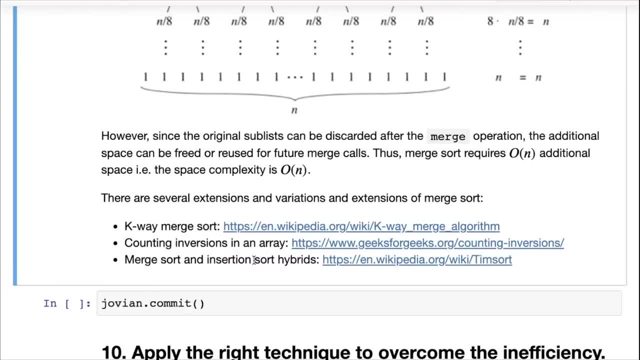 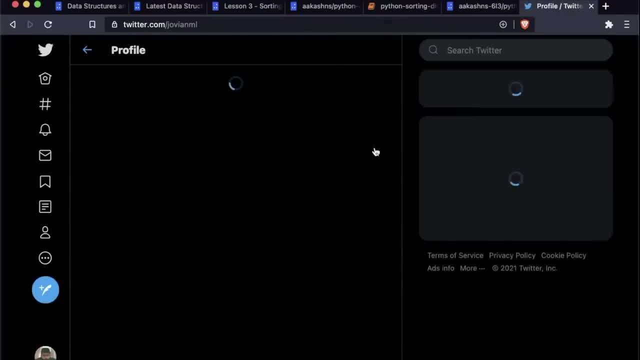 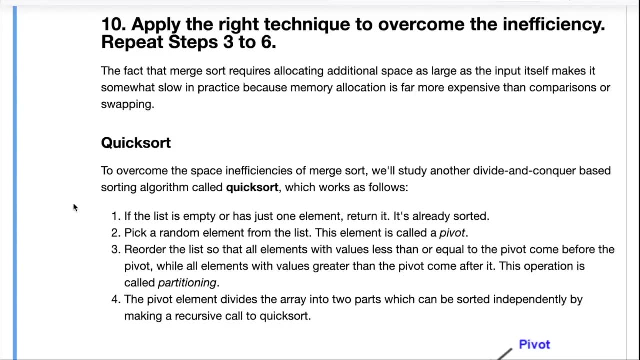 Problem, let's say, 10 or less elements. they use insertion sort. And that brings us to our next question, where we make one level of optimization and then we stop. but here we'll go one step further. What we'll do is we will apply an another technique to overcome the inefficiency in merge sort. 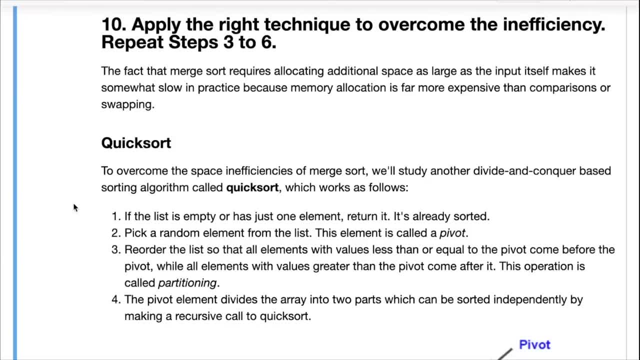 Now the time, complexity is pretty good. You can actually sort millions or even tens of millions of elements With Merge sort quite reliably. but it's a space complexity that causes a problem now, because merge sort requires allocating additional space, and that is additional spaces as large as the input itself. that makes it somewhat slow in practice because memory allocation is more expensive than computations. 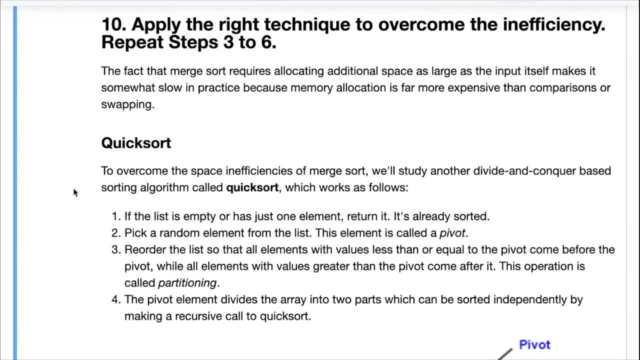 So doing a comparison is very easy. You just tell the CPU to compare two things in the memory. or swapping them is also easy, because you're still working with memory that you already have. But when you have To allocate new memory you often have to then request the operating system to allocate the new memory and then you have to get its address and do a whole bunch of operations. 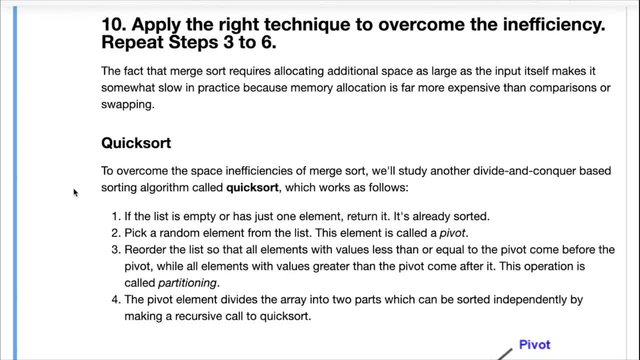 So it's, let's say, an order of magnitude more expensive than simply doing some computations. So you should try and avoid memory allocations as far as possible. Now, one or two variables is fine, but if you're dealing with a million elements, so you're probably going to need maybe a few MB of additional space. 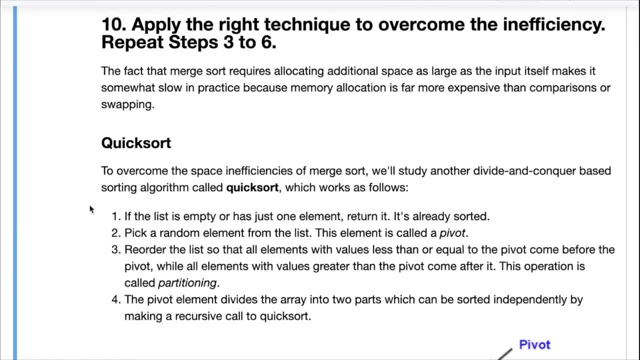 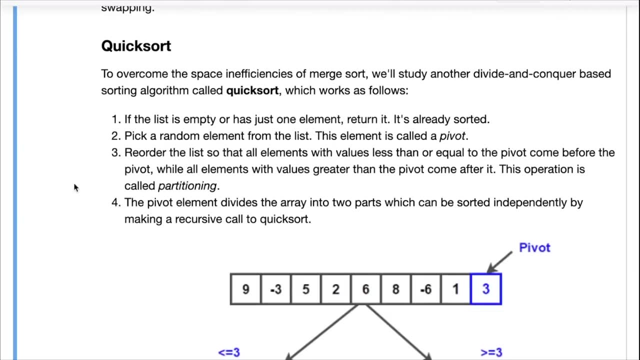 And that is what may slow down Your algorithm a little bit. it would still be N log N, but the constant factor. Now the cost of each operation will be higher because it involves an allocation. Now, to overcome the inefficiencies, the space and efficiency of Merck, Merck sort, we will study another divide and conquer based algorithm, sorting algorithm. 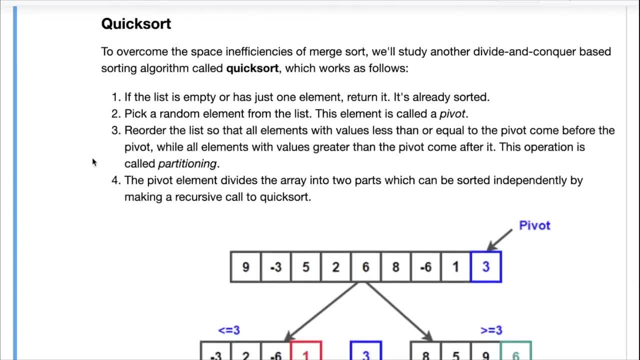 And this is called quick sort, and quick sort sorts the area in place, which means it does not create a copy of the area Internally For sorting inside each operation, inside each combination operation. So let's see how it works. It's a pretty interesting, a pretty smart trick. 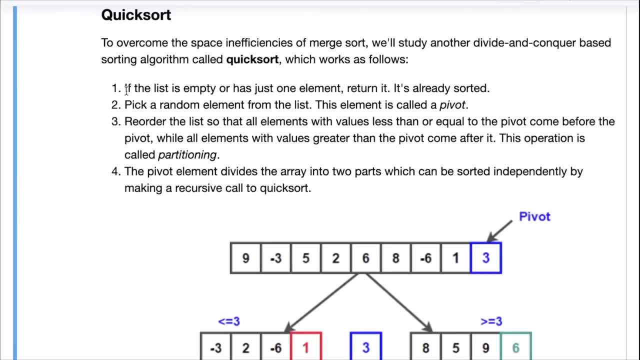 So here's how it works: If the list is empty or has just one element, return it. It's already sorted straight forward. then pick a random element. If not, pick a random element from the list. Now this element is called a pivot. 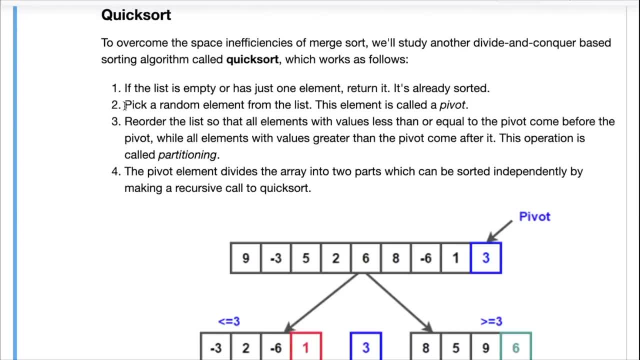 Now, there are many strategies for picking a pivot. One is to pick a random element. One is to maybe pick the first element, the last element. What we'll do is we will pick the last element, but you can easily augment our implementation to pick a random element. 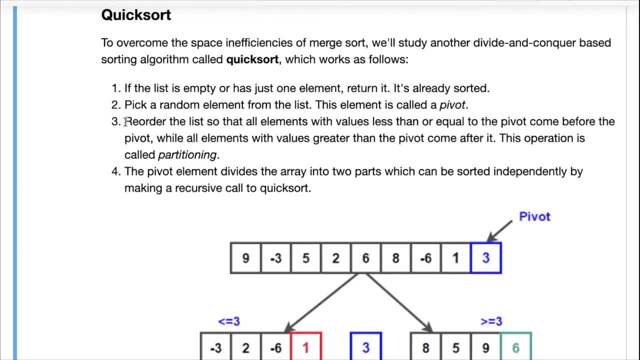 And then reorder the list. And this is the key operation here: Reorder the list so that all the elements with values less than or equal to the pivot come before the pivot element, while all the elements with values greater than the pivot come after the pivot element. 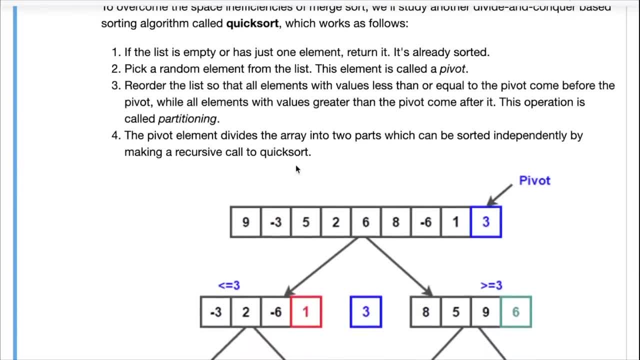 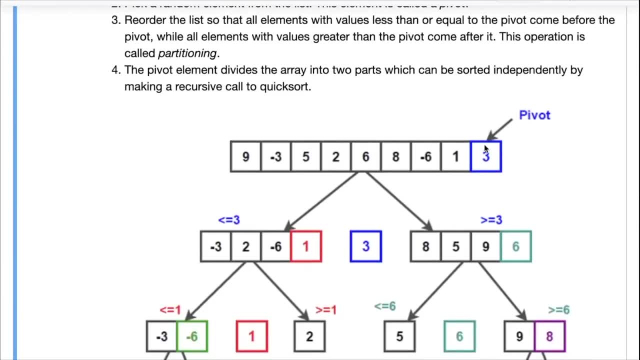 And this element is called partitioning, your partitioning The array around the pivot. So here's an example: You, let's say we take three as the pivot element, the final element. Now, what we want to do is we want to reorder the elements and the way we reorder this, by doing swapping and comparison, in whatever way we can. 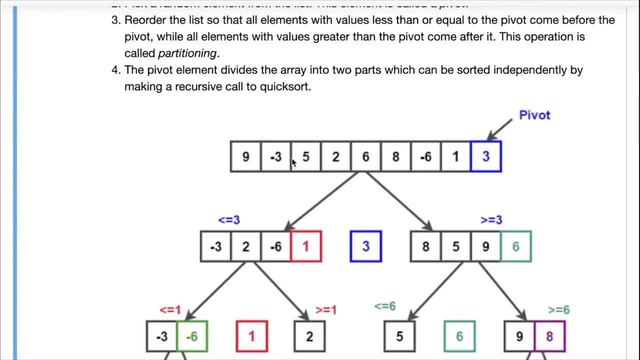 And that's what we will really focus on: the partitioning algorithm, and you reorder it in such a way that all the numbers to the left of the pivot are smaller than it and all the numbers to the right of the pivot are larger than it. 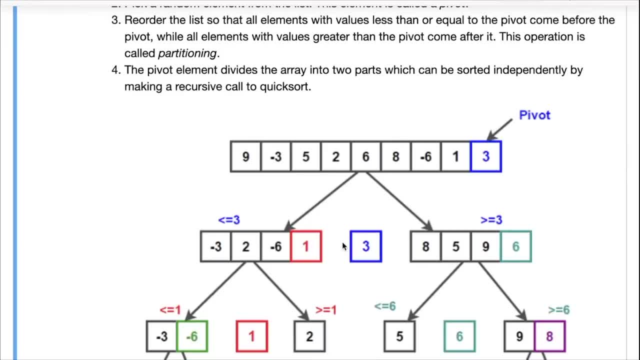 Now here's the key observation here: Once you do that, you can tell that all these, all these numbers can now be sorted independently and none of the numbers from here will move to the right of pivot. And similarly, all these numbers can also be sorted independently and none of the numbers here will move to the left of the pivot. 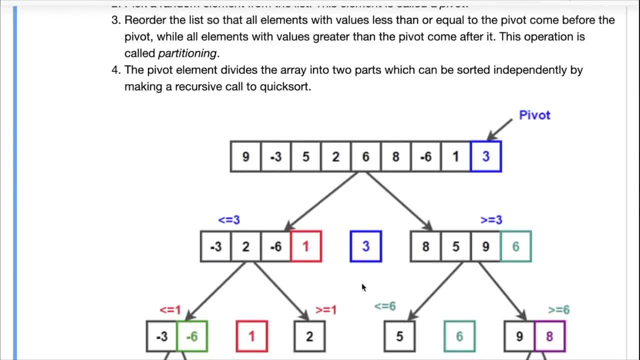 So the pivot is in the correct position in the final sorted area. So it's now in its correct final position And you can simply call quicksort on this half or less, Less than half this portion of the area and this portion of the area. 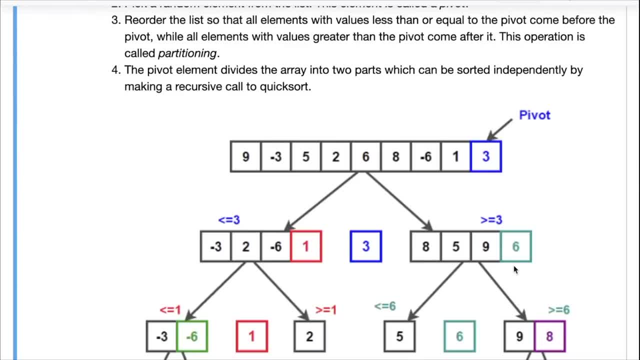 And there's no real combination required anymore, right? So, because we're doing it all in place, we simply call quicksort on each side of the area And once this gets sorted, and this gets sorted recursively, then you will end up with the entire sorted list, right? 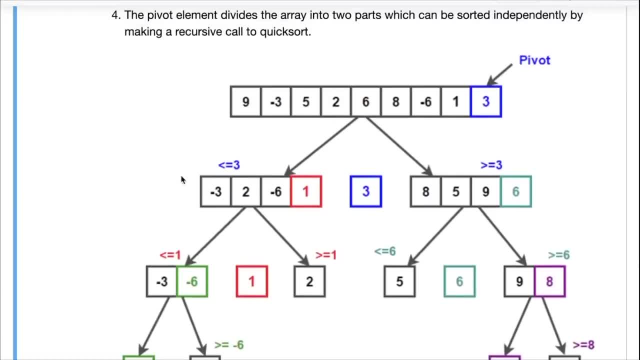 And that's that's how we then continue doing the process recursively. Now, on the left half, you once again pick a pivot and then you are easy elements around the pivot. on the right half, You once again pick a pivot and arrange the. 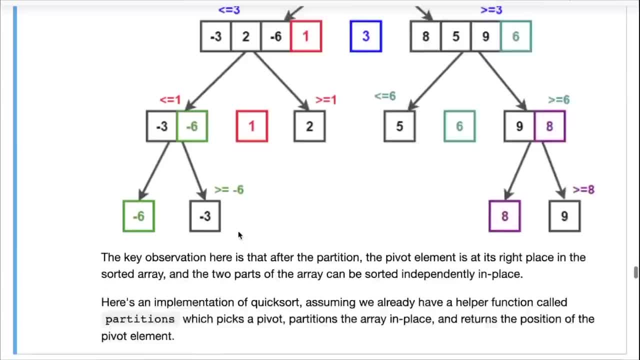 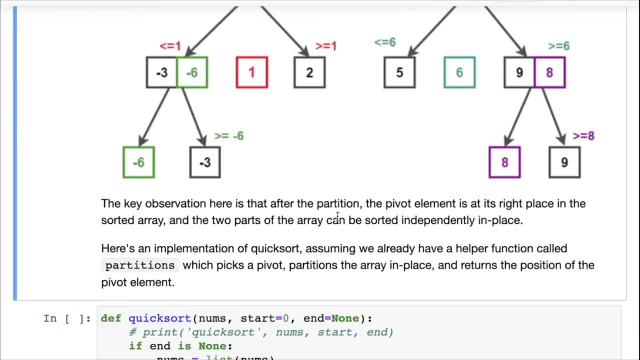 Elements around the pivot and so on and so on. Okay, So, as he said, the key observation here is that after the partition, the pivot element is at its right place in the sorted area. The two parts of the area can be sorted independently in place. 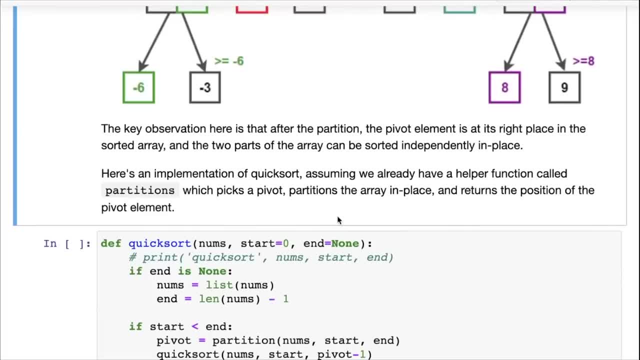 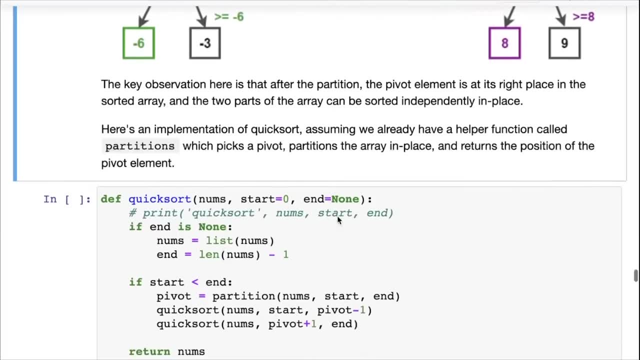 Now maybe once again take pen and paper and try to work it out yourself Again. all of this makes a lot more sense when you actually put it down and solve a real problem as a real example. So here's an implementation of quicksort. 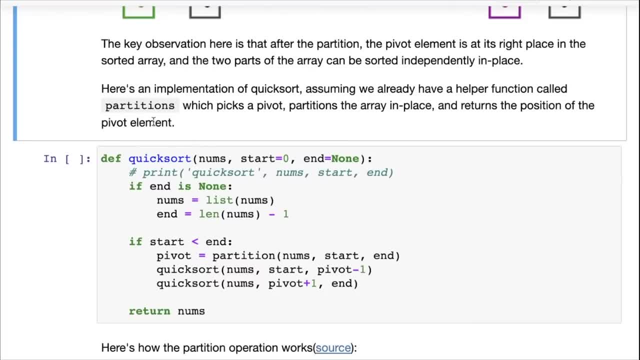 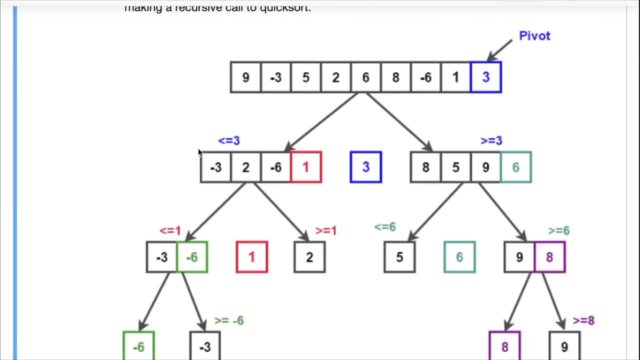 And, once again, we will assume that we already have a helper function called partition which can pick a pivot partition, the area, and return the position of the pivot element for the next quicksort step. Okay, So this entire process going from here to here. this is where we'll assume that we have a function and write the quicksort. 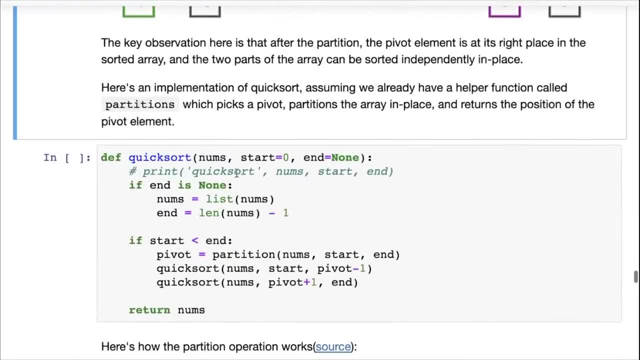 algorithm and then implement the partition function. So here's what quicksort might look like. now. quicksort takes a bunch of numbers and apart from the numbers, it also takes a start Index and an end index. Now why are we doing this? 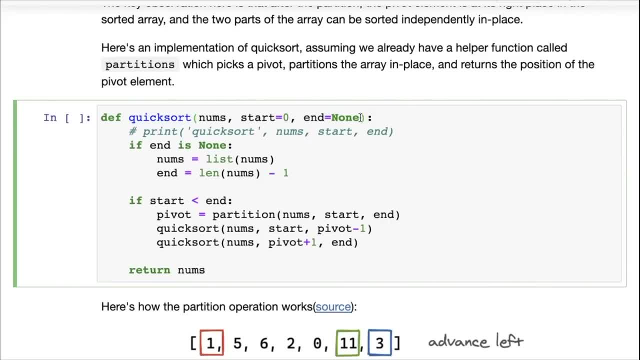 Remember, we want to avoid creating copies of the list. That's the whole pro, that's the whole thinking here, the line of thinking. So we will call quicksort not with a sub list, which is which is a copy of a portion, but we will call quicksort simply by. 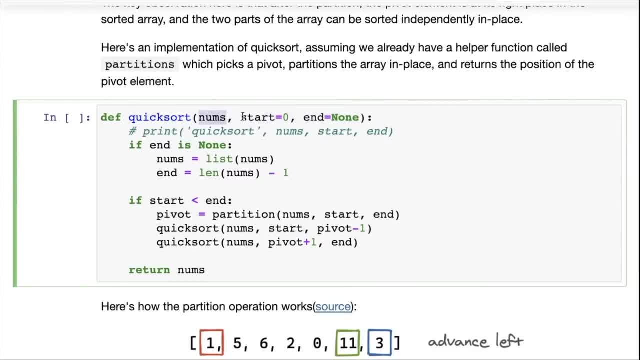 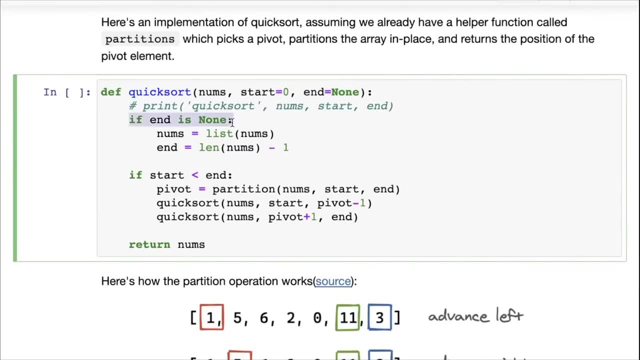 changing the bypassing the same original list, but by changing the start and end index. Okay, Now there is some code here: If end is none, Then we are setting end to the length of the list minus one. And here's one more thing that we're doing. 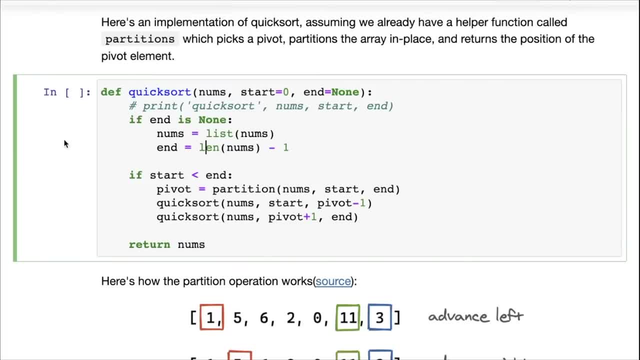 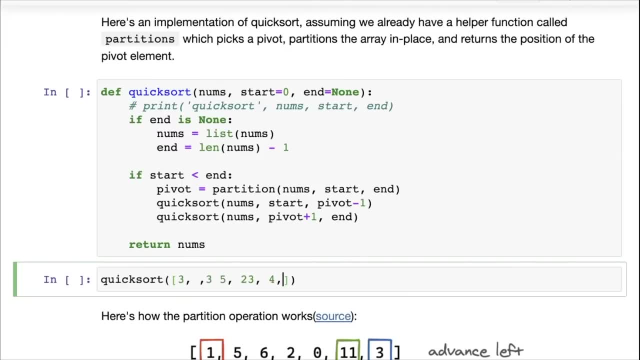 So the final invocation to quicksort that we'll make will be something like this: We may call quicksort- Let's say there are a few numbers here, So we may call quicksort on a list, something like this- And in this case, automatically start will have the value zero and end will have the value none. 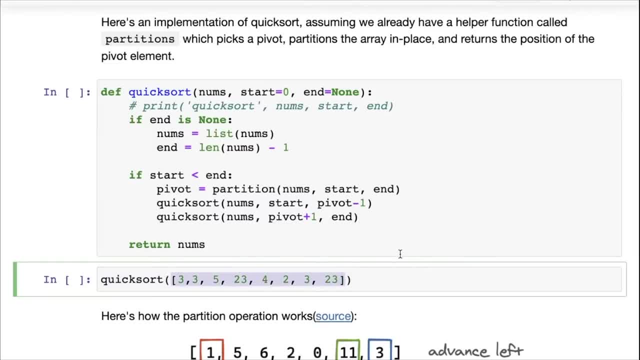 Now, Remember, the quicksort is going to sort the array in place, but we also said that we don't want to modify our test cases. So here's one assumption we are making: that if end is none, which means if quicksort is called just with the, just with the list, then we'll create a copy of the list, right? 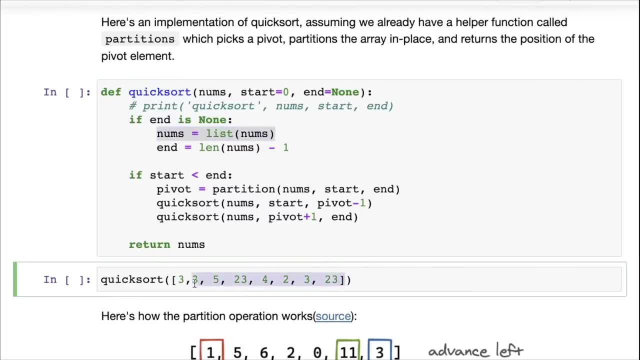 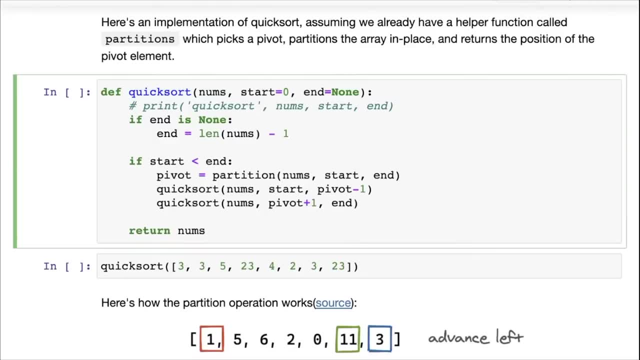 So we'll just create one copy at the very beginning, right When the list is passed for the first time, and then we'll not create any more copies, and you can even skip this line entirely. But the only trouble is that we'll start changing our test case input. 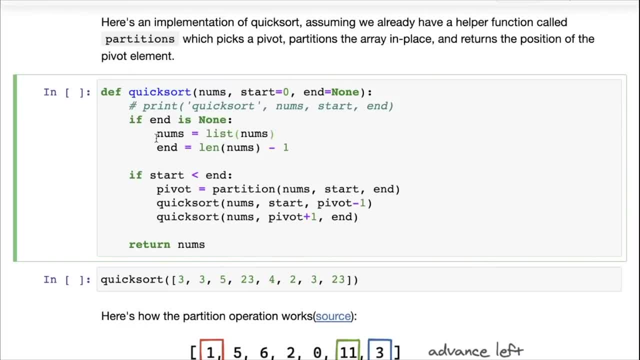 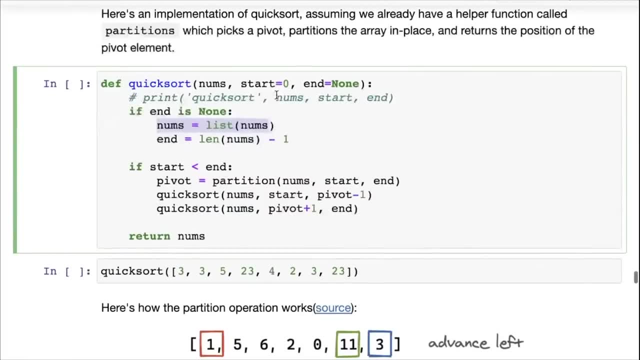 So that's why Let's keep it and let's keep a copy, but this is only done at the very top level, right? So only when we start we create a copy so that we are not modifying the input list, but never again. 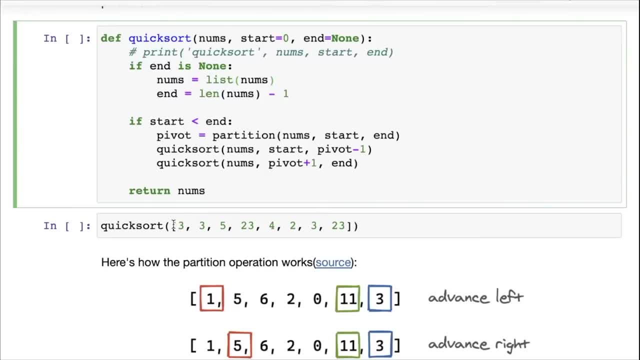 So that's what we're doing here: Creating a copy If a quicksort was called with a list and setting end to len nums minus one, which is the final valid index in the list. Anyway, putting this aside, this is the real condition here. 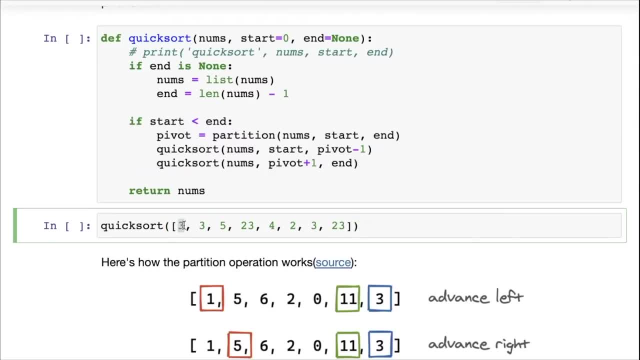 So if start is less than end, which means Let's say, here you have start and here you have. and now if start is less than end, that means you have two or more elements. right? If start and end are equal, that means you have just one element. 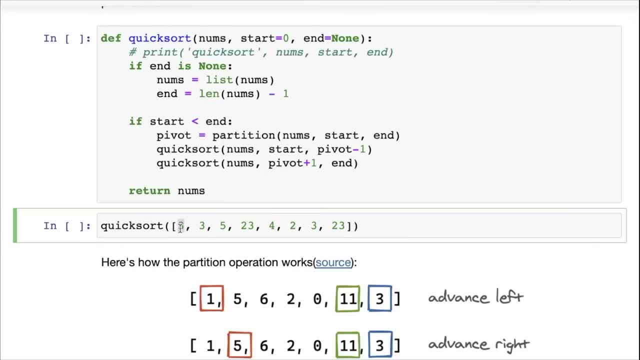 And if start is greater than end, that means you have zero elements really. So if start is less than end, that means if you have at least two elements, then we call the partition function, We call the partition function on nums and we say that we want to partition the region start to end. 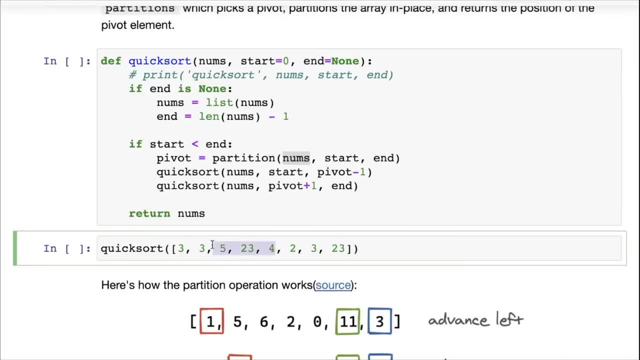 So let's say this is the region, start to end. We want to Partition it. So we want to pick a pivot and then partition it in such a way that elements to the left of the pivot are smaller than it And elements to the right of the pivot are larger than it. 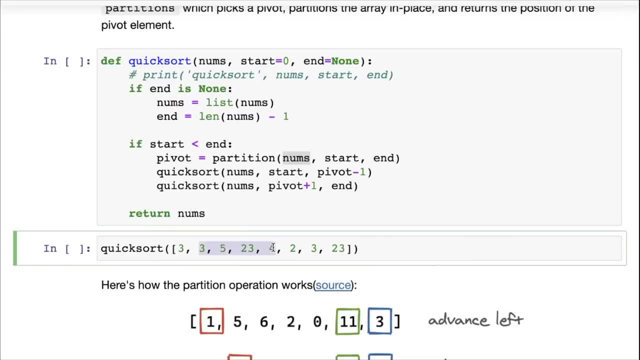 For example, if you want four to be the partition element, for it to be the pivot element, then we will partition the area as three comma four, comma five comma 23.. So that three is smaller than four and five, 23 are bigger than four, and we will return the position of the pivot element. 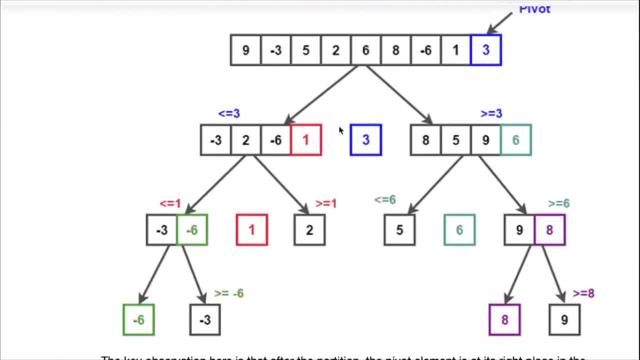 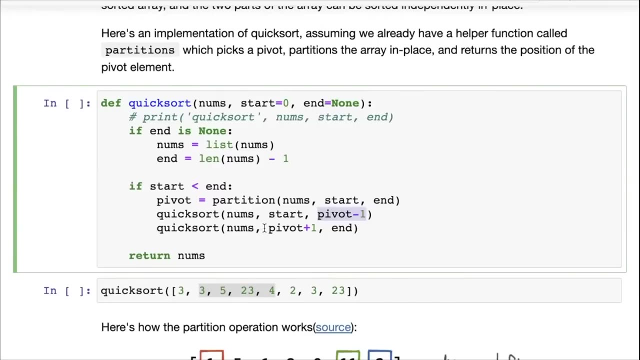 Okay, So now You partition the area and return the position of the pivot element. So this is the position we get back and then we can call quicksort on this region and on this region. So we can now call it quicksort on start to pivot minus one and we can call quicksort on pivot plus one to end. 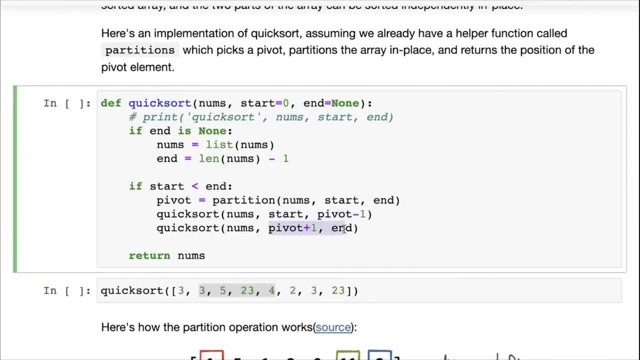 Okay, So now we are passing- actually explicitly passing in values for start and end, So this will not kick in the next time. So no more copies of the list will be created. So all the recursive calls will keep More Modifying in place. 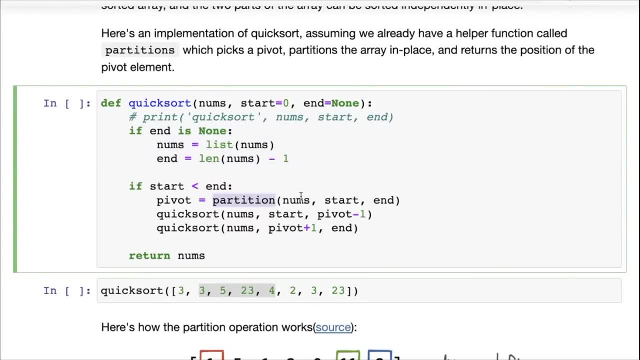 So all the recursive, even the partition call, will modify in place and we'll see how partition works in just a moment. So partition gets the slice of the original list and it returns the position of the pivot element. Then we call quicksort on the left slice, which is before the partition, the elements smaller than the partition. 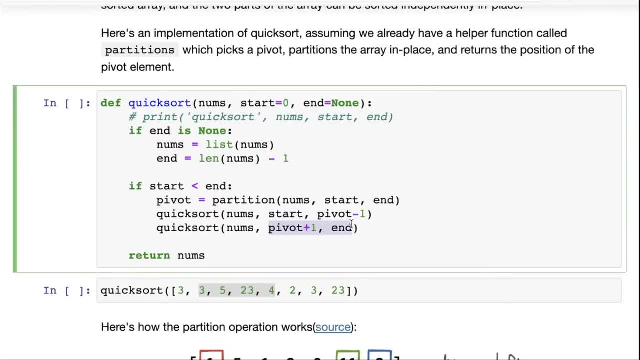 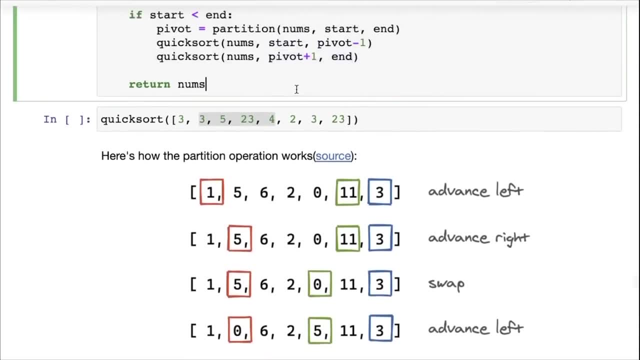 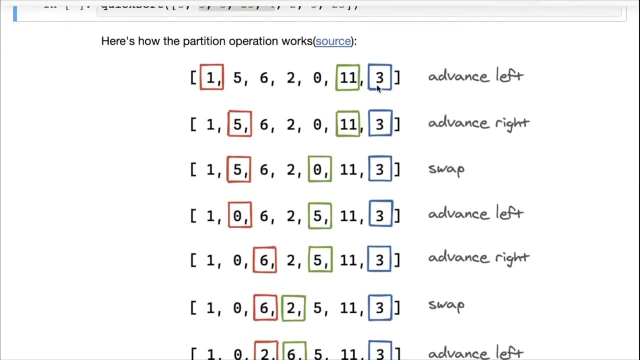 And then we call quicksort on the right slice, which is elements that come after the partition. Okay, Now here is how the partition operation works. It's pretty straight forward to not that difficult. So what we'll do is we will pick the final element as the pivot element. 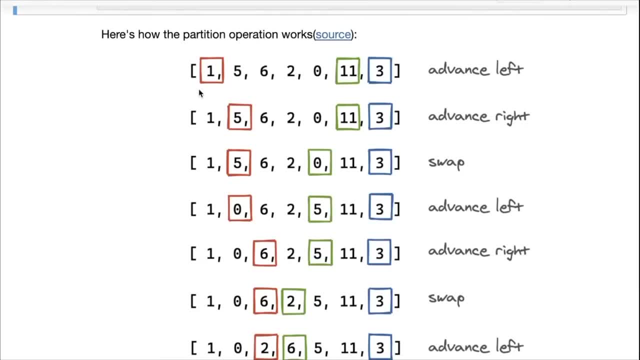 But if you don't want to pick the final element, you want to pick a randomized element? Well, just pick a random position and move that element to the final position, And that's as good as picking the final element now. So random pivot simply involves picking an element, moving it to the final position, but assuming the pivot is in the final position. 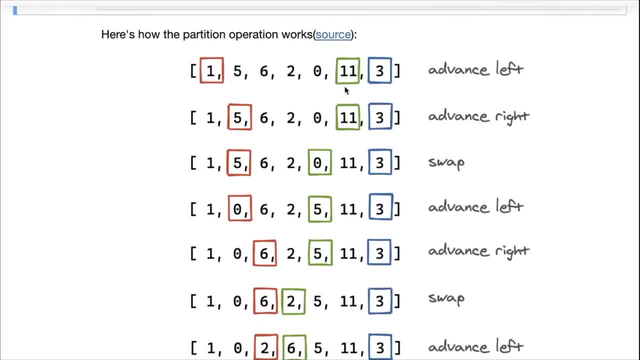 We then Keep two pointers, left and right. Now remember we want to create: we want to push all the numbers smaller than the pivot to the left and we want to push all the numbers larger than the pivot to the right. Okay, 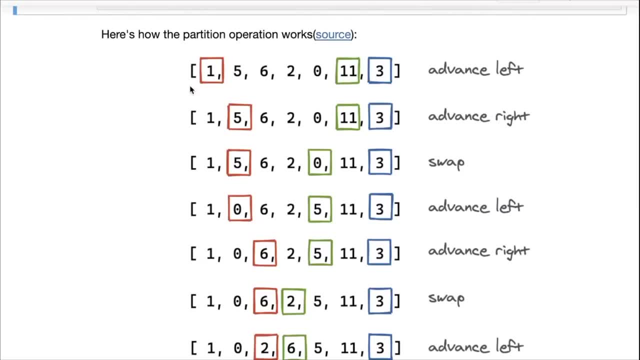 And what we'll do ultimately is we will arrange them in such a way that some of these are smaller than the pivot And some of these are larger than the pivot, and then we'll move the pivot between them. So we'll see how to do that. 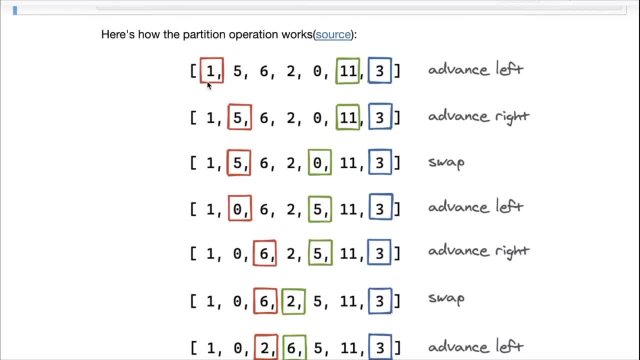 So you have the left pointer and the right pointer. Now here's what we do Inside partition, while these two pointers are far away from each other. First we check if the element at the left pointer is smaller than the pivot. Well, if the element at the left point is smaller than the pivot, which it is, you simply advanced the left pointer forward. 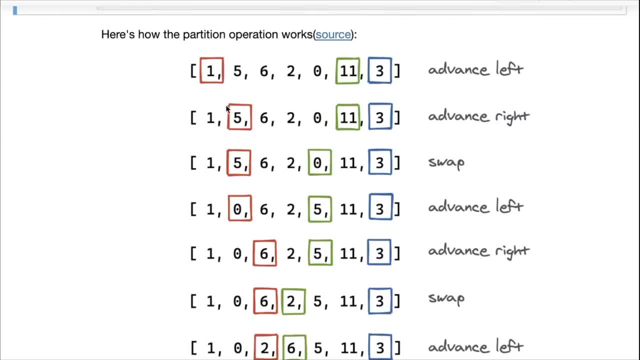 So this goes to five, and then we go back to the next loop. Now, this time, once again, we check if the element that the left pointer points to is smaller than the pivot. Five is not smaller than three. five is greater than three. 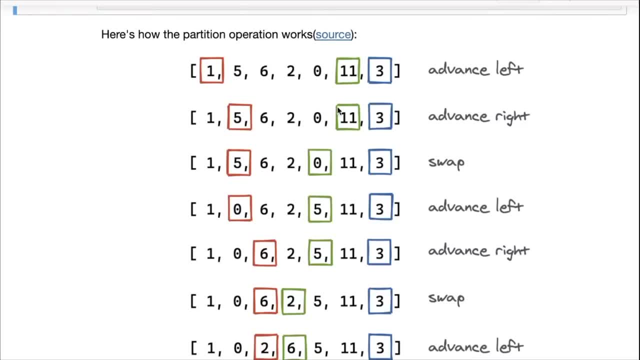 So if that is the case, then we check if the right pointer is greater than the pivot. Now, if the right pointer is greater than the pivot, that means this number is in its right position. It's greater than the pivot. So we move the right pointer back one space. 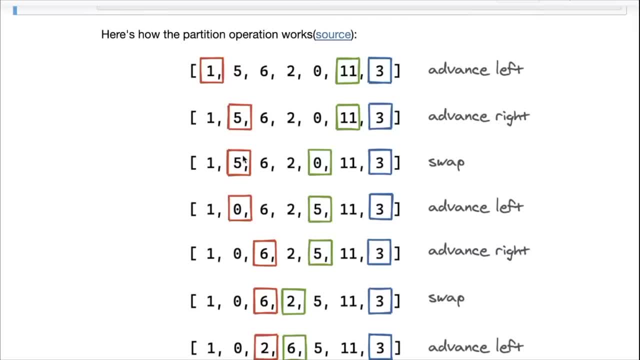 Okay, So that's the operation we just did. Now once again we check: is the left pointer smaller than the pivot? No, it's not. Is the right pointer Greater than a pivot? No, it's not. So that means these two numbers are out of place, right. 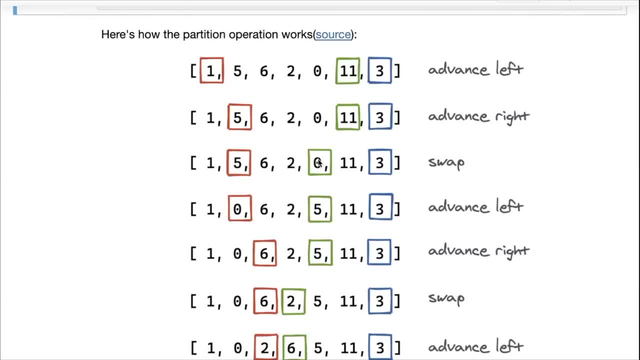 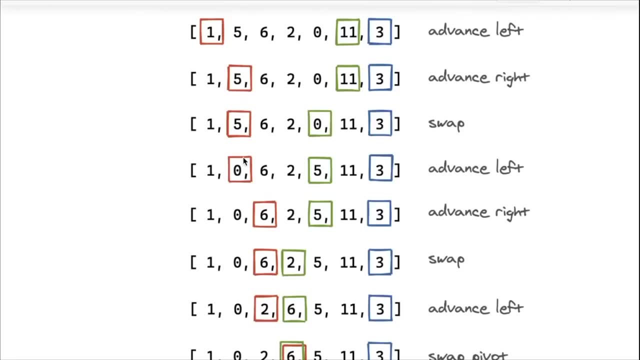 We ideally would want this to be smaller than the pivot and this to be larger than the pivot, So we swap these two elements. So now zero comes here and five comes here. Now once again we can check, is zero, The left pointer, smaller than the pivot? 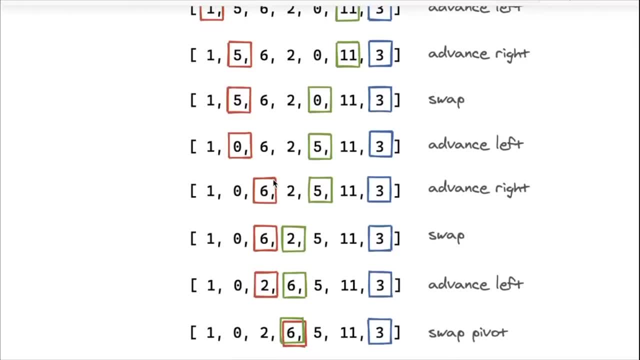 Yes, So move the left pointer forward. Then we is the left pointer smaller than the pivot. No six is now greater than three. So we check: is the right pointer larger than the pivot? Yes, So we move the right pointer forward, because five is still in its correct position. 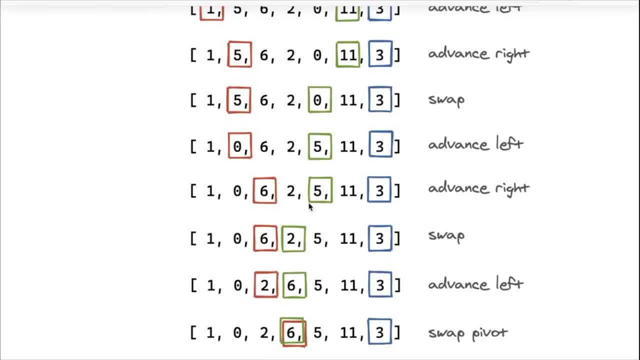 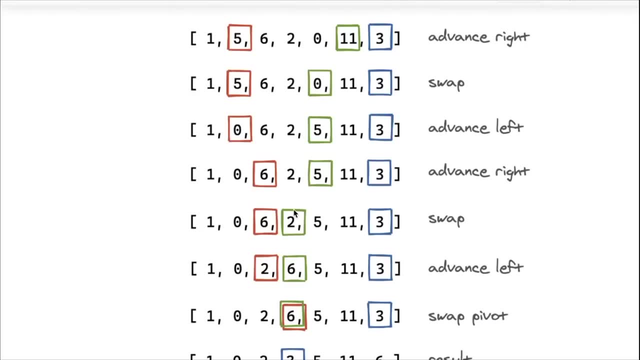 It's on the right edge and everything is greater than three. So now, once again, we ended up in this position: that the left element is smaller than the is larger than the pivot. So we check the right element. The right element is smaller than the pivot. 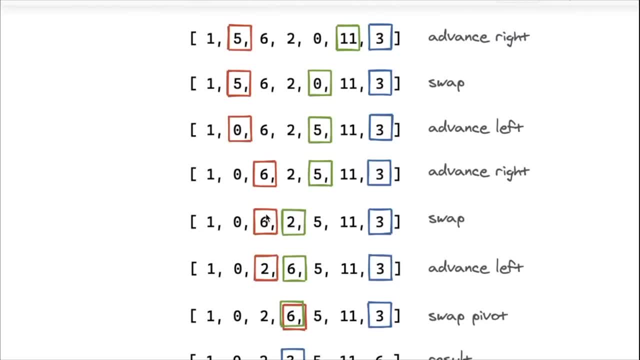 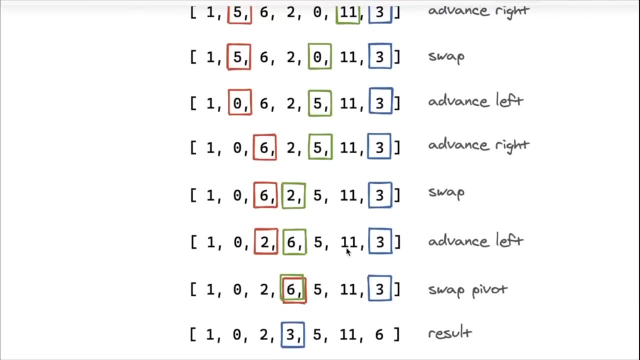 We want it to be larger, So we swap these two, because these two are once again out of order. And now you can see that one zero two are all smaller than the pivot and six, five, 11 are all larger than the pivot. 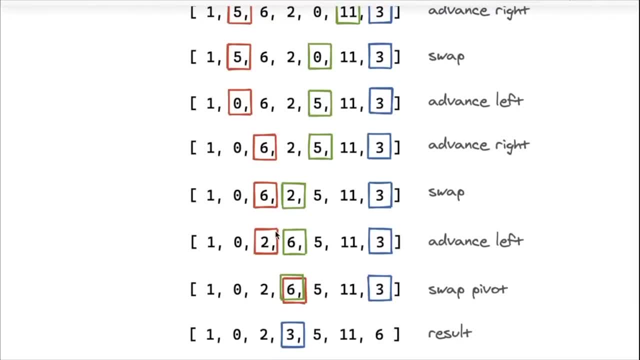 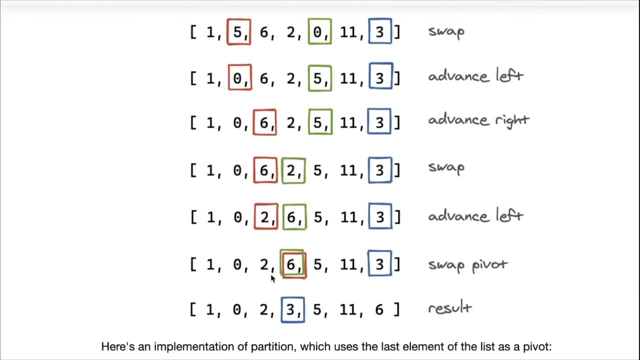 So we do one final check: is two smaller than the pivot? Yes, So we advance the left pointer, and now both of the pointers are at the same position. So now we can tell at this point that here, or from this point, position onwards, all of these 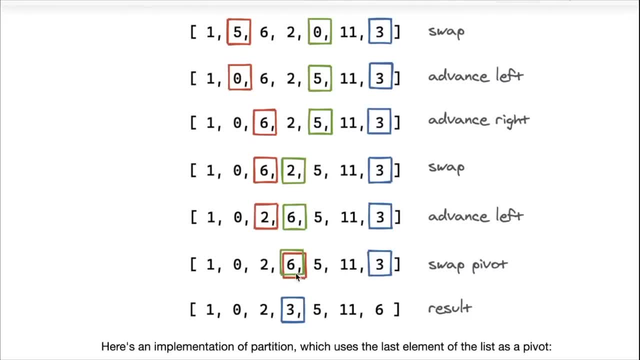 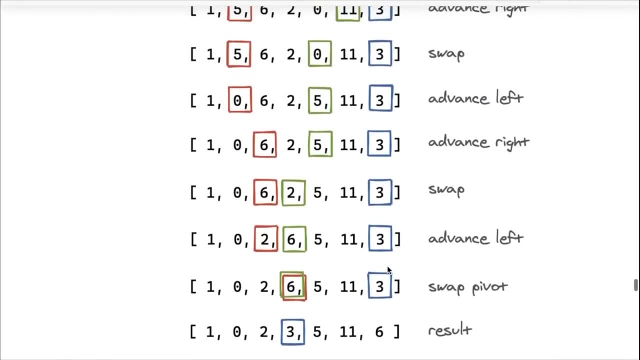 numbers are larger than the pivot, So we simply, simply swap this element with the pivot. So there you go. So you end up with one, zero, two, three, five, 11, and six. Okay, So that's the partition operation. 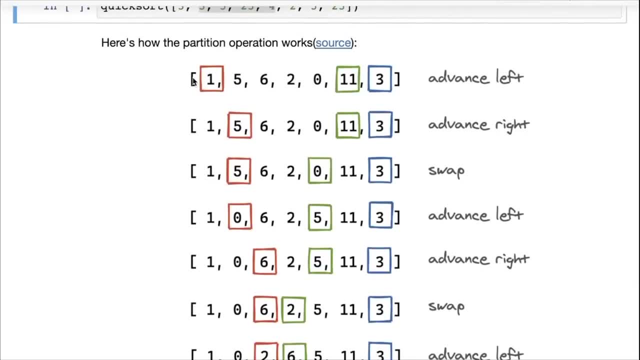 So again, to understand it yourself, do it on pen and paper, write out, write out, write out this array: create the pivot, create the left pointer, right pointer, and keep creating copies of the area for each step of the loop. 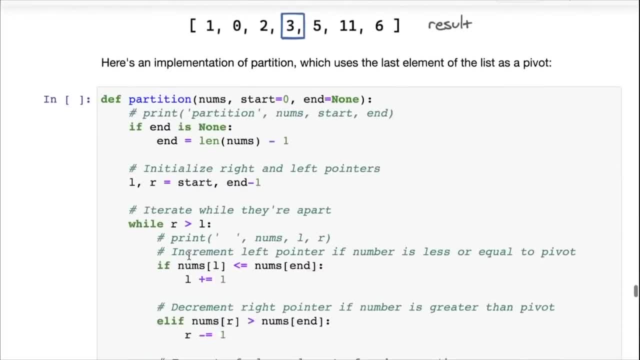 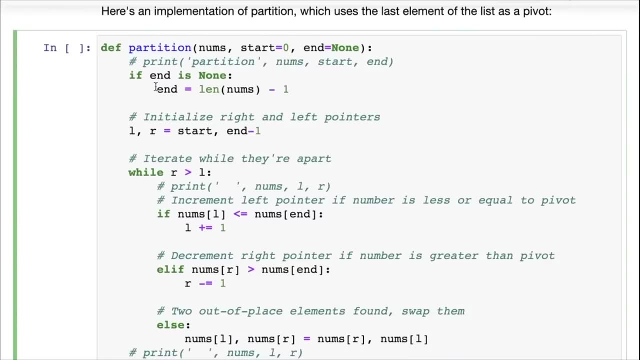 Okay, And that's how you understand these things. It's not that difficult, It's just it involves two pointers, So it's a little tricky. Now, this is the code for partition, and I will let you follow this code. 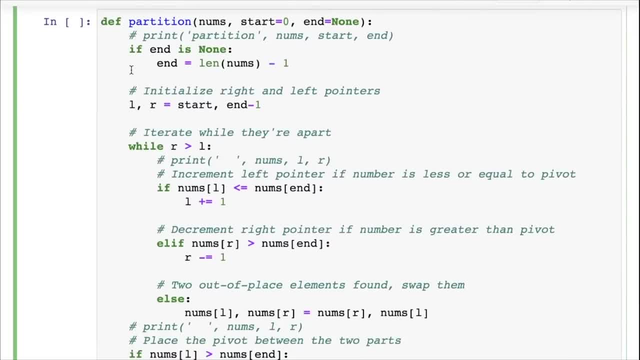 We'll go over this briefly, but by this point, since we are halfway into the course now you should be able to read the code- And then there are also comments here- and understand what we've just discussed in plain English. Understand that in terms of code. 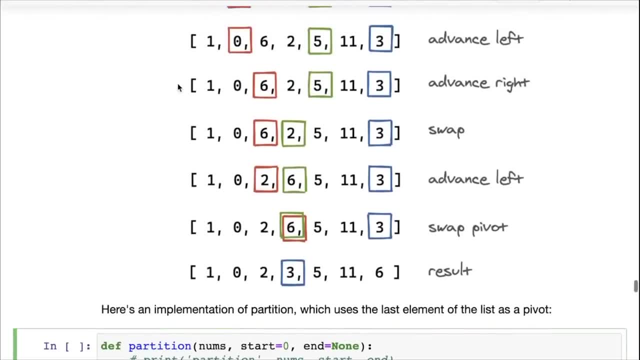 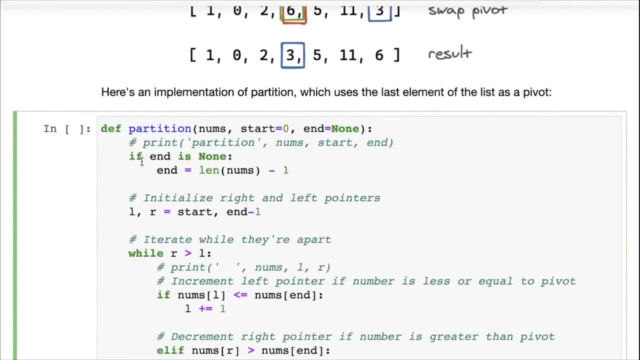 Okay, So one exercise for you is to explain this visual approach in plain English, step by step, And then the second exercise for you is to read the code and understand it, or maybe even try to write it from Memory. So just take the English description and try to write the partition function from your memory. not memorize the code itself, but convert the English text into code. 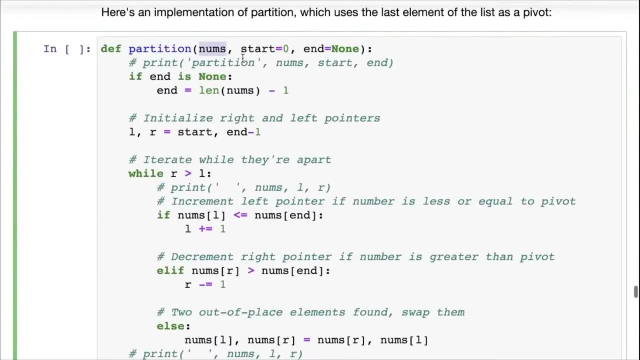 Okay, Uh. so once again, here you know, we have the nums, the numbers that need to be partitioned, the start and the end. And if end is none, we simply set end to the last index, which is Len nums minus one. 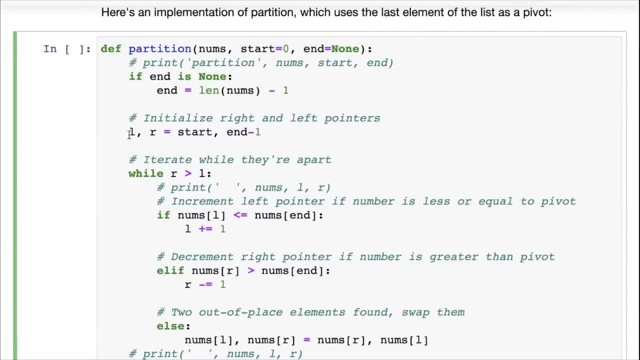 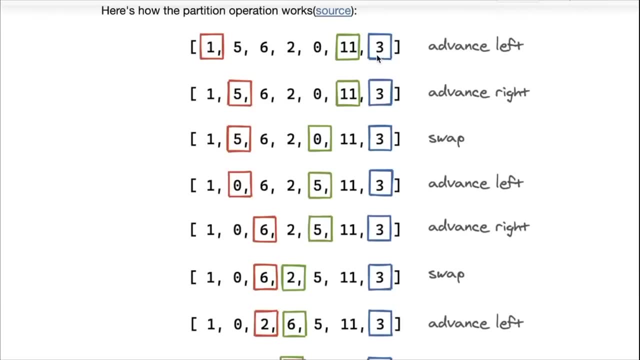 Then we initialize the start and end pointers. So we initialize the left and right pointers. Remember, we want to use The end element, So this is the end element, So we want to use the end element as a pivot. So the left, the left pointer is start and the right pointer is N minus one. 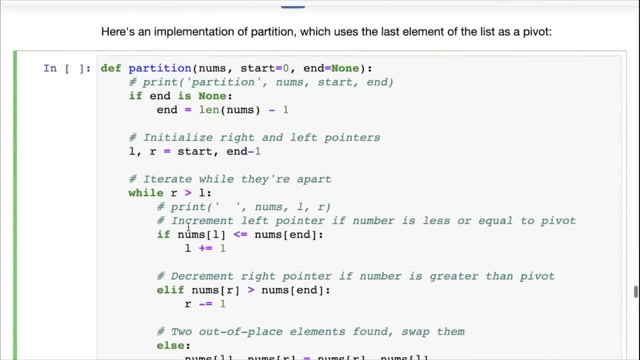 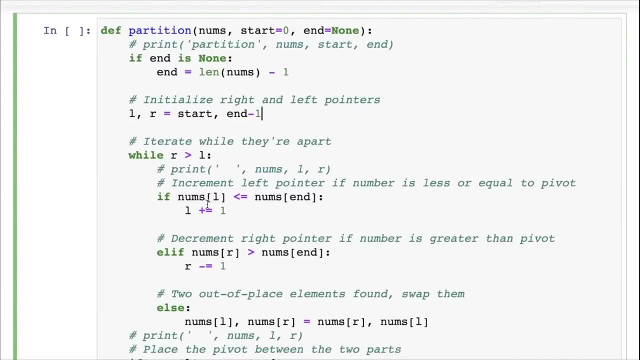 That's what we, that's what we've said here. And then white: while the right pointer is greater than the left pointer, we increment the left pointer. If the number at the left pointer is less or equal to the pivot, we decrement. otherwise we decrement the right pointer. 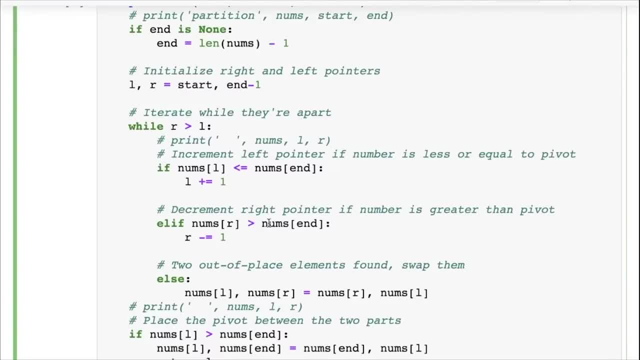 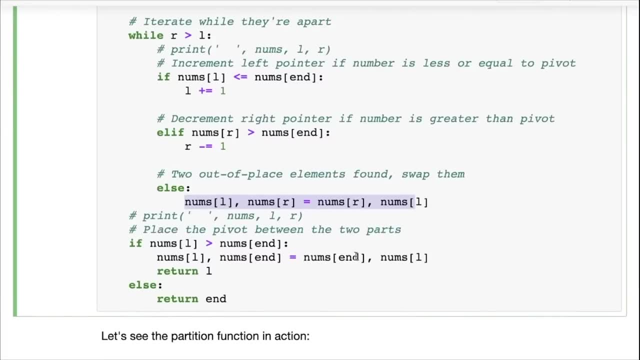 If the number on the right pointer is greater than the pivot. otherwise the two of them are Out of place and they can be swapped. So we swap them here And finally we place the pivot in place between the two parts, and that's it. 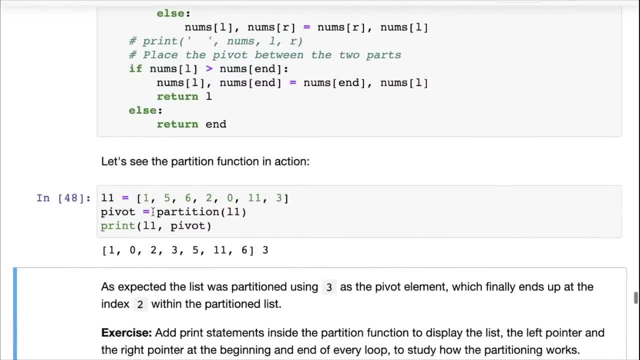 That's exactly what's happening here. So let's see here, let's see this partition. We are taking this list and we are calling partition on it, And three is the number that was used as a pivot. So now three ends up here in between. 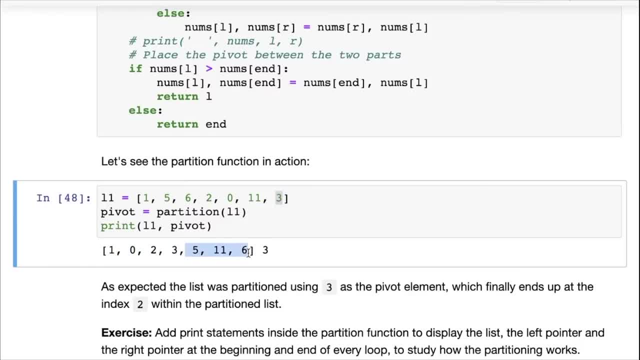 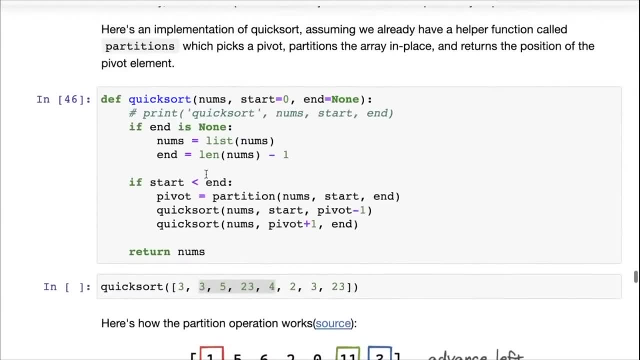 So you have one zero, two and five, 11, six, and the partition function returns the position of the pivot. So now You can see how it is used in quicksort. the partition function returns the position of the pivot And then we call quicksort on the left partition before the pivot and on the right partition after the pivot. 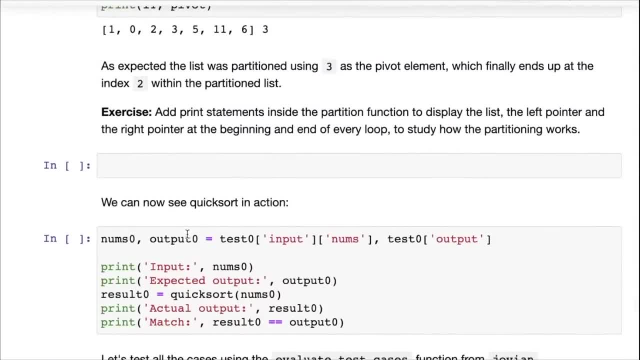 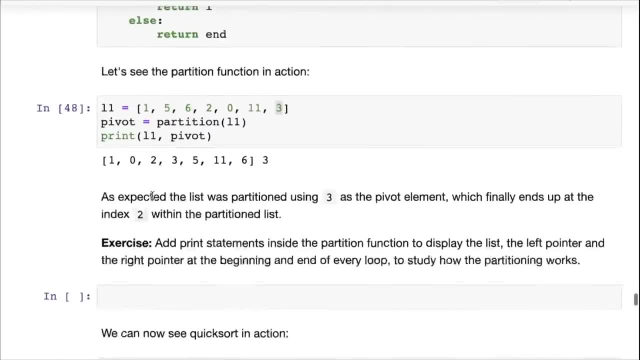 So now we can test out quicksort. Okay, And here's another exercise for you: add print statements inside the partition function. So there are already some print statements. You can simply uncomment them. uncomment the print statements to display the list. The left. 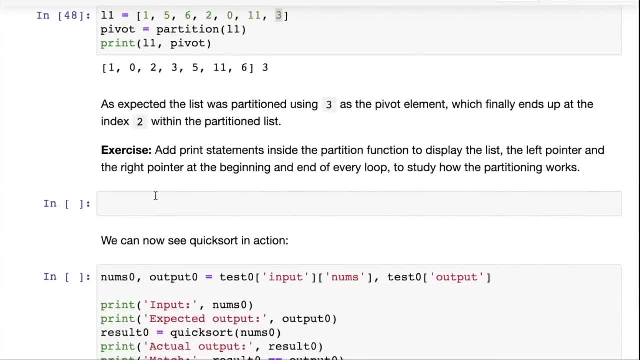 Pointer and the right pointer at the beginning, at end of every loop to study how partitioning works. And similarly, you can also add print statements inside the quicksort function to study how the recursive calls are going on. So study what we've done in merge and merge sort and add the same print statements in quick and quicksort. 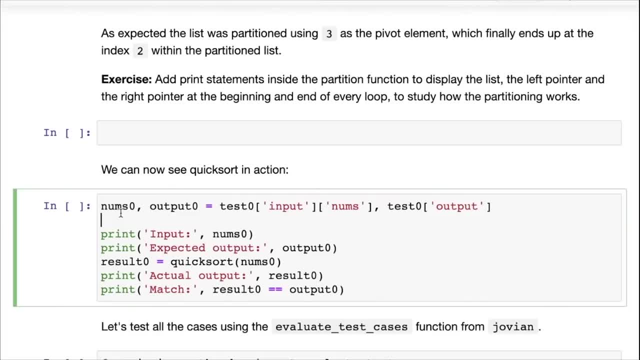 And look at these recursive calls. Now, what you want is to have a completely clear and perfect idea of what your code is doing. You don't want to be lost about it, And that's why adding print Statements and looking at small examples and making sure that it's working perfectly really helps. 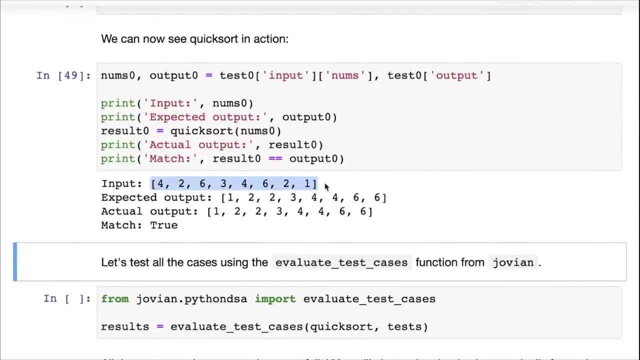 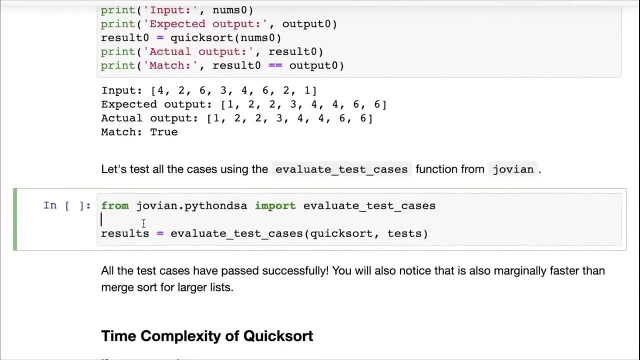 So let's look at quicksort in action. So here's an input and here's the expected output and here's the actual output. and they match great. And we can now evaluate all the test cases using the evaluate test cases. functions for function from Jovian. 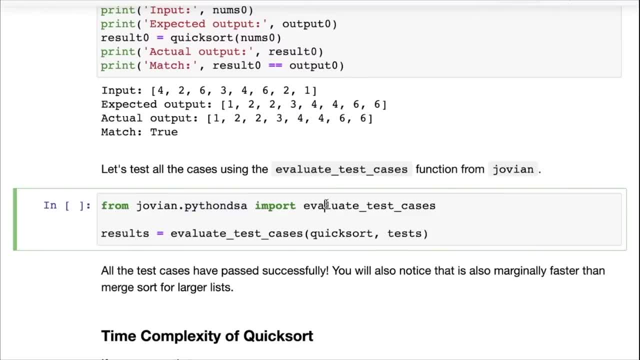 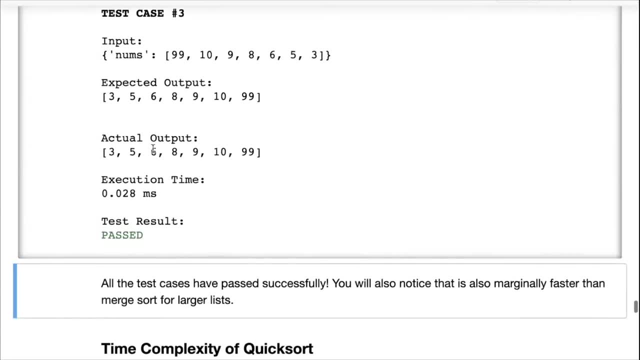 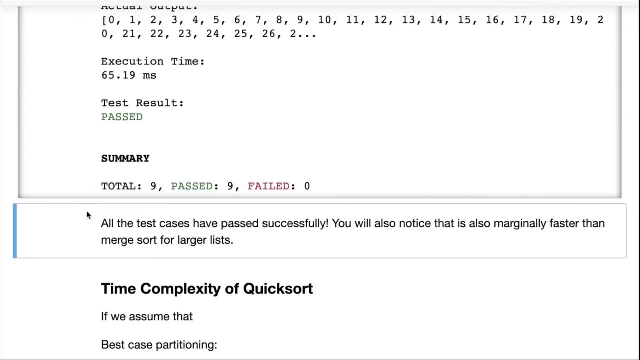 So we import from Jovian or Python DSA evaluate test cases and call evaluate test cases here And you can see that it passes all the test cases. And not only that, you will also notice that it is marginally faster than merge. sort for sorted lists. 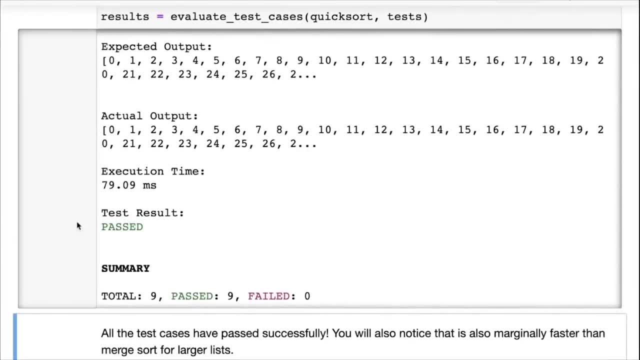 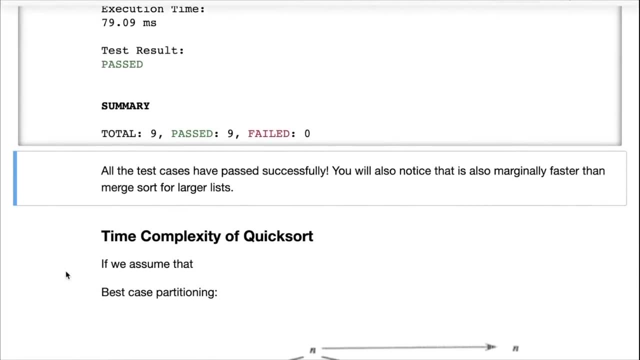 Sometimes you may not see that, but yeah, you can see here that it's. you will see that in most cases quicksort is marginally faster than merge sort for larger lists And that's because it is not allocating new space. Okay. 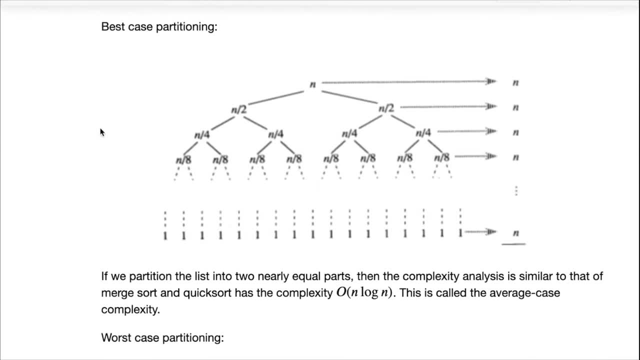 So now coming to the time complexity for quicksort. Now, assuming that we are able to have a good partition each time. So each time we are dividing the list into roughly equal halves, roughly equal parts. like you started the list of size N and you partition it into N by two and N by two. 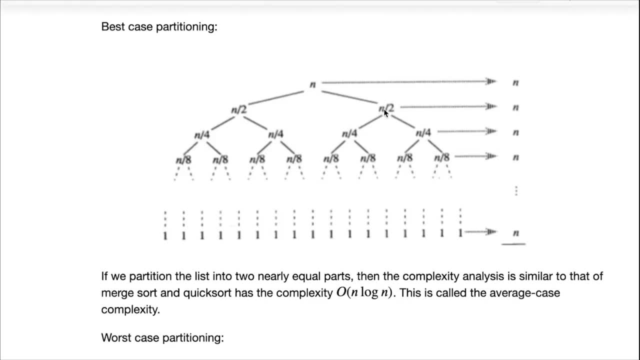 So this is what the sub problem tree looks like. So you call quicksort with two lists of N by two, N by two. then you call quicksort with four lists of size, N by two, N by four, N by four and so on. Now what is the activity that we're doing inside quicksort, in each quicksort? 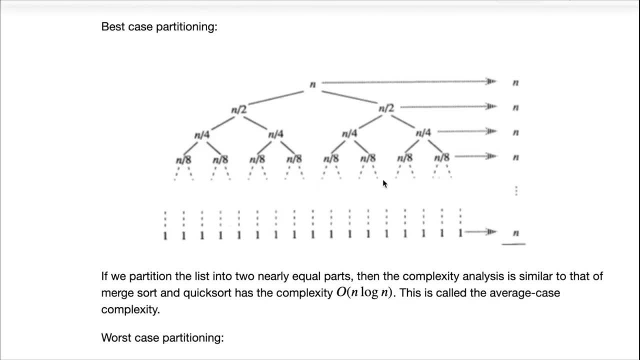 The core Operation is partition right, And that's what puts one element, the pivot element, into its right place, And then the element smaller than it to the left of it, the elements larger than it to the right of it. So the partition is where the actual work, the comparison and swapping happens. 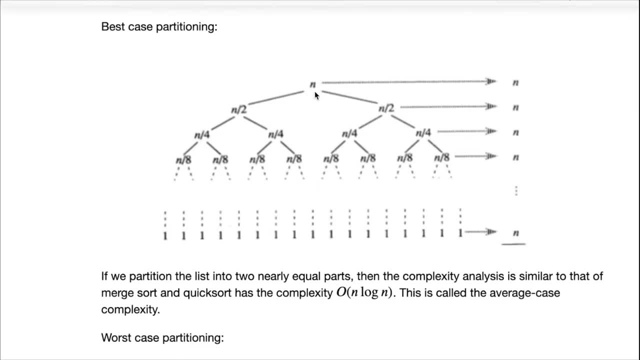 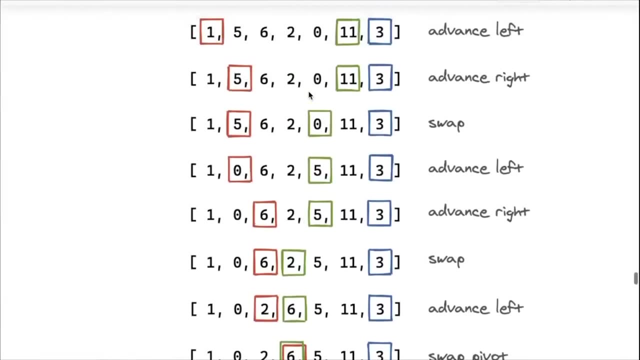 And how many comparisons do we perform in the partition? I would say that the number of comparisons is equal to the size of the actual list And you can see that here. you can see that we are going on comparing numbers Like this. we are comparing each number to the pivot. 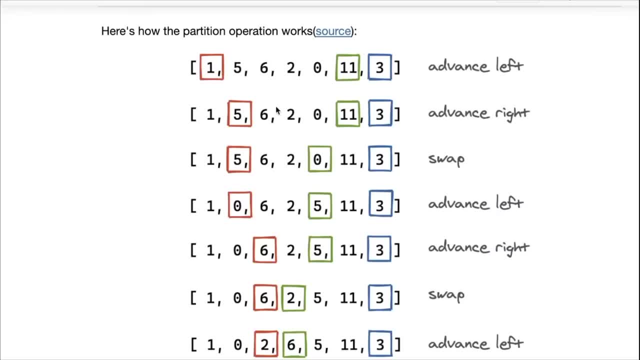 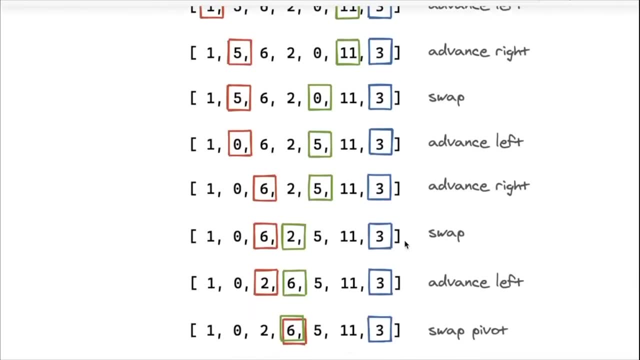 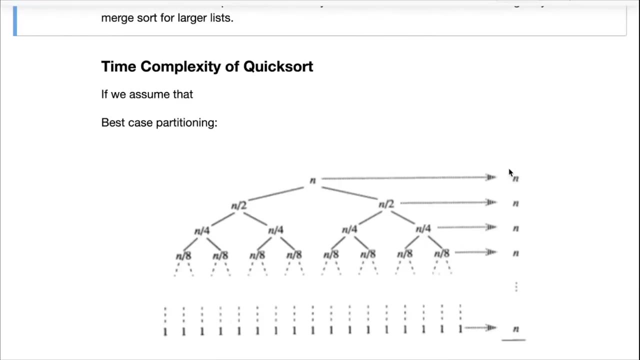 So each number gets compared to the pivot exactly once, roughly, And that means that there are a total of N comparisons If N is the size of the list. Okay, So we have N comparison and partition. So partition performs N operations or partition is an order N function. 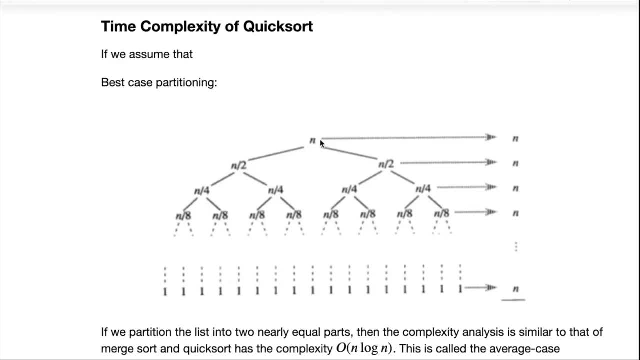 And what is the height of the tree? Once again, the height of the tree is log N, because to go from N to One it takes login steps. You keep going N by two and by four and by eight and so on, N by two to the. 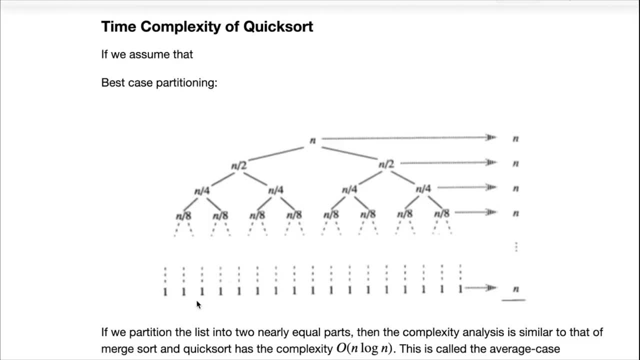 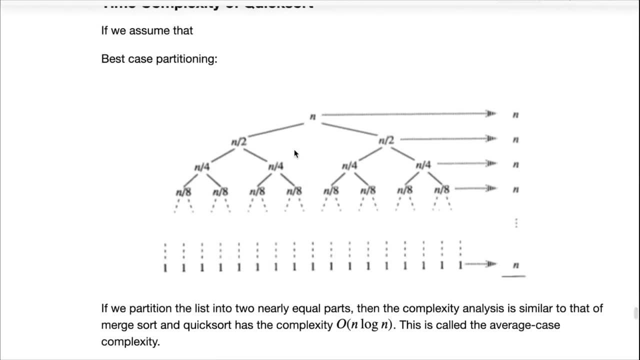 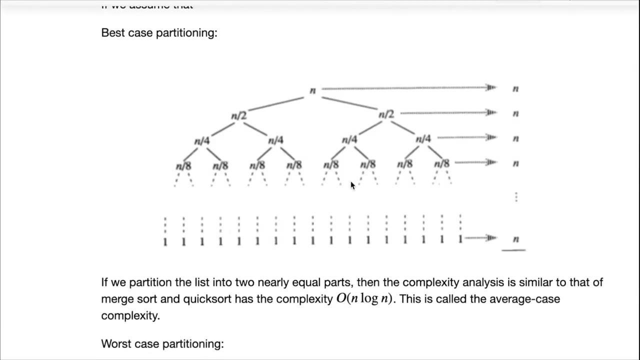 power log N becomes N by N one, And so the time complexity of quicksort is N login. If you're able to partition the array into roughly equal parts- And that is what happens on average- If you're picking random pivots each time, then you do end up with roughly equal parts. 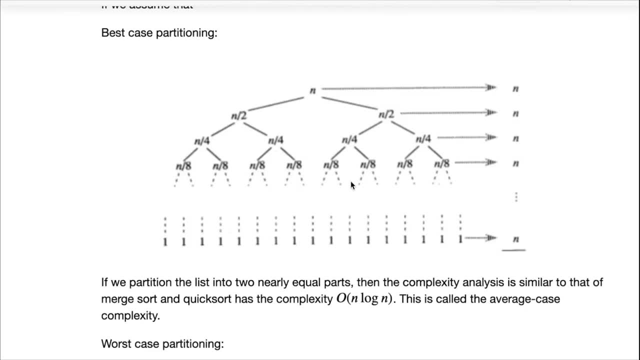 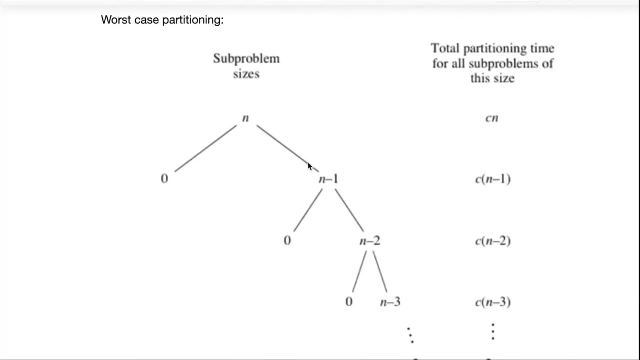 Maybe it's 75, 35, 75, 25.. But that's still more or less in the same range. So the quicksort complexity is about N login and this is called the average case complexity. On the other hand, if you have a really bad partition- and a really bad partition is maybe 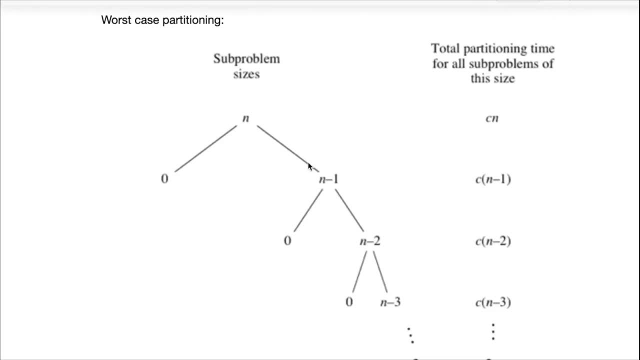 you picked the smallest element as the pivot. Now, if you pick the smallest element as the pivot, then all the elements will go to the right of the pivot and you will end up calling quicksort on a problem of size N minus one. And then 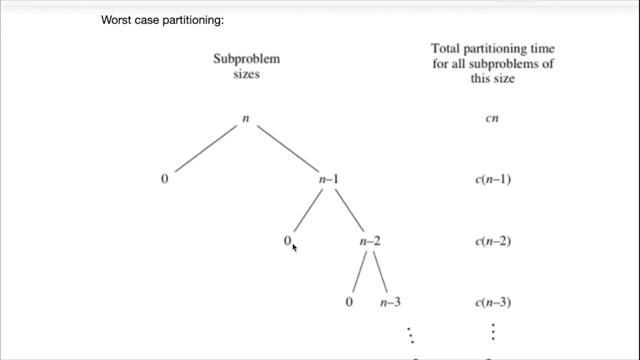 Maybe once again, if you pick the smallest element as pivot, all the elements will go to the right of the pivot once again and you will end up calling quicksort with a problem size of N minus two. Now this is an unbalanced T or a skewed tree. 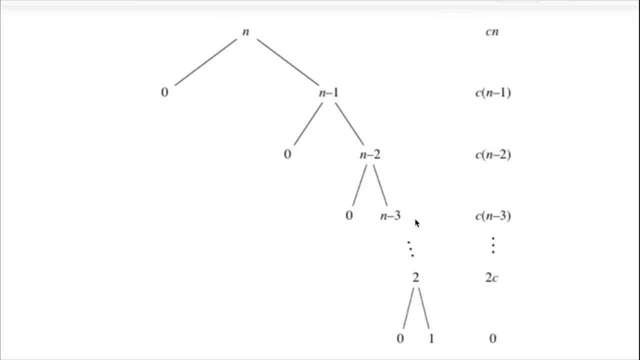 And what happens in a skewed tree is that the height this time is the same as N. you can see N, N minus one, N minus two, N minus three. So, going up to one, the height of the three is N, but the amount of work involved in partitioning is the same because 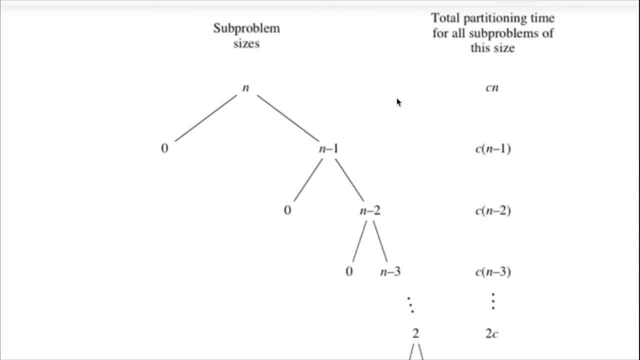 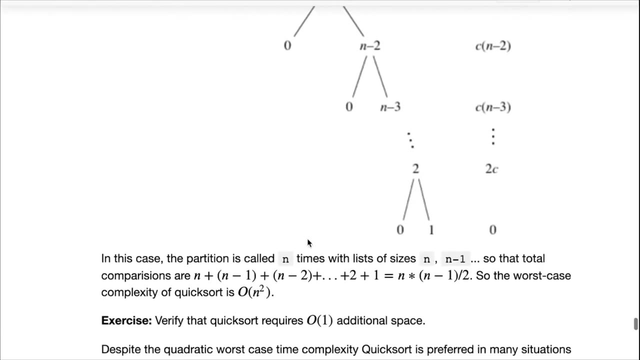 you have to run through the entire list to partition the list right, So that in this case the time complexity is roughly N times N minus one by two. So the time complexity is about order N square, and that's bad, because that's as bad as bubble sort. 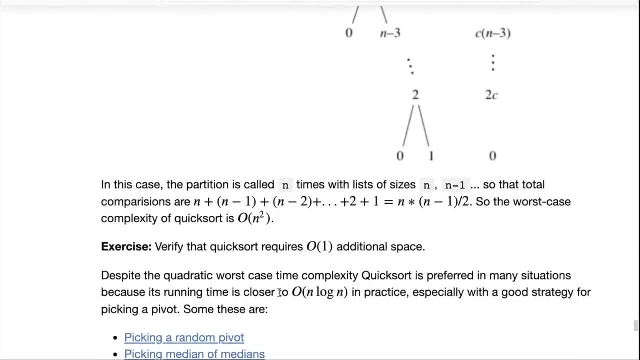 But despite the quadratic worst case time complexity, quicksort is still preferred in many situations. Now it really depends on what kind of Algorithm you need to use and what kind of memory constraints you have, because quicksorts complexity is closer to N login in practice, especially with a good strategy for picking a pivot, and a good strategy is picking a random pivot. but 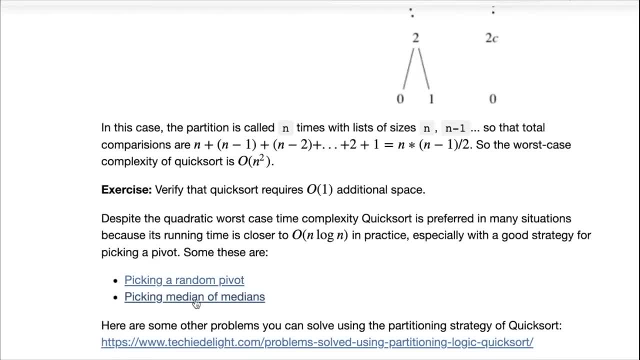 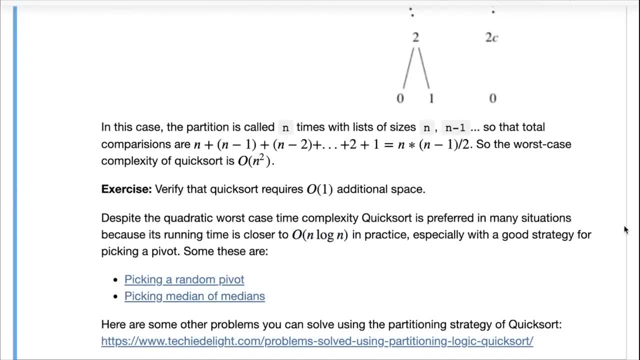 there's another one called picking median of medians. You can check that out as well. So that's: N login is the average time complexity of quicksort, And then N square is the worst case time complexity of quicksort. Now here's an exercise for you. 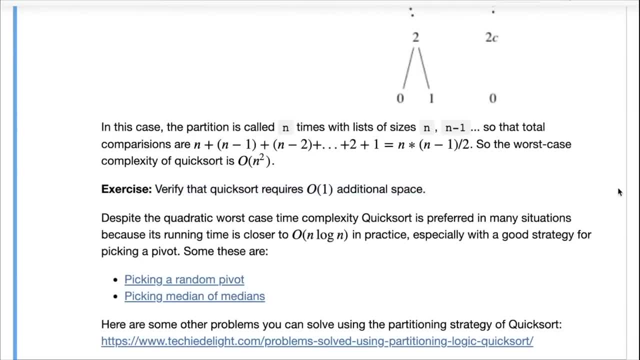 Verify that quicksort requires order One additional space, which means that it does not really need to copy the area. We did create a copy because we did not want to affect our test cases, but we could have removed that line and quicksort would work just fine. 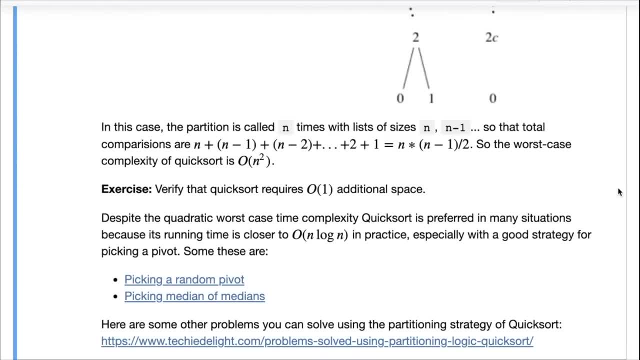 So because you do not need to create a copy of the list or the array, it requires order one additional space, but because space complexity also includes often the size of the space required to store the input, So you can say that quicksort has the space complexity of order N. 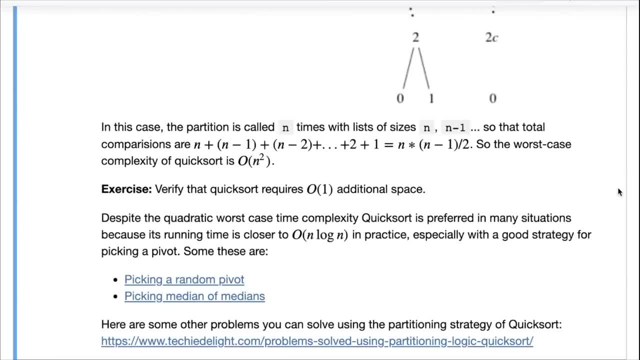 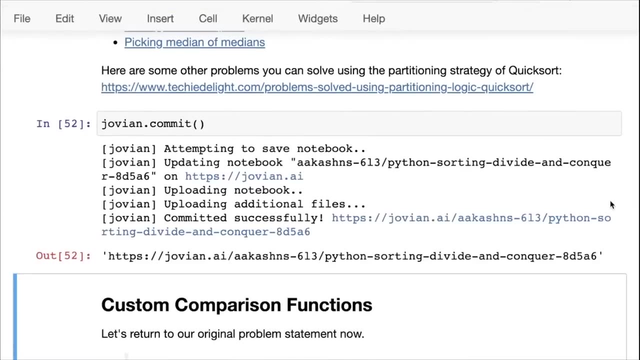 Okay. So if you get the question about space complexity, you may want to ask: are you talking about the additional space or do you also want to include the input in the space complexity? So that's quicksort And those are the two sorting algorithms we've looked at. 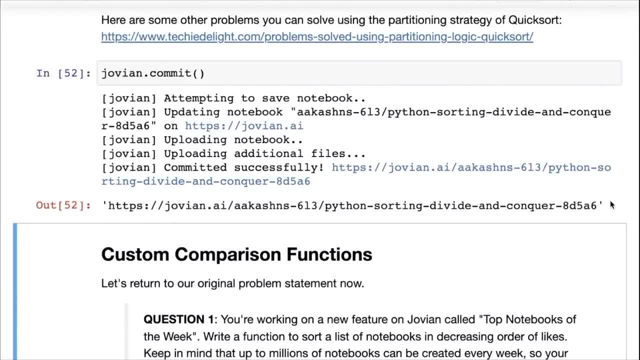 So we've looked at, we've looked at bubble sort and we've looked at insertion sort, and then we optimized it using divide and conquer and got to merge sort, which is order N logic. So we're going to look at that one. 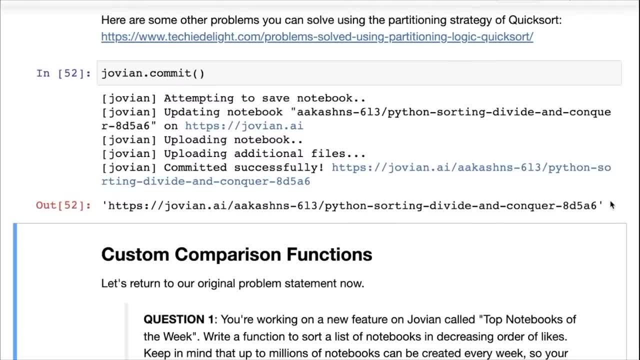 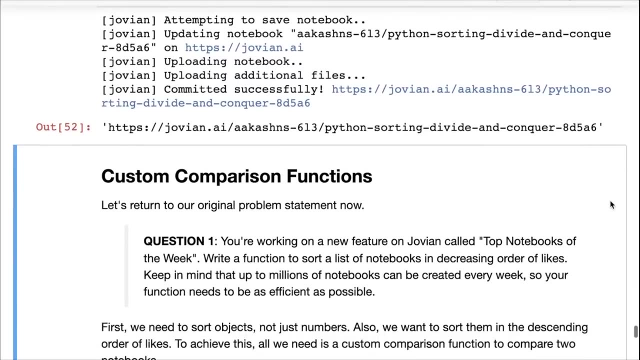 Okay, So we're going to look at a sort of n log N, but it also has the space complexity of, or the additional space requirement of, order N, which can be avoided using quicksort, which uses order one additional space but can have order N- square complexity in the worst case, time complexity, but with the right choice of a pivot it is closer to N log N. 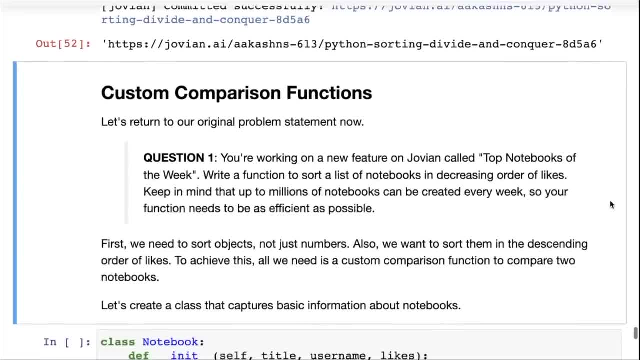 So that sorting- and you can see that Python is such an expressive language that all these sorting algorithms are actually using the N log N that's used for the type of space that the table is. Okay, So, Okay, So, Okay, Okay. 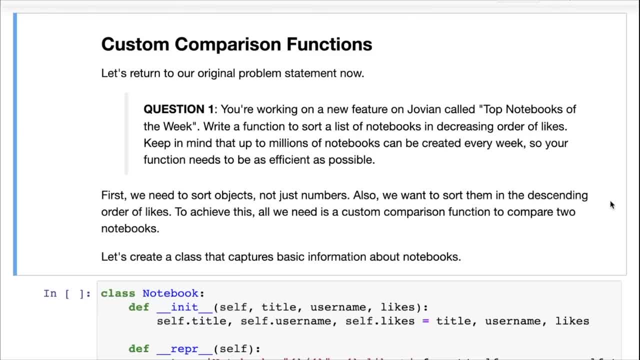 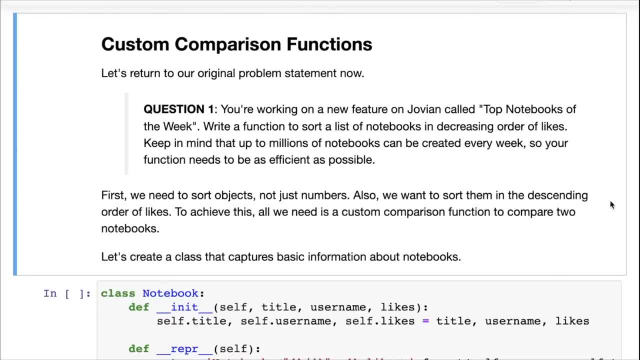 some test cases ready to test your function and then write your code carefully, checking each line for errors, and create small functions wherever you need to. So try not to have too much logic in one function. A good rule of thumb is about seven to eight lines of code per function, no bigger than. 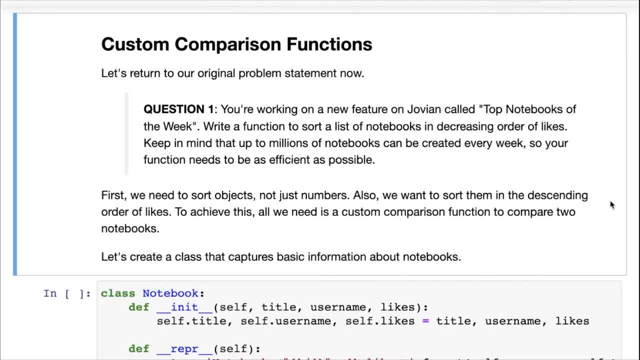 that, And that's not just for toy problems, but that's also, even as a software developer, something that you can try to follow. Just have seven, eight lines of code in any function. If you have more than that, try to split it into two functions, and this way it's very. 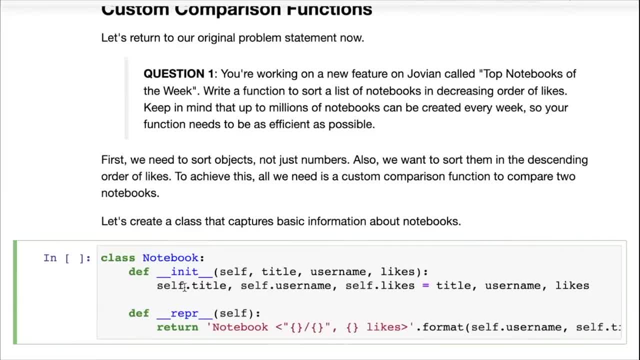 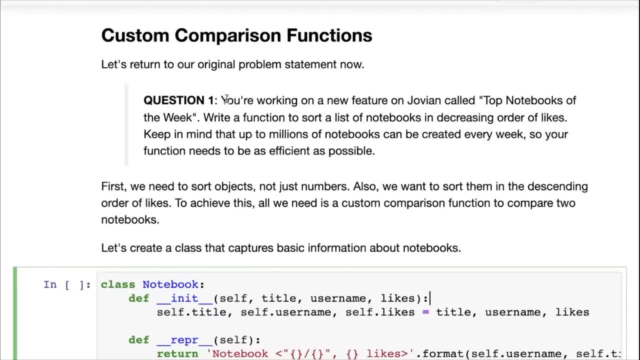 difficult for you to go wrong. So now let's return to our original problem statement and let's read it Once again. you're working on a new feature on job. We in called top notebook of the week top notebooks of the week and I had a function. 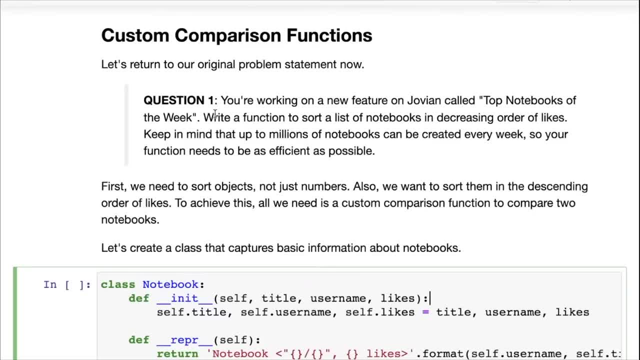 to sort a list of notebooks in decreasing order of likes. Now keep in mind that up to millions of notebooks can be created every week. You want to build this for scale, So your function needs to be as efficient as possible. So first we need to sort objects this time, and not just numbers. 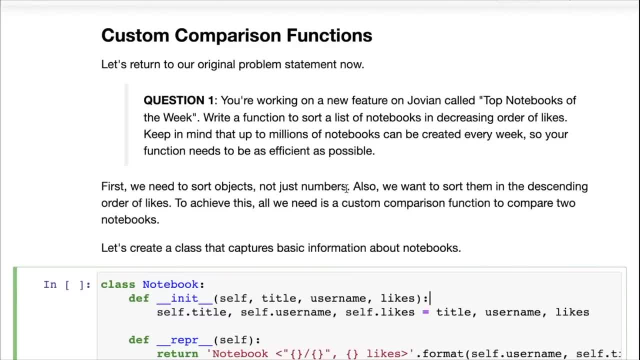 And second, we also want to sort them in the decreasing order of likes for each notebook. Okay, So all we need to do it To use Our merge sort or quick sort techniques that we've already discussed is to define a custom comparison function to compare two notebooks. 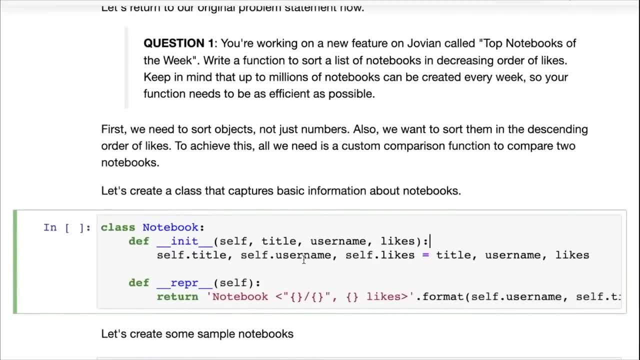 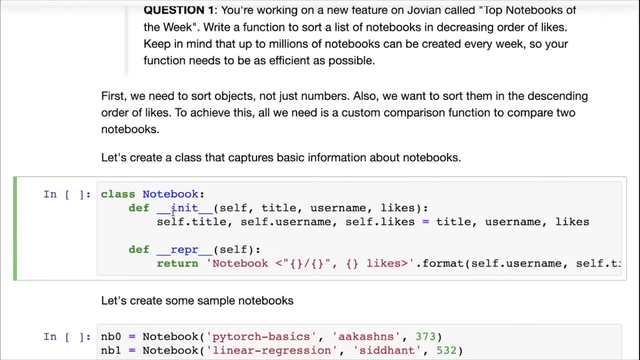 Okay, But before we do that, we let's create a class that can capture some basic information about notebooks. So here we have the class, So we're still following the method, so to speak, right. The step one was to come up with the input and the output format. 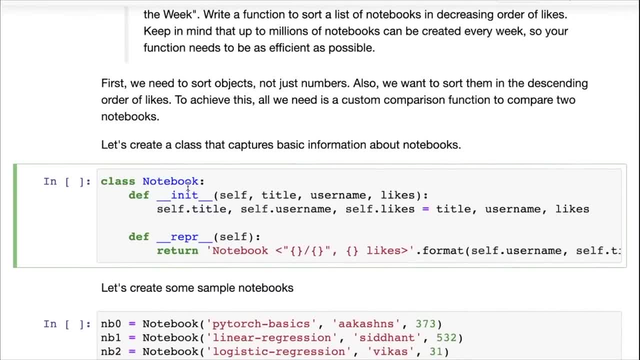 So here is the input format. Our input format would be using this class. So we create, creating a class notebook which is a title, It is a title, username and likes. So we create the class and that gets stored as properties, titles, username and likes. 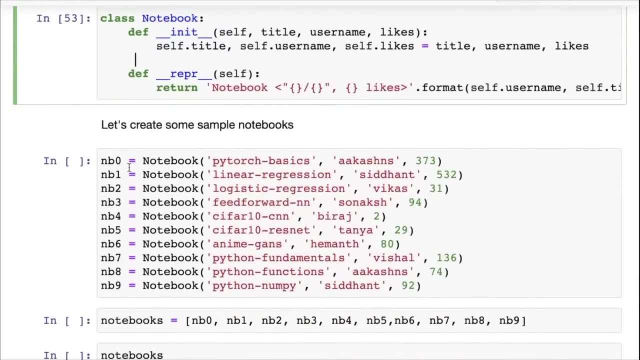 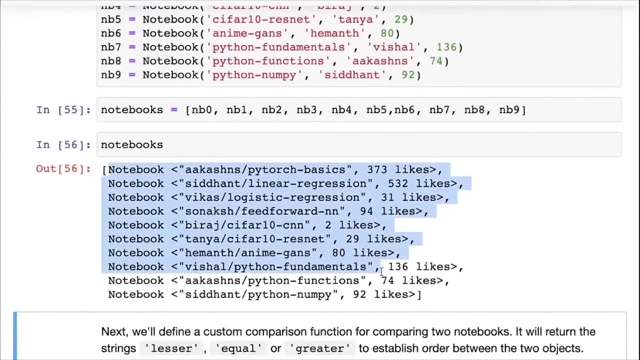 And then we also have a string representation here- Then create some test cases. So now we are creating some test cases here, So we are creating some test cases in NB zero to NB nine and let's put them all into a list and you can see here that we now have a list of notebooks and B zero to NB nine. 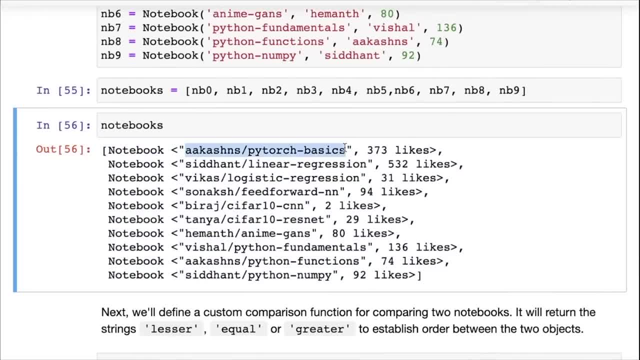 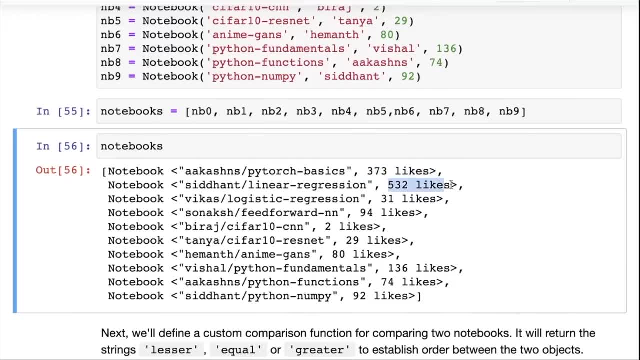 And you can see that. Okay, So because we have a string representation, we can see that the first notebook is this: Akash Ns slash PyTorch basics, and it has three, 73 likes. And the second one is this, and it has five, 32 likes, and these are clearly out of order. 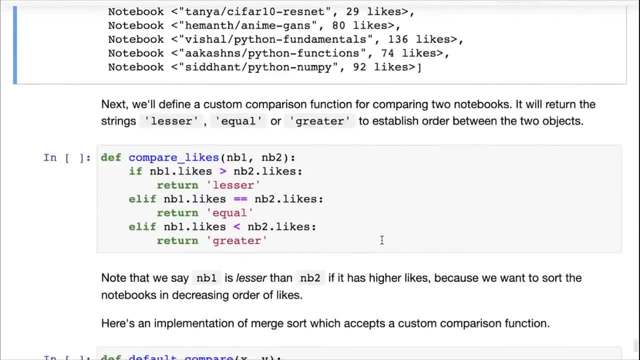 in terms of likes. Next, we'll define a custom comparison function for comparing the two notebooks. What it will do is it will return the strings lesser, equal or greater to establish the output order between the two objects. Okay, So it should return lesser. 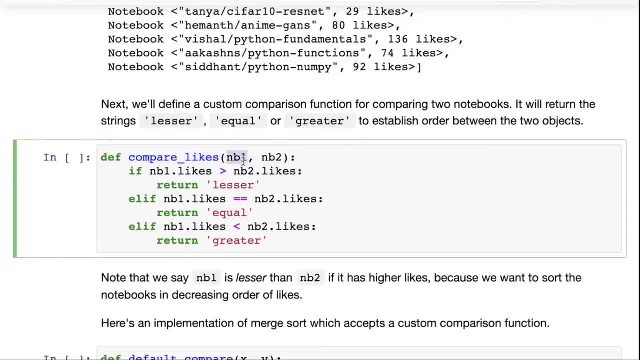 Okay, So in this case, NB one should come at a position or a index lesser than the position of NB two in a sorted list. Okay, So in in. in case of our problem, what that means is: we want to sort things in the decreasing. 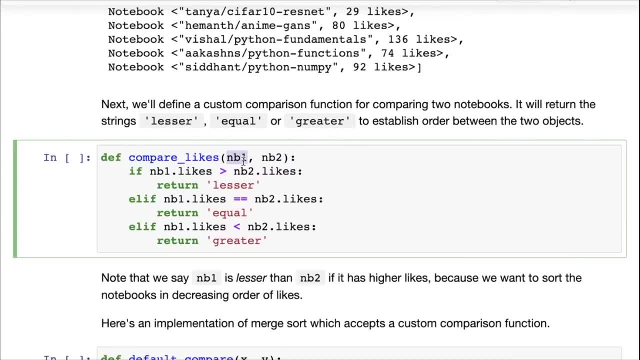 order of likes. So the first notebook should have the highest number of likes and then maybe the second notebook should have the second highest number of likes and the third notebook will have a lower number of likes, and so on. So if you have two notebooks, NB one and NB two, 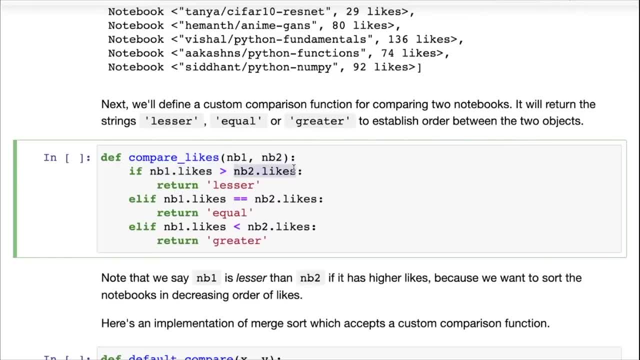 Okay, So if NB one dot likes is greater than NB two dot likes, so then NB one should come at a lesser index. Okay, So we will return lesser because it should come at a lower position in the sorted list. So we return lesser because we want a decreasing order. 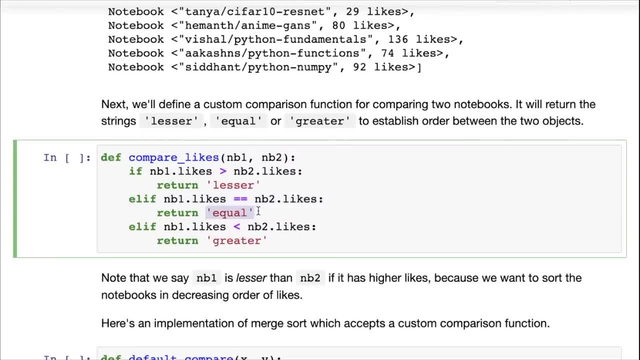 And if NB one dot likes is equal to NB two dot likes, then we return equal. And if NB one dot likes is less than NB two dot likes, So that means this is not a is. NB two is the more like notebook, NB one is less. 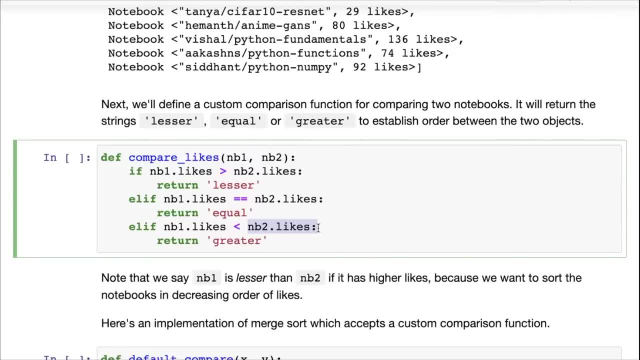 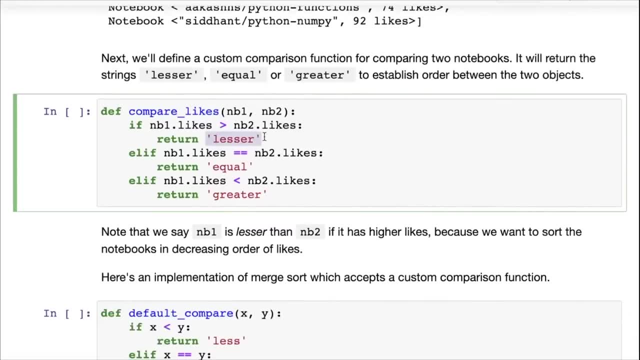 One is the less like notebook, Then NB one should actually come at a greater position, So we will return greater. Okay, So this is this comparison function should return whether the first input to it should come up. should show up at a lesser position in the sorted list compared to the second. 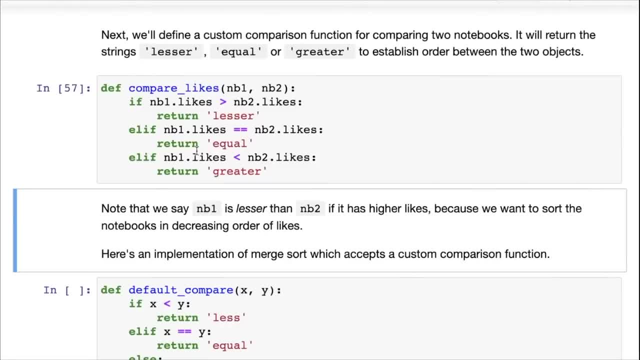 input. Now in languages like C plus plus in Java, normally the convention is to return a negative number, zero or positive number, But I find that Python allows you to return strings. Strings are first-class citizens in Python And it's a lot clearer when you are debugging things, when you face issues, to look at actual 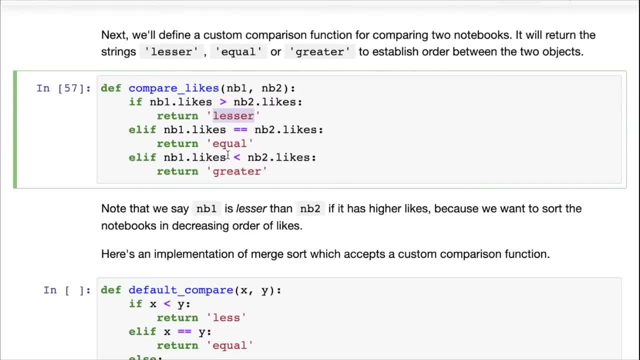 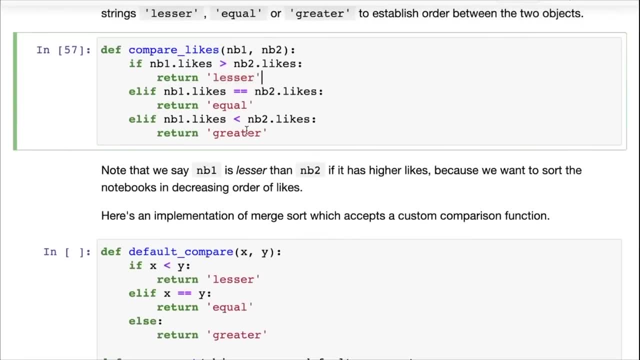 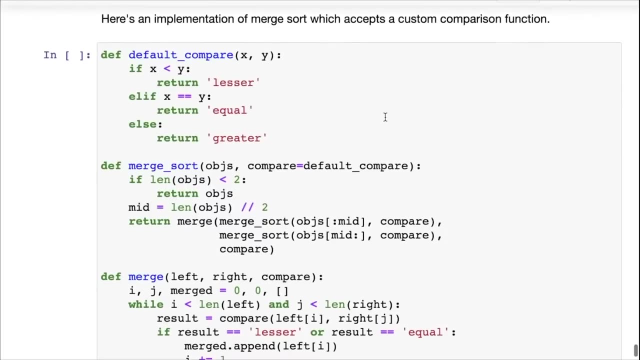 strings and it's also easier to write write code, So I prefer using strings. but you can also use- you can also use numbers like negative, zero or positive. That's totally up to you. So now here is an implementation of merge sort which accepts a custom comparison function. 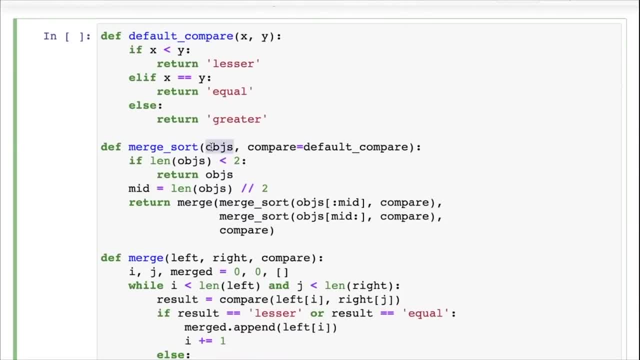 Okay, So the merge sort function. so the merge sort function uses: it takes a list of objects, this time, not a list of numbers, And it also takes a compare function which by default we also provide a default comparison so that we can still use it with numbers. now with numbers, and default assumption is if 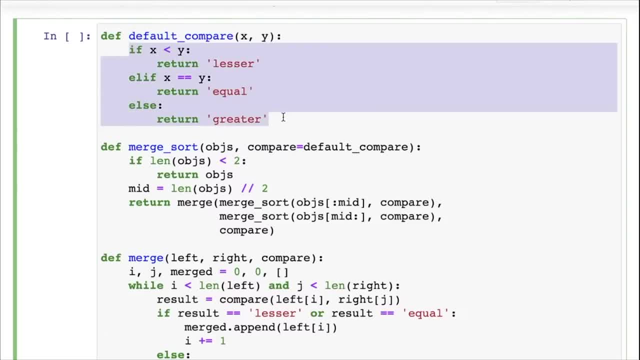 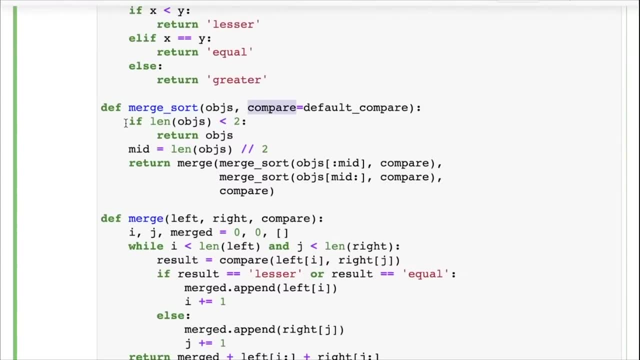 you want sorting. you want sorting in increasing order. So this is what the default sorting looks like for numbers. So that's pretty straightforward. but you can also pass a custom comparison function. So here we have the terminating condition. If the length is less than two, then we simply return the list. 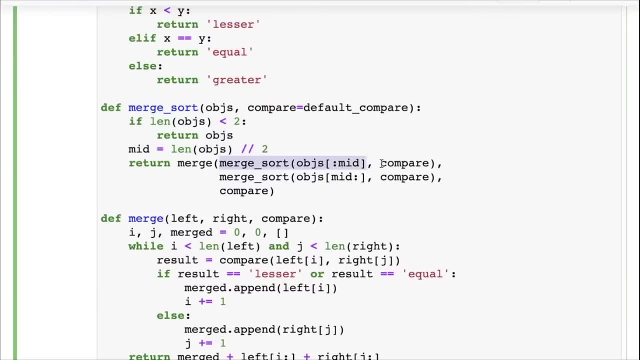 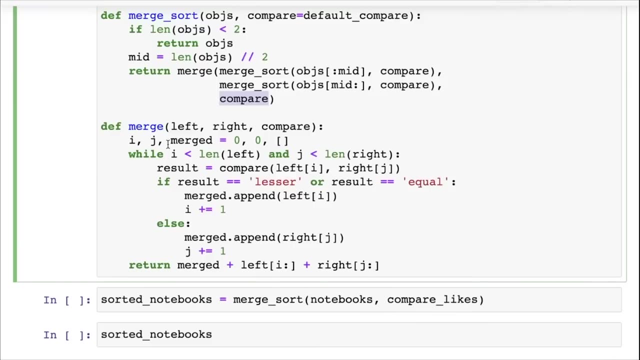 Then we get the mid index And then we call merge sort on the left half with the custom comparison function, We call merge sort on the right half with the custom comparison function And we call merge with the custom comparison function. Now what happens inside merge, inside merge. earlier you know, once again we have these. 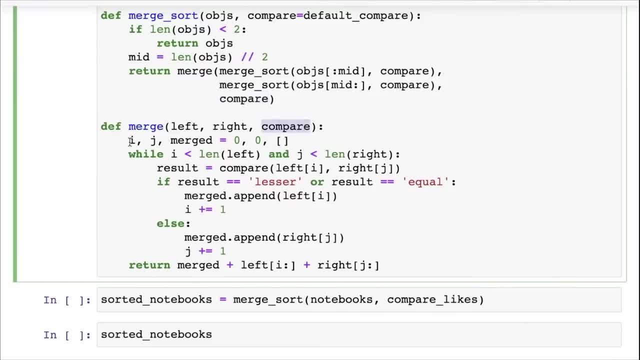 two halves, left and right, and then we have a custom comparison function, So we create pointers for the two of them, And then we also create the final result list, which is merged, And then we iterate over the left list and the right list. 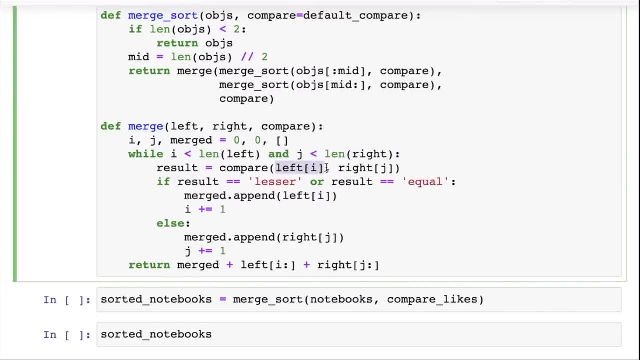 So while we are going through these, we compare the left element and the right element. So now we're calling compare, Now we're not doing the greater than less than comparison and we're calling compare. And if the result, if the element on the left is lesser or equal to the element on the right, 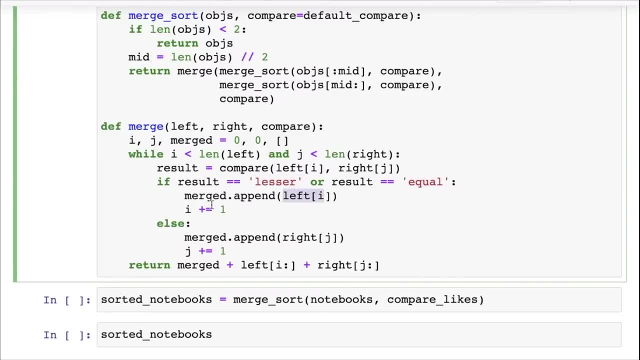 then we append it to the result area and we increment the left counter Otherwise. So lesser or equal means that the element on the left, the first element on the left, should show up at a lower position in the sorted- final sorted list. So that's why we appended first 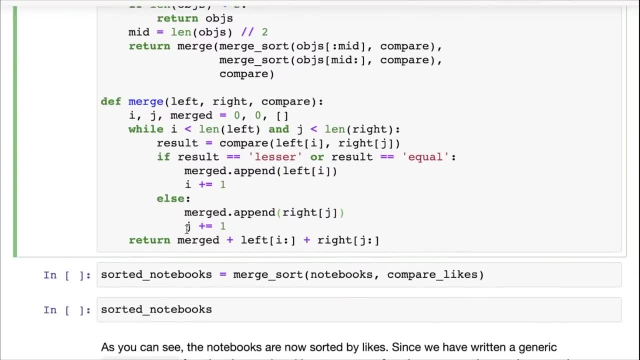 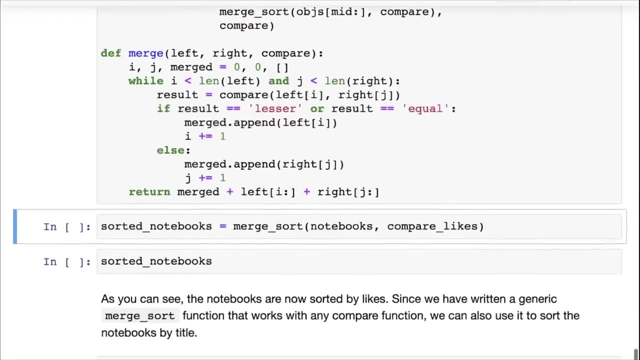 Otherwise, we append the right child, the right element, and we increment the right pointer And finally, we attach any remaining elements here. So this is something that you can review, something we've covered in a lot of detail. So now let's see, let's call merge, sort on our notebooks and let's check if the notebooks 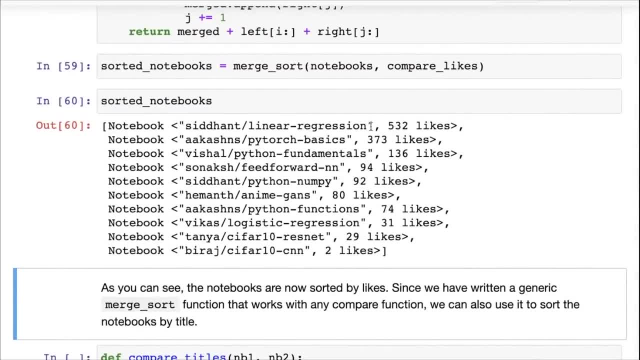 are sorted by likes. And if they are sorted by likes, Okay, Indeed they are. You can see that at position zero, you have the notebook with the highest number of likes, and then you have the next one, and the next one, and so on. 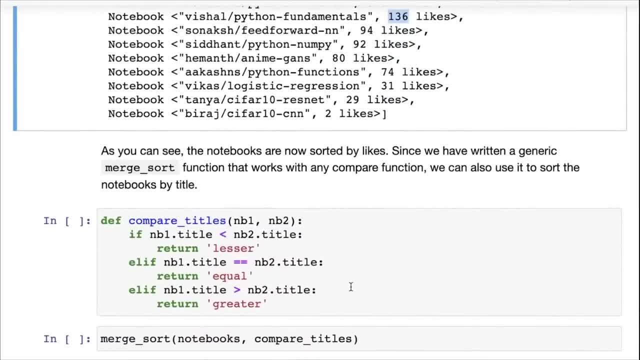 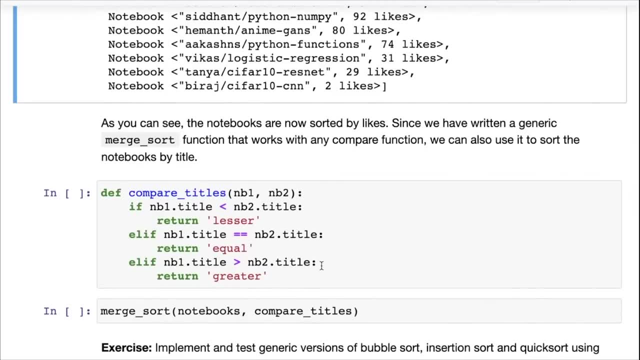 Now, since we've written a generic merge sort function that works with any compare function, we can now very quickly use it to sort the notebooks by title as well, Or, if we had maybe the number of views per notebook or the number of versions in each. 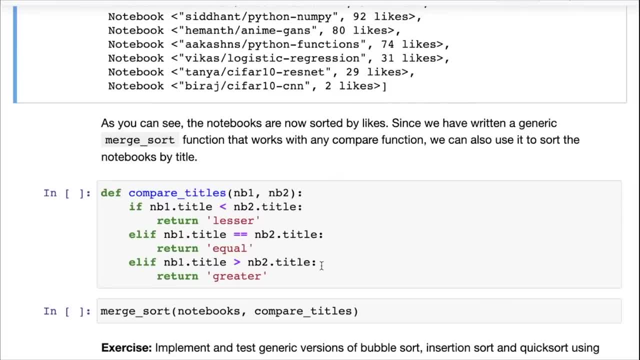 notebook or the number of comments on each notebook. we could do that sorting as well, So we could even use a hybrid of those. So here the example we're taking Is comparing by titles. So here we have NB one and NB two, and simple comparison strings can also be compared using 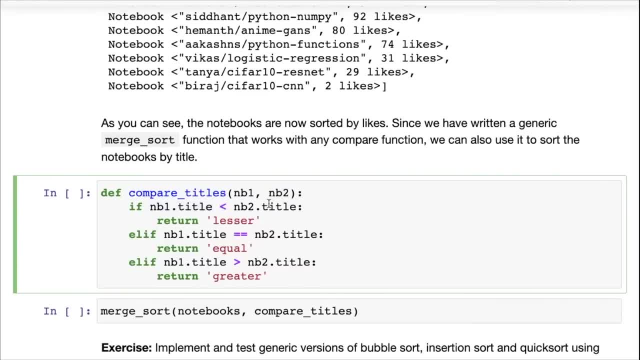 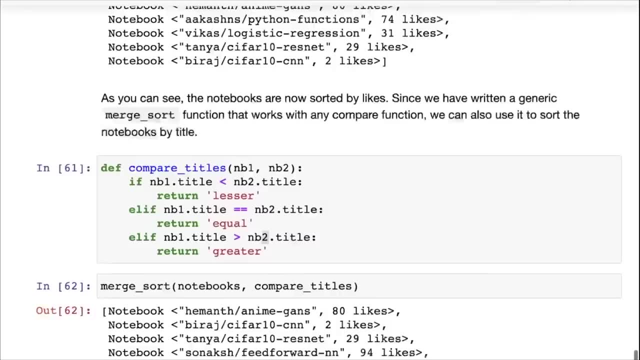 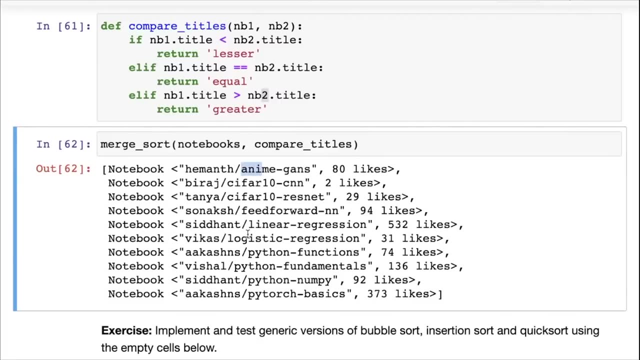 the comparison operators. So if NB one dot title is less than NB two dot title, then we return lesser. Otherwise we return equal or greater, And with this we should be able to sort them in the ascending order of titles. You can see a, N, C, I, C, I, F, E, L, I, L, O, P, Y, P Y. 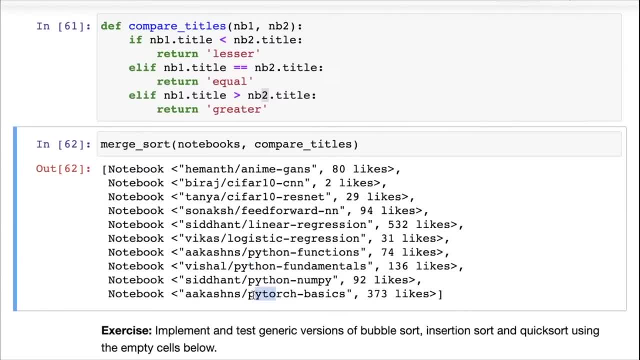 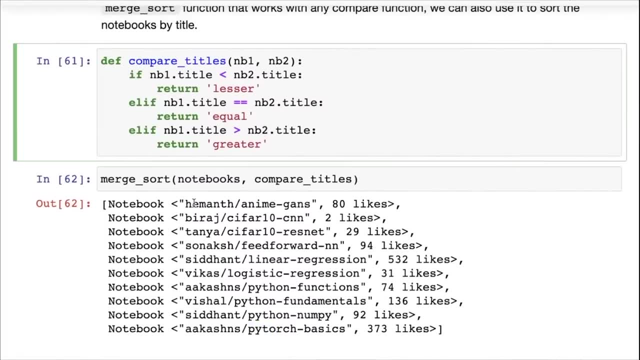 Okay, P Y T H P Y T O By torch. Okay, So there's no order sorted in the order of titles. An exercise for you is to sort in the order of username slash title, which means you first compare the username and if the usernames are equal then compare the titles. 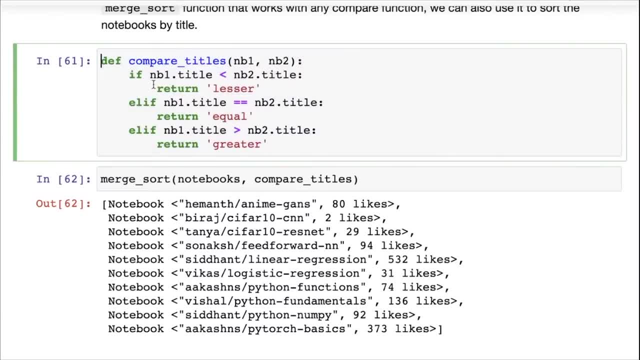 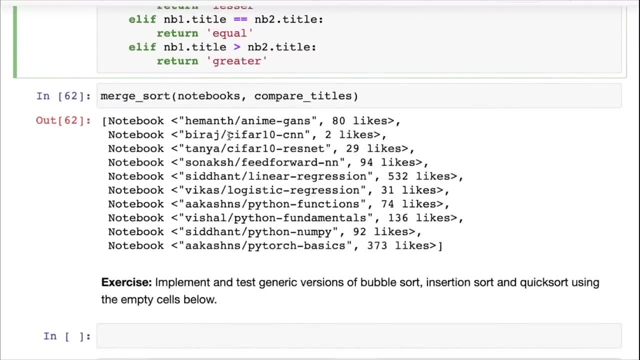 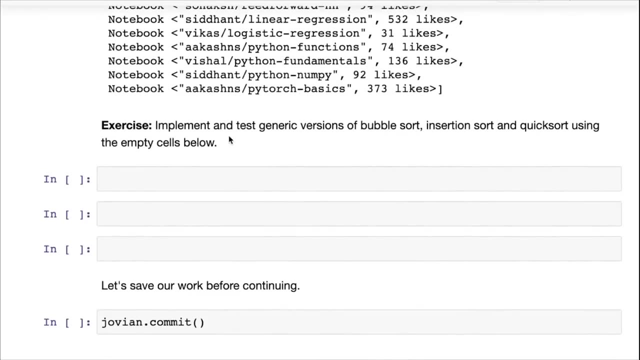 So you can compare. you can probably write another comparison function- compare username and titles- and use that to do that two level comparison and use that for sorting. Okay Now another exercise for you- Okay Forward- is to implement and test the generic versions of bubble sort, insertion, sort and. 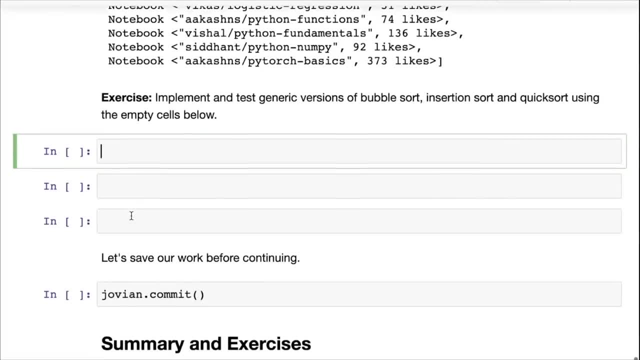 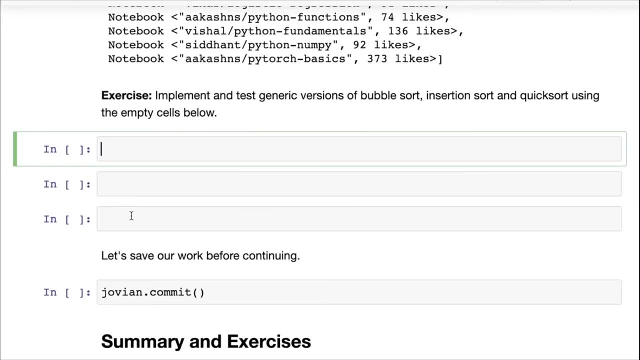 quick sort using these empty cells that are given here Right Now, at this point in the course, you should start writing code. You should be writing maybe solving one problem every day to really practice the concepts and internalize them. And while you're doing that, you can also any problem that you work on, any notebook. 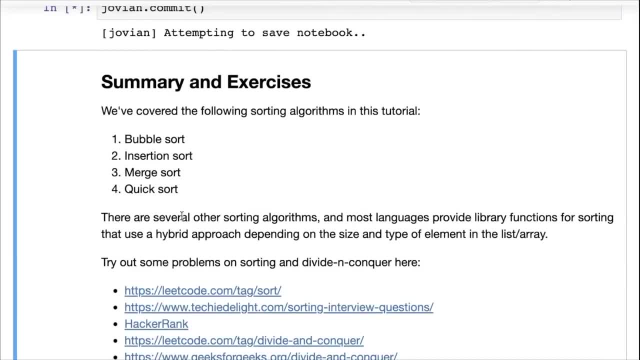 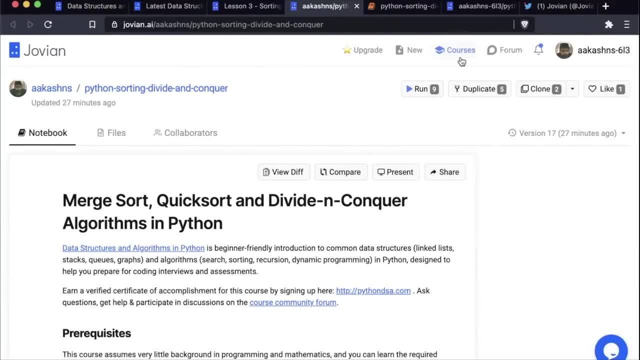 that you create, you can save it. Okay, Let's move on to Joviancom it and I'll show you also how to create new notebooks. So one way to create new notebooks is to go to Jovian, your window, di click the new button. 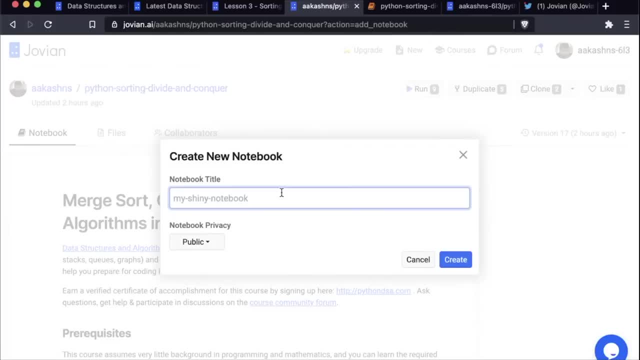 and click blank notebook And you can give it a title. Let's say you are doing quick, sort Generic, And you can set a privacy and create a notebook and that creates a notebook for you And then you can click the run button and run it. 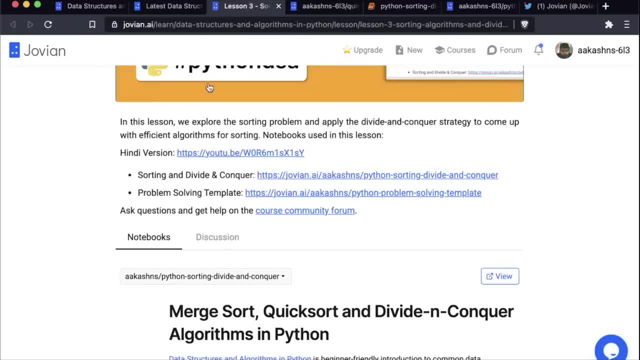 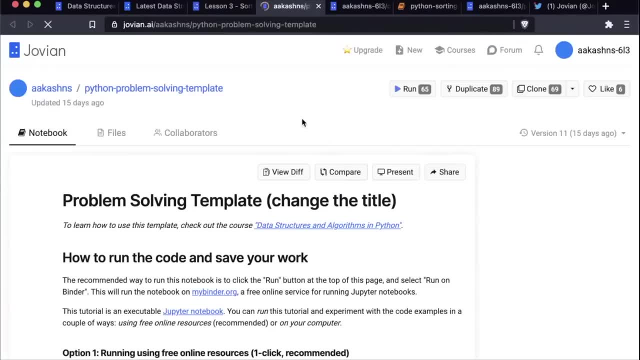 So that's one way to do it. another way You can do it is: we've given you a problem solving template. So if you come back to the lesson page, you will find a problem solving template here. Now you can click on the problem solving template and click duplicate to create a. 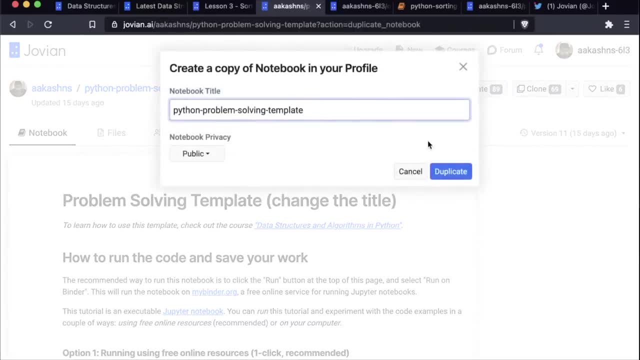 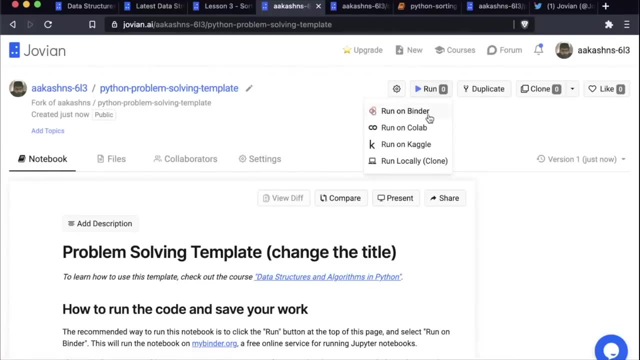 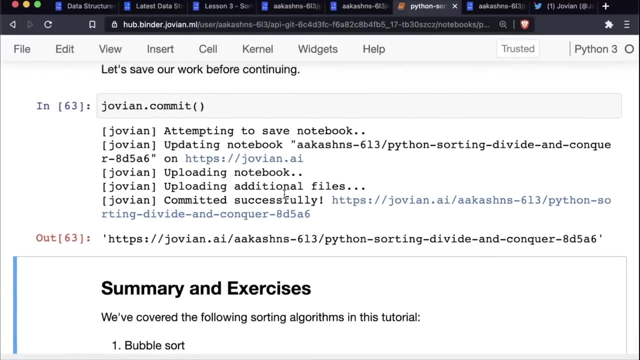 copy of this notebook in your profile. So let's do that. And now this is on your profile, so you can now click run and then run it on binder, or you can even run it locally on your computer and make some changes to it and come back and run joviancommit, and you will end up with a link that you 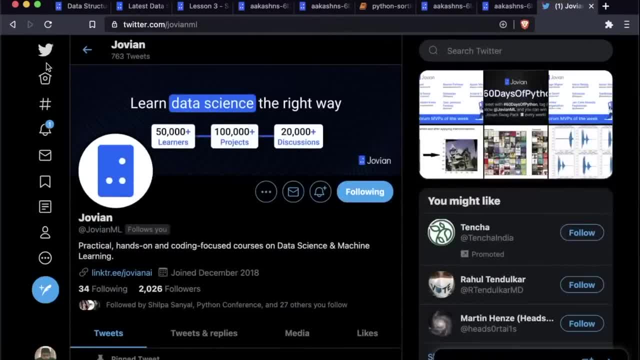 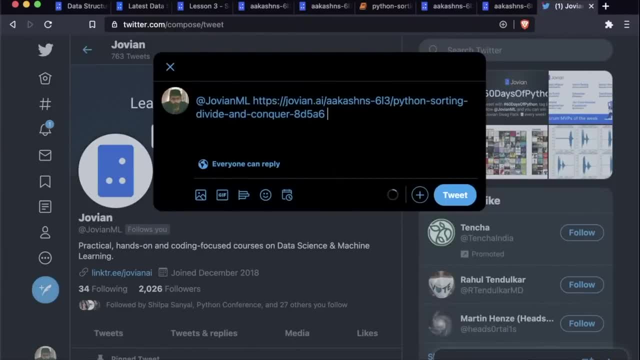 can share. So now you can now go on Twitter and you can just share this link. So write out a tweet and a tag us and also use the hashtag 60 days of Python, Okay, And maybe say: this is your quick sort algorithm for generic objects. 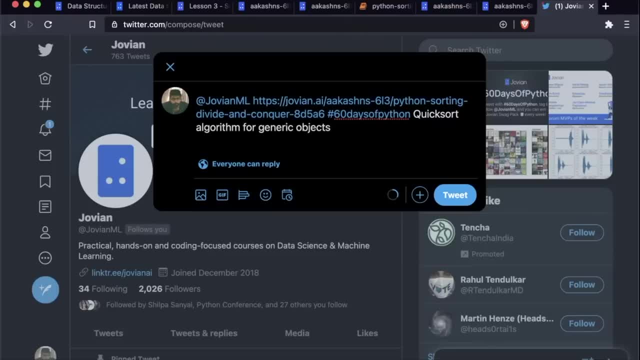 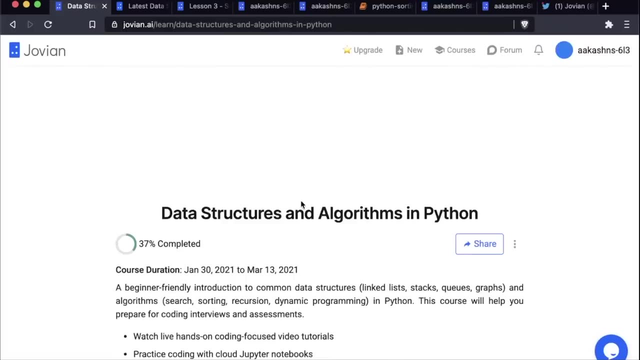 And tweet it out and we will retweet your tweet. So we want to support everybody who's taking part in this course. on the course page, you will find a link to the course community forum, which is where you can go and ask questions, where, if you have questions about any of these and you 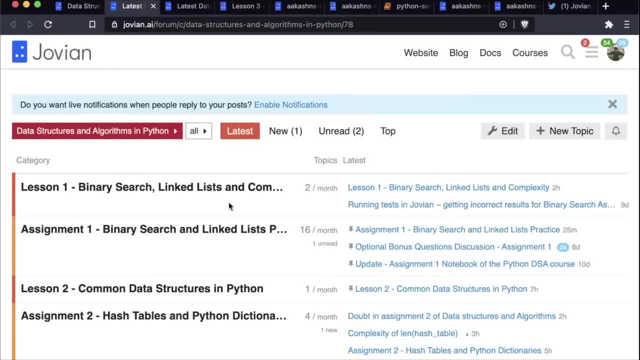 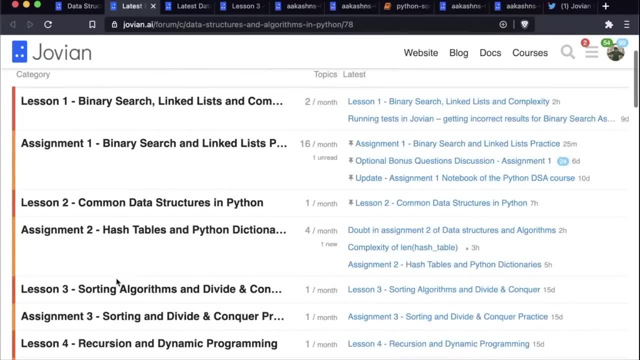 can even discuss some of the ideas that are discussed here, some of the exercises that are shared, so you can go into Lesson three, for instance, and create a new topic. Maybe you want to talk about the generic implementation of quicksort. 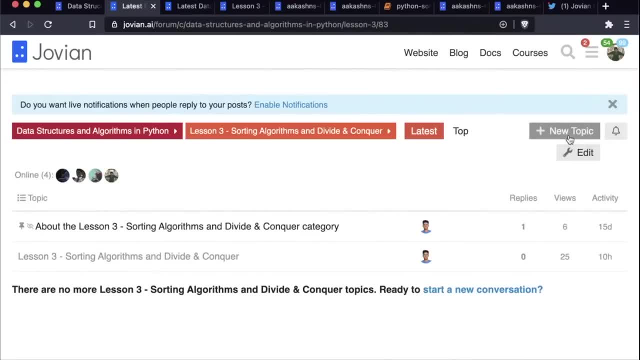 So maybe you want to talk about the generic implementation of quicksort. So maybe you want to talk about: Okay, Maybe you can create a new topic and post a query there. If you're not able to make it work, post your notebook there and ask a. 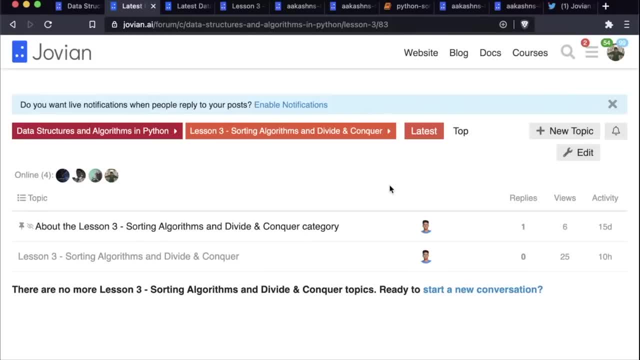 question, have a discussion And if you are helping other people out, if you're answering other people's questions and you've written some really great posts, there are links to some more problems that have been shared here, So you can check out these links on each of these links. 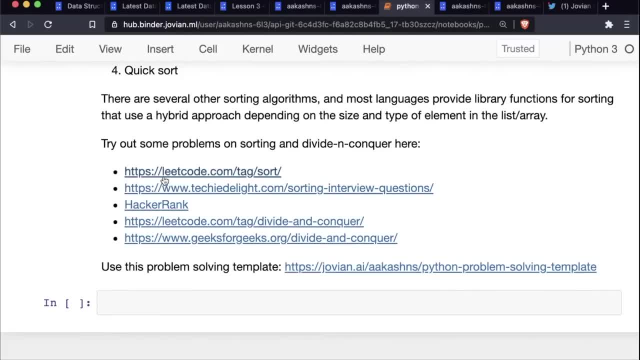 You can try out problems, You can make submissions, You can solve these problems. Some of these are interview questions as well. You can check if your results are correct and you can use this solving, problem-solving template as a starting point, as we've just shared. 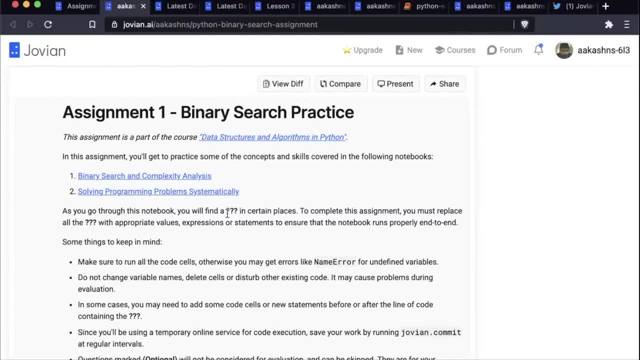 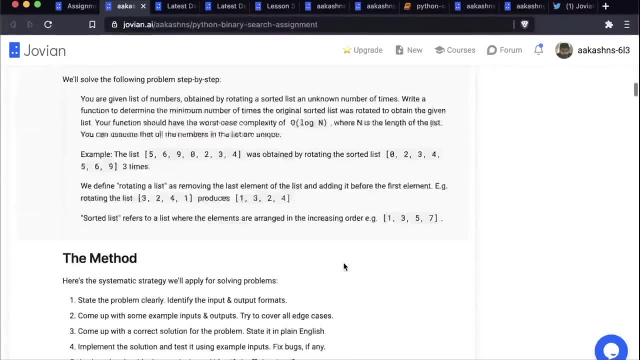 So there is a starter notebook with each assignment and in the assignment all you need to do is run the notebook so you can run it on binder, for instance. And then there is a question mark in a bunch of places. You will find like question marks here in the text and you will find question marks here in. 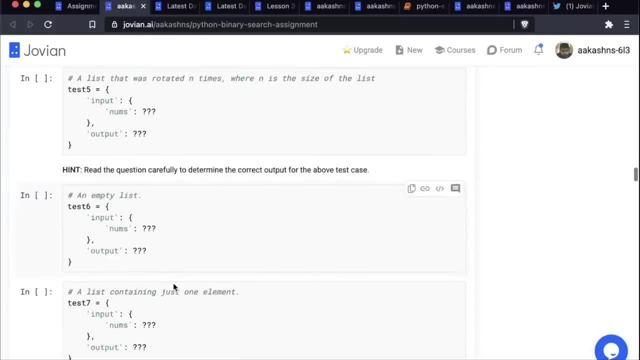 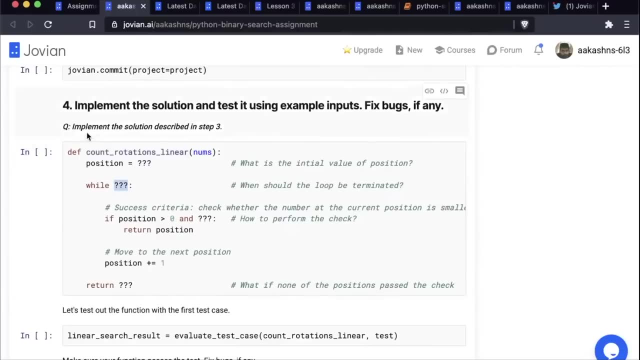 the code. So you simply need to put in your code, your answers into the question marks. So replace that with your code. You can see here there are some question marks here, So you replace that and step-by-step there there are instructions to guide you. 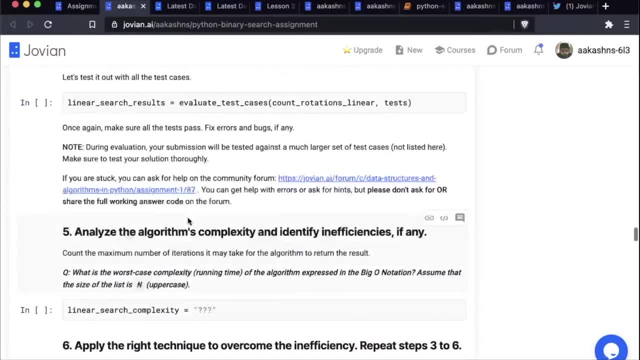 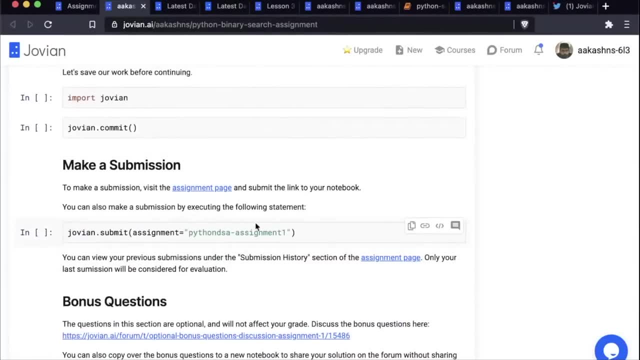 There is, there are comments to guide you, So, step-by-step, you can solve it And then, finally, you can also make a submission. So, right at the very end when you run the code, you will also be able to submit directly. 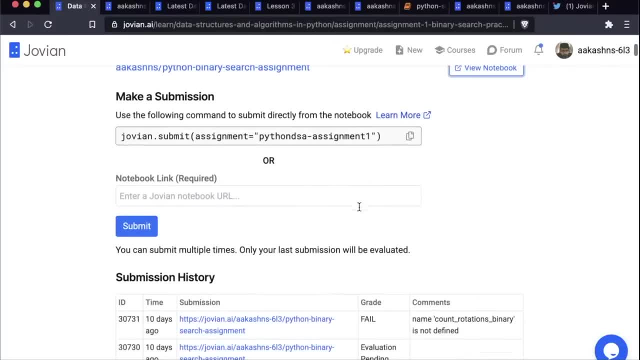 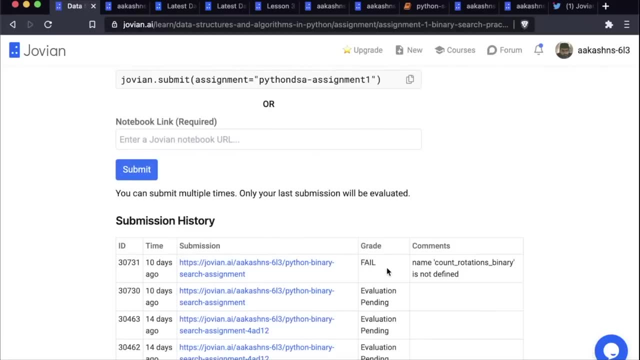 And when you make a submission, then the assignment will get automated, will get evaluated in an automated fashion instantly And you will get a pass or a fail grade. Now, if you get a pass grade, that's great, But if you get a fail grade, then you will also get some comments about what went wrong. 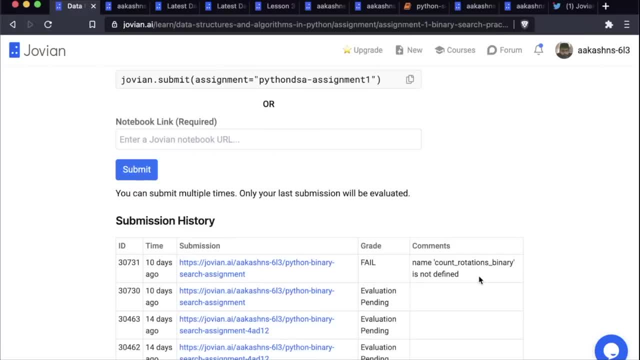 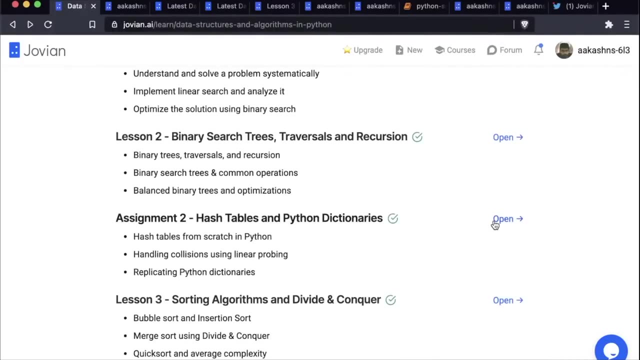 in your solution So you can use those comments to fix the issues. So it's a great way to get quick feedback and keep fixing your issues and especially watch out for edge cases. So that's assignment one And then assignment two. It's called hash tables and Python dictionaries, a very interesting assignment where you are. 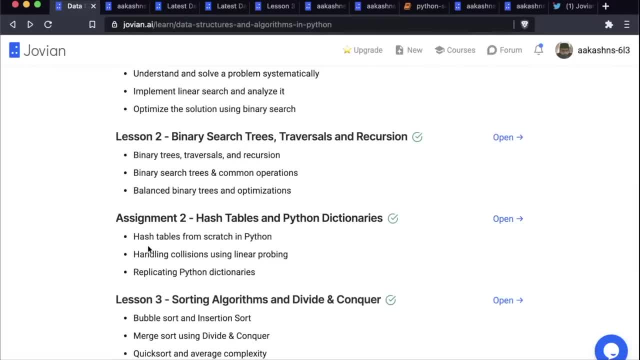 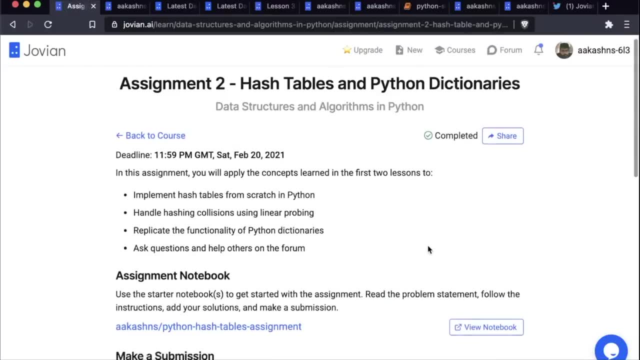 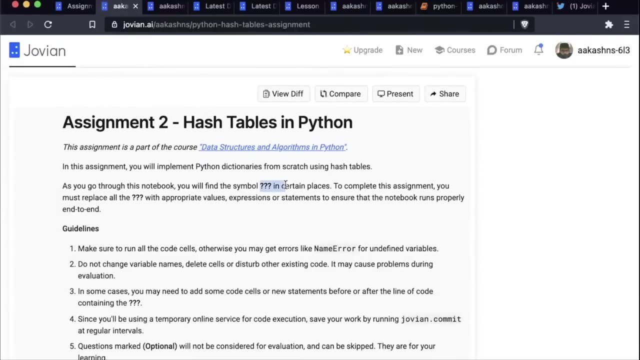 going to implement hash tables which power Python dictionaries from scratch in Python, And you will also replicate the interface of Python dictionaries, So do check it out. a very interesting assignment. again very similar format. You will find question marks in certain places. 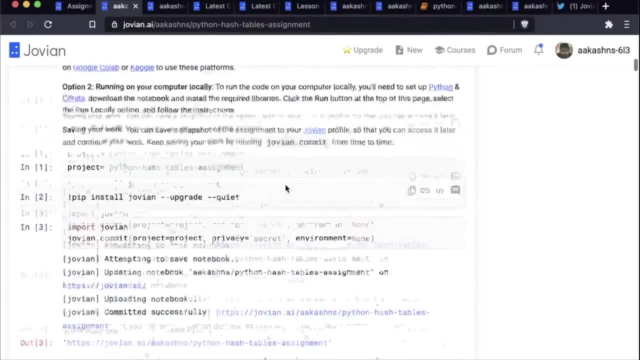 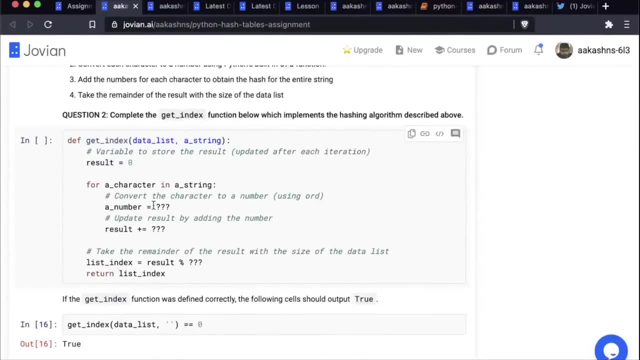 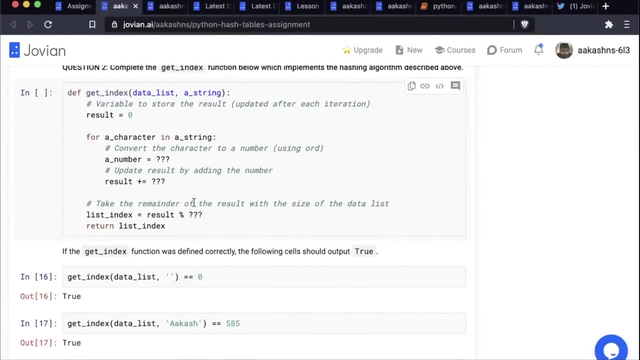 You need to replace them with appropriate values, expressions or statements And in this way, By working through each of these Step-by-step, you can see here, by working through each of these, you will implement hash functions and hash tables, which, again, are very commonly asked in interviews as well. 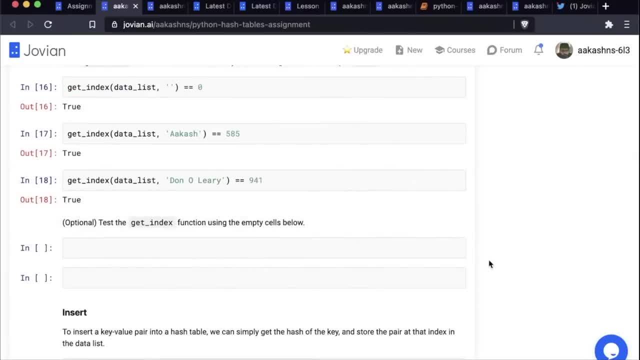 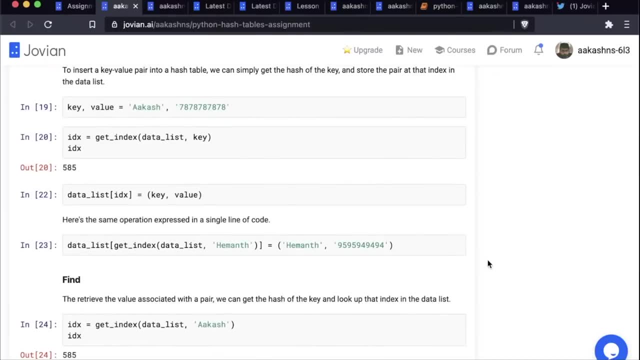 So this is an important assignment for for from an interview preparation or coding assessment preparation as well, And it also teaches you a lot of really good practices in Python programming in particular. So, dude, check out assignment two as well, and we will send you an email as soon as assignment. 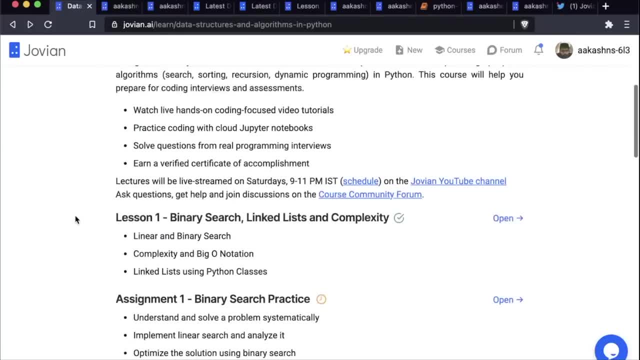 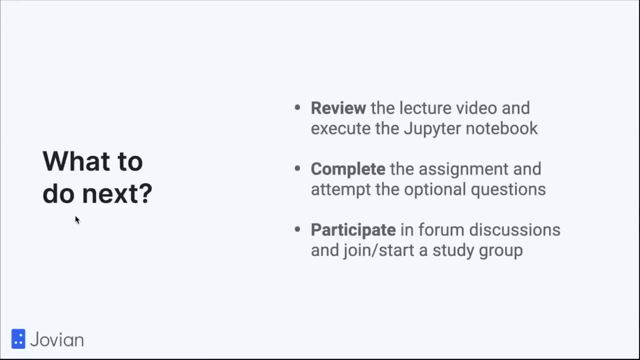 three is ready. check back in a couple of days and you should see it on the same page: python- DSAcom. So what do you do next? Review the lecture video and execute the Jupiter notebook. use the interactive nature of Jupiter to experiment with the code, complete the assignment and attempt the optional questions. 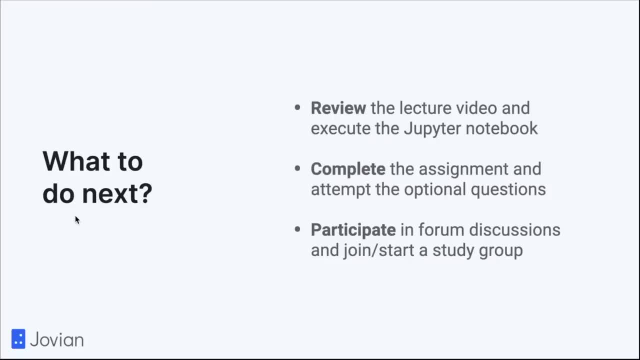 as well. So each assignment has some required questions and you can make a submission as soon as you're done with the required questions. But there are some optional questions which are slightly harder. but I highly recommend doing that because they will improve your understanding, give you more practice, help. 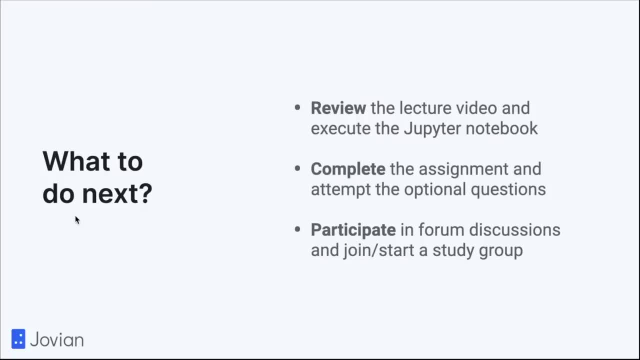 you internalize the concepts better and then participate in forum discussions and join or start a study group. So this is a great way to learn. get together with some friends, maybe watch the lecture together over a zoom call. pause the video. have discussions wherever you have doubts. 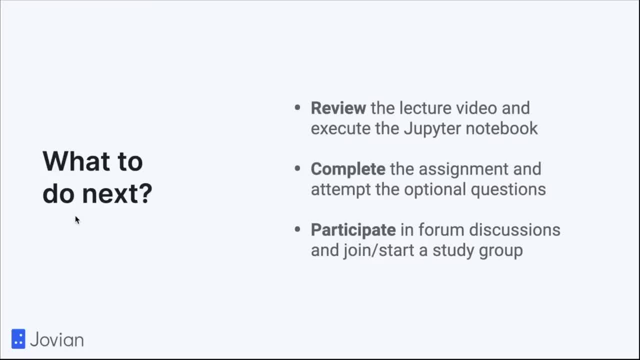 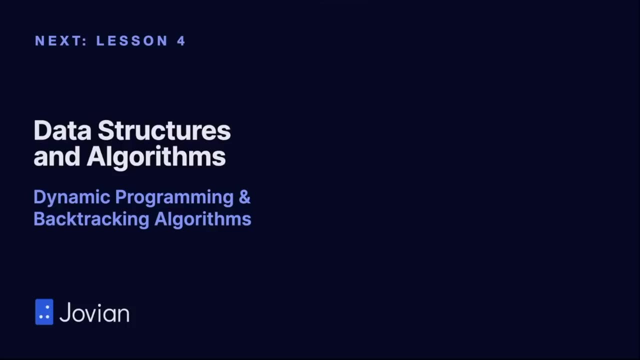 Discussion is a great way to solve the specific doubts that you may have, and it will also help you to articulate Your understanding better, because you, when you explain to others, you also answer a lot of your own questions, So please do that. This is data structures and algorithms in Python. 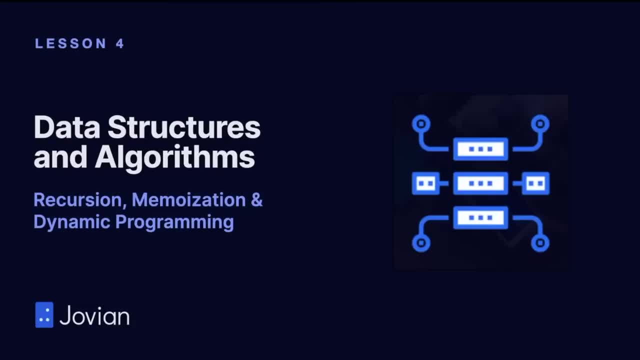 Thank you And good day or good night. Hello and welcome to data structures and algorithms in Python. This is a live online certification course being organized by Jovian. Today we are on a course. Today we are on lesson four: recursion, memorization and dynamic programming. 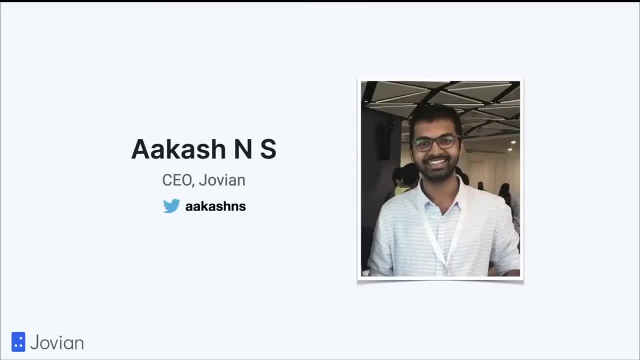 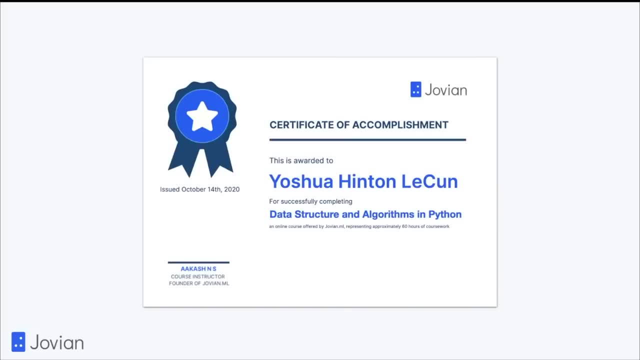 My name is Akash and I'm your instructor. You can find me on Twitter on at AkashNS. If you follow along with this course and complete the weekly assignments, you can also earn a certificate of accomplishment which you can add to your LinkedIn profile and you will. 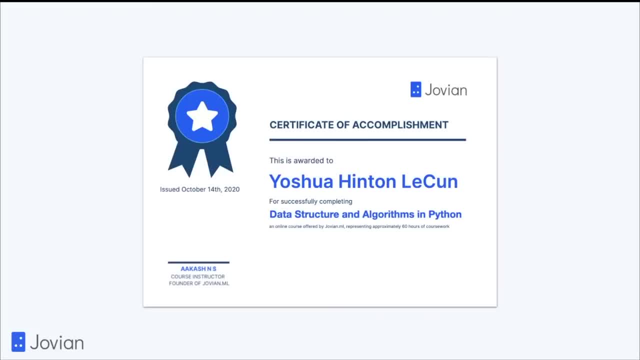 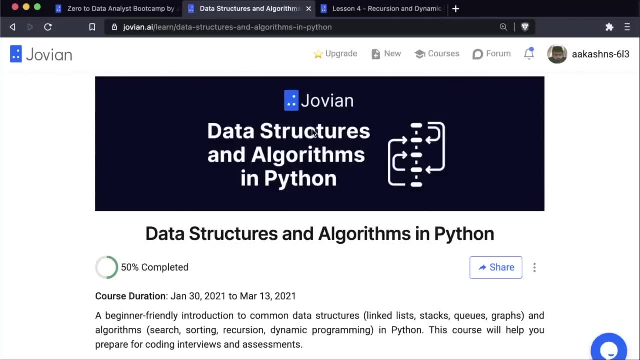 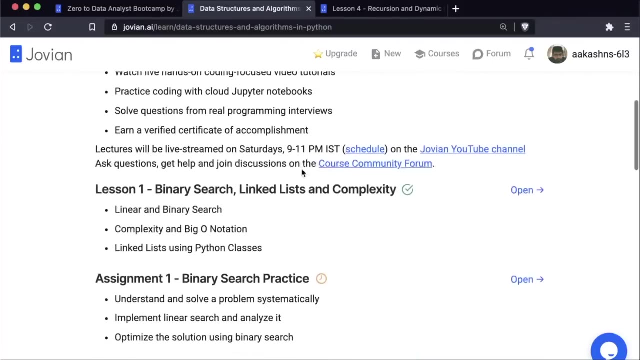 find hosted on your Jovian profile as well. So let's get started Now to the data structures and algorithms course. this is pythondsacom is the course website, and on the course website you will be able to find all the information about. 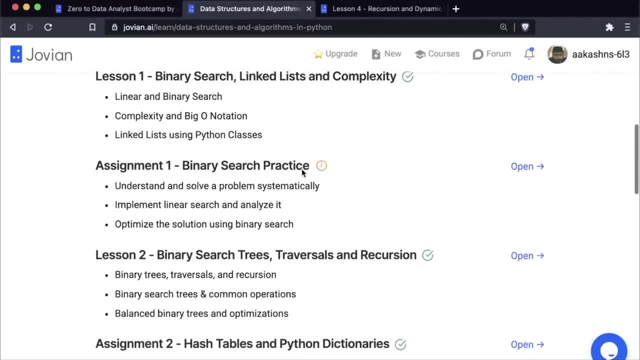 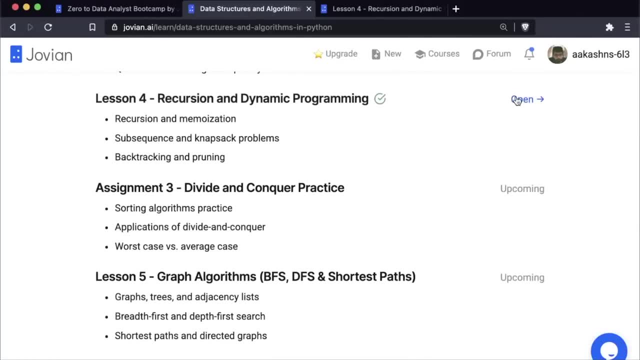 the course. So you can view the previous lessons- lessons one, two and three- and you can also view the previous assignments, assignments one and two. today we're on lesson four, So let's open up lesson four. The topic is recursion and dynamic programming. 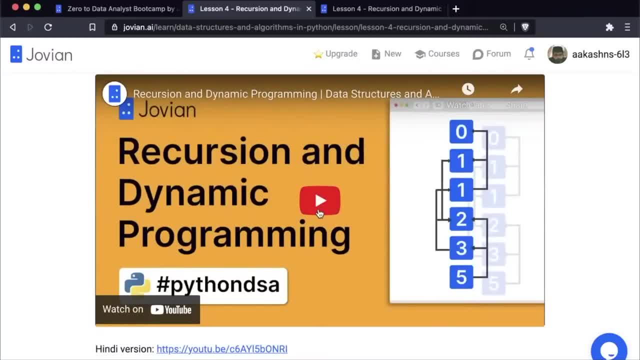 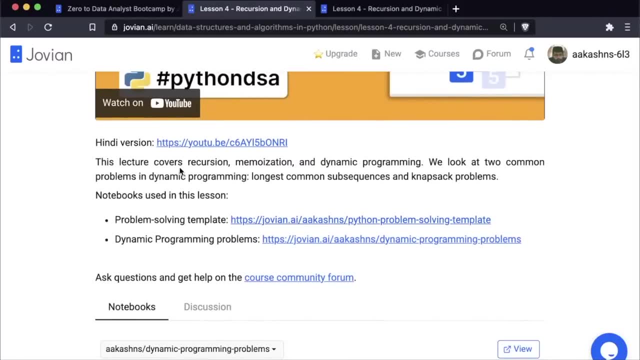 Okay, Okay, Okay, So we have a lesson here and you can also watch a version in Hindi, If you would prefer that in this lecture we will cover recursion, memorization and dynamic programming, by looking at two common problems in dynamic programming the longest 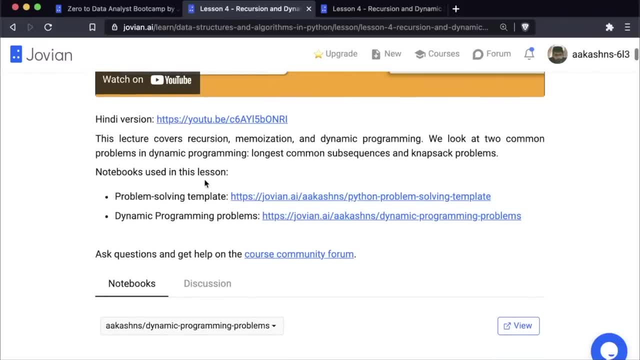 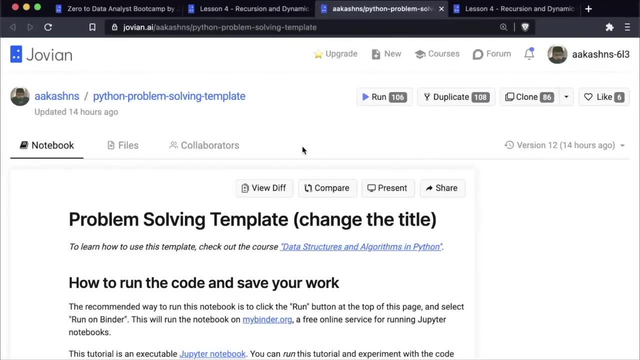 common subsequent problem and then the knapsack problem, And we'll do this by coding these problems live using the problem solving template that we have been using one in one way or another since lesson one. So let's open up the problem solving template. this is a template that you can use to solve. 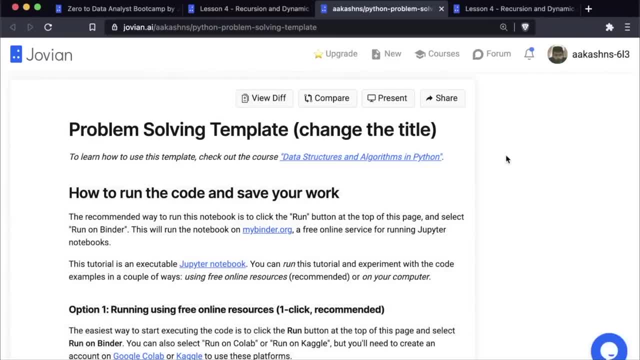 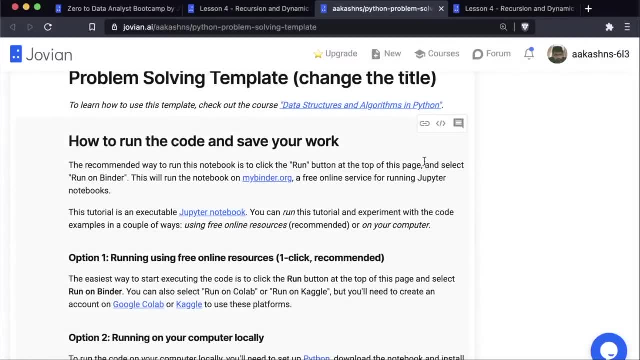 any coding problem, And we will illustrate this by solving two problems using this template today. So the first thing we need to do is to run this template. You can see that there is some explanation, and then there is some code here as well. Now, to run this code, you have two options. 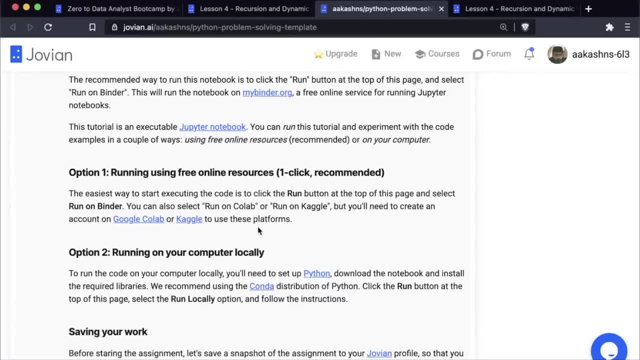 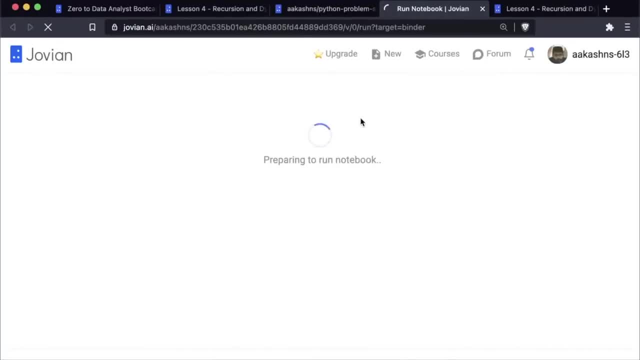 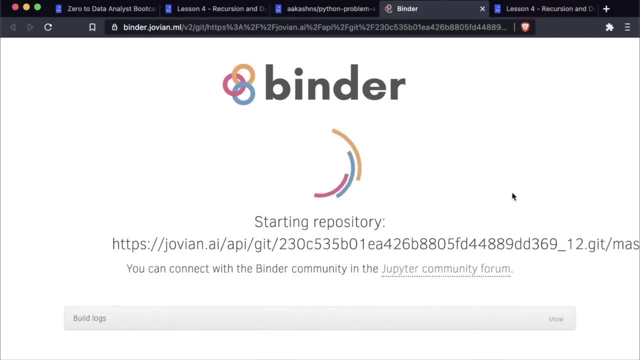 You can run it using free online resources or you can run it on your computer. Okay, The simplest way to run it is click the run button here and select run on binder, And with just one click this will set up a machine on the cloud for you. 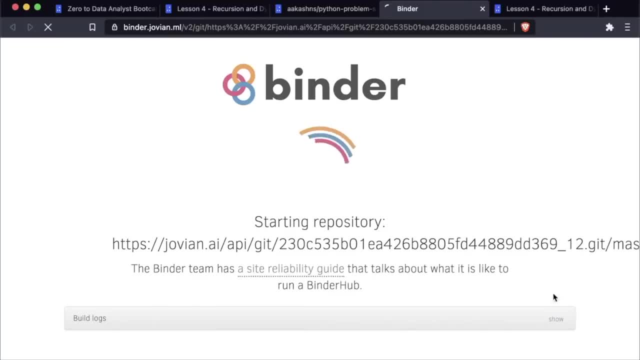 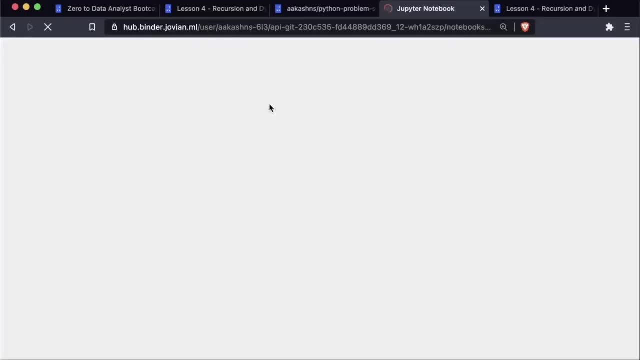 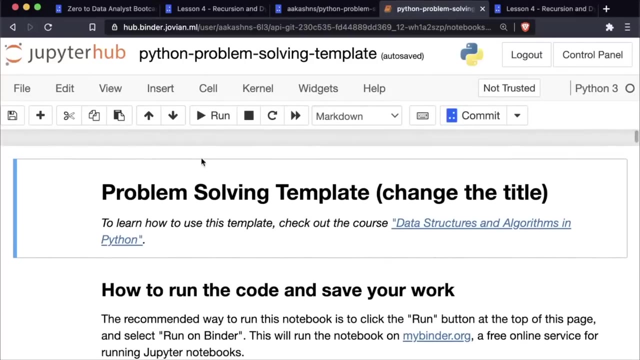 Start a Jupyter notebook server and you will be able to then execute the code and modify the notebook and save a version of it to your own profile so that you can continue working. Okay, So there we have it. Now we have a running Jupyter hub server. 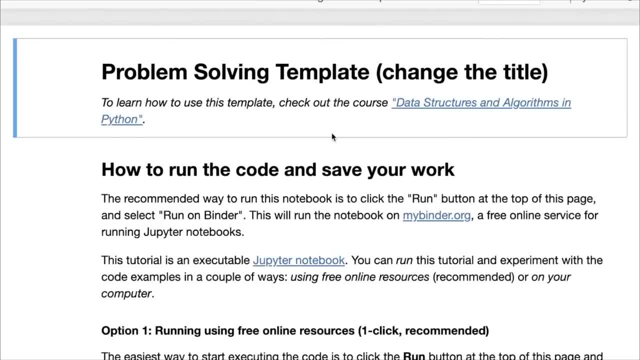 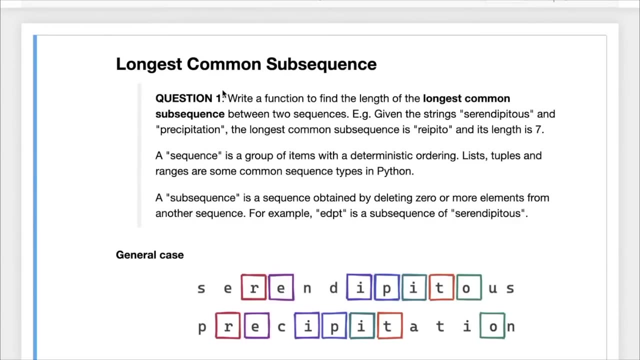 I'm just going to zoom in here a bit so that you can see things clearly. Okay, So this is the problem solving template And I said we're working on two problems, So I have some problem statements listed out here. You can see the first problem, longest common sub sequence, is listed here. 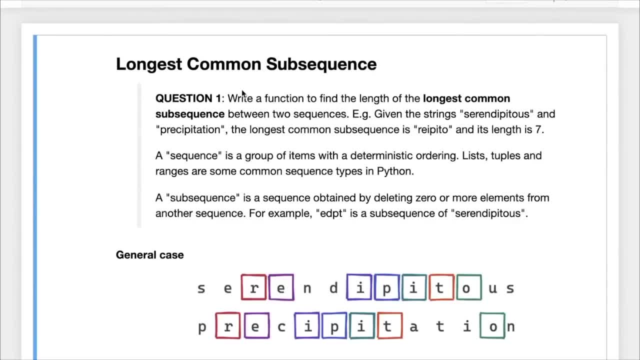 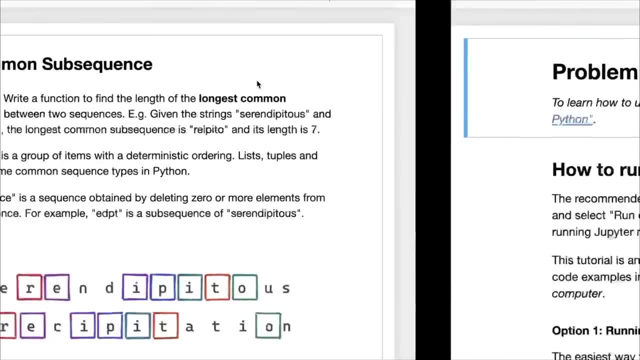 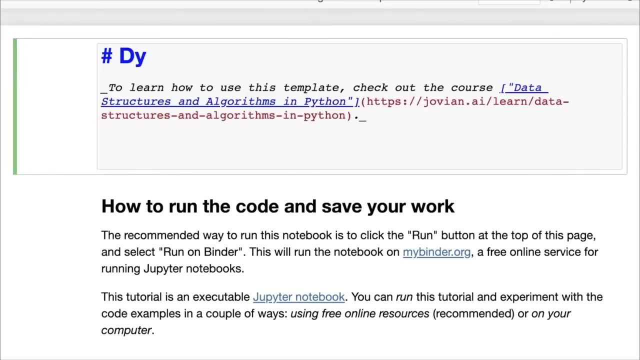 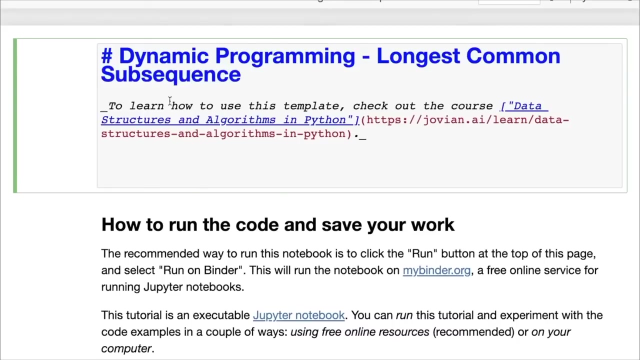 And this is a part of the lesson Notebook Lesson page as well, So you will find link to this problem statement on the lesson page too. So let's first modify the title of this notebook problem solving template. Let's change this title to dynamic programming: longest common sub sequence. 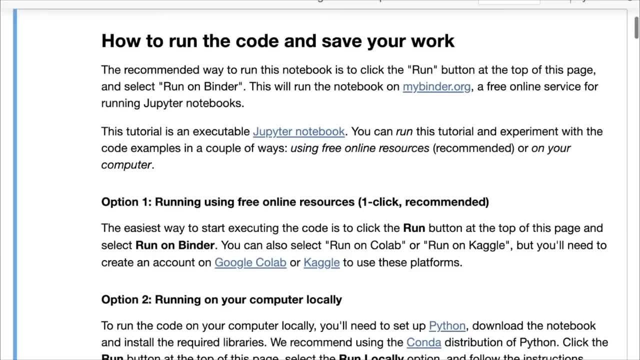 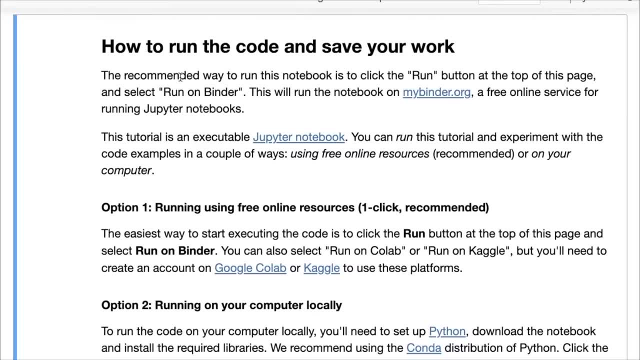 Let's get rid of this. I don't think we need this. Then I'm going to keep the section on how to run Jupyter. Okay, run your code so that if I share this notebook with somebody else, they have a way to run it. 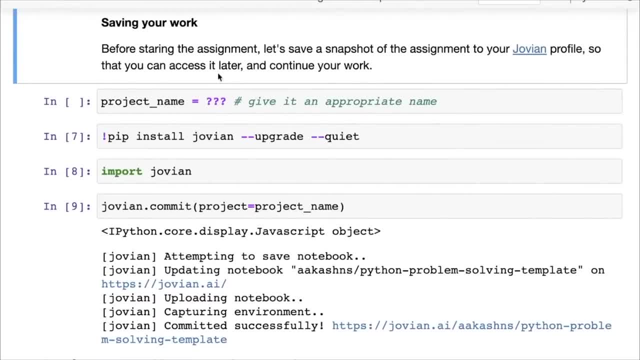 And then, before we start the assignment or the problem, let's just save this to our own profile, So I'm just going to give it a name: Longest common sub sequence- This is an appropriate name for it, So I'm going to give it this: a project name. 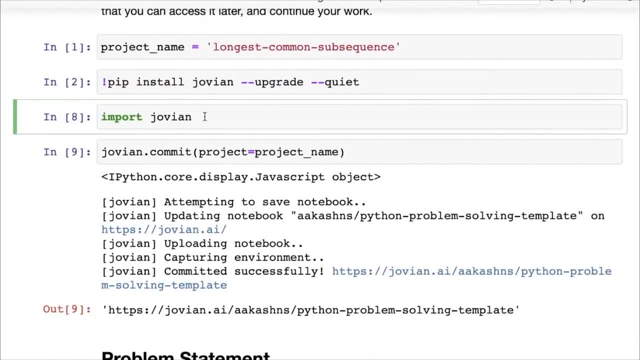 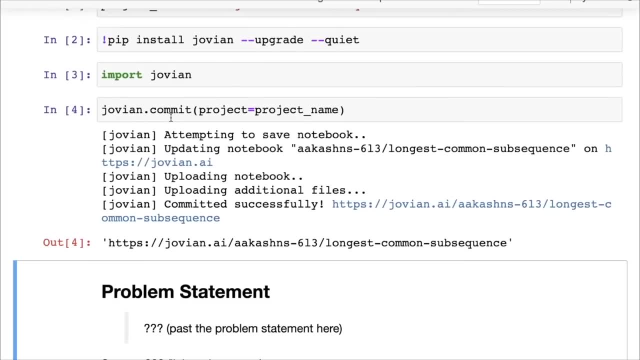 Install the Jovian Python library and just run Joviancom it. Now, what this will do is we started out with a template and now we're editing the template by running Joviancom it. We've saved a copy of the template to our own profile. 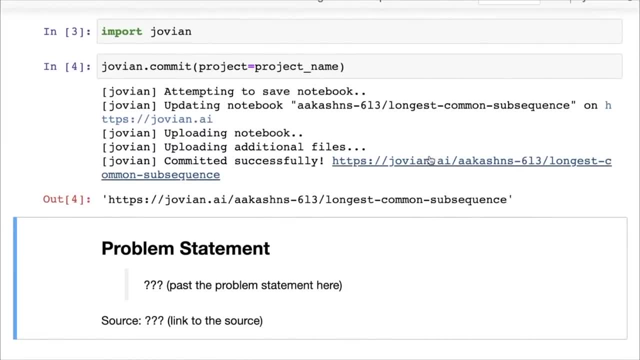 You can see, this is the link where you will be able to access this notebook and you can run it and continue your work If this Jupiter notebook shuts down, if you want to continue tomorrow, for instance? Okay, So now let's look at the problem statement. 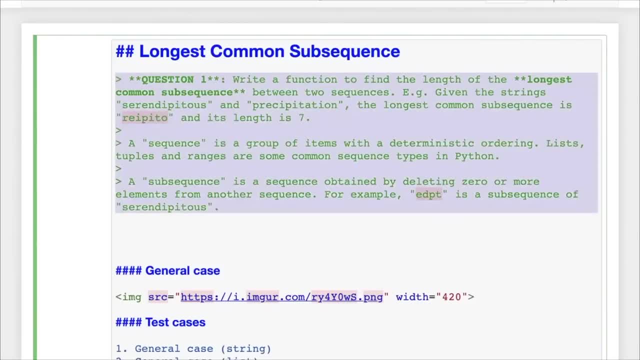 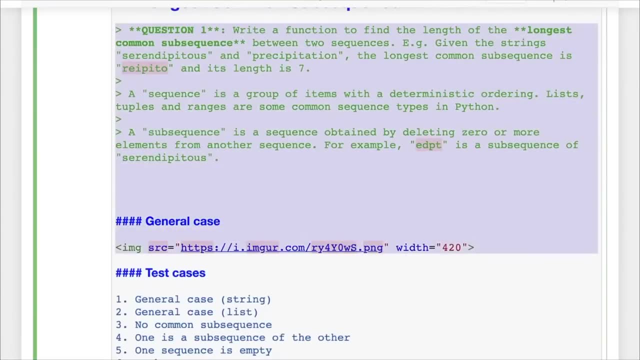 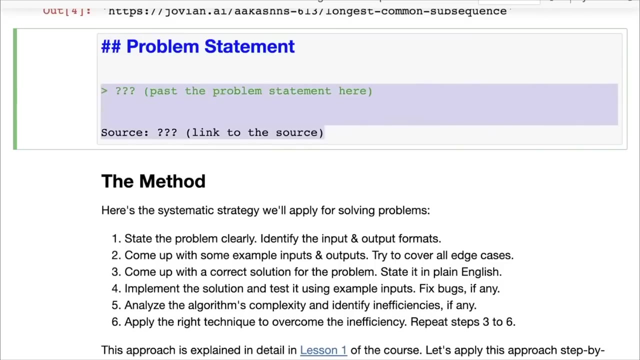 Now I'll just copy over the problem statement here as well, so that we can see it directly within the notebook. There we have it. Now you can paste the problem statement, And if you are getting this from statement from some other source, then it's always a good idea to include the link to the original source as well. 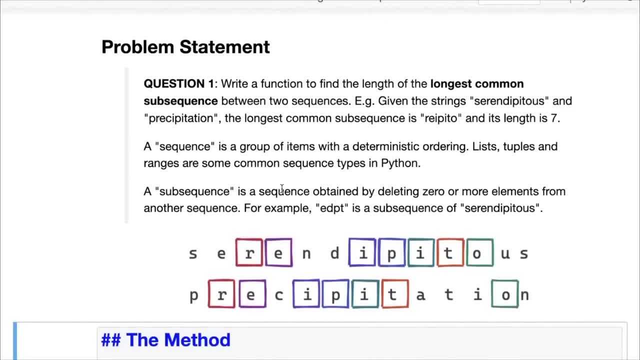 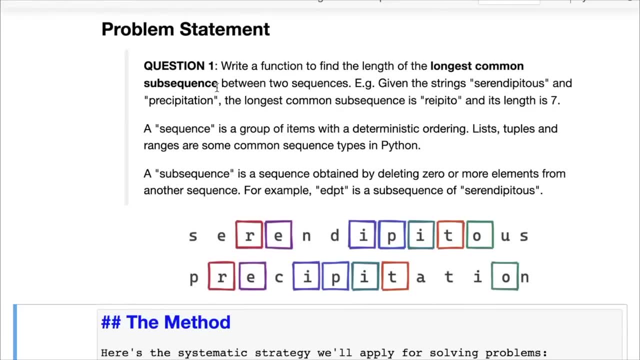 Okay, Now we have a problem statement In front of us. So the question is: write a function to find the length of the longest common subsequence. So that's a new term. We'll unpack that between two sequences. Now let's first learn what we mean by a sequence. 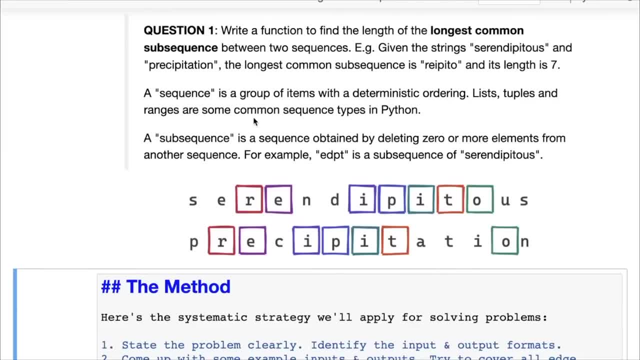 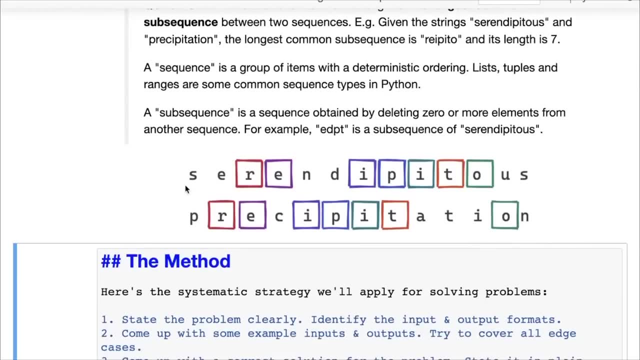 Now, a sequence is a group of items with a deterministic ordering, for instance a list, a tuple, a range or even a string. These are some common sequence types in Python. So here I have the string serendipitous. This is a group of items. 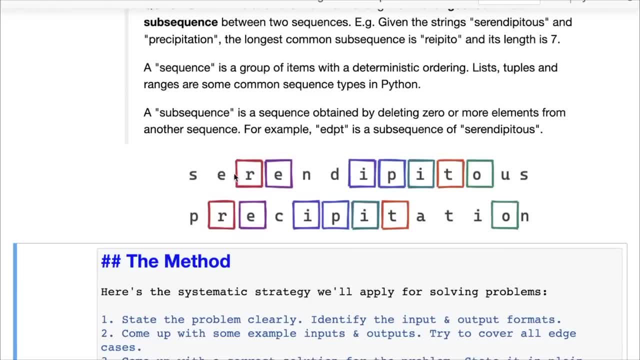 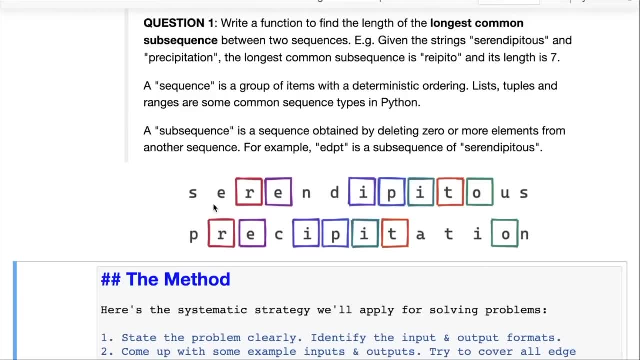 And this also contains an order. You can see that E comes after S and R comes after E, and so on. So this is a sequence. A list would also be a sequence. So that would be a list of numbers. That's a sequence. 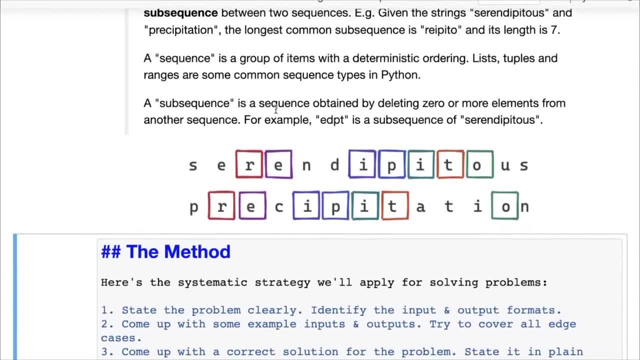 Then we're looking at sub sequence. What is the sub sequence? Now, a sub sequence is a sequence that is obtained by deleting or removing zero or more elements from another sequence. For instance, if you look at serendipitous and if we remove the characters S, 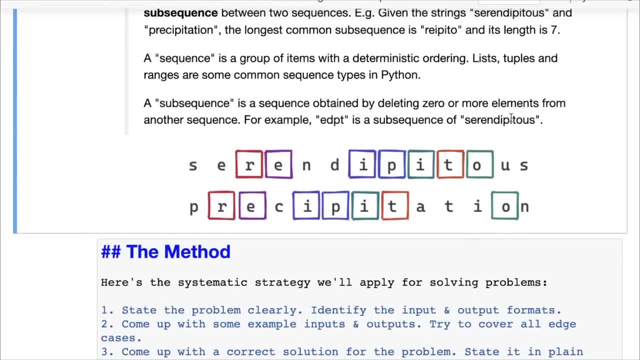 R E N I I O U S. then you will be left with E D P T. So EDPT is a sub sequence of serendipitous. Now two things to note here. EDPT does not have to occur continuously. 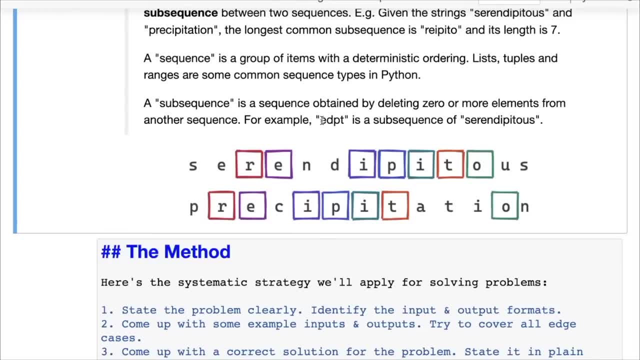 So these elements can occur anywhere within sequence, but the order should be the same. So EDPT occur in this particular order here and EDPT should occur in the same order here. So D should occur after E And P should occur after D and T should occur after P. 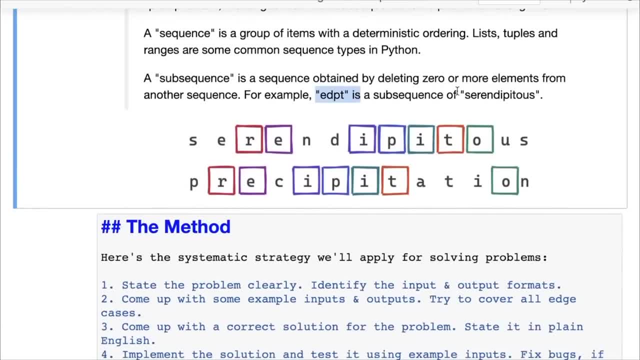 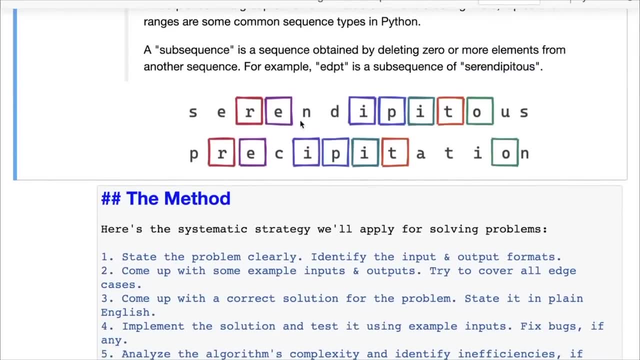 So those are the two requirements for EDPT to be a sub sequence of serendipitous. And, visually speaking, what we can see is if you take a sequence and then you draw boxes around some of these characters or some of these elements of the sequence. 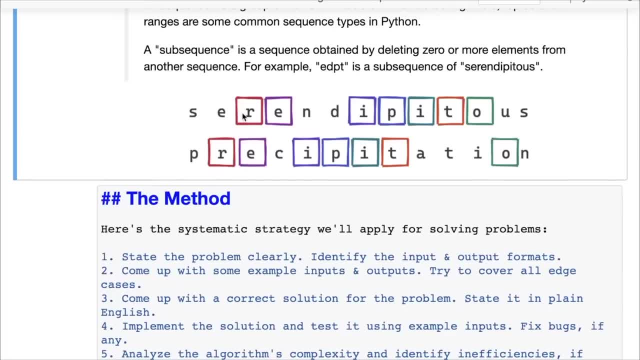 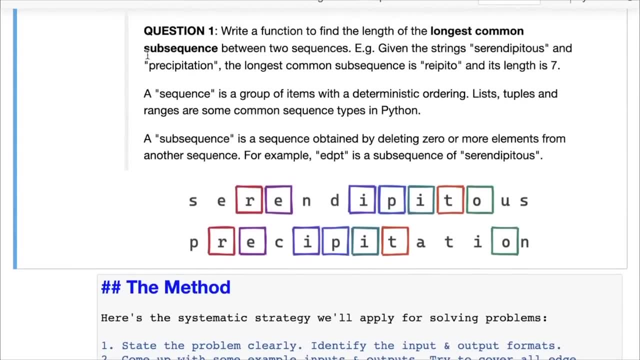 And if you just take the elements in the boxes, then in the same order, then you end up with a sub sequence. So now we understand what a sequence is and what a sub sequence is. And once again, if this, this question, is asked in an interview and you're not sure what you mean by a longest common sub sequence then, or even what a sequence is, then you should ask the interviewer: what do you mean by a sub sequence? 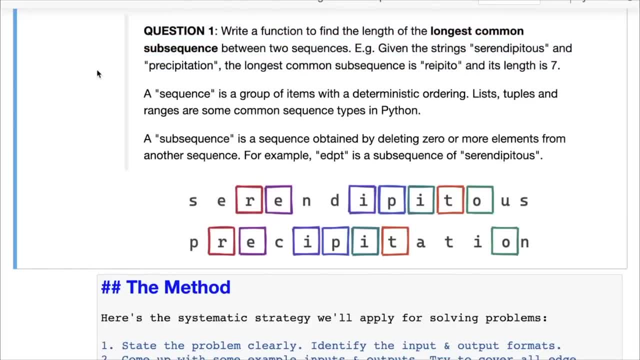 Or what do you mean by sequence, And they'll be more than happy to tell you. It's very important to communicate, whatever you're thinking, whatever questions you have. contrary to what you might think, asking questions is actually a good thing. The more questions you ask, the more it is appreciated. 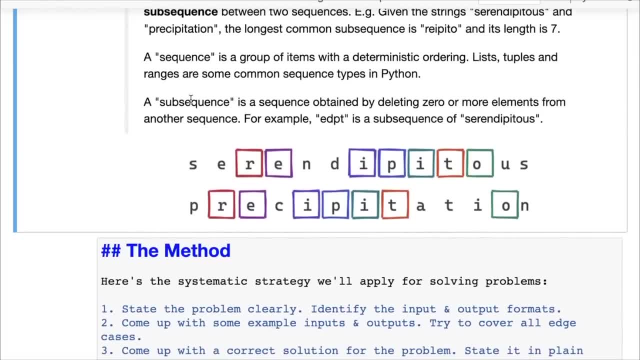 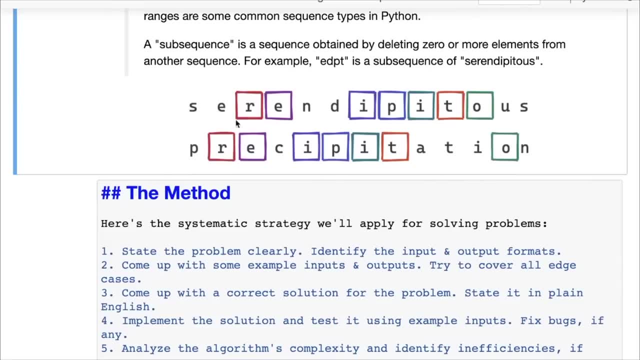 Okay, So now we've talked about a sequence, Uh uh- and a sub sequence. Now, what's a common sub sequence? So let's look at these two strings: serendipitous and precipitation. Now, if we pick just these elements that are in the boxes, R E I, P I T O. 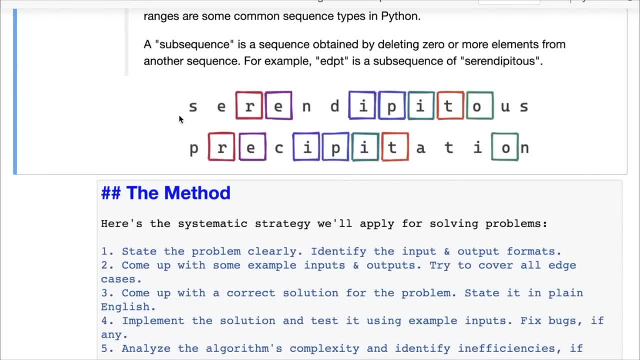 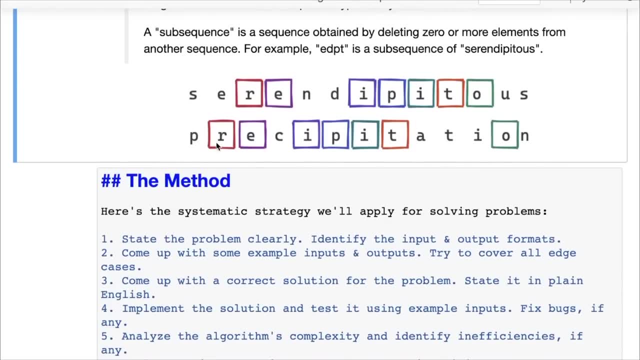 Now you can see that R E I P I T? O is a sub sequence of serendipitous and R E I P I T? O is also a sub sequence of precipitation. So a sub sequence up which is common, Which is a sub sequence of both sequences, is called a common sub sequence. 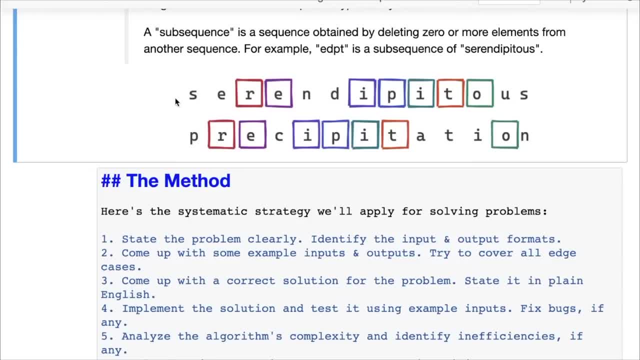 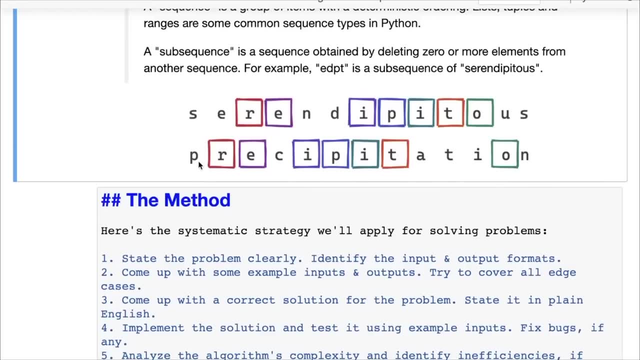 So R? E I P I T? O is a common sub sequence between serendipitous and precipitation. Now you can have many common sub sequences. For instance, we could just look at R? E and R? E here, and R? E would be a common sub sequence too. 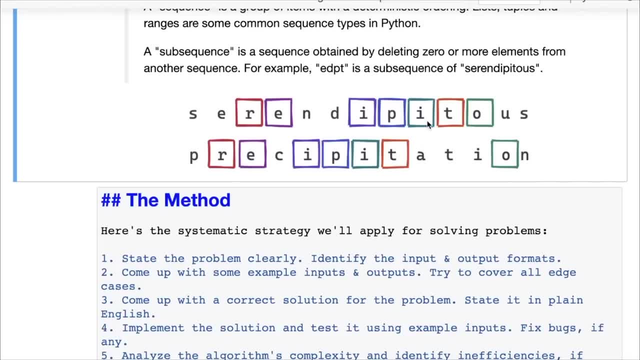 Or you could just look at it and it, and that would be a common sub sequence as well. or we've not picked N here, but you could also pick R E N and R E N, And that would also be a common sub sequence between the two. 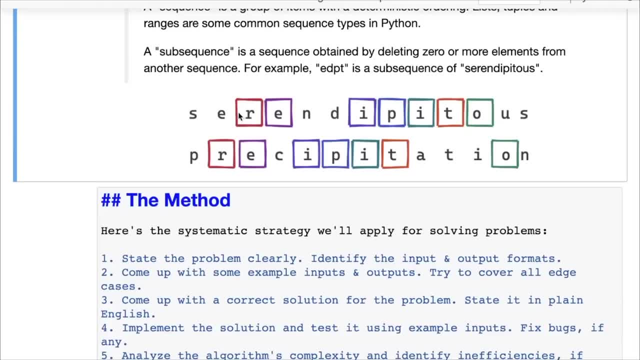 Now, the longest common sub sequence, as the name suggests, is the sub sequence which, between the common sub sequence between the two sequences, which has the maximum possible length, And you can verify this. You can try different sub sequences and see that R E I P I T O is the longest common sub sequence between these two strings, these two sequences. 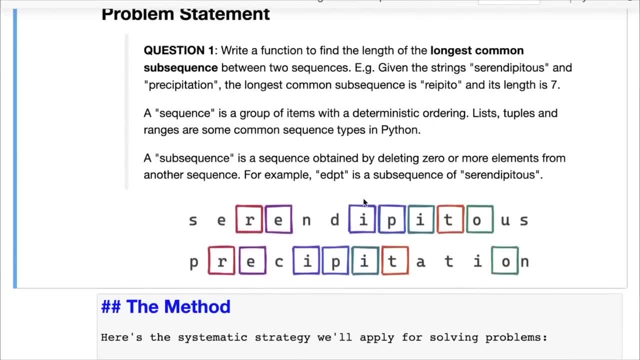 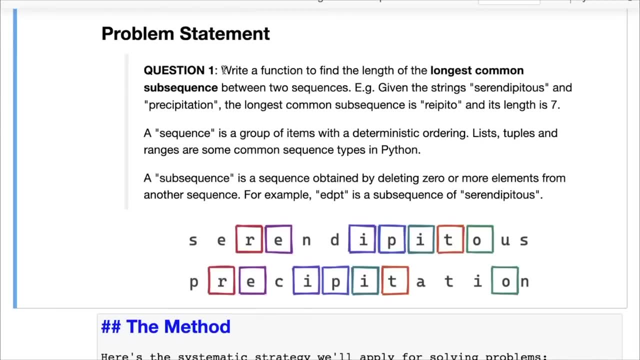 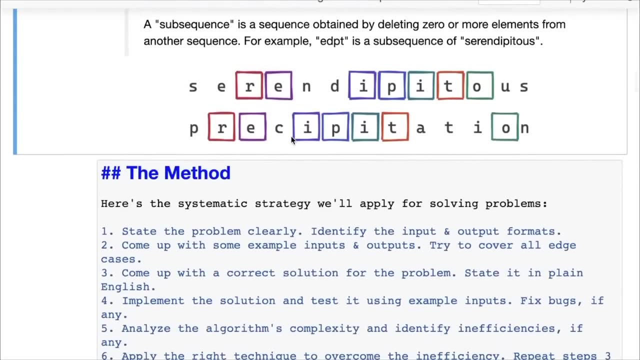 And it's length is seven: one, two, three, four, five, six, seven. So you have to write a function to find the length of the longest common sub sequence between two sequences. So that's a question And this is an visual example that tells you the answer. 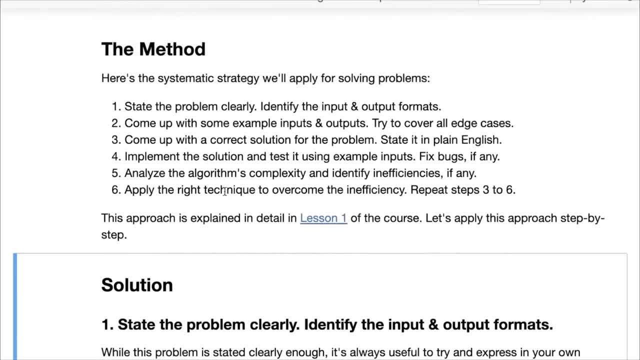 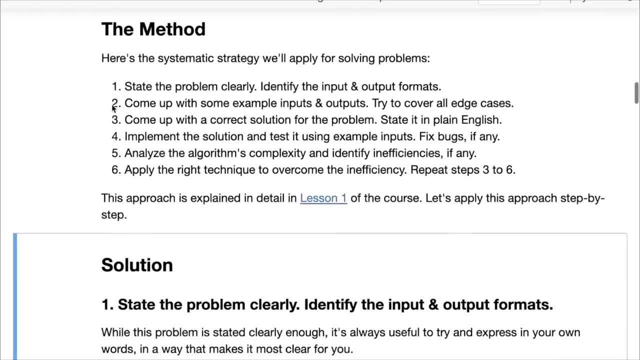 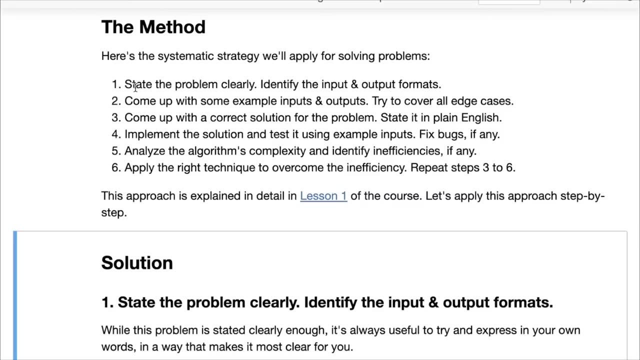 Okay, So now that we have the question, we've understood the question, We can start applying the method that we have been learning throughout. So this is the systematic strategy that we will apply, and nothing About this method has changed since the first lesson, even though we've covered a whole variety of topics like binary search and binary search trees, and then sorting algorithms and divide and conquer. 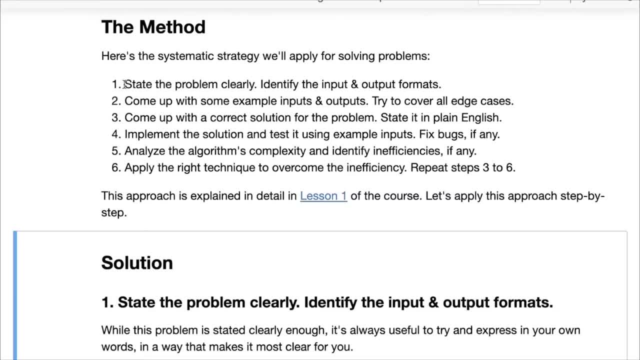 This method has remained the same. The first step is to state the problem clearly and identify the input and output formats. Then the second step is to come up with some example inputs and outputs, and these will be used to test our solution. So we should try and cover all the edge cases. 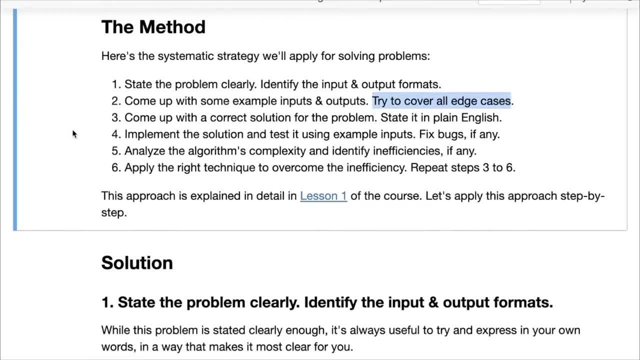 And that will Help us write code that is correct, anticipating all the errors that we might face. Then we come up with the correct solution to the problem and stated in plain English. very important for you to state the problem in plain English before you start coding, so that you communicate your ideas and you also make it clear. 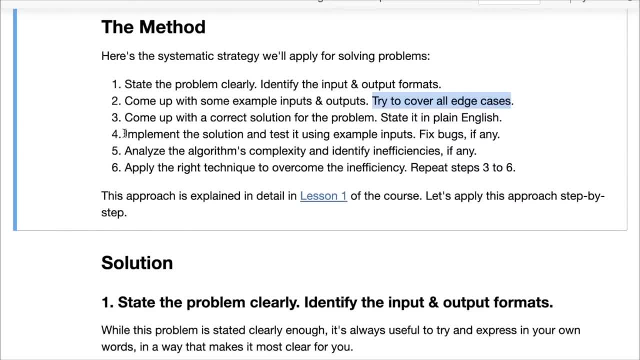 Once you express yourself, then you implement the solution and tested using example inputs and you fix bugs If you find any of them- and you will be able to find bugs If you have Written good test cases- then you analyze the algorithms, complexity and identify inefficiencies. 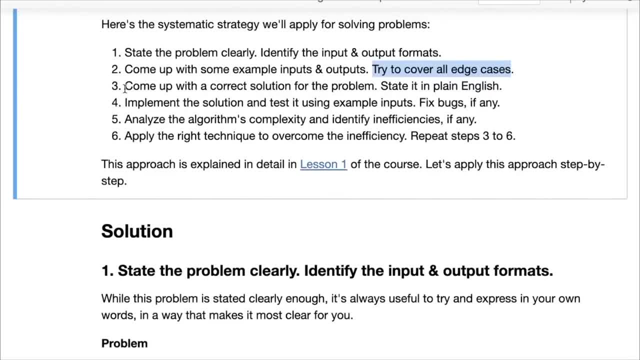 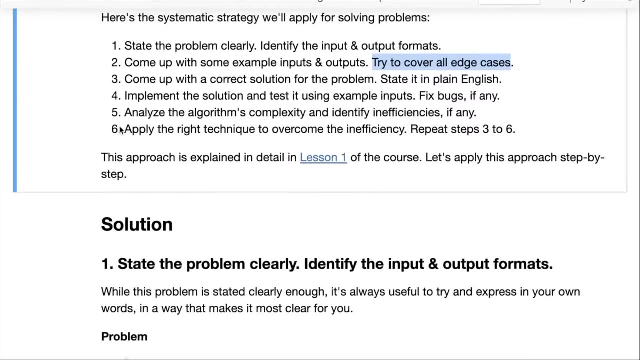 If you have any and most likely the full solution that you come up with. it doesn't have to be optimal, It just has to be correct. So there will be some inefficiency. but it's important to go through that process of first finding a brute force solution and then finding the inefficiency, and then apply the right technique to overcome the inefficiency and repeat steps two, three to six. 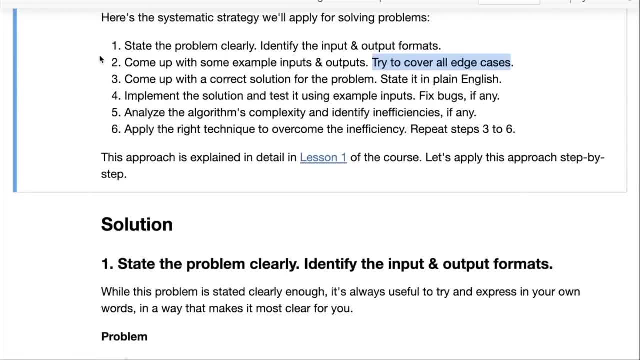 So you identify what's the right technique, And in this case we will learn a couple of Techniques called memorization and dynamic programming, And then we go back and state the correct solution again. Then we implement the solution and test it, and then we analyze it again. 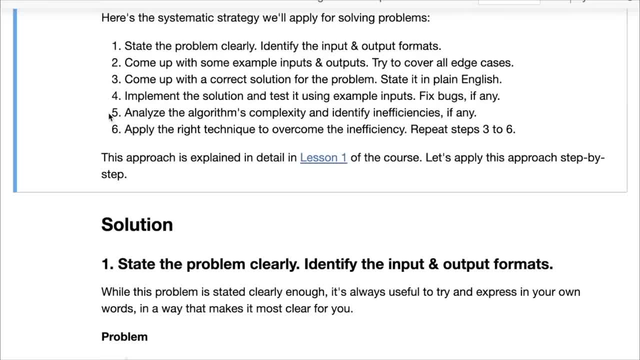 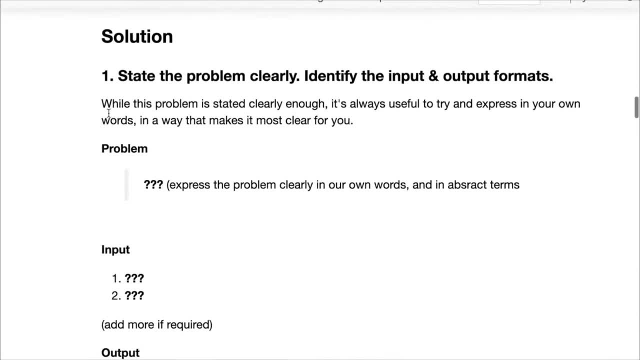 And if there's further scope for improvement, we do that. Otherwise, we say that we've arrived at a optimal or good enough, optimal enough solution. Okay, I hope by this point this you've started to memorize this process, and that's why we keep repeating it over and over, that it should become second nature every time you see a problem. 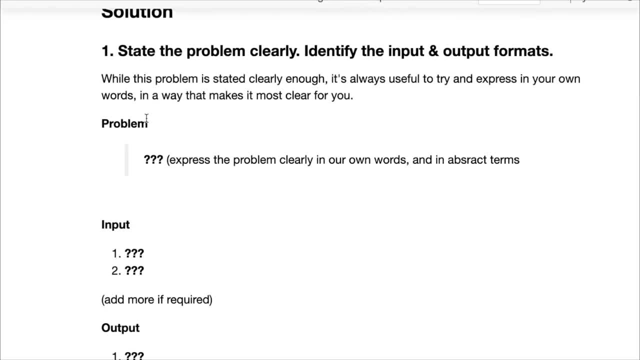 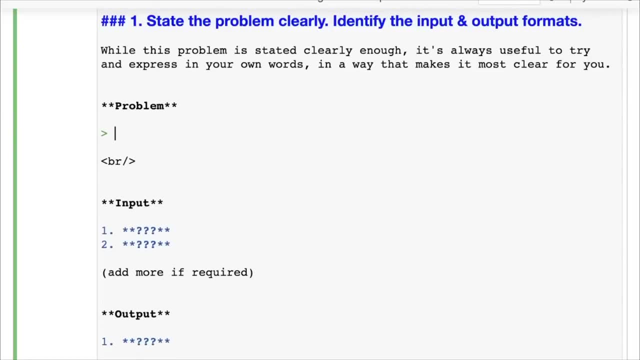 So the first thing is to State the problem clearly and to identify the input and output formats. Now the problem is already stated clearly enough, but let's just state it slightly more clearly. So let's say we are given, and just write it in your own words. 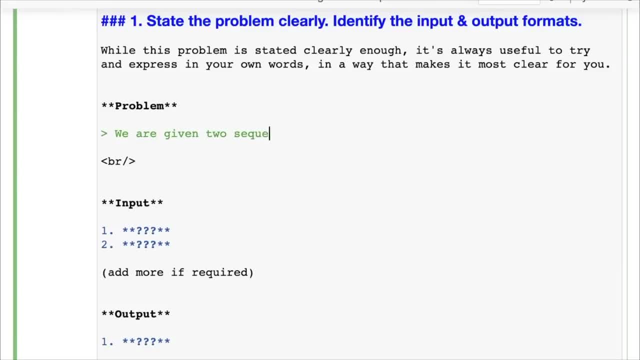 That's more important. What, whatever is clear to you. So we are given two sequences and we need to find the length of the longest common Sub sequence between them. Simple enough. Then we have two inputs. Now we decide the input and output formats. 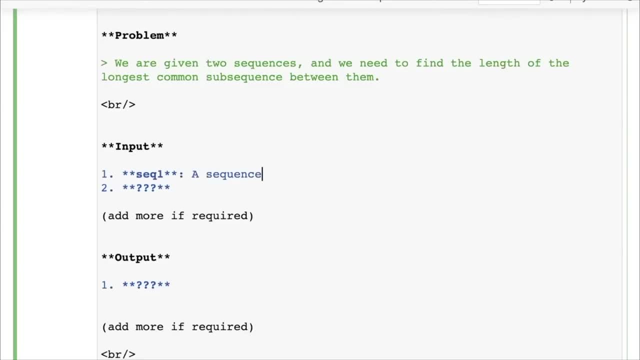 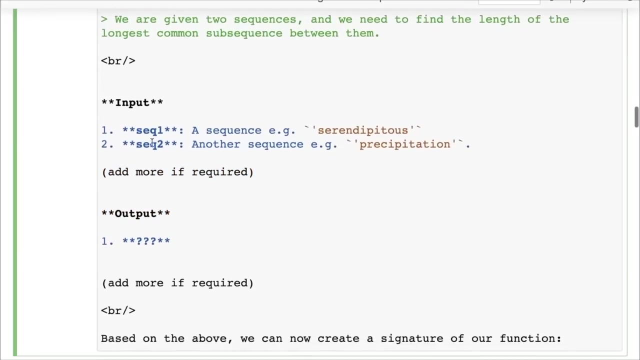 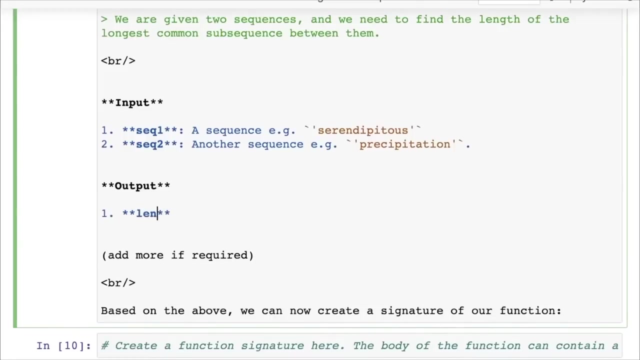 We have sequence one, a sequence example, serendipitous sequence to another sequence example. And then we have: we have two inputs and the output would be the length of the longest common sub sequence. Let's just abbreviate that as LCS. 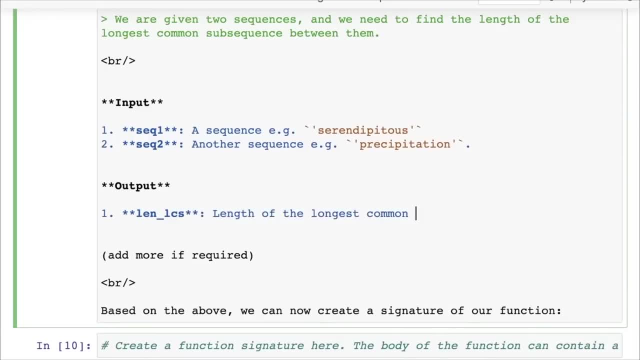 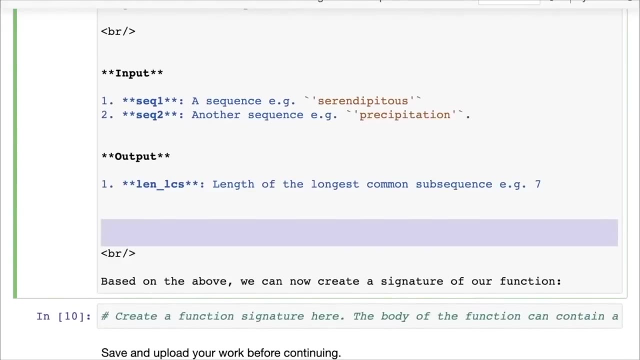 Okay, So we have two inputs and the output would be the length of the longest common sub sequence, Which in this case is seven, and we know what that sub sequence looks like. We've just seen it above. So now, based on this, we can now create and you can see, the problem is now created. 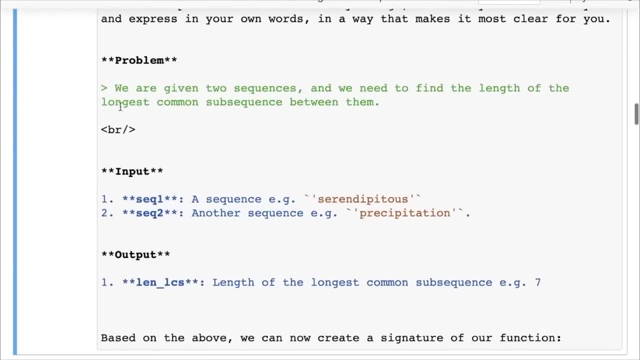 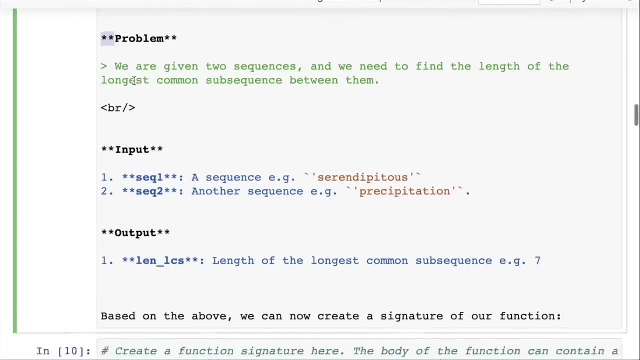 And before I talk about the next thing, if you double click on a textile, you can start editing it, And here we are using a language called Markdown. So you can see, this creates a block code, This creates a bold font And 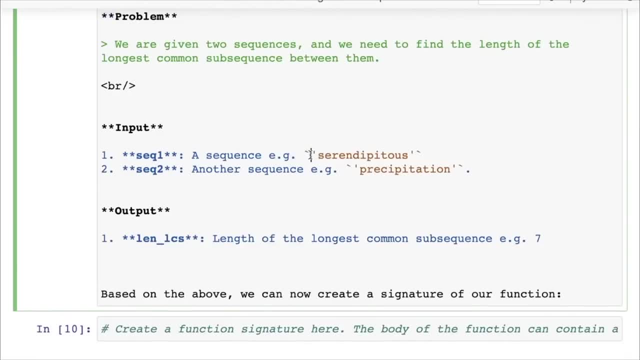 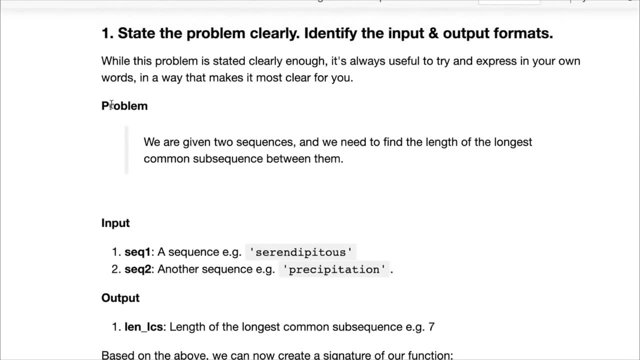 This creates a code like font. So let's see here: And the way to go back into the display mode is to press shift plus enter. So now you can see here that now we have the problem, We have the block code and then we have all the styling. 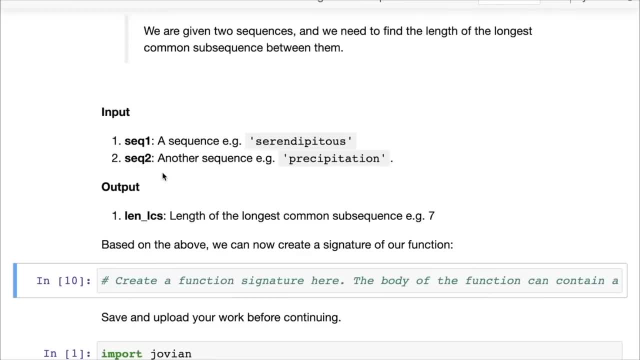 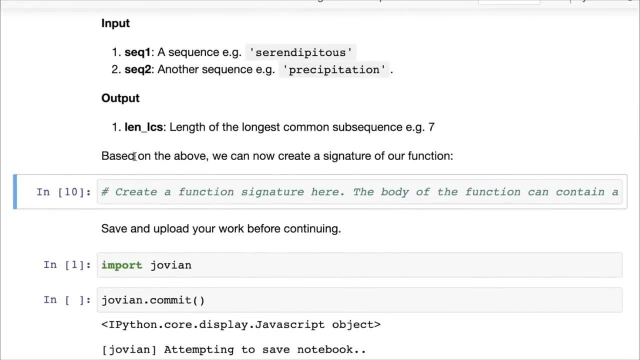 So Markdown is a really useful and easy to learn language for formatting your text, especially in Jupiter notebooks, to do learn it. But now, based on this, we can now create a signature of a function. So our function, Len LCS. We'll accept a sequence, sequence one and sequence two, and it will return something. 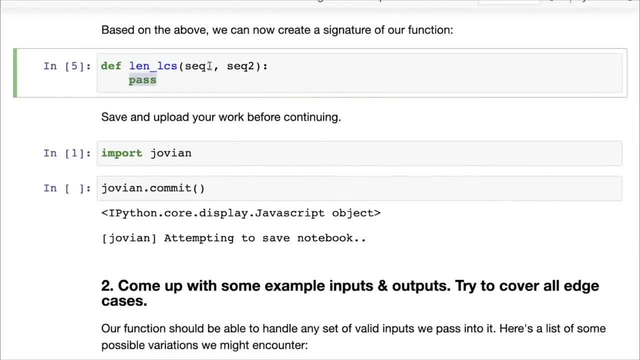 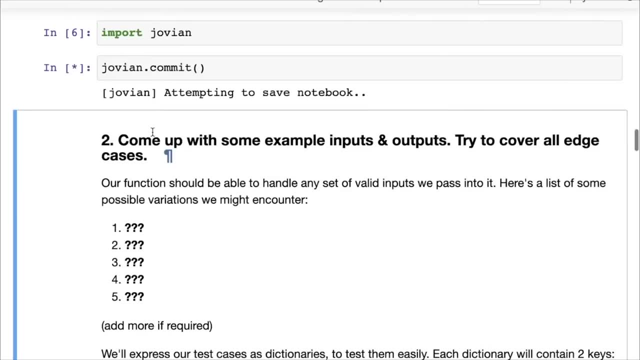 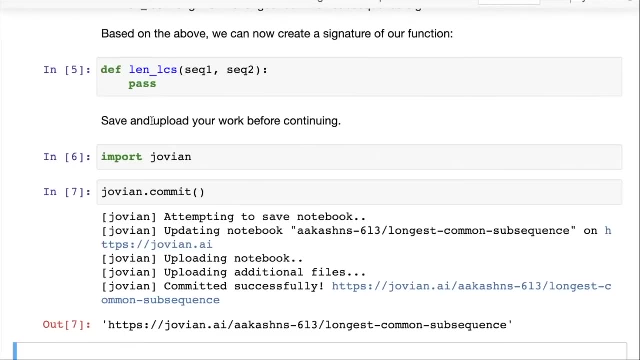 Okay, So that's the basic signature of our function And, even though it's not doing much, just establishing what the arguments are is the first step towards solving a problem, And let's just save our work from time to time. It's very important to keep saving your work on Jovian, because this is running on a free online service. 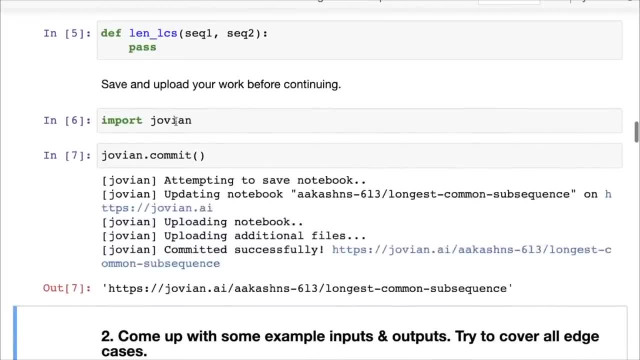 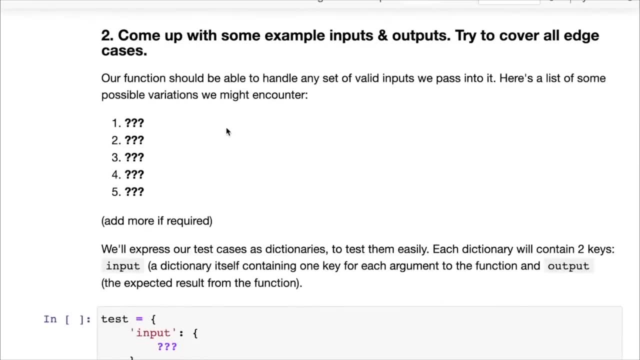 So this will shut down after some minutes of inactivity. So just run Joviancom It And that will save the notebook to your profile and you can read on it. Okay, So then now the next step is to come up with some example- inputs and outputs, and here we need to try and cover all the edge cases. 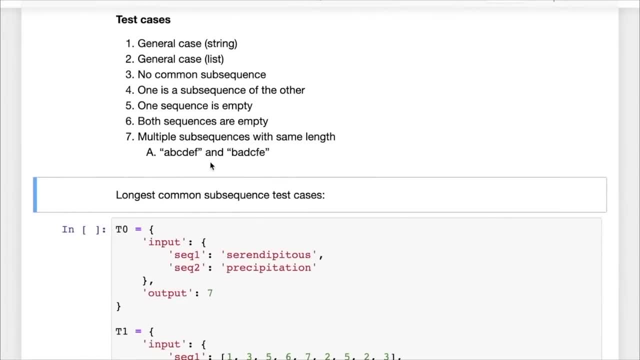 So I have written out a few test cases here already. Now. the most common case is a general case of a string, Like we had serendipitous and precipitation. That's a common case. That is one of them. Both of them have some common elements and there's a subsequent 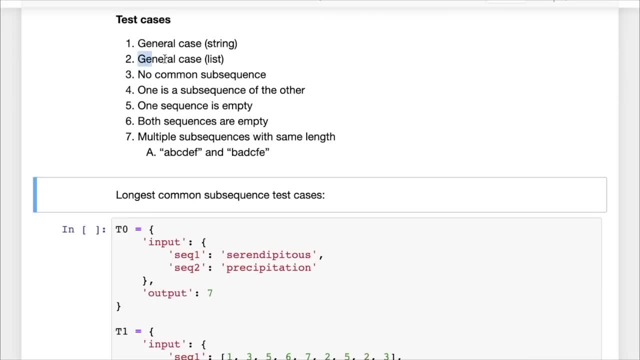 Common subsequence of length seven. but we may also want to test out another type of data- And this is one of the nice things about Python- where you can write functions that operate not just on a particular class and it's subclasses, but on any kind of data, as long as it satisfies certain criteria. for instance, strings and lists both allow indexing into them and picking out the element or the element from the sequence. 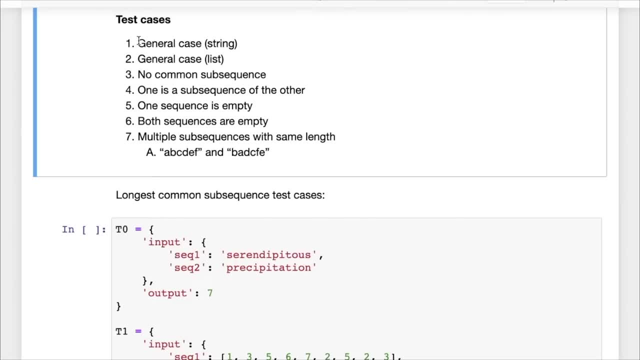 So they're both sequences. So our function should be able to work with both strings And with lists. then here is another case where we have two sequences and they have no common subsequence. A function should not throw an error here. It should gracefully return the number zero, because the empty sequence is a subsequence of every other sequence. 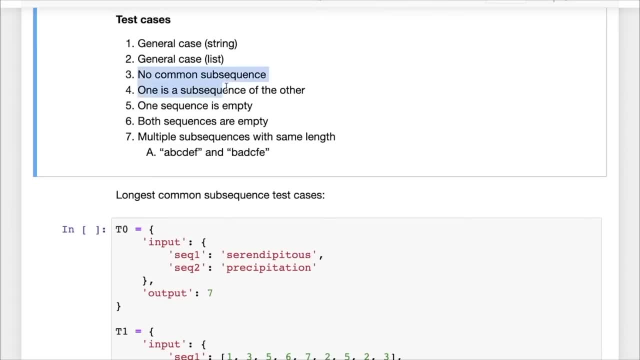 Does that make sense? Think about it. So in that case, if you, if there's no common subsequence, then the empty sequence is the common subsequence. So the answer is zero. And here's one other extreme case where one is a subsequent. 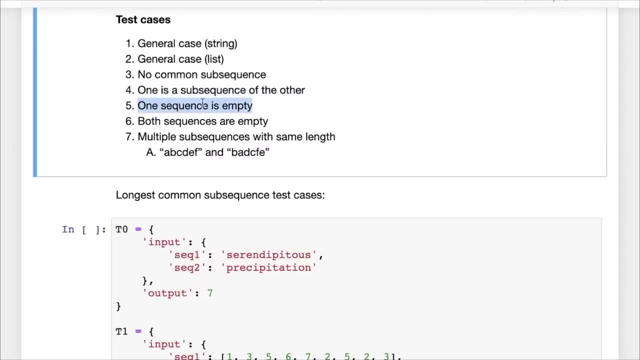 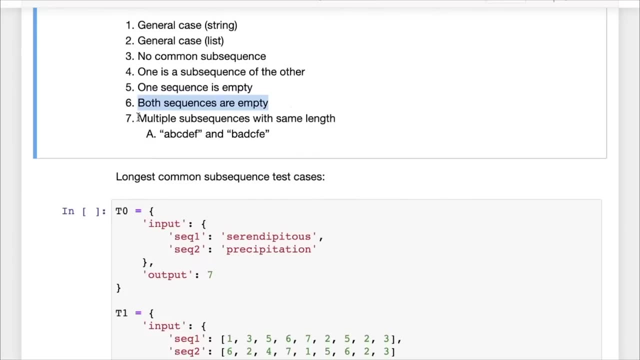 The sequence of the other. here's another case where one sequence is empty. Here's another case where both sequences are empty. All of these are important. Otherwise you might miss out certain special cases and you will face an error when you code your solution. 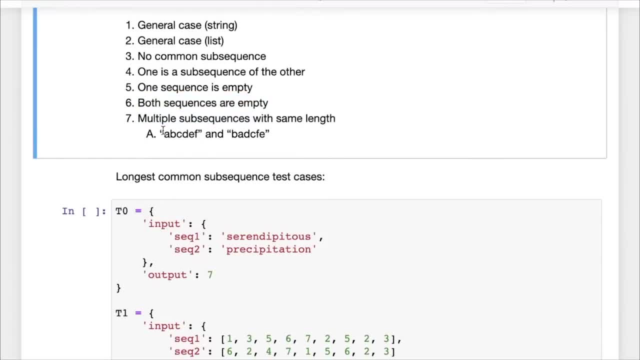 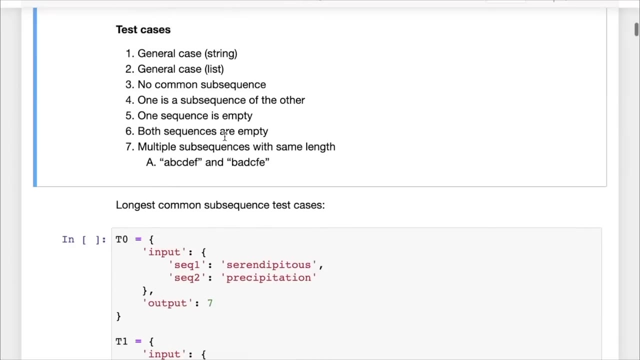 Finally, you can also have this case where you have multiple sub sequences with the same length, For instance, if you have ABCDEF and BADCFE and ACE. ACE is one long subsequence, of length three, and that's the longest, And BDF is another subsequence which is common to the two and also has the same length. 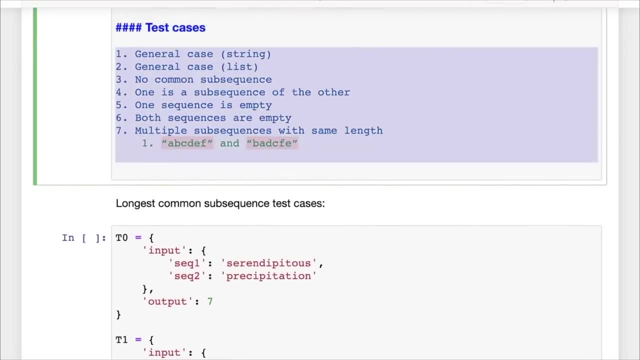 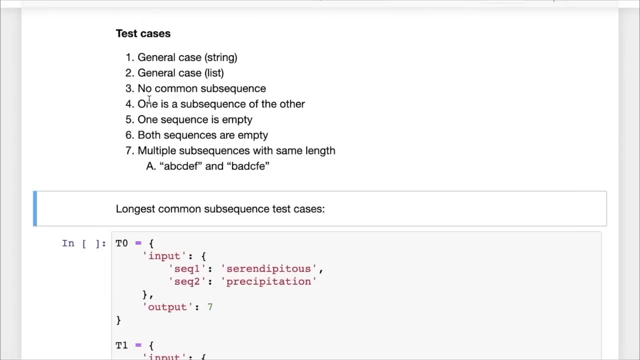 Those are some test cases. Now let's copy over these test cases here in an interview or a coding assessment. What you might want to do is just write these as comments, If you have just a single coding screen, and try to list at least four or five. but go as far as you can, because this will also help you streamline your own solution. 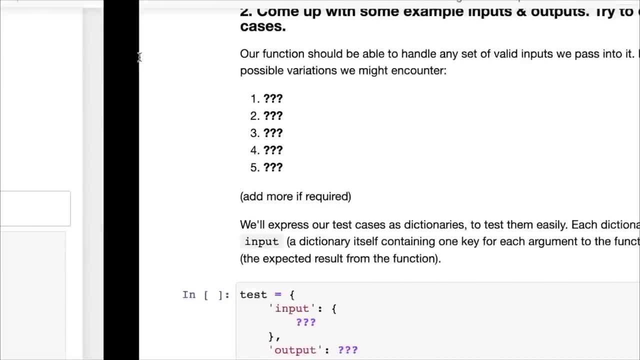 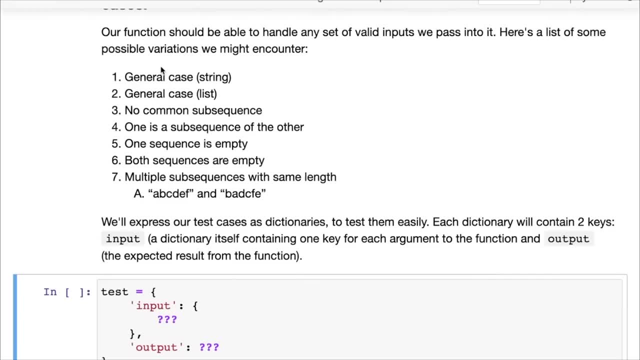 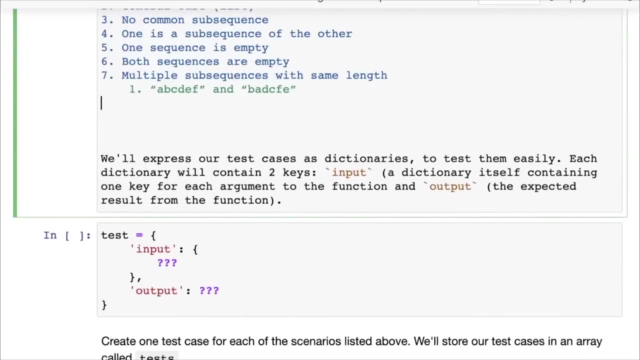 And it's always something that is appreciated by interviewers. Let's do that, Let's get, let's copy over these test cases here and you can think of more. So if you have some more ideas of things you should test, come up with them. 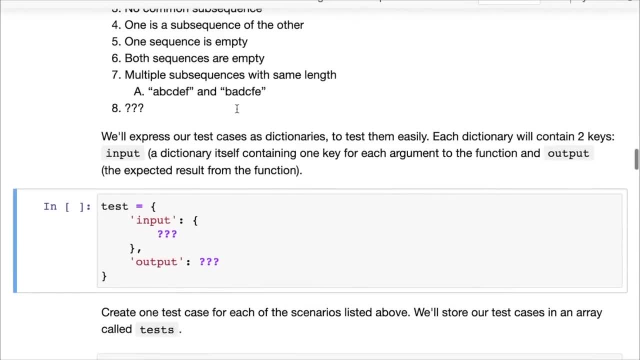 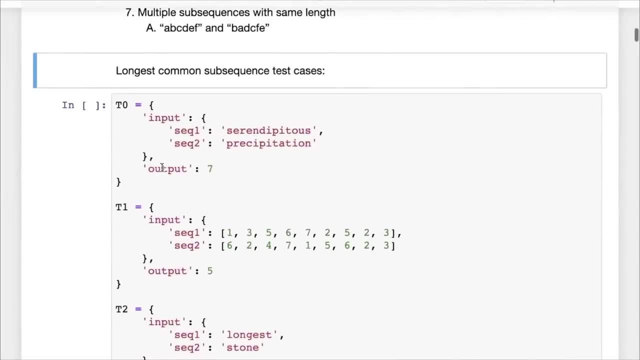 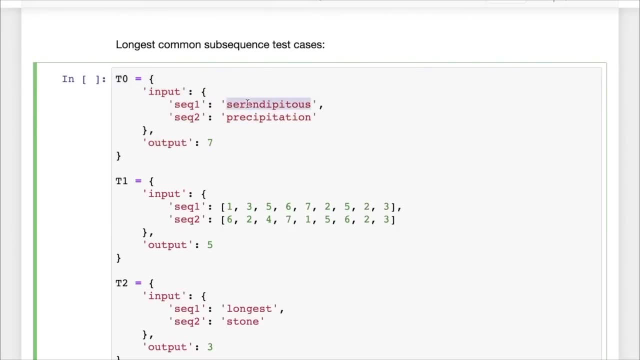 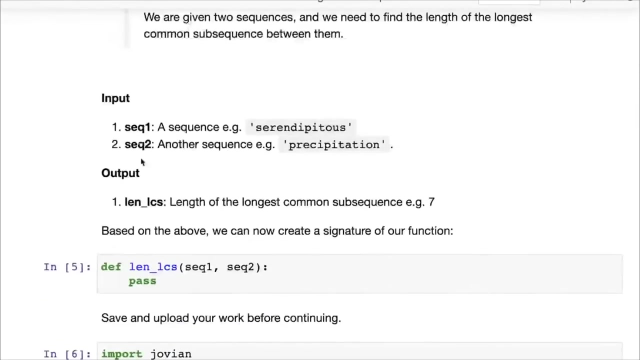 There's no right number of tests. whatever it takes for you to feel confident is what you need to do. Okay, So now what we've done is we've taken these test cases. So you can see, here we have this first sequence, sequence one. and remember, that's why we've written out, oh, that's why we've written out here the names of the inputs and the signature of the function. 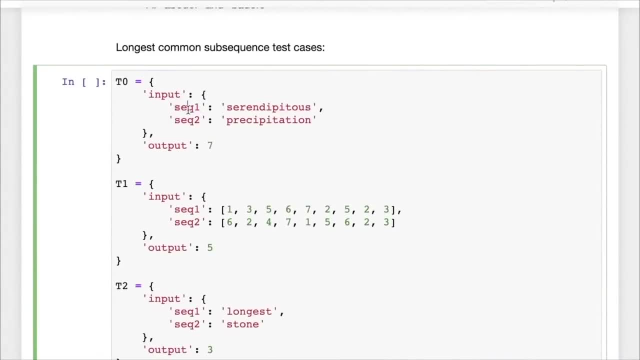 Now we can create test cases, Yes, dictionary, so that we can test them all easily, all at once. So we have the sequence one and sequence two in the input sub dictionary, inside the main test case dictionary, And then we have the output, which is the output of the function, which should be seven. 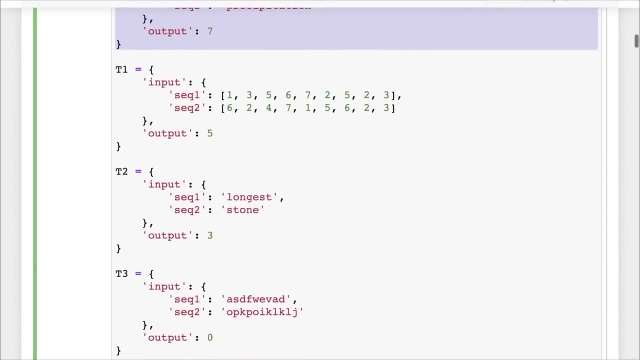 And this you can see, This you can verify. So this is a general case. Then we have another case. In this case we have two sequences. These are both lists of numbers And in this case, the output that we expect is five. 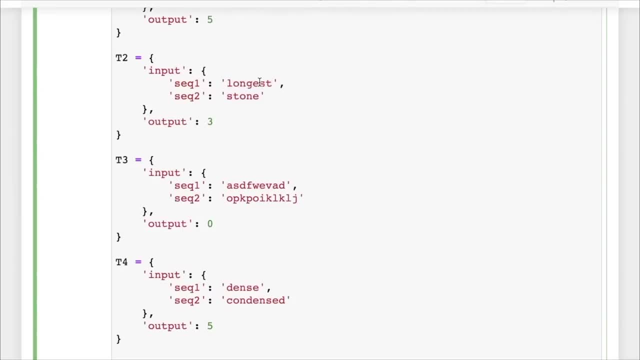 And we have another general case longest and stone. In this case you can verify that O and E is the common sub sequence. It has the output three. Then here we have two sequences which do not have any common elements. All of these come from the left half of the keyboard. 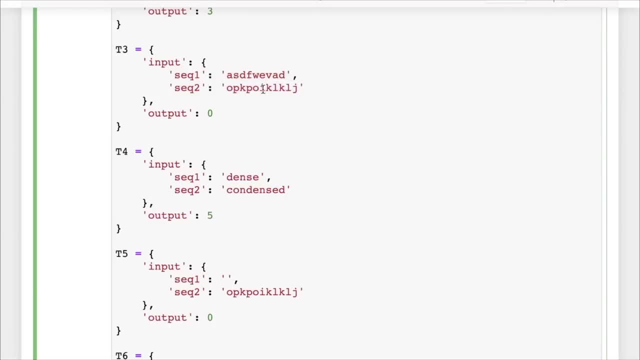 All of these come from the right, So the keyboard. So that was a quick way to generate these two sequences. Then here we have dense and condensed, and you can see that dense is actually a piece inside condensed. So this is a special case where dense is a continuous sub string of the string. 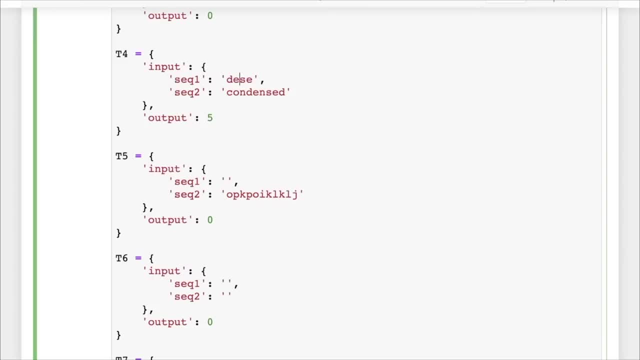 Uh, but it even if he had D E S E, that would still be a sub sequence, because D E S E occur in this order. So that's one example, And in this case the Sequence one is itself the longest common sub sequence and it has length five. 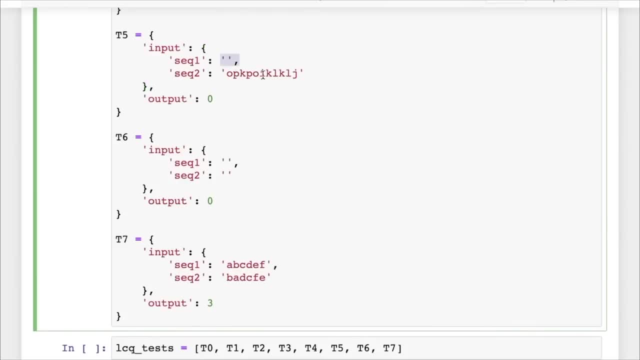 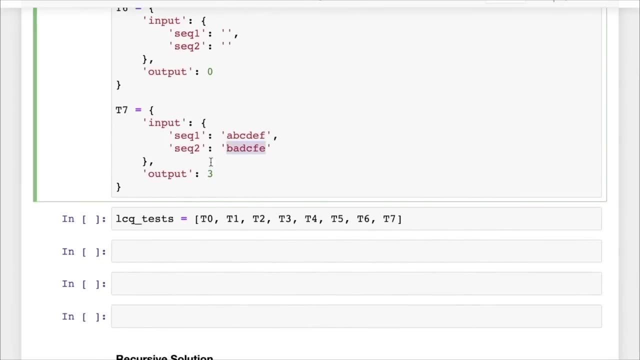 Then we have this case where one of the sequences is empty And you can see, in that case the output should be zero and both sequences are empty. And here is the case where you can have multiple longest common sub sequences And even in this case your function should be able to figure out the answer correctly. 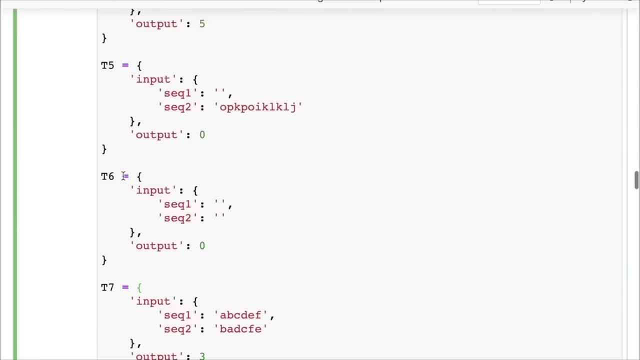 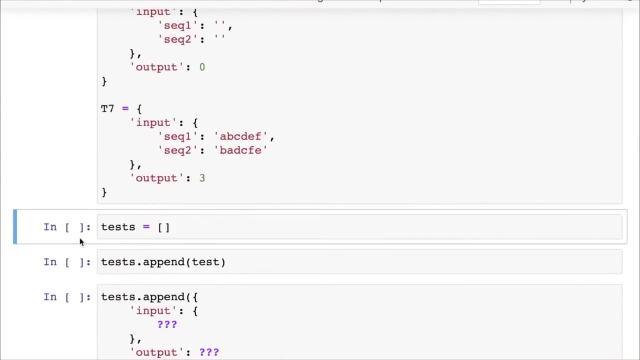 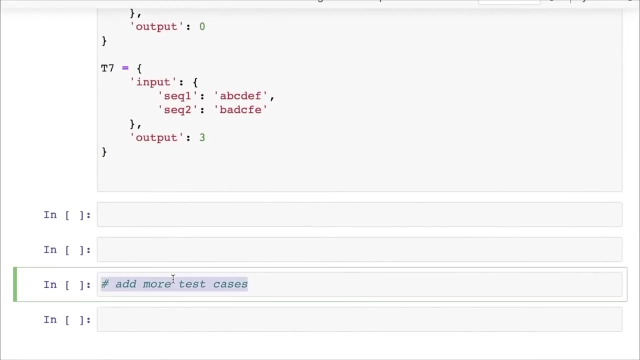 So let's take this and let us copy over these test cases here. So we have T, zero, Two, three, seven, So that's eight test cases, And you can add more test cases here. Please feel free. coming up with good test cases is a skill that you should develop. 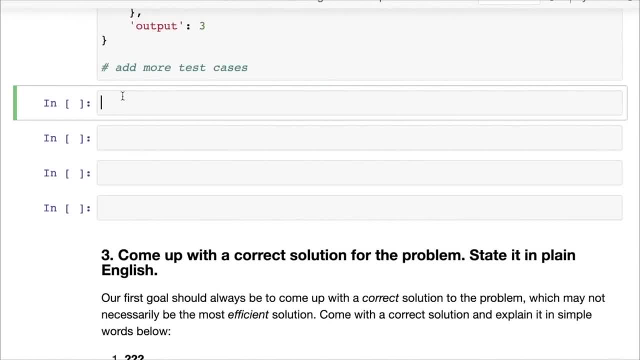 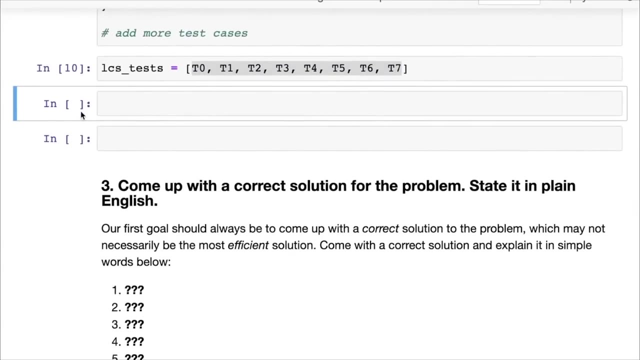 And what we'll do is we'll also put all these test cases into this function called LCS or longest common subsequent tests, So that we have all of them Easily available for testing at once. Okay, Okay. Now next step is to come up with a correct solution for the problem. 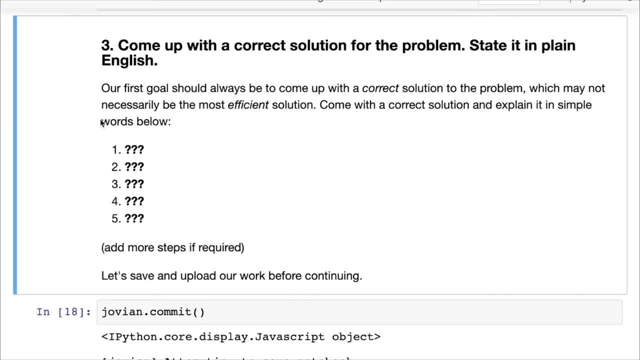 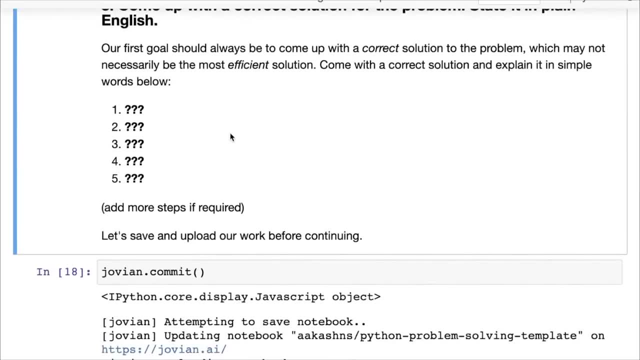 Now we've seen the problem, We have identified some scenarios. Now we need to come up with a simple, correct solution and stated in plain English. It doesn't have to be efficient, It just has to be correct. So here's one idea. 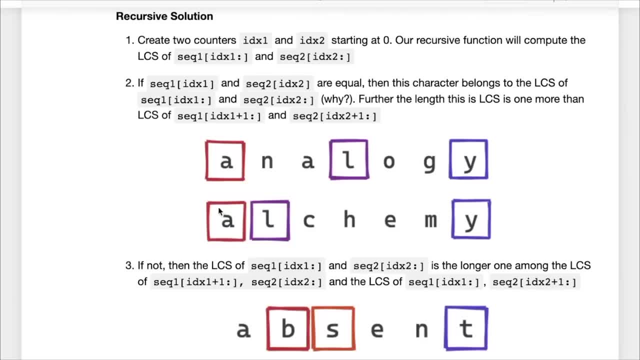 Here's one idea. here You can see we have a couple of Sequences. Let's create two counters, IDX one and IDX two, both starting at zero. So IDX one will be a pointer which will start tracking elements in the first sequence. 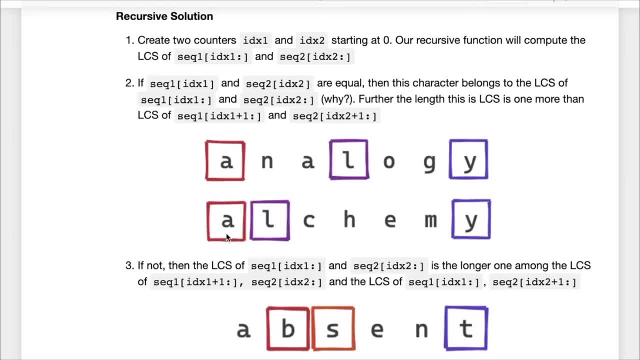 And IDX two will be a pointer which will start tracking elements in the second sequence, And what we do is we will write a recursive function. So we'll write a recursive function which will compute the LCS. Okay, So we'll write a recursive function which will compute the LCS of sequence one from IDX to the IDX one to the end and sequence two from IDX two to the end. 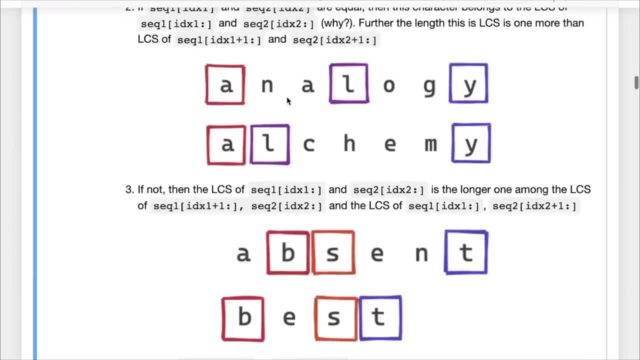 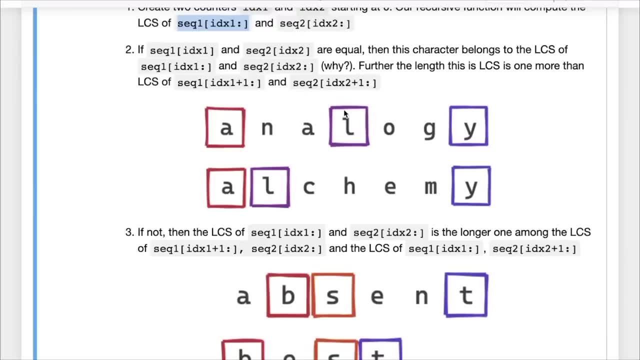 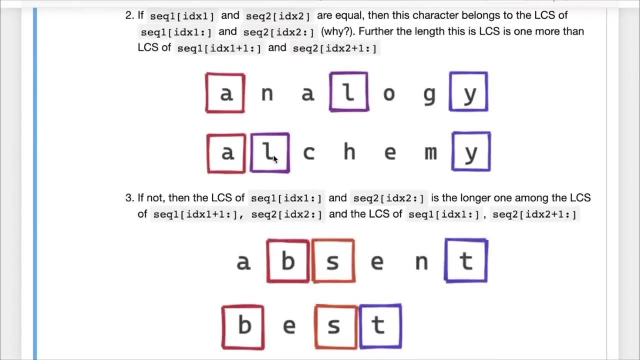 So what does that mean? Let's say IDX one has the value three and IDX two has the value one. So you can see zero, one, two, three. So sequence one, IDX one onwards is L O G Y and sequence two, IDX, uh. IDX two onwards is LCHM. 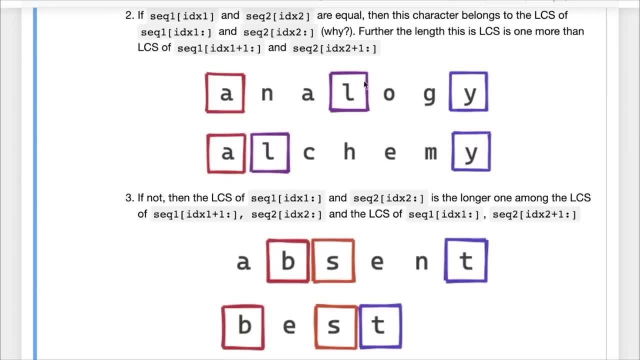 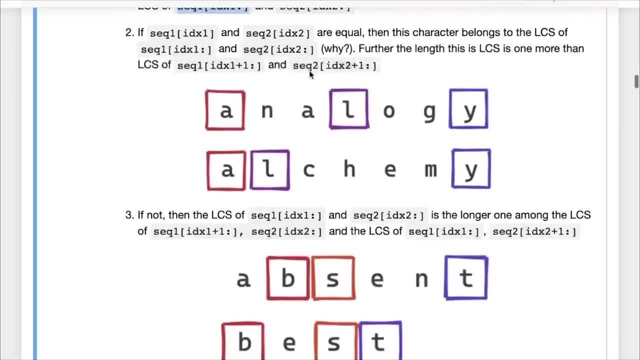 So we're looking at this portion of the problem and this portion of the problem and a recursive function, when invoked with IDX one and IDX two, should return the length of the longest common subsequence between these two portions, So L O G, Y and LCHM. 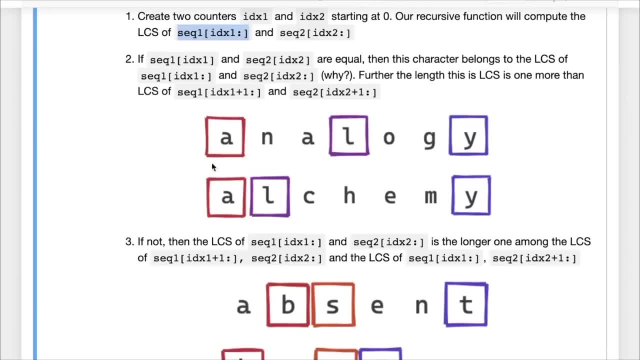 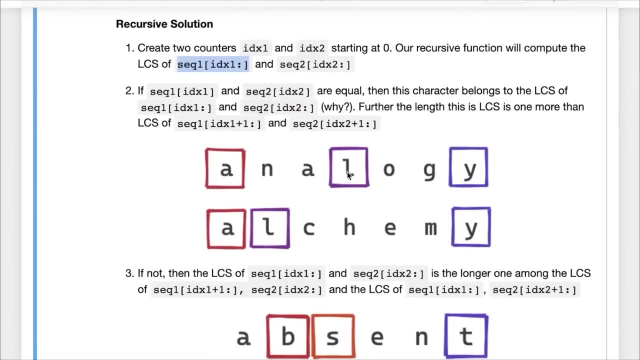 Now, why are we doing this? We need this longest common subsequence for the entire string, Don't we? Now here's the logic Why: Why we're writing this recursive function which can theoretically compute this subsequence for from any position onwards. 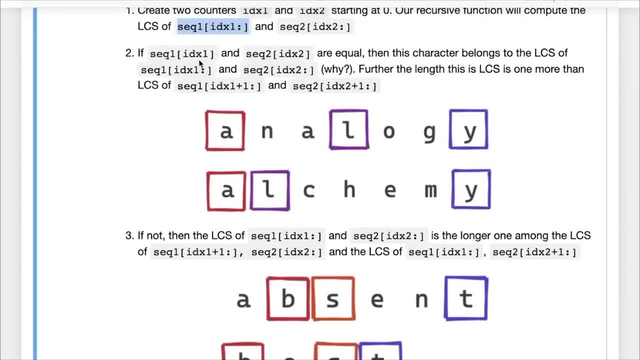 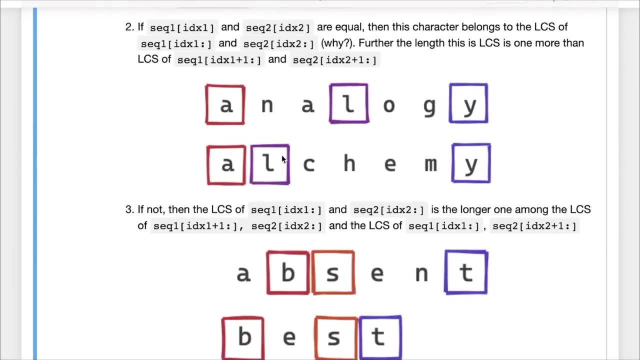 So here's how we do this: If sequence one of IDX one, So if IDX one was pointing to L and IDX two was pointing to L- here as well, if sequence one of IDX one and sequence two of IDX two are equal, then this character L belongs to the LCS of. 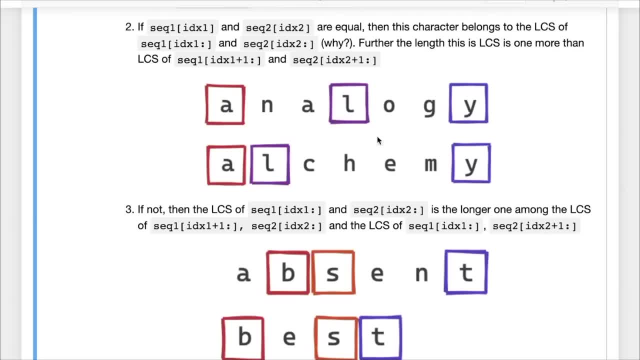 This portion and this portion. Okay, Why think about it? It makes sense because these, these elements are equal. So if you pick the longest common subsequence of this and you pick the longest common subsequence of the remaining, then you can always add L to board to that subsequence. 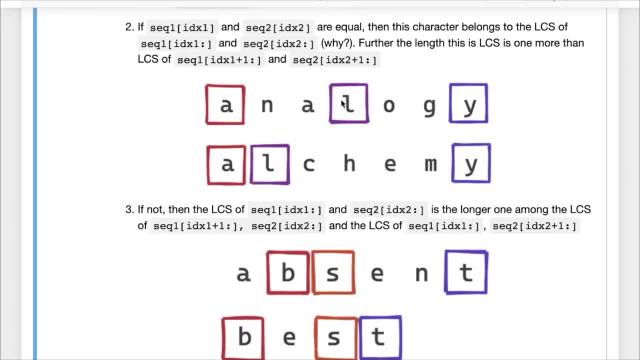 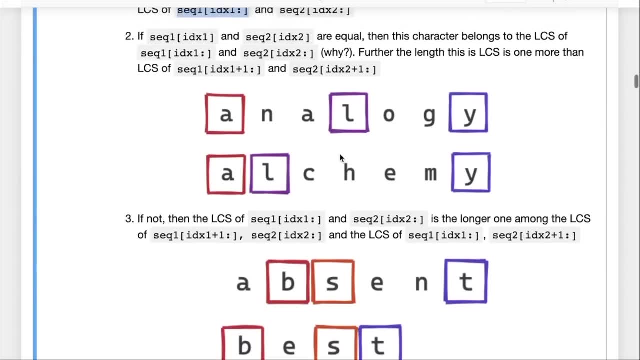 And that will make the subsequence longer. right, And that way it follows that L will always occur in the longest common subsequence between L O G Y And L C, H, E, M Y. Okay, So we know now that this will occur. 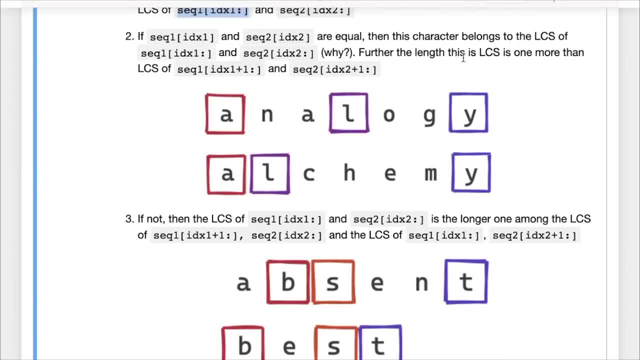 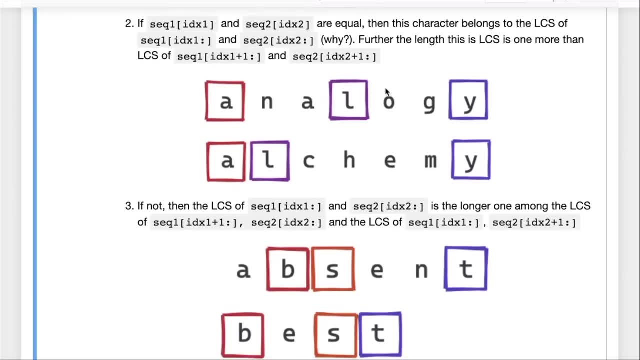 L will occur in the longest common subsequence. further, the length of this longest, the length of this longest common subsequence will be the length of the longest common subsequence between O, G, Y and C, H, E, M, Y plus one. Okay, And now you can see why a recursion is required, because what we can now do is we can say that if 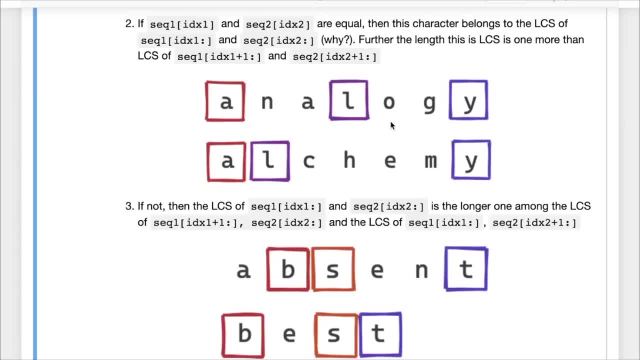 Sequence one of IDX one and sequence two of IDX two are equal, then we simply call the recursive function on sequence one of IDX one plus one, So O, G, Y and sequence two of IDX two plus one C, H, E, M, Y, and assume that recursion will give us the solution there and simply add one to it because this is equal. 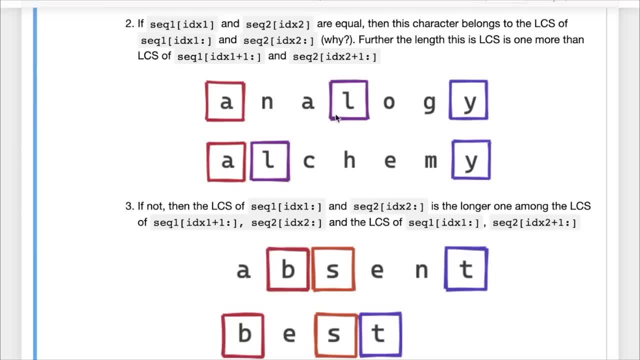 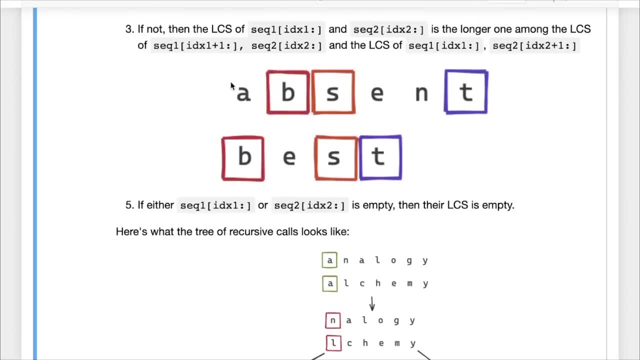 Okay, So that's one case. if sequence one of IDX one and sequence one of IDX two are equal, Great, But if they're not equal, Right. So for in this case, for instance, you can see that if IDX one and IDX two are both zero, 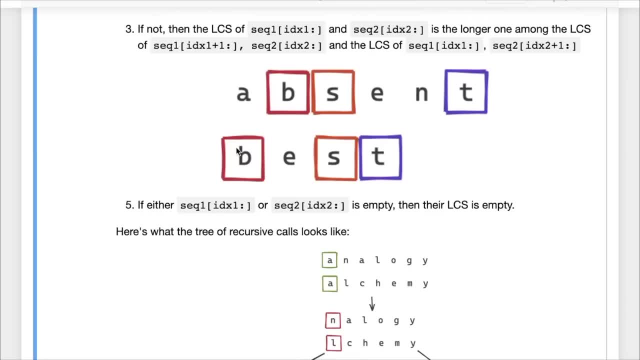 So IDX one points to a and IDX two points to B. So if they're not equal, then one of the two things should hold. either a does not occur in the longest common subsequence between the two strings, or B does not occur in the longest common subsequence between the two strings. 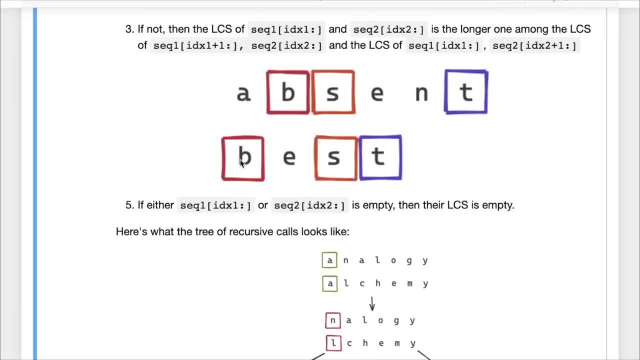 Now we don't know which one, but that's the power of recursion, that we can Just try both. so we can simply ignore a and we can get the longest common subsequence between B, S, E, N, T and B, E S, T and check its length. and then we or we can simply ignore B and we can get the longest common subsequence between a, B, S, E, N, T and E S T and check the length. 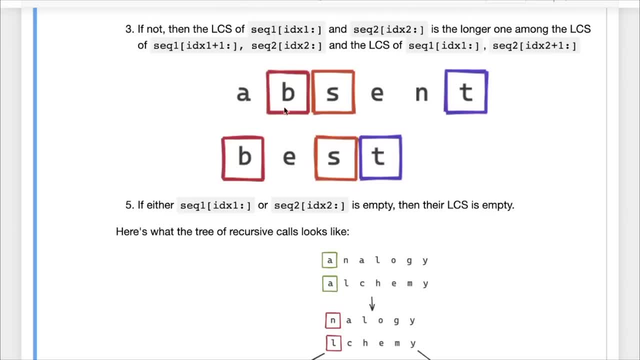 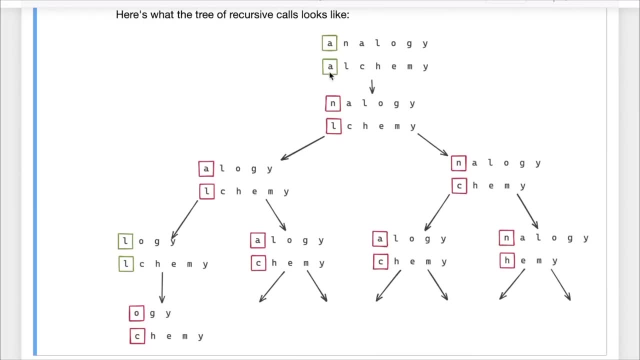 Now, whichever is longer in length, that becomes the solution for the two strings. Okay, So this is what it looks like. We start out with analogy and alchemy, So we compare a and a. uh, these two are equal. So we know that the longest common subsequence is one. 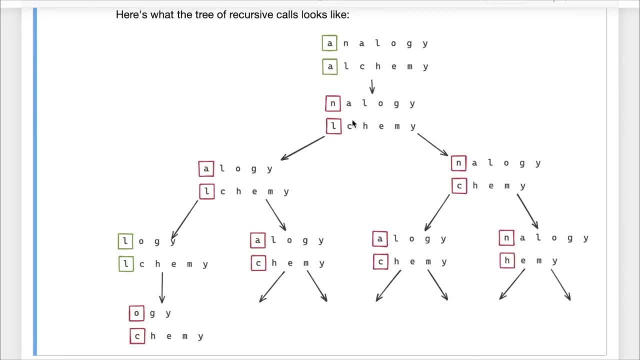 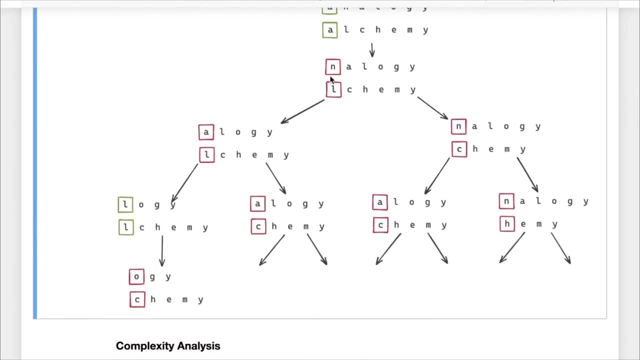 The length is one plus LCS of analogy and alchemy. Okay, Now we compare N and L, and now we see that they're not equal. So either N does not come in the longest common subsequence or L does not come in the longest common subsequence. 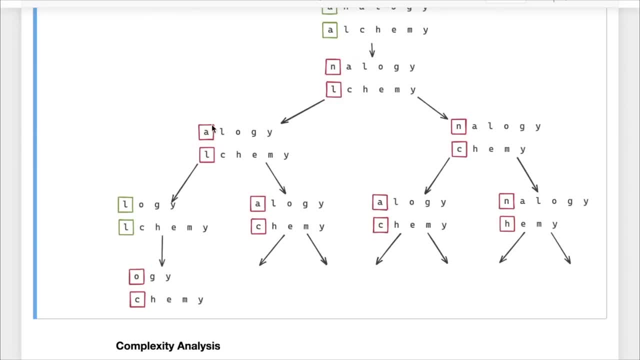 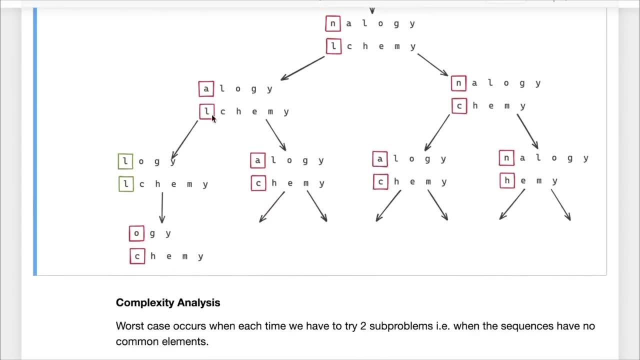 So we try both. We remove N- here You see a L O G Y, And we remove L- Here we see C H E M Y. Now, once again, a and L are unequal. So either a does not occur in the LCS of these two strings, or L does not occur in the LCS of these two strings. 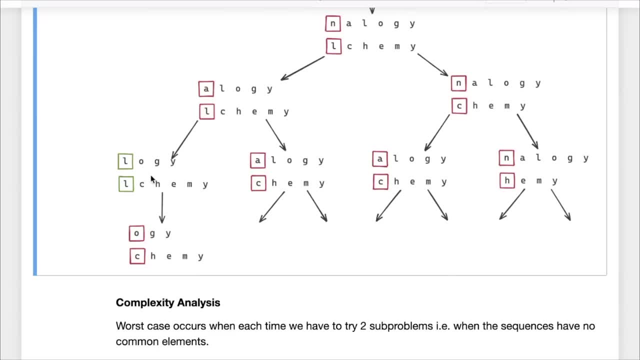 So if a does not occur in the LCS, we can remove a and try again. If L does not occur in the LCS, we can remove L and try again, And here, once again we get a match. So in this case we know that L occurs in the longest common subsequence of these two elements. 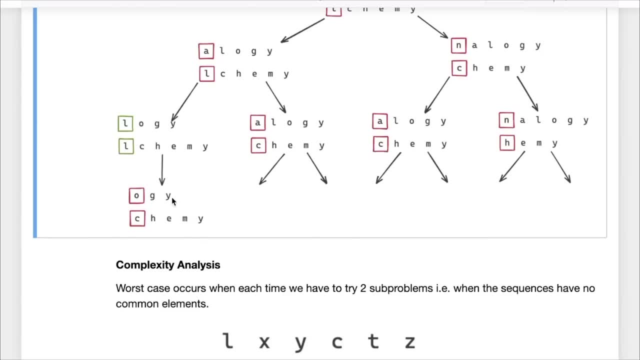 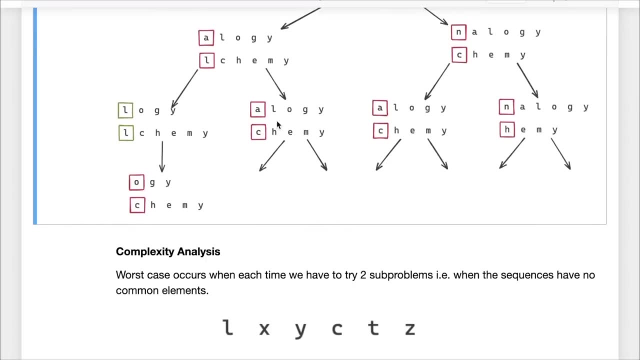 So now we can get the LCS of O, G, Y and C, H, E, M, Y, Okay. And then, as these recursive calls complete, you can see that this entire tree pans out. You can see that each time, you either get one child or you get two children. 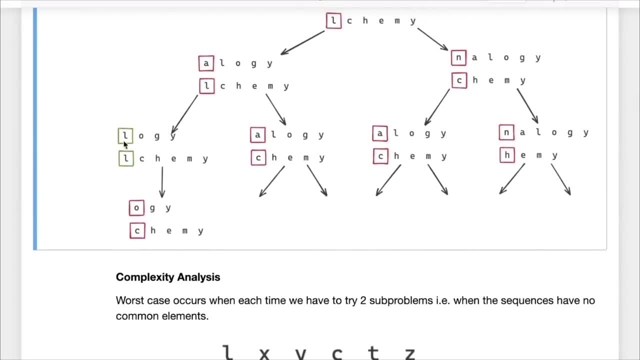 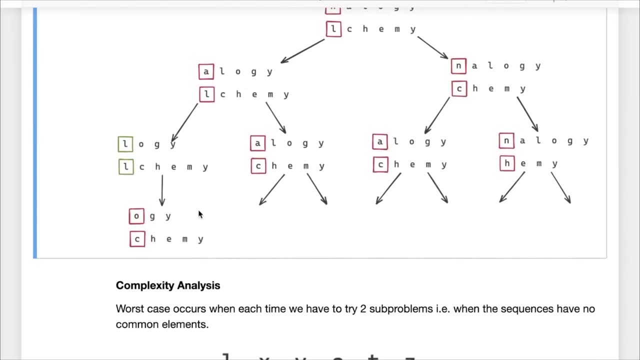 And if you go all the way down and then you go back up and simply count the number of matches for each path, you will key And you take, keep taking the maximum. So here you get back an answer. Let's say you get back an answer of size two. 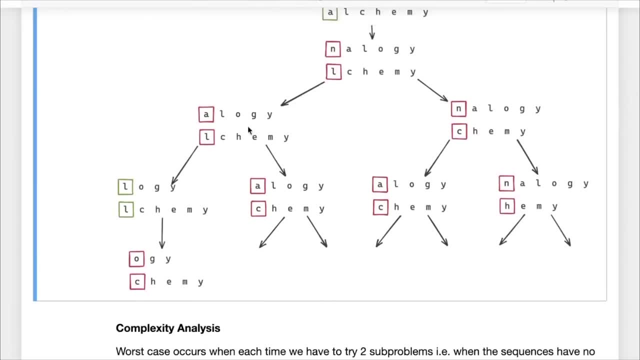 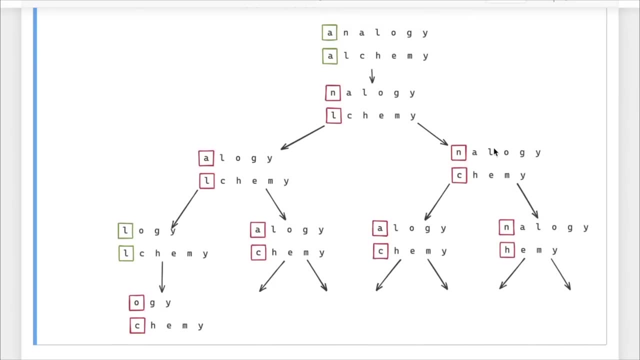 Here you get back an answer of size one. So the answer for this Is simply the maximum of two, and one which is two, And then the answer for this is simply the maximum of two, And let's say this is three, then three. 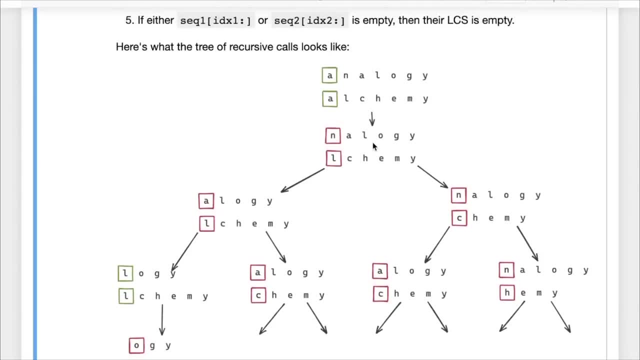 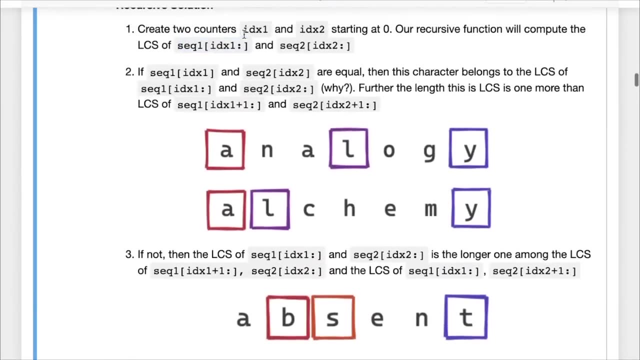 And the answer for this is simply one plus three, four. Okay, So this is the way that we will build up the solution. So we've now looked at the recursive solution expressed in text and we've looked at the recursive solution expressed as a tree. 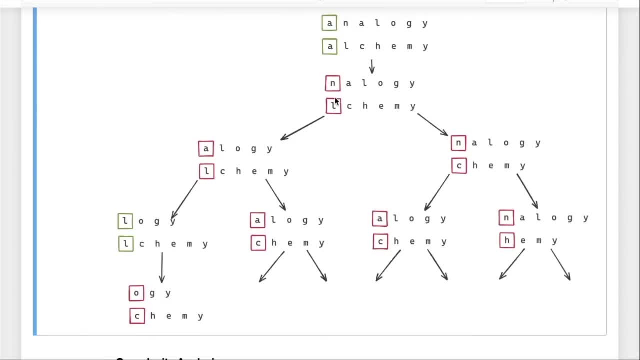 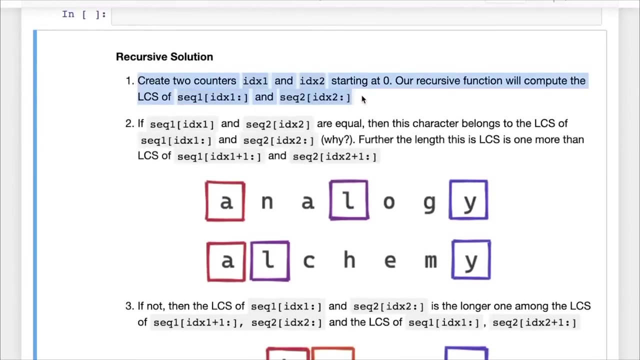 Now it's possible that it still may not make sense to you how exactly this is working, And that is where you should start trying to create this tree yourself. So pick up a pen and paper and then start drawing on pen and paper. Take an example and try to read each step here and try to work it out like a computer. 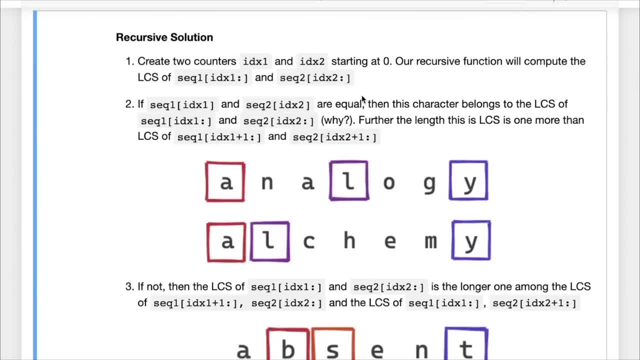 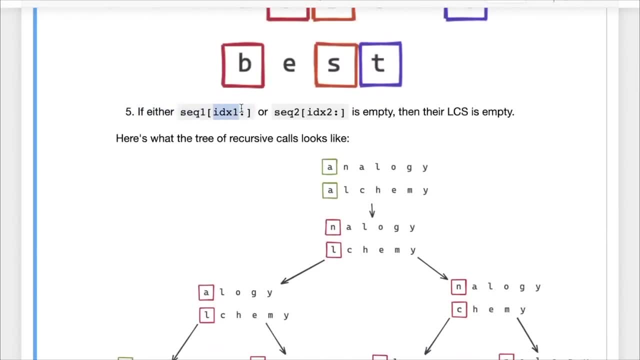 Okay, And just thinking about it that way will help you understand this algorithm. Now, one last thing is that if either of the sequence one from IDX onwards or sequence two from IDX onwards is empty, which means the index has reached the end, Okay, 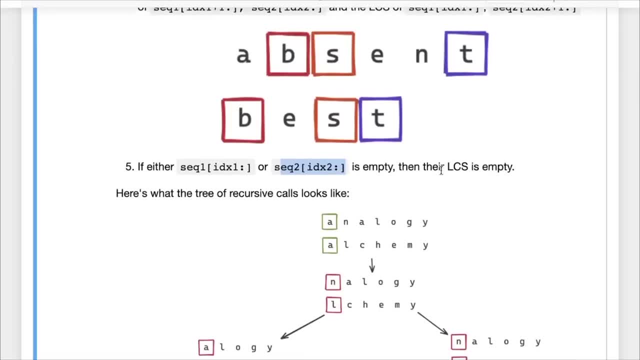 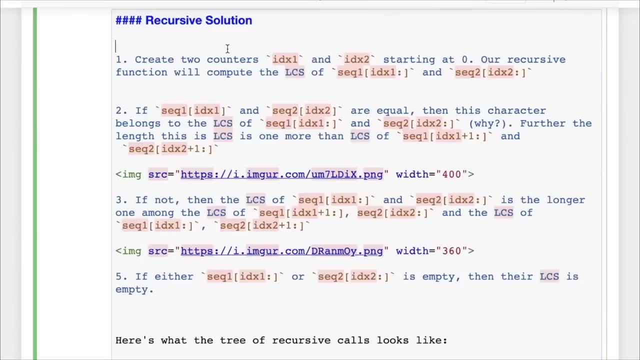 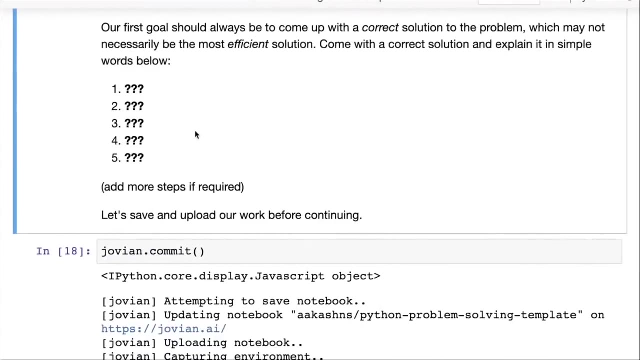 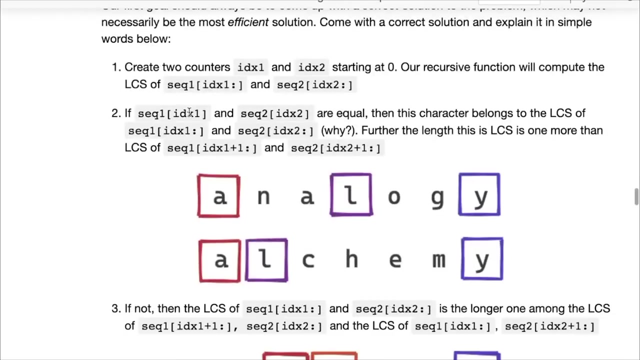 Endpoint in. after doing some recursion, then their LCS is empty, So the length is zero. Okay, So that is the recursive solution here. I will just copy over this recursive solution to along with the entire tree. Now, obviously, in an interview you do not need to write all of this in in a lot of detail, or you do not need to. 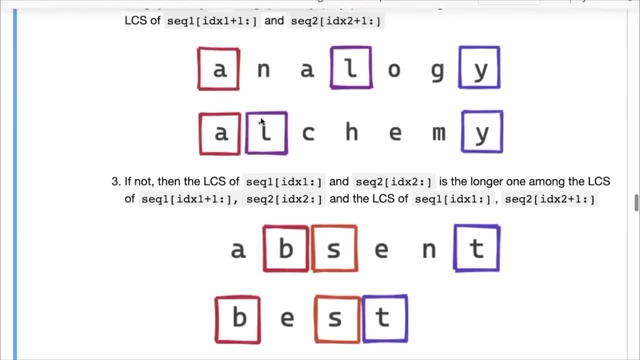 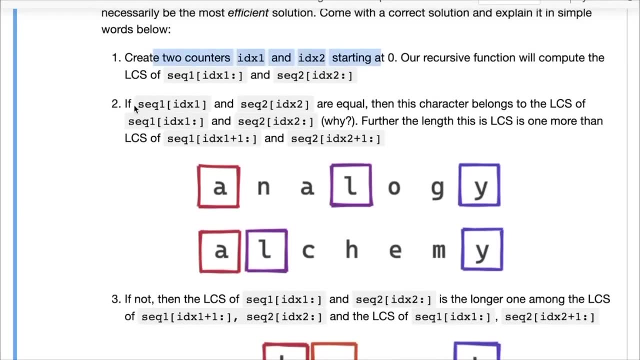 So it's helps to show a diagram sometimes, but you don't really need to do all of this. All you need to do is express yourself clearly that we will create two counters, And the condition to check is whether these two elements at those counter positions are equal. 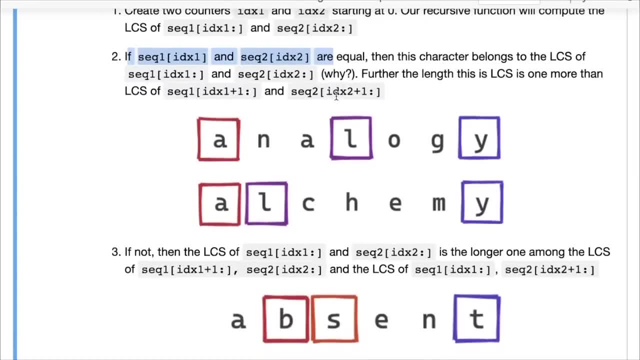 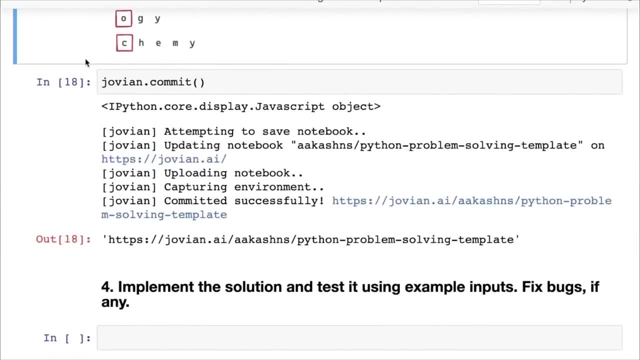 What do we do if they are equal? What do we do if they are in equal, and why are we using recursion here? So we are using recursion We can, because we can use reuse some of the sub problems to compute the final problem. 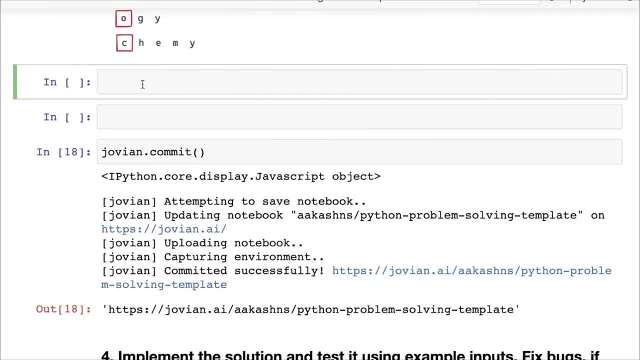 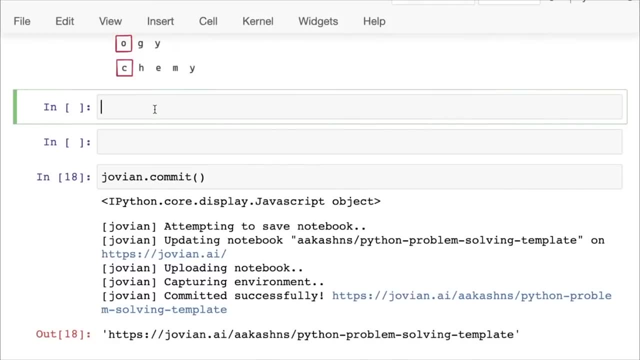 Okay, And understanding recursion is. It's really important for solving data structures and algorithms from this, because it's like a superpower pretty much. pretty much every problem that you see one way or another can does boil down to recursion in one way. 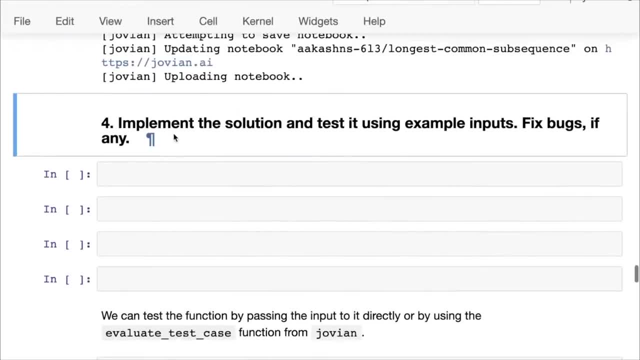 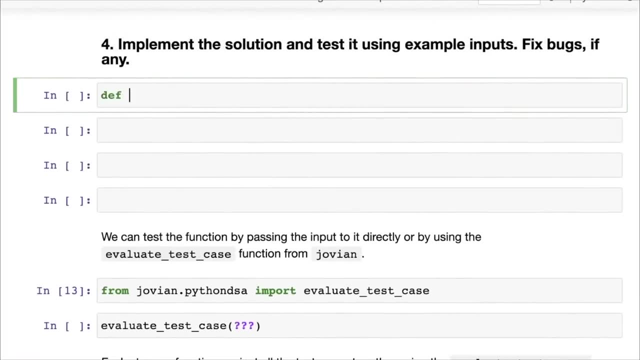 Okay. So now let's save our work once again, and now we're ready to implement the solution. So we have the recursive solution in front of us And if you remember the four steps, let's go. let's go ahead and implement it. 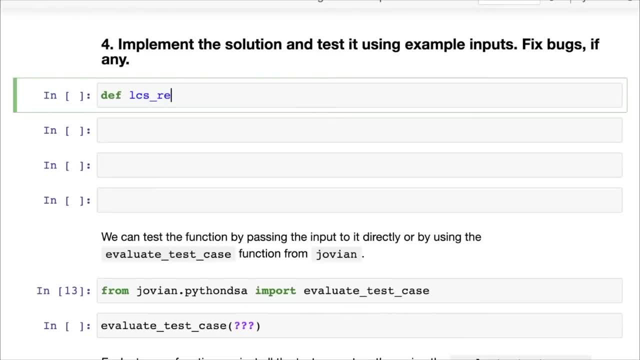 So we see, let's just call it LCS Recursive, and this will accept a sequence one and a sequence two, And let's also initialize IDX one and IDX two, because we will be calling this function recursively. So we'll simply use these two counters, IDX one and IDX two, and set them to zero. 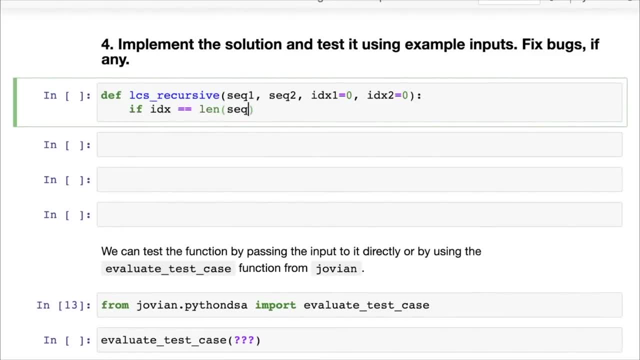 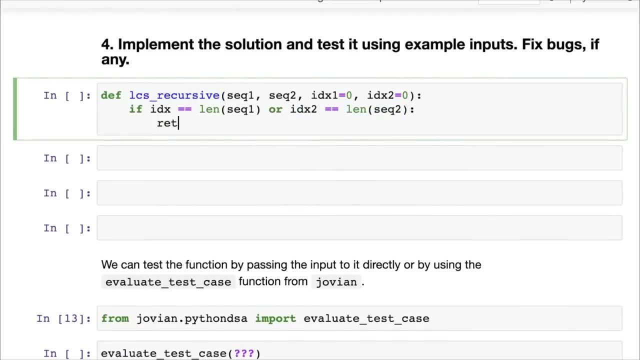 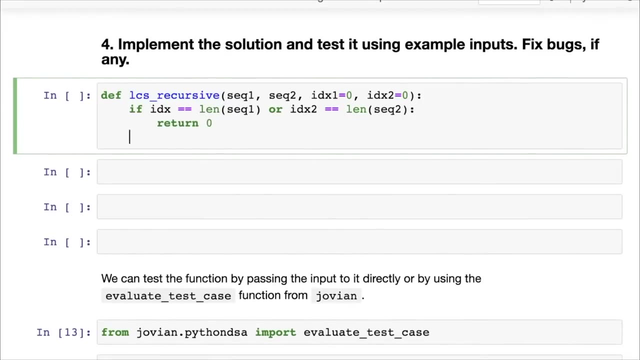 Now the first thing we need is if IDX one is equal to the length of sequence one or IDX two Is equal to the length of sequence two, then we return zero Again. this is a common thing that happens, that the base case, or the end scenario is something. when you're describing the algorithm, you will describe at the very end. as you're drawing the tree, you will notice what the end case and scenario is. 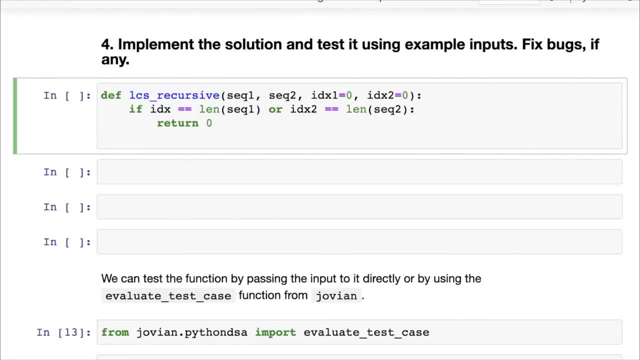 But when you're coding the algorithm, the end scenario or the base case comes at the very top, because otherwise we'll try and access IDX one from sequence one and that will throw an error. So that's what you need to handle: The base case at the very beginning. 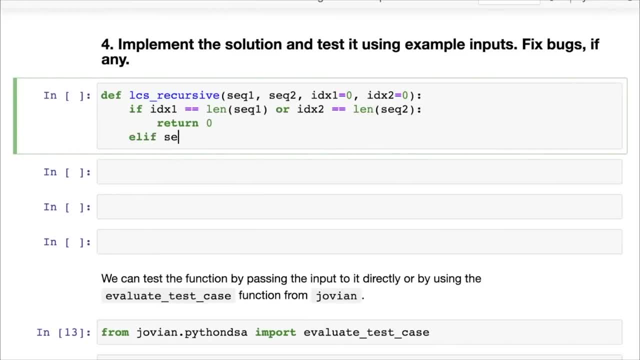 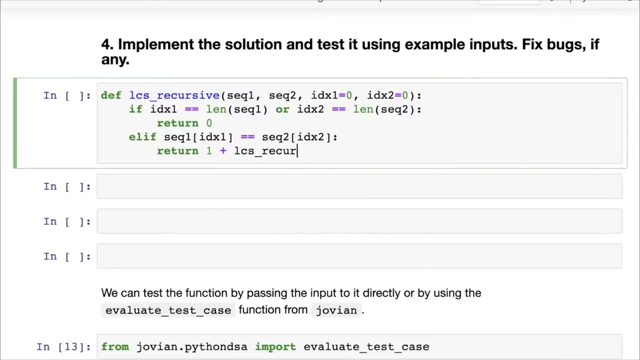 Okay, next, moving ahead, If sequence one of IDX one equals sequence two of IDX two, Great, We found a match. So we simply return one plus. Now we can call LCS recursive on sequence One, sequence two and we increment IDX one by one. 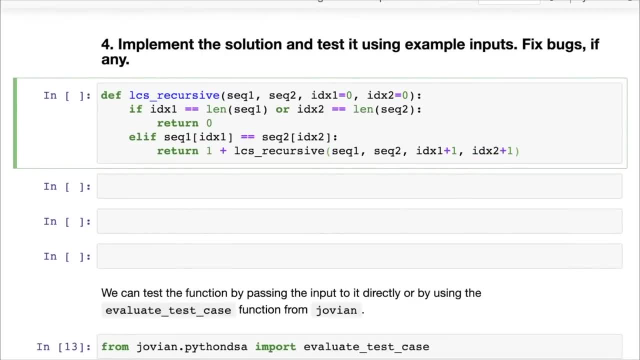 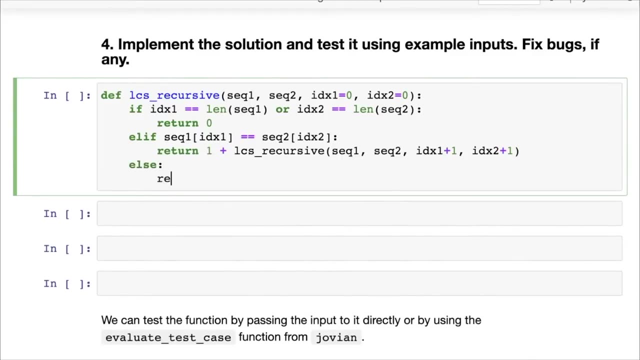 And we also increment IDX two by one. Both of these need to be incremented because we are going to use this element, this common element, as an element in the sub sequence. Okay, So there's just one recursive call here. That was nice. 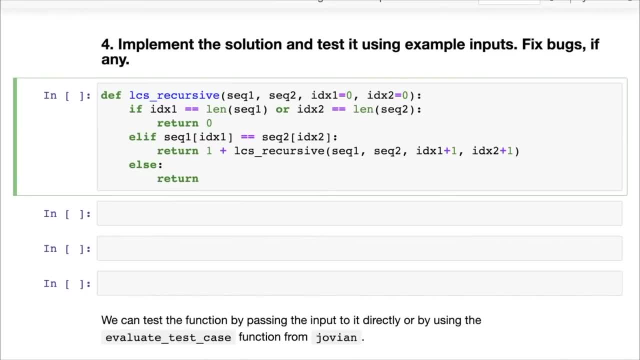 Otherwise we have to either ignore the first element Of all, the current element from sequence one or the current element from sequence two. So we have two options. So we have option one, which is we ignore the current element of sequence one. So this becomes LCS recursive sequence one, sequence to IDX one plus one and IDX two. 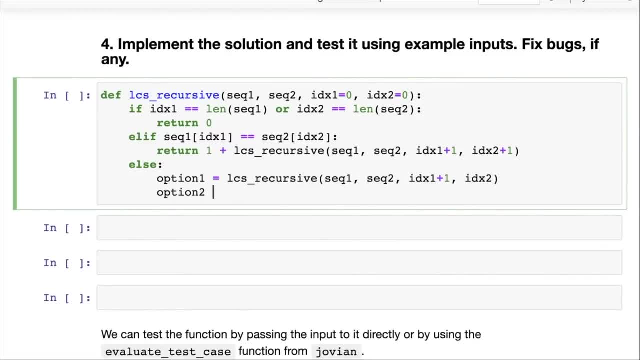 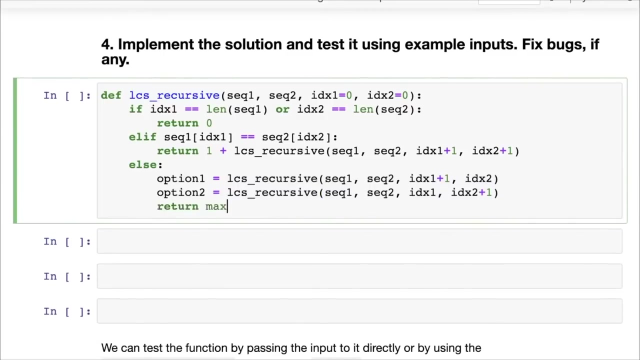 And then we have option two. This is LCS Recursive, once again with sequence one and sequence two, and this time we increment IDX two. Okay, So make sure you understand this piece, because this is really the key here. And then the length of the longest common sub sequence is simply the maximum of option one and option two. 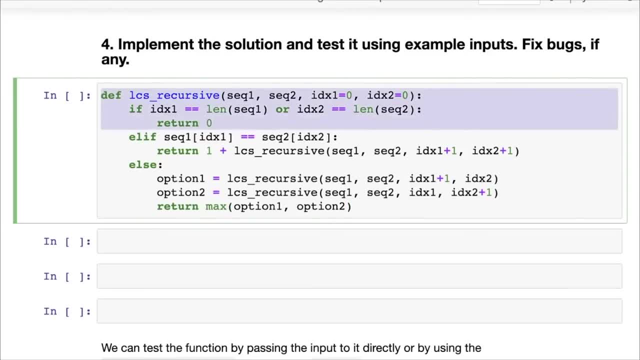 Okay, And that's it. What may have seemed like a fairly tricky problem Once you start thinking About it recursively. Okay, What happens if we simply compare the first two and they're equal and they're unequal. Okay, Now we need to solve the problem for the remaining um. either we add one or we take or we ignore one of the elements. 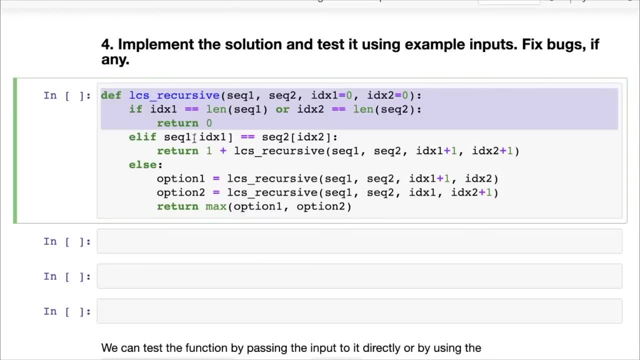 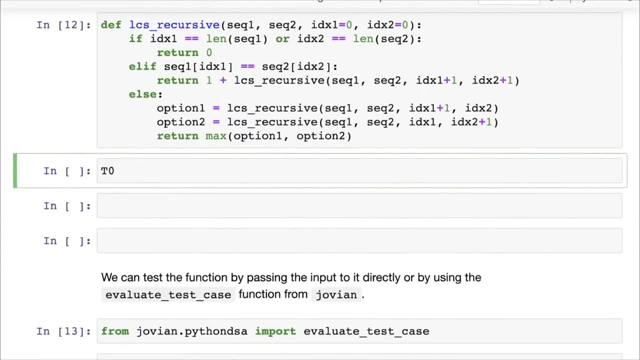 Right, Once you get that thought, the recursive thought, then the solution and the code simply presents itself to you. It's just about seven lines of code. Okay, That's our LCS recursive solution. Now let's test it out. Let's look at a test case: T zero. 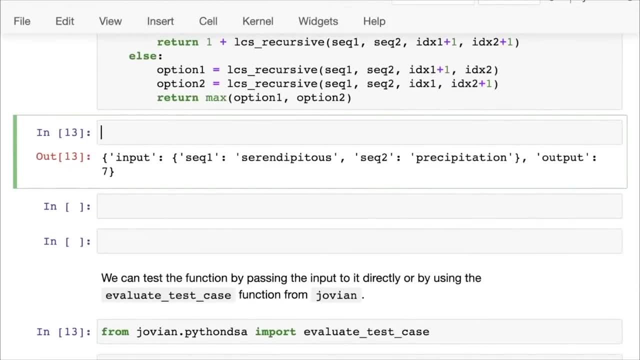 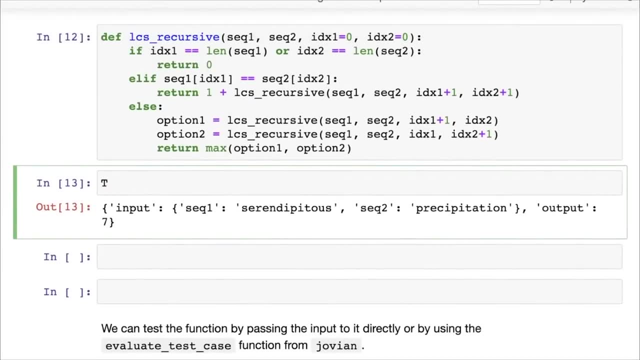 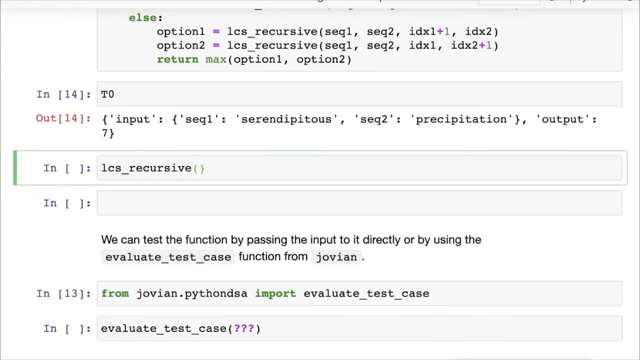 Okay, So here we have serendipitous and precipitation as the inputs. let's call LCS. Let's keep that around so that we can view it later. Let's call: call LCS recursive on T zero. But of course we need to fetch from T zero the input and uh get sequence. 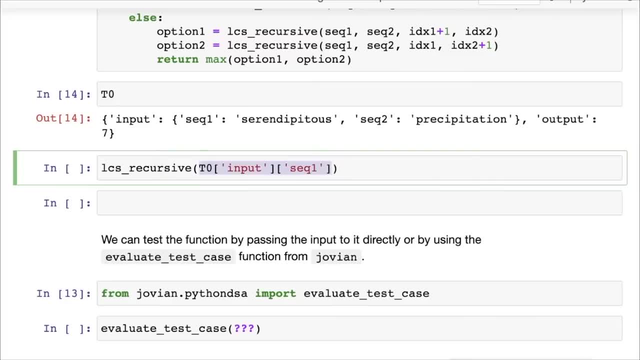 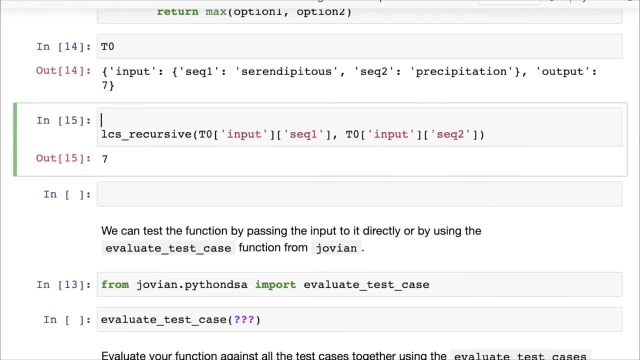 One out of the input And similarly, we need to get the input and get sequence two out of the input. You can see it: it takes, it returns the value seven, which is equal to the output, by the way. So if we simply put in here T, zero, 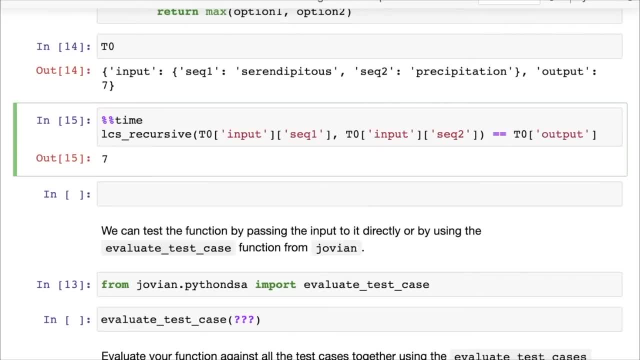 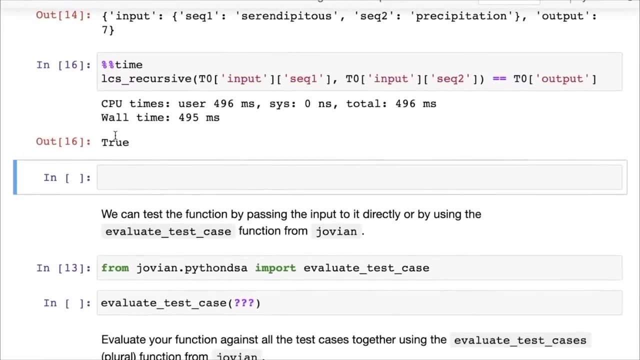 Output And I'm also going to put in this special command called percentage percentage time. This is going to tell us how long the cell takes to execute. Yeah, So now you can see here that if we get back to, and the cell takes 495 seconds, or half a second, to execute. 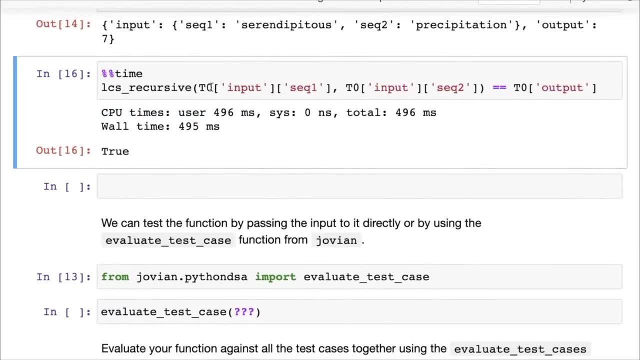 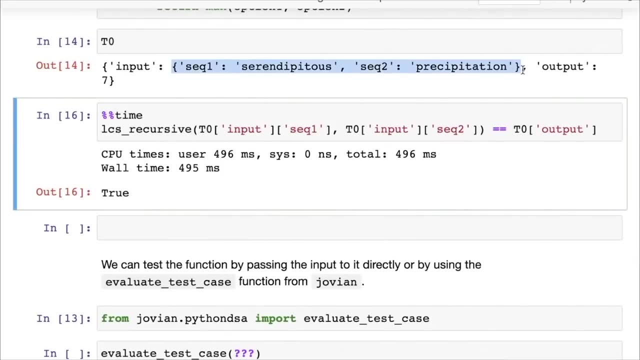 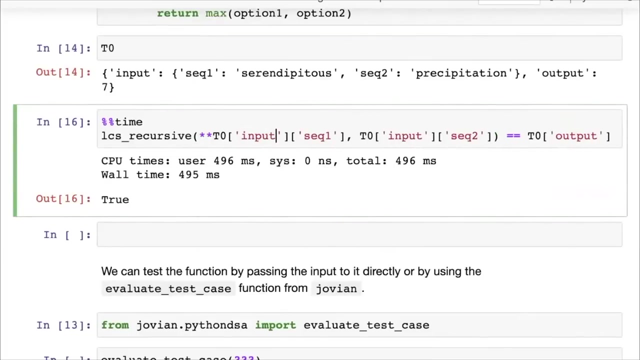 And that's it. So now we have tested this test case. One small thing I can tell you how to improve this slightly is because, Okay, Okay, So in T zero of input is a dictionary and because the names of the elements of the dictionary are sequence one and sequence two, which also match the argument names of LCS recursive. you can see, here we have sequence one and sequence two. what you can do is you can simply say star, star, T, zero input, and Python will automatically grab each key. 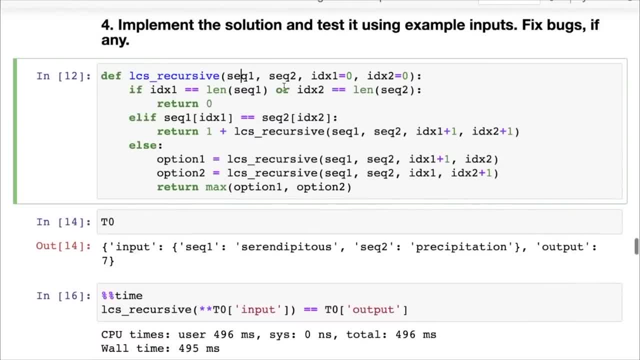 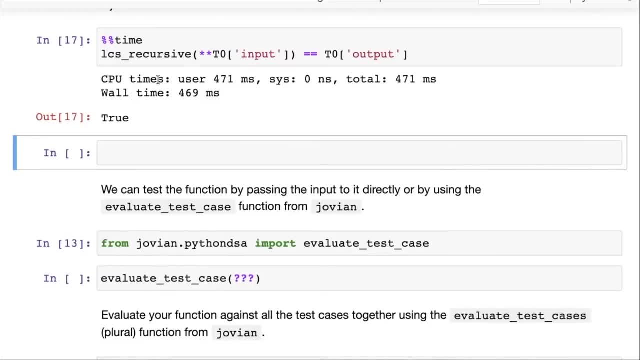 So sequence one will be passed as the argument sequence one, and sequence two will be passed as the argument- sequence two, That's. this is a small trick here That helps us speed up The reduce the amount of code we need to write. Okay. 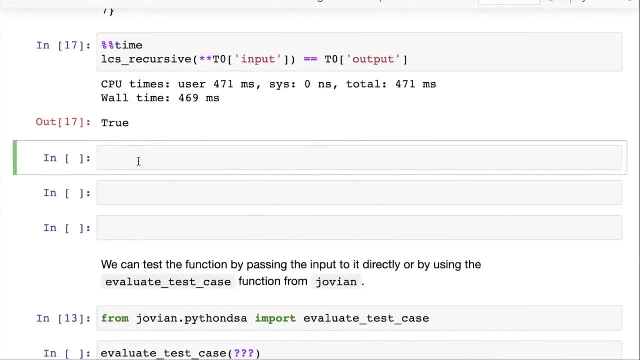 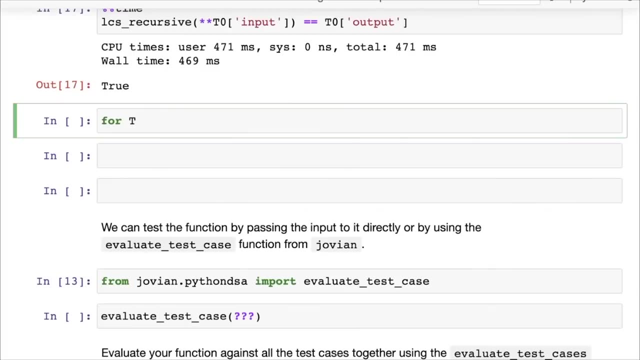 Now we've tested one test case, but that's not enough. We should be testing all the test cases. So to test all the cases, we can write a for loop for T in tests, et cetera. But we can do something else too. 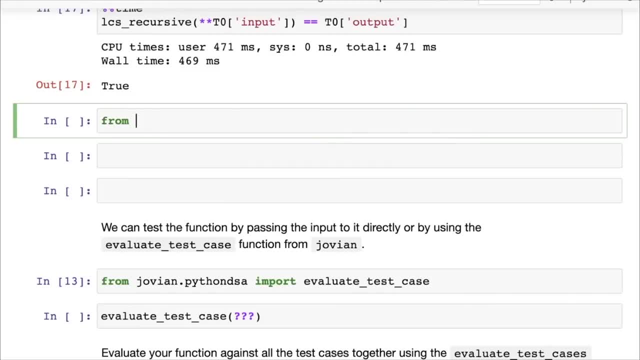 We can use the evaluate test cases function from Jovian, So from Jovian, not Python, DSA the module. Okay, We will import evaluate test cases. It's a helper function that we've created for you, but it's really simple to write. 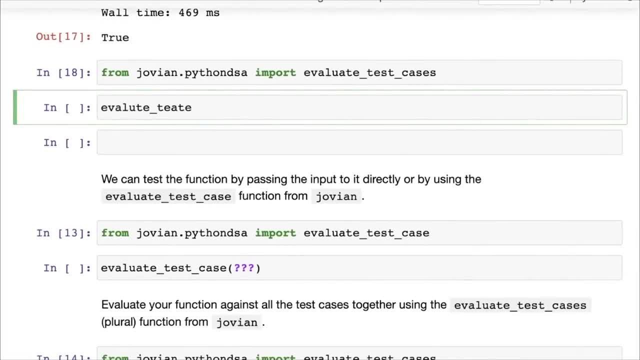 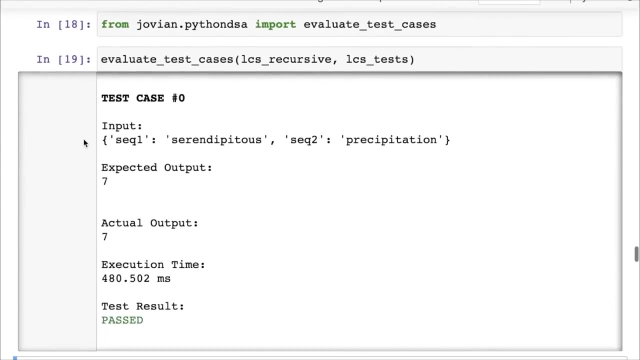 You can just use a for loop as well And we call evaluate test cases on the function that we want to test, which is LCS recursive, and the tests that we have, which is LCS tests, And when we do this, it is going to try out each test case. 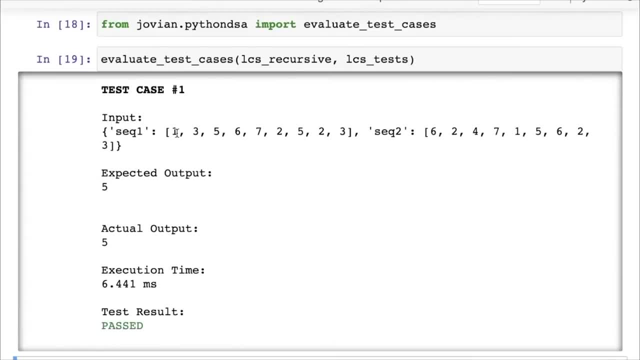 You can see it's tried test case zero. That was a pass. it tried test case one And it's also printing out the Input, the expected output, in the actual output. the test case One was lists, and lists work too, because all we've used here is indexing and length. 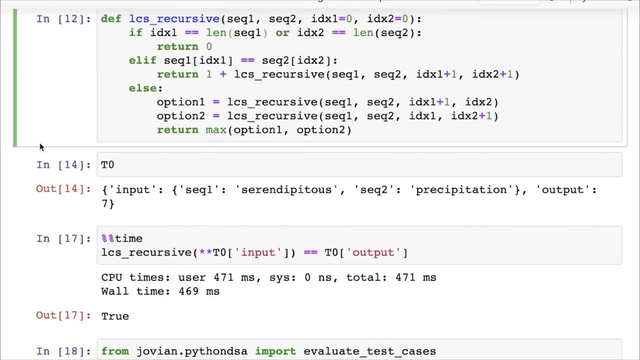 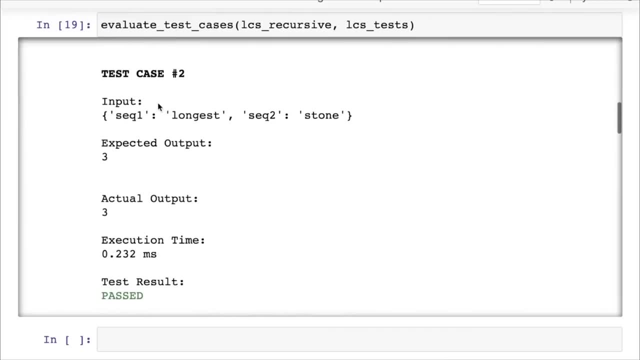 And these are both things that are available in both strings and lists, And this is something that's very nice about Python: the dynamic nature of the functions. Oh, once again, this worked perfectly fine. And then here we have another one, longest in stone. 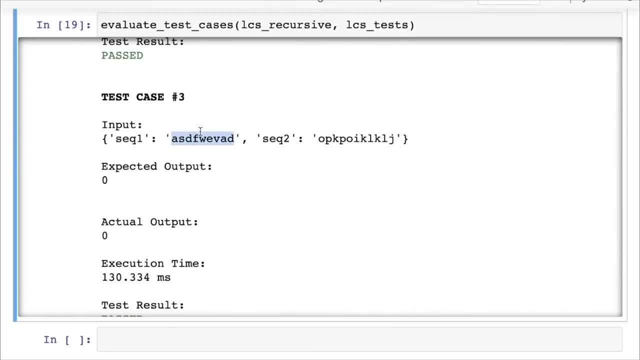 The expected output was three and the actual output was three as well. Here we have ADS, F, E, W, a, D and another string. They have nothing in common. So the expected and actual output are both zero. Here's one where one is. the is already a subsequence of another. 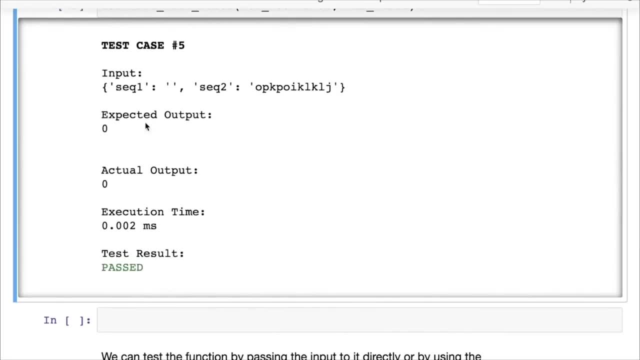 So the smaller one becomes the longest common subsequence, And then we have an empty string, and then we have two empty strings And finally we have multiple longest common subsequences. We still get back the right output. Now, if any of these failed, you would know exactly what went wrong, for instance, if you had an issue in this. 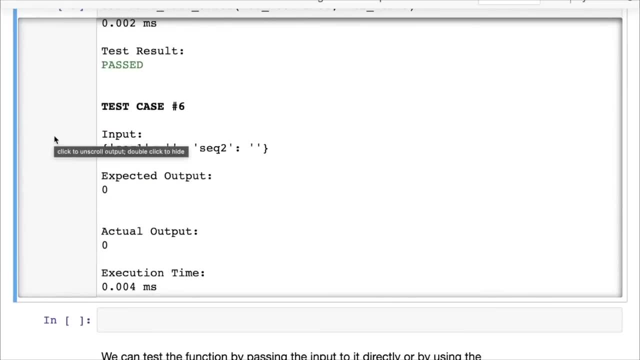 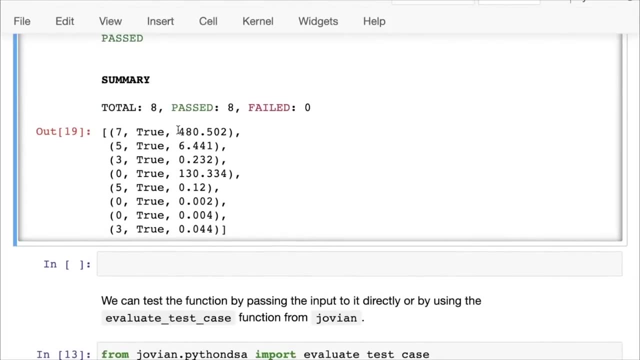 In this case, where the two of these were empty, and that would tell you that you've probably not handled that empty case properly, And that is why having great test cases is very important. Okay, And we can see the timing. So these as well. each of these took about, uh well, four, 80 milliseconds was the highest. 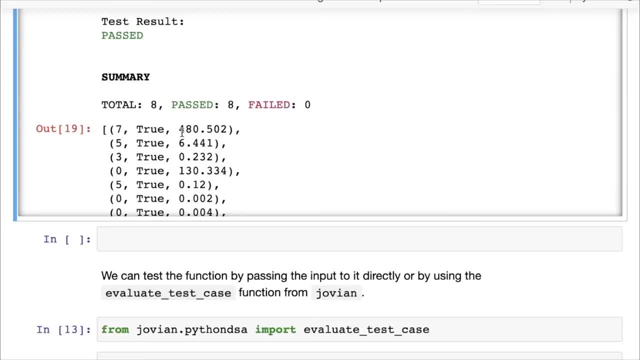 Now that's still a bit high. I would say the four, 80 milliseconds, because we are just looking at a sequence of serendipitous and precipitation which are of very short Length If you're looking at a really long sequence, for instance this: 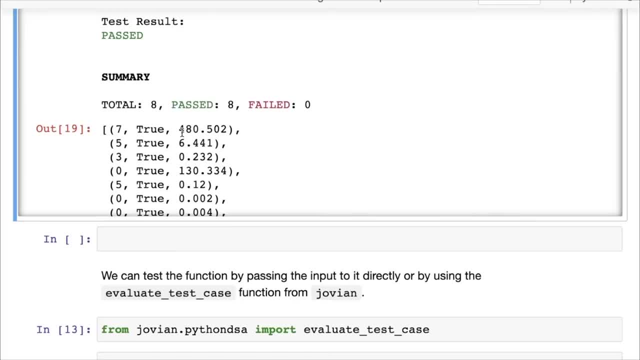 This technique is used for DNA sequencing and we were looking at two DNA strands, uh, or two DNA, two DNA strings, and trying to get the common subsequence out of them. And these can go into thousands or sometimes millions of elements. that would make it rather slow. 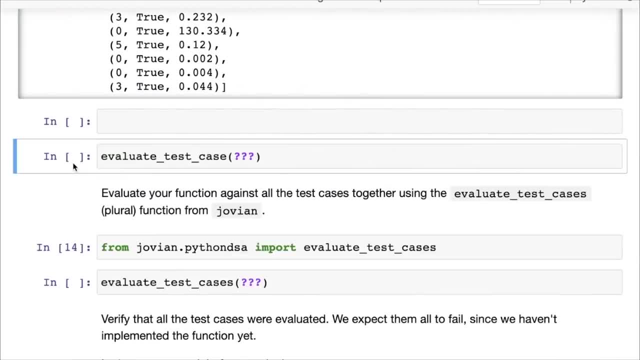 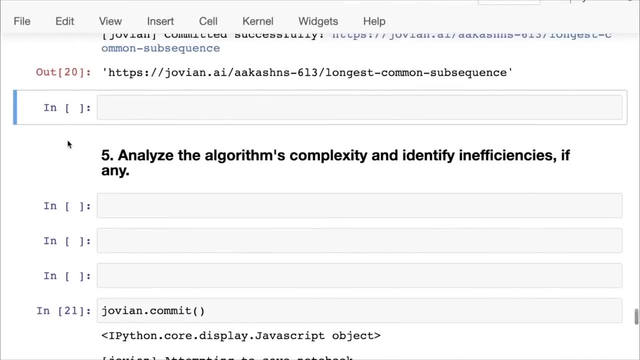 Okay, So we do want to improve this algorithm further, but let's do that, And before that we can just commit our work once again. Uh, but the first thing before we improve Is to analyze its complexity. How long does it really take? 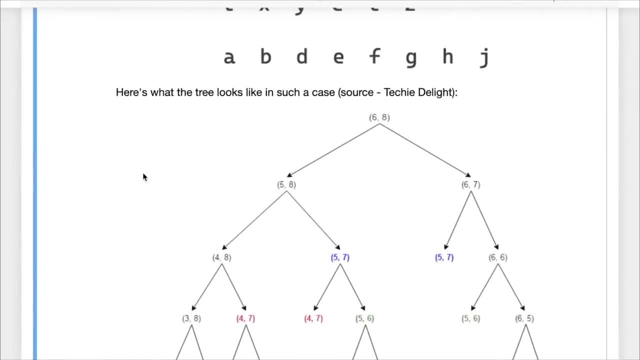 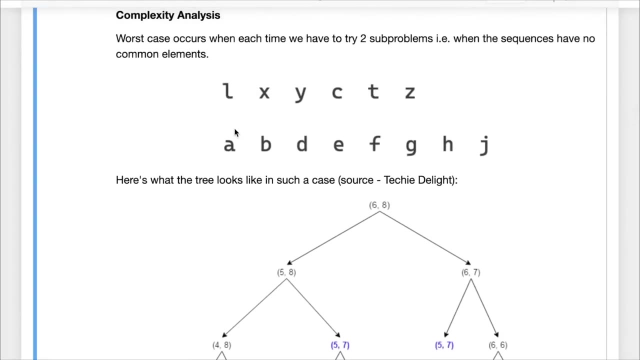 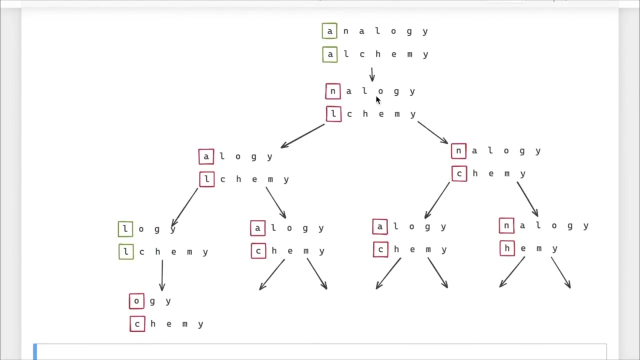 Okay, And identify any inefficiencies. now to analyze the complexity, Let's look at an example and, uh, let's consider the worst case. Now, when does the worst case occur here? We've seen that if two elements match, then we simply have one sub problem or one recursive call. 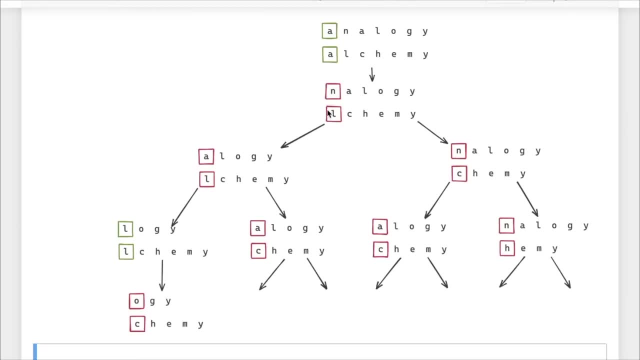 But if the two elements- are two elements of the sequences- don't match, then we have two recursive calls. So if you have two Completely distinct sequences where none of the sequences, none of the elements match, then each time we will end up with two sub problems. 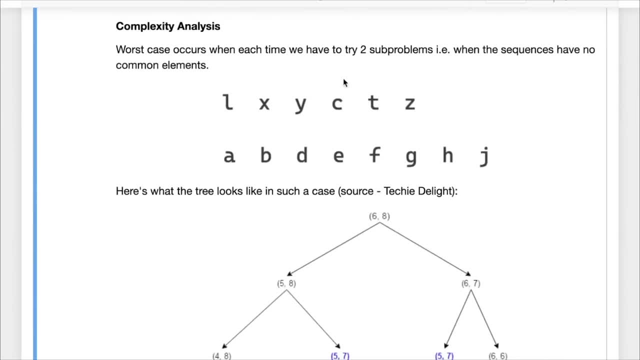 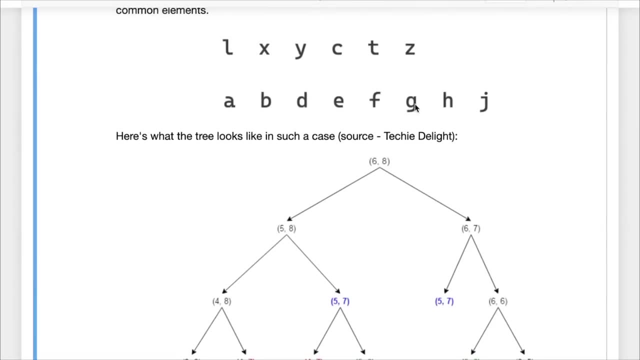 So that becomes the worst case. So the worst case occurs each time we have two sub problems where the sequences have no common elements. And here's an example. This is a sequence of length six. Here's a sequence of length eight, and this is what the tree will look like. 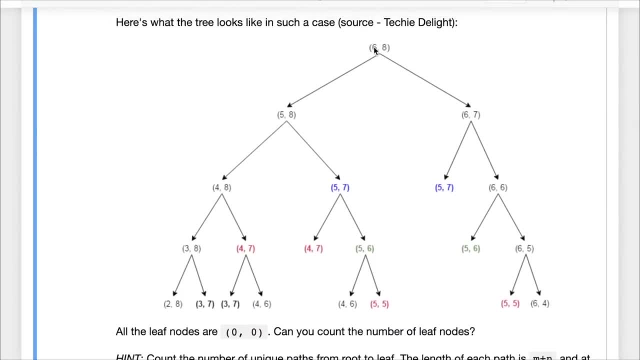 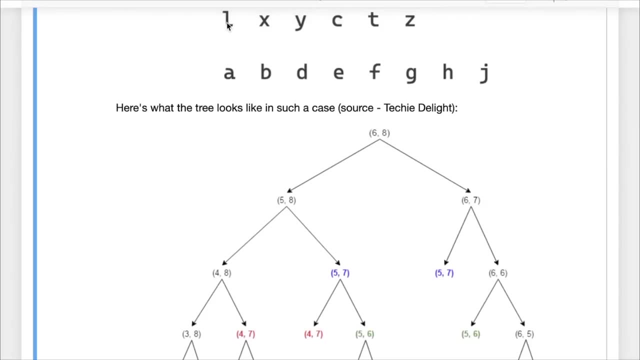 So now we have no longer put the actual sequences, We've simply put what is the length of the string that we started with. So here we started with strings of length Six and eight, And then we say that we either ignore the first character of the first string or the first sequence, or we ignore the first element of the second sequence. 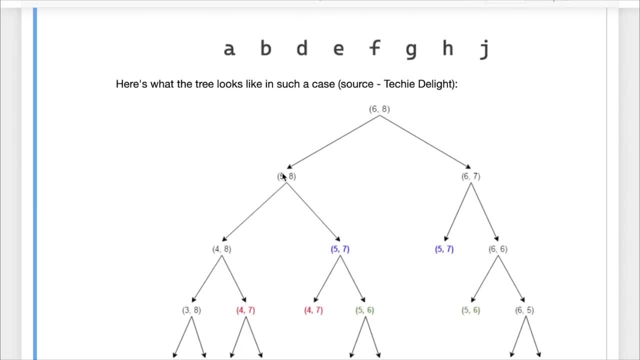 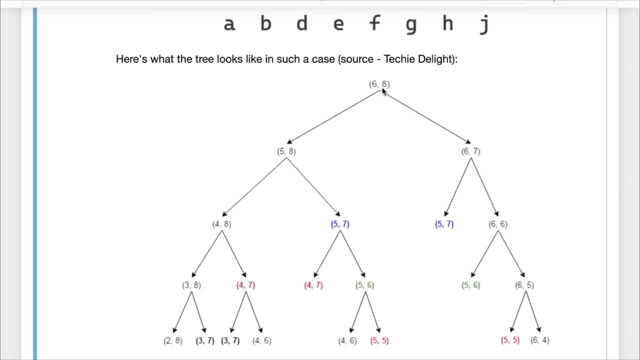 And that gives us two sub problems. And this time the sequences have length: five and eight in this case, and six and seven in this case. Okay, So we either reduce one from the left or we reduce one from the right. And once again here, we either reduce one from the left or we reduce one from the right. 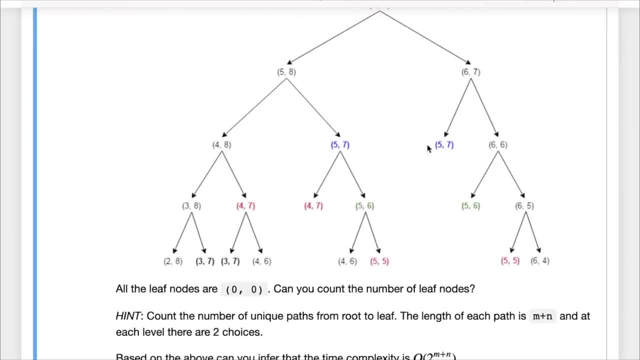 So this way we create a tree, and you can also see that a lot of common trees get created, And that, Really, is what is the inefficiency, And we'll talk about that. but what will happen here is five, seven. we'll then call four, seven and five, six and five, seven here. 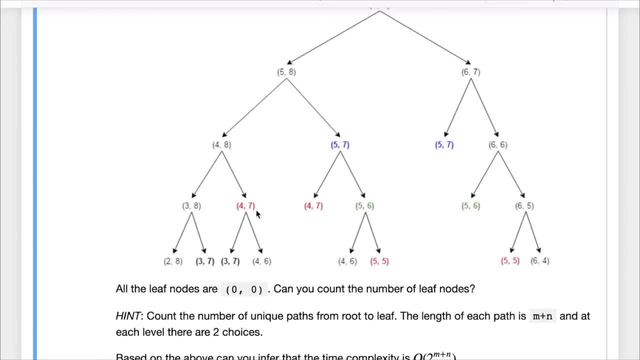 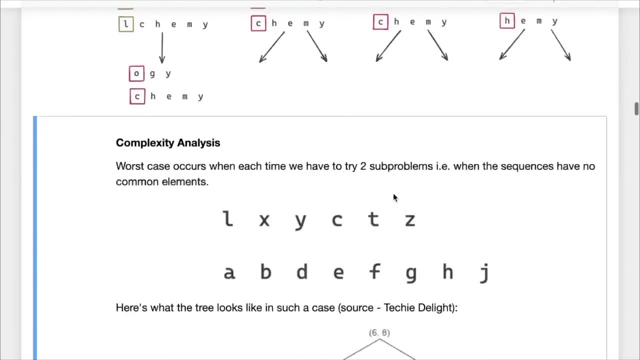 We'll once again call four- seven and five six, and four, seven and four- seven will get repeated here in five- six, and five- six will get repeated three times here. So there's a lot of repeated calls that are going to occur. 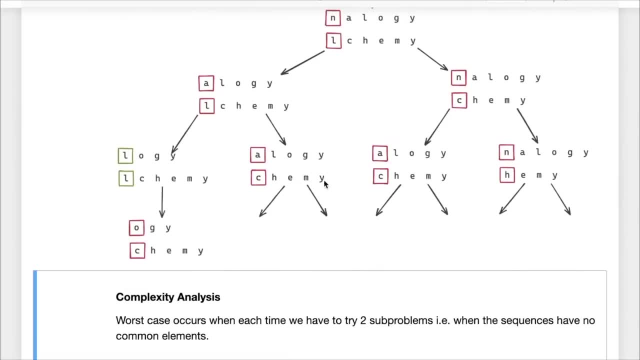 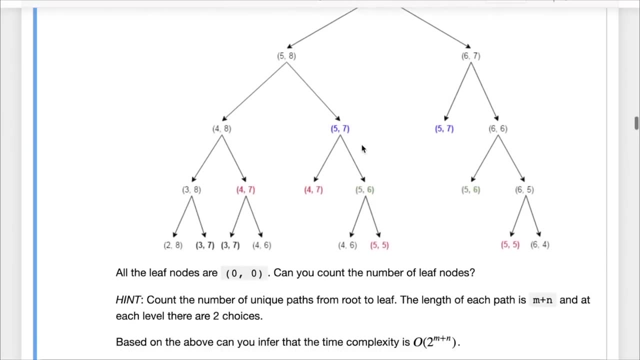 And you can even see this here at the top. you can see that a L O G Y, the problem was called repeatedly: Um, so that's really a source of inefficiency. but Now the question becomes that we know that all the leaf nodes will end at zero, zero. 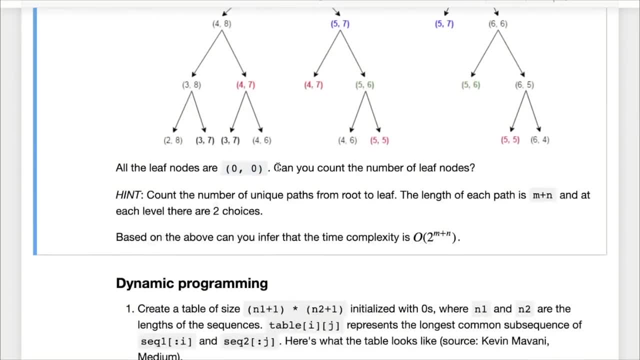 That's when the entire three ends. So can you count the number of leaf nodes? Okay, Can you count the number? If you keep expanding the street, completely expand each of these, don't skip any of them. Can you count the number of leaf nodes? 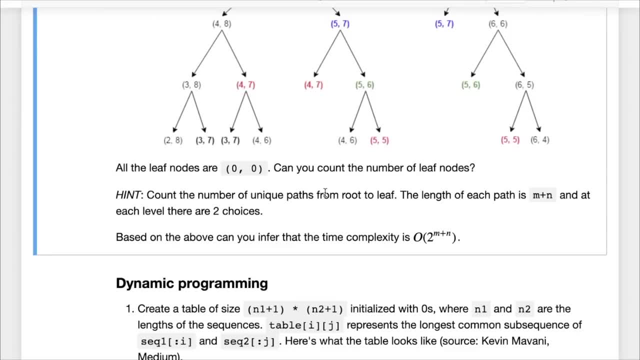 Now, if you count the number of leaf nodes, we know that in a binary tree the number of leaf nodes, if the number of leaf nodes is L? um, then the height of the tree is Oh, if the number of leaf nodes is end, then height of three is log N. 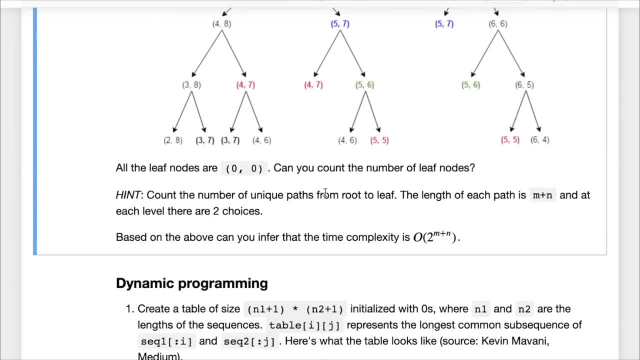 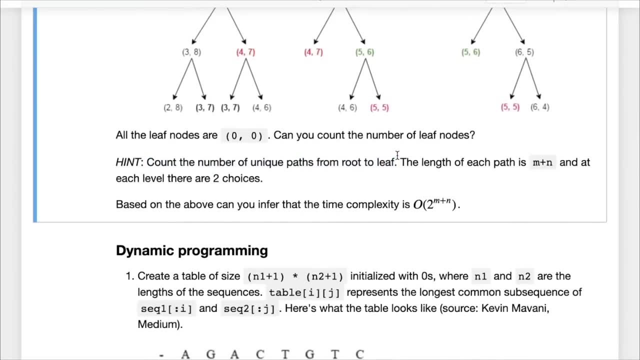 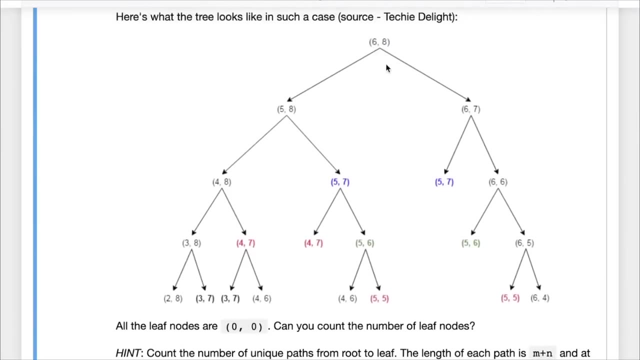 And based on that we can actually determine the actual size of the tree as well. So we know that to count the number of unique parts from root to leaf will give us the number of leaves right. So each time we have two choices: we either reduce from the left or we reduce from the right. 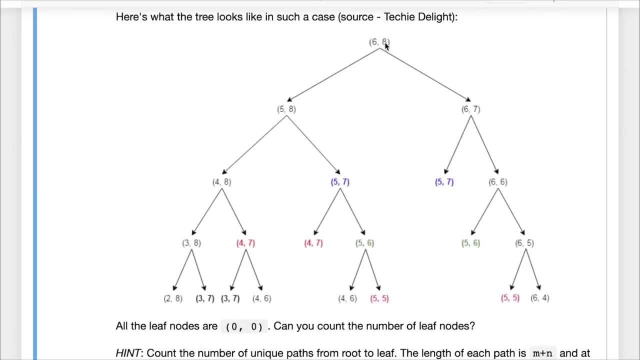 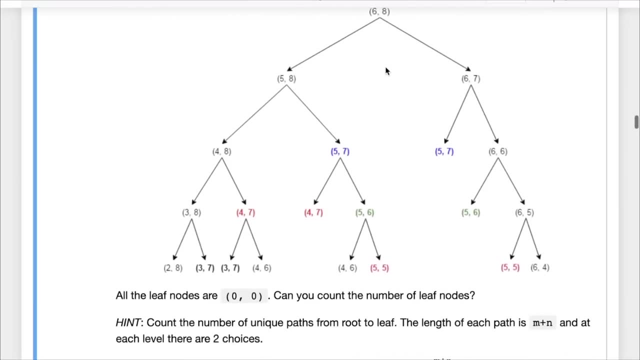 So to get to zero, zero, we would have to reduce all the elements from the left and we would have to reduce all the elements from the right. That means if you have strings, Or if you have strings of length or sequences of length, M and N, then you would have to make M plus N choices in total. 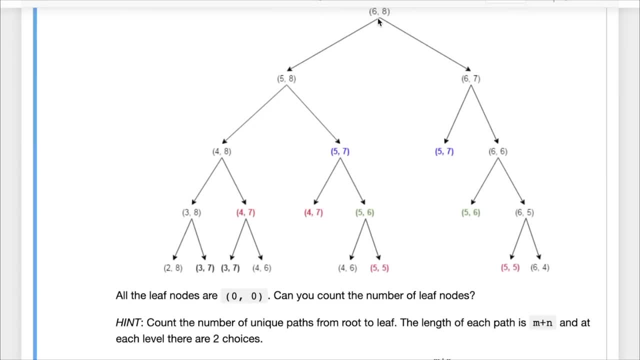 And so each time you have M, you have to make M plus N choices. And each time you have to choose whether you want to reduce from the left or from the right, you have two choices And you have to make those two choices M plus N times. 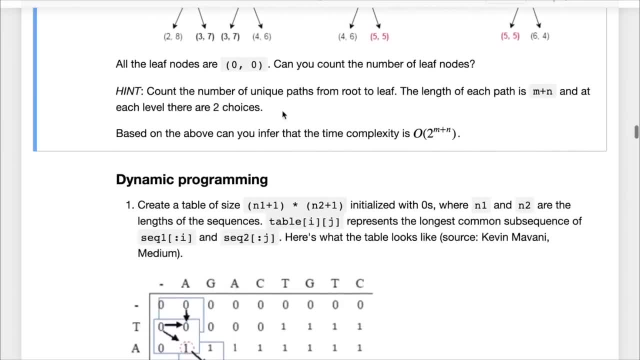 That's the right way to put it really. So that means each time you come you do two choices. So you have to multiply it by two, multiplied by two, multiplied by two, And you keep multiplying that and you will end up with two, to the power of M plus N leaf nodes. 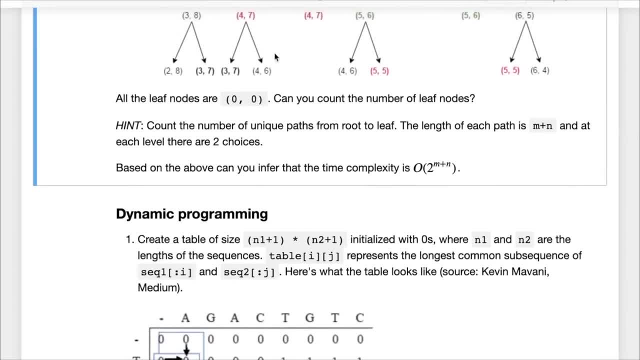 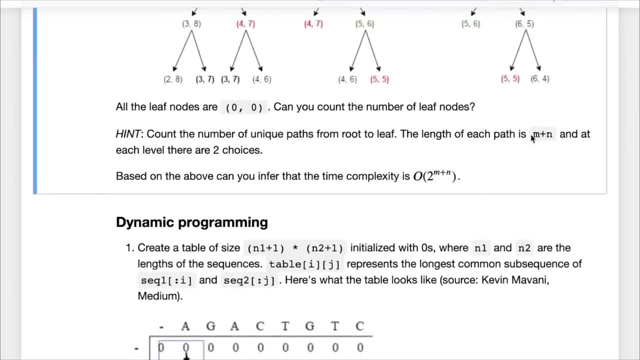 Okay, So here is an exercise for you: draw this tree on a piece of paper, Mark out how the number of leaf nodes, how the length of each part is M plus N, Figure that out And based on that can you conclude that it takes two to the power of M plus N leaves to complete this tree. 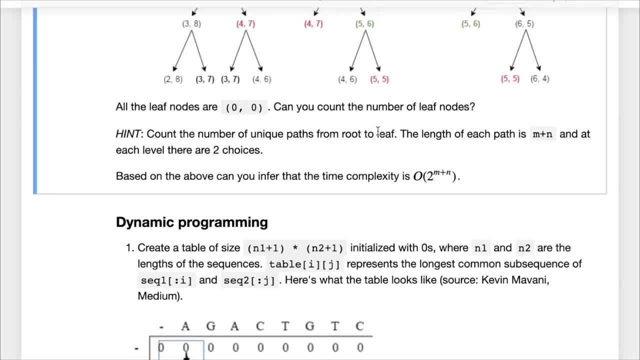 And if two to the power of M plus n leaves, M of M plus N is the number of leaves, Then the total number of elements is in the tree: simply double of that. Once again, this is something that is very easy to verify. 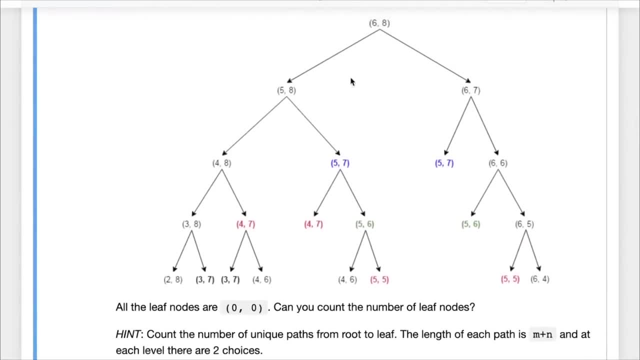 You can check it here. For instance, if you just consider these two levels, the, if you have two leaves, then the total number of elements in the tree is two plus one three. actually it's double minus one, So two into two, four minus one three. 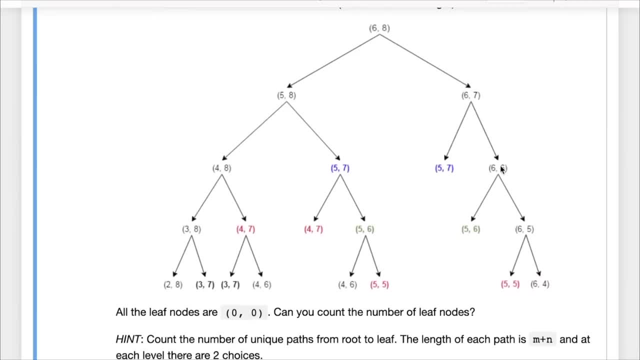 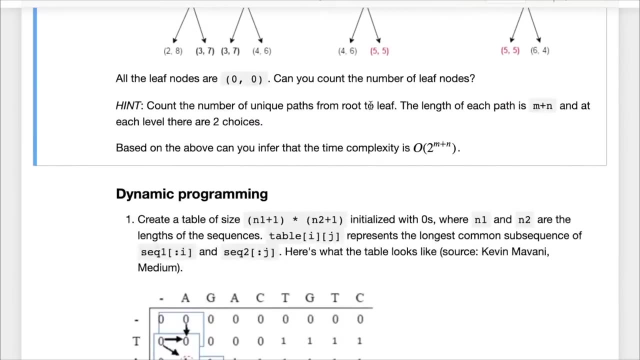 If you have three levels, you can see here that if you have four leaves and the total number of elements in the tree is four, into two, eight minus one, seven, And you can see that here. So it follows essentially that we have an exponential number of sub problems. 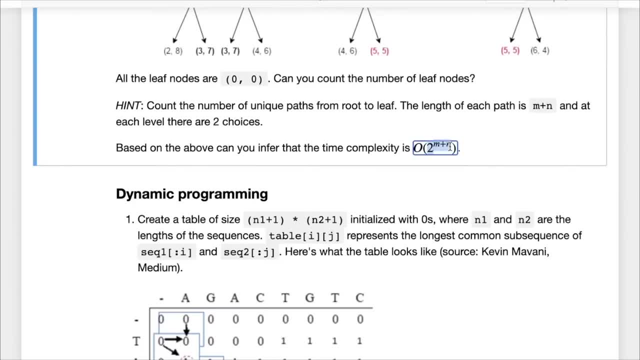 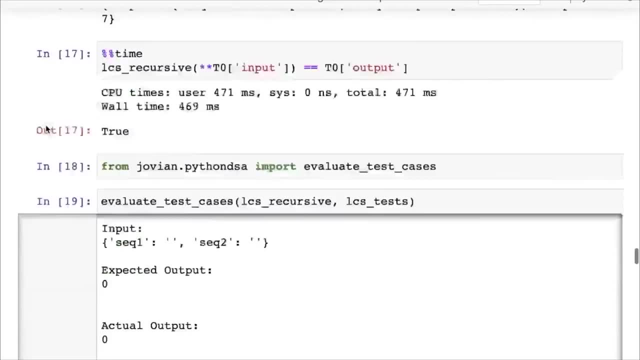 We have, we are calling the recursive function and exponential number of times, And inside the recursive function we are doing inside the recursive function, We are doing a constant time work. So you can see here that there's no, there's no special work that we're doing. 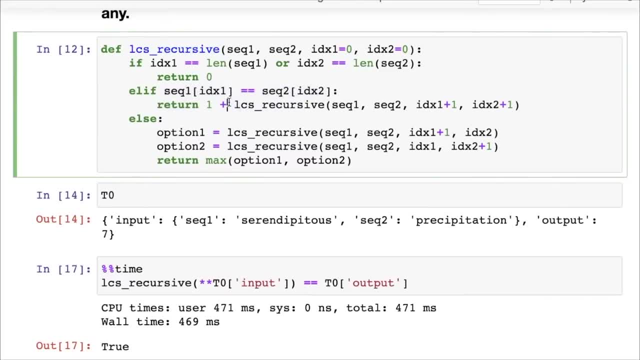 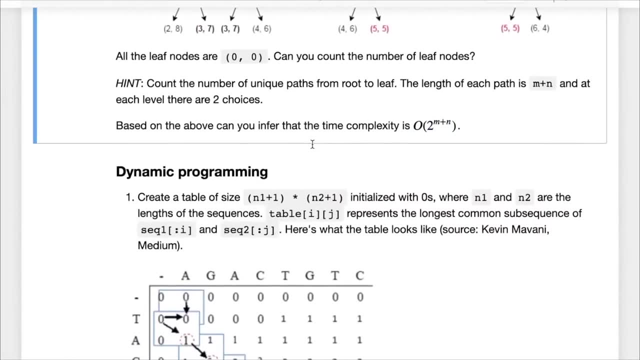 All we're doing is some comparison and we're doing an addition. Both of them are constant time. So we make two to the power of M plus N recursive calls inside each. We do constant work. So the time complexity is order of two to the power of M plus N. 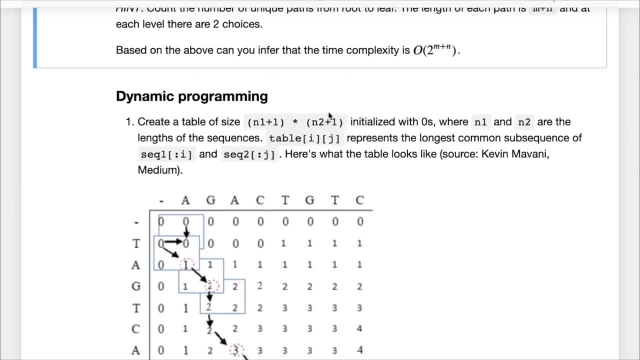 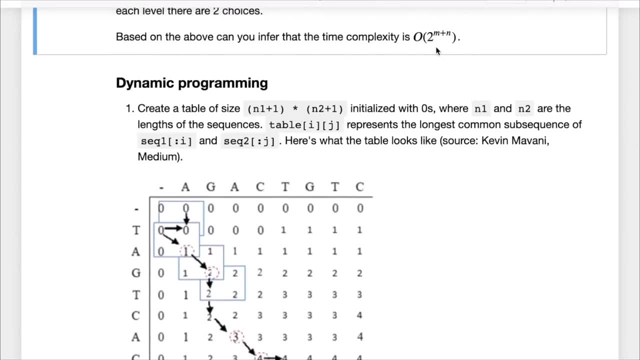 Okay, That's a rough explanation. We've not gone into a lot of depth because we've covered this over and over in the lessons, But the exercise for you is to verify how exactly it is to the power of M plus N. Okay, 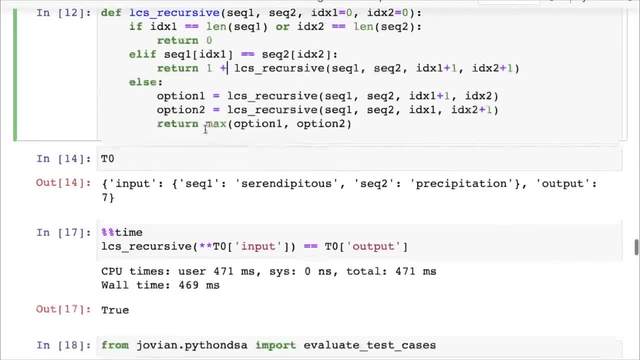 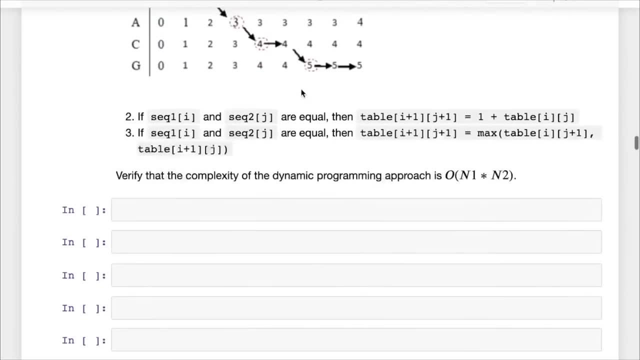 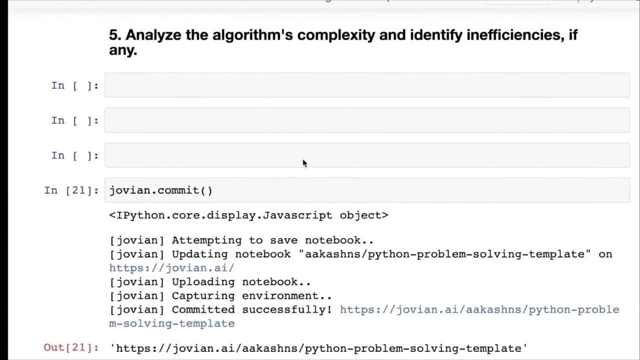 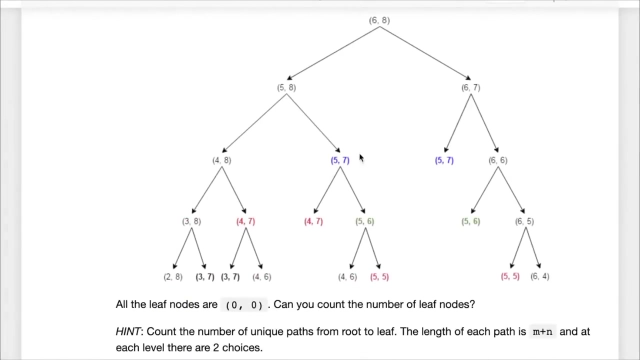 So that's our recursive solution. And we know, we now know that the time complexity is two to the power of M plus N. Let's just copy that over here. And the inefficiency, as we said, in this algorithm is that we are calling the same problem. 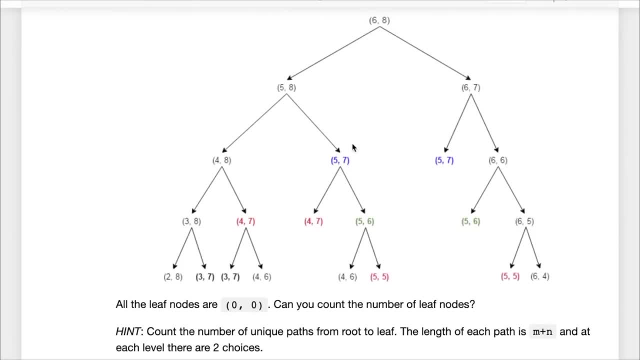 We're calling the exact same problem, though LCS recursive function is called, with IDX equal ideas, one equal to five and IDX two equal to seven and IDX one equal to five and IDX two equal to seven. The same time twice. So each of these sub problems will be called twice. 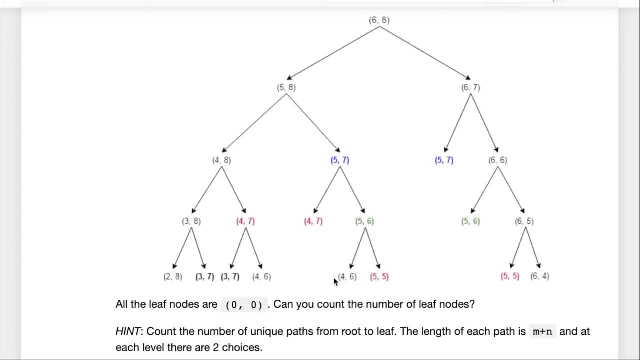 And then each of the sub problems within them will be called twice And, of course, some of these sub problems will once again get shared. So there's a lot of repetition. Now there's a simple solution here, which is simply to remember some of these results. 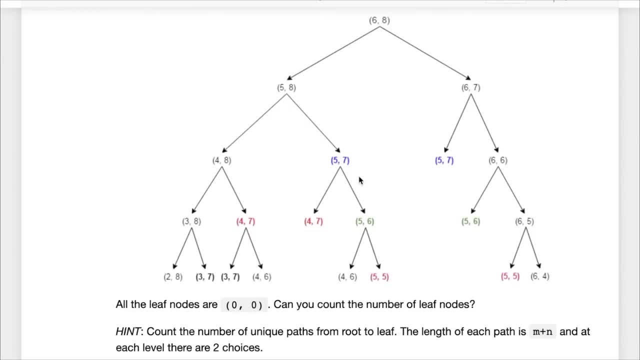 Okay, And this technique is called memoization, And you may also just call it memorization, because you're just remembering some of these things, but memoization is a technical term for it And we remember These solutions in our dictionary called memo. 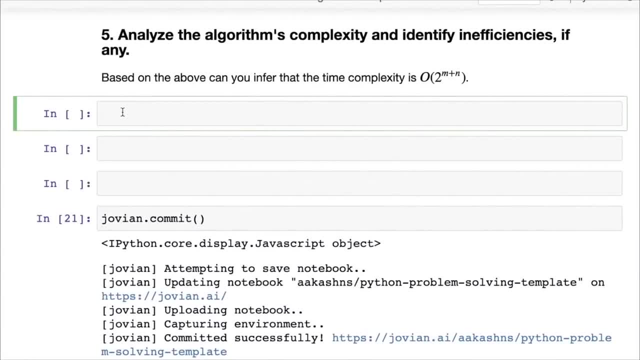 So what we're going to do is we're going to follow the same recursive strategy, but this time we are going to maintain a dictionary called memo and we're going to track intermediate results within the dictionary, And if we find an intermediate result already exists in the dictionary, then we will not compute it again. 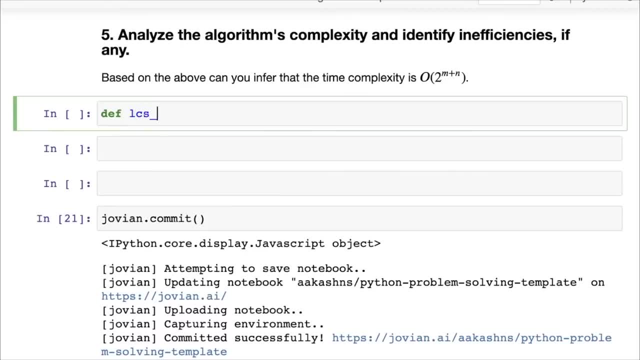 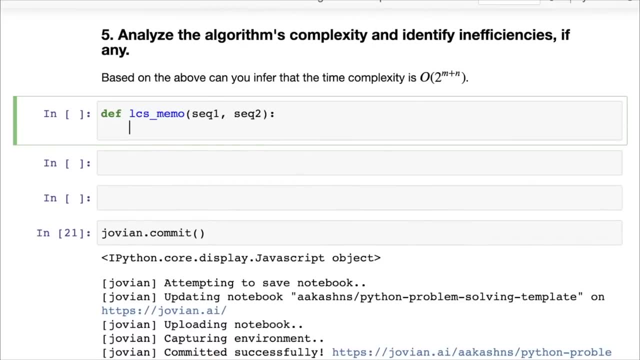 Okay, So let's see. So now we write LCS memoized, or let's just say LCS memo for short. it takes a sequence one, and it takes a sequence two, And this time we create this dictionary called memo, and then we write a function inside it. 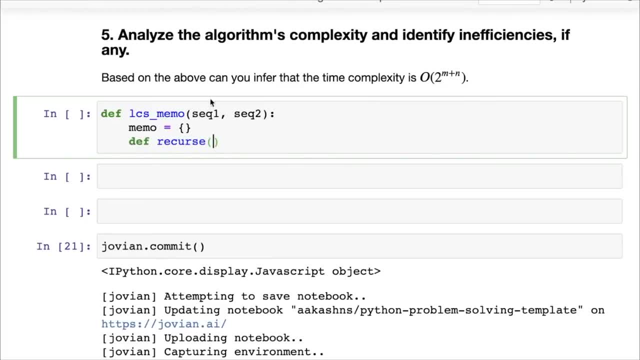 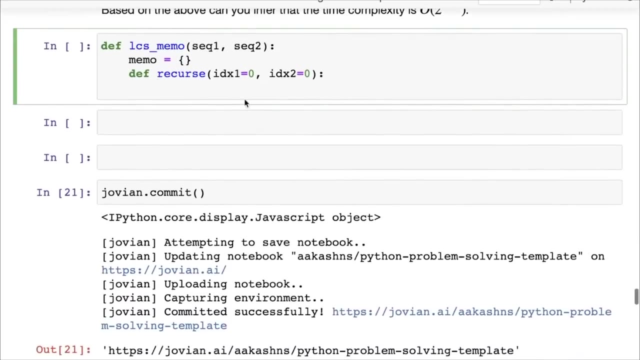 So we will write a helper function, a recursive helper function, inside the LCS memo function, so that it has access to sequence one and sequence two, And we will simply start it out with IDX one as zero and IDX two as zero as well. IDX one will track the position in sequence one. IDX two will track the position in sequence two. 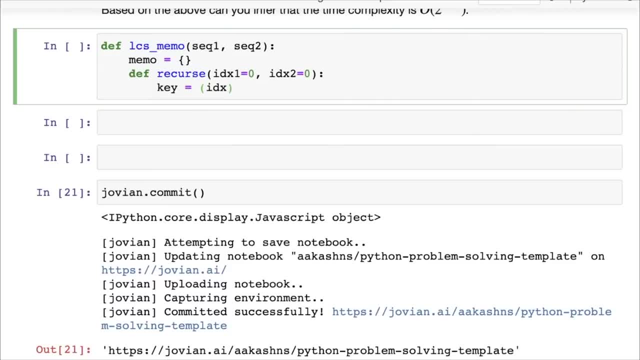 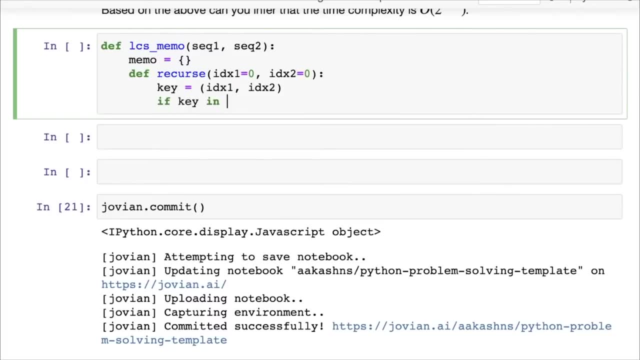 Now the first thing we do is Create, using the two indices, create a key. So we are going to create the key IDX one comma, IDX two, And if the key is present in the memo. so this is the way to check. 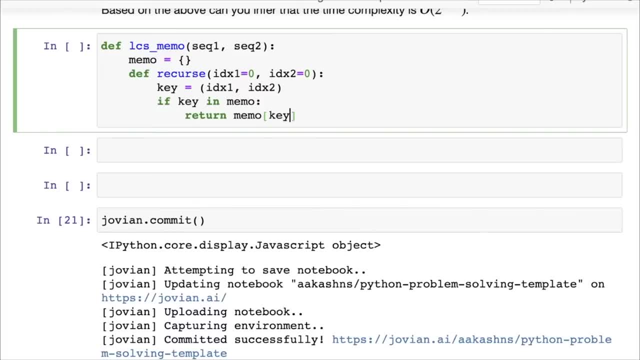 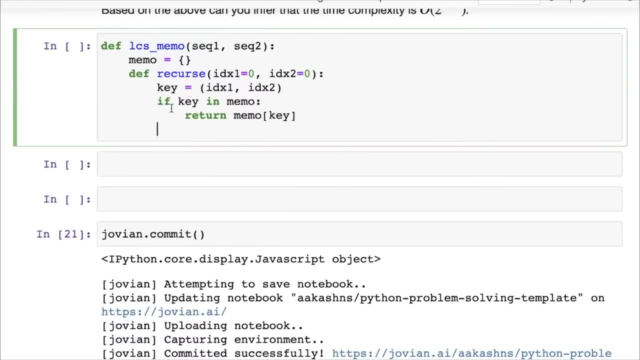 If a key exists in a dictionary, then we simply return memo of key. Simple: The problem is solved. We don't have to solve this problem because it's already. it's already something that we've solved. If it isn't, then we need to solve the problem and save it in the memo. 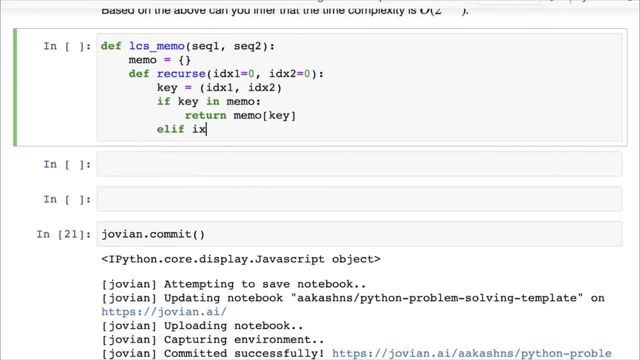 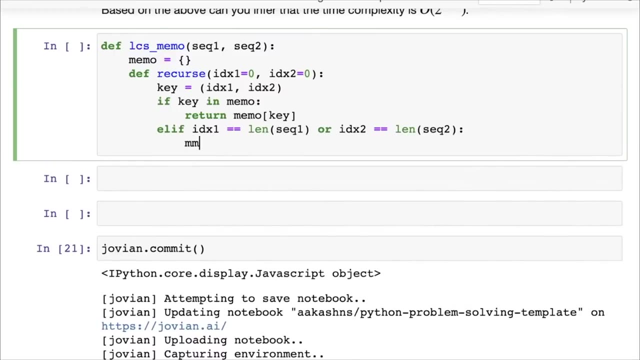 Now, here we know that we can now write our Same three recursive cases. Now, if the base case, if IDX one is equal to the length of sequence one, or IDX two is equal to the length of sequence two, then we simply set memo of key as zero, because by this point we have reached the end of the strings. 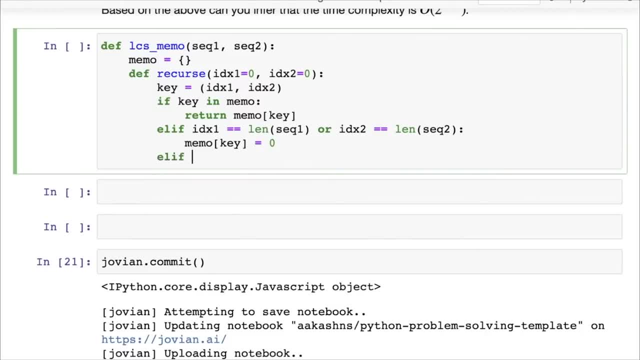 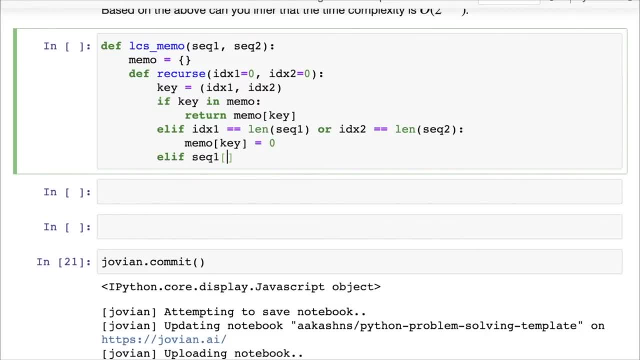 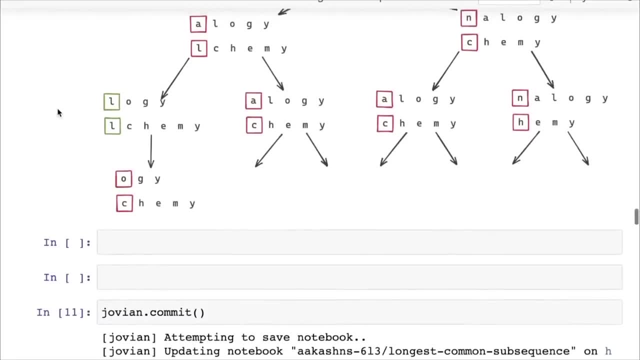 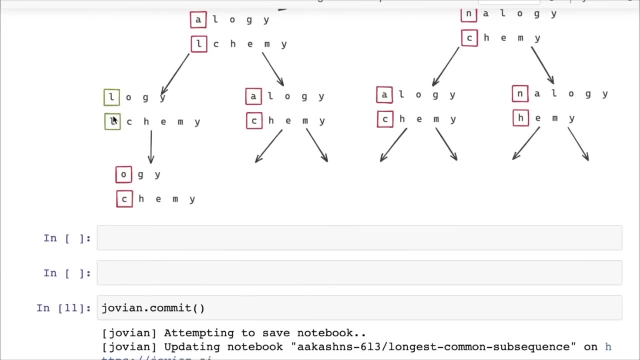 So this is if you go up here and look at the tree once again, this is a case like this, where the current characters that we are pointing at are equal. So in that case, we simply return, we simply get the result as one. 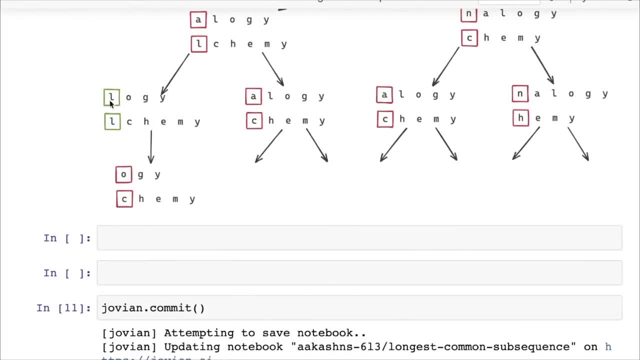 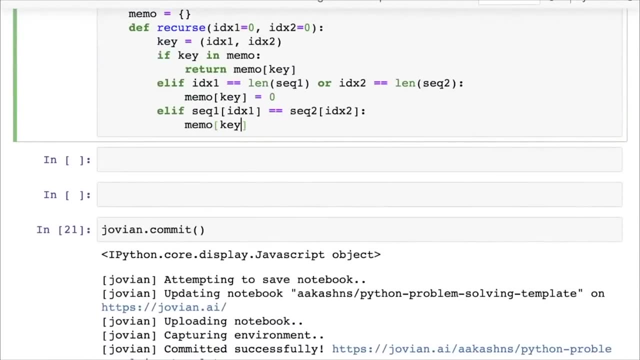 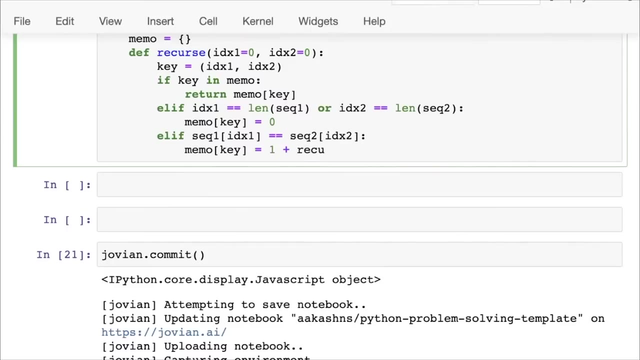 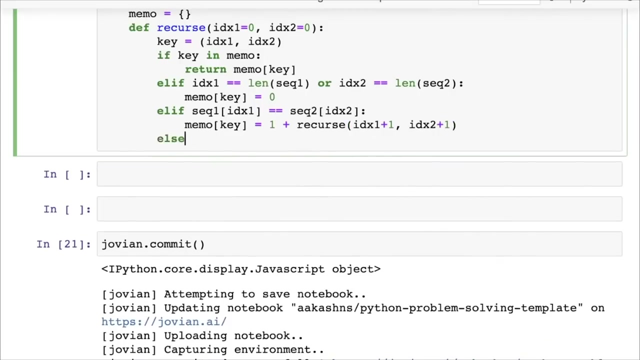 Plus The result for the remaining, with the first character removed. So in this case we simply set memo of key to one plus we call the recursive function again recurs: IDX one plus one and IDX two plus one great else. So this is a case where the two elements are not equal. 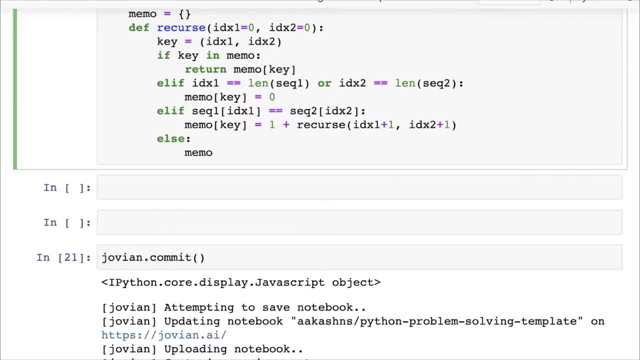 And this is where we have two options. So I'm not going to write the two options separately. Let's just do a max directly here. max, And we say: records with IDX one plus one, comma IDX two and records with IDX one comma IDX two plus one. 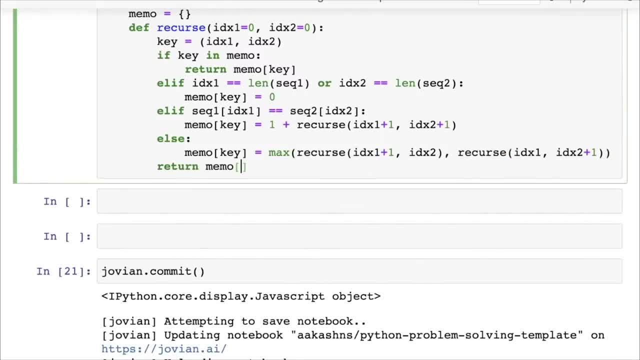 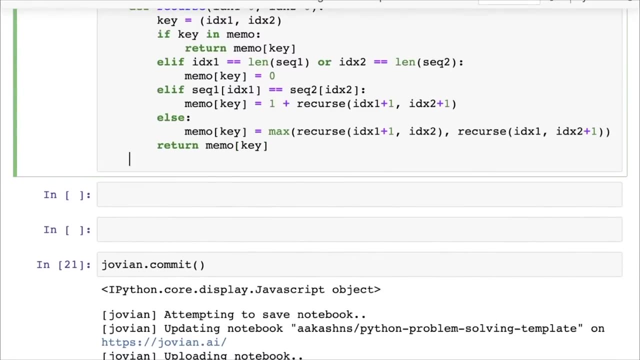 Okay, And finally, from the records function we return memo of key. So we have, whichever case it is, we have computed the result and saved it Okay In the memo. So this time these computations will not get repeated again and again and 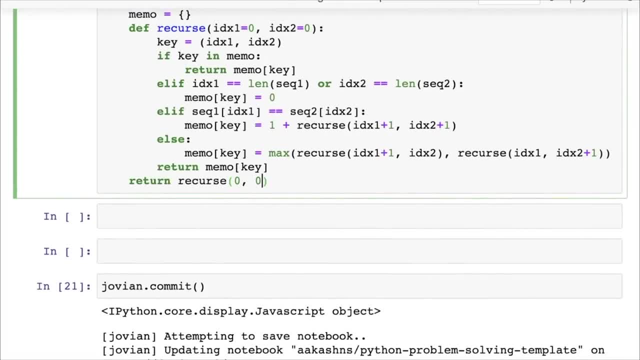 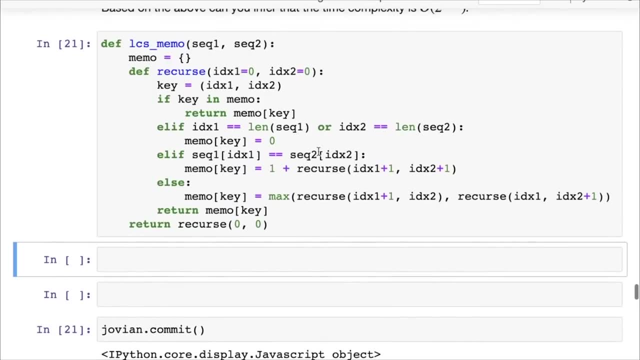 let us now return recurs of zero comma zero, because zero comma zero is the entire string and that's it. And this is the common strategy that you should apply Whenever you come up with a recursive solution and you see the inefficiency coming because of the same problem being called again and 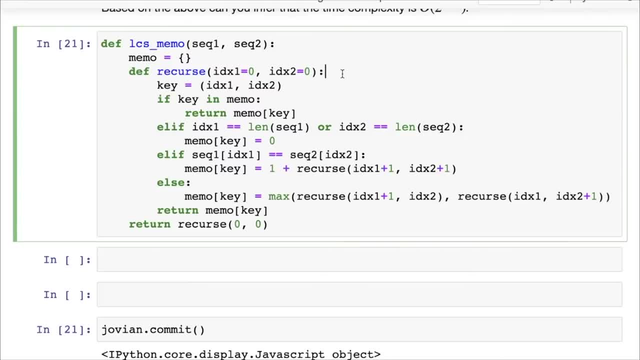 again and again. this is where you need to apply this technique called memoization right, And in this technique you will then be able to simply store intermediate results. So it's really simple: You just create a dictionary and then you add one or two lines of code here and 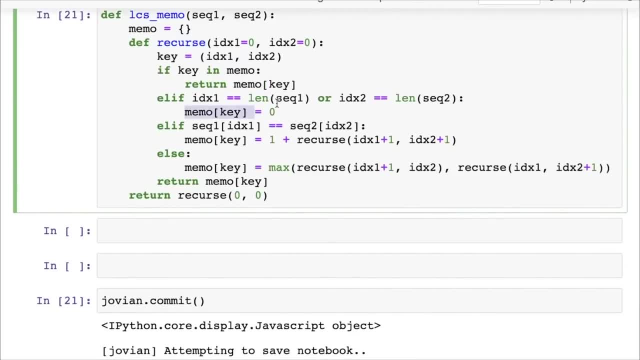 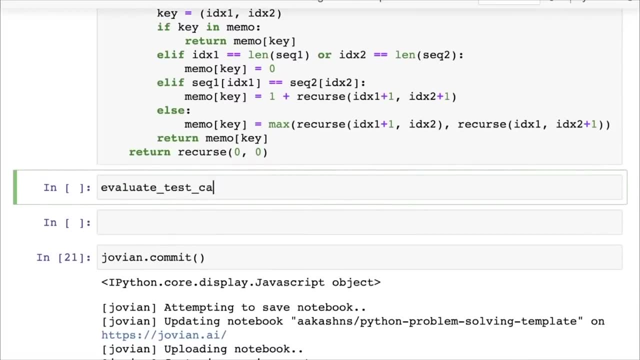 you make sure to save the result in that dictionary Whenever you compute a result. the next time you don't have to compute it. Okay, And we can test it out. We can test it out with all The test cases. evaluate the test cases, the LCS memo and LCS tests. 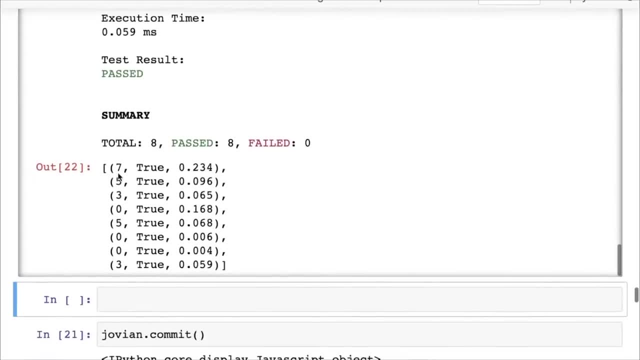 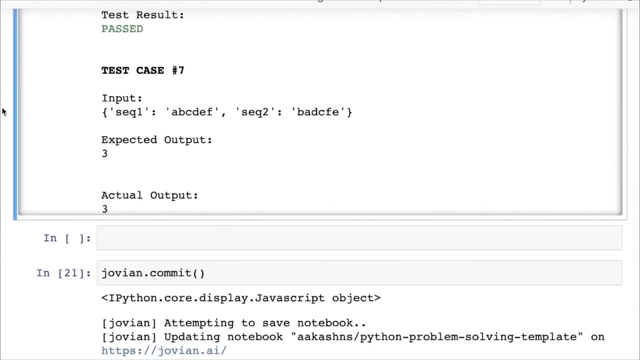 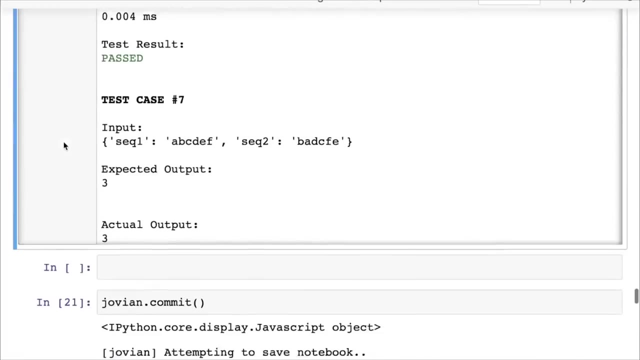 And you can see that all the test cases pass. Now, not only do all the test cases pass, you can see that the time taken is now lower. Okay, So that's nice. The time taken is now lower. Now we went from 450 milliseconds. 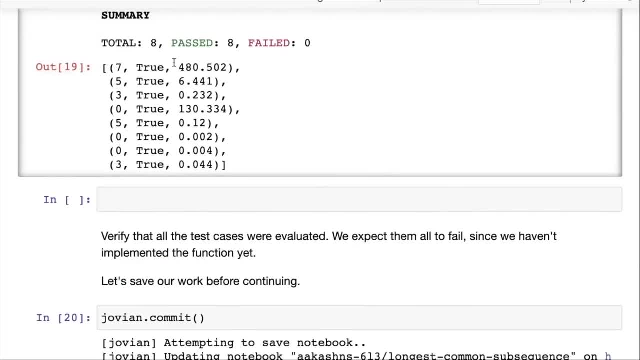 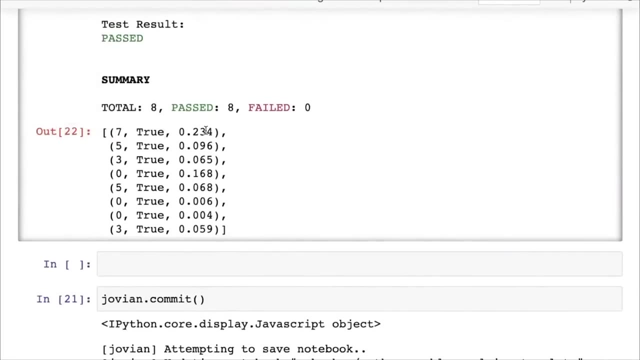 If you just go up here you can see that it took 480 milliseconds for the for finding the longest common subsequence between precipitation and serendipitous, But in this case it only took about 0.234, which is 0.2 milliseconds. 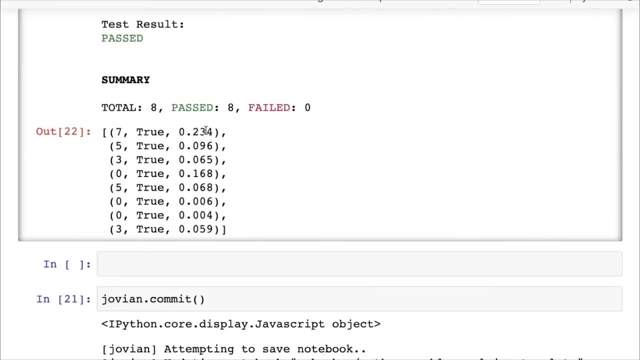 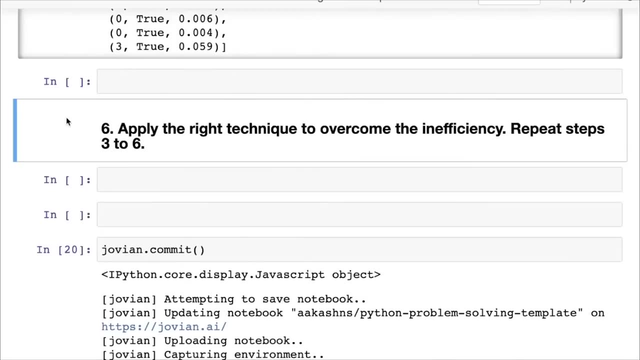 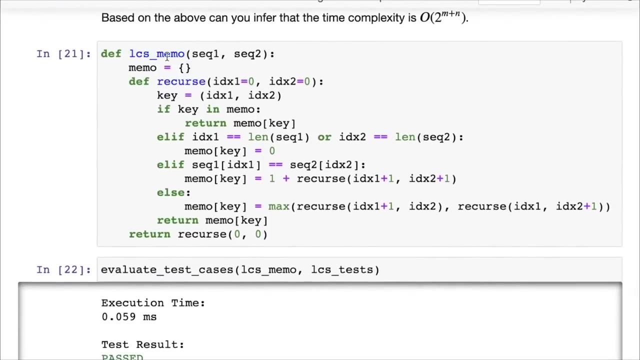 So it is 2000 times faster, even for strings of length seven or eight, And that's a huge boost. Let's analyze the complexity here. Let's look at the complexity Now. a quick way, an easy way to find the complexity of the solution is to see where the computation 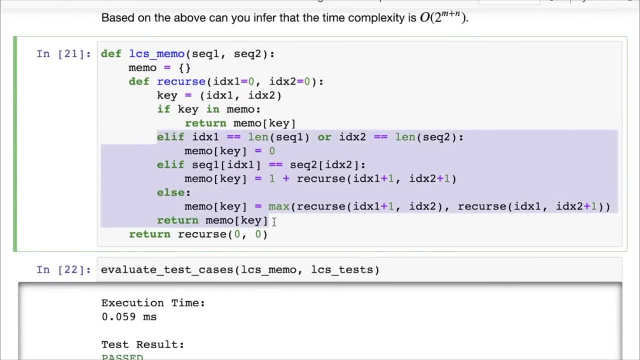 how many times the computation can occur. Now, this is where the bulk of the computation is occurring in a recursive call, And this computation is avoided if we already have something in the memo. Okay, So that means that the only number of computations that we need to do is equal to the maximum number of elements that can end up in the memo. 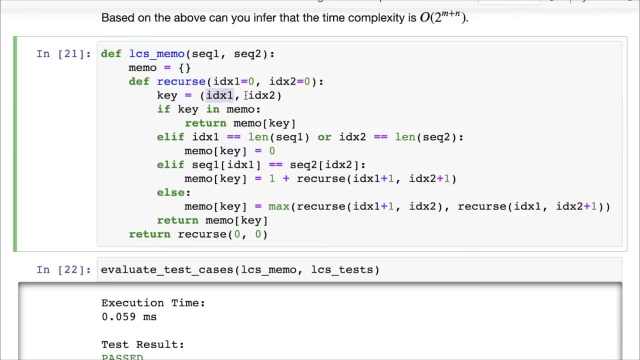 Now, what are the keys in the memo? look like The keys in the memo. look like IDX one and IDX two. Great, And what values can these take? IDX one can take zero to M values If M is the length of sequence one, let's say an IDX two can take zero to N values. 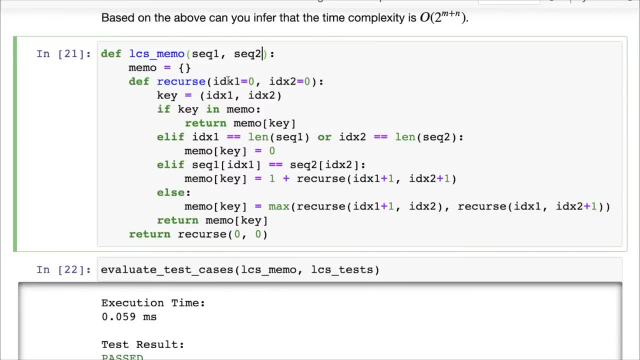 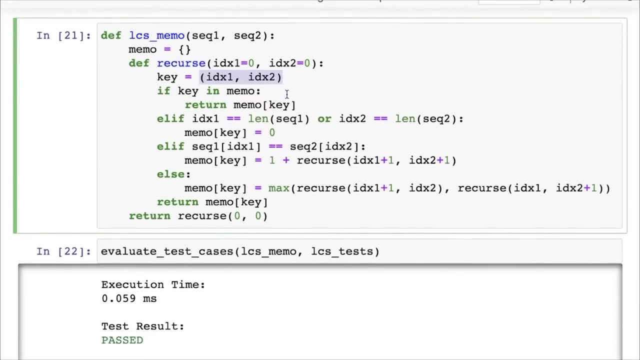 If N is a sequence, a length of sequence two. So in total, the possible number of keys is M times N. The possible number of keys is M times N. The possible number of things that you need to store in the memo is M times N. 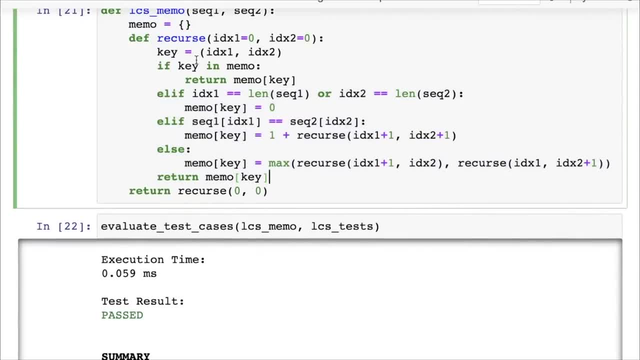 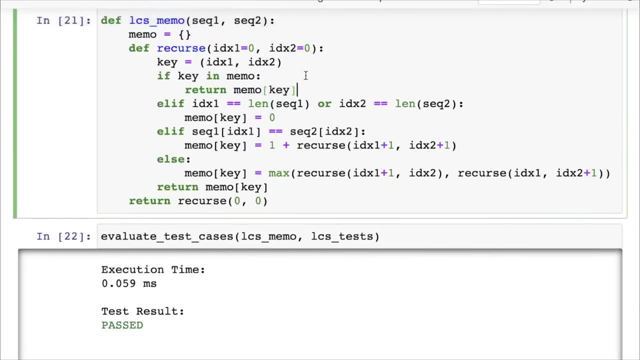 And for each of them you do constant work, And then the next time you try to access this, you do not need to do the work, You do not need to call any recursion, You can simply access the memoization right. So what that tells us is the complexity of this case. 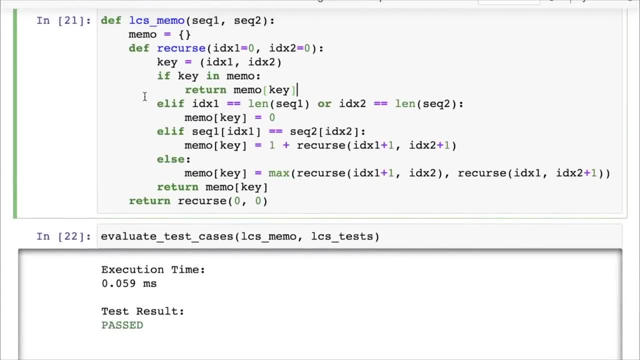 Okay, And in any memoization case in general, is equal to the number of keys, which in this case is M times N. So the time complexity here is order of M times N. So we've gone from two to the power of M plus N, which, if you, if M plus N was, 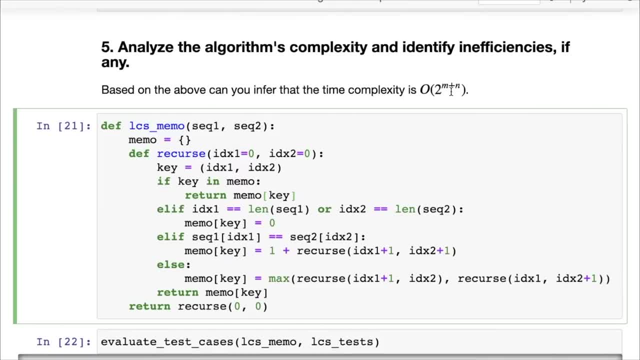 equal to 30 would be 1 billion to M time. order of M times N. So let's say both strings were 15 and 15, but that would just be 225 operations. So we've gone from 1 billion operations to 225 operations simply by storing intermediate results. 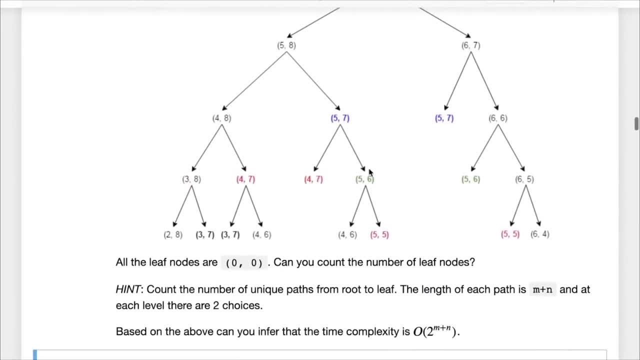 And it's a very powerful technique that we apply all the time. So now you can see here that the first time five seven is computed, The next time five seven does not need to be computed again, And that's why this tree here is actually marked out. 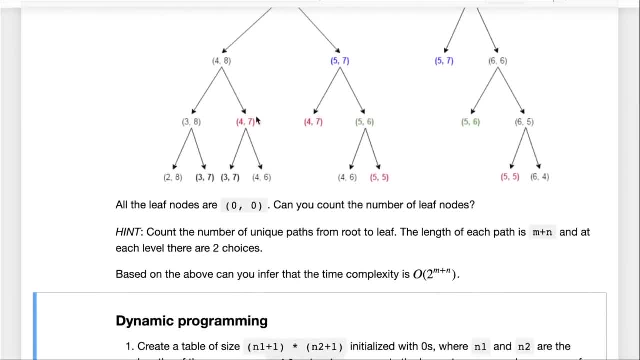 So this is the tree for memoization. This is the first time four seven was computed. It never needs to be computed again. So this entire tree of computation gets eliminated and similarly this entire tree of competition Gets eliminated. We are eliminating from 1 billion computations almost all except 225 computations. 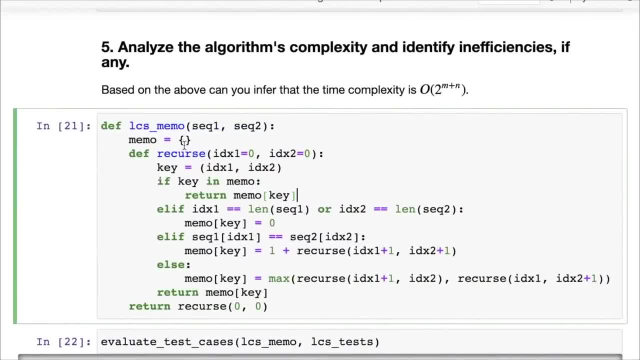 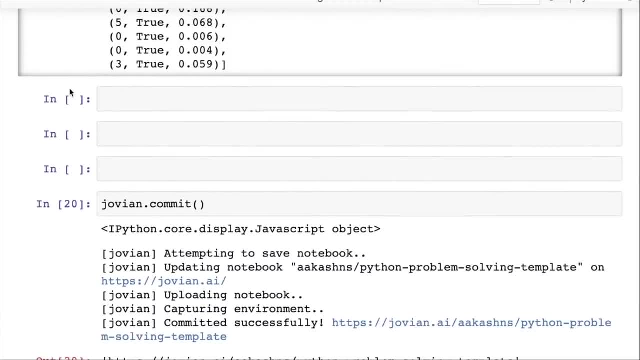 So we are left with practically nothing, And that speeds up your algorithm by a huge, huge factor. So that's memoization And, as he said, it's really easy to compute the time complexity of memorization: Just simply count the number of keys and then just track. how much work do you need to? 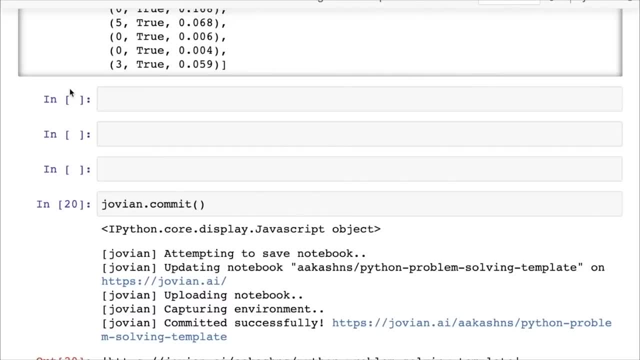 compute Each key, assuming that you already have the recursive solutions for the remaining. Okay, So how much work do you need to compute each key using some other existing solutions? Now, in this case, that was constant, because all we needed to do was compare and add. 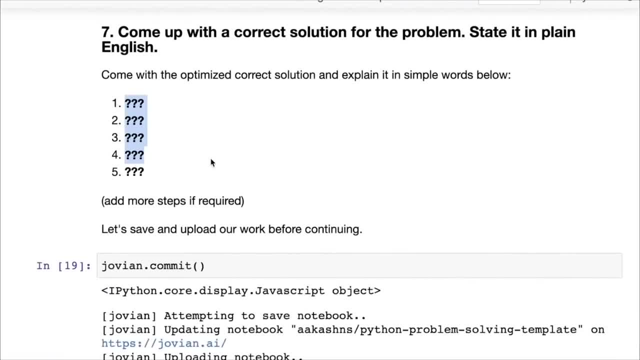 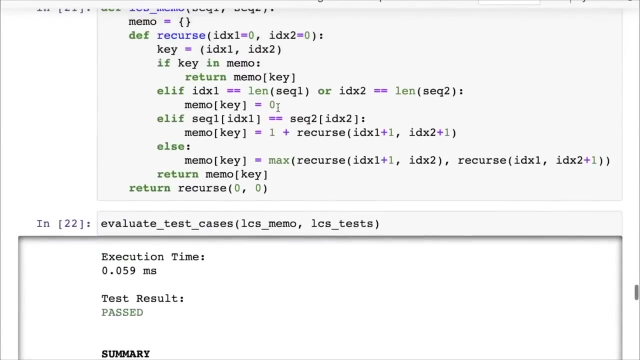 Okay, And I let you write here a simple, optimized, so plain English explanation of memorization. It's worth a. it's a good exercise to try, But what we will also look at is another technique called dynamic programming, And the downside with memorization is that it requires recursive calls. 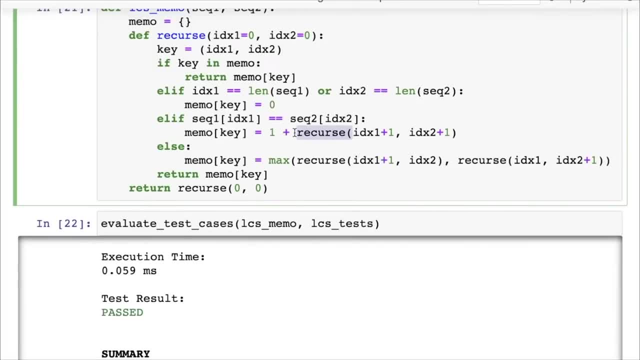 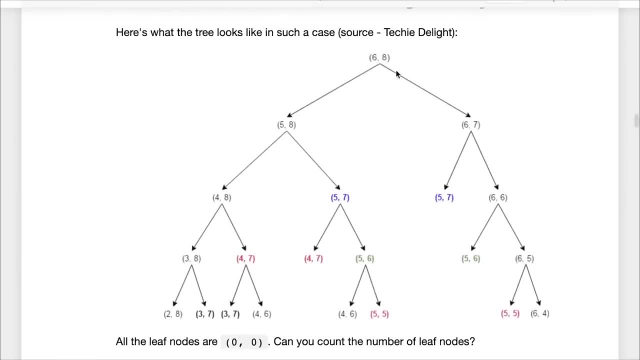 And while it's not a problem for small cases, when you have really large problems, the recursion has an overhead and the overhead for a question, If you see this way, is that for this function execution to complete, you need this function execution to complete and this to complete. 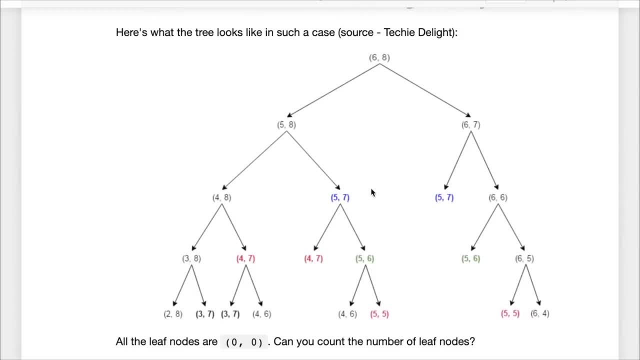 And for this to complete, you need this to complete and this to complete, right? So the idea here Is that for each new recursive call takes more space in the memory And it also takes longer because now we have to allocate some memory and then set up that. 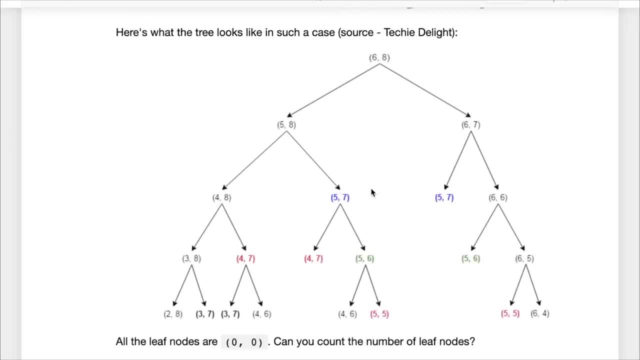 function stack, the function stack for the execution of that function. So if you have a large tree, then you're creating hundreds, thousands or possibly millions of open functions, all of which have their own memory, and that can eat up a lot. 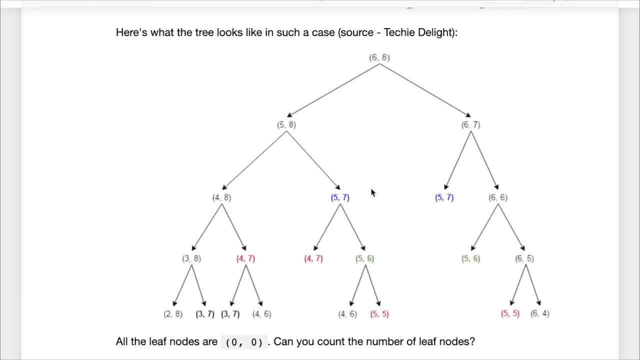 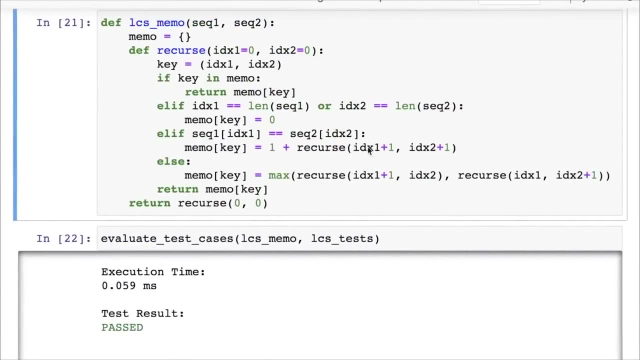 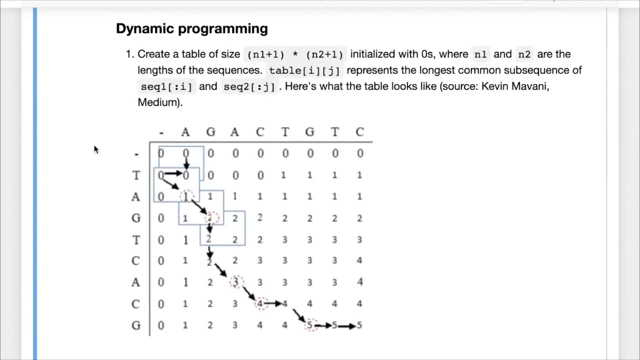 of memory And sometimes that can also take up a take longer time. So the solution to replace recursion is iteration. And how do we do that? We do that using a technique called dynamic programming. So we'll do almost the same thing. There are a few changes here. 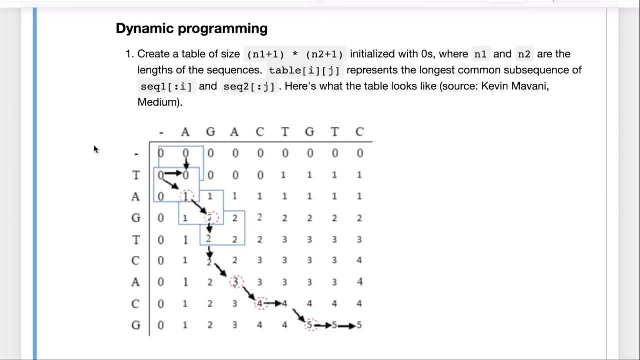 Instead of using a dictionary to track intermediate results, we will create a matrix, because we know that sequence one, the IDX one, can go from zero to N or zero to N one, let's say where N one is the length of sequence one and C. 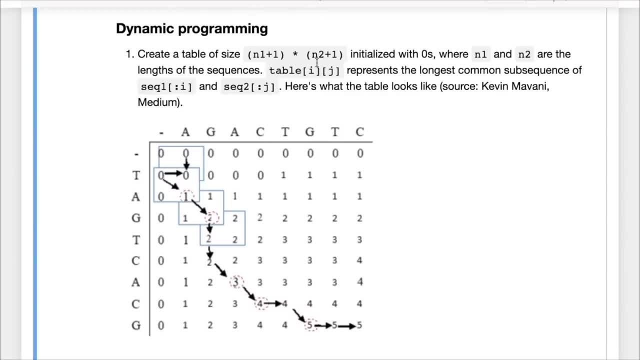 Equal IDX two can go from zero to N two, where C N two is the length of sequence two. And what we can do is we can use a for loop or a couple of for loops to fill out all these sub problems without having to require a recursion. 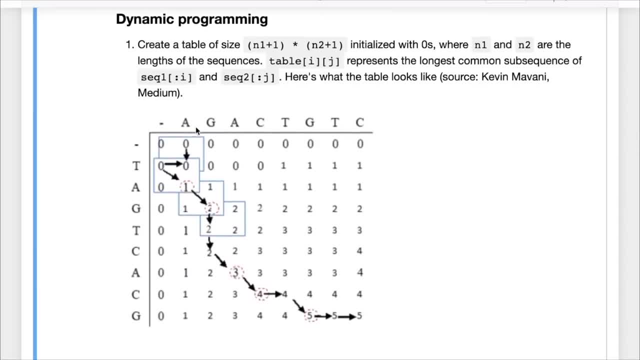 Okay, And this is how we'll do it. So let's say, these are the two strings that we're working with. This is string one, T, A, C, G, T and this is string two. And these: this is what DNA sequences look like. 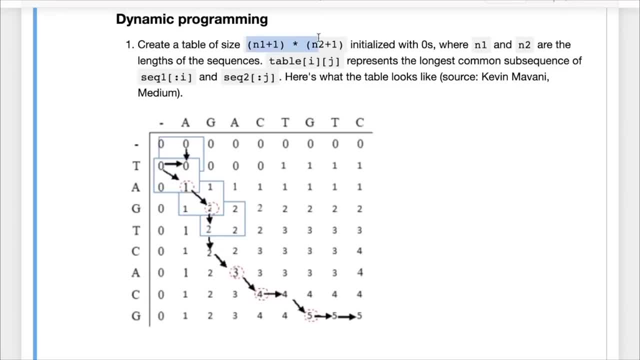 So what we'll do is we will create a table of size. This is N plus one plus one and N one plus one and N two plus one. So you can see that there are N one plus one rules. So if this is of length N one, these are N one rows, and then there's an additional row. 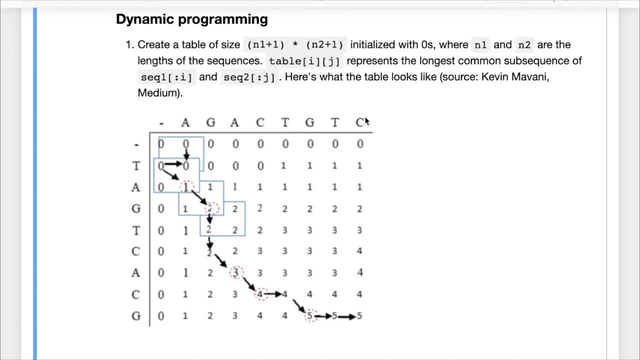 And similarly there is there are N two plus one rows here. So if this is of length N two, there are. there are N two plus one columns. So you can see these are N two columns and there is an additional column here and table of ING. 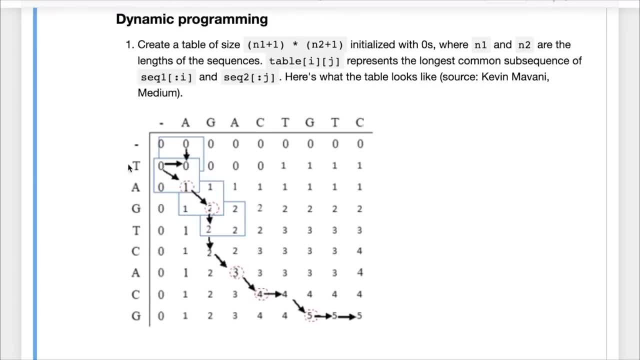 So let's say, table of uh, N and J are zero. So I is a pointer for the first sequence and J is a pointer for the second sequence. So I selects a row and J selects the column. So table of INJ represents the longest common subsequence of sequence one up to I, which means sequence one. 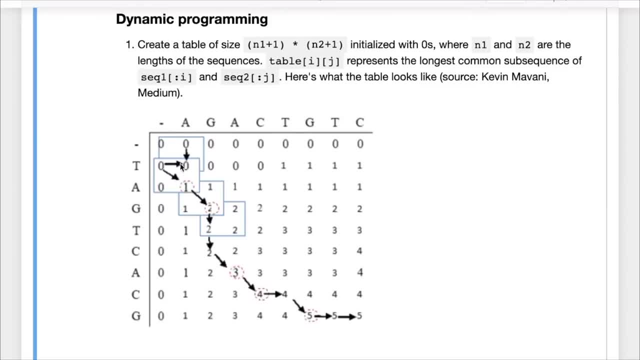 So here, if let's say I was one and a J was one, So this represents the longest subsequence of sequence one up to I, so all the positions before one, which means only the zero position, just T, and sequence two up to J, which means all the positions up to the first position of up to up to one, which means only the zero position, so which means a. okay, so table one and table IJ represents the longest common subsequence of these two, of just A and T, which is zero. 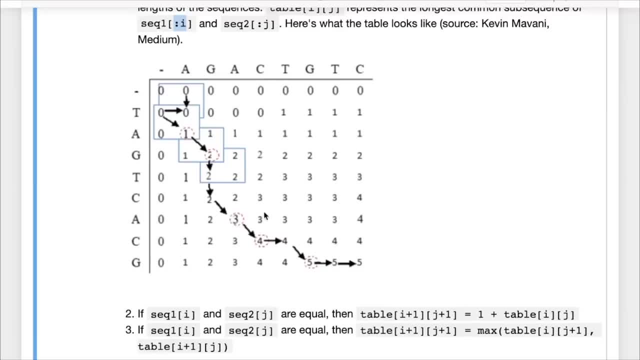 On the other hand, if we skip ahead a little bit, if we skip ahead to, let's say, this position, you can count, here I goes, zero, one, two, three, four, five, six. So this is six here. 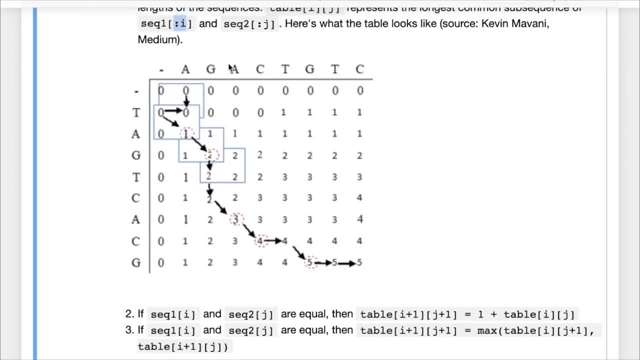 And here we have zero one. zero one, two, three. So this is so. this is table of six comma three. the table of six comma three takes the first six elements, which is T, A, G, T, C, A, and the first three elements, a, G, of sequence two, and it stores the result of the longest common subsequence between these two. 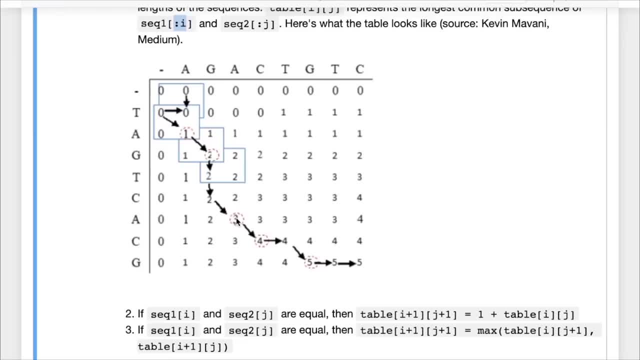 Okay. So I'll just let you look at the table and maybe even draw the table on a piece of paper and verify that the length three is right. You can see here a G a. a G a occurs here. So a G a is a subsequence of T, a, G, T, C, a. 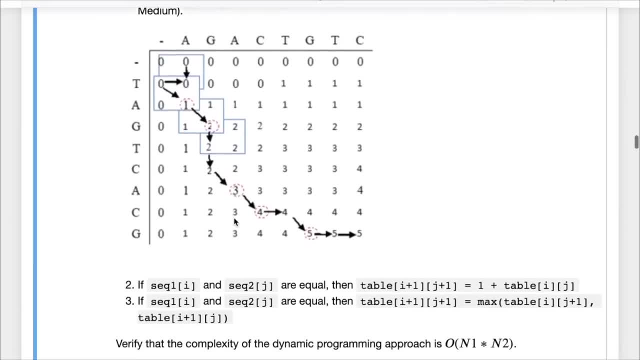 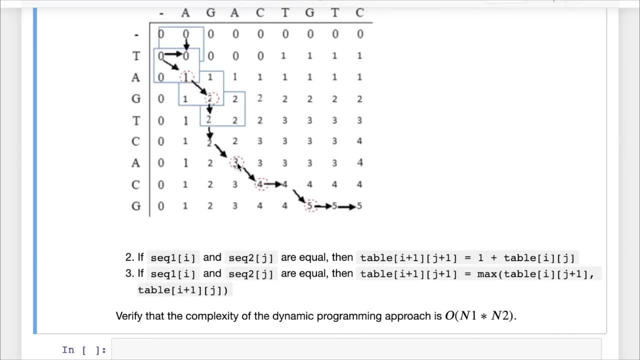 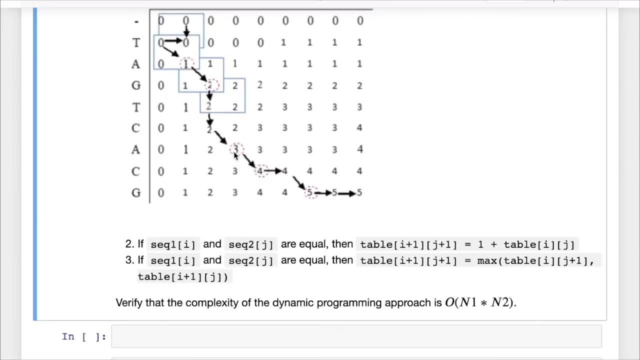 So the longest common subsequence between them is three. Now what we'll do is we will now compare the next elements of. we'll now compare sequence one of I in sequence two of G. So let's say we are looking at, let's pick an example. 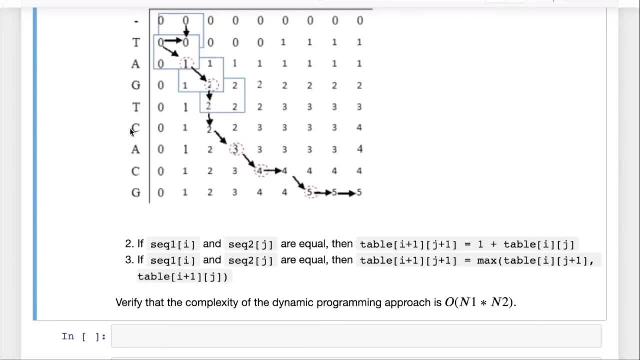 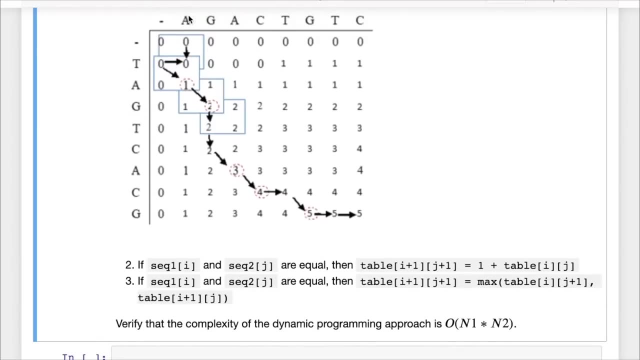 Let's say sequence. let's say I has the value. I has the value zero, one, two, three, four. I has a value zero, one, two. I has the value two. And let's say G has the value One, one. so zero one. 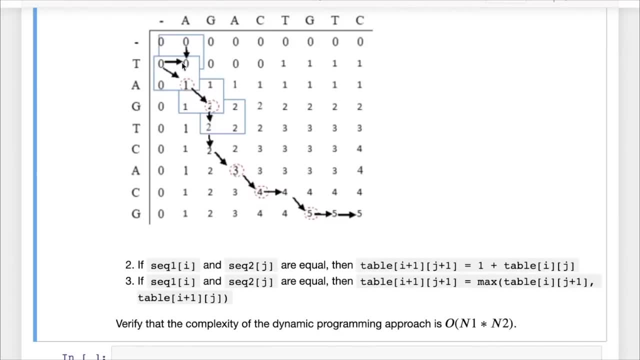 So if we compare sequence one of I, so, which is G, and sequence two of a sequence two of G, which is also G, And if they're equal, so if they're equal, then able of I plus one on J plus one, which is this value right. 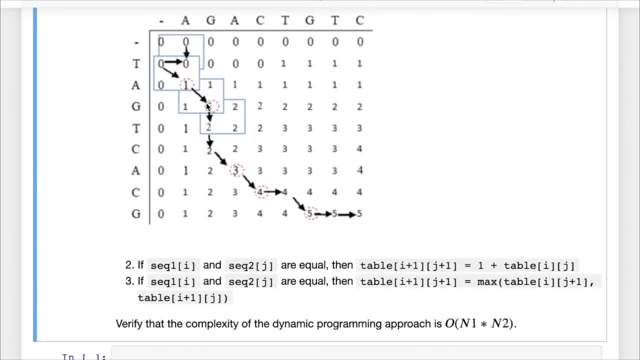 So remember, I is two and J is one, So table one of I plus one, So table one of three is zero. one, two, three And table and table one of I plus one, J plus one is able One of three and table a table of I plus one and J plus one, I being two and J being one, is stable. 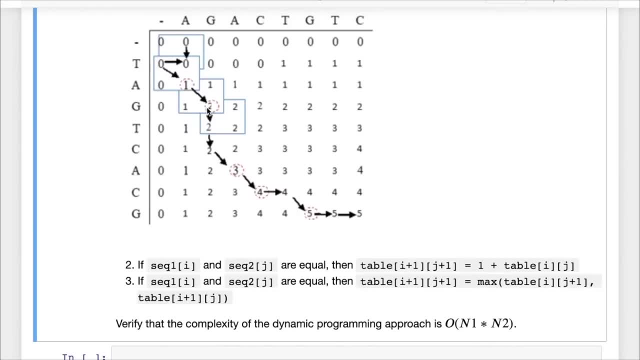 One of three and two, and table one of three and two is the value two. So this value is obtained by adding one To table one of I comma G. So because these two elements are equal, when we can then say that if we take the longest common, 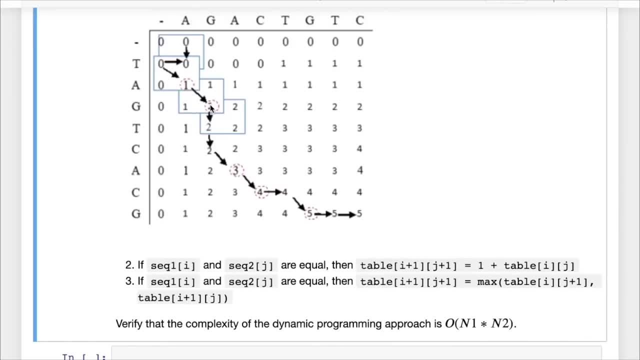 subsequence of T and E and add one to it, that will give us the longest common subsequence of The AG and AG. So the exact same logic as recursion. we have simply now reversed it. So we now- now we're looking at the last element, so that we can keep filling out the last value using some previous value. 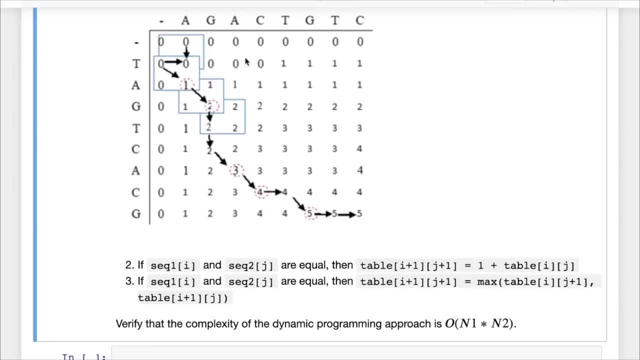 So okay. so this is one case. Similarly, here's one other case where a and a are equal. So the longest common subsequence between TA- GTCA and the longest common subsequence between EGA is one, plus the longest common subsequence between TA, GTC and EG. 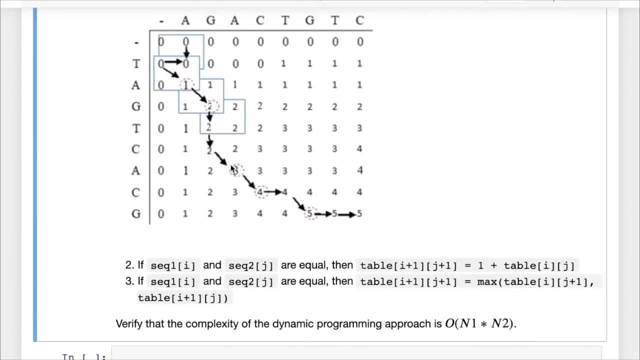 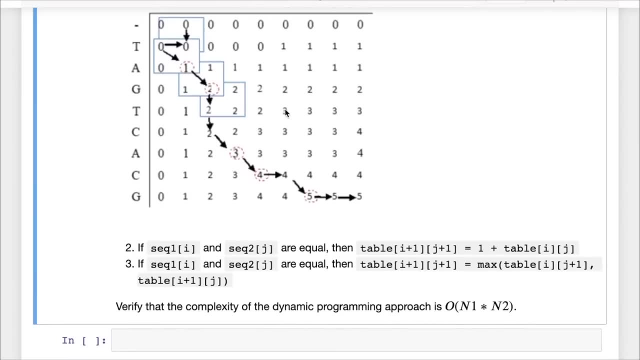 Okay, One plus this value. So that's one case. The other case is if they're not equal. So let's look at this value, for example over here. So we have TA GT on the side And then we have: okay, let's, let's look at this one. 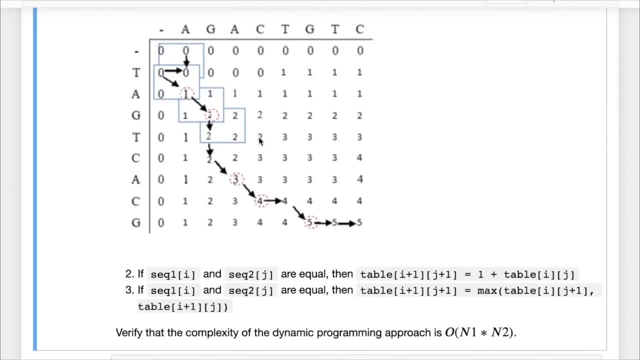 Uh, if we have TA GT on the side and we have AGAC on this side, now T is the element here and C is the element here. They are not equal. So that means the longest common subsequence between these two either does not contain T or it does not contain C. 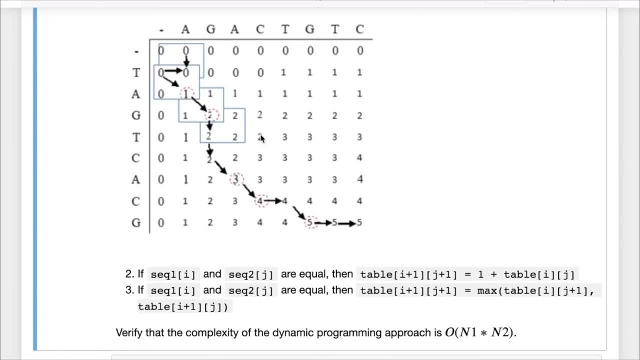 It cannot contain both, obviously, because one of the strings has to end. So if it does, If it does not contain T, then it is this result, And if it does not contain T, or if it does not contain C, then it is this result. 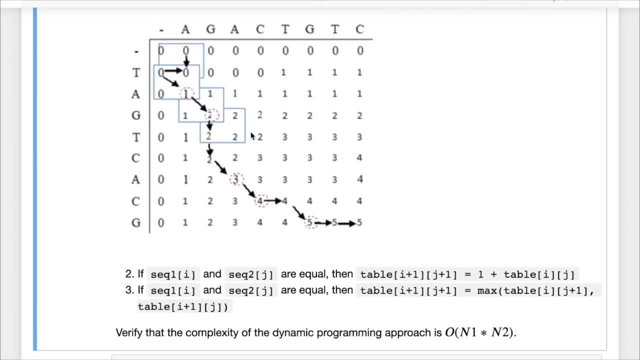 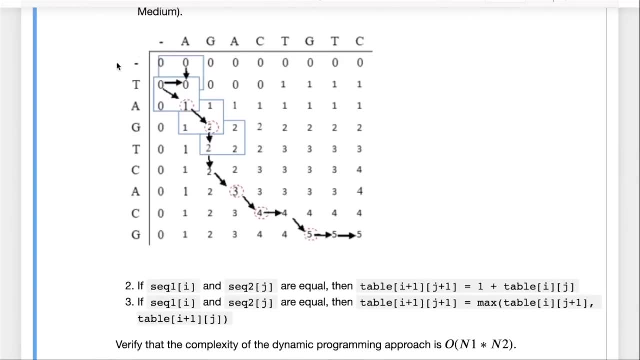 So we simply take the maximum of these two, maximum of these two to get the result for this. If these two elements are not equal- and that is how you fill out the table- you start from the top. The first row is zeros, because we are. we have empty strings. 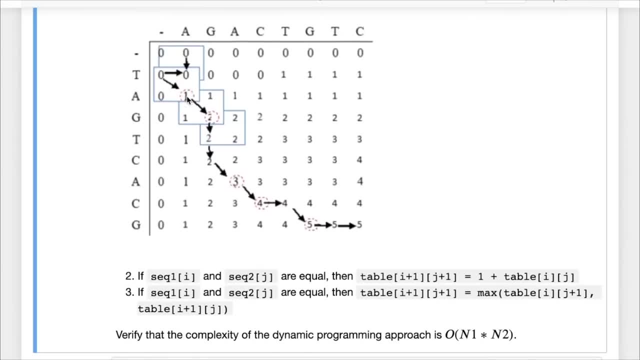 And the first column is also zeros, because we have empty strings to fill out an element. You compare if the two elements are equal and if they're equal, we simply add one to the left top left element. If they're unequal, then we take the maximum of the element above it and the element to the left of it. 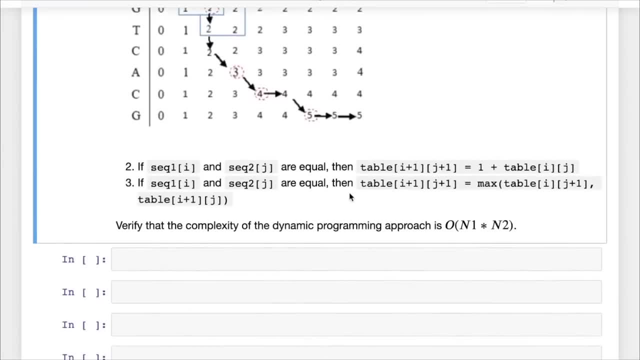 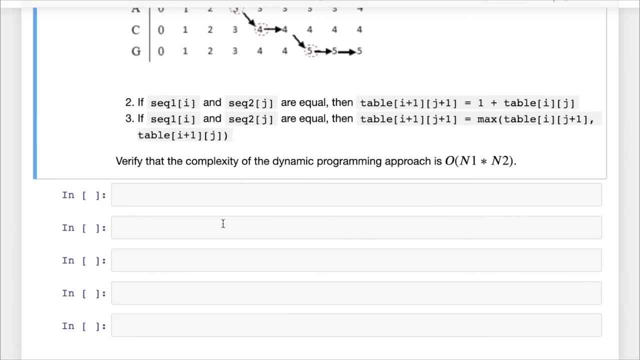 And that way we fill out the entire table. Okay, So that's the dynamic programming solution, And I know this can seem a little bit complicated. Honestly, I still get confused with dynamic programming a lot of times, And that's why I like to just draw tables and write things out carefully. 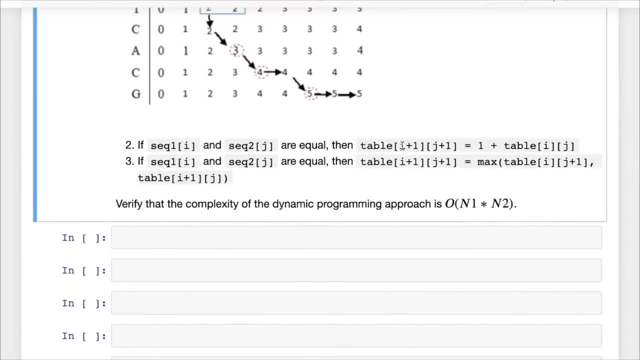 Okay, And and especially, You have to be especially careful with indices, because here we are saying that if sequence I one I and sequence to Jr equal, then table one of I plus one and J plus one is one plus table IG. 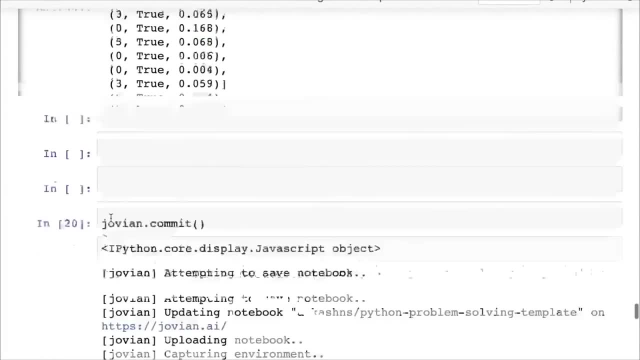 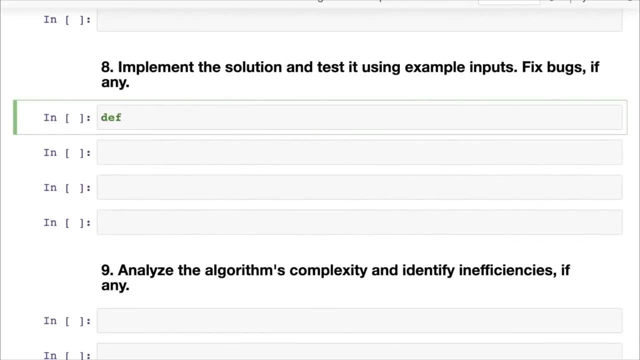 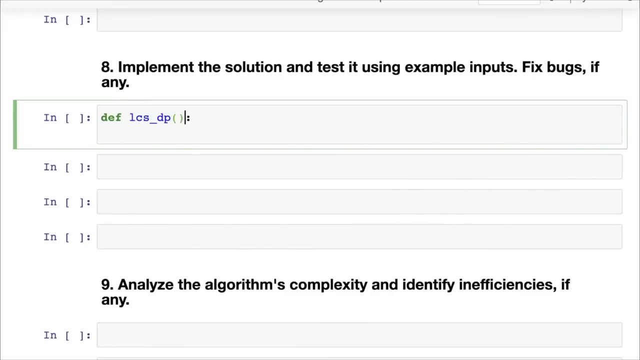 So be? just watch the indices carefully here. but let's implement the solution, Let's implement the dynamic programming solution. So let's say LCS, dynamic programming. So we'll just say DP here, and we have sequence one And we have sequence Two. 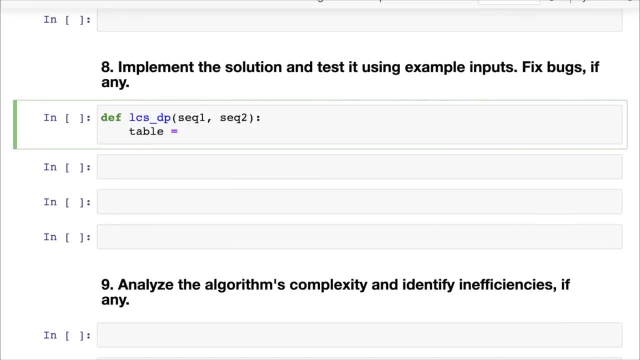 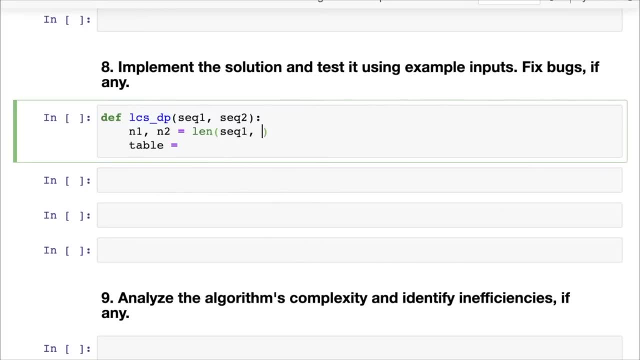 And the first thing we need is we need a table of results. Now, this table for it. let's just grab N one and N two, So length of sequence one and length of sequence two, And now we need to create a table with all zeros. 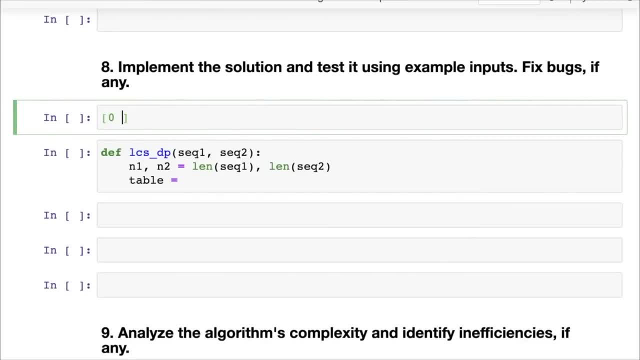 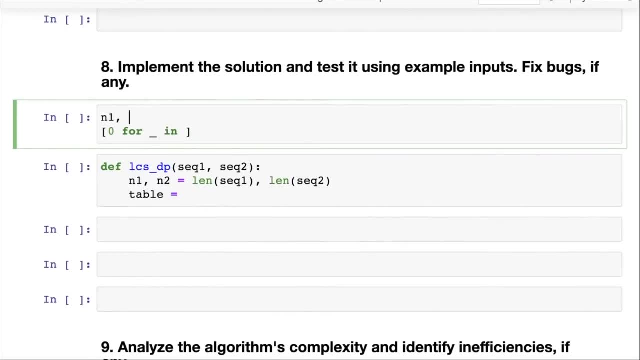 How do you create a table with all zeros? The way to do it, a way to create a list of zeros, is this: zero, four, underscore in, let's say, and let's give anyone an end to some values. Now, if you want to create a list of zeros of length and one use you simply say zero for underscore or zero for X. 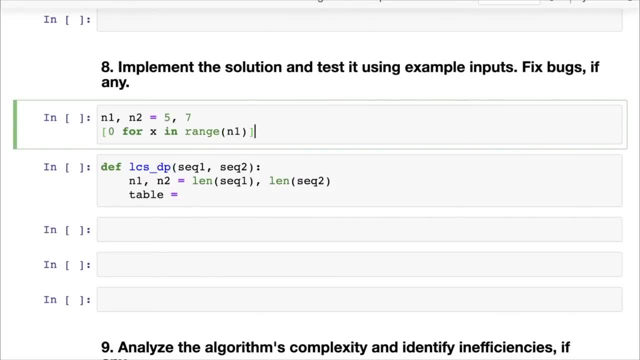 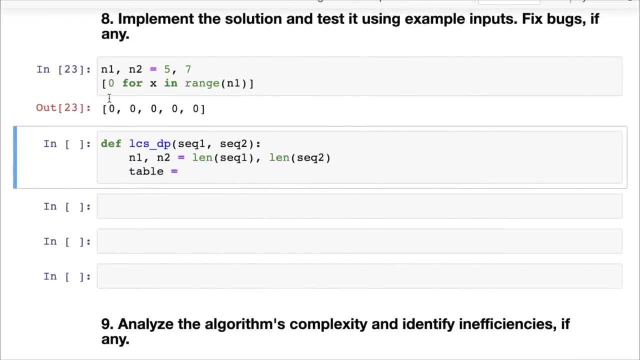 You're simply ignoring whatever value you're getting from a range. a range and one, and that's going to give you a list of zeros. but we don't want a list of N one zeros. We want these more. These want to be rules. 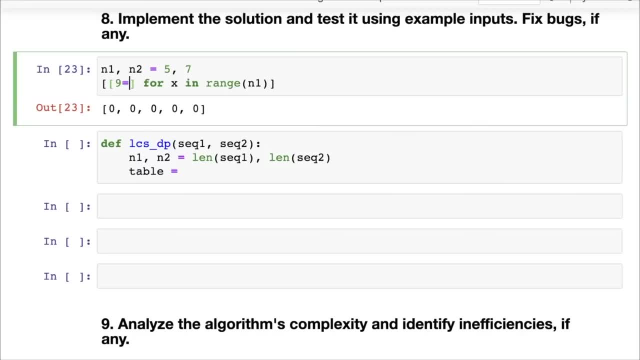 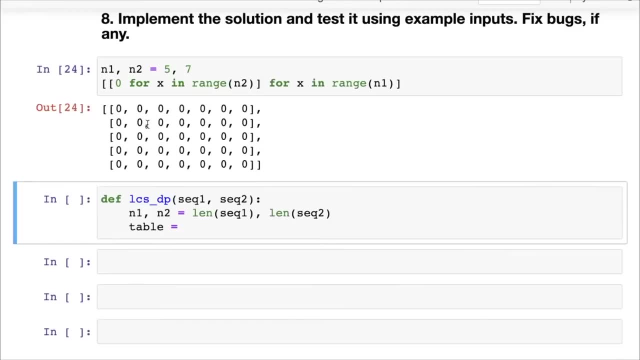 So we want each of these to itself be a list Of zeros of length and two, so zero. four, X in range and two, And now we have. you can see that we have five rows: one, two, three, four, five. 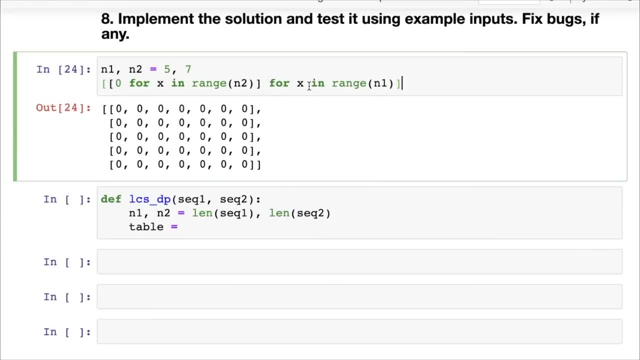 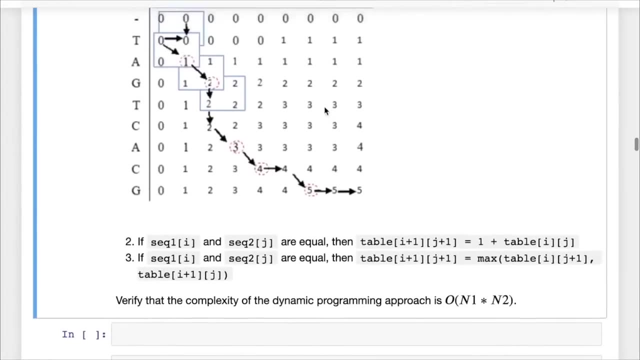 Then we have seven columns: one, two, three, four, five, six, seven. So this is the table that we want to create initially. Okay, Now there's a table that we've created. This is going to be this exact same table. 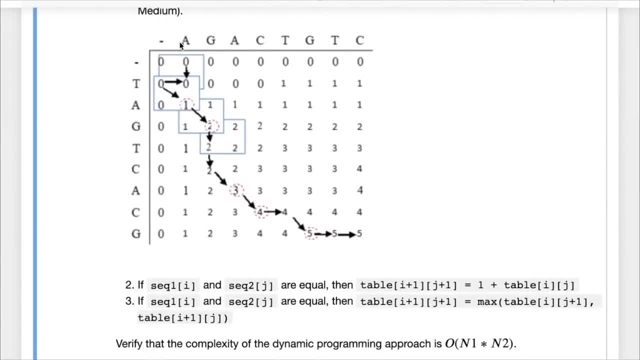 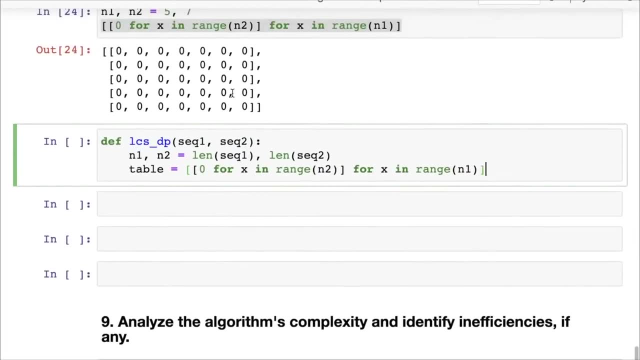 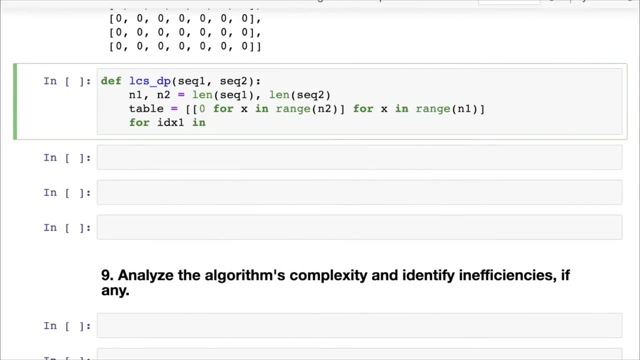 And we're simply going to start each string from position one, this time, not from position zero, Because we want to have this additional row where we don't consider either of these. that just makes computations a little easier. Now we say for IDX, one in Len addicts, one in range and one. so that's, that's going to iterate over the rules. 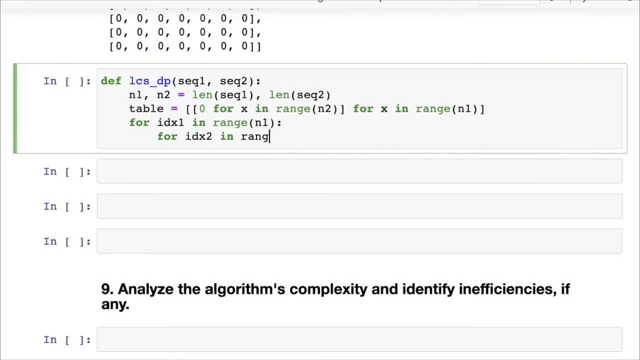 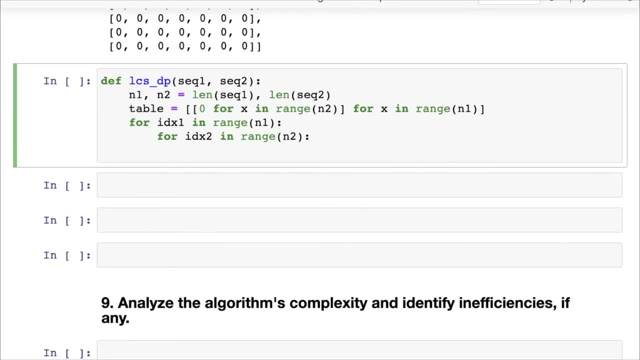 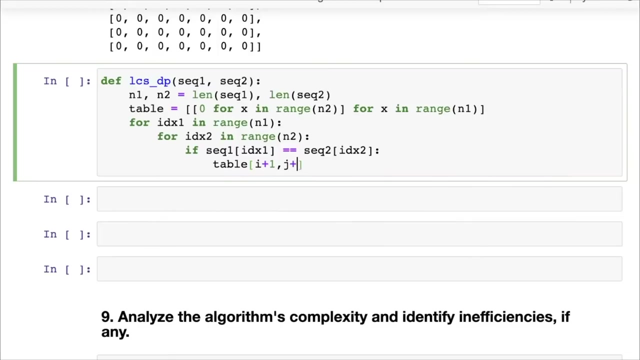 And then for IDX true in range and two, and that's going to iterate over the columns, And first we compare If sequence one of IDX one is equal to sequence two of IDX two. if they're equal, then we can fill out table of I plus one and J plus one as one plus table of IJ. 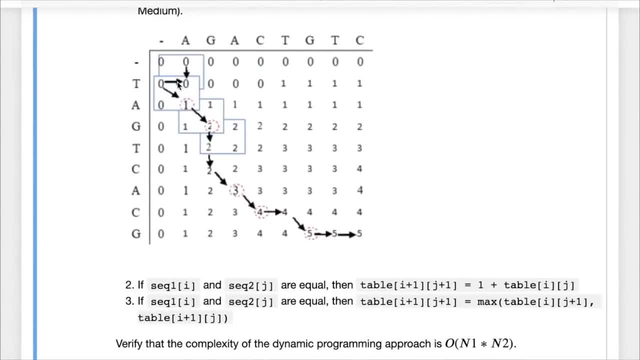 Okay, And we can see This, we can see this here. Suppose the first elements were equal, So suppose this was. suppose IDX one was zero and IDX two was also zero. Suppose they were equal, Then this value should be one. So this value should be one plus the diagonally top element. 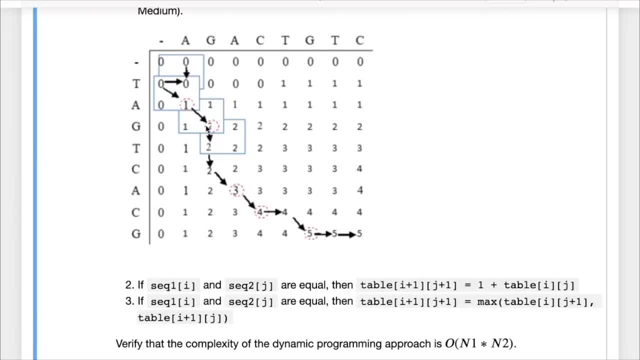 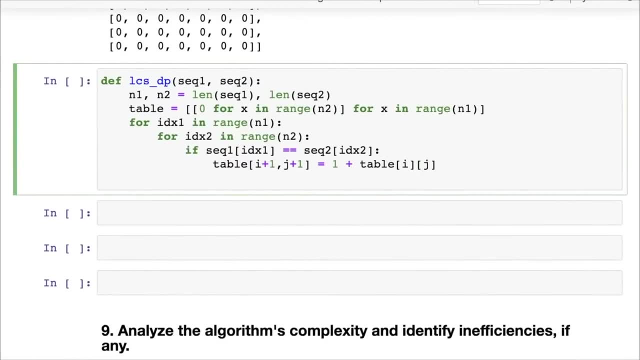 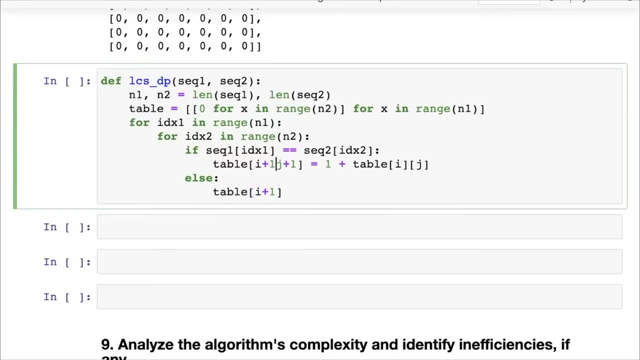 And that holds true anywhere within the list. So wherever you have two elements equal like G and G are equal here. So this value is one plus this value. Else we have table I plus one and J plus one is max of able I comma, J plus one. 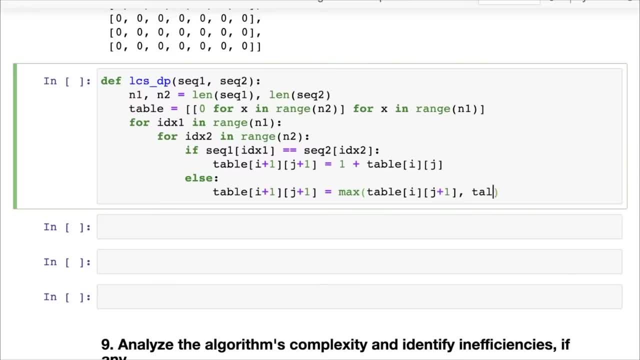 So you stay in the same row, or you go to the previous row, or you go to the previous column, which is stable of I plus one, So you stay in the same row. So you stay in the same row, or you go to the previous row, or you go to the previous column, which is stable of. 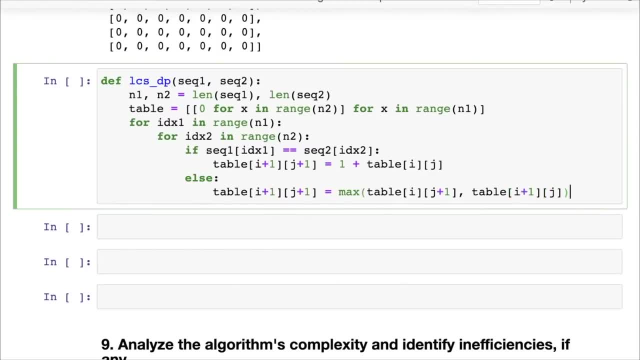 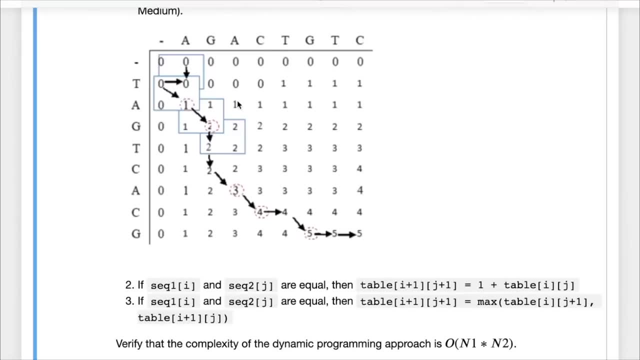 I plus one comma J, And this is the previous column. Okay, So this is this case where G and a are not equal. So if G and a are not equal, then we take the maximum of these two values and that's it. 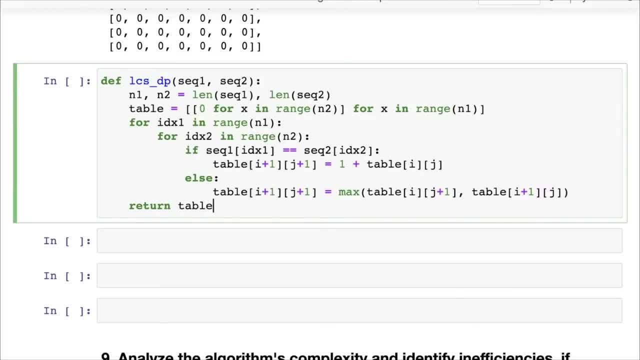 That is going to fill up the table for us, And then we simply say: return able. We simply want the bottom right element, So we can simply say: return table minus one, minus one. So this is going to get that last row, last column, and that's our dynamic programming solution. 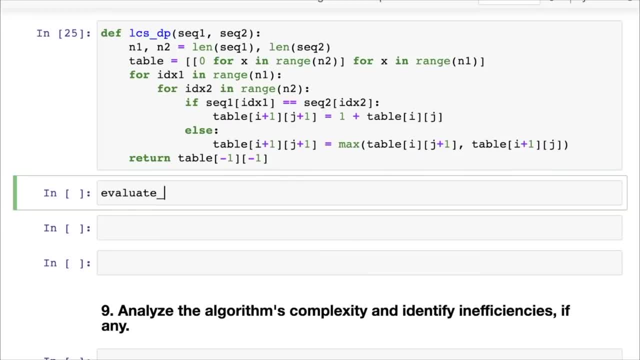 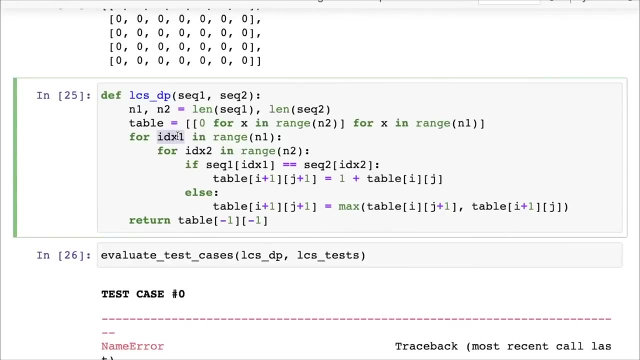 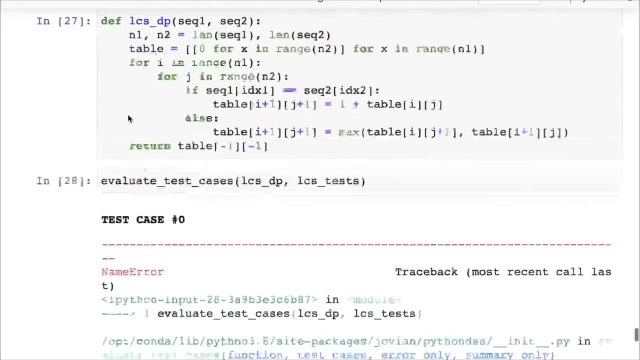 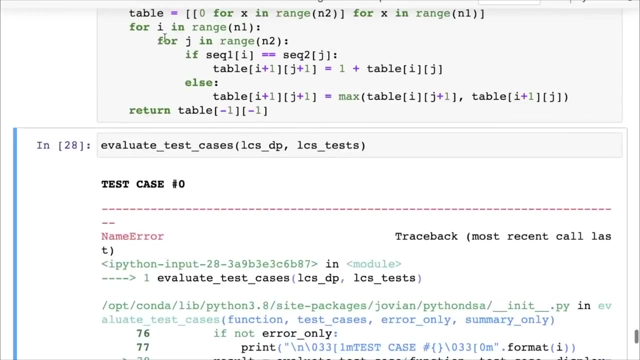 Let's do evaluate test cases here. Okay, It turns on. There's no I. okay, Let's just call this I and J Turns out IDX. one is not defined, Let's just make these INJ. Now that we're doing this coding live, you can see that even after a decade of coding, I still make all of these issues. 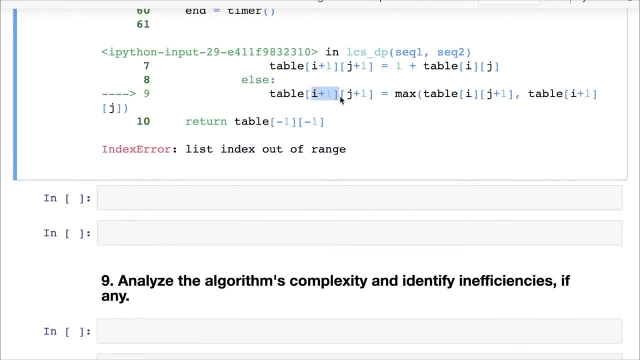 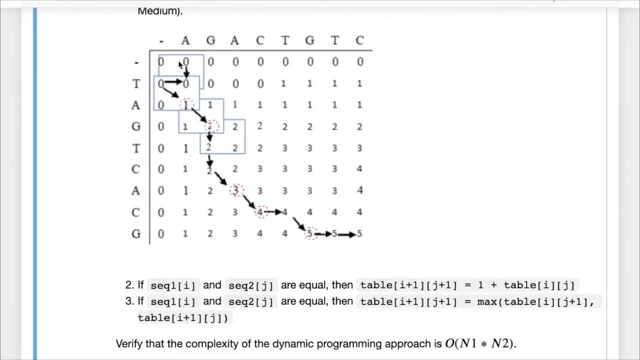 It says the list index is out of range. It seems like I plus one and J plus one. Ah, that's because, remember, we need an additional row and an additional column to track the case where either of the strings is empty. So we need to get range and two plus one here. 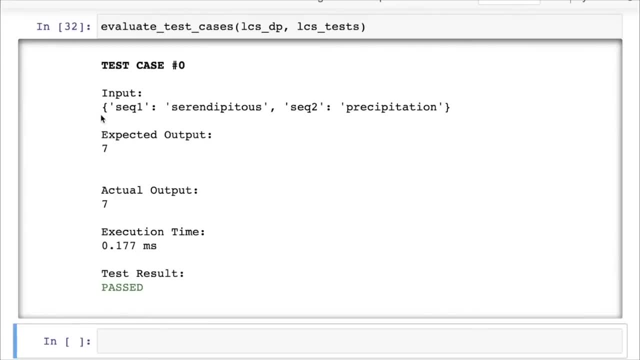 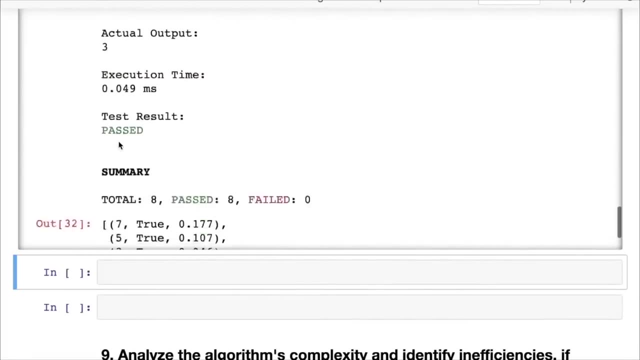 And we need to get range And And one plus one here. Okay, And that's why it helps to have test cases, so that you can fix all of these issues. Now you have test case zero- it passes, and test case one, two, three- all of them pass. 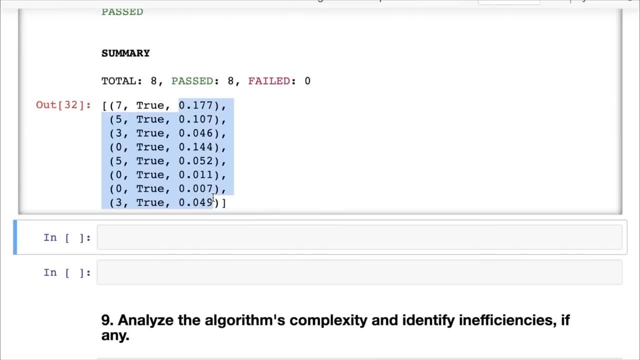 You can see that all test cases have passed, and you can also verify that the amount of time it took is now lower than the amount of time it took for memorization. Okay, And so that's the dynamic programming approach. You simply create a table and you fill out the table. 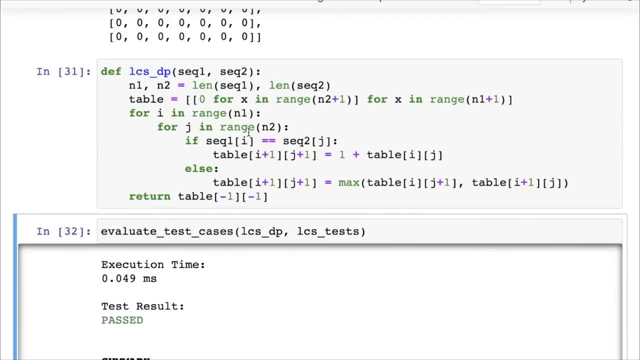 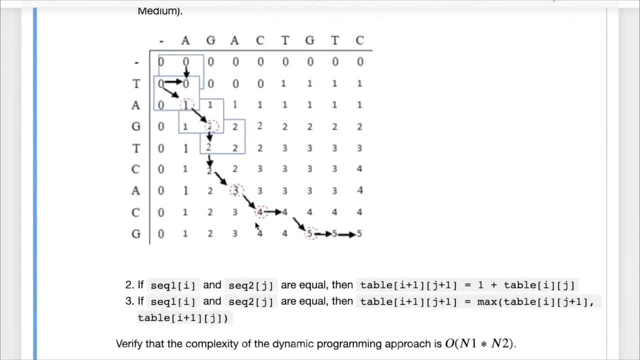 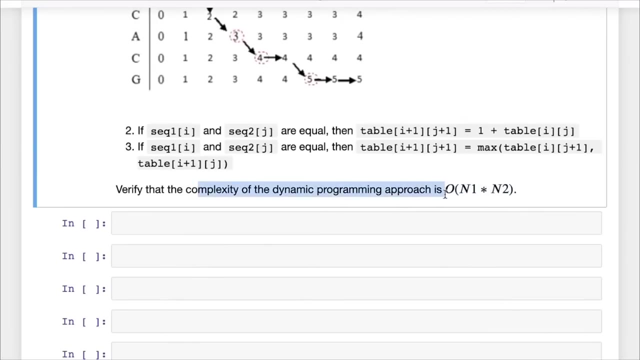 Sometimes just working with Indices within the table can get confusing, So it helps to work with it on paper and make it clear to yourself and then write it in English. That's why we've written it in plain English here And now. an exercise for you is to verify that the complexity of this dynamic programming approach is. order of N one times N two. 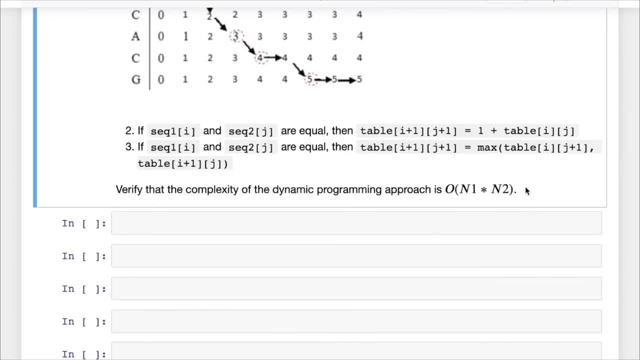 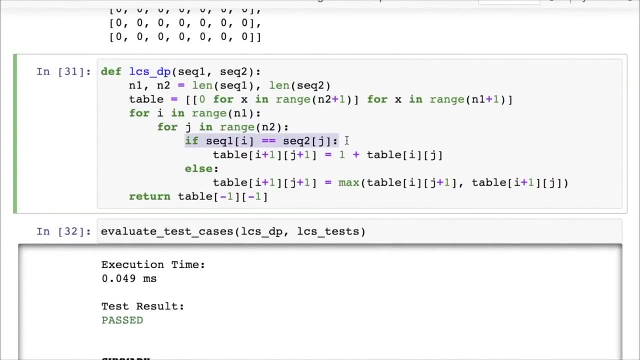 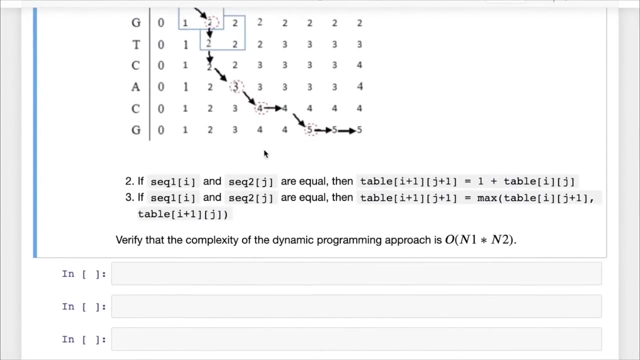 So, which is the same as memoization, And it's actually more straightforward to see here, because you have two for loops and then each of these for loops. You are simply doing a comparison and an addition and there's not even any recursion to where, where, if there's not even any recursion for you to vary or worry about. so you just do a comparison and you do an additional, you take a maximum, pretty straightforward, the order of N one times N two, and it does not even invoke an another function. 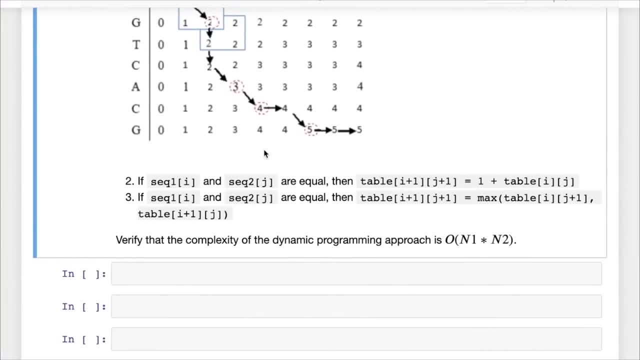 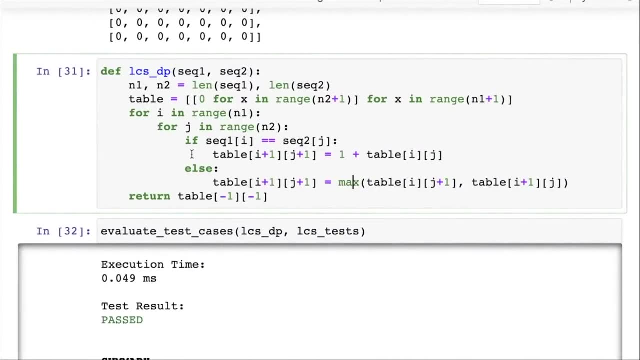 So it does not take up too much memory, It does not take up too much time, It's very, very efficient. And this is how you solve pretty much every dynamic, pro dynamic programming problem. You write a recursive solution, you come up with a brute force solution, and keep in mind that recursion is almost always the way to go about creating a brute force solution. 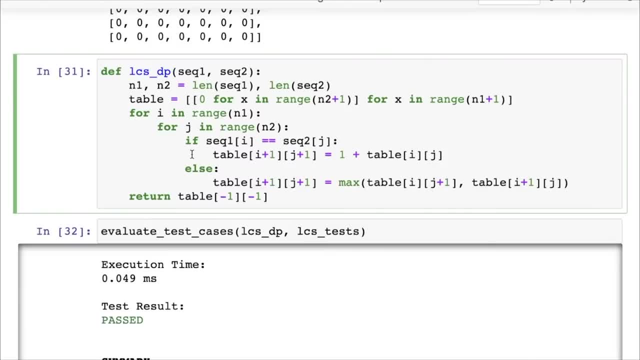 So you come up with a recursive solution and then you identify, you draw the recursion tree And if you see that the same sub problem is being called again and again, that is a point where you can introduce memoization, So you introduce memoization. 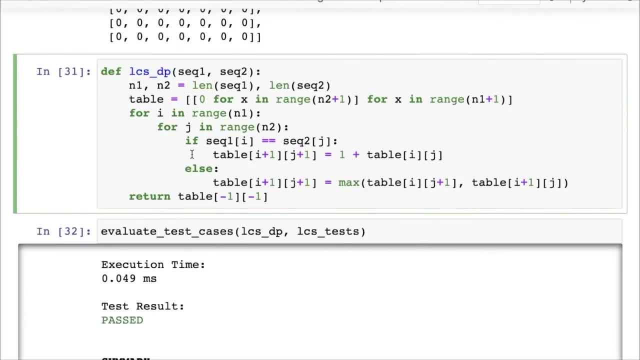 And sometimes you can just write the memoized solution and that's enough, because it's easy to reason about. You just put in a memo and you're done with it. Um, even the interviewer or the coding assessment will accept that solution. Uh, but in some cases you will be asked to then remove the recursion and write it as a in an iterative fashion. 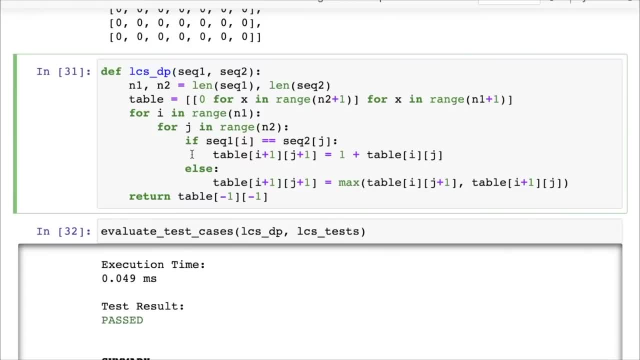 And that is when, then, you have to start drawing a table and think about what are the rows and columns in that table need to represent. So here the I J element of the table represented The first. the first I elements of sequence one and the first I J elements of sequence two. what is the longest? 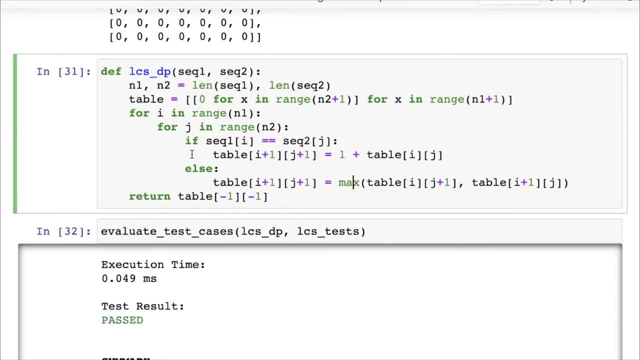 sub sequence between them And we use that to build the next row and the next next column, And we then filled out the entire table and we simply use the last value. Now again, this is not very straightforward. uh, how to come up with this and the way you do that is by solving problems. 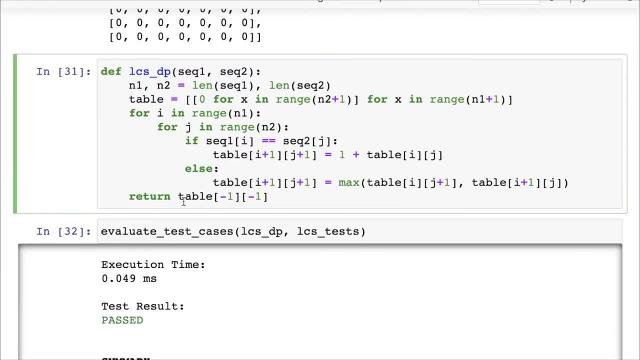 If you solve five to 10 dynamic programming problems, you will get some intuition about how to build the table, And it's always very helpful to solve it on pen and paper first, especially with dynamic programming, so that it's clear to you What each element of the table represents. 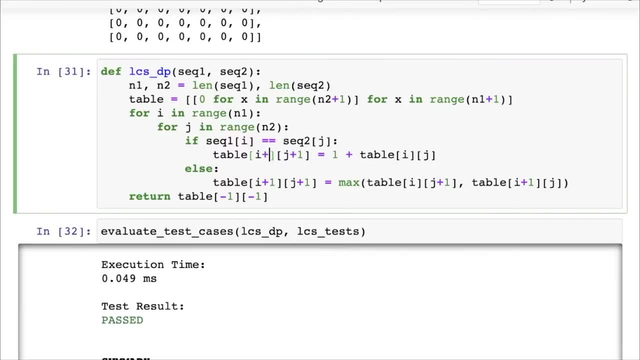 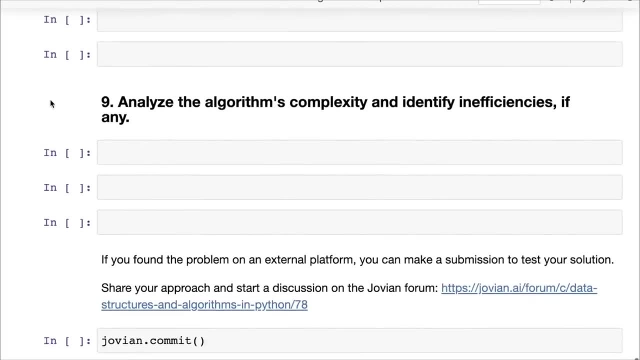 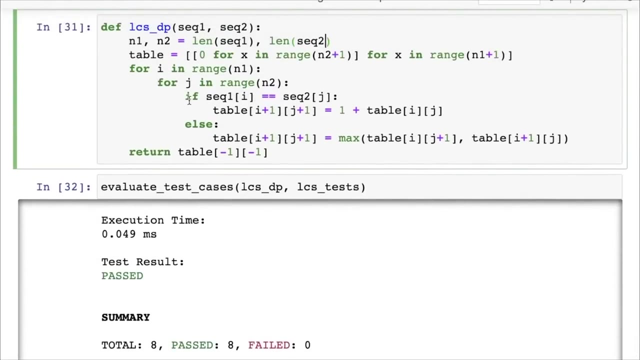 Otherwise, you may make a lot of off by one, errors like missing the plus one here or missing the plus one here, and get confused, just like I did pretty much. And that's the time, The time. complexity is pretty straightforward: in most cases it is simply the size of the table, but sometimes you may have to do more than. 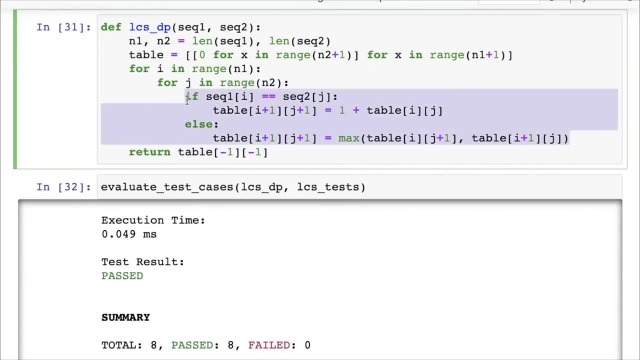 constant work here. So keep that in mind. see what it is that you're doing inside your loop, Now, inside of inside your loop. if you have to go back and check the entire length of the string, so that will introduce another factor into the equation. 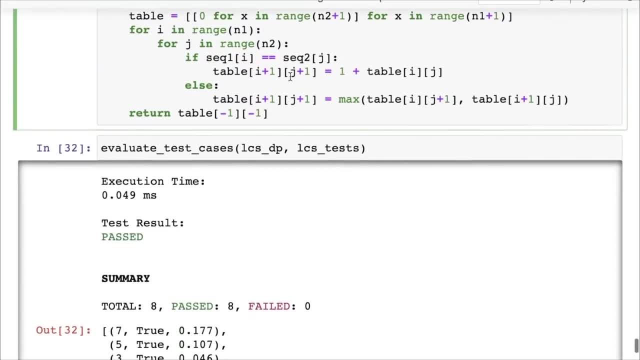 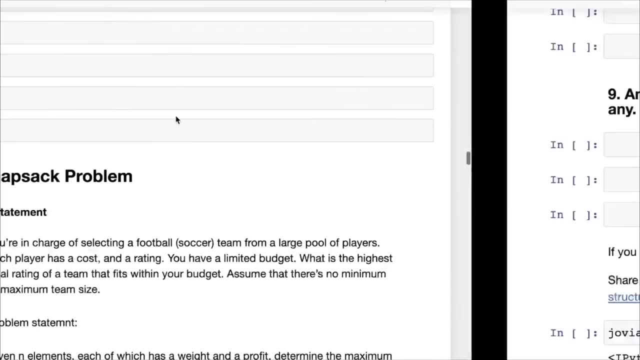 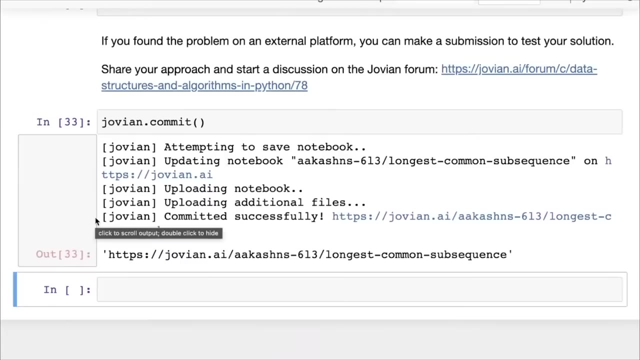 So keep that in mind. But in most cases, counting the iteration should be good enough to give you an idea of the time complexity. Okay, So that's the first problem, and let us just commit this- And now it's saved- To my profile. 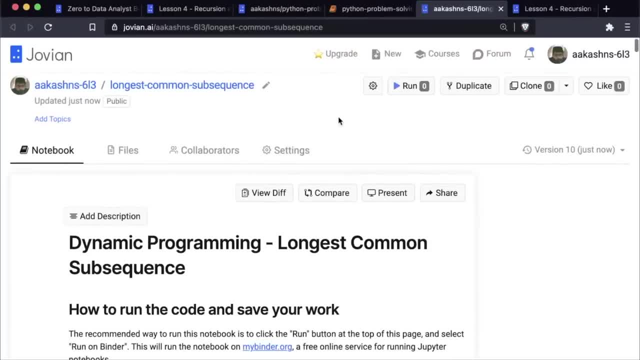 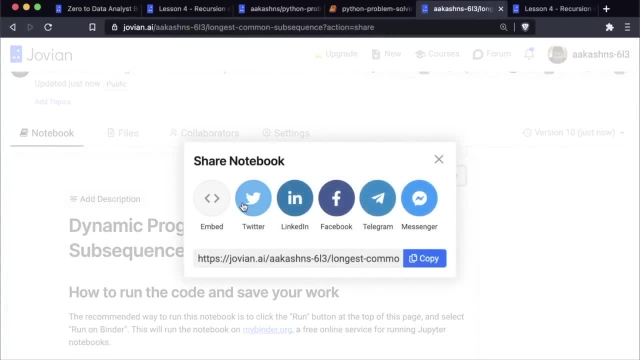 If I just open this up here, you can see that now I have this notebook, or longest common sub sequences, and I can share it online. Whenever you work on a notebook, it's always a good idea to make it public. put it up on Jovian. 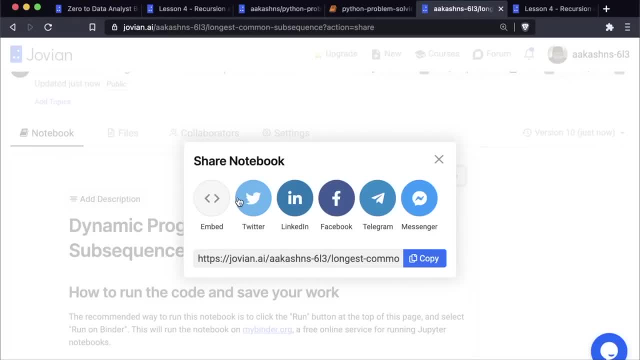 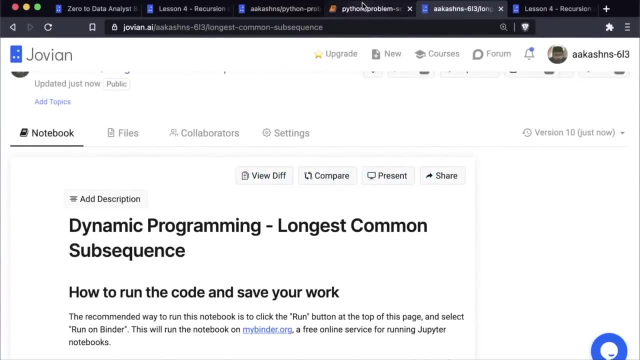 All you need to do is run Joviancom it and share it online. Just press the share button and then you can share it on Twitter, LinkedIn, Facebook or wherever you like. So that's the first one that we looked at. 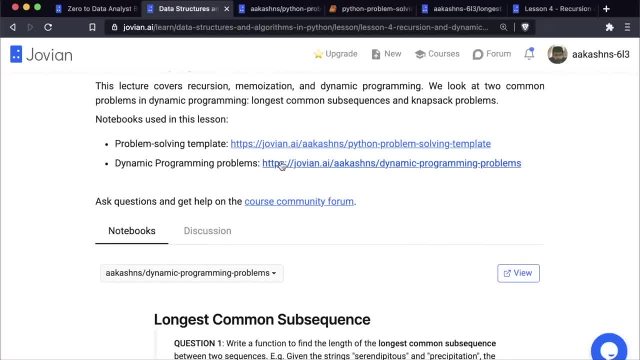 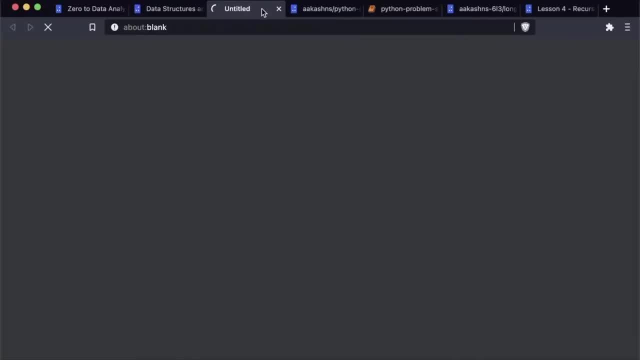 Now let's come back to listen for- And- uh, by the way- the problems that we're talking about, all the problem statements, the graphs, the images- you can see them in the second link here. but we will once again open up the problem solving template and now we'll use it for the second problem. 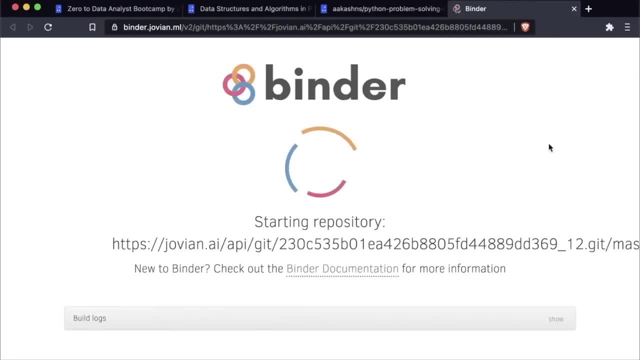 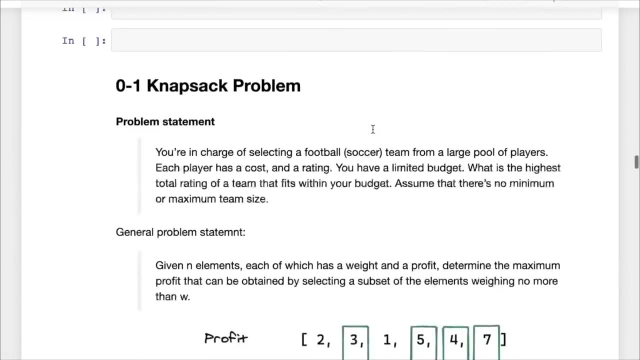 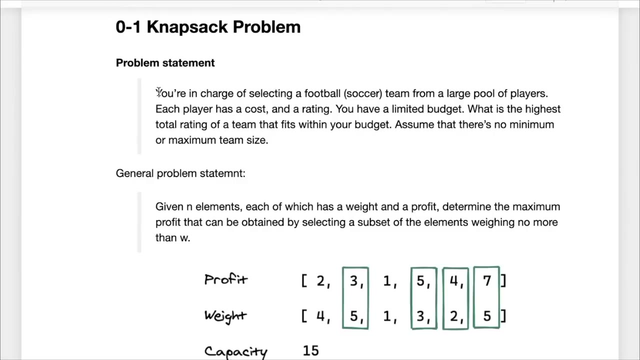 Let me run this once again. We're going to look at the second problem, which is the knapsack problem. So let's read: the knapsack problem. It's also called a zero one knapsack problem. Okay, There are many variations of this problem, but here's one way to state it that you might come across, or something similar. 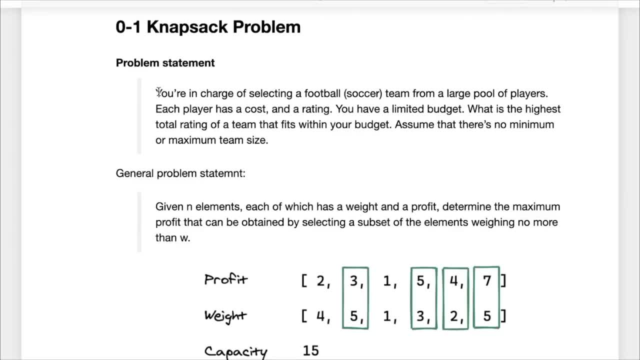 You are in charge of selecting a football or a soccer team from a large pool of players, and each player has a cost and a rating, So there's a selection going on. You have to come up with a team for this year and you have a large pool of players. 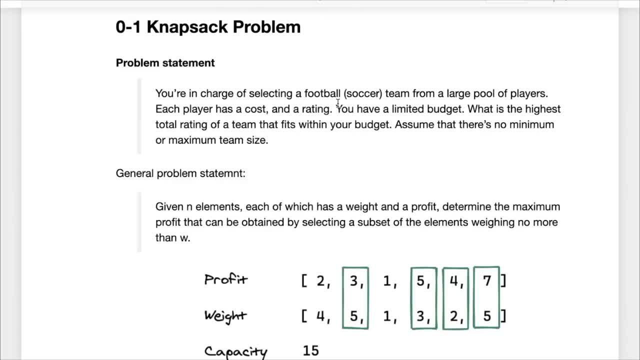 Each player has a cost and each player has a rating. Now you have a limited budget, So you need to build a team Within the budget. So what is the highest total rating of a team that you can create which fits within your budget? 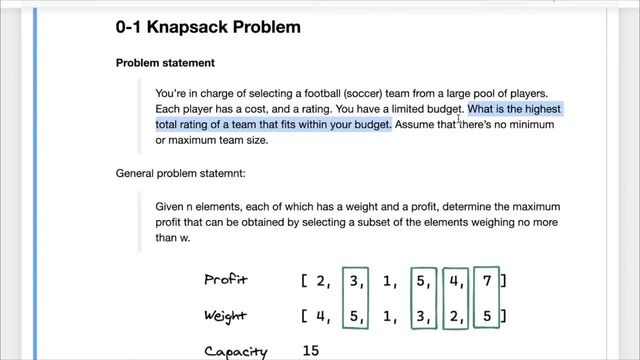 Okay. So this is the question here: You have to maximize the total rating, but fit it? fit the total cost within your budget. So we have two variables here: rating and variables. rating needs to be maximized. Cost needs to be simply optimized to the extent that it fits in the budget. 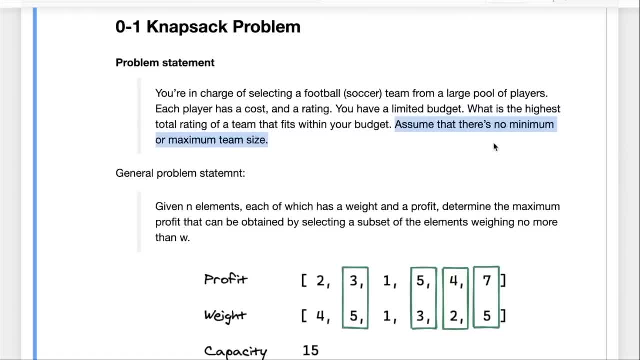 And just a simplifying assumption here is that you can assume that there is no minimum or maximum team size. This is simplification, And later you can introduce a criteria there as well, that you want to build a team of exactly 10 people and see if you can also solve that problem in a way. 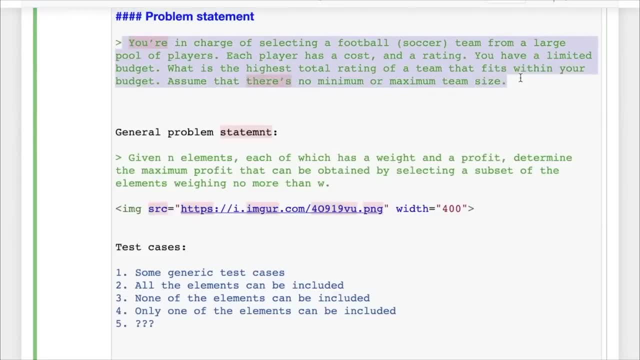 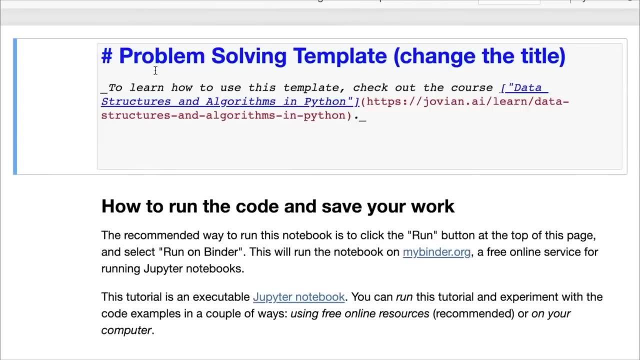 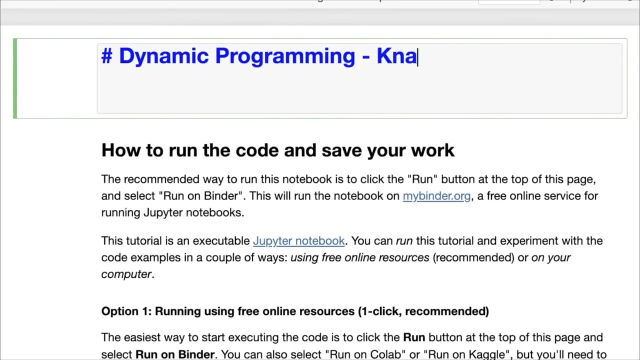 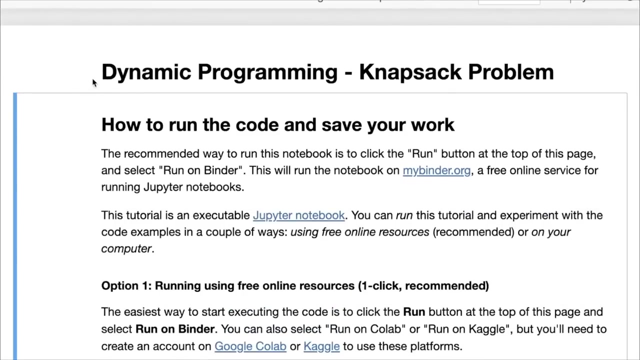 So that's the knapsack problem. Let's copy it over. And here's a Jupiter notebook, a fresh problem solving template. Let's simply change the title here. Okay, And this is also called the zero one knapsack problem, because each item can either be chosen or not chosen. 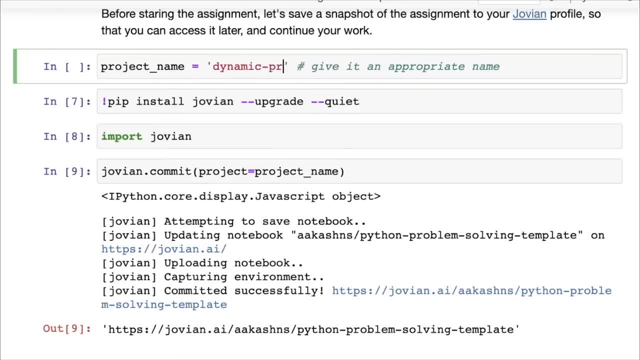 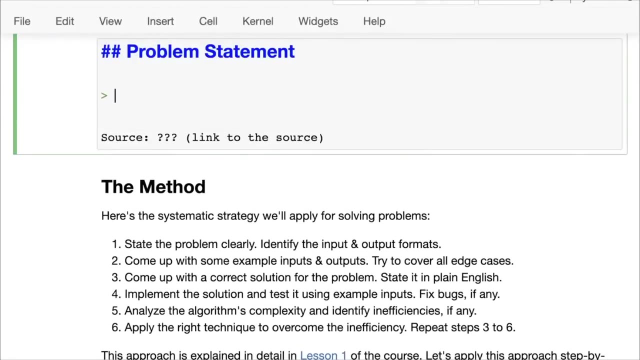 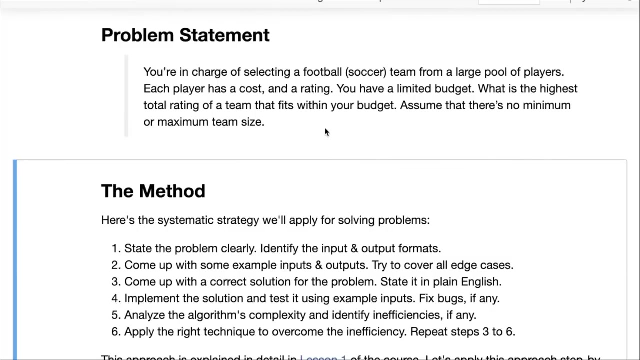 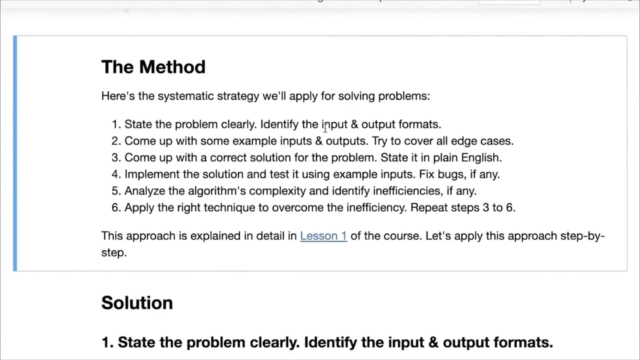 And let's give it a project name here too, Let's commit it and let's paste the problem statement here. So that's the problem statement, and this is a specific or a special form of a more general problem statement. And we look at the general problem statement in a second when we try to state the problem clearly. but here's once again the systematic strategy we'll apply. 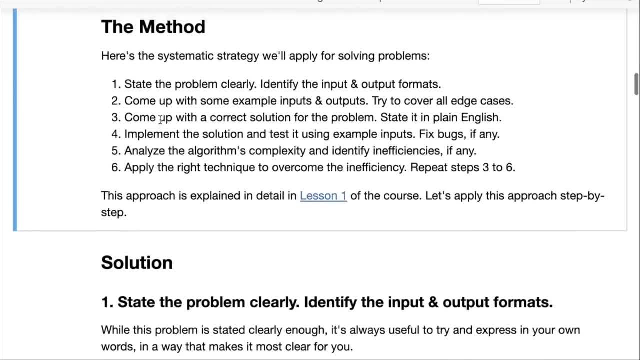 We will state the problem clearly, identify the input and output formats, come up with some example inputs and outputs and try to cover all the edge cases. Then we will come up with a correct solution for the problem and state the solution in plain English. 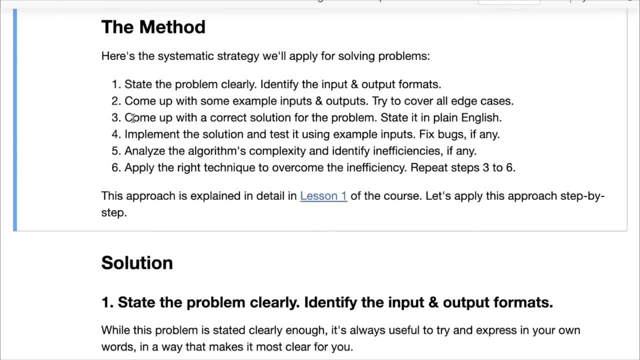 It just has to be simple, correct solution, not too complex. Then we apply the right technique to overcome the inefficiency And then we uh. so we analyze the algorithm and identify any inefficiencies after implementing the solution. And finally, we apply the right technique to overcome the inefficiency and then repeat the process of stating the solution, implementing it and analyzing it. 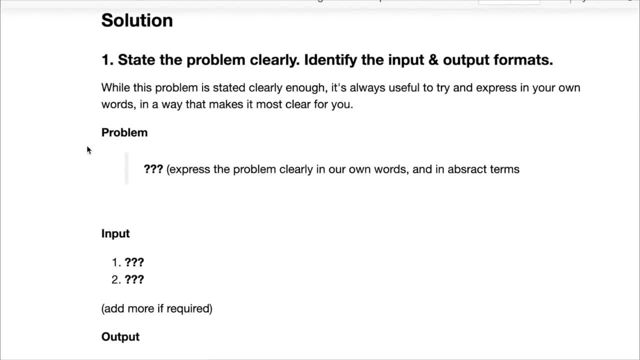 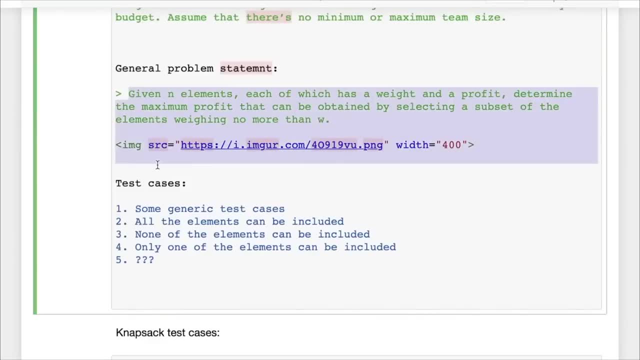 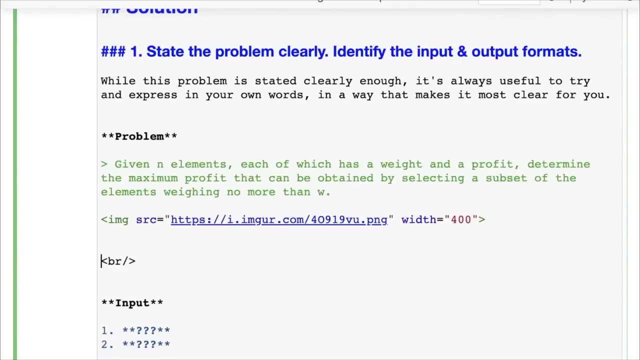 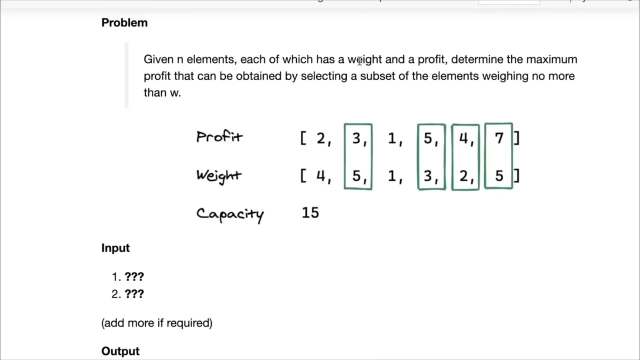 So, to state the problem clearly, What we can do is we can abstract on the problem in more general terms, And that is what is stated here, And let's just grab that and we'll take a look. So here we have. we are given N elements, and each of which has a weight and a profit. 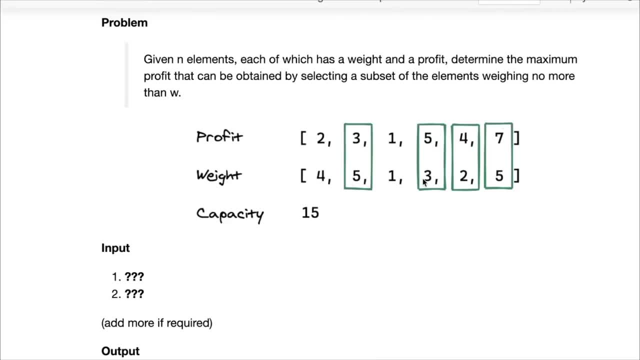 So you have N elements and here's the profit of each element And here's the weight you can uh of each element. So you need to determine the maximum profit that can be obtained by selecting a subset of the elements weighing no more than a given weight w. 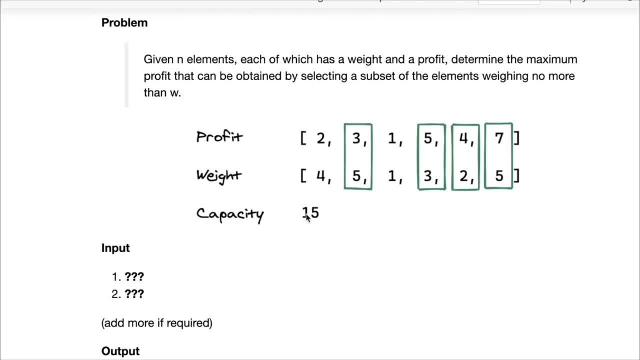 So you have a capacity, a maximum capacity- Let's say the maximum capacity is 15- and you have to select certain elements so that you fill out, the total weight is no more than the capacity and the total profit is maximized. That's, and this is why it's called the knapsack problem. 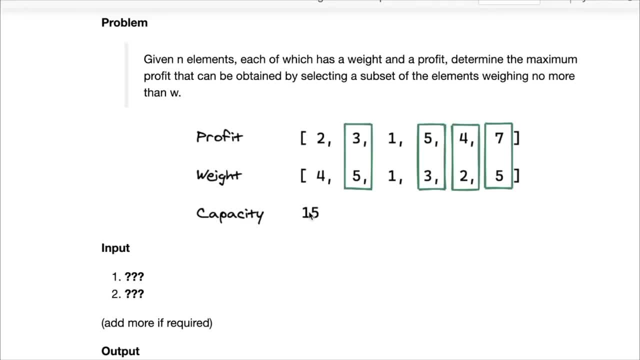 It's assuming, here you have a bag or a knapsack With a capacity of 15. Kilograms, And these are the weights of the items And these are the profits. Now, in this case, you can see, in this example, the optimal selection is these four elements which have the weights five, three, two and five. 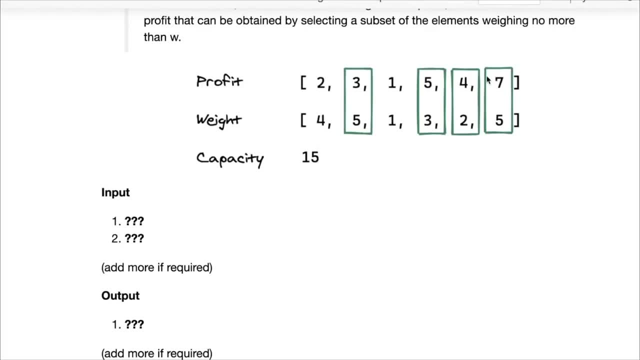 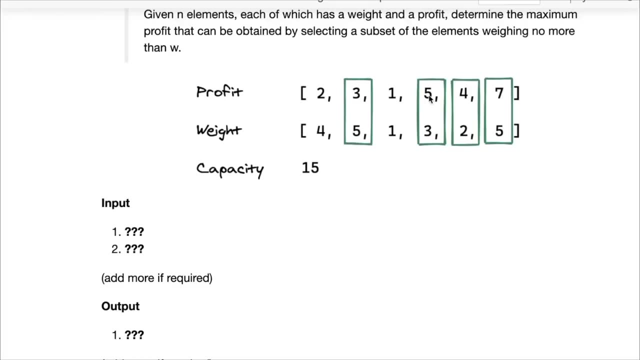 So that you fill out the total capacity of 16 or 15.. And the the solution on the maximum profit that you can obtain is seven plus four, 11 plus five, 16 plus three, 19.. Now you can try other combinations and verify that this is actually the best. 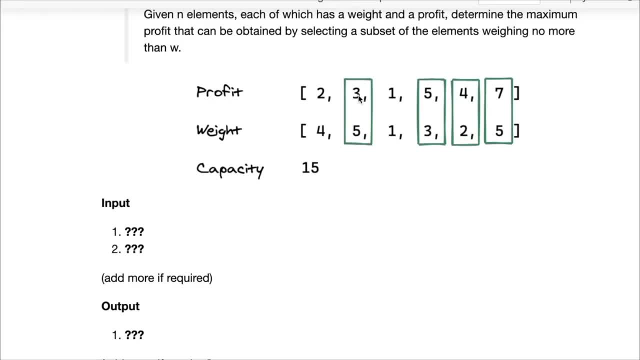 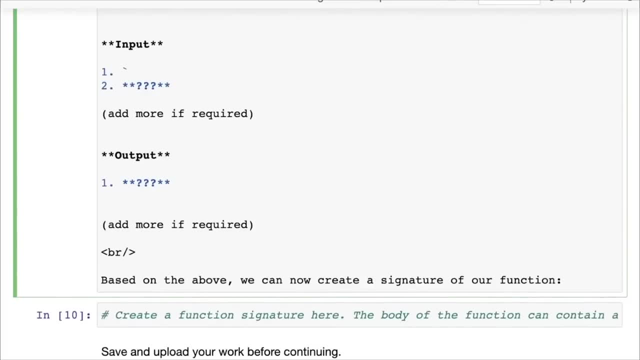 Solution. do give it a shot. So what are the inputs here? So we have- it's pretty clear, We have- an input: weights, but these are the weights of the. this is a list of numbers containing weights. and then you have profits: a list of numbers containing profits. 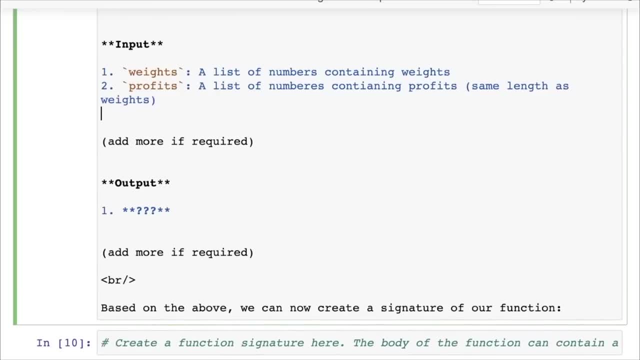 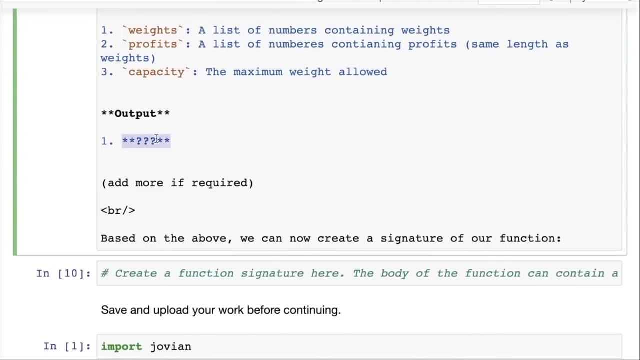 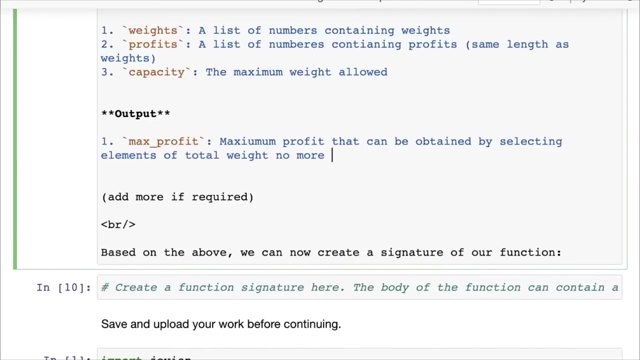 And this should have the same length as weights. And then, finally, you have a capacity, the maximum weight allowed, And there you go, And now we have outputs. So now the output would simply be the max profit. This is the Mac, So this is the maximum profit that can be obtained by selecting elements of total weight no more than w or no more than capacity create. 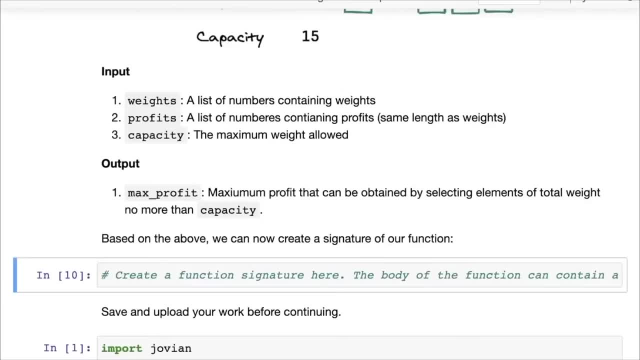 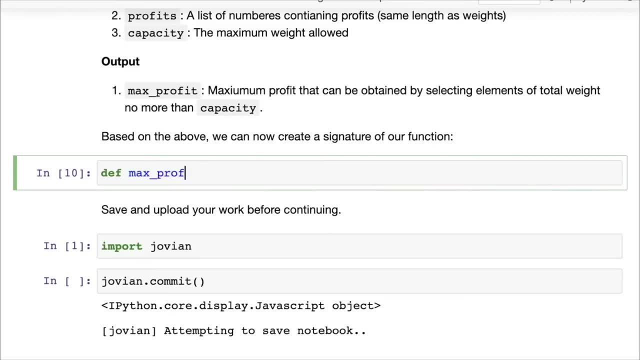 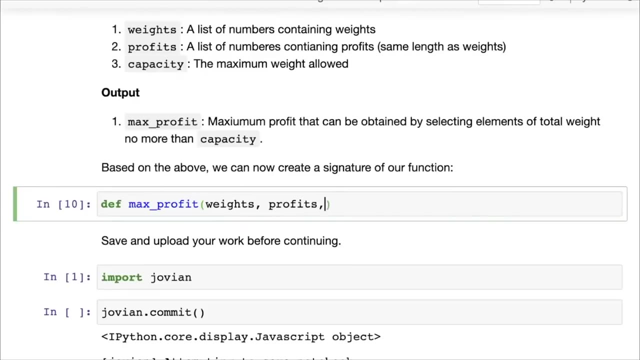 So that gives us a pretty good starting point. Now we can write a function signature. So we write max, let's say def, max profit, and we can give it weights, and we can give it profits, and we can give it a capacity and we pass. 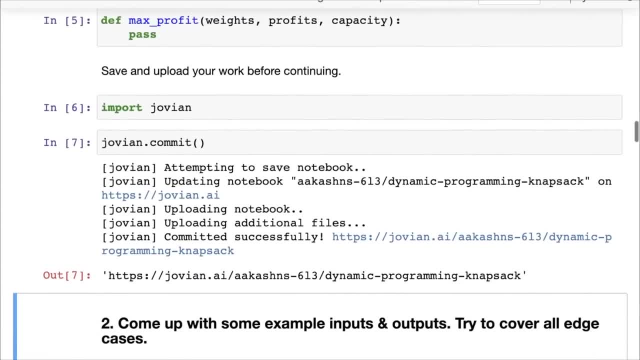 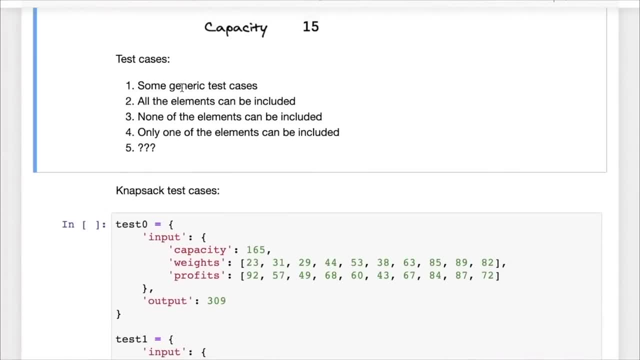 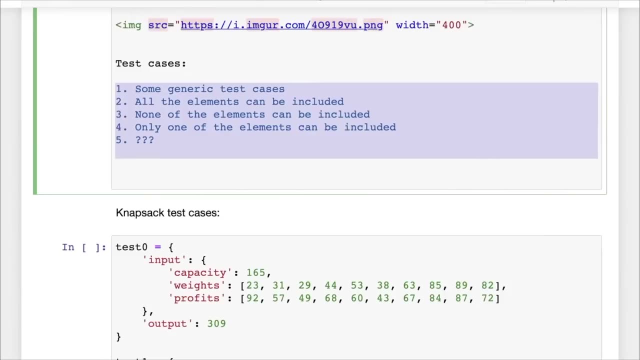 So now we have defined the problem, We have stated we've identified input and output formats, Now we need to come up with some example inputs and test cases. Once again, we have listed out a few test cases here, So we will have a few generic test cases where you have just a random set of weights and profits and you identify the knapsack, the optimal solution. 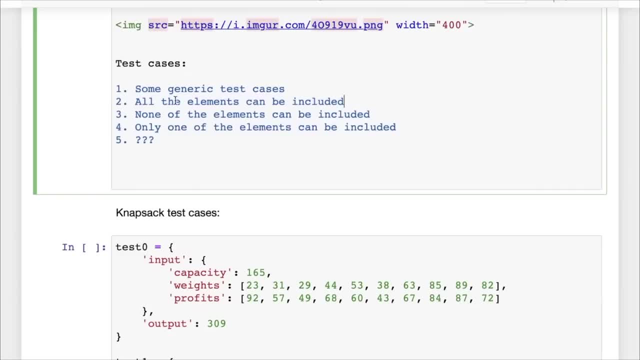 Then here's one option where all of the elements can be included. You can take everything. Here's another option where none of the elements can be included. You have to think about all these scenarios. Here's one where only one of the elements can be included. 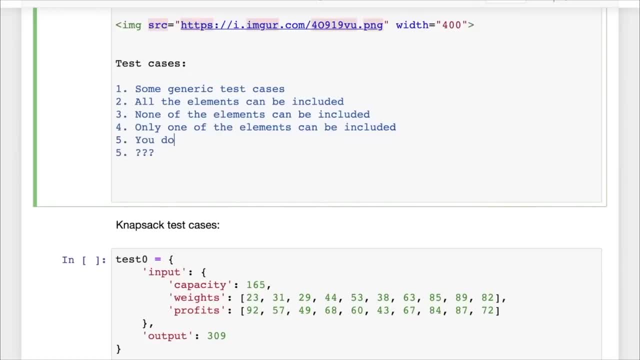 Then you may also think about areas where You do not use the. You do not use the complete capacity because the optimal solution is actually taking a lower capacity. So there may be a way to fill out to capacity but that may have a lower profit than another option which takes less than the complete capacity but has a higher profit. 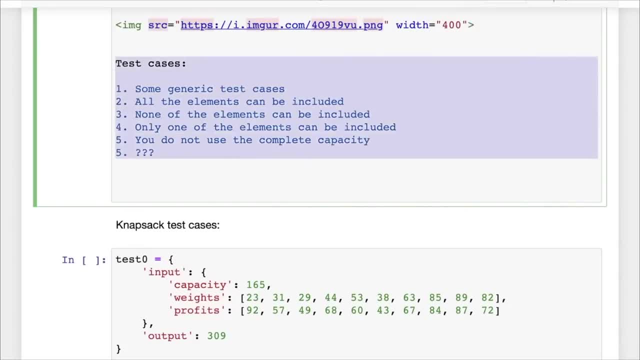 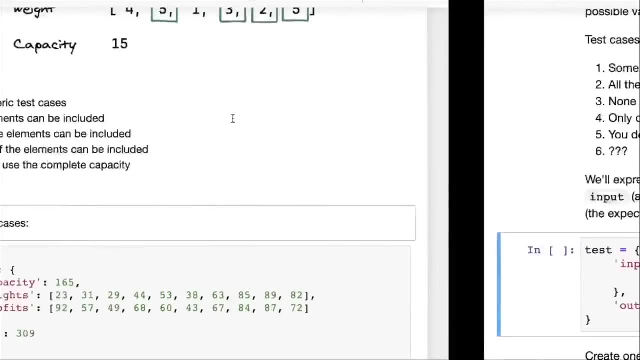 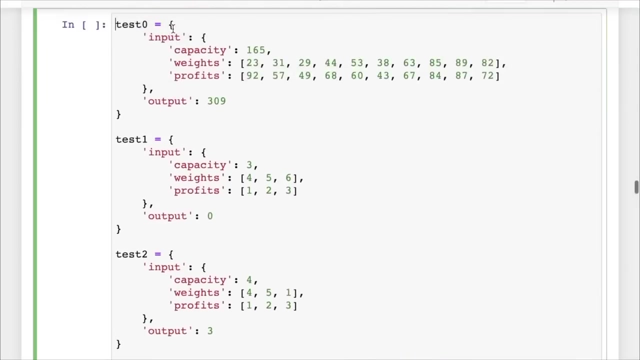 So think about some cases here, think about some good test cases here, and I will just copy over these for now, And then what we'll do is we will express these test cases Once again as dictionaries. we have test zero, test one, test two. all of these express and dictionaries, and these are covering all the test cases that I mentioned here. 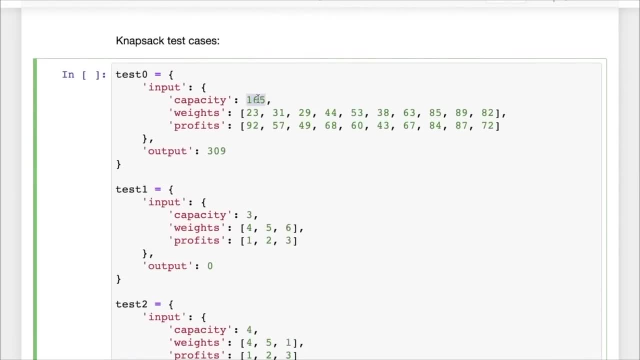 You can see, here are some weights and some profits, and the capacity is one, 65. And then the optimal solution is three zero nine. Now we are simply asking here for the optimal solution, the maximum profit that can be obtained. but an extension of this problem is to identify which are the elements that 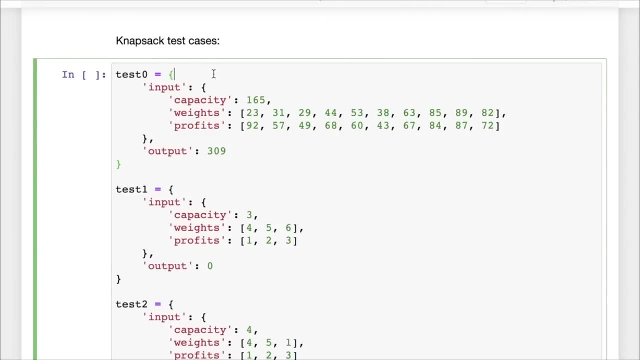 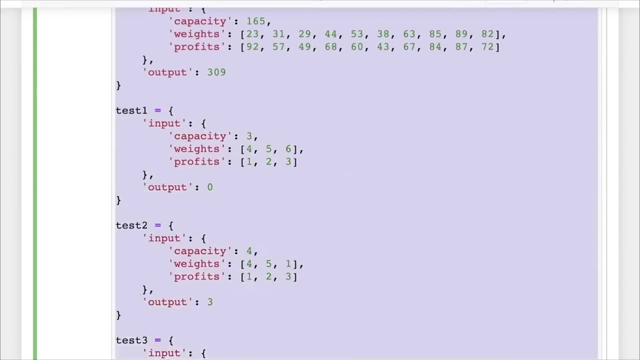 Should, Should be chosen, And it's a simple extension. It's a good exercise for you to try out and you can discuss it in the forums. We have test zero, test one, test two, test three and four and five. 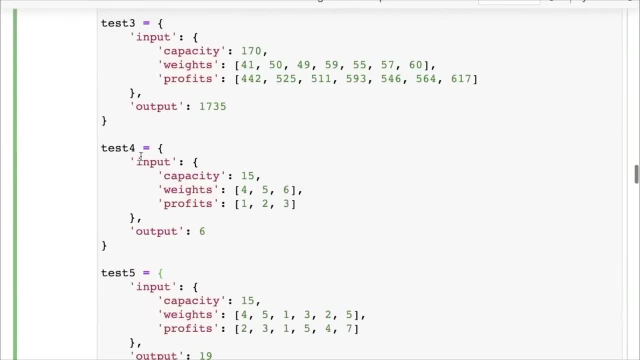 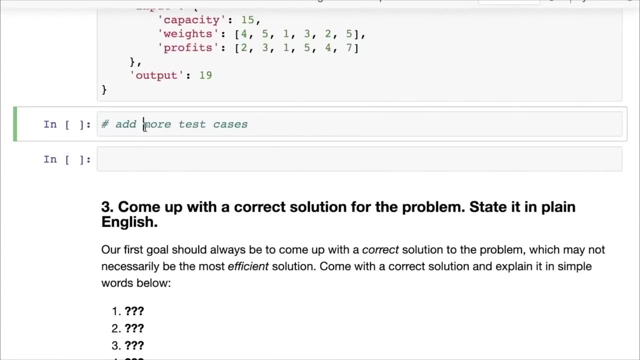 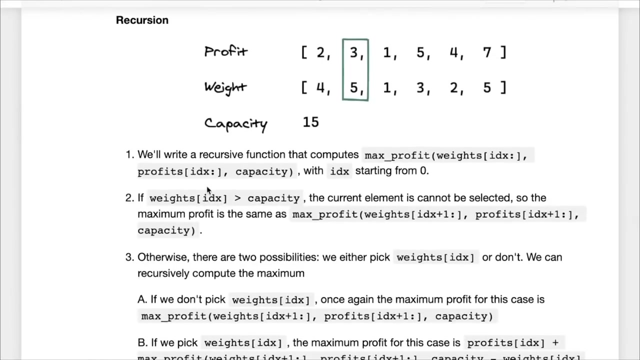 So we have a total of six, six test cases. Let's copy over these test cases here and let's put them here into a single string, And that gives us the test cases. Okay, Now coming up with a solution. So, once again, the first step is to try and come up with a recursive solution, and a recursive solution is, again, quite straightforward. 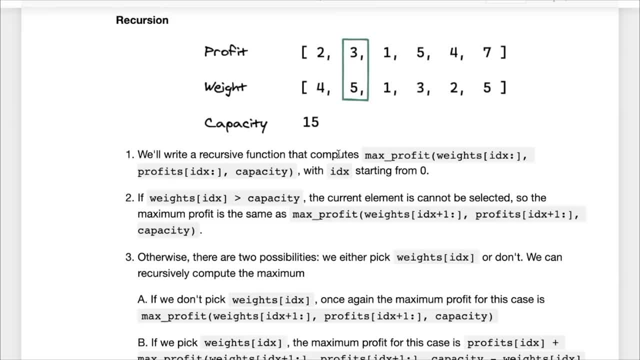 We'll write a recursive function: max profit, that given an index. So this time we have just one sequence, So given an index within the sequence. So let's say you have an index, IDX, it computes the maximum profit that can be obtained using the elements from IDX onwards. 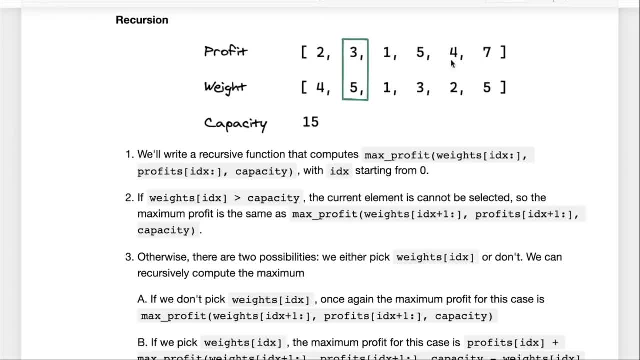 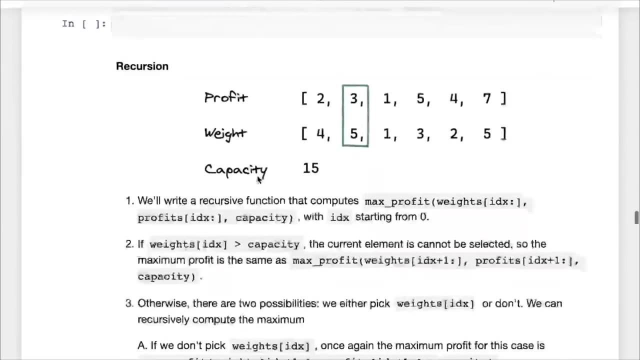 So three, one, five, four, seven, using all of these elements, IDX onwards the maximum profit that can be obtained right And using a given capacity. So it will take an index, So it will take an index and a capacity. 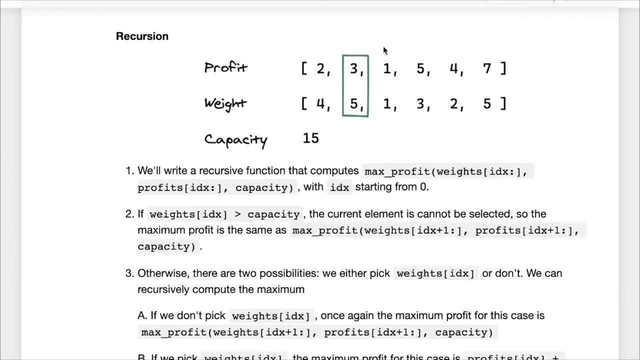 So if let's say the IDX is one, so it will then look at just these elements and have: the capacity is 10.. So it will try to fill the capacity of 10.. And that's the recursive function. And one. Why are we creating a recursive function like this? 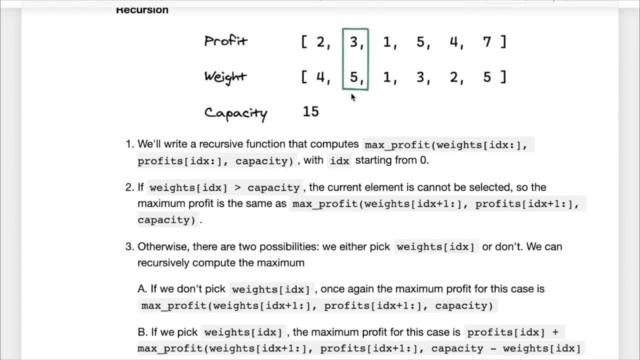 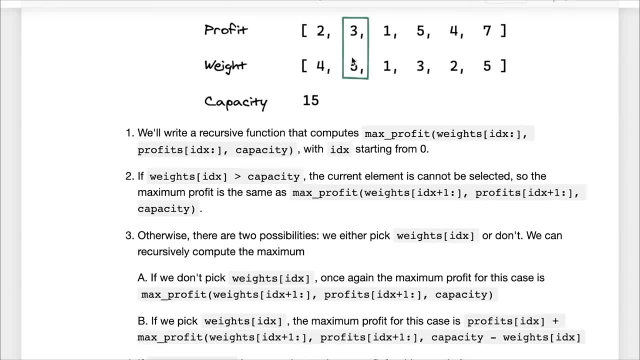 There's a simple reason. Now suppose IDX has the value one and the capacity is 10, or let's say the capacity is three, Then the weight of this element is greater than the capacity. So that means it cannot show up, It cannot be selected, because it cannot fit inside the bag, the knapsack that we have. 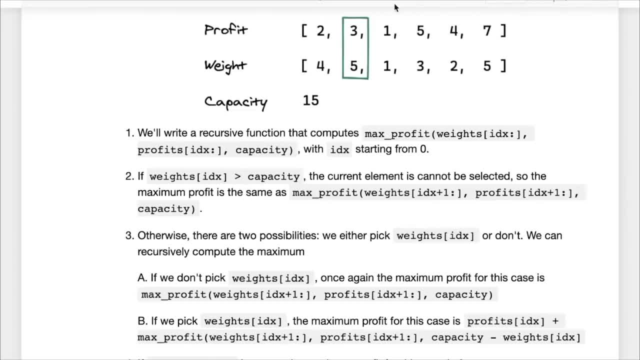 So then, the solution for this sub problem with IDX equal to one and capacity equal to three Is same as the solution for this sub problem with this element removed, because you cannot include this element within the knapsack right. So if you remove this element and simply consider these elements, the remaining elements, which essentially means IDX plus one, 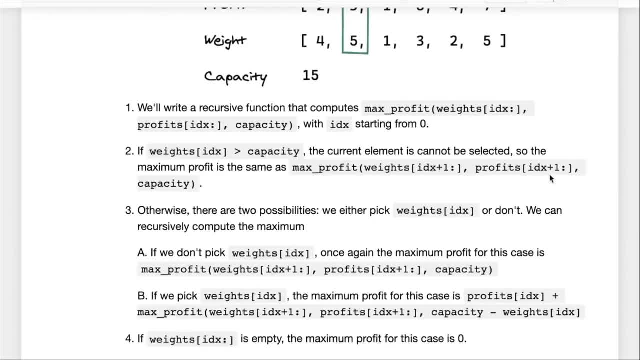 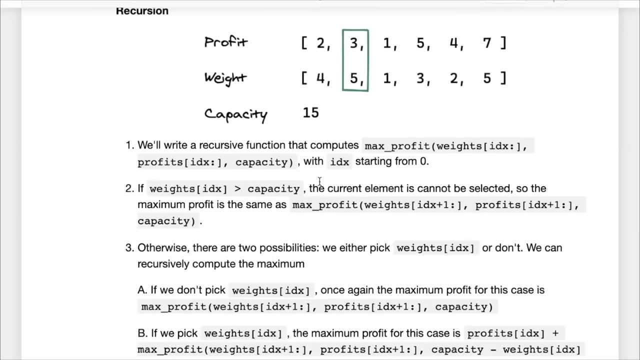 So max profit of IDX plus one, profit of weights IDX plus one, profits IDX plus one and capacity is the answer, or max profit of weights IDX, profits IDX and capacity, Because the current weight five is greater than the capacity three, which is which the recursive function has been invoked with. 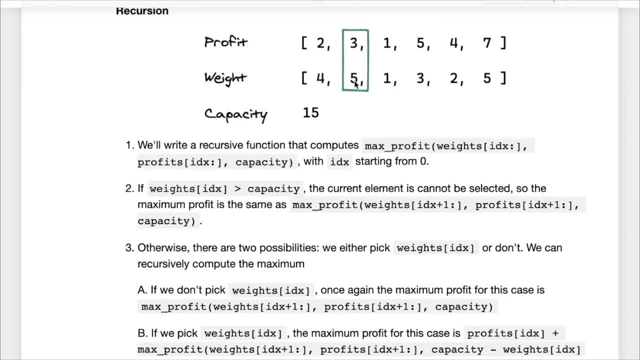 So that's one option. but the more general case is that you have enough capacity. So let's say you have a capacity of 10, recursion was called with a capacity of 10 and you are at IDX one. So then you have two choices. 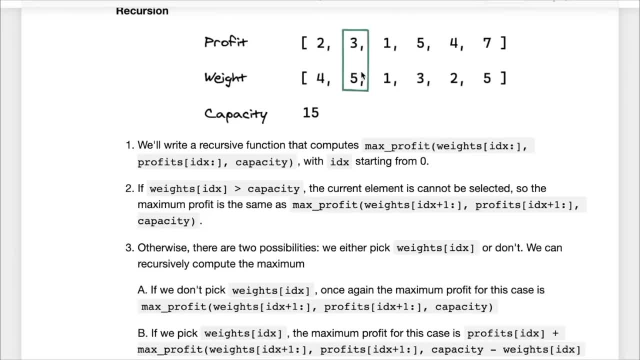 Either you include this element in your knapsack or you do not include this element in the in your option, because you don't know whether the optimal solution will have This element or not. So you try both. So there are two possibilities. 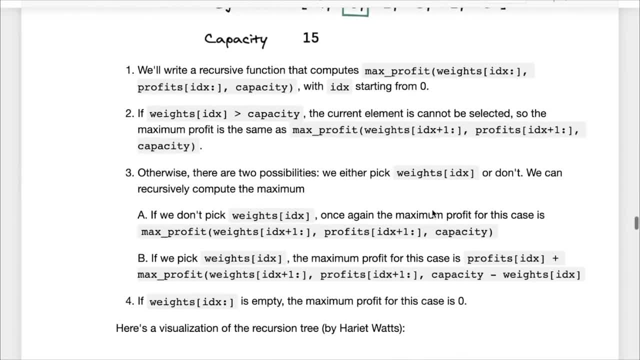 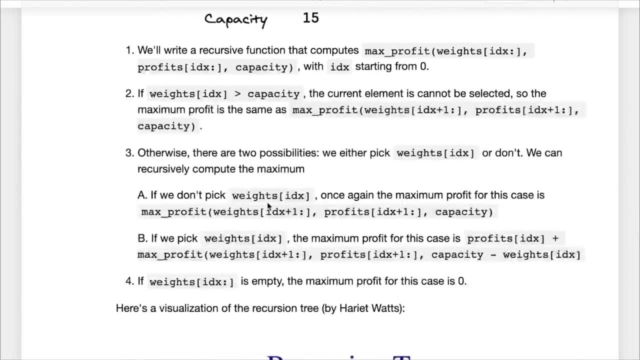 We either pick weights IDX, this element, or we don't, And what we can do is we can simply compute the result in both cases and pick the maximum. So if we don't pick weights IDX, then once again, if we don't pick this element, so the capacity remains the same. 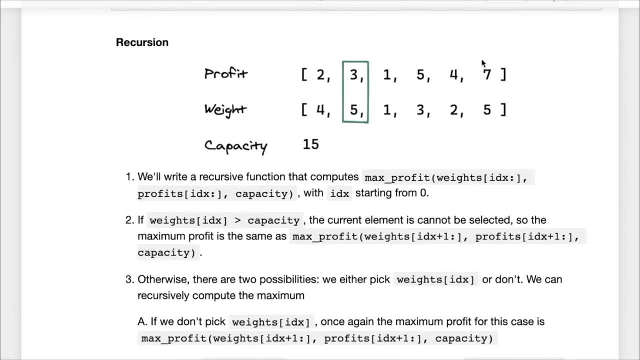 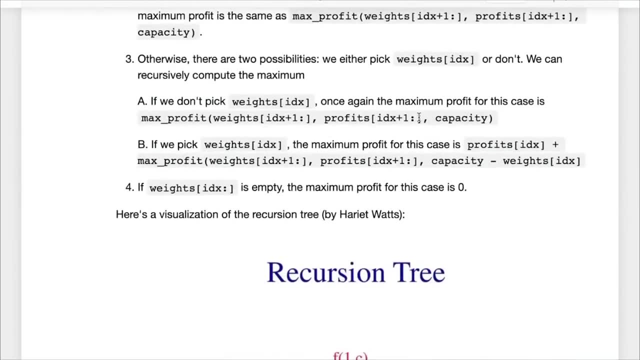 Let's say the capacity was 10.. So we simply try out to fill out the capacity of 10 using the remaining elements. So we simply call max profit with weights: IDX plus one, Profits IDX plus one onwards and the remaining capacity, which is 10.. 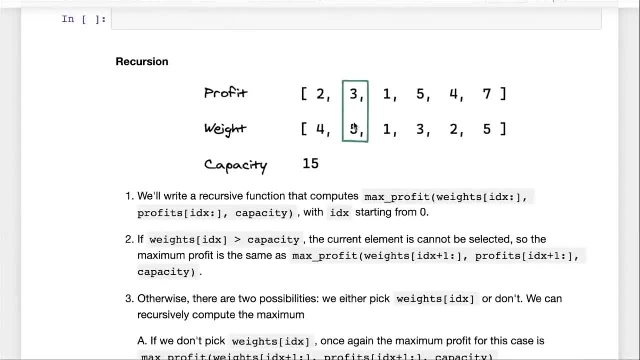 But if we do pick the element, if we pick the element and we had a capacity of 10, then the optimal, then the solution, the best solution in this case will have a profit three more than the solution for this case And since we also use of some capacity, so we need to add three in the profit and we need to subtract five from the capacity. right, 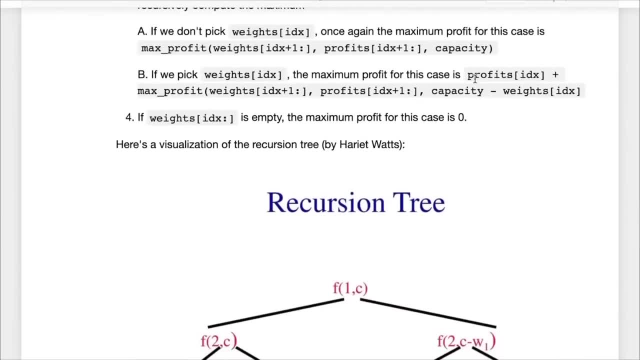 So if we pick weights IDX Then the maximum profit for this case is profits of IDX plus max profit of weights IDX plus one onwards profits IDX plus one onwards. But because we've used up some capacity, we reduce the capacity in the recursive call. 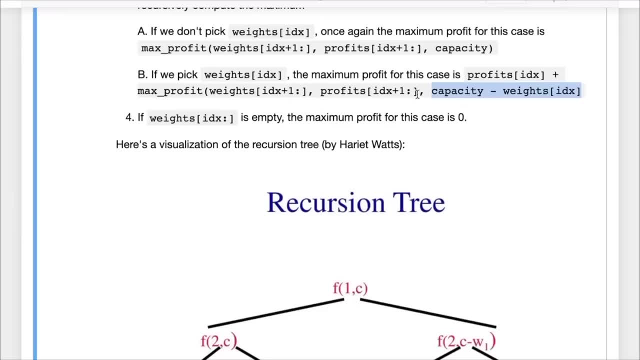 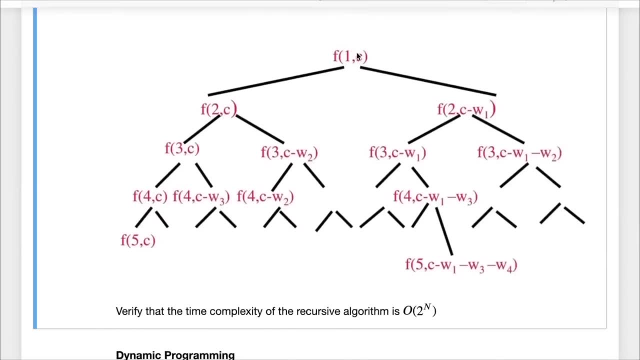 Okay, And that is why a recursive call takes both an index and a capacity. Okay, I hope that makes sense. So here's a recursive tree that tells you the same thing. We started the first index and we, we have the capacity. 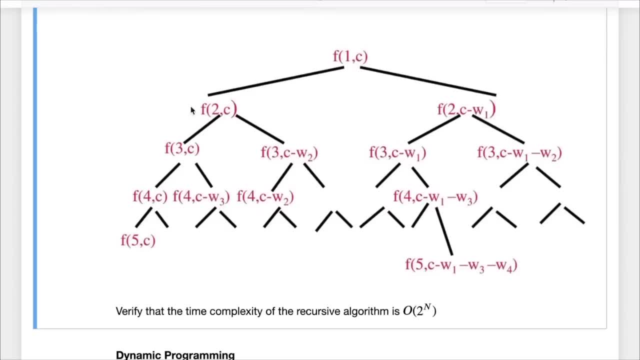 Okay, Okay. So if we don't pick the first element, then we simp. the answer is simply the the best solution for second index, onwards with the same capacity. If we do pick the first element, then the answer is the second solution: onwards with the reduced capacity, with a profit added. 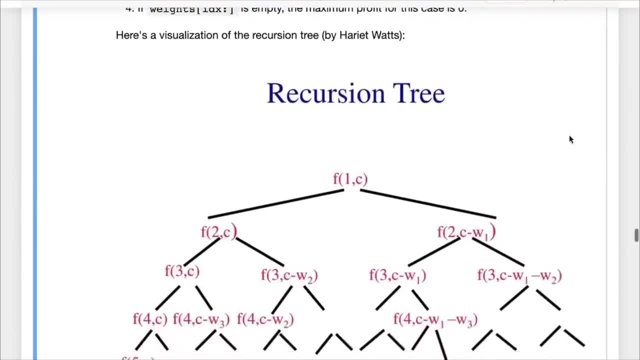 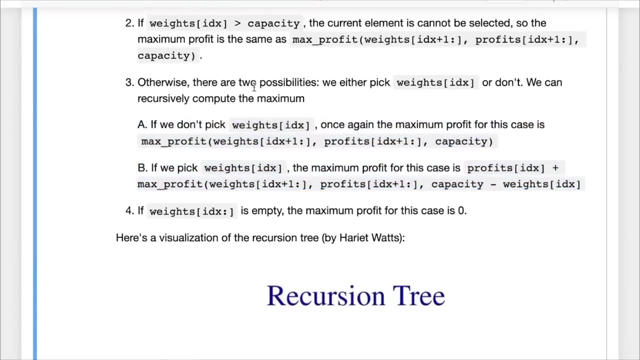 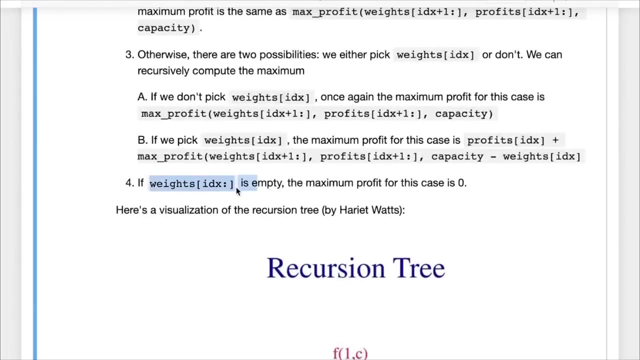 Okay, And then we simply take the maximum of these two cases. So we call these two recursive calls and then we simply take the maximum of these two cases to get back The final result or the final best answer. And the final end case is that if we've reached the end, if weights IDX onwards is empty, if the index that we're tracking has reached the very end, then 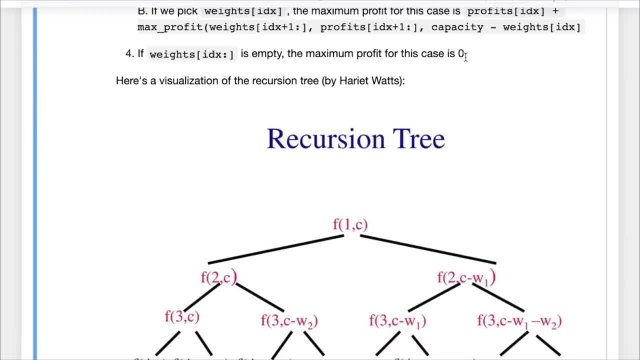 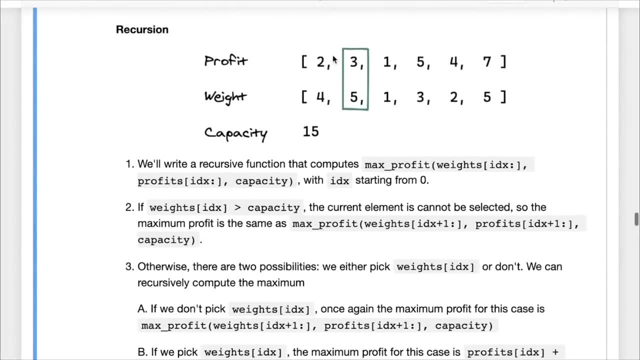 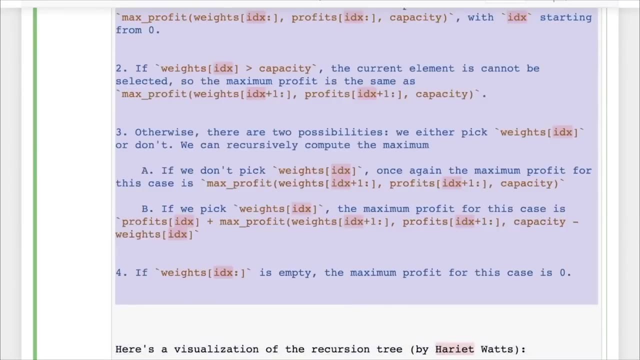 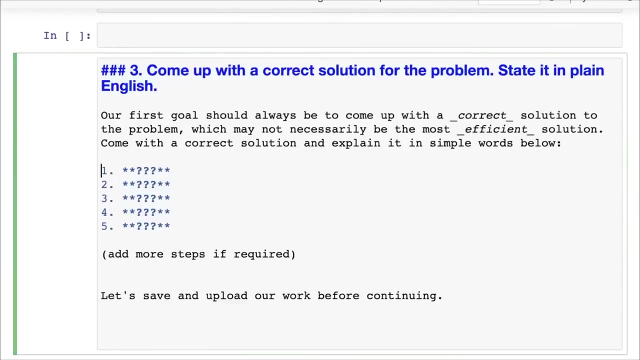 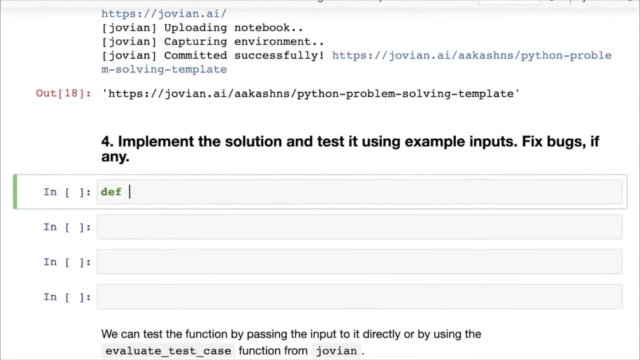 irrespective of what the capacity is, the maximum profit is in that case is zero. So let's try and implement this Now. let's copy this over as the explanation: Okay, Okay, Okay, And let's try and implement the solution. Let's say: let's call it max profit recursive. 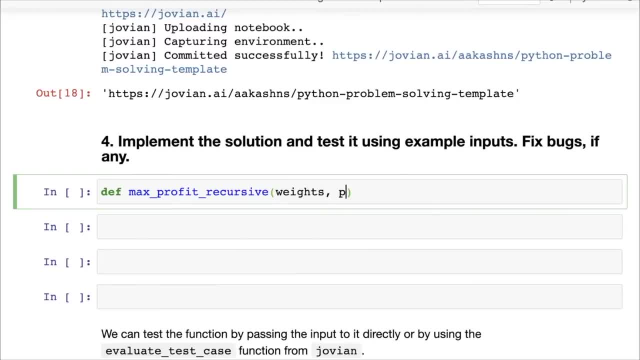 Okay, And this is going to take a set of weights, It is going to take a set of profits and it is going to take a capacity, And it's also going to take an index, which the index will start out at zero. So now, if the index is, we started with the base case. 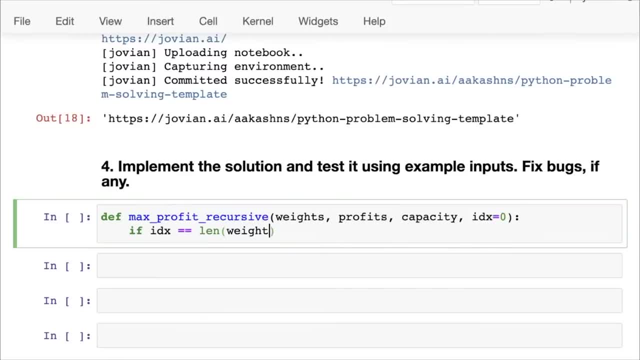 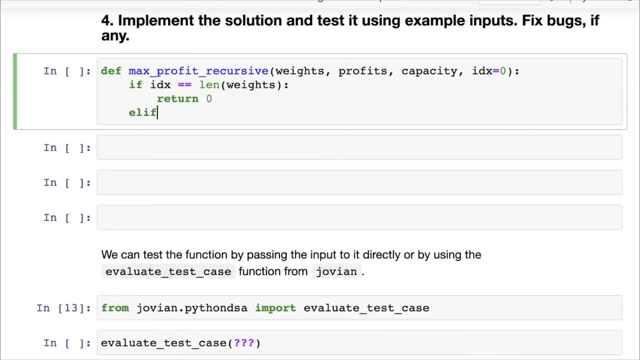 So if IDX equals the length of weights, in this case there's nothing left to do. We simply return zero because we don't have any more elements. Then we check if the weights IDX is, so the current element is greater in weight than the capacity. 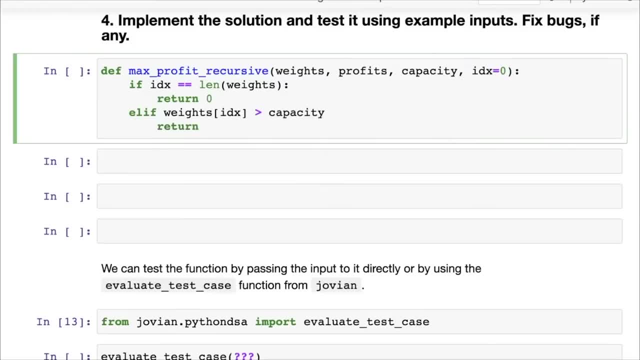 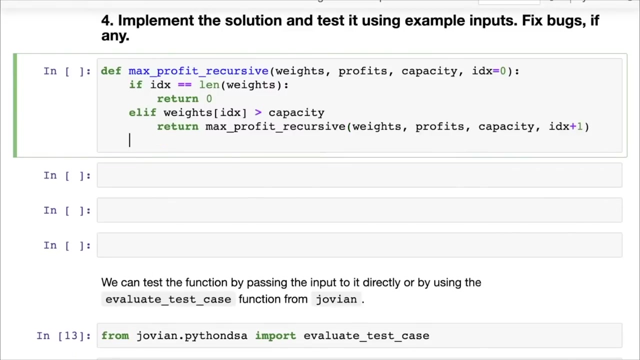 Then it's a pretty straightforward solution. We simply return max profit, recursive of weights, profits, capacity plus one- I'm sorry, capacity- and IDX plus one. So we simply ignore this element because we cannot fit it in the capacity that we have. 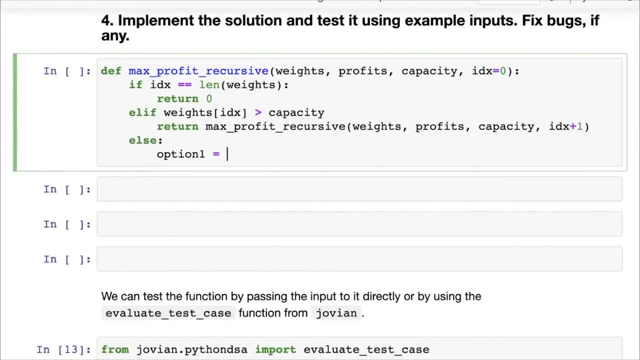 Else. we have two options. We have option one. Option one is: even though it can fit within the bag, we don't take it. We because the optimal solution may still not have it. just because it fits does not mean we should take it. 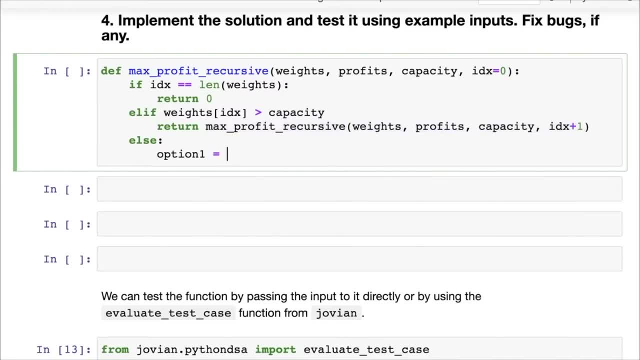 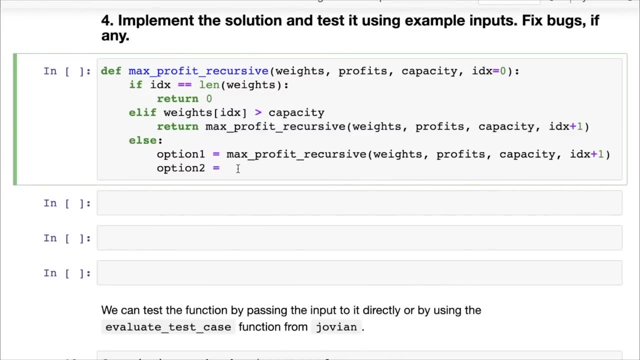 So we look at the option one, which is once again the same as this, where we ignore this element. And then we have, we look at option two. in option two, we actually put this element into the bag. So since we are putting this element into the bag, then we get- we get profit from it. 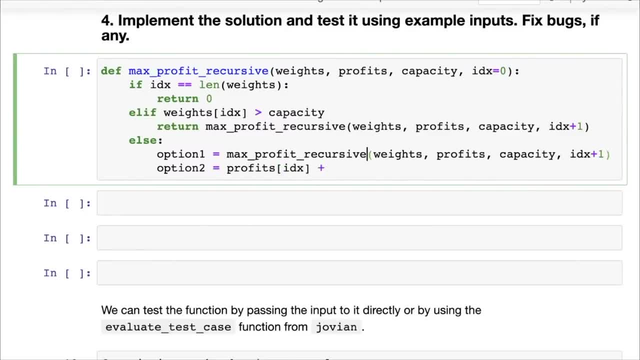 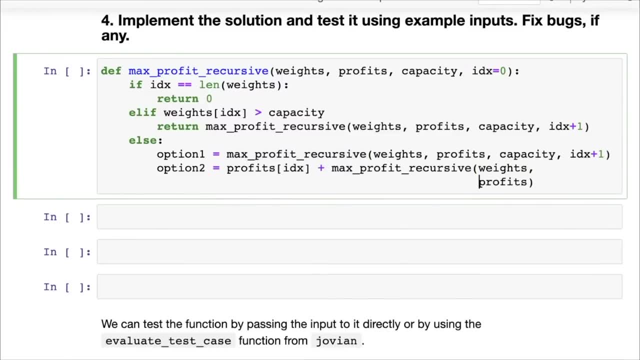 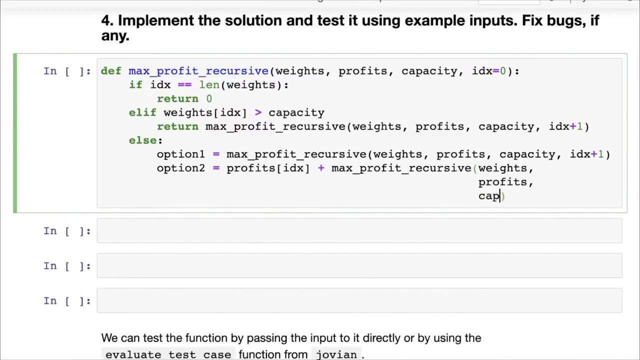 So we get profits of IDX And then we call max Profits recursive And this time we call it with weights and profits, And now the capacity has reduced a little bit because we have taken this element. So now we can, now we need to fill the remaining. 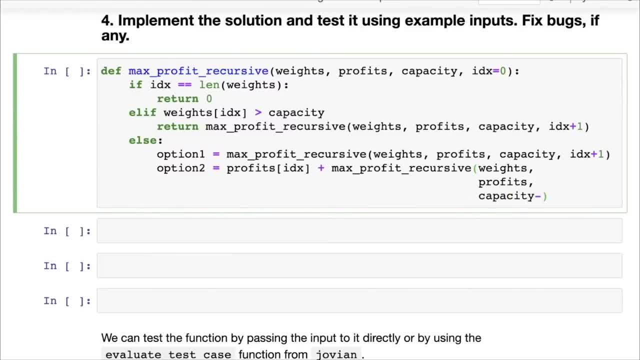 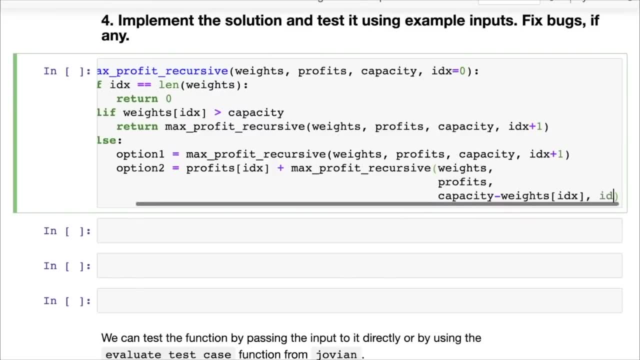 We feel the need to fill the bag with the remaining elements, from IDX plus one onwards, with a limited capacity of capacity minus weights of IDX, And then, finally, we just put in IDX plus one So that we can Start calculating the solution from the next element onwards. 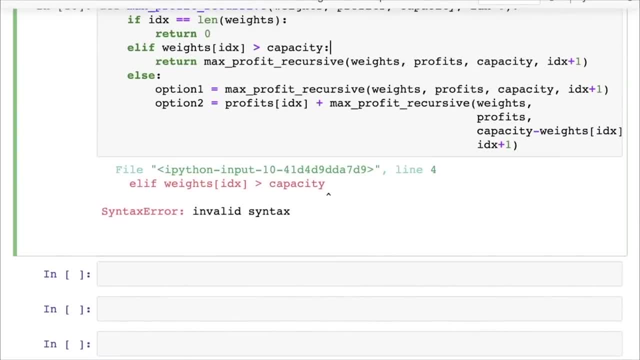 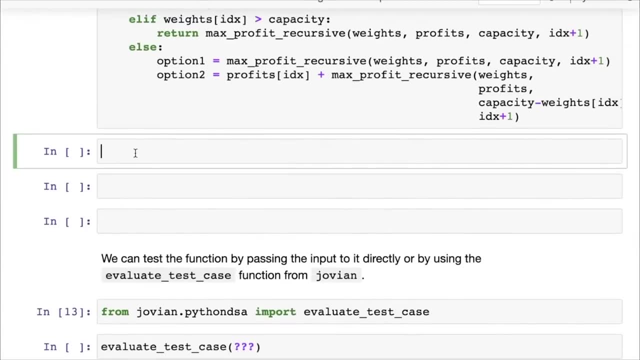 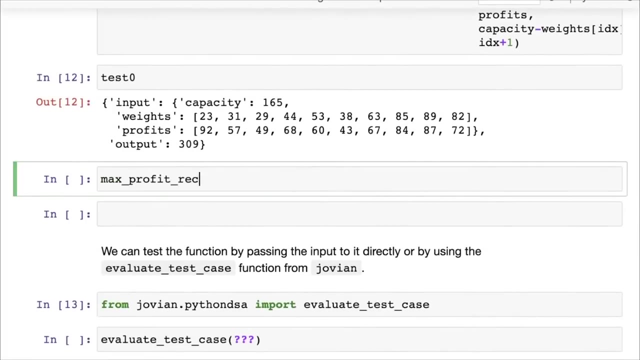 So that's max profit recursive. again, not very difficult, It is just about six, seven lines of code and let's try it out. Here's test zero. Let's try max profit recursive with test zero input. Okay, Okay, Okay. 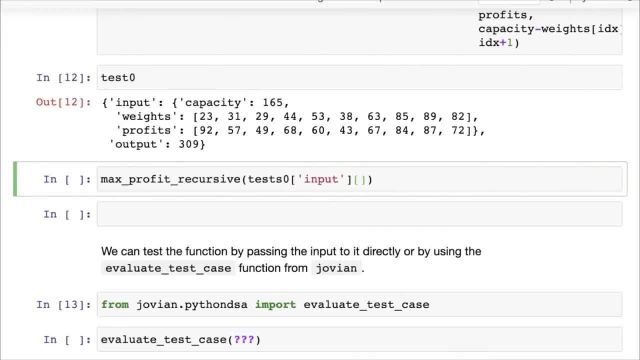 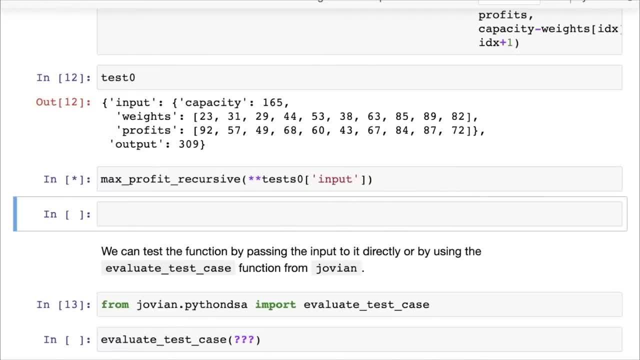 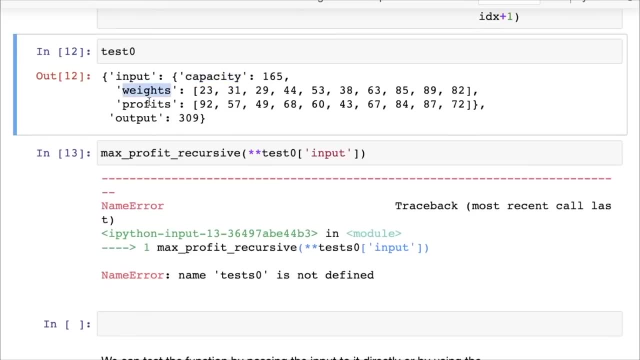 The simple way to do that is simply to put in star, star and we'll get back. All of these will get passed in capacity: We'll get past as a capacity parameter. in vates, We'll get past, and as the weights parameter and profits as a profits parameter. 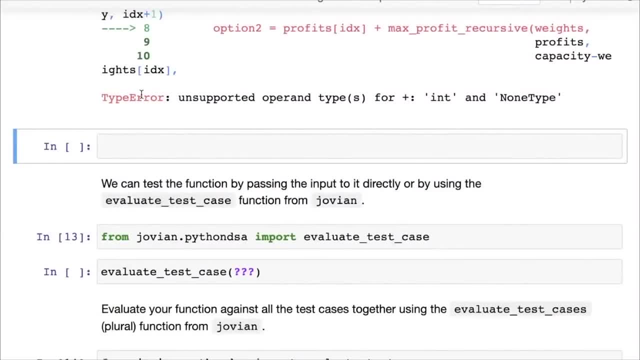 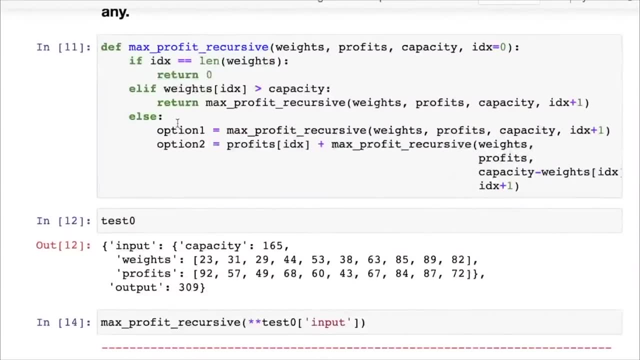 Okay, So we've encountered an error, and that's completely fine. Completely fine to encounter an error. I see So what we've done here. So here is a. we have not really taken the maximum of these two, We've just defined the two options. 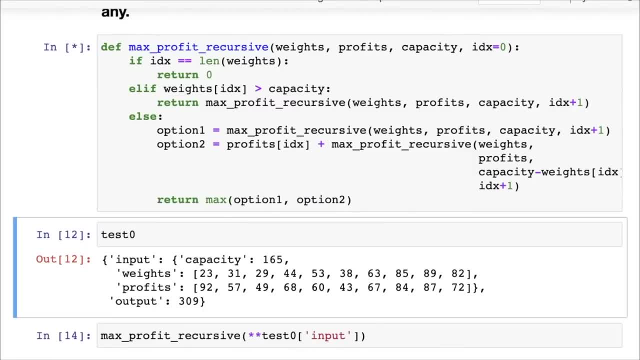 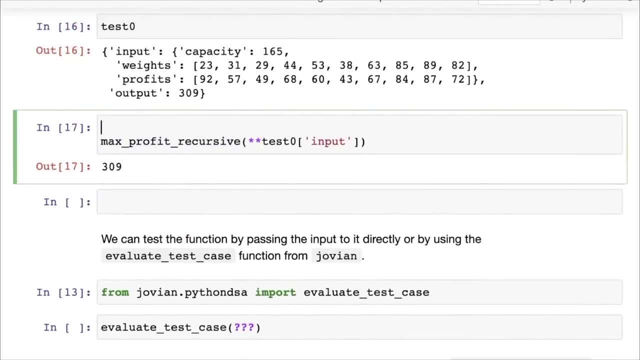 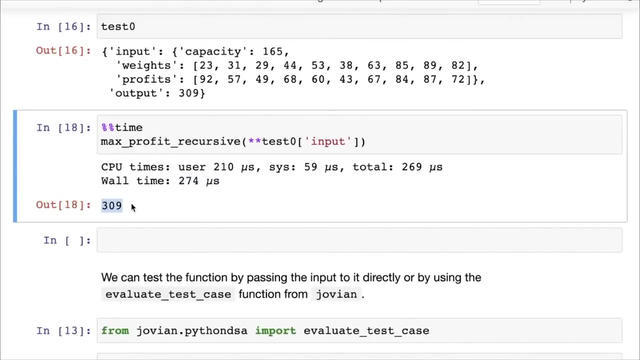 So we do need to take max of option one and option two. Okay, Once again. this is why helping test, having test cases, helps And you can see that now we call max profit and we can also add a timer here. The max profit. it takes 210 microseconds but it result, it returns the result 309.. 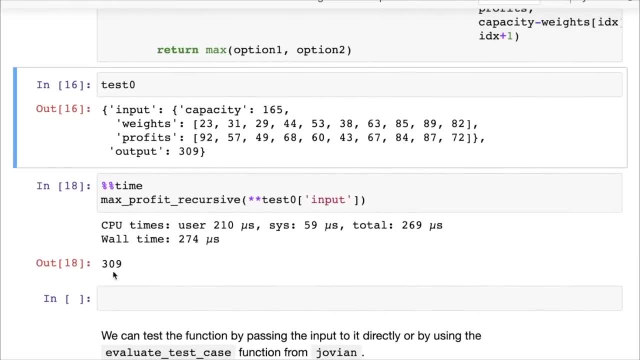 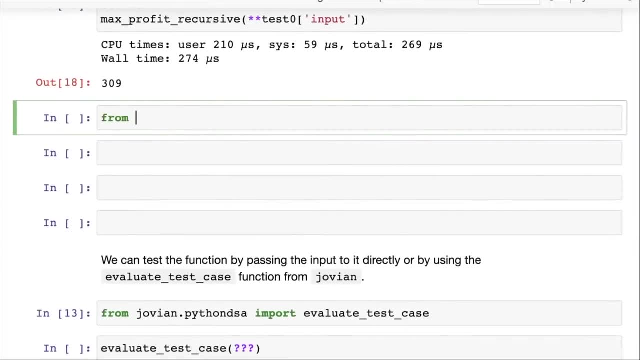 Great, We get back the result 309 here, which is what we expected. So our function is working correctly. We can even evaluate it on all the test cases. So from Jovian dot Python, DSA, we import evaluate test cases. 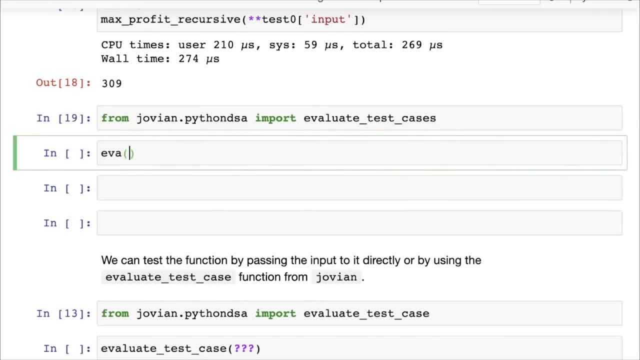 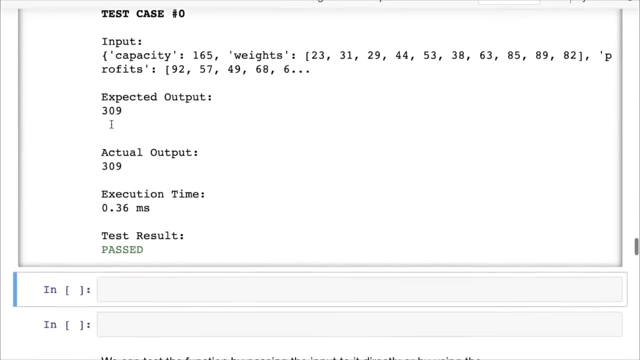 And then we simply call evaluate test cases on all the inputs. So we pass in max profit Recursive And then we pass in all the test cases as tests. Now you can see that we have these test cases and each test case seems to be passing. 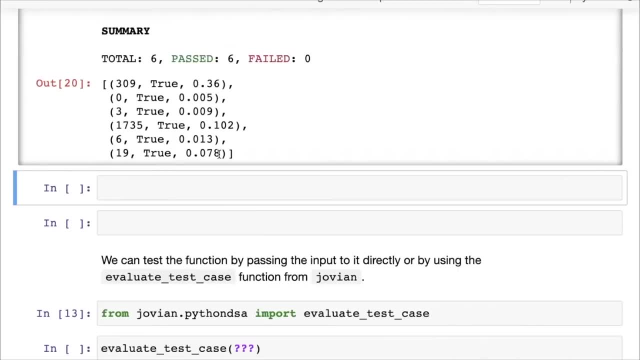 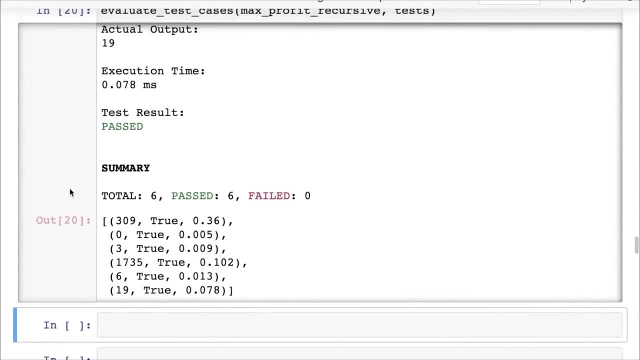 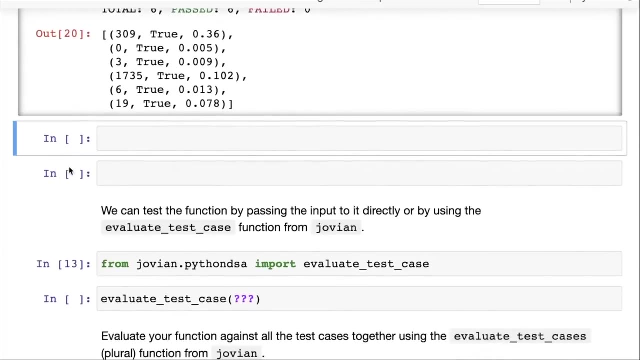 Just fine, All six X test cases have passed and these are the times they took. So that's your recursive solution, Pretty straightforward Once you reason it out. once you maybe just look at an example, draw a tree of recursion yourself, work it out. 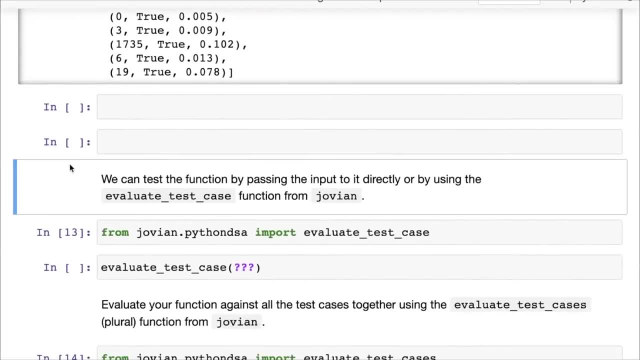 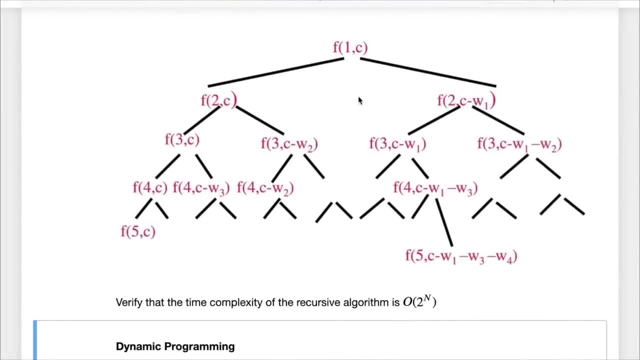 Okay, The code is, in fact, in most cases, fairly simple, And this is what the recursion tree looks like Each time we make a choice to either include the element or not include the element. And now you can reason the complexity very easily, because now we have N elements for each one. 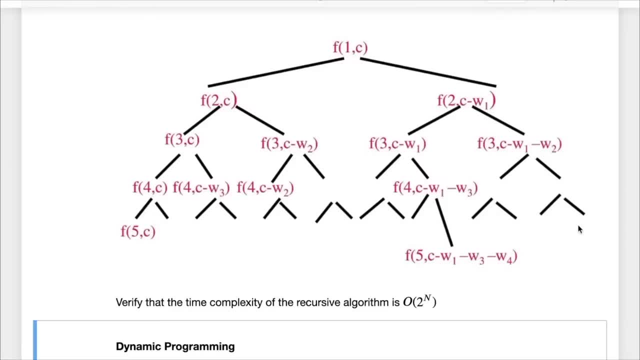 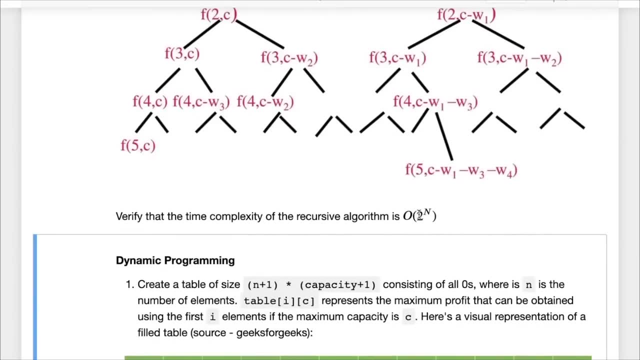 We keep making this choice. So that means we end up with two to the power N leaves, And from there it follows that the complexity of the recursive algorithm is order of two to the bar N, right, So it could be two times or C times two to the bar N. 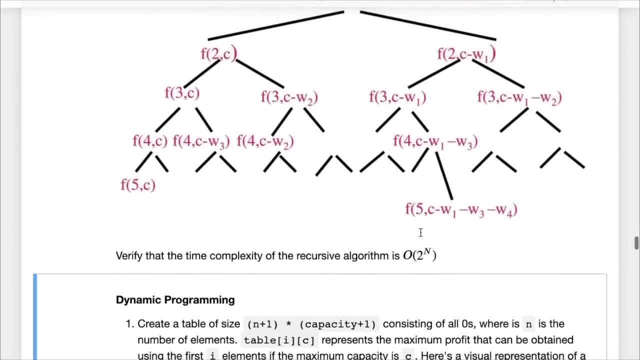 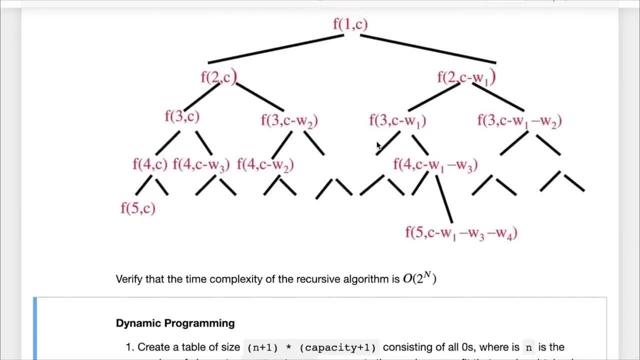 But uh, and in the bigger notation it's order of two to the power of N, So it is exponential. and complexity- And why is it exponential? complexity, once again, there are. it's a possibility here that we may be computing a. 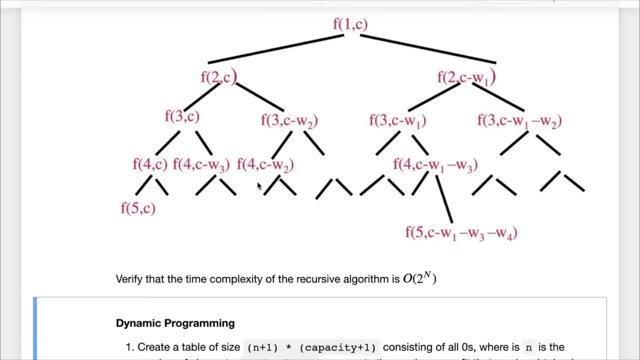 lot of things repeatedly because we are creating so many of these sub problems. So it's possible that we may be creating, we may be re-computing a lot of data here. So now the task for you, or the an exercise for you, is to 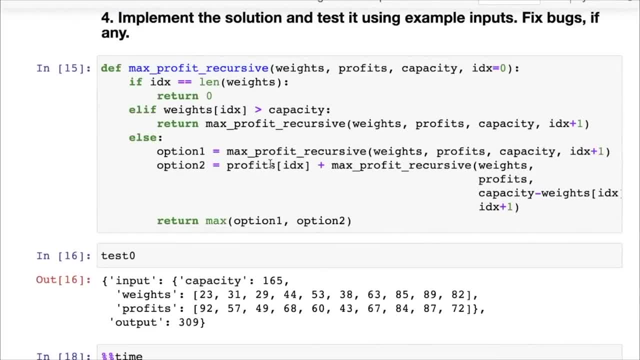 To write the memoized version of this. So what is it that you need to memoize Now? the trick here is to look at what is changing within the recursive calls. So now, in max profit recursive, you can see that weights and profits remains the same, but it's the 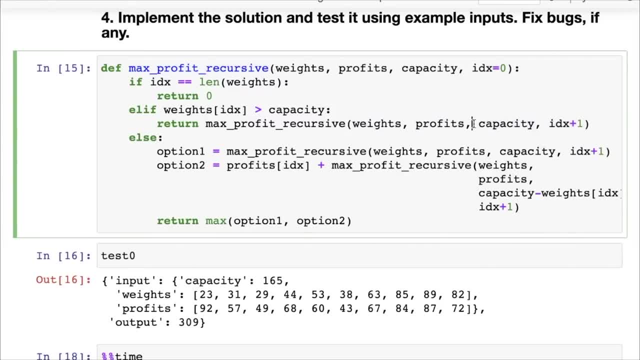 capacity and the IDX that change. So you can take the capacity comma, the index, the IDX, as the key in your memoization dictionary and each time you compute. So each time let's say you compute this or you. Okay. 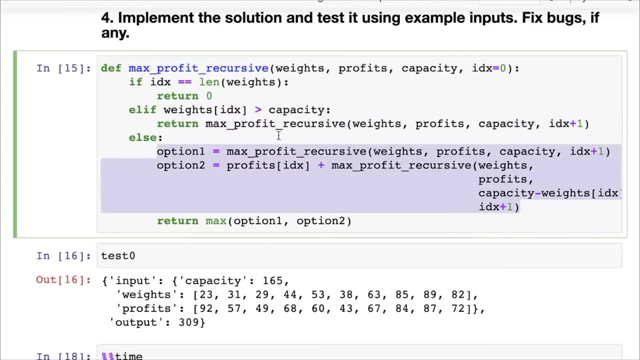 Okay, So you compute this, or you compute this, store the result in the dictionary before returning it, And then, at the beginning of the recursive function, check within the dictionary if this value is already present. Okay, So remember what we did: for longest common subsequence, we defined a recursive function internally. 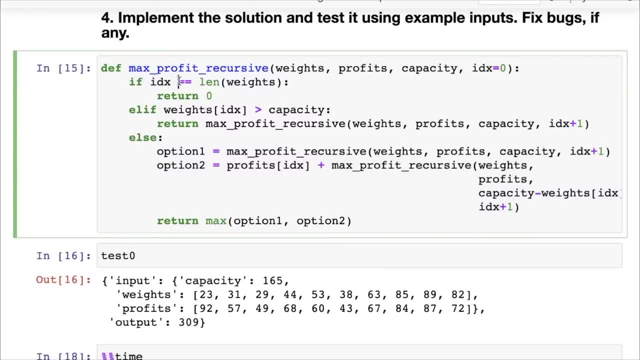 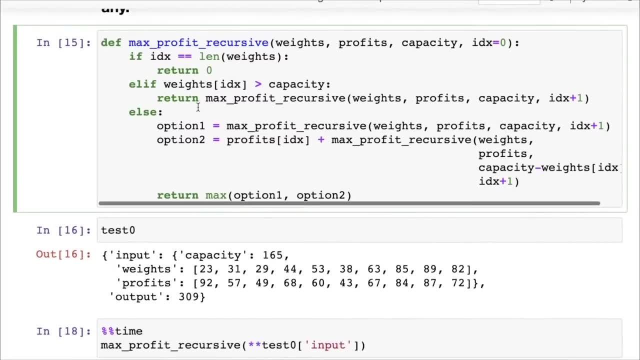 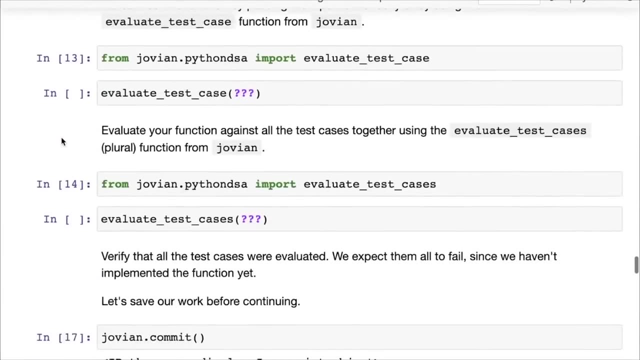 We defined a memo, a dictionary, internally, and the recursive function kept either checking the dictionary or filling the dictionary if it could not find a value. Okay, So you can eliminate a lot of the repeated work in your problem. Okay, So that's a challenge for you to try out implement the memo solution. 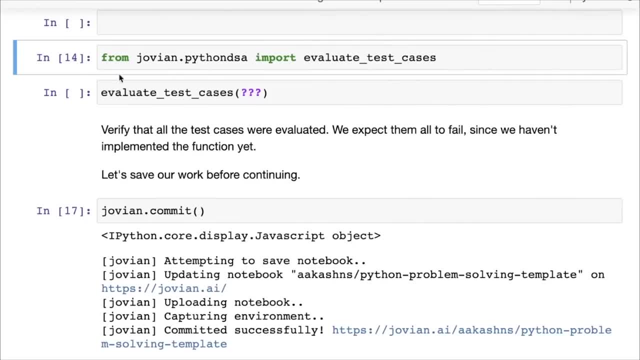 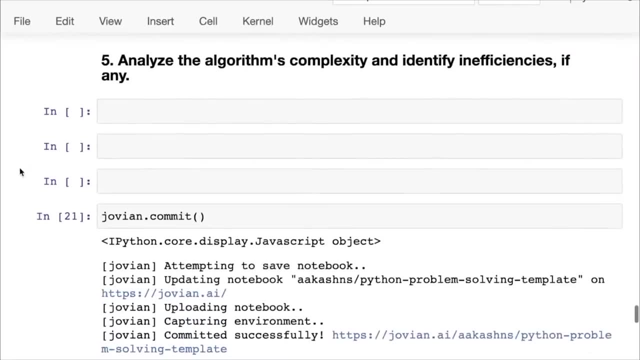 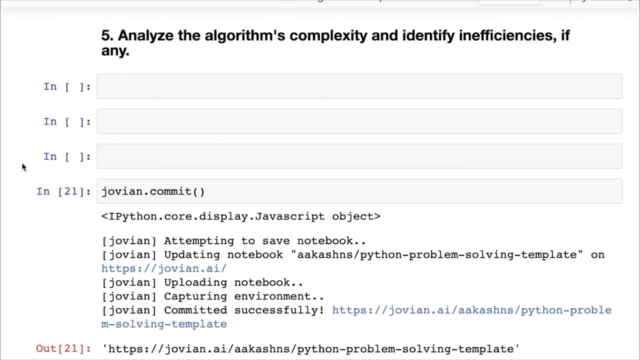 And what we'll do is we will go ahead and we will implement the dynamic programming solution. So let's just come at our work once again, and we've analyzed the algorithms. complexity in recursion: It's order two to the power of N In memoization. 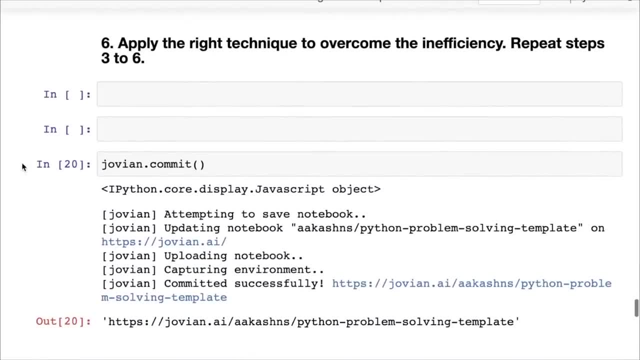 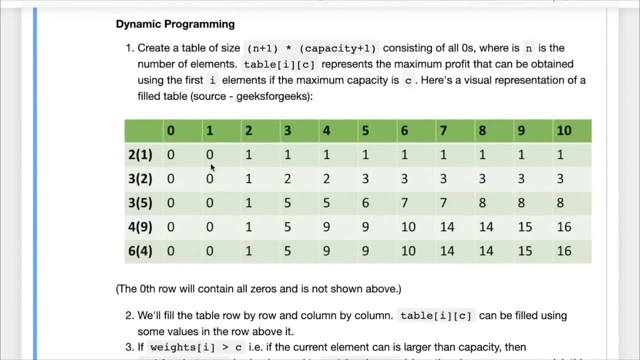 Now, that's an exercise for you. What do you think the complexity will be? but let's apply dynamic programming. So let's look at a dynamic programming solution. Now, once again, for dynamic programming you have to create a table. You always, almost always, have to create a table. for dynamic programming, 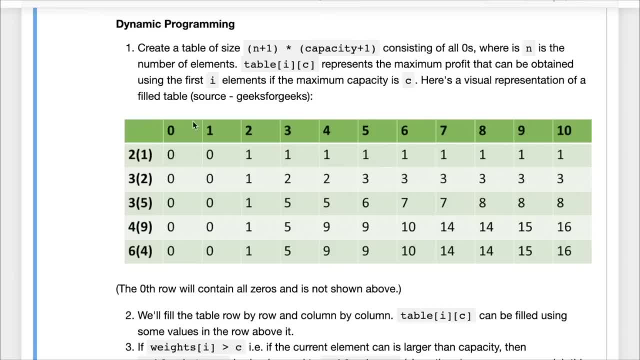 And in this case we can see that there are N elements. So there are N rows within the table because we have N elements to choose from, And we are. we have a number of columns going from zero to capacity, plus one going from N. 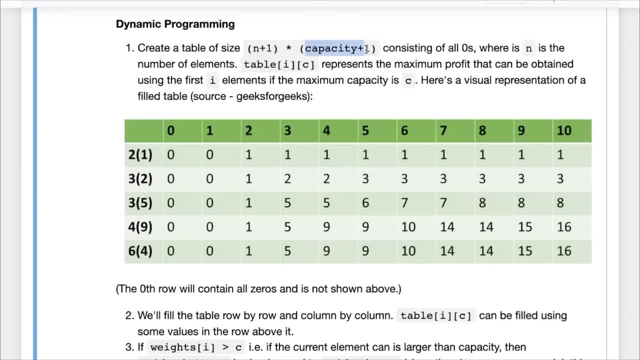 Going from zero to capacity, And that's why there are total of capacity plus one columns, And in fact, what we can do is we can also include another column at the top here, another row at the top here, which we have not, which is not shown here, but what N represents, uh N is a number of elements. 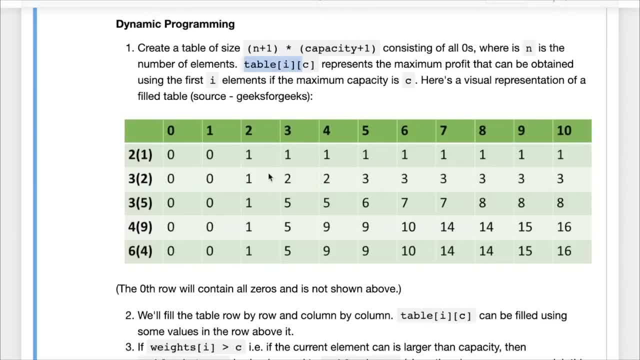 So what N represents or what the particular element in the table represents. so table of I, comma C: what it represents is the maximum profit That can be obtained using the first I elements If the maximum capacity is C. okay, So if your maximum capacity is C, let's say your maximum capacity is three- what is the maximum profit that you can obtain using the first two elements? 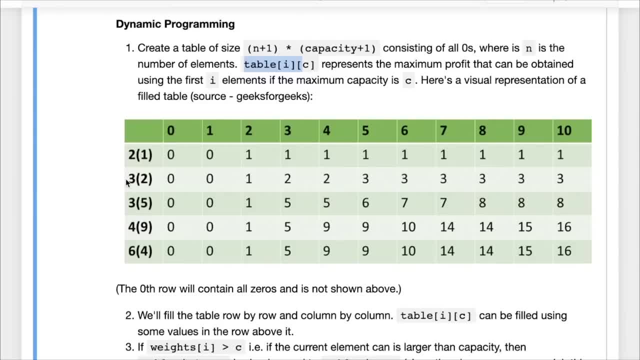 So, um, here, let's say we are at this person, So using the first two elements off the list within this capacity. Okay, So the first two elements have weights one and two and the capacity is three. So you can, you can actually pick a. sorry, the first two elements of weights two and three and the capacity is three. 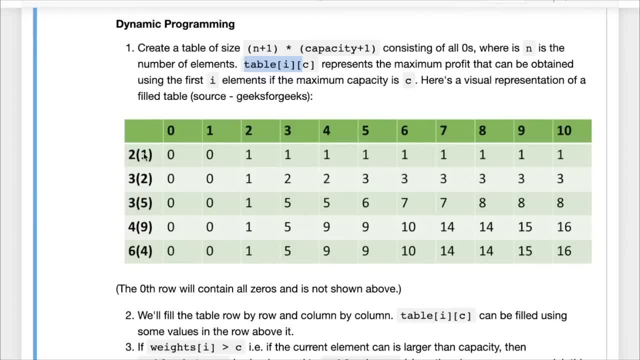 So you either pick this element or pick this element. Now, if you pick this element, the profit is one, And if you, if you pick this element, the profit is two. So the solution is to pick this element and you get- uh, you fill the capacity three and you get a profit of two. 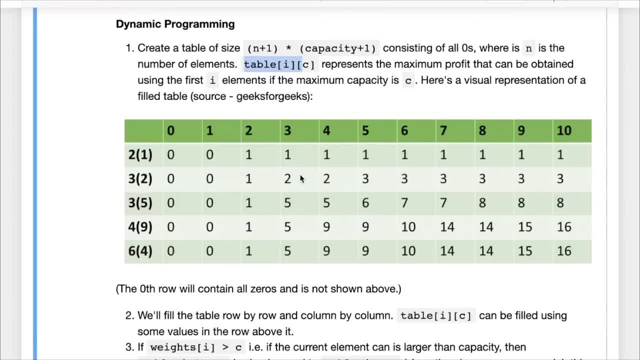 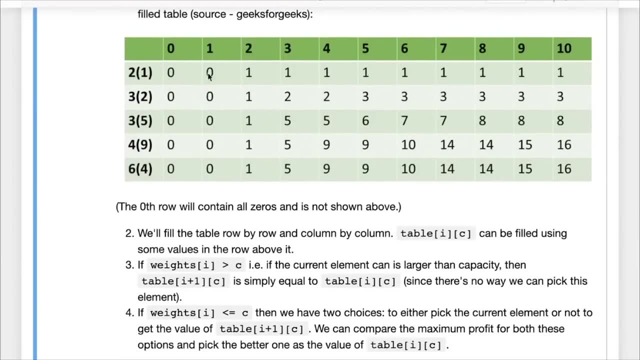 You cannot pick both because your capacity is three. Okay, So that's the logic here. A very simple visual representation. Now remember that there will also be a zero throw here, which we have not shown, but this is something that should be here. another zero throw. 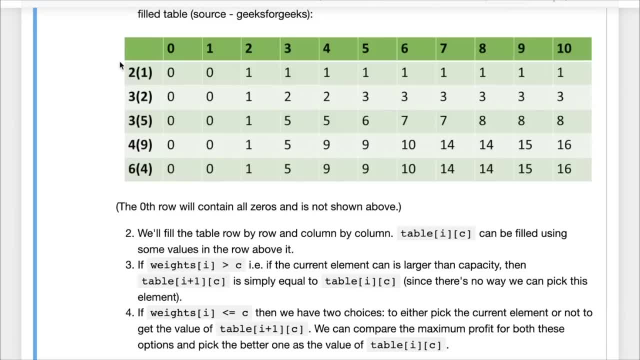 So the zero throw represents that you've not picked any of the elements. And if you don't pick any of the elements, it is simply going to contain all zeros, And that's why it's not shown here. The first row assumes that you have picked. you can pick only the first element. 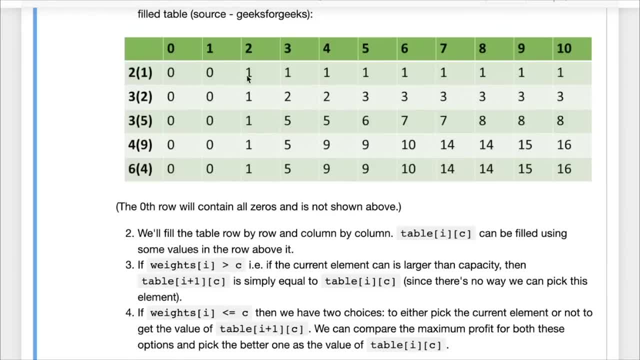 So you can. you, you can't pick the first element till a capacity of two and then, from a capacity of two onwards, you pick the first element and that has the maximum capacity of one, the maximum profit of one, the second row or the row number two with row with index. two represents the fact that you can pick both of these elements. 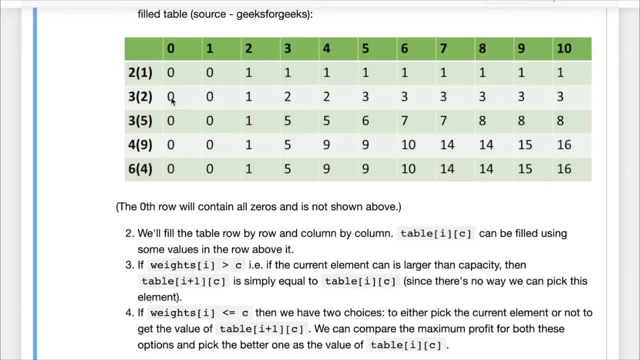 And if you can pick both of these elements once again at capacity zero- none of them can be picked at capacity one- None of them can be picked at capacity to- this element can be picked, which has a way to, and it gives you a maximum profit of one. 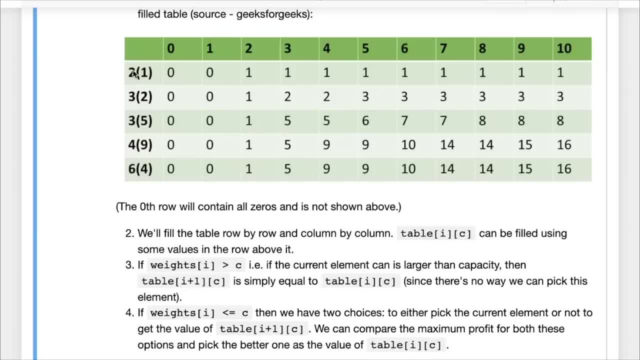 At capacity three, this element can also be picked. So now you have a choice to pick between the two of these. So you might as well better pick this one, because this is going to give you a higher profit, And then, finally, when the capacity becomes five, you can pick both of these elements, and you can pick both of these elements. 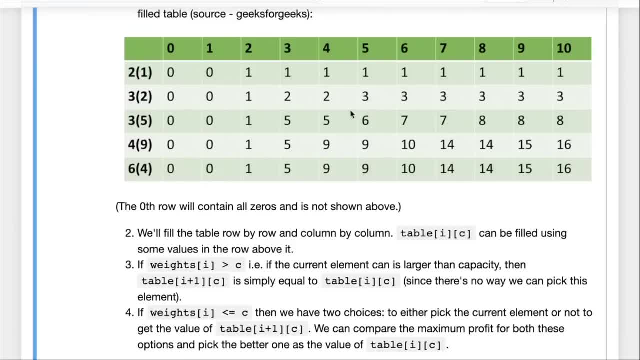 And that is going to give you a profit of two plus one, three and so on. So you keep filling out the stable. for each step here, or for each set of first I elements, you fill out the capacity Table and then you use the information to fill out the next row and the next column, and so on. 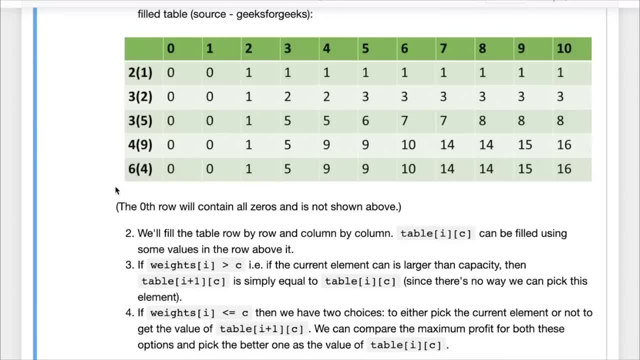 Okay, And finally, what we need is using all the elements and using the maximum capacity that we have. what is the maximum profit that we can obtain? So the last element of the table will give you the result. Okay, So what does the logic look like? 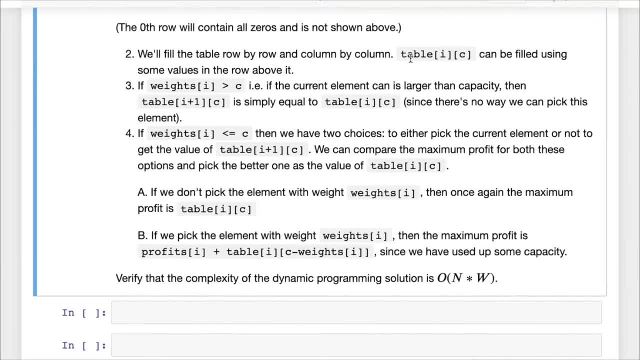 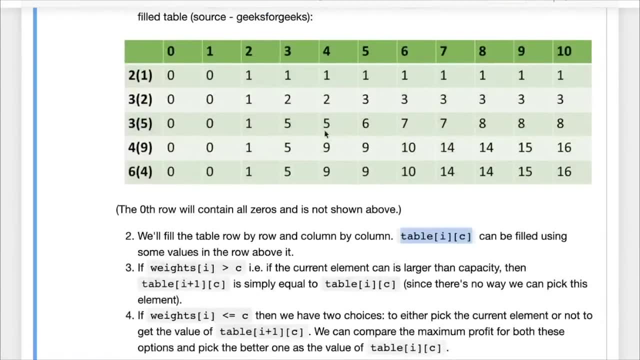 We will fill the table row by row and column by column. Now, if table of I comma C, table of I comma C, let's say this is a certain position here- Table of I comma C can be filled using some values in the row above it. 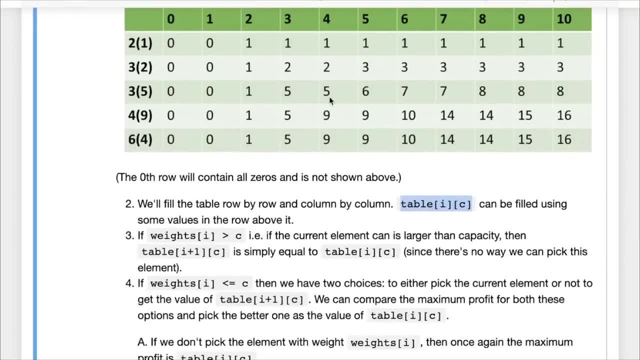 Okay, Now, if you look at the table of I comma C, you look at, look at this element, for example: yeah, let's look at this element here. So in here, C has the value three, and then I has the value zero, which is a role that is not shown. one, two, three, four. 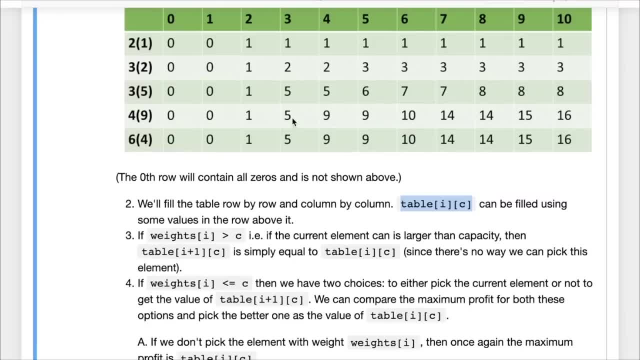 So I has the value four And C has the value three. So if, yeah, So if weights of I is greater than C, so zero, one, two, three, four, Um, if, if, the, if this, if this weight, so this weight, the weight of this element is greater than the capacity. 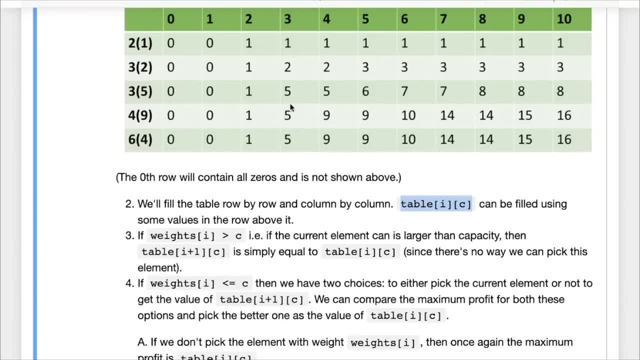 So the weight of this element is, for it is greater than the capacity, Then this element cannot show up in this maximum profit. Why? Because it's weight is greater than the capacity, So obviously it cannot show up in the maximum profit. Now, if it cannot show up in the maximum profit, then this? then this cell can be filled using the value above it, because in any case you cannot put in this element. 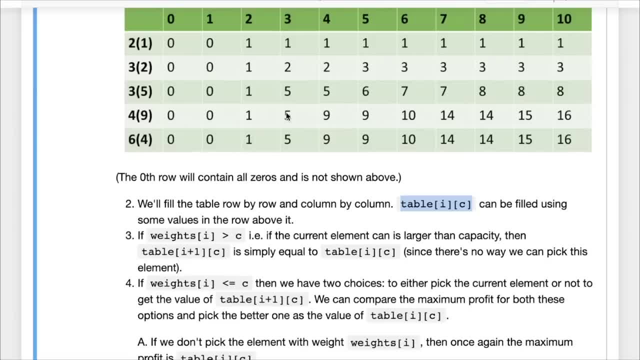 So you might as well get the result by using the first three elements, And in that case the value of the cell is obtained from the value of the cell above it. That's one case. Now, on the other hand, let's come here. 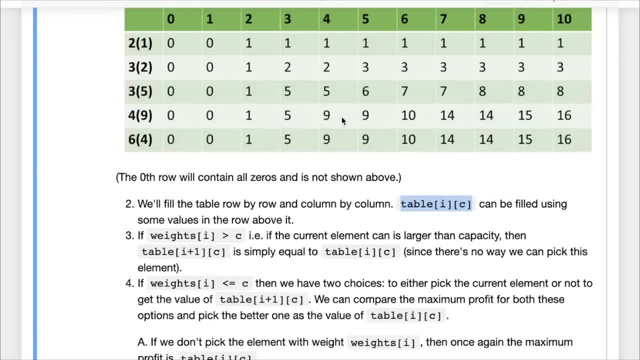 You come to this case, It to this cell, In to fill this cell because you have a capacity of four. you have the option of either choosing this element or of not choosing this element. Now, if you do choose this element- let's say you choose this element with a capacity of four or with the capacity of four, you get back a profit of nine. 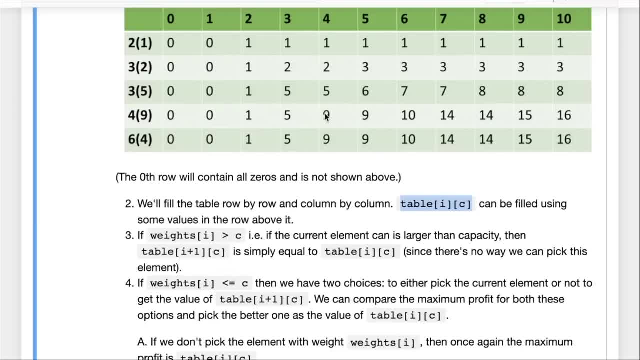 And now you have no more capacity left to create more, to fill more elements. On the other hand, if you do not choose this element, then that's the same as this value, Because if you do not choose this element, then you have to fill the capacity of four using the value of using the first three elements. 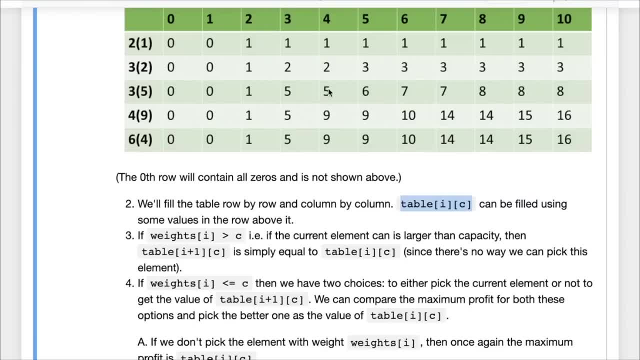 And that simply gives you the same highest profit as the previous cell right. So you just consider these two cases, whether we choose the element or we do not choose the element. Now, if, if you do not choose the element, the value comes from above. 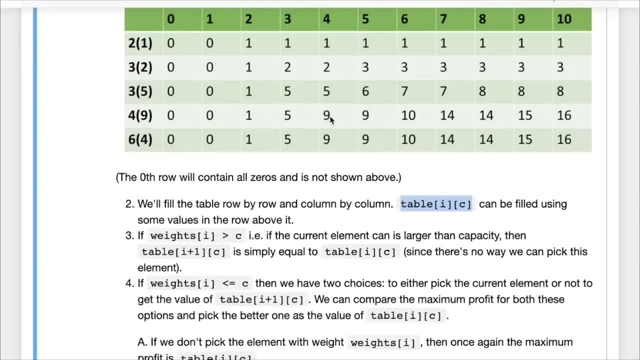 If you choose the element, then the value comes from where. let's see: if you choose the element, the profit of nine comes and you fill out a capacity Four, So you have no remaining capacity. but on the other hand, if the capacity was six and you choose the element, then you have chosen the element and you've used up the capacity for, so you can still use the previous three elements to fill the remaining capacity, which is six minus four. 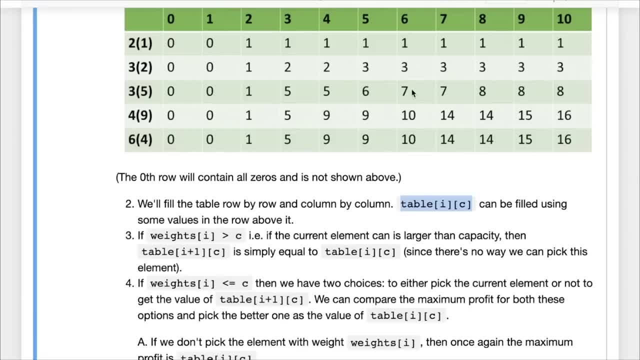 So it is your capacity of two. So you can go back to the previous row and check the capacity too and see how much was a maximum profit that you can obtain with capacity too. And it turns out that with capacity- Okay, So with capacity two, using the first three elements, you can obtain a maximum profit of one. 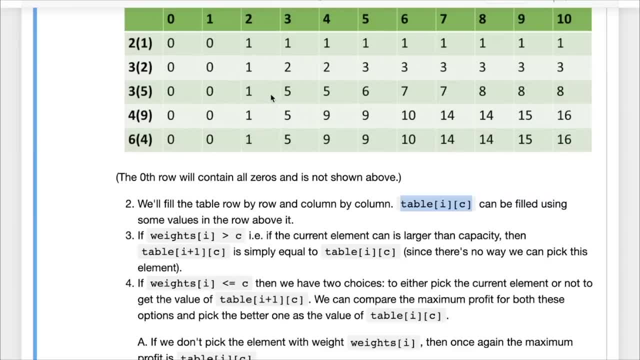 So the maximum profit here, when you choose the element, is nine plus one N. similarly, here, the maximum profit that can be obtained If you choose the element is nine plus seven minus a plus. from the previous row you pick the element with a capacity seven minus four, which is three. 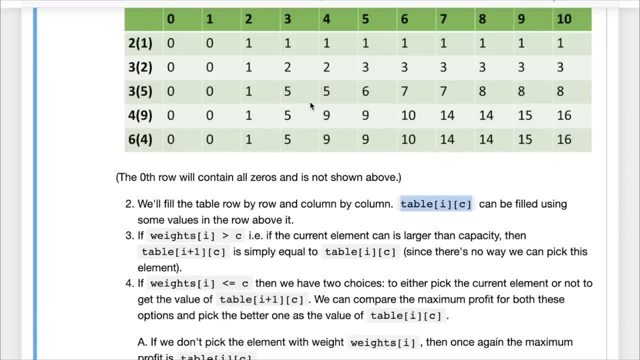 So nine plus five, 14.. Okay, So that's the logic here. So sometimes you choose the element, sometimes you don't choose the element And in fact, the solution, the result of the cell, is simply the maximum of either not choosing the elements- the maximum of this cell- or choosing the element and subtracting the weight, which is six minus four two. 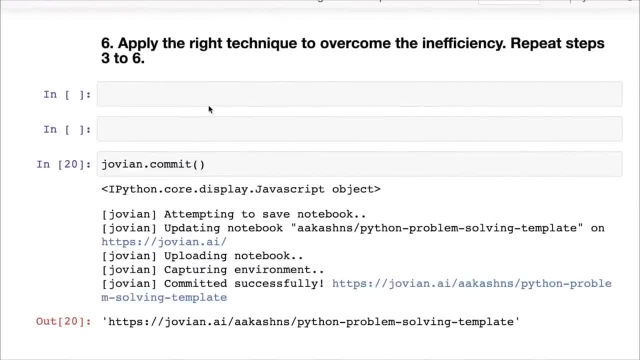 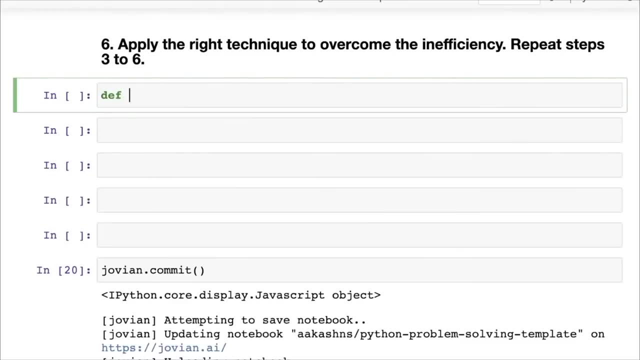 So maximum of this and that. okay, let's implement this same dynamic programming solution Once again. do work this out on paper. It really helps to work it out in paper. So let's say we have max profit, DB, the dynamic programming solution- we have weights, we have profits and we have a capacity. and then let's say N is Len weights. 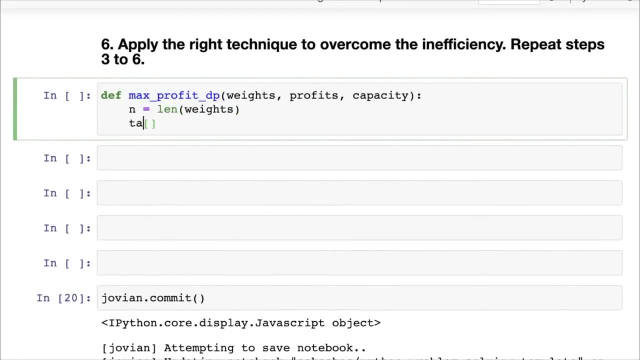 So we need to create a table. So this is our table. Our table contains N rows, So we have Len And then in. for each of the rows we contain, we have capacity plus one. Oh, we contain N plus one rows. 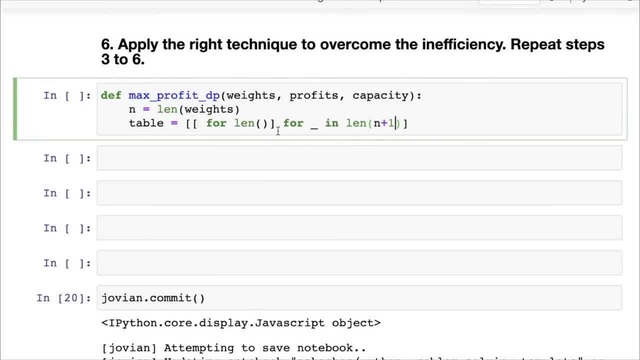 Remember. but we also want to consider the case where we don't consider, where we don't take any of the elements, and it is filled with zeros and the number of columns is capacity plus one to check the values from zero to capacity. So that's a table right now. 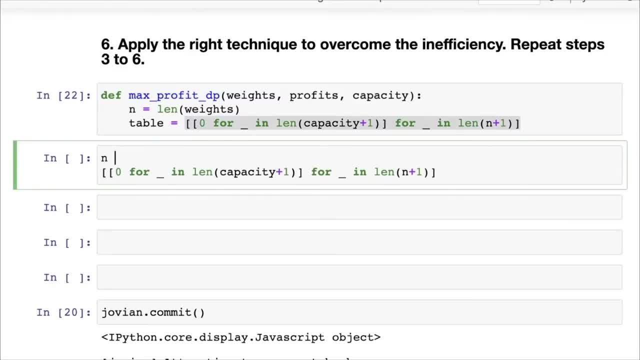 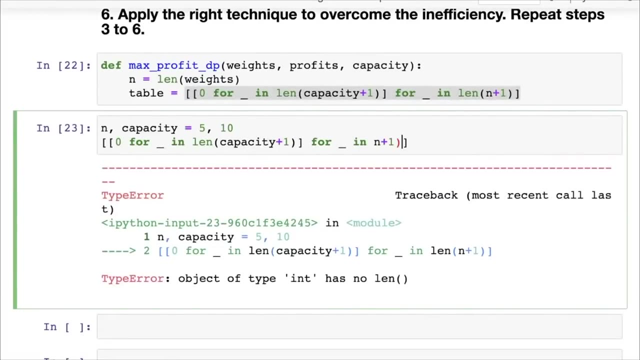 You can check what this capacity looks like. Let's say, N has N and capacity have the values here And in this case is five and capacity is 10.. We don't need a line here. We don't need a line here as well. 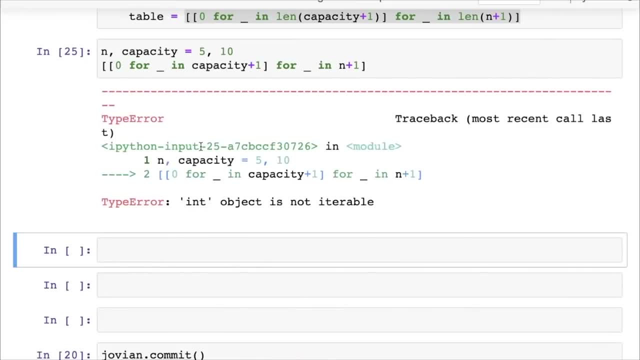 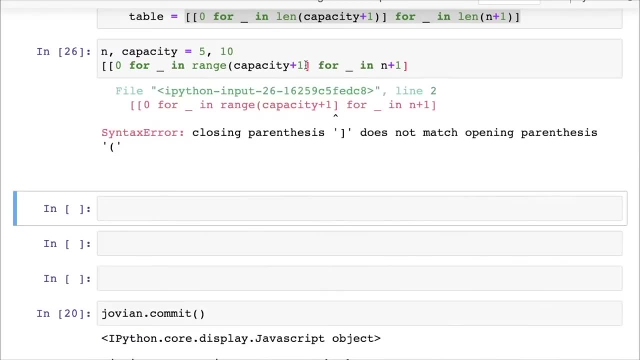 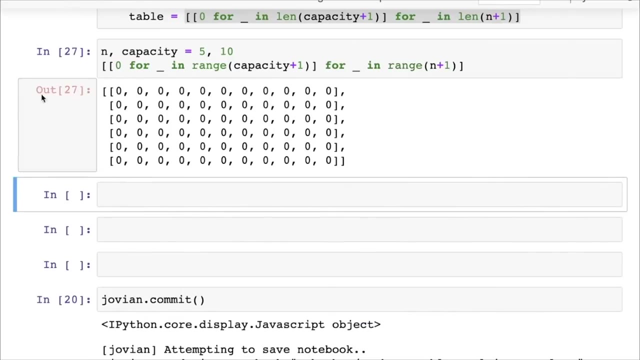 It's all perfectly natural to make these mistakes. Now, this should be range, not Len, but this should be a range and this should be arranged to. yeah, now you can see that we have created N rows, or N plus one rows. 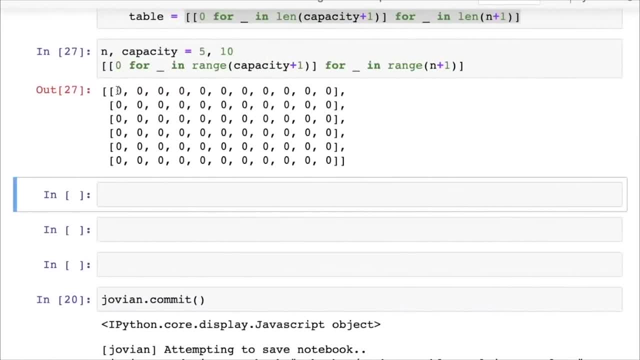 So one for each of these and then one more row above containing all, which will contain all zeros. This is in the case where we don't pick any of the elements and then we've created 11 columns. So this is for capacity zero. 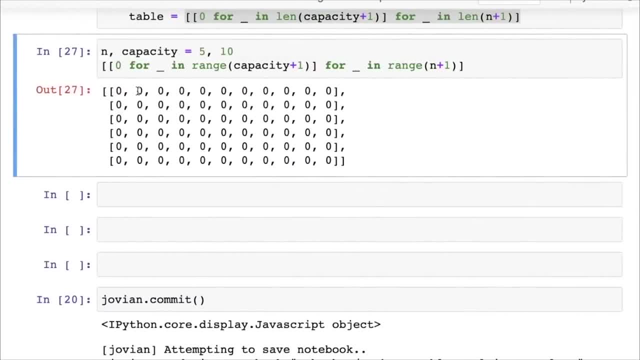 So, again, the first column will also contain All zeros, And this is something that you will often see in dynamic programming. You will have an additional row at the beginning or at the end containing all zeros, And that is simply to make your calculations or computations easier, but what that will lead to is off by one error. 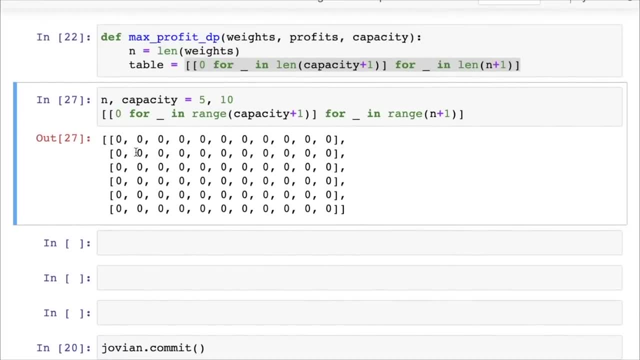 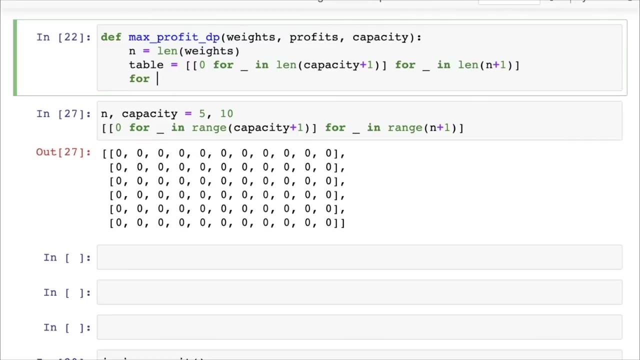 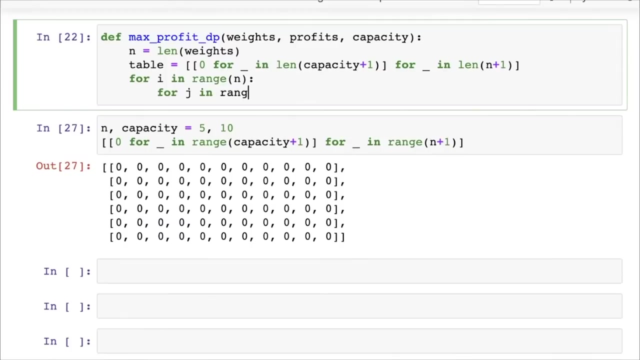 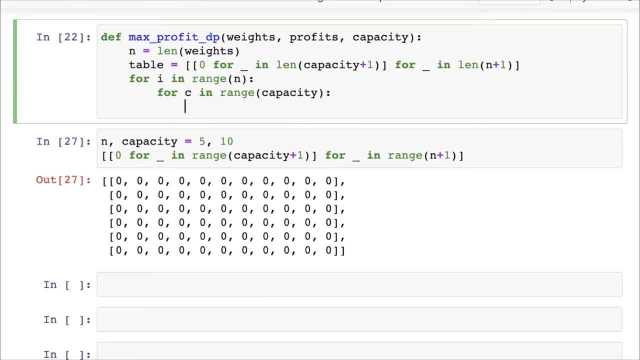 So you need to be very careful while doing this. And now we'll fill out this value using either this value or by subtracting the weight of the element that's here and getting a value from the previous row. So now we start iterating. So when now we say for I in range N and for J in range C, let's just say for C in range capacity. it should be capacity. table of I comma C. 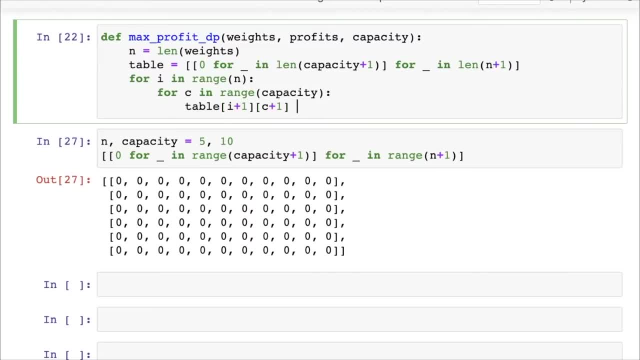 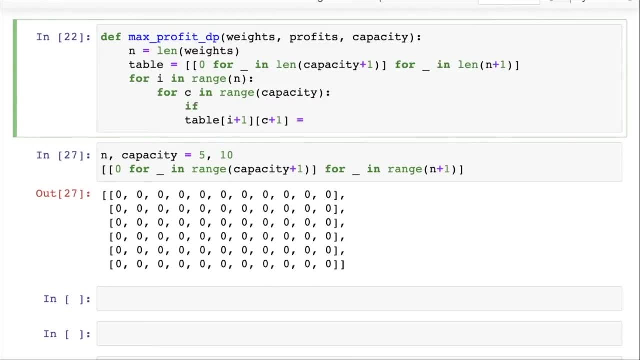 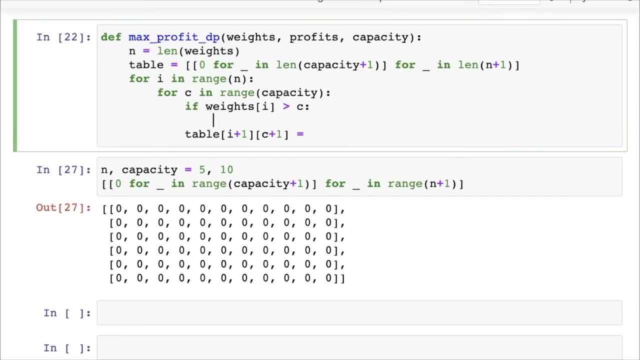 And it's actually going to be I plus one and C plus one because we have these additional Rosen Columns able to fight I plus one comma. C plus one is there are two cases here. If weights of I is greater than C- the current capacity- then we can simply look at the previous row. 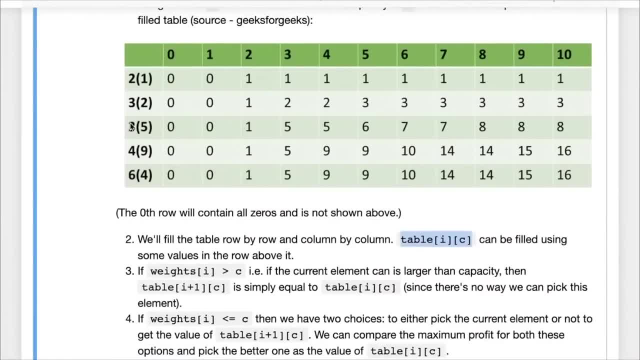 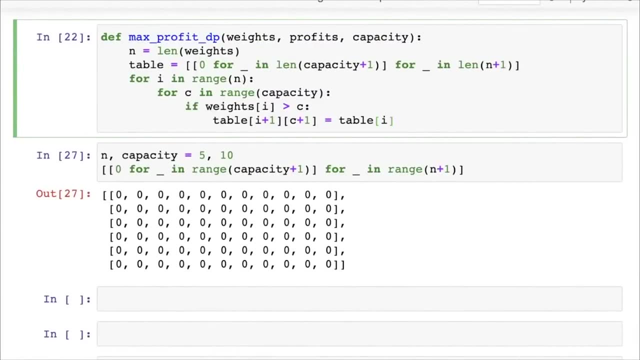 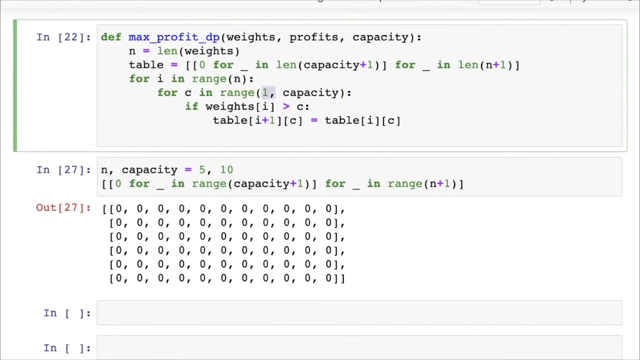 So, which is this case? let's say, the weight three is greater than the current capacity too. So then we simply copy over The value from the previous row, the same column. So we just say table of I, comma C plus one. We see, so our capacity should go from the value of one, because we don't want to affect the first column. 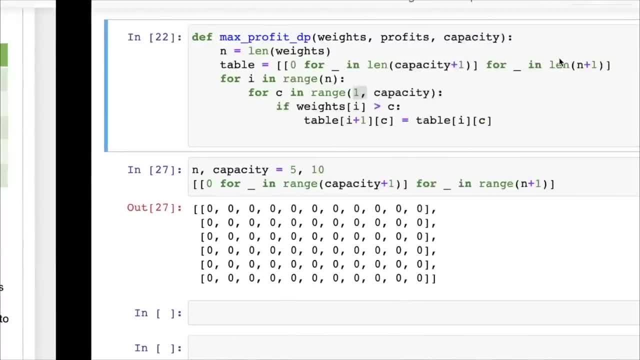 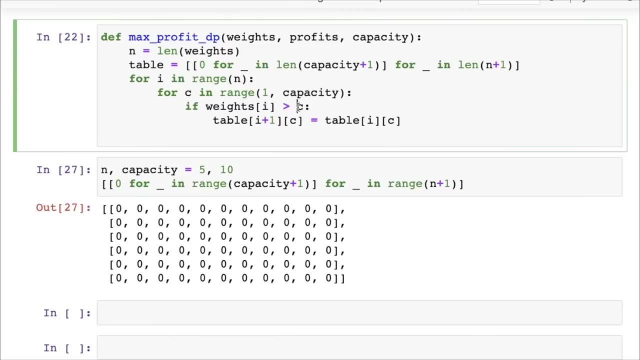 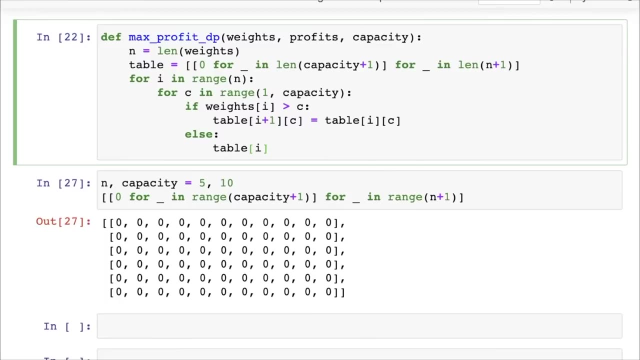 So the capacity goes from the value of one to a value of 10.. So capacity C goes from the range of one to capacity. And if the weights I is greater than the capacity, then we cannot fill the table on the other. On the other hand, if it is, if it fits within the capacity, then we have two options. 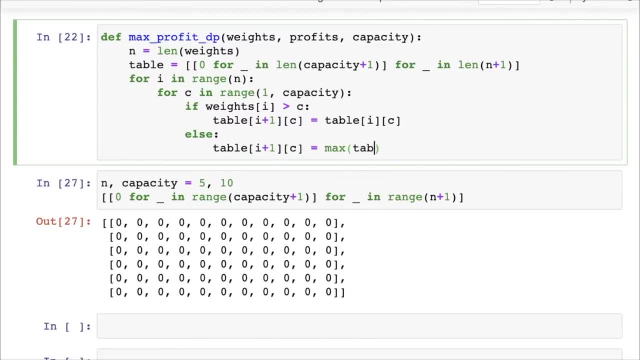 The table of I plus one, comma C has two options. So one is we don't use the current element. We don't use the current element, and that gives us table IC Once again. the other option is we use the current element, So we get profit from the current element. 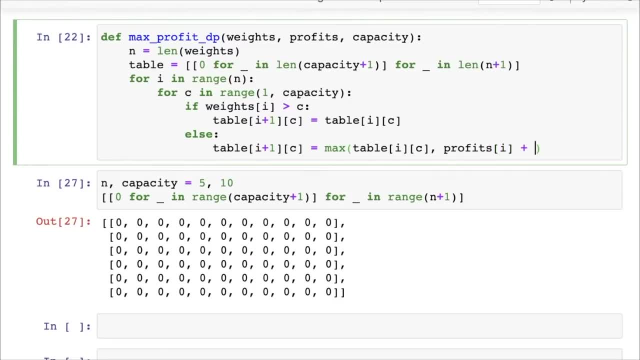 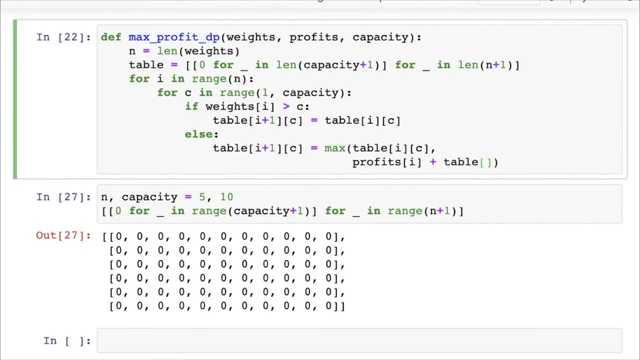 So profits I, but we do not get profits, but that reduces the capacity. So we then have to pick table of I. but now we have to pick C minus weight, weights of I, okay, And that should fill out the entire table pretty much. 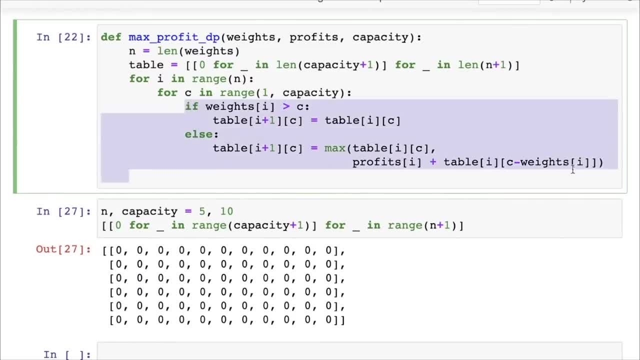 And that's a nice thing about dynamic programming: You simply just have to write this one solution or this one recurrence and be careful about it, And everything else is taken care of by this loop here Now we simply return table of minus one And minus one, and let's see if that works. 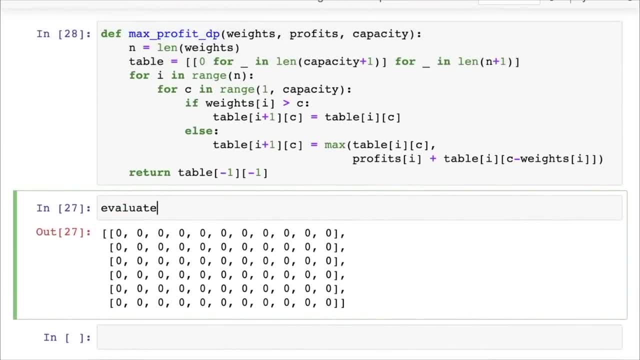 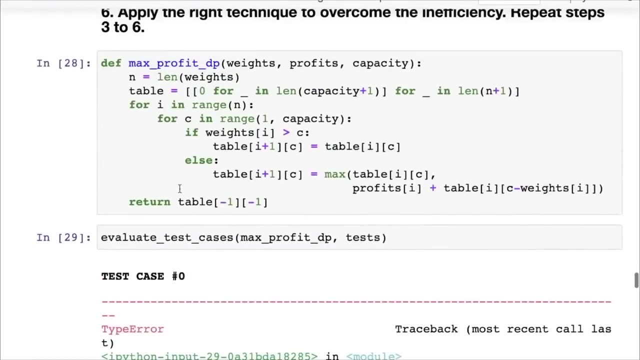 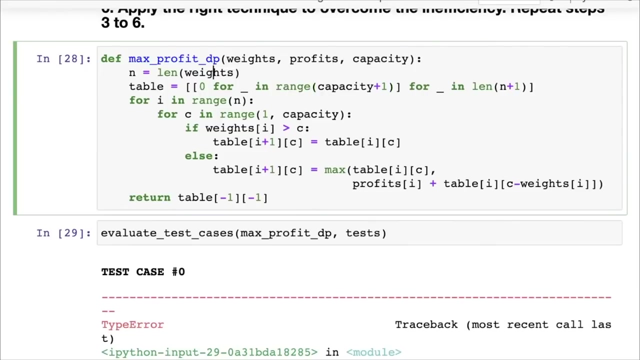 It's likely that there are some issues here. but let's see, we have test cases, max profit, DP with the tests that we have create. So we are seeing an issue already. I see here that this should be range and this should be range. 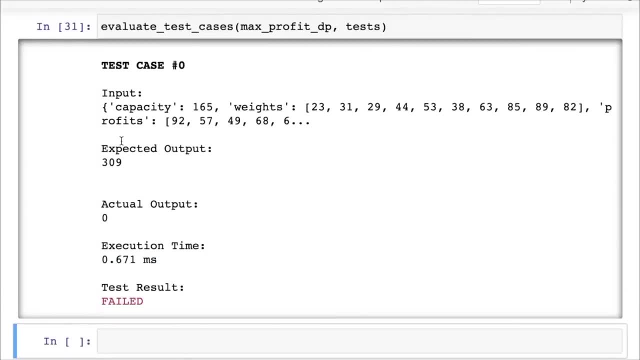 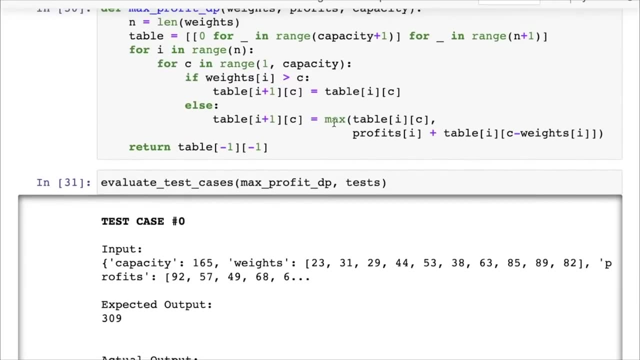 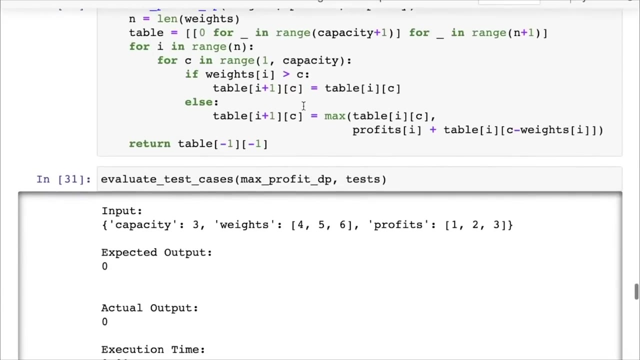 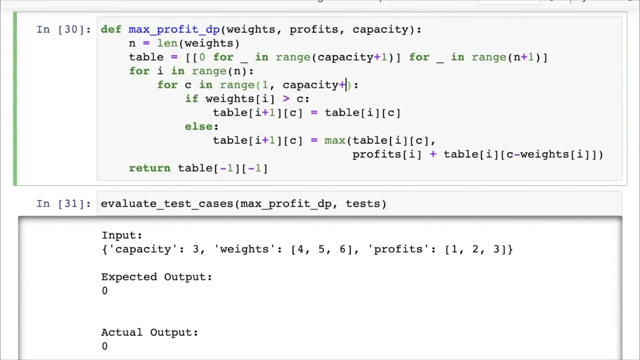 Is that enough? Yes, But how can we fix it, man? Yeah, okay. One thing that we haven't done here is: Well, it seems like our solution is always zero. Okay, This should be capacity Plus one, up to the maximum capacity, and the range does not end. 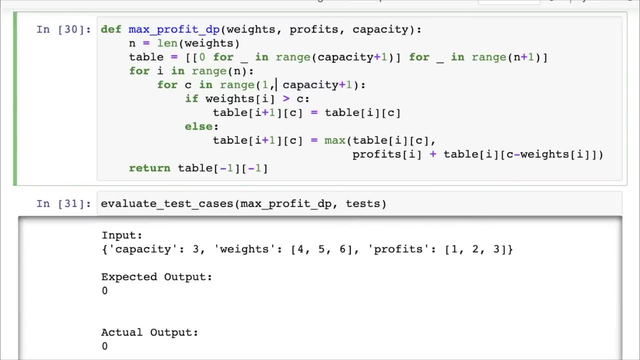 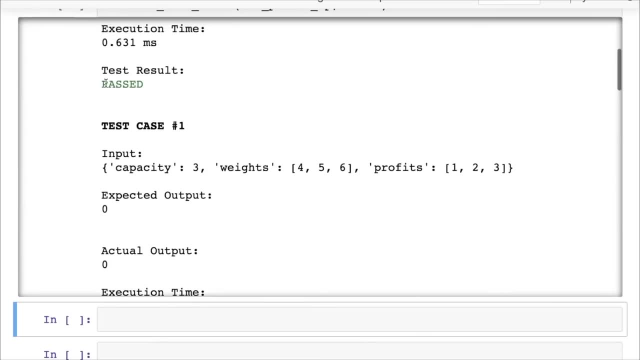 Uh, so the range does not include the end value, So you need to put capacity plus one here. Okay, Now, with that out of the way, you see, once again, these off by one errors are always going to bug you with dynamic programming. 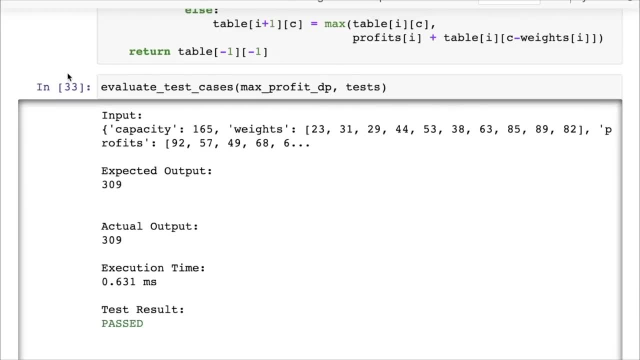 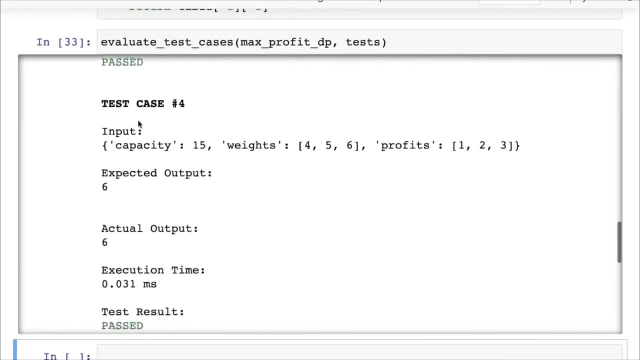 I've probably sold uh 50 or a hundred problems in dynamic programming, but I still make these errors, Um, but with that out of the way, you can see now that each of the test cases seems to pass. Now there may be other cases which you have not accounted for, but overall we've covered. 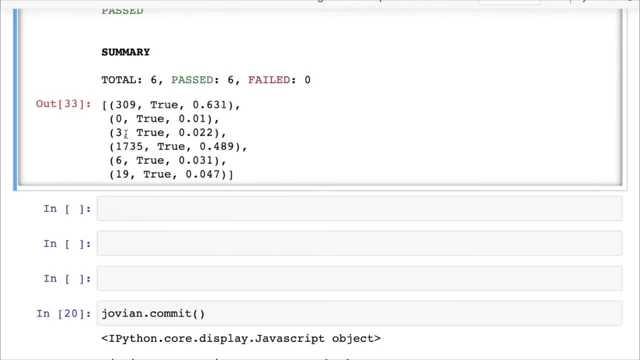 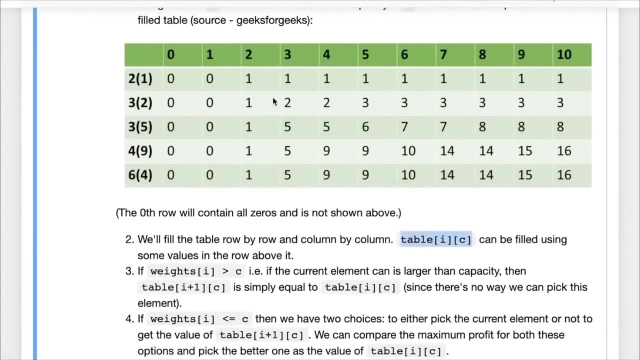 all the test cases here and we've ended up with now a dynamic programming solution, And I let you figure out the complexity here. but once again it's pretty straightforward, because we are filling up this table, and filling up this table simply requires this constant amount of work, which is a comparison. 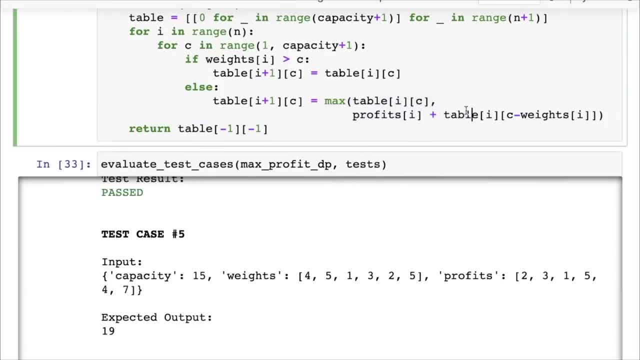 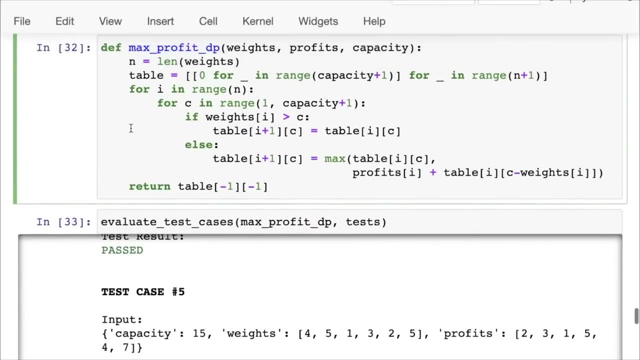 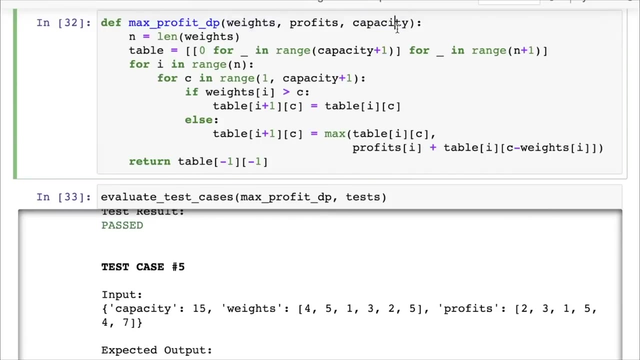 And then potentially another comparison and an addition and a subtraction, so like four or five operations. So you have this end times and uh, you have this end times, get past uh, end times. capacity. So where N is the length of weights and capacity, or w is a total capacity, 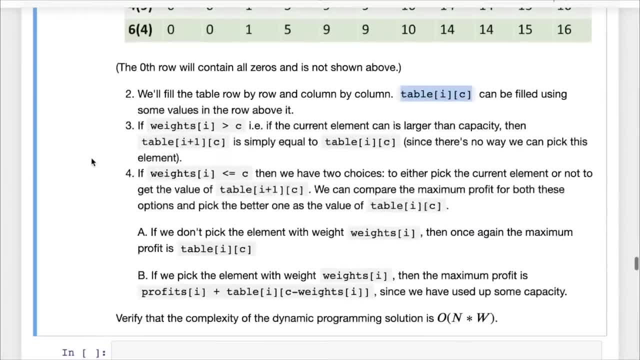 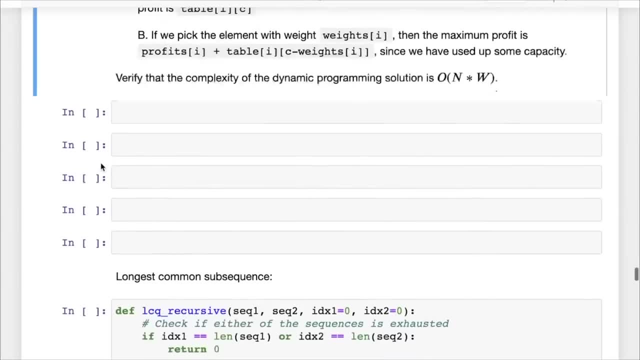 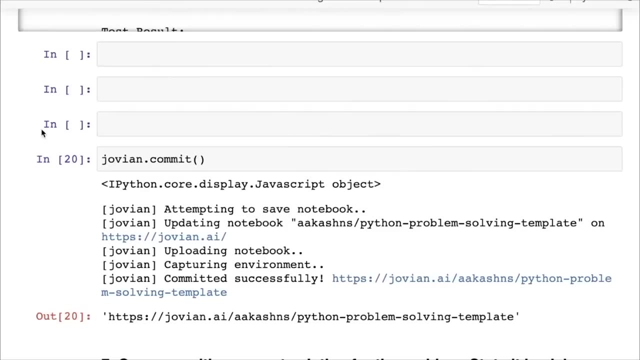 So N times w is the number of iterations, And that really also is the complexity, the time complexity, of the algorithm. So that's the knapsack problem, And now what you can do is try and figure out not just what is the maximum value, but also how to. 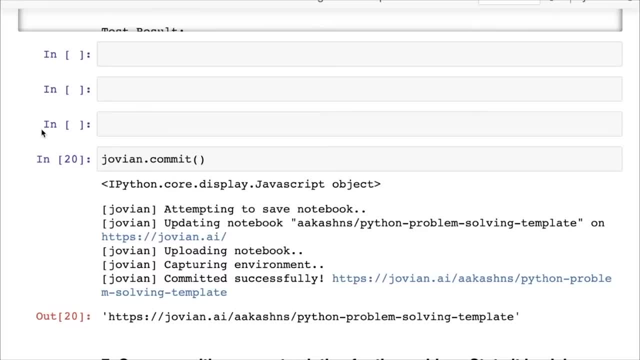 Okay, Figure out what are the actual elements that were chosen. Now. you can do this for the knapsack problem and you can do this for the longest subsequence problem. figure out the actual longest subsequence, and it should be possible to do that with just a small modification. now use the forum. 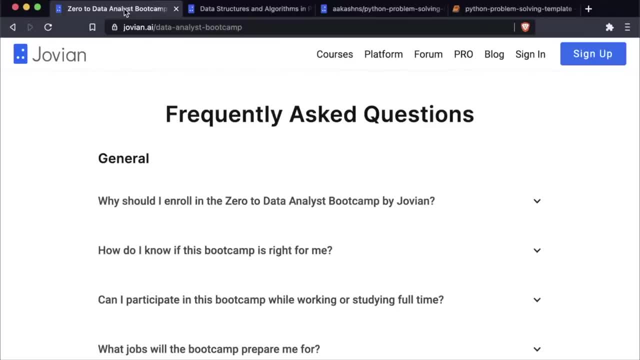 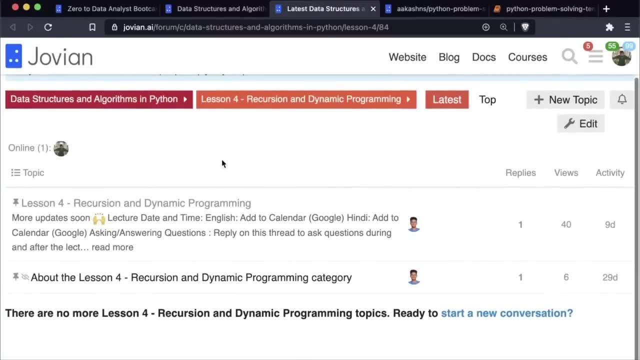 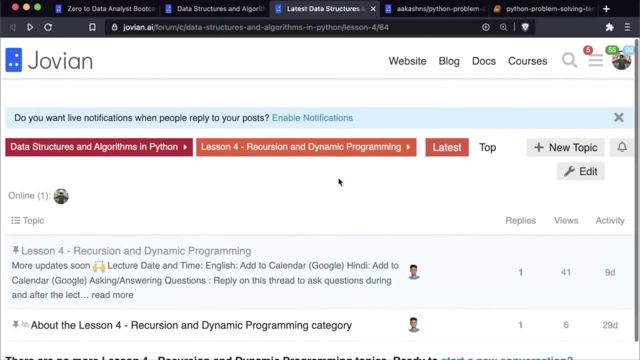 If you have any questions about the contents of this lecture, go back to the lesson page and open up the course community forum here. you can see here that, uh, this is the lesson four, The question and dynamic programming lesson. You can post your question here and you can also discuss ideas on how to figure out what the 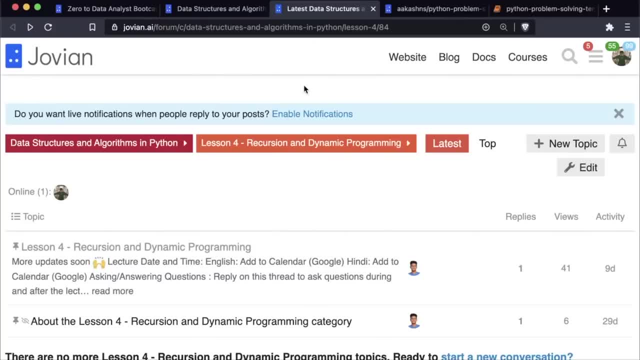 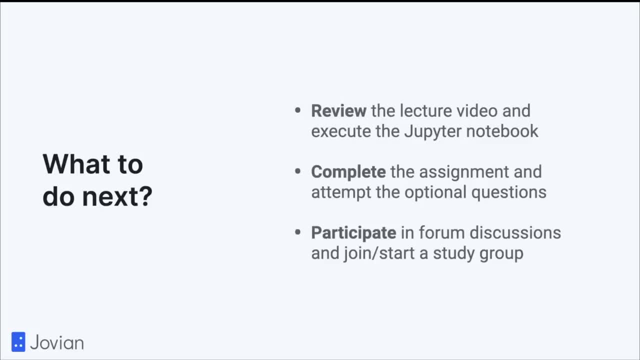 longest common subsequence is and what the best selection for the knapsack problem is. So what do you do next? Well, you can review the lecture video and execute the Jupiter notebook. The next step is also to complete the assignment. Now we have released assignments one and two. 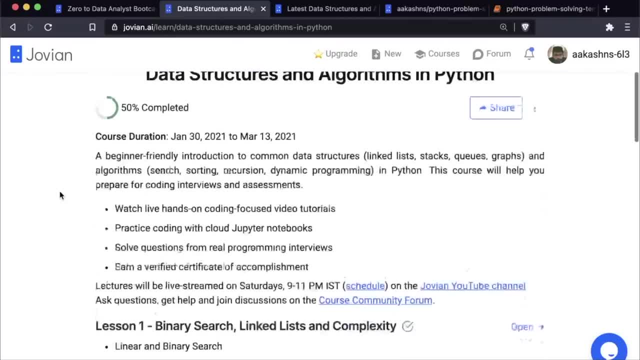 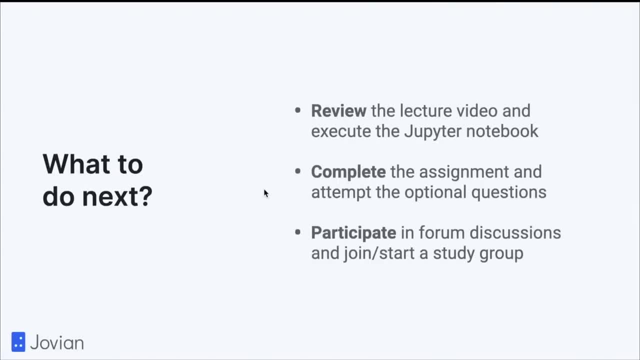 So far. if you go back on the lesson page, you will find lessons, or you will find assignments one and two and you can work on them- There is sufficient time- and also work on optional questions and do participate in forum discussions And, if possible, join or start a study group too, and that's a great way to stay motivated. 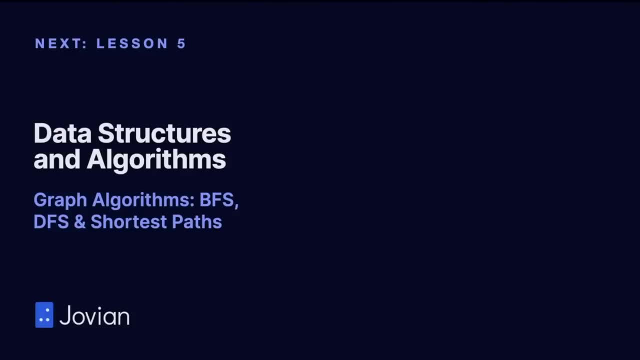 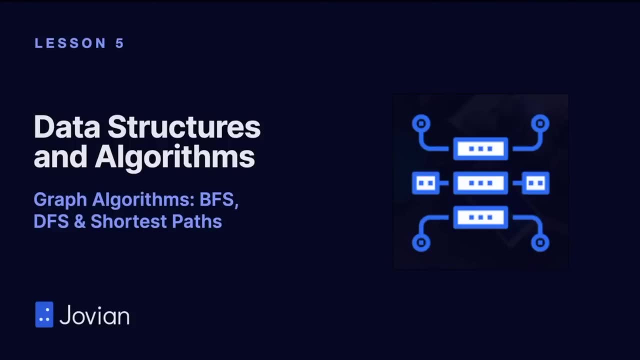 This was lesson four of data structures and algorithms in Python. Thanks And talk to you soon. Hello and welcome to data structures and algorithms in Python. This is an online certification course being conducted by Jovian. today We are on lesson five. 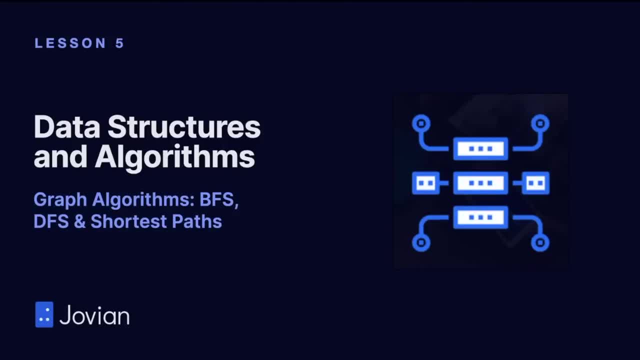 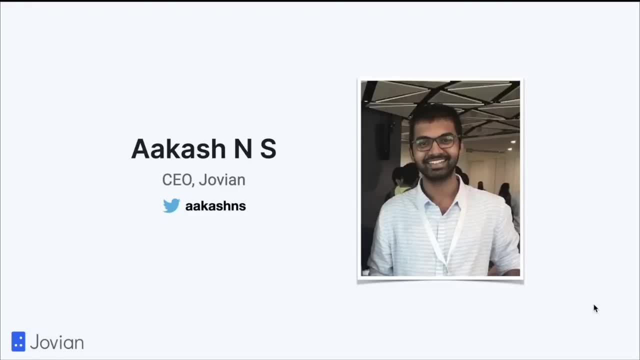 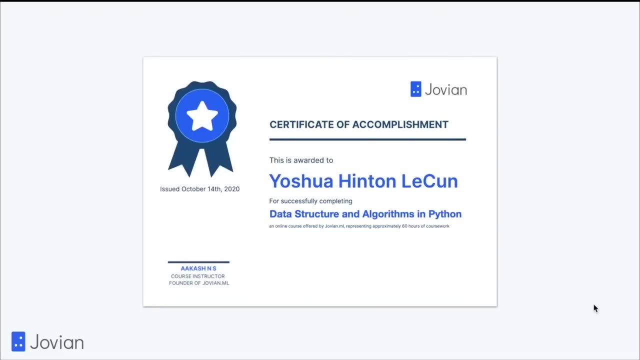 Graph algorithms like BFS, DFS and shortest paths. My name is Akash and I'm your instructor. You can find me on Twitter on at AkashNS. If you follow along with this course and complete all the assignments and build a course project, you can earn a verified 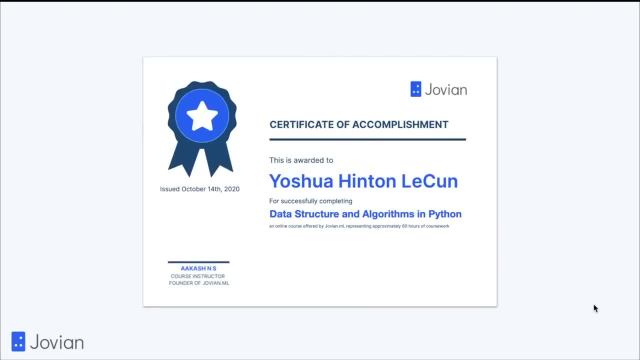 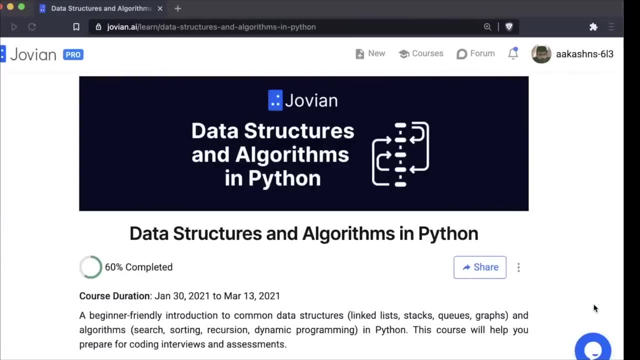 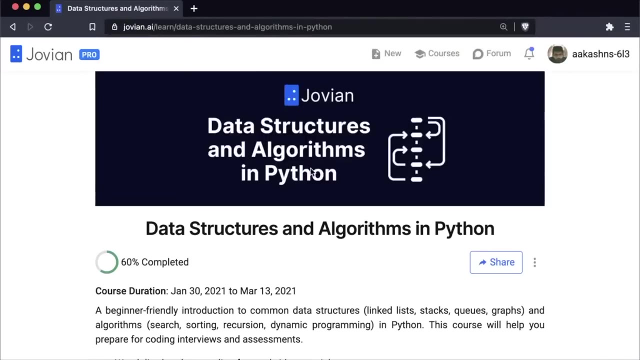 certificate of accomplishment for this course. So with that, let's get started. The first thing we'll do is go to the course website, pythondsacom. Now you can point your browser to pythondsacom to open up the course page and on the course page you can enroll for the course and you can view all the previous lessons and assignments. 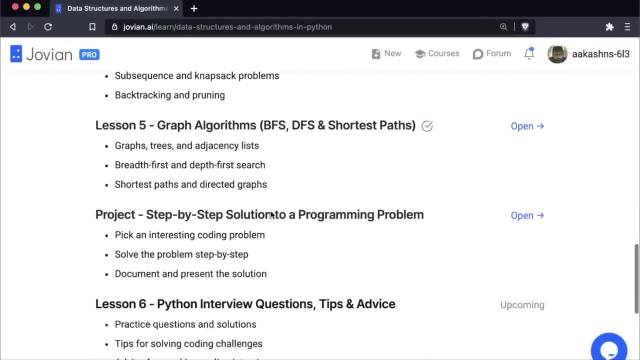 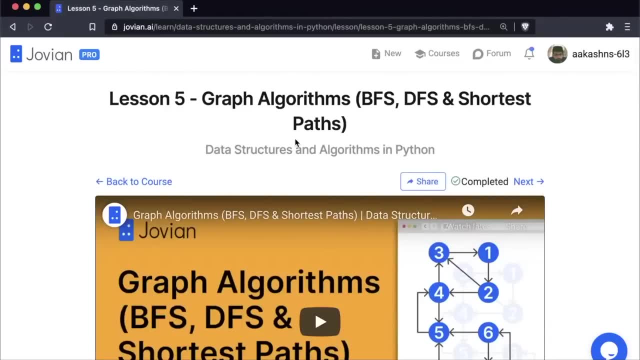 So do check it out and do check out the course project as well, But for now we'll open up lesson five: graph algorithms. Now, on this page, you can watch a video for the lesson later, the same video that you're watching right now. 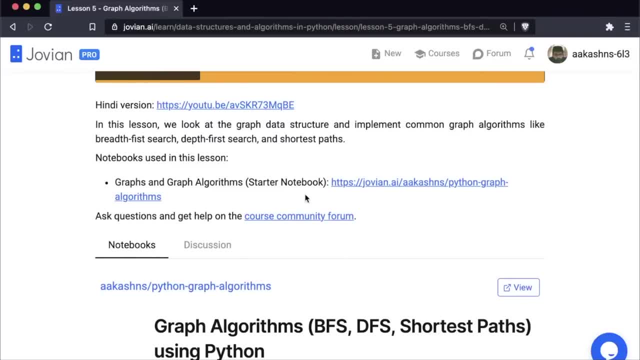 And you can also catch a Hindi version if you wish. And here is the code that we are going to use today, The first notebook under the heading notebooks. So let's open it up. and this is a Jupiter notebook hosted on Jovian. 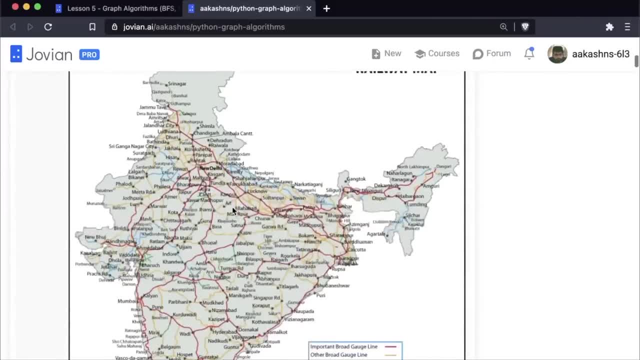 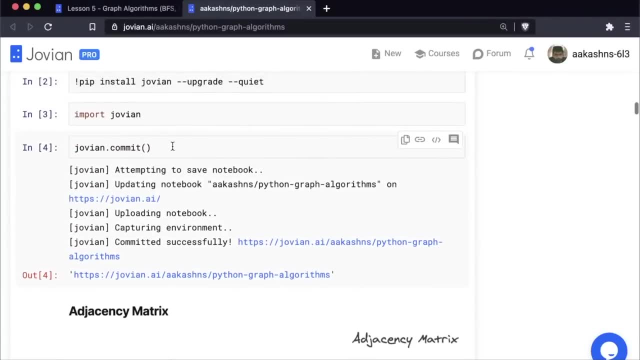 You should be familiar with it by now. but here you can see that there are some explanations and then there are some code cells where we can write some code. You can see that there's some code here. Now to actually Execute and edit this code, we will need to run this notebook. 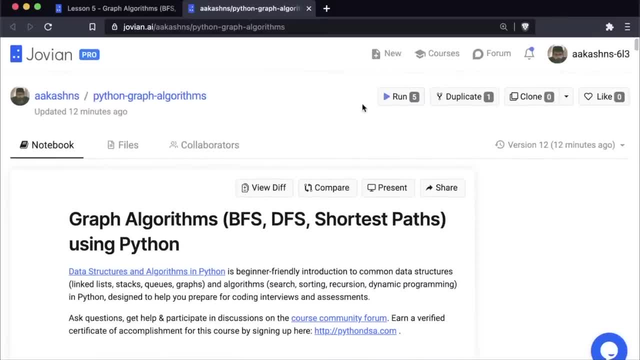 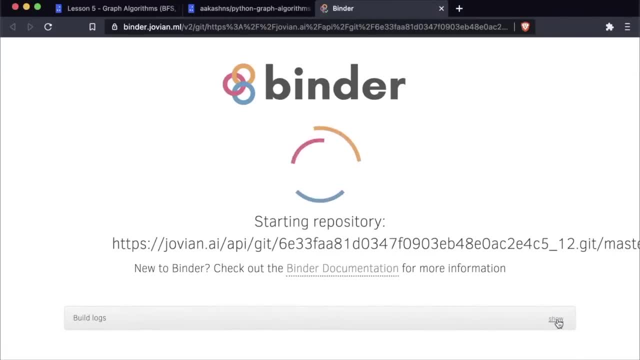 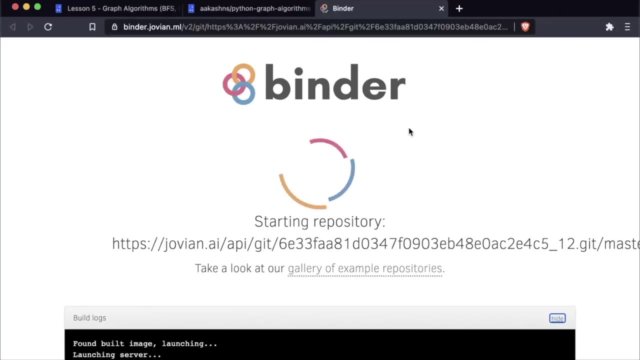 And you can find the instructions to run the notebook right here. but the simplest way to do it is to click run and select run on binder. Now this will take a second or two, but this will take your Jupiter notebook and create a new machine in the cloud and send your Jupiter notebook to that machine for execution. 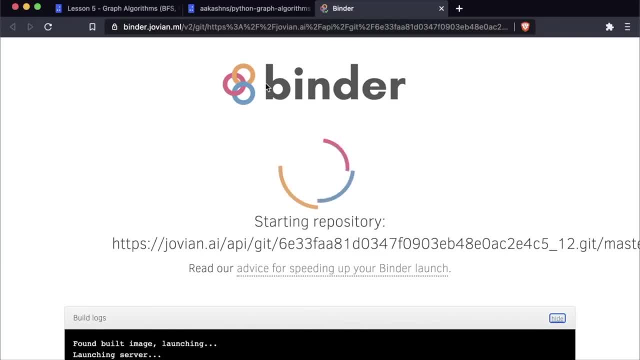 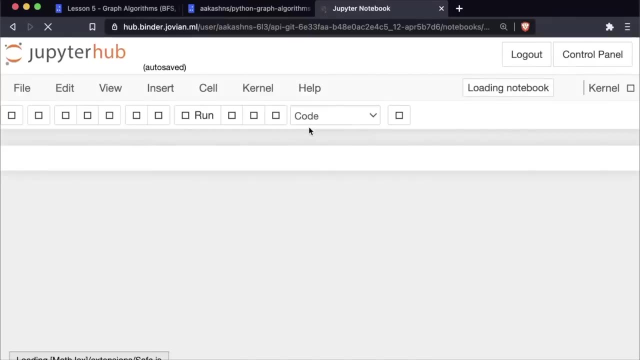 This is a free service That you can Access via Jovian. You can also run this notebook on your own computer directly if you wish. before that, you can check the run locally option here. Okay, So our Jupiter notebook server is now ready. 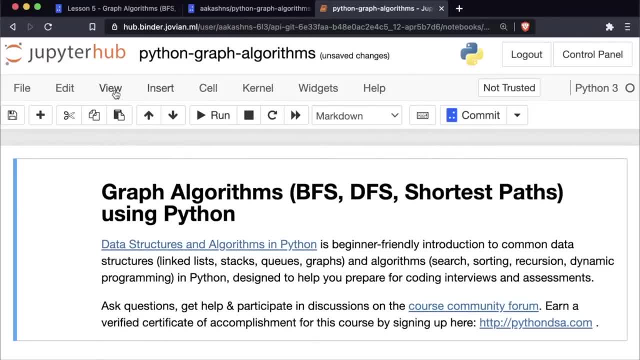 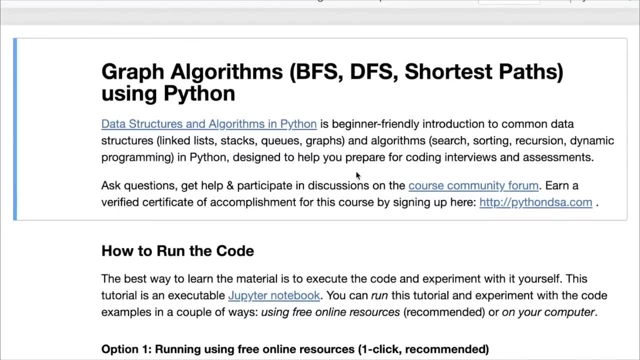 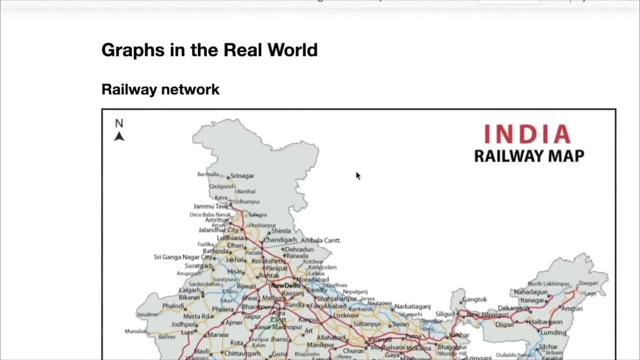 So we can now start editing and writing some code. Let's just go full screen here, Okay. So the topic today is graph algorithms: BFS, DFS And shortest parts using Python. Now, before we talk about graph algorithms, let's just try to understand intuitively what graphs are. 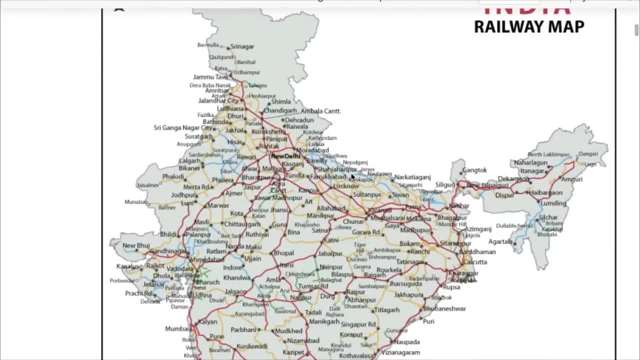 Now here's an example of a graph in the real world. So this is the railway map of India. You can see here all the train stations that you have in India. they're represented using these black dots points. They're also labeled. 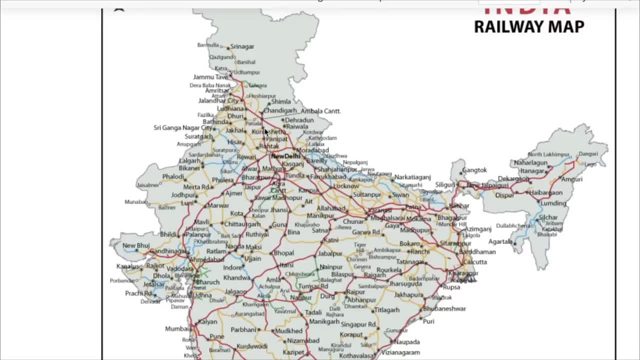 So each train station points to a city or a village, So all these are also labeled, And then you can see connections between these stations. So these are, as you might guess, railway lines, and you see that there are three or four colors involved. 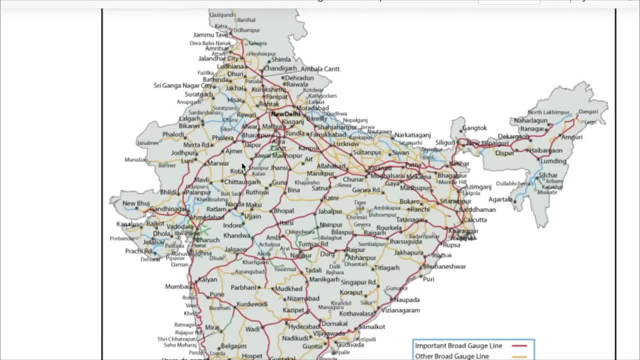 So these colors could represent different types of railway lines, like different gauge, meter gauge, broad gauge, et cetera, or these could represent different zones. So there's some information contained in the connections as well. Now, another important thing is that each railway line between two cities will also have 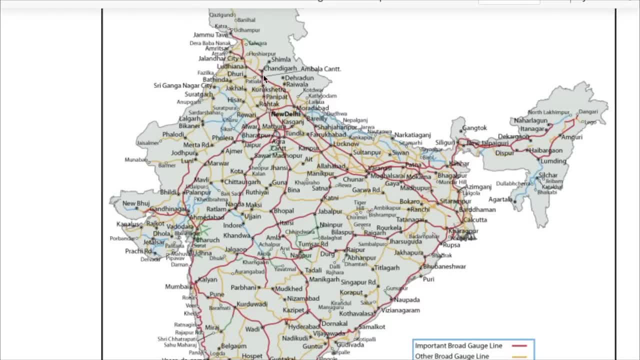 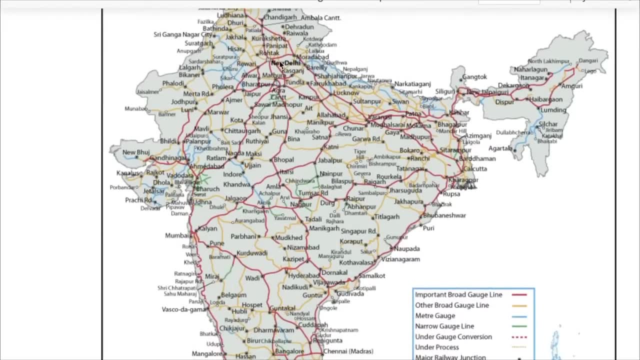 So that's what a graph is, roughly, and the kind of questions that you may want to ask here is, for example, is there a path from new Delhi to Hyderabad? So, given this information, first of all the question is: how do you even represent all this information? 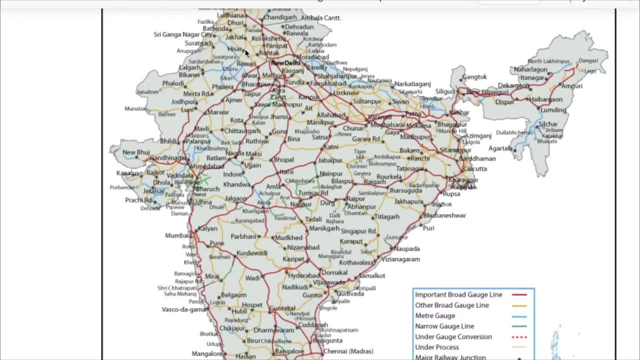 Because you have so many railway lines, connections between different cities, so many hundreds of cities. how do you even represent this so that you can start writing Algorithms to answer these questions, right? So if you're building a search, a train search website, then you would have to answer: given new Delhi and Hyderabad. 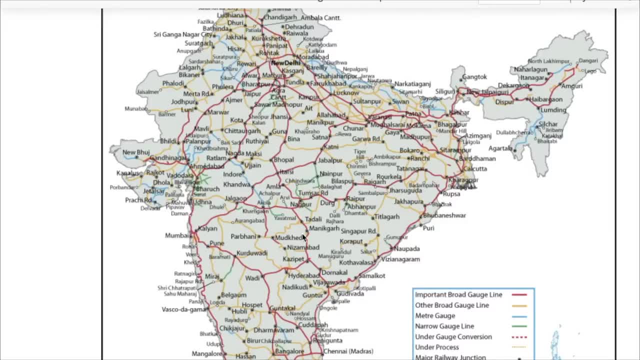 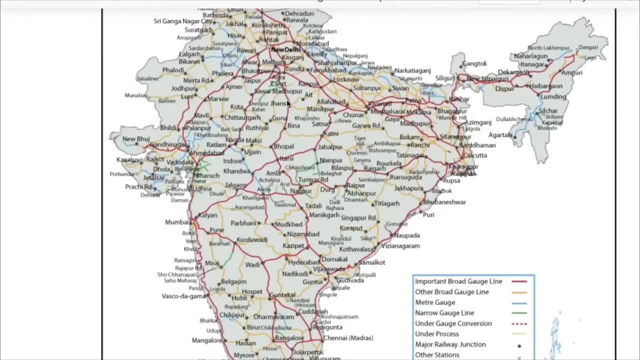 Is there? is there a way to get from new Delhi to Hyderabad? Okay, That's the first question that you might ask. Now, if there is a way, then the next question might be that what is the path with the shortest number of stops? 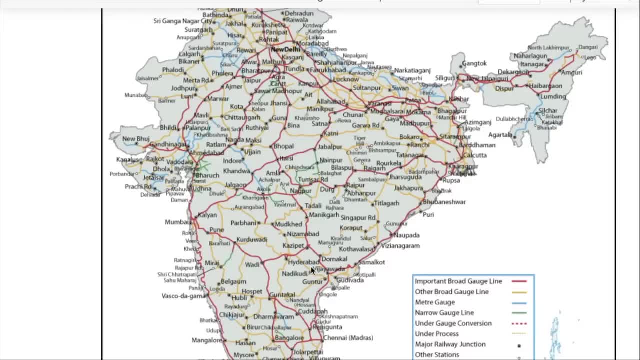 So do you go this way for the shortest number of stops, or do you go this way Or do you go this way? Another question could be: what is The path with the shortest distance right? So sometimes, if you measure the distance and if you measure the number of stations, the number of stops, they may be different along different parts. 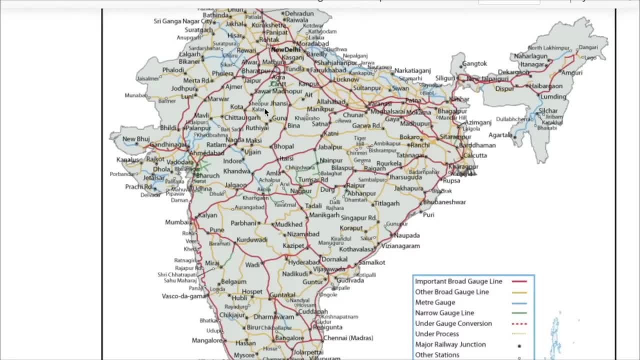 And one may be greater than the other in in in certain cases. So those are the kinds of questions that we want to ask and answer today. Oh, another question could be: what are all the stations reachable from new Delhi within one stop, or two stops, or three stops, or 10 stops? 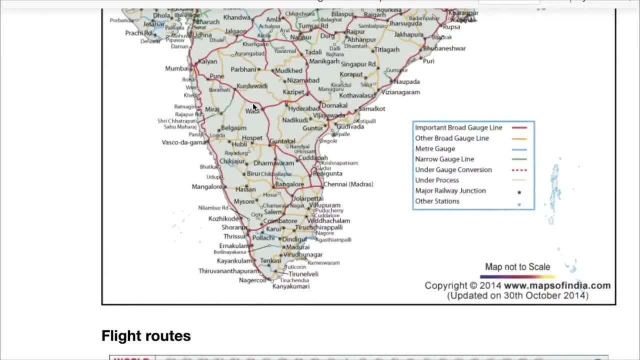 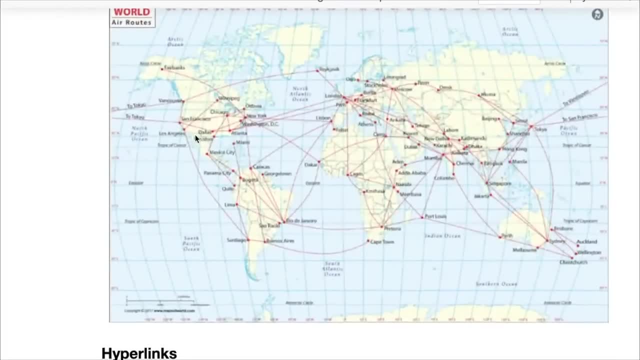 So those are the kinds of questions we'll try and answer, And for that we need a way to represent graphs in a more abstract fashion, because the same question can be asked in a different context. For instance, here we are looking at flight routes, international flight routes. 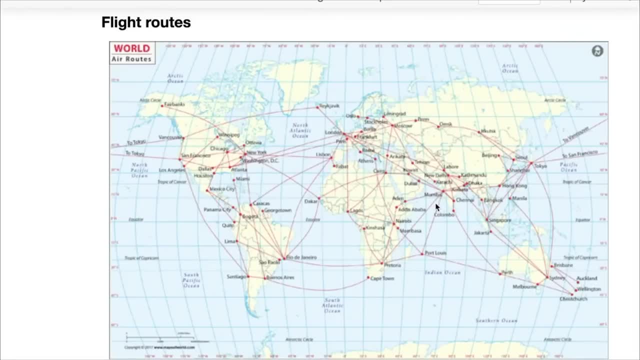 And once again, you can ask the exact same thing here: Is there a way to get from new Delhi to Vancouver? Now, if there is, then how many stops will that require? What is the minimum number of stops, How many stops we can take to get from new Delhi to Vancouver, or what is the minimum time it might take, maybe if you are okay with taking multiple stops, but you want to minimize the, the, the time taken or the distance traveled because you're concerned with the miles, for for some reason. another thing that you could ask is: what is the minimum cost, if there is a cost along each route? 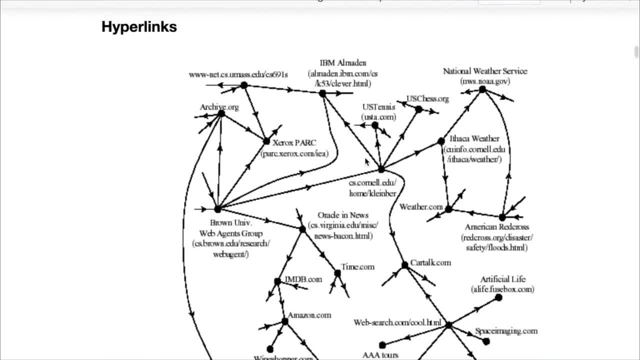 Okay, Now here's one more example from a very different domain. This is hyperlinks, The internet, essentially. So you can see here, here you have a whole bunch of websites and you have links on websites. Now, links on websites point to other websites. 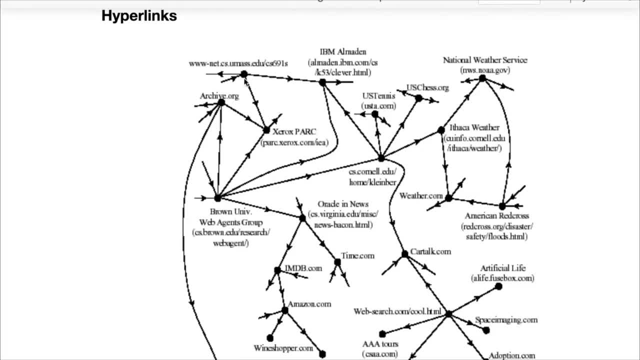 And in this case it is a one way connection. You can see that from this particular course website we have a link to IBM, but from IBM you may not have a link to this course website. Now, that's an interesting thing. 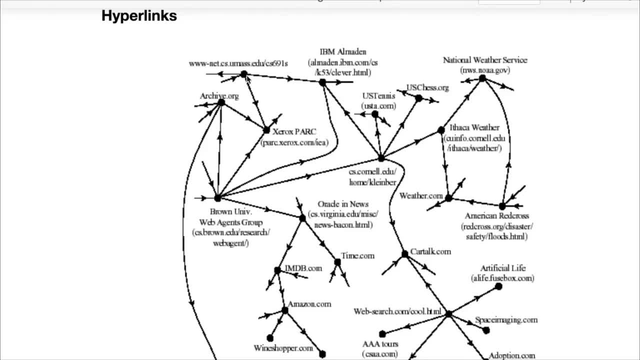 There's a slight variation here, and this is called a directed graph, because each connection here Is has a particular direction. Now this is again interesting to ask: is there a way to navigate from csumassedu to Ithaca weather? 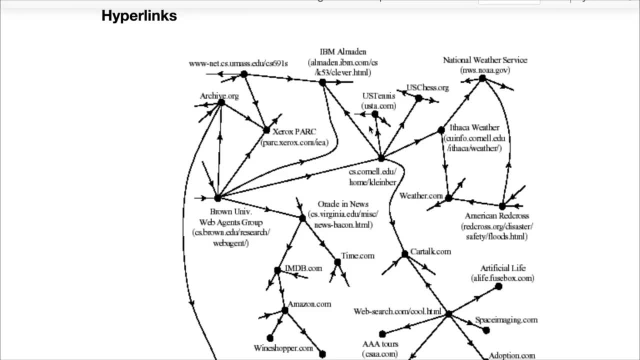 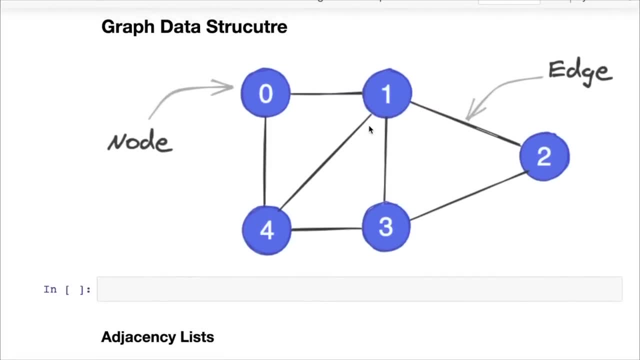 If there is, what is the shortest way, What do what does that path look like? So those are the kinds of questions that we want to answer today, And to do that we will need a more abstract representation of graphs, and we start with the simplest possible representation, where you have certain. 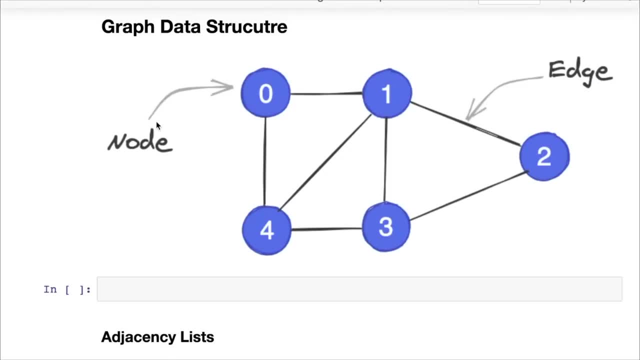 Points, or what we will call nodes or vertices, So these are two terms that are used for these points. So nodes or vertices, or graph has certain nodes or vertices, And, just to make things easy, these could be cities, or these could be web pages or these could be something else. but just to make things easy, what we'll do is we will number the nodes. 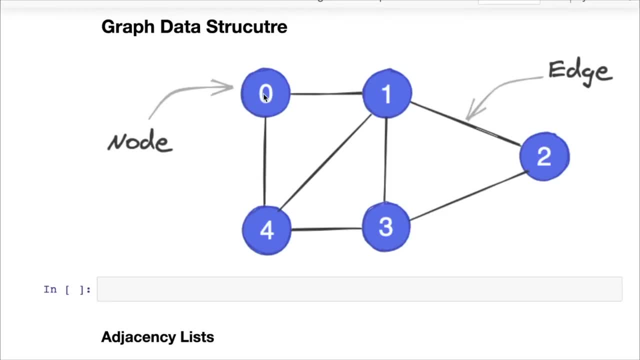 So in our graph, if we have 10 nodes, then we will number the nodes from zero to nine. Okay, This is, and they can be numbered. Okay, Well, completely arbitrarily, there's no reason to name, name, number the zero number. 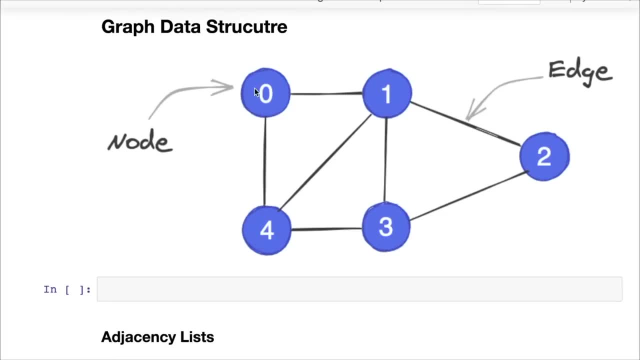 This one. what's more important is that we should use up all the all the numbers, from zero to N minus one, If we are dealing with N nodes. Now why do we do that? We'll see in a moment when we try to represent graphs using certain data structures like adjacency list, et cetera. 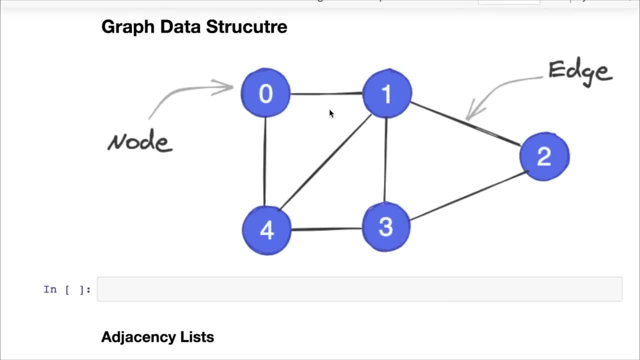 But we want to number our nodes from zero to N minus one, And this number is arbitrary. This one doesn't represent anything in the sense that one, It's just a number being greater than zero or so on. Okay, So these nodes have labels, and then you have edges between nodes. 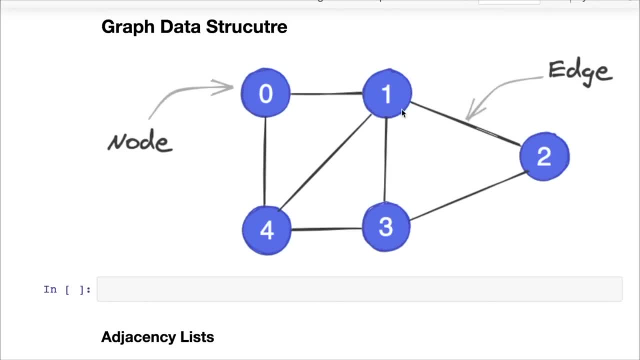 So an edge is simply a pair. An edge is simply something like one comma two. So a pair- one comma two tells you that there is an edge between the node one and node two. Okay, Now, as we move forward, we will also store some information within an edge and we will call that weight of an edge. 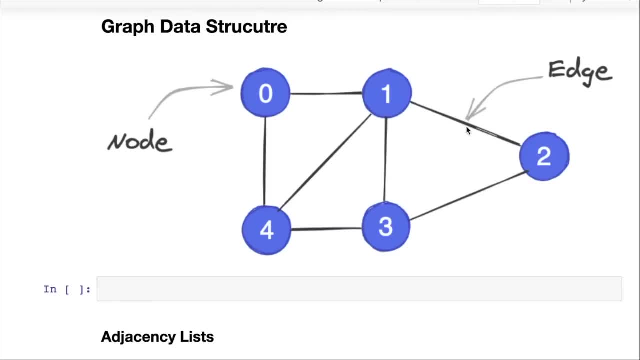 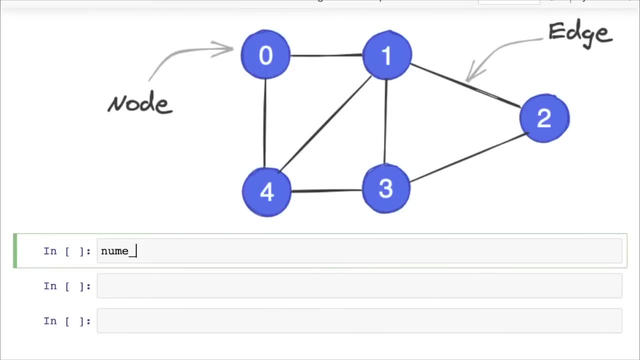 And we will also later look at Directed edges. So those will get us directed graphs. but let's start with this and let's see how we can now represent with this basic structure, how we can represent a graph. So we can represent a graph using two variables. 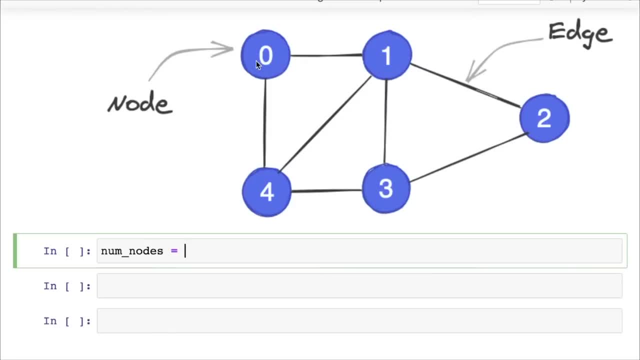 So one is called a number of nodes, and the number of nodes is, in this case, five, and then we can represent the edges using a list of pairs. Okay, So in this case, the pairs are zero comma one. In this case, the pairs are zero comma one. 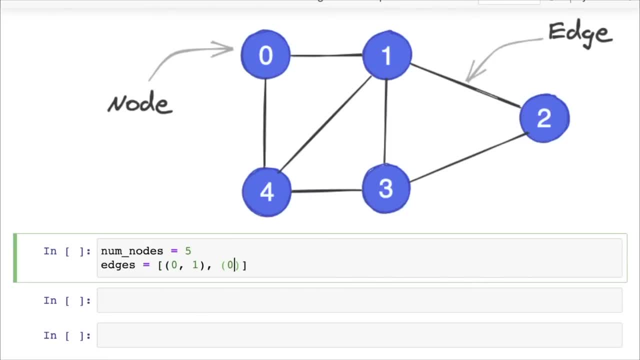 That's an edge. Then zero comma four, That's an edge too. Uh, then we have one comma two, So one is connected to two and the edge in this case is bi-directional. So when we are saying zero comma one, we're saying it automatically says that. 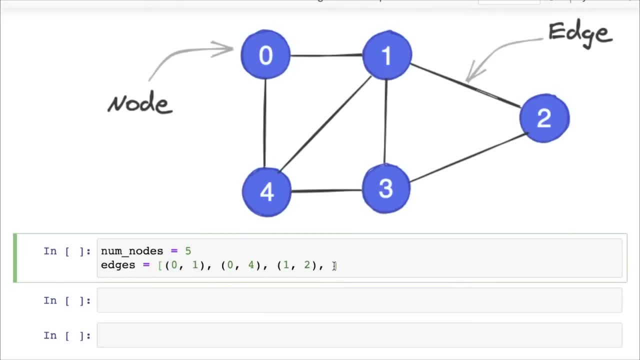 One and zero are also connected, right. So one comma two, and then we have two comma three. and which order we write these in doesn't matter. We could have just written three comma two here as well. Oh, we also have one comma three, and then we have one comma four. 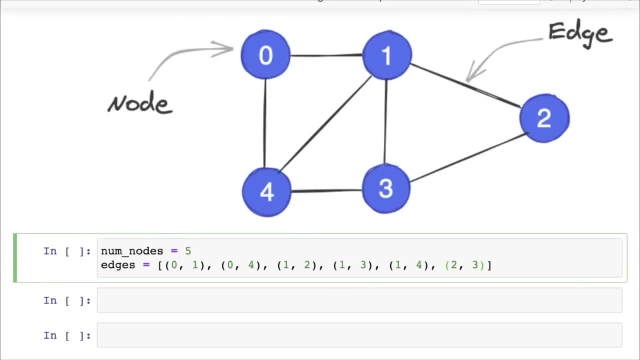 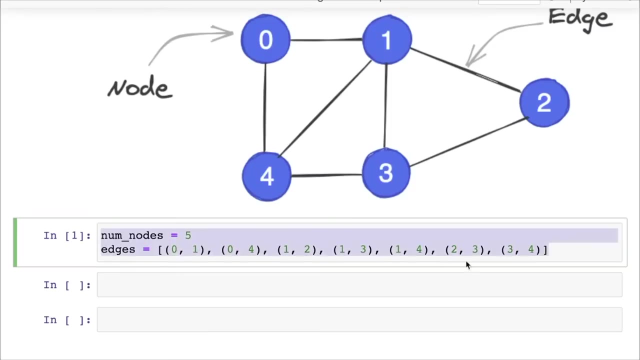 Great. And then, finally, we have three comma four. Okay, So this is how we represent This data structure, which, what we've drawn here is now represented in code using these two variables, And we can check here. If we simply print the number of nodes and the length of edges, we can verify if this is roughly correct. 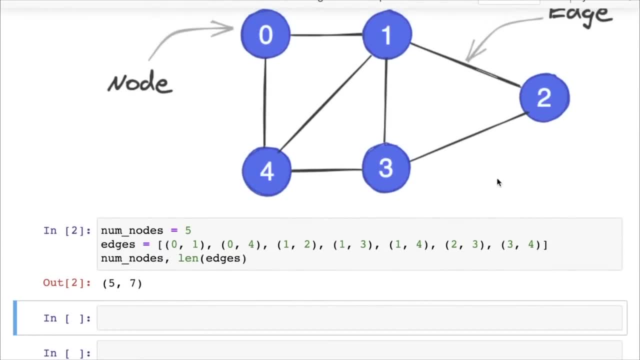 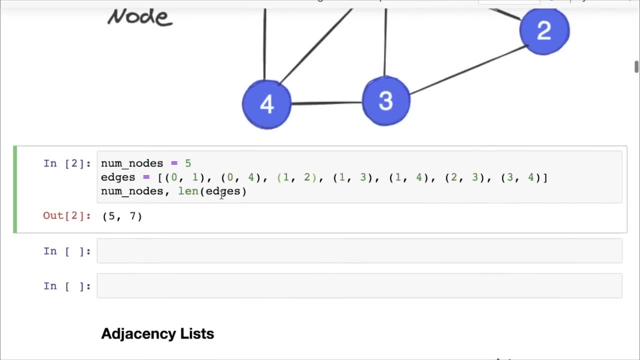 So you see we have five nodes and we have one, two, three, four, five, six, seven edges. Okay, Seems right to me We could. there may be a mistake here, but roughly we have set things up correctly. 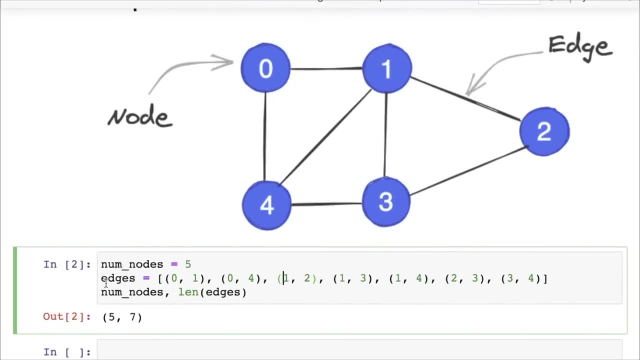 Okay, Okay. Now the question becomes is this question: is this representation good enough? Now, this representation is good enough. If you want to convey the structure of a graph to someone, I could give you these two variables and then, without showing you this image, and you could use this information to draw the graph on a piece of paper. 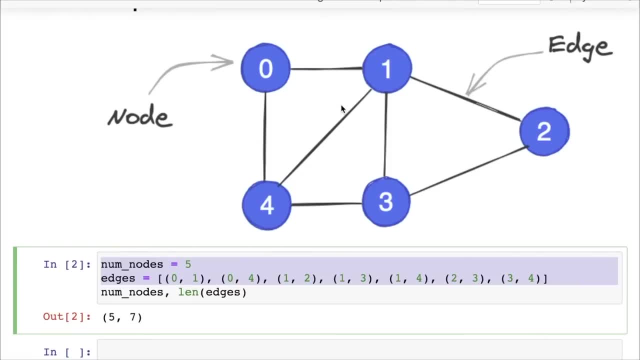 So this representation is complete. It provides all the information about the graph, but it may not be efficient. For example, if you want to find out which nodes the node one is connected to, we would have to Iterate over the entire list of edges. 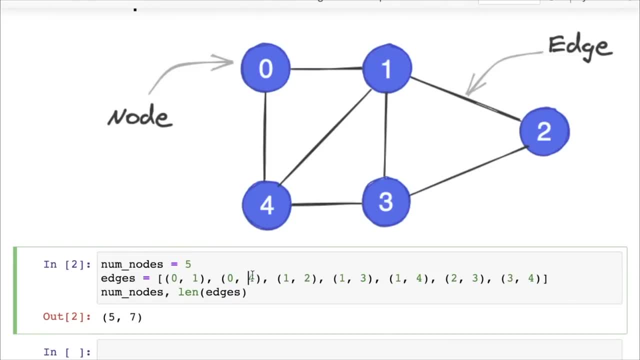 We would have to go through this one and then check if either of these is one, and check if either of these is one, and so on. So that makes it very tricky to access any information efficiently. Rather, it'll be much nicer to just look at a list of nodes that one is connected to in some way and go from there. 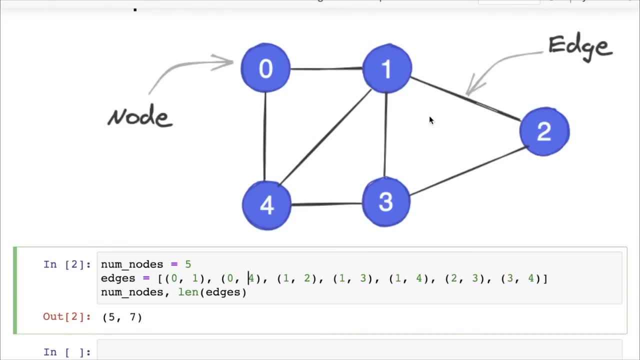 Now, if you want to find a shortest path, we would first have to find all the nodes that one is connected to, And then for each of those we would have to find their neighbors, And then for each of those you would find, I have to find their neighbors. 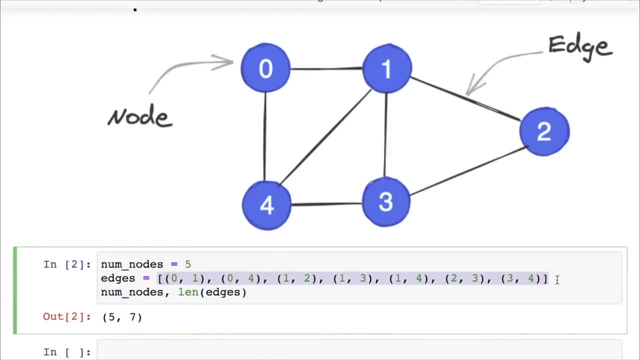 And so on. So it would get pretty tedious to go through the list so many times. So that's why- and by the way, by a neighbor we represent we mean two nodes that are connected by an edge. So zero and one are neighbors, but zero and two are not neighbors. 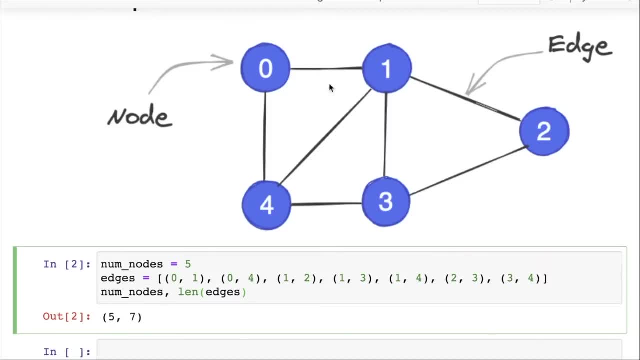 And so that's a very simple nomenclature that we can use, And what we can say is, if we track the path, we say 0, 1, 2, and then, if there is an edge between both of them, we say that 0, 1, 2 is appropriate. 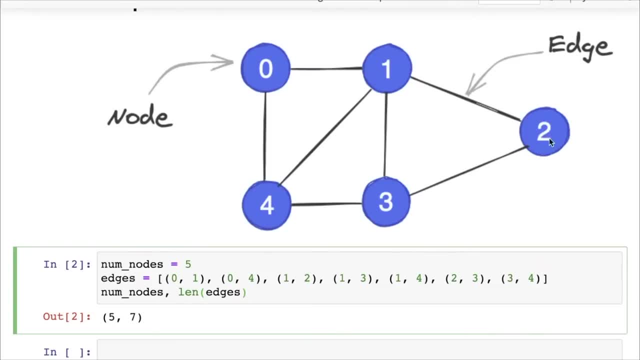 So 0, 1, 2, in this case, is a path, but 3, 0, 1 is not a path, because there is no path, but there's no edge between three and zero. Okay, And we'll see what what we mean by paths and neighbors and so on in some time. 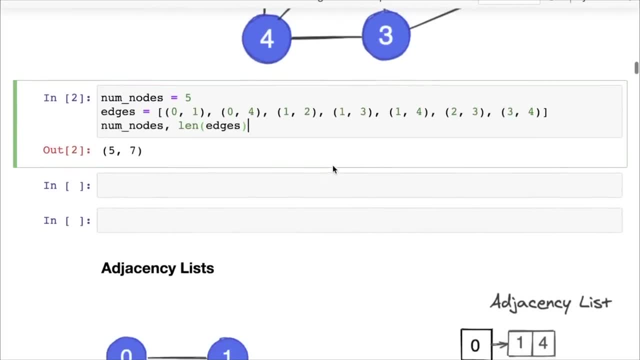 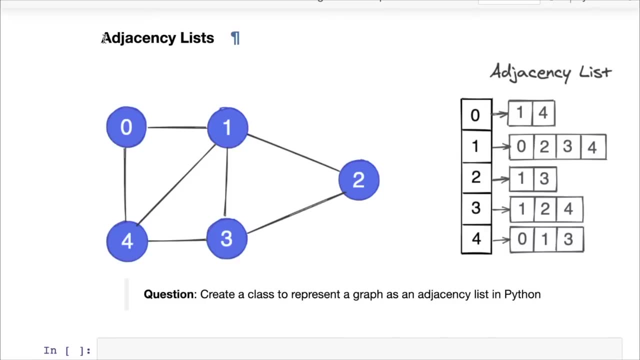 But to work with graphs more efficiently, we will represent them using what's called an adjacency list. Now the name it explains what it contains. So the adjacency list contains a list for each node and it contains a list of all the nodes that are adjacent to that node. 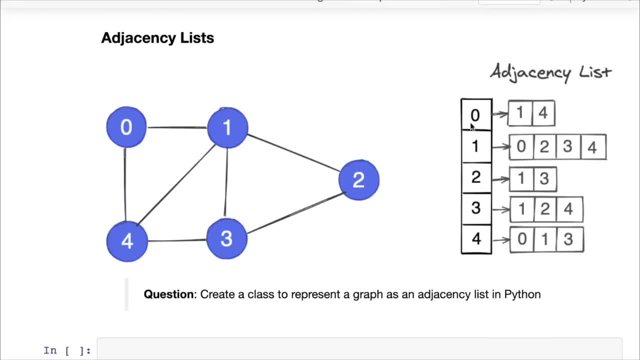 Now again, adjacency is the same as an adjacent the same as neighbor. So if for each node, so for example for the node zero, we maintain a list, and that list contains the numbers one and four indicating that zero is adjacent to, or zero is a neighbor of, or zero is connected via a direct edge to one and four, 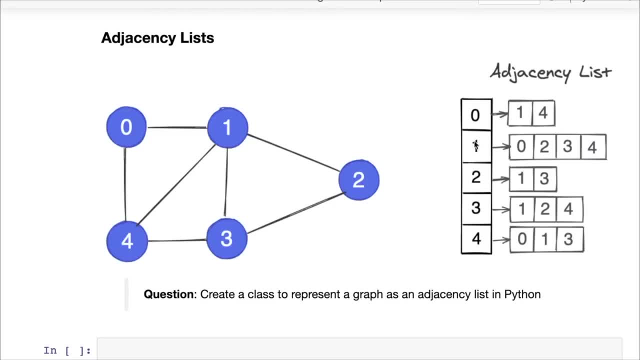 So that's why you have one And for here and then. one is connected to zero, two, three and four. You can see that one is connected to zero, two, three and four. Similarly, two is connected to one and three, three is connected to one. two, four and four is connected to zero. one, three. 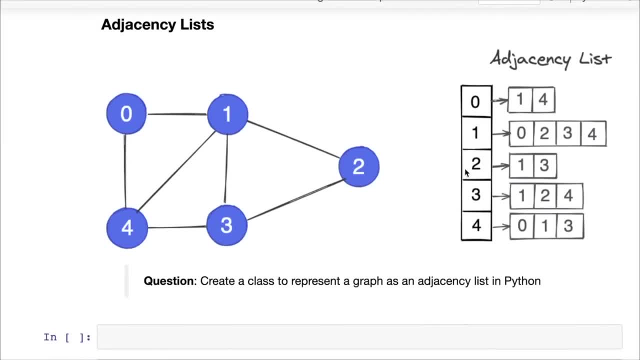 Now, this is more convenient, for sure. One, because, since this is- and this is a list, if you want to find, let's say, which nodes two is connected to, we can directly access the index. two within the list, And this is why we number the vertices, or the number of the nodes, from zero to N minus one, so that we can access them directly in an adjacency list, right? 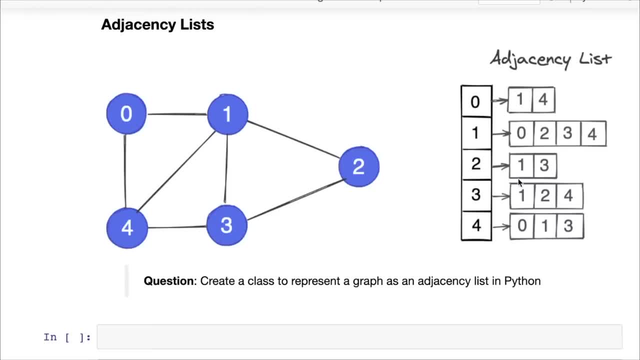 So we directly access the numbers stored next to two, And so we have one and three here. So that's what makes it convenient. And one important thing to notice here is that edges, each edge goes twice, So the edge zero one shows up in the list for zero. 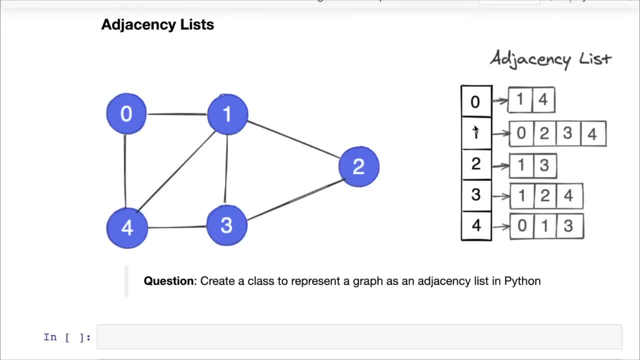 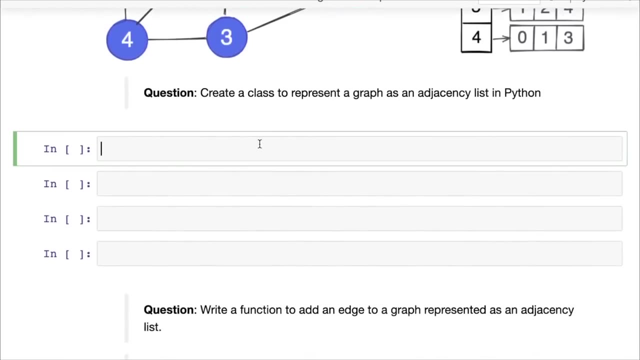 You can see here, in the list for zero we have one, And similarly in the List for one we have zero. So each edge shows up in two adjacency list of each of the nodes that it connects. Okay, So now the obvious next question might be to create a class to represent a graph as an adjacency list in Python. 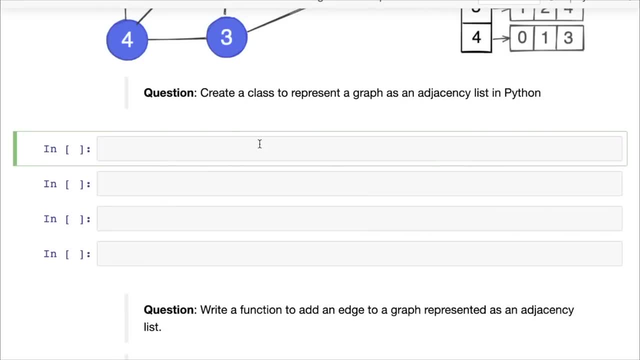 Okay, This is again a question that you might get asked a step or this might be part of another question that you may get asked, where you're asked to perform a breadth first search or depth first search or find the shortest path. Okay, 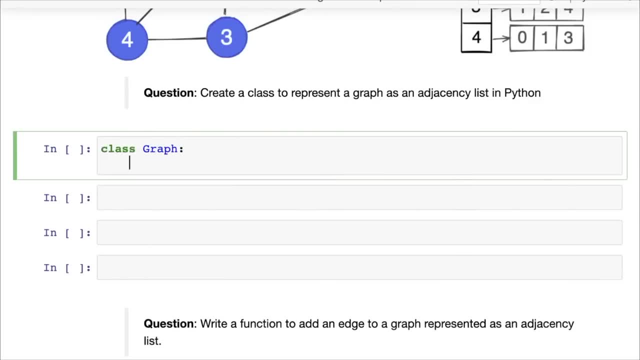 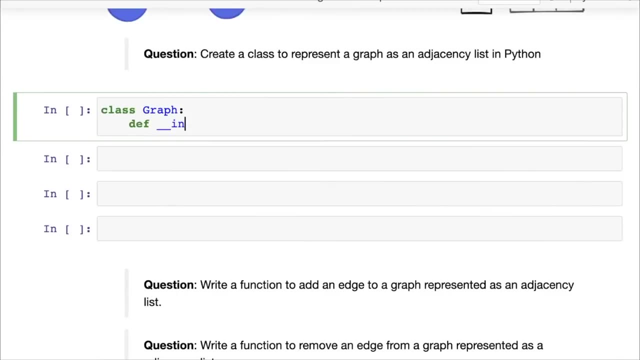 So the first step you will have to do is define a class for a graph to maintain the information about the graph as the adjacency list. Okay, So here we're creating a class graph, And the first thing we'll need inside the graph is a constructor function. 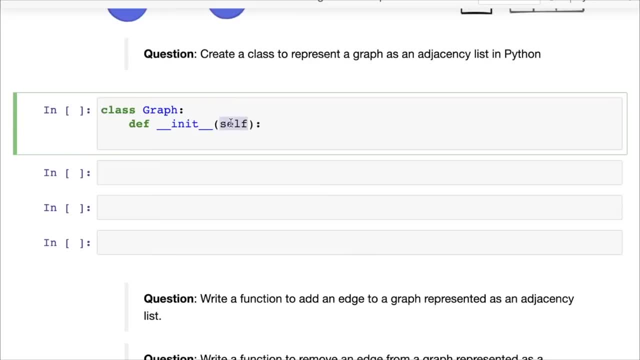 So we need to put something inside the constructor function, And we know that the first argument to any graph, any class, method and Python is self, which represents the object that will get created ultimately When we create an object of the class. but apart from this, what information? 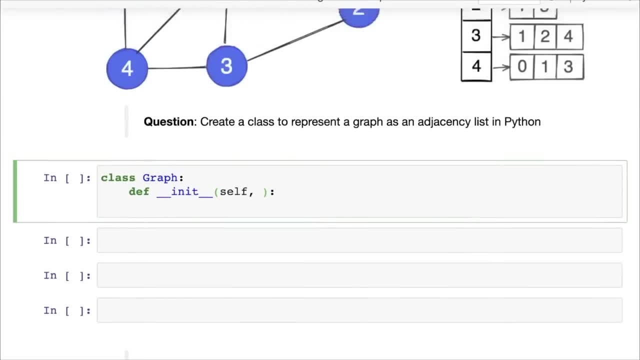 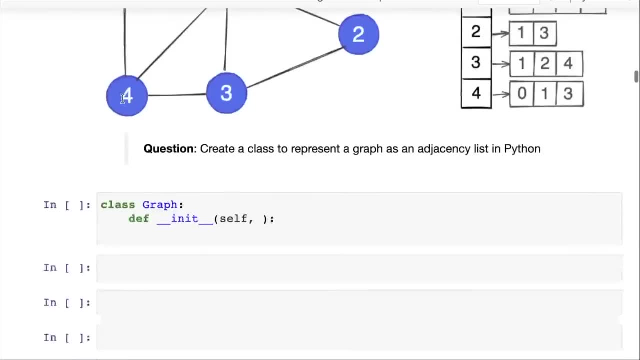 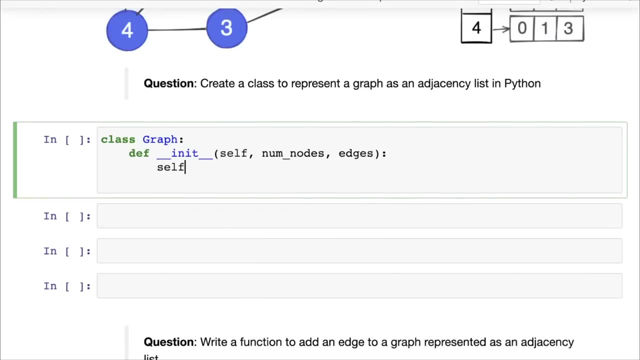 do you need to create a graph Now? it's pretty straightforward: We can simply work with this information, because these two variables together specify the graph completely. So let's simply accept numNodes and a list of edges as the information. The first thing we can do is simply store numNodes in selfnumNodes. 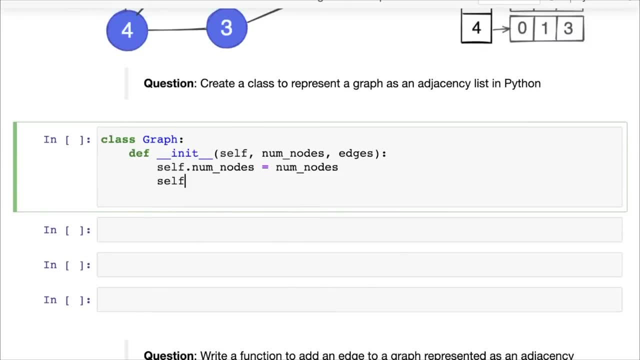 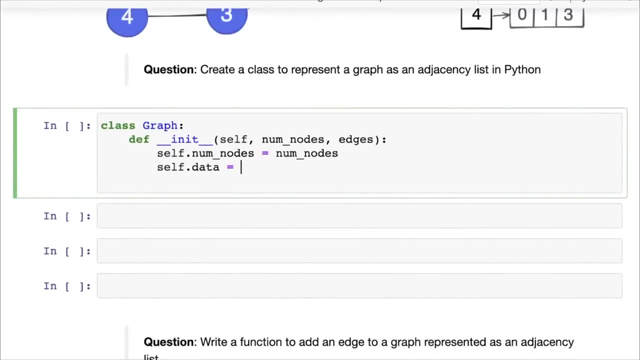 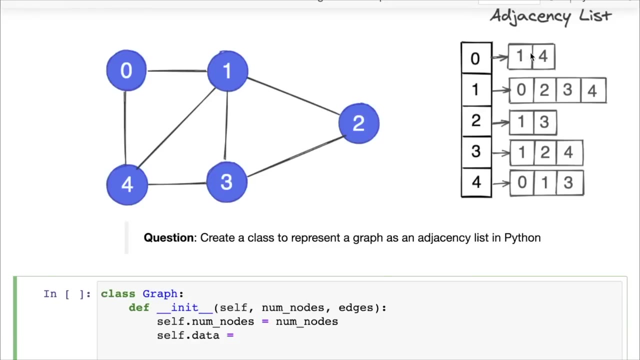 So that once we create a graph, we can access the number of nodes very easily. Then we need to create the adjacency list. So we need to create the adjacency list. We'll call it selfdata, And initially we will create a list containing empty lists, because- and then 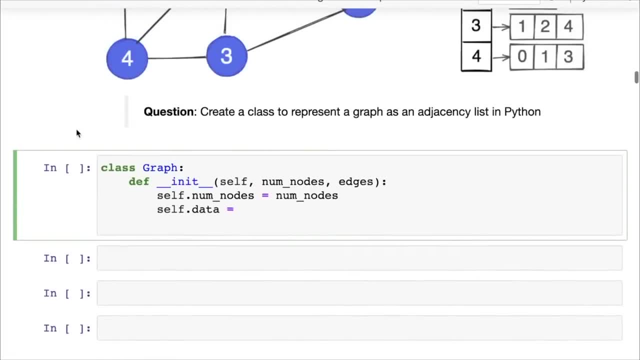 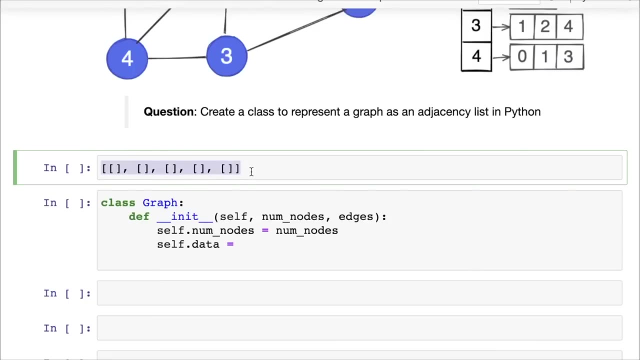 we will fill out the empty list step-by-step to. what we need is something like this In this case: because there are five, because there are five nodes, So this is what we need: to create the five empty lists. Now, in general, the way to create repeated elements is this: you can say, if you want: 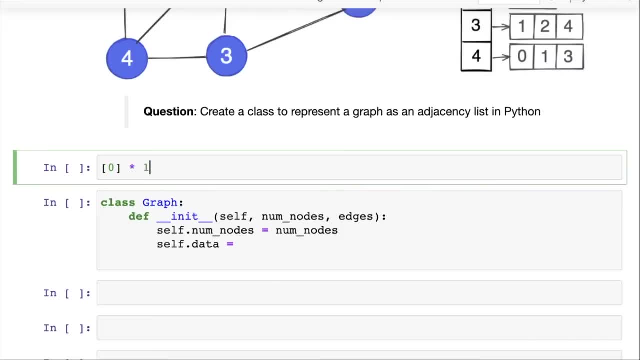 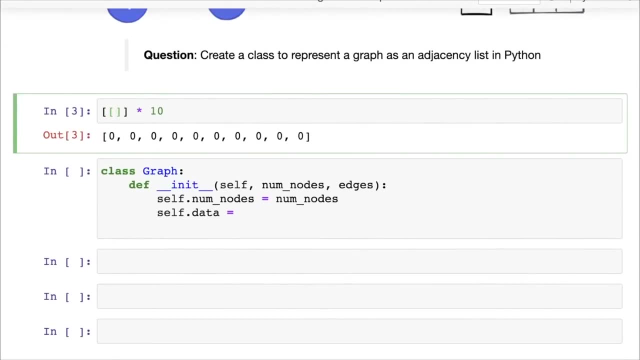 to create a repeated element like this: zero times, you type zero times 10, and that gives you this list: zero, zero, all containing all zeros. On the other hand, if you create empty list times 10, and let's call this L1,, let's see. 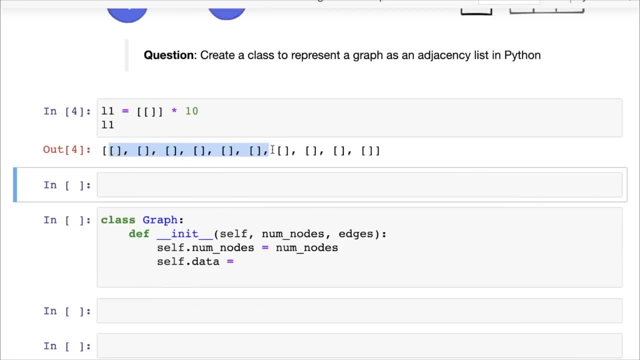 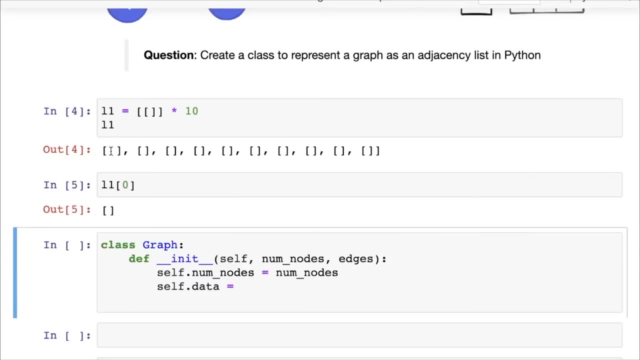 what L1 is. It looks like you've gotten an empty list, or you've gotten a list containing 10 empty lists, but let's just go into the first element. So the first element is this first empty list, and inside the first element let us add the value one. 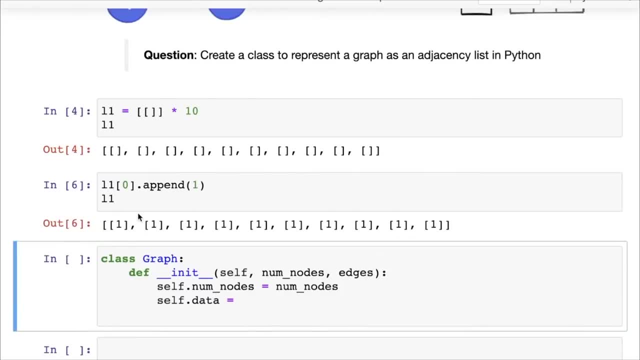 Okay, And then let's look at the. let's look at the list L1 once again, and you see what happens: This one gets inserted into all of these lists. Now, what's the problem here? on? the problem here is that when we do this, 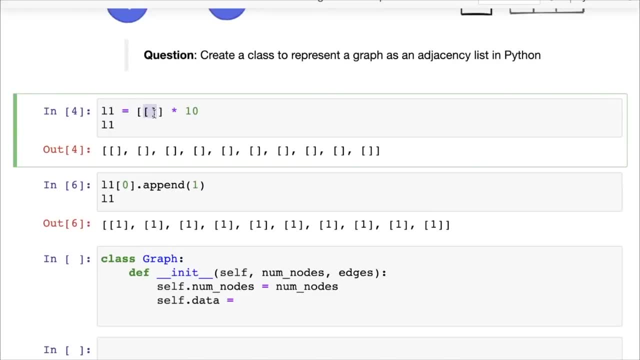 when we create a list containing an empty list or containing any object, then the same object gets replicated 10 times, but Python does not create copies. Now, when you're working with numbers, it's fine, because when you're working with let's. 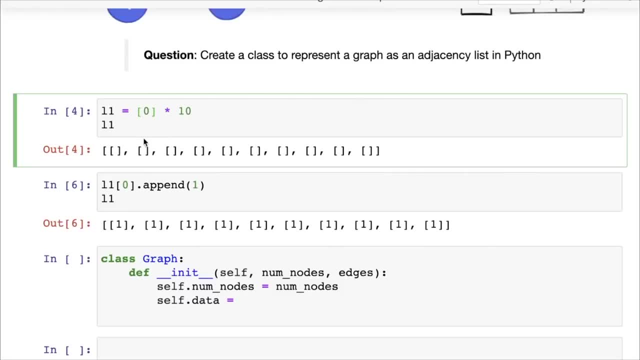 say the number zero, that's fine because, uh, there's no internal structure inside zero, right? So there's nothing you can change inside the zero. It's a fixed value, fixed, immutable value. So what so you can? you can't really say L1 of zero. 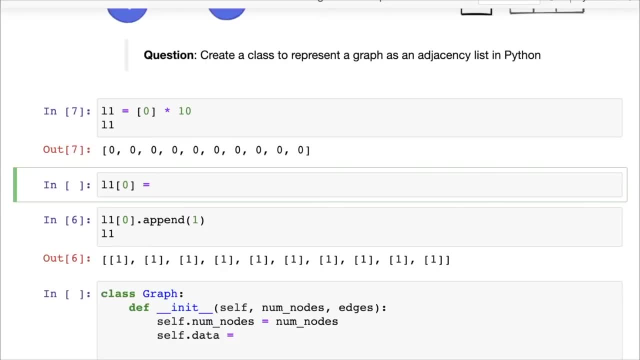 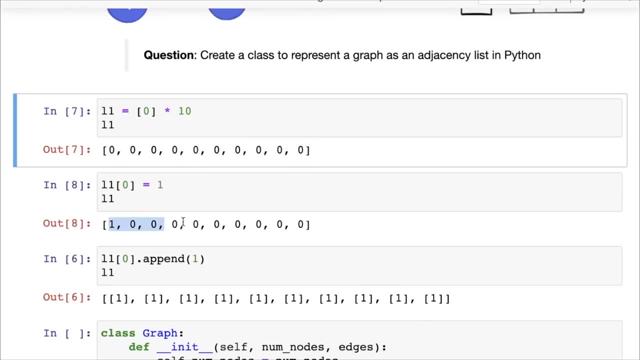 And change its value internally. What are you going to do is you can set L1 of zero to another value. Let's say you can set L1 of zero to one. So instead of getting all zeros, you get all ones. but you cannot take this. take the zero and change something inside it. 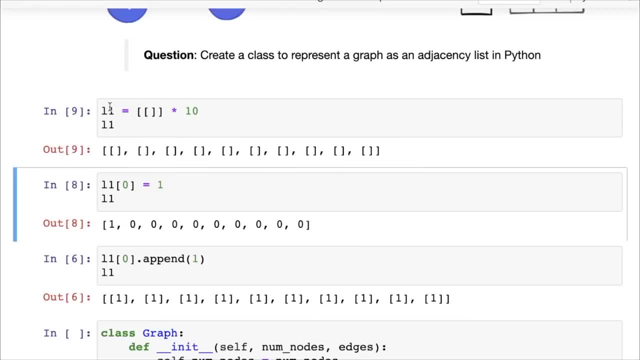 On the other hand, when you have an empty list here, so this is the same list that is showing up in 10 different showing up 10 different times. Each of the each of the elements in the list- outer list- is simply a pointer to this same empty list. 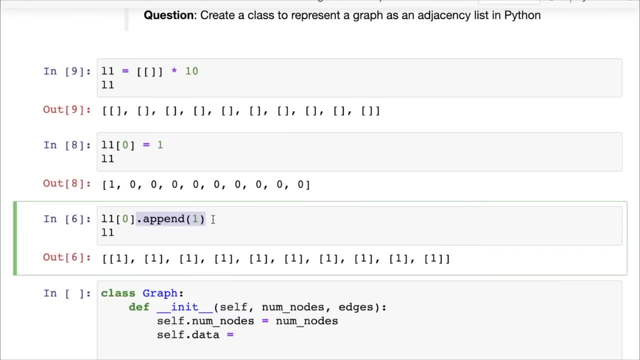 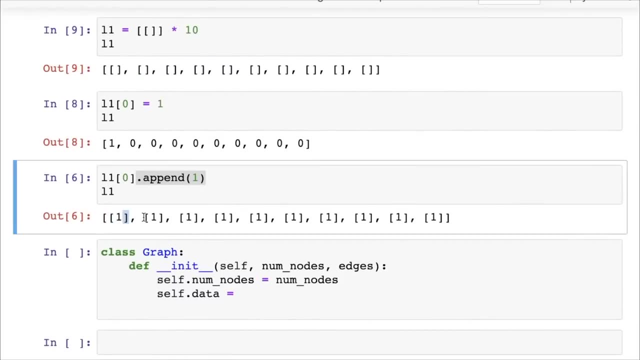 So what? What we can do is, since we can go inside this empty list and append something to it. So, since this is the same object that we are seeing over and over, the one gets appended to the first list, And because the rest of them are the same object, we get back all ones inside here. 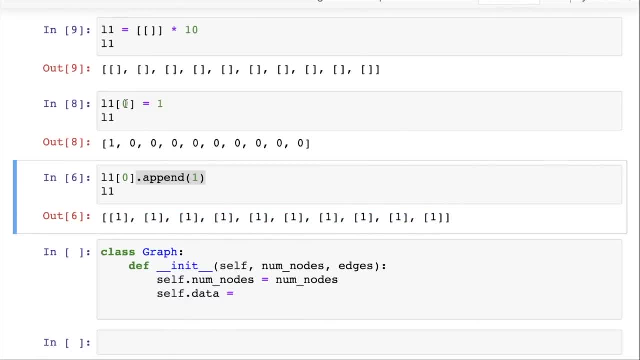 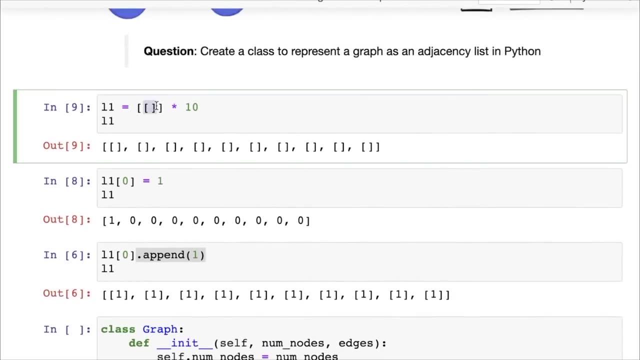 Okay, So this is the reason we're spending time here- is because there's a common, a common bug that you may unintentionally execute whenever you want to create an list of empty lists. do not use this method. So what's the method you should use then? 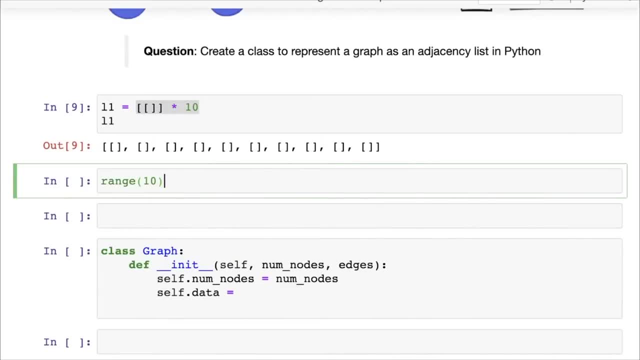 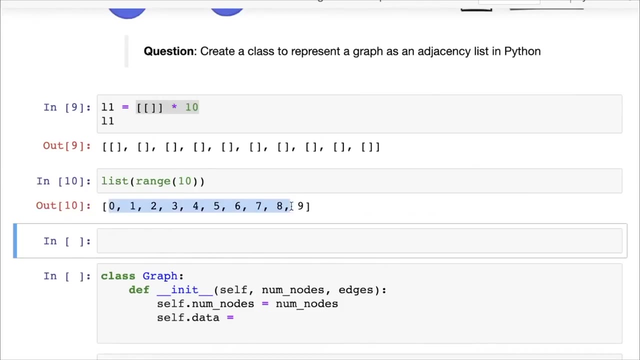 So here's one method you can use. Let's say you want to create a list of empty list of size 10.. So you may be familiar with this object, this, this object called range, this function called range. What this does is, if you view it as a list, you can see that it contains all the elements from zero to nine. 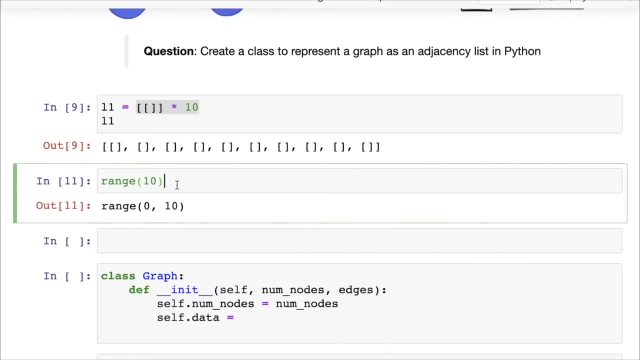 Okay. Now, if you view the range itself, it simply shows you zero to 10, but when you convert it into a list, you can see that internally it contains It contains the value zero to nine. Okay, So you can take this range and you can do something like this: put this range or put anything which is iterable inside these brackets, the list brackets, and then say for X in range and simply put X. 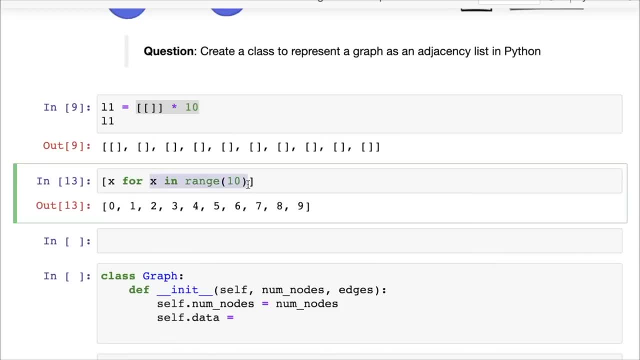 So what did that do? that did practically nothing. We simply took X from the range of zero to 10 and returned X itself. So we created a new list like this: But suppose we multiplied it by two here, X by two, So for each element in the range we are multiplying it by two. 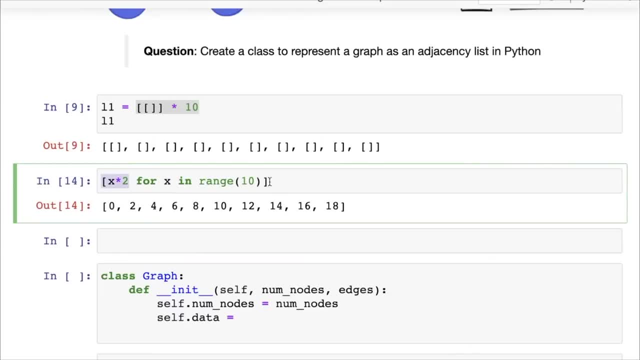 And so we get back a new list which is zero to four, six, eight. So this is: each element is the double of the elements that we have in the range. Now, what we need is we need just empty lists, right? 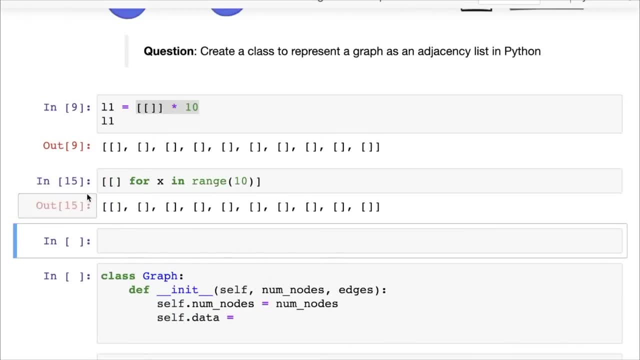 So we can simply put an empty list here and we can ignore this value X that we get here. So now we get back a whole bunch of empty lists. So let's call this L two, And what we're now doing is for each element in the range. 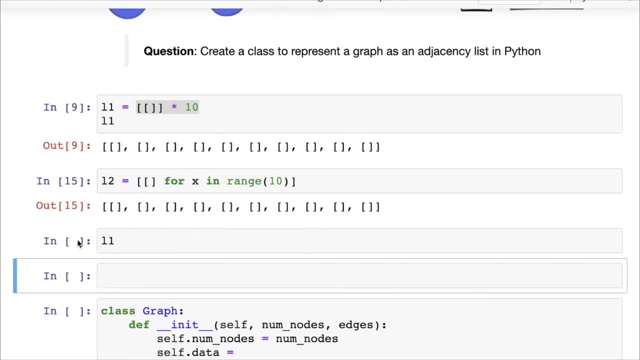 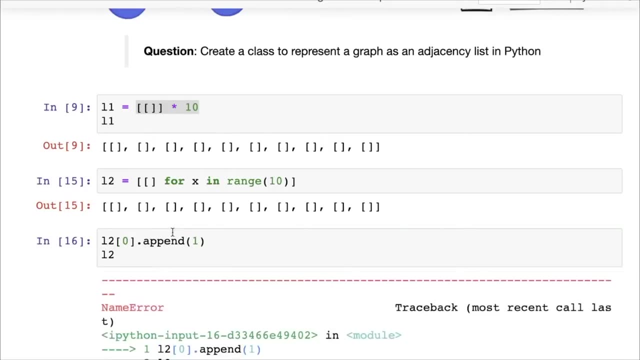 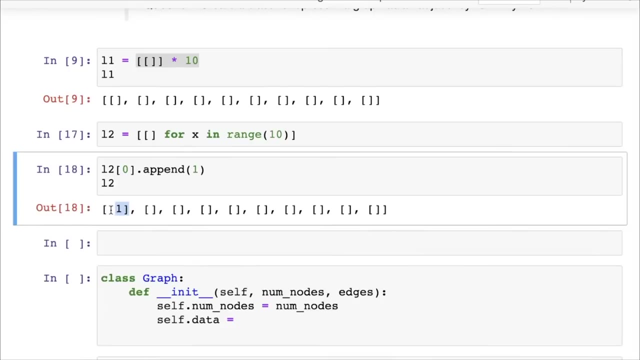 We are creating a new empty list, So this is important. So now when you do L two, zero dot, append one, and then check L two, you can see that one was only inserted inside the first list. Okay, So keep keep out. watch out for this. 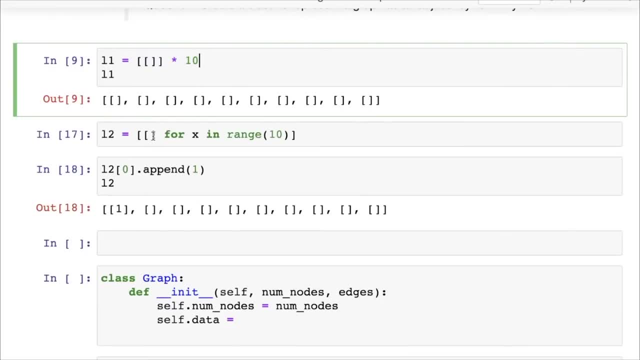 This is something that you will probably go wrong with at some point. I've gone wrong many times, And one last change we can make here is, whenever you're not using a variable in Python, it's always a good idea to just call it underscore. 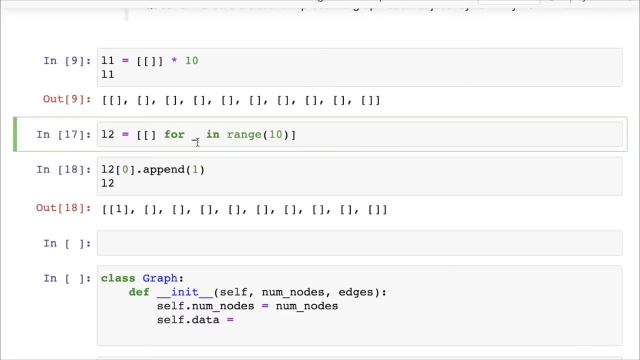 You can still call it X, but your sometimes somebody reading your code may not understand why you have declared a variable and not used it and assume that maybe you've made a mistake. So just to make things very clear: it's always a good idea to make something underscore a V. it's also a variable. 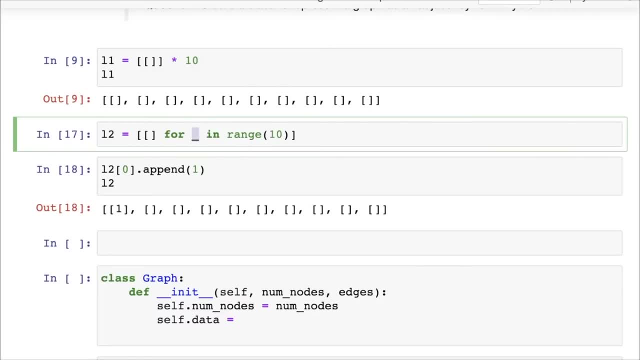 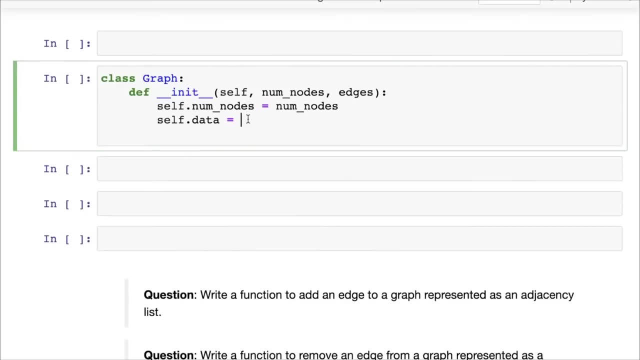 name a valid name and mark something as underscore if it is not being used. Okay, So with that whole discussion about lists, we now know how to Create a list of empty lists. So here you have a list of empty lists, or underscore in range num nodes. 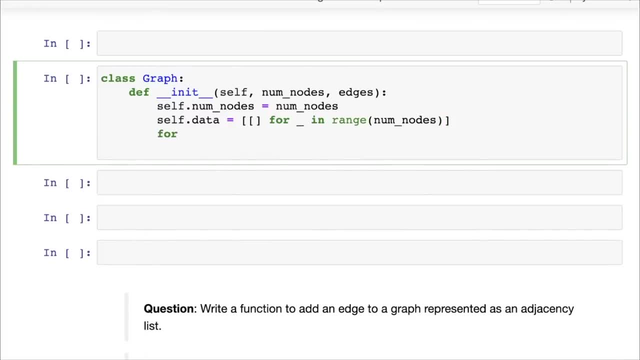 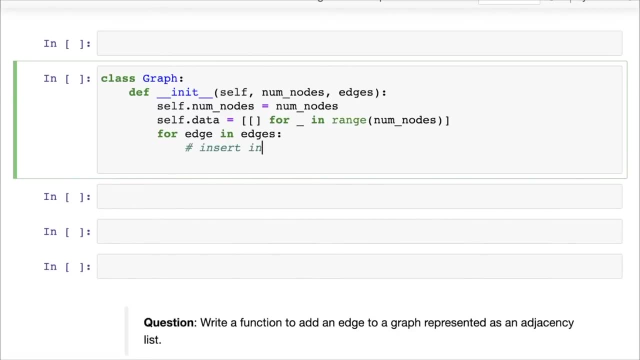 So now we have created a list of empty lists, Then for each edge in edges, we need to do something, So we need to insert it into the right lists. Okay, Now what does for edge and edges look like? So let's see for edge in edges. 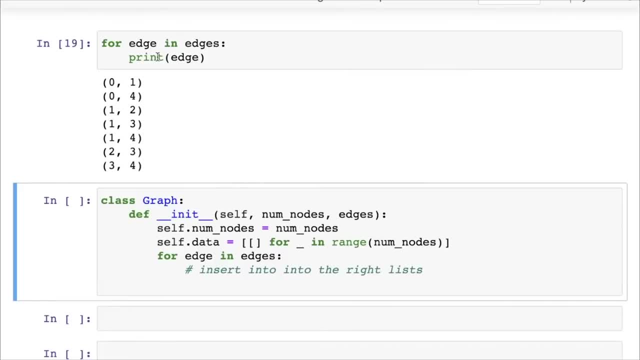 Print edge. Okay, Each edge is a pair. We already know that, And when you have pairs or tuples here, you can get them, get the values out. So let's say let's call them N one and N two, node one and node two. 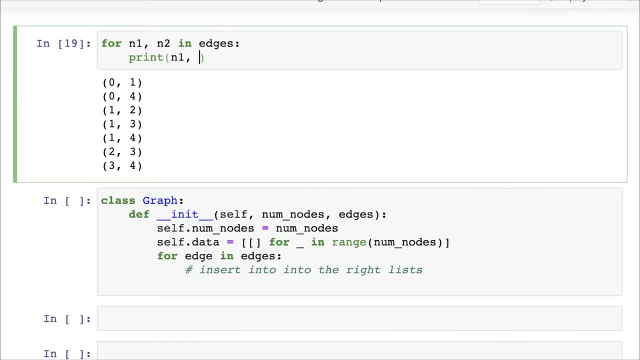 You can get the values N one and N two out like this. So now we can say, print N one and print N two, Okay, And you can see that we are able to get values N one and N two out directly within the for loop. 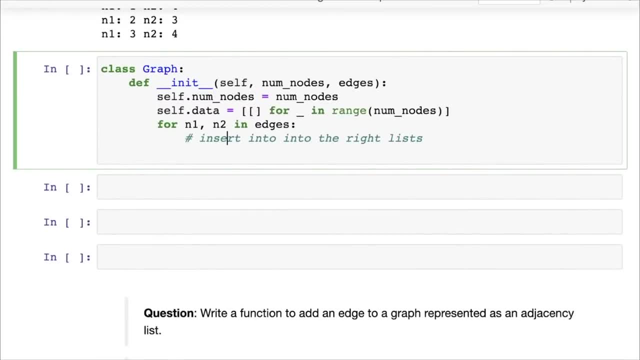 So let's call this N one and N two, And now this is a much more Pythonic way of writing code. So one of the things that we are also learning is how to write code which is more Pythonic or which is idiomatic in Python. 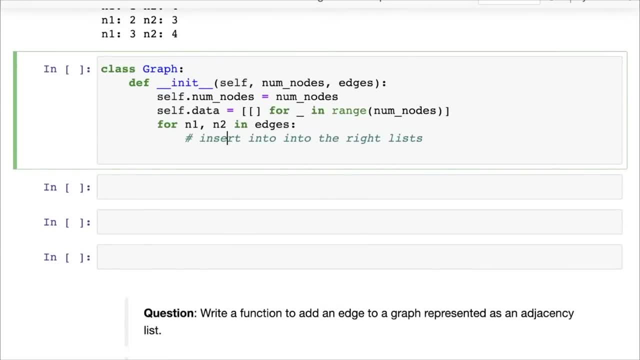 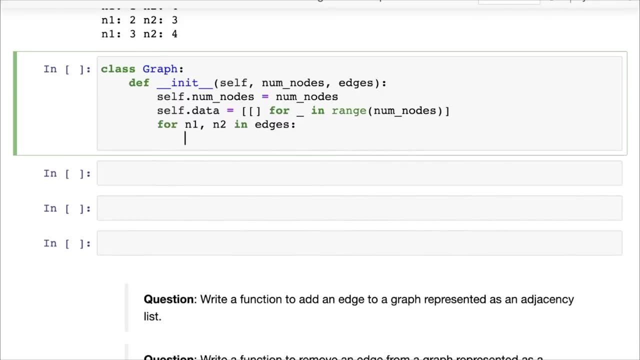 And this is again something that will impress people when you use it in an interview or a coding challenge. So for N one and N two in edges, what we need to do is first we get Self-draft data of N one. 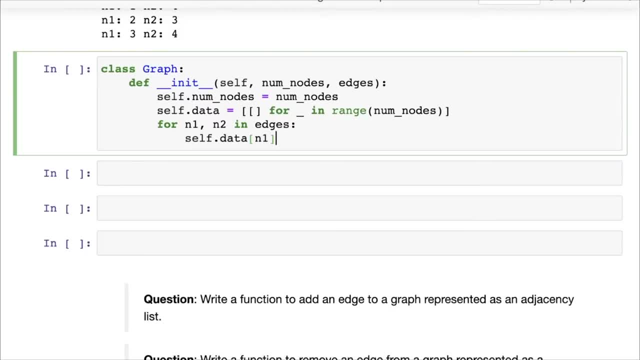 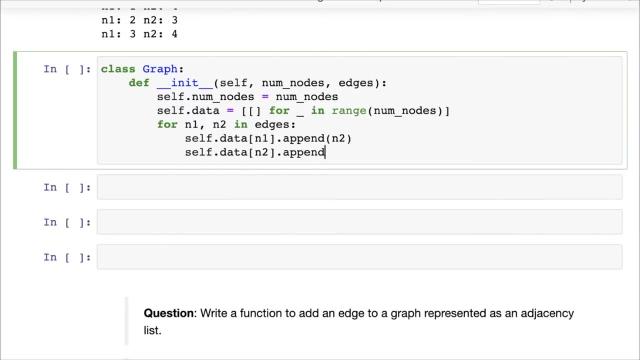 So this gives us the adjacency list for N one, the first node, and here we append the value N two. And similarly we do the same for N two and we append N one to it. And that's it. Now we've set up the graph. 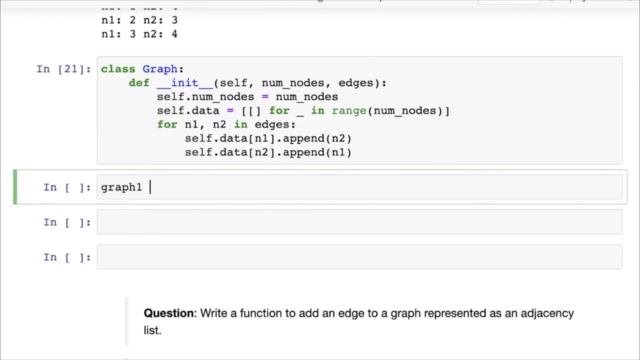 Let's create a graph G one- Let's call this graph one, maybe- And we simply invoke the graph function and then we give it a number of nodes and the edges right. So remember self, We'll be passed in by Python automatically as the object that is getting created. 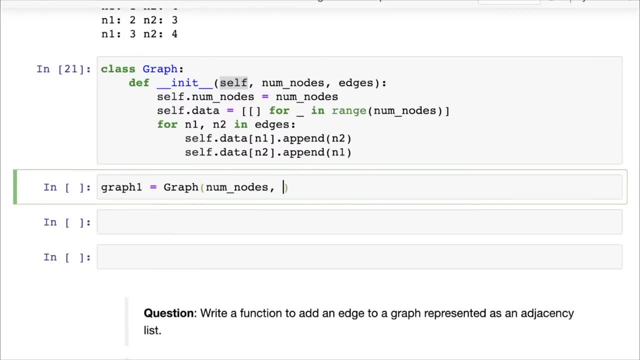 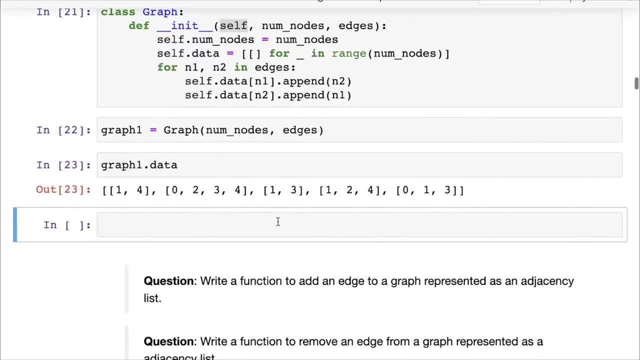 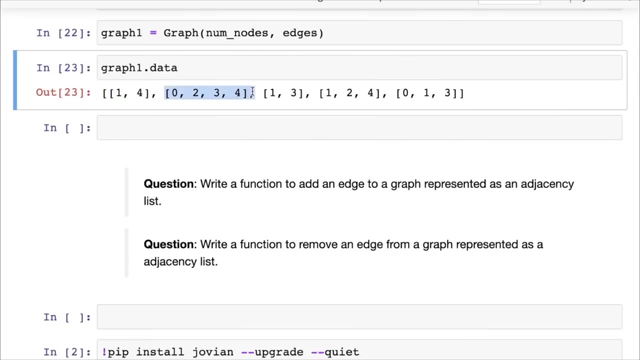 So the graph one object essentially. So now the number of nodes is five and we have a list of edges and let's see what graph one dot data looks like. So there you go. You can see that zero is connected to one and four and one is connected to zero, two, three, four and so on. 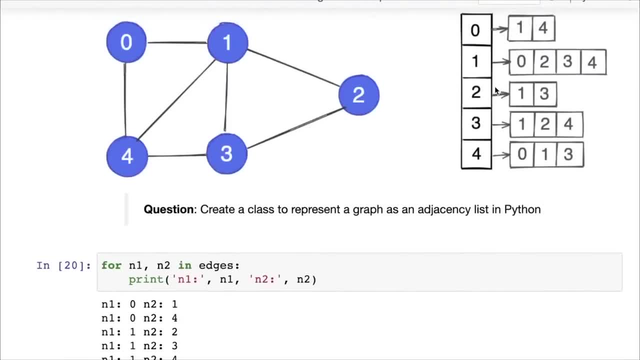 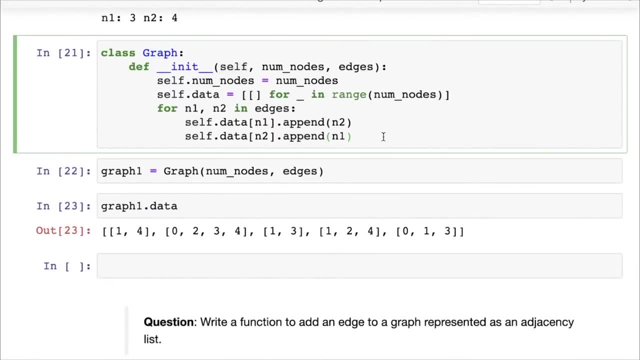 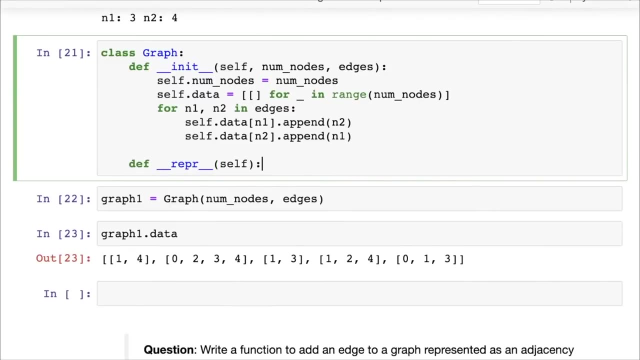 Now, while this is okay, it would be nicer to print it like this. So maybe let's see if we can print it like this. And the way to do that is to define a wrapper function. So we define a function called underscore, underscore R, E, P, R, and it contains. it simply takes self as the input. 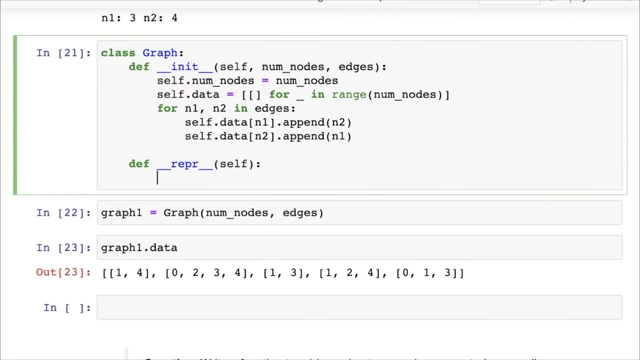 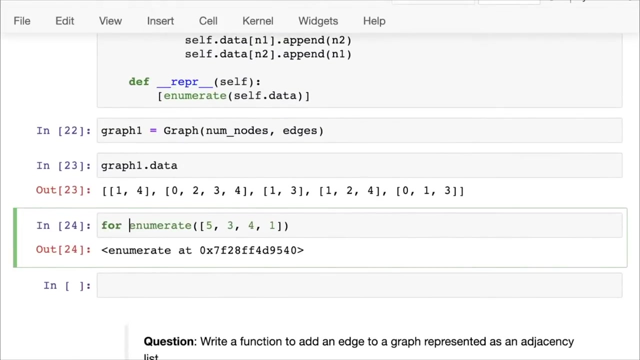 And what we are going to do is we are going to go over, We're going to call enumerate On self dot data. Now, what does that give us? Let's just check what enumerate on self dot data give us gives us. Well, maybe, before we do that, let's see what enumerate on a list gives us. enumerate on a list gives us this object, but let's just get the value out of it in a for loop, because you can use an enumerate in a for loop and then just print X. 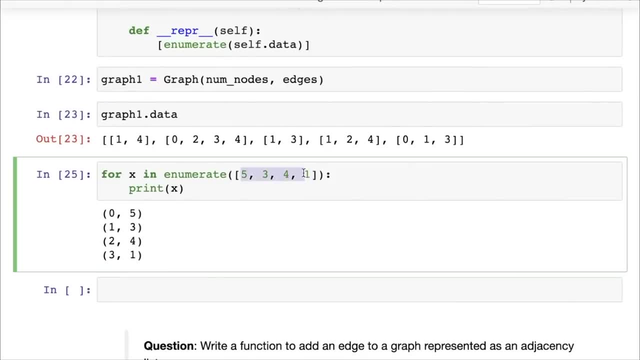 So what enumerate gives us is? it gives us the values from the list, But apart from those values, it also gives us indices. Okay, So you can get an index I and a value B out of enumerate. So then you can see that you can print both I and we here and you will get back the same output. 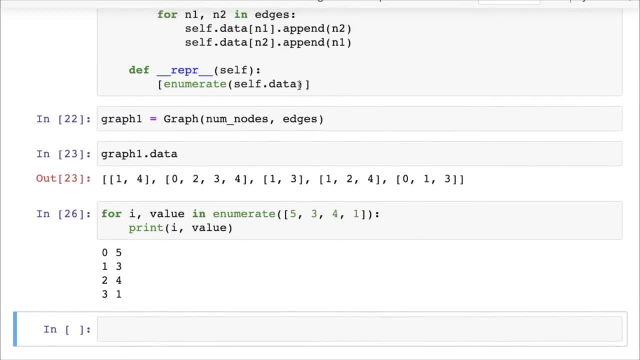 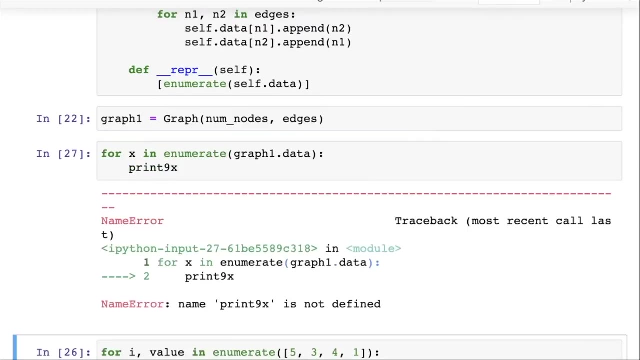 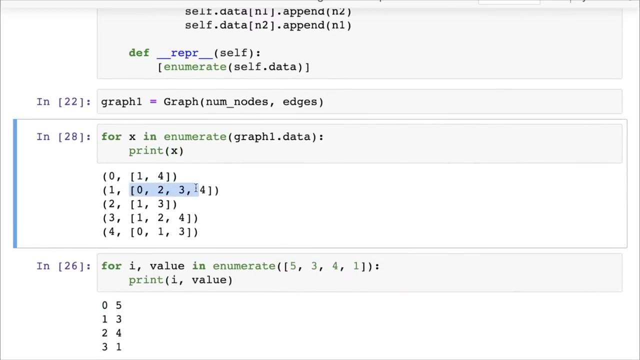 Okay, So what we can say is: we can do enumerate self dot data now, because self dot data contains these elements. So what we'll get back is we'll get back pairs. Let's see here. So we'll get back pairs: zero comma one. four. one comma zero two, three. four. two comma two, one, three. 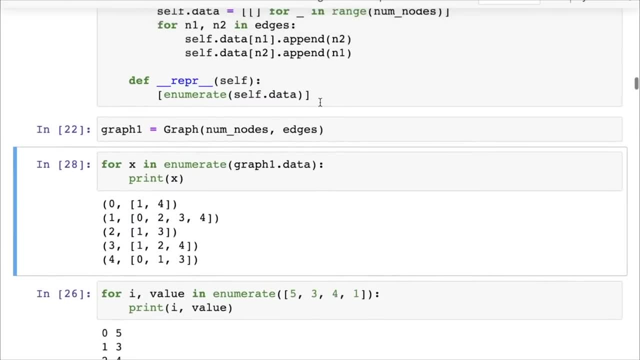 Now this is starting to look a lot like what we want. Okay, So we'll just take enumerate self data and these will take these pairs. So the pairs will be a node, So node N and it's neighbors, The. we have the node N, so the node N will first be zero and its neighbors will be one in four node. 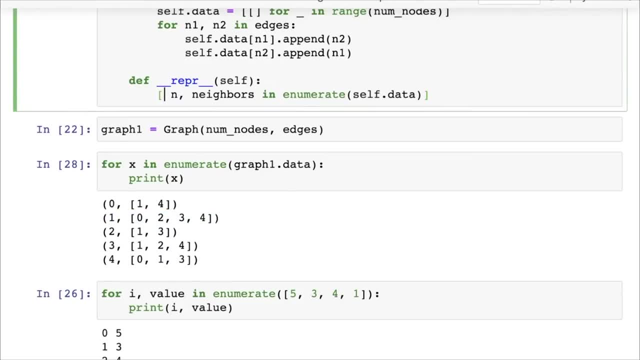 N will be one and its neighbor will be one and two and so on, And then so for N comma neighbors in enumerate, what we'll do is we'll simply create a simple string, And here we are using string formatting. We're simply creating the string. 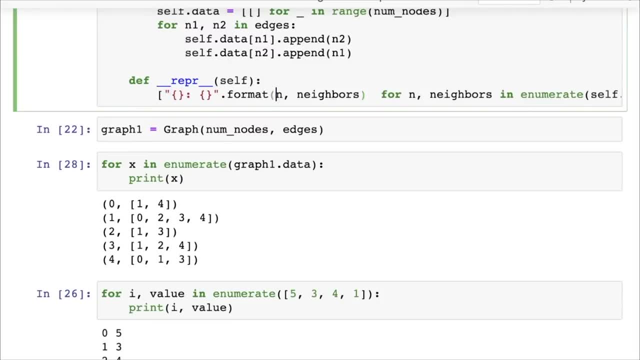 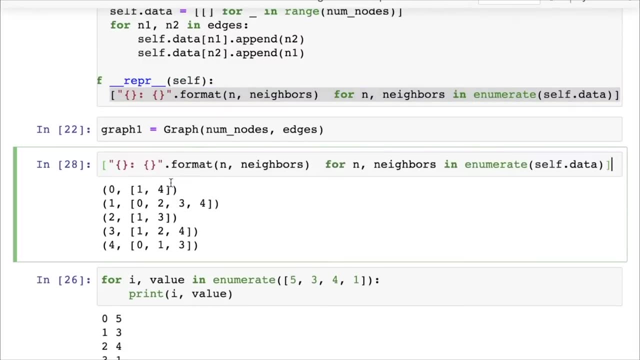 where we put this. Here we place a placeholder where we put N, and then here we put a placeholder where we put neighbors Again. let's just see what that looks like- And this is the best thing about Jupiter- while you're writing code. 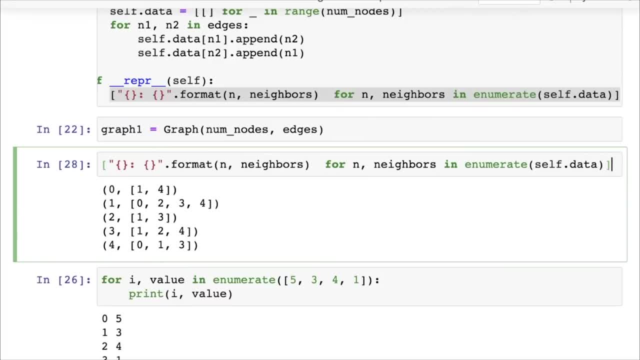 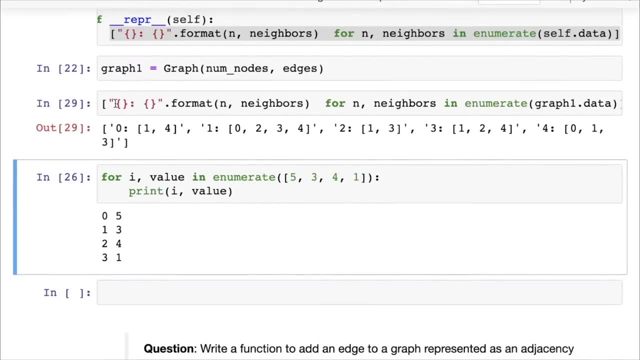 You can test your code right then and there, simply by creating putting data into a new, into a new cell. So let's see graph one: dot data. You can see here that now we have, now we've converted that enumerated list into a list of strings. 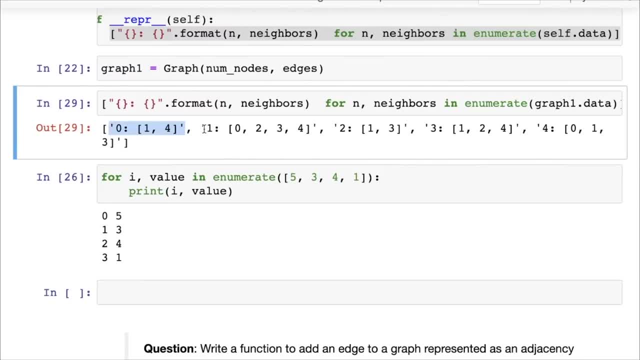 So we have a string here- This is the string zero- pointing to one comma four. This is a string one point. this is one pointing to zero, two, three, four and so on. But this is still a list of strings. 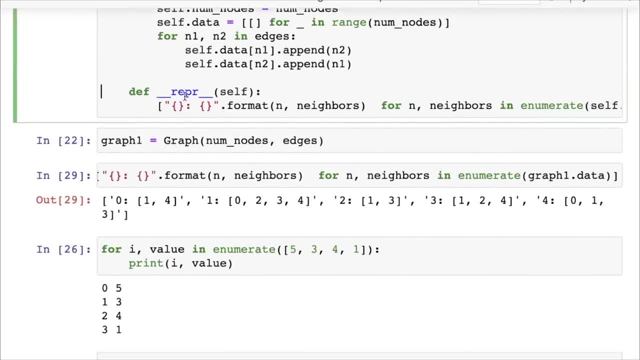 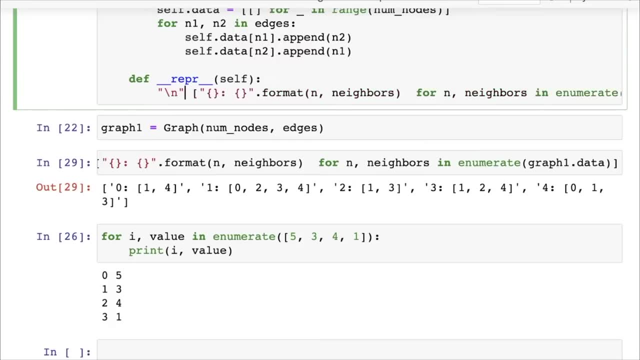 What we need to return from the wrapper function is a single string. So the way to join them together: whenever you have a list of strings and you want to join them together, all you need to do is you say what you want to join them with. 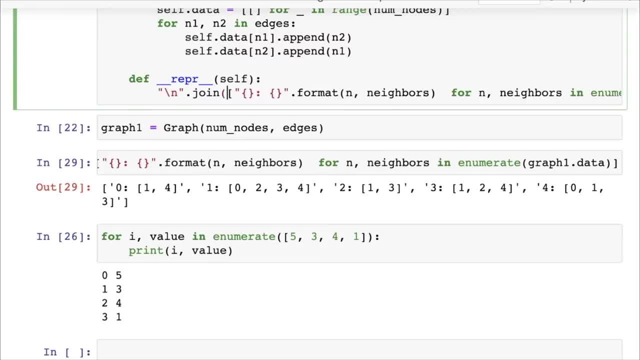 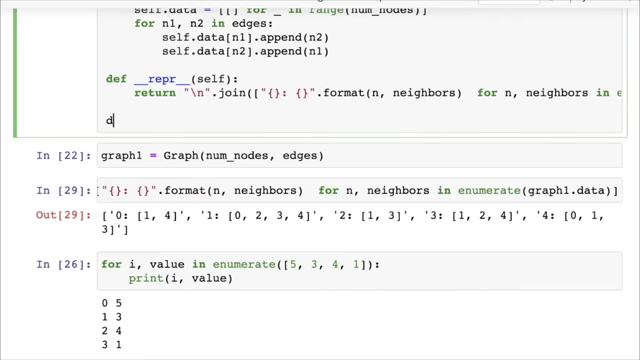 So we want to join them with a new line and then call the joint function on that string and return that right. So that is our wrapper function And we'll see its users in just a moment. And similarly we have another function called STR. 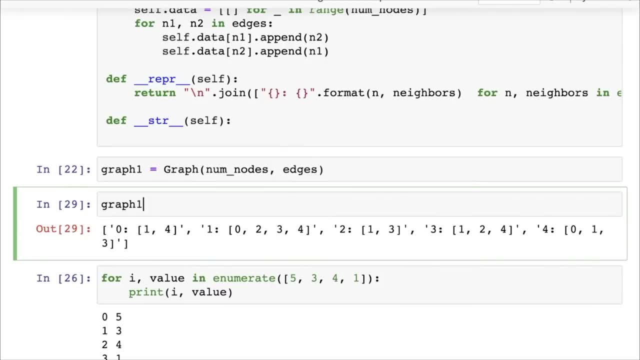 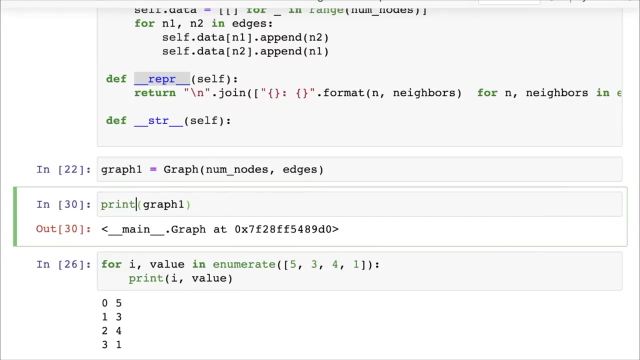 Now wrapper is used when we simply type graph one. So when we type graph one, this is the output of the default wrapper function. Now this will get replaced by the wrapper function that we are defining. But when we do STR of graph one, or when we do print of graph one, or when we insert graph one into a string, that is when the STR function is used. 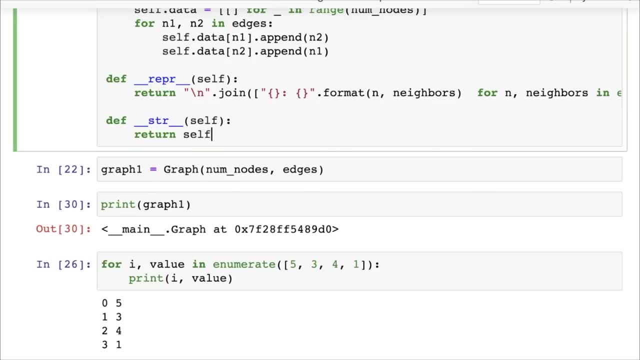 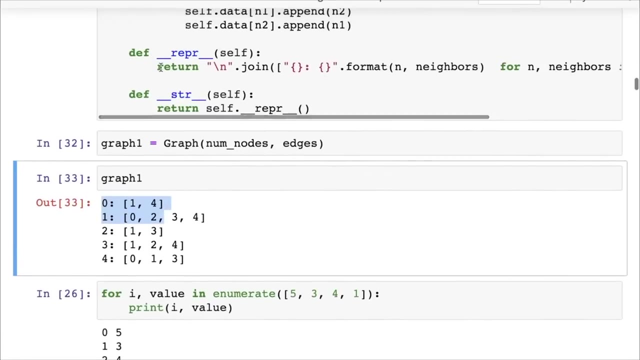 Now we will simply use a wrapper representation. So let's just put self dot, Okay, Okay. So let's just put self dot, underscore, underscore, RDPR, and that's it, Okay. So let's see, now let's put, let's type graph one here, and you can see that now we have this representation printed using this wrapper function that we've defined. 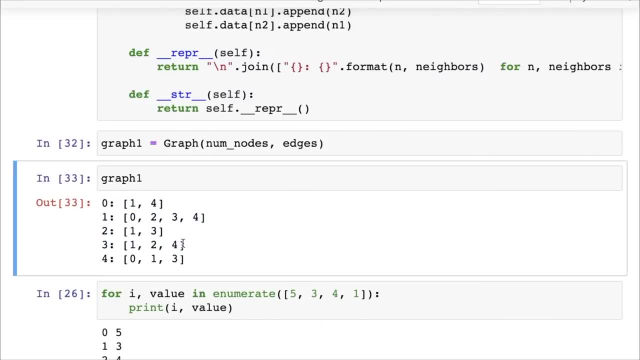 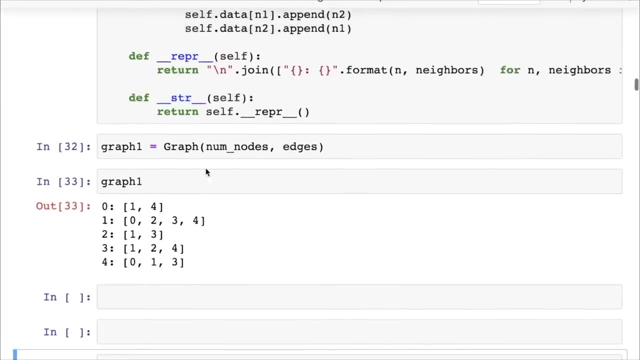 So we have zero, one, four, one, zero, two, three, four, two connected to one, three, three connected to one, two, four and four connected to zero, one and three. Okay, So now we have a graph data structure that we've implemented using a class. 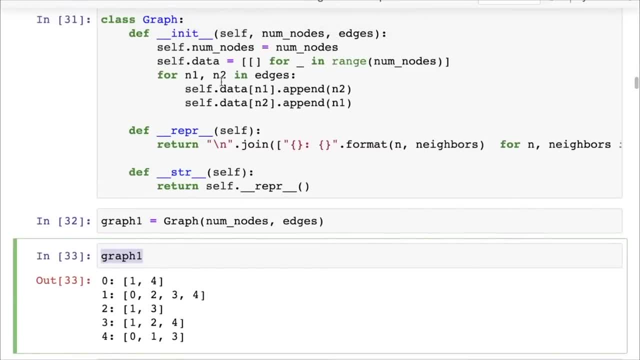 So the adjacency list, and we have a nice way to print it out, And this is just good programming practice. Now you don't have to do this in a coding competition, or you don't have to do this. It's good If you do it in an interview, if, let's say, you're able to type this out quickly. but when you are working, or when you are working on your own problems or on your own code or on a project, always make sure that any classes you define have a good string representation. 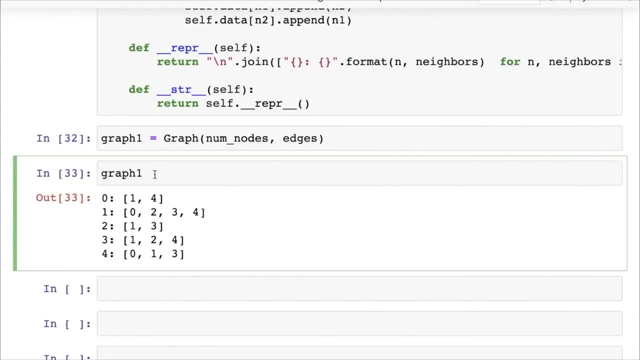 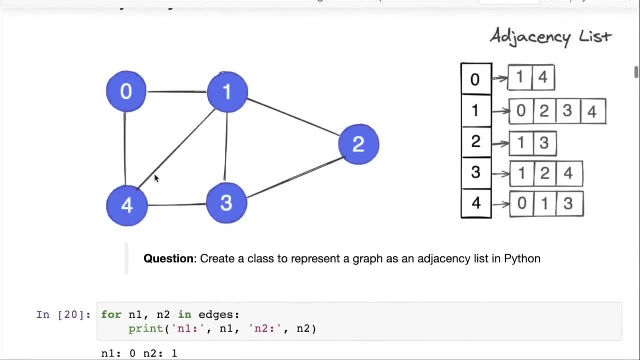 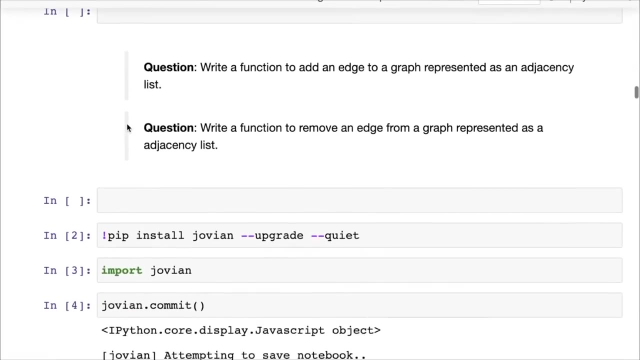 So that when you type the name of a variable, you understand what it represents and you don't have to spend time thinking about it. make it clear to yourself, Okay, So that's the adjacency list, And we'll see how that is useful in just a few moments. but here are a couple of questions for you. 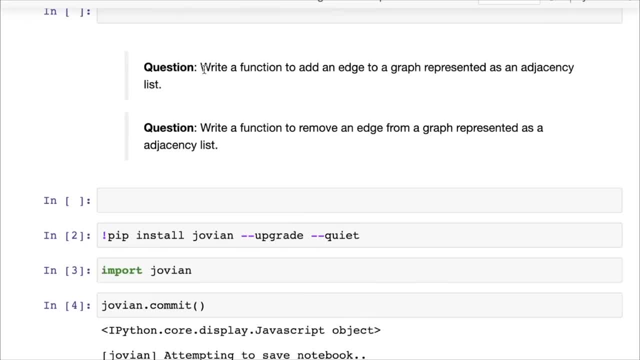 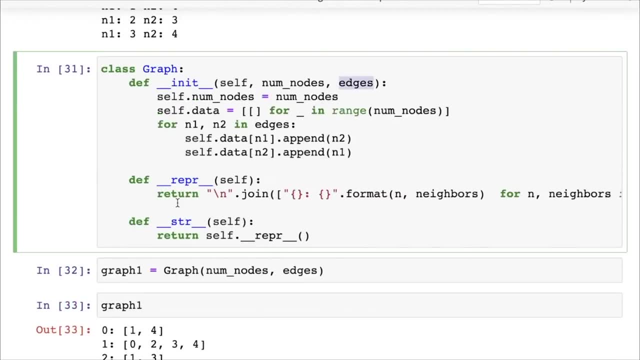 Try writing a function to add an edge to a graph that is represented as an adjacency list. Okay, So here we've specified all the edges right in the beginning, but can you write a function- add edge- Which takes a couple of nodes and it inserts an edge between those two nodes? 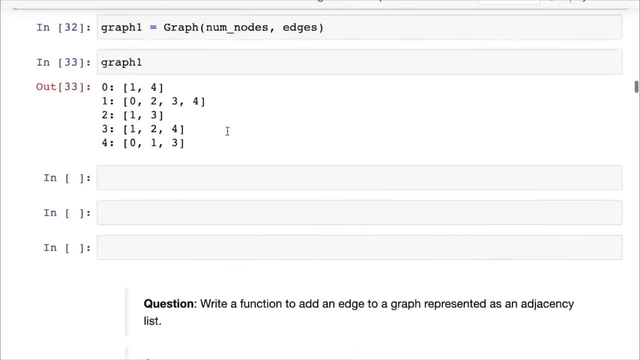 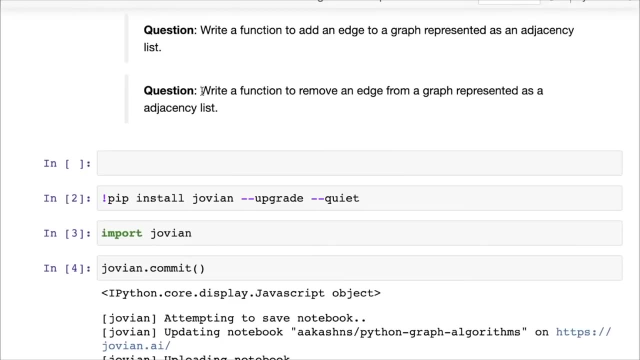 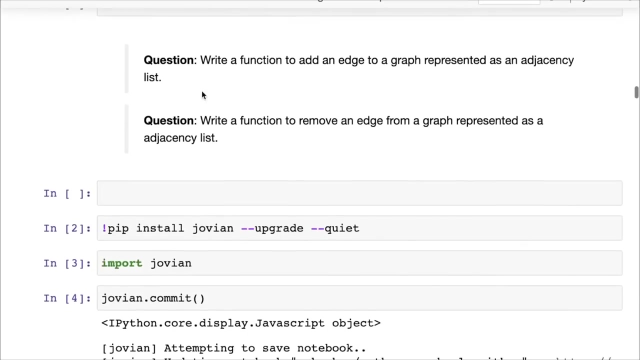 And here's a hint. This code might be useful, So do try that out. Now here's another one. Can you write a function to remove an edge from a graph which is represented as an adjacency list? Here you may have to use the list remove functions to remove a particular element from a list. but these are two good exercises to complete here. 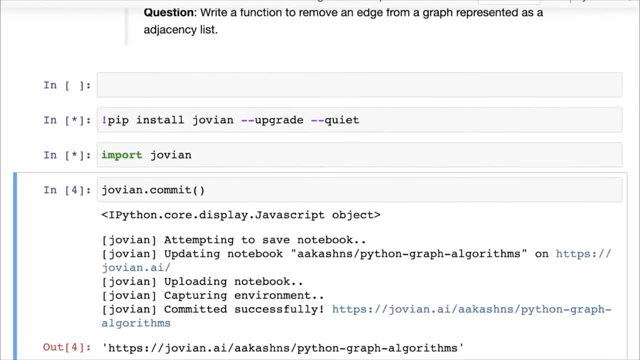 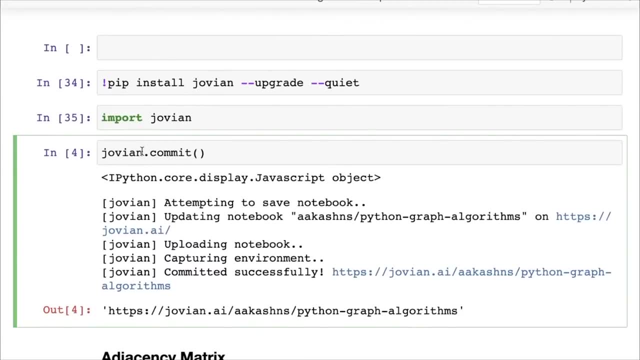 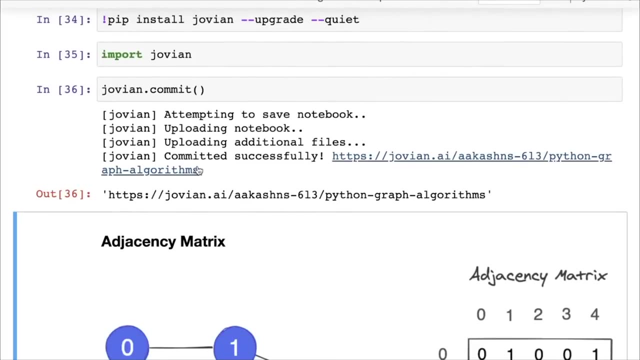 Okay, Now, before we continue, let's just save Our work, And we know that this notebook is running on binder, which is a free service, So we'll just save our work by running Joviancom it, And what that will do is that we'll capture a snapshot of this notebook, all the changes that you've made, and put this on your Jovian profile. 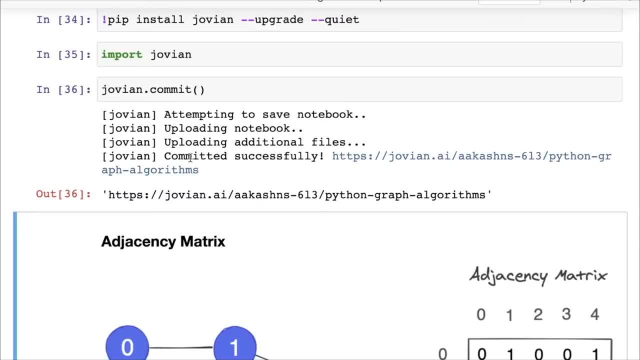 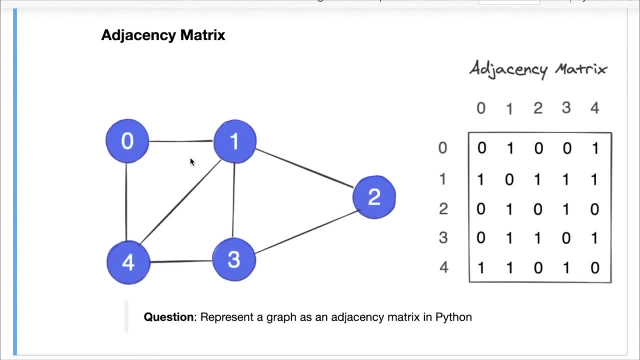 Now this will go on your Jovian profile, from where you can continue running it, continue executing it from where you have left off. Okay Now. another common representation for graphs is called the Adjacency matrix, which is slightly different from adjacency lists. 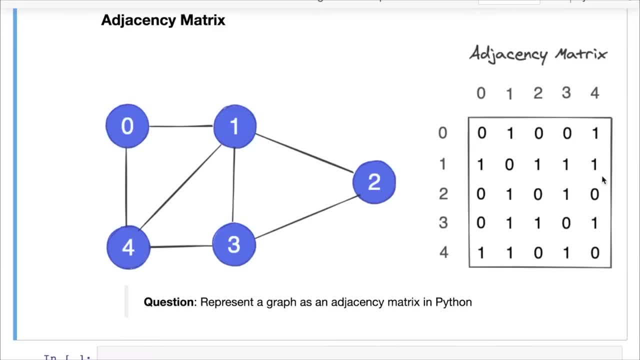 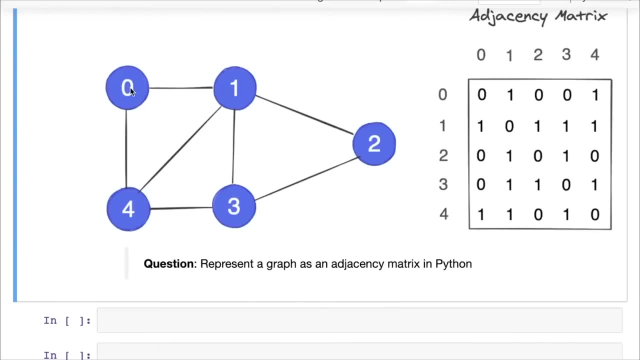 In this case, for example, the same graph here is represented using this matrix. So what we do is we create a matrix of size N by N, If N is the number of, if N is the number of nodes in the graph, and then for each node, for instance, since we have zero and since we have an edge between one and two, 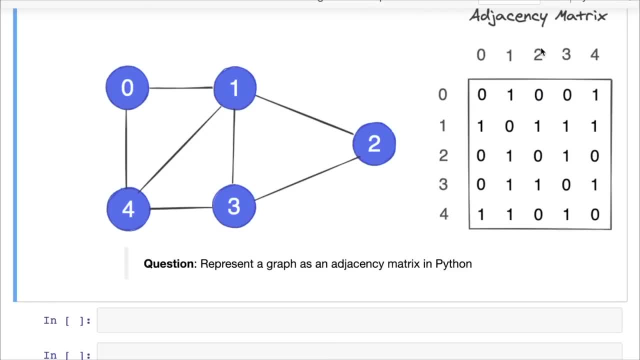 So If you take the first row, row number one, Okay, And column, You put a one there. Otherwise, if there's no edge- for example there's no edge between zero and two- to take the zero through and column number two, the, you put a zero there. 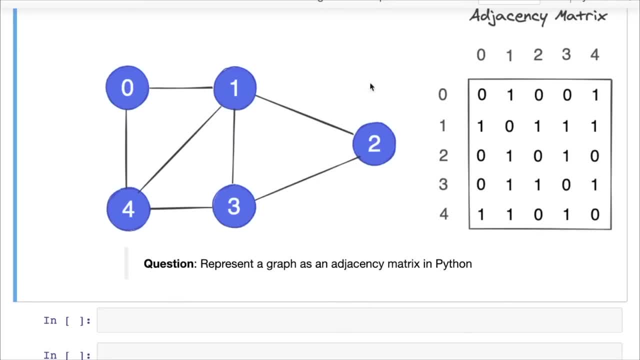 Okay, So you put a one wherever there is an edge between the two nodes and you put a zero wherever there isn't. You can see that there is this reflection reflexive property here, because one, two is one and two one is also one, because these are undirected edges. 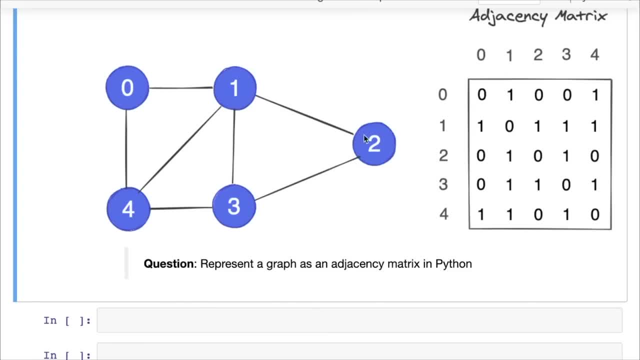 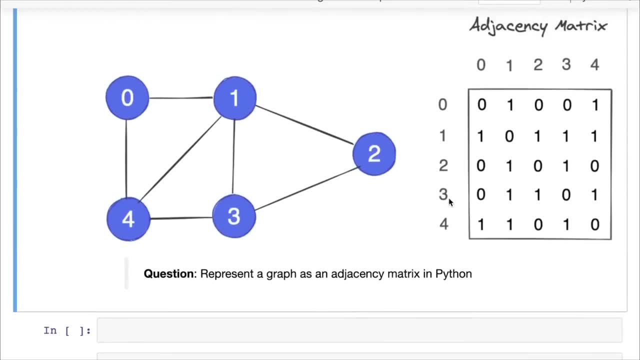 Now, of course, if this is a directed graph, this would be different. Okay, So an exercise for you once again is to represent a graph as an adjacency matrix in Python. Shouldn't be too hard. All you have to do is, instead of so in adjacency list, we initialized a list of empty lists here. 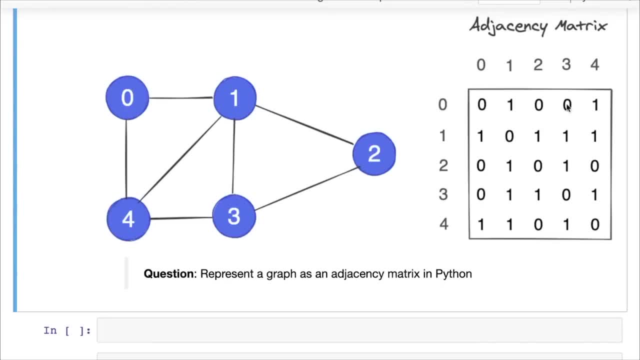 You may want to initialize a list of zeros, a list containing lists of zeros, Okay, And then you may simply just want to fill in the zero ones in the right places. Now, adjacency matrices have their own benefits. Uh, sometimes they are. 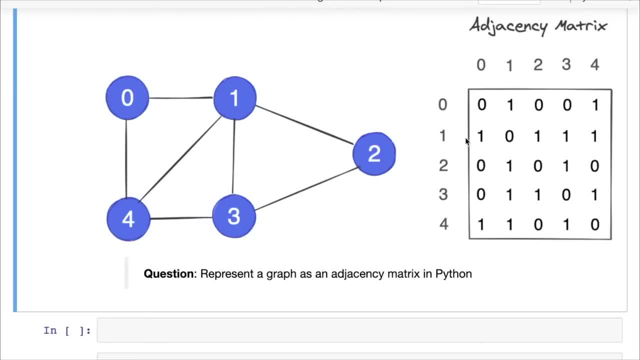 More useful. for example, when you want to immediately check if there is an edge between two vertices or two nodes, you can quickly look up. look it up in the adjacency matrix. but in the adjacency list you will have to get the list for one of them. 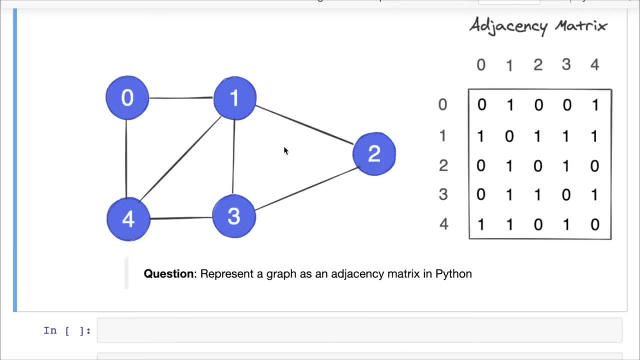 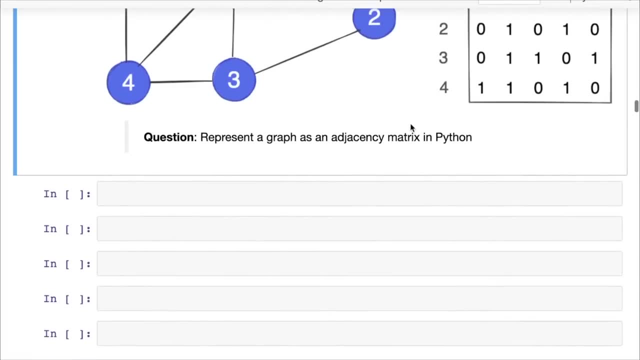 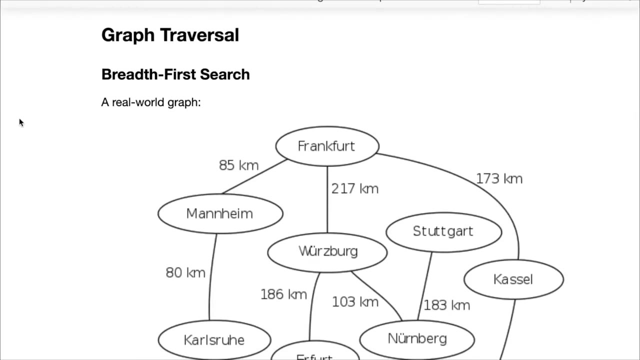 And then search through that list, which is fine for most cases, but in some cases you may just want an adjacency matrix as well, So that's one other way you can represent a graph and that's an exercise for you. Okay, So now we know who we've represented graphs, and now we can start looking at some graph algorithms, and probably the most common graph algorithm- something that you will ultimately get asked in one interview or the other if you're interviewing with a bunch of companies- is breadth first search and breadth first search. 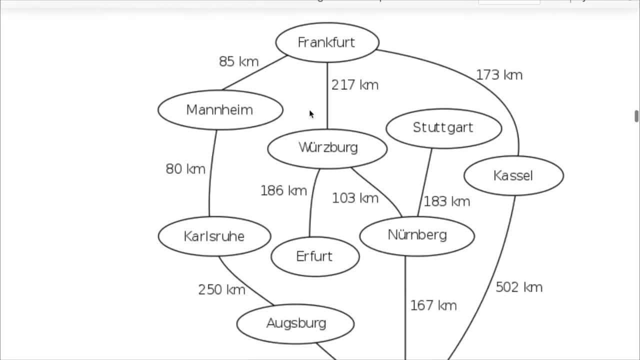 Well, this is what it looks like, So suppose you have this re. this is a real world graph that we're looking at. So these are cities in Germany And you can see that there are roads between these cities and we have lengths of each road and we can ignore the lengths for now. 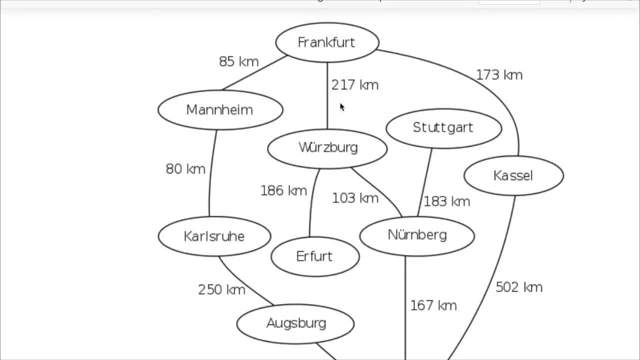 What's important is that these cities are connected to each other, but not all cities are connected to all of them, all of the others. So, starting from Frankfurt, you may want to find out which are the cities that are that you can reach from Frankfurt without stopping. 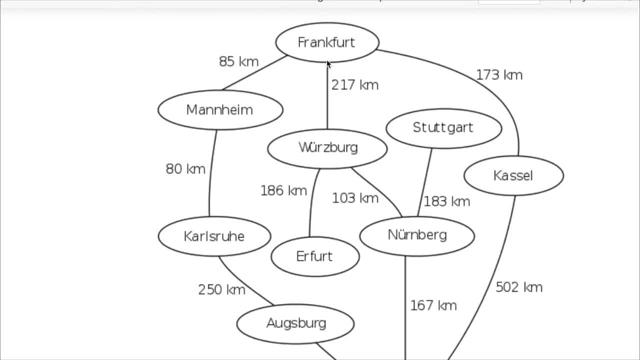 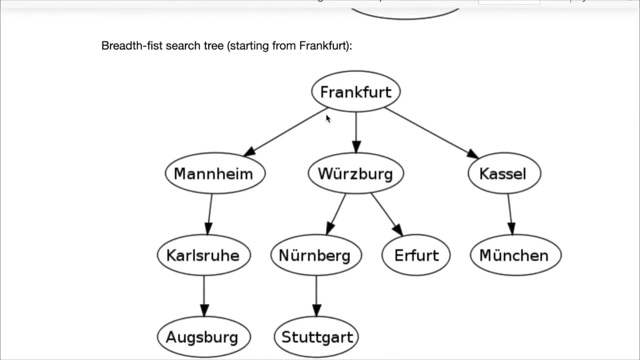 So which are the cities that are one edge of it From Frankfurt? And if you look at it this way, it turns out that Mannheim, castle and was bug are the three cities that are one edge away from Frankfurt. Right, So if you start drawing this tree of sorts, you will find that Mannheim, was bug and castle are one edge away. 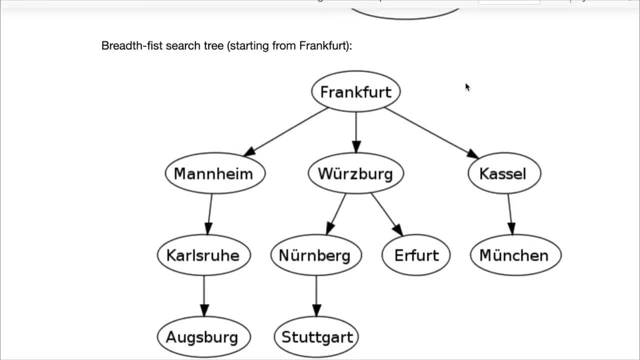 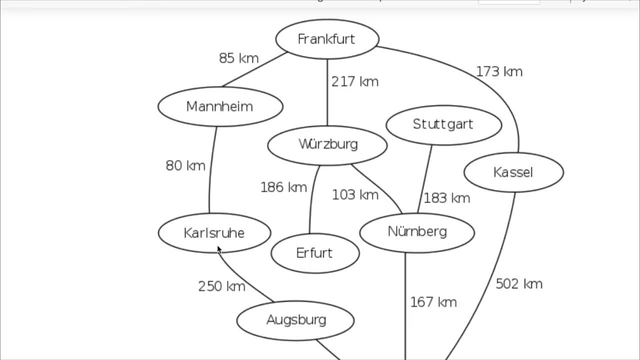 Okay, Then you might ask which are the cities which are two edges away from Frankfurt. So now the cities that are: Mannheim is connected to, Okay, Karlsruhe and was bug is connected to these two cities and then castle is connected to this city. 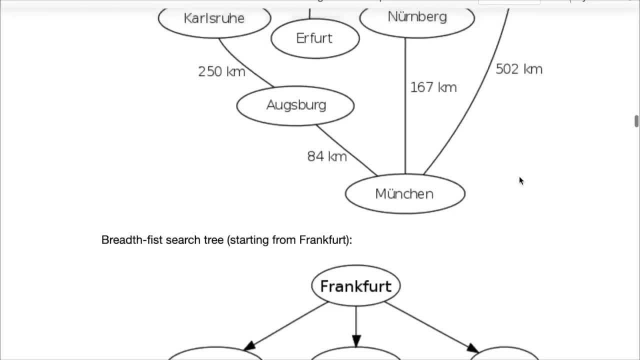 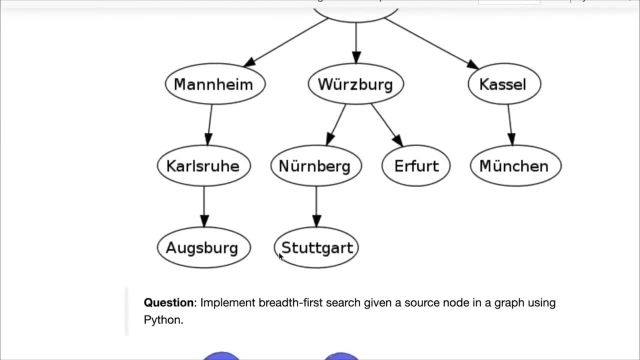 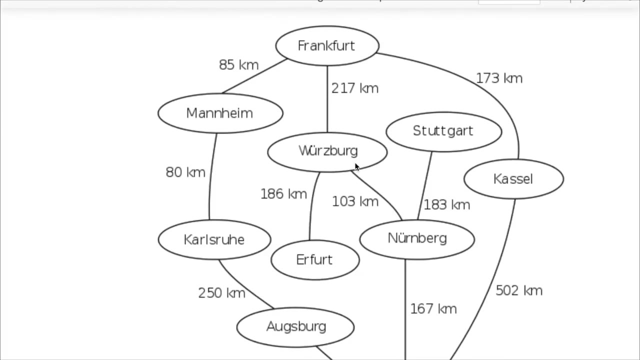 Okay, So here you have these other cities, and then you might ask which are the cities that are three steps away from the, from Frankfurt, And that would be the remaining two cities, Augsburg and Stuttgart. Okay, Now, I let you think about this. but what you will find in this way, as you go step by step by step, like first, you're finding all the. 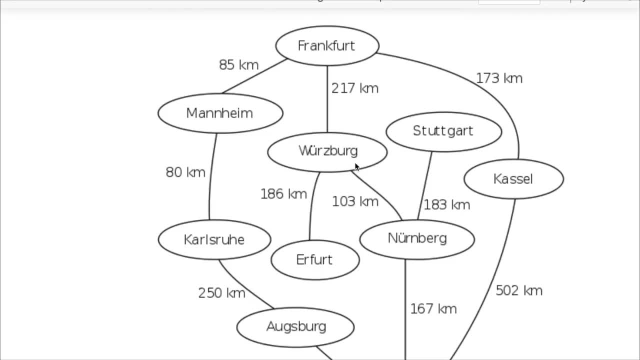 cities that are one Step away. So all the nodes that are one step away from a source node. then you're finding all the nodes that are two steps away from a source node. What this will give you is, ultimately, you will end up for each node. 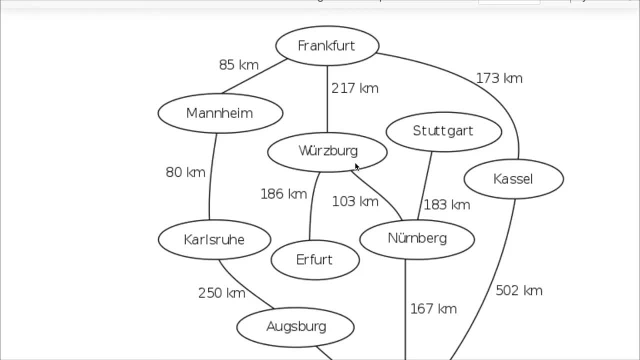 You will find out how far away it is from the source And that will be the length of the shortest path between the two. Okay, And you can verify that. I'll let you think about it. For instance, if you see you can go to castle by going this way from was bug to, 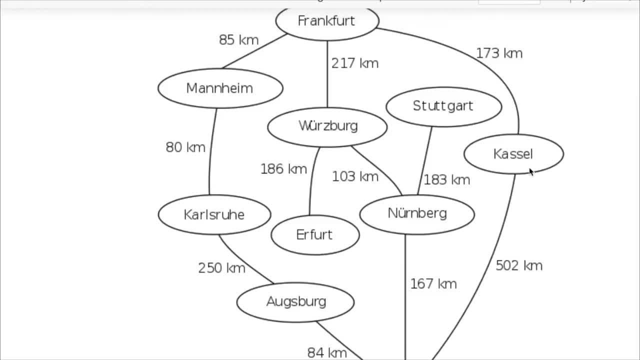 Nuremberg, to mention to castle. but that would not be the shortest path, but binary search, the. this is called breadth First search. breadth first search will always discover the shortest path, because we're first finding all the nodes at distance one. 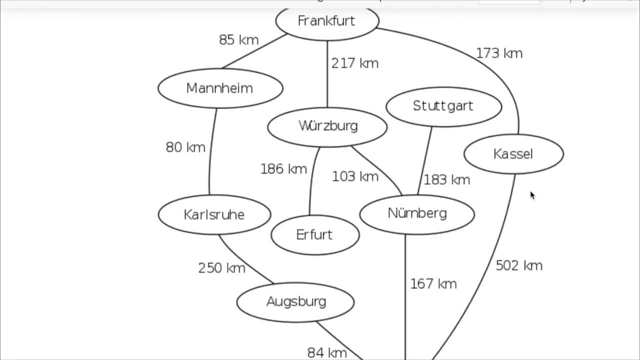 And then we're finding all the nodes at distance two, and then we're finding all the nodes at distance three, And if a node at distance three has a shorter path then it would have been already fine found when we are finding nodes of length. 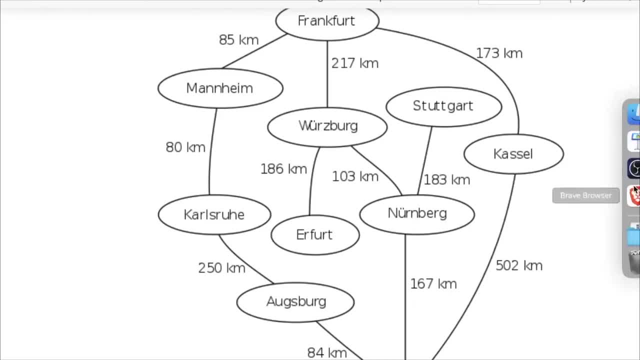 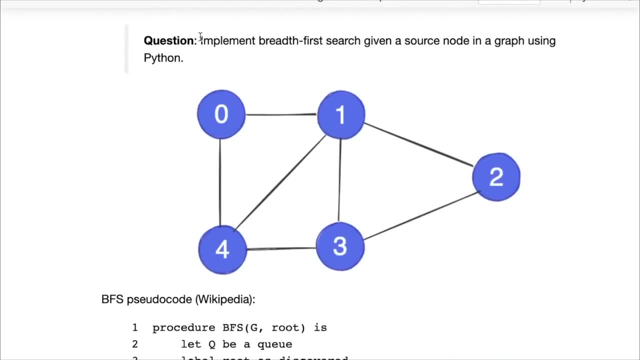 one or two, or distance one or two. Okay, So that's breadth first search. So here's one problem that you might face in an interview: implement breadth first search given a source node in a graph using python. Okay, And here is some pseudo code. 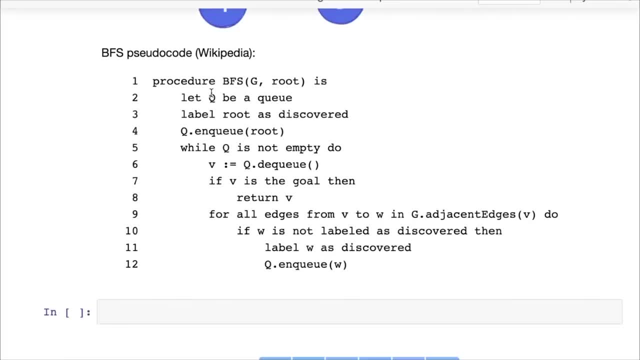 This is so. it's always a good idea to write or explain your approach in plain English before you implement it, so that you do not make mistakes while coding. So here is a pseudo code. So if you do not make mistakes while coding, Okay. 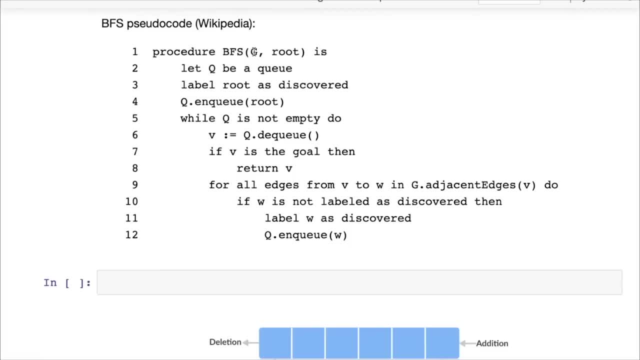 So here's a pseudo code. So if you have to write a function BFS which takes a graph and a root or a source node, So first we say create a queue, So we create, and this is taken by from Wikipedia. 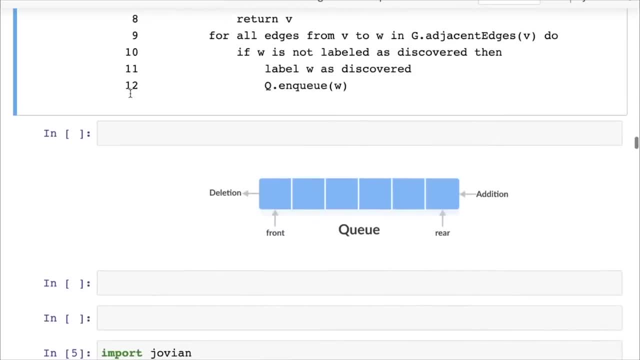 So first we create a queue. and what's the queue? Well, a queue is a very simple data structure. A queue is simply a list and it follows a first in, first out of policy. So when you have a list and you want to add something into a queue, it's 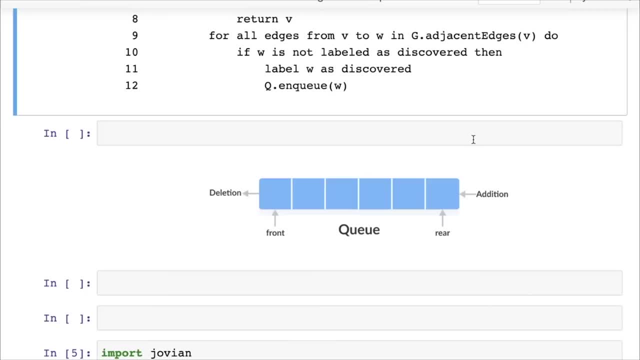 also called NQ, the NQ operation. So when you want to add something into a queue, you add it at the end. Okay, So you have a list and then you simply keep adding things at the end. You just append things at the end of a list, but when you want to access, 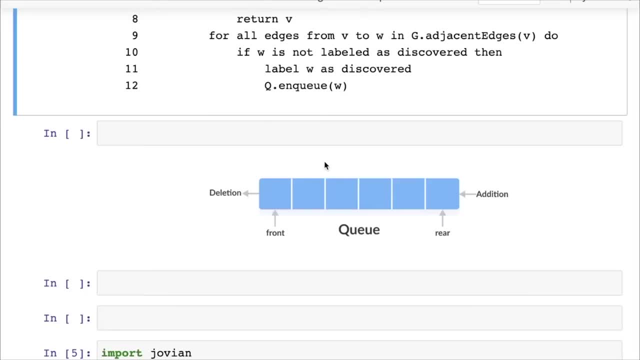 something from a queue. you do not access any value directly. No, you always access the first available value. Okay, You access the first available value. in this case, what? what is called the value in front? and when you access a value, it gets removed. 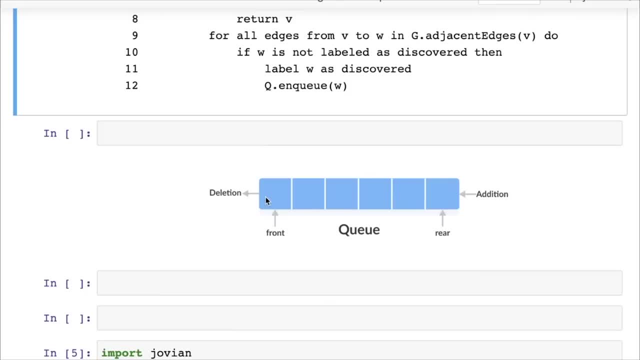 Okay. So in this way you can see that it implements the the first in, first out policy, like if first we NQ one, and then we NQ three, and then we NQ four and then we want to DQ, and when we want to DQ we simply get the first value. that 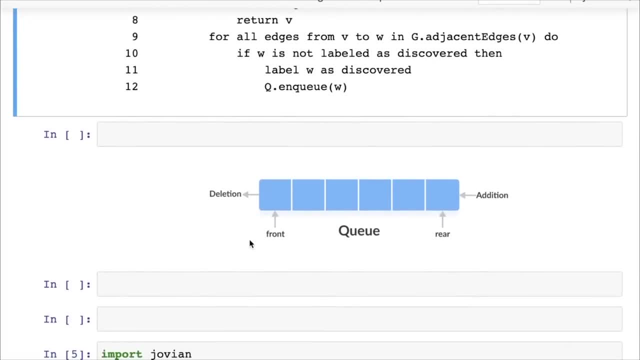 was inserted, which is one, then maybe we NQ a few more numbers, five to seven, then we DQ and then we get back the first value that we had inserted, which is not yet DQ. So then we get back four or whatever was. the was the second. 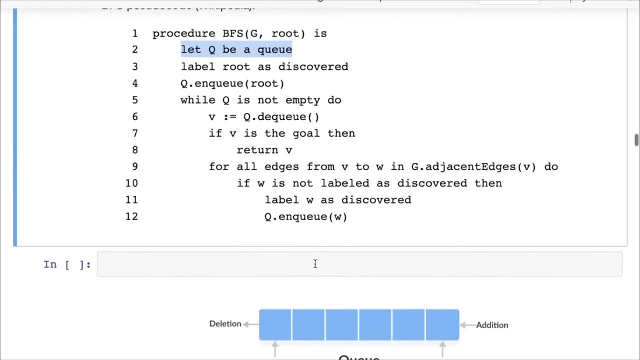 value inserted initially, Right, So that's a queue and we let's see how a queue is useful. So we create a queue and then we mark the label, or we mark root. We label the root node as discovered. Okay, So we need to somehow track which nodes have been discovered or visited. 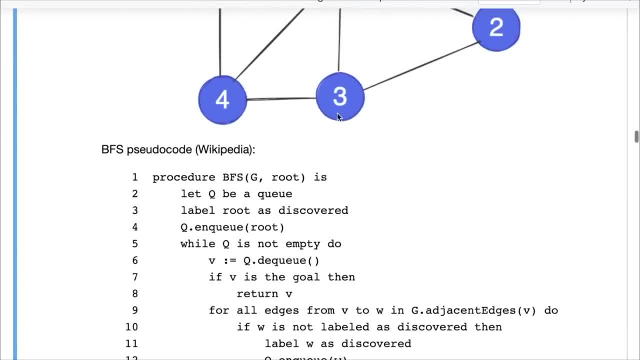 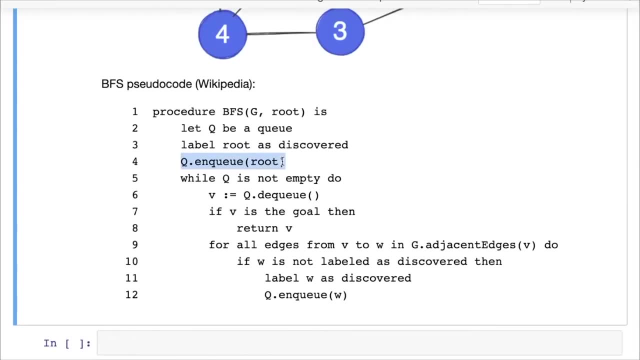 And first, what we'll do is we will mark the root node. So let's say we, starting from the node three, we will mark three as discovered. So three is now discovered, And And as soon as we mark something is discovered, we will NQ it. 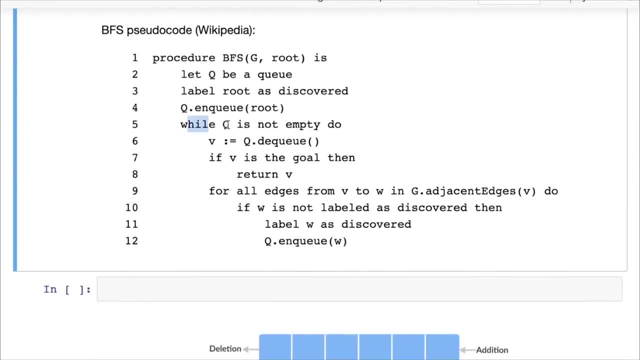 Okay, Then, while the queue is not empty- which is why we have not accessed all the elements in the queue- or while we have not DQ all the elements from the queue, we DQ an element. So we take you the first element which has not yet been removed from the queue. 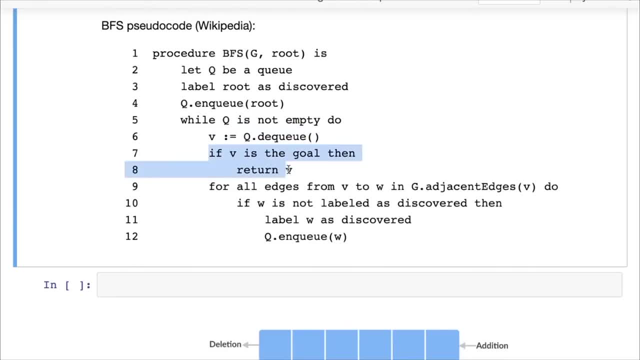 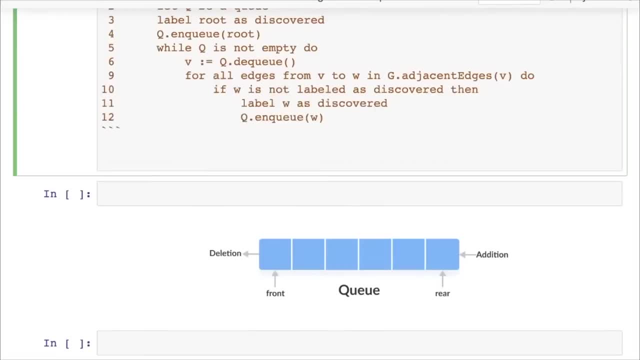 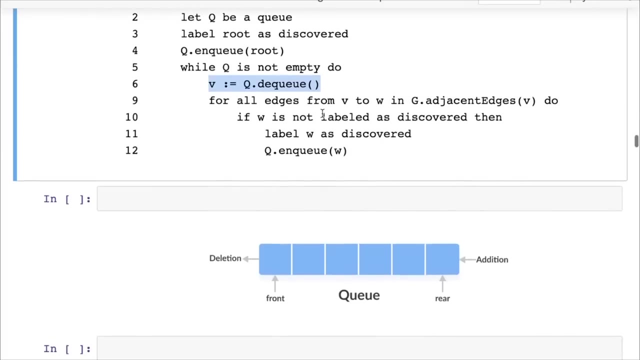 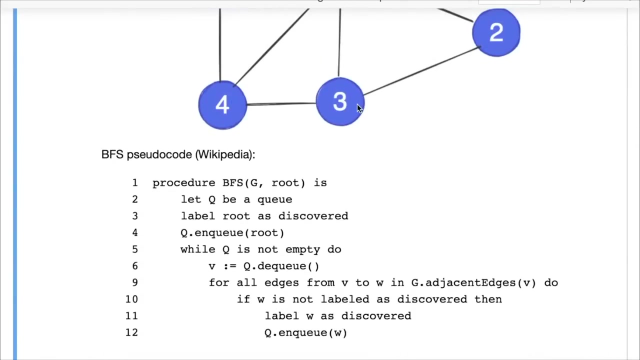 And if you're looking for a particular goal node, then we can simply end there Like we found that node, but we are not looking for a goal node, So let's remove this score. So we get, we get the first element or the first node from the queue which is not yet DQ, and then so, for example, initially we just have three in the queue, so then we get back three. we get three back from the queue, then we check all the edges for three. 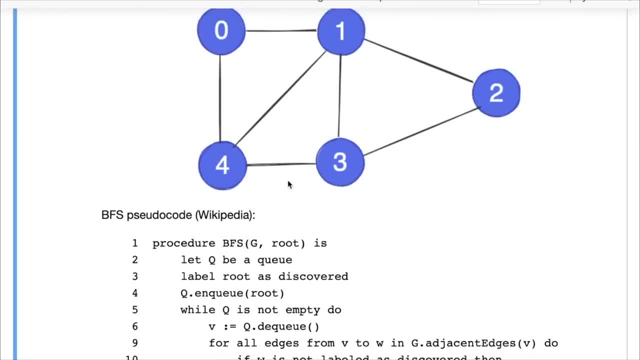 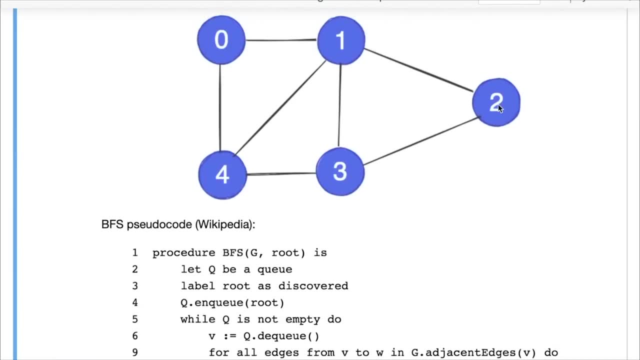 So we check that three is connected to one and three is connected to two and three is connected to four. So we see all the edges for three And if The other End of the edge we check for each node, let's say the other end of this edge is two. 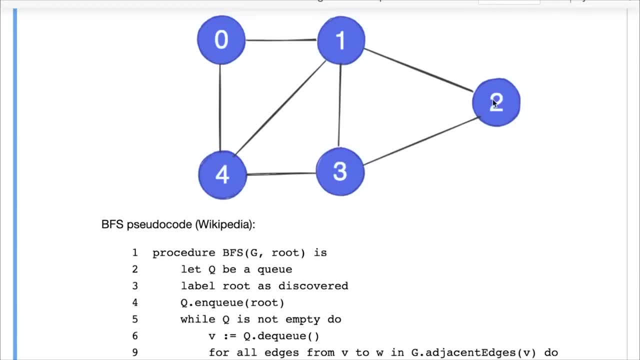 We check. if two is not yet discovered or not yet visited, then we NQ two into the queue. Similarly we check for one, and if one is not yet already discovered, we NQ one into the list. Similarly for four, we NQ four into the list. 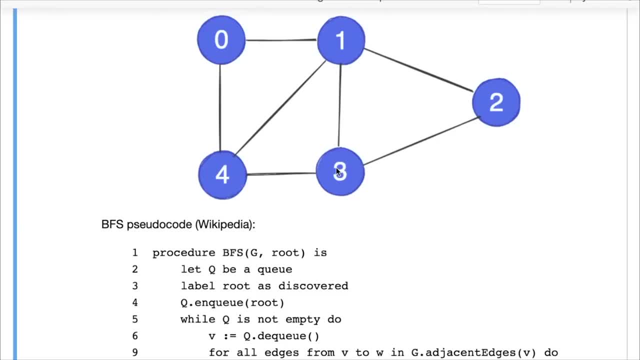 Okay, So we have DQ three, So three is no longer in the queue. or we've moved forward or we're no longer going to get queue three out of the queue. but now we've NQ two, one and four, and two, one and four. 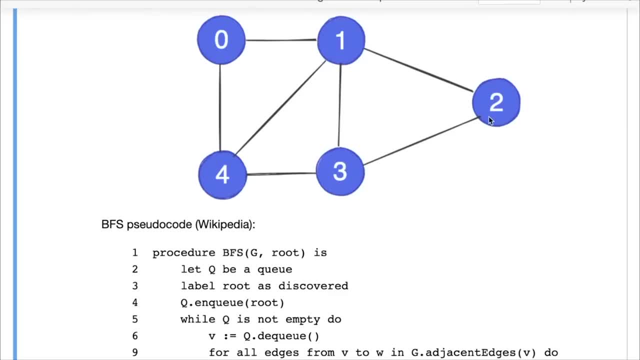 We now understand they are at distance one. So when we pick the next element of the queue, we DQ the next element, the first in the first and first out, we get back to and then we mark two is visited Great. 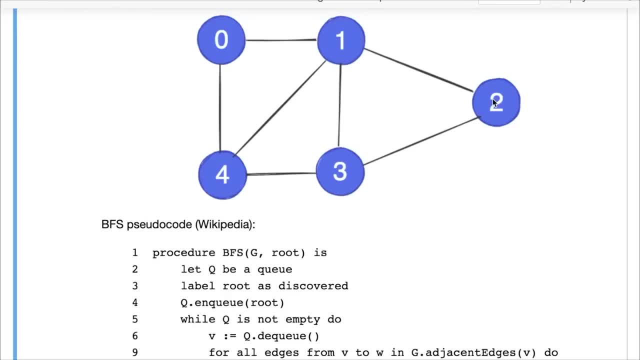 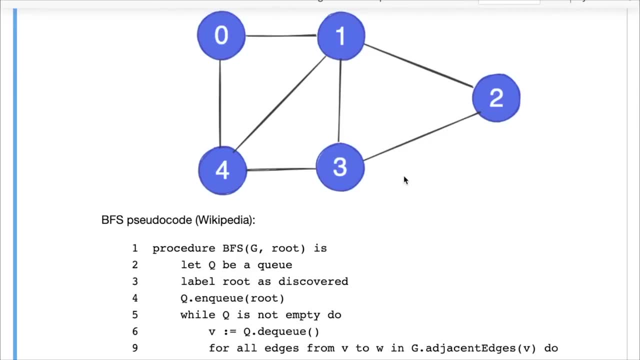 Now we visited two. Oh no, we, we. we mark as soon as we are adding something to a queue, we also mark them as visited, because we've identified that two, one and four are all at distance one from three and we've added them to a queue. 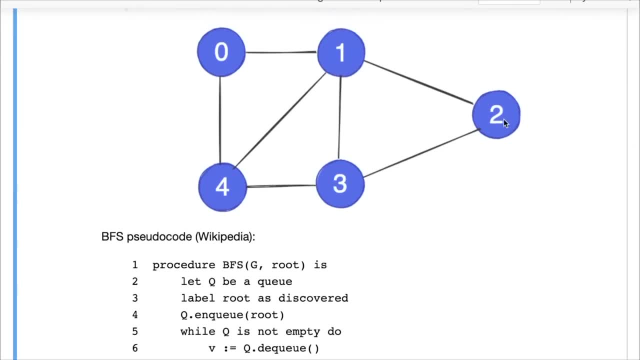 So we mark them as visited. Now when we get two out of the queue in the next iteration we check if there are any nodes which two is connected to. those are not yet visited. So two is connected to one, but one is already visited. 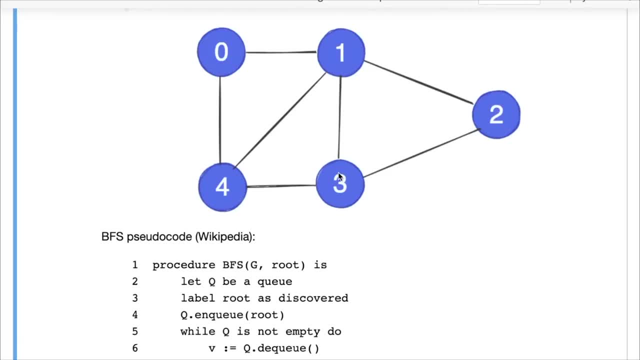 So there's no need to NQ it again. And then two is connected to three, but three is already visited, So there's no need to NQ it again, And so we Just move forward. Then we go to one, And when we go to one, we realize that zero is not yet visited. 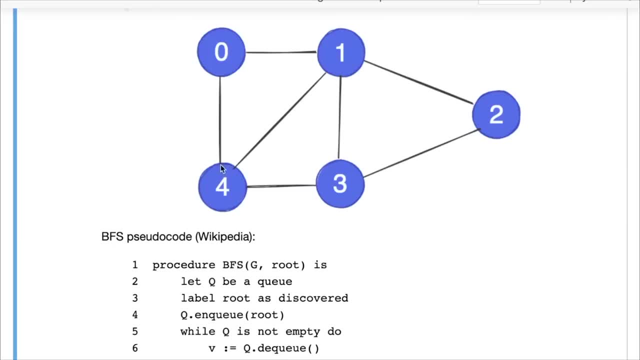 So we NQ zero four is visited, So we don't NQ four. Okay, And that's how we proceed. So now what you should do is you should draw this on a piece of paper and work it out. Just write on a piece of paper. 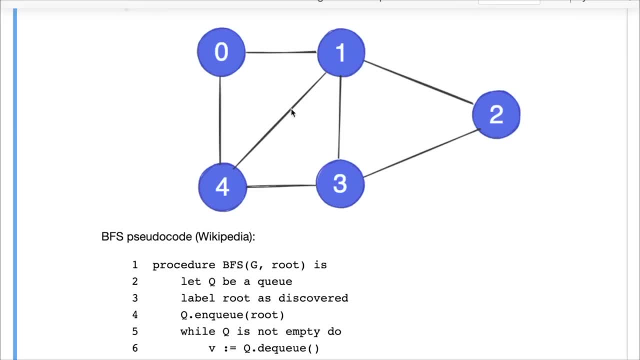 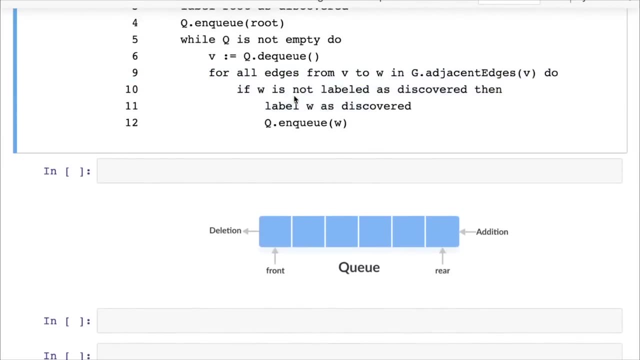 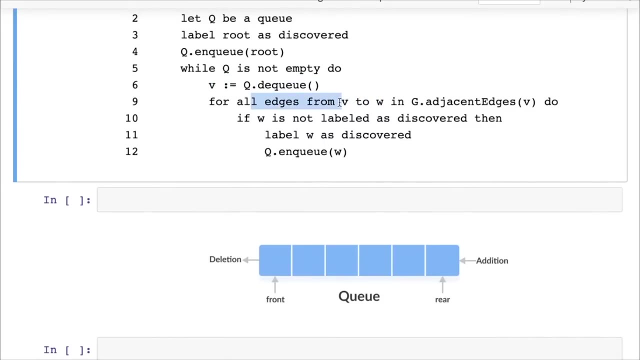 What would be the first element that gets inserted, and what will be the elements that we will insert into the queue, et cetera, et cetera. But This is the algorithm here, Exactly what we, what we just discovered. So we DQ in a vertex or all the edges that start from the vertex V or the node V. 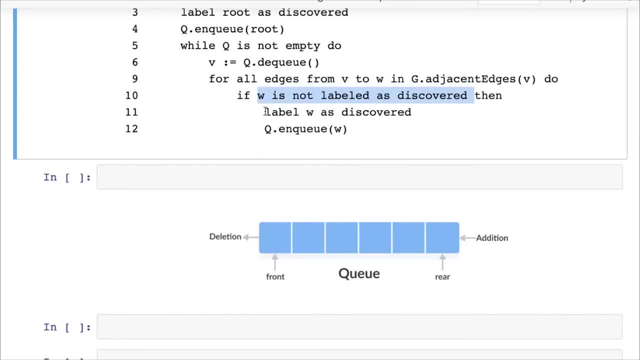 If the other end of the edge is not labeled at discovered, then market is discovered and NQ it into the queue. Let's implement this. Let's see if we can implement this life. So we are implementing BFS, where we will get a graph and a source node. 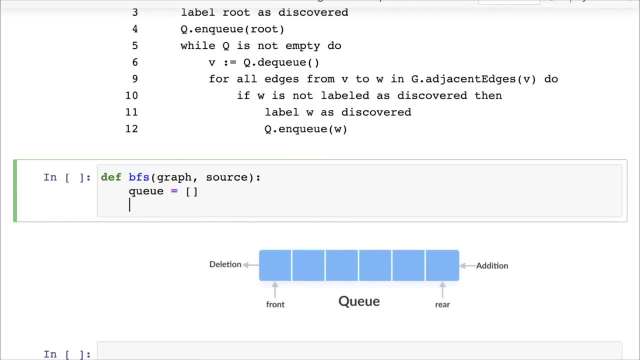 The first thing we need to set up is a queue, So the queue is empty. Then we set up discovered, and discovered will be false initially and it will have the length. So we want to market false for all the elements. Okay, And remember now we can use this notation here, because false is an immutable value. 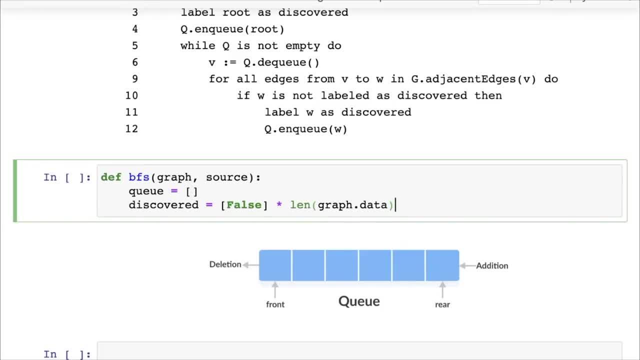 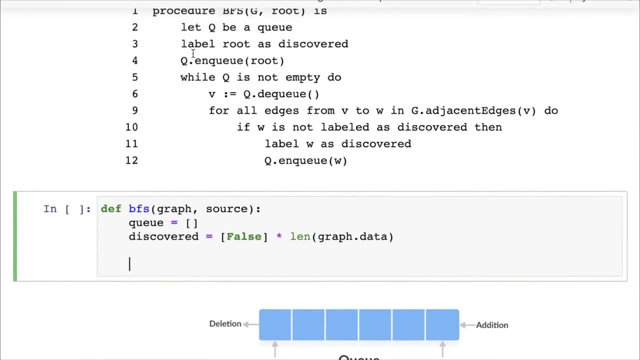 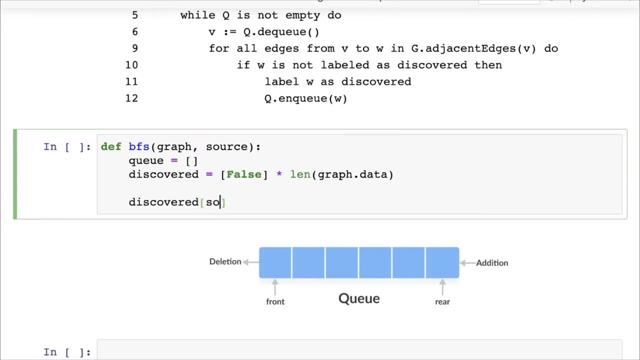 So it doesn't matter. So so we don't really need to use the range or the list comprehension notation here. Okay, Then here let's come here. so we mark the label root as discovered. so discovered of source. let's just call it root. 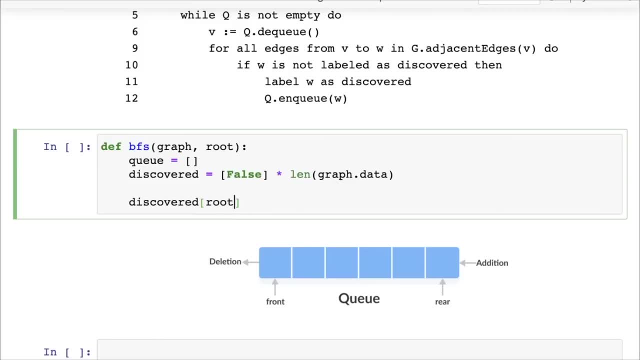 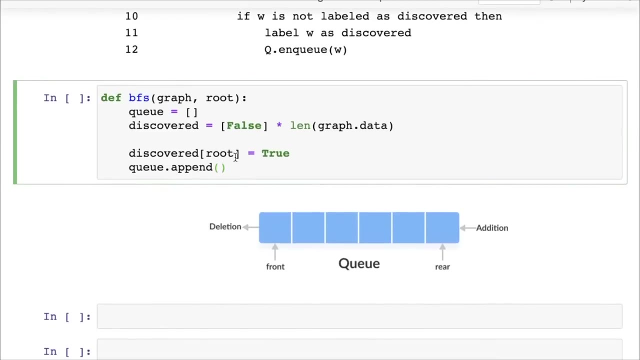 So that we don't get confused with the terminology. So we mark discovered of root as true Great. Then we insert or we NQ the root. So we we Okay, Type Q dot append. Now NQ simply means adding something to the end, and you know how to do that in a list. 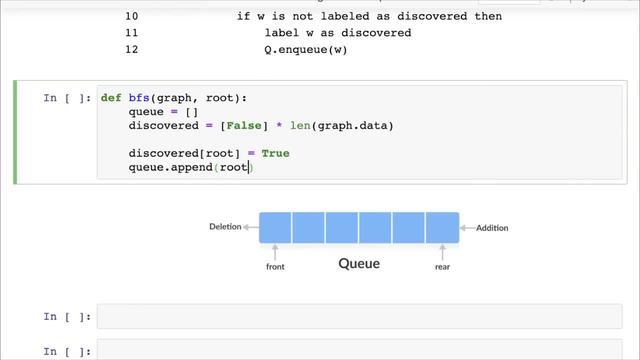 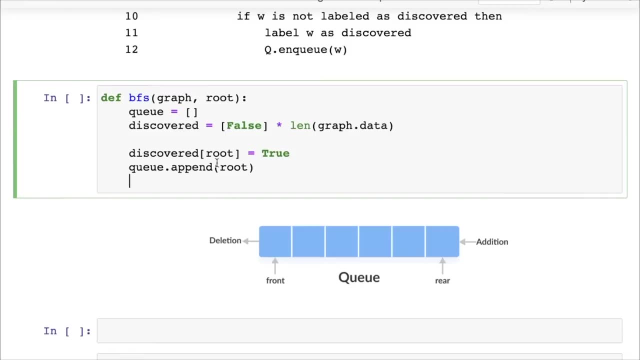 You simply call Q dot append, So Q dot append root. Great Now, Python lists by default do not support a DQ operation, So what we will do is we will set up an index which will track the first available element in the queue. 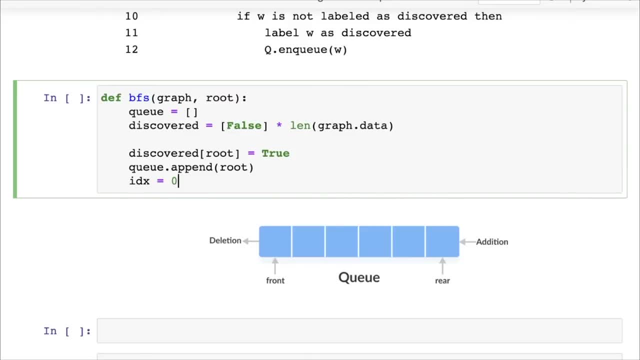 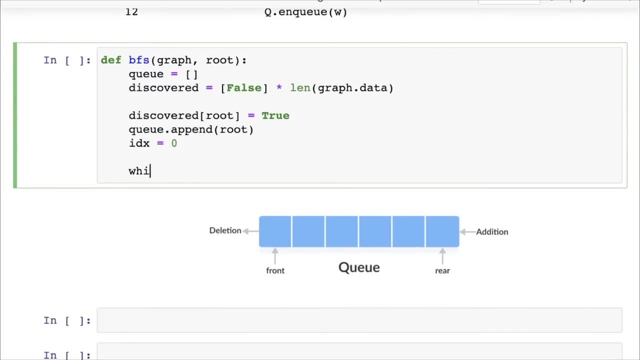 Okay, So whenever we DQ an element, we will increase the index So that we move forward. So here we have the index IDX equal to zero. So now, while there are elements in the queue, which means while the next available index is less than the length of the queue, 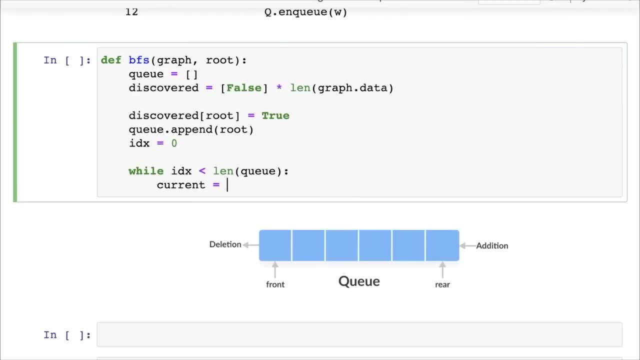 First we will get the current or we will DQ. So DQing simply means getting the car getting the first in element, the element that was most recently inserted and has not been DQ. So we get current. So the current is Q of IDX and then we can also increase IDX. 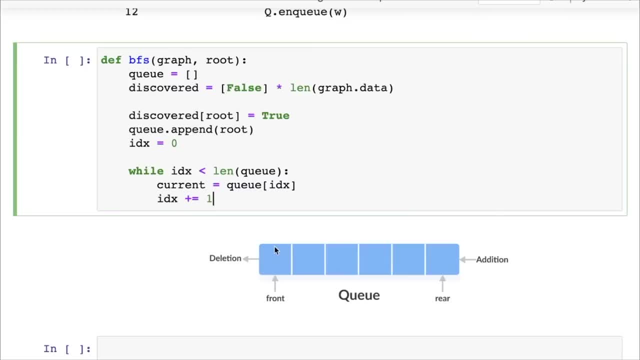 So as soon as we DQ something, we update the index. So you can imagine that the index starts out here and when we DQ this or delete this, and we get that value out, and then we update the next to the next position. 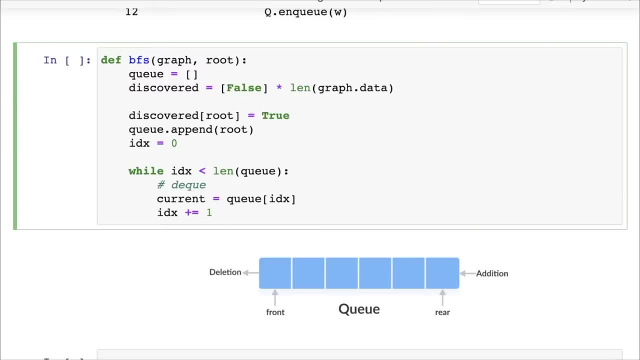 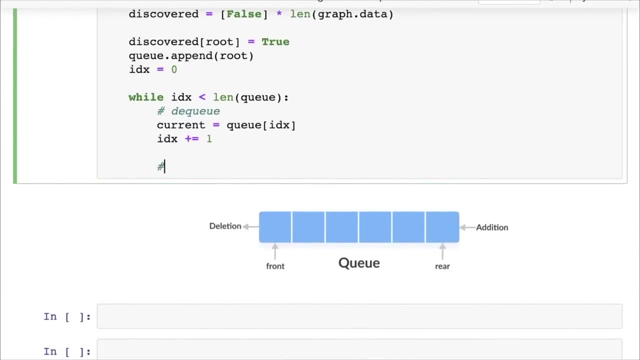 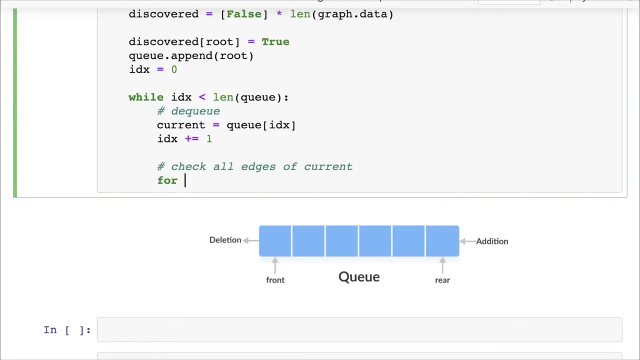 Okay, So now we have the current, this is a DQ operation. Then what do we have next? Now we want to check all the edges Of current right. So we are going to say for, so remember, we have the adjacency list representation, so we will get for node in self dot data current. 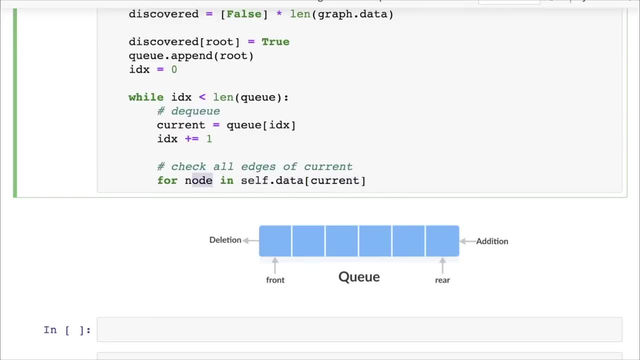 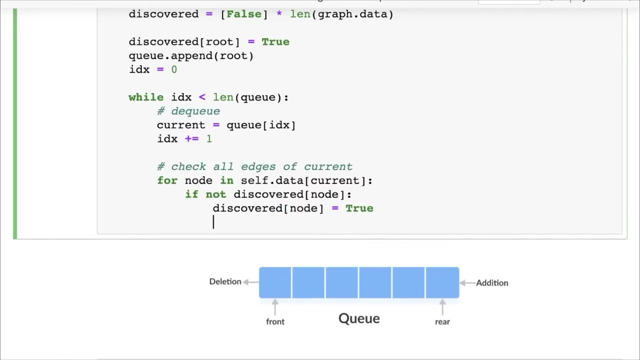 So self dot data current contains a list of all the nodes that are connected with the current node. So for node in self dot data current, if not discovered node, So if you have not yet discovered The node, then we first marketed this as discovered and then we added to the queue. 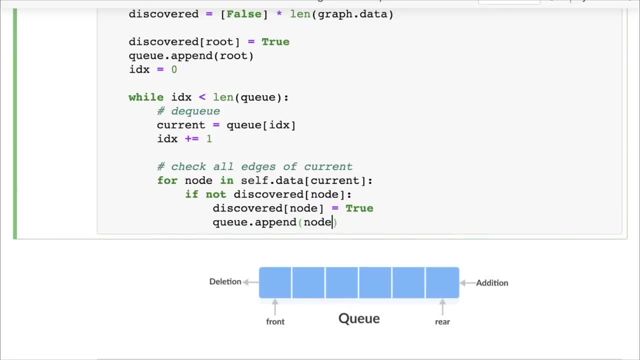 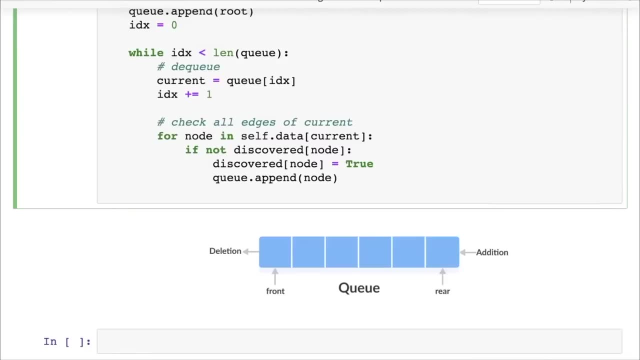 So we do queue dot append node. Okay, So what you end up with this way is: first you have the source that got added to queue and then we inserted all the inserted all the nodes which were at a distance one from source. 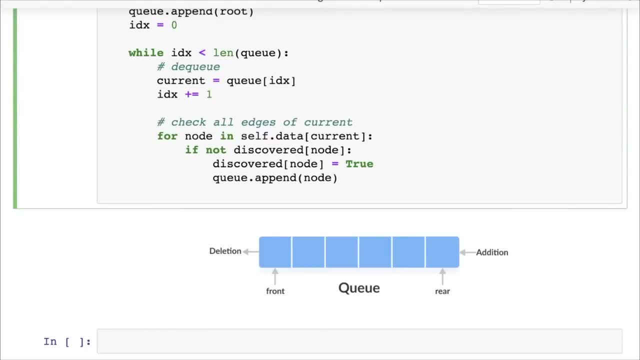 And then we insert. then, If you follow the trajectory, we'll see that we will insert all the nodes that are at a distance two from queue, and so on, Right? So ultimately, when we end up with this entire process, we will have the queue and the queue will contain the list of nodes as they would be visited in a binary in a breadth. first search: 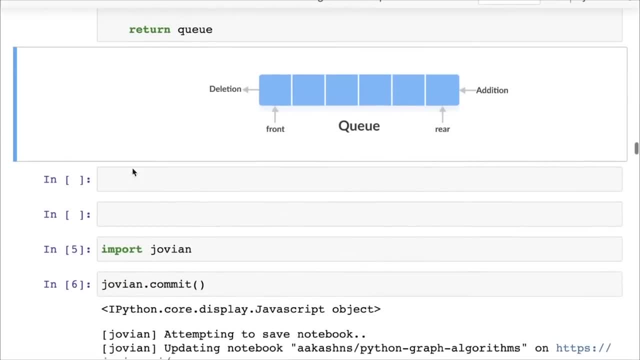 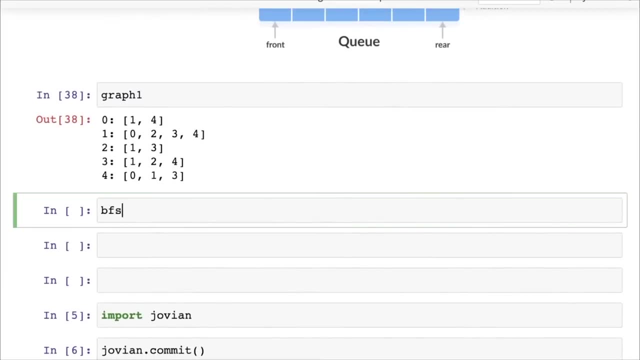 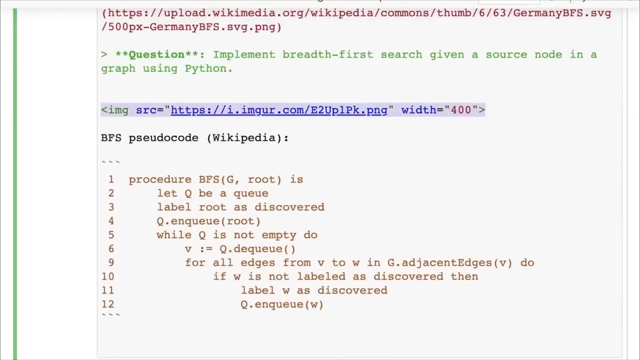 Okay, So we can simply return the queue here. So let's try it out. So we have graph one And let's call BFS, And graph one is this graph, So let's grab this image as well. So let's simply copy the code for the image and come down here. 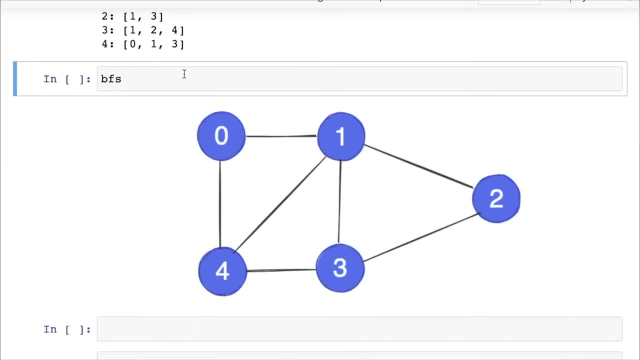 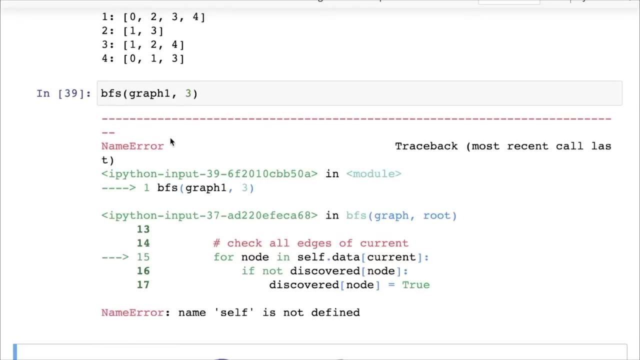 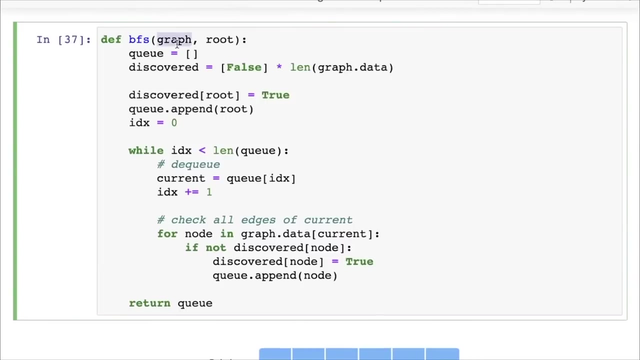 Let's come down here and put the image here. Okay, Let's call BFS on graph one, starting at the node three. Okay, Of course, this should be called graph dot data. So, because Graph is the graph that we're working with, 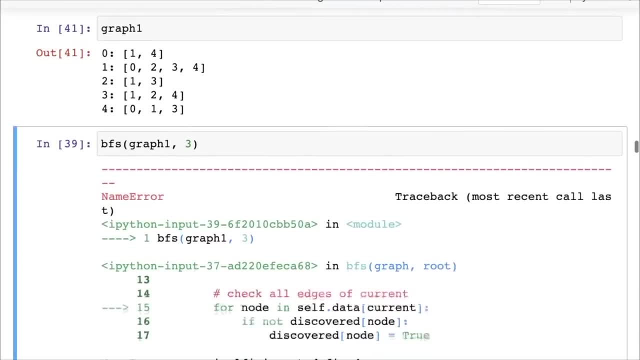 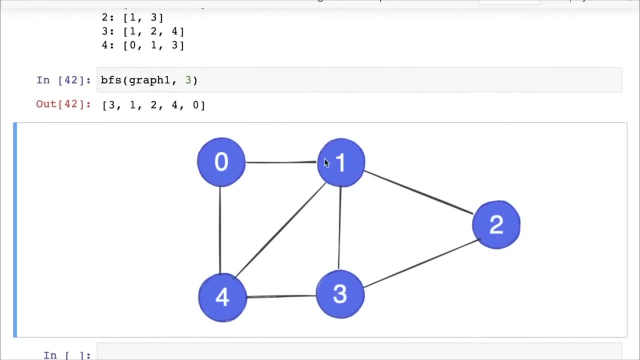 So we need to check graph dot data here. Okay, So we start out with the note three, and you can see that three first causes one, two and four to get inserted, And then one causes two to get inserted. Okay, Now that's BFS for you. 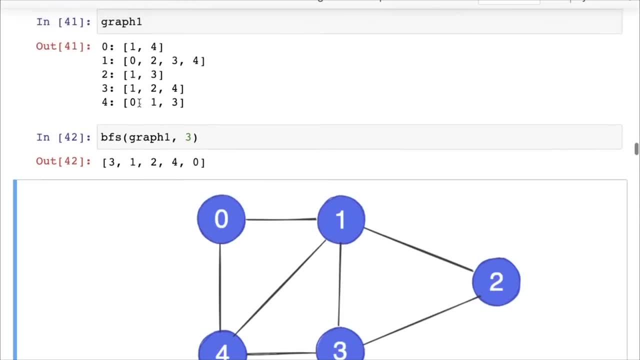 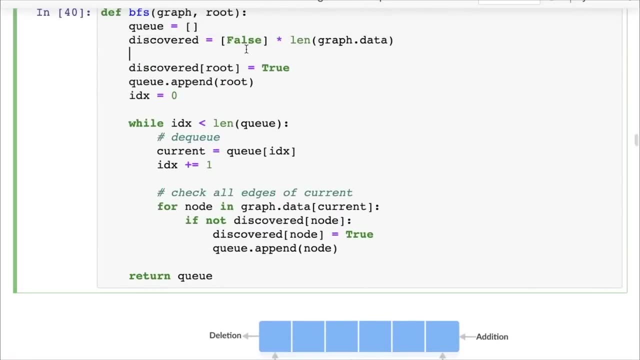 It's pretty much done at this point, but what would also be helpful is maybe to keep track of what is the distance of each node right, So we can also track. We can also keep track of a distance. So, let's say, we have a distance which we initially said to none, or, yeah, which we initially said to none. 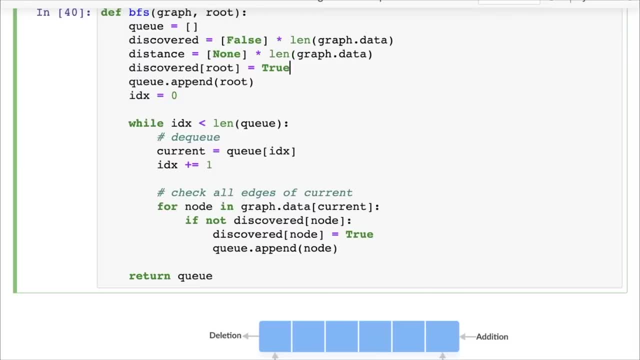 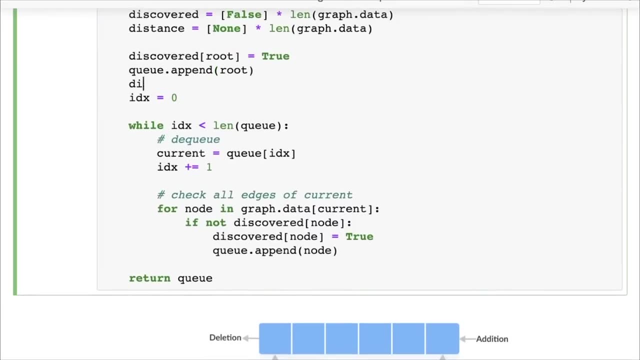 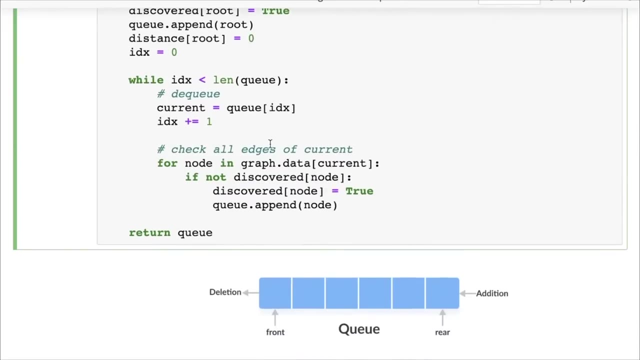 And we will track a distance for, for formation, for each node. So we have the distance here And initially we are going to set the distance for the root to zero, of course, because the root is at zero distance from itself And the distance here means the number of edges, right. 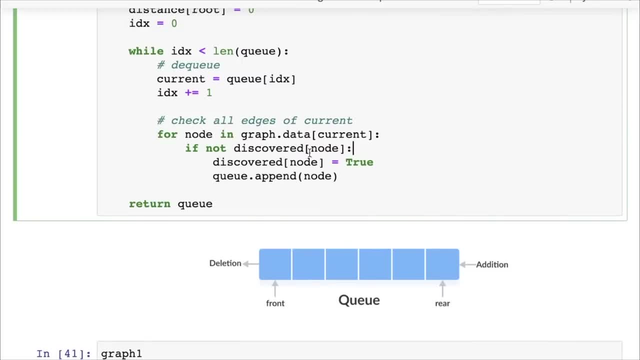 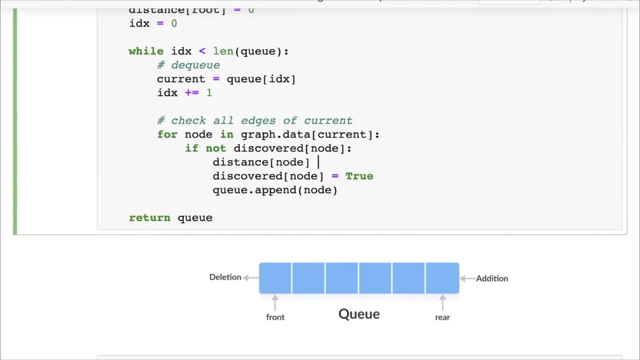 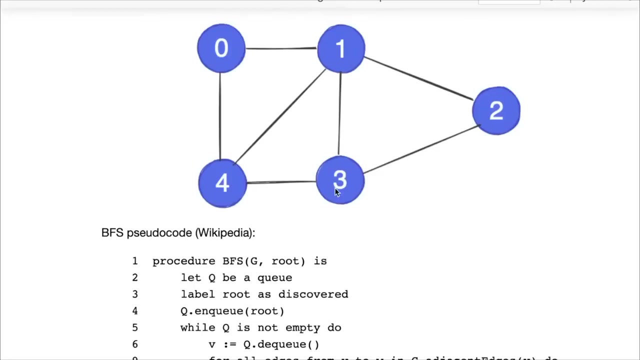 Then when something is discovered, so when we are discovering a node and that node was not already previously discovered, that means that the distance for that node is one more than the distance for the current node which caused it to be discovered, right? So the distance for so, for example, if you're starting with three, the distance for one is one more than three, which caused one more than three. 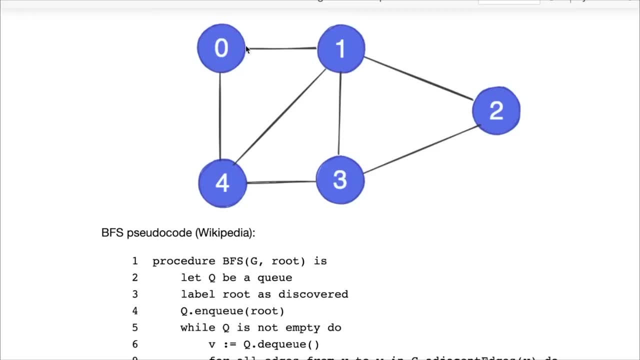 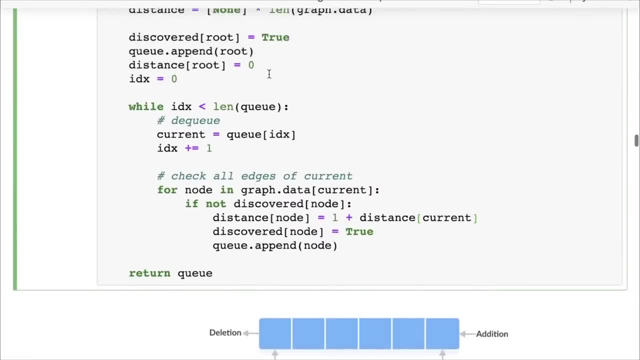 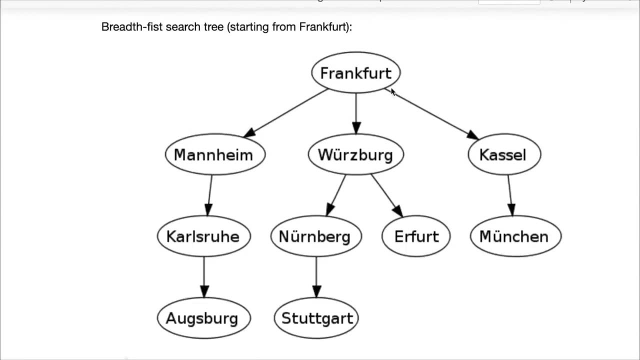 So that's the distance. Great We've. we've now also tracked the distance. One other thing that would be nice to have is what is called the parent. You, if you see, if you go back here, you can see that it would be nice to know what led to calls through being discovered. 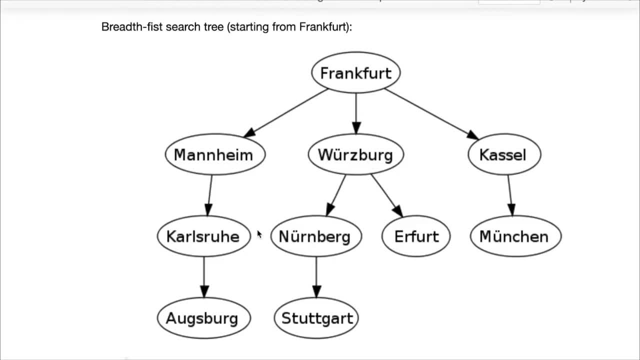 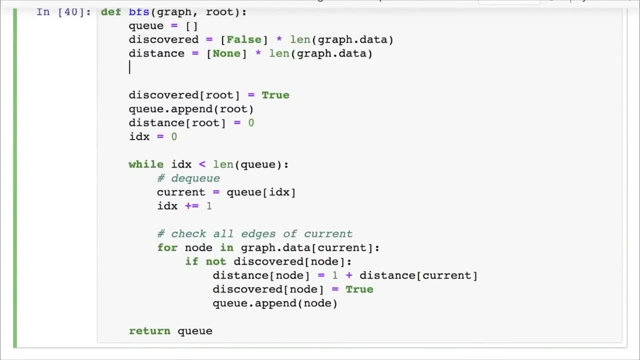 Was it Manheim? was bug or castle, so that we can work our way backwards and find a path from Frankfurt to Karlsruhe. Okay, So for that, what we can do is we can keep track of a dictionary, of a list called parent. 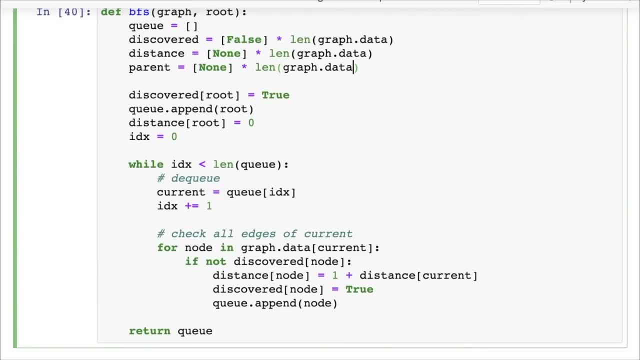 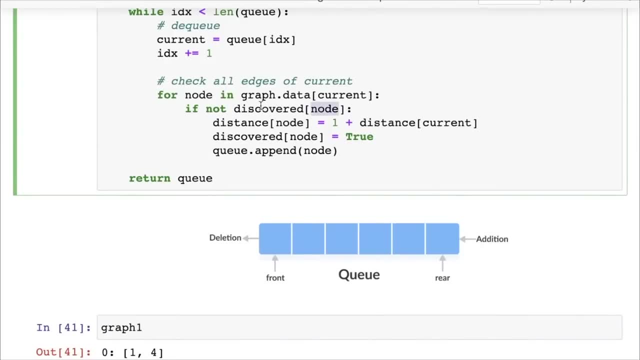 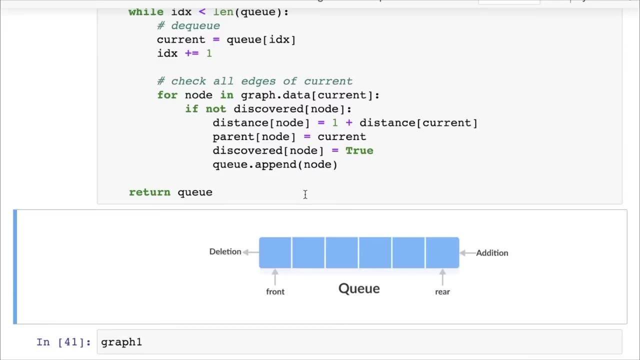 Once again, we will have no parents by default, So parent none And whenever we find a node and that node was not already discovered, then we can set the parent of that node to the current node which caused it to be discovered. Okay, 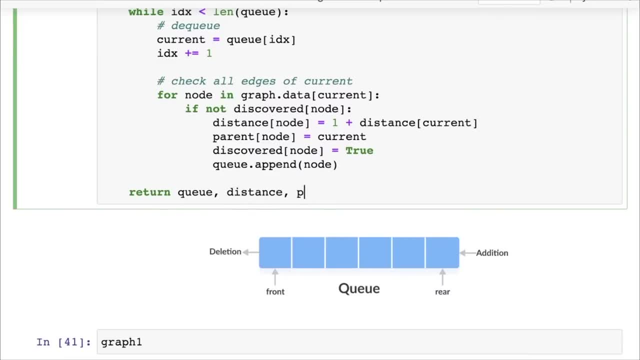 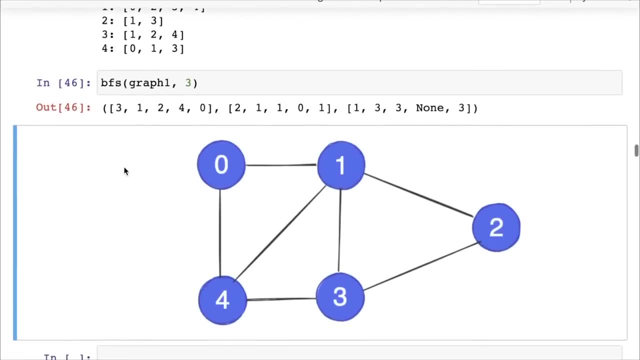 And now we can return from the queue, the distance and the parent, So let's see if that works. Okay. So it seems like now we have these are. this is the. this is the order in which the nodes are being visited. 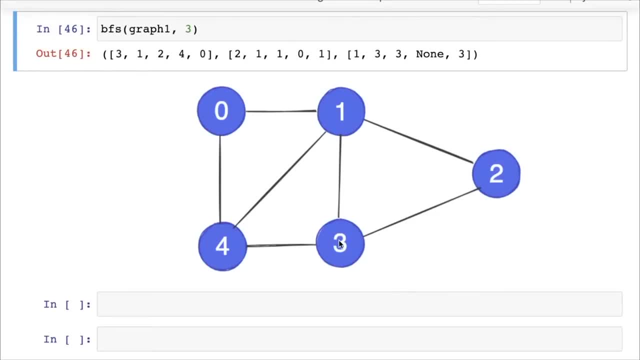 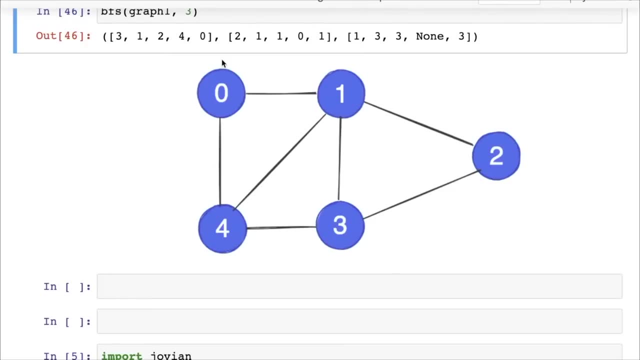 So you can see that three is the first node to be visited And three has. and if you want to check the distance of three, you can see that the distance of three Three is zero. So this is distance is given in the order of the nodes in the order. 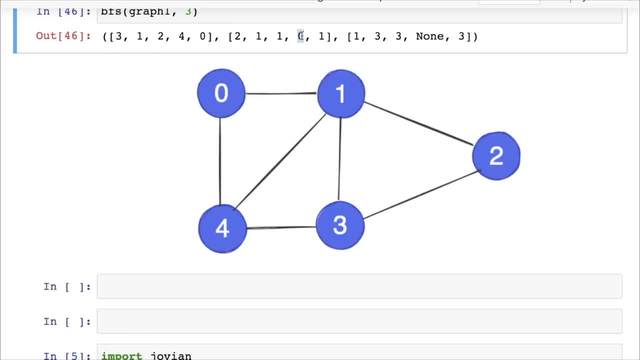 of the original numbering of the nodes. So you can see that three is at a distance zero from itself. obviously, then you have one, two and four. Now, if you want to check the distance of one, just check the index number one here. 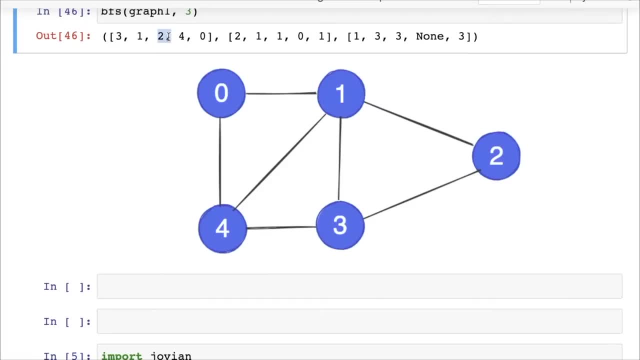 So one is at a distance one. If you want to check the distance of two, now that is at a distance of one as well- You can check here. and then you want to check the distance of four. Four is also at a distance of one right. 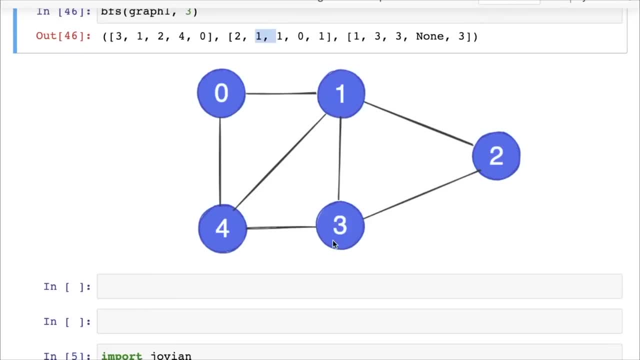 So all of these, One, two And four are at a distance of one from the root, node three. And also you can see here that the parent of one, remember these are zero. one, two, three, four. these are the indices of the nodes. 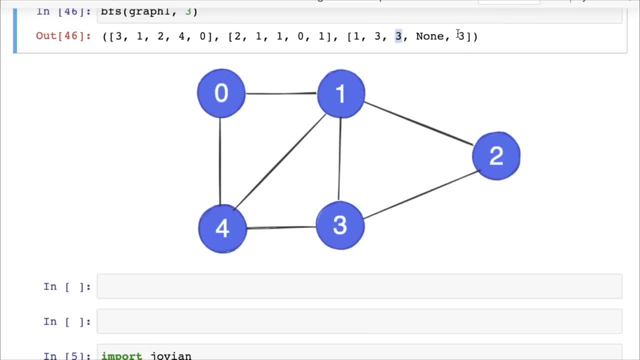 So the parent of one is three and the parent of two is three as well, And the parent of four is three. three itself does not have a parent. That's why this is none. And finally, the last node we visit is zero, and it is at a distance too. 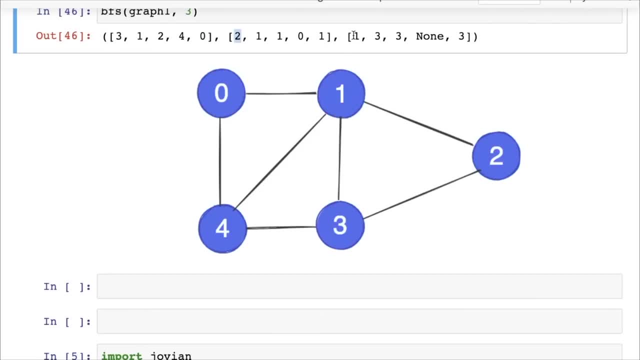 And you can see it, as the distance here is indeed the highest, and the parent for zero is one right. So, because one was the first node that caused zero to be visited, it could have been four, two, but in this case, just how we implemented it, one was the first node which caused it to be visited. 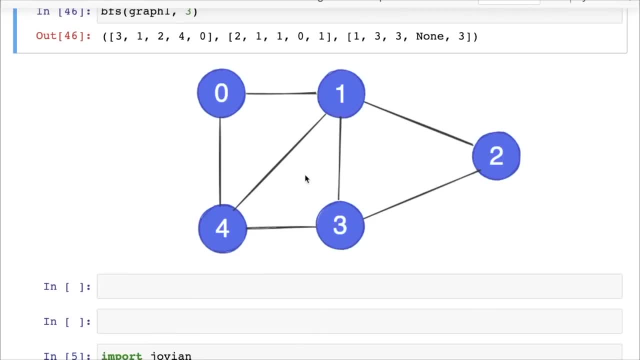 So one is the parent of zero. So if we now want to find the path from three to zero, you can look at the parent of zero, That would be one. And then you can look at the parent of one, that would be three, and we're done. 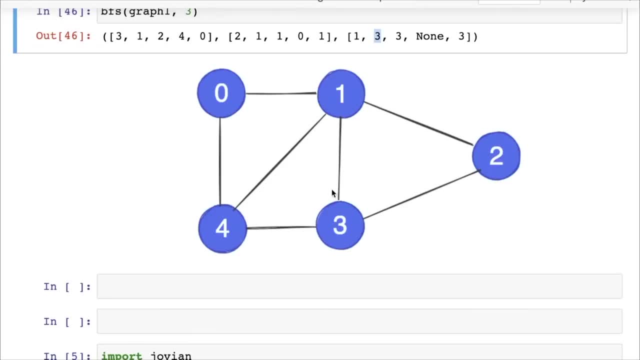 So we can walk backwards from the target. We can keep checking the parent after parent of the target And that will give us the entire path. So now we have the path, we have the distance and we have the order in which these nodes will be visited. 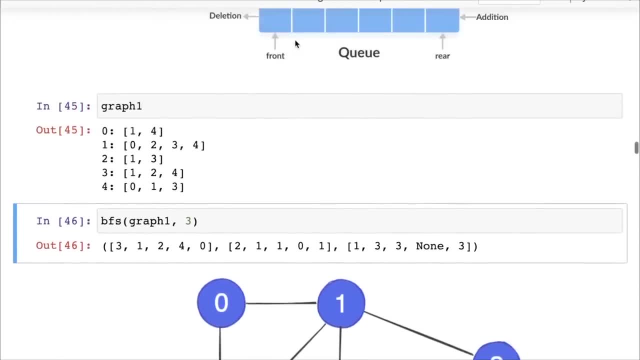 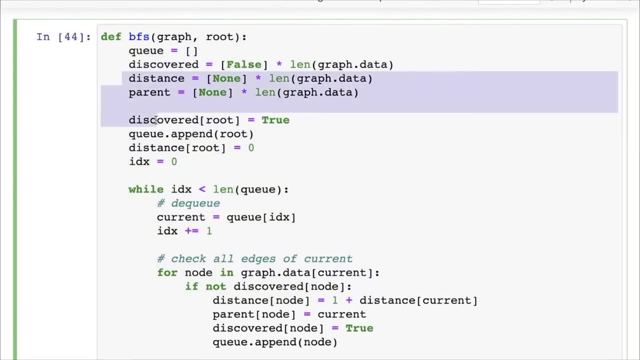 So you may get asked: breadth first search in all these different variations. but roughly this is what the code looks like And you can see here that the code is not too long. Now we have created all these additional, additional lists, but you don't really need them. 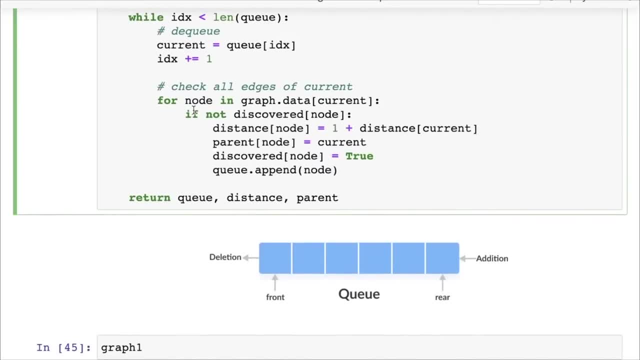 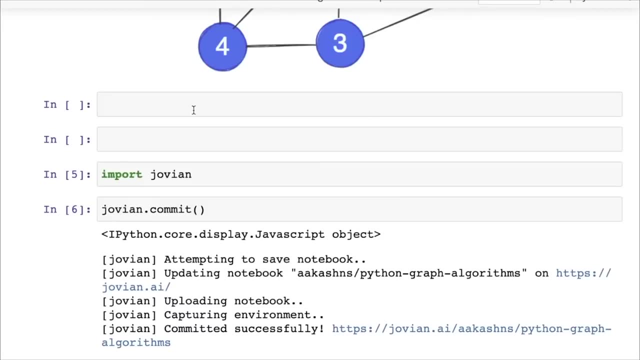 So the code is about 15 lines of code, 10 to 15,, 12 to 15 lines of code, not more than that. So that's BI. Again, if you're working on a BFS problem, it always helps to first state it in simple words and work it out with an example and then start coding, so that you do not make mistakes while coding. 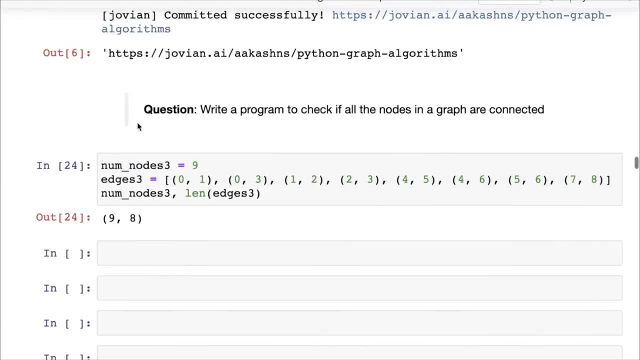 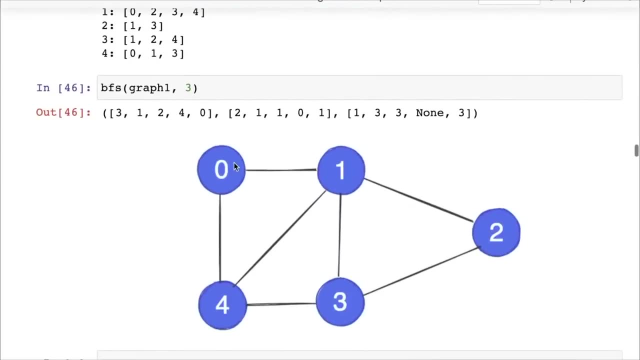 Now, one question that you can work on is to check if all the nodes in a graph are connected. This may not always be the case, but, for example, here you can see that all the nodes in the graph are connected, but some. 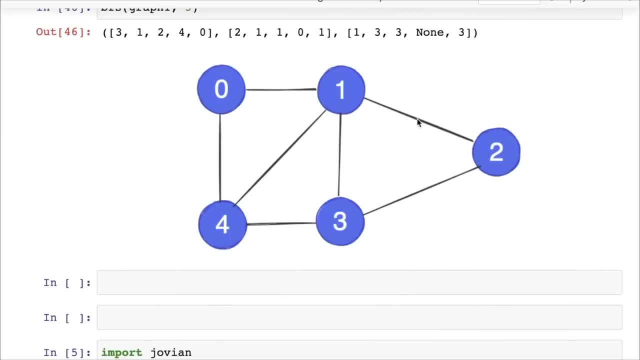 Sometimes you may have a situation where some nodes are not connected. For instance, if these edges- one, one, two and three to one present, then two would not be connected to zero, And maybe two is connected to five and six, et cetera. 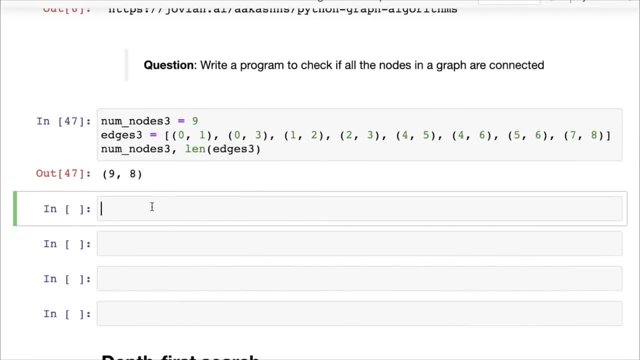 So here is one graph where not all the nodes are connected to each other. You can see that there are nine nodes but there are only eight edges, And if you look carefully you will see that zero, one, two, three, zero one, two, three are connected, but there is no connection from these notes to four. 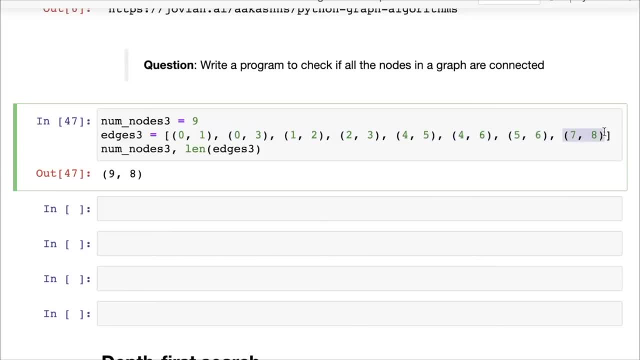 So four, Five, six are then connected separately, and then seven, eight are connected to each other but not to one another, Right? So can you use breadth first search to determine if all the nodes in a graph are connected? I would reckon. 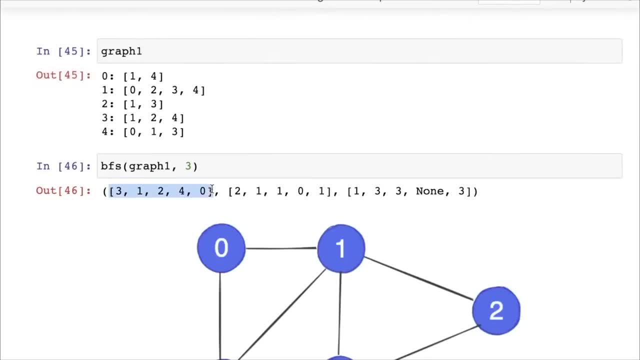 Yes, Look at this queue Now. this queue gives you all the nodes that, starting from the source node, are connected to the source node by zero, one, two, three or so many steps. If something is not connected, it will not show up in the queue. 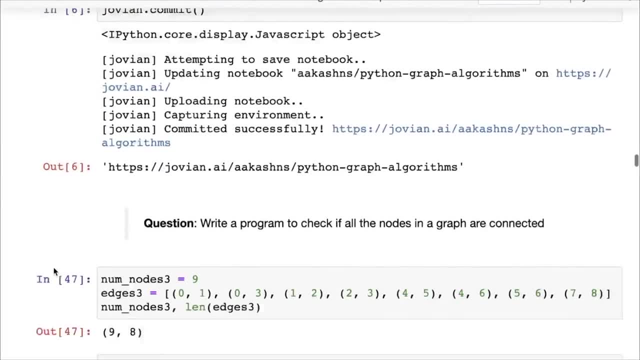 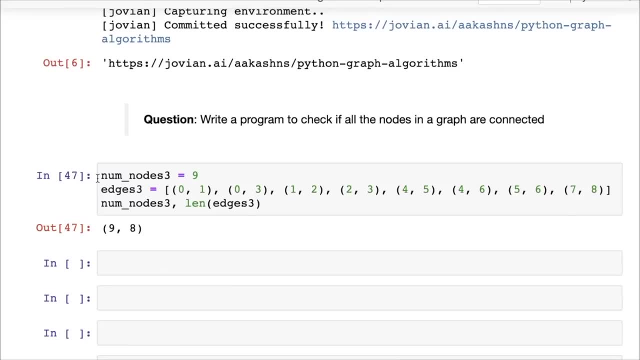 So you can simply check the length of the queue and see if that is less than the total number of nodes And then use that to determine if all the nodes are connected or not. Now another related question that you may get asked is to find the number of connected components in the graph. 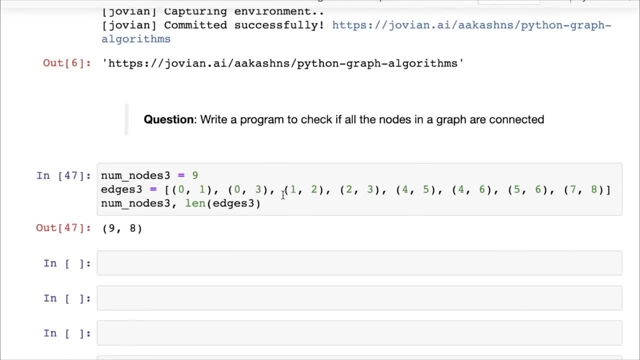 Now, what's a connected component? If you take a set of nodes that's connected, that's one component. And if you remove that, then you look at the next set of nodes that's connected, That's two components. If you remove that, then you take the next set of. 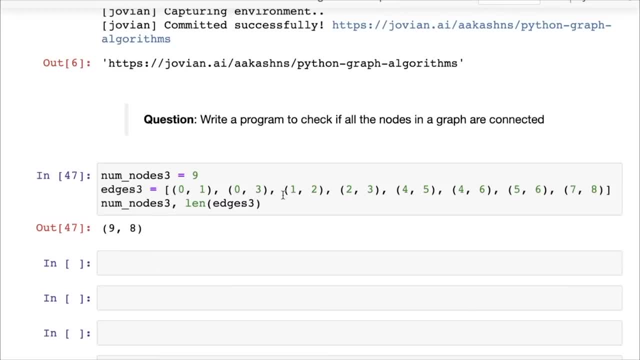 Nodes that connected, that are connected, that and that gives you the third connected component, and so on. So in this case, for example, you have: this is one connected component. You can check by drawing the graph and then this would be one connected component and then these would form one connected component. 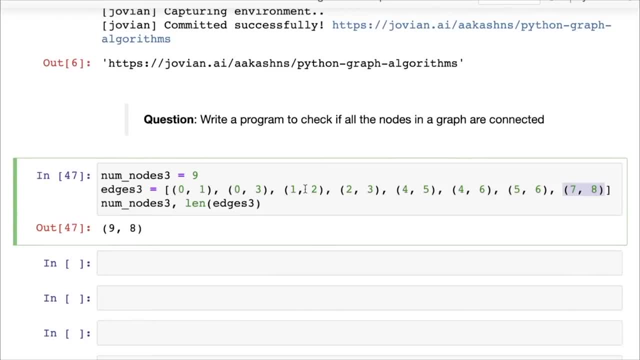 So zero, one, two, three would be one connected component, Four, five, six would be another and seven, eight would be another. Can you find the number of connected components, or even can you list all the connected components of a graph Using BFS? 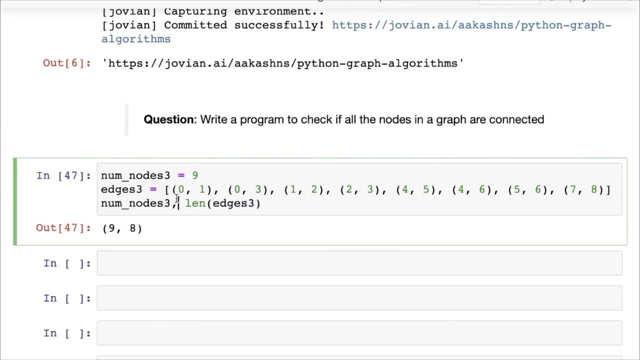 Yes, you can. Again, a very simple way to do it is just pick the first node, perform BFS from the first node. that gives you the connected component that contains the first node. Then find the first index, which is the first node which is not yet visited. 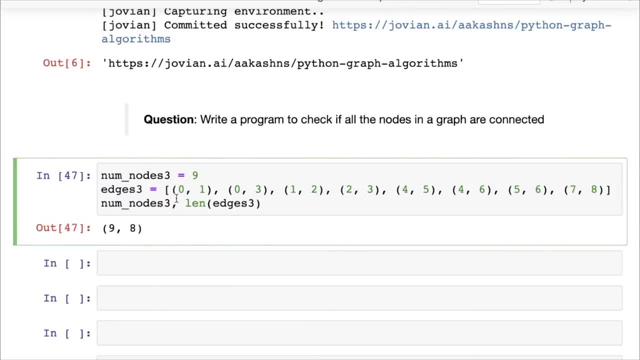 Start BFS from that node Now. that will give you the connected component for the second node, and then find, and then keep doing, keep repeating this till all the nodes have been visited. Okay, That's another question that you might get. Find the number. 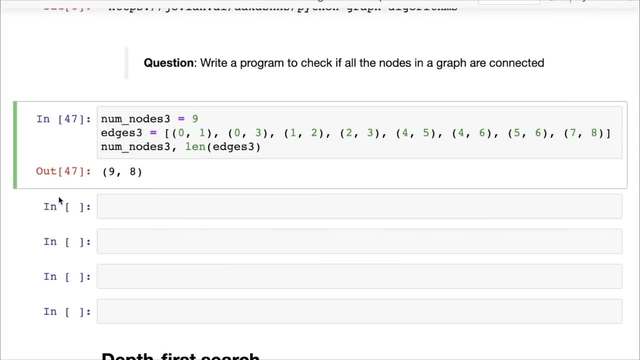 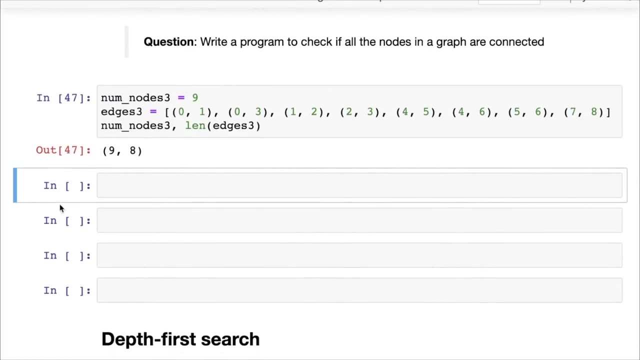 Of connected components or find a list all the connected components in a graph. The BFS is a very versatile algorithm that can be applied to solve pretty much most graph problems that you may get asked in an interview. So do do work on a few BFS problems and get some practice with it. 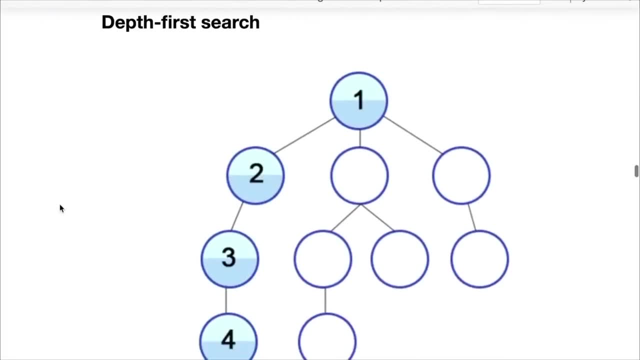 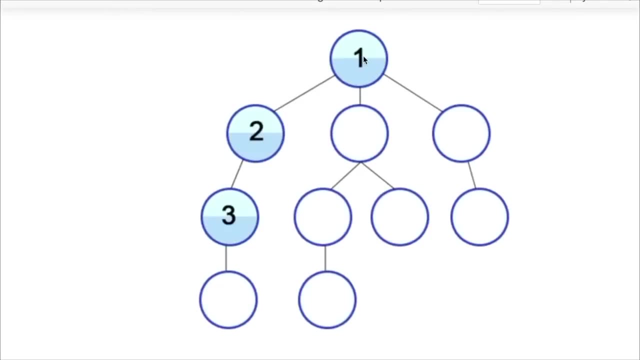 Okay, Now, another way to work through a graph, to look through a graph, is what is called DFS, And this is the way in which you would normally explore a maze, Where you start out in one direction and then keep going. So, for example, we started out here and then we kept going till we hit an end. right? 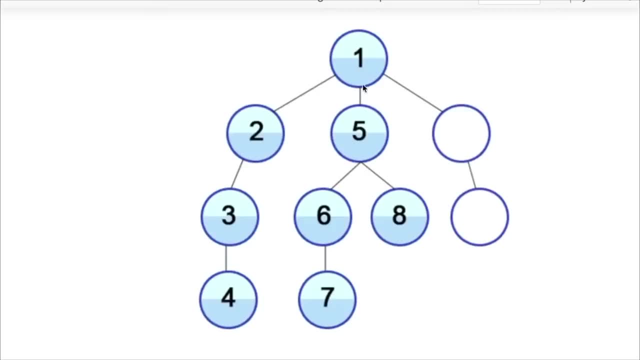 So you can see here that we kept going until we hit an end, and then we turned back, and then we tried the next part, and then we turned back and tried the next part, and so on. So we go like this and then we turn back. 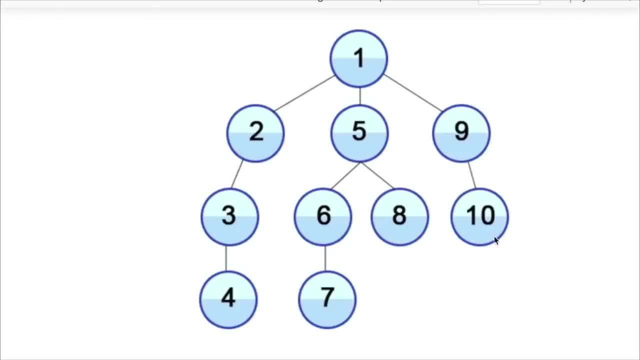 We try five, go like this, turn back. We try eight, Then we turn back, try nine, 10.. Okay, That's another way to go about it, And it's some cases. in some cases, BFS makes more sense. in some cases. 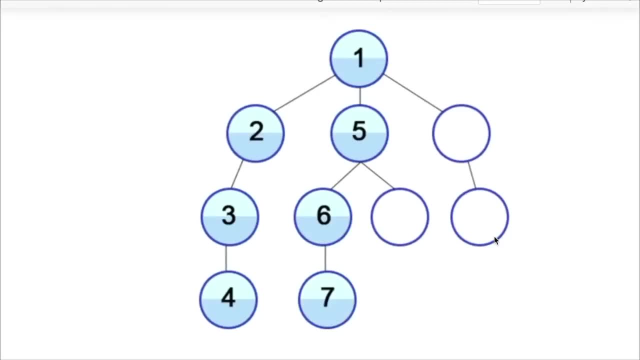 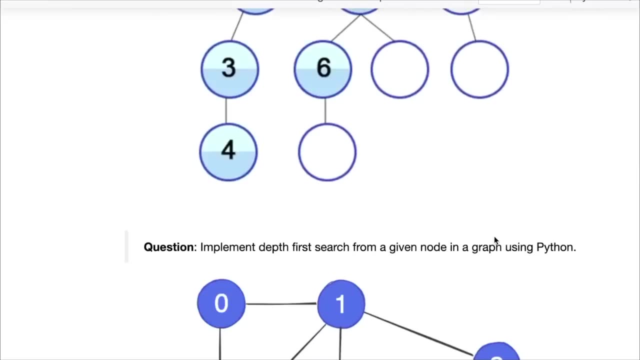 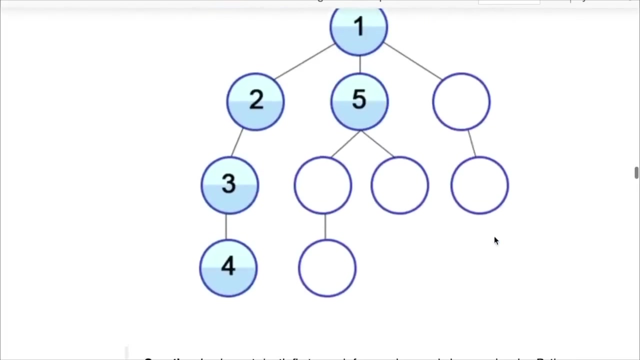 DFS makes more sense And you can in most cases, both of them work just fine for most problems, So you can implement either one when you are faced with a graph problem. So let's implement DFS or depth first search. Now, here is a depth first search. 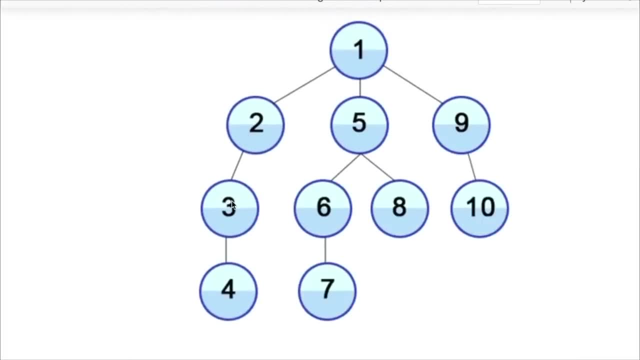 It's pretty straightforward. You have you pick a node and then you pursue the node, and then you next node, then the next node, and so on Among the edges. you pick one node And then once. once you've exhausted the path along one edge, you 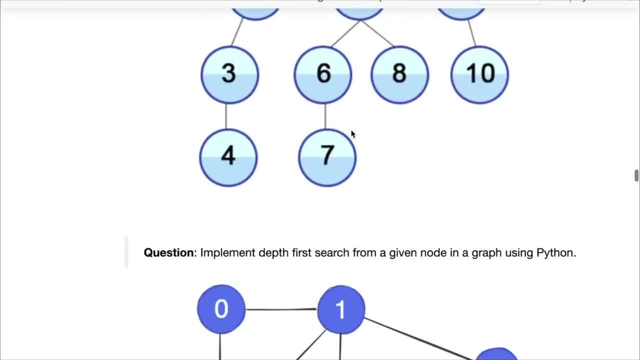 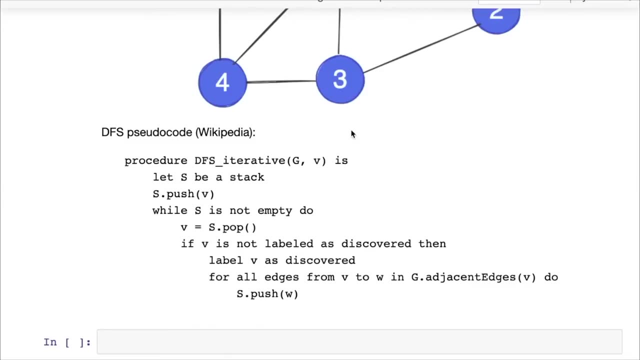 Come back and try the next edge, and then you come back and try the next edge. So there are two ways to write it. There is a way to write it recursively, and then there is a way to write it without recursion, And I leave it as an exercise for you to write it recursively. 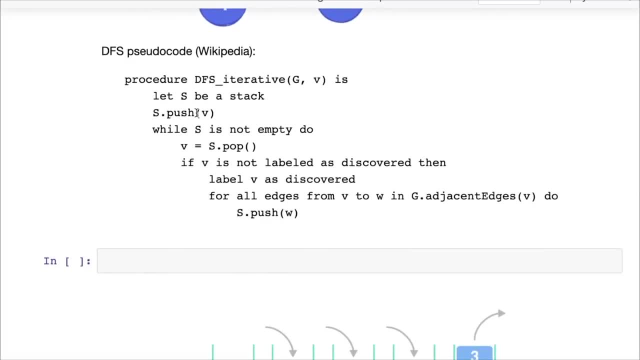 But what we'll do is we will write it without recursion and write without recursion. We will use something called a stack. We will use a stack and a stack is another data structure. very simple list like data structure, but it's just like a queue. 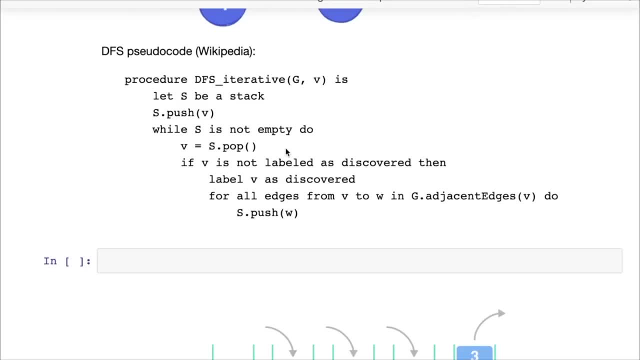 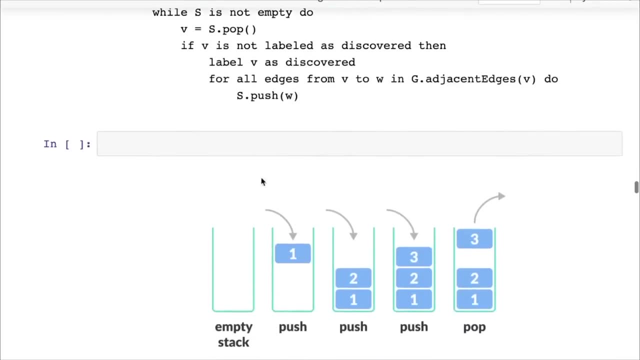 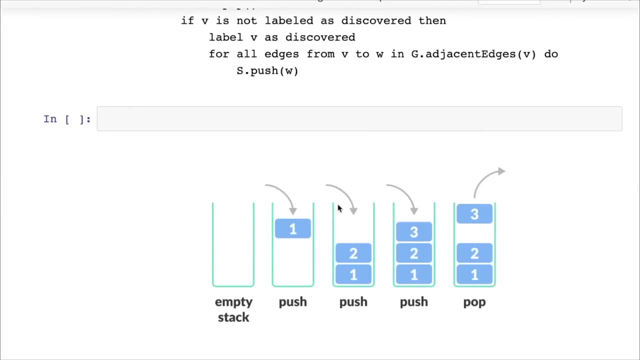 But it's different: instead of being first in, first out, which is what we do in a queue, in a stack, We perform last in, first out. So here's how it works: You start with an empty stack- So you can think of it like this container or a cookie jar- and you start putting in things into that jar. 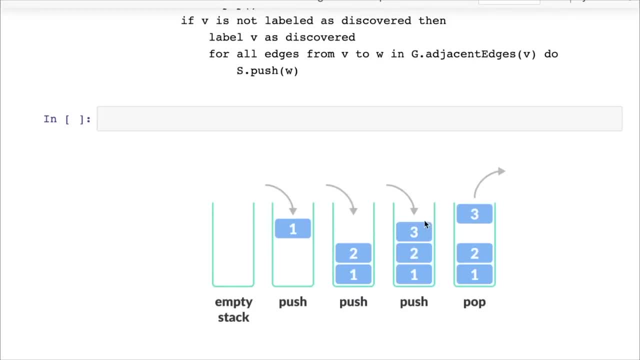 You put in one, and you put in two and you put in three. So now, when you have to remove an element from the stack or you want to access an element on the stack, the only element that you can access is the element That was. 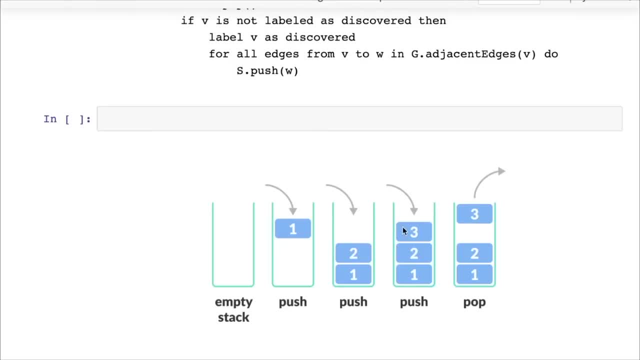 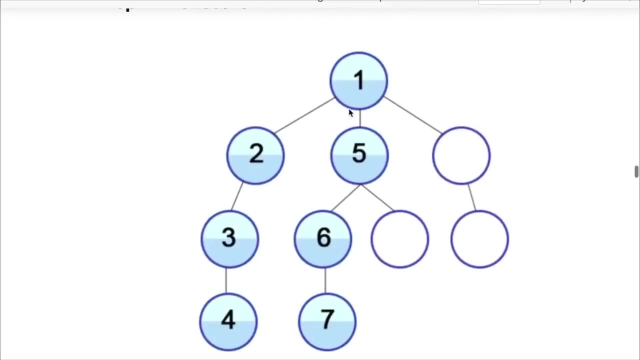 Inserted most recently. So last in, first out, that's a stack. How is that going to be useful? It's pretty straightforward, If you think about it, because this node, when you start from this as a source, you will add all these three into the. or let's say, you add these three into the stack. 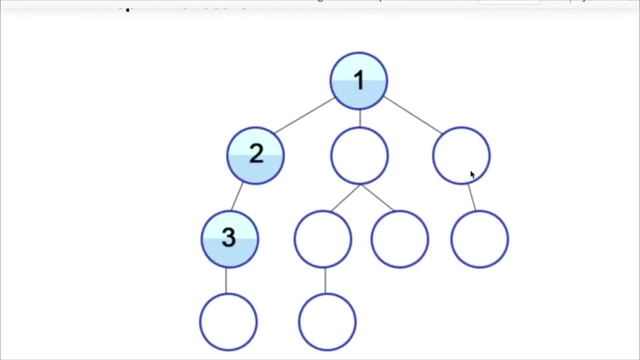 Now, if you add these three, let's add them in this order. So you start with this node, then you add this, this and this, So you add these three into the stack. Then the last in a value was two. 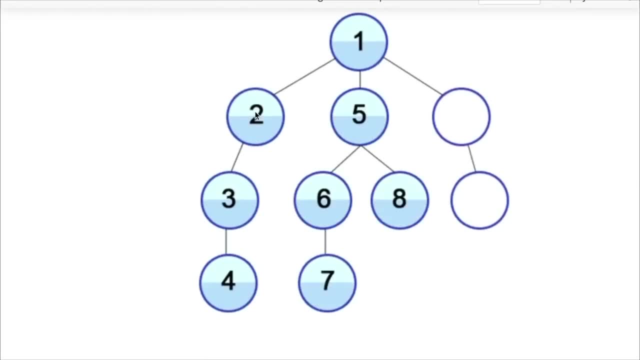 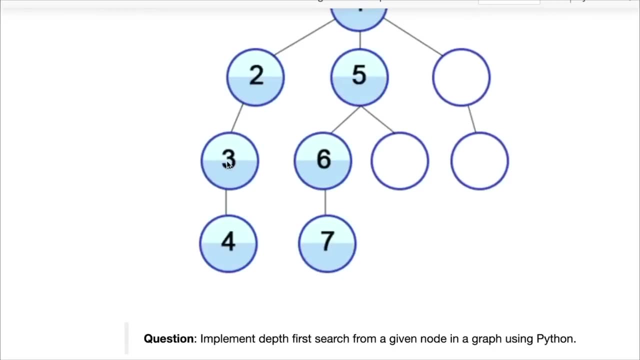 Okay, So then what you do is you extract two out and then you insert everything that two is connected to into the stack. So you insert three into the stack and then you- the last in value was three. So you insert, you take out three and then you insert four into the stack. 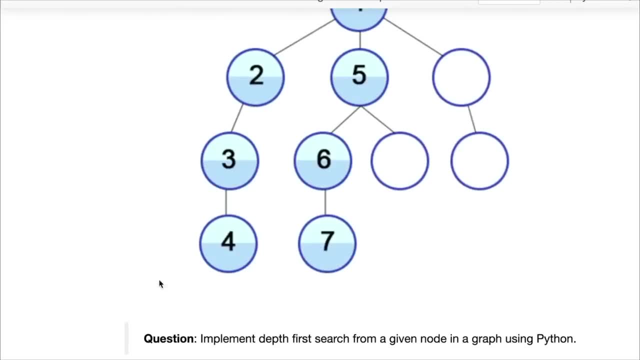 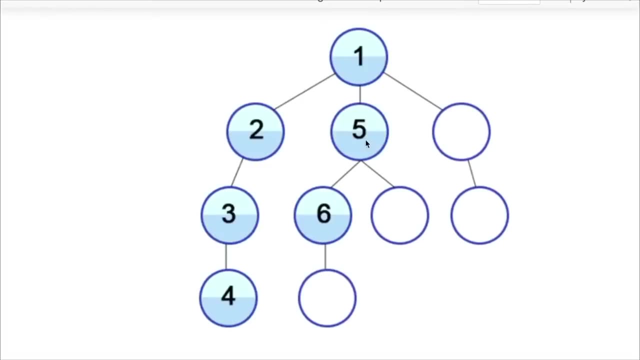 Then the last in value was four. Then you take out four and you have nothing left to insert. So now this entire path has been exhausted. So then you end up with this five. Now, when you end up with five, you can insert its neighbors eight and six into the stack. 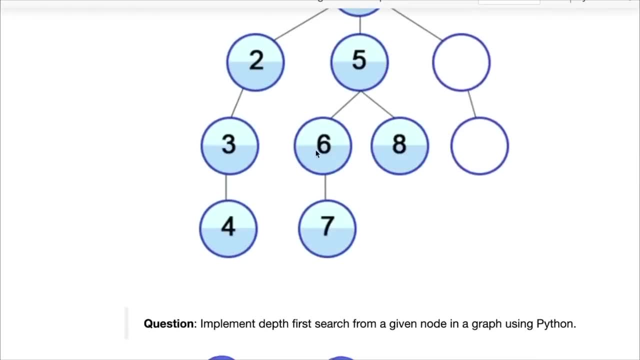 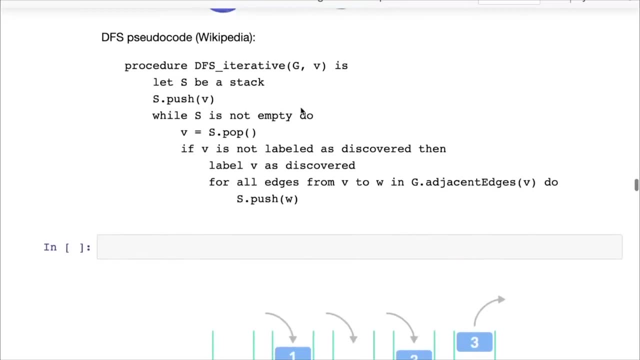 And once six gets inserted into the stack, then you take out six and you put seven into the stack, and so on. Right, So you can see how depth first search is working using a stack, And roughly. this is what the procedure, the process, looks like. 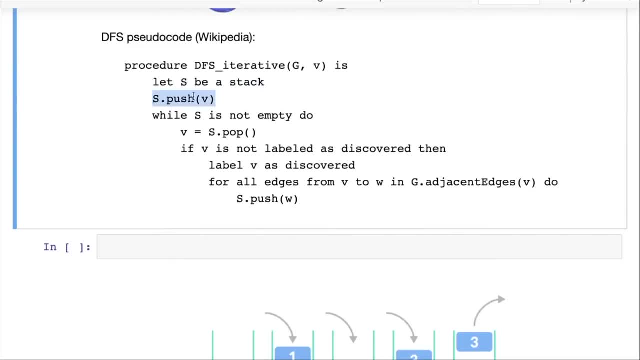 You start a stack. it's empty, push. push the current source, Let's say the root node, which you were starting with. put the root into the stack. Now, while the stack is not empty, pop the stack So get the last. 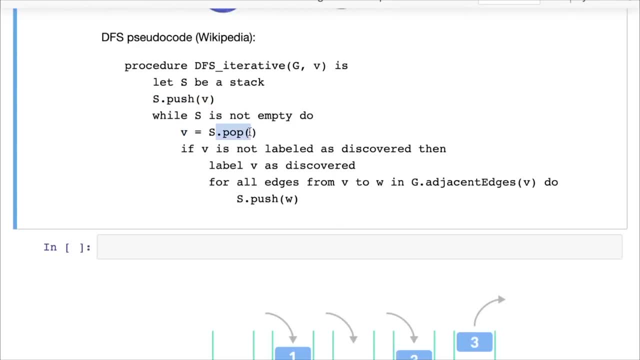 In value from the stack And that gets removed as soon as we call pop. Then if that node is not already discovered, then we mark it as discovered, And then for all the edges, from V to W, so for all of its neighbors, we 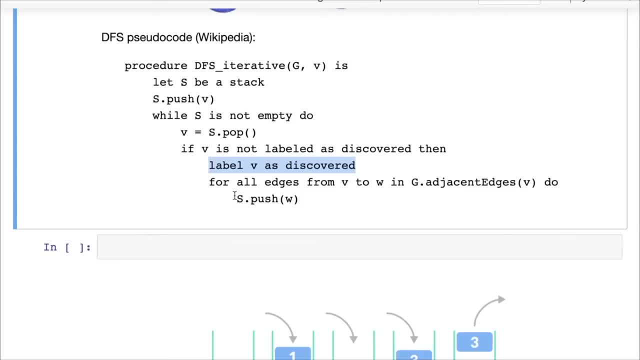 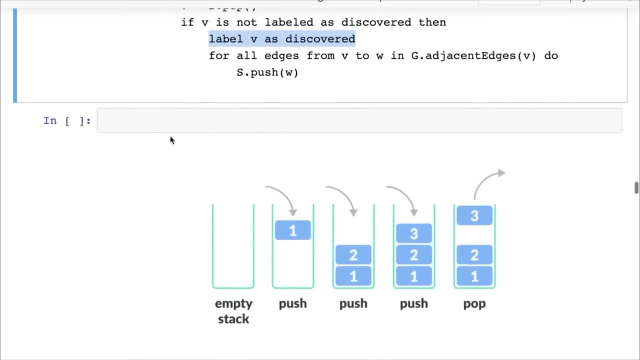 simply push them into the stack, right? So that's it. That's all we're doing. all of its neighbors which are not already visited? We can simply push, push them into the stack. Okay, So let's do that. Let's implement DFS. 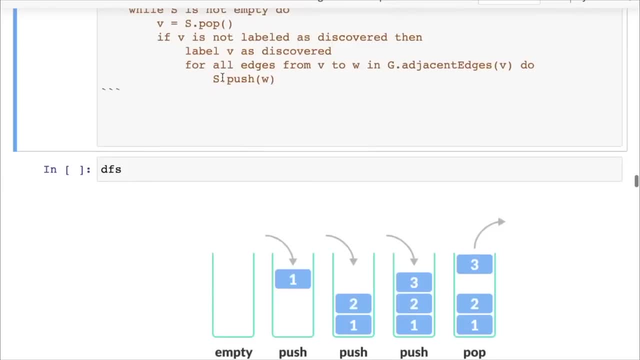 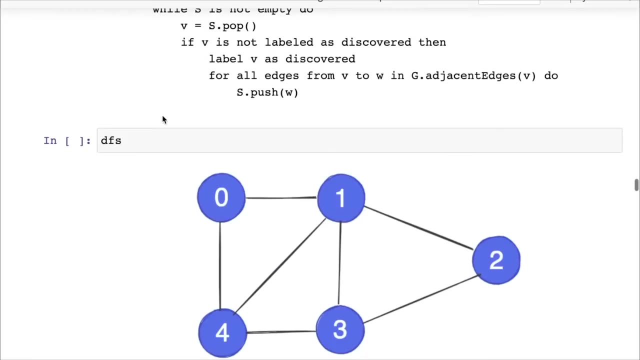 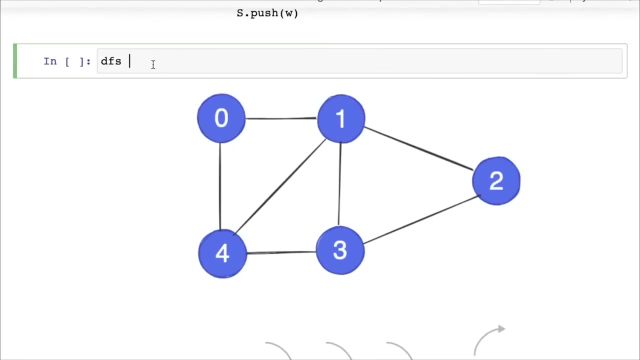 And, once again, we will keep this picture in mind, So let me just grab this picture here as well. This is one of the nice things about Jupiter: that you can take these images and simply include them within your Jupiter notebook while coding, so that you don't make any mistakes. 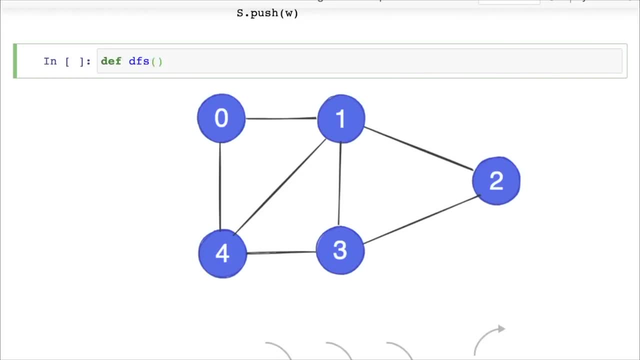 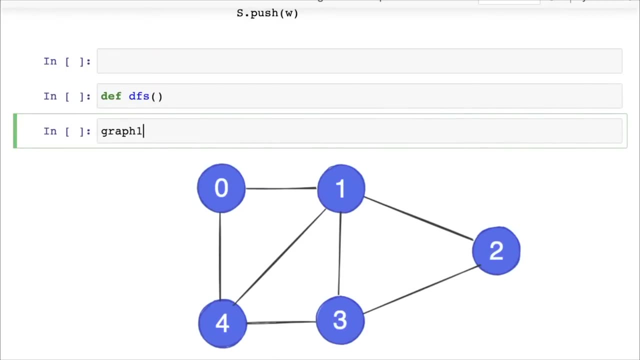 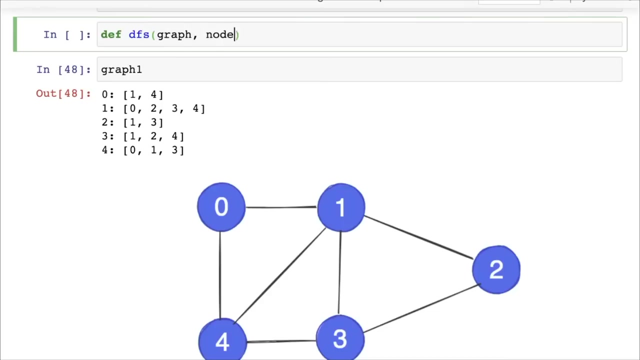 So let's say we are writing defined DFS And once again, let's assume that we are Going to start from three and this picture is graph one. So let's say we are starting from three, So defined DFS graph and we have a root node that we want to start with. 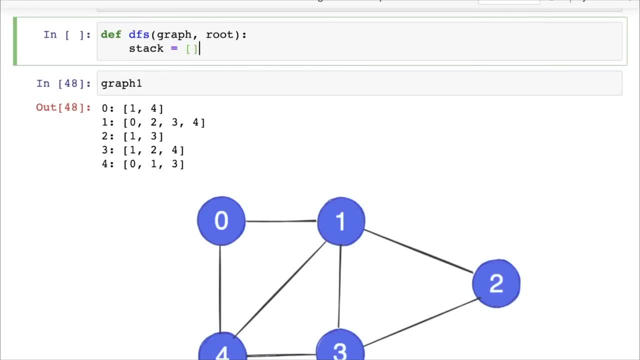 And the first thing we want to do is we want to create a stack and you can use a list as a stack adding. you can simply add things to the end and then pop them from the end. So we create the stack and then we find this: 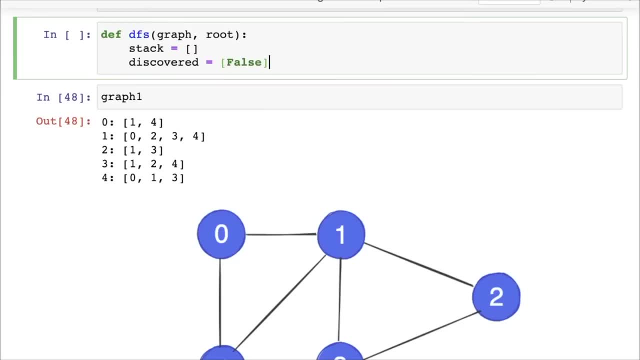 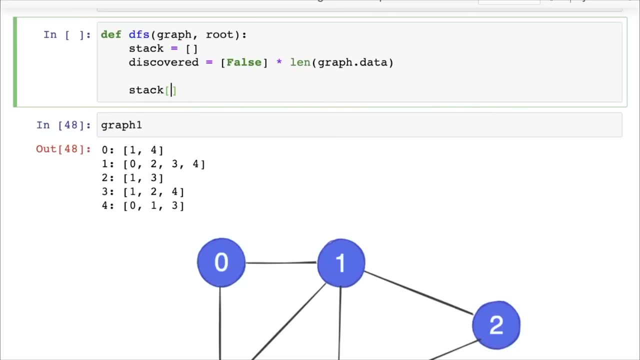 We mark discovered, we mark discovered as false, or every node, Len, graph or data. Then we say stack dot insert. So stack dot append. So we simply add the number three to the end or the root number to the end: Stack dot- append, root. 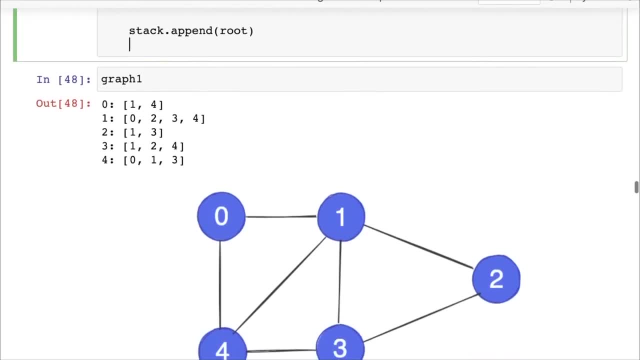 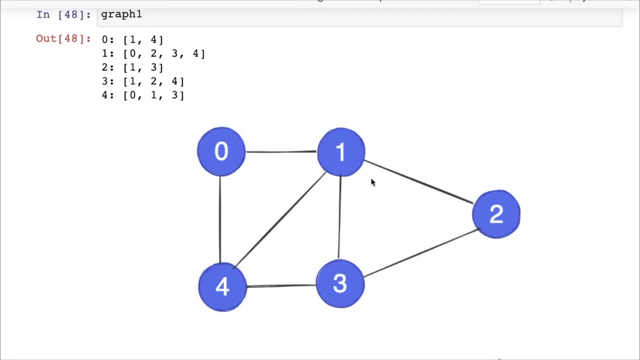 And then we don't market as discovered yet. Now, this is the interesting thing in DFS, because, remember, when you start out with three, you want, You don't want, to mark four, one and two, all of them as discovered. You want to put them into the stack, but only when they come out. you want to market as discovered because 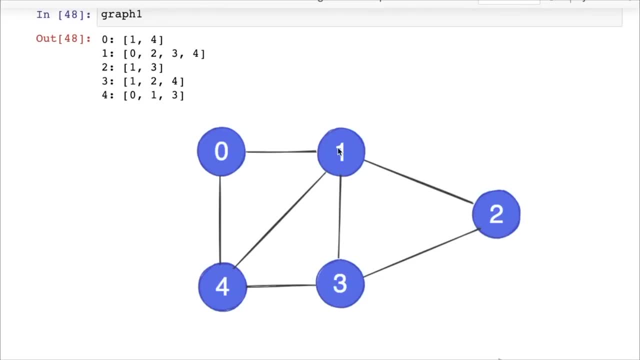 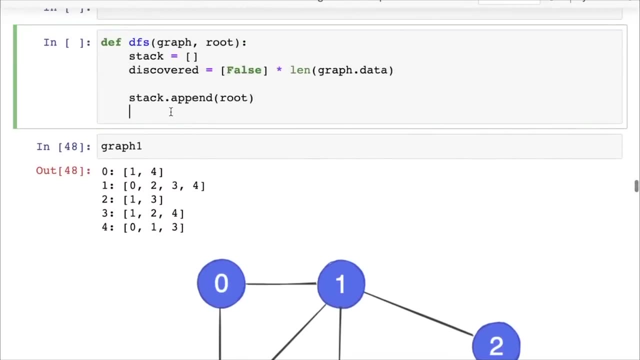 you want to discover four, and then you want to discover zero before you discover one. So that's why we put these into the stack, but we don't really mark them as discovered just yet. So that's why we're not marking the root as discovered. 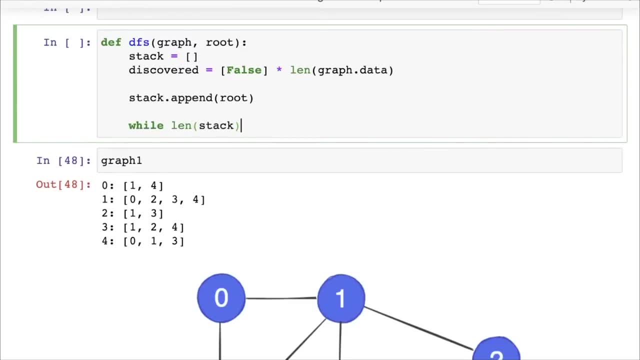 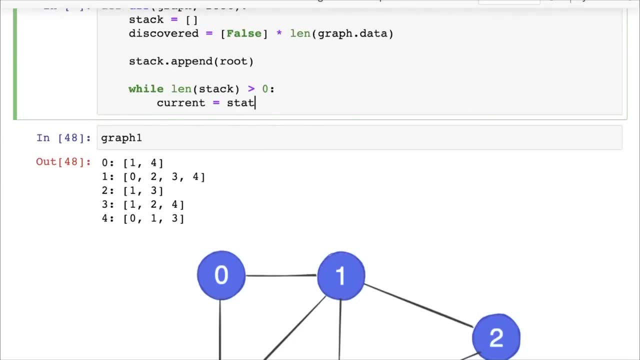 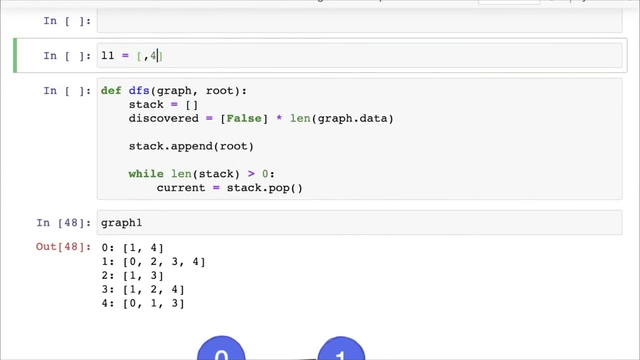 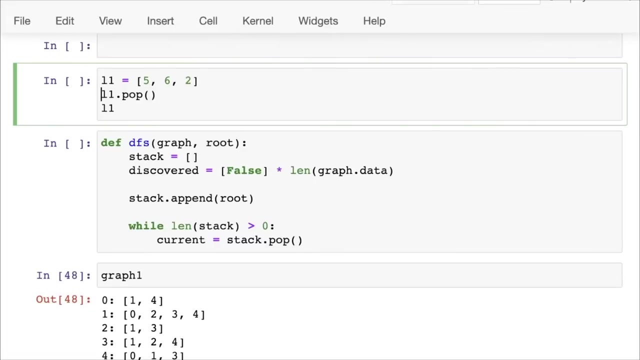 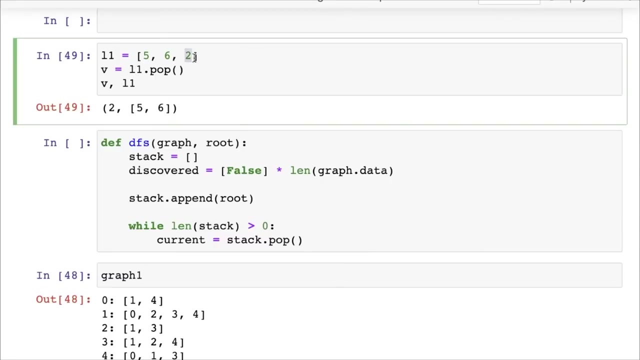 Then while Len stack is greater than zero, we get the current value. So the current value would be stack dot pop. So interestingly I can list to support a pop operations. If you have a list and then you do L one dot pop, you can see that the value we that you get from L one dot pop is the value two and L one now has the value five comma six. 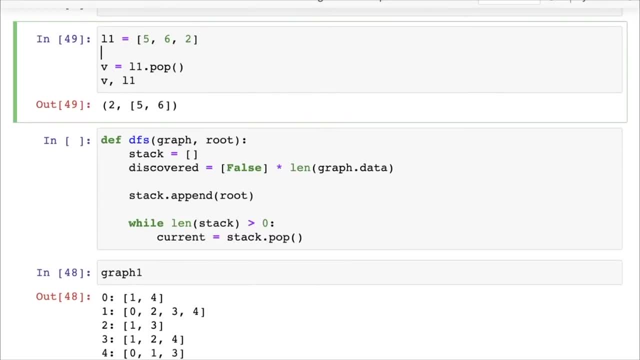 Okay, So you can use a dictionary or you can use a Python list like a stack. In fact, we can even try append here to see the entire process. Let's say we are appending three and then we are popping three, We get back three and five, six, two remains. 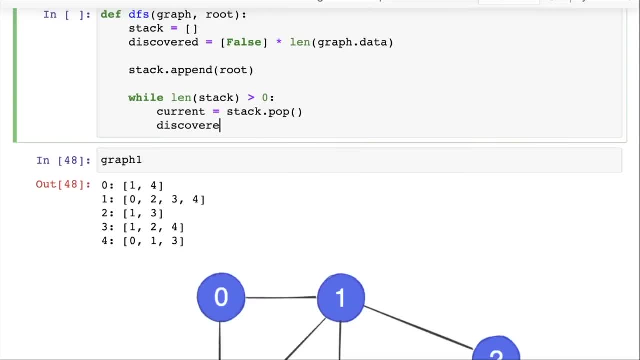 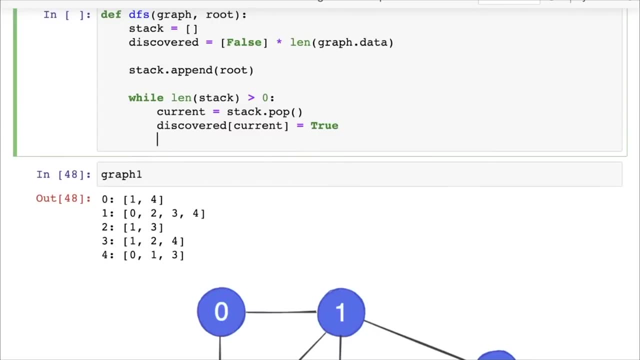 So we pop the current node and then we mark it as discovered. We mark it as discovered here. Mark discovered of current is true And we may also just want to store that. this is the result that we have. So we may also just want to create a result list. 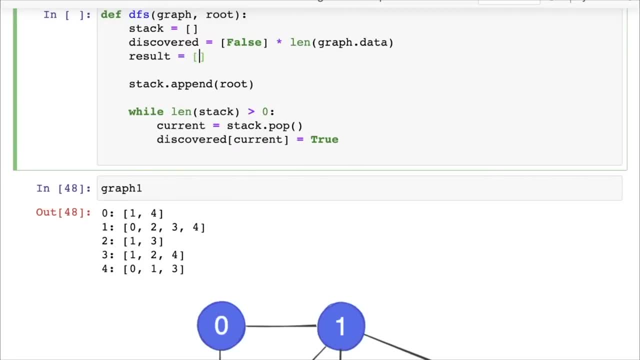 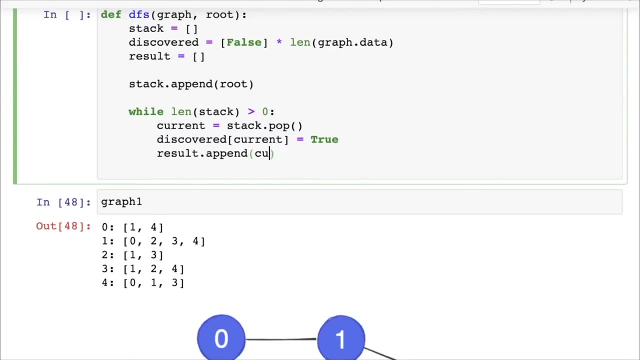 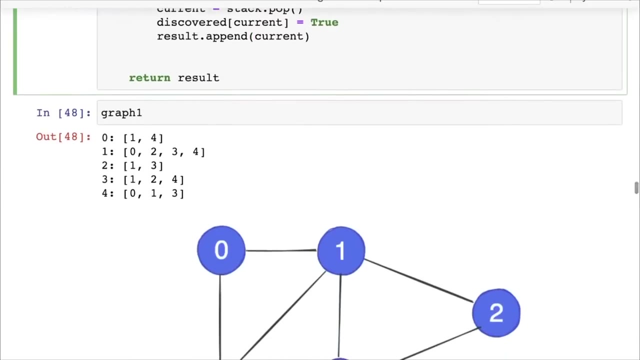 Okay, Where every time we pop something, we are also going to add it to the result list. So let's say, result dot, append current, and then we are finally going to return the result. Okay, But here's the main logic. So for all the nodes in graph- dot data current, we are simply going to push those notes into the stack. 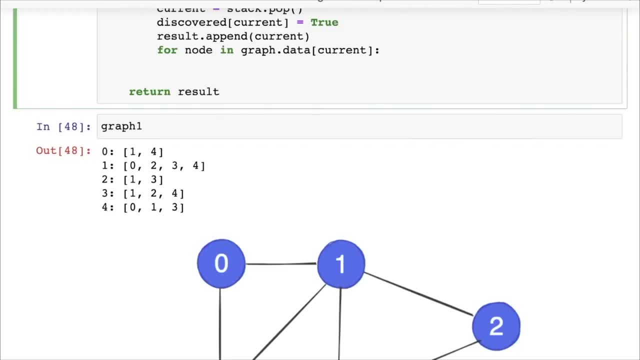 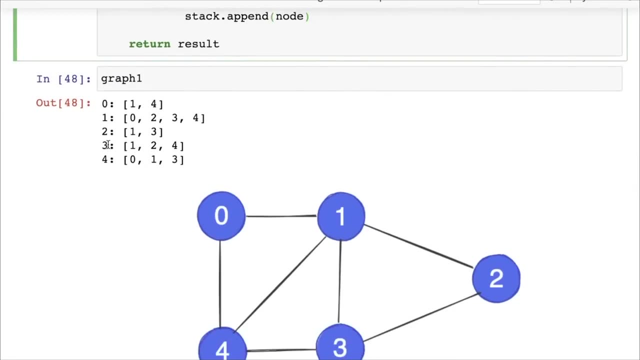 So We are simply going to say stack dot, append node. Okay, So what we do is we start with three and we then pop three and add it to the result, And then we put one, two and four into the stack. We don't mark them as discovered yet. 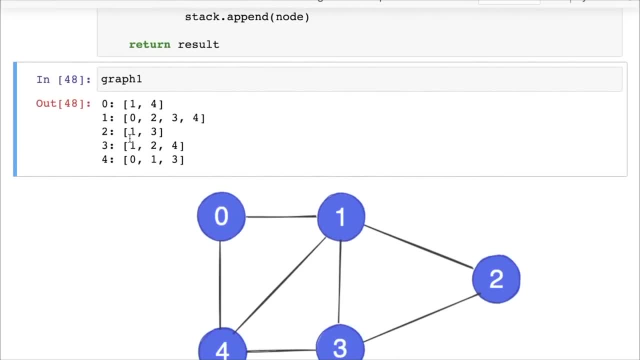 Then we pop one, and then we put all of these zero, two, three, four into the stack. We don't mark them as discovered, yet We mark one as discovered Now. then we pop zero because the sorry. then we pop four, not one, because we insert one, two, four. 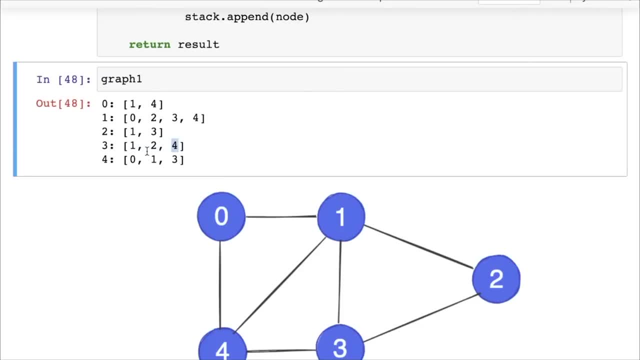 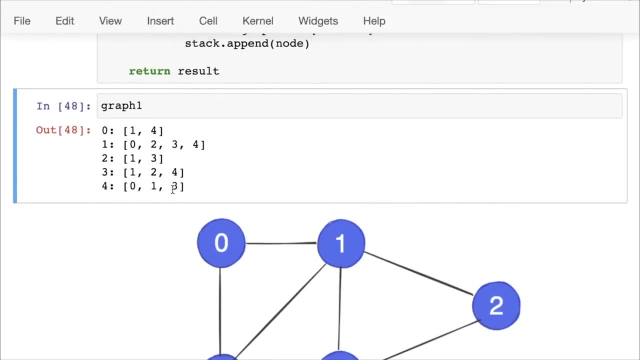 So four is the last inserted value. So then we pop four, four- the market has discovered. and then we insert zero, one and three. Now you can see that there is some repetition here. We're also inserting three once again. 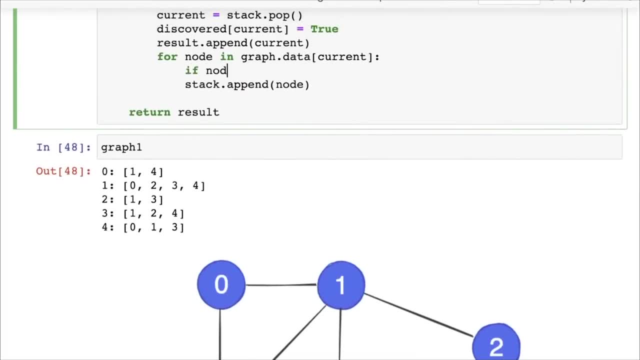 So just to avoid that, what we can do is we can say, if not discovered node, only then add it to the stack. right, There's no point in adding something. We can add something to a stack if it is not all, if it is already discovered. 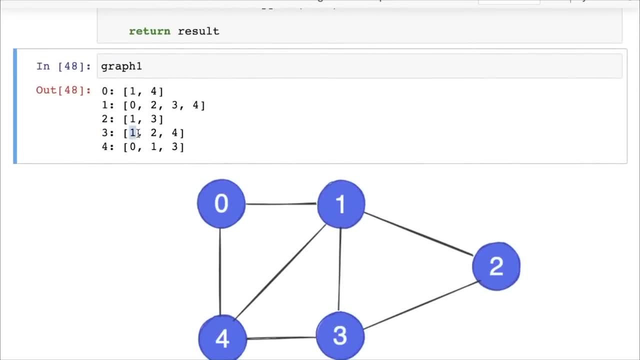 So now, with that in mind, let's see: we start with three and then we insert one, two and four. Great, What is the last value inserted? So three is discovered. now four is the last value inserted. So we pop four and then we insert zero one, but we don't insert three because it's visited. 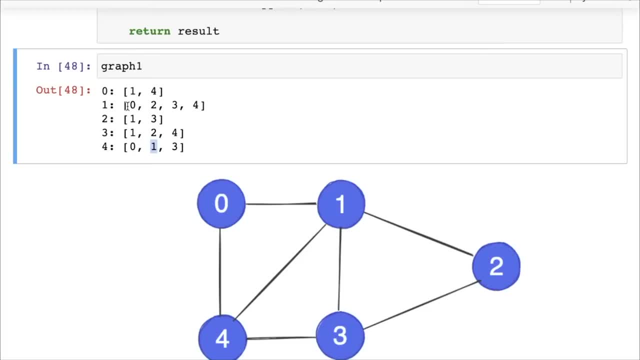 So now one is the last value inserted, Then we pop one, and then we try to insert some of these other values. It seems like everything is already inserted. Everything will get inserted. Then the only thing that remains is zero. So we pop zero, then we pop. once we have popped zero, we are going to pop four. 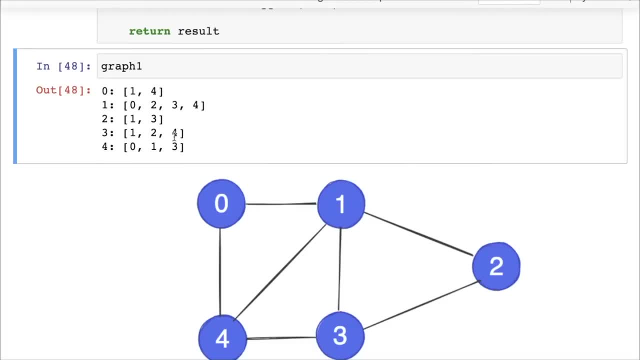 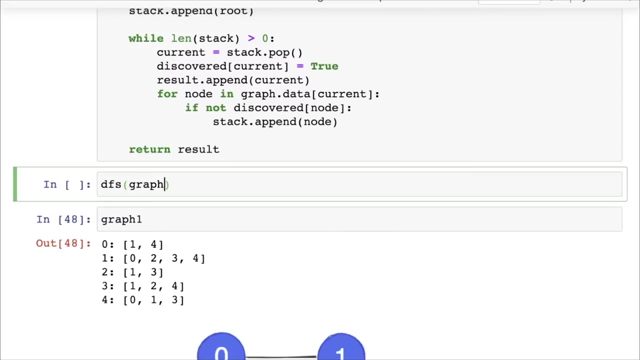 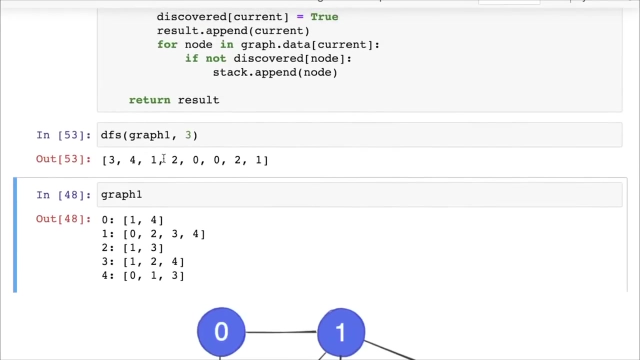 So the order in which we expect to see things is three, four, one, zero, two, I believe. Let's see DFS graph one, starting at the node three, Okay, Okay. So it looks like we have zero one. So it looks like we made a mistake because we got some repeated values here. 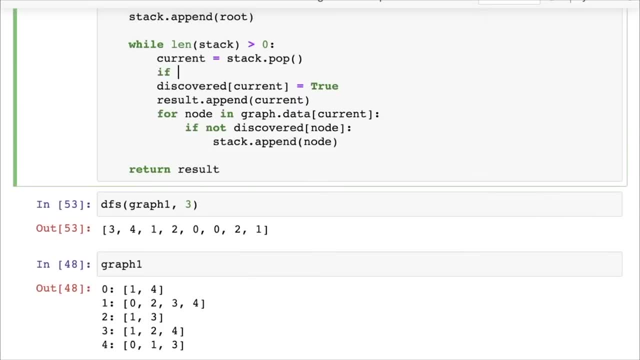 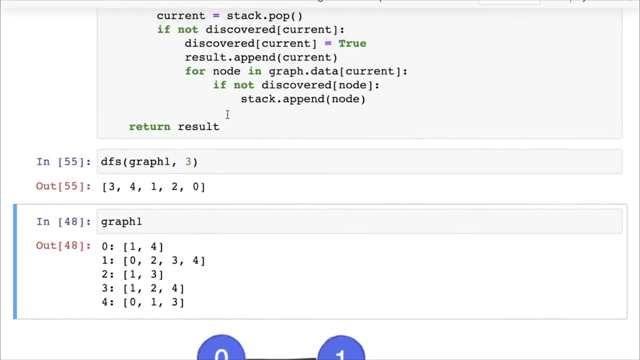 And that's because we may want to just check. If not discovered current, we may want to just add this check and put everything inside this check so that any older values that have been inserted into the stack which are already visited later sometime through another. 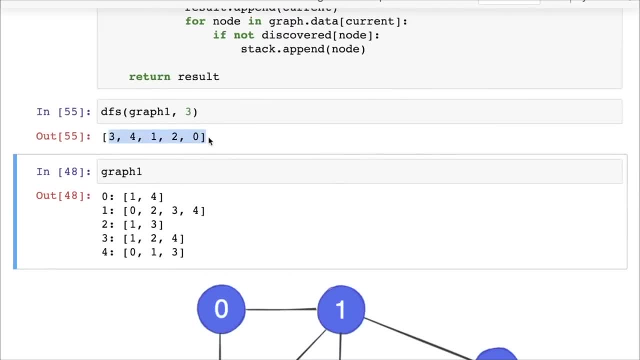 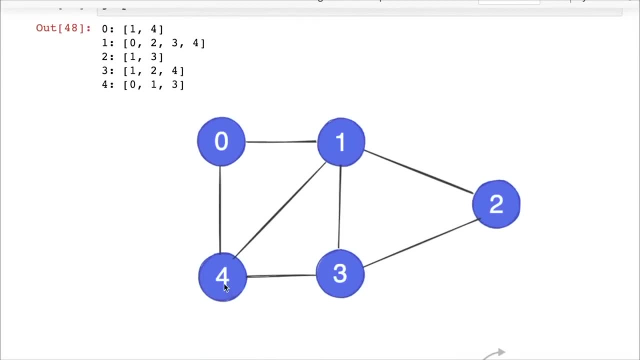 Right Right, Right Right value in the stack. that gets ignored. So we end up with three, one, three, four, one, two, zero, right? So it goes like this: First we go from three to four to one to two, and then we go from three to four to zero. 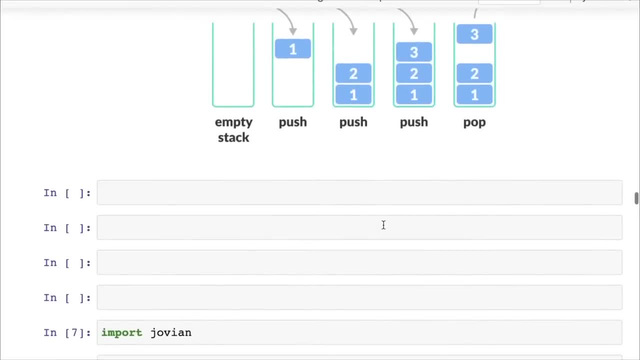 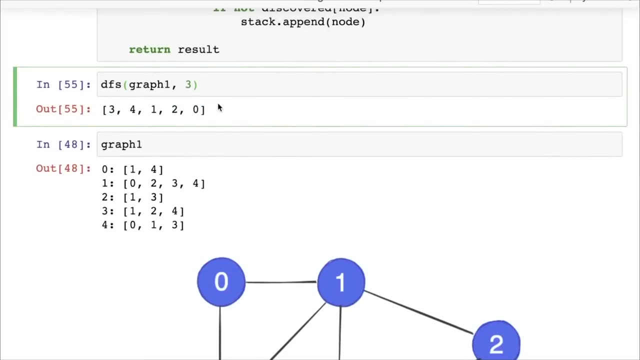 So that's how it goes. Now a challenge for you is to also implement distance. Now, in this case, the distance will not really make sense because this is not the shortest distance anymore. So when you want to get shortest distance from one node to another, then 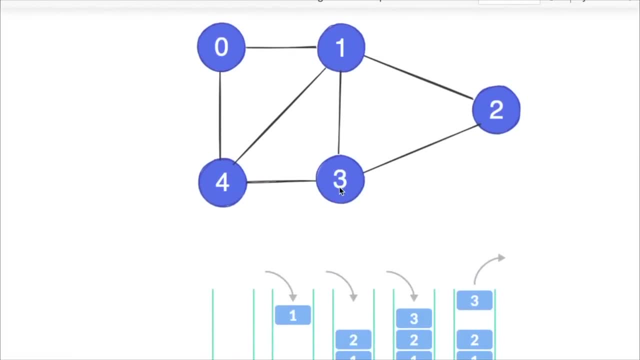 you want to use BFS, not DFS, because if you track distance here, you may end up going by DFS: three to four to one to two, And that is going to give you a distance of four, a distance of three to getting to two, although the shorter distance is one. 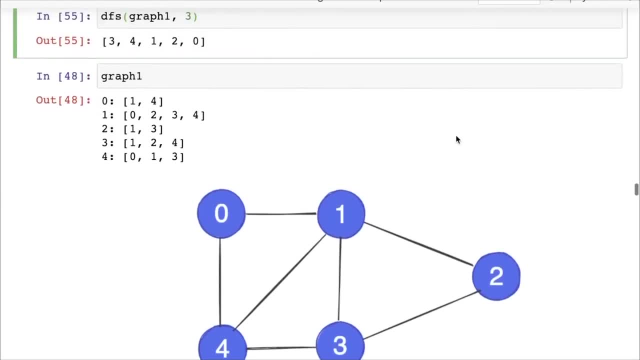 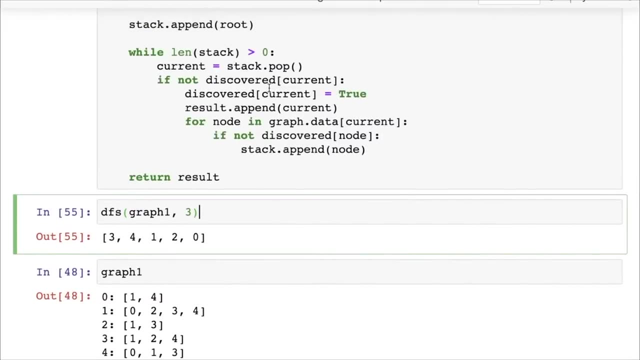 So maybe distance doesn't make sense here, but what you may want to put in is the parent. You may want to track the parent, for each node should be simple enough to do. Whenever you are Popping something, you may just want to track it's parent. 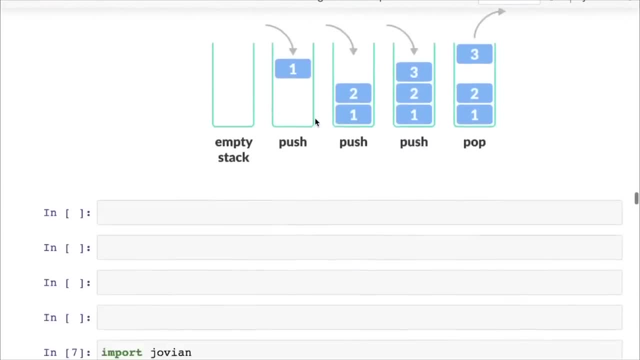 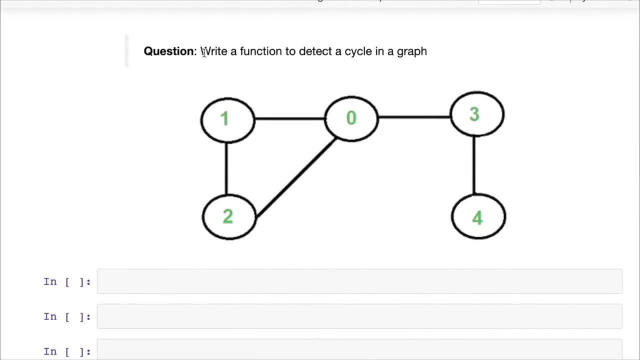 Okay, That's an exercise for you. Another exercise that you can try is to write a function to detect a cycle in a graph. Now, when you're performing DFS, let's say you are going about performing DFS starting at one And you do this, and then you end up here back at one, right? 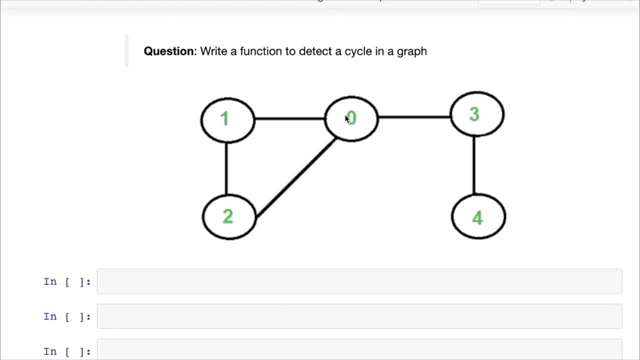 Because you go to from one to two, two to zero, And when you notice that, Okay, Zero points to one which is already visited, that gives you an indication that there is a cycle in the graph. A cycle is simply a path which leads from a node to itself. 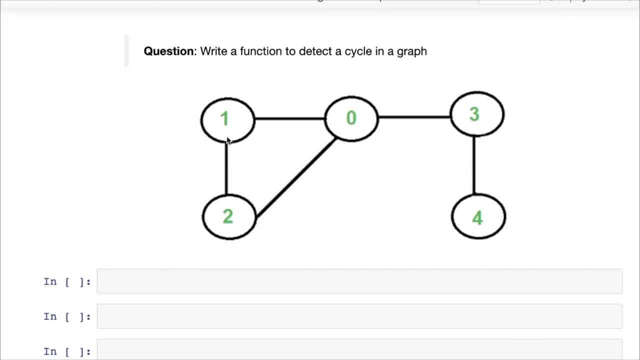 So one, two, zero one is a path, and a path is something. a path is a sequence of edges. So one, two is an edge, two, zero is an edge and zero one is the edge. So this is a path, but one, two and two, four is not an edge. 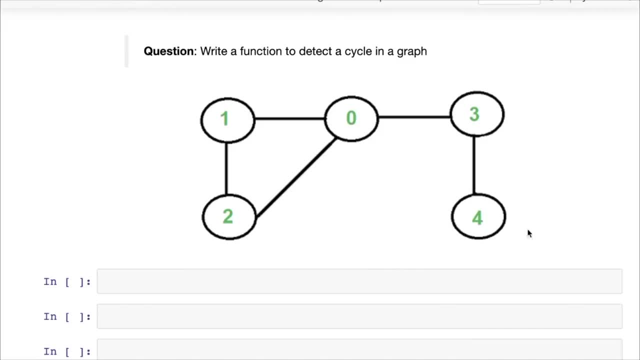 So one, two, four is not a valid path, right? So cycle is simply a path that leads a node, leads from a node to itself. So the challenge we used to To write a function to detect a cycle in a graph, Another challenge for you is to detect, maybe, the number of cycles in a graph. 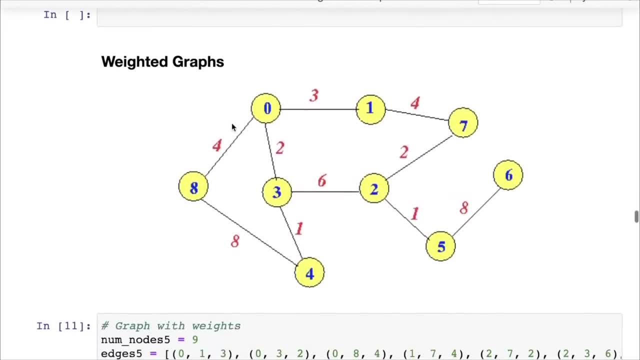 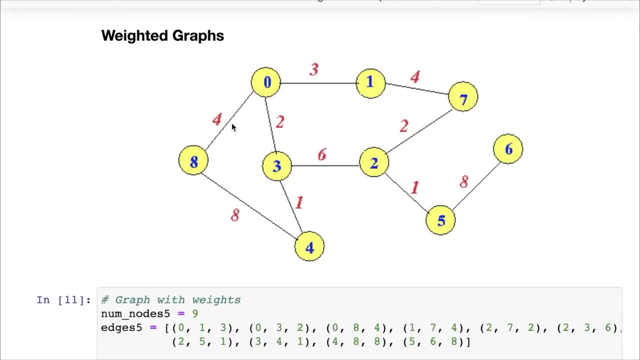 Okay, So that's another thing that you can try out, but we'll move on to another problem. Now. we'll talk about weighted graphs and get closer to that example of the railway map that we looked at initially. So here you have nodes. 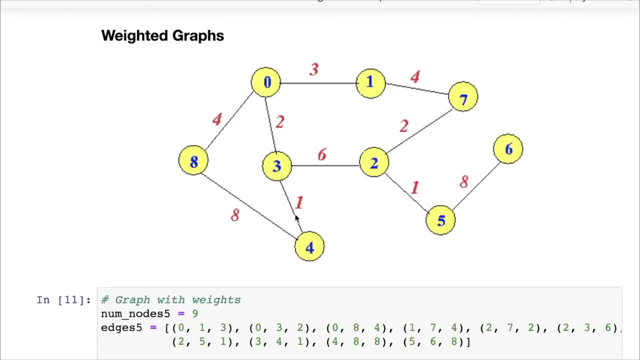 So you have nodes numbered from zero to, Okay, Eight, So you have a total of nine nodes, and you have edges too. Now these edges also have weights, and this could be distances, for example, the railway line, or this could represent any other information which is of value to you. 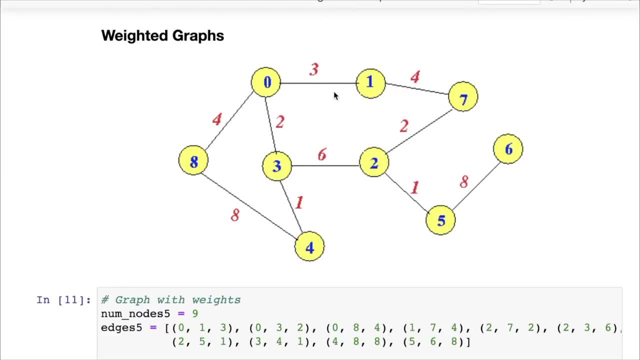 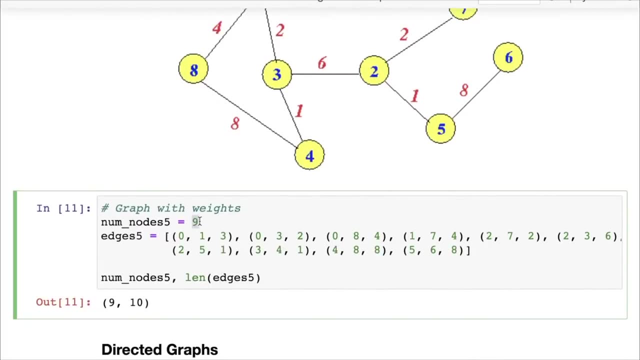 Right. So you decide what edge weights are, what they mean in the abstract representation. we simply call them weights. So this is a weighted graph, And here is an example of how we can convey the information about a weighted graph. I can give you the number of nodes. 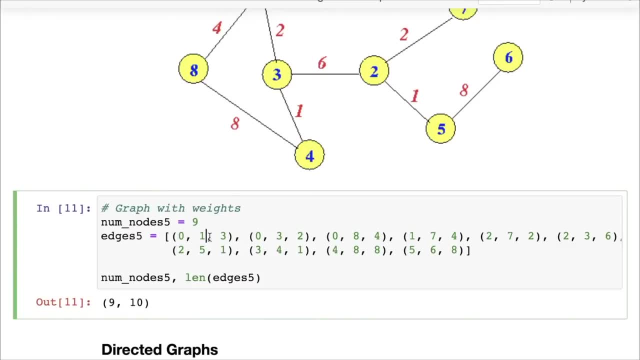 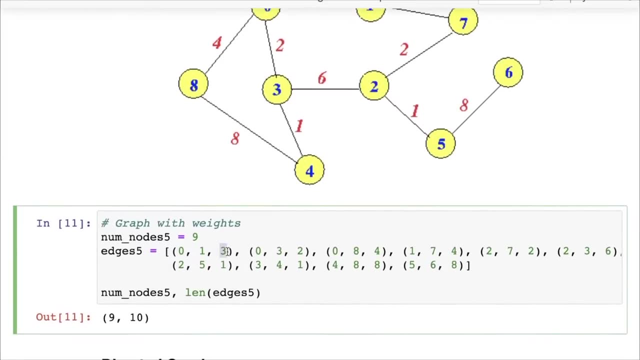 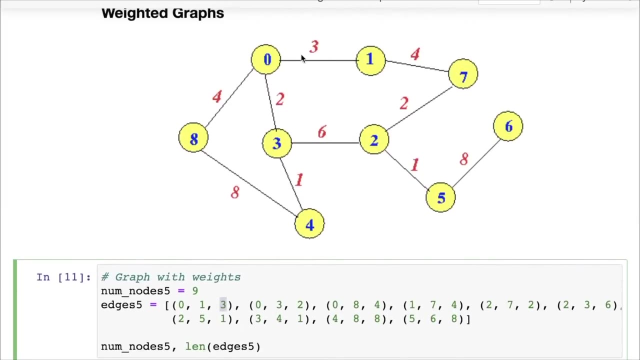 And then I can give you a list of edges. So the first two elements of each edge tell you which nodes are connected, like the nodes zero and one are connected here. And then the last element of the list, or the third element of the list, tells you if it is weighted, if there is a weight associated with the edge. 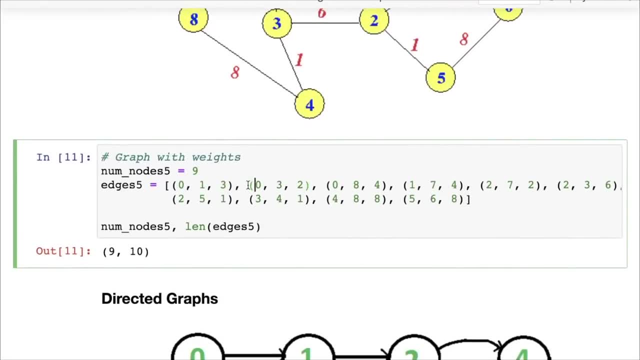 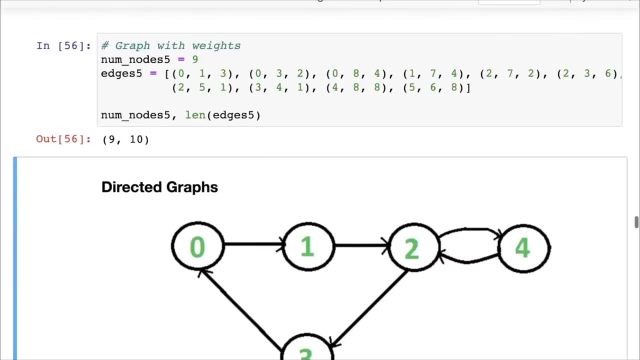 Okay, So you have zero one- three, and then you have zero three- two. So zero is connected to three and it has a weight two and so on, And you can verify that there are 10 edges here And these are: 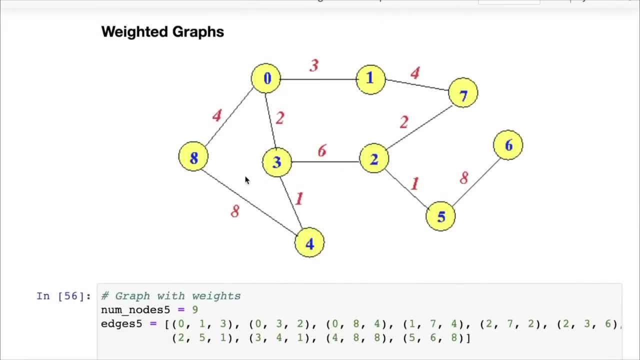 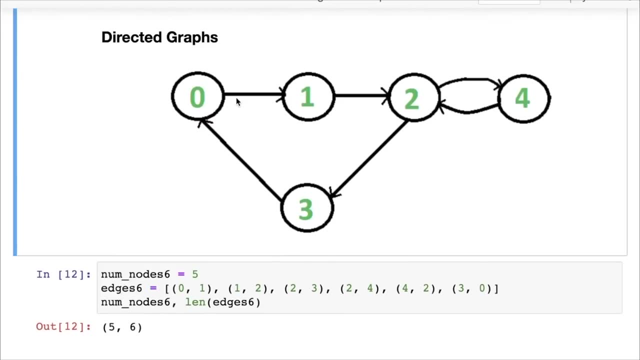 The 10 edges with the 10 weights. So that's one variation that we see in graphs. Here is another variation. This is called a directed graph. in this case edges have a certain direction. So this corresponds to the example of hyperlinks, where we have pages, web pages on the internet and one page can link to the other, but the other page may not necessarily link back. 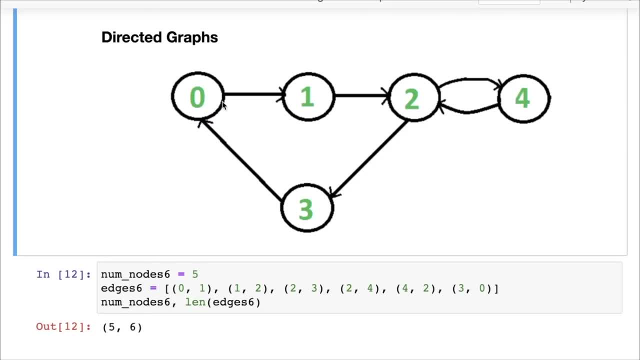 It. they may, in which case you may have a bi-directional edge, but in most cases there you would have a single unidirectional edge. So you have zero, one, one, two And two, three. now directed graphs can be represented just the same way as undirected graphs. 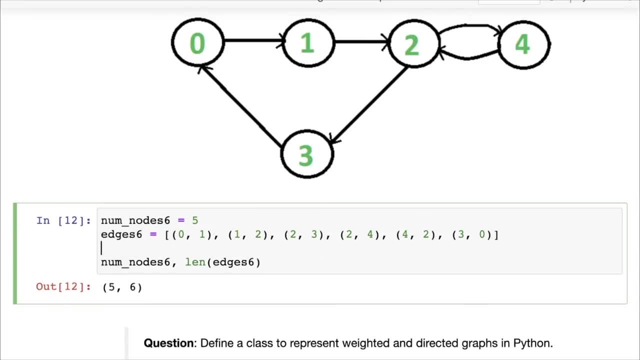 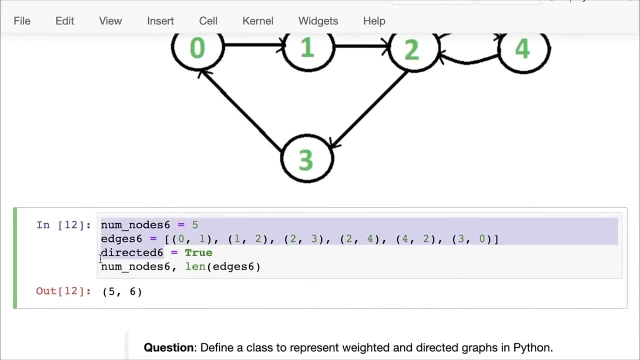 All we need to do is we need to provide some information that this is a directed graph, right, So you can simply say, uh, directed equals true, And that will simply, and once you provide all these, all this information, that can then specify to the person who is going through this data that this is a directed graph, right. 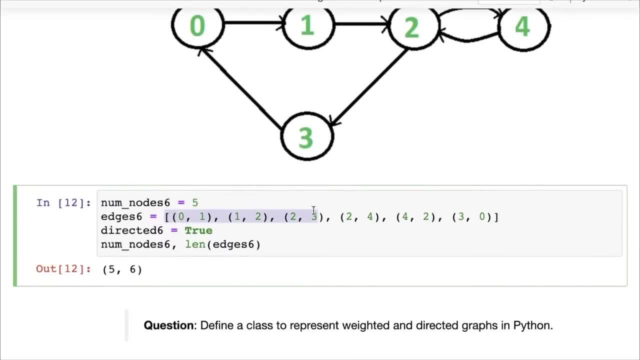 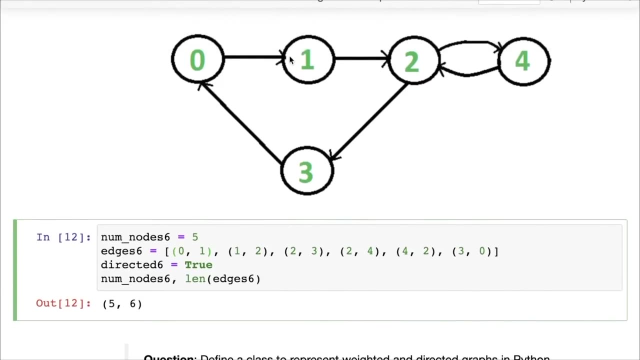 Uh, so here's how. it's exactly the same as a normal undirected graph, But When we create The adjacency list, we can have a graph or we can have a node from zero to one, but we should not put zero into the adjacency list for one, because there's no way from two, there's no direct edge from one to zero. 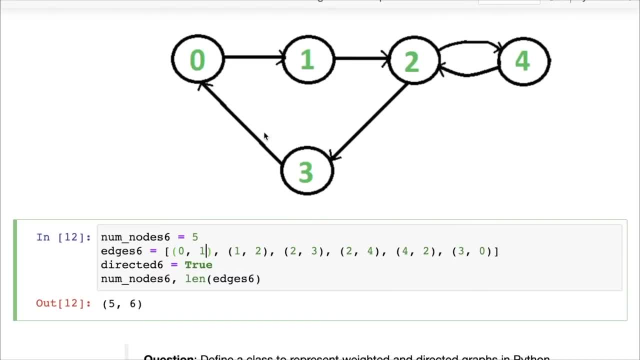 There's only a direct edge from zero to one. So keep that in mind And similarly in the adjacency list now, you will not set both the values: zero one and one, zero two, one, You will only set one of them or responding to the one direction, unless of course there is a bi-directional edge. 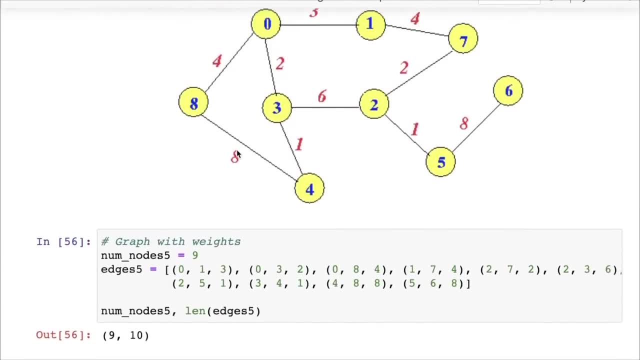 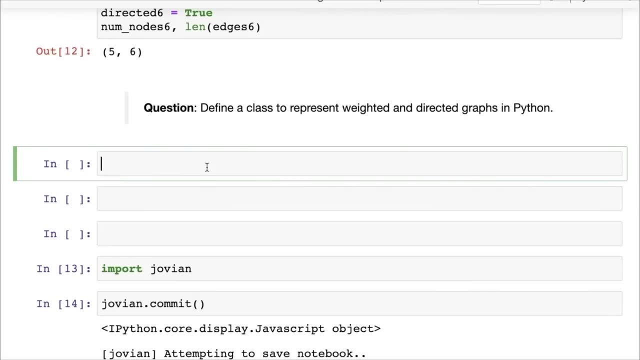 Okay, And what we can do is we can even combine directed graphs and weighted graphs. So here's the here's what we'll do: We will define a class which can represent weighted and directed graphs in Python, So we'll use it to represent undirected graphs, directed graphs and weighted graphs- all of these. 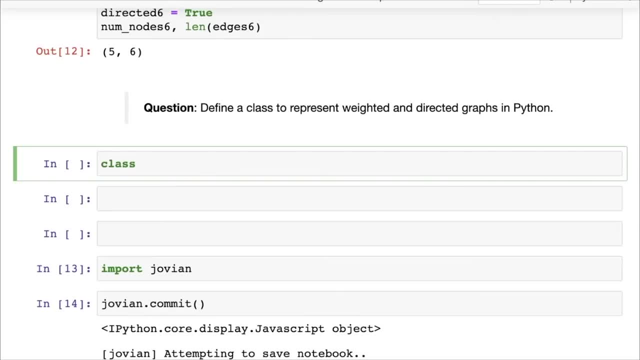 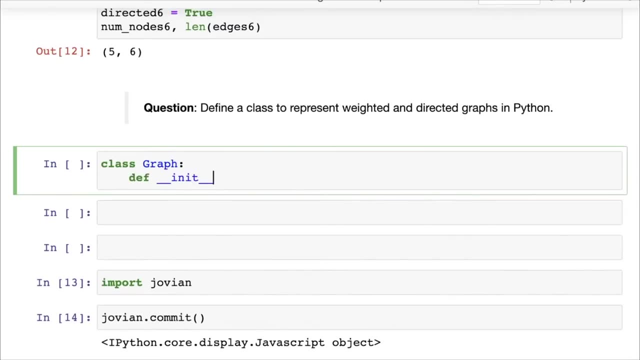 And we will take some information in the constructor to capture this detail. So, let's see, let's create a class graph. Once again, we will create a constructor. Okay, Okay, Okay, Okay, Okay. Now this has the self, which is the object that gets created. 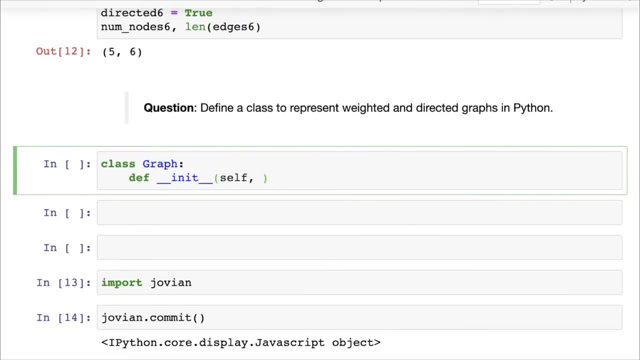 Always the first argument to any method in a class in Python. Then we take the num nodes, then we take the edges and then we take a couple more arguments. We take a argument directed which has a default value false, And we take the argument weighted which has a default value false. 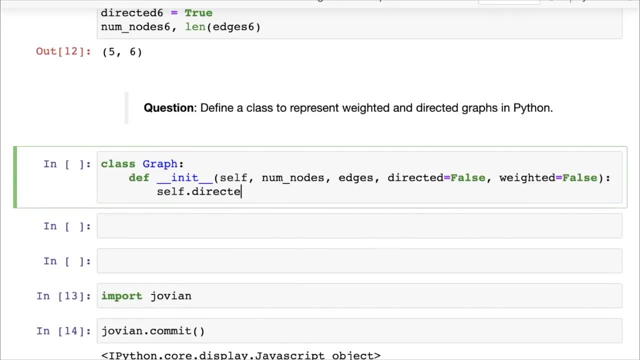 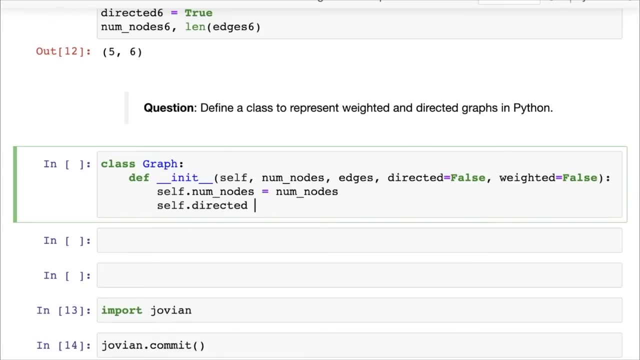 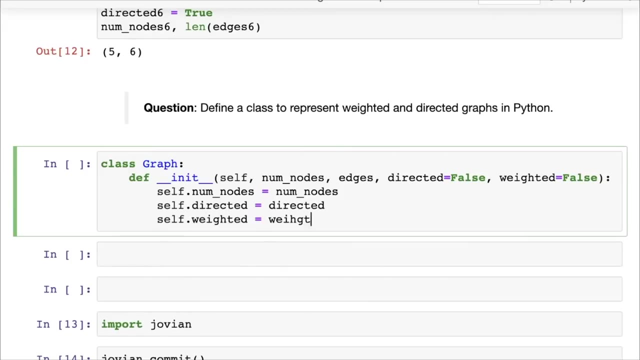 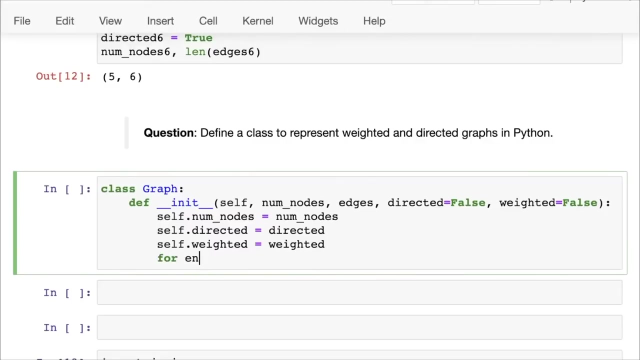 Okay, And we're going to store the information. self dot directed. let's store self dot num nodes As num nodes. self dot directed as directed. self dot weighted is weighted. Okay, So now we come to the edges. So for edge in edges, what do we do now? 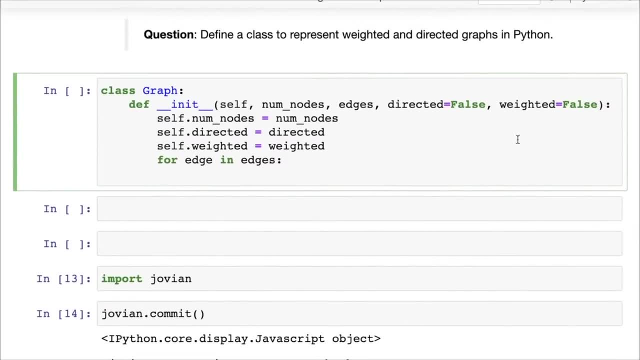 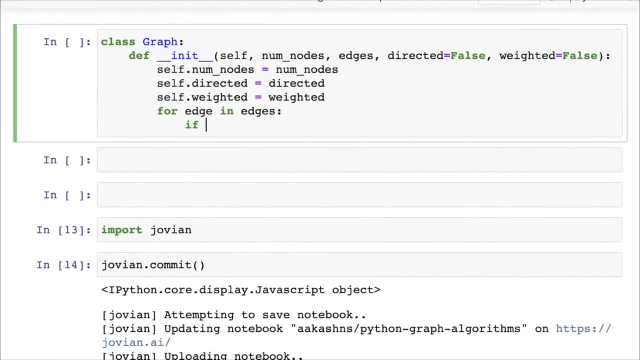 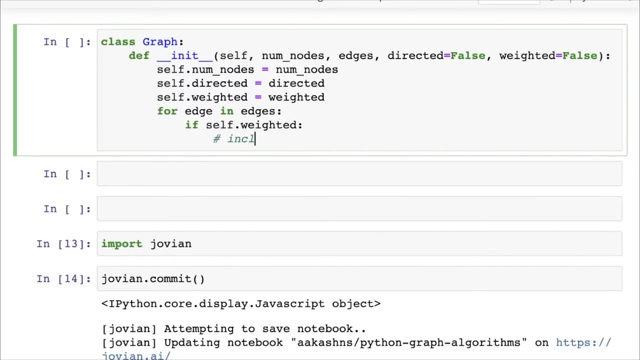 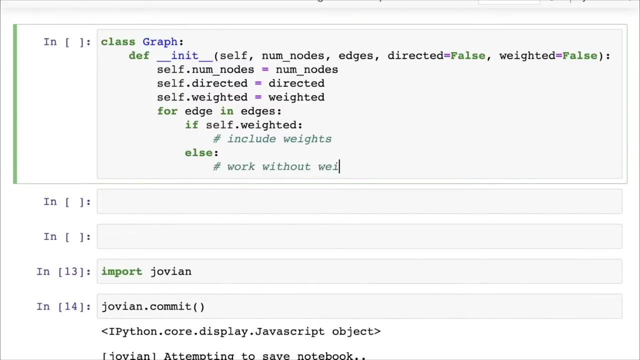 An edge, can either have two values or three values, If it is weighted. if it is unweighted, then it'll have two values. If it is weighted, then it'll have three values. So we need an if condition here. if self dot weighted, then include weights, else work without weights. 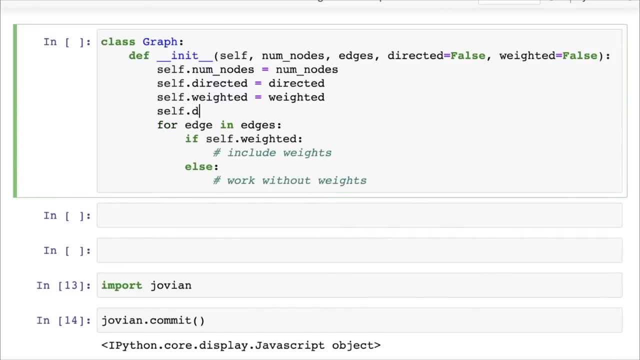 Okay, Now we may want to also because we need to create an adjacency list. So we'll create self dot data, just as we have been doing so far, And in self dot data We will create a list of empty lists, as we have done for underscore in range num edges. 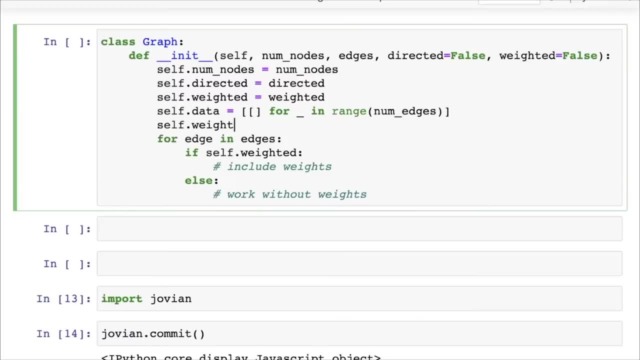 Now what we'll do. along with self dot data, we will also create something called self dot weight, And self dot weight will store for each corresponding value in the adjacency list. It will store the weight of the edge between the two elements. So far. 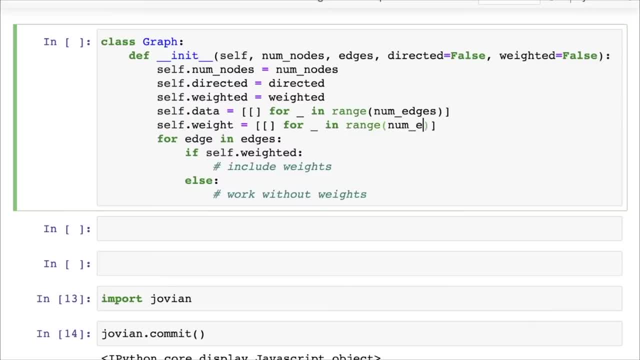 And this annual. We'll see how how it works in just a moment. Num edges. Okay, So we have self dot data and self dot weight, and this will make it easier. Another way you can do it is, instead of storing single values, you can store tuples inside self dot data, which will correspond to the node and which will also contain the weight right. 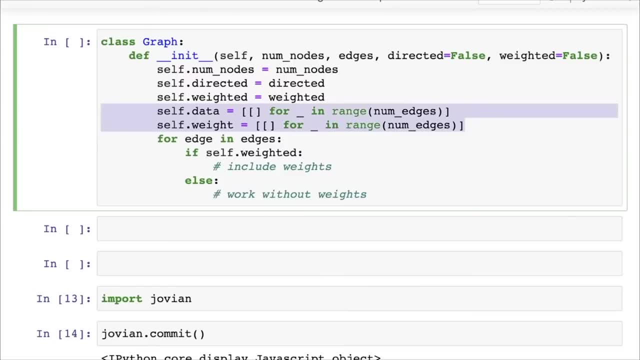 So that both these are both ways to do it. I'm just doing it this way, but you can do it the other way as well, where you can store tuples directly inside self dot data. But suppose it is weighted, then first we get the values out of the edge. 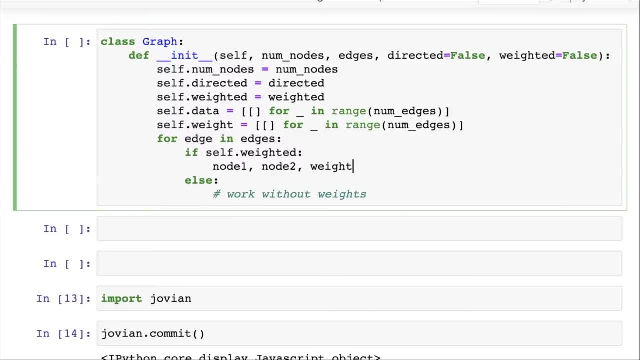 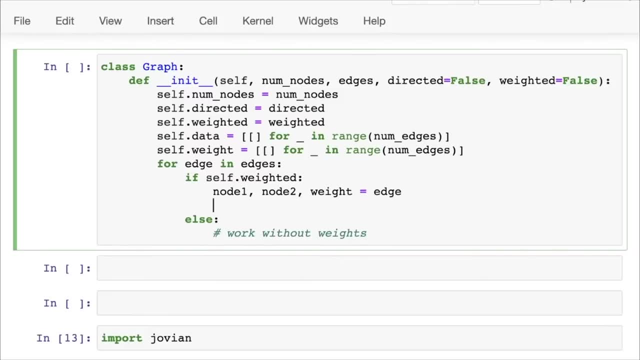 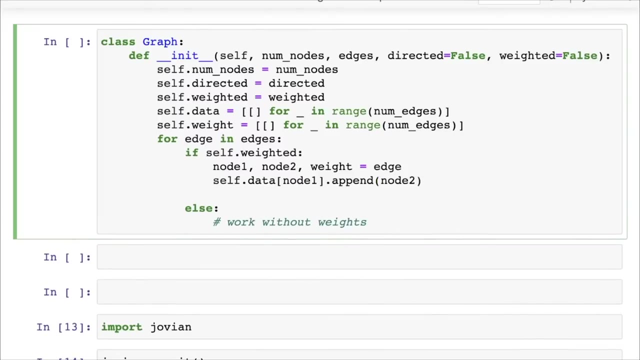 So node one, node two and weight from the edge. Remember the edge is a tuple if and then. first we set self dot data, node one, and append to it, node two, And then we also set self dot weight, node one. So at the exact, 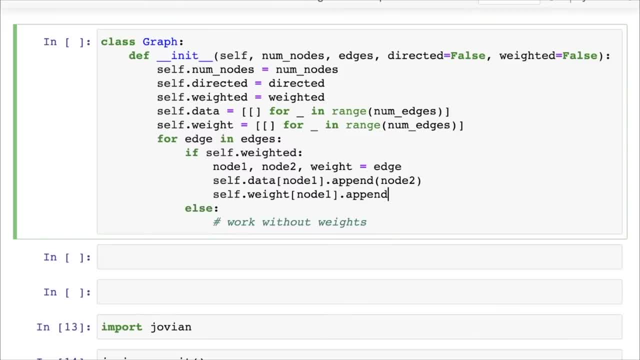 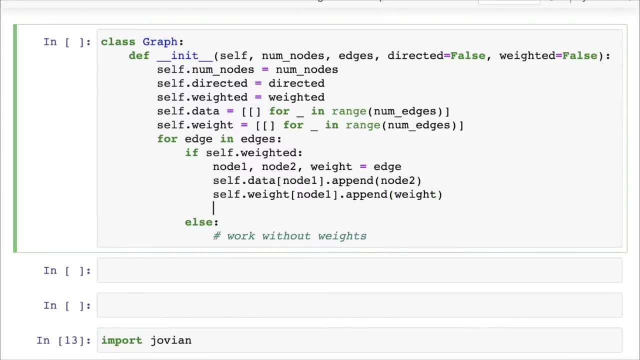 Same location, where we have node two, at the exact same index, we store the weight between the of the edge between node one and node two, which is weight. Okay, So now we've stored one direction, which is node one, to node two. 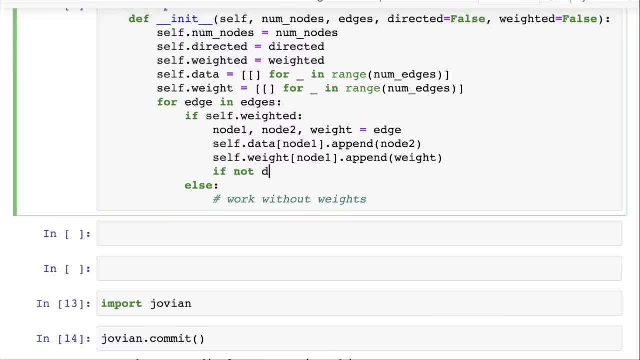 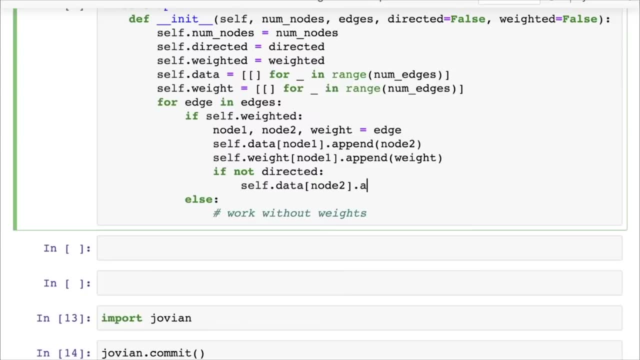 We may also need to store the second direction. So if not directed, so if if the graph is not directed, only then we need to store the second direction. So we just say self dot data, node two, dot append, node one, and then self dot data. 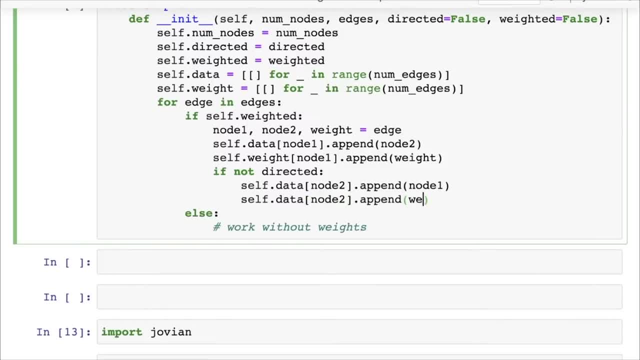 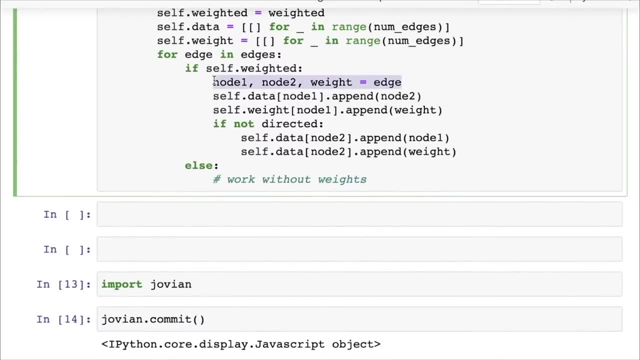 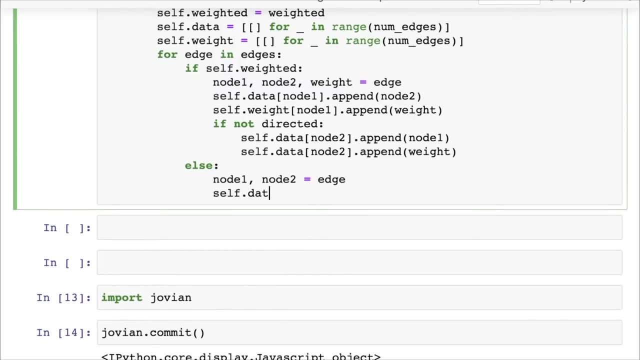 Node two: dot append weight. Okay, And that's the case when it is weighted. if it is not weighted, well, the code is actually simpler. So we simply get node one and node two from the edge and we say self dot data. node one: dot append node two. 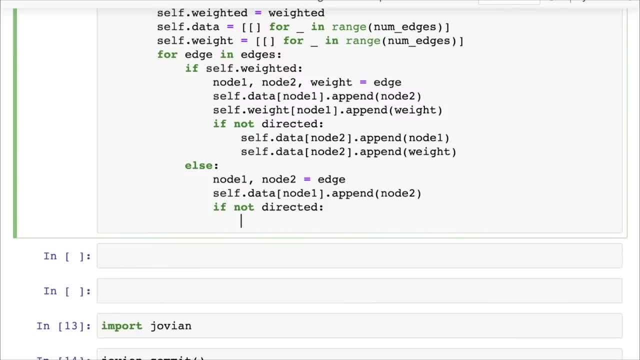 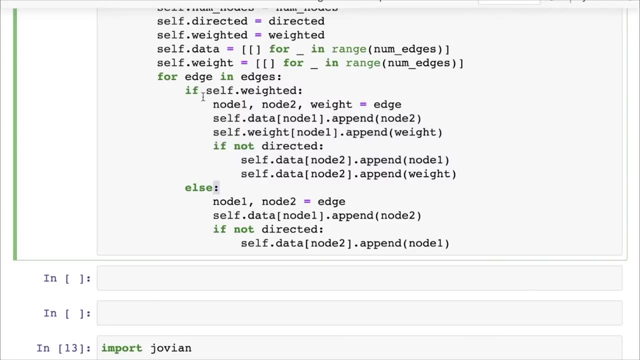 And then if not directed, so there's no weight here. So we simply check if the graph is not directed, self dot data, node two, not append node one. Okay, So there's a bit of code here, but the code is again fairly straightforward. 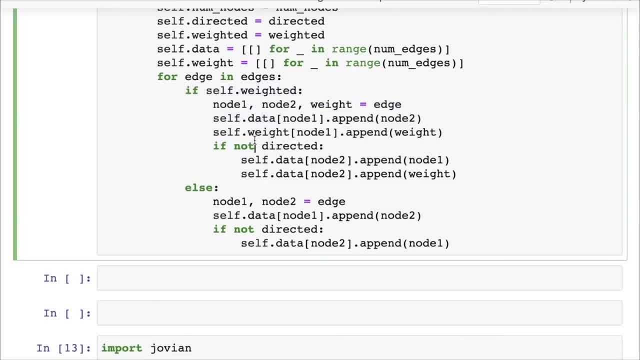 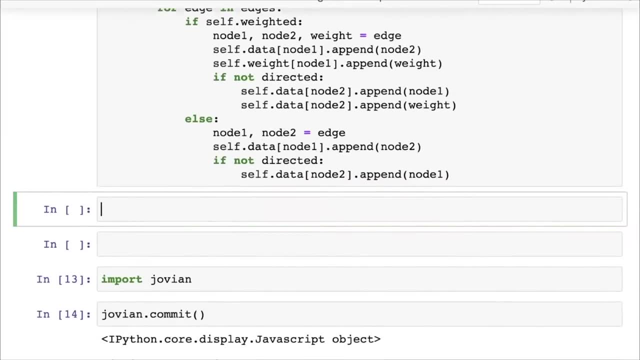 It's just a couple of things that we have to take care of, whether it's weighted or not, whether it's directed or not. But now that we've done this, we have a fairly generic representation for a graph, right. So now we can take this graph. 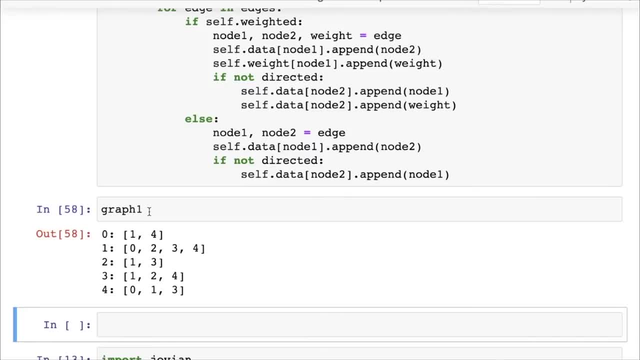 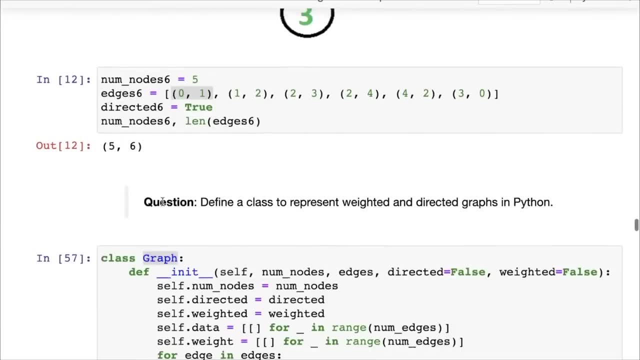 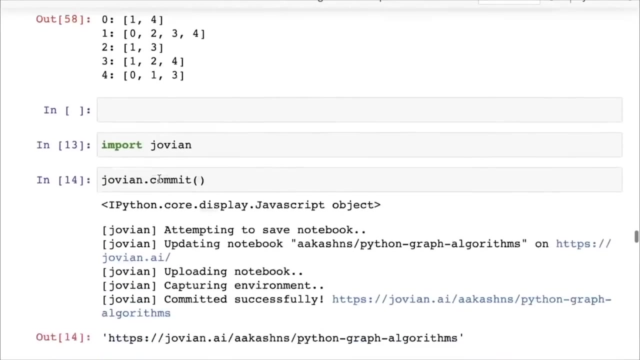 And remember graph one. the graph one had this information. So, similarly, we can take, we can create this graph, or we can use this graph class to represent graph one, but we can also use it to represent one of these, which is a dry directed graph, a graph with weights or a graph with directed edges, or a graph with both, a graph with both weights and directed edges, which we'll see in just a moment. 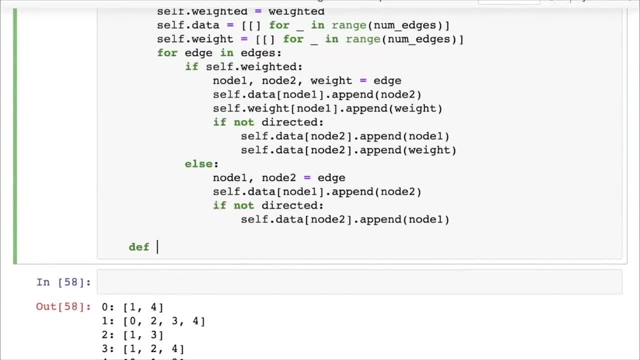 Now, one thing that we'll also do here is create a nice representation. So let's just create a representation here. Now I'm not going to get into the code of this, but roughly what we want is we want, while showing the graph, if there is a weight, we also want to show the weight. 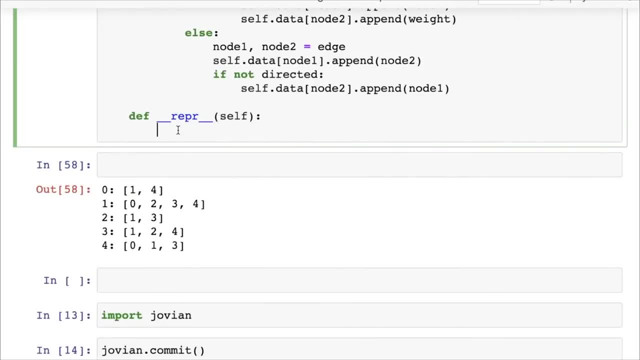 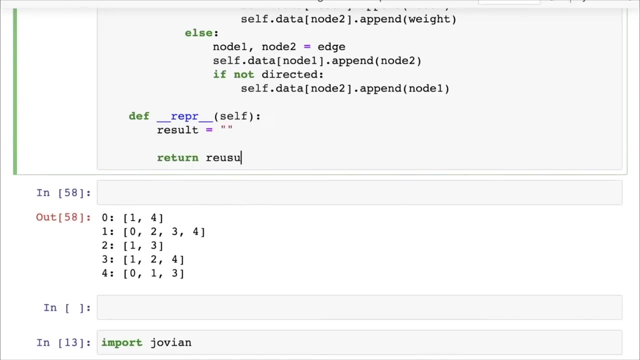 We'll show the weight alongside the other node. So let's see we create a result. The result will be this: the empty string, and then we'll return that result. Then we are going to say form Or I, comma nodes, comma weights in enumerate self dot data and self dot weight. 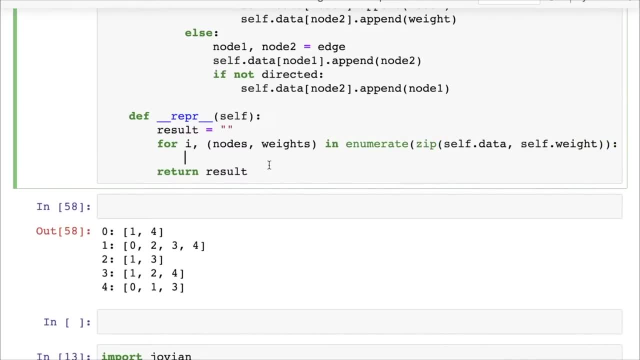 So now this is an exercise for you to figure out what exactly this is doing, and you can apply the exact same technique. take, create a new, create a new cell and put this data into a cell, put the zip into a cell and then see what that represents. 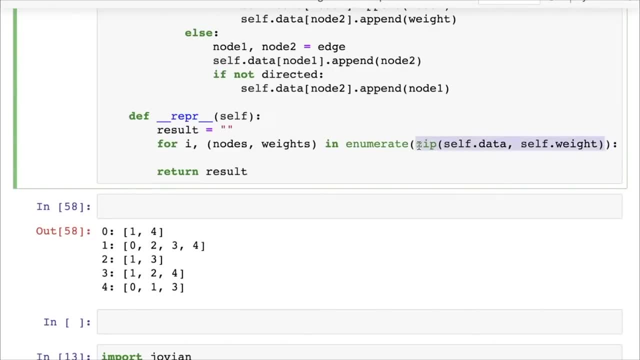 If, if you're not able to, if it doesn't show, Then try converting it into a list or using it in a for loop and then put, enumerate around it and see what that represents, so that you understand what I nodes and weights represent. but I am simply going to write it here so that you see the final result. 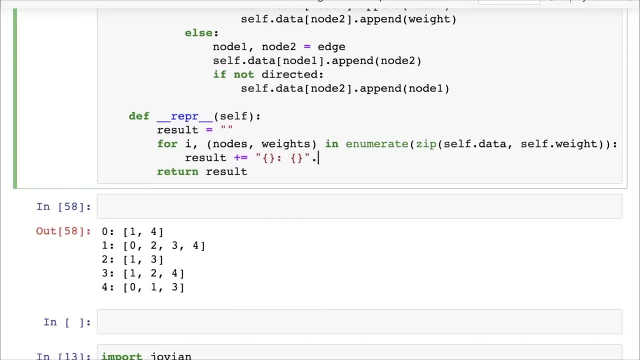 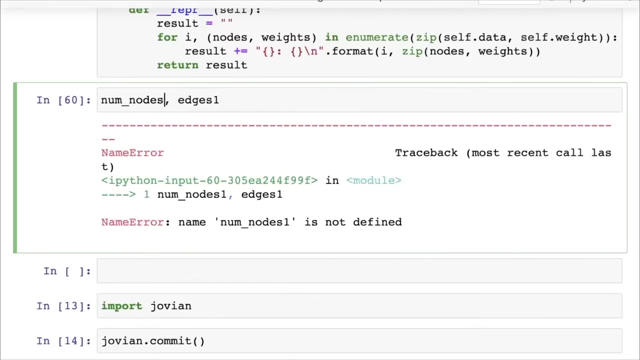 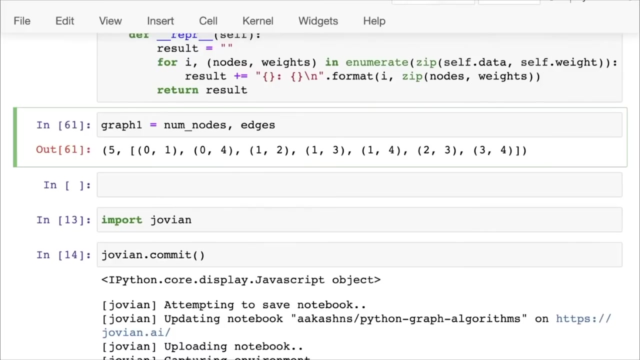 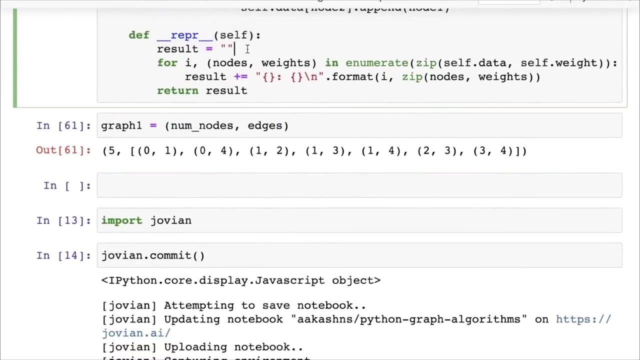 Okay, Okay. So let's take nom nodes one once again and edges one. it was called nom nodes and edges, So this was the initial data data that we were working with. Let's create graph one, And of course, we want to do this only if it is weighted. 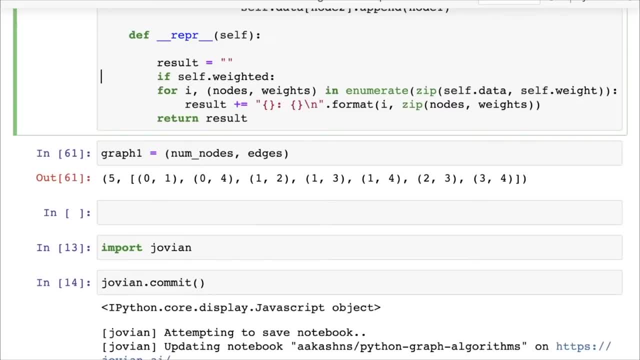 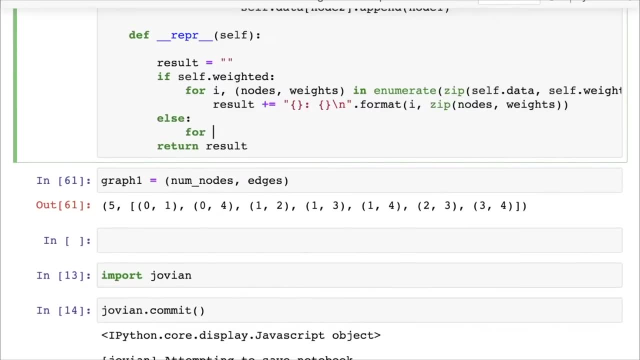 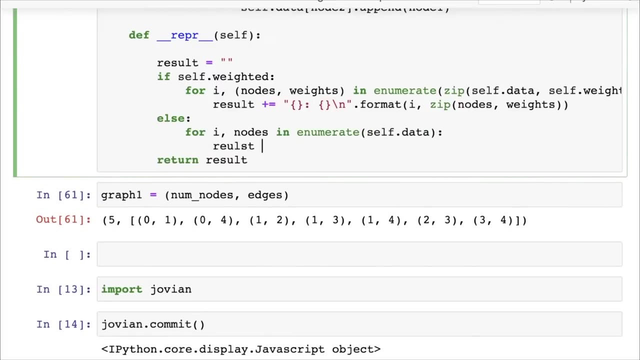 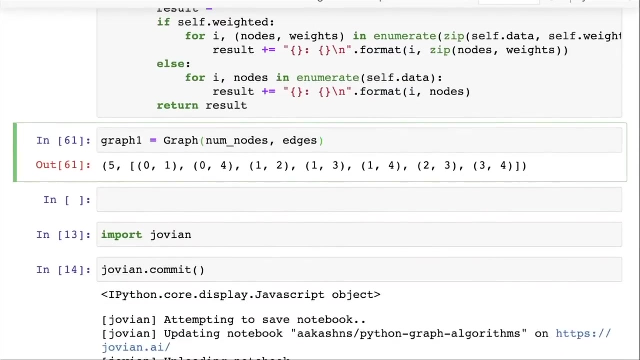 So if self dot weighted, if it is not weighted, then we have a different case where for I comma nodes in enumerate self dot data. Let's create graph one: Uh, result plus equals. Okay, let's see So graph one. we are going to use the graph and we're going to pass nom nodes, edges and, by default, weighted and directed are both false. 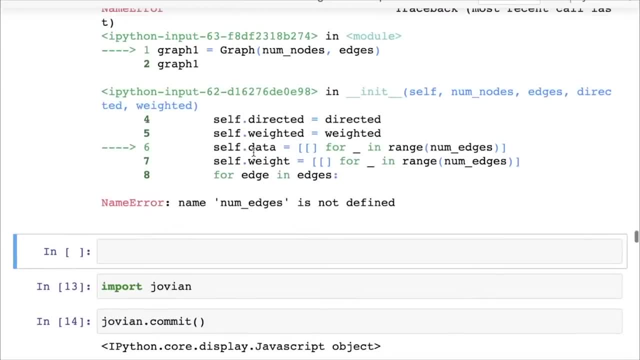 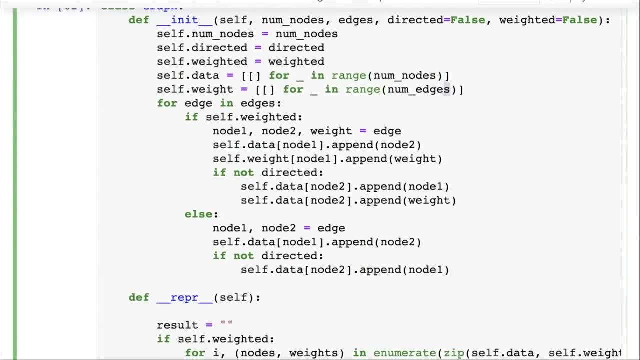 So we don't need to specify them. and let's see Graph one. So you can see, with live coding we always make mistakes and it's almost always bound to happen. That's where Jupiter notebooks are very helpful, And it's always helpful to just test your function while you're writing it. 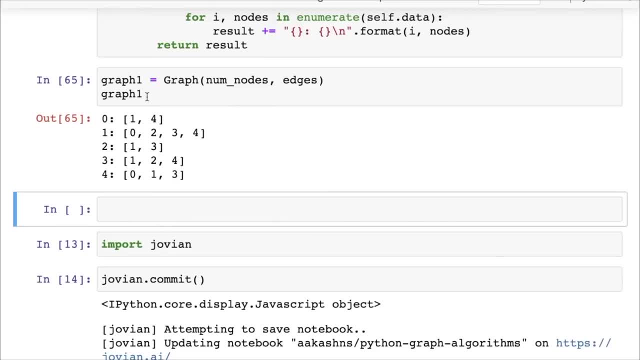 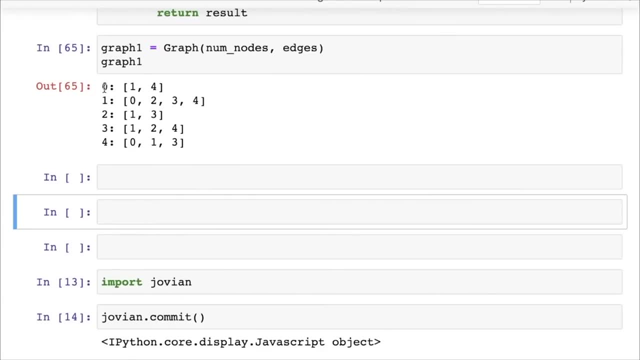 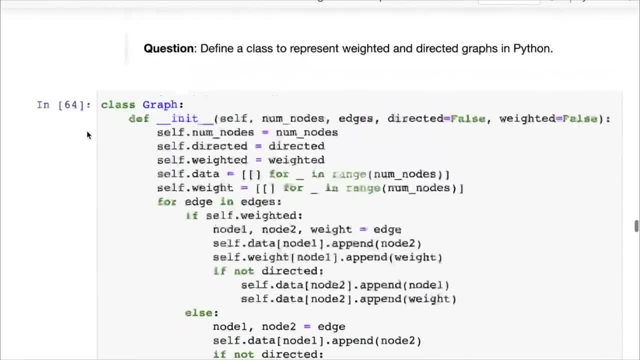 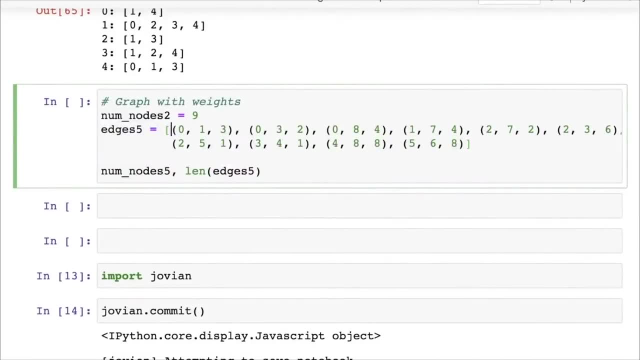 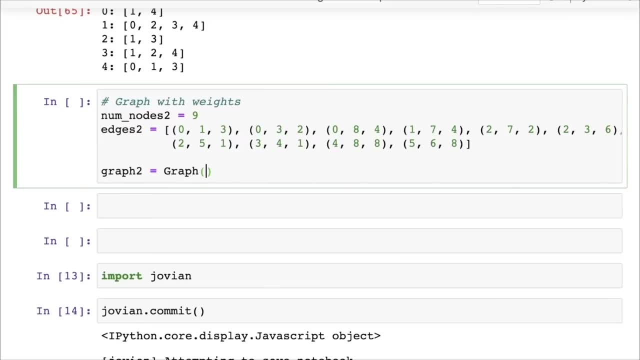 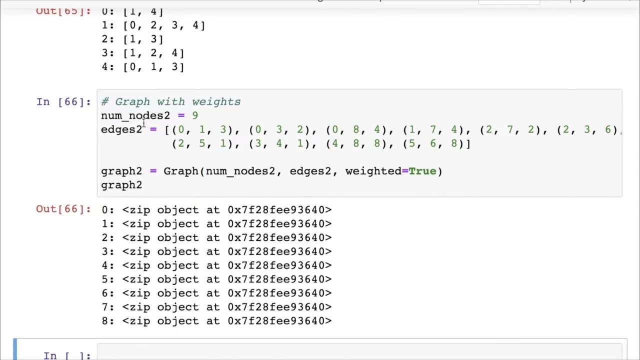 So now let's create a graph to graph, And here we pass in num nodes to, edges to, and weighted equals true. And let's say graph two, So we can do the same thing with the other two. Okay, There's a small change here. 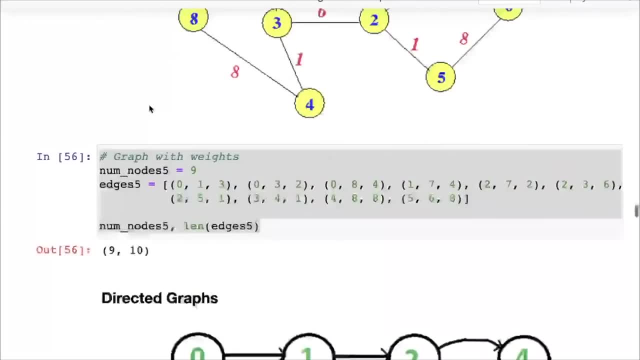 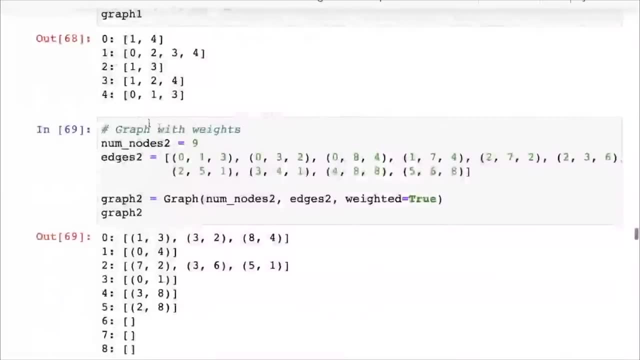 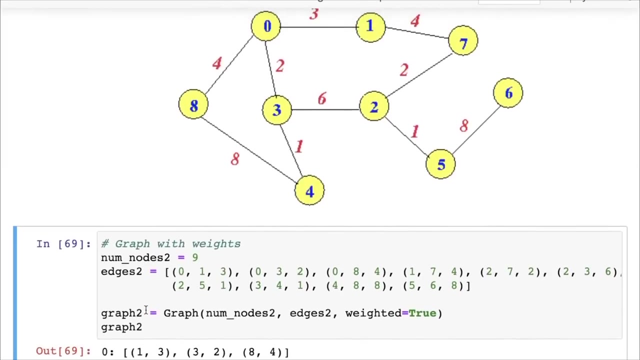 Yeah, So now you can see. for graph two, this was the graph we were looking at here, This graph, Let's grab this image as well. Yeah, this is the graph that we were looking at and you can see that zero is connected to one and three. 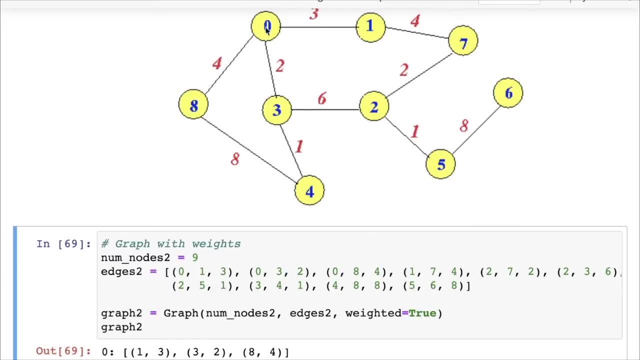 And so zero is connected to one, three and eight, one, three and eight, And there are also weights associated. So zero one has the weight three, zero three has the weight two, and zero eight has the weight four, and so on. 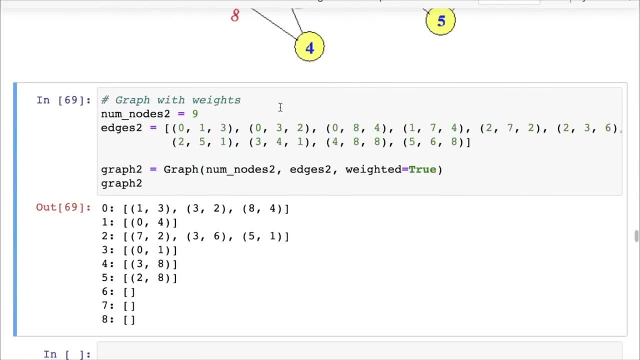 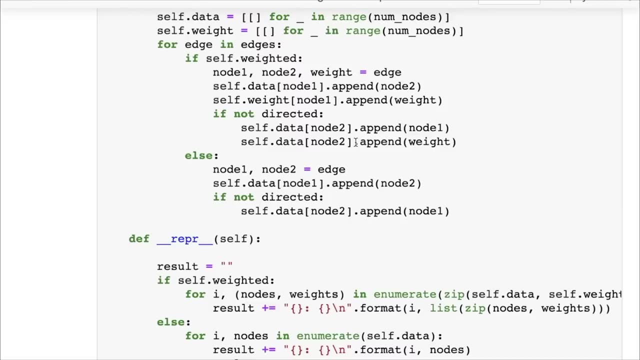 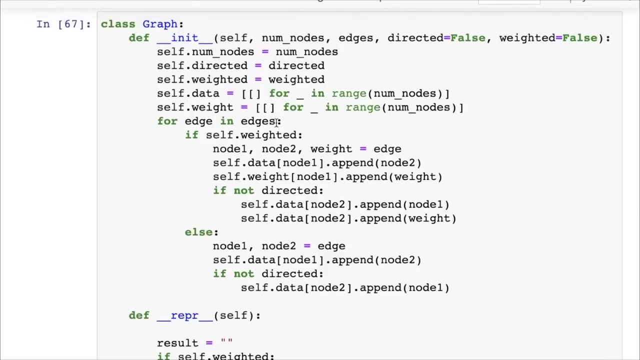 There seems to be something off here, because zero one only seems to be connected to zero. I think we may have made a mistake somewhere in the code. Okay, So we may just have to debug this code. It seems like we may have made a made a small mistake somewhere, because zero one one seems to be connected only to zero, but one should also be connected to seven. 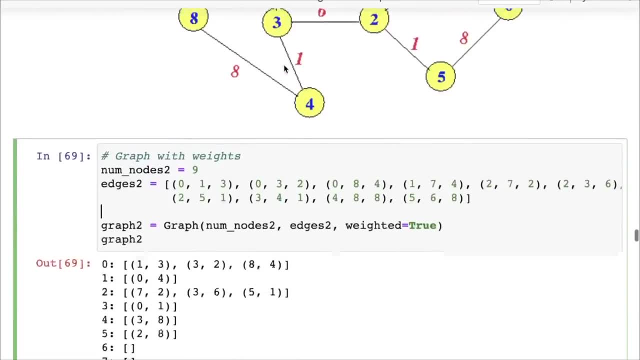 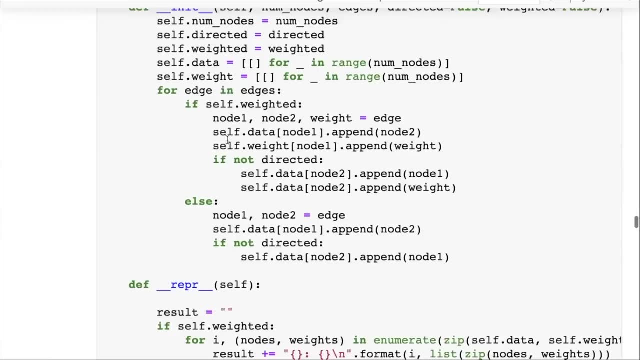 I don't see why that did not show up here. This is the curse of life- coding- and that's why I have created a new one. So I can see that the code is not connected to zero. So I can see that the code is not connected to zero. 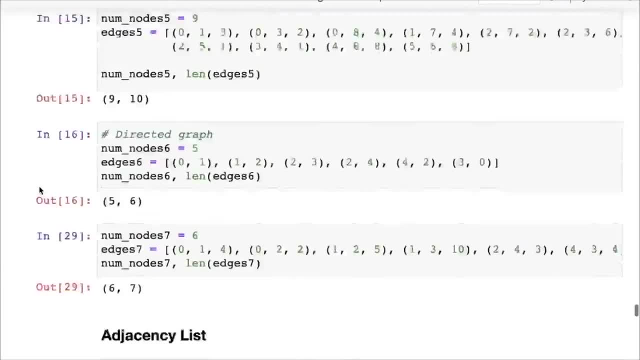 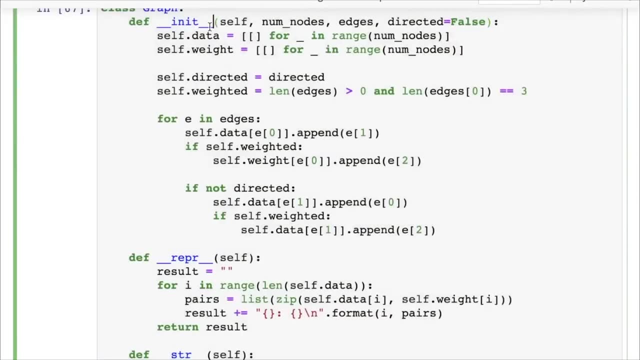 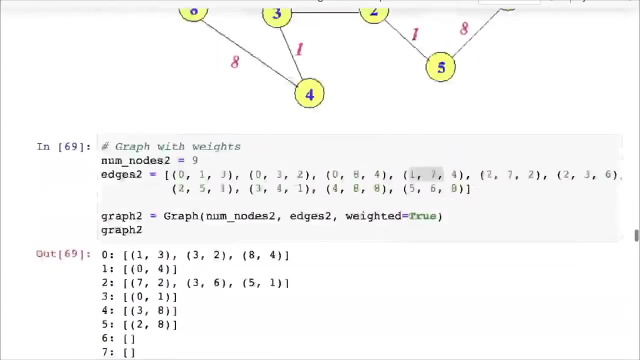 So I can see that the code is not connected to zero. Well, let's just check it, Let's see. Okay, So I can see that I have detected a working. I have some working code here. I'm simply going to grab the working code right now and we'll just replace that, but see if you can detect the bug in the code. 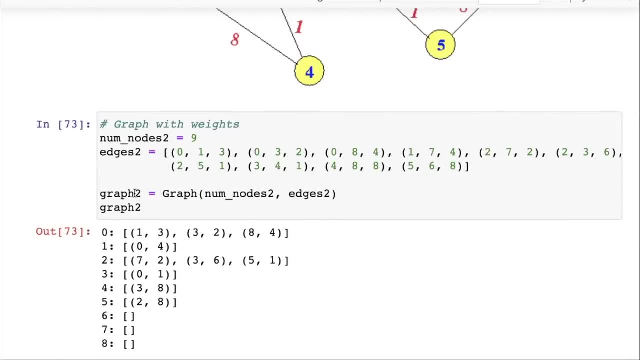 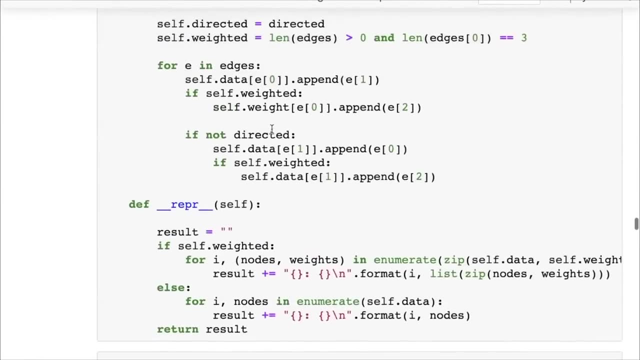 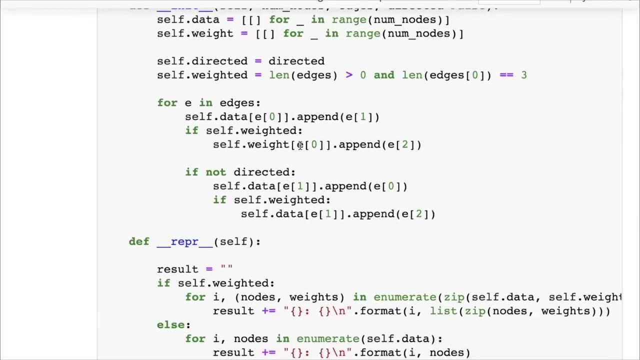 Okay, We don't. the version I have does not require you to specify weighted, so we can simply skip weighted here. It detects automatically If the graph is weighted going wrong. So we are going through the list of edges here and we are appending. 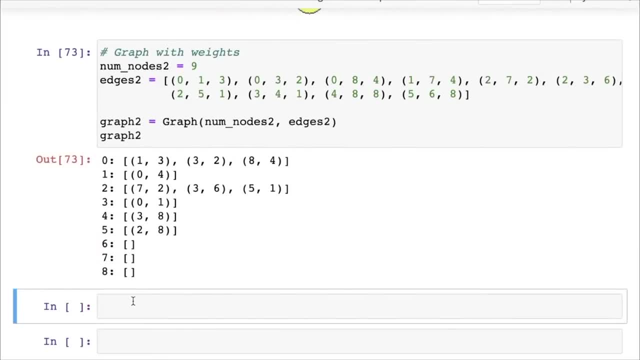 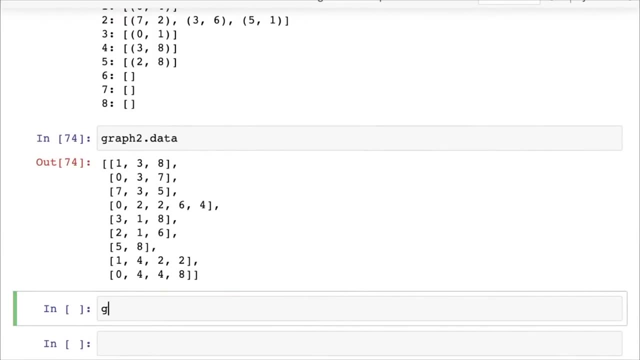 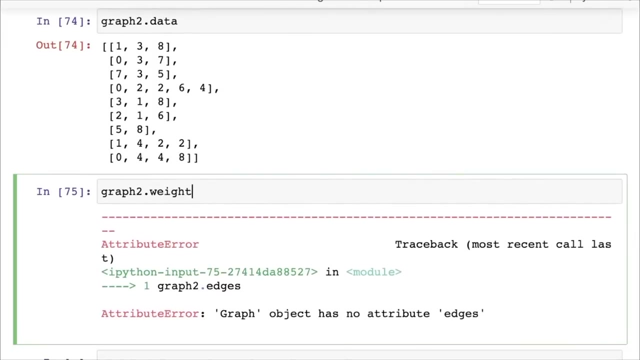 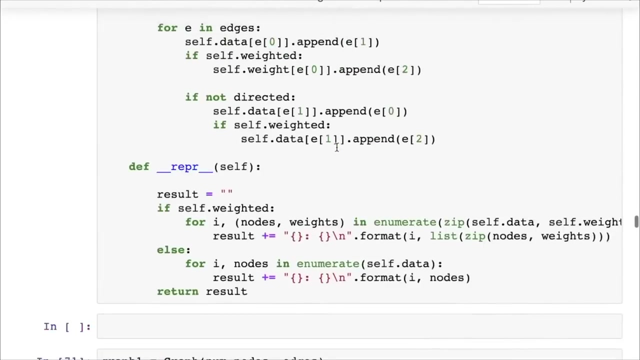 Maybe let's just print: graph two dot. graph two dot data. maybe the issues in the representation and not in the code. graph two dot edges: There seems to be some issue in the weight here, but we may not have inserted the weights correctly, I see. 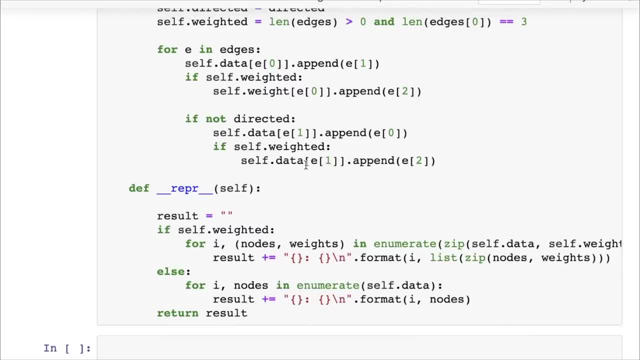 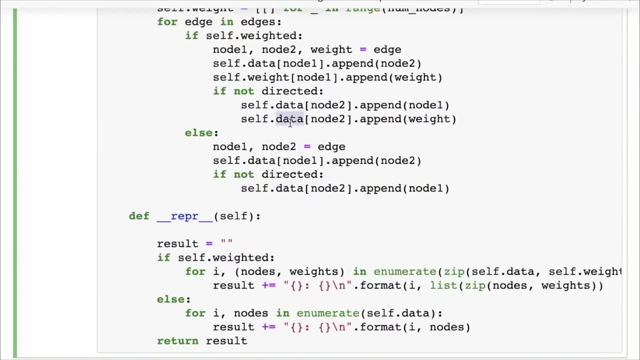 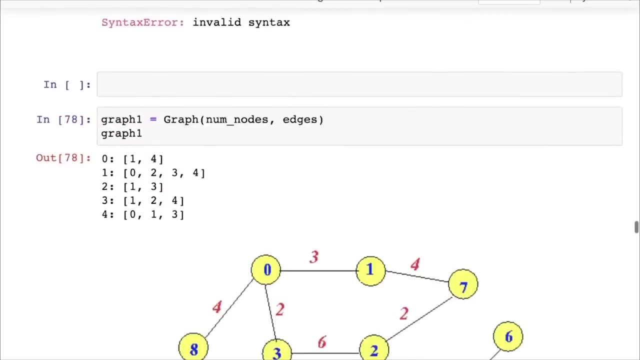 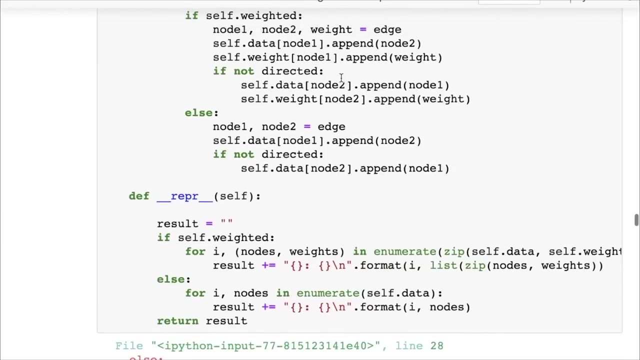 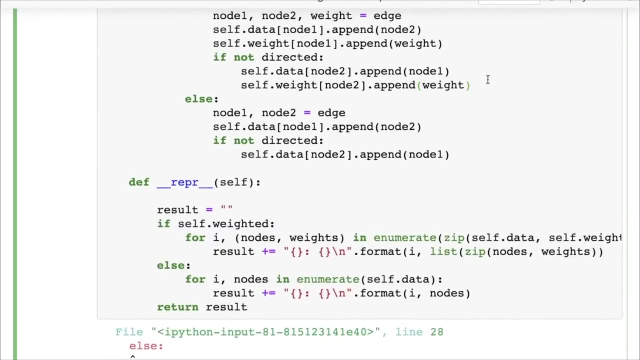 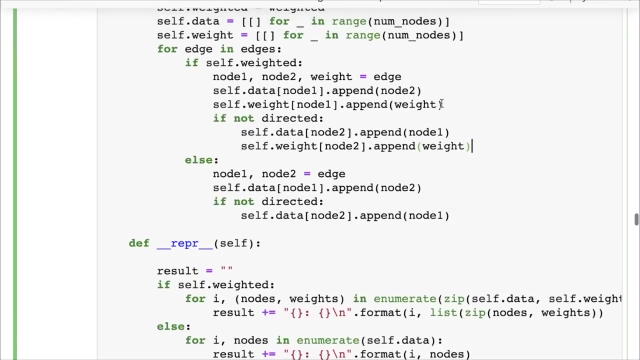 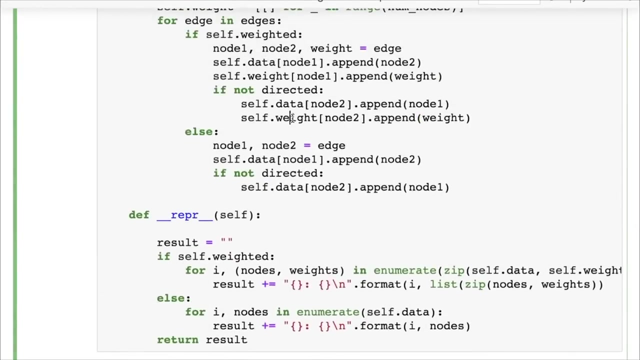 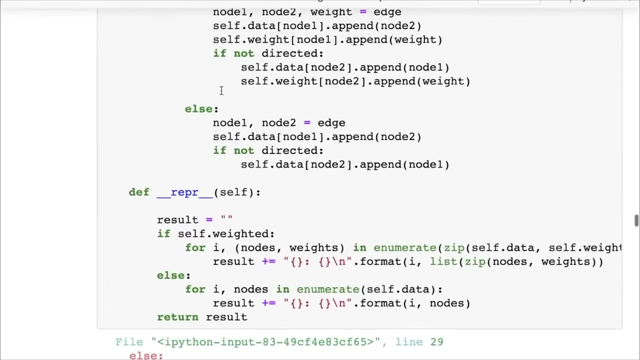 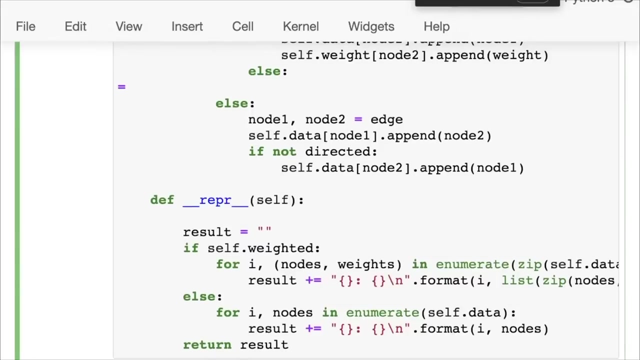 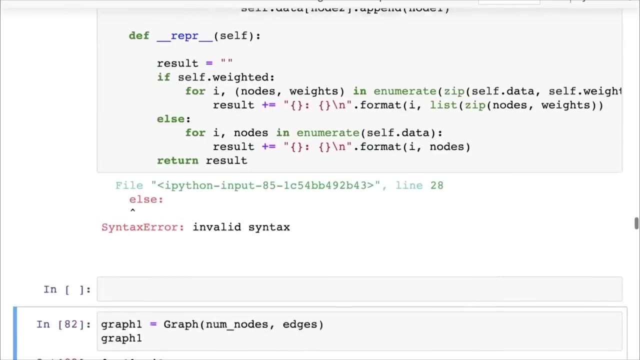 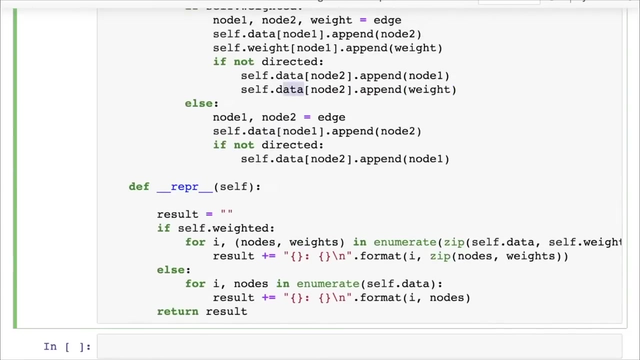 So this should be called weight, This should be called weight. So this should be called weight, And so should this be called weight. or there was a syntax error here? Let's see. Okay, I think we fixed it. Finally, Let's see. 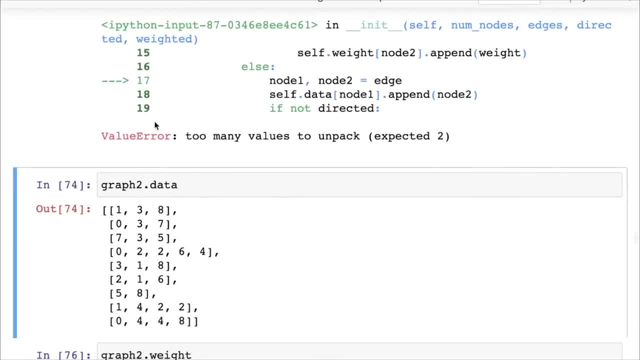 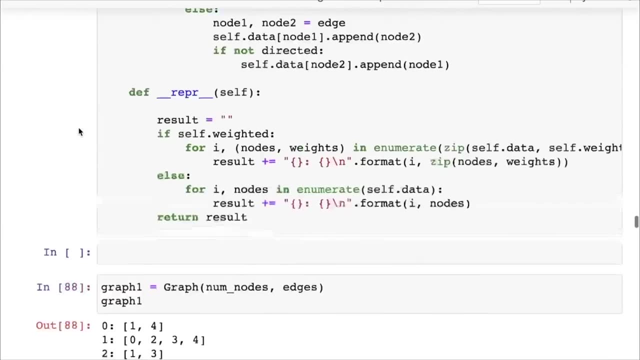 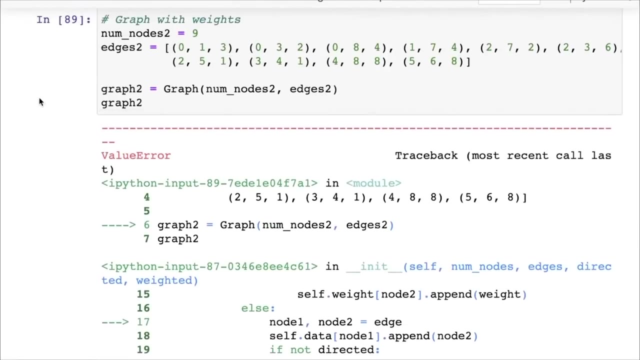 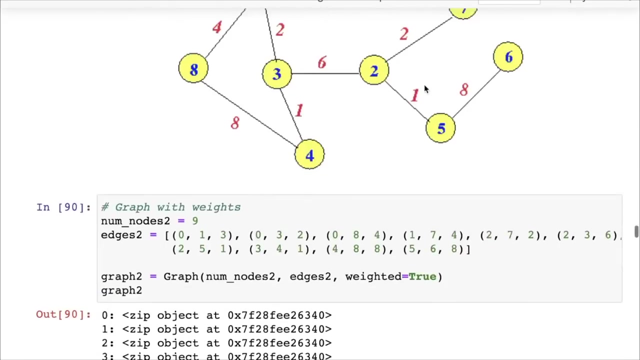 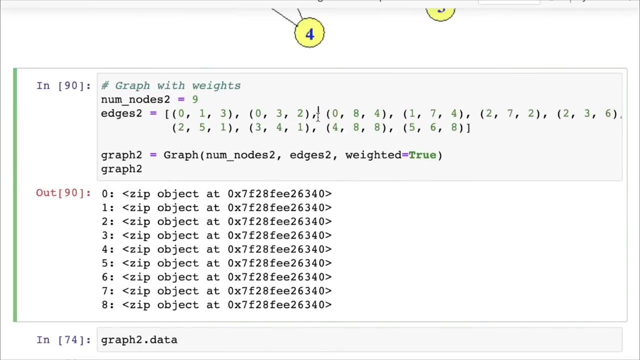 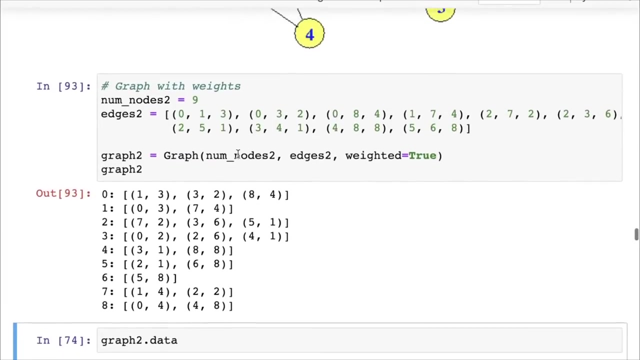 This should be called weight. So we have an edge here. We have too many values to unpack? Ah, we simply pass. weighted equals, true? finally, And we need to make this a list, It's finally done: some good, hardcore, live debugging, but we have this finally and again. 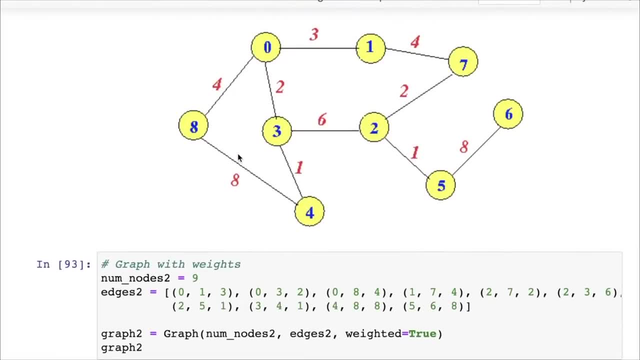 you get to see that when you're coding you will fail, You will make issues. You just need to. but if you have a clear idea of how you've written the code, it's easier to narrow down the issues by looking at the errors. but let's see this graph here. 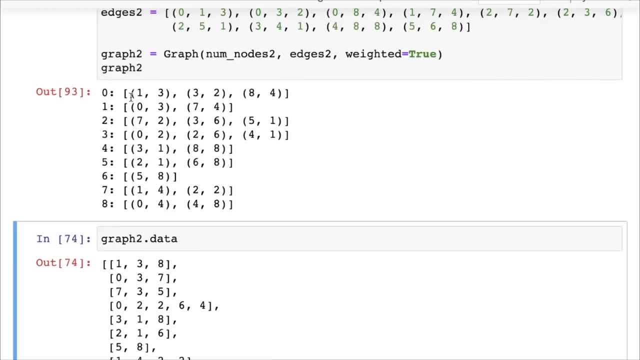 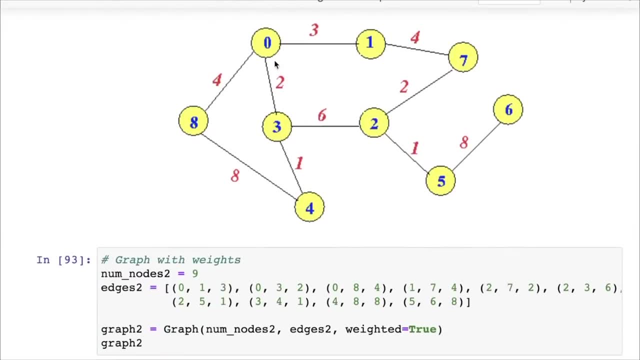 So we have zero connected to one, three and eight, And that's, you can see that here, one, three and eight. a zero connected to one, three, eight, with the weights three, two and four. Then we have three connected to zero, two and four. 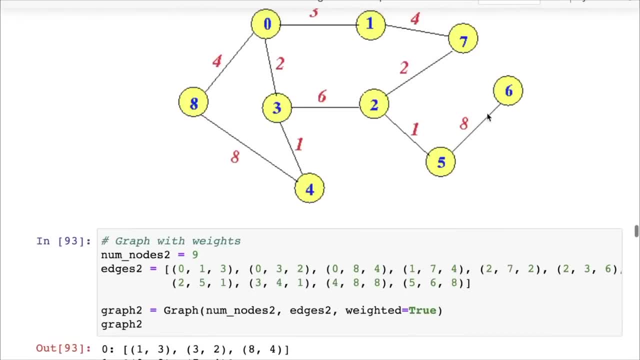 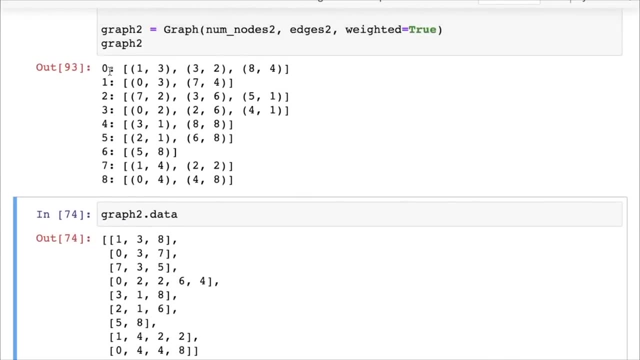 So we have three connected to zero, two and four, and we have six connected to five and eight. You can see six connected to five with the value eight. So great, We have now represented a graph properly, and this is why a representation is really. 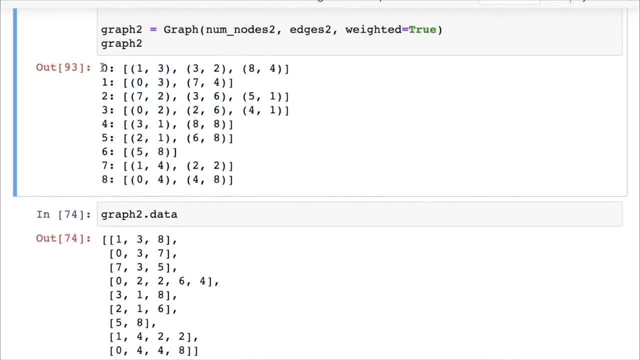 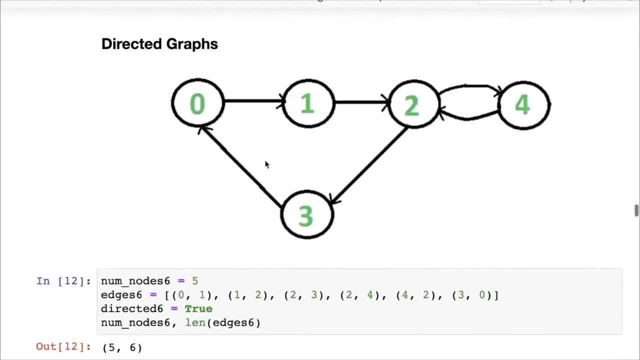 useful because now we can check if our implementation is correct before we go on and implement any graph algorithms. We can check if our representation is. Let's try one more. Let us also try this directed graph. So we're going to grab this code and put it here. 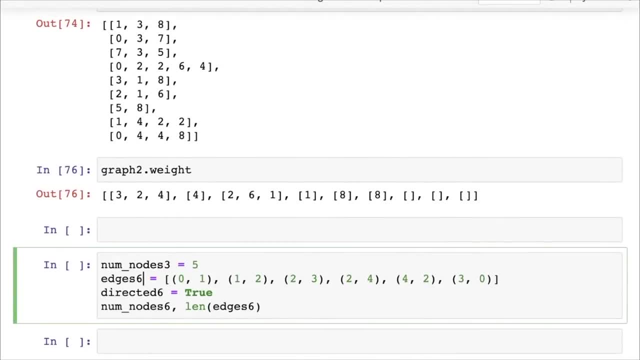 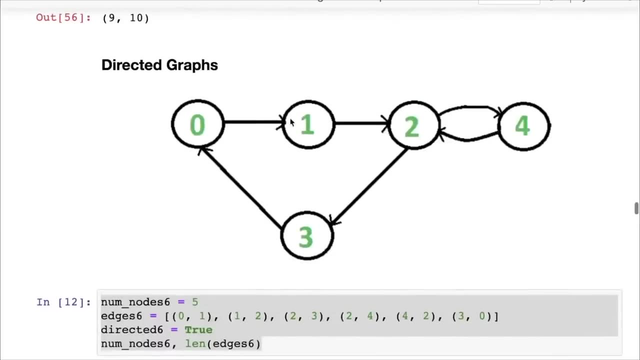 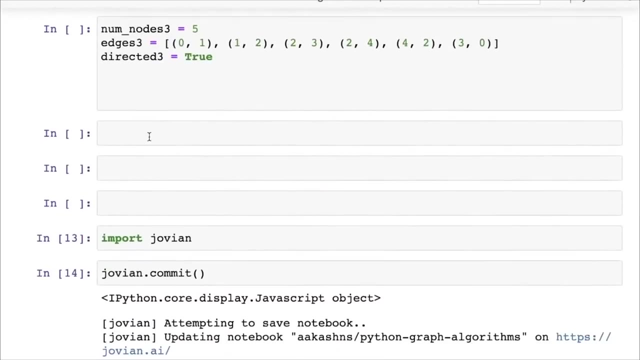 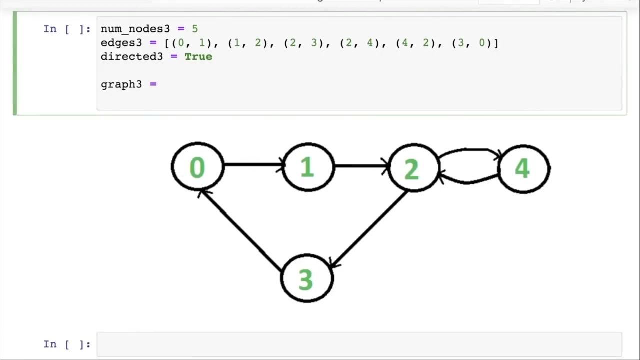 Let's call this num nodes three, edges three and directed three. Let me grab this graph code here as well. We're working with this graph And let's create graph three. so for graph three, we have graph and we pass in num nodes three. 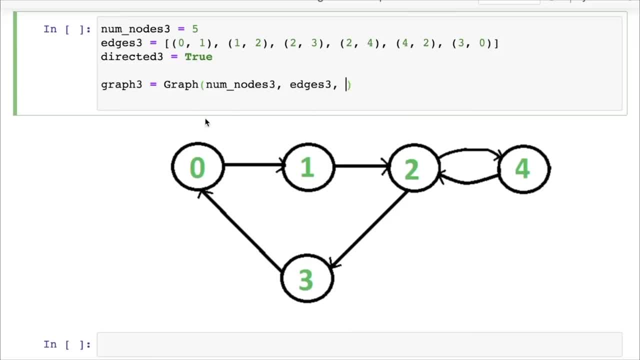 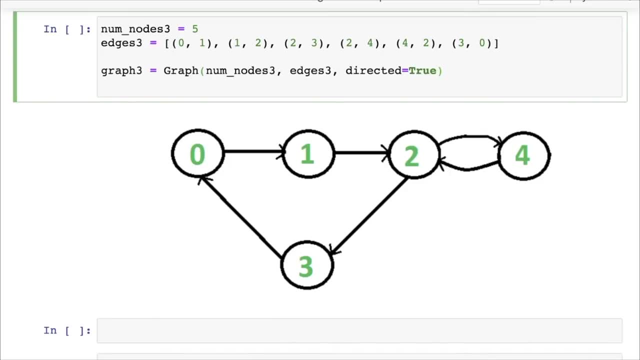 We pass in edges three and you can verify that the edges are set up correctly. And we just specify: directed equals true. So we don't really need this. at this point We can just say: directed through and weighted by default is automatically false. 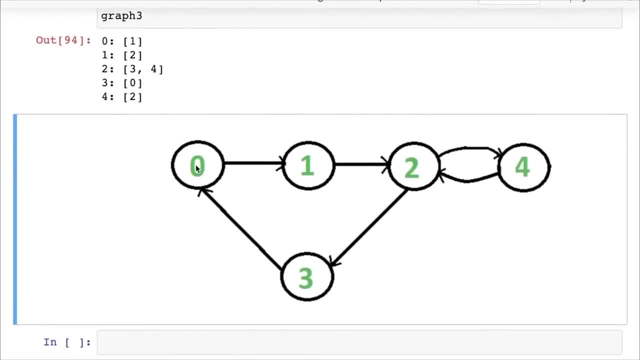 So we have graph three here You can see the zero is connected to one And one is connected to two but not to zero. So now we haven't inserted the opposite edge. and then two is connected to three and four, Then three is connected to zero and four is connected to two. 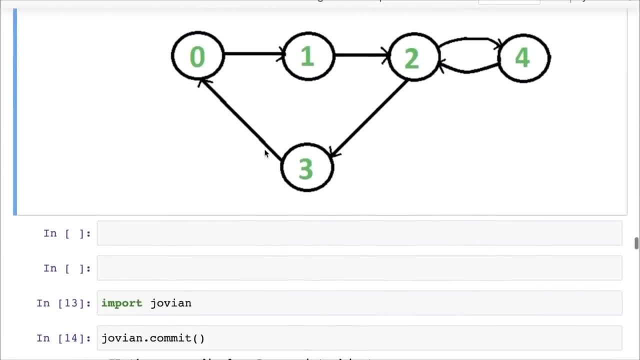 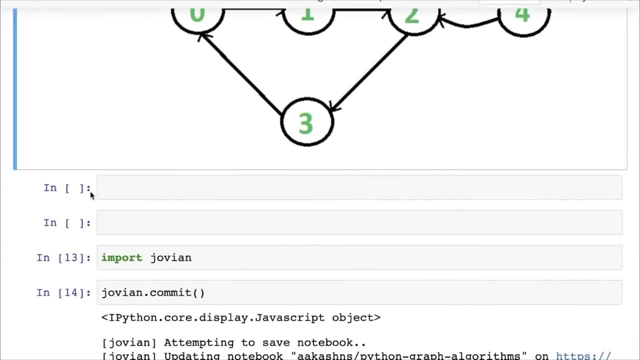 Great. So we've implemented. we've now set up another graph And now here, similarly, you can check that if you have a weighted directed graph, the code is still going to work fine. Okay, So that's an exercise for you. 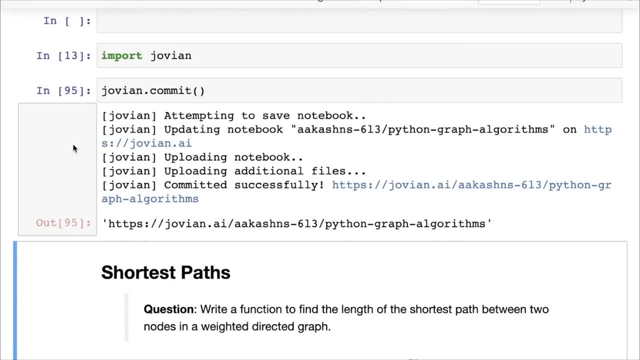 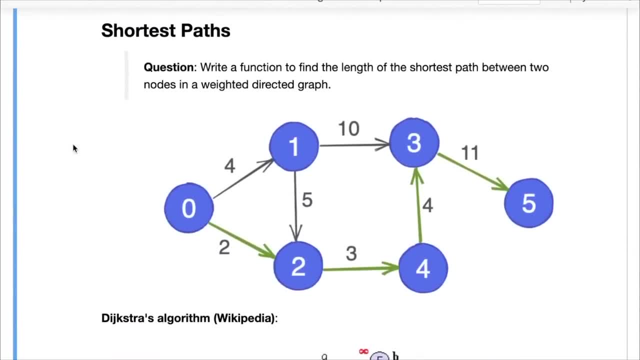 Okay, Okay, Okay, Okay, Okay. Next question that we're going to look at is called the shortest path question, And this is really what we started out with. Let's say, you have a bunch of nodes and this is. we've taken a directed graph here, but you need not have a directed graph. 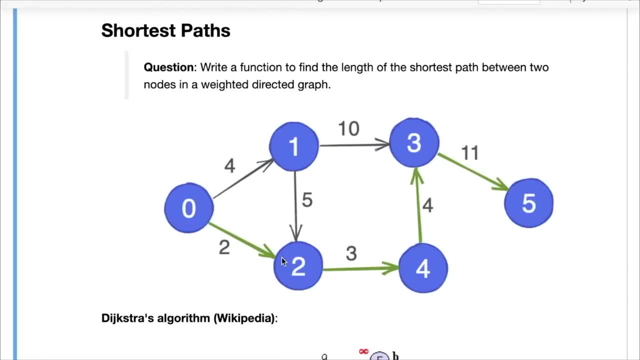 You can do this with an undirected graph too, and that will be an exercise for you, but you do need weights here. Now, whenever you're talking about shortest parts in terms of weights, that is when this algorithm makes sense. Now, if you do not have weights in the 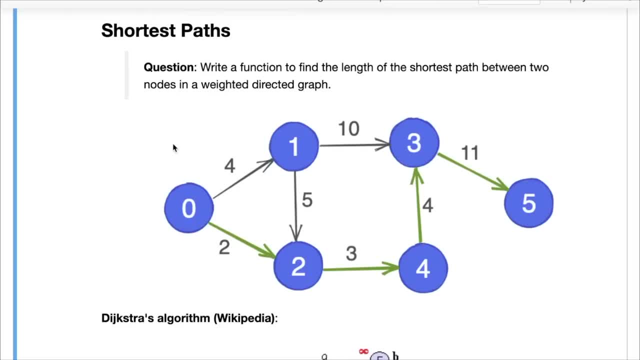 Graph, then the shortest path can be found simply by performing breadth first search. Okay, So whenever you're asked to find the shortest path, the first question you should be asking is: is there a weight involved or are there no weights? Now, if there are no weights involved, then we're simply concerned with the length of the path, the number of nodes in each path. 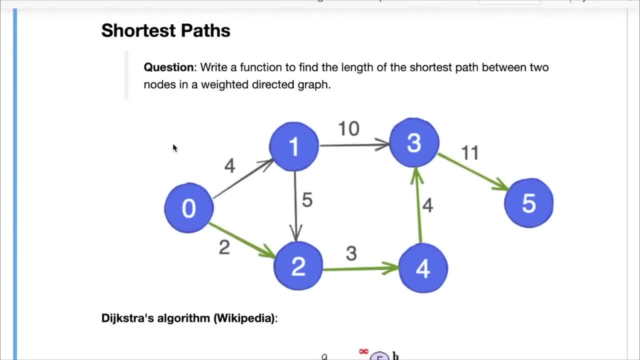 And in that case you can simply perform a breadth first, a breadth first search. But if you have weights, whether it's directed or undirected, then the breadth first search alone may not be enough right? Because It may turn out that certain paths- for instance, you go from zero to three- 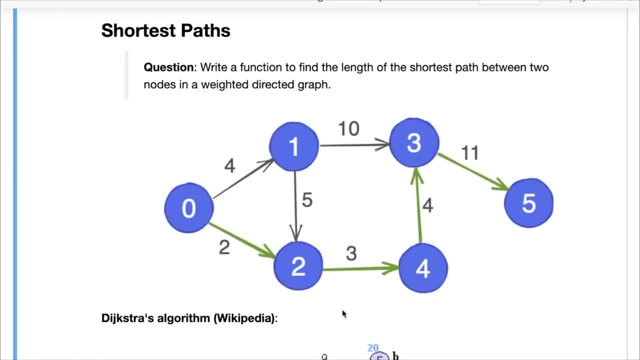 So you say you go, if you go via zero, two, four and three, the length of the path is two plus three, five plus four, nine. But if you sorry, the, yeah, the total size, the total size of the, the length of the path is two plus three, five plus four, nine. 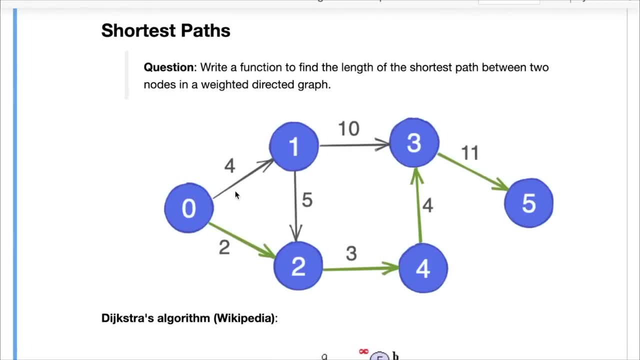 But the number of nodes is four: zero, two, three, four. On the other hand, if you go via zero, one, three, in this case the number of nodes is smaller, So there's just one One in between. 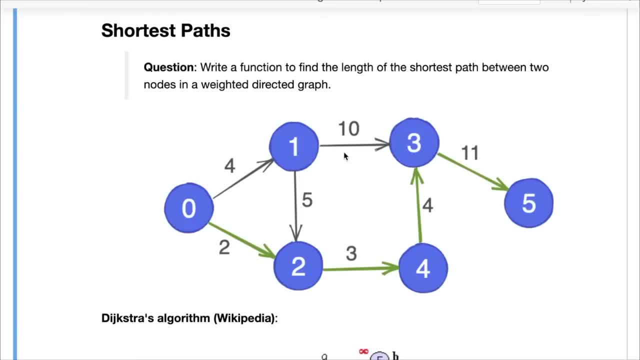 So zero, one, three. there's just three nodes total, but the length of the path is 14, which is far higher right. So this could represent that you go to a far off place of via a train and then take a train to something that was actually closer even. 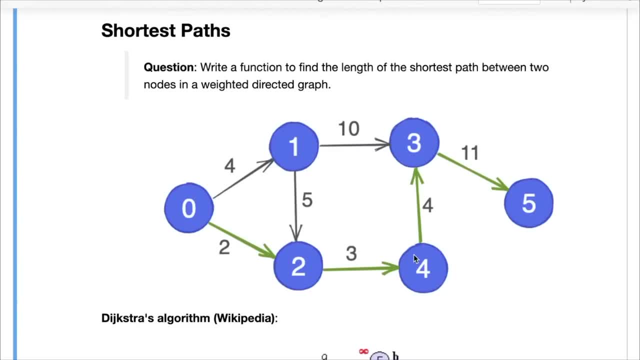 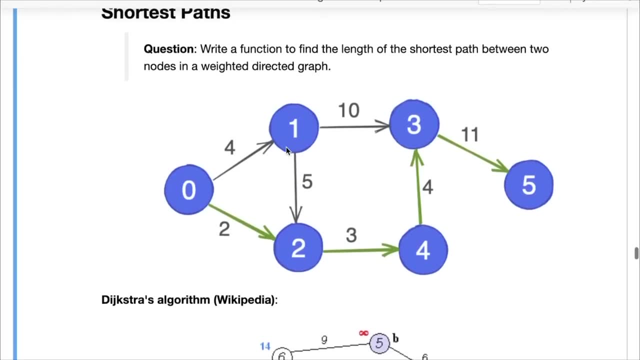 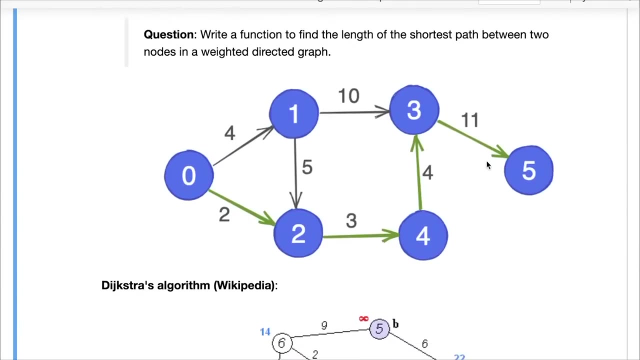 though there were more stops in a different route. Okay, This is what we're going to implement. Now, we're going to implement an algorithm to identify the shortest path from a given node to a given target. Okay, So now, this time we are going to focus our search between a node and a target. 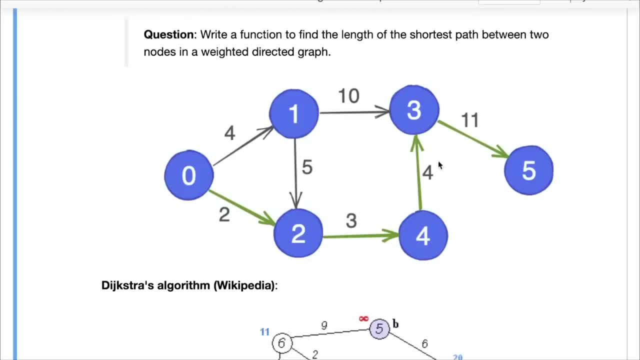 So what is the shortest path in terms of the total weight of the path, not in terms of the number of nodes in the path. Keep in mind what is the shortest path in terms of the total weight that we can find from a starting node to an end node. 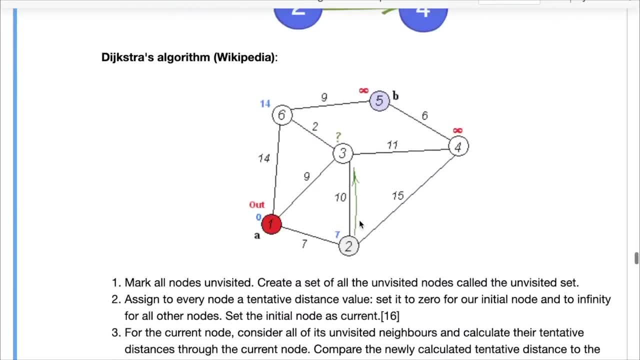 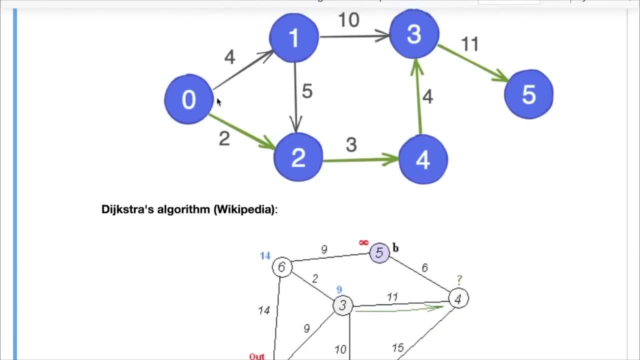 And roughly. the strategy goes like this, And the strategy is called the Dijkstra's algorithm, Lovely. The strategy goes like this: You have the source node, and the source node is at a distance zero from itself. So there's nothing there, really, but the first thing that we know, the first and the only thing that we know, is that for one of the siblings, 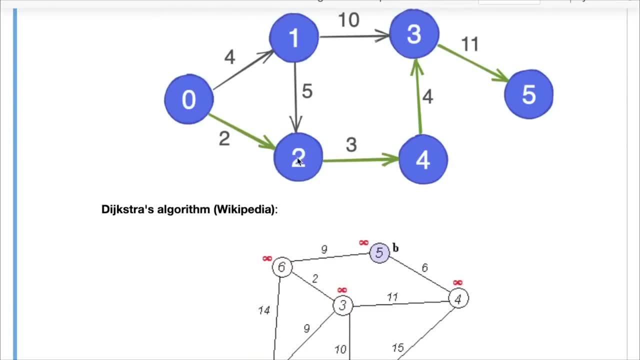 for one of the neighbors of the source node, the direct edge will be the shortest path. So, for example, we have one and we have two. Now you are directed, You have direct edge is from. You have direct edges from zero to two. 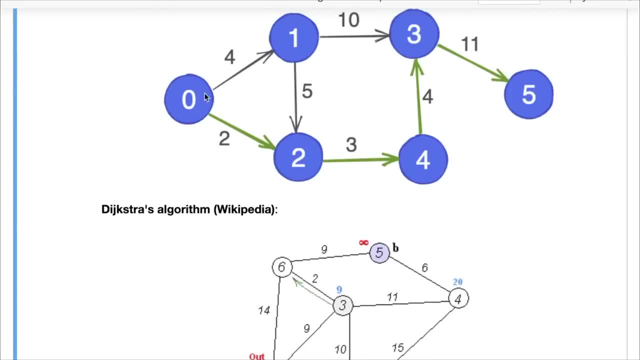 And you have a direct edge from zero to one. zero to two has the way to zero two. one has the weight for know. in this case, suppose we had an edge from two to one and that edge hate had the wait one. then you could go from zero to two. 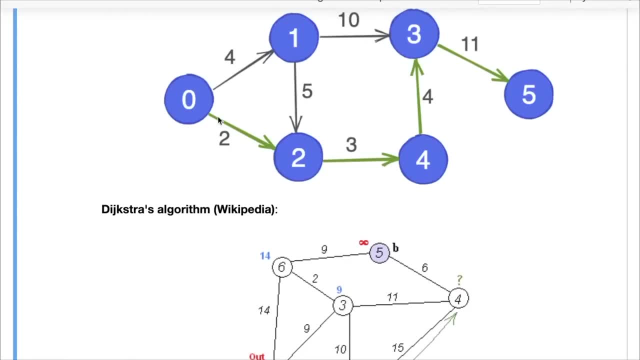 with the weight two And then go from zero two to one. Hmm, Little bit better, Yeah Yeah, But that is weight one and the total weight you would incur to get to one would simply be three, And that would be smaller than the short and smaller than the direct edge. 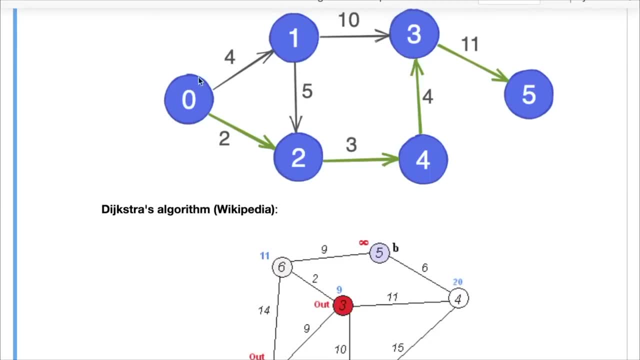 Right. So even if you're looking at direct connections of the route, we can't say that the direct edge is the shortest path, except for one of the nodes Right. So if we just look at the node where the edge weight is the smallest, 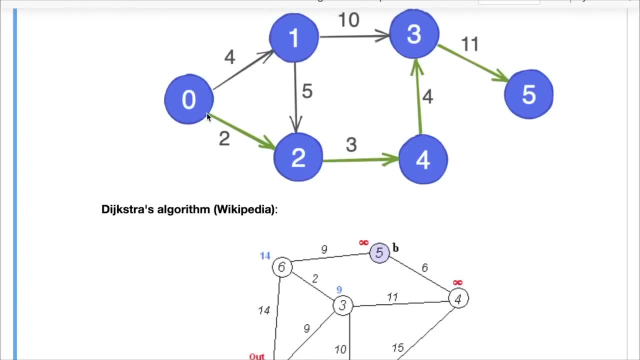 So you started the route and you look at the edge with the smallest weight, Then we can say for sure that the shortest path from the route to the next node, to the node two, is the direct edge. Why? Because this direct edge is smaller than, or smaller than equal to, any other direct edge. 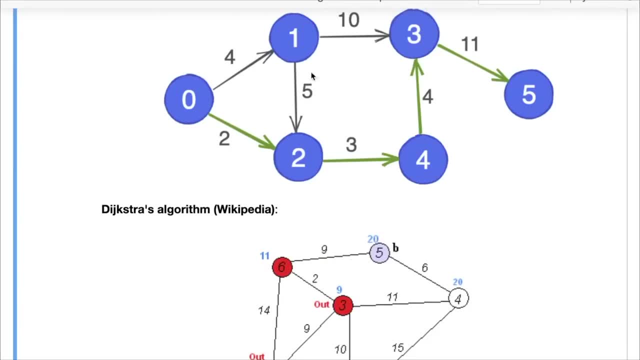 So any other path that comes to do indirectly will contain an another direct edge and then some other edges, right? So it will have a length greater than or equal to this direct edge. right? So that's the key insight Here: That at every point you maintain a group of visited nodes. 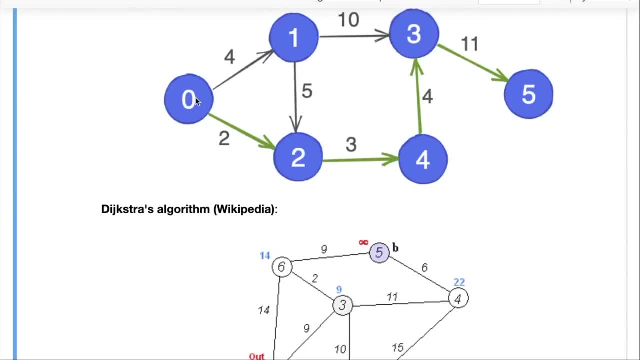 So in this case, initially just two, zero is visited, and then you find the first node which is at the closest distance from any node within the visited group. Okay, So, for example, if we start out at zero and then we look at one and we look at two, we 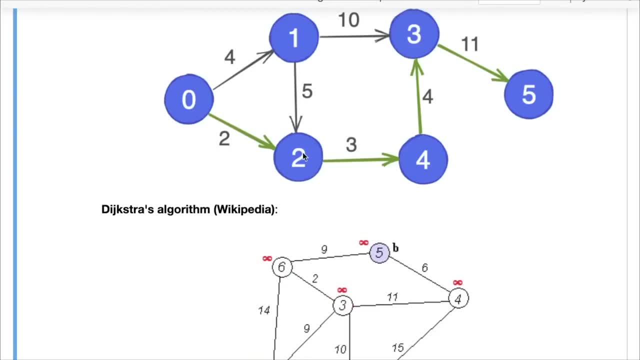 see the smallest edges too. So we add two into our visited group because we know that this is the shortest path from zero to two. And at this point now we take all of the siblings or all of the neighbors of two and update their weights now because we know that zero to two is, as a direct, shortest path. 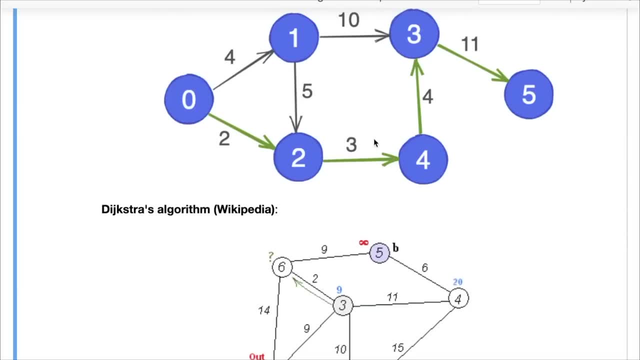 So we can update the distance for four. that four could be at a potential distance of two plus three, five or there could be a shorter path. So we've not yet added it, We'll just update for and similarly, if there was a edge to one, we can update the distance. 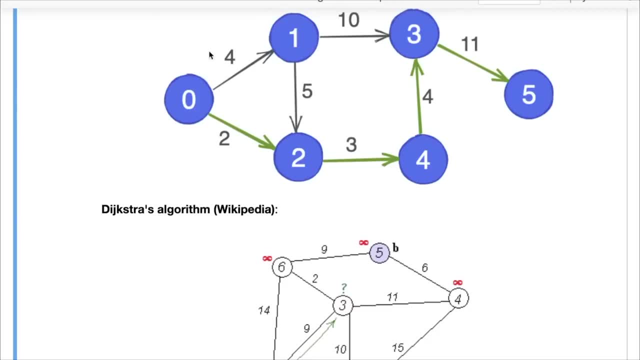 of one, And we can say that the distance of one is Either four, which was a direct edge, or it can be two plus one, if there was a direct edge from one. So now we'll get to know that one is at a distance of three, which is smaller, right. 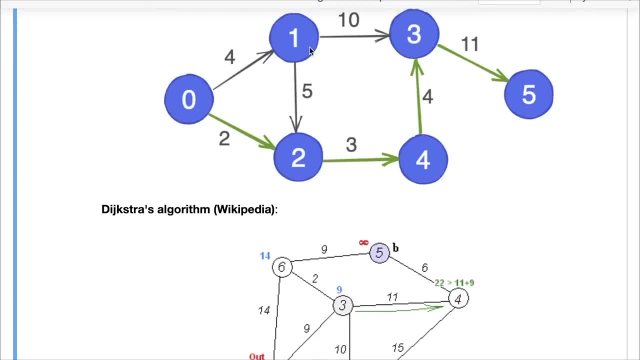 In this case it's not. but suppose there was a direct edge from two to one of weight One, we would get to know that one is at a distance three. So each time you add a new node, as you mark a node as visited you, you update the weights. 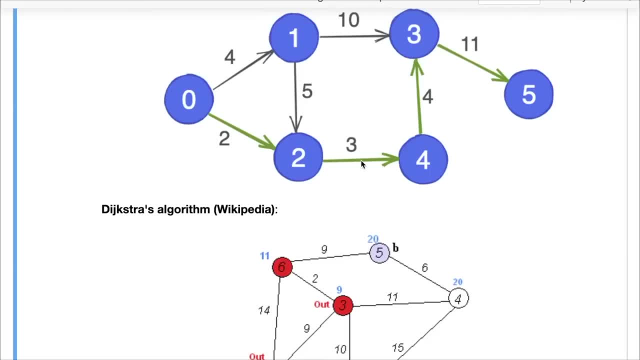 of or update the distances of all its neighbors, And then you simply find that The next node with the smallest distance right. So you will find that the next node with the smallest distance in this case is four, and then you update the neighbors of four. 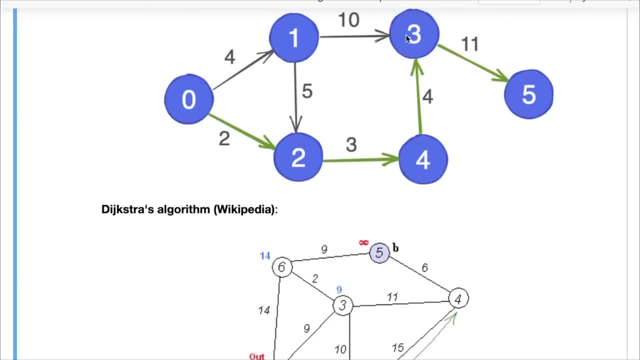 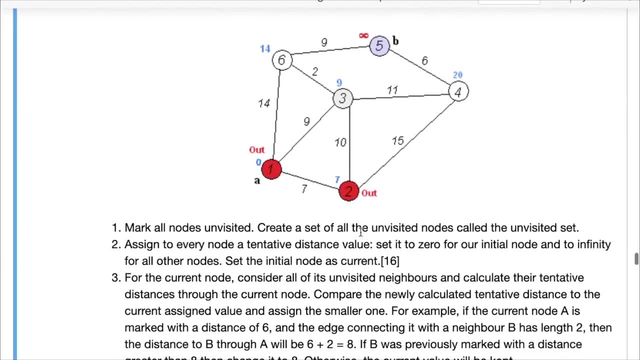 There's only one neighbor. The next node with the smallest distance is three. You update the weights of three and so on. So that was shortest path in a directed graph, but here let's see a shortest path in an undirected graph, where we have more such cases. 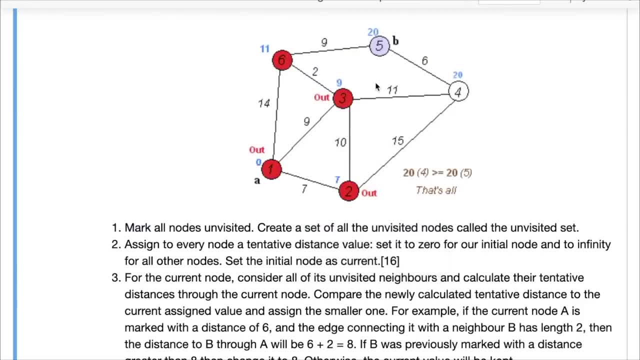 Let's just watch this from the beginning, Let's wait for the animation to start again. So we start at zero, then we check two. okay, we mark two is updated. Then we check nine, then we mark three as updated, Then we update the distance of 14.. 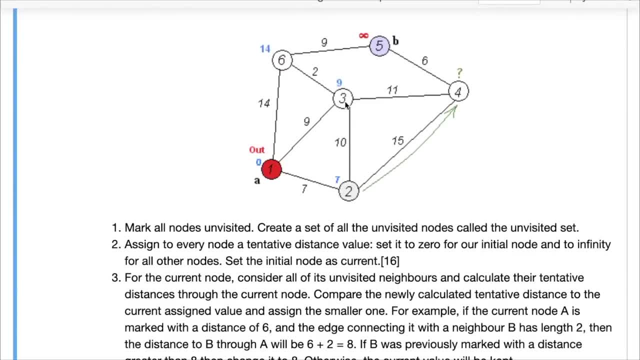 But now we can see here that we have another path: to go to two or we go to three. That's why we attract that And finally we get to. we mark two as visited. Now we are considering three and using three. We are updating the weights of all the other graph, all the other nodes. 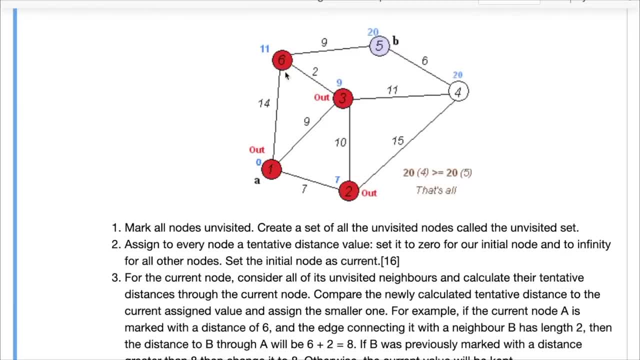 And then we are marking three as visited, Then we are using three to mark six as visited, and so on, right? So at each point you have a group of visited nodes and you have distances for all the nodes that are connected with the visited nodes. 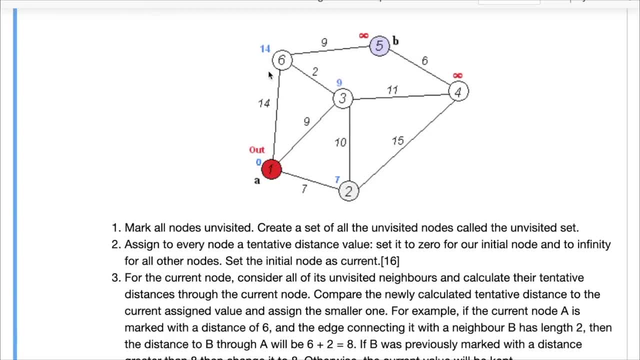 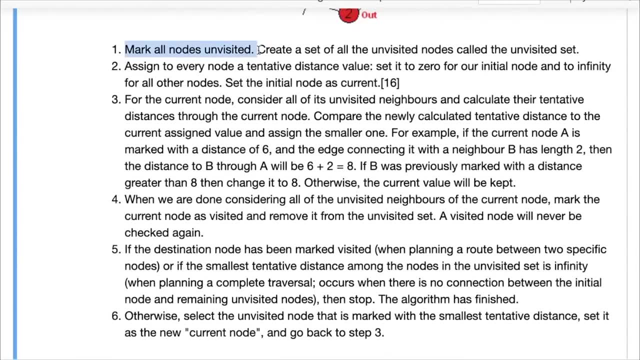 And then you pick the first unvisited node with the smallest distance. Okay, Now let's read the algorithm. You first mark all nodes as unvisited, and then you create a set of all the unvisited nodes and you call it the universal set. 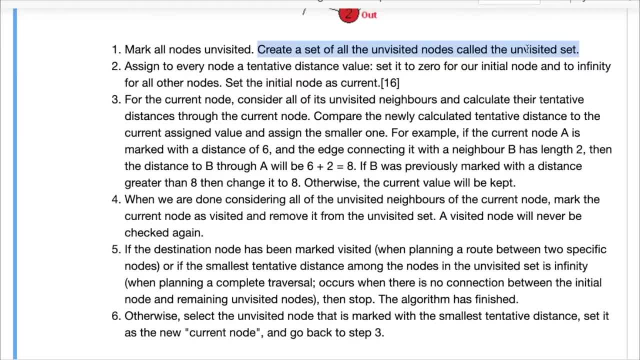 So a set of all the unvisited nodes. The unvisited nodes is called. the call it the unvisited set. assigned to every node a tentative distance value. Now set it to zero for the initial node, because the initial node is at a distance zero, and set it to infinity for all the other nodes. 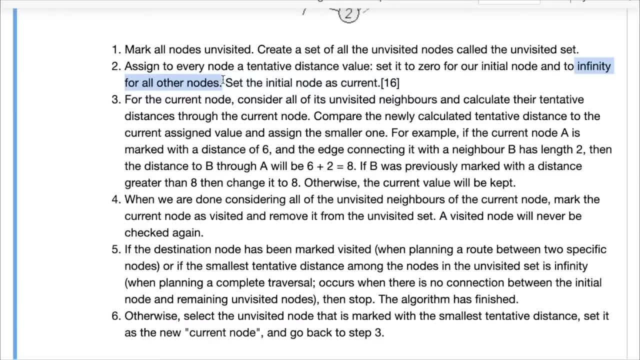 So we now set the distance to infinity, because we've not yet visited the nodes, We don't know their distance. Then you set the initial node as the current node. So there is always a current node that we're looking at. In this case, we'll start with the initial node. 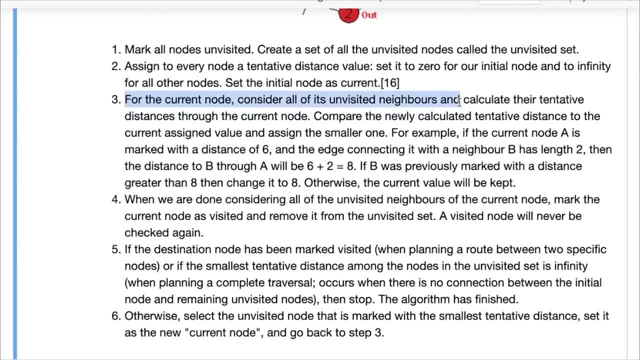 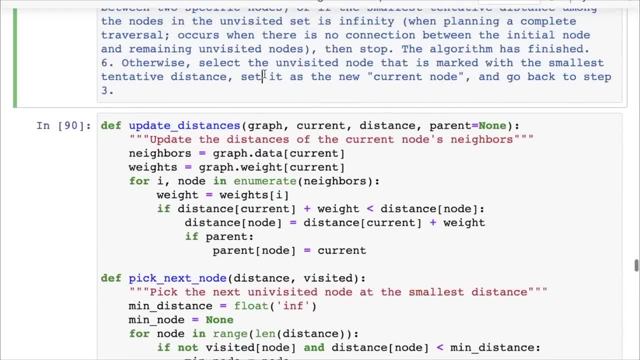 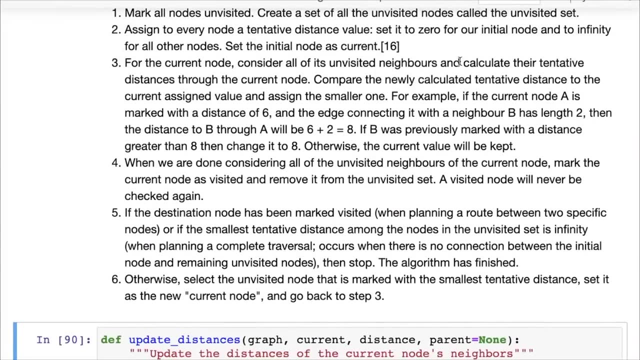 Now for the current node. consider all of its unvisited neighbors and then calculate their tentative distances through the current node, right? So you have the current node, and the current node is connected to a lot of unvisited nodes, And if we look at each unvisited node, we know the distance up to the current node, because the current node is visited and using that we can calculate distances for the unvisited nodes. 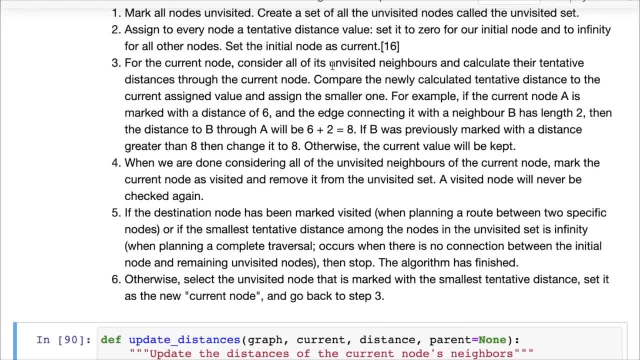 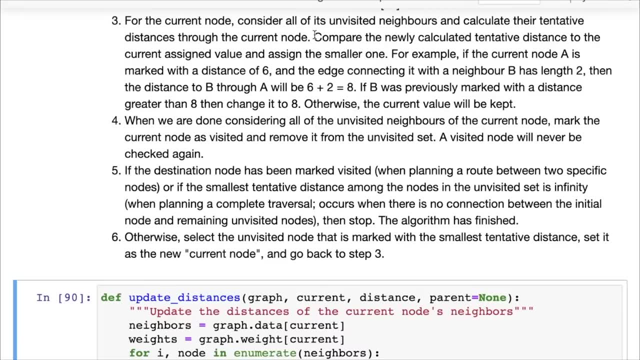 Now, if the unvisited nodes have distances set to infinity, then we know that the distance from the current node- distance why for going via the current node is going to small- is going to be smaller than the distance infinity that has been set. But on the other hand, if the if a distance has already been set for an unvisited node through some other node, then we can simply compare whether it is better to go through the current node or whether it is better to retain the retain the distance that was obtained by some other node and just maintain that. 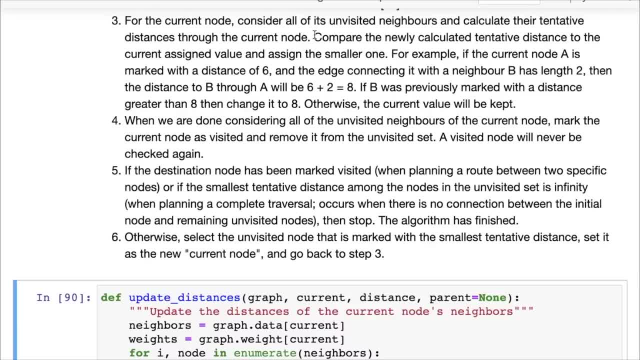 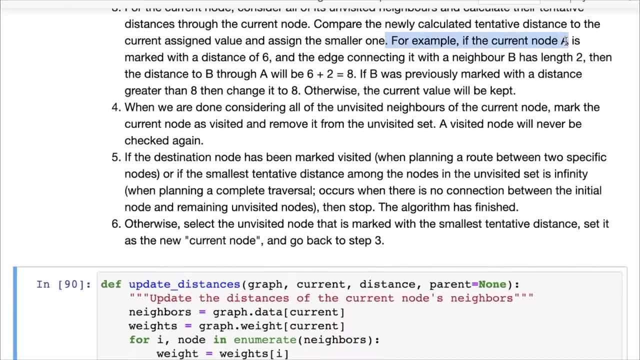 right. So in this way we simply update the distances of all the unvisited nodes that are neighbors of the current node. Okay, So, for example, if the current node is a and it is marked with a distance of six, and then there is an edge connecting it with a neighbor, B, and then that edge has the weight or the length two, then the distance to go to B through eight from the source will be six plus two, eight, right. 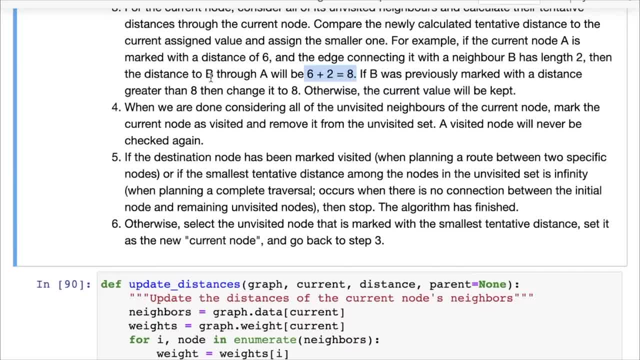 So from the source to a is six, eight to B is two. So the distance if you want to go to B through a will be six plus two eight. On the other hand, if B was already previously marked with a distance right, 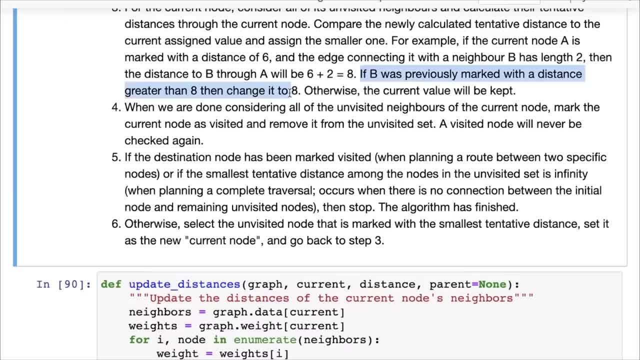 So it was not visited, but it was just marked with a distance greater than eight. Then we know that we have found a shorter path via a, so we update its distance to eight. On the other hand, if we have a value- let's say the value of for visiting B via another node, D, was seven. 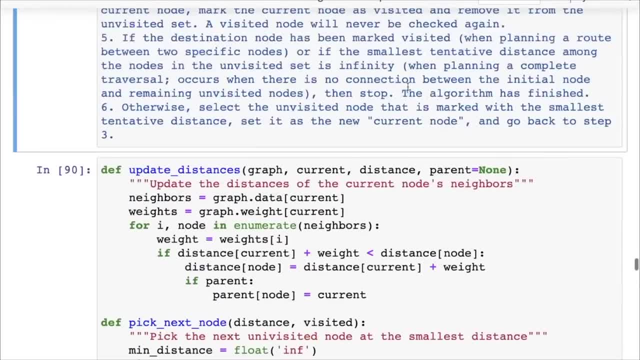 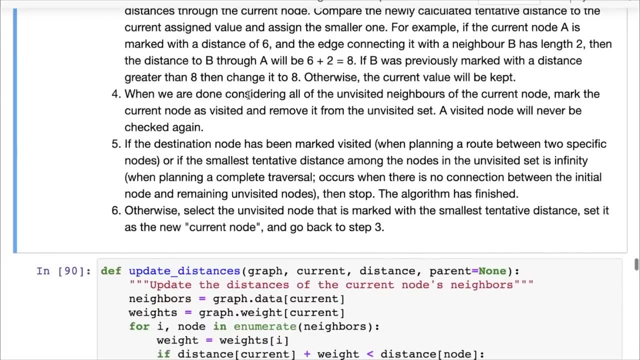 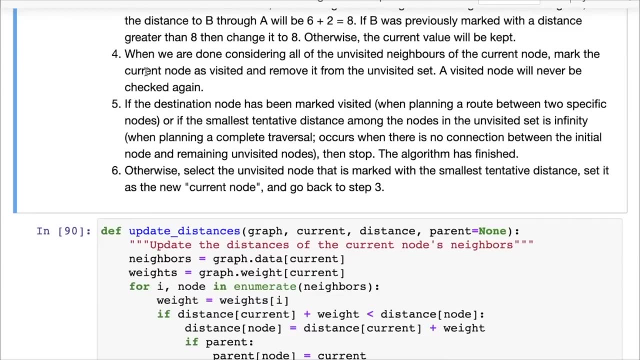 So we keep the distance as seven right. So we are simply updating the distance. We are not yet marking These new. we are not yet marking B as visited. Now, when we are done updating all the distances for the current node, then we mark the current node as visited. 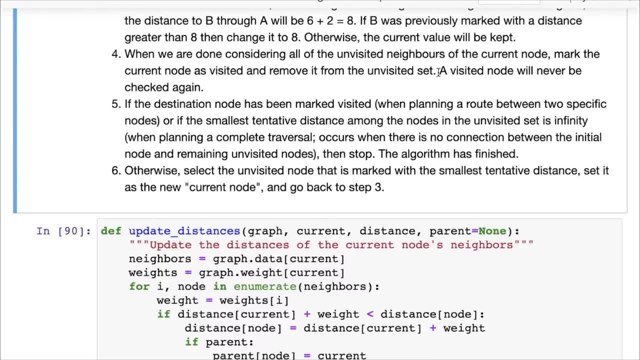 And of course we remove it from the unvisited set right. So we mark the current node as visited. Then a visited node will never be checked again, because once you have visited a node, you have found the shortest paths to it and you have used it to update the distances of all its neighbors. 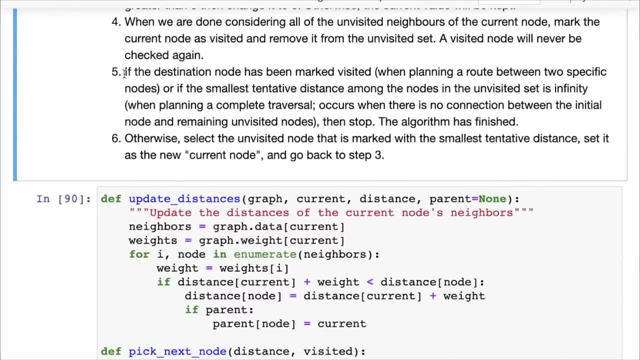 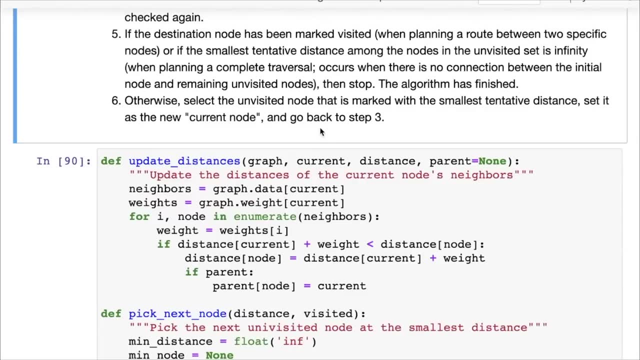 So you'd never need to visit it Again. so then, find the first unvisited node. find the first unvisited node that is marked with the smallest distance, right. So now we have a bunch of visited nodes and then we have a bunch of unvisited nodes. 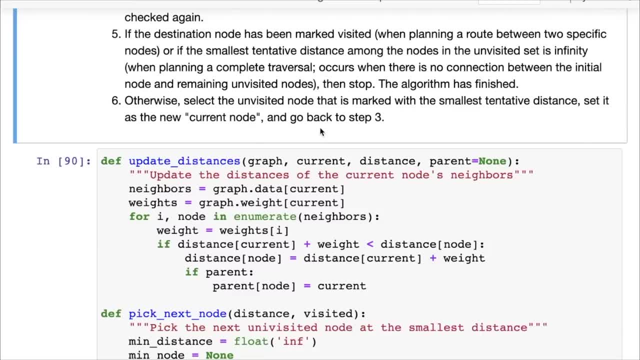 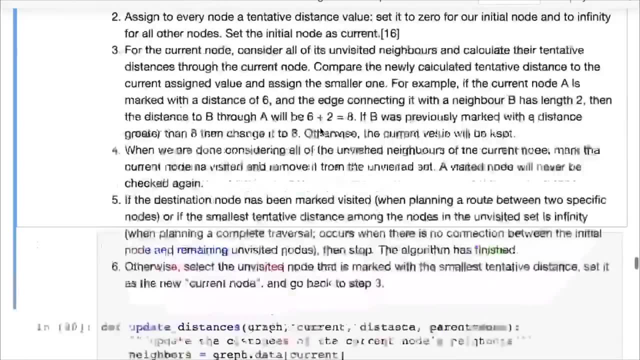 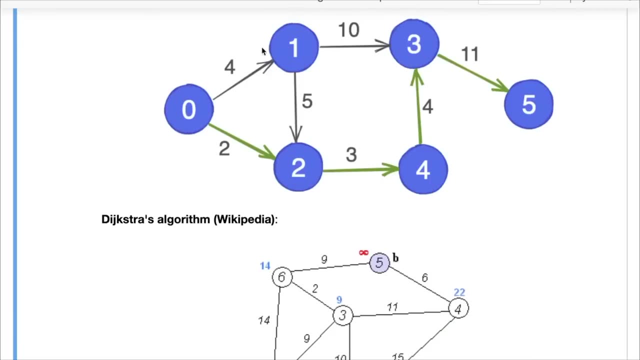 Many of those unvisited nodes have been marked with a distance. So you simply get the first unvisited node with the smallest distance and make it the current node and then repeat the process. Okay, So you start out with zero. you see that you can mark two, as you can mark the distances of four, one and two. 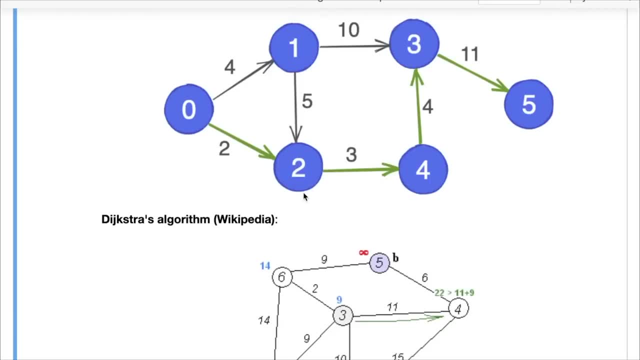 So one gets the distance four and two gets the distance two. Now then you mark zero as visited. Now you see that the node with the least, the unvisited node with the least distance is two. So you get two, and then you mark the mark, the edges from two. 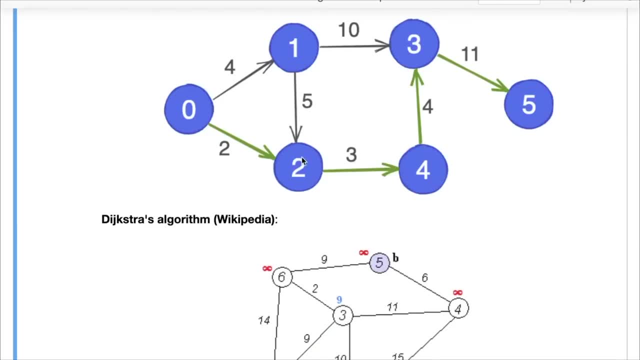 So you mark the distance for four as two plus three, five. And suppose two had an edge to one. Okay, Then you would mark the distance for one as two plus one. If one was a weight of the edge, let's say you would mark the distance for one as the minimum of four and two plus one. 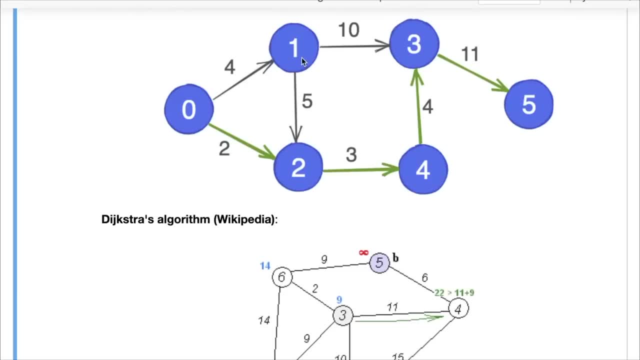 So which will be three. So you can mark the distance for a one as three and that's it. And then you remove two from the unvisited set. Next you find the next unvisited node, the, which has the lowest distance. So if this edge existed, that would be one. 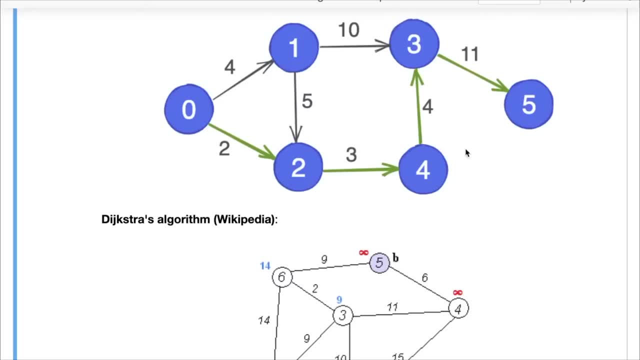 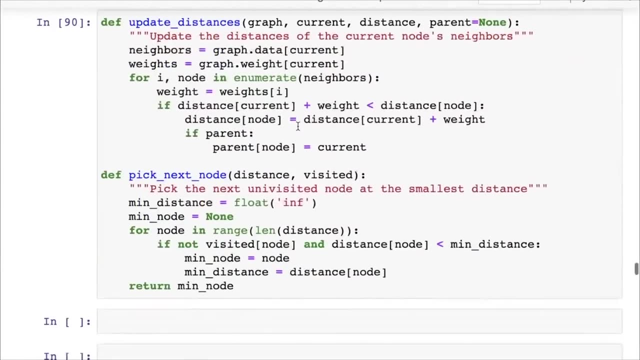 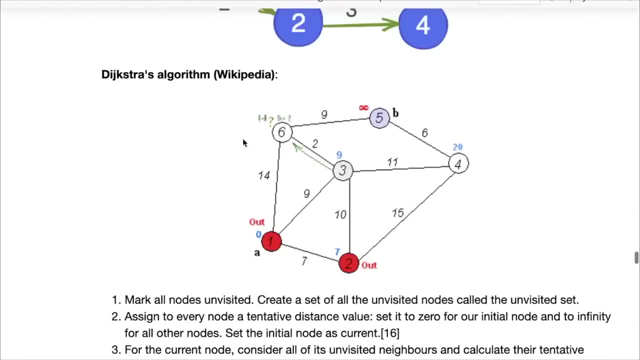 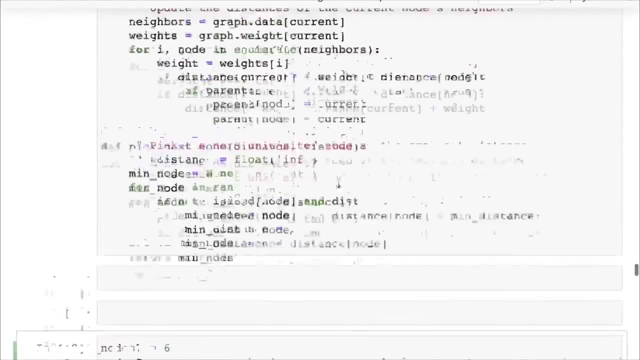 But if, Since it says, if this edge does not exist, that would be four, So you get four, and then you mark the distances for the neighbors of four, and so on. Okay, So what we'll do is we will create this, we'll create this graph here which contains: okay. 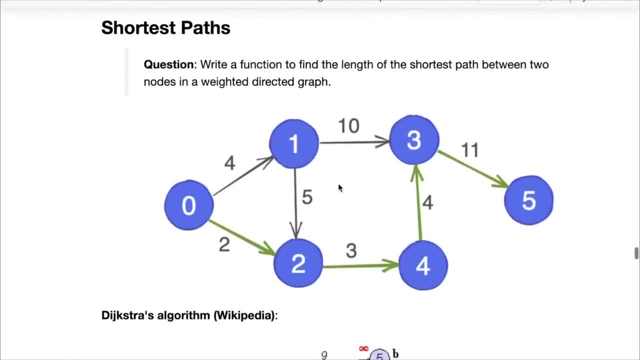 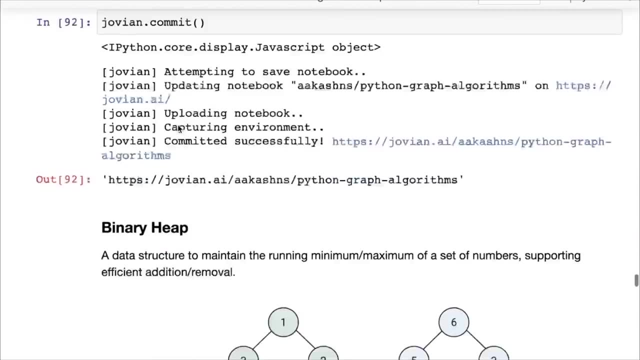 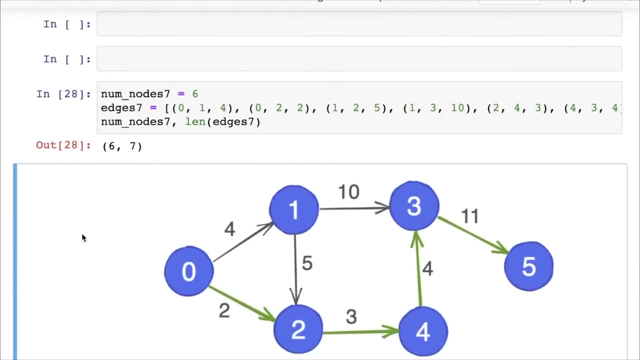 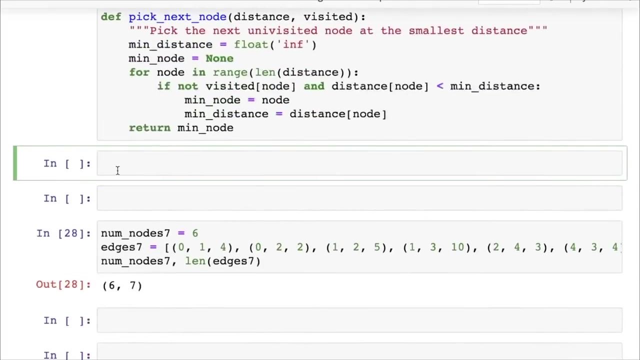 There should be a graph here that we can look at. Yeah, So we'll create this graph here, Which contains a zero to six, which contains six nodes, zero to five. This is the graph you're creating. Let's just put it here, this graph. 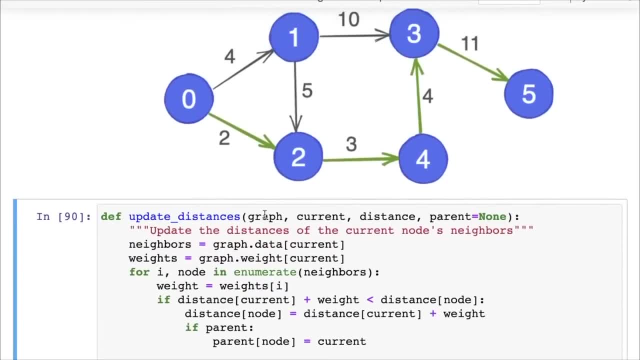 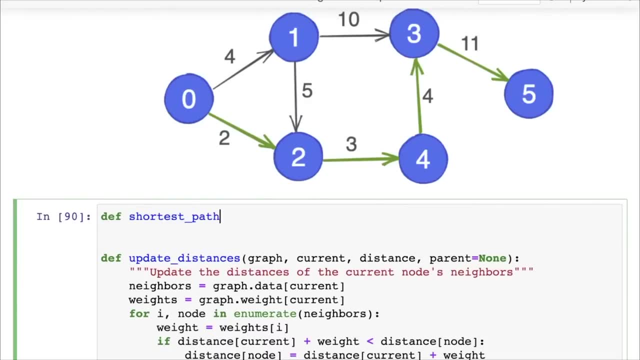 Yeah, So this is a graph that we'll work with and let's start writing our shortest path algorithm, So dev, shortest path algorithm, And then we have a graph and that's it. We have a, we have a start node, so let's call it source. 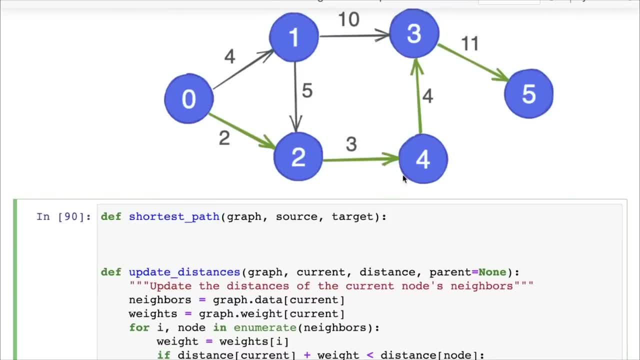 And then we have a target node, that node that you want to get to. So we want to go from zero to five And as soon as we have the, as soon as we mark the target node as visited we, our algorithm is done right. 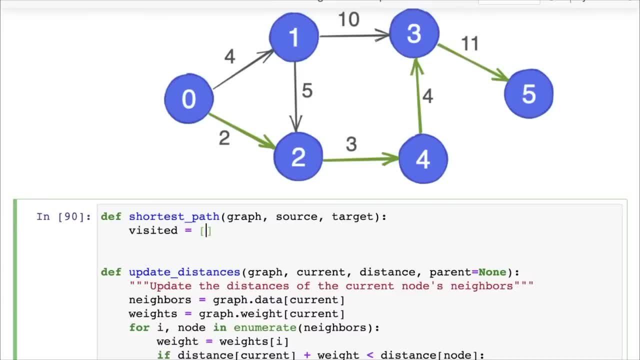 So first we mark everything as unvisited by setting: Okay, Visited falls, times, land graft or data. So here we have marked visited. then we have distance, So we take. we take the distance as infinity. But here's a way to create infinity in Python. 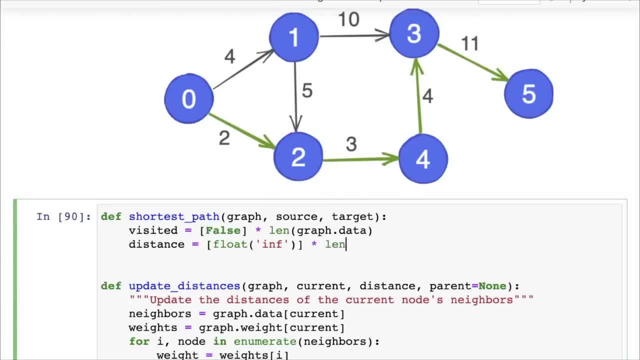 You just say: float inf and once again we set all distances to infinity. Then we are going to maintain a queue. So because we have this first in, first out kind of structure, So we're going to maintain a queue. The first thing we'll do is we will Mark the distance for the source node as zero. 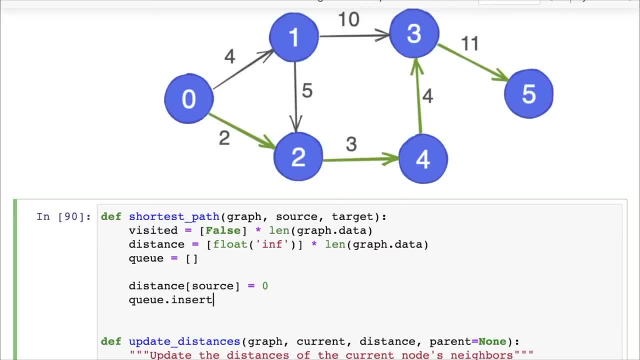 Then we can insert the source node into queue. So queue dot- insert or queue dot- append source, And then we'll set an index to keep track of what is the next element that we need to dequeue. So the first element is what we need to dequeue. 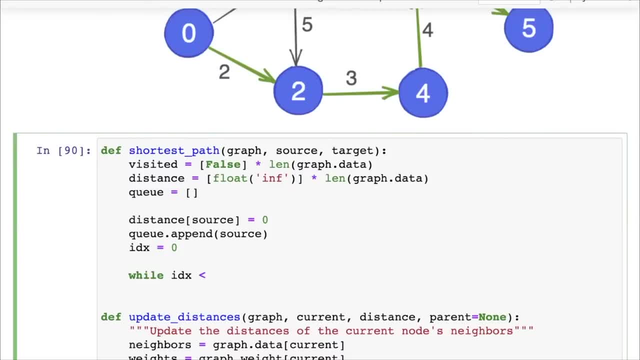 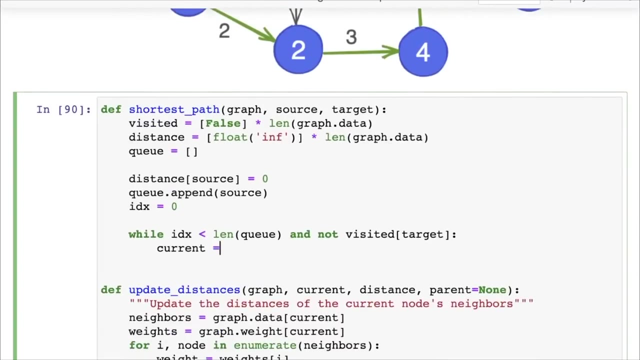 So while index is less than zero and not visited target, So while index is less than the length of the queue and the target is not visited. So what do we need to do? We need to get the current element from the queue. So we simply get queue of IDX and then we increment IDX by one. 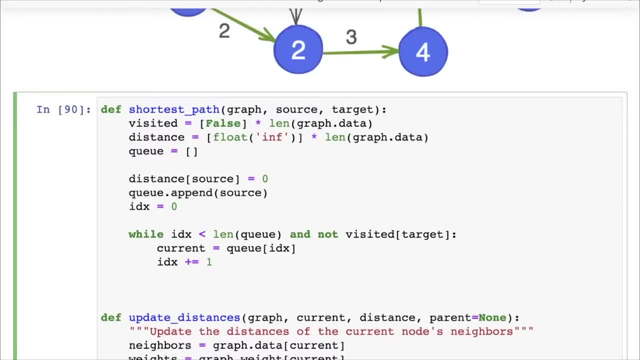 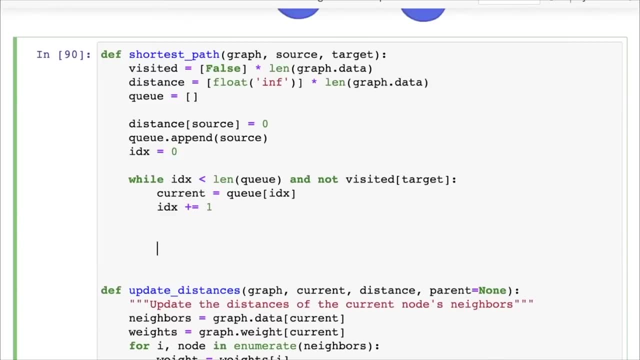 So we increment IDX by one here. Then we need to take all the neighbors of queue, all the neighbor. Oh, we also need to finally mark it as visited. So let's just put in visited. current equals true here. But in between what we need to do is we need to update the distances. 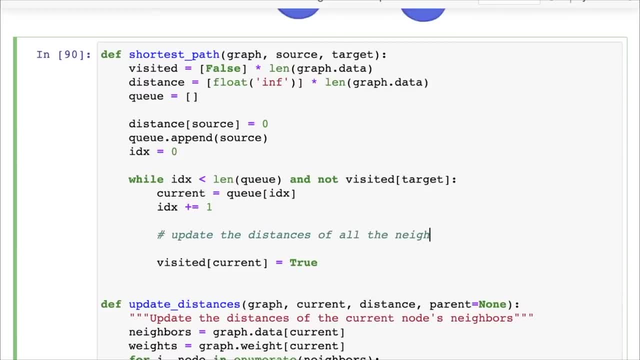 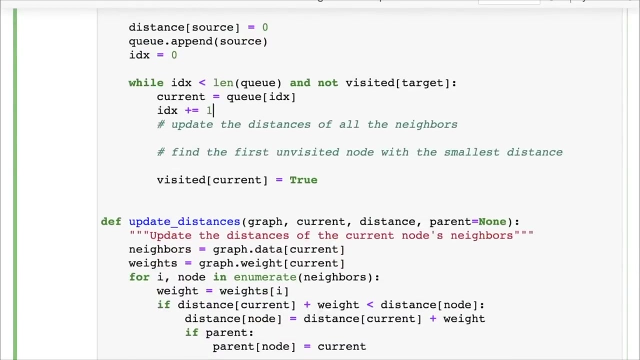 of all, All the neighbors. and then we also need to find the next node with the, find the first unvisited node with the smallest distance. Okay, So to update the distance of all the neighbors, we have written a function called update distance. 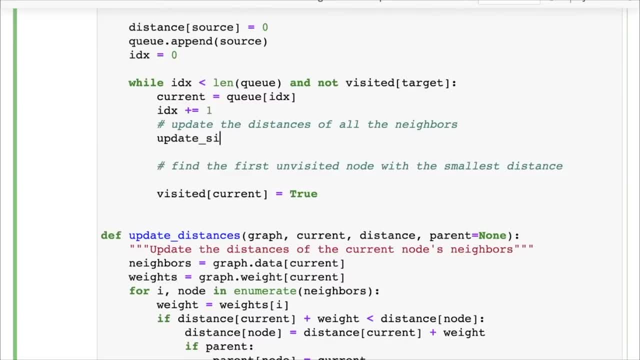 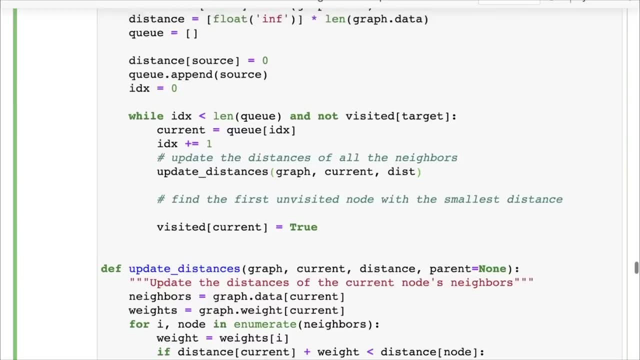 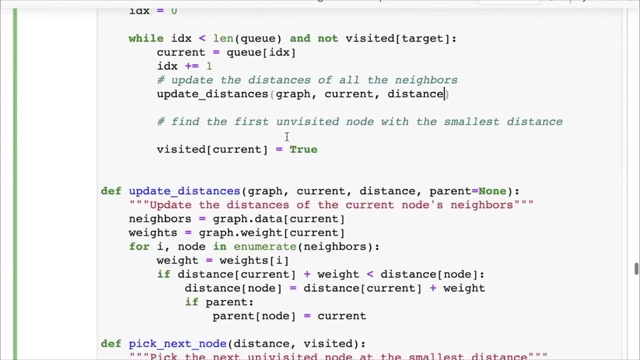 So we'll call this function update Distance or update distances, where we will pass in the graph and we will pass in the current node and we will pass in the distance matrix or the distance array And we pass it in this way and what update distances does? 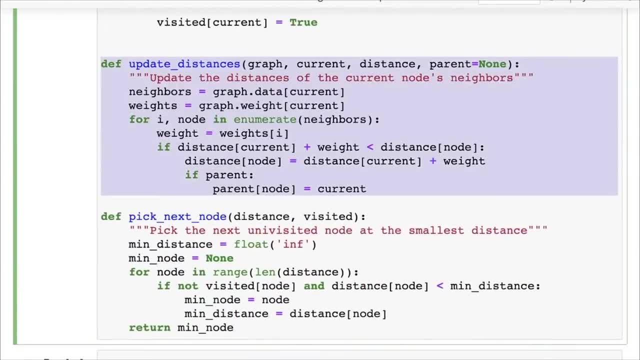 Let's look, let's look at it here And again. it's always a good idea to extract out specific pieces of logic into separate functions. So here we are calling update distances, where we have a current note, and then we have the graph, and then we have the. 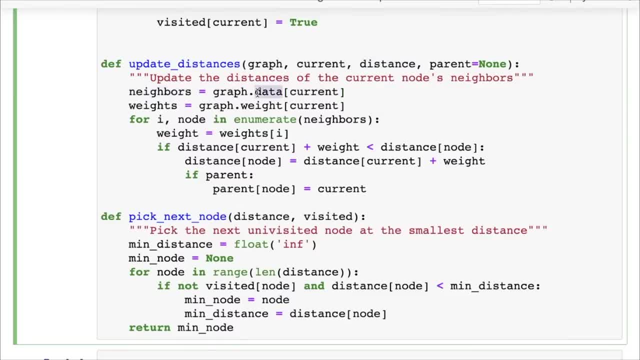 distance. So we get the neighbors of the current node using graph dot data. graph dot data Current will give us the neighbors of the current nodes. Then we get the weights of of the neighbors of the edges connecting the current node towards neighbors. 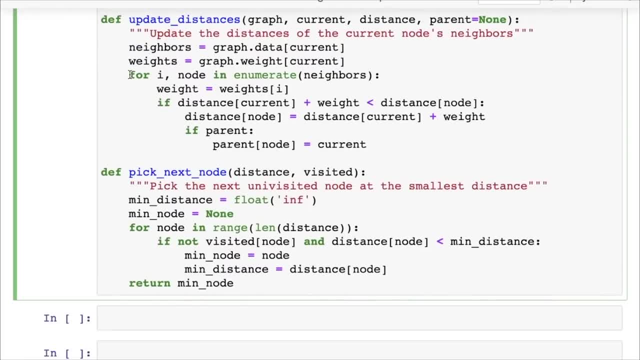 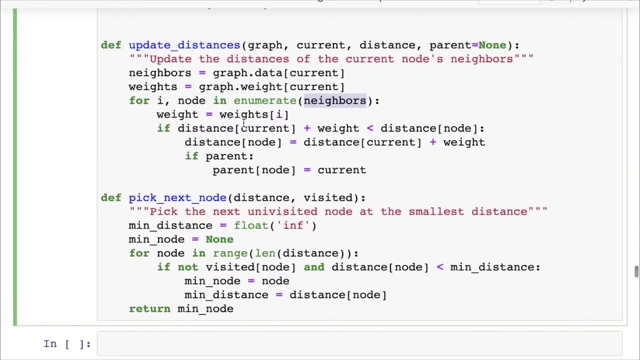 So we get the weights as well. Now we go through each list of neighbors, So for I common node in enumerate neighbors and then we check we get the weight. So we now we have the node and we have the weight. Okay, 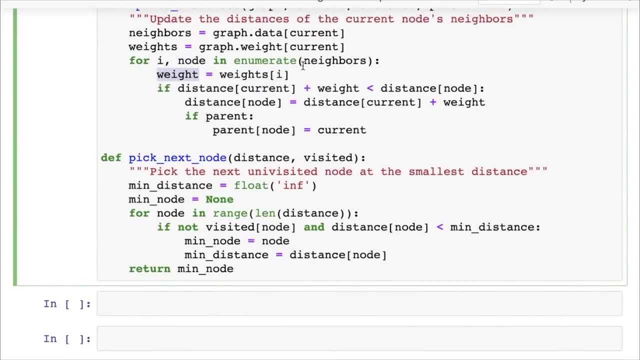 So we have for each edge the node that it is connected to and the weight of the edge, and then we check the distance for the node. If the distance for the node- let's say it hasn't already been said- then it is infinity. 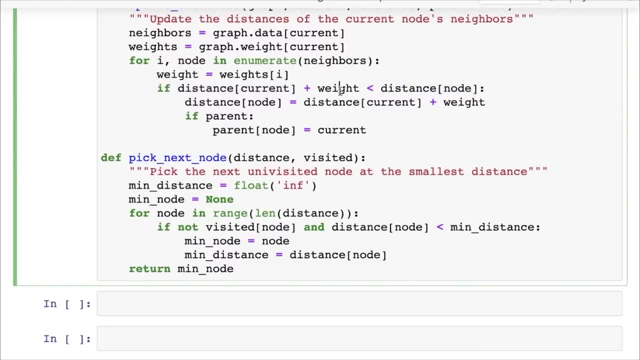 So in that case distance to the current node from the source plus the weight of the edge from the current node to the next node will be less than the distance. So if the distance of current plus Weight is less than the distance, We simply update the distance of the node. 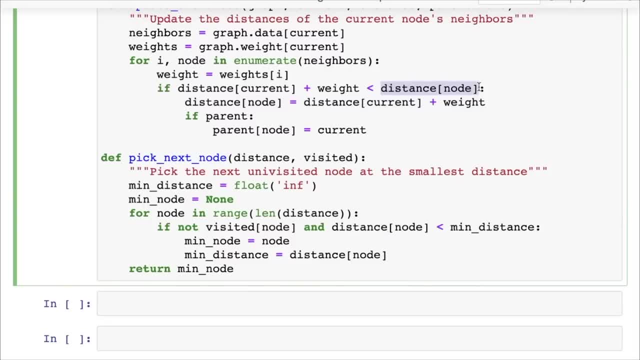 On the other hand, if the distance of the node has already been set via some other node and that is less than the distance via the current node, then we do not update the distance. Okay, So that's all we are doing here and we can ignore this for now. 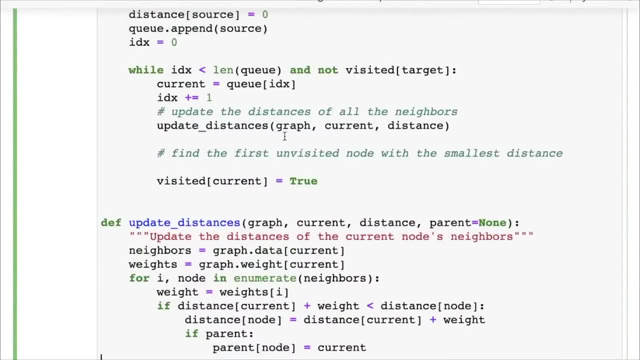 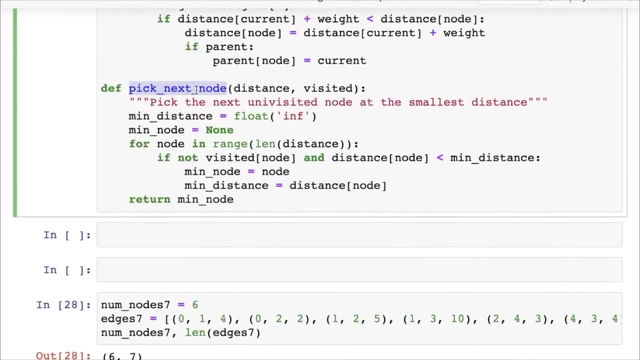 We'll come back to it, but this is performing exactly that update distances function that we talked about. the next: We want to find the next unvisited node, So here we have a function called pick next node, which has a list of distances and it has. 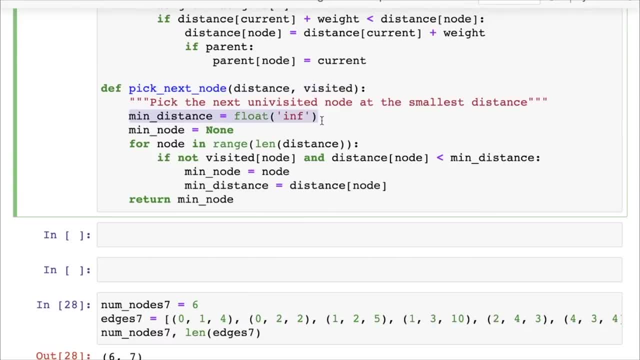 visited. So we want to track the minimum distance. So we first set a variable called minimum distance to the value infinity and then we set a variable min node. So this is the node with the minimum distance to the value None. Then we iterate over the, all the lists, all the nodes in the that we have in the graph. 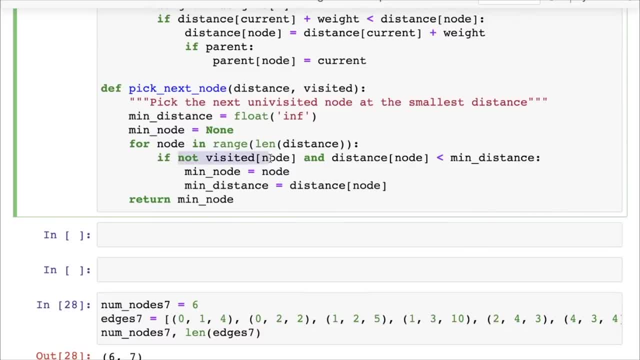 So from zero to N minus one, and we check that if the node is not visited and the distance of the node is less than the minimum distance we've obtained so far, Then we said that note to the minimum node and we set the minimum distance to that value. 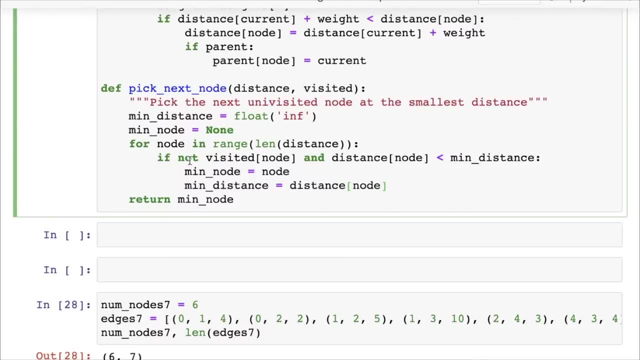 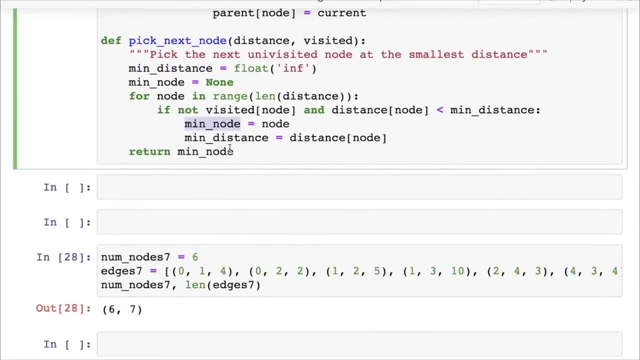 Okay, So we track the minimum distance, the running minimum distance, by going over all the nodes in the graph and we keep track of which node has the minimum, which unvisited node has the minimum distance. So, finally, what big next node gives us is the first next unvisited node. 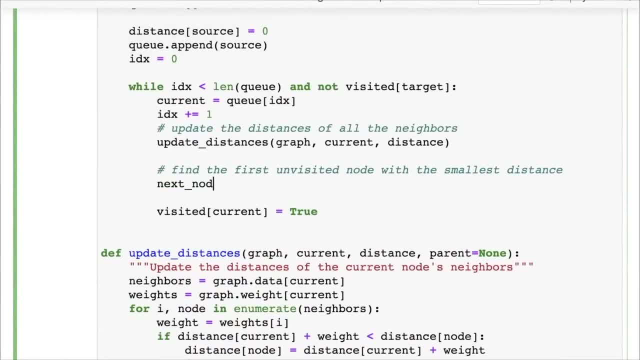 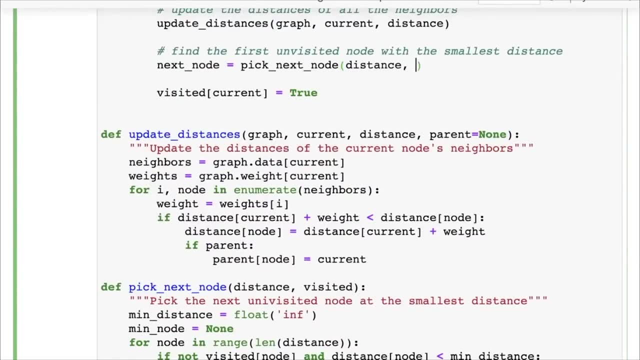 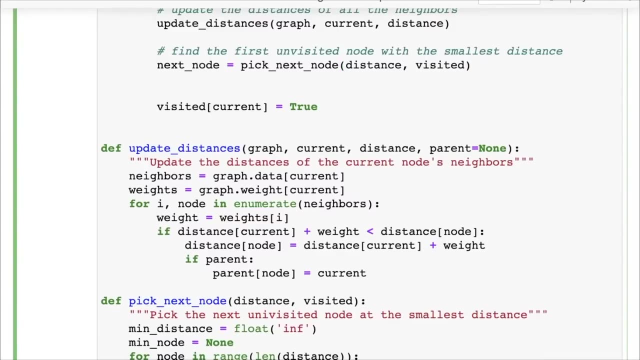 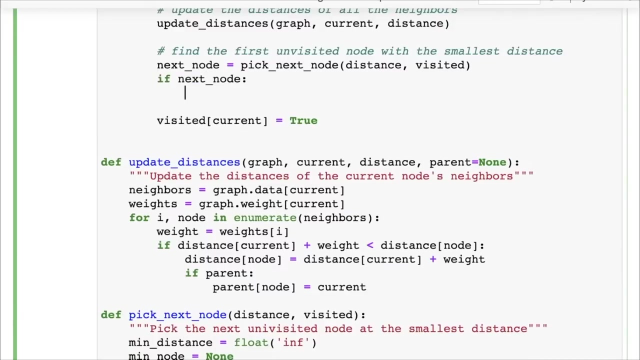 Okay, So here we can get. next node is Big next node and we give it the distance and we give it visited. Okay, So now if there was an X node, it's possible that there is no next node because we've probably already visited. 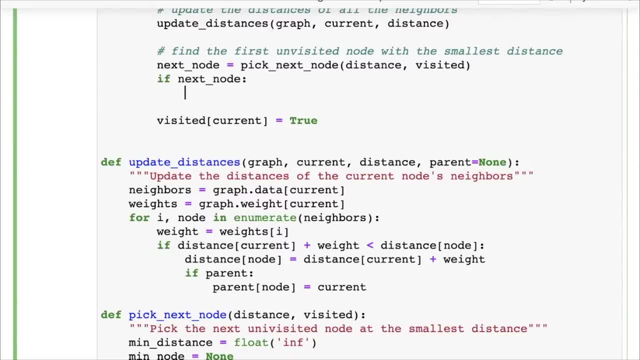 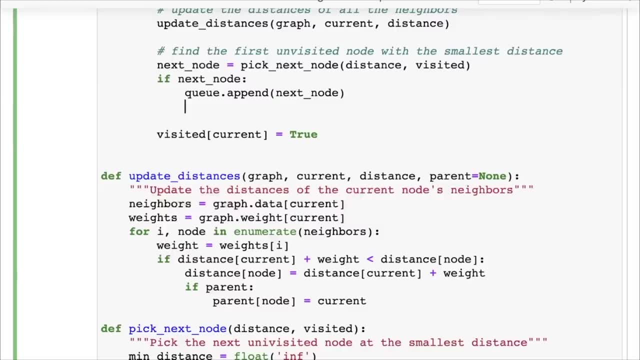 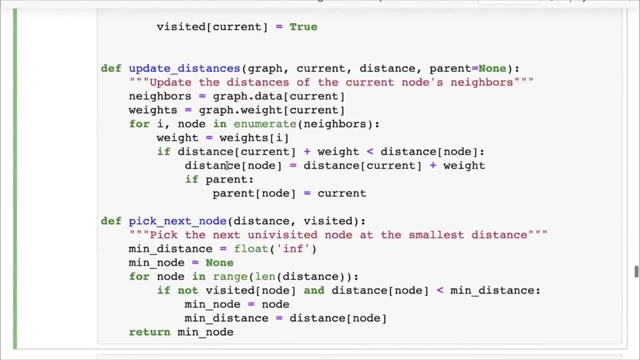 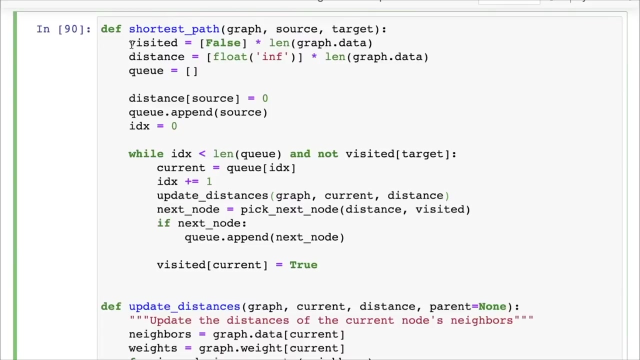 everything that we can visit. So if there is an X node, then we NQ it. So we say Q dot, append next node And that's it. that's pretty much it. So that is our shortest path algorithm. We create a visited list. 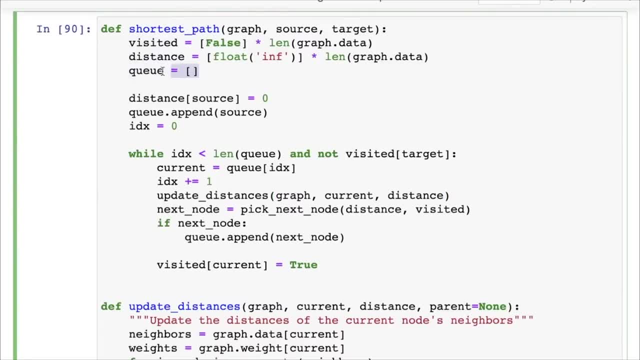 We create a distance list, We create a queue where we will add things. So these, this will be all the, all the nodes that we have visited. We'll go through it, go through this one by one And the Q in order. 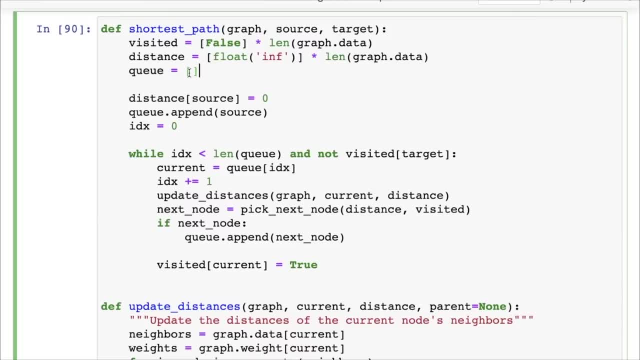 We'll give us A list of all the nodes And then their order of distance from the source node. Now, what we need to return here is we simply need to return distance of the target, And since that was what was asked here, 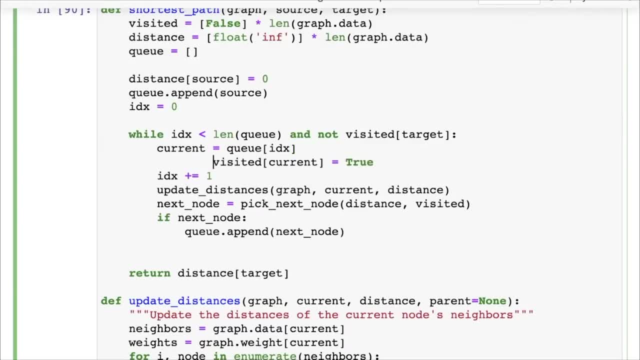 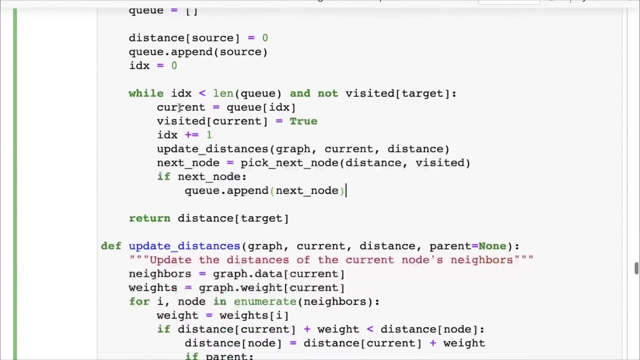 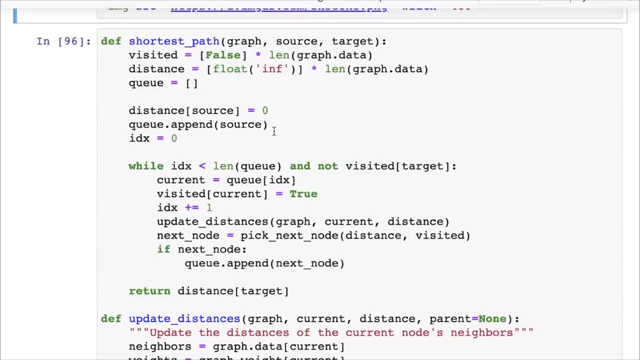 let's also mark current as visited through here soon enough, so that we don't end up visiting current again and again. All right, So let's run the shortest path algorithm. Then here we have a graph. This is the same graph that we see here. 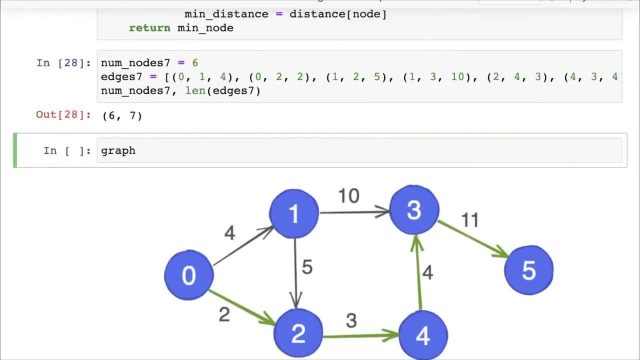 Now we can create a graph, graph seven, and this is weighted and directed. So we will pass in graph, We will pass num nodes seven, We will pass edges seven And then we will pass weighted equals true and directed equals true, And this is graph seven. 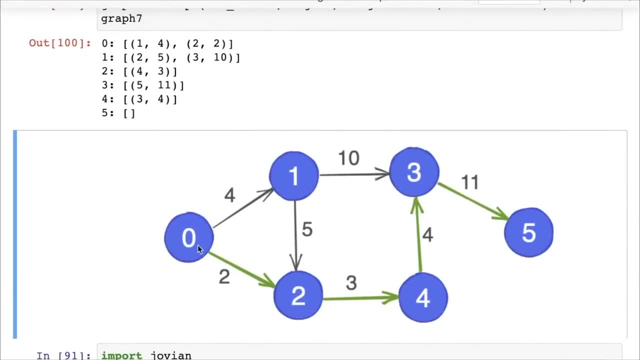 Okay, This seems like it was it worked out right. Zero is connected to one and two, with the weights four and two respectively, And five is connected to nothing. Four is connected, Three is connected to five. four is connected to three. 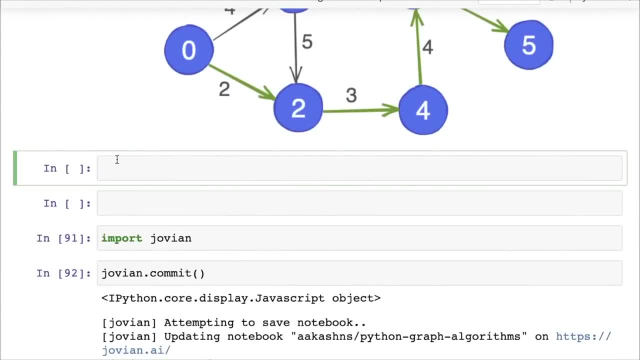 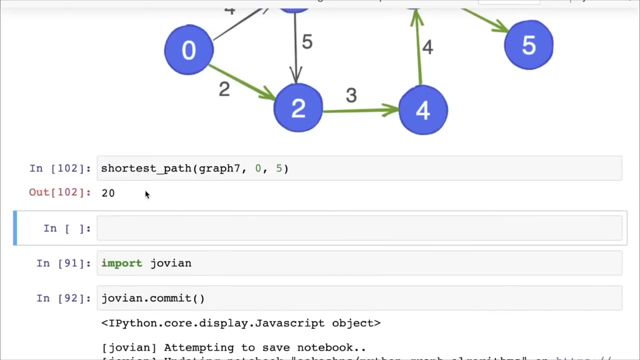 Okay, This looks fine. So now we can see Shortest path in the graph from, let's say from zero to five in graph seven, and it says that the length of the shortest path is 20.. So you have two, three, four, 11.. 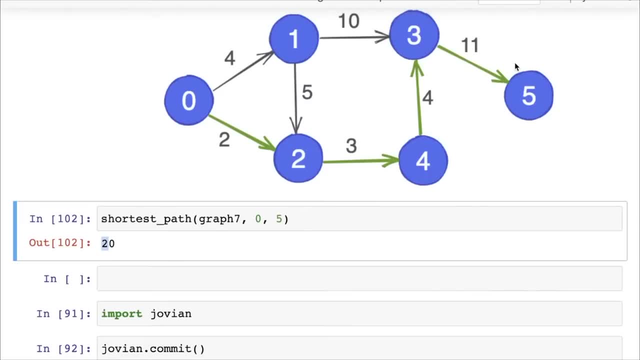 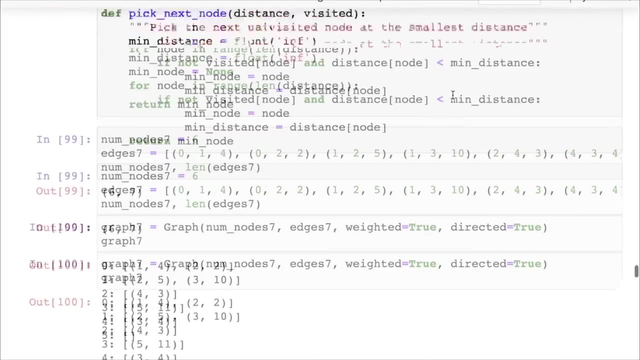 So two plus three, five, five plus four, nine, nine plus 11,, 20.. So that seems to be right. What would also be nice to get is just to see what that path is, And for this we can introduce something called a parent. 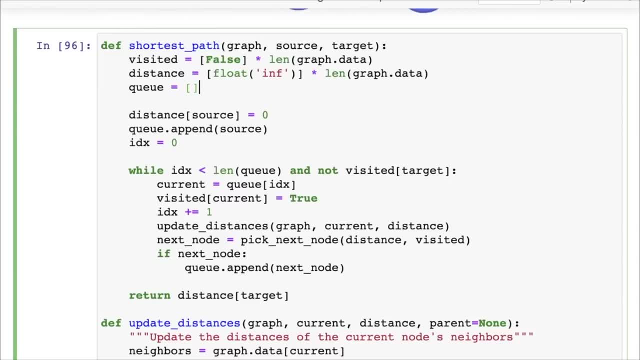 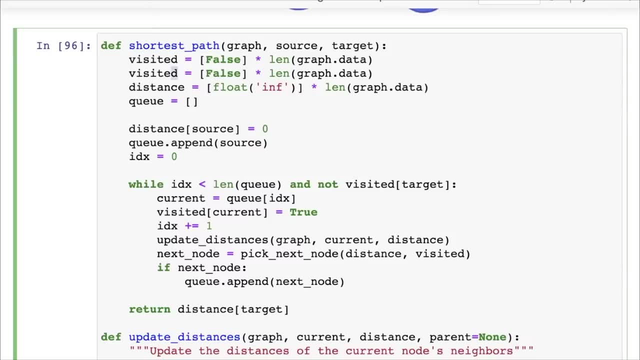 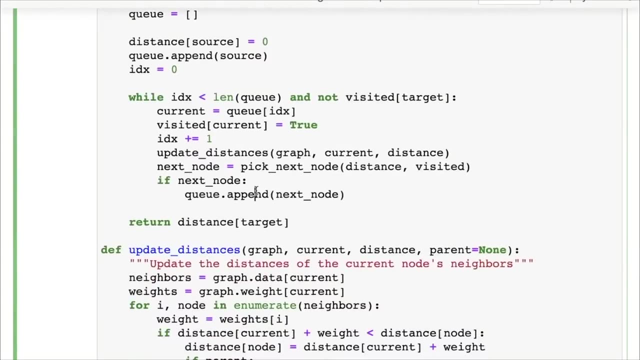 So here we can simply have another thing called a parent, which is set to none for each element So visited, let's call this parent and let's set it to none by default, And all we need to do is whenever we are enqueuing a node, we need. 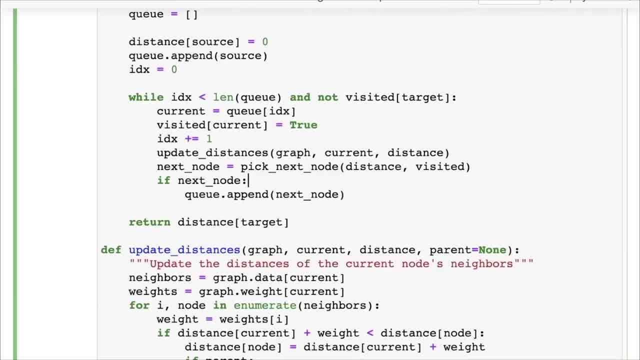 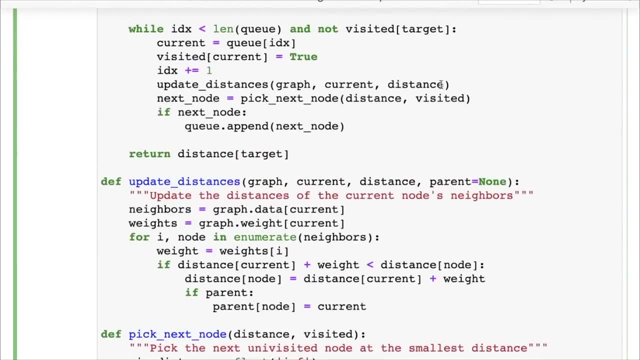 to track why it got enqueued, right? So if an, if a node is getting enqueued, then it is probably getting enqueued. So so sorry, not whenever. Whenever we are enqueuing, whenever we are updating the distance of a node, we 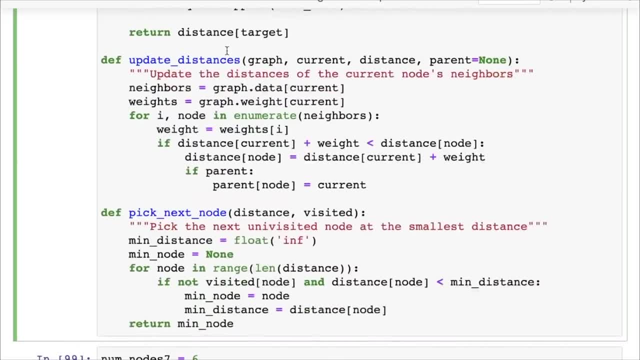 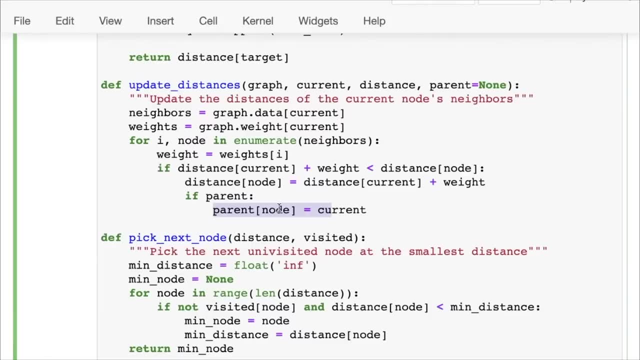 need to track why. why it's distance got updated, So inside update distances. whenever we update the distance of a node, we also set the node- the parent of the node- to that current node from which the distance got updated right, And that's all we need to do. 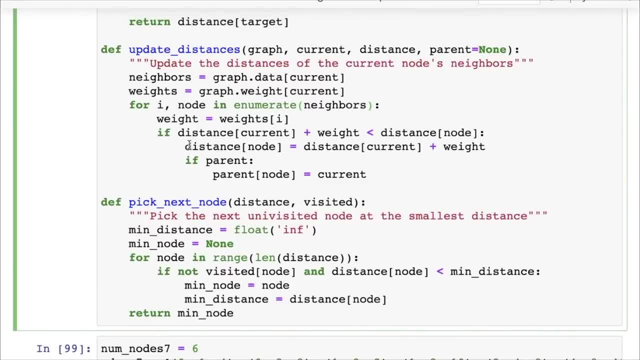 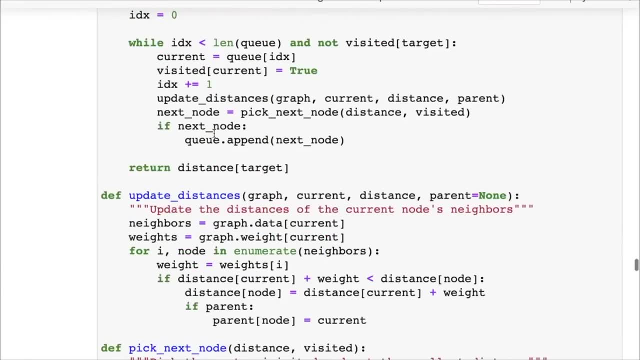 When we update the distance of a node we need to track. why did we update this distance? by which node we did We come to update this distance? So this way we have not tracked the parent. and let's return not just the distance of the target, but let's also return the queue. and let's return. 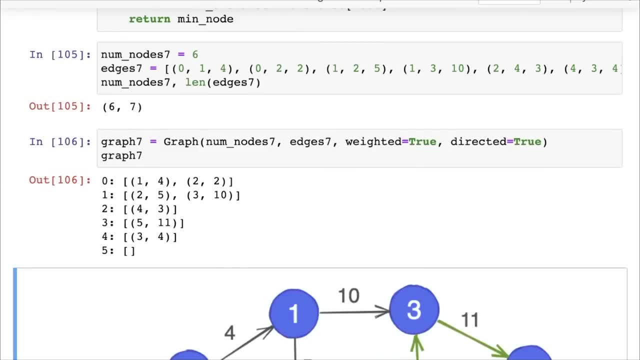 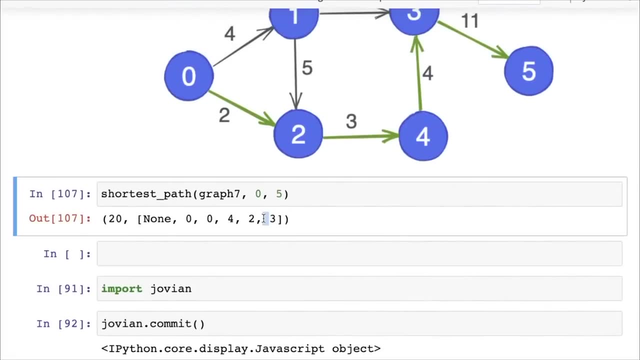 Let's just return the parent for now. I think this should be fine. Okay, So now you have the parent for each one. So if you look at the fifth element- 0,, 1,, 2,, 3,, 4,, 5, you can see. 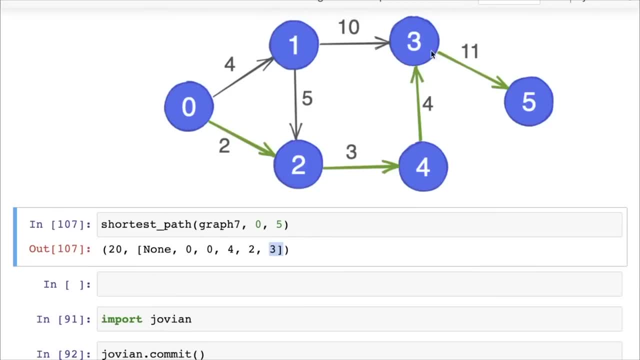 that the parent of five is three. So it seemed like we arrived at five from three. And then if you look at the parent of three, so 0,, 1,, 2,, 3.. The parent of three was four. It seemed like we arrived at three from four. 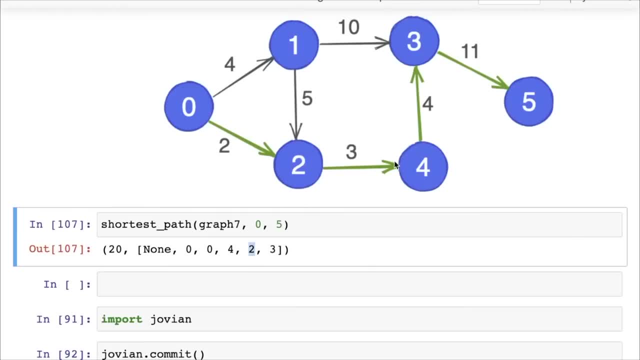 Then you look at the parent of two, It seems like we arrived at four from two. Then you look at the parent of two and it looks like we arrived there from zero And zero was our source. So the path is, if simply going reverse: 0,, 2,, 4,, 3,, 5.. 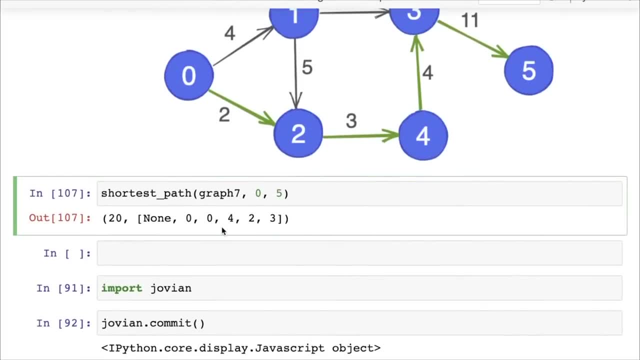 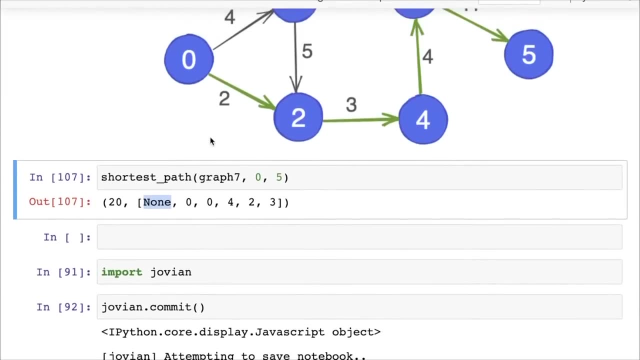 Okay, And that's how you get the shortest path and not just the shortest path distance. I noticed that zero itself does not have a parent, because that was the source. Now you can repeat this with another graph. Let's say, we take this other graph that we had. 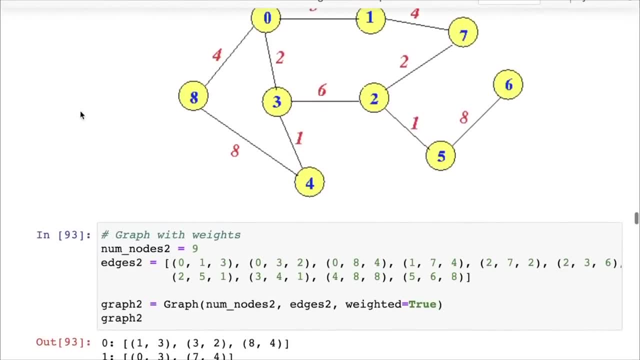 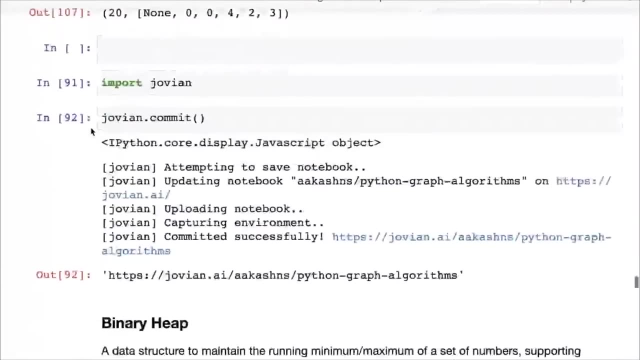 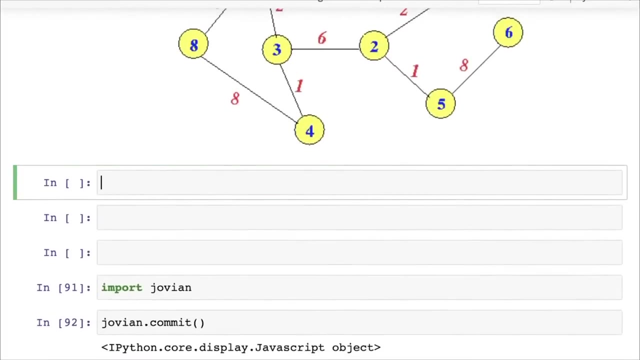 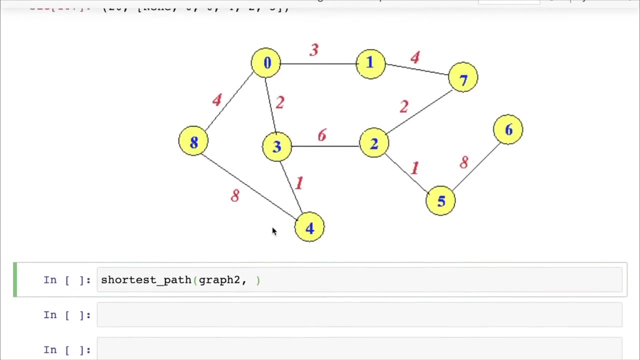 This was graph two. So let's grab this image here. So let's get graph two and let's say shortest path, graph two. And let's get the shortest path, maybe from zero to seven. So it seems like there are two parts. 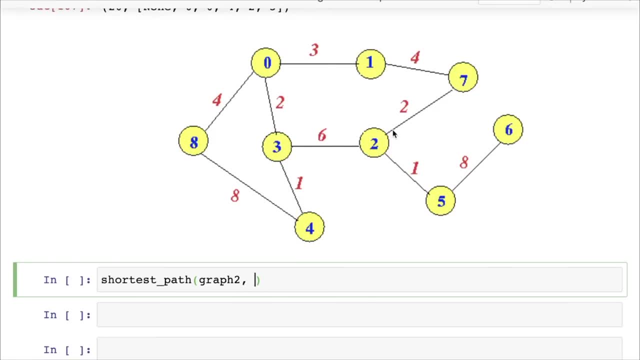 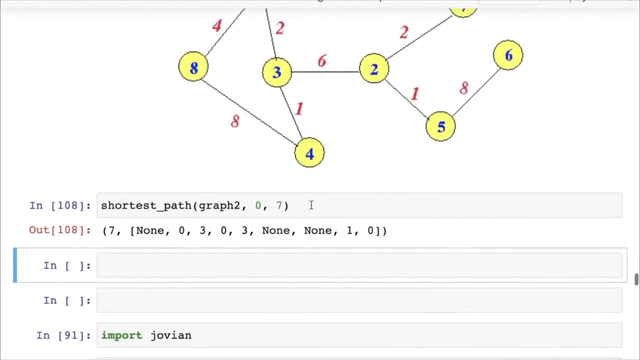 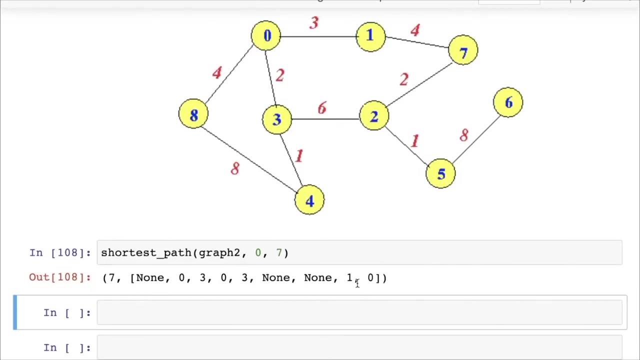 One goes via one and one goes by a six, or two, three, three, two and seven. So let's get the shortest route from zero to seven. Okay, So we started out with zero and we ended up at seven. So zero, one, two, three, four, five, six, seven. 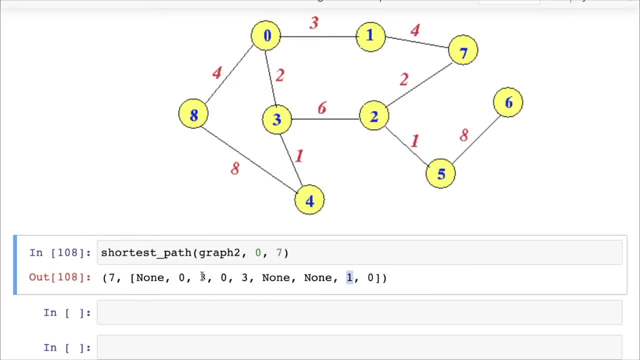 It seems like the parent for seven was one And then the parent for one was zero, So it's clear that it picked the path zero, one, seven and the total length of the path was seven. Sounds good, We can try another one. 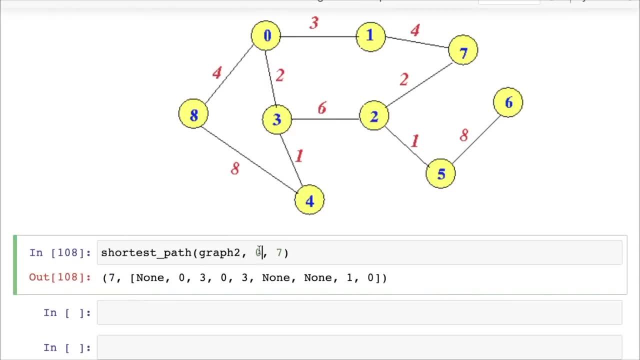 We can try two and eight. So there are a couple of ways to go from two to eight. One is to go via three, So you can go to six, two, three ways actually, but six, two, six. you can go at three, zero and eight, or you can go at three, four and eight. 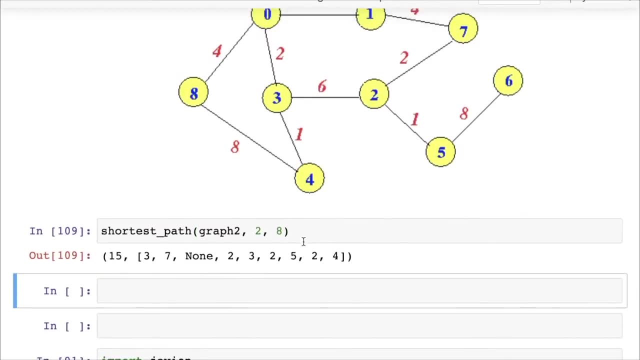 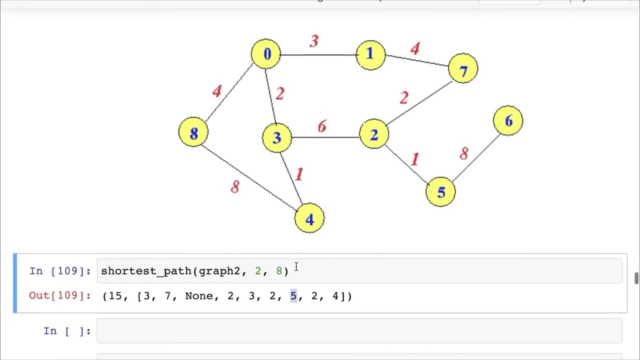 Let's see which Count Out. Okay, So now, zero one, two, three, four, five, six, seven, eight. So the parent for eight is five. Oh sorry, Zero one, two, three, four, five, six, seven, eight. 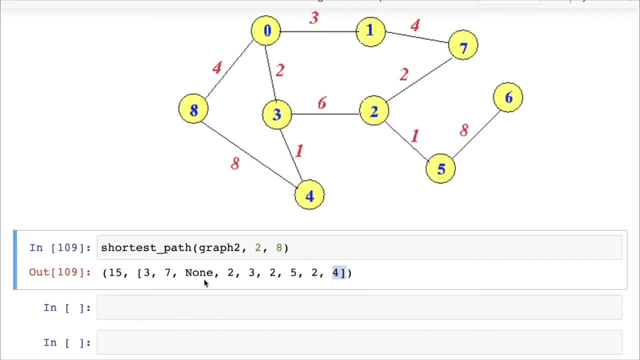 The parent for it is four, So we came to eight via four, and then the parent for four. zero. one, two, three, four, the better for forestry, So we came to four via three, and then the better for 30,. one, two, three. dependent for three is two. 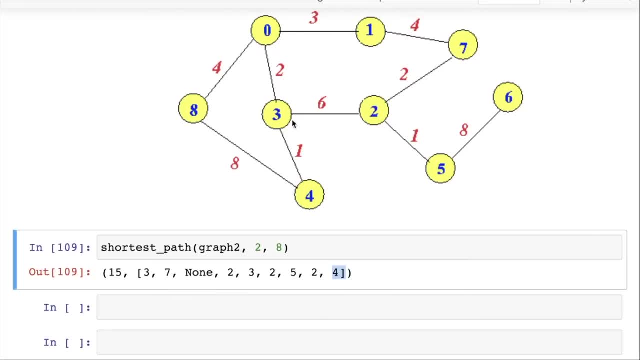 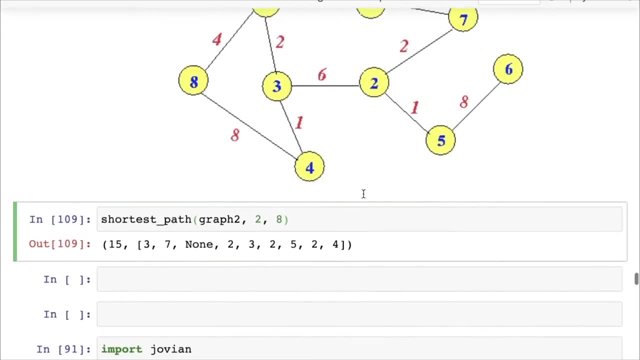 So we came to three. why six? Uh, via two. So two, three, four is the path, and the length should be eight plus one, nine plus six, 15.. Great, It seems like we figured out the shortest path once again, and this: 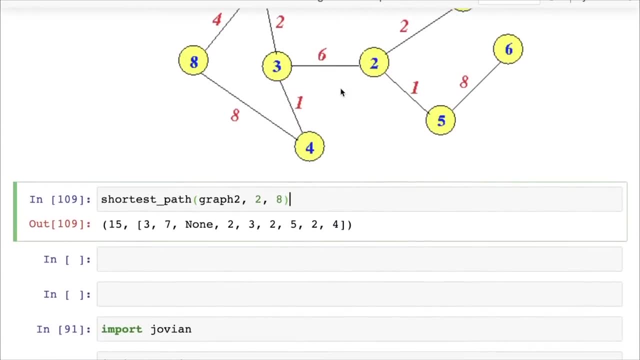 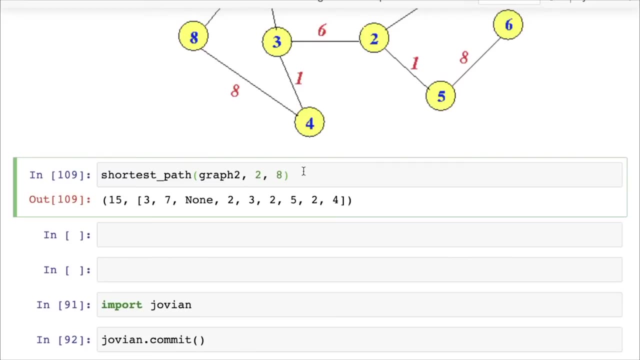 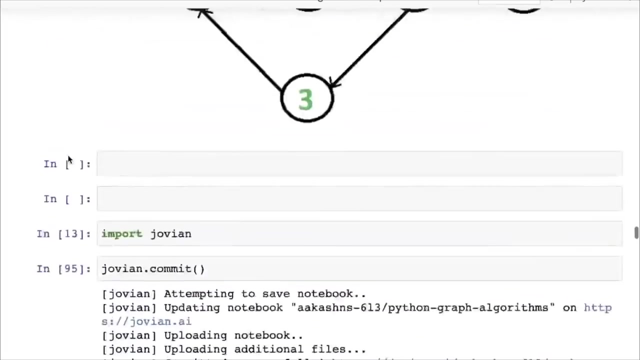 time, this was an undirected graph. Okay, So as long as you have weights, you can apply this algorithm, and this algorithm is called the Dijkstra's algorithm, And that's it. So that's all we're going to cover today. Now, one thing that we have not looked at very closely is the running time complexities. 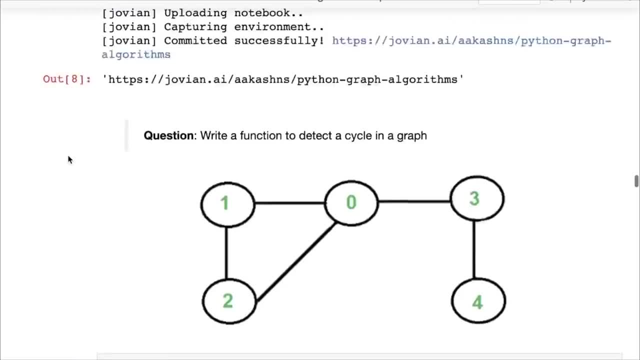 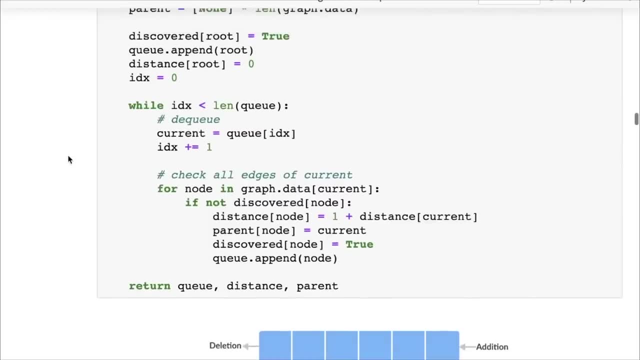 So let's do a quick look at that. Let's do a quick look at, let's say, BFS and see if we can identify and get or guess the running time. complexity And the full proof is left to you as an exercise. but roughly it looks like this: 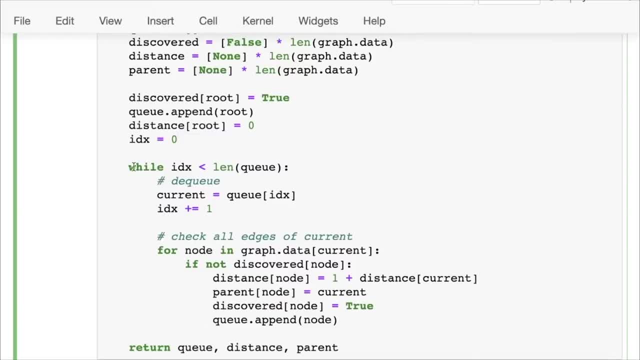 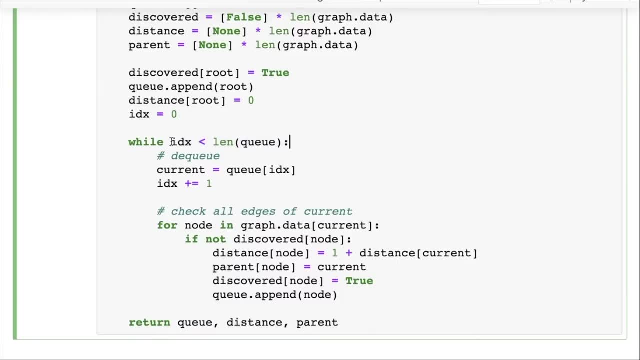 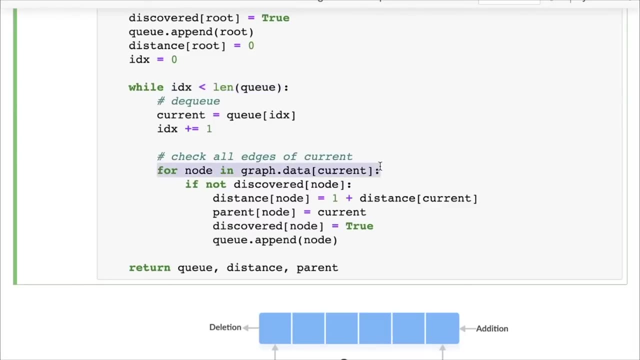 This is the main, this is the main loop here, So where we are going through the queue. So the number of times this may happen is N, or which is the number of N, which is the number of nodes and the number of times this might happen now, inside each for each. 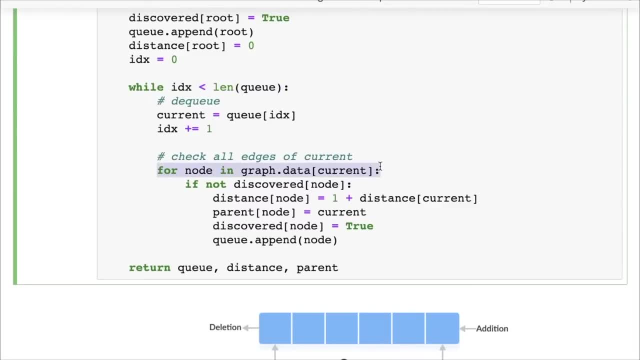 node inside BFS. remember that we check a full list of nodes inside each node for BFS, So the number of times this may happen is equal to the number of. for each node, we may perform an additional number of steps equal to the number of nodes it is connected to. 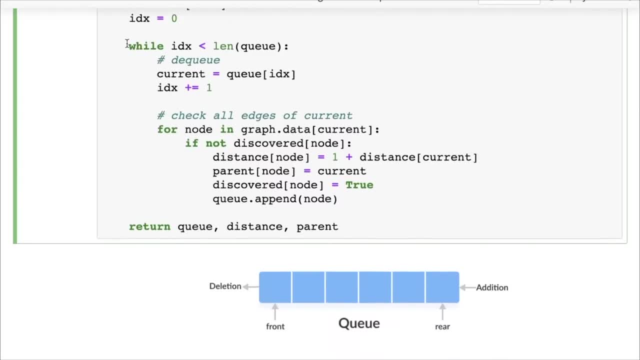 Right. So if we have N nodes, so we have NY loops, and then if we have a total of M edges, and let's say those M edges are split across, if I count the number of edges for each node, the number of edges is E1, E2, E3, E4, and so on. 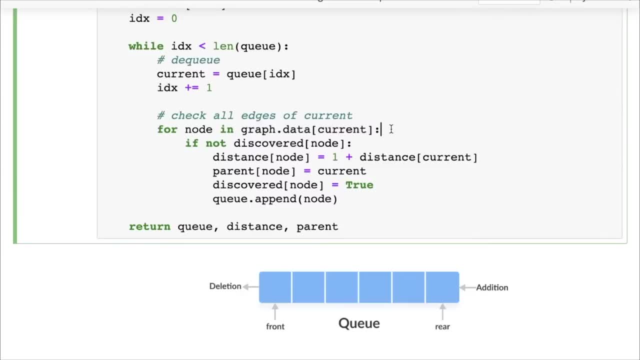 And then we So the number, the number, the size of this loop for the node N1 is E1.. The size of this loop for the node N2 is E2.. The size of this loop for node N3 is E3.. 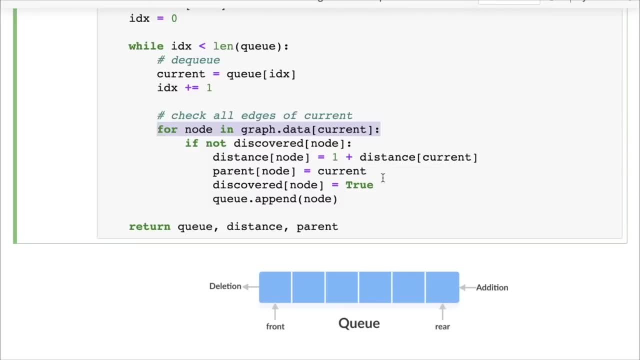 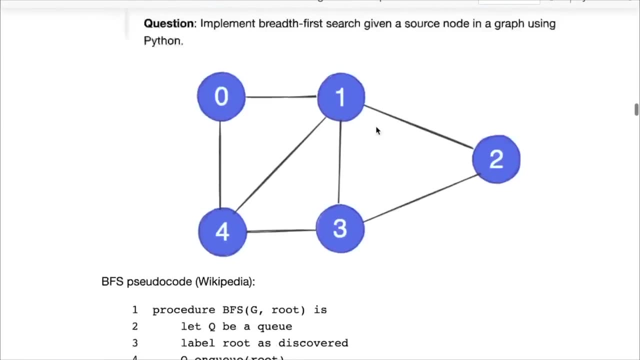 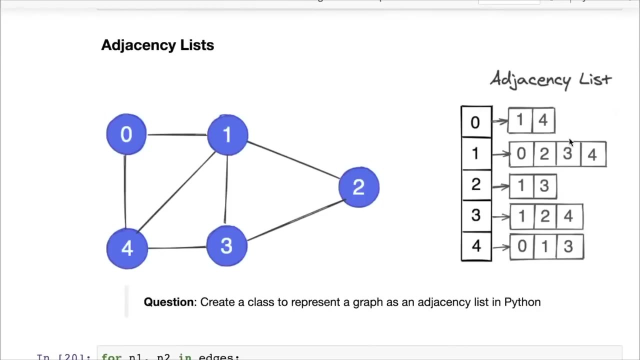 So if you add up the list of all the edges- E1 plus E2 plus E3 plus E4. So the total number of iterations inside this for loop turns out to be: you can see here: the total number of iterations inside the for loop will turn out to be the total, the sum of all. 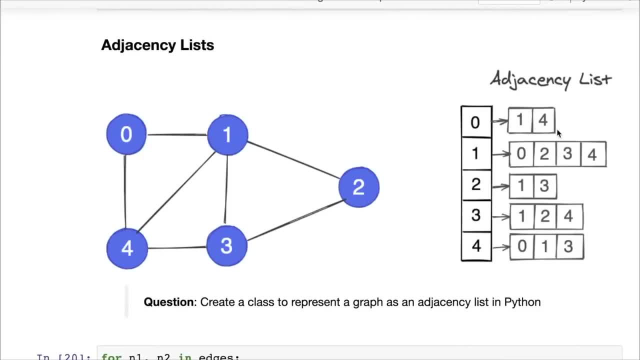 The adjacency lists. Okay, And this total sum of all the adjacency list is equal to twice the number of edges. You can see here the number of edges is 1,, 2,, 3,, 4,, 5,, 6,, 7, and you can verify that. the 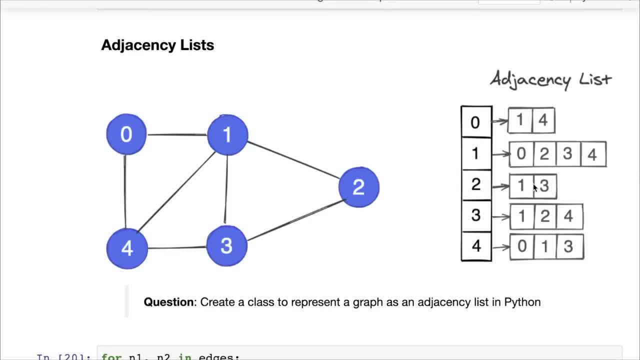 number of elements of all the adjacency lists put together is 14, because each edge is represented twice, right? So we end up if we have N. so if you have N, F, N vertices and M edges, we end up with N plus two M operations, right? 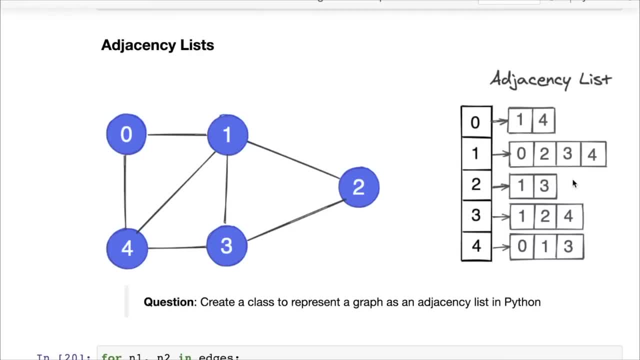 So each of the N operations to start the while loop, and then each of the two M operations. those are to iterate over each adjacency list right And now. when we are talking about complexities, we can ignore the M. If M is a number of edges, we can ignore the factor two associated with it. 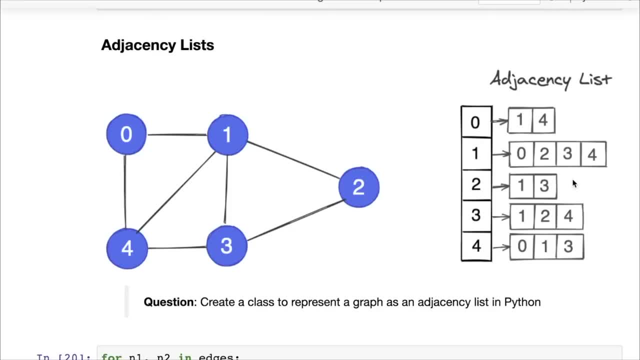 So what we end up with is order of N plus M. So order of N plus M is the complexity of breadth. first search, And now, by this point, you should be able to just work it out by looking at the code. So do try it out. 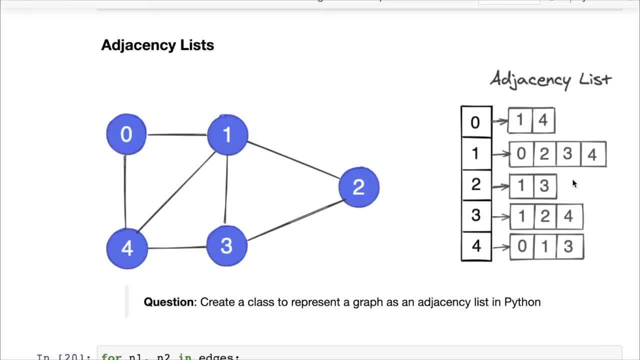 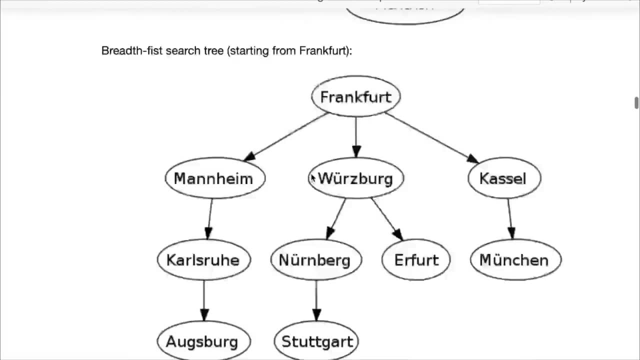 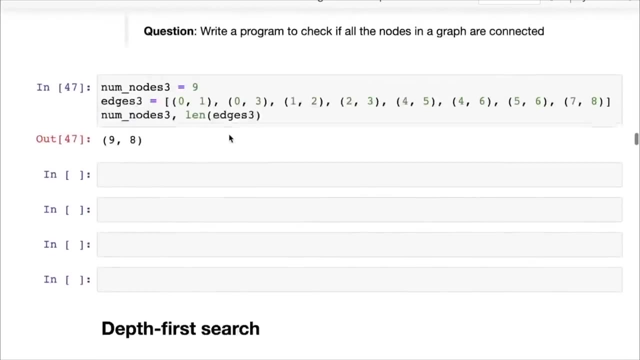 And if you, if it's not clear, do ask on the forum. but order of N plus M is the complexity of breadth first search And you will find a similar complexity for depth first search as well. Order of N plus M for the shortest path algorithm. 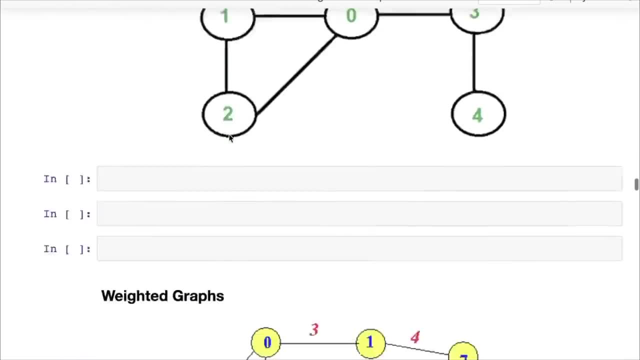 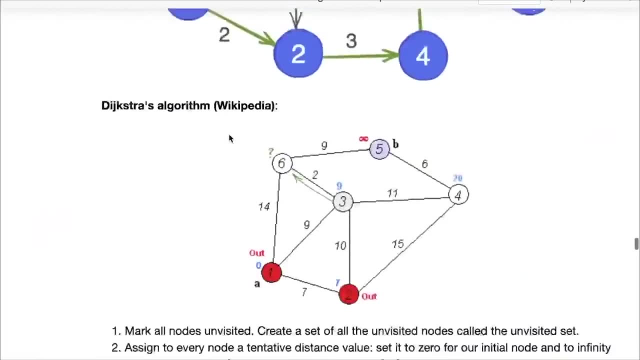 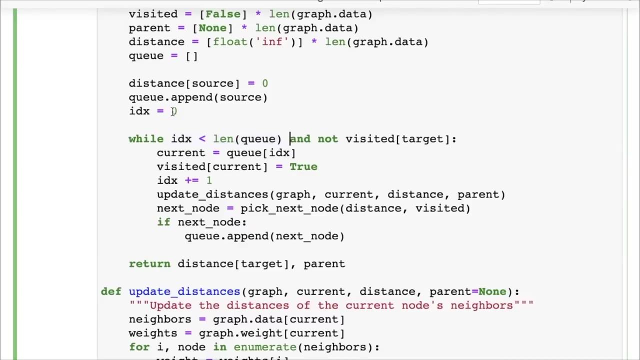 However, the complexity will be different, because in the shortest path algorithm- let's see it here- In the shortest path algorithm, what we do is we go over all the vertices, So that's we insert each vertex or each node into the queue once, and then we take it out once. 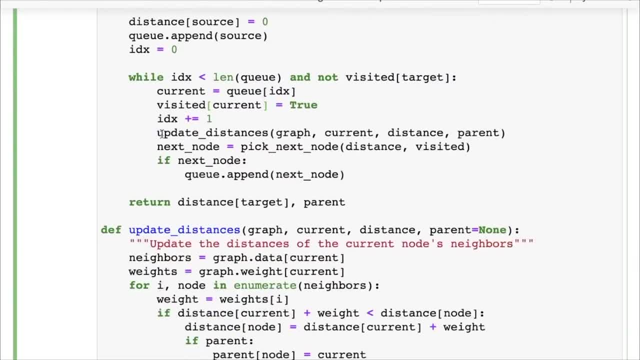 So this contributes a factor N, Then when we are seeing update distances, then it also contributes the factor M. But when we are picking the next node we may revisit all the vertices once again. right, So here we are performing N operations inside, when we are picking the next node. 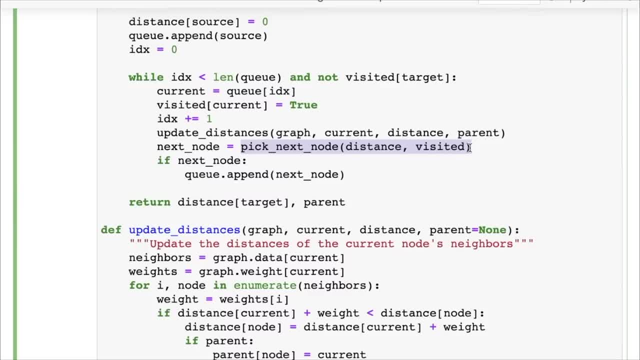 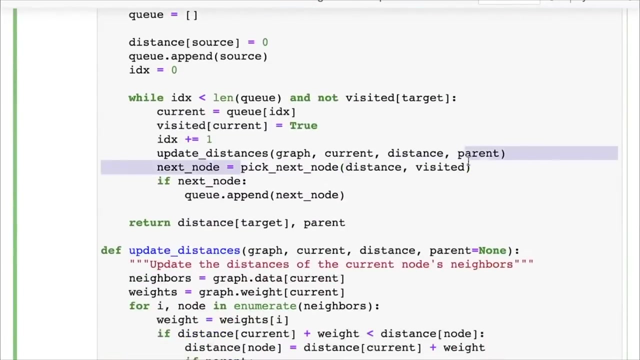 So that gives us order of N square plus N M, N square plus M. Yeah, something like that. So order of N square plus M or N N plus M into N. So that's, those are some complexity. Is that you will see reported for shortest path and a way to improve this, a way to improve the picking of the next node, is to use what is called a min heap, so that you don't have to look through the entire list of nodes each time to pick the next node, but you can simply pick the next node in a very short time. 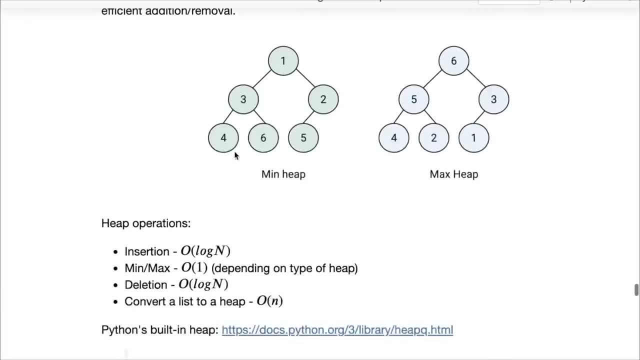 So there's a data structure called a min heap that you can look at. the min heap allows is used to keep track of a bunch of numbers and easily track the minimum. So you can keep a bunch of Numbers around in a binary tree like this and the root will always be the minimum and the numbers on the left and right will always be larger than the root. 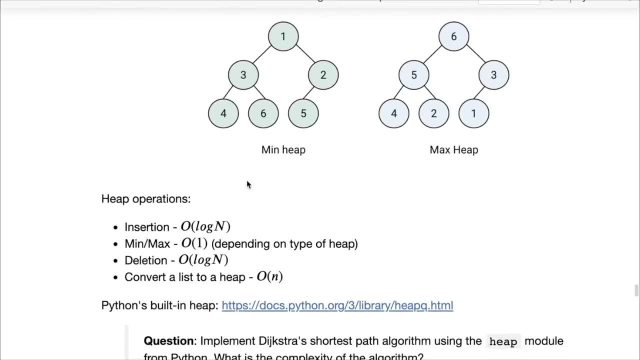 And then the same will be true for each sub tree as well. An insertion into this heap is of order login and deletion into this heap is of order login as well. And then the min max, in this case of fetching the min or the maximum value, is of order one. 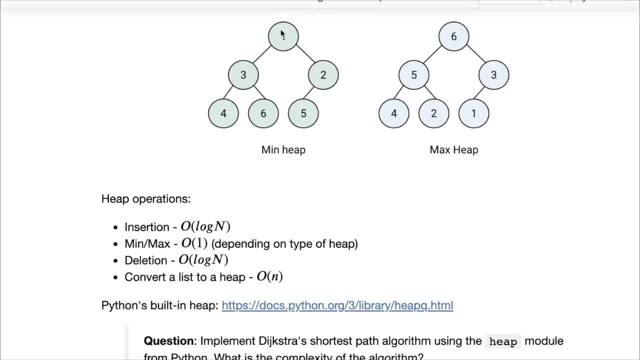 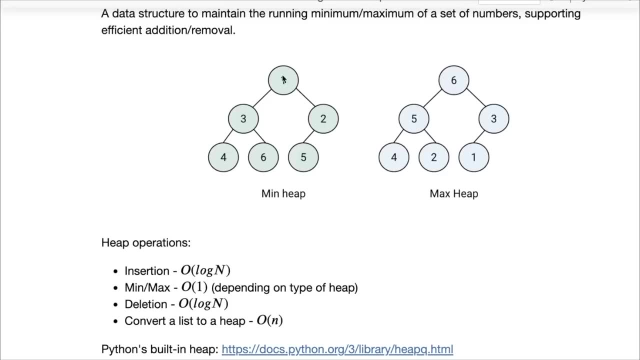 So, instead of minting, instead of looping through the entire list of nodes each time, what you can do is you can simply insert Nodes into this min heap and delete nodes from the min heap when they become visited, and getting the next node is as simple as fetching the minimum value. 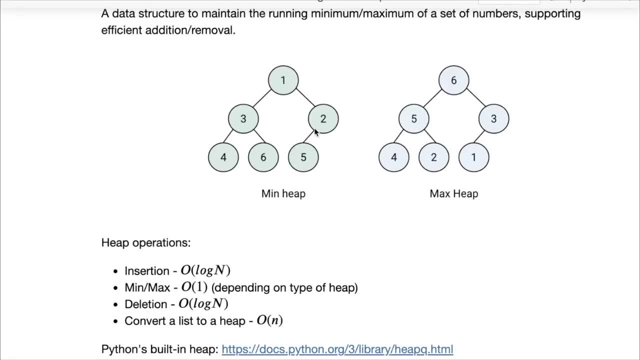 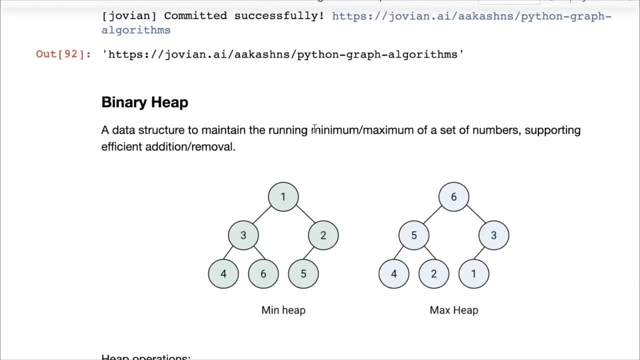 Okay, So check this out. This is not something that will generally get us. This is a more advanced concept, In fact, even the diastra shortest path algorithm. it's very unlikely that you will get us, but do review it and do try as an exercise. 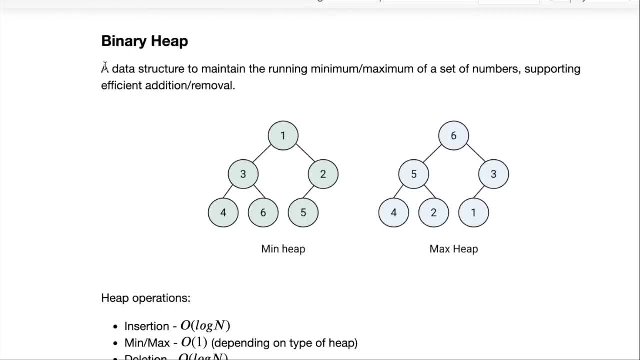 If you want to go further, try implementing and improving the diastras algorithm using a binary heap, So that will take the complexity for from M plus N times N to M plus N times login- Okay, And that may be better, So do check that out. 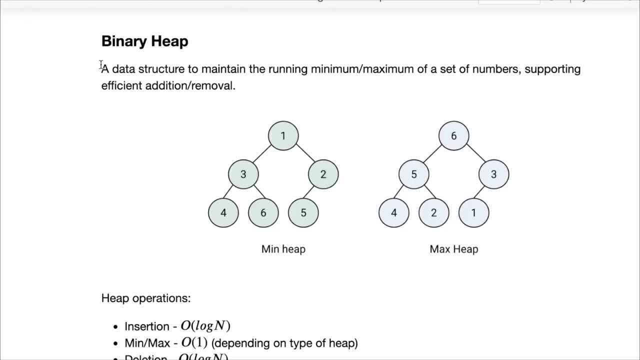 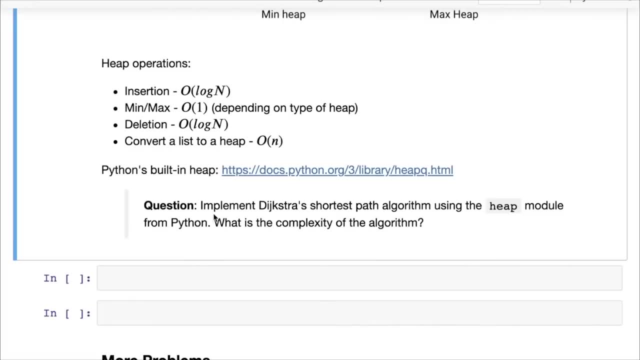 That's obviously going to be better for larger graphs, but do try to implement it. In fact, inside Python there is a built in heap called the heap queue data structure and that will. that will optimize the pick. next node. Okay. 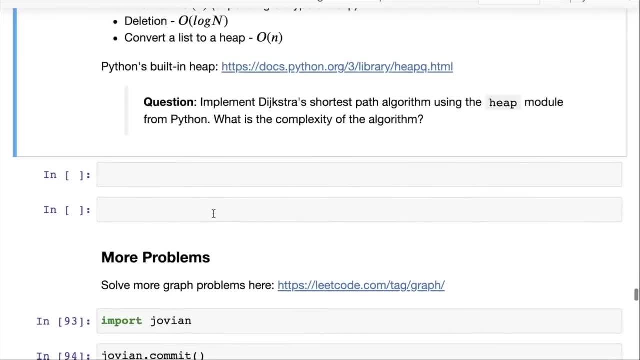 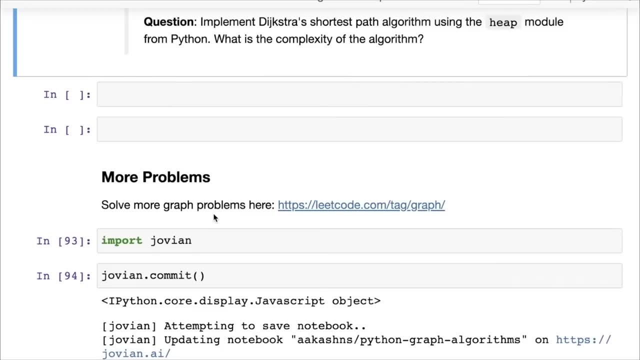 So that concludes our discussion of graphs here. there's a lot more in graphs. graph theory is an entire course in itself, but since this course is particularly concentrated on data structures and algorithms from the perspective of coding interviews and coding assessments, this is as far as we need to go. 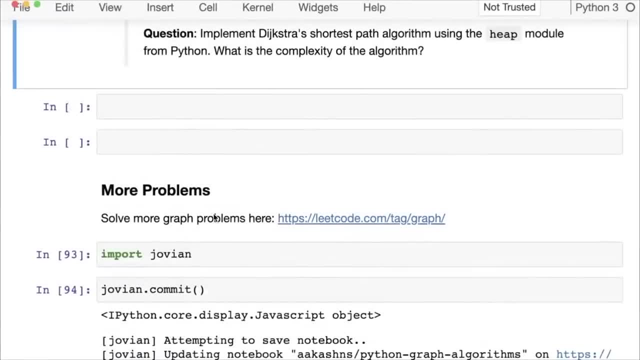 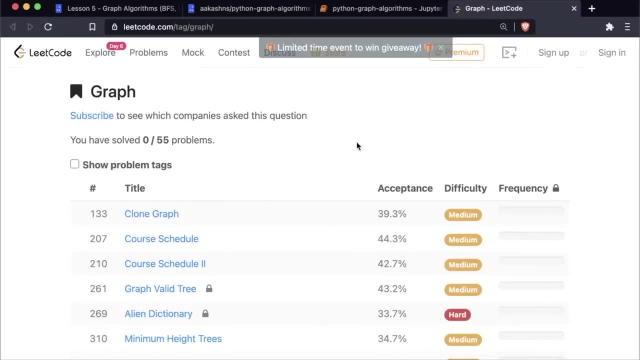 So what you should do is you should practice more graph problems related to breadth first search and depth first search. That is really something that you need to become very familiar with: Breadth first and depth first search and shortest path. maybe in sometimes some some really hard interviews you may get asked to shortest path as well. 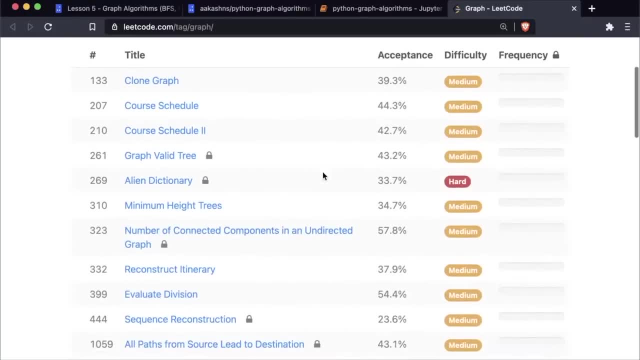 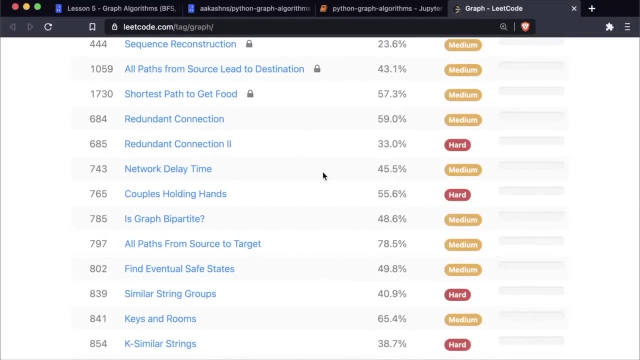 So do familiarize yourself with that. But apart from that, you don't really need a lot more. but there are other algorithms. You can look at minimum spanning trees. You can look at topological sorting. You can look at connected components. 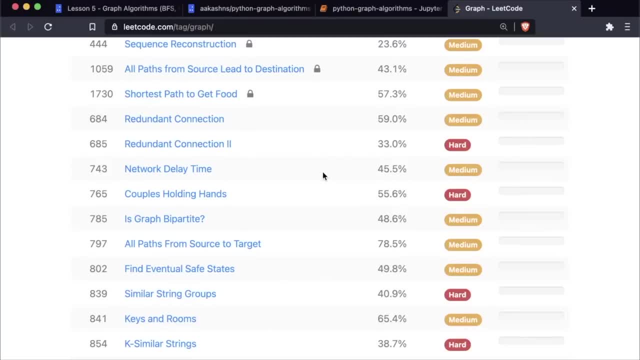 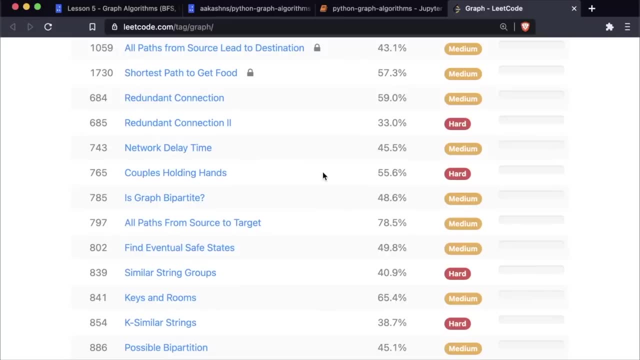 That's another path. You can look at detection of cycles And there's something called It is joint set. So there's a huge, huge number of topics that we can cover in graph, but we'll stop our discussion here. So what do you do next? 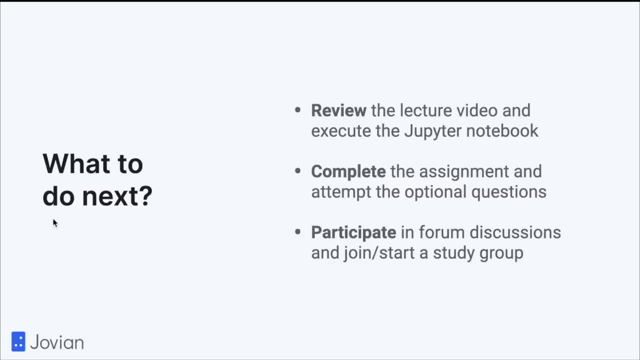 Review the lecture video and execute the Jupiter notebook, complete the assignment and attempt the optional questions And finally, participate in forum discussions- Very important. If you're stuck at any point, just go on the forum, ask a question. You can also share your code, as long as it's not working, to get help. 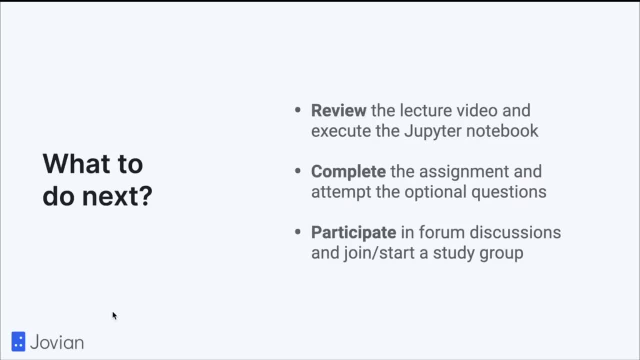 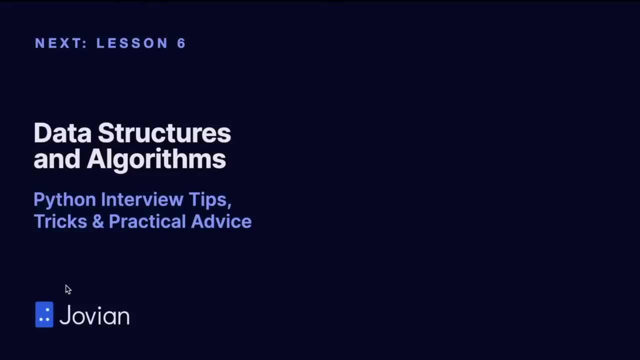 And you can also join or start a study group to learn together with friends, And you can also find us on Twitter, at JovianML and at AkashNS. And the next lesson is data structures and algorithms. In data structures and algorithms is Python interview: tips, tricks and practical advice. 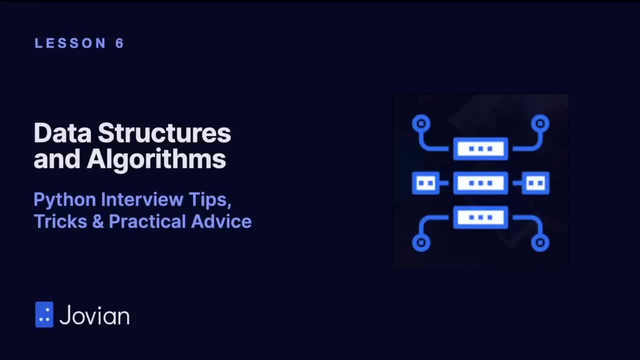 Thank you, Hello and welcome to data structures and algorithms in Python. This is an online certification course being conducted by Jovian. Today we're on lesson six: Python interview tips, tricks and practical. This is the final lesson of this course, so I hope you're excited. 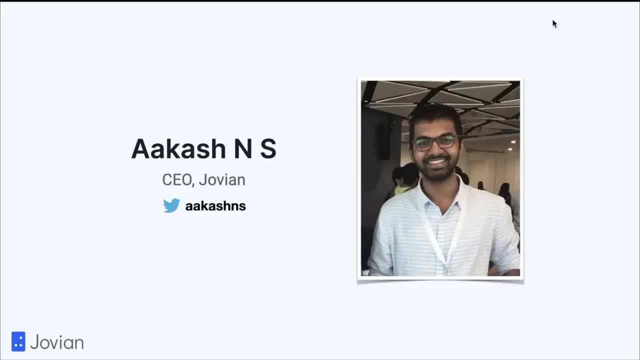 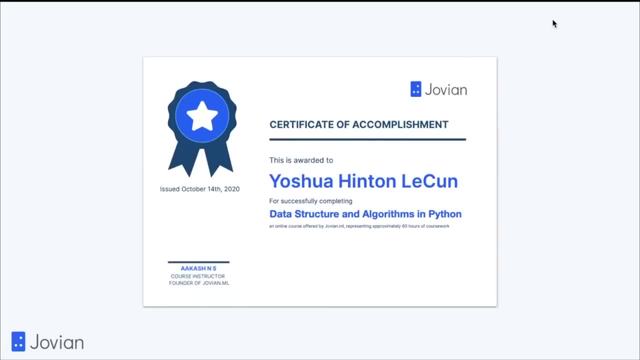 My name is Akash and I'm your instructor. You can find me on at AkashNS. If you've been following along with this course and you have been working on the assignments, and if you complete a course project as well, then you can earn a certificate of accomplishment for the course, which you can find on your JovianMLcom. 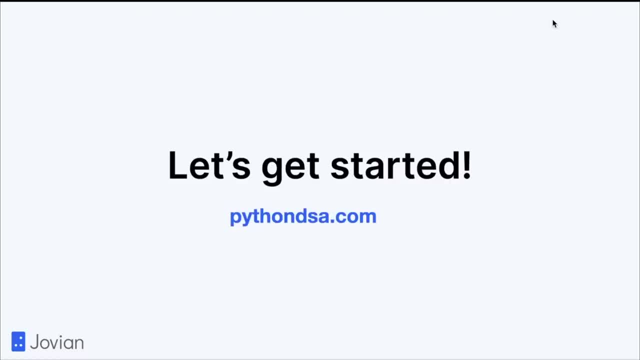 You can also add to the JovianML profile and also add to LinkedIn or download as PDF. So let's get started. First thing we'll do is go to the course website pythondsacom. So this is the course website, pythondsacom. 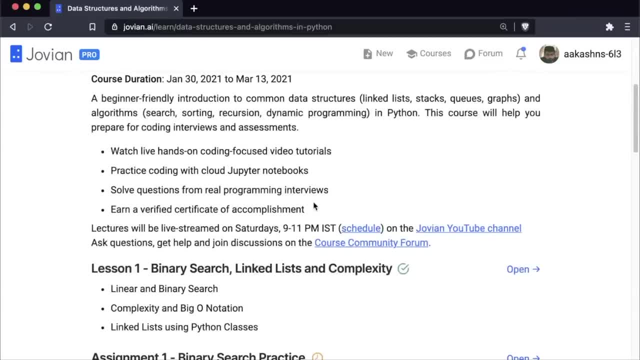 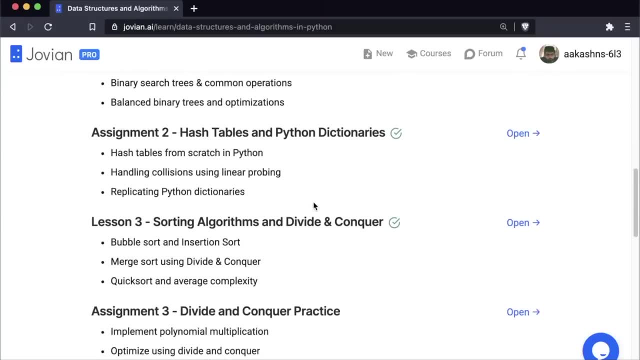 This is where you'll find all the information about the course. You can watch all the previous lessons, lessons one through five, and you can also check out the previous assignments- assignment one, two, three and you have the course project as well. 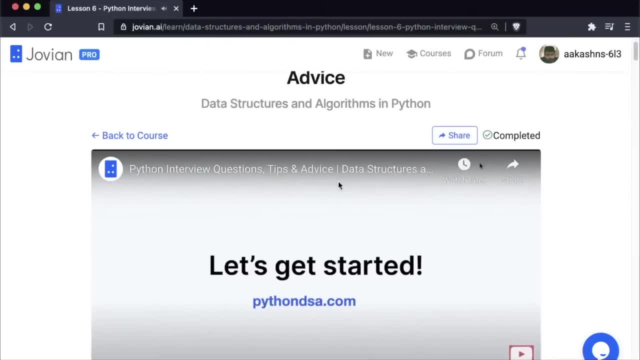 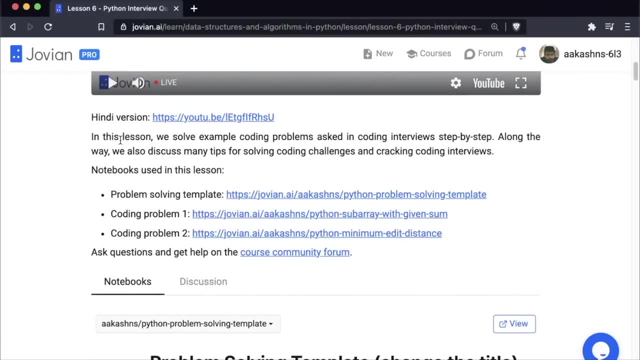 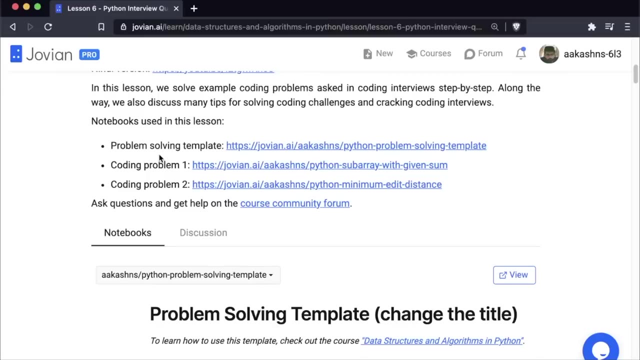 Let's open up lesson six. Now, on lesson six, you will be able to find a video recording of the video you're watching right now, And here is the code that we will look at today. So today we'll do something different. We will simulate the experience of being in an interview. 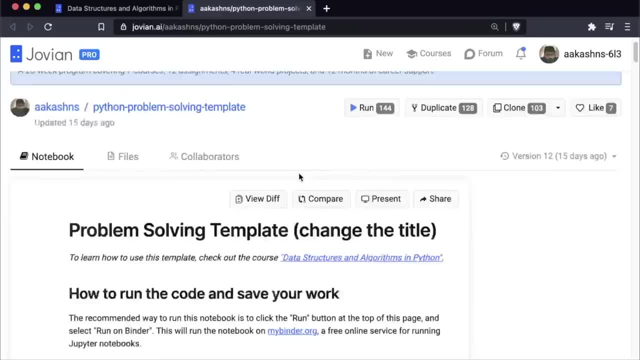 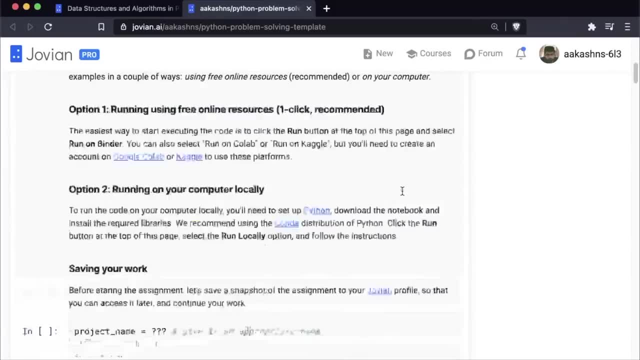 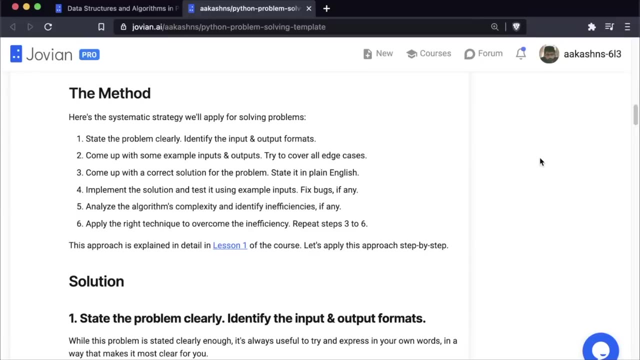 So, while we have given you a problem solving template and we recommend that you follow this template- What any project, Okay, Or any notebook that you work on, any coding problem that you work on- And here on the problem solving template, we also have a method, something that we have been applying throughout this course to different kinds of problems, different kinds of data structures and algorithms. 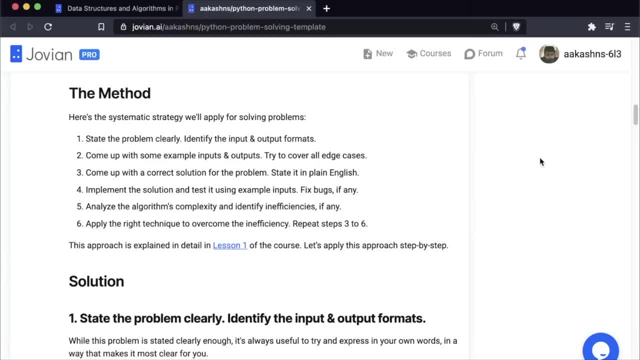 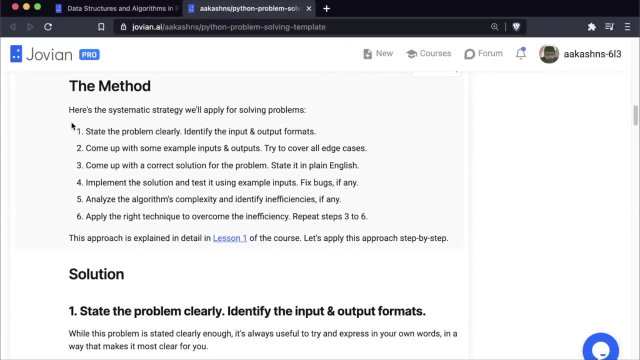 But in an interview, obviously, you will not have this template, So we'll see how to apply this method during an interview And before we do that, let's revise some methods so that we can recall it from memory when we are working on the interview. 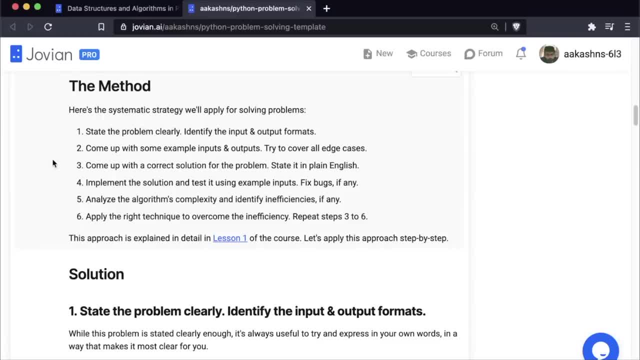 So here is the systematic strategy that we have been applying so far for solving problems, and do check out the previous lessons, If you haven't seen them, for examples of how to apply it in detail. So the step one is to state the problem clearly in your own words and identify the input and output format. 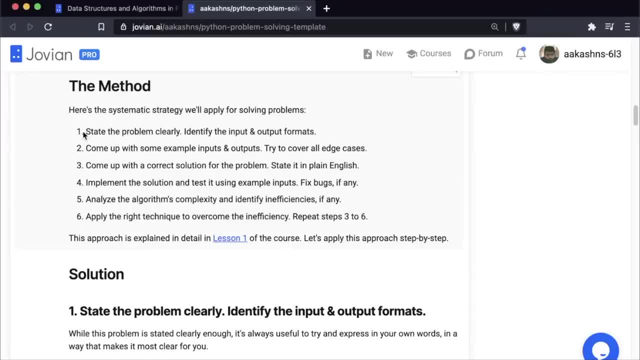 And then the second step is to come up with some example inputs and outputs and try to cover all the edge cases that you can think of. Do you want to think of all All the possible scenarios and that will help you write your code properly. 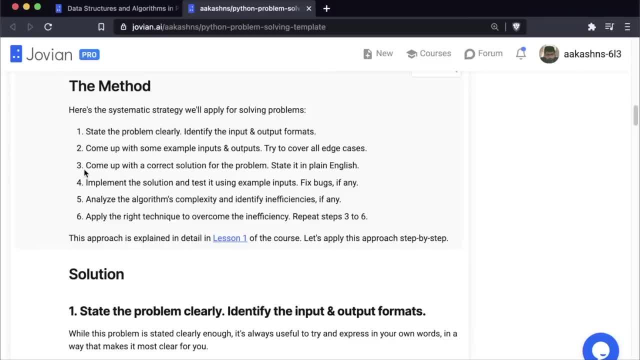 Then step three is to come up with a correct solution for the problem and state that solution in plain English, And then step four is to implement the solution and test it using some example input. So this is important while you're practicing, but initially, when you come up with a correct solution, it will be a simple solution. 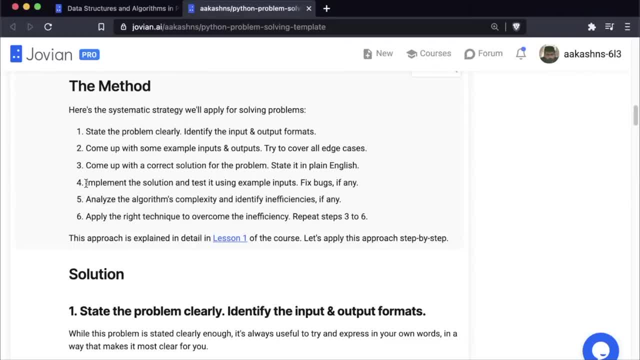 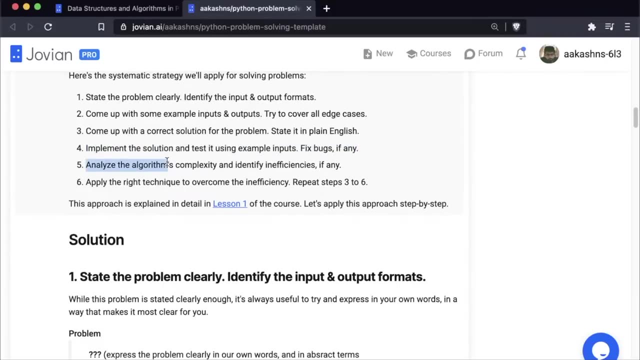 What is often called a brute force solution, And in an interview setting you may not have the time to implement it from scratch, So You may skip. if the brute force solution is too straightforward, Then step five is to analyze the algorithms complexity and identify any inefficiencies in the algorithm. 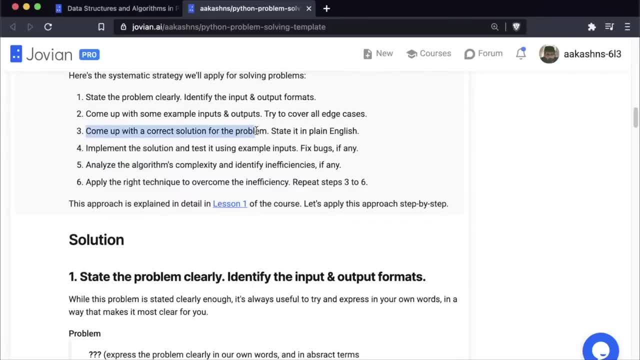 So what you can do in an interview is come up with a correct solution and describe it to the interviewer and then analyze its complexity directly and start identifying inefficiencies and then move on to apply the right technique to overcome the inefficiency. So this is where you need to identify what 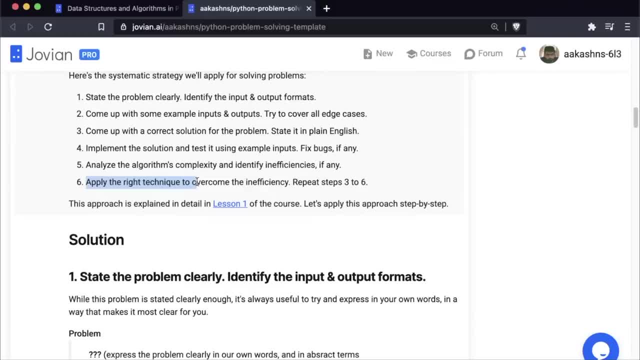 Which one of the techniques That you've learned in this course do you need to apply? Is this a binary search problem? Is this a divide and conquer problem? Is this related to binary search trees? Is this something that you can solve in a similar way? 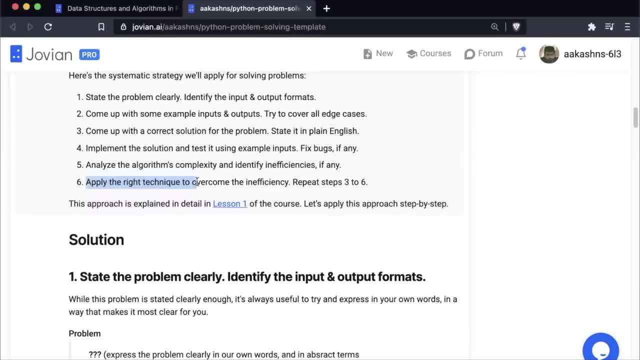 You'd solve sorting. Is it important to look at the worst case or average case complexity? Is this a graph problem or is this a recursion? or is this a dynamic programming or a memoization problem? So all of these things are something that you have to think about. 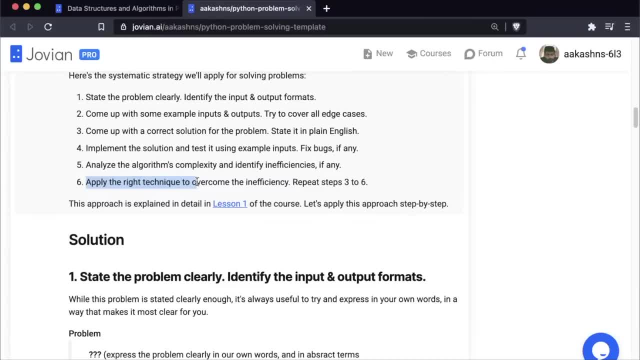 And as you practice more and more problems. So for each of the lessons, if you try and practice about five to 10 problems, then you will start to recognize these patterns And when you're on step six, when you're trying to come up with the right technique to overcome the inefficiency, the ideas will automatically come to you. 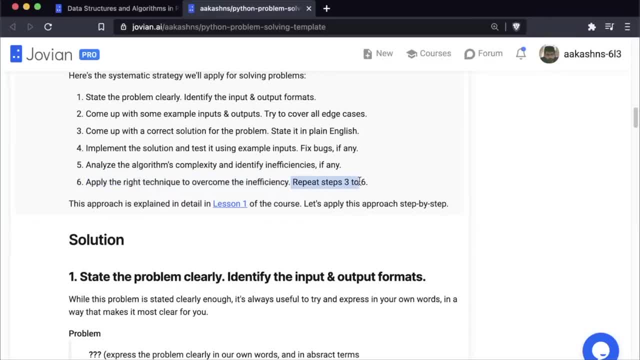 The practice is very important to succeed in step six. And once we have determined how to overcome the inefficiency through the right data structure or algorithm, then we state that solution implemented. analyze the complexity right. So this is how your a coding assessment or an interview should proceed for you. 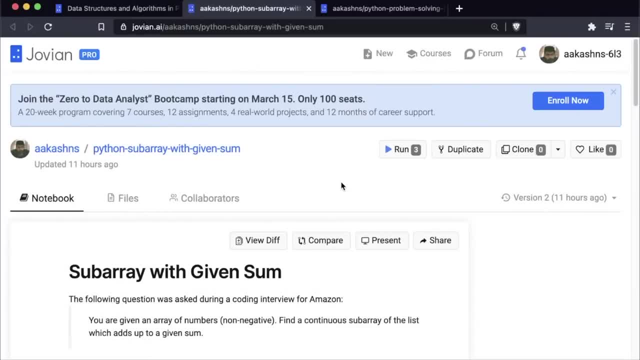 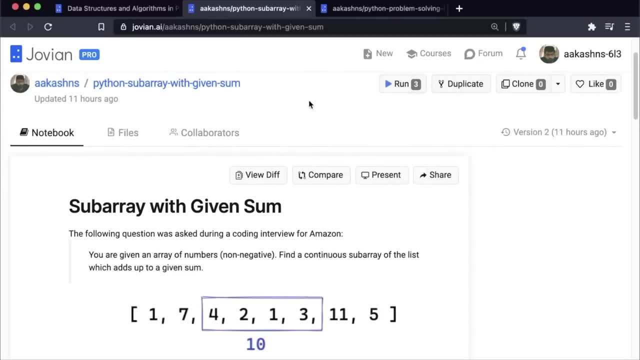 And let's see, let's pick up a coding problem and let's go from there. So here we have a coding problem, Python sub array with the given sum, and we read the problem, But before that you can see that here this notebook is fairly empty. 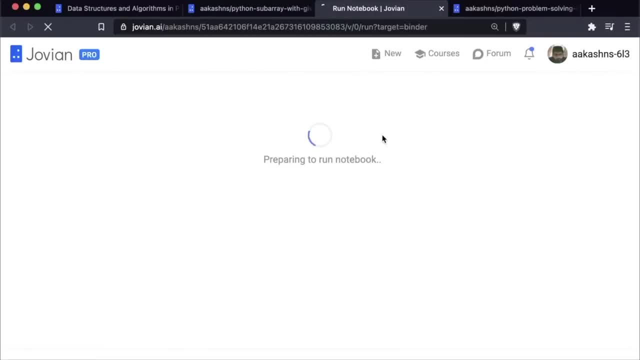 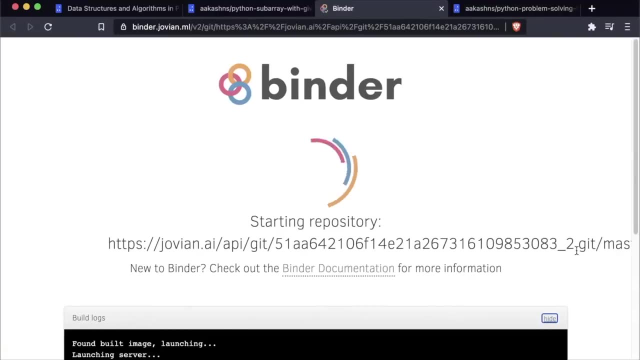 And we'll. what we're trying to do is we're trying to simulate the situation where you are on a call with somebody and they're interviewing you And typically they would be using some platform Like a collab edit or maybe a platform where you can also run the code, or a platform where the question is somewhere, let's say, on the right. it's already printed. 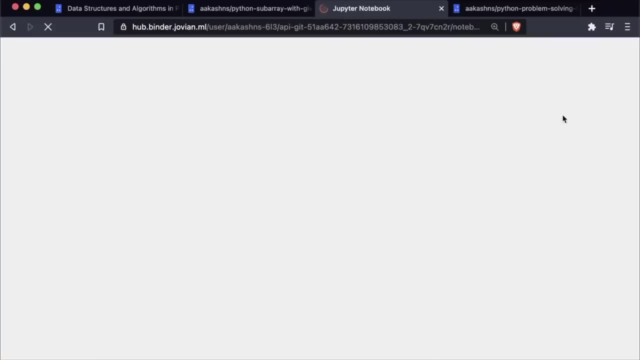 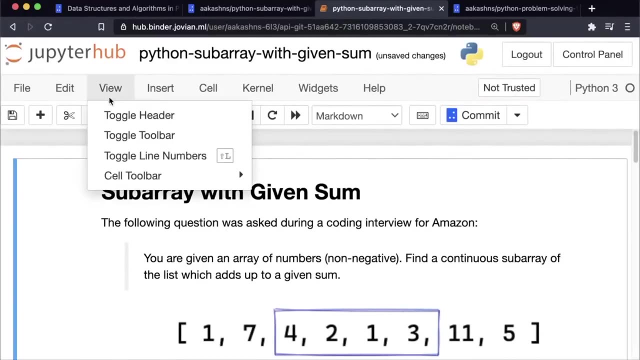 It's from a pre-selected database on on the right, on the left and on the right. you can type your code and you can experiment with it. Now we're not using any third platform here. What we'll do is we'll simply simulate that in our Jupiter notebook. 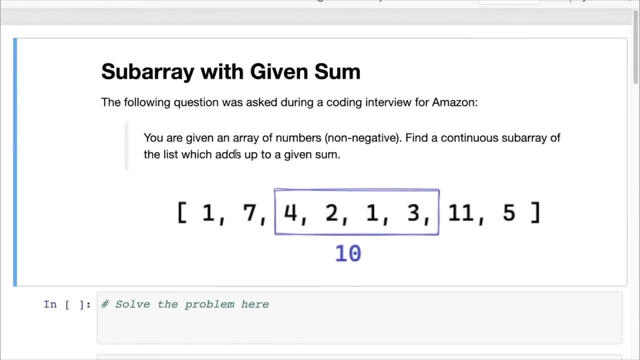 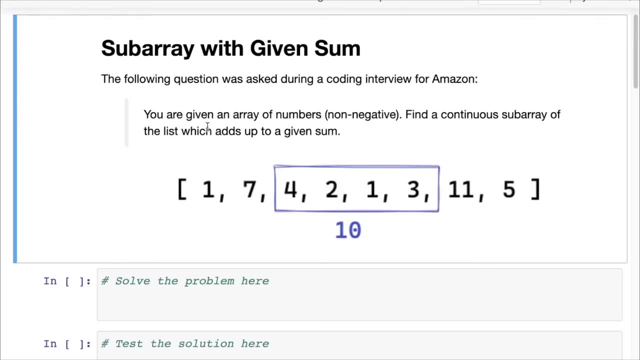 Okay, So now we have this notebook running, We've clicked the run button. Okay, We've clicked the run button on the Jovian notebook, and here we are Now. the question is- and this is a question that was asked during a coding interview for Amazon- 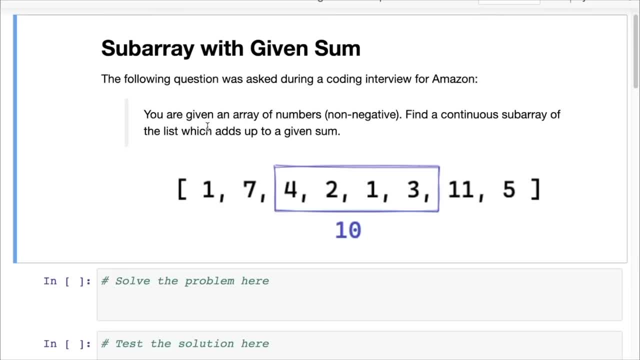 Of course, a lot of other companies may ask similar questions too. You are given an array of numbers and these numbers are all non-negative. You need to find a continuous sub array of the list which adds up to a given sum. This is how an interviewer might state the problem to you. 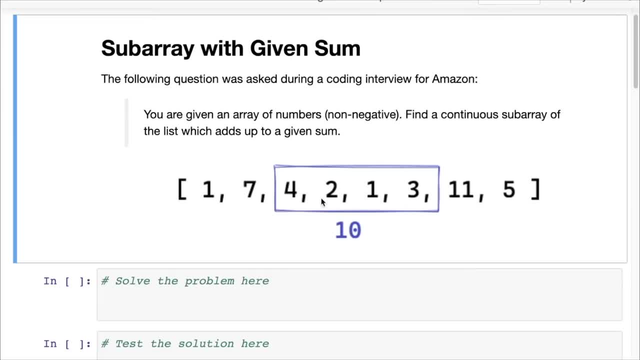 And then they may also tell you An example. sometimes they don't, And if they don't, it's always a good idea to ask. For example, you might sometimes feel that maybe if you ask too many questions, the interviewer might think that that you don't know this or you're dumb in some way, but that's not true. 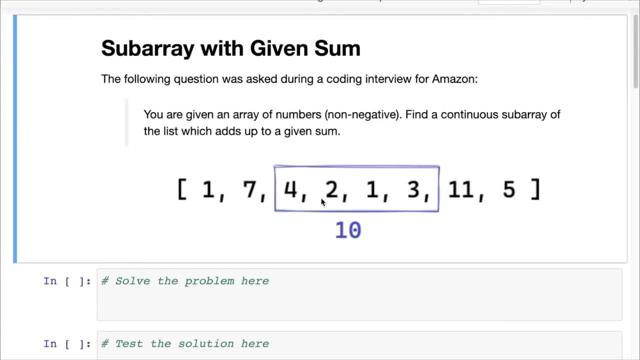 It's actually the opposite: The more questions you ask, the better the interview, the better the interviewer is able to convey what they want. right now They're busy. They're doing five interviews a day and they have their entire day's work. 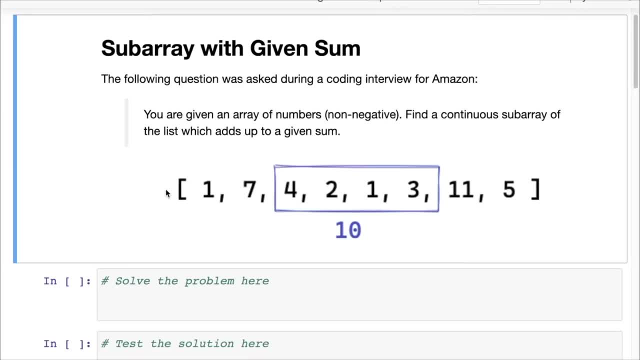 Sometimes they may just fail to state the question in its Entirety And if you don't ask for clarifications, you may assume the wrong thing and go ahead and implement something that's completely wrong And that completely deals your interview. and, trust me, it happens more often than you might think. 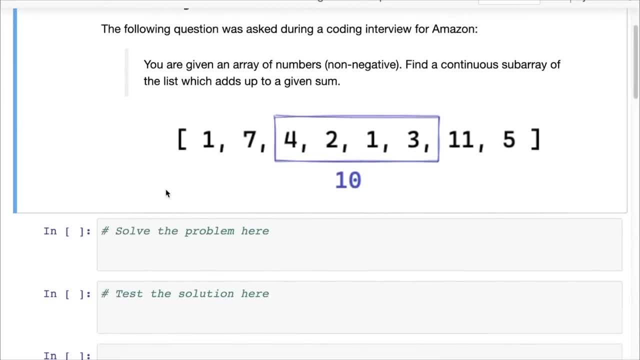 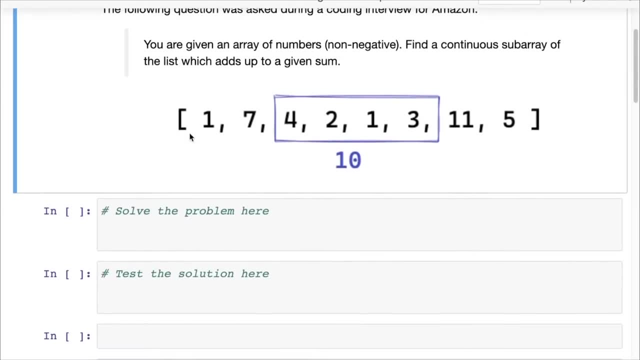 Okay, So we here is one example. So let's say, if the interviewer did not provide an example, you can ask them: can you please give me an example for this problem? And then they come back to you and they say, suppose we have this one. 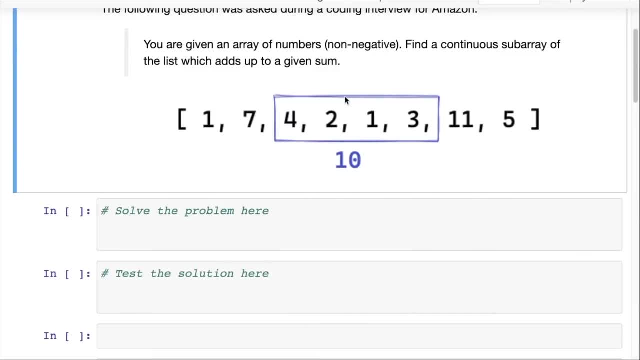 It's seven, four, two, one, three, 11, and five. These are, these are all numbers and they're all non-negative. Some of these could be zero as well, but suppose we have this area and I give you the number 10 that I want you to find the large. 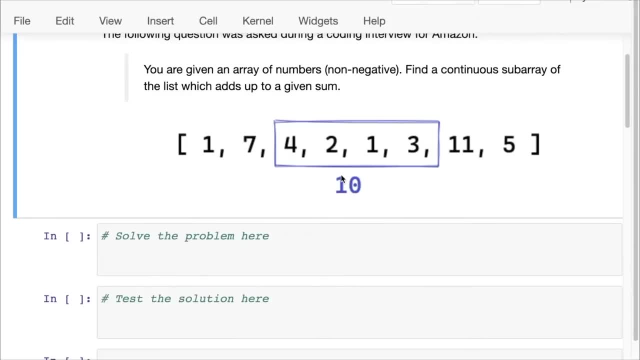 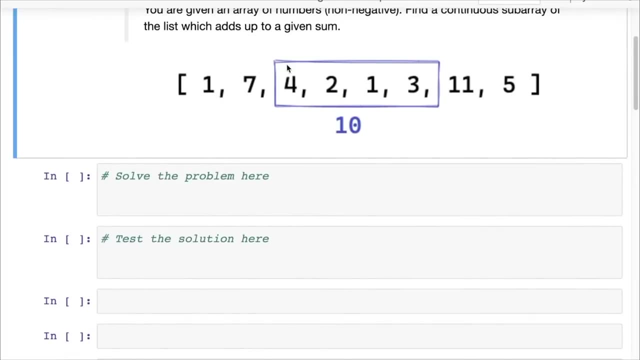 I want you to find a continuous sub-array of the list which adds up to the given sum, which is 10.. So then they might also tell you that in this case, the solution is this sub-array, starting from position four, or starting from the number four and going all the way up to. 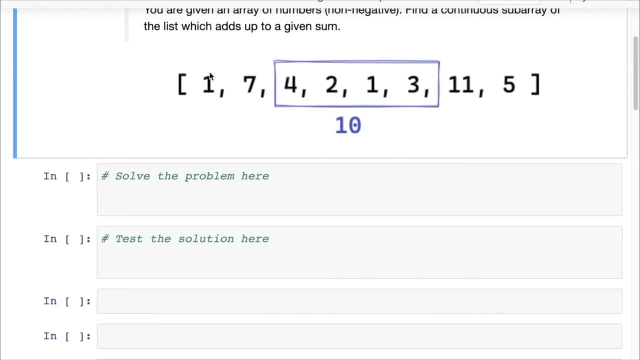 three, And you can check that. there are no other ways to create 10.. Like, if we took one seven, that would be eight, and one seven, four would be 12.. On the other hand, seven, four, two would be 12 again, but four, two, one, three turns out to be 10.. 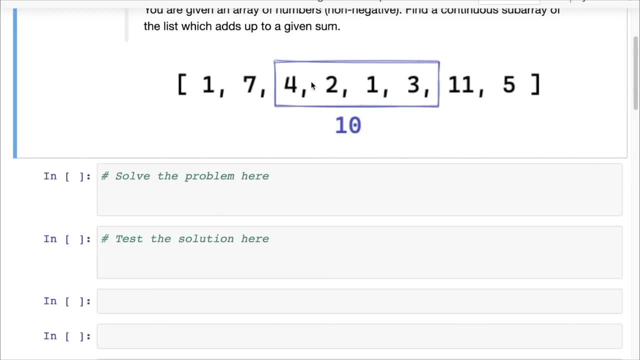 And once again on the right, you will not be able to create the total of 10.. So this sub-array is what you have to return. Now, what does it mean to return a sub-array? to return a sub-array means to return the indices, which is the index of the starting term or and the index of the. 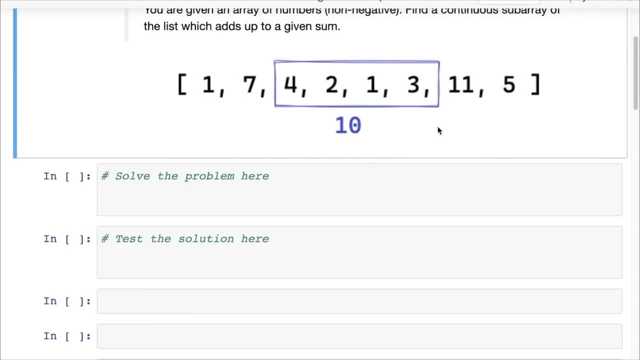 ending term, And sometimes we know in Python when we're working with ranges, typically the end index is outside of the actual data. So you could return the index of four and the index of 11.. So that we, so the index of four is zero. one, two, two is the index of four, three, four, five, six. index of 11, six. 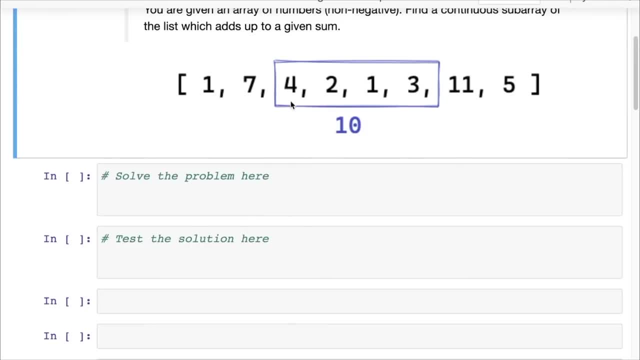 So if you return two and six and then I try to access the two to six, two colon, six, range of the list, then you will get get this list four, two, one, three, And in fact that's something that we can very quickly verify here. 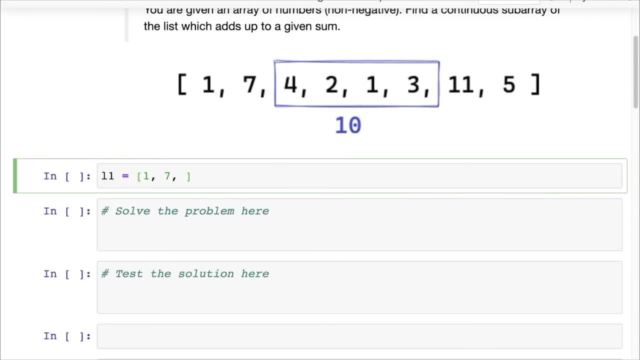 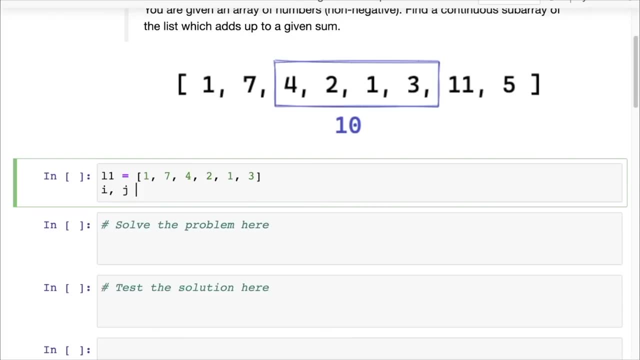 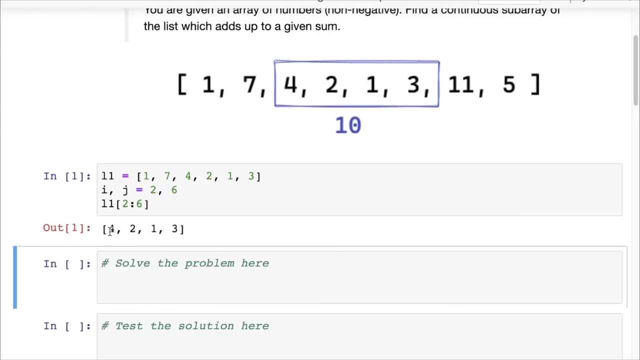 Let's say L one. So you have one seven, four, two, one, three. Now if I say that the start index is the start index I and the end index J are two and six respectively, And you can see, L one of two to six is four, two, one, three, right. 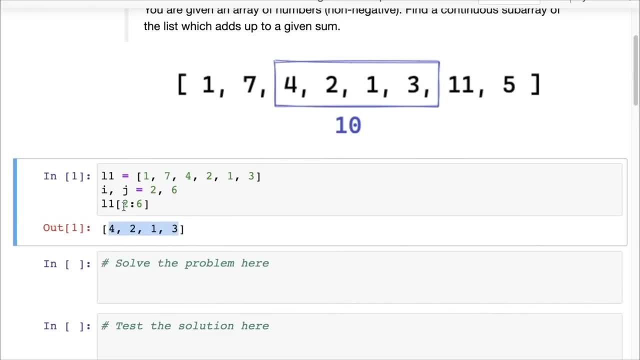 So although J is outside, so that doesn't get included when we put it as a range, And then we put in four, two, one, three, And you can also verify that the sum is 10.. Okay, All right, So that's the problem. 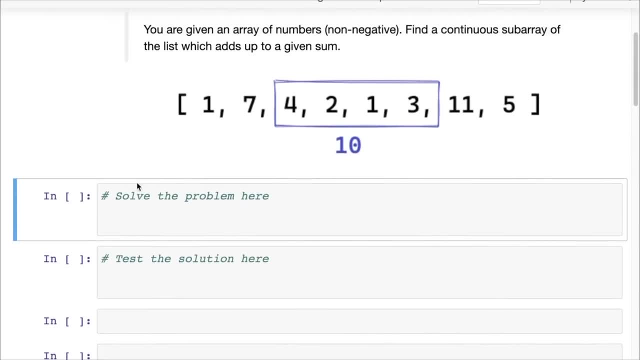 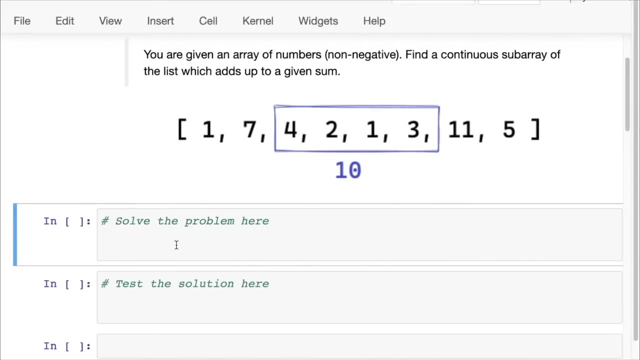 Now I've explained it to you in a lot more detail than an interviewer would, but this is the process that you have to apply in your own mind. What- and sometimes what you can also do, is you can repeat the problem back to the interviewer. 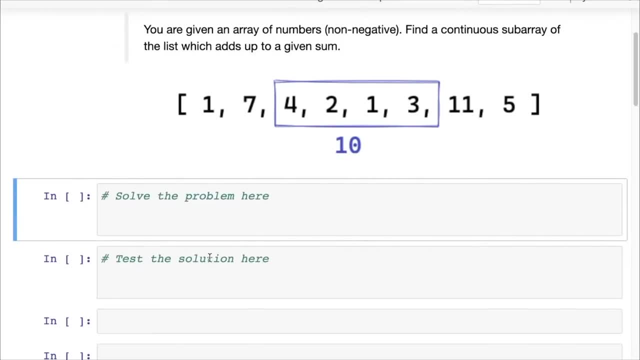 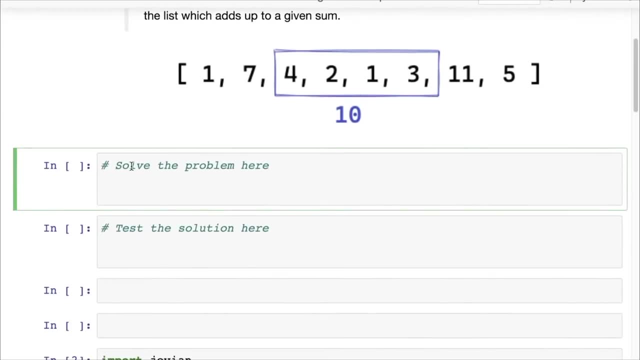 That's a great idea. You, you, they've stated the problem to you. They may be given you an example Now you state the problem yourself in simple words. Remember, that was step one. So in the same way that I just have, you can see it. 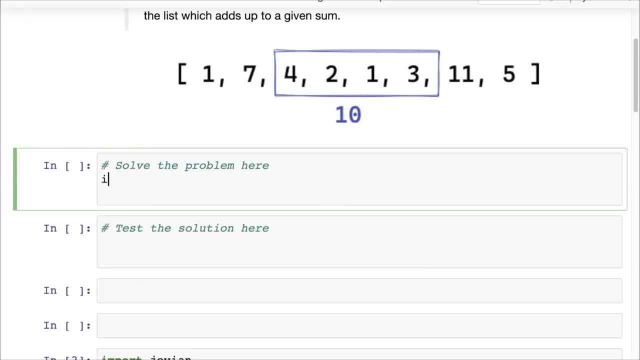 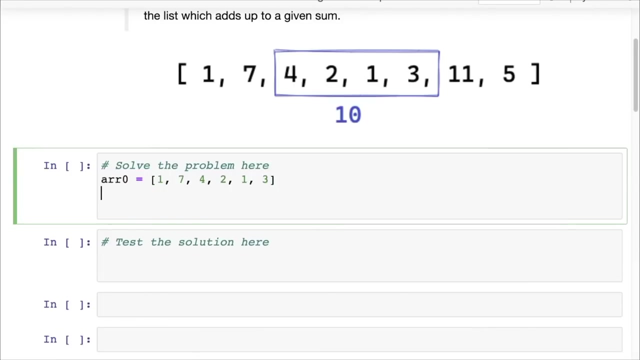 The problem. and then you have to figure out what are the inputs and the outputs. So the input, you have an array, or array is also a list in Python. So let's say ARR zero. let's create, let's make this the first- an example, first input, and that would be one, seven, four, two, one, three, and then the target. 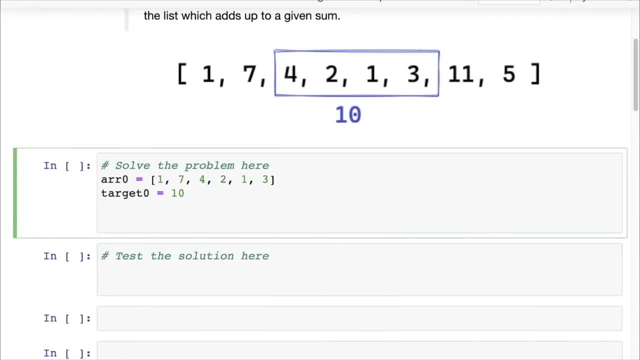 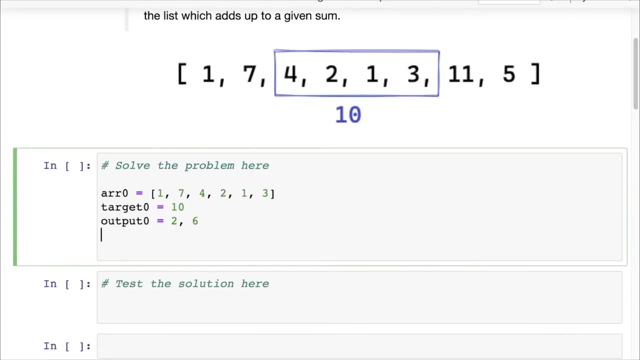 So your target sum is 10.. So that's the input here, And then the output that we want to want is: So this is the Output zero. That would be two comma six, as we've just verified. So this is the input and output format. always makes sense to just create some variables for that before you start coding. 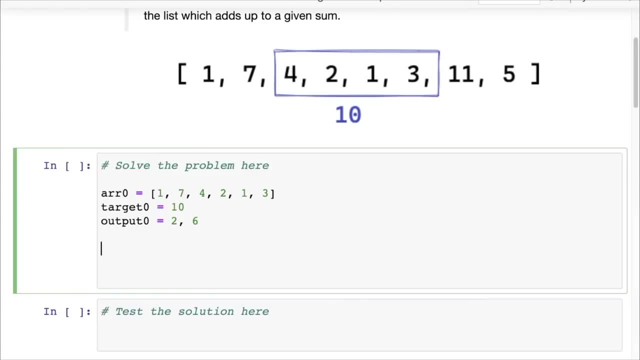 The next step is to think of what are all the cases that a function should be able to handle. But actually, before we do that, we should also write a function signature, because we know what the input looks like. We know what the output is going to look. 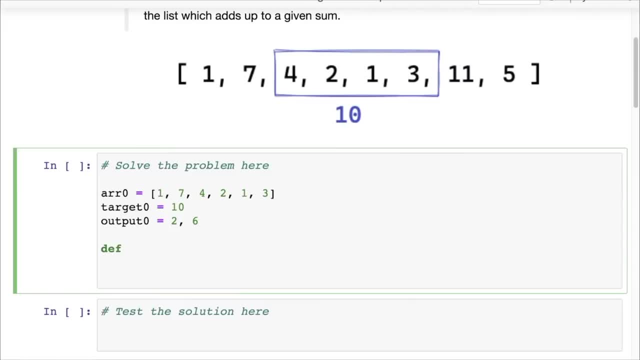 And we know what. so we know what the function should look like. So we can just say def and let's call this sub array sum, and it's going to take an array, It's going to take a target and there's going to be some logic inside it. 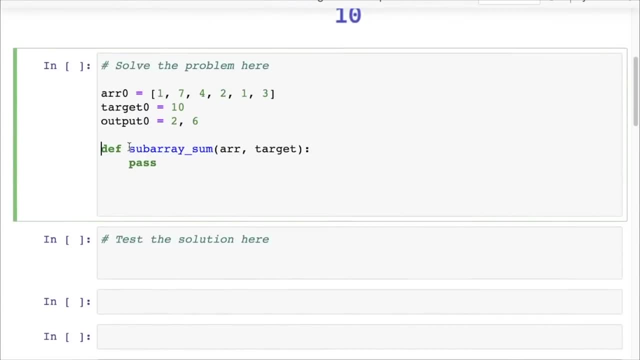 Okay, All right, So that was step one. Sorry, I forgot about the function signature, but it always helps to just write the function signature, because if you've misunderstood the problem still, the interviewer can immediately correct you and tell you: Hey, but you haven't taken a certain input or you've assumed. 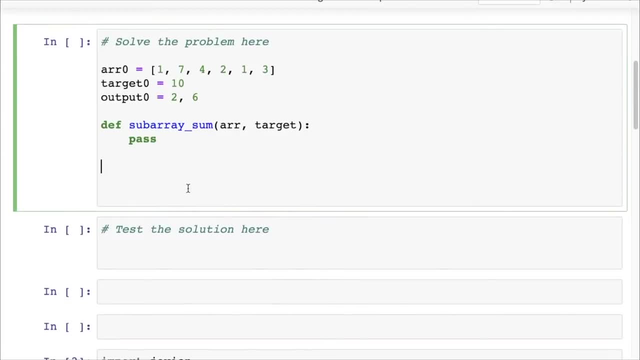 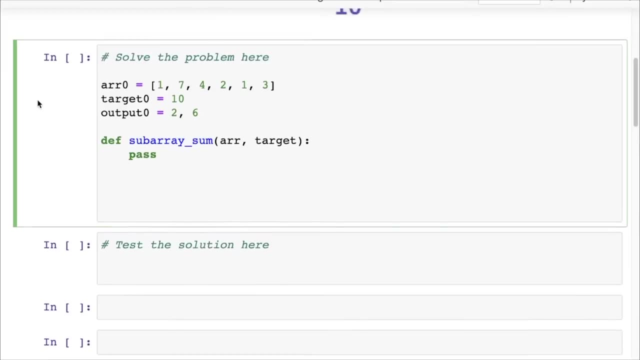 An input which I have not provided. All right, So now we have the function signature. Now step two. remember, step two was come up with an exhaustive list of test cases to test the problem. So you can do this in comments. 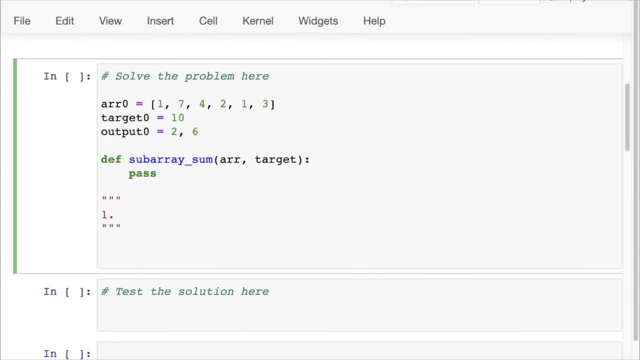 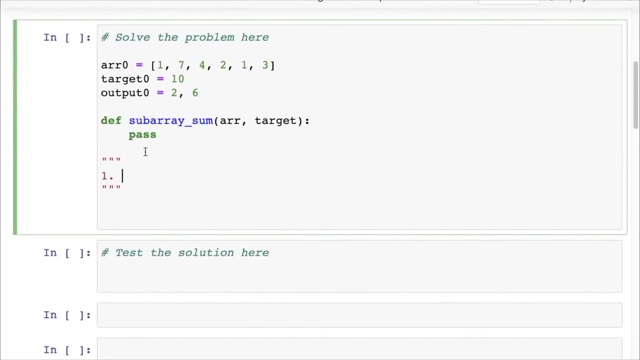 You can just create some comments and you can say: I'm thinking about the problem And I'm just trying to think what are all the cases we need to handle, And this is a great quality. This is not something people do often, but they should, because this indicates that you are doing what is called test driven development, which means you are thinking about all the 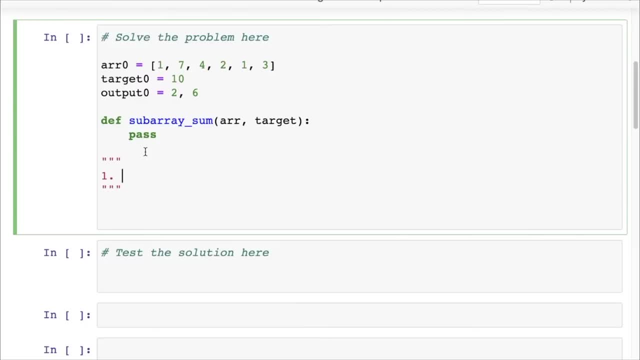 ways in which your board should code might be used and accounting for those before writing the code, So kind of working backwards, and it's a very useful way to avoid errors. So now the first one could be a generic area, where the sub area is in the center, somewhere in the center right. 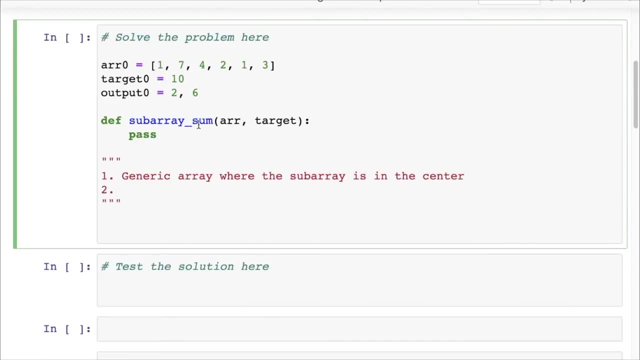 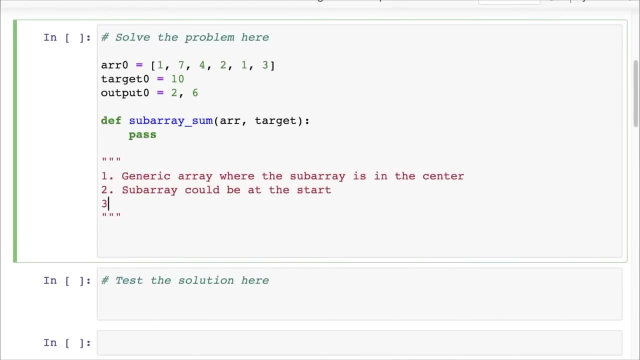 So, which is what we have already seen here now, the sub area would be in the center, or the sub area would be- Could be- at the start, or the sub area could be at the end, or it's possible that the sub area- there is no such sub area. 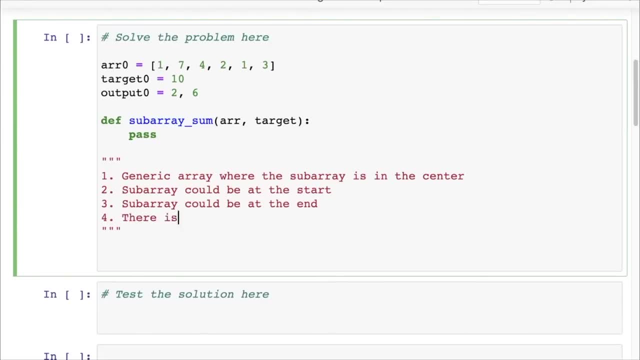 So there's no sub area which adds up to 10.. You may also have the situation where You have a few zeros, So you have a few zeros in the list. That's one option. Here's one thing that can happen. 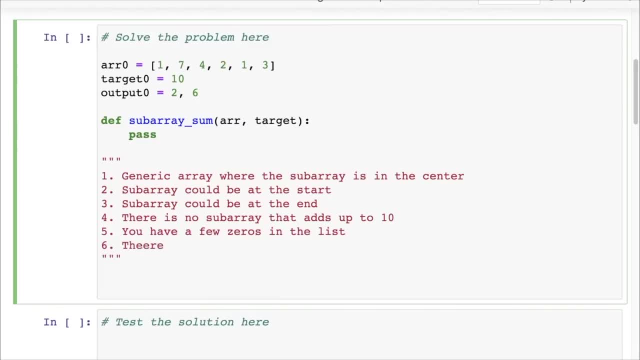 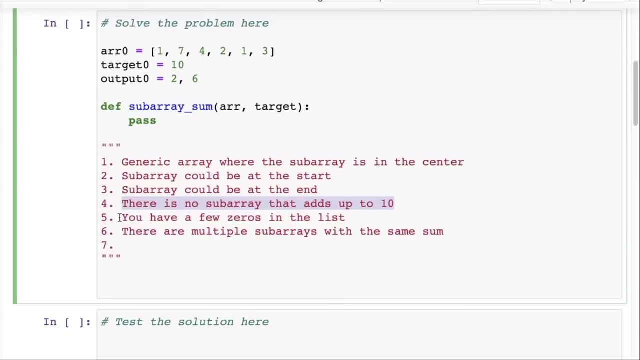 This could be that there are multiple sub areas with the same sum. Now this is where you might want to just clarify with the interview: Hey, what happens if we get two sub areas which add up to the same number- The target- and the interviewer might say: find the shortest one, or find the first one, or find any one, but it's always good to clarify that next one option could be that. or you could also ask them: what is what happens if there is no sub area that adds up to 10, and then they may tell you you can return none, none, or you can return minus one or whatever it is, or assume that there is always a sub area. 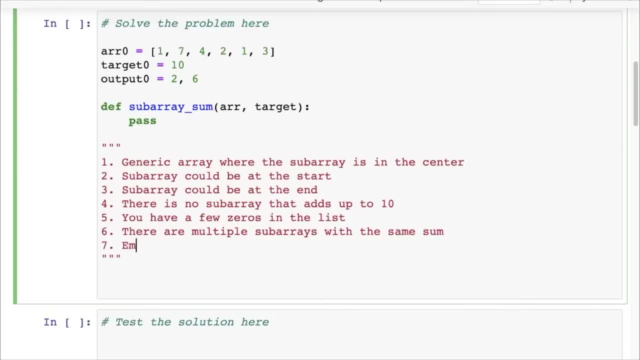 So that will help you write your code, And then you couldn't. obviously you may have to work with the empty area. You may also have to work with. the sub area is a single element And whenever we say rate we also mean list in Python. 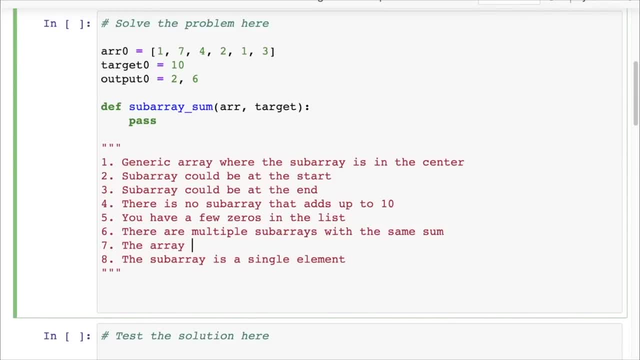 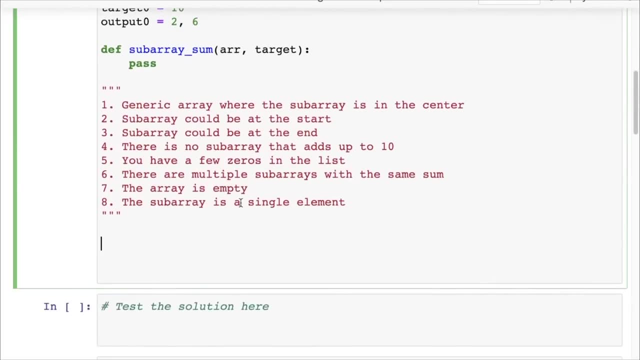 They're, practically speaking, the same thing for our purposes. Okay, We've listed quite a few test cases and in that process we've come across a few more questions which we've clarified. So now we're ready to start solving the problem. 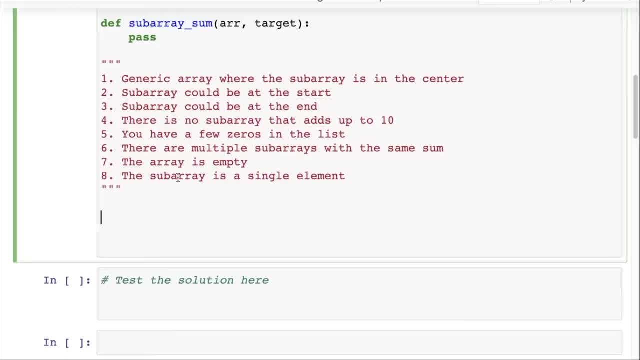 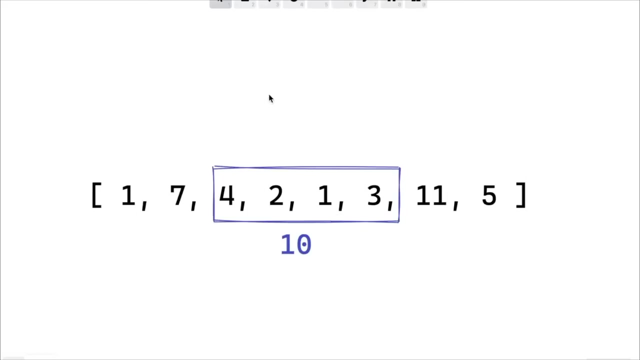 Now, at this point, what you may want to do is maybe just ask for a couple of minutes and keep a pen and paper close to you. I'm going to use this tool instead. Yes, I'm going to use this tool instead. So, keep a pen and paper close to you so that you can work on this problem. 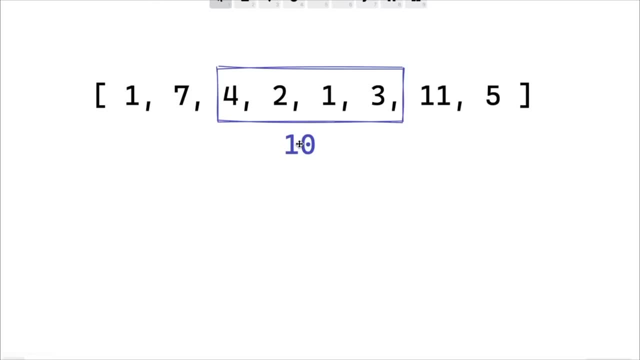 Now let's come up with the simplest possible solution. So we have about two, three minutes to come up with a solution, And often the simplest solution Is pretty obvious. So in this case, one simple solution could be. if I could simply try every sub area, then I will find at least one. 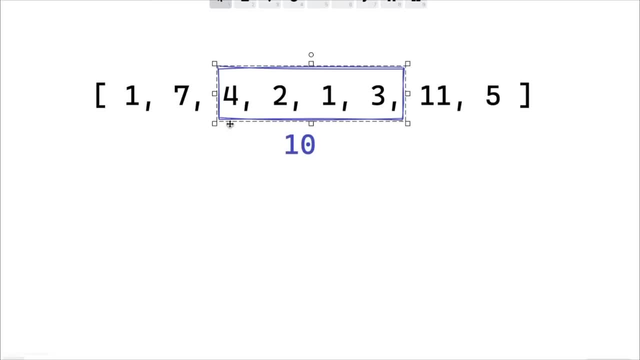 If that adds up to 10, if there is one. so all I need to do now? each sub is defined by a start index- That is where the first element of the arrays, and then and N index- the end index is just next, the next index, the first index which is not in the area. 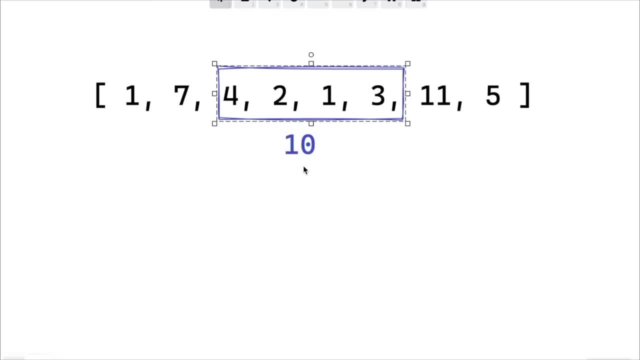 Right. So that's how we define a sub area, Remember. So all we need to do Is try all such values. So all such values: I, I, comma J, where I goes from zero to N minus one and where J goes from. 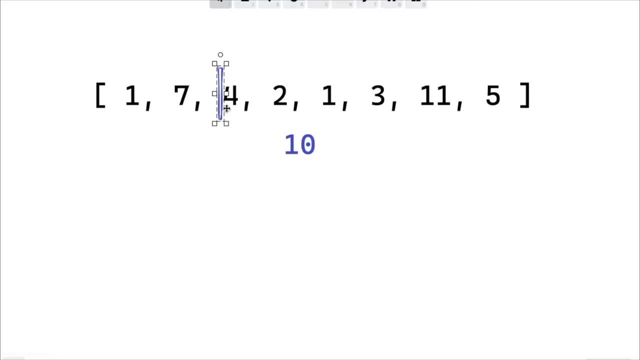 Remember you could start out with the empty sub array, which means J also has the value I. so here we are saying I and J both have the value two, So L. one of two to two becomes the empty area. So J grows from I to all the way beyond the last element, which means if the last elements index is N minus one, so J. 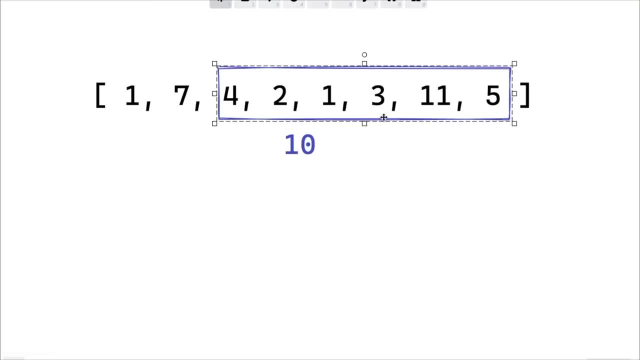 Can go all the way up to N, All right. So I goes from zero to N minus one and J goes from I to N, and each time we started an eye and we check each J. So we check: Jake was zero and Jake was one equals two, J equals three, four, five and so on. 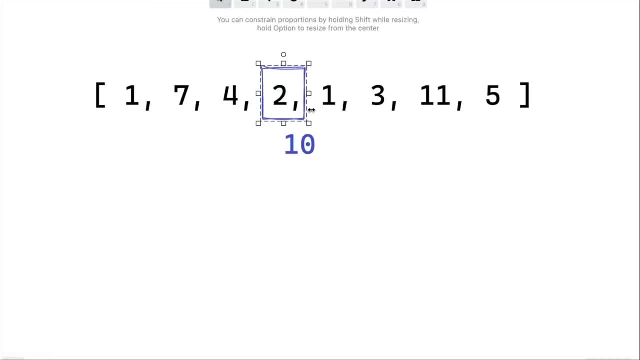 Then we move I again, and then we start over again, And then we say we start with J equal to zero, J equal to one, J equal to two, three, four, Okay, And- and we keep doing this to be finding an area and we've exhausted this way. 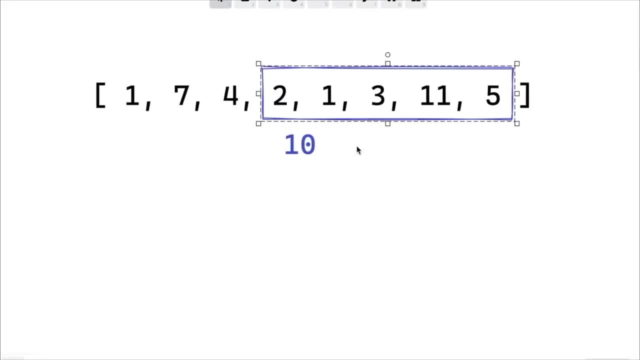 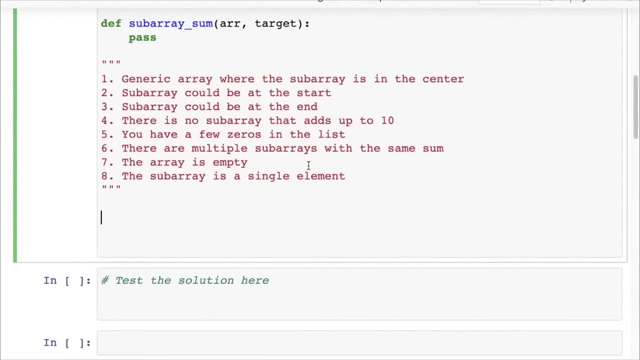 We'll test all this So the problem is solved. So that's the brute force solution, And what you should do first of all is explain that brute force solution. It may seem that this is an obvious solution. What's the point of explaining it? but to mention it because at this point the interviewer knows nothing about you. 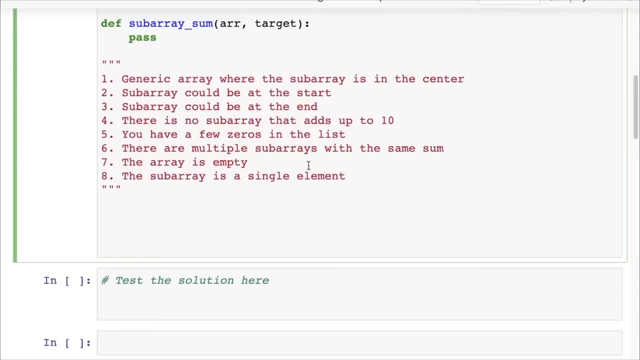 So they don't know if you can even come up with a solution to the problem, right? They're trying to assess. can you think about problems and they're trying to assess, can you write code? now, If you don't tell them the brute force solution, then they don't. 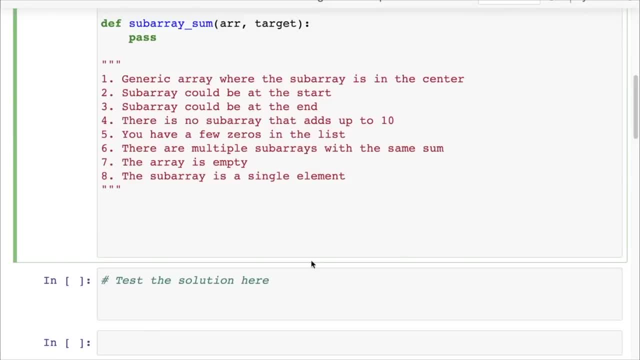 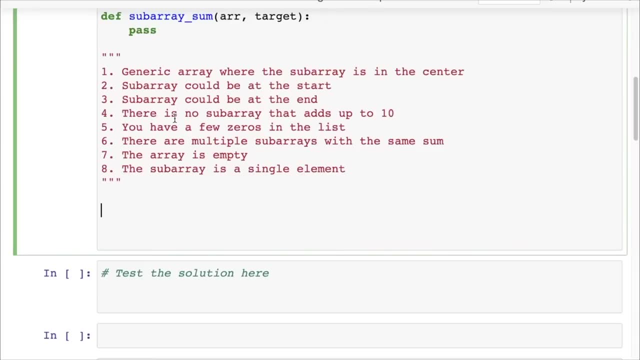 Even know if you figured out the brute force solution. So do tell them the brute force solution. And generally you do not have to hold it. You can do the analysis in your memory or in your mind and you can sort of write the code in your mind, picture the code. 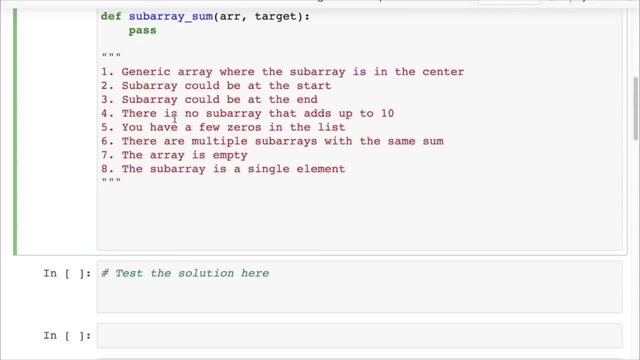 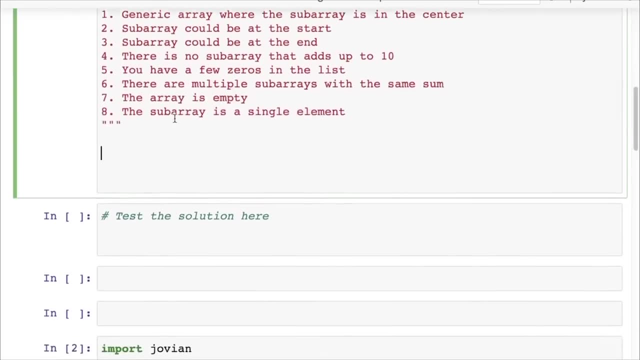 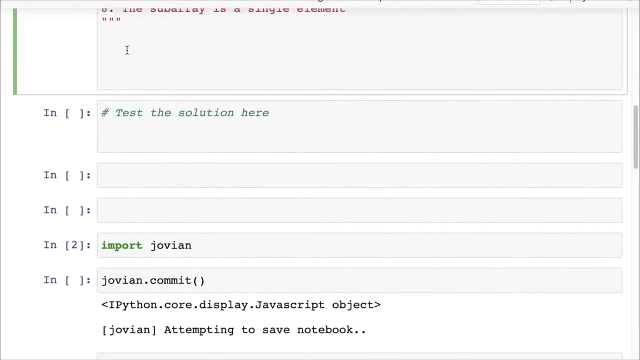 And, based on that, come up with the complexity analysis and directly say that the brute force algorithm will have such and such complexity. Okay, Now we will just write the code right now, just to be very clear about it, In case you have not. you're not yet clear on how to write the code, but in an interview this is the part which you can skip in the interest of time. 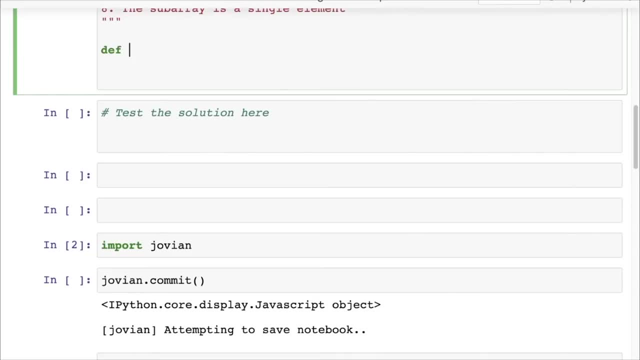 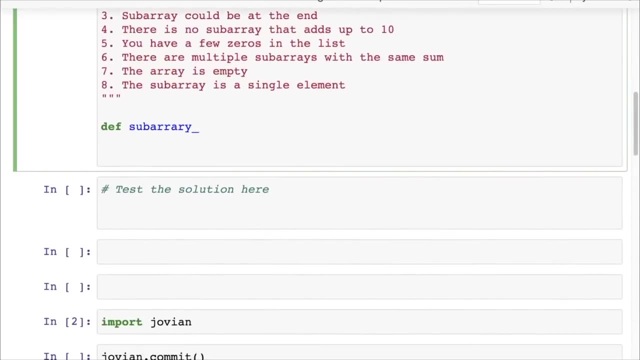 So def subarray- I think it was called subarray sum, subarray sum and let's call this subarray sum one. the first approach that we're taking here: We have array one and that's it. We have array, and then we have our target. 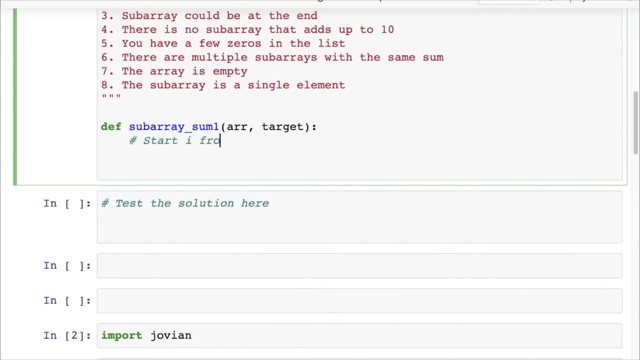 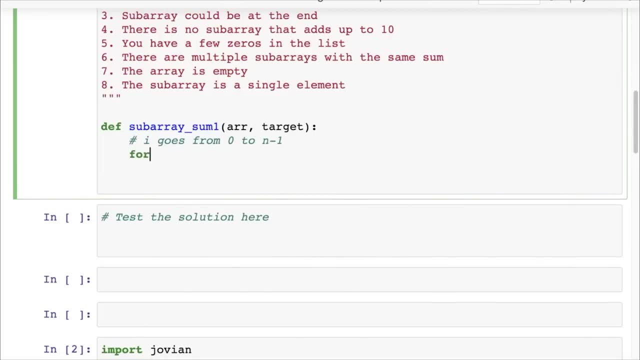 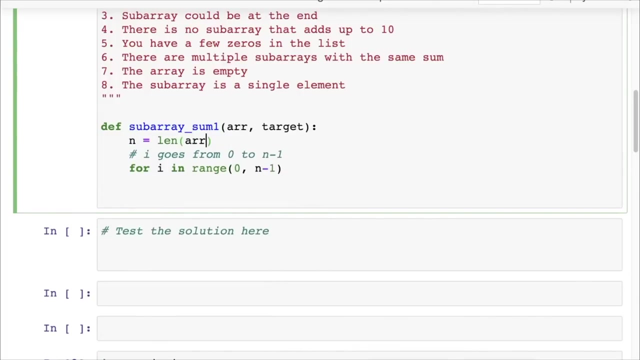 And we're saying: remember that, start I from the. I goes from zero to N minus one. That was the first thing. So for I, in range zero to N minus one. and what's N? well, N is simply the length of the array. length of the array. 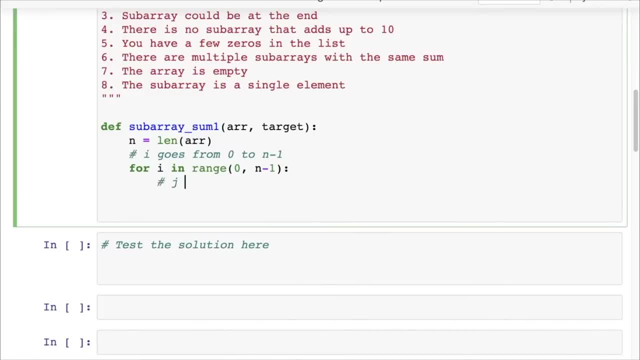 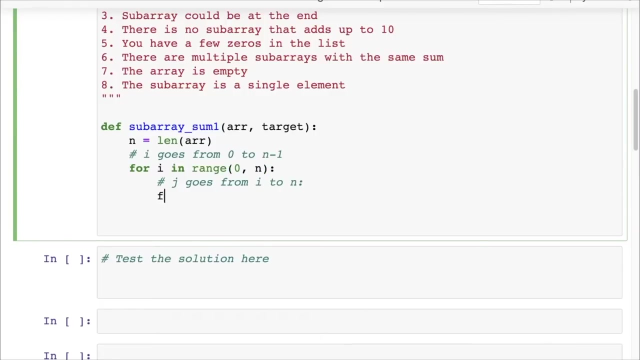 Then J goes from I to N. Oops, So I made a small error here. This should say zero to N, because even in a range the last value is not taken. The J goes from zero to I to N. So for J in the range I do, this should be N plus one then, because we want Jake to go all the way up to N. 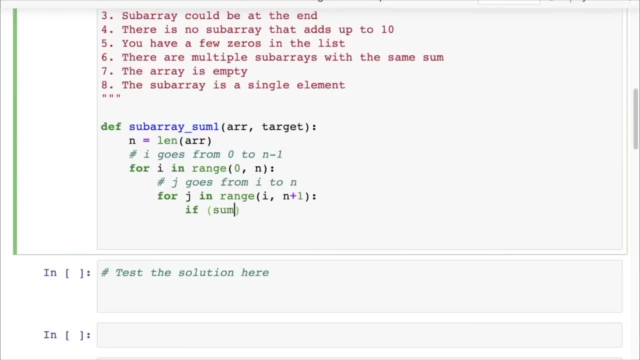 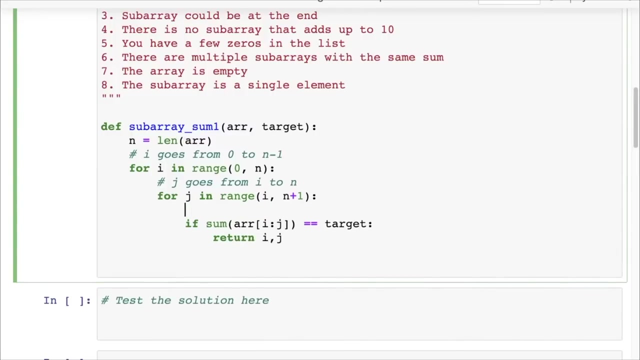 And now we simply check if the sum of array I to J- and then we've seen this array I to J is going to give us all the indices. So it's starting at I but ending just before G. So if the sum of array I to J equals target, then we found the answer: return I comma G. that's it. 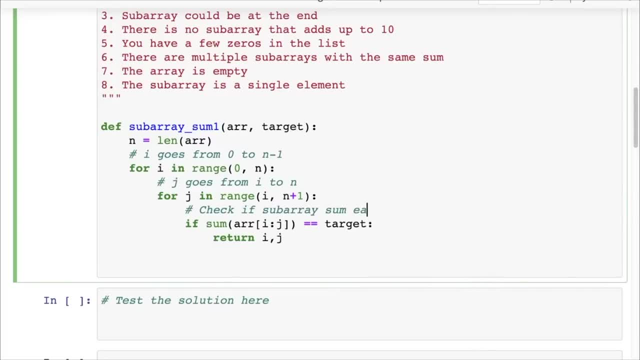 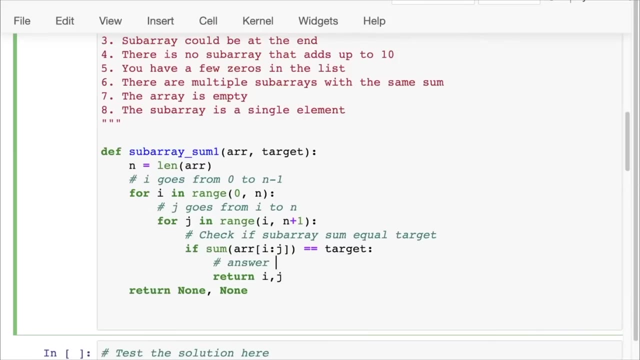 So check if subarray sum equals target, and if not, let's just return none, none. maybe this is what we agreed, but let's return none, none, And That's it. So that's your, that's your code. 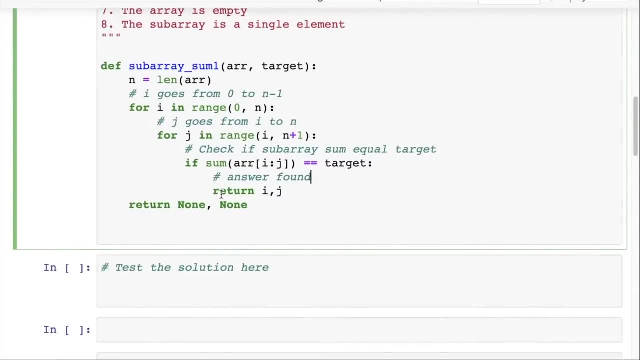 It's about one, two, three, four, five lines of code, maybe six, but that's a brute force solution. If it's really short it doesn't hurt to write it, because then it's going to sit there And at least as a reference you have it. but it's something you can discuss with the interviewer. 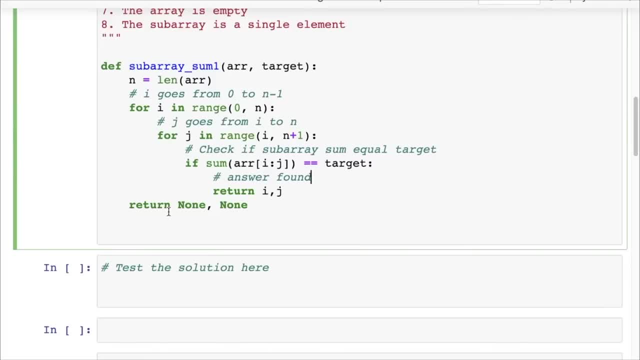 Should I? I mean if you, if you are clear about the brute force solution and you can tell its complexity, then you don't have to write. One other tip is: whenever you're coding, it's always helpful to simply add a small comment above so that, even if the interviewer is not able to follow your code, they can just follow your comments and they can tell if your general strategy is correct. right? 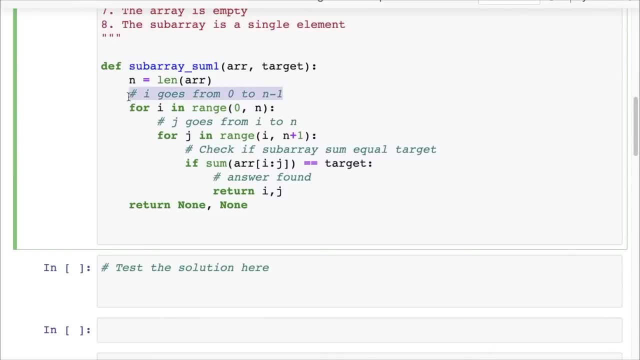 Once again, reading code is hard And especially when you are not familiar with the coding best practices in the industry, the code that you write is Sometimes difficult to read. So while you learn how to write good code, in the meantime it always helps to just mention: comment: makes it makes their job easier. makes them easier. makes it easier for them to evaluate you. 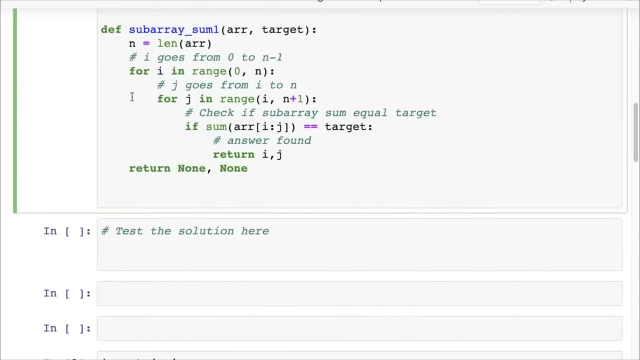 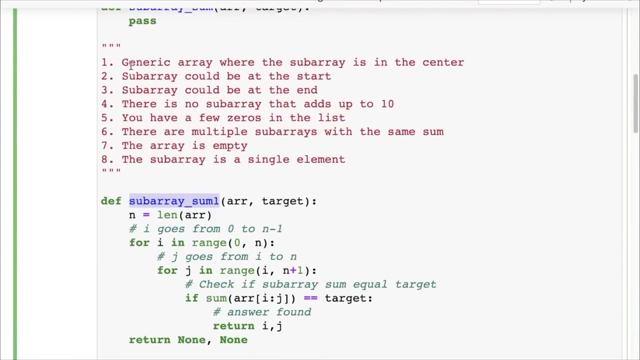 Otherwise, you may spend five to 10 minutes talking about something in your code which either they misunderstood or you made a typo, et cetera. Okay, So we have here the somebody, someone we've implemented the brute force solution. Maybe let's also check out some cases in. 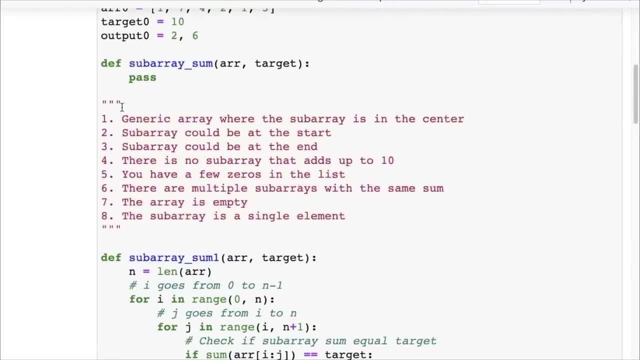 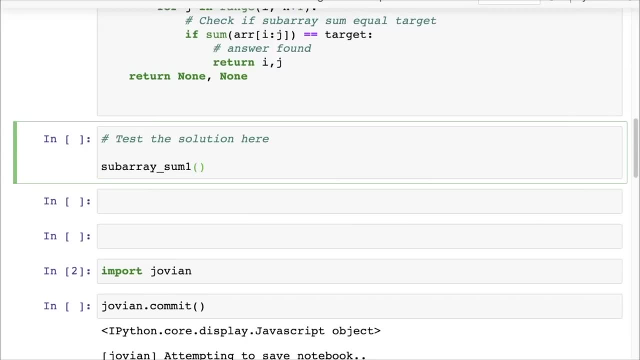 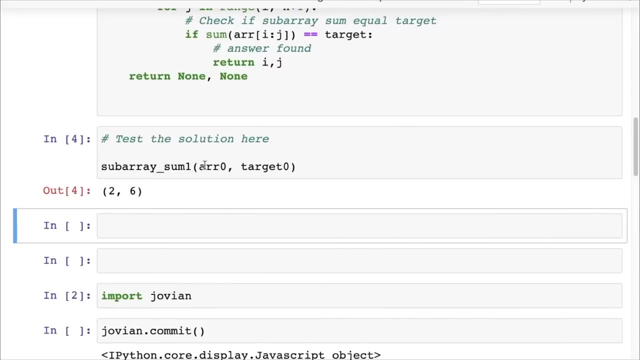 And see if this brute force solution works correctly. So in an interview, if you have the ability to run the code, you can just run a few samples. So let's say I simply take at a zero and target zero and you get the value to six. and remember output zero also has the value to six. 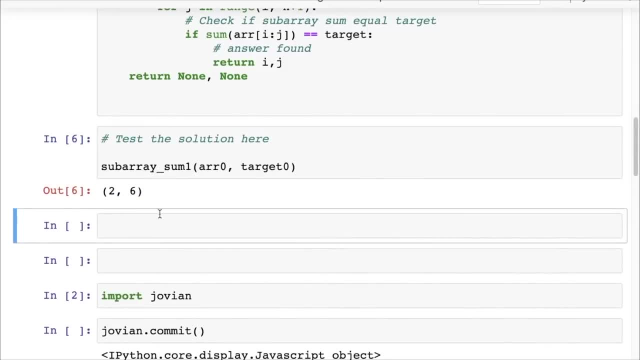 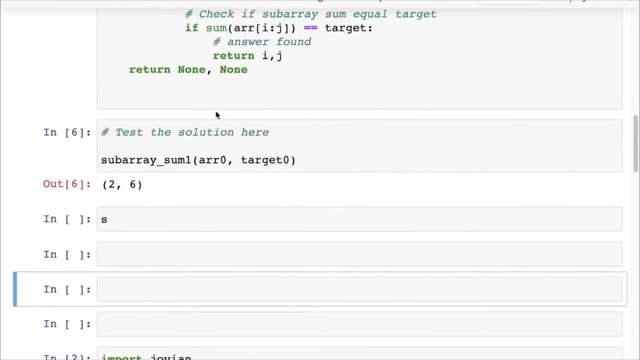 So it seems like our, our technique book. Let's test a few more cases just to be sure. So bury at the end, so where at the start? let's see if we can fix that. So here is at a zero. 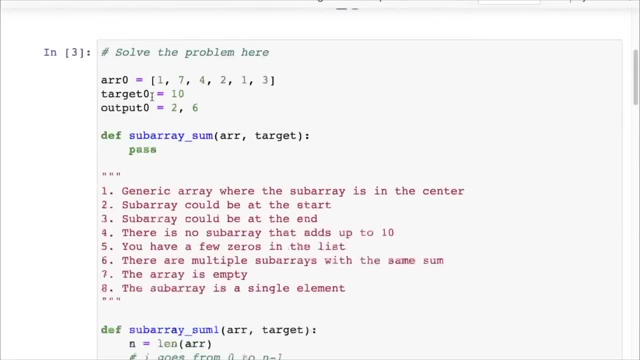 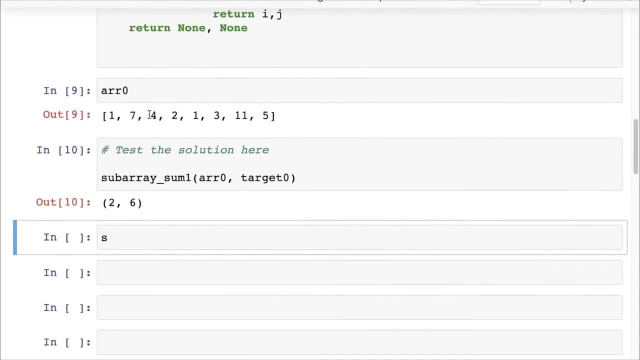 Now, if I take this, I remember four to one, three. oops, I think I didn't complete it. Let me also put in 11 comma, five here. Yeah, So remember four to one, three is the solution Now, if we simply take four to one, three, 11,, five and call sub array sum. 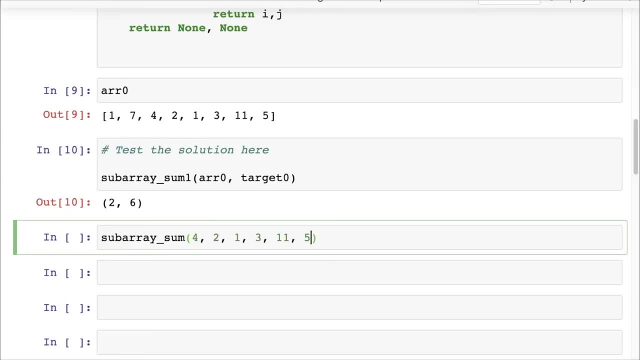 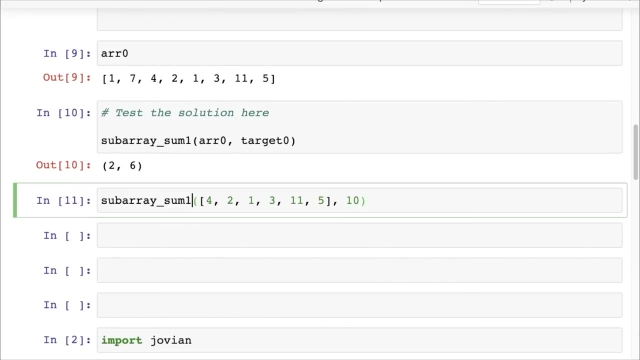 And put in this number here and put in once again: the target zero was 10, or they should be somewhere, some one, Okay, Yeah, So now you can see: four to one, three is zero. one, two, three, which is the range zero to four. 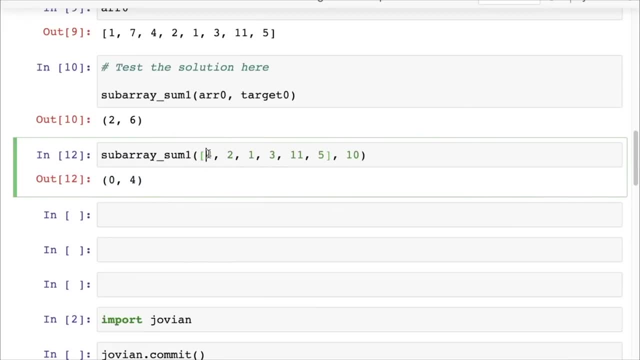 So it seems to have worked correctly. Let's do the same thing Now. let's this time. let's put this at the end: So one, seven, four, two, one, three, 11,, five. This works fine too. 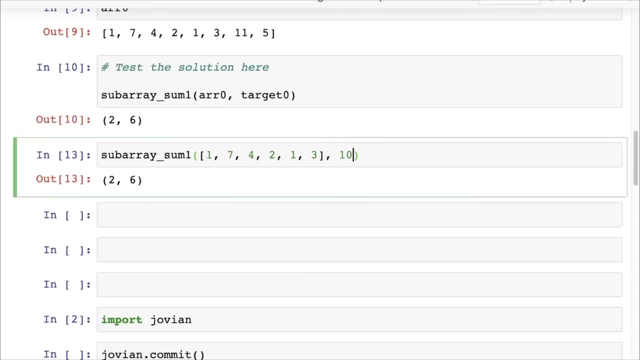 Two, six. Let's try another one, Let's try maybe 17, and that probably cannot be formed. Oh, it can. one, two. Let's see one, zero, one, two, three, four, five, probably the sum of all of these four. 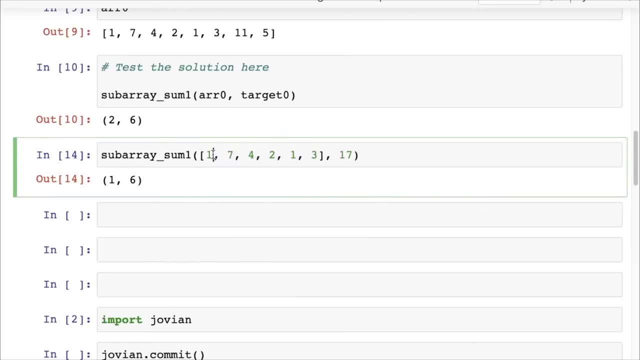 Let's do six plus four, 10.. Okay, Now, maybe there's a problem here, because it seems like 17 is not the right sum. So you have one plus seven, eight and eight plus four, 12.. 12 plus two, 14,, 14 plus four, 18.. 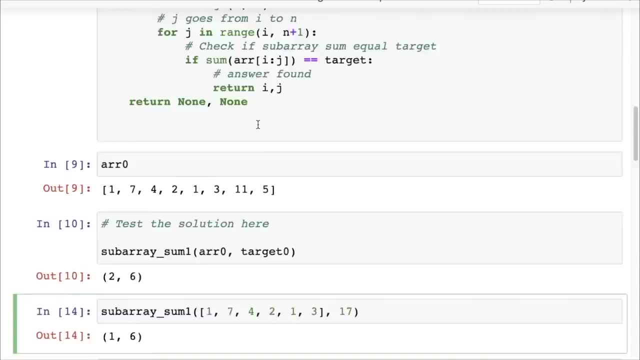 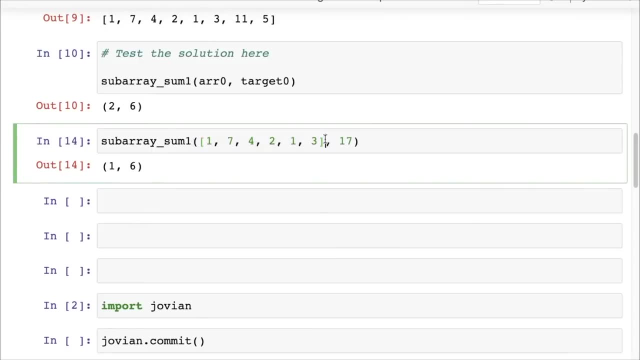 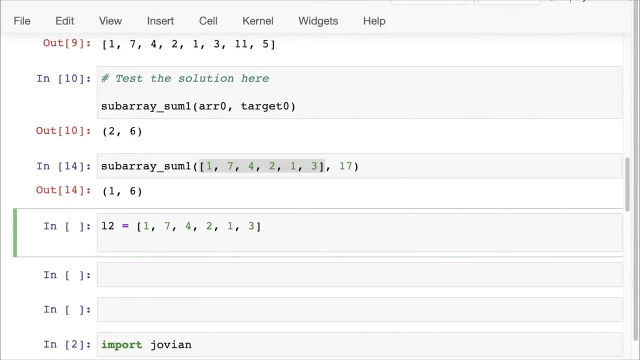 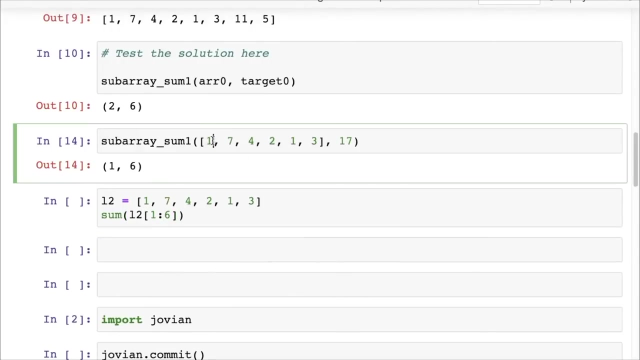 Okay, So this seems like a mistake, then, and we can even check this out. So we have L one, that's that. let's call that L two. L two, Oh, it says one to six. I think I misread it. So we are ignoring. 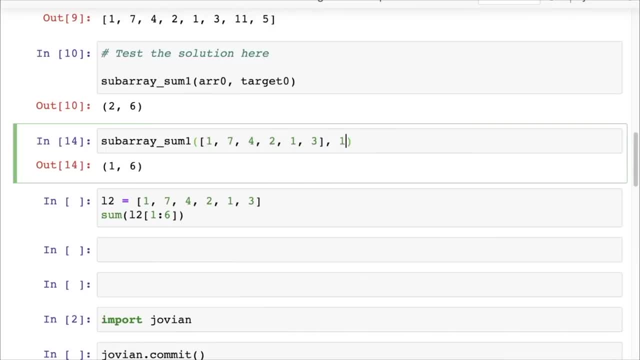 The zeroth element. So this does add up to 17.. Okay, So 17 does show up. Let's try 18,, which takes up the entire area, works fine. Let's try maybe four, which should just take the single number. 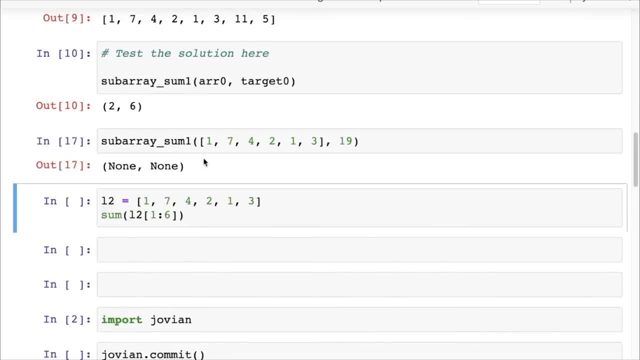 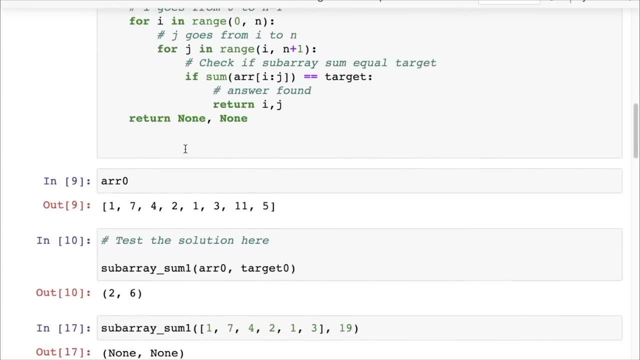 So that works fine too. Let's try 19.. That should be none, None, Okay. We've tested this extensively and overall, our solution seems correct. This is the process: Whenever you write any code, you should also test it out. and it also gives more. 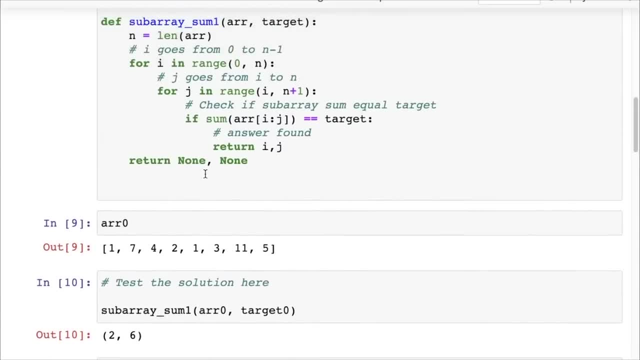 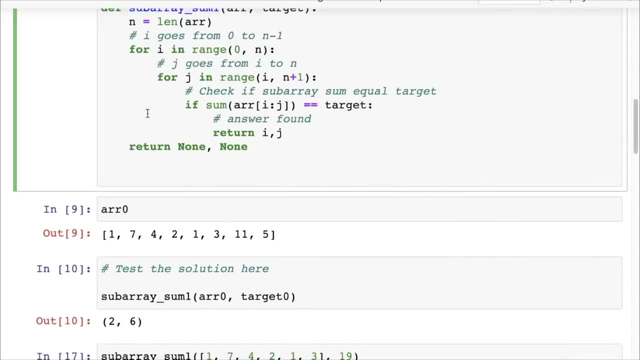 confidence to the Interviewer. but if you do not have the option to test it out, if you do, if you're not able to run the code right now, then simply walk them through an example yourself, like look at this example and then walk them through the example. 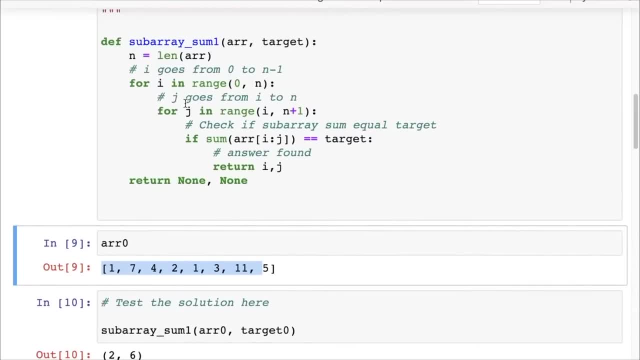 Okay, So now we have the brute force solution. The next step is to analyze the brute force solution. Now let's analyze it. So you have here one for loop, and we know that counting for loops helps us count the number of operations. 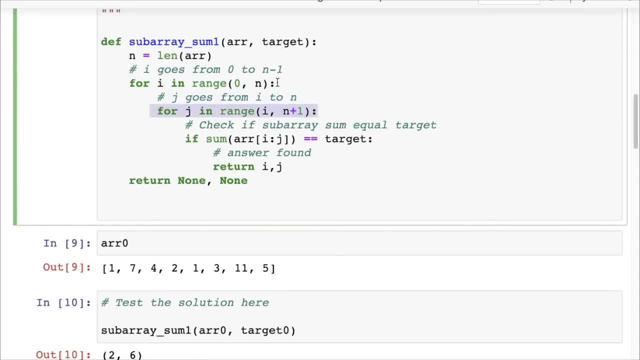 Then we have another for loop, So one for loop can go from zero to N, So this may run N times. Then we have another for loop which goes from I to N plus one. Let's approximate here and say that it can run at most N minus one times or N times. 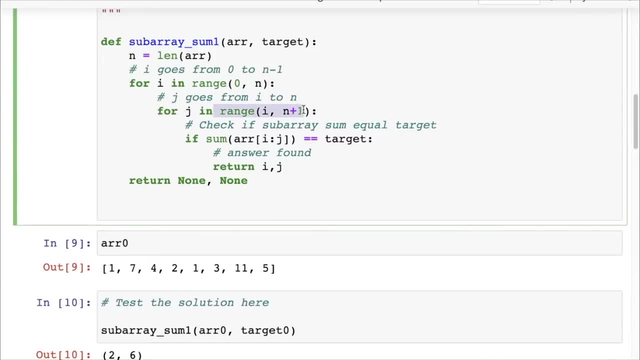 So N, and inside each of these up at most N, And then inside the second for loop you have the sum. So this is very important. Now always carefully observe the operation inside your for loop. So you have a sum which can be on an area of I to J. 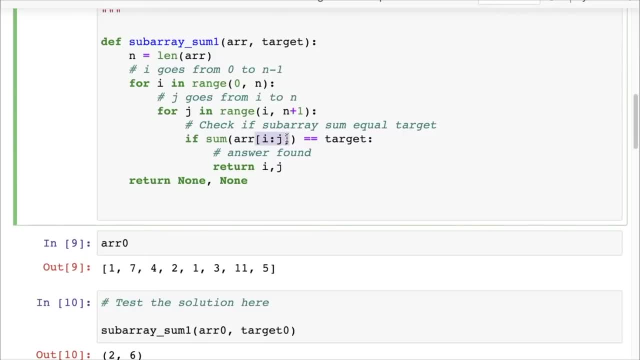 Now remember, I can be zero and J can have the value N. That means in the, the largest area that you can work with will have approximately the size N as well. right, So you have N and inside each of those you do N other loops, and inside each loop 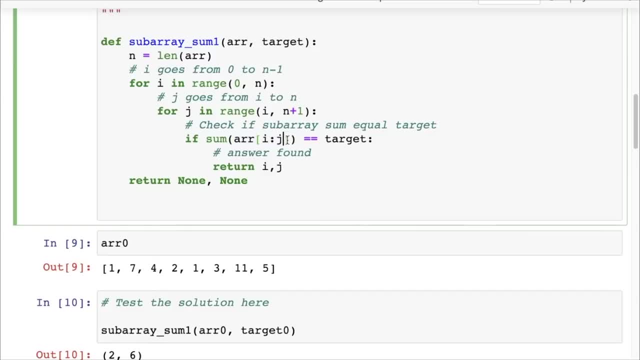 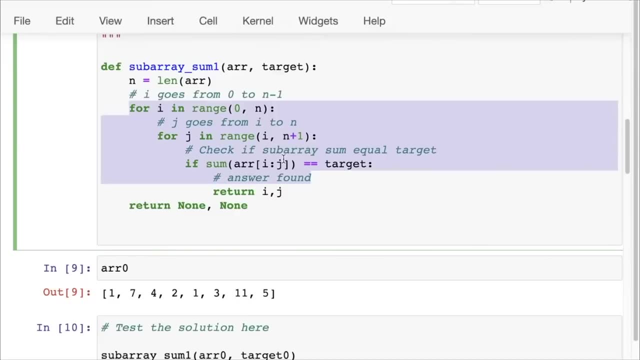 you do work, you do N additions, right At most, N additions. So that roughly gives you that this is going to be N times N times N. So this is going to be an order N cube solution. Okay, So, if you are able to arrive at the order N cube solution, 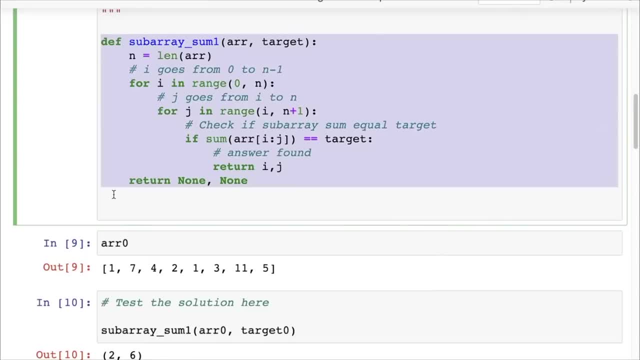 Okay At the order N cube complexity without implementing the solution. great, You have learned it. but if you're not able to arrive um at the order N cube, the order N cube complexity for the brute force solution, then you probably need a little more practice, because this should become second nature. 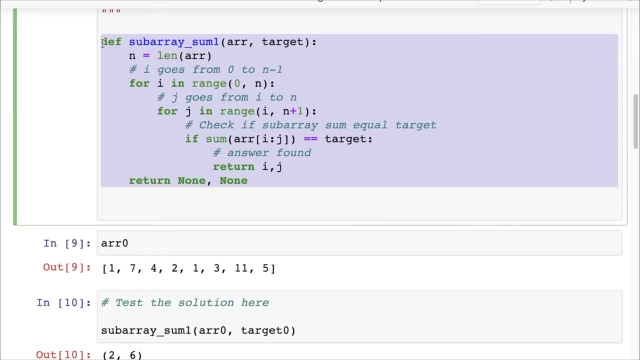 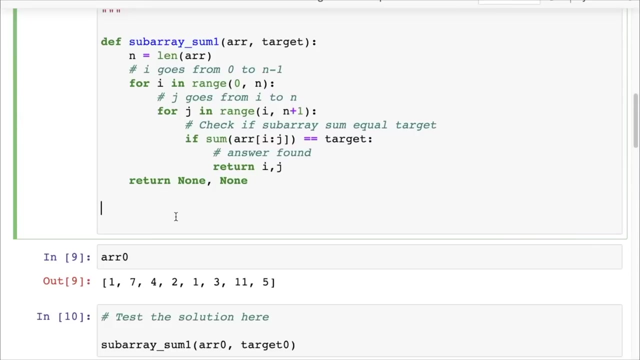 to you, just looking at a problem, identifying the simplest solution and then finding the complexity of the simplest solution. Okay, All right. So now we have implemented it, tested it and we've identified the complexity. Remember the next step: find the inefficiency and overcome that. 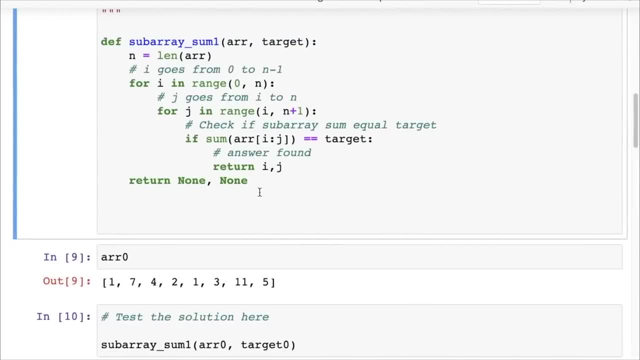 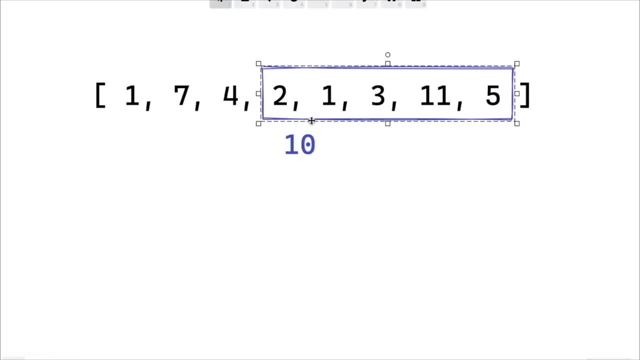 inefficiency by applying the right technique. So let's find the inefficiency. then Here we have, let's say we are at this position. So let's say you are looking at seven, four, two. Let's say I has the value one. 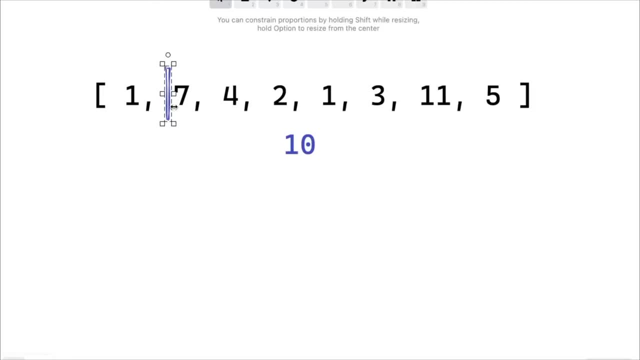 So you start out with I equal to one and J equal to one in the inner loop. Then what we do is we increment J by one and then we calculate the sum, and the sum is seven. Then what we do is we increment J by one more and we calculate this loop and the 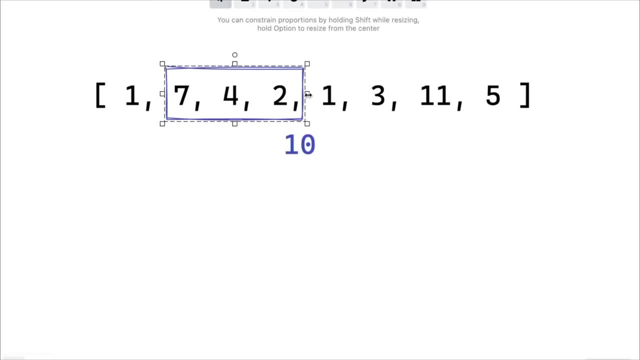 sum, and the sum is seven plus four 11.. Then we increment this window once again and then we calculate the sum, and that is seven plus four plus two. So seven plus four 11 plus two. And then we move this, and then we check it again. but we're doing this over and over and over many, many times, right? 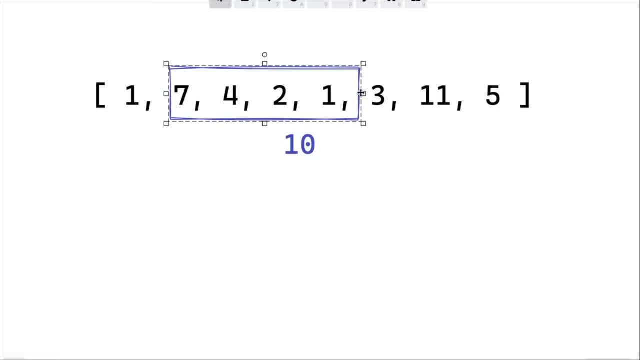 Each time we are doing seven plus four plus two plus one and seven plus four, four plus two plus one plus three. That seems like a lot of additional work. Maybe we can just avoid that. What we can do is we can, when we start out with a J, we can keep a running sum and each time, simply before incrementing J, 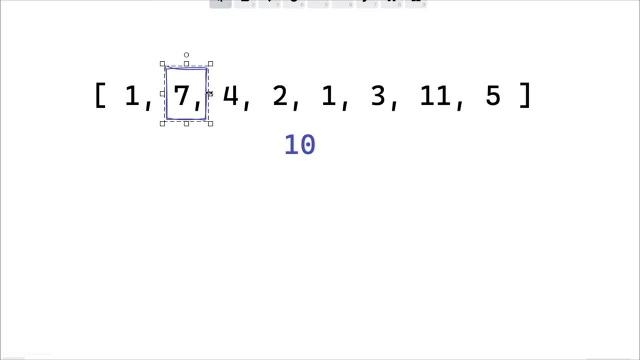 add this upcoming element, which is the J element, into that running Some right, And that way we don't have to do that entire sum inside each of the inner loops. So that's one optimization and this is how you should explain it. 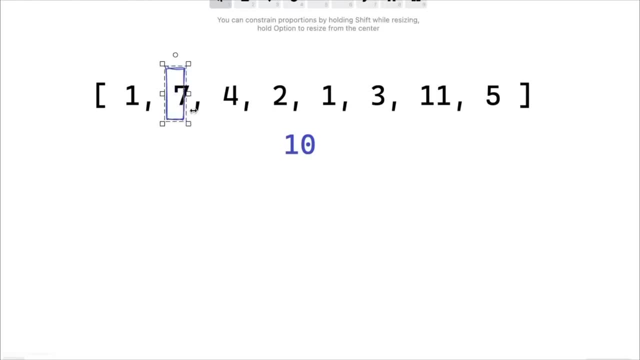 That's one optimization that I have come up with. The second optimization that we can come up with is that the moment the sum, the running sum that we're calculating, the moment the sum becomes greater than the target value, We can skip all of these right. 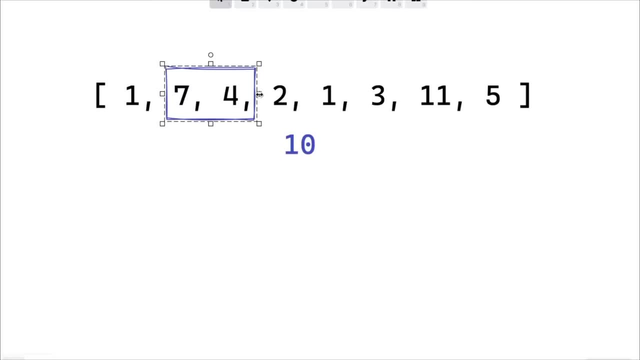 So we know that seven plus four is greater than 10, and we know that the area only contains Non-negative number. So what that means is seven plus four plus any of these numbers is always going to be greater than 10.. And you can- obviously you can- see this. the number is not going to decrease if we keep adding positive numbers. 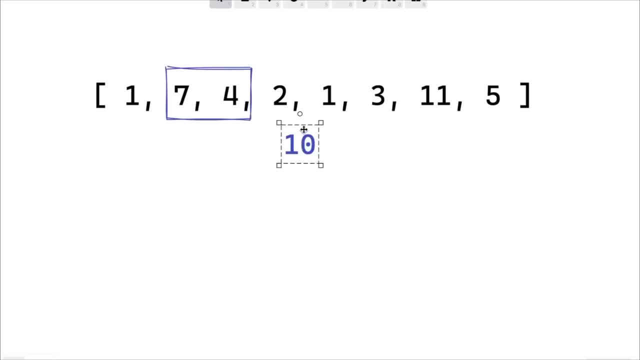 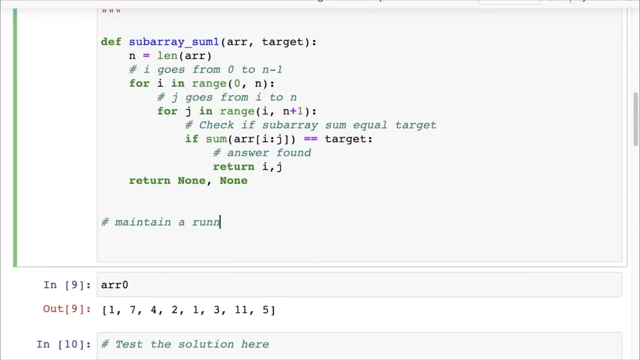 And so as soon as the running sum crosses this value, we can break out of the inner loop. We do not need to continue and look for higher values of G. two optimizations, Ed's. to just write them down: Maintain a running sum so that you don't forget it. 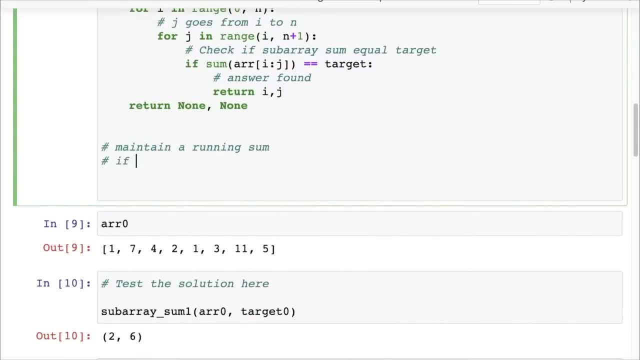 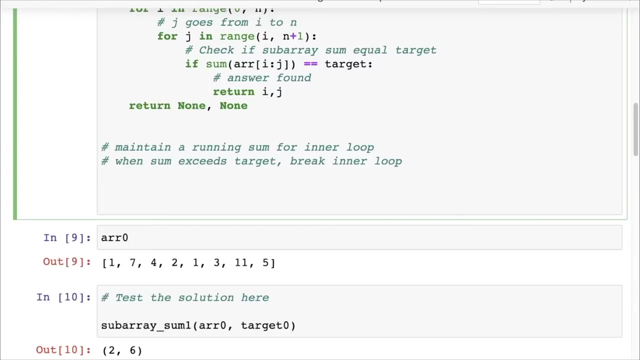 And find the end. Second optimization is when some exceeds target break in a loop. Okay, So now we have applied an optimization simply by just looking at the data And a lot of cases it's very straightforward. You don't even have to. 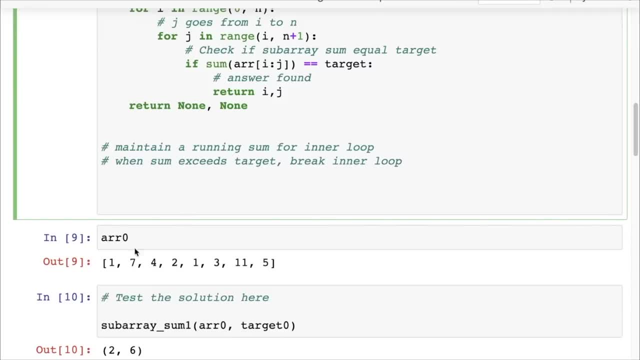 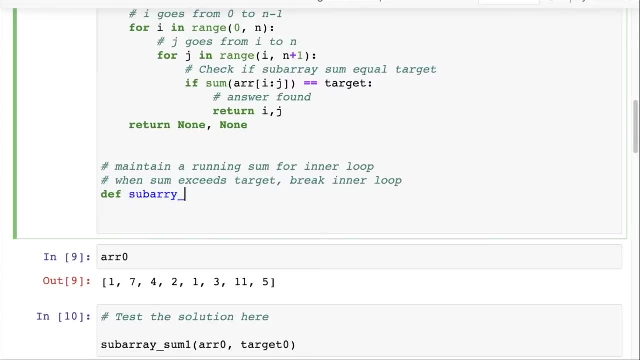 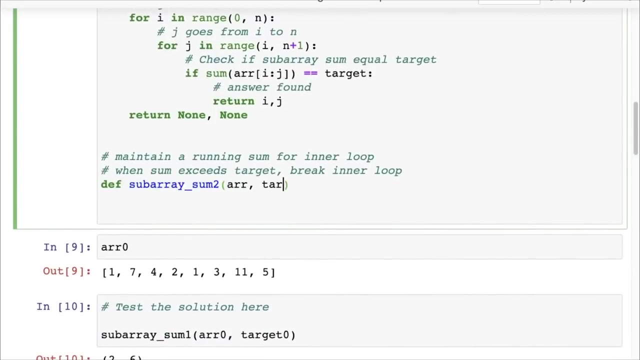 Apply any special technique, And in this case we found these couple of optimizations, So let's apply them. So what we'll do is we'll define def, sub array, some two, And here, once again, we have the area and we have the target, and this time we get the length of the area. 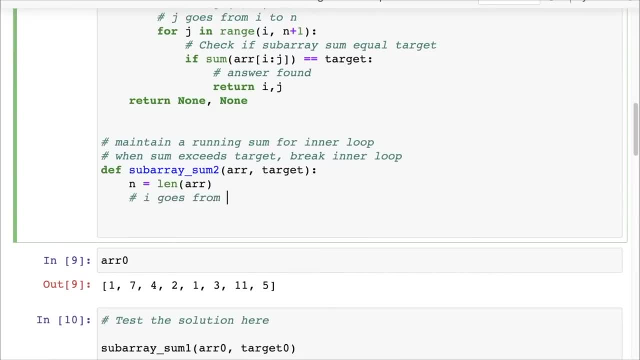 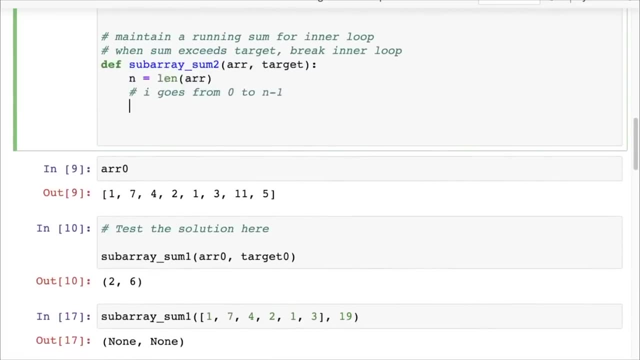 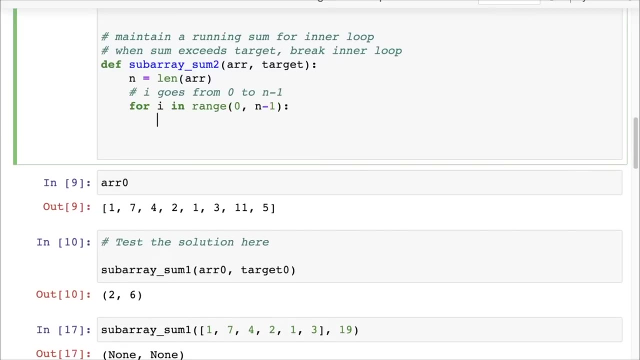 And now, once again, I goes from the same value, So I goes from zero To N minus one. nothing changes here, for I in range zero to N minus one. Now here is where we want to start a running sum. So S equals zero. 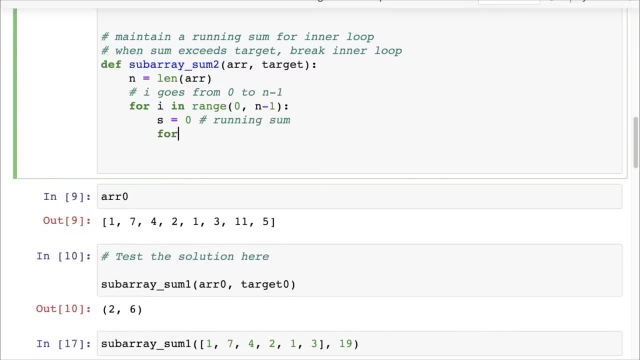 This is our running sum. Then for J in range. remember we start out with I and we'll go all the way this. I keep making these mistakes all the time And, by the way, these are called off by one: errors here. 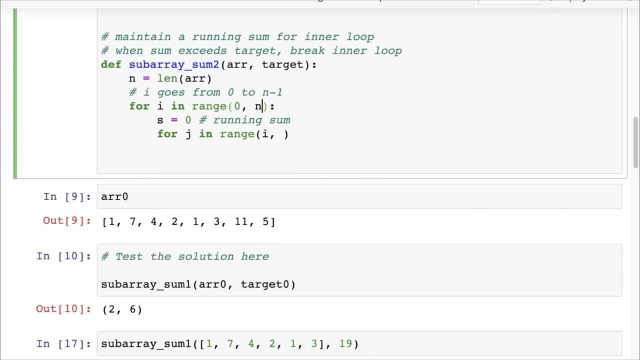 What we did was I wanted to go to at the address N minus one, but because ranges do not include the final value, I put in what I put in- N minus one was wrong. I should be putting in N, and I make these mistakes all the time, even after many years of coding. 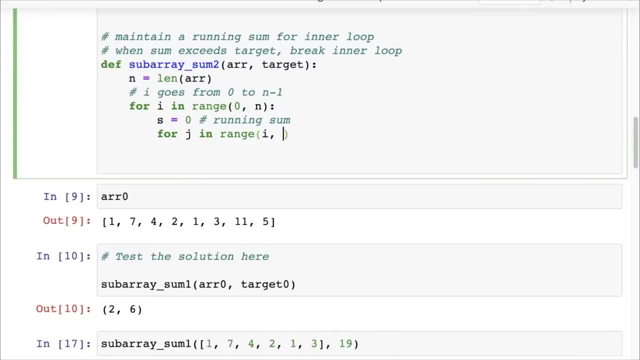 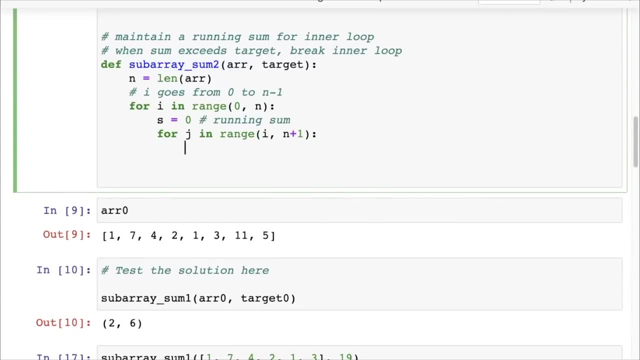 So always watch out for off by one errors. Anyway. so J can, J can take the range of zero of I to N. So here we should put in N plus one. And now, first we want to check if the running sum is equal to the target right. 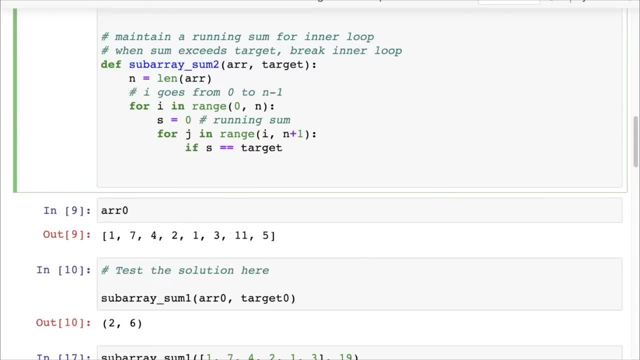 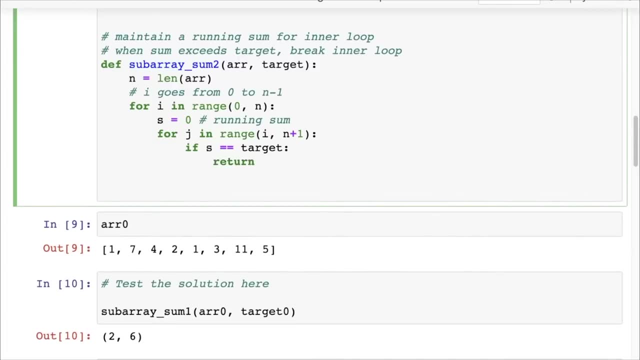 So so assume that we've been calculating the running some step-by-step and we'll write an N at this current point, The sum has become equal to target. If the sum has become equal to target, then we simply return I comma J, because this sum includes the sum from index I all the way up to just before J. 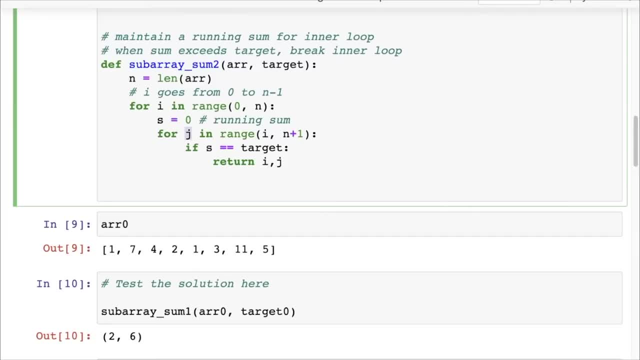 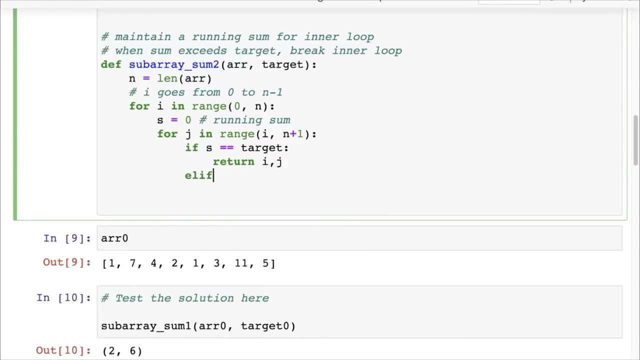 So initially the J also has the value I, so the sum is zero, which makes sense. But if that is not the case, we check if it is greater than the target. So is it possible that our sum has already exceeded the target? 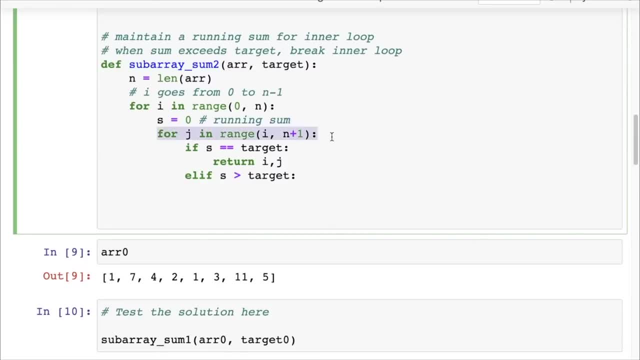 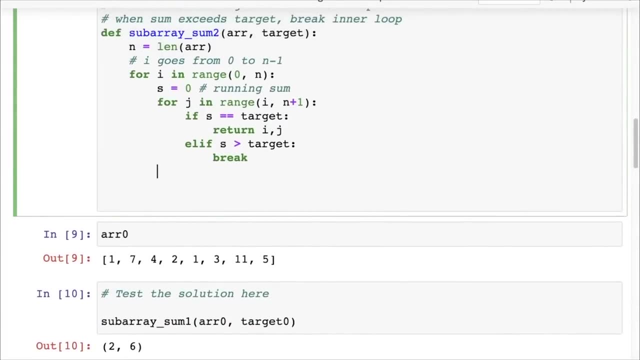 In that case, we don't need to continue this inner loop. We can break out of this inner loop, And the way to do that is by simply typing break. And then, if neither of these held true, Okay, If neither of these was true, so, which is that the sum was not equal to the target and it was not greater. 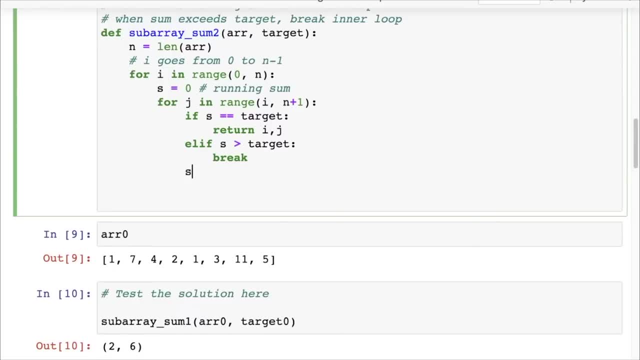 That means it is still less than the target. So that means we need to then add area of J into the sum So we can say some plus equal to some plus equals area of J, which is the same as some equal to some plus area of J. in any case, area of some plus equal to area of J. 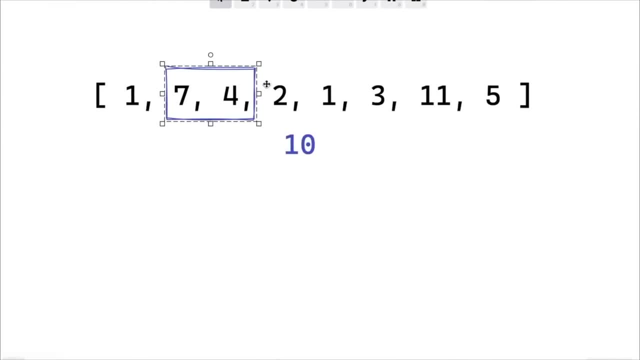 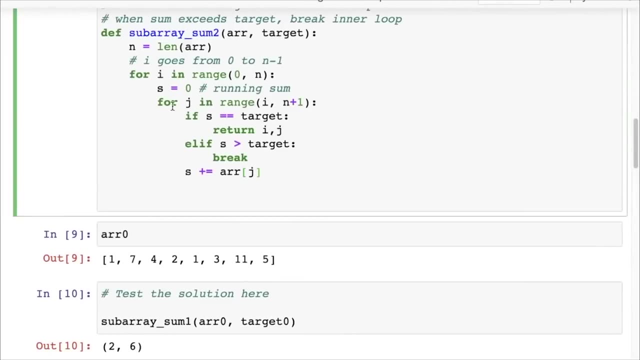 So we have added the J element. I remember, If this is the pointer J, we added the J element and then we we will set J to J plus one. That will happen automatically when we come into the next iteration and the next iteration we'll once again check if the sum is equal to the target. 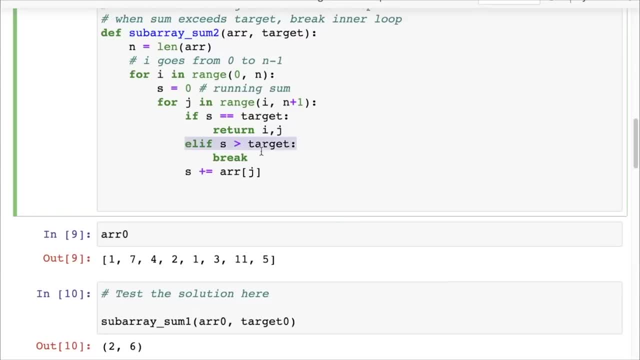 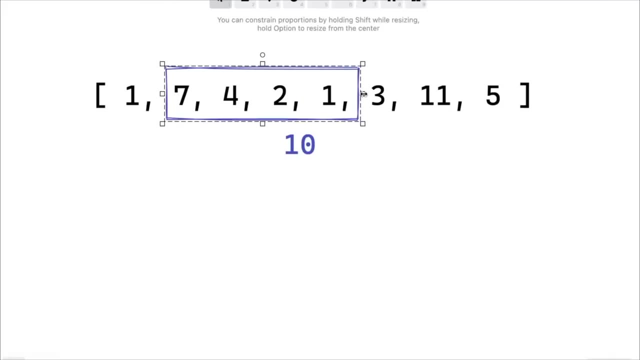 If it is equal, we return I comma J. Otherwise we check if it is greater than the target. If it is so, we break. if it is still less, we increment, we move J once again. So we add one, and then we move J once again, and then we check again, right? 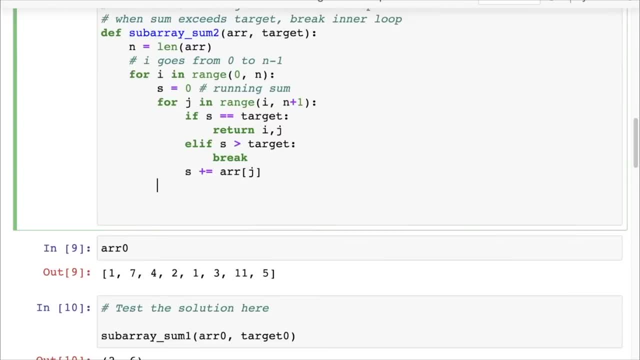 So that's our running sum. Looks good. Now, once again, if we were, if it was found, it would have been returned somewhere here, since it seems like it was probably not found. So if we come to the very end, so here we return: none, none. 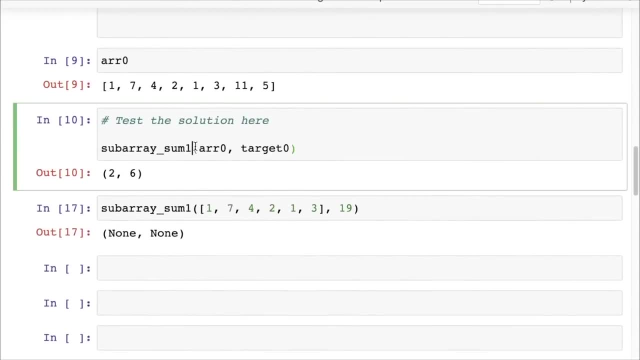 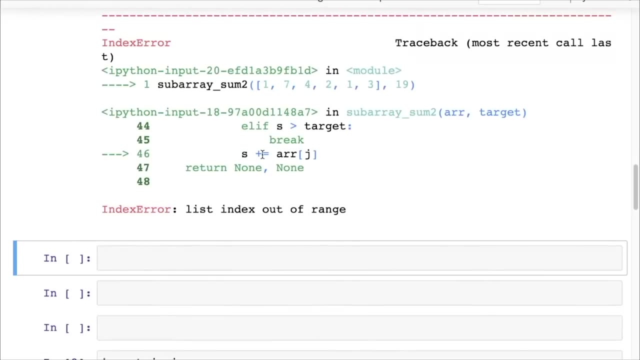 Okay, And once again, let's test it out. So let's try some, very, some two. it gives you two, six, some two of none. Okay, Seems like there is an issue here. Yes, So this is why you need. 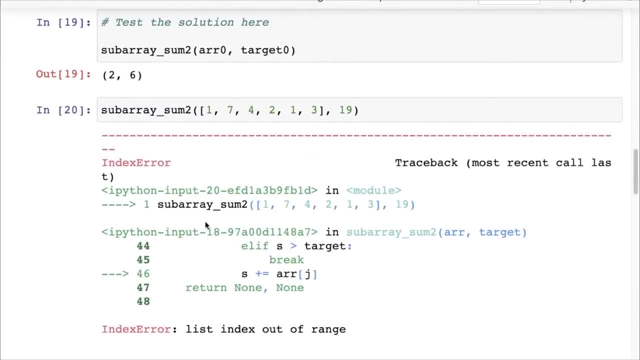 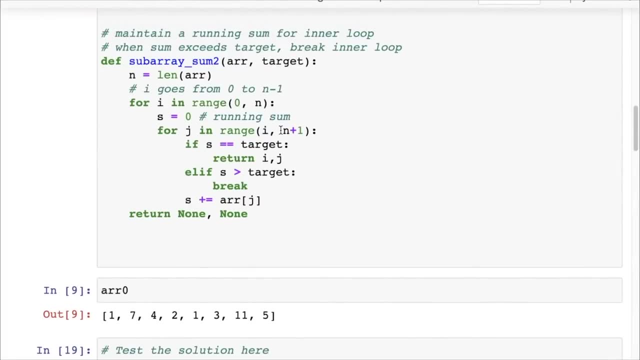 Test cases. So it seems that LHA took up an invalid value. So why is that? Oh well, that was because Jay can go to the point of N, So the maximum value Jay can take is N, So which means that you have already arrived at this position. 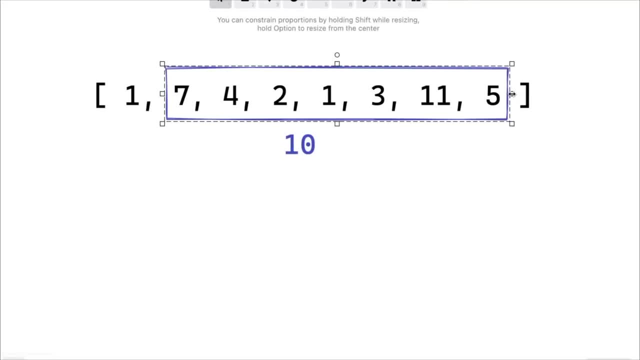 So now you can no longer increase the sum further, right? So if you arrived at this position but you've still not reached the total Of N, then that means you may need to increase it further, but you can't increase further. 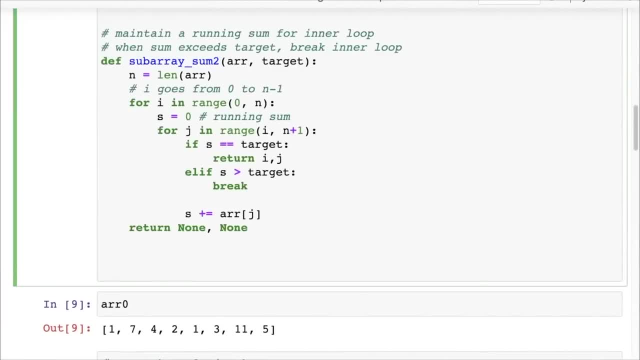 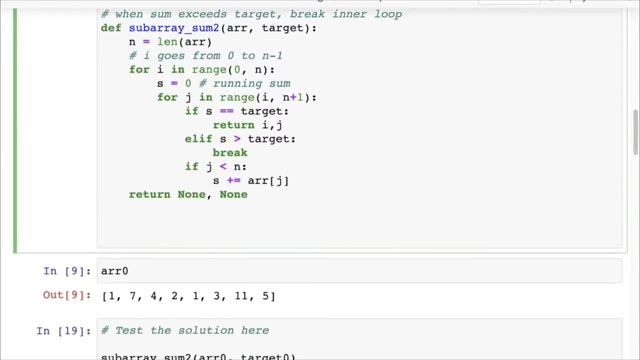 So there's no number here to add. So what we should do is we should add a check If Jay less than N, it's since Jay can go all the way up to N and that's it. So we had a small bug and we fixed it. 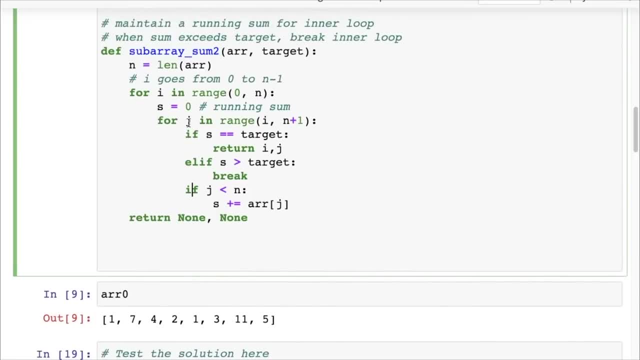 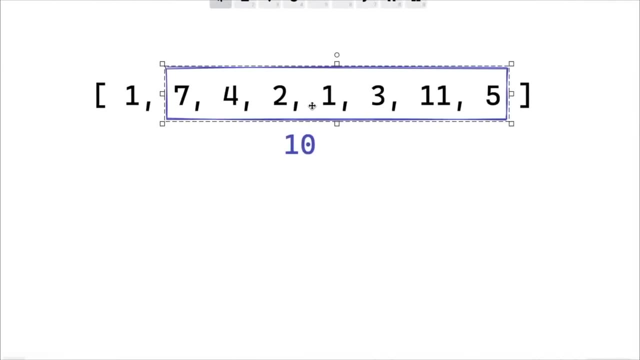 Now, again, this is something that you should work out for yourself on pen and paper. So, even while doing the optimization, you can ask For a couple of minutes. play around with it on pen and paper, write a few examples, relax. 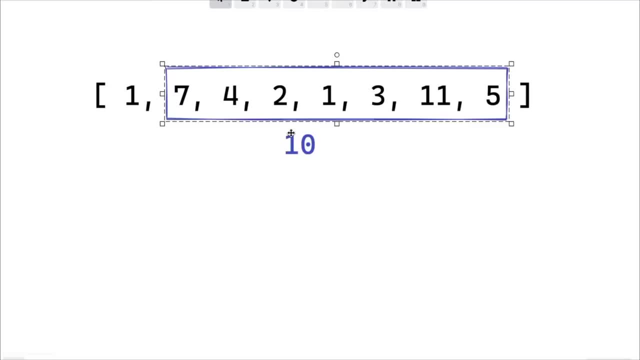 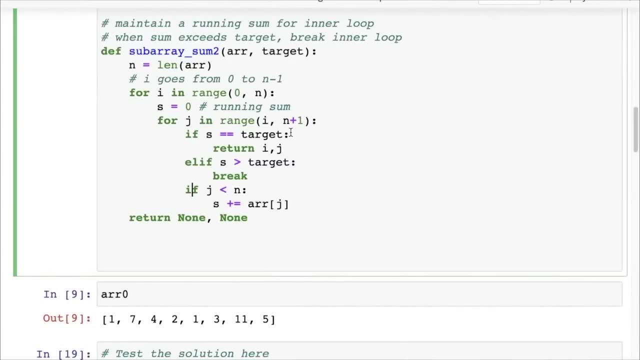 You can even take up to four or five minutes And if you if you're not getting any ideas, you can simply talk to the interviewer. You can speak out loud, explain your thought process And in a lot of cases they will give you a hint because they want to see you succeeding. 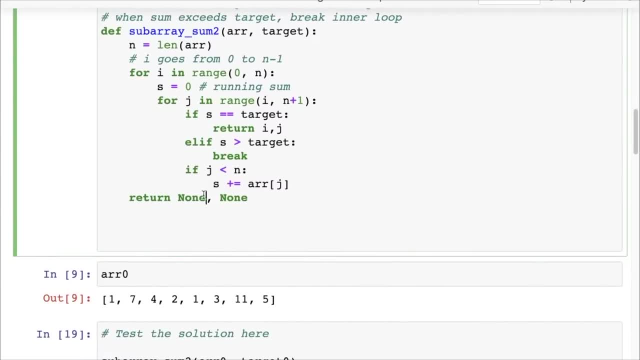 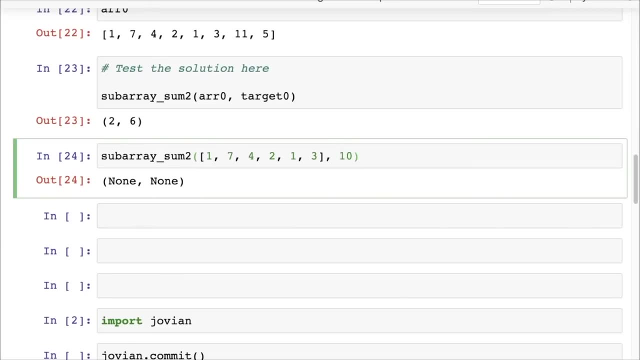 Okay. So now this is the second implementation. Let's see. Okay, This time it worked. Okay, None, none or two, one, three. Let's put in 10 here. They should give you the value of two comma six. 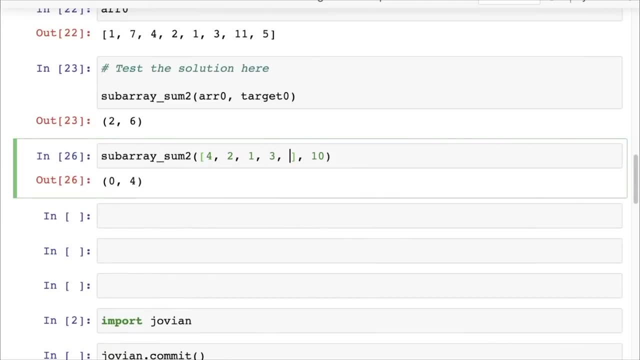 Let's put in this: So that's zero comma three. Let's test this out too. So that's zero comma four. Yeah, zero comma four. So it seems like it's working just fine. Yeah, So it seems like this is working pretty well. 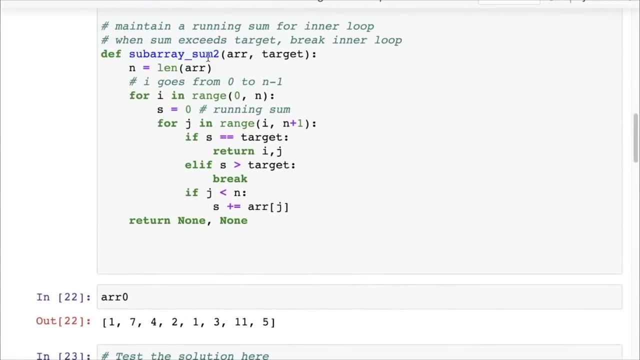 So now we have the second Optimize solution. So let's look at the optimized solution and analyze it. So we have one loop and then we have a second loop. These two are the same, but inside the second loop we are simply doing a constant operation. 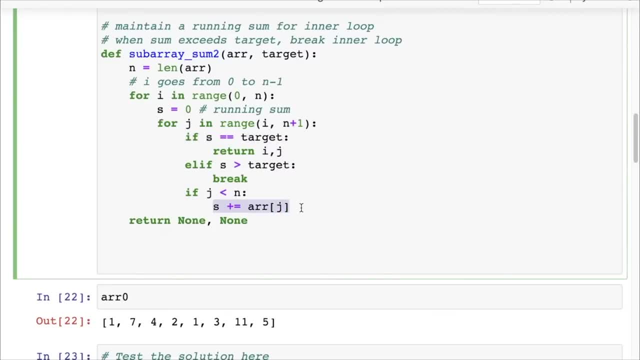 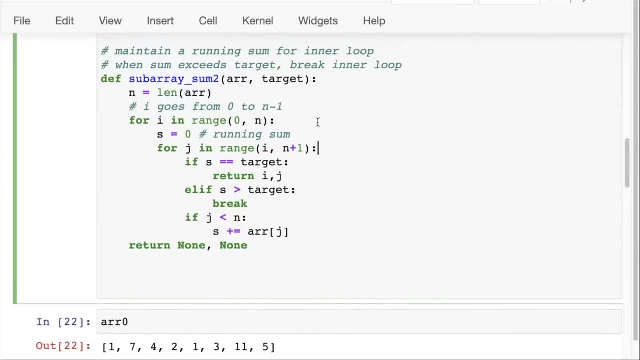 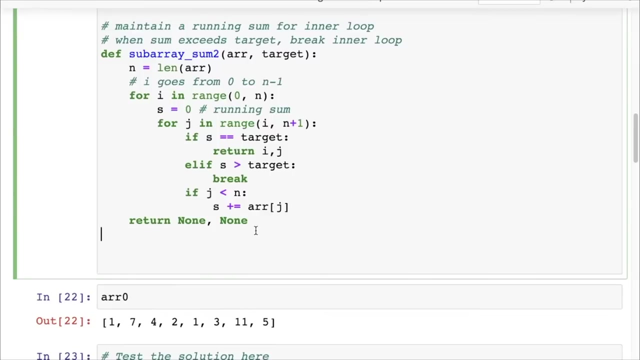 We are just doing some comparisons and one addition, not up to N additions. So the complexity goes from order of N cube to order of N square by maintaining a running sum. Great, Now this. at this point, when you've described the solution to the interviewer and maybe also coded it, you might ask them: is this good enough? 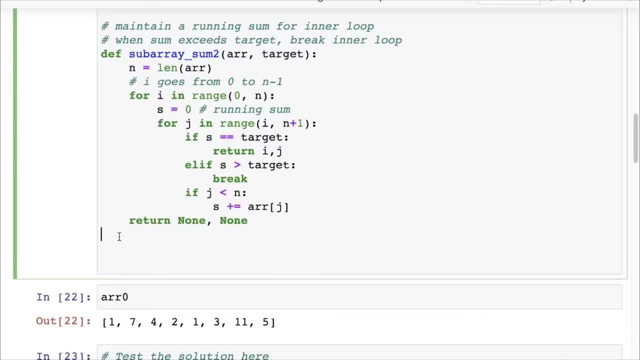 And they can see that you've you've thought about it, You find the solution and you've tested it and it tests well. And at this point they may just say, yeah, I'm happy with the solution, This is good enough. 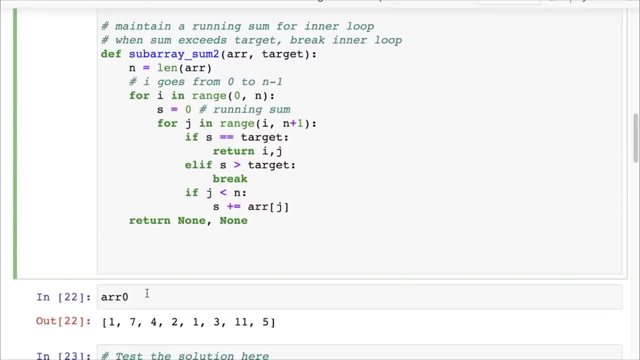 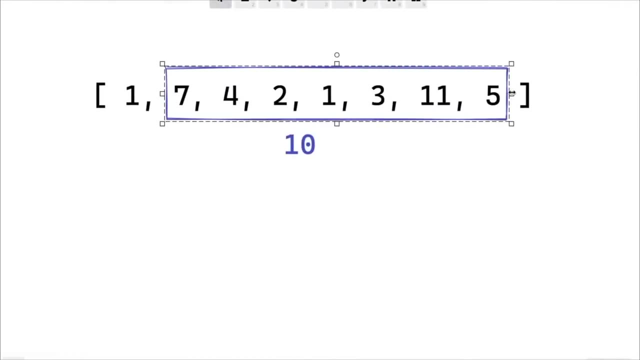 Or they may say: can you do better? And when they say can you do better, Most of the time it suggests that there is a better solution. So let's see, let's think about it a little more and let's see if there is a better solution. 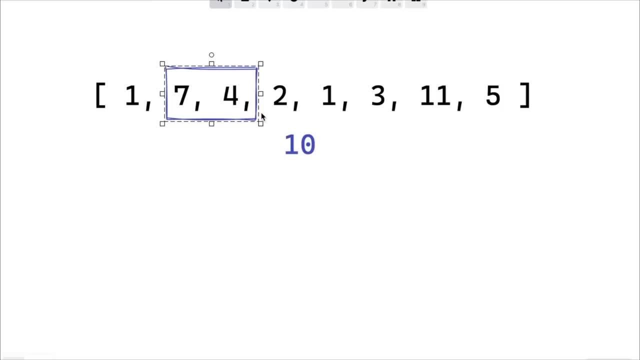 Now to can, to can you do better? We apply the exact same technique. We have analyzed the complexity and now we need to look for inefficiency. Okay, Now we have removed the inefficiency on this side, which is as we move J. 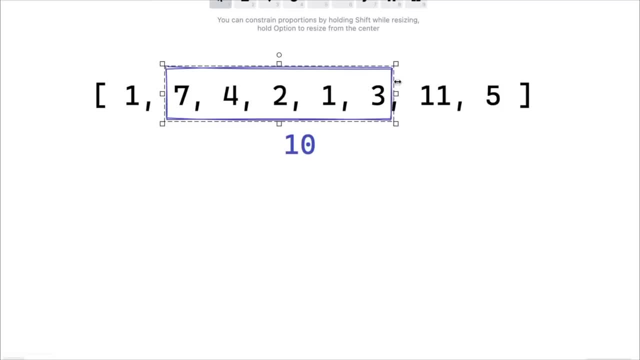 That is when we reuse the previous sum to compute the next sum. So we've removed the inefficiency on this side And we've also added this, also added this condition, so that J only goes up to a certain point. Now, of course, in the worst case, 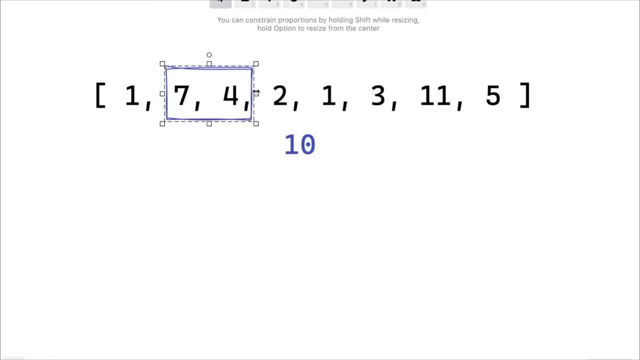 J may always go up all the way to the end, but at least in a lot of cases J will not X, J will not not go beyond a point where the sum becomes larger than the target. So these are good optimizations, but what about I? what about the left window? 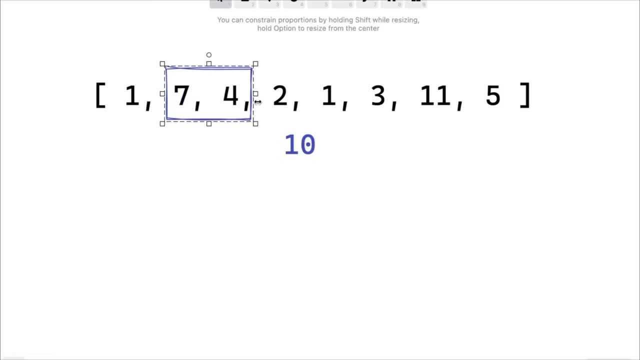 Now look at this year Now, when you have seven, four or let's start out all the way at one. So we have one. that's so. first we started with the empty, empty sub array that has the sum zero, Then we increment. 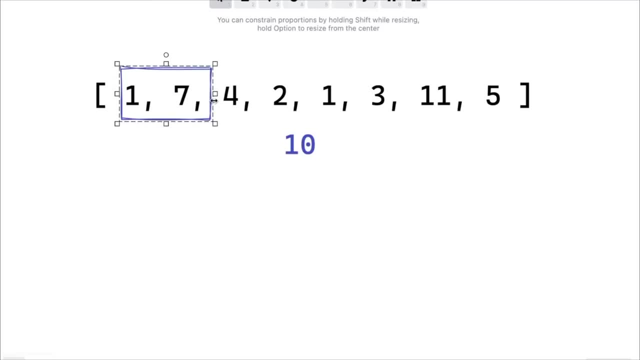 So now the sum becomes one, Then we increment J, Now the sum becomes eight, Then we increment J once again, and now the sum becomes 12.. Okay, The sum has become 12.. Now that's a problem. So what do we do? 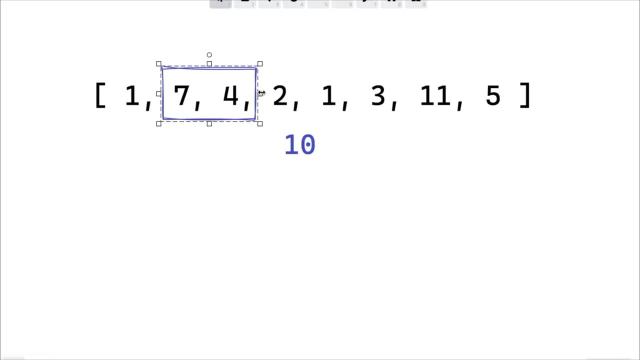 What we are saying is we will take I and set it to the next value, And then we'll bring J back to zero or back to the value I, so that we start with the empty sub array once again. So now, when we do seven and when we so that's, that's just has a value seven. 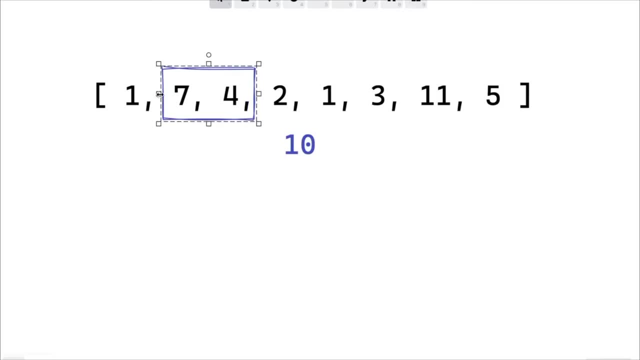 And when we do this, We have to add up seven plus four. Now, here's something that we could have done instead. Now, as soon as the value became larger than the target value, we could have simply moved this year. Does that make sense? 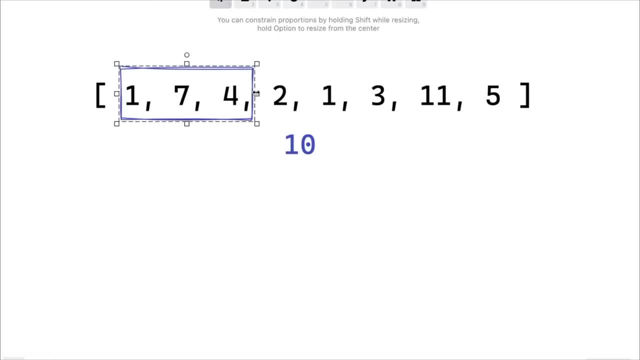 Let's think about it. So in this point this total was less than 10.. As soon as we added this number on the right, this total became more than 10.. Now we know that this total became more than 10.. That means that if we slide this window, if we slide the left window forward one step, then the total may become less than 10, right. 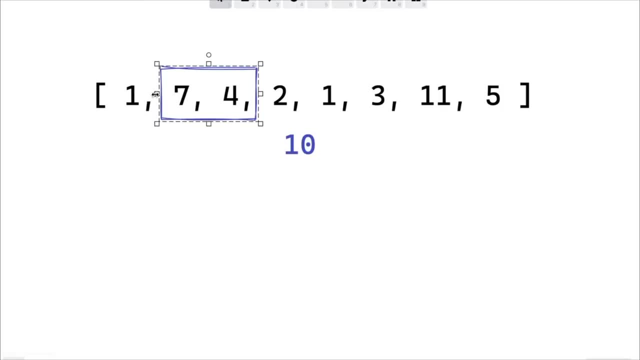 It may still became stay larger. in this case it stays larger or it may become less than 10.. So if the total now becomes less than 10, then we can once again move this, but the total has not become less than 10.. 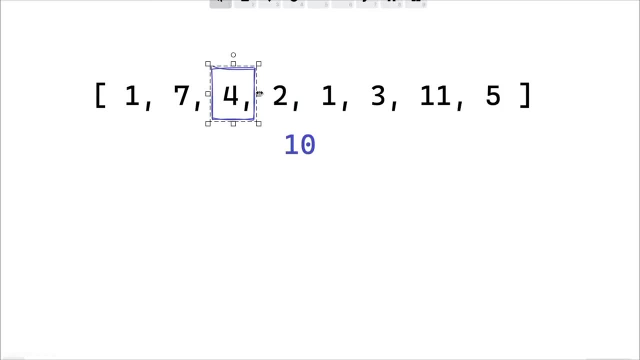 So we will move this instead. So now The total again is less than 10,. but we can once again move this, And now the total is still less than 10.. So we move this, or the total is still less than 10.. 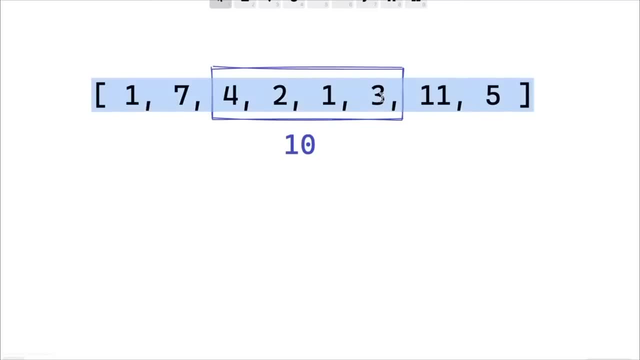 We move this and we encounter 10 here, but suppose we had not encountered 10.. Suppose this number was four instead, then what we would have to do is move this And now the now the number becomes less than 10.. So we always go, we always try to maintain a window of size less than 10, the moment the window becomes greater than 10.. 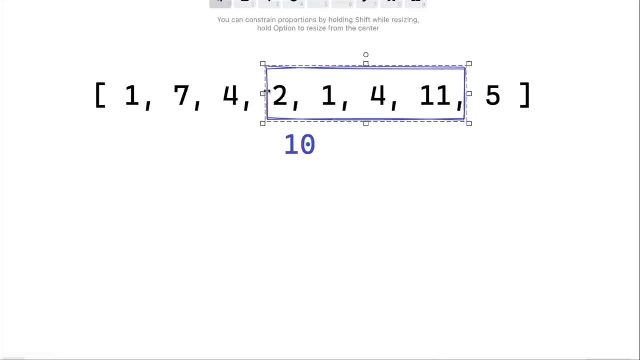 We keep trying to reduce its sites further to less than 10, right, Or exactly 10 as well. It's possible that the size may become exactly 10.. And then the problem is solved, but we keep trying to reduce its size to a value till it becomes less than 10.. 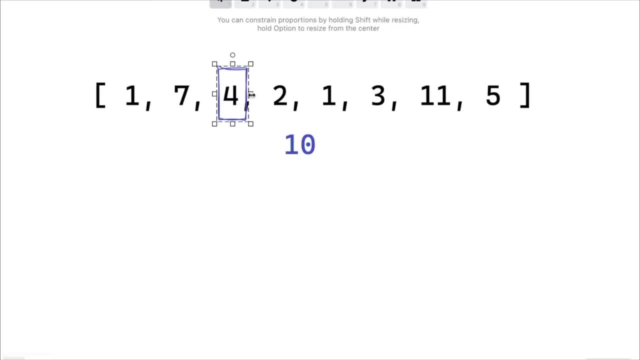 So, to revise the algorithm, we start out with both I and J at zero, Then we increment J while the running. now we have a single running loop and a single loop, essentially. So we increment J while The sum is less than 10.. 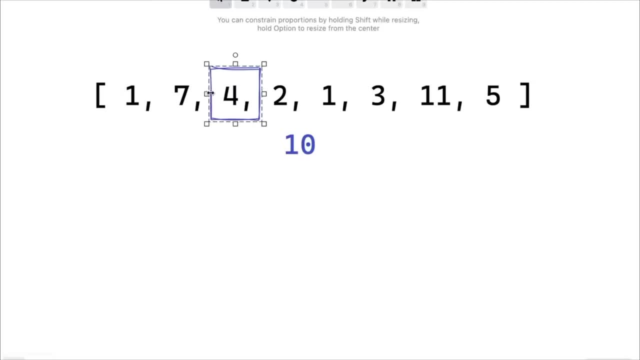 The moment it becomes greater than 10,, we start incrementing I. the moment the sum becomes less than 10 or less than target, we start incrementing J, And if we encounter the point where the sum equals 10,, we have found the answer. 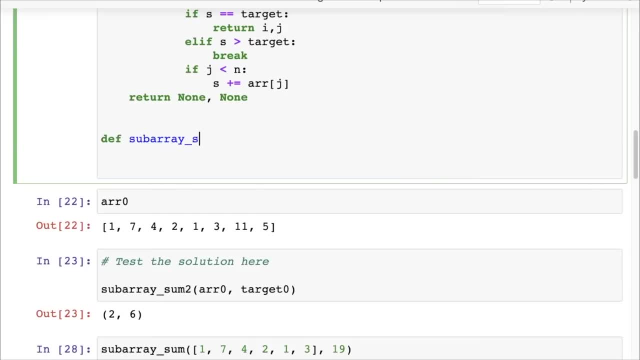 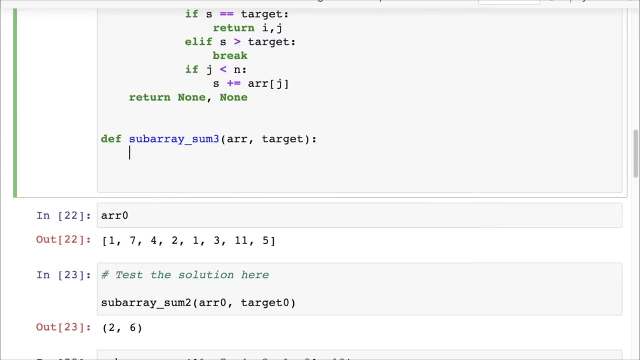 So that's the algorithm, So let's write it. So, Barry, some three. Now this is the area target. Now we have a, So we have I, we have J and we have some, all of them. let's call it S, because some is a reserved word in. 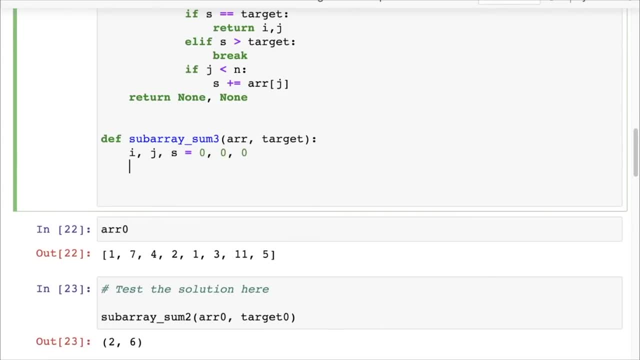 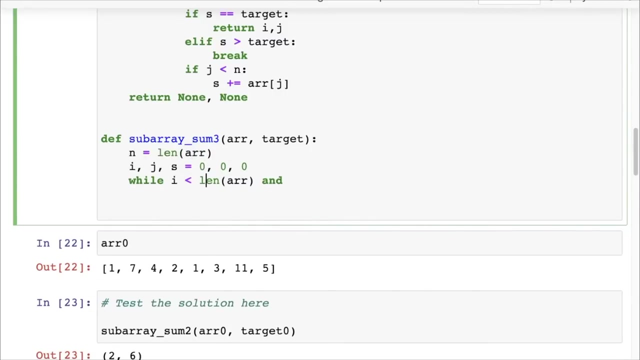 Python and existing function. So all of these have the value zero. Then we say: while I is less than Len area, let's call that end. So let's create N equal to Len ARR. I is less than N and J Is less than N plus one. 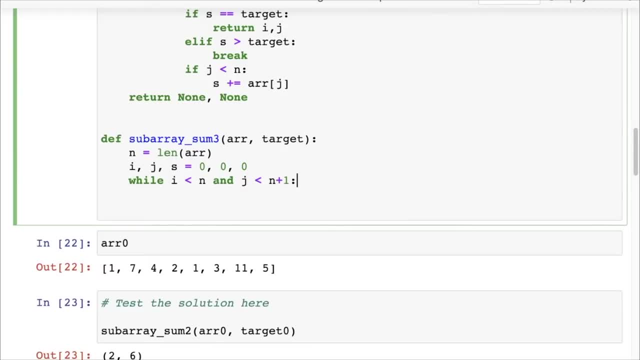 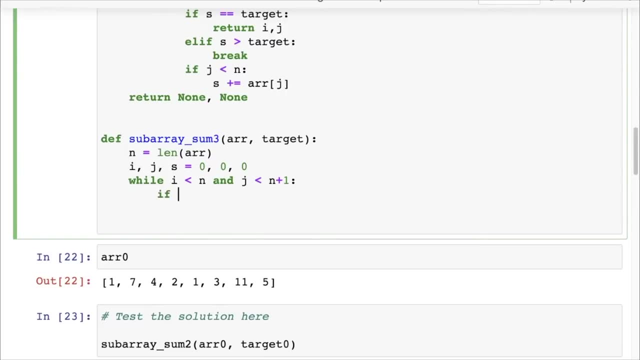 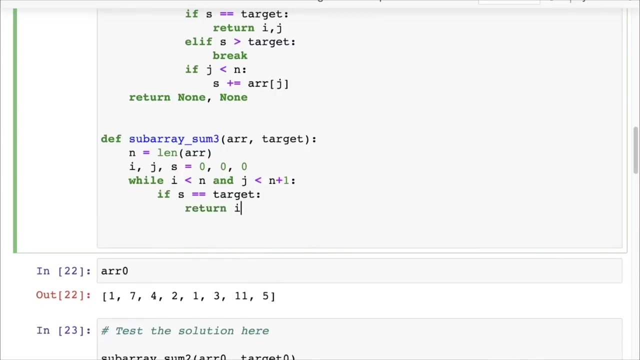 Remember, because Jay can take the value N as well- It is the exclusive end index. Now, at this point, you want to check first. So if the sum S the current some running some, is equal to the target, then we simply return. 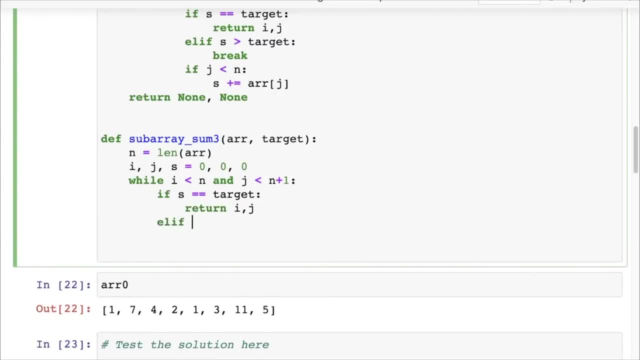 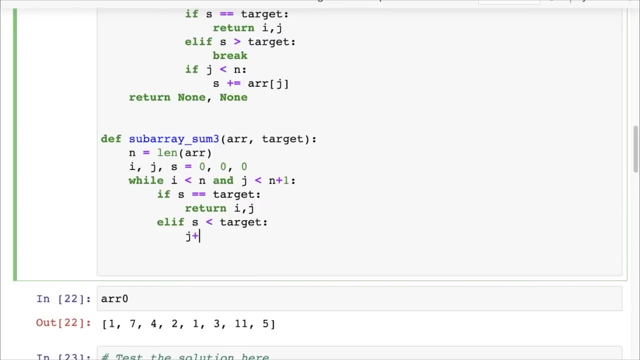 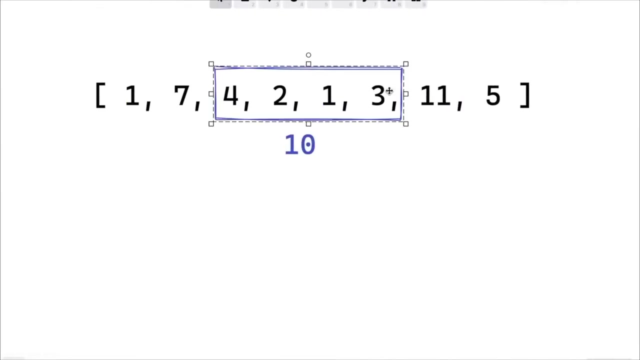 I come a J LF. Some is less than the target, Then we simply Increment J. okay, So now we can move the window forward. So we we are incrementing J. if the sum is less than the target, So we increment J. but before we increment J we should add the J element to maintain the running sum. 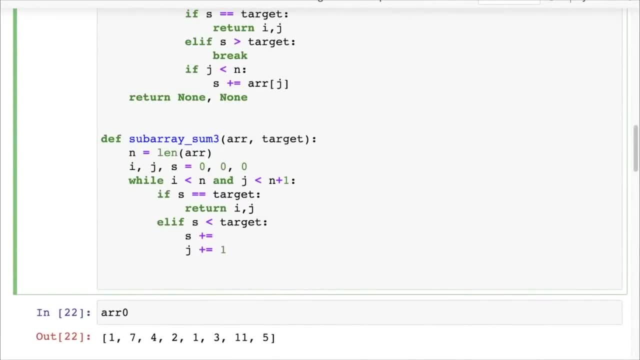 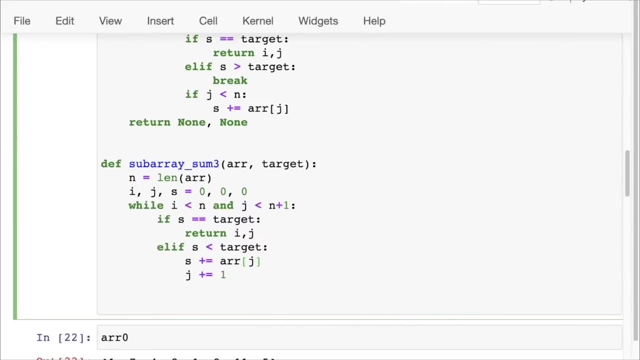 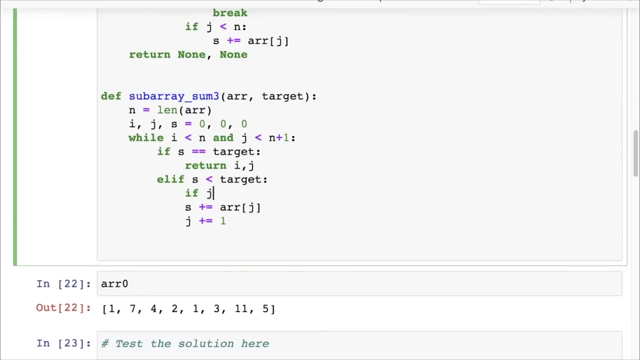 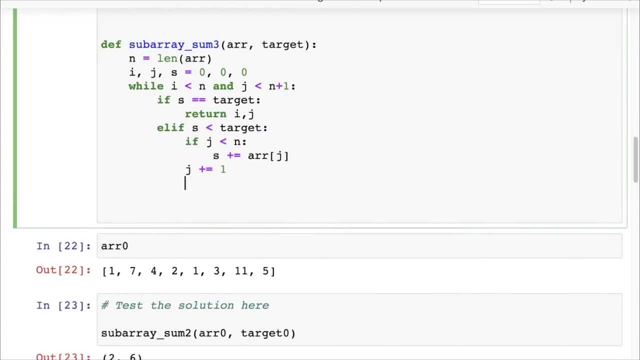 So here we say S plus equals J or area of J, And remember, Jay can take the value N as well. Okay, So that's where we do this only If Jay is less than N, if there is indeed an element for us to add. this is an error we faced last time. 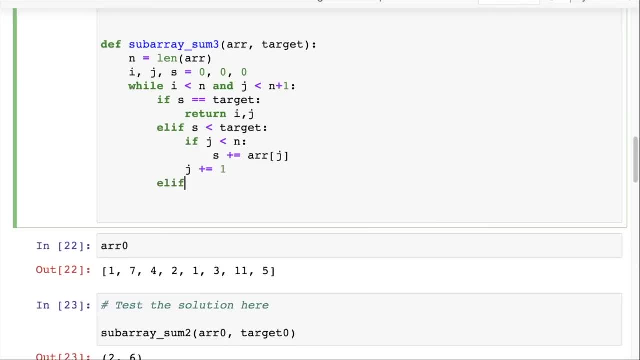 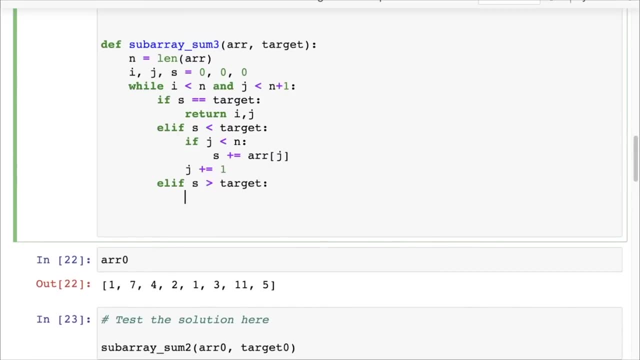 And you will discover this when you write the test anyway. and then we say LF, S is greater than target, And we can also just say else here, but just for clarity let's say LF in this case. what we want to do is we want to move- I forward. 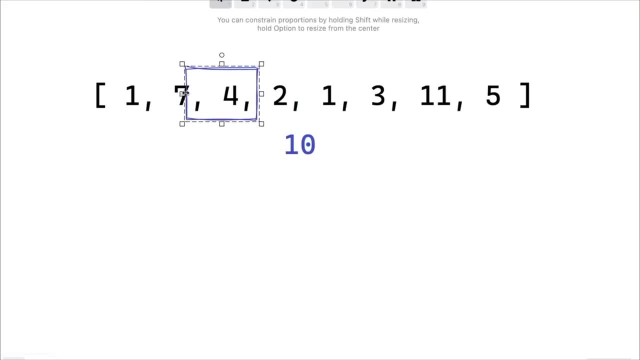 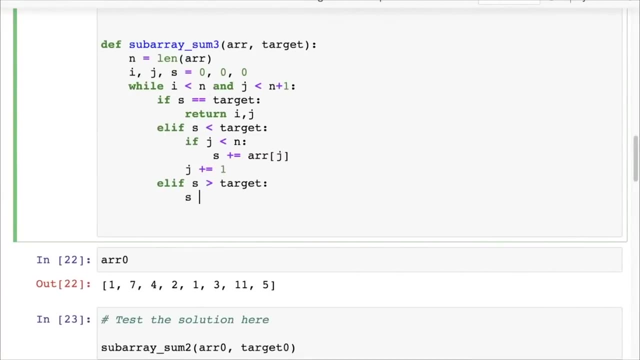 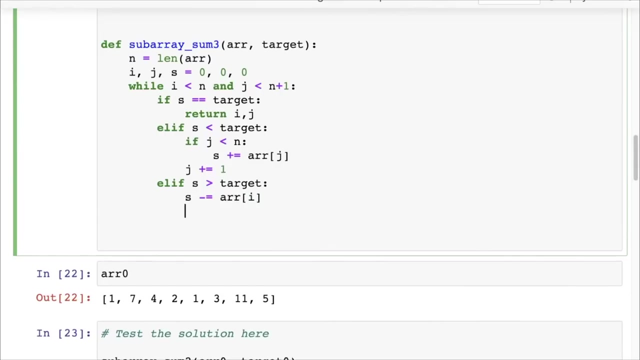 So the post. we end up in a situation like this and we want to move this forward. for that We need to subtract S array of I first, So we S, we say S minus equals, which is equal to S minus, which is the same as S equals S minus area of I, and then we increment I. 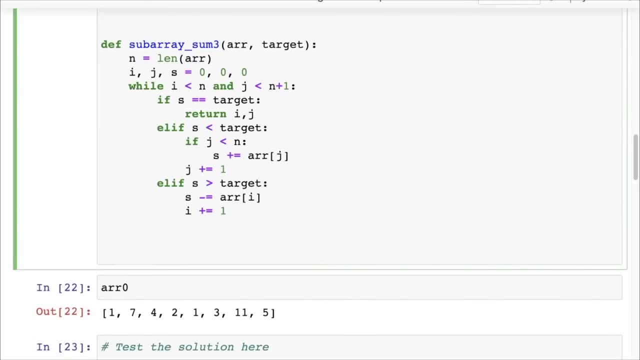 So we move the left window forward as well. So we then repeat this. So we first move J to a point, Then we, as soon as we cross the target, we start increasing I, and then we keep doing that till we match the target. 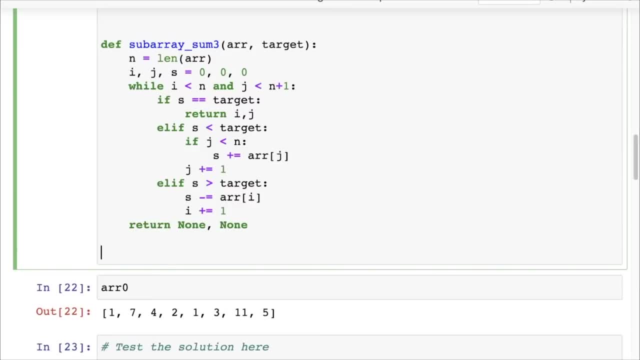 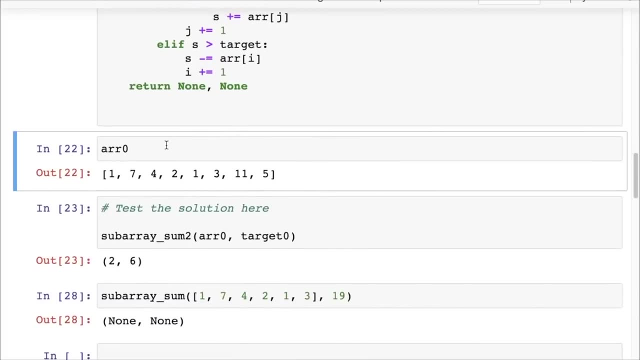 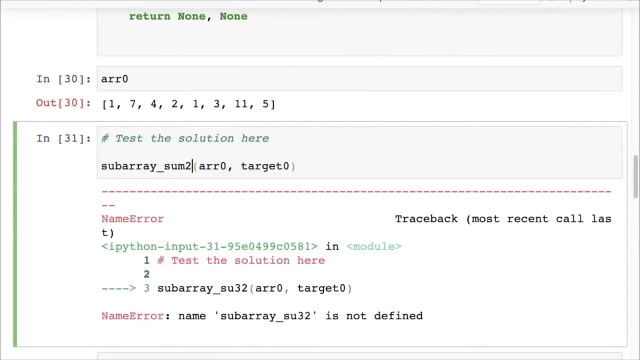 And then, finally, we return none, comma, none, if we have not found it. So that's our subarray sum three. This is seems like the most optimized solution, and let's test it out. So here we have subarray sum three, And let's test subarray sum three here as well. 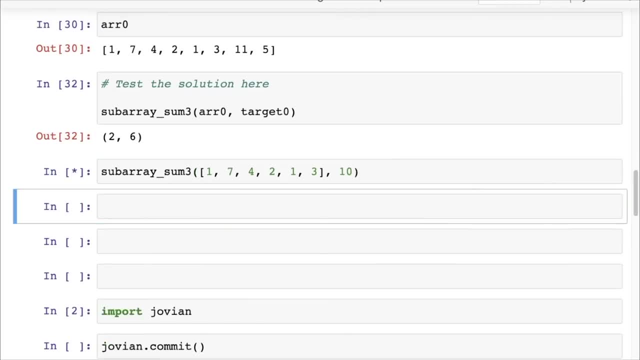 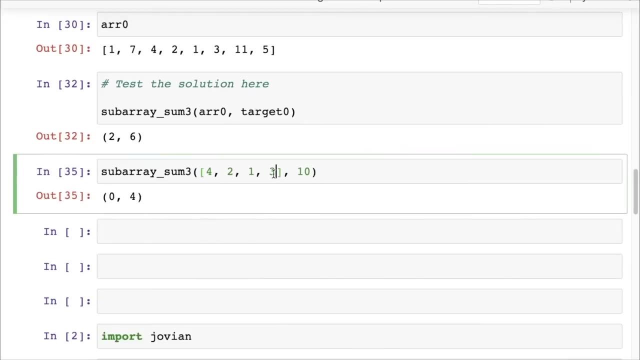 Seems like it worked, Let's see. So if you put in 10 here you get two comma six. Let's say: this is four, two, one, three, zero comma four. Let's put in 12 here, that doesn't show up. 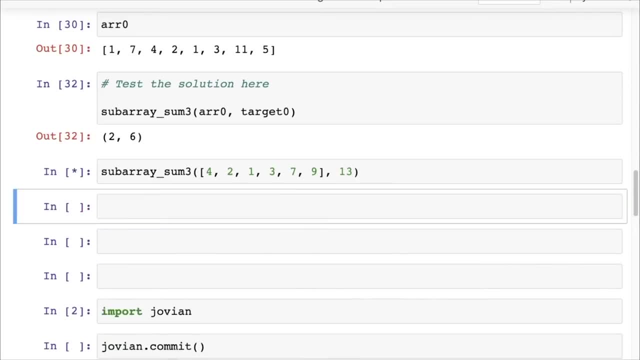 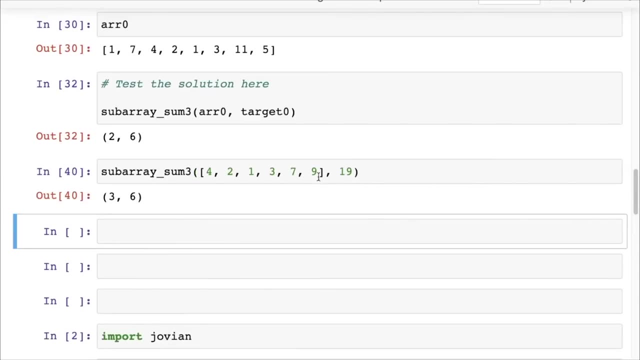 Let's put in 17 year: zero comma five, 13,. one comma five. Let's try 19, that's three comma six. Let's see one plus three plus seven plus nine. Yeah, That has the value. Let's throw in a zero there and see if it works with zeros, as three comma seven works fine. 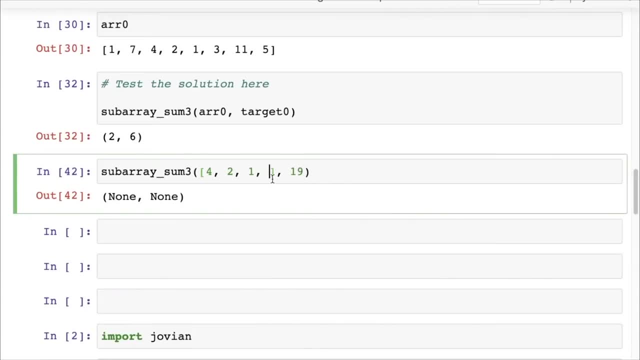 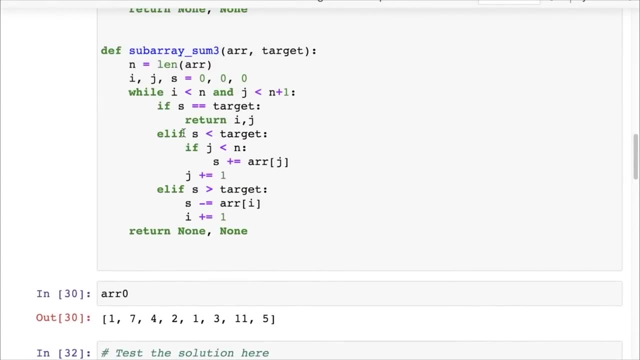 And let's see. if it doesn't work out. Yeah, Okay, great. So this solution is correct too. Again, if you don't have the option to run the code, you can simply pick one example and walk through the working of the example. 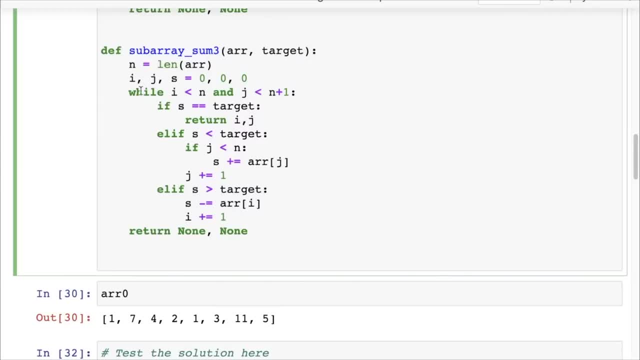 Now we have subarray sum three And once again we are ready to analyze the complexity. And in this case the complexity would be somewhat tricky. This is a little bit unusual because there is a while loop with two variables, But remember that in each while loop, either we exit, which is the best case, 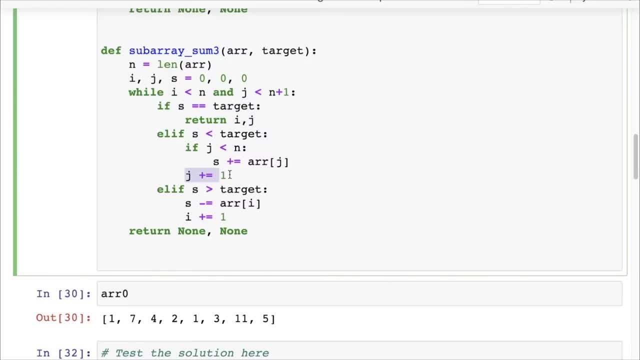 So we can ignore that, Or we either increment J or we increment I. right, So increment J or we increment I. And if we increment, Uh, so J can Go from the value zero to N and I can go from the values zero to N minus one. 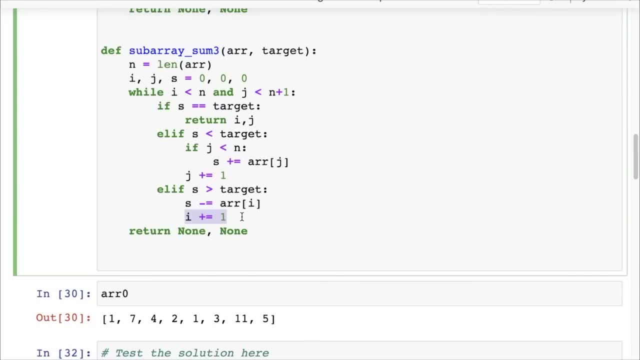 So the total number of increments. can we and we can do, is that some of the number of possible values of I and number of possible values of G? right, Remember, this is not a product this time because this you do not have a nested loop. 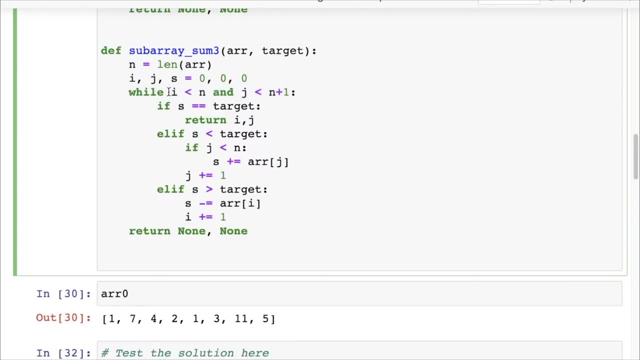 So for each value of I- you're not doing this other- you are incrementing each one and I only one of them each time. So the sum of total number of values I can take is in. the total number of values J can take is N plus one. 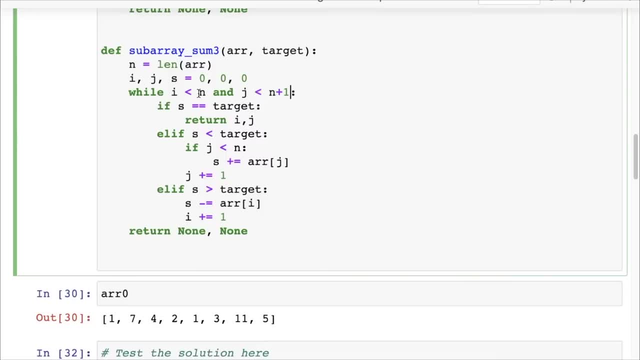 So the total becomes this number of iterations becomes two N plus one. Now, of course, uh, there's the. you can verify that a constant amount of work is being done here. So we finally end up with the conclusion that this is an order N algorithm. 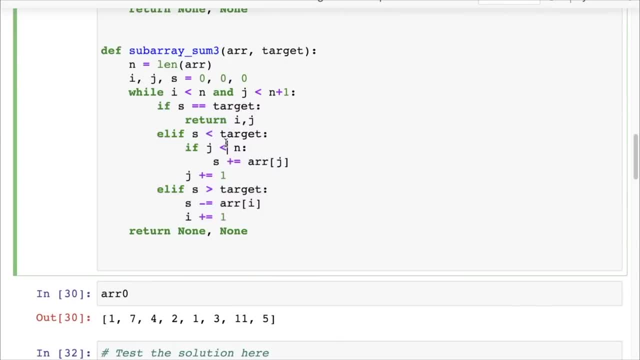 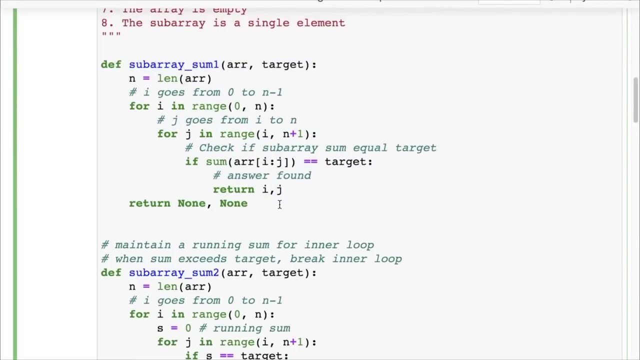 Okay, So this is finally an order N algorithm. So this is a good example of a problem where the step-by-step solution- coming up with a simple solution and then thinking about the inefficiency in the problem and then applying, in this case, just common sense to solve the inefficiency step-by-step- leads to the perfect solution, and a very good solution, in fact. so you start out with an order and cube solution. the order and cube is going to be pretty slow when you start hitting, let's say, even a thousand, even a thousand elements. if you have 10,000 elements, it'll take forever. 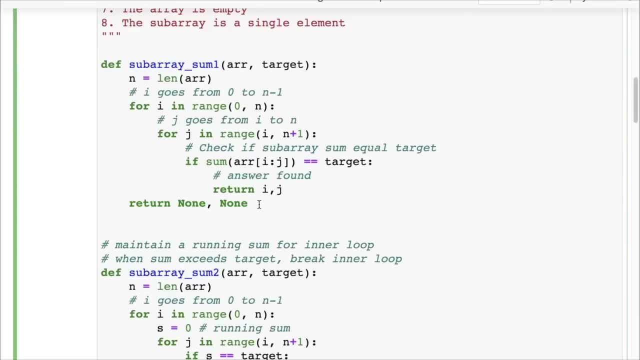 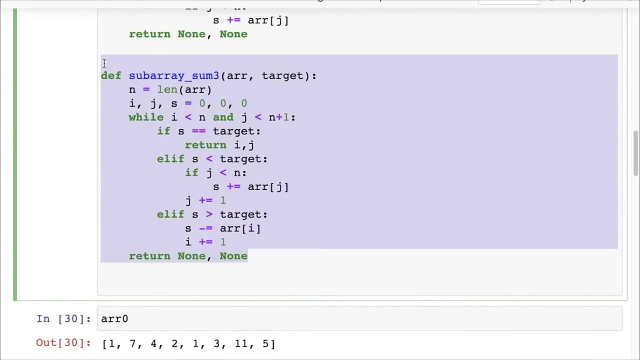 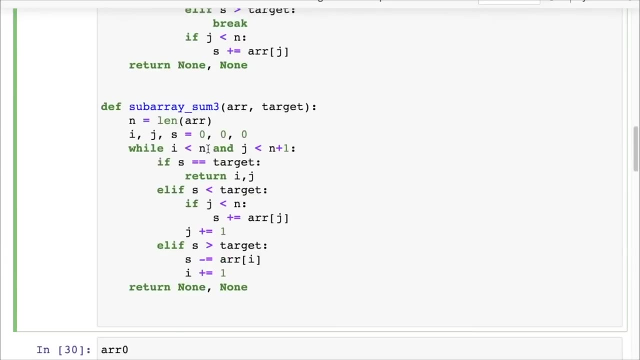 It'll take maybe an hour or so. If you have a million Elements, it will take hundreds of years. On the other hand, order N can work fine all the way up to a billion elements, right. So there's a huge difference between the severity. some one, two and three, some three can work instantly for a billion elements. 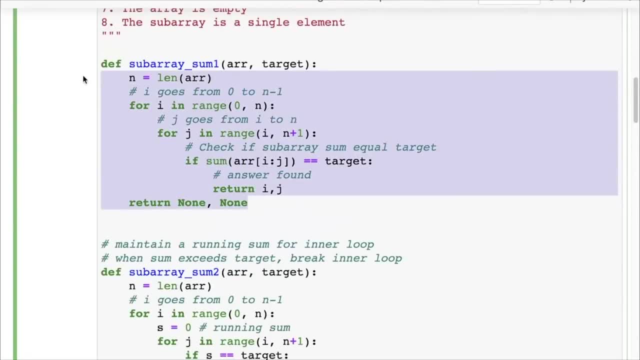 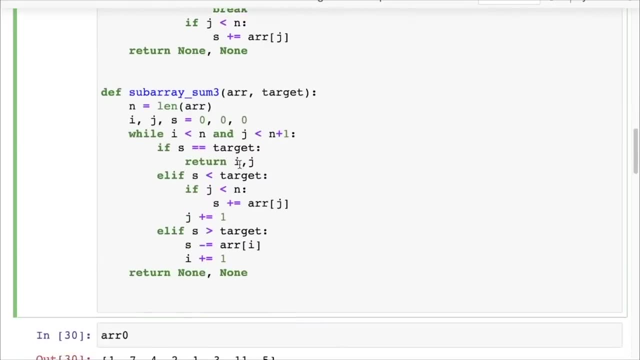 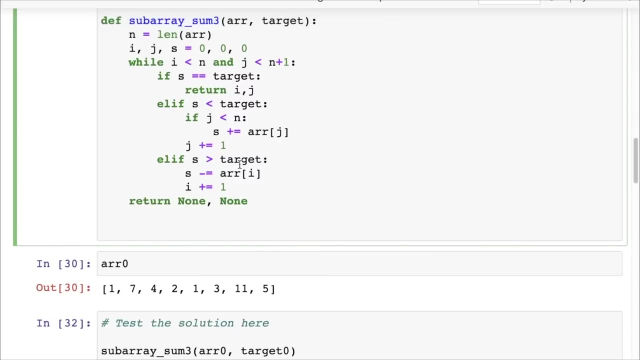 So that is some one will take whatever, even for a hundred thousand elements, and somebody who is in between, and you can do the math, You can calculate that Um and this technique where you can almost certainly tell what the next chart, what the next step is. 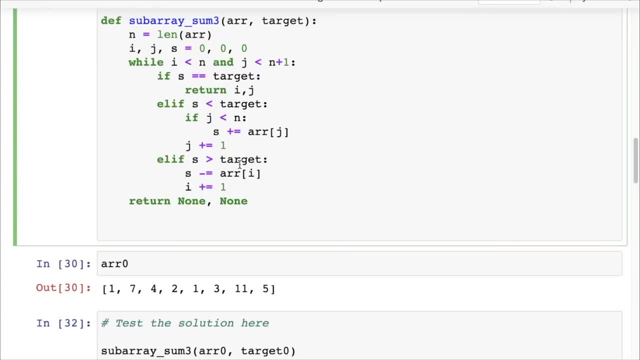 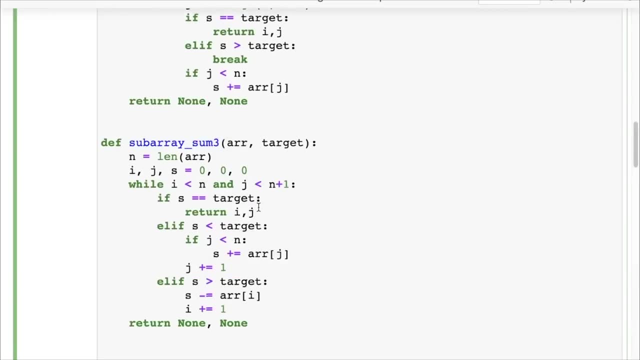 So this was not really related to any of the algorithms or data structures that we have talked about. This is what is called a greedy approach, where you know some optimal strategy about the problem. In this case, you know that we can calculate the sums by maintaining a running sum. 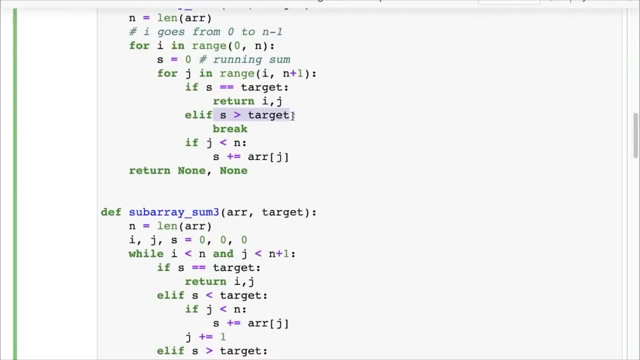 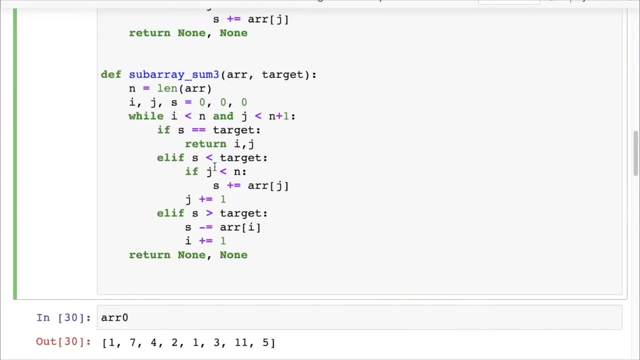 So we just do that. And then you also know that as soon as it becomes greater than a target, Yeah, We need to break out. and then you know the next thing: that when it becomes greater than target, rather, you can simply update I. so this is what what. 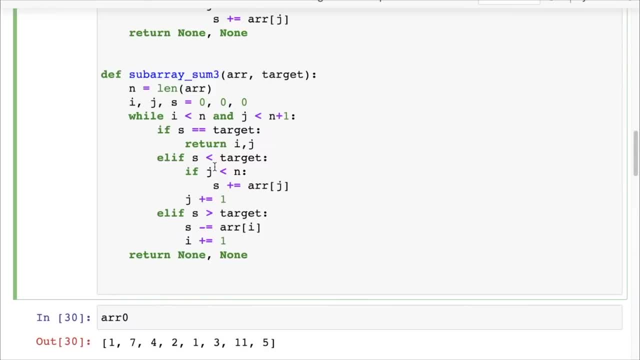 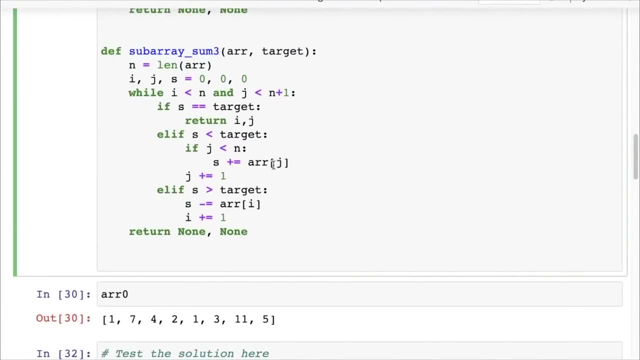 is called a greedy approach, where you somehow know that just doing this will fix it right. there's no real technique to be applied and these problems are somewhat tricky, but you get the hang of these problems as well. If you search for greedy problems online, you get the hang of these by. 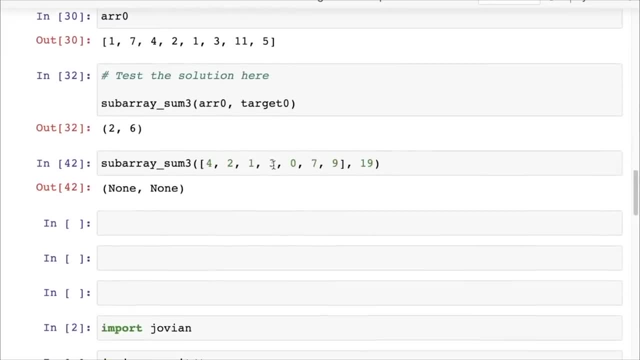 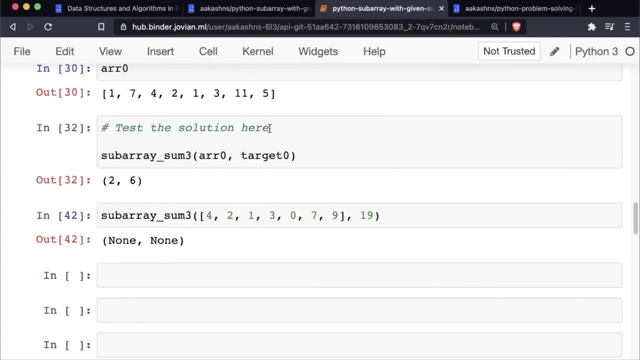 solving a few practice exercise. Okay, so that's our first interview problem and we've solved it in about 45 minutes and this is approximately how long you will have for an interview. A typical 45 minute to one hour interview will have about a couple of minutes of. 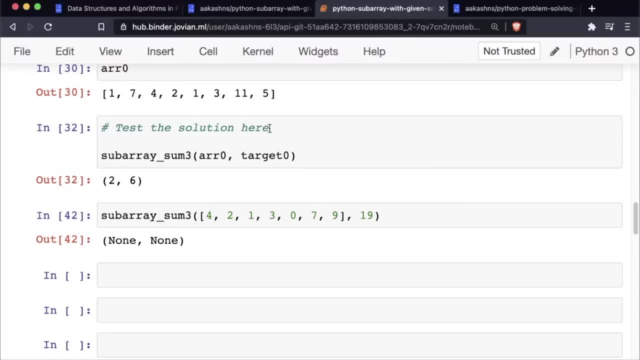 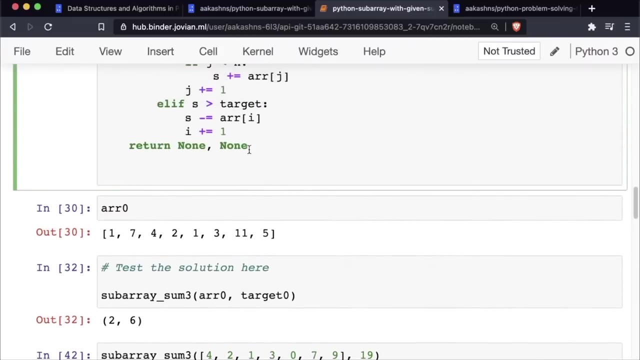 introduction, maybe a few minutes just you talking about a project and the interviewer asking you questions, but then the next 30 to 40 minutes will be dedicated towards solving a problem, And this is what roughly the process will look. Let's do one more example. 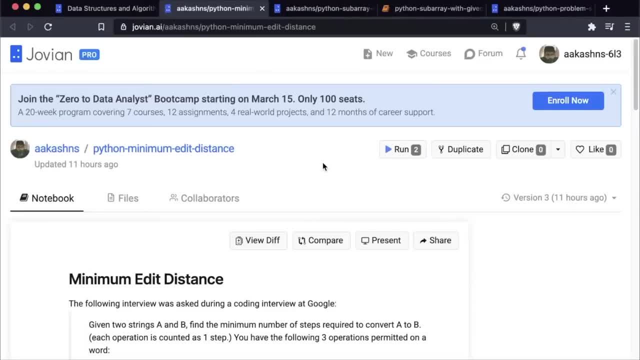 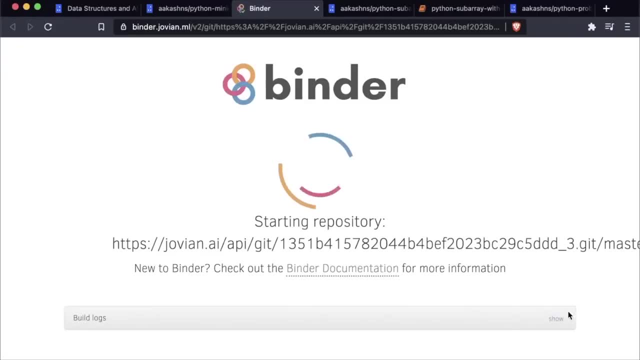 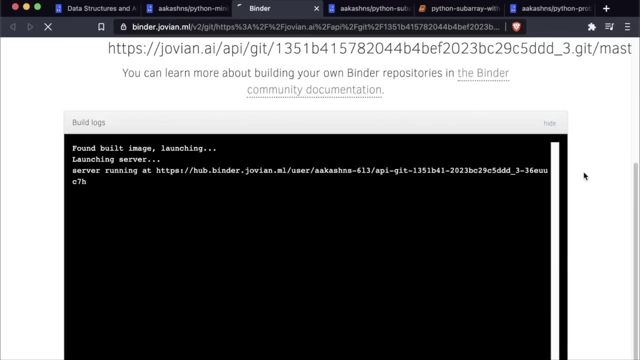 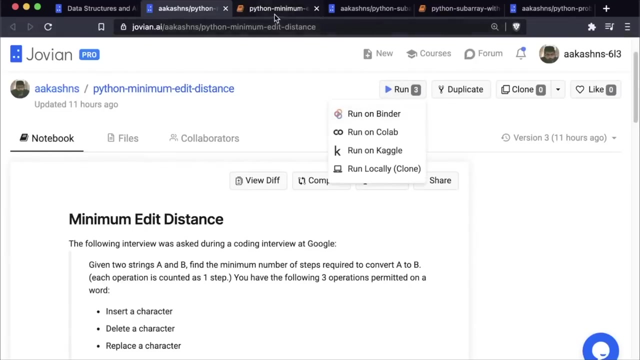 Let's pick another interview question and let's see if we can solve this one. So this is slightly different. So this gives us one more variation to study. By the way, to run these, you simply click the run button and select run on binder. 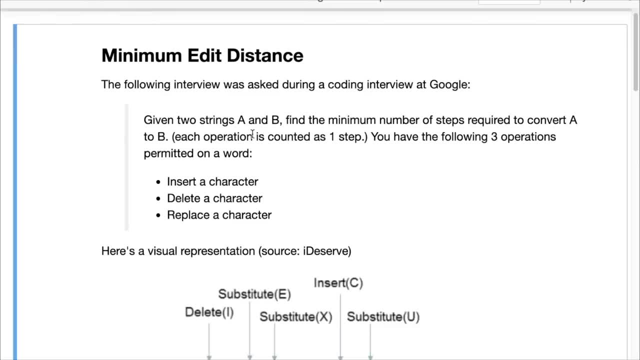 Okay, So this is an interview question that was asked during a coding interview at Google, And the question is: given two strings, a and B, find the minimum number of steps required to convert a into B. So what you can do is you can perform operations, and each operation is. 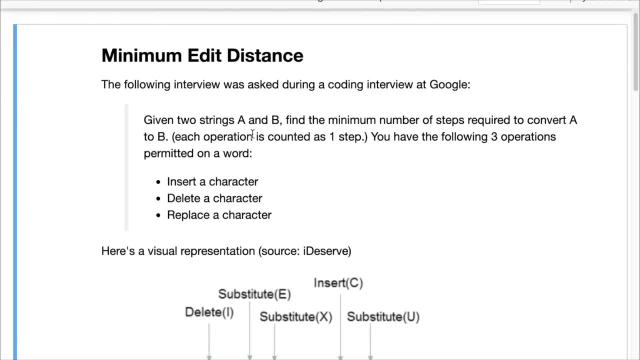 counted as one step, and the operations you can perform on a word are these: You can either insert a character into the word or you can delete a character from the word. So, for instance, here you can see that if we are trying to convert intention into 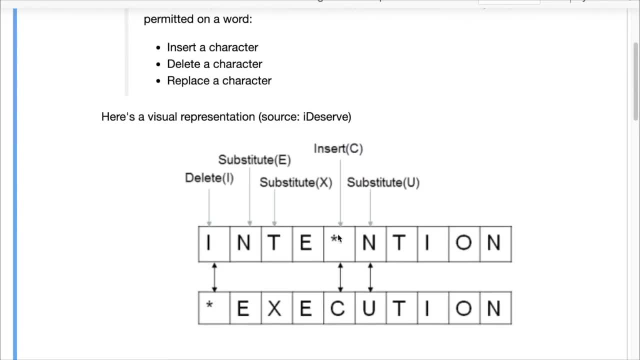 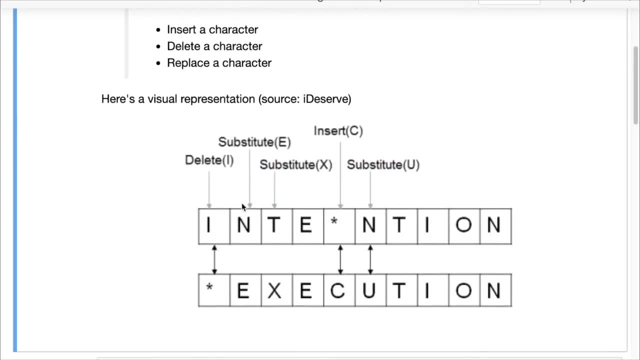 execution. so either you can insert a character- for example, you could insert C here- or you can delete a character- For example, you can delete I here- or you can replace a character, that is, you can take N and replace it with E. 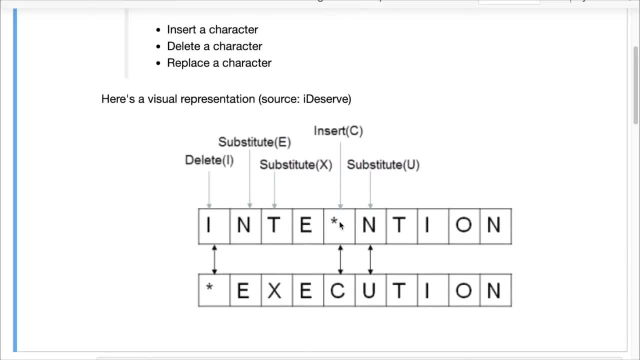 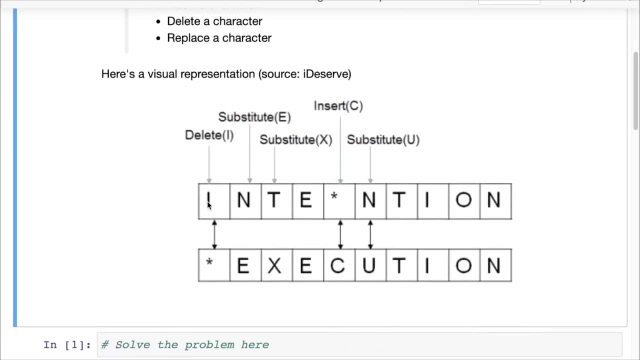 You can take T and replace it with X, and E does not need to be replaced. And here we've inserted C and then here we substituted N for you right. So we've taken the word intention and, by performing a few changes, character by. 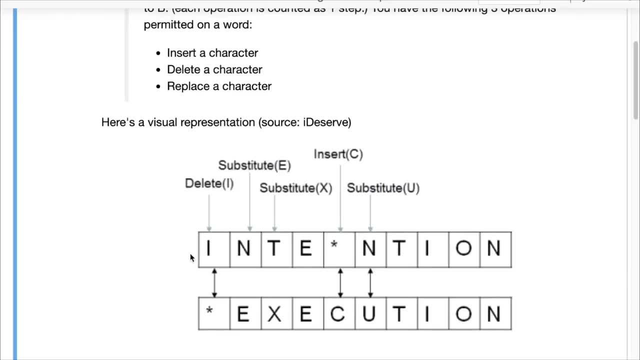 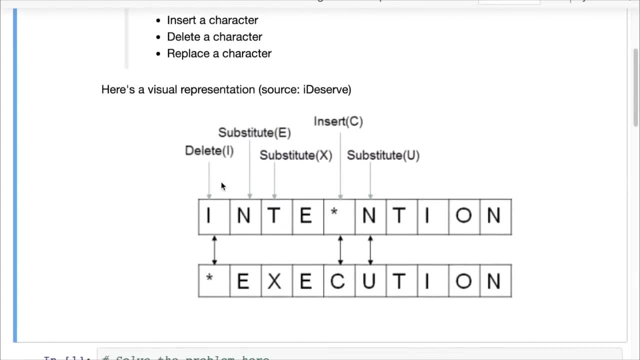 character. by either inserting, deleting or replacing a character, we have converted it into the string execution. So the number of steps required here is 1,, 2,, 3,, 4, 5.. Now here's a challenge for you. 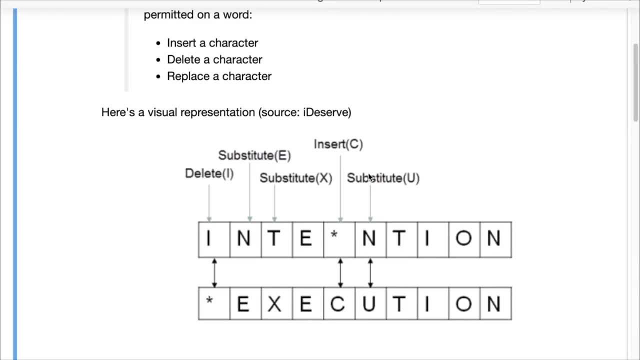 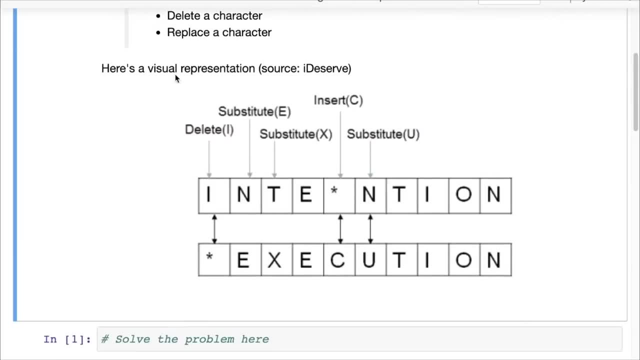 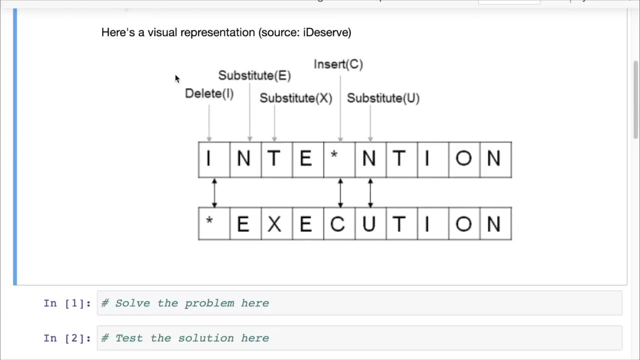 Try and work this Out on paper and prove that this is the best solution, because we need to find the minimum number of steps required to convert A to B. So that's the problem, And this is a moderately hard problem, and variations of this show up as well. 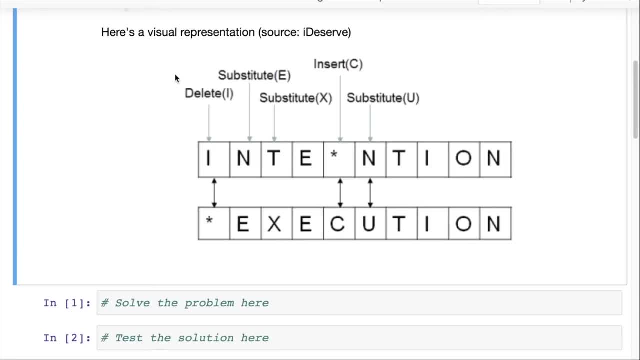 So let's start applying the method Now. when you hear the problem, a solution may not strike you upfront. That's perfectly all right. Don't panic. sometimes When you're not able to immediately come up with a solution or identify how to solve this problem, you enter a sort of panic and then you're unable to think. 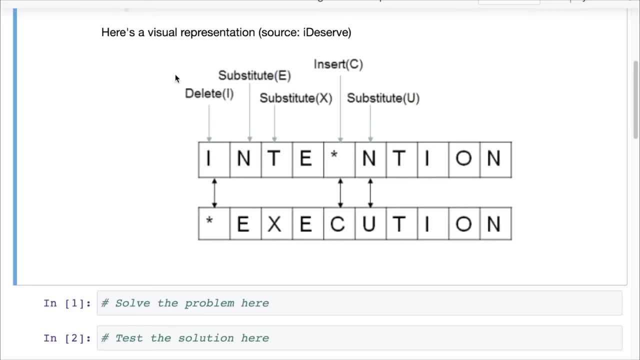 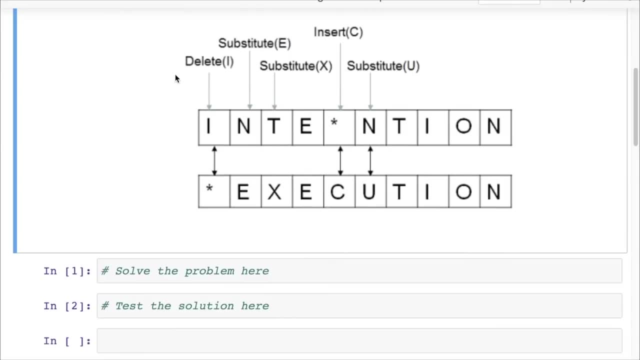 Don't do that. Remember: have faith in the method and we will apply the method and come up with a solution step by step. So the first thing is to state the problem in your own words. So, given two strings, we need to perform operations, a series of 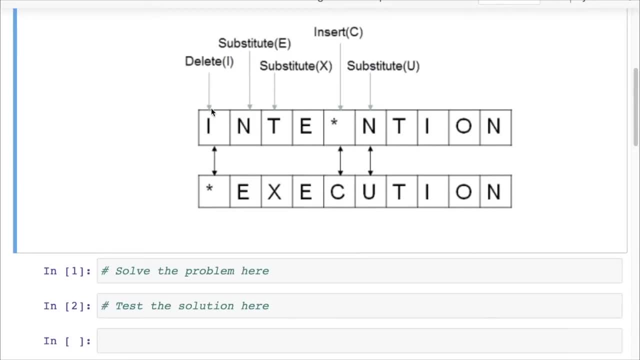 operations on the first string. The operations could be deletion of a character, Substitution of a character with another character or insertion of a character, And through these operations we need to convert it into a second string. Okay, We have understood the problem. 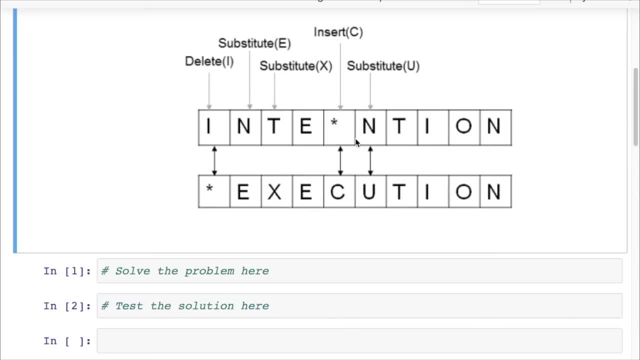 If the interviewer had not given an example. either you can state the example or you can just ask for an example. whatever makes works for you. So we've stated the problem. Now what are the inputs to the problem? So the inputs are two strings. 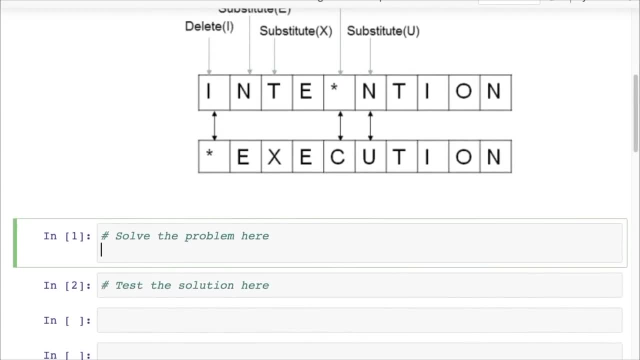 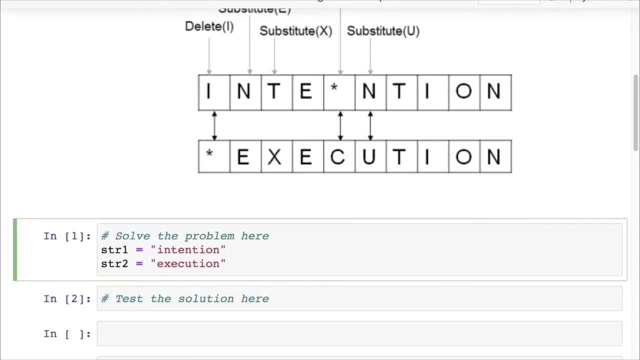 So the inputs are strings like intention and execution. Let's see. Maybe let's call them STR one, This is intention, STR two, This is execution. Now, one thing you have to be careful about here is you do not want to capitalize, because sometimes what might happen is this: I may match up with an I. 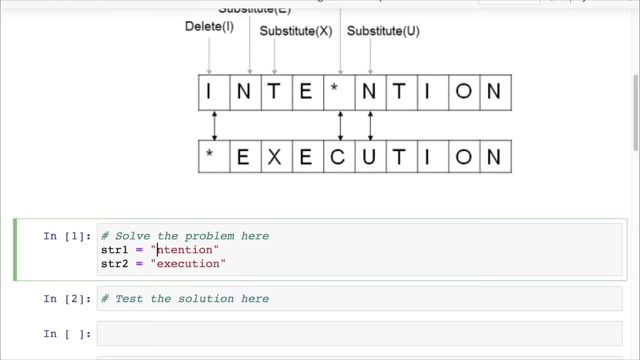 here in the in the proper solution, but Python obviously treats small and capital letters differently. Python doesn't know what's that. The I which is lower And the I which is uppercase is the same, so you will not be able to compare them. 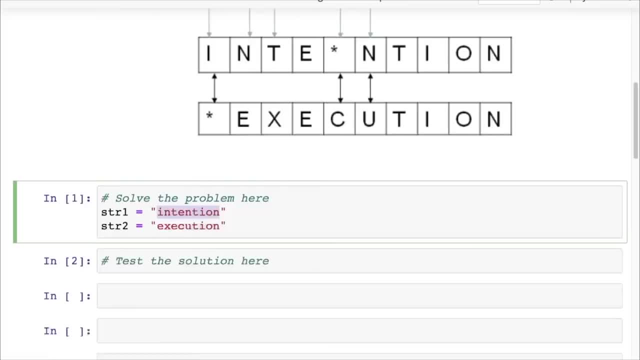 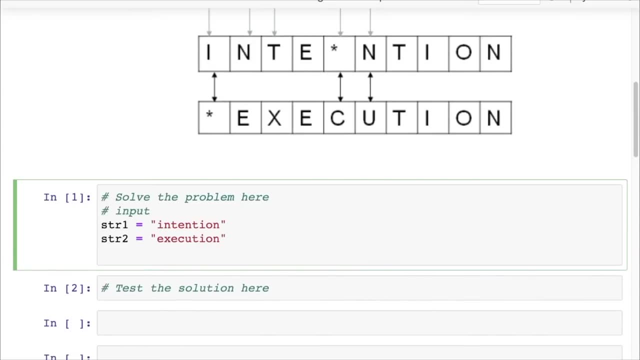 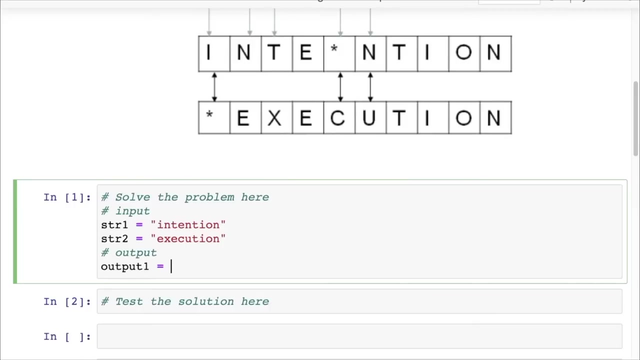 So, just to keep things simple, either make everything uppercase or make everything lowercase, but yeah, this is what the input looks like and the output is going to be a single number. So the output is simply going to be the edit distance. So let's just call it output one and it is going to be the number five. 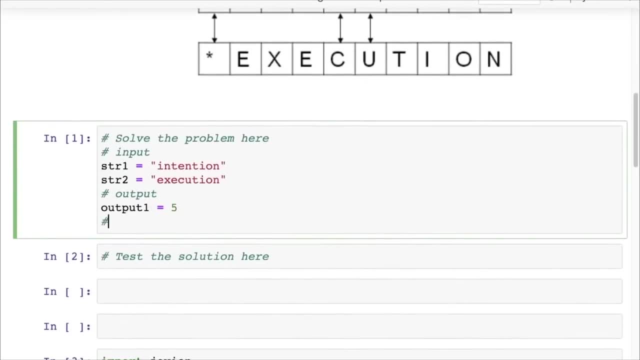 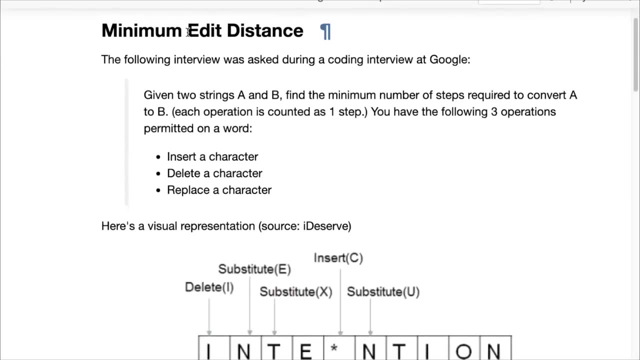 And here is something that you can verify. So that's the input, That's the output And Function signature. So of course, this term edit distance is how this problem is described, but here there is no edit, There's no concept of edit distance. that's mentioned. 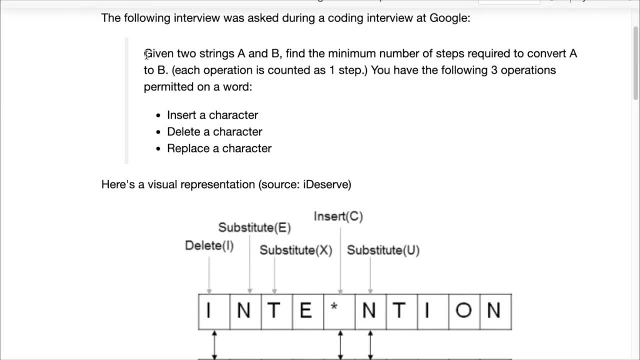 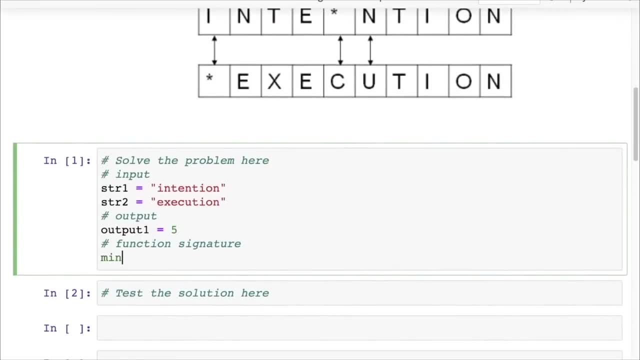 So you can give a function name that makes sense for this problem. So find the minimum number of steps required to convert A to B. Okay, So let's just call it min steps for now. So the function definition would be min steps and this would take an. 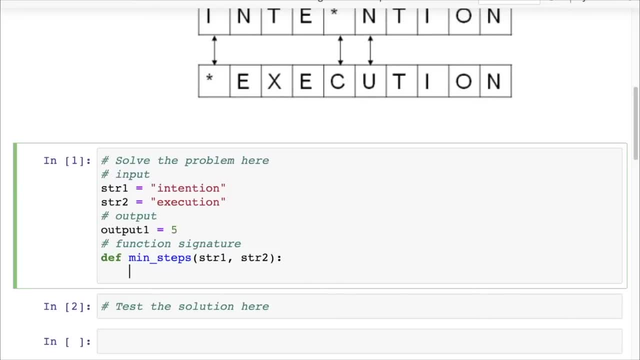 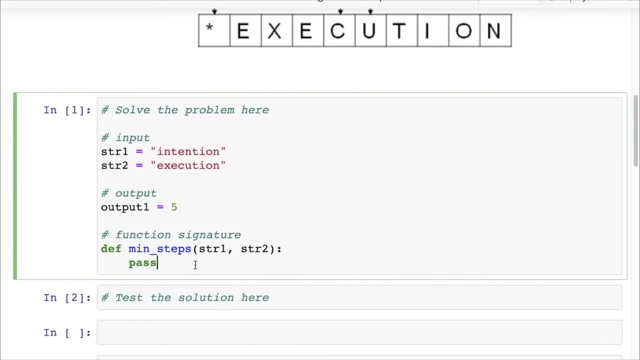 STR one and this would take an STR two and it would return an output. for now We'll just put in pass here, All right, So now we have already clarified the problem. If you had any questions, this is this would have been a good time to ask the interviewer and make. 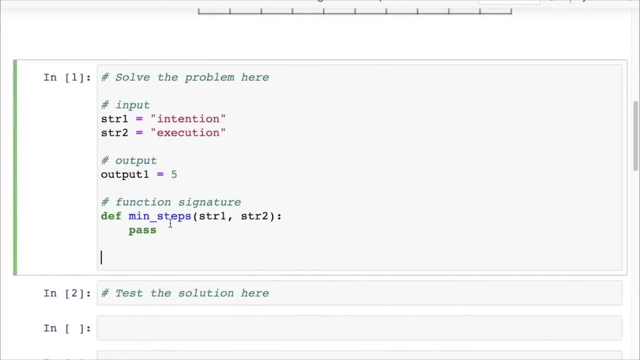 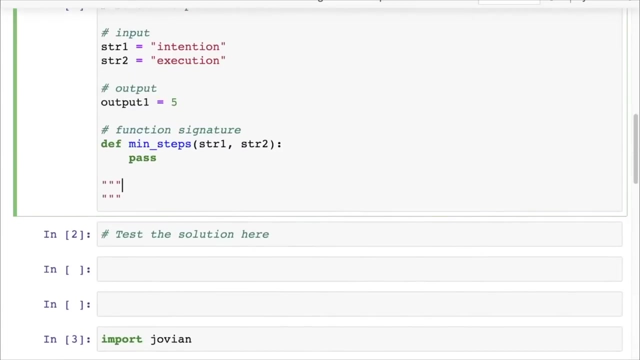 sure that you have a clear understanding. Now you have stated the input, output and function signature, The problem has been communicated back and forth properly. The first step is done. The next step is to List out some test cases. right, Once again, a very good quality. listing out some test cases. 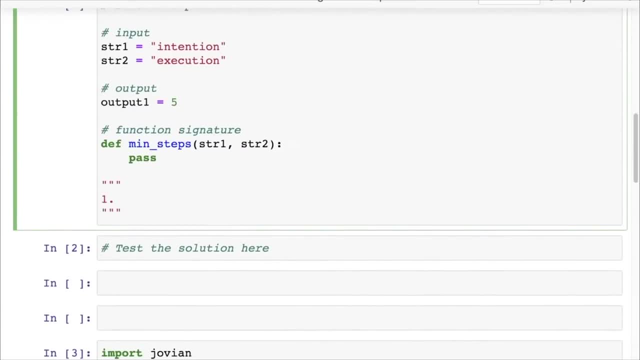 So you can say that now I'm just going to list out a few cases that I want my function to cover so that they will help me. It will help me while writing the code. Now, one is the general case which is listed above. 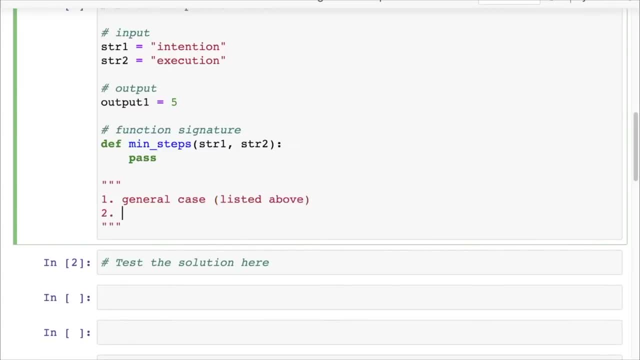 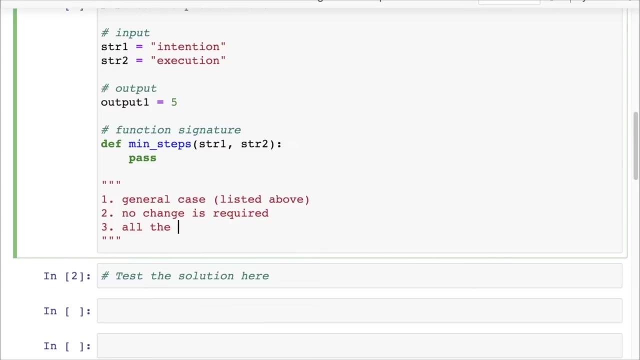 So this would be intention execution, And we can take a few more examples like this. Now, one example could be where No change is required, So you are given the same strings. One case could be that all the characters need to be changed. 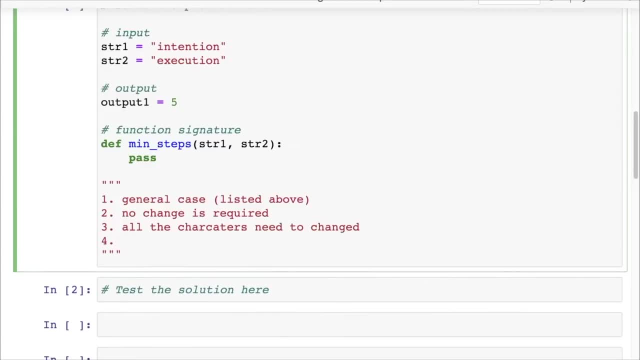 So these are the two extreme cases. One is no changes required And second is all characters need to be changed, Maybe added, removed, deleted, lots of such things. Then you can check both strings of equal length. So in this case they are in fact of equal length, unequal length. 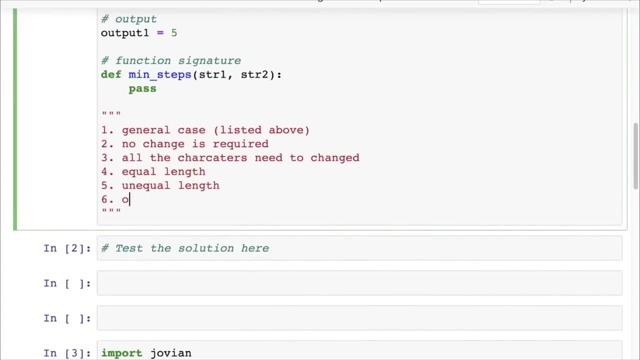 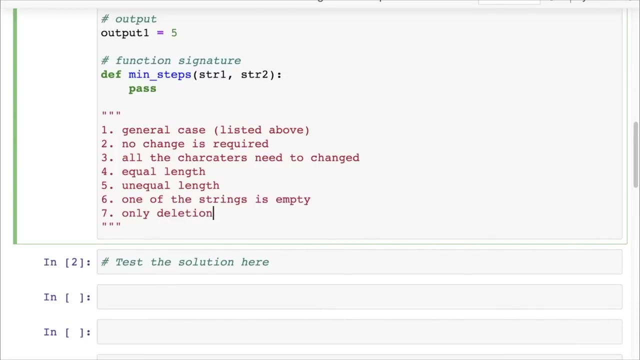 You can check both strings of unequal length. One of the strings is empty. Your function should be able to handle that too. Then you may check things like it will: if something only requires deletion, if something only requires addition or if something only requires swapping right. 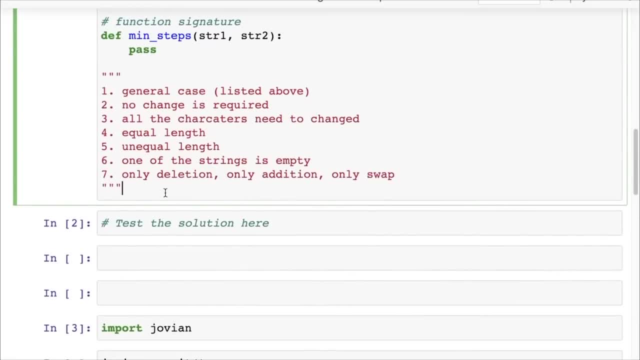 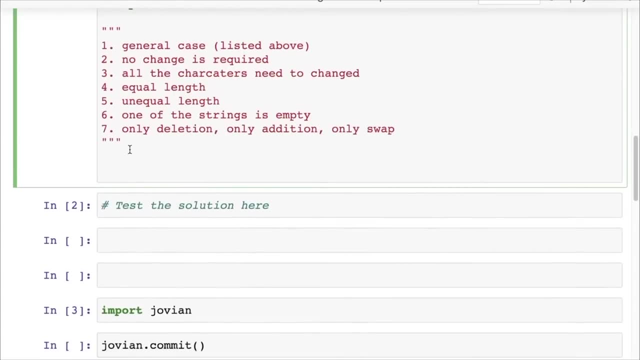 Such things. I guess this is pretty good at this point. So now we can probably move forward. So we have stated some test cases Now. you don't need to create all the test cases right now in an interview. It can take a lip, take a bit of time. 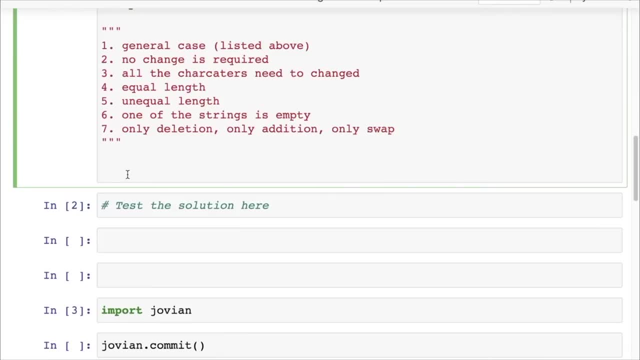 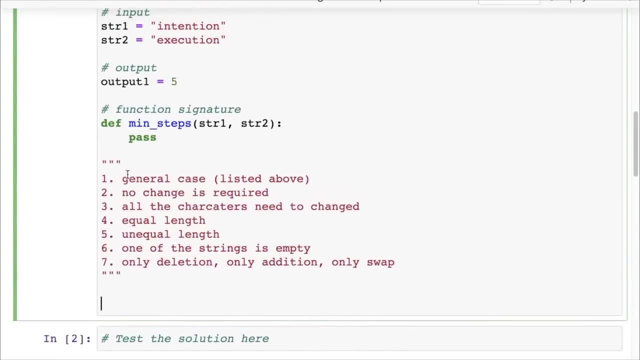 So let's just move ahead, And the next step is to come up with the simplest solution to the problem, which is also called the brute force solution. So now we have a lot more information about the problem. in this meantime, probably it has sunk into you and you may have been able to think of a brute force solution. but if not, 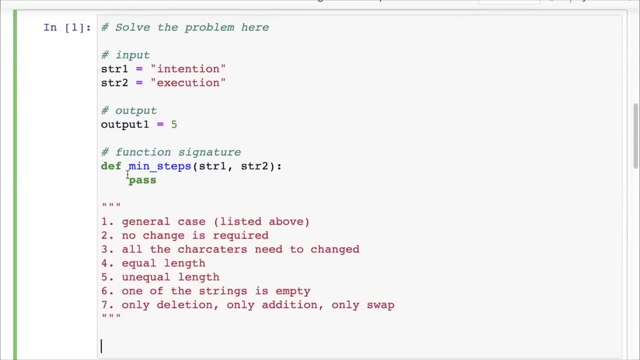 don't worry, there is a simple trick I'll tell you, which you can apply whenever you are stuck and you can't think of a brute force solution. So we are looking at- you're looking at it- intention, execution. What am I going to do? 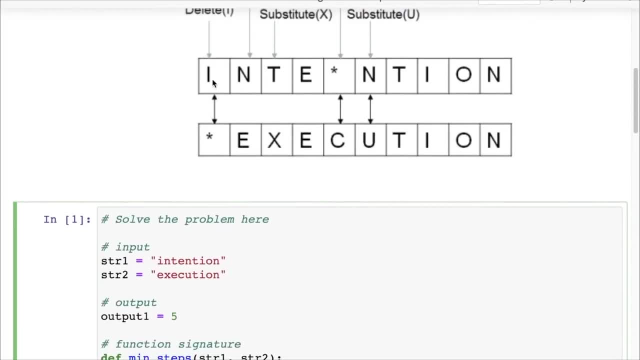 Am I going to start from the left and right? How do I check which one is? how do I know if this is going supposed to be inserted or executed or replaced or substituted or deleted? So that simple trick is when ever you're in doubt. 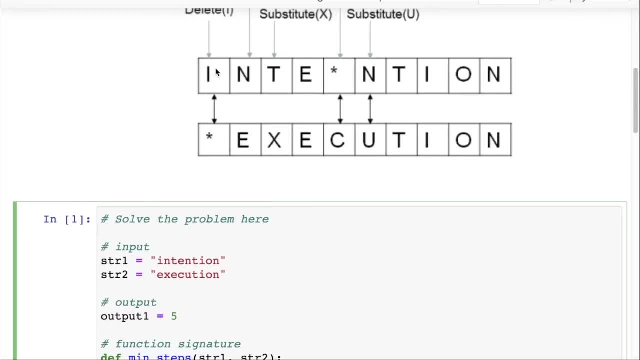 Think about recursion, see if there is a way to solve this problem recursively. And what do you mean by solving a problem recursively? Can you reduce the overall problem to a combination of one or more sub problems. So if you take a portion of the input and can you solve the same problem on the portion, 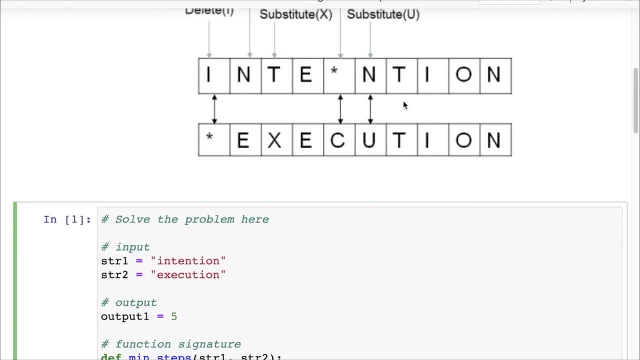 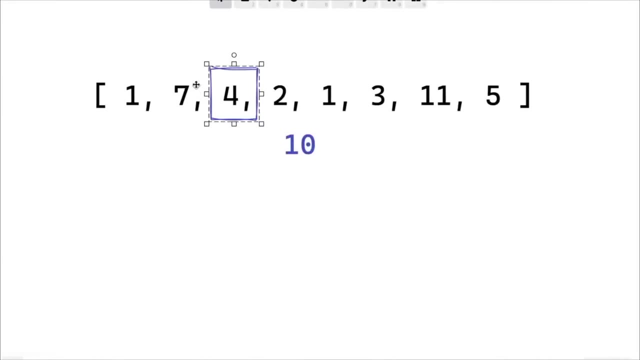 of the input and then use that to solve the overall problem. Okay, So let's see. let's see if there is a recursive solution. So let's see if there is a recursive solution. Okay, Okay, Okay. So let's see if there is a recursive solution possible here. 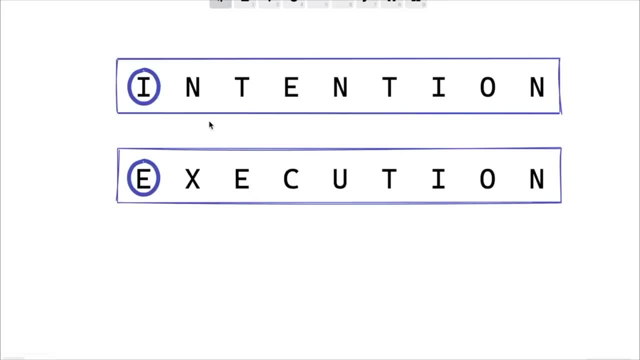 So here I have the same thing: intention and execution- Now with recursive solutions. normally you either start by looking at the first character or the last character, So let's look at the first character of each string, right? So we've given these two strings and we need to find the number of operations. 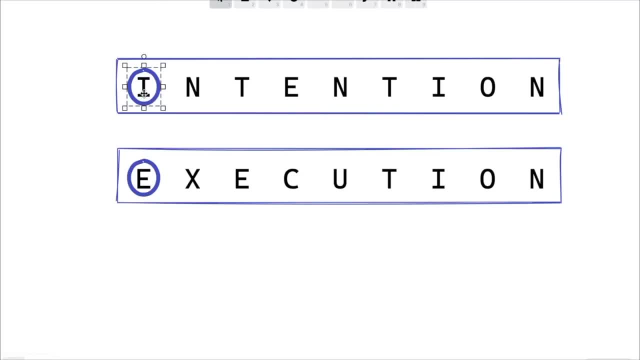 to change this string into this thing. Let's look at the first character. Now suppose the first characters. So suppose this was not intention, but this was intention and this was execution. So now we compare the first characters and we know that the first characters are equal. 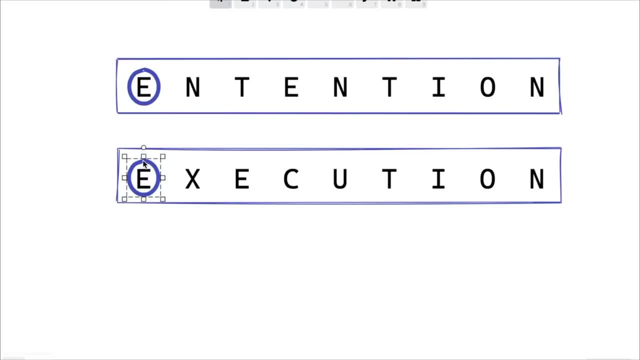 Okay, So if the first characters are equal, then obviously neither of them needs to be deleted or removed, or obviously this character does not need to be deleted or removed or switched. It's already matching. So what we can do is we can just ignore the first characters. 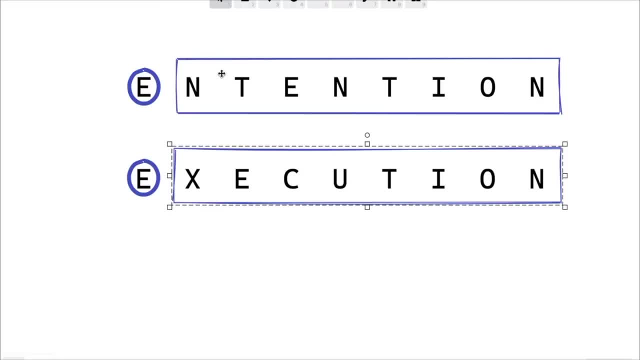 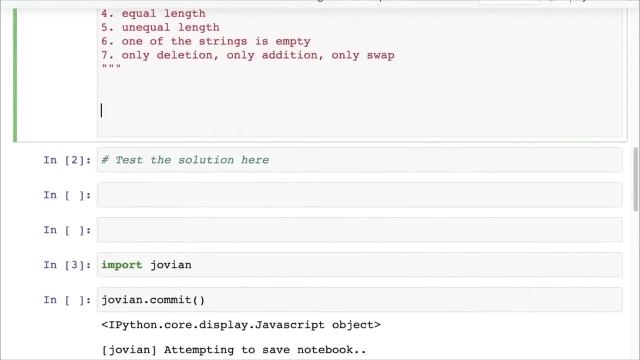 Okay, Okay, Okay. So now we can simply look at the remaining string. Okay, So intention and execution: because the first characters are already equal. Let's write that down so that we don't forget it. And this is the recursive solution. 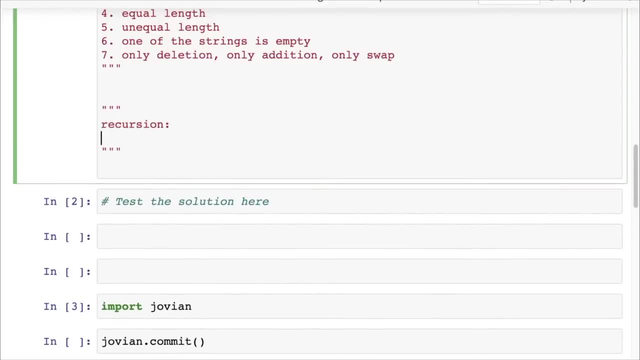 Now this is where you can take a moment to work this out on pen and paper, and that's perfectly all right. What helps us to just talk? keep talking about what you're doing. but for recursion Now, first thing we know is if the first character is equal. 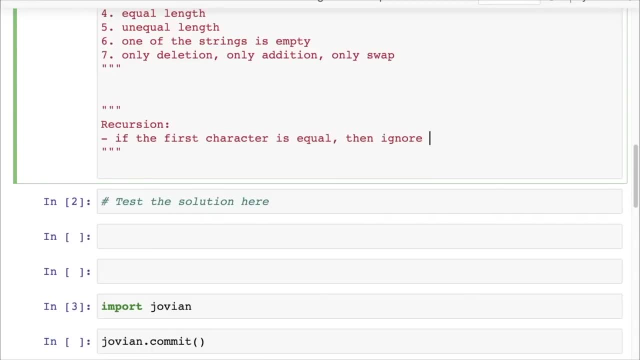 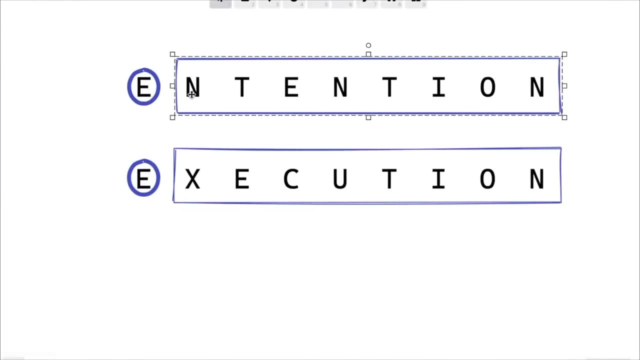 So the first character is equal. Can we just ignore it? Then ignore from both, So you just ignore the first character of both strings and simply recursively solve the problem for the sub list and the order sub string without the first characters in each of the strings. 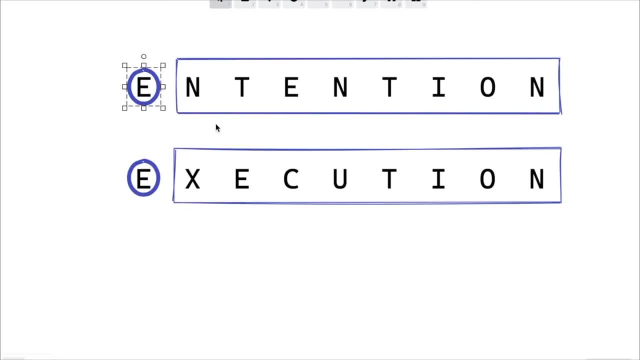 Right, So you're: exclude E and exclude E from this and solve the problem for these two, Perfect. Now suppose the first character isn't equal, So that's another case. now, Right, So that is the case where you have intention and execution. 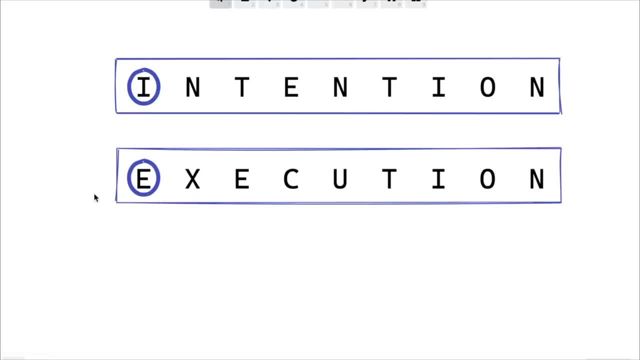 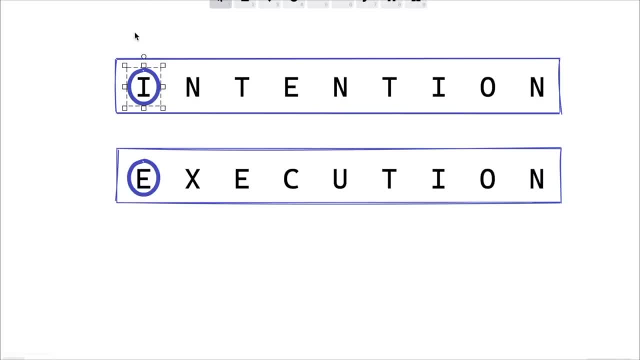 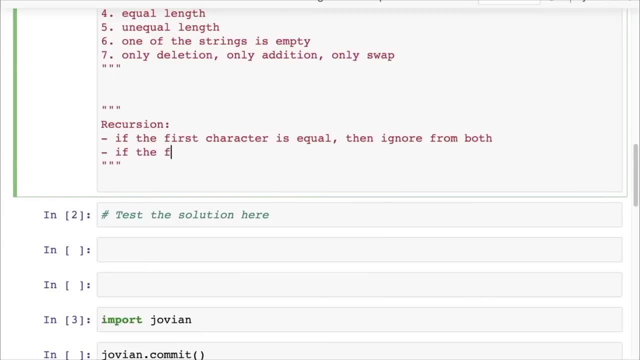 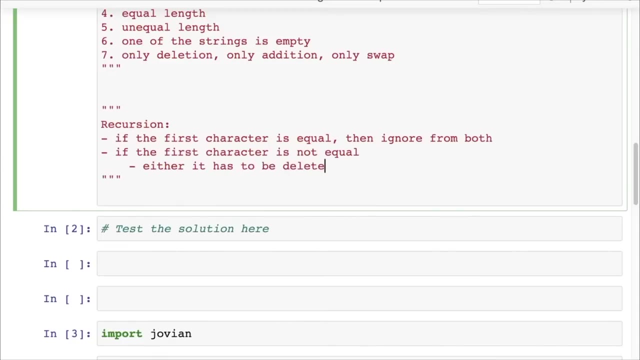 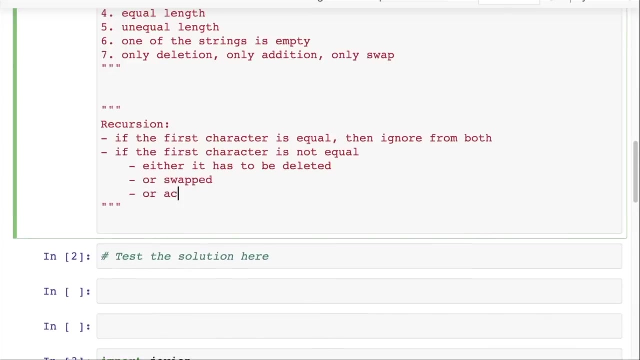 needs to be added before the first character. Okay, Now let's see one by one. So if the first character is not equal, either it has to be deleted Or swapped, or a character inserted before it. there are only three possibilities, right? 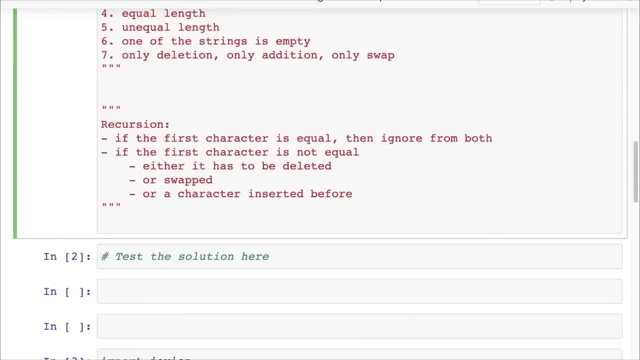 Of course, it's possible that we may do some other things, insert characters after, after it, and so on, but at that position, after applying an operation, either the first character will get deleted or the first character will get swapped and will be changed. 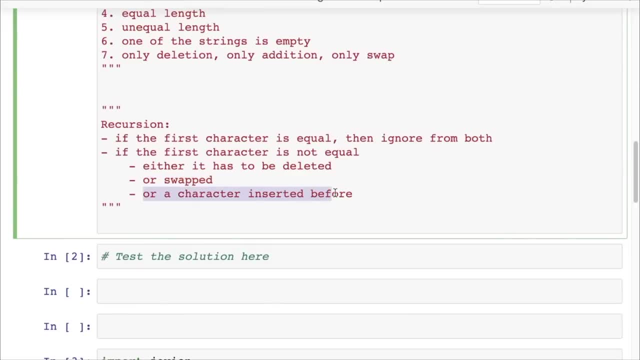 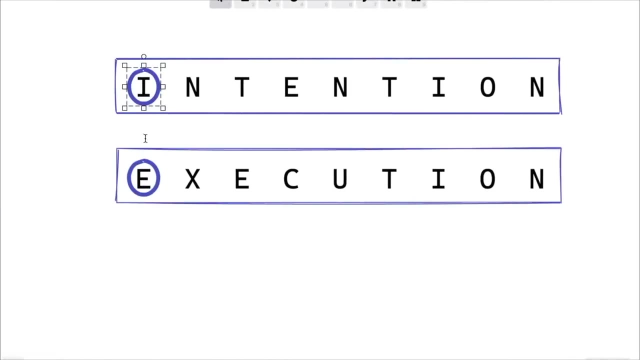 To E, or the first character will not change to something else And the first original first character will become the second character. Okay, Now let's look at each case. The first case is: it has, if it is deleted Now, the power of the duty of recursion is that we don't need to guess which solution it is. 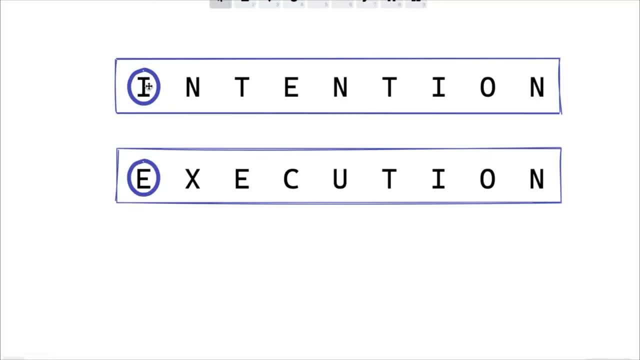 We can try all three recursively and then simply pick the best one. So suppose we choose to delete the first character. So suppose we say that we are deleting the first character. Now what that means is, we've performed one operation And we've deleted the first character. 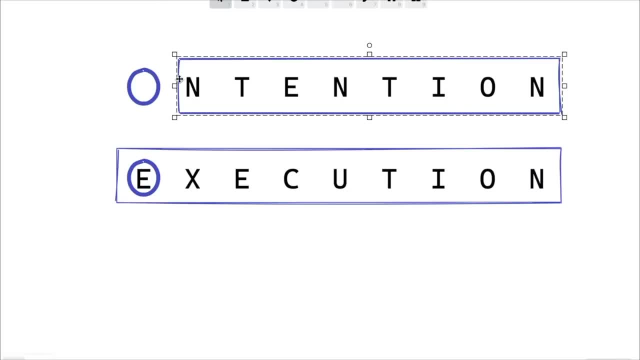 So now what we're left with is this. So now what we end up is the second: the string has remained the same, Only the first string has changed, where we have lost the first character. Now what we end up with is with a sub problem where we need to find the minimum number of 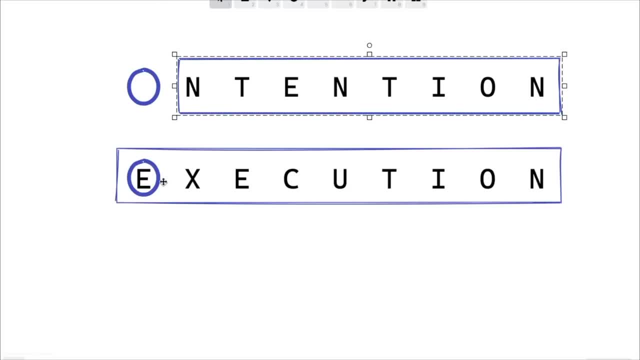 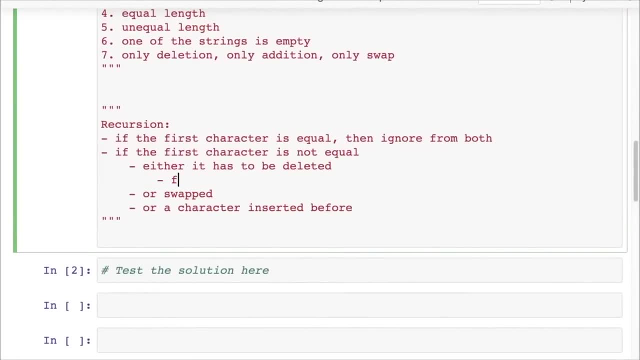 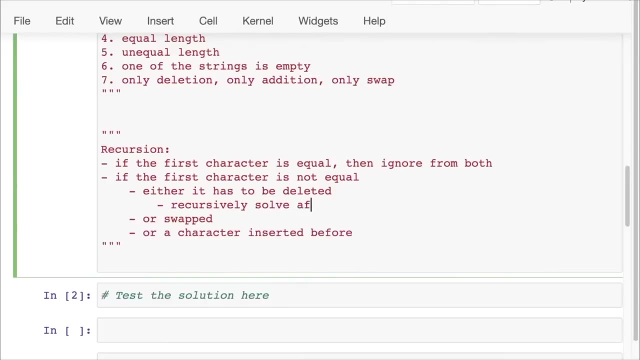 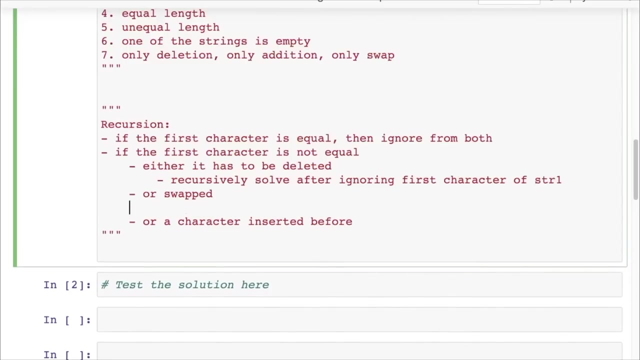 steps to change intention N T E N T I O N into execution. Okay, So in this case, if it has to be deleted, then Recursively find, Then recursively solve, after ignoring first character of STR one. Okay, That's one possibility. 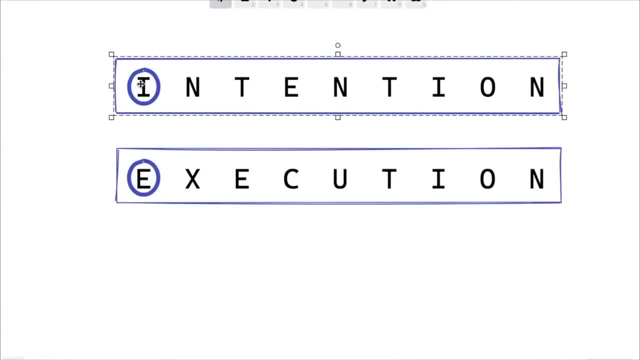 And the. you get the recursive solution and you simply add one to it. that tells you the solution. If you delete the first character. the next option is that we change the first character I to E. Now, if we change the first character I, 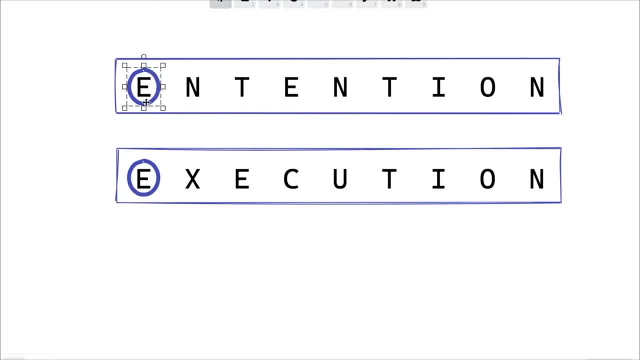 To E, so one operation has been performed, and then now these two have become equal. Now that these two have become equal, we can move this forward, and we can move this forward. So now we can simply recursively solve the problem for intention and execution. 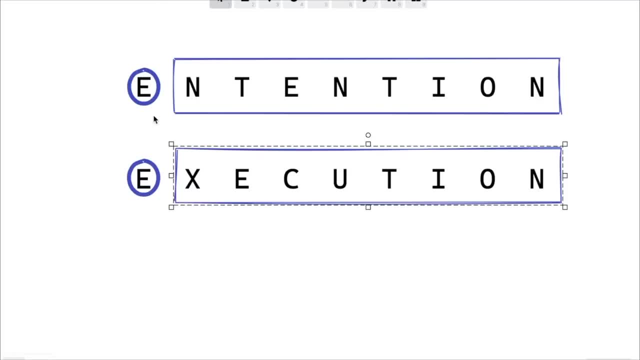 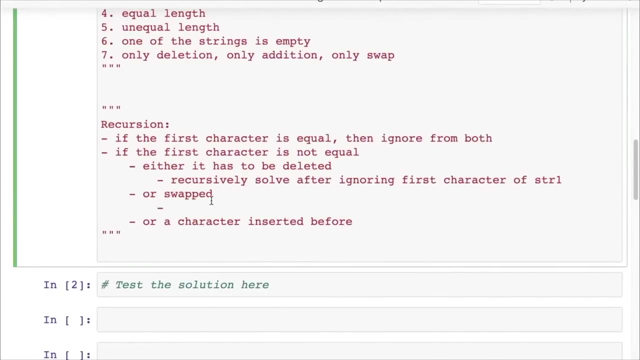 Find the minimum edit distance between the two and simply add one to it to get the number of steps required to change intention to execution by swapping the first character Right From I to E. So in this case you recursively solve after ignoring the first character of each right. 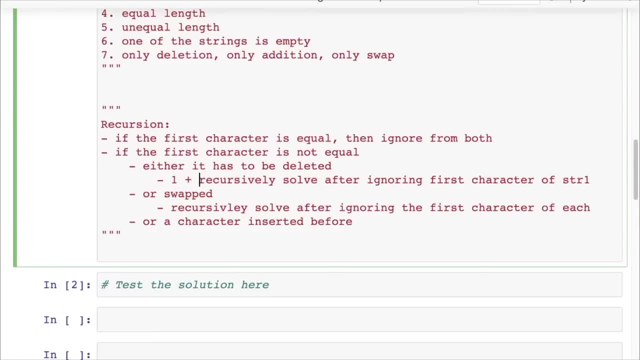 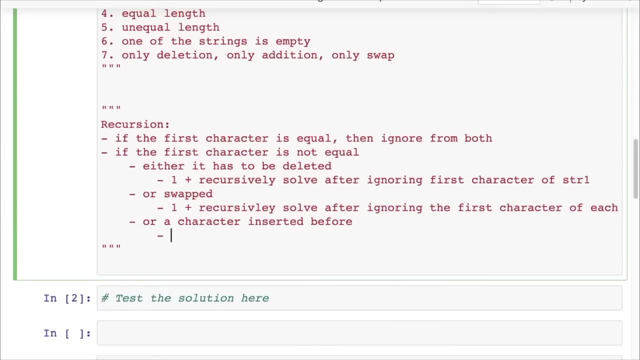 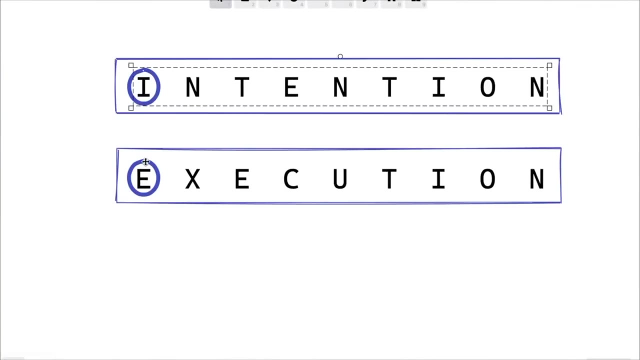 So it is one plus in both cases. it is one plus the recursive solution, after ignoring the first character of each, because the one operation is something that has been performed. Okay, Now the final case. the final case is: You have intention and execution. 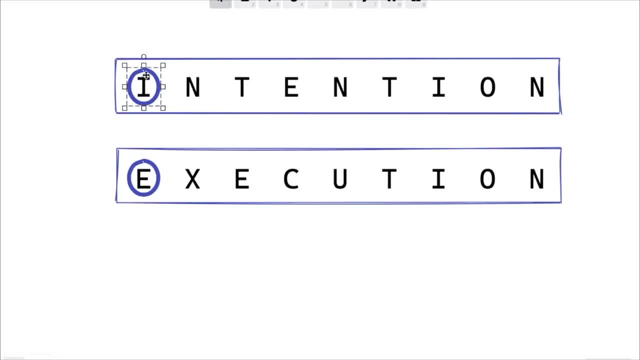 Now we decide that we are going to shift the string forward and we are going to include: we are going to introduce an E here, So we are going to introduce E here. So now what happens is the E is matching the E. now I has gone on to the first position. 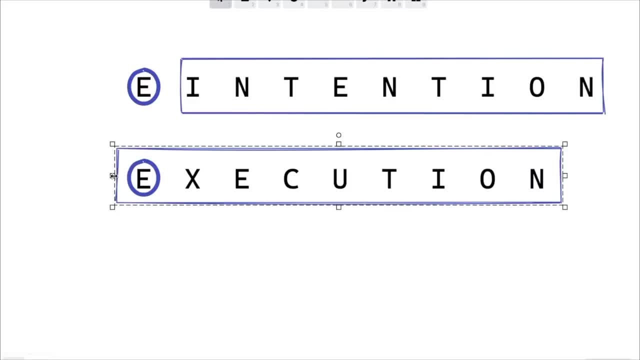 I has gone on to the next position here. So, effectively, what has happened is that we need to recursively solve the problem, or the original string intention And the second string with the first character removed, because we have inserted something before the first character in the first string. 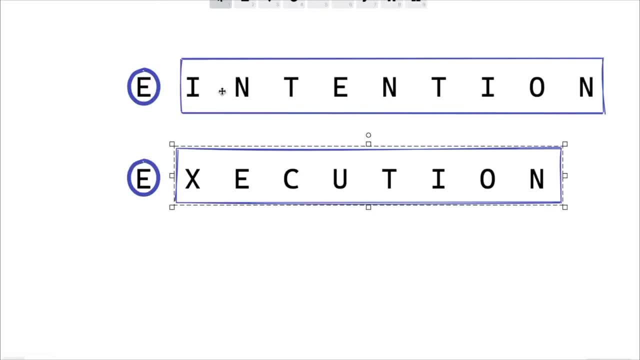 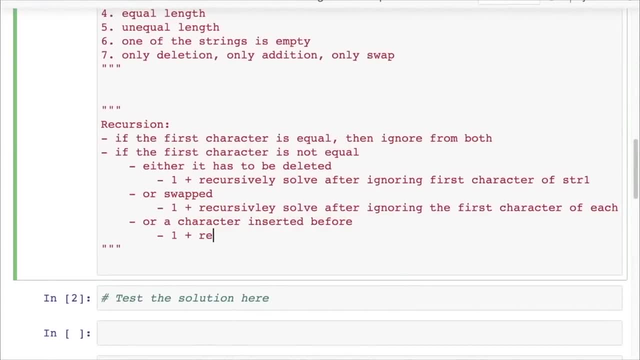 So that is going to match with the first character of the second string, And hence we simply need to recursively solve the problem for these two. In this case, what we are doing is the solution is one plus recursively solve, after ignoring the first character of STR two. 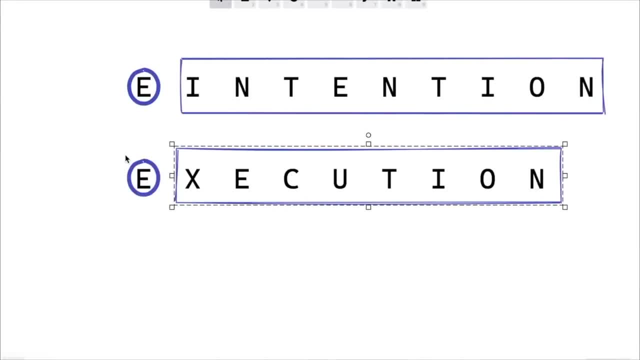 Okay, Sounds good. Looks like we've done that. Now what's the end solution going to look like? the end case, Remember, in recursion. this is all well and good, but at some point we are going to hit some kind of an end. 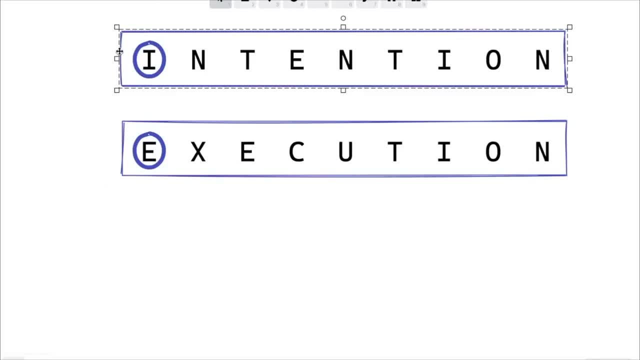 So let's see. let's see if we can define such an end scenario. So maybe let's say we have been performing recursion and then we ended up at a situation like this where there is nothing left in the second string, but you still have some characters left in the first string, right? 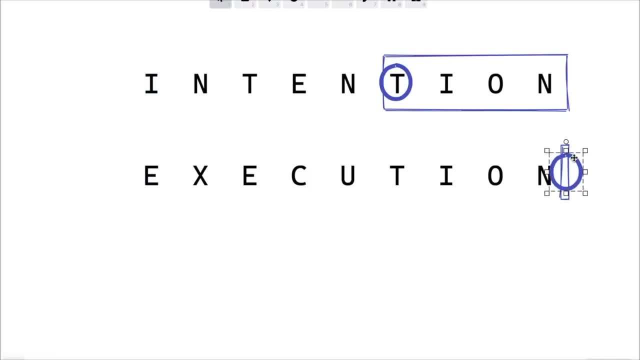 So you are at this position now And here this is gone. There's nothing left in the second string. So in this case, to change recursive, to change T I O N into the empty string, all we need to do is delete all four. 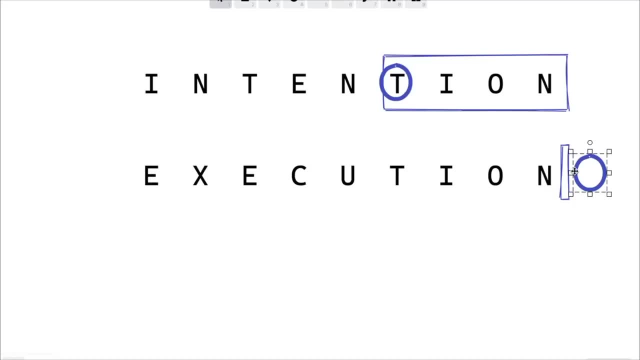 So if you have a few characters, if you, if the second string becomes empty and you simply find the number of remaining characters in the first string and delete them. So that is the number of operations. or the other possibility is that the second string still has some characters. 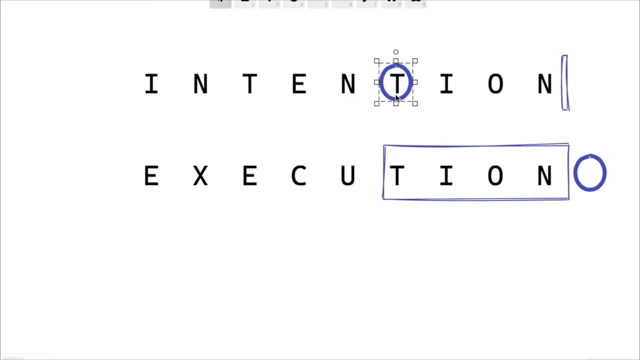 But you've run out of characters on the first string. So if you've run out of characters on the first string but the second string still has some characters, then in that case what you need to do, obviously, is you have the empty string and you need to take this, convert this empty string into T I O N. 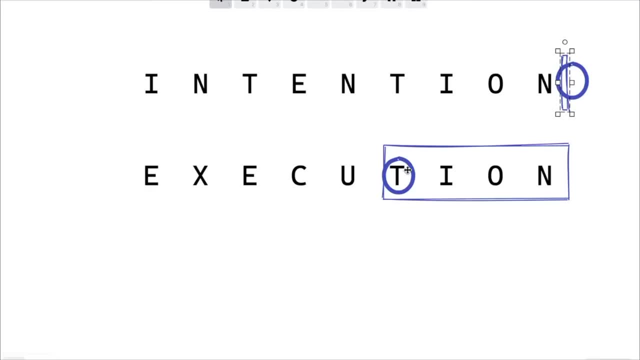 That is a recursive problem you're solving. So you that you can do by adding T I O N, Great. So you add T I O N and that is again going to be four steps, which is The number of characters remaining in the second string. 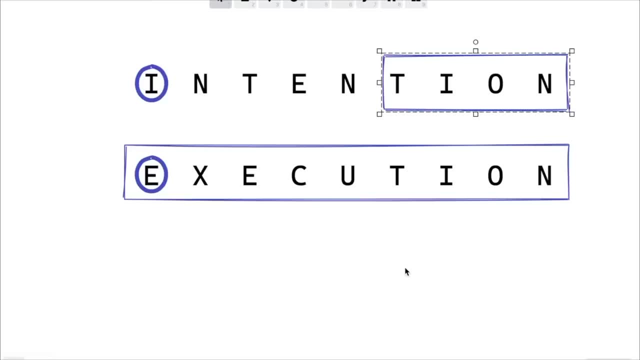 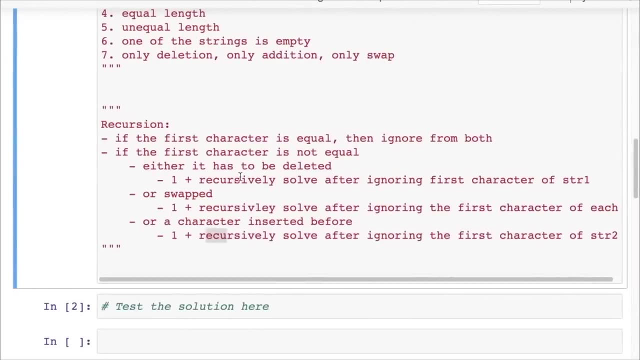 Okay, So these are the two end cases. Now, of course, if both of them are empty, then the answer is zero, But if either of them is empty, the answer is the number of remaining elements in the other one. Let's write the solution. 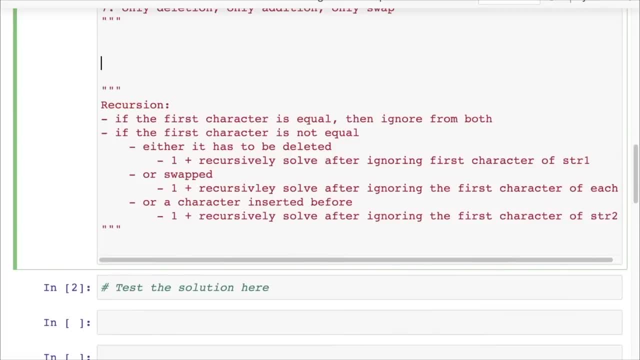 Have you figured out the solution? It took some time, but, again, this is not a very straightforward problem. So there are a few cases to figure out And while you are doing this, while you're identifying each case either, you can say it out loud. 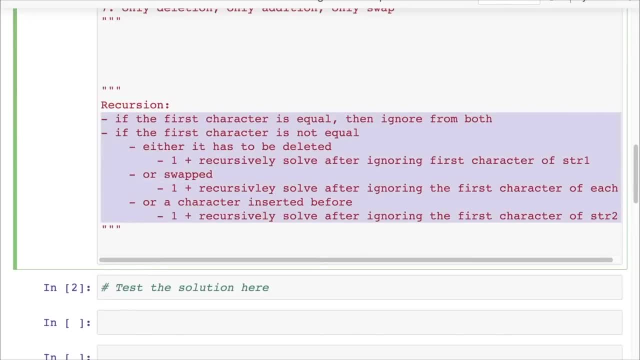 To the instructor, or you can write it as a comment, whatever you feel more convenient with, because the interviewer cannot see the work that you're doing on paper, So it's very important for you to be able to convey it, And that is why all this while in this course, we have been saying that you need to express the solution in simple words, because you need to tell the other person that you know the solution, and they should be able to understand what you're saying without looking at your work, without looking at the images that you've drawn. And that is why all this, while in this course, we have been saying that you need to express the solution in simple words, because you need to tell the other person that you know the solution and they should be able to understand what you're saying without looking at your work, without looking at the images that you've drawn. 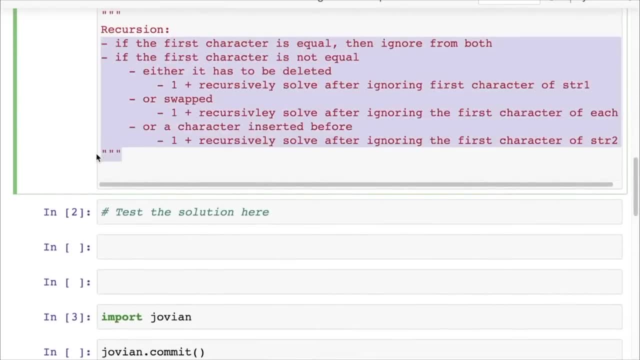 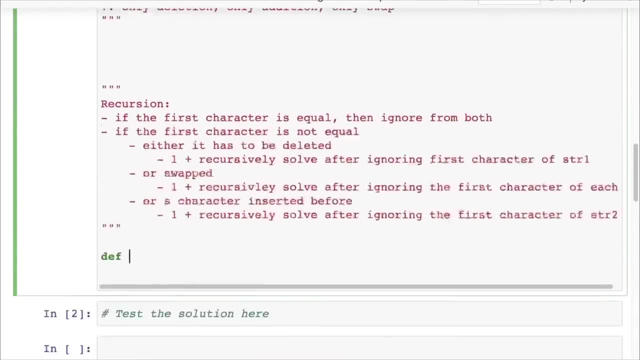 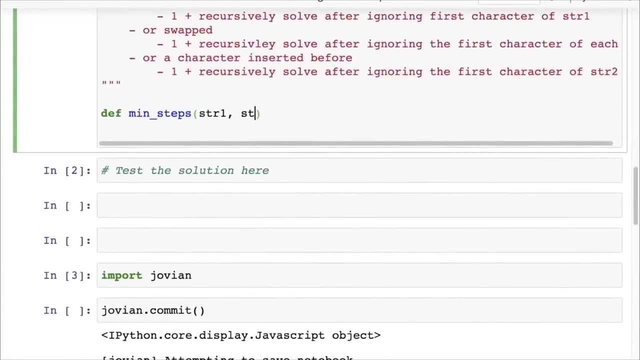 And a great way to do it is either by writing or by speaking, And a great way to do it is either by writing or by speaking. Let's define it then. def what's it called Min steps, and min steps is it takes STR one and STR two. 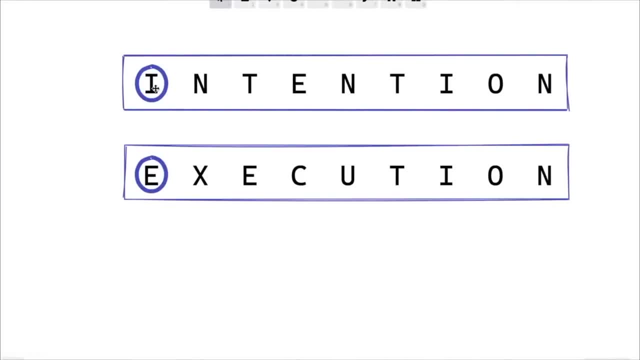 Great, Now we are doing recursion, and in recursion what we're tracking is the, the which character we are currently at. So we could be at The zero character, or the first character or the second character in string one, and we could be at the zero character, second character, first character, second character- in string two. right, 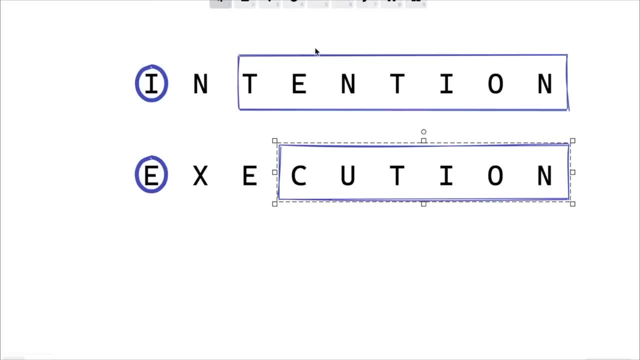 So the starting point of this window determines the sub string that we are solving the problem for. So ideally we, when we want to solve this problem for these two sub strings, we can simply pass those sub strings. but creating subs, sub list or sub strings as a cost because you have to copy those characters out. 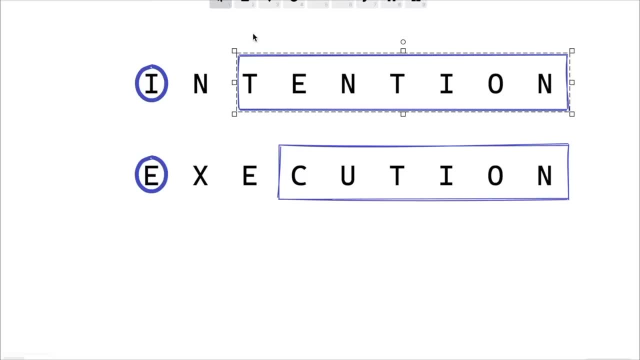 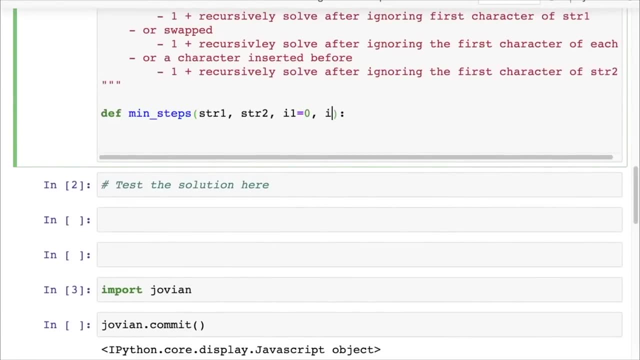 And then Allocate some memory and put them into a new place. So an easier way is to simply keep a pointer. So we will keep two pointers- I one and I two- and these will signify that we should be skipping while computing min steps. 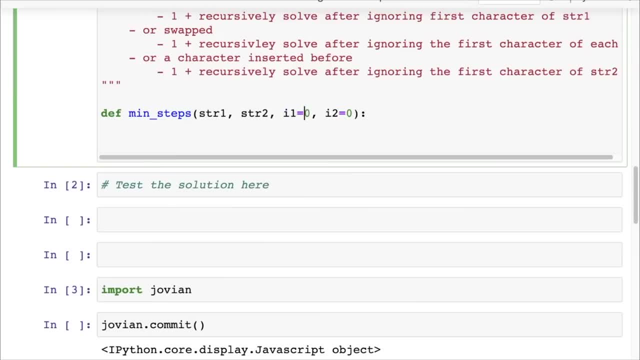 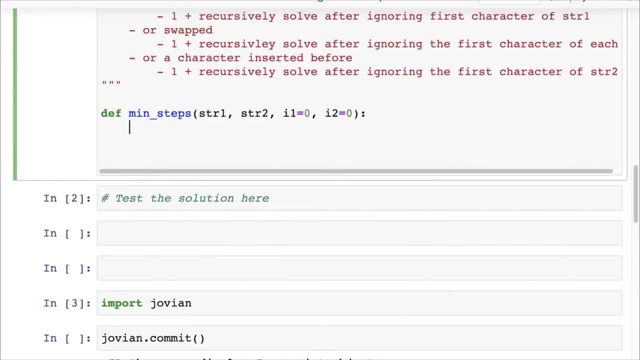 We should be skipping the first I one characters, or we should be starting from the I one index and we should be starting from the I tooth index for STR two. Okay, So in your window, if the I want to index, if the starting, if the 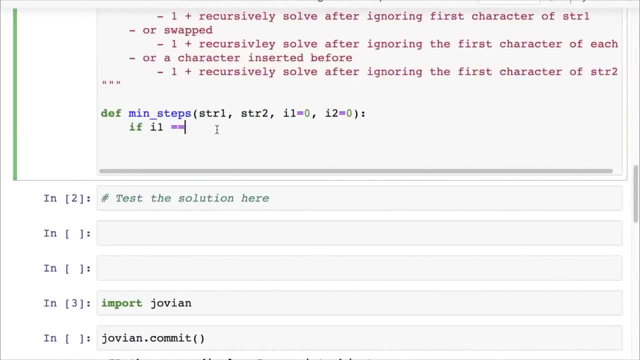 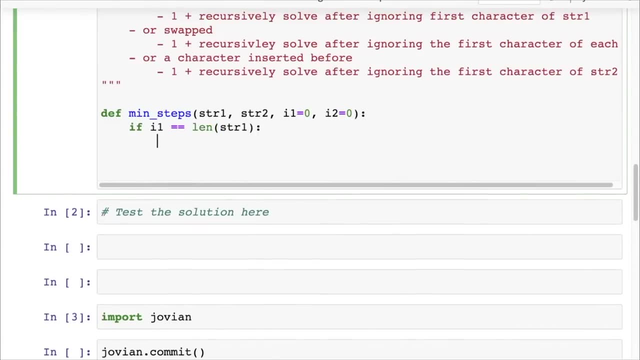 Starting index is equal to the length of string one. So this is the end case And remember the end case while coding is always written first. So if this is equal to length of STR one, then we have known, we have seen here that we need to perform these many additions. 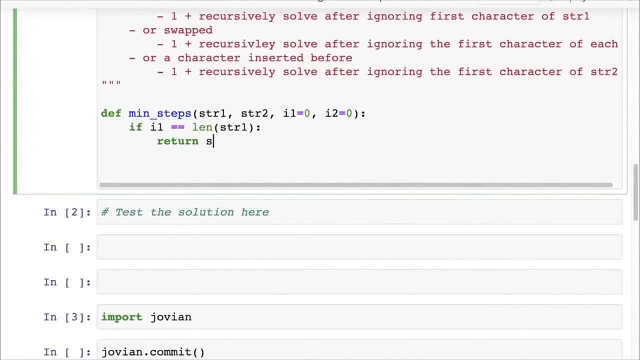 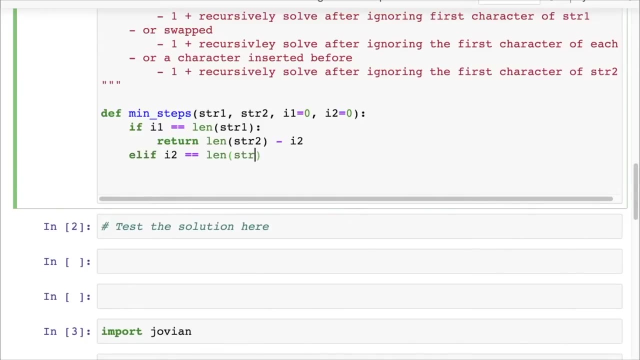 So we simply return, in this case STR, Len of STR two minus I two, right, And you can verify that. this is the amount, number of additions Required. And if, on the other hand, I two is equal to Len of STR two. 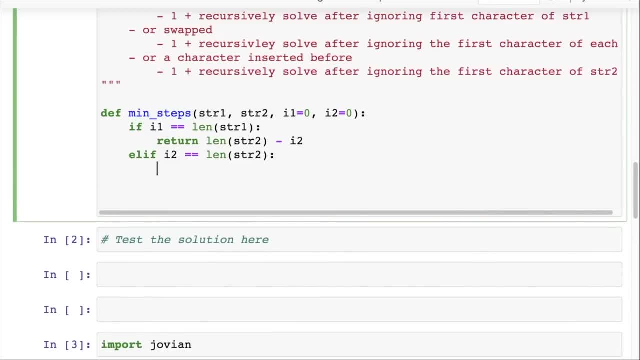 So, which means that you have exhausted the second string, but the first string still has some values left. So in this case you need to remove the, delete the return remaining values in the first string. So you just type: Len of STR one minus I one. 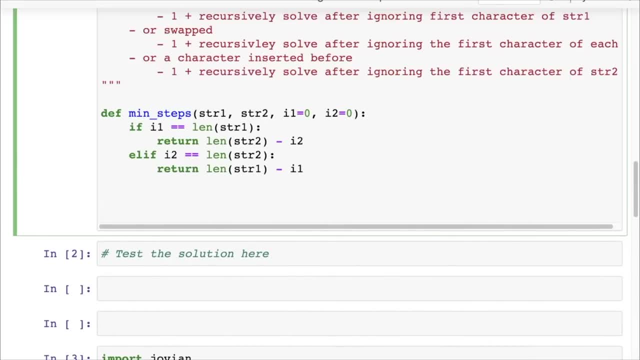 Great. So these, we have now solved the trivial cases. Now let's see LF: STR one of I one and STR two of I two, which means the first characters of each substring that we are working with, right? Remember, we are just using areas as a. we're just using indices as a optimization. 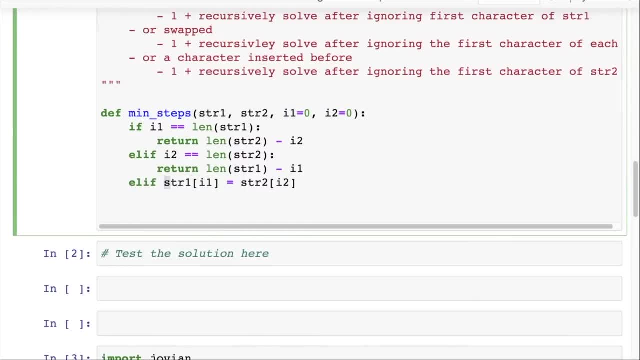 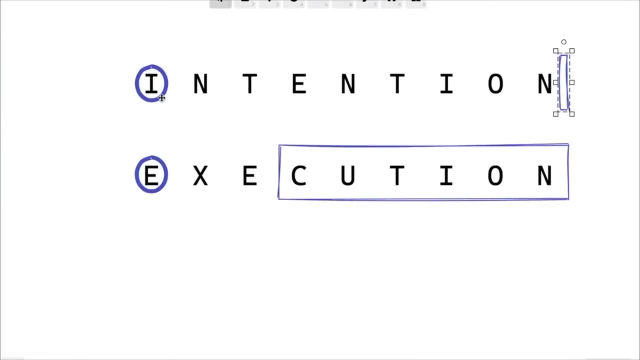 What we really want to work with a substring. So the first character of each substring, STR one of I one and STR two of I two, is equal. Now the first character is equal: E and I are equal. Then we simply ignore both and solve the problem for the remaining string. 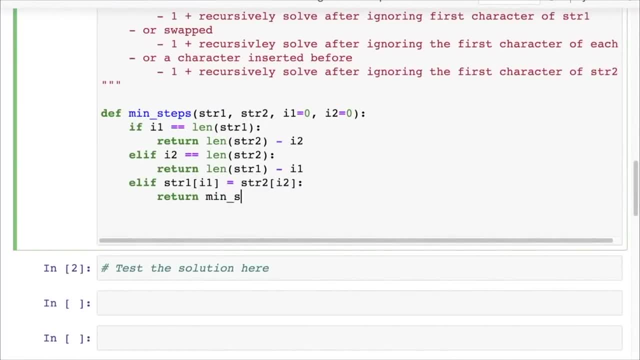 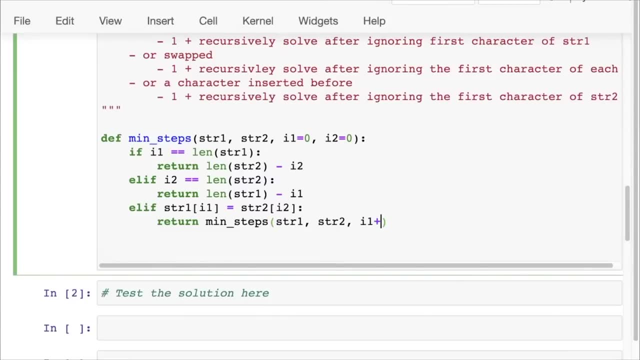 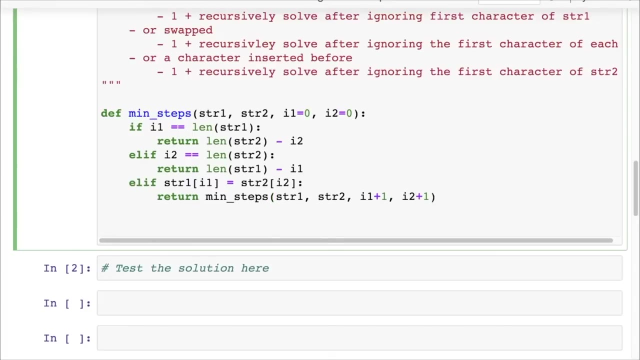 So we simply say: return main steps and we pass in STR one, we pass in STR two and then we simply pass in I one plus one here and we pass in I two plus one here. So what this is saying is that now we want to recursively solve the problem or a substring, starting at I plus I one plus one. 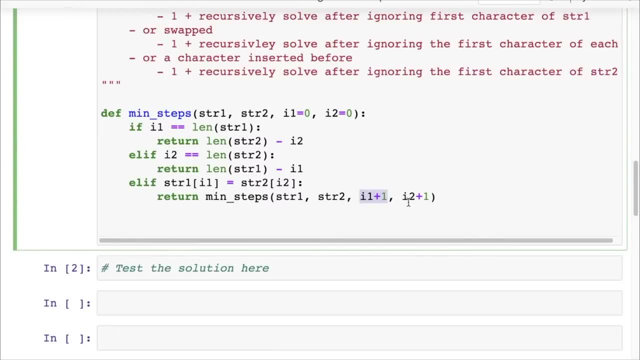 So we have ignored the first string of the current substring And, similarly, we have ignored the first character of the current substring or of the second string. Okay, So we ignore the first characters and that's it, And there are no steps required here. 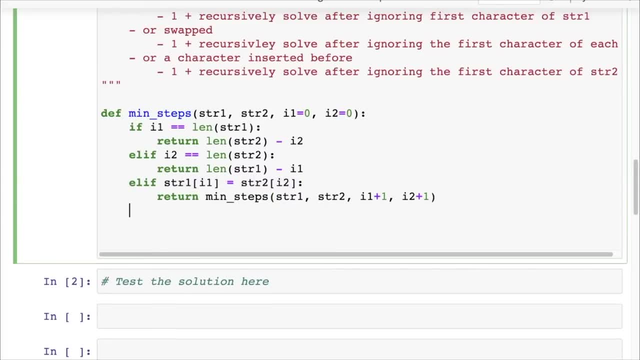 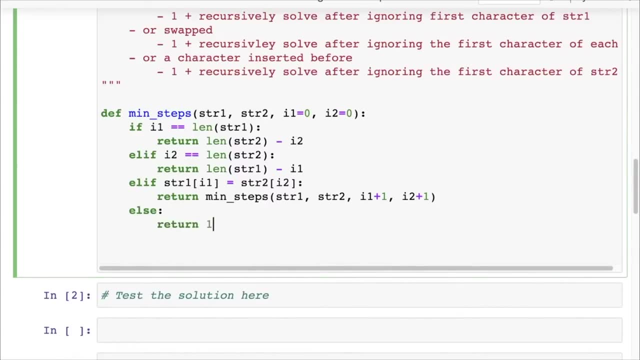 No operations required here right now, because the first characters are equal. Now, finally, this is the final case, else here we want to return one. So we have to perform one operation. either it is an insertion, deletion or swap- And what we can do is we can recursively check the cost or the number of minimum steps required for each case of insertion, deletion. 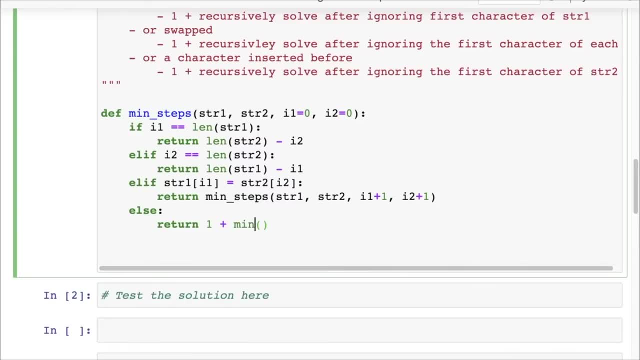 And Swapping and simply pick the minimum one And if, to do it, we add one, then we get the total minimum number of steps we need to perform for the entire list Right? So, again, recursion is very useful because you can simply assume that you have the function which solves the problem. 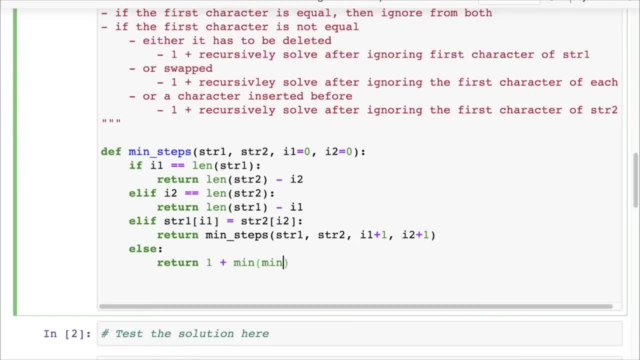 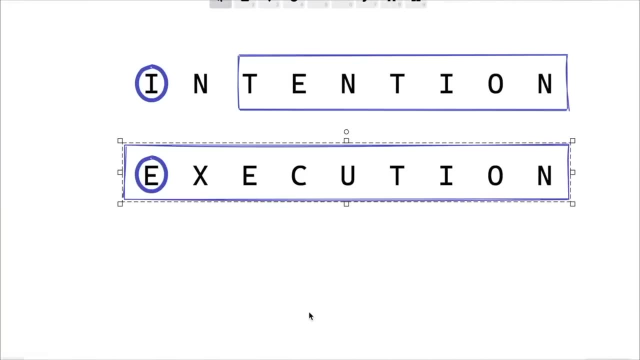 And you simply need to take the result of the sub problem and combine them. So we take the minimum of the first option is if the first character of STR one has to be deleted, which is, let's say, we choose to delete I. if we choose to delete I, then that means we have to solve the problem for these two. 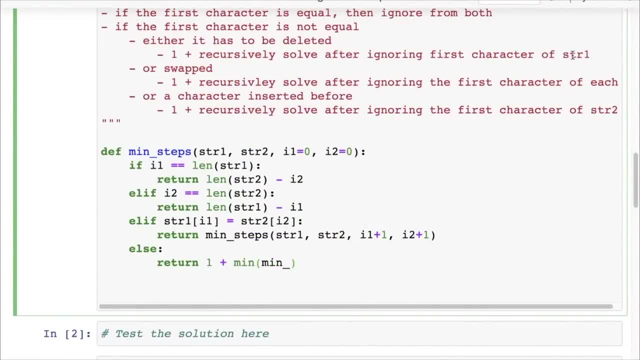 So we say one plus recursively, solve the problem after ignoring the first character of STR one. So we solve min steps for STR one, STR two. Now, since we have deleted the first character of STR one, we can skip ahead into the next, because we are solving the problem now for them, from starting from the next index. 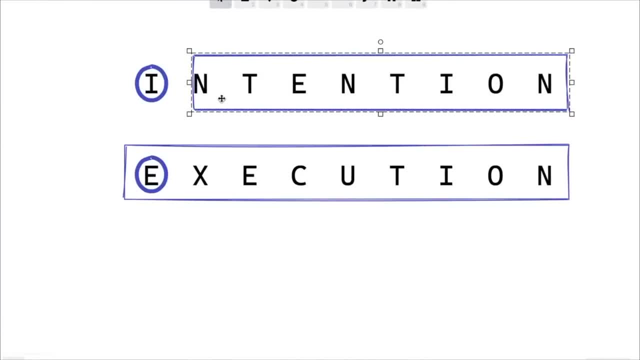 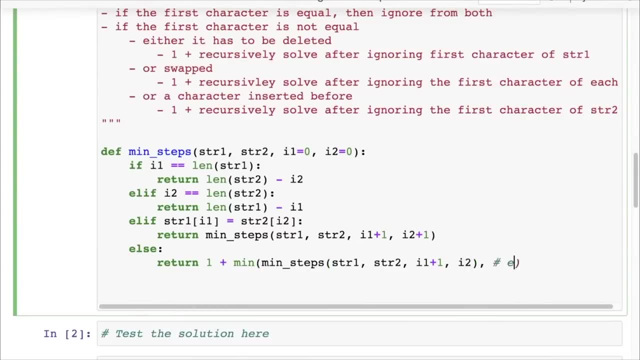 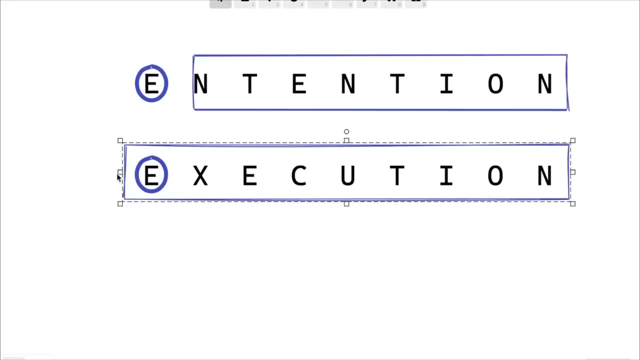 And I two remains the same right. So remember here we have not affected it, So we need to solve This problem recursively. So this was a case of deletion. Next, we have the option where you have swapped the first character. So we have taken E and we have converted that it. we have taken, I converted it into an E. if we did that, 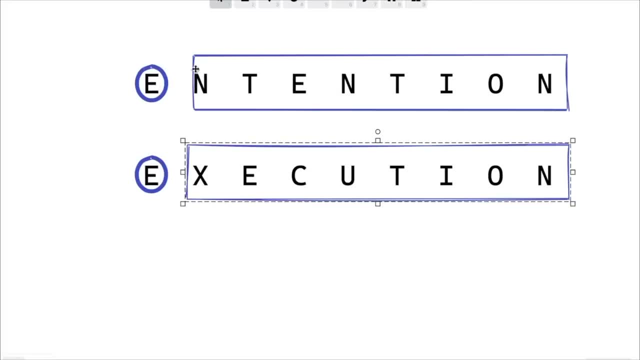 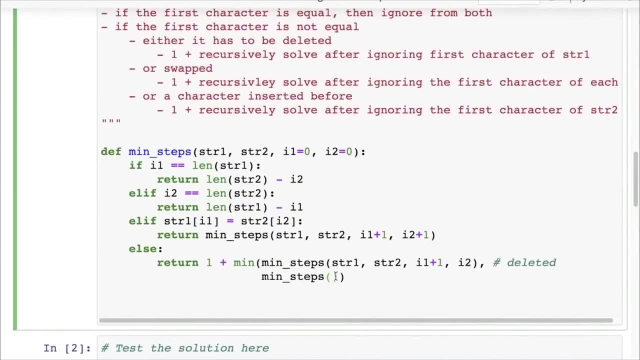 So then we can say that okay, now these two characters are matching. So now we can simply recursively solve the problem or the next character onwards, After Ignoring the current character. So this becomes STR: one plus STR, two plus I. one plus plus one plus I, two plus one rate. 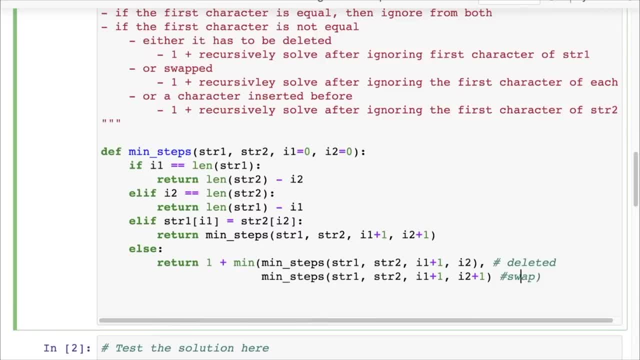 So this is swap or replace, and you might notice that this is: this turns out to be the same recursive call as this, except that we will add one to it because we have done the swap. And finally, if you Are adding, 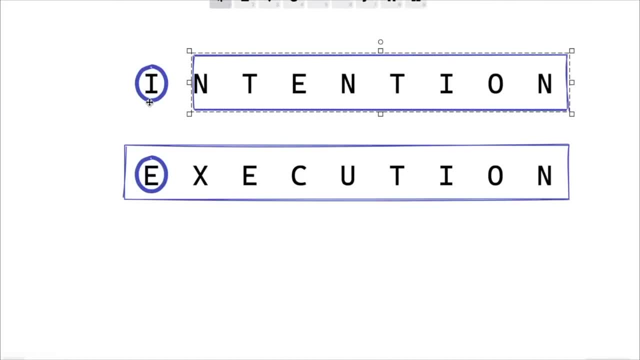 So if you're at inserting, so finally, if you're inserting here something, So if you are inserting E here, let's say So. in this case, what we'll do is now we'll recursively solve the problem for intention and execution without the E in front. 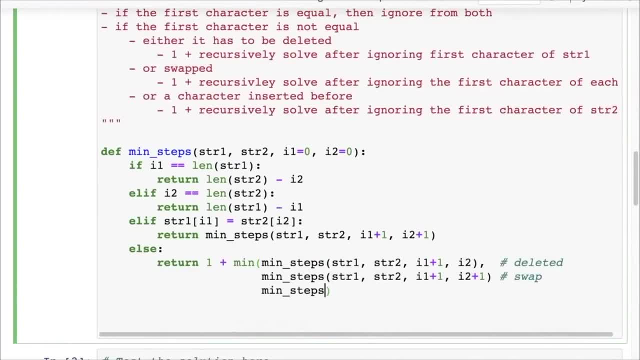 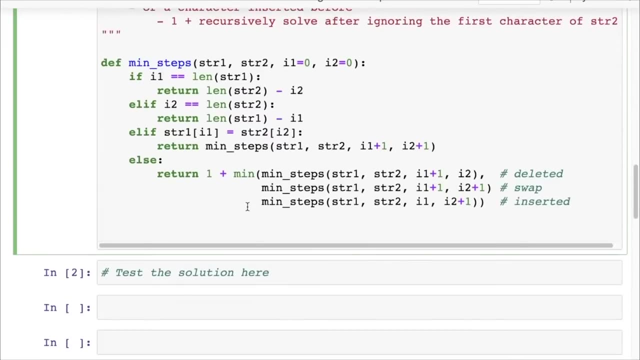 So we skip the first character of the second string. So we have min steps: STR one, STR Two, I one and I two plus one. So this is rather nice and symmetric, And that's it. So this should be it. 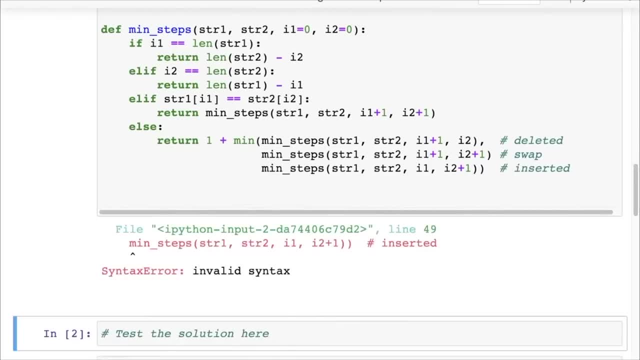 Let's run this. Okay. There is a syntax error here, That's perfectly fine. There needs to be a comma here, That's fine too. I make a lot of syntax errors all the time And, of course, off by one error. 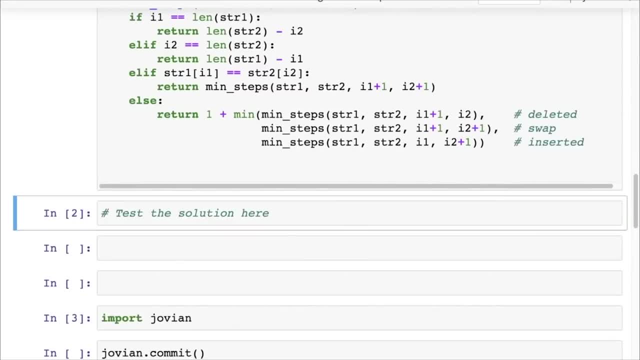 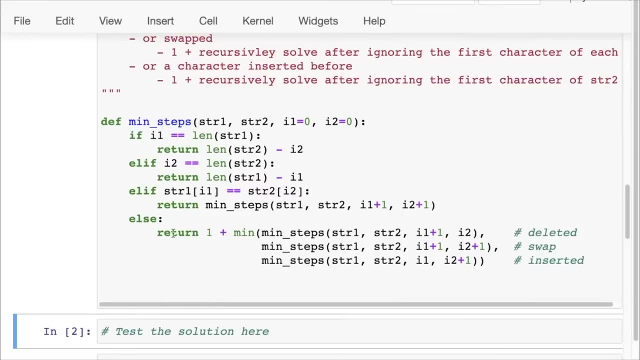 I'm sure there are a few, but yeah, this is the minimum number of steps and this is our recursive function. Not too bad: two, four, six, around eight lines of code. And let's test out some of the test cases here. 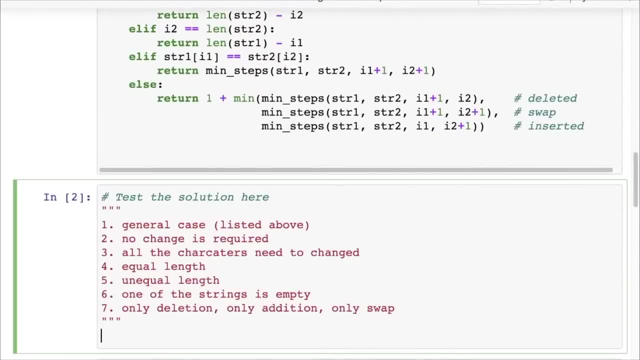 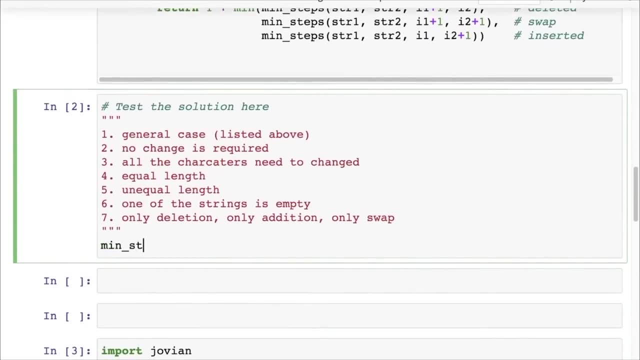 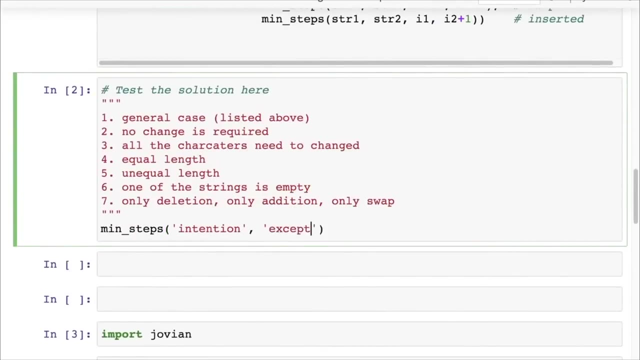 I'm just going to copy the test cases out here below and let's try as a general case, which is intention and exception. So let's see min steps. Okay, So I give it five, intention and exception. It says five, four. 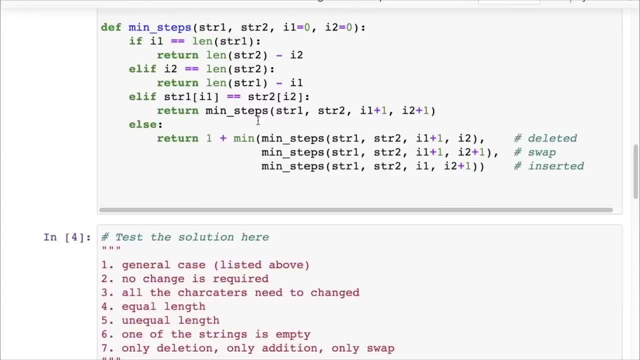 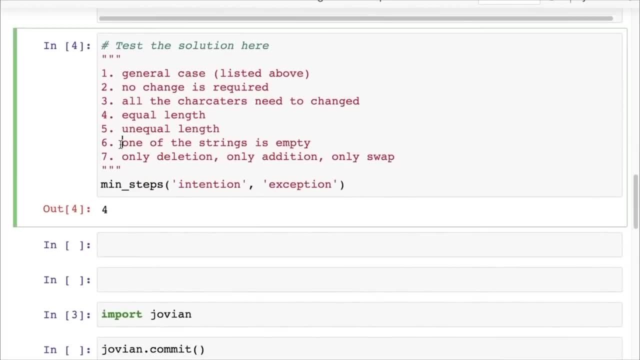 Okay, Why does it say four? Maybe let's test. Let's test a more simpler case first. which is one of the strings being empty? Let's say we have intention, and another things is empty. We will need to delete a, let's just say int, and one of the strings is empty. 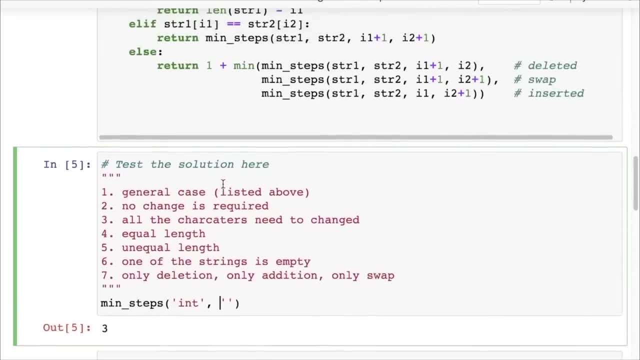 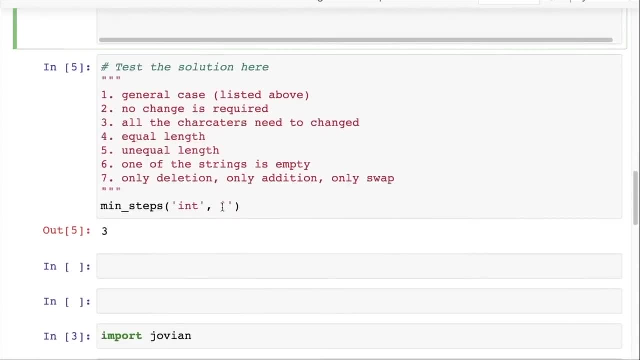 This looks fine. We will need to delete all three of these And that in some way tests out this case where- or, sorry, tests out the second case where the second string is empty. Now we can test this case. in this case Also, the. in this case also, the solution is three great looks fine. 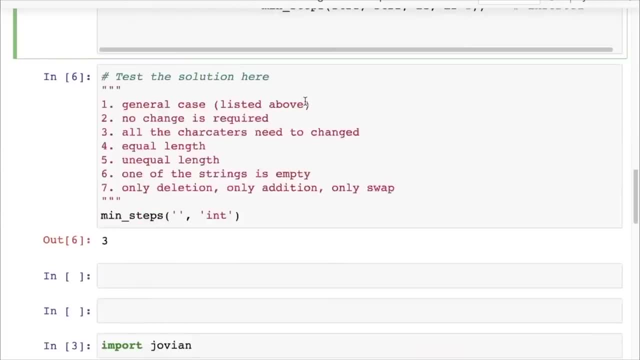 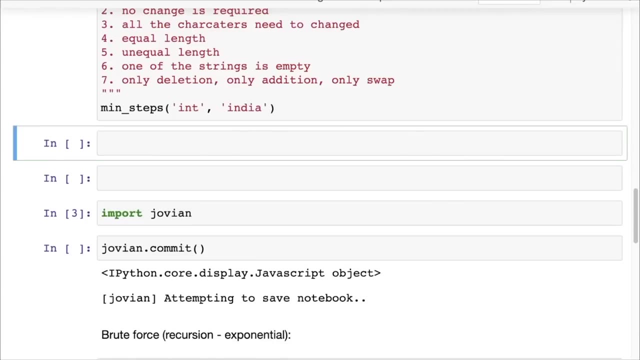 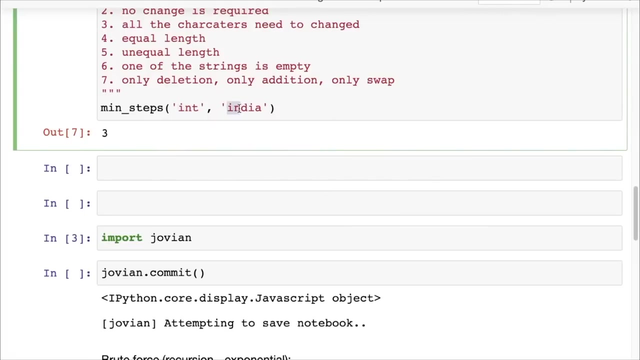 Let's test this case where STR one- I one and STR two I two are equal. So if you have integer and let's say you have India, so I N, I N would be the same. So these would get skipped. and here is where the recursion would kick in. 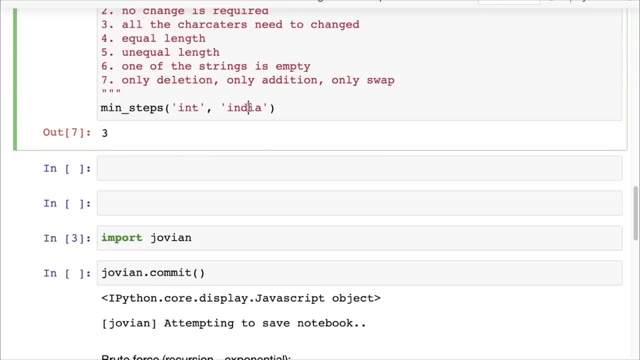 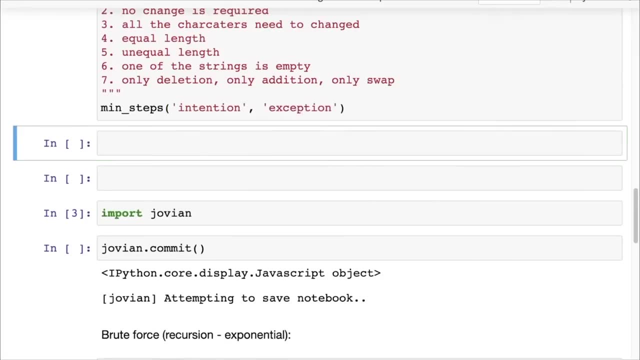 So T would have to be changed to D, and then you would have to add I and T. Okay, That looks fine too, And let's check intention and exception Once again. I don't know what's there Wrong here? Let's see. 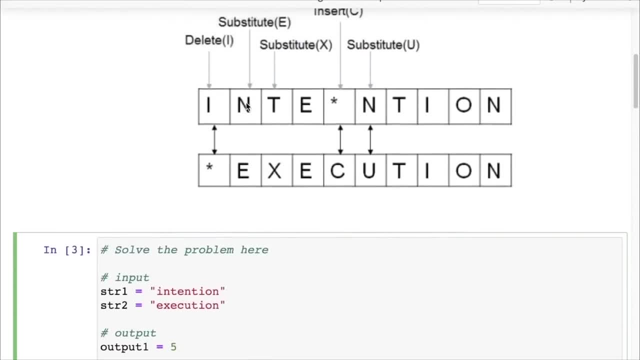 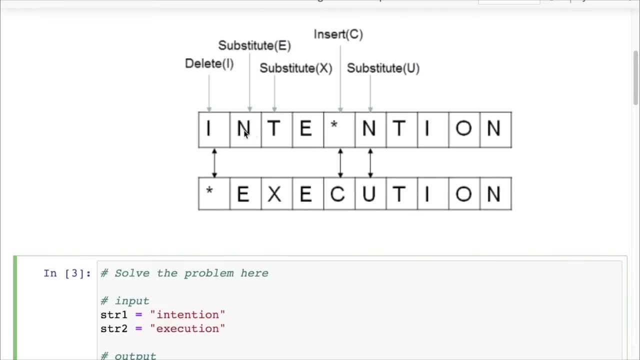 So is it possible to do it with four? I don't know. It's maybe possible to do it with just four inches. If you change I, you delete I, and then you delete N and then you delete T, delete. I substitute these two: 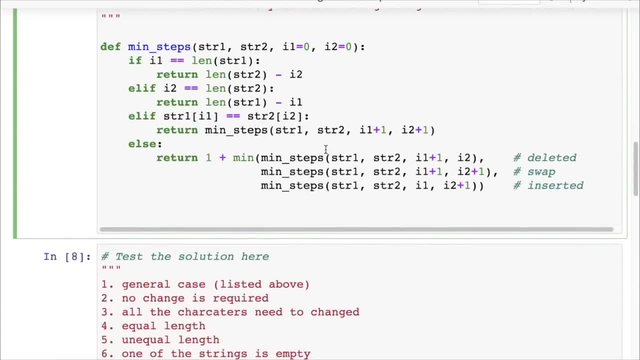 I don't think it is possible with just four changes, So there's probably an issue. Okay, Okay, Okay, Okay, Okay, Okay, Okay. I don't know what's wrong here. It's possible. I may have made a mistake here. 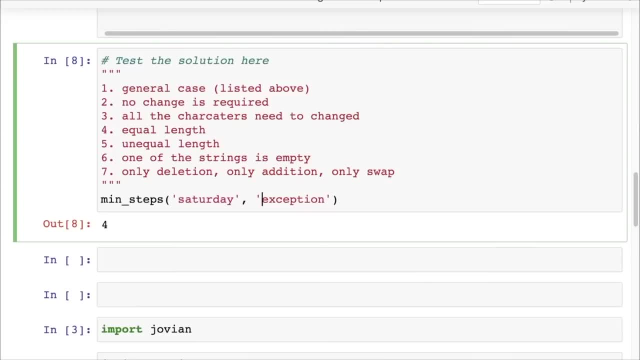 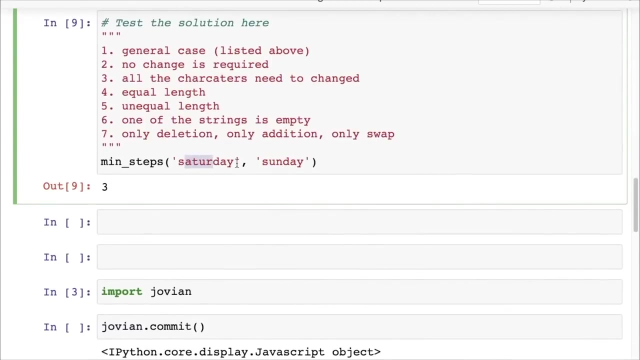 Let me try another: Saturday and Sunday. Okay, So Saturday SATUR needs to be changed to Sunday S U N. now S is the same, So ATUR needs to be changed to U N, so U remains the same. Now, if we can, what we can do is we can probably delete a, delete P and 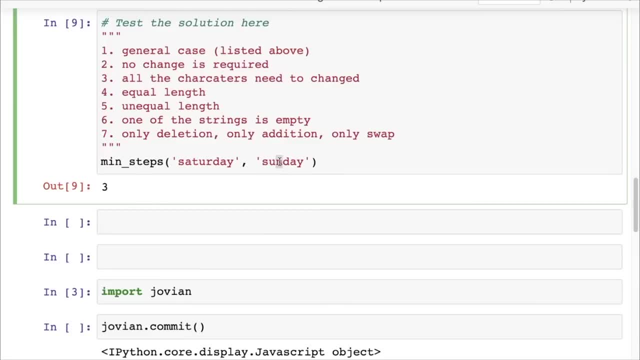 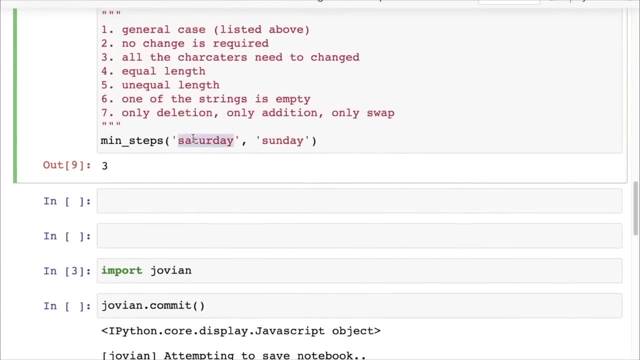 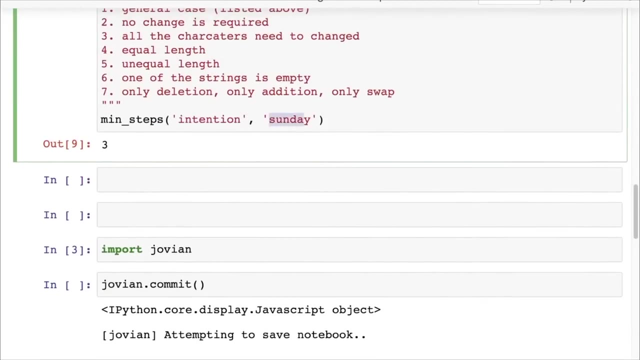 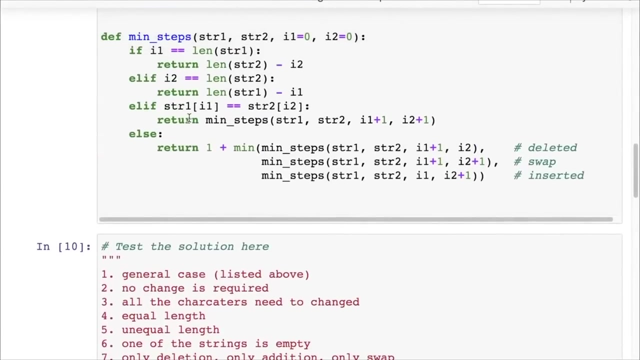 take: replace R with N. So this seems to be fine. All right, So we'll probably, unless I'm not seeing this. so you have in tension and you have, except, unless I'm not seeing something, it seems like We may have made a mistake. 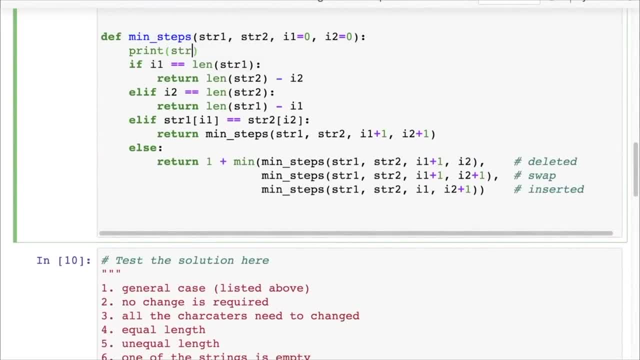 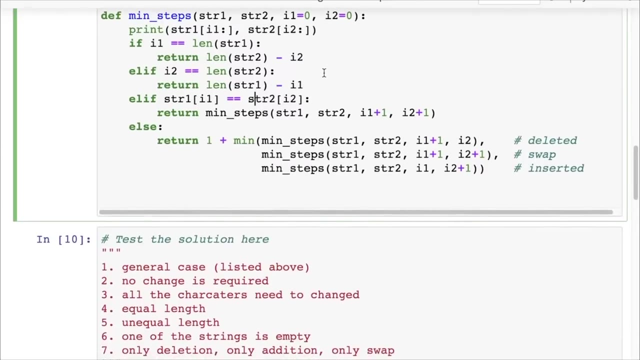 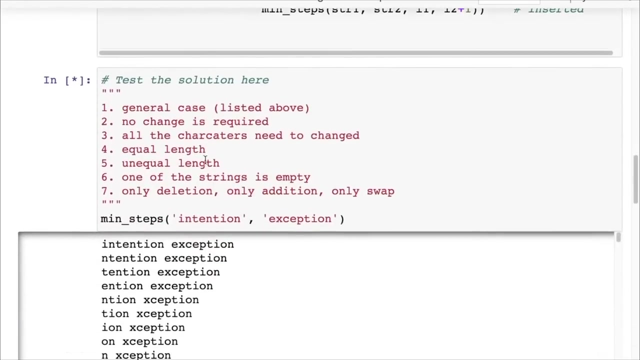 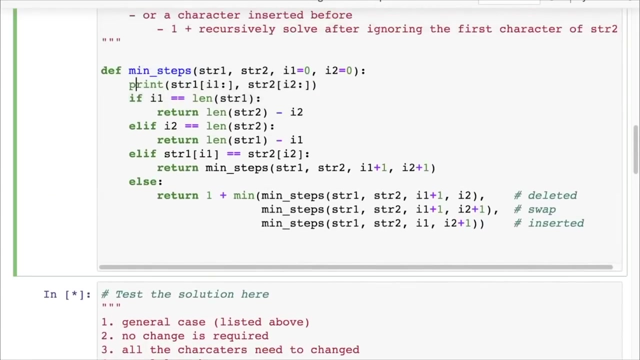 One. one thing we could do is we can simply print out the strings that we are checking. So let's see: STR one is Ivan onwards and STR two is I two onwards. We are first checking intention and exception, Then we check. Let's also print the result here. 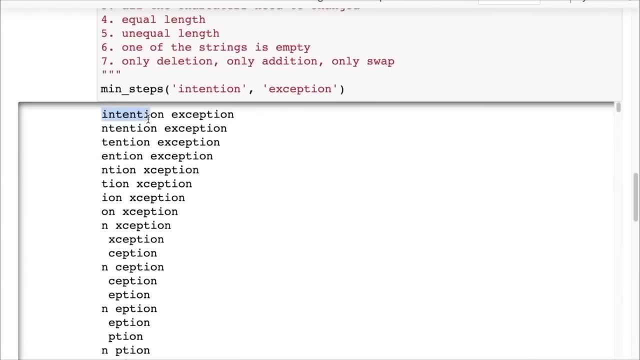 Okay. So at this point I would probably look through the loop here and see if the see, if it is correct and coming properly. So you have intention exception: First we delete I, then we delete, and then we delete, and then we delete P, then we delete. 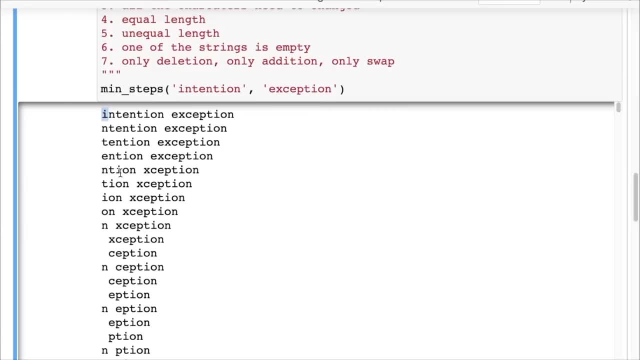 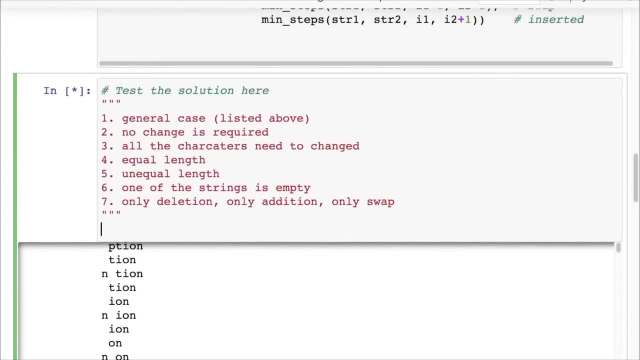 Okay, Then we compare E and E, So then we come back to And an exception and so on. I think we'll have this. might take some time to fix. We'll come back to intention and exception, but supposing we've solved the 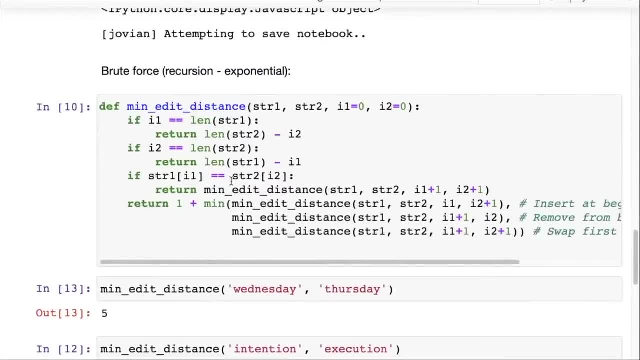 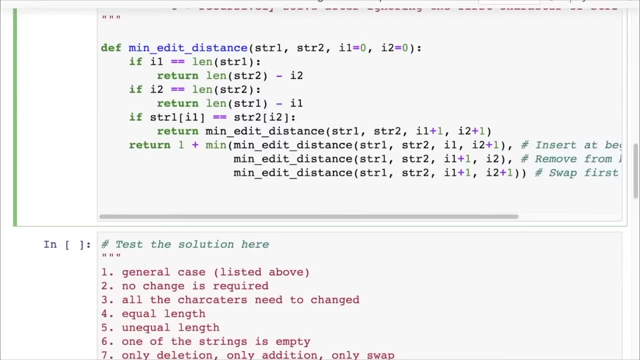 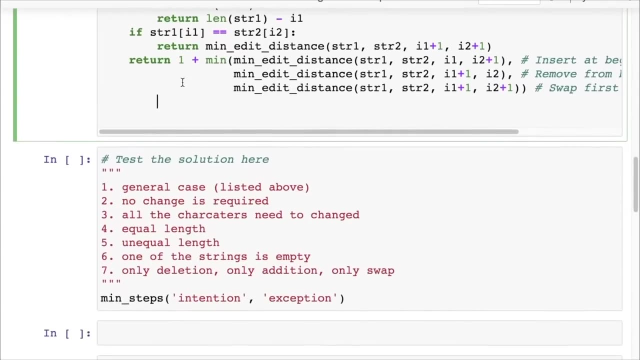 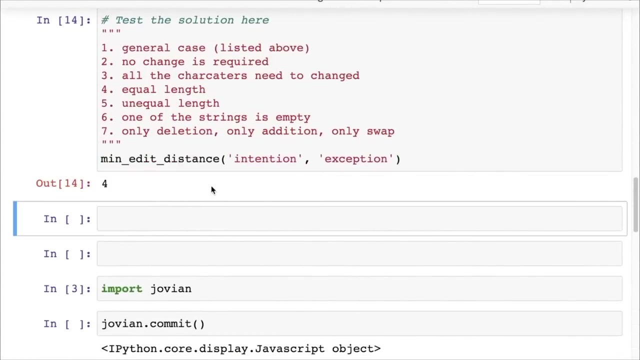 supposing we've written the recursive solution correctly And I do have the recursive solution here, Let me just grab that and put that in here. Let's see what's different. Okay, probably the answer is four, because I'm still getting four, but supposing we have the recursive solution here. 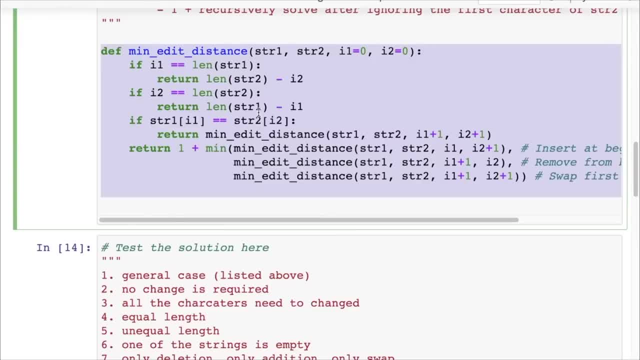 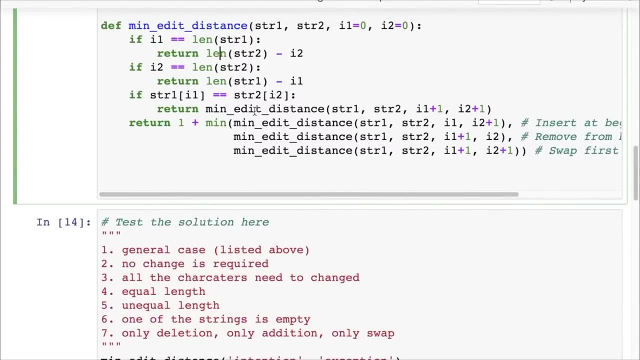 So we have main edit distance. This is the recursive solution. And now what you need to do is you need to find out the complexity of the recursive solution. in order to find the complexity of the recursive solution, What we can do is Simply look at the recursive calls. in the worst case, 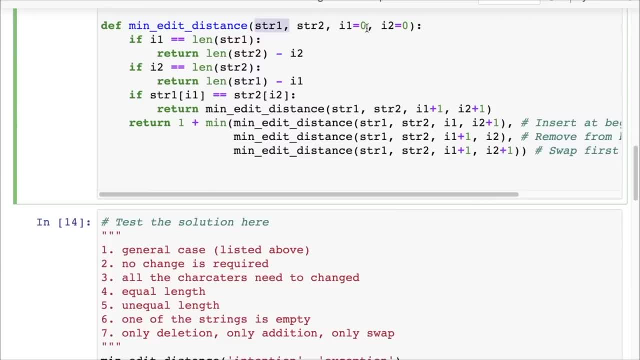 So how you start out is you start out with a string of length and one, let's say, and a string of length and two. we have one string of length and one and one string of length and two. then you call either: You call this main edit distance, with I one plus one and I two plus one, the STR one and STR two. you call them with I one plus one and I two plus one. 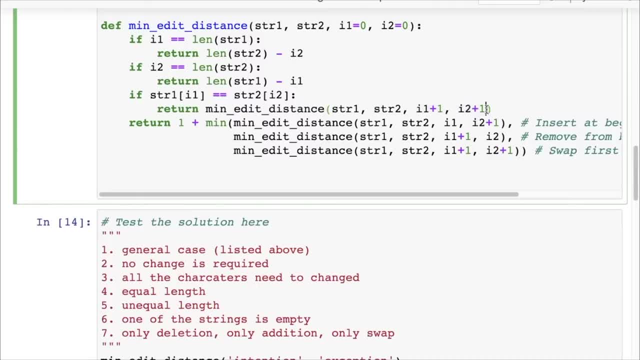 So that's one possibility. Oh, You will just have to choose that string to match up or not. You call three recursive calls. Now one that goes have called is the good case where these two match up. So we want to look at the worst case where these two things don't match up. 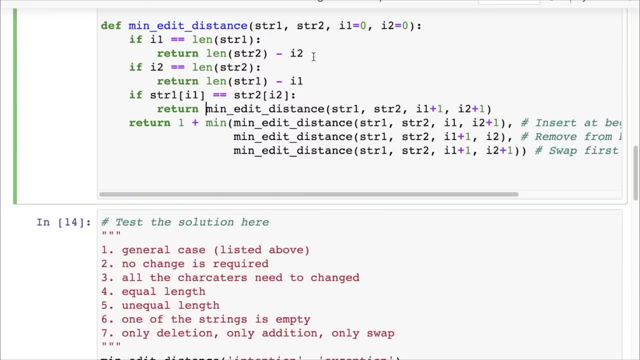 So in that case you make three recursive calls. right, So you make three recursive calls and in each recursive call you are then going to reduce the problem size by one. So you're either going to decrease I two or you're either going to decrease the size of the first string or you're going to decrease the size of the second string. 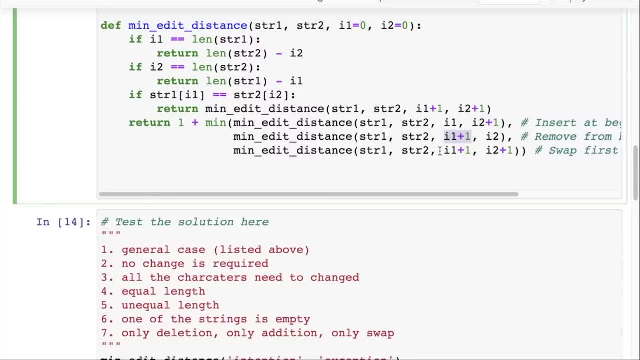 Okay, Or you're going to decrease the size of all- Okay, Okay, Okay- size of the second string, or you're going to decrease the sizes of both strings, right? So just to keep things simple, let's assume that in all three we are decreasing the size. 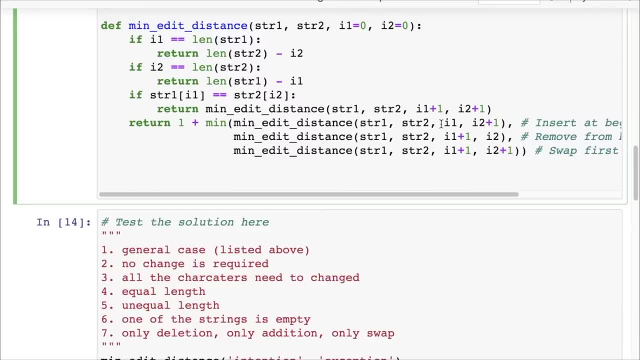 of either one of the strings by one. So we are decreasing the total problem size, which is N one plus N two, by one right. So the number of levels of recursion is going to be the total number of total length of each of the two strings. 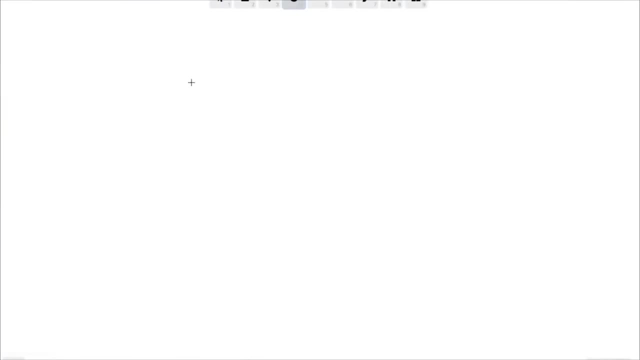 So let's maybe just draw that graph here as well. So let's take this. but here you have N one comma N two, So let's assume these are the lengths of the two strings Now, N one plus N two. what happens to it? 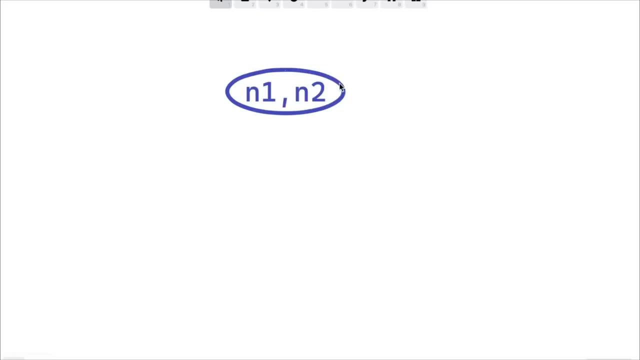 It decreases the length of each of the two strings. What happens to it is that this N one plus N two calls three recursive functions. So there are three recursive functions. So let's just draw those three recursive functions. So we have those three recursive functions here. 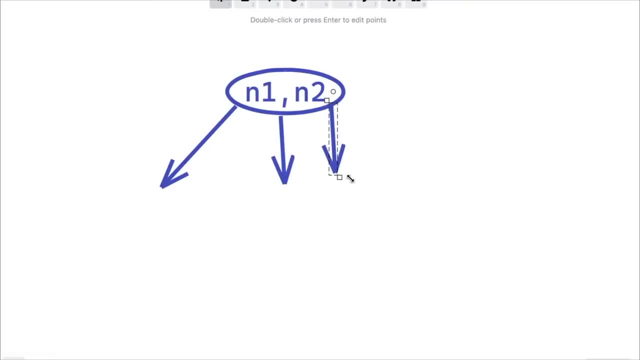 Let's take this too. And then those in those three recursive functions. what we have is either you reduce- either you reduce the size of the first string, or you reduce the size of the second string, or you reduce the size of both strings. 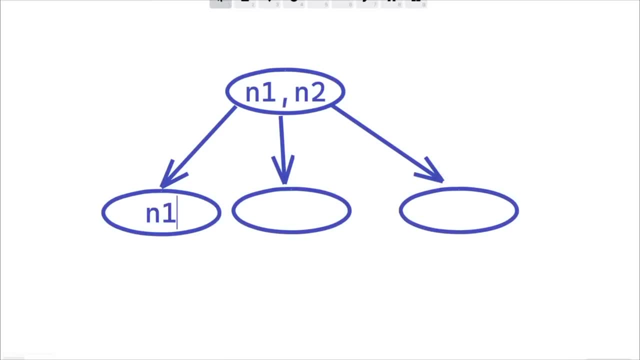 So either you end up with N one minus one and N two- And let's reduce the size of that- Or we end up with N one and N two minus one, or we end up with N one minus one and N two minus one. 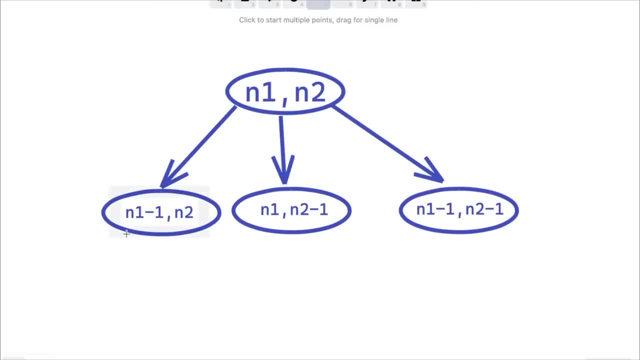 Okay, So these are the three recursive calls that we're doing, and then each of these will once again make three more recursive Calls, and so on. Now, what is the depth- overall depth of this recursive call? now, because we can see that each time the 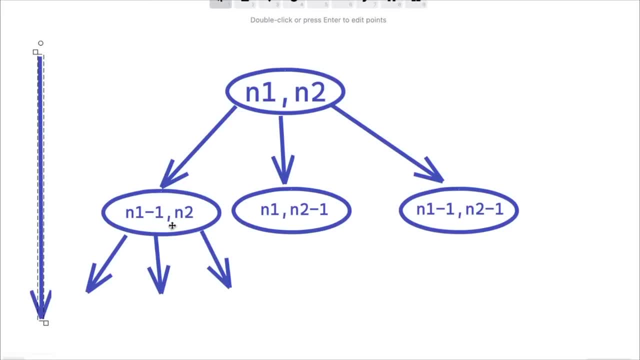 size of the problem reduces by one. So if the size of problem is N one by plus N two, in this case it reduces by one, in this case is reduces by one, And in this case it reduces by two. but for simplification let's say it reduces by one here. 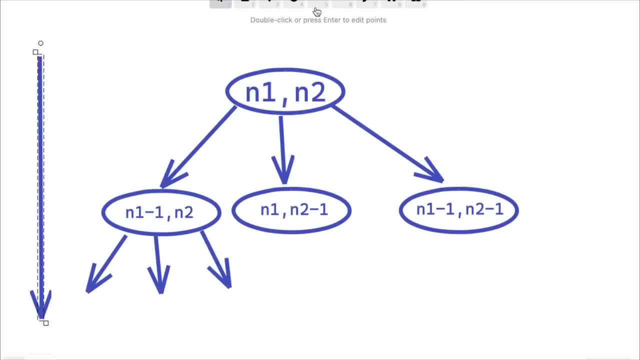 So the total size of the problem, the total number of levels in this tree is going Going to be, and one plus into, so you have three problems in the first layer. The second layer will have three square problems. The third layer will have three cube problems. the three times, three times three. 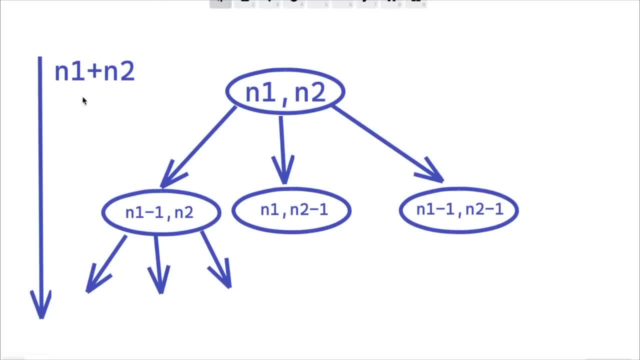 And similarly you can go ahead and you will find that at the last layer you'll have three to the power and blown plus N, two minus one layers right. And if you then add together all the layers, what you end up with is that total, total number of problems is straight. 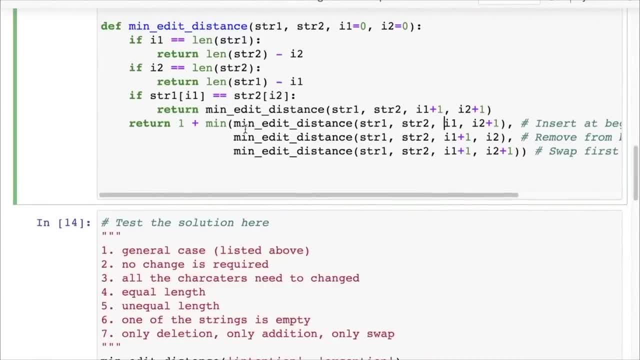 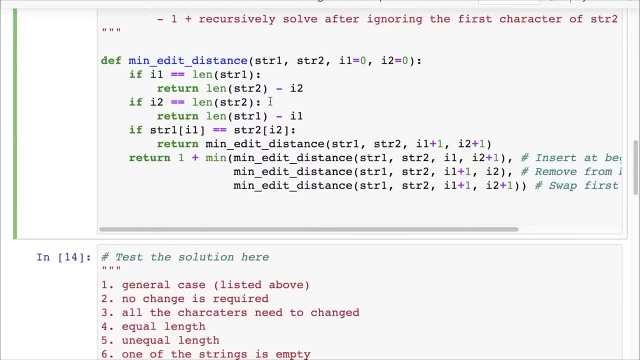 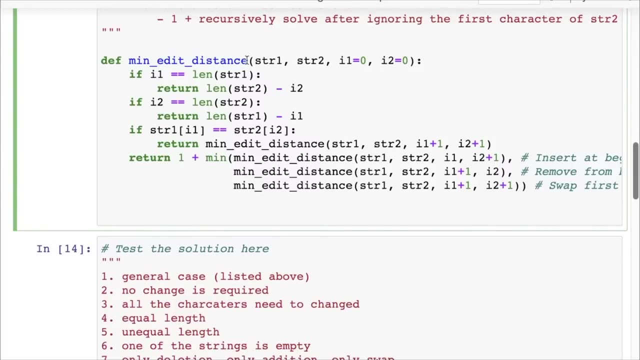 to the power N one plus N two, right. So you have a total of three to the power N one plus N two sub problems that you end up creating And because of that you have the complexity: three to the power of N one plus N two, in this case. 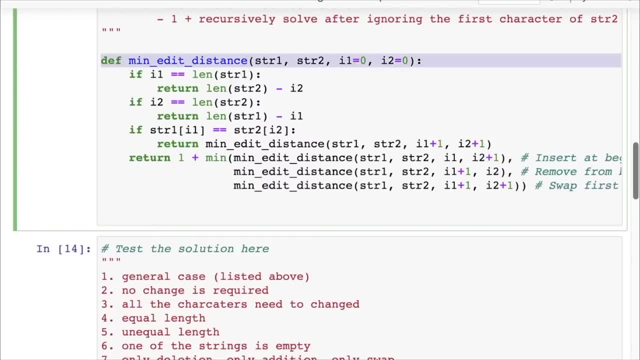 Okay, So that's. that's the complexity. So here we have a recursive solution and then we have the complexity of the recursive solution, which is exponential, three, three, three, to the power of N one. Now, at this point it will make sense to add memoization. 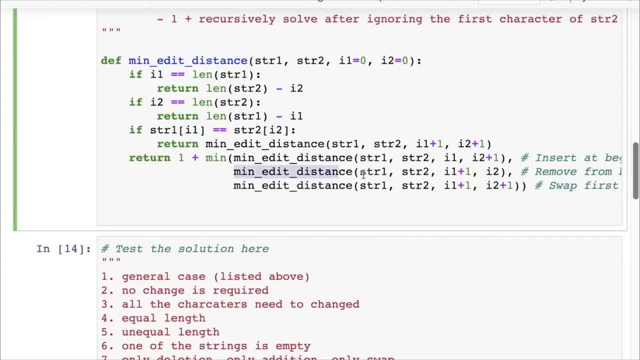 So whenever you see recursive solutions and you see repeated problems- for example here itself, you can see a repeated problem And then you can see that this problem will get repeated inside this problem and inside this problem too. So there are a lot of repetitions and all we need to do is remove some of those repetitions and to remove those. 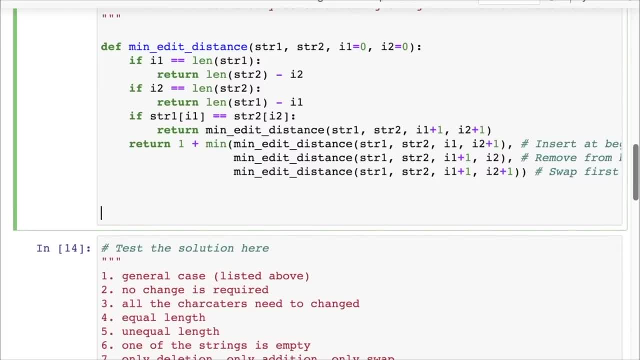 repetitions, we can use memoization. So what happens in the memo solution? It is exactly the same as the recursive solution. but before doing any computation We check a memo, we check a dictionary- If we already have the solution for the changing variables, which is I one and I two. 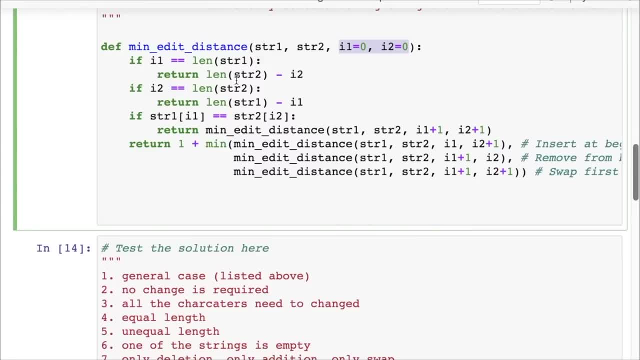 And if we have those? if we have those solutions, what we need to do is just return them directly. If we do not have those solutions, we need to compute the solutions, put them in the memo and then return the value from the memo. 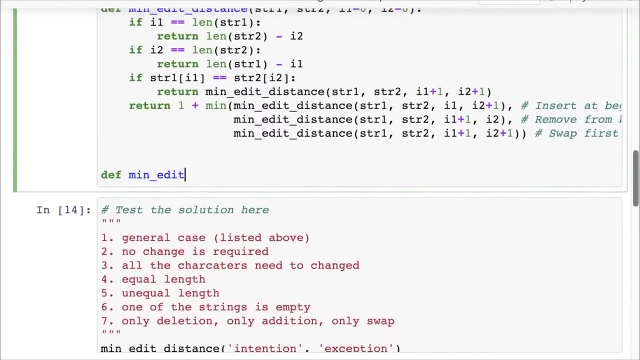 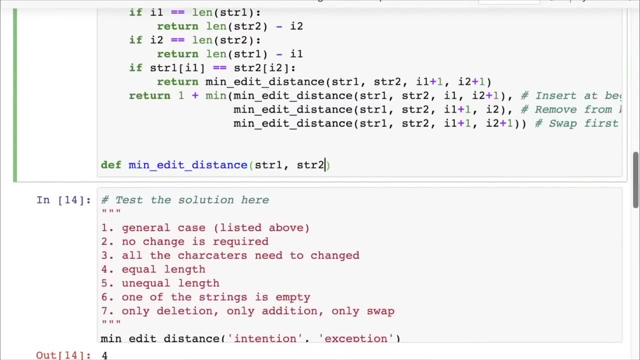 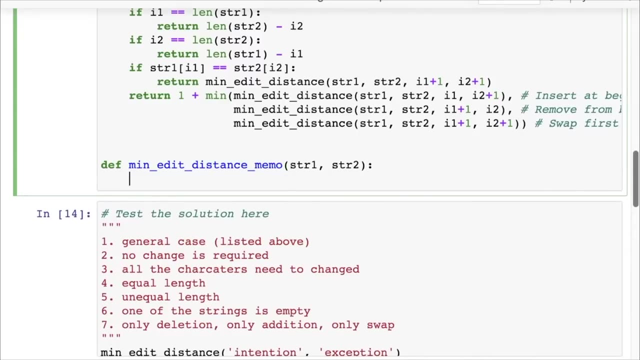 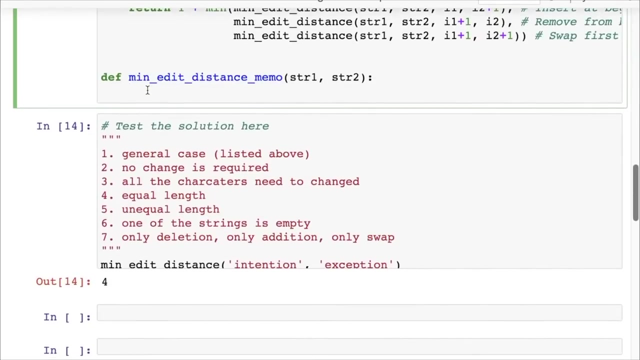 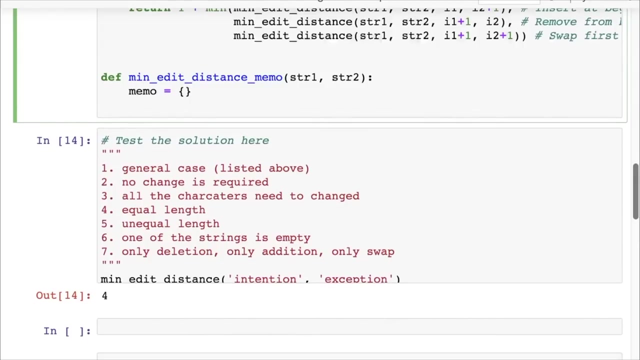 So let's write the memo As Version. So we have min edit distance with STR one and STR two and this we're calling memo. Okay, This we're calling memo. Now we have a A memo. The memo is going to be a dictionary and the dictionary is empty. 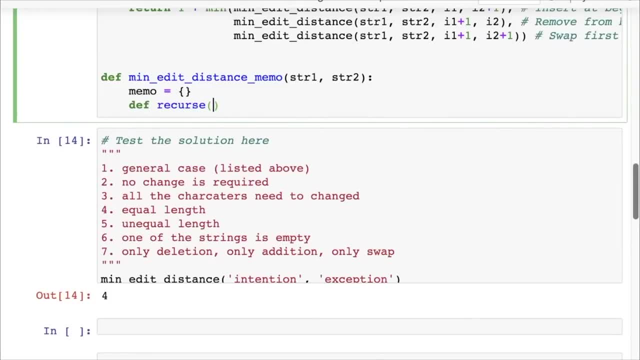 And then we define a function: recurs- So insane memoization. normally you have to write a recursive helper function. Now you can either write this outside or inside. I like writing this inside because, well, it will have access to STR two and they do not need to be passed in. 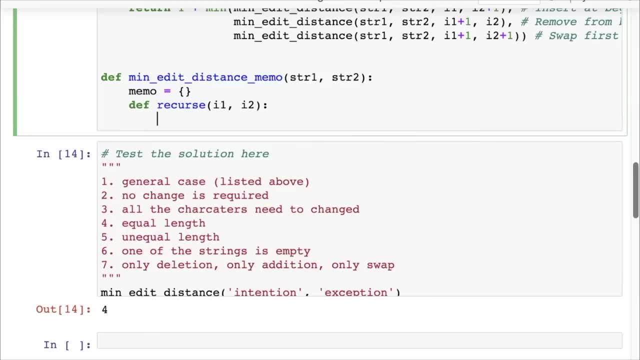 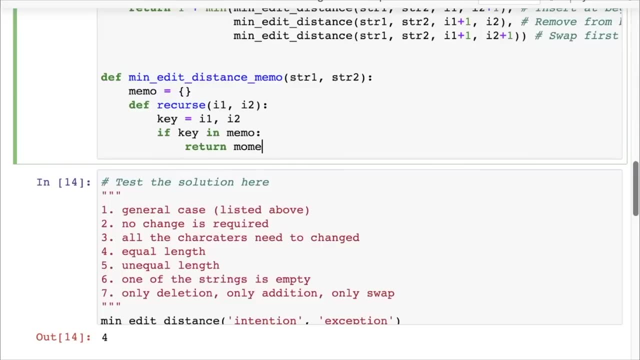 So here we have, Ivan and I do, And first thing we do is we create a key to the key. is I one comma, I two? Now, if key in memo, which means if you have already computed the solution, then we simply return memo of key. 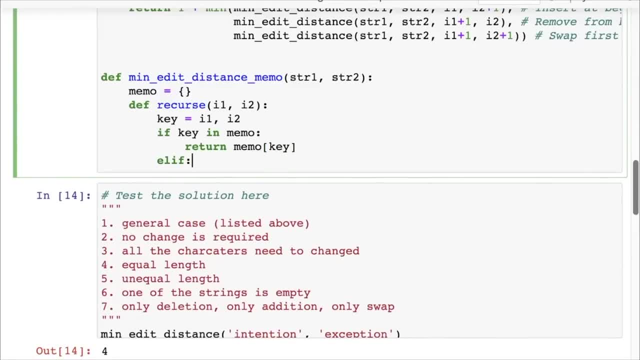 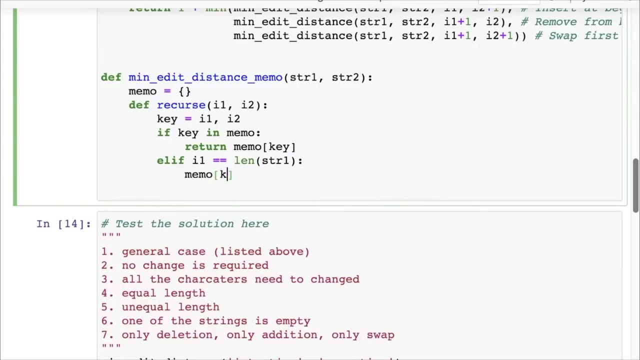 If not, then we have all the other cases. So now we have LF, Now we can check if I one equals land of STR one. in that case don't return, said the memo of Key, to land of STR two minus I two LF: I two equals land of STR two. 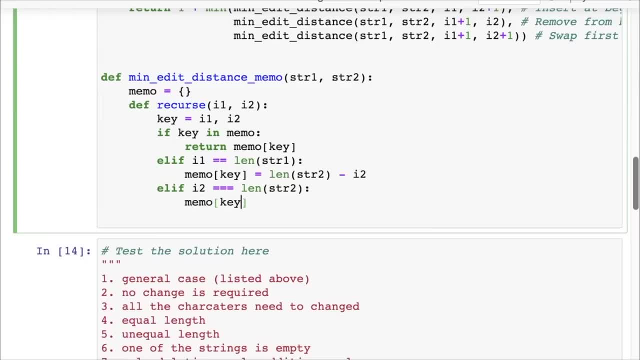 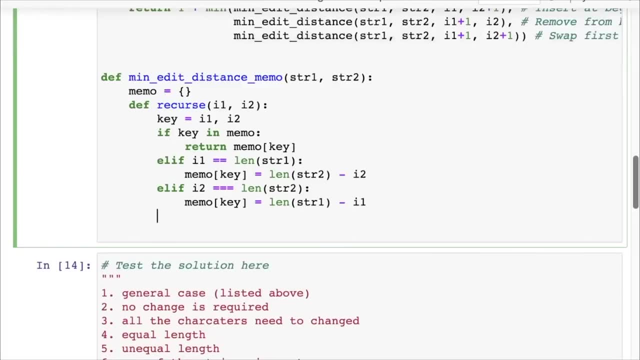 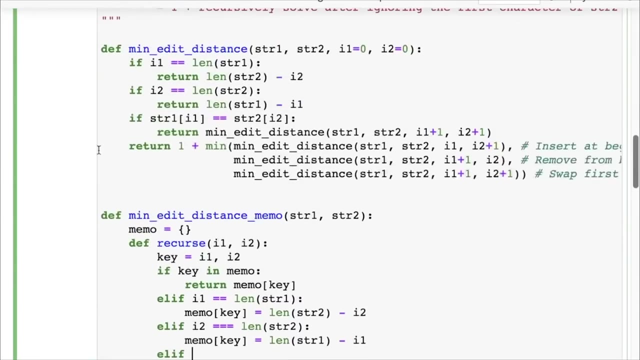 Then we return memo of key is land of STR one minus I one LF. Okay, In this case, then we check if the first elements are equal. So we have the exact same logic. You can see the same cases coming up here. 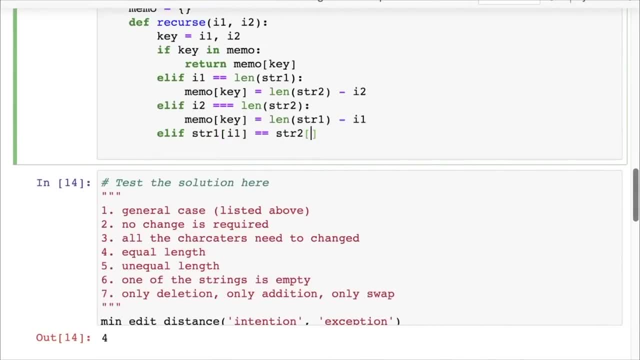 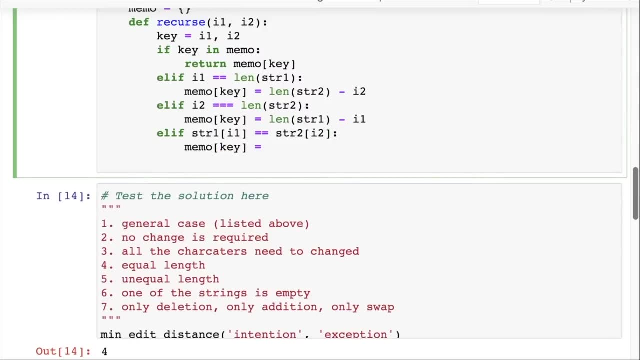 So if you have STR one of I one equals STR two of I two. in this case we have memo of E equals. We simply ignore the first character, So we increment I one and I two, So exactly what we have done here. 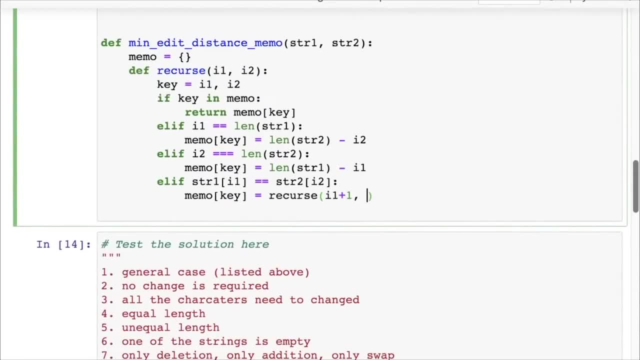 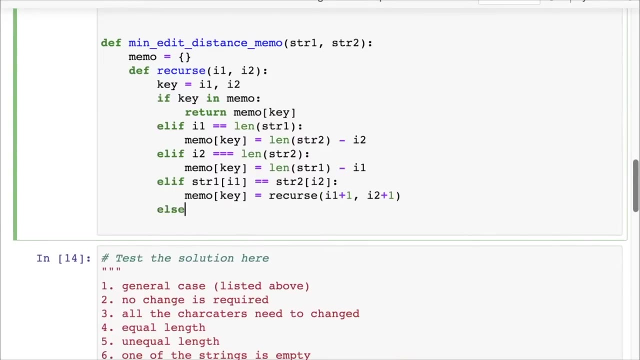 So we simply call recurs, this time with I one plus one and I two plus one, right. So we always call the recursive Function. but inside the recursive function, if it has already been computed, it will return from the memo. And finally, if we have- and this is the final case, which is where they are not equal to here- 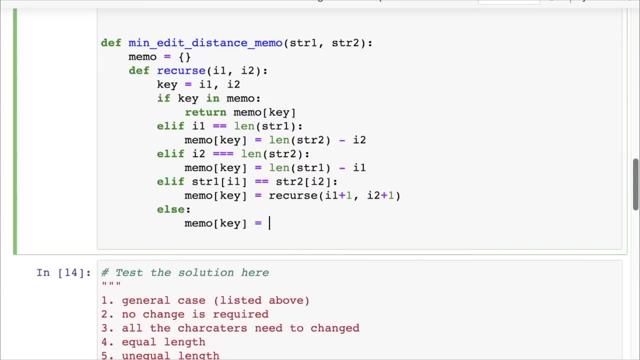 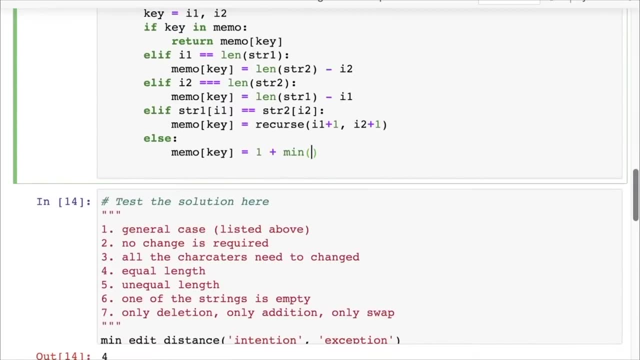 Memo of key becomes one plus min of. let's see here. So we have recurs. So the insertion cases: we will ignore The first element, sorry. the deletion cases: We will ignore the first element of the current range from the first string. 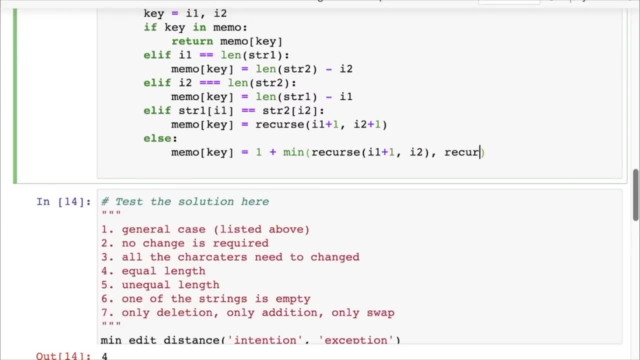 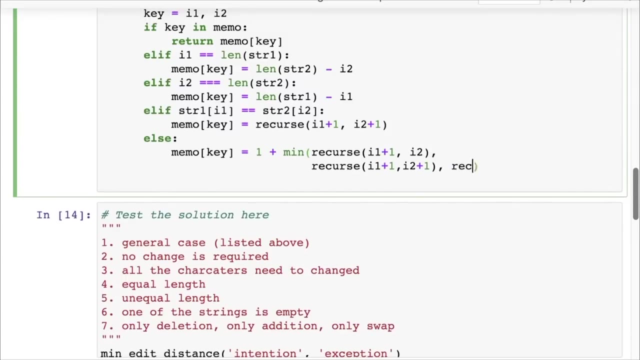 So we recall recurs with I one plus one and I two. Otherwise we call recurs with I one plus one and I one plus I two plus one. This is the case where we swap the first element of the first string, So we can just recursively check after ignoring the first element of each, and then we have recurs with I one. 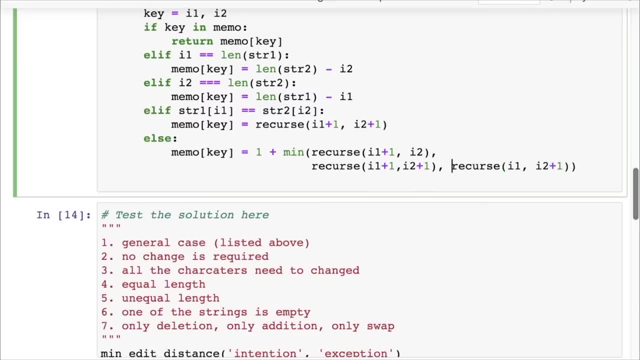 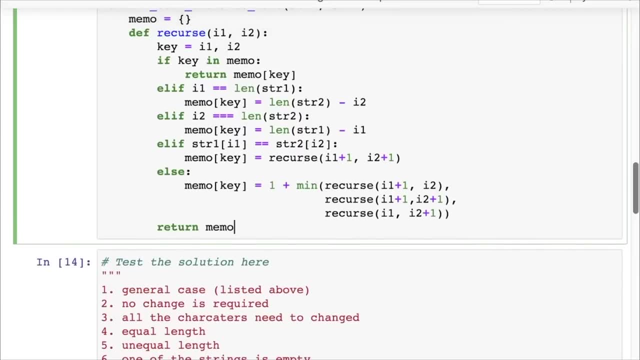 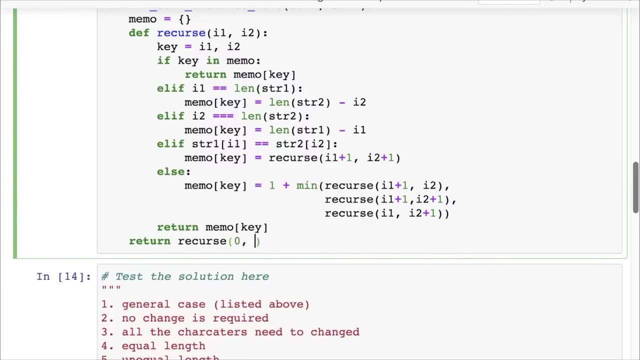 For my two Plus one, I two plus one, And there we go, And that's it. So now we have stored it in the memo and then we simply return memo of E at the very end, And finally we call recurs: zero, zero, and that is our solution. 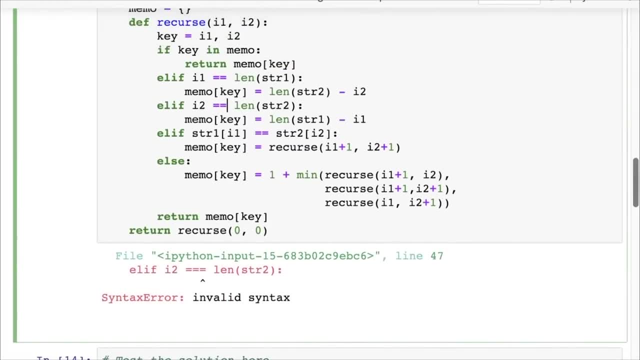 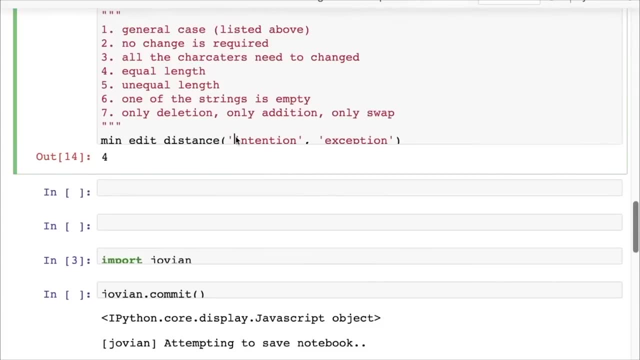 Okay, And there is a syntax error. You can click fix the syntax. That is very easy to fix, And I've just realized that the solution in this case might actually be four, Because what we can do is we can change N to P. 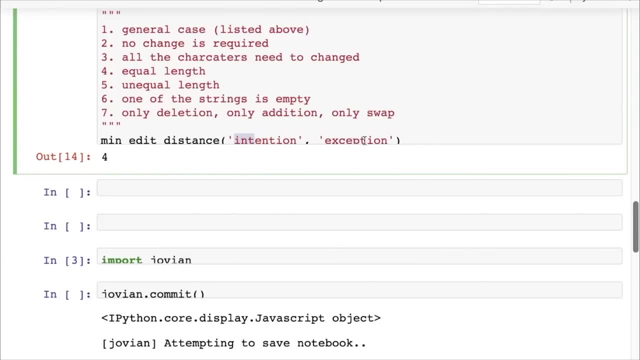 So that's one step. we can replace INT with EXC. So we replace INT with EXC. That's three changes. We don't change E and we replace N with P. the solution is four. So our solution was correct. There was no issue there. 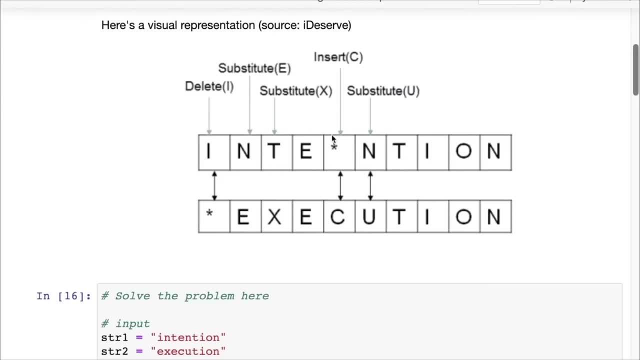 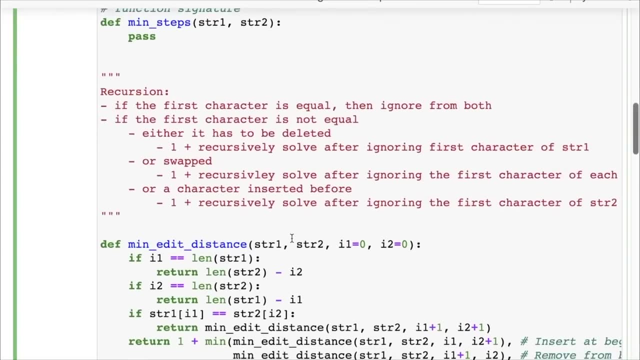 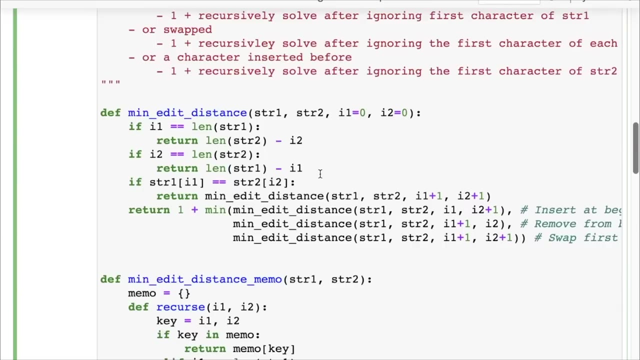 In fact, this is not the best solution. This is a suboptimal solution. So this output should be four, and that's okay. This is something that happens all the time, where you miss something and you just assume that you just say that you're going to come back to it at the end. 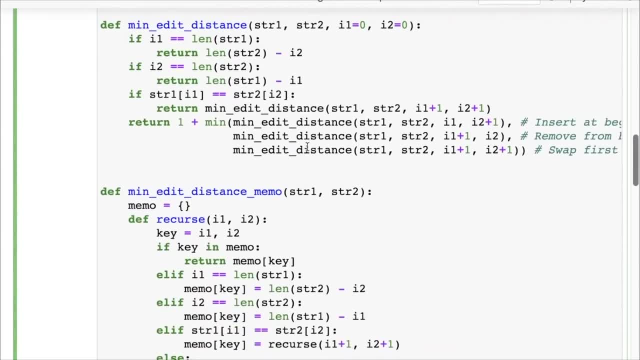 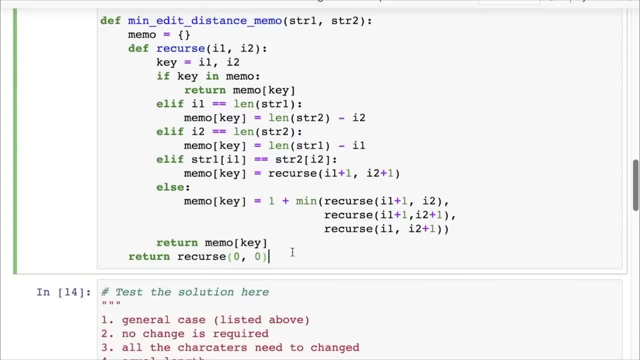 And then you move forward assuming that that code was right, And then you realize that either you were correct or what your mistake was. It's probably going to happen in one of five interviews anyway. Okay, So now we've written a memo solution. 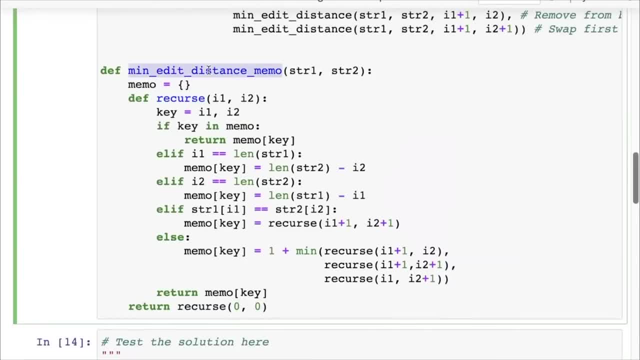 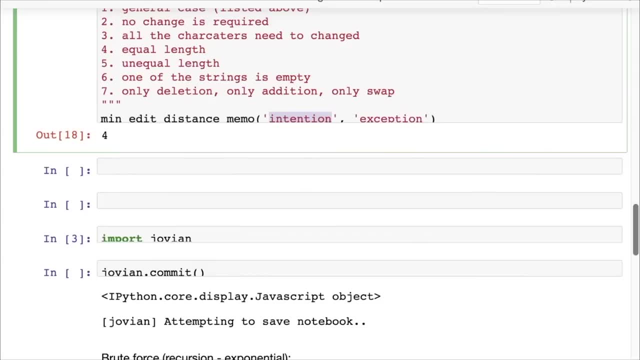 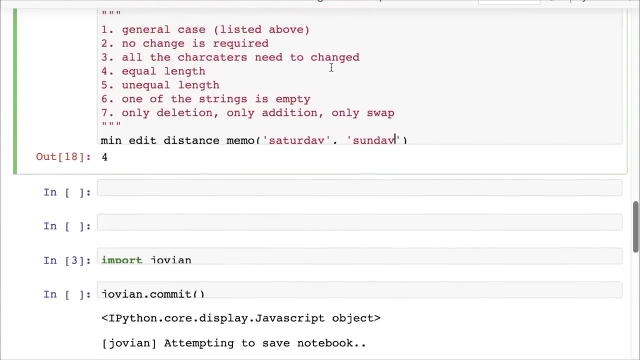 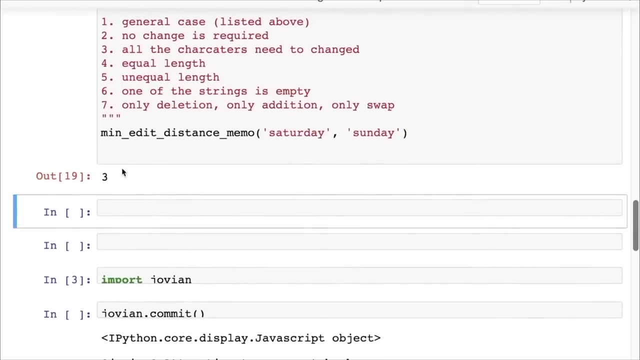 Great, And we can start checking the memo solution now. So minimum edit distance memo, let's call main edit distance memo and we get back the value for looks fine, Let's try Saturday and Sunday, as we have. So that's three. 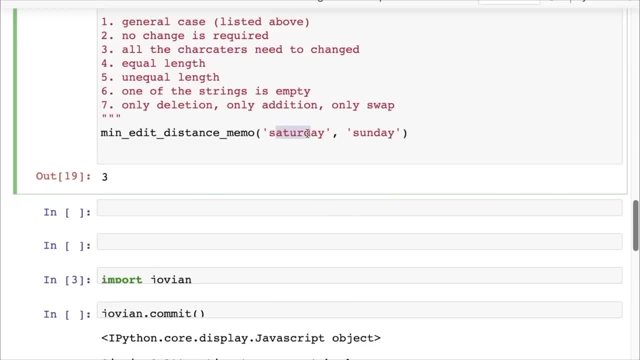 So what you will do is you will leave a as it is, change 80, you are. Do you win by removing 80 and changing our twin? That seems fine. Let's test out some cases like this. Okay, This is three, six, eight characters. 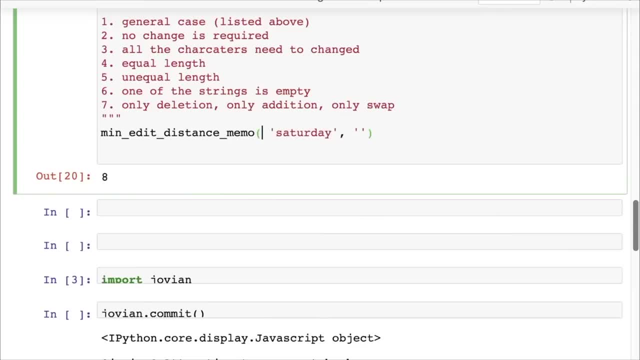 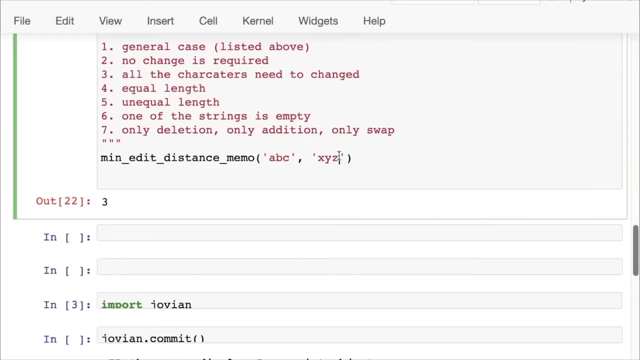 So that seems right. We simply delete all the characters. Let's check out this. You're also eight characters. We have to add eight characters. Let's say we have ABC and X Y Z, So this should be three. If it is X Y Z, K. 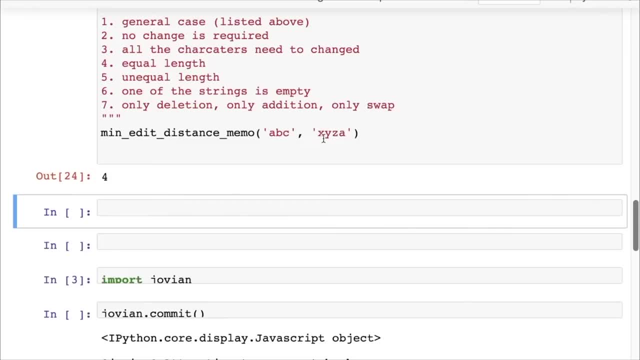 Then maybe that will be four. What if it's X, Y, Z, a? in this case also, it's four. So this seems to be working fine. We have now taken the recursive solution. identified the inefficiency, calculated the complexity which was exponential. identified the inefficiency. 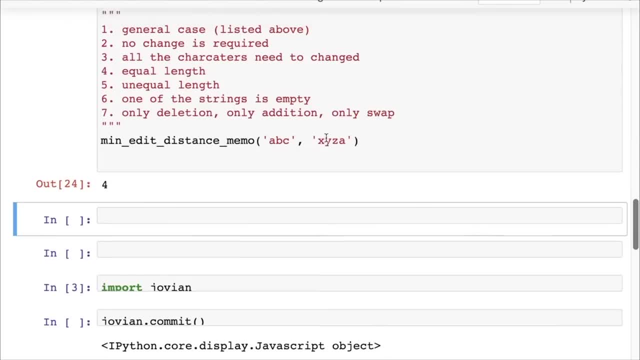 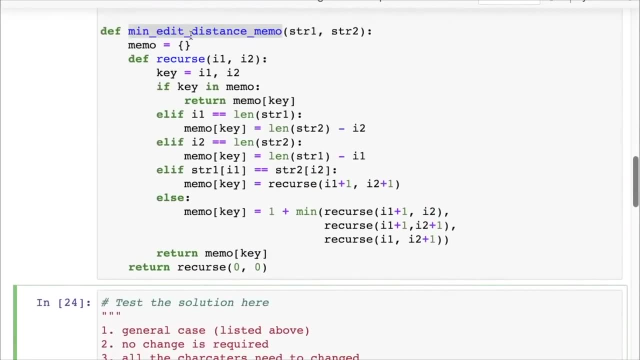 and the, which was repeated, sub problems, and then fix the inefficiency by calling main. edit this by by using memoization. And now, how do you compute the Time complexity of memoization? Well, the argument is: if you only need to compute the solution for a key once, and the computation 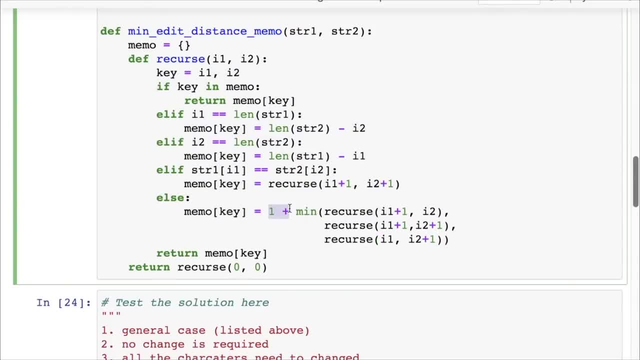 apart from the recursive calls, simply involves some comparison and a fixed number of comparison and an addition. So the time required to compute, assuming you have the recursive solutions, is constant. So that means, if you simply count the number of memoizations that can possibly occur, that 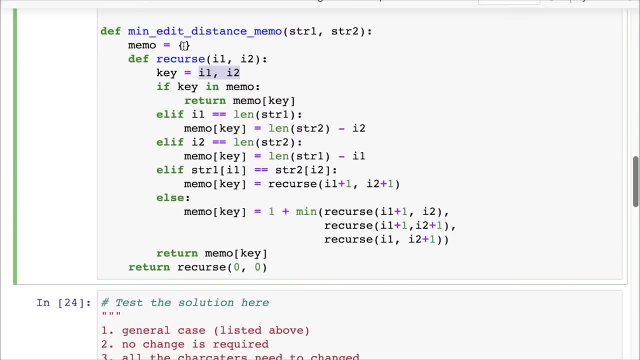 gives you an upper bound on the total number of operations, It will be equal. Okay, It'll be some multiple of that, some constant multiple. So I one can take the value zero to N one, where N one is the length of string one. 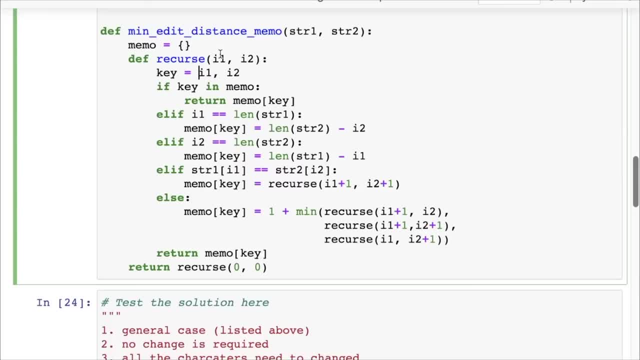 And I two can take the value zero to N two, where N two is the length of string two. So memo: the keys in memo can be I one, comma, I two. So you have N, N one values for I one, N two values for I two. 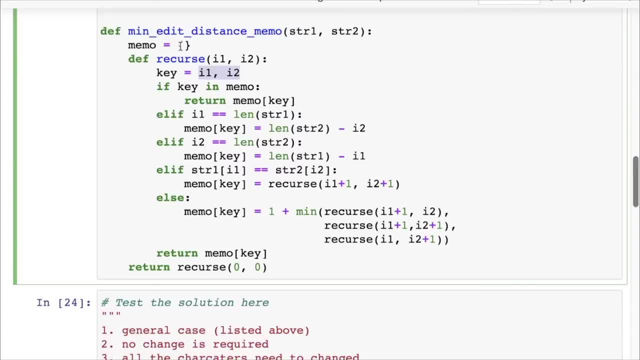 So that makes it N one times N two. That's the number of keys And that because there's a constant amount of time, X additional time required to compute the Solution for a key. that is also the complexity. So the complexity is ordered N one plus N two. 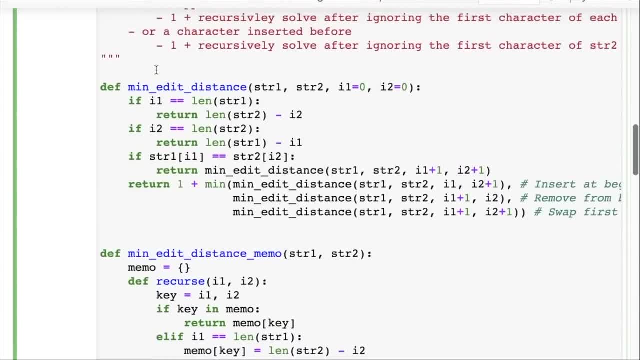 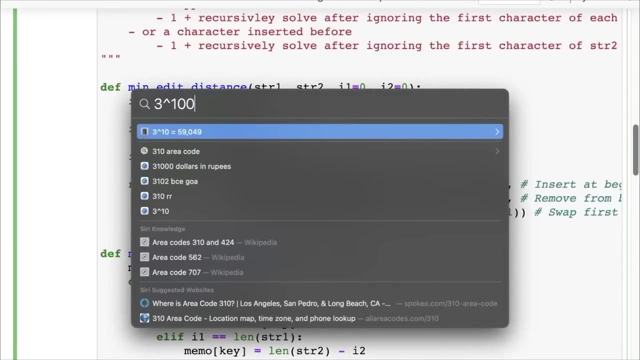 So we've gone from three to the power of N one plus N two, which grows very quickly even for three, to the power of three. to the power of uh. N is pretty high. We can check it out here: Three to the power of 10 is something like 59,000, three to the power of a hundred. 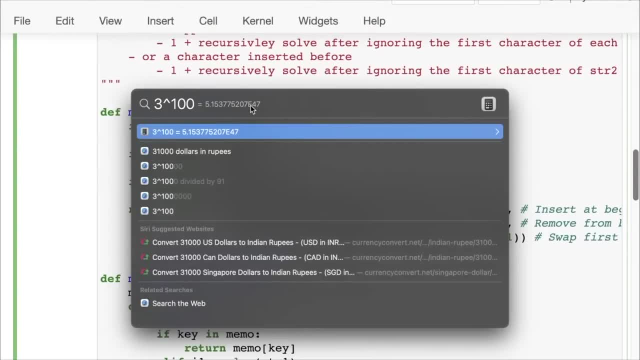 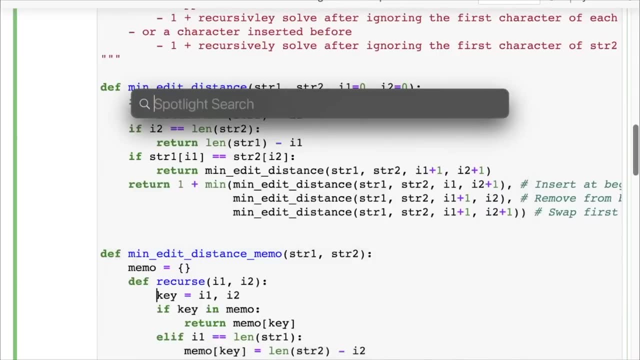 So if you have N one plus N two, then that's E to the 47, that's going to be a lot of operations. on the other hand, if Or in with memoization, it is only going to take, let's say, the a hundred is split as two strings of length, 50 and 50, only going to take 2,500 operation. 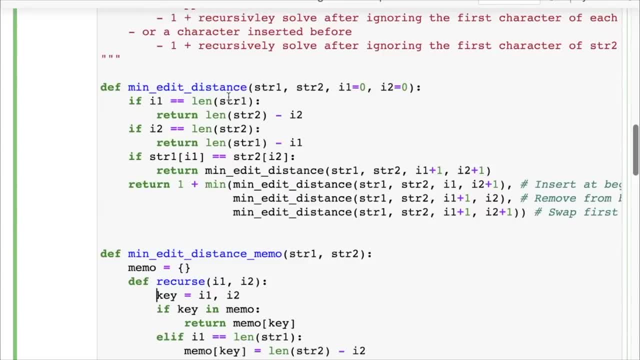 So where it was taking 10 to the 47 operations, Now it takes only 2,500 operations, which is pretty small. So you can still work with lists of size up to 10,000 or a hundred thousand very easily using the memo solution. 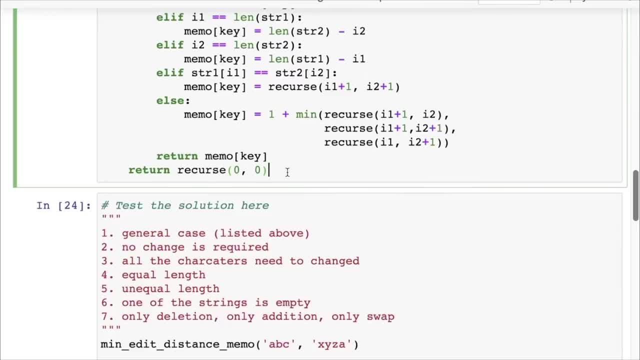 So that covers this problem- And keep talking through your solution. even as you're stuck, even as you're confused- just as I was- it's helpful to just keep a spend maybe two or three minutes trying to solve the issue, And if you're not able to solve the issue, just say that this is something I'll fix later and then move on. 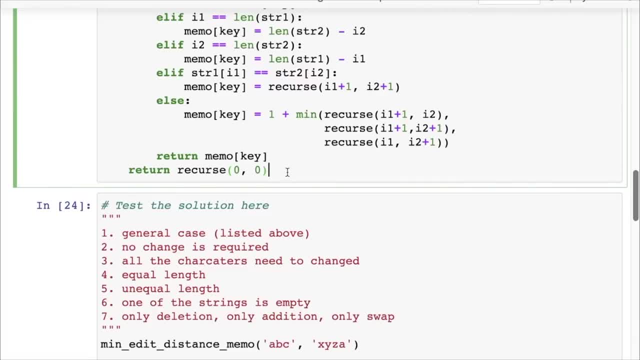 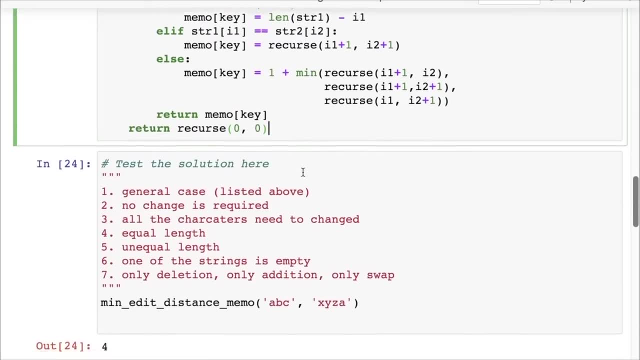 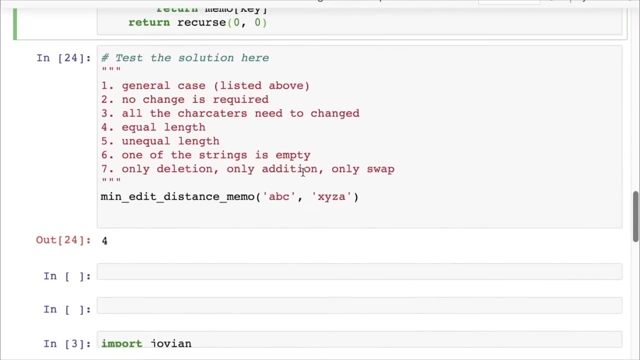 Assuming that you've fixed it- and then keep talking and keep, continue, keep working on the solution And at some point later it's possible that the solution might like you. Okay, Now, at this Point, you may be asked sometimes to implement a dynamic programming or an iterative solution. 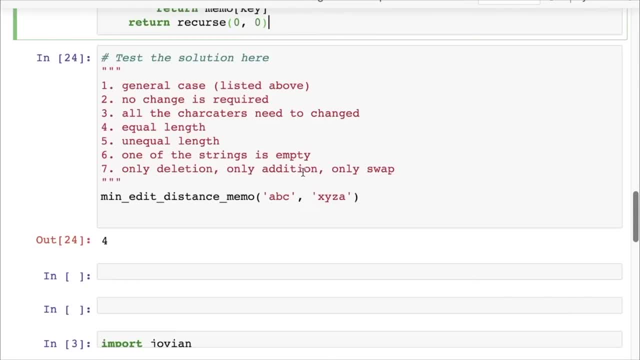 Like the, when you talk to the interviewer and you're telling them that this is how I'm thinking, I'm doing. I'll do a recursive solution first, And I can see that maybe there are going to be some sub problems there. Then I'm going to then, uh, apply dynamic programming. 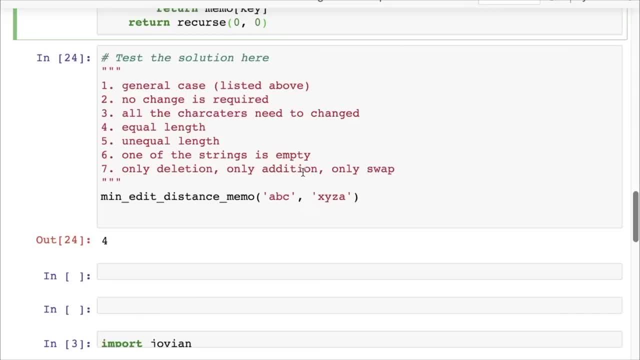 So you can just check with them And in most cases they will accept a memoization solution, because the dynamic programming solutions can take a little bit of time- Okay Okay- To solve, to implement and they're always off by off by one errors. 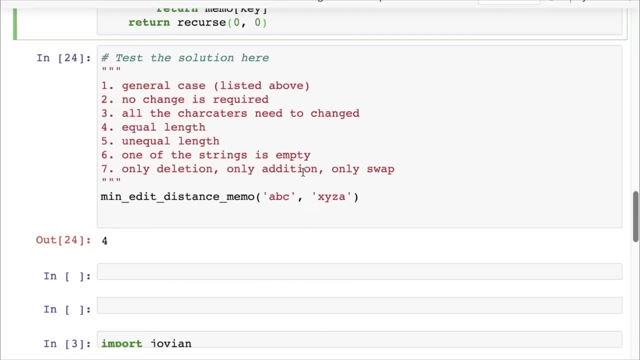 And it's also difficult to explain the solution. So you can most, most cases, get away with memoization. but if they do ask you to do it with iteratively, with dynamic programming, then you'll have to go ahead and implement a dynamic programming solution. 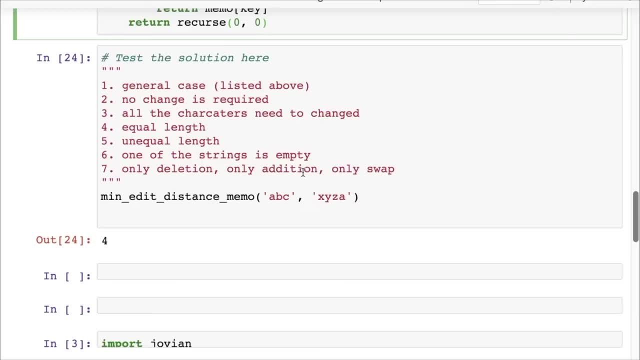 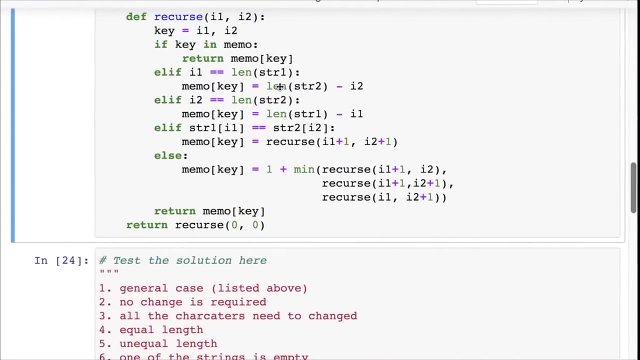 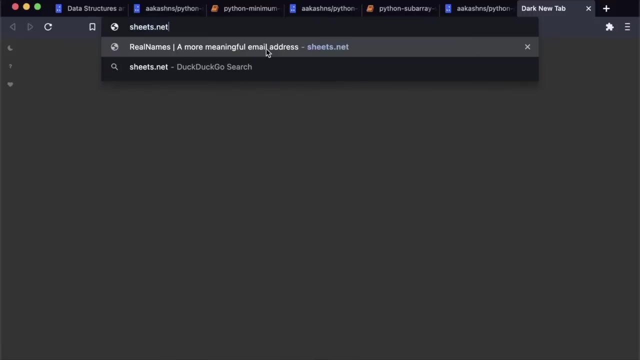 So, once again, take a couple of minutes now and work it out on a piece of paper and then go back to them. Now for dynamic programming. remember, you have to create a table, essentially. So what the table will look like In this case is: let's see if we can simulate a table, or the table will look like is: let's create a new sheet. 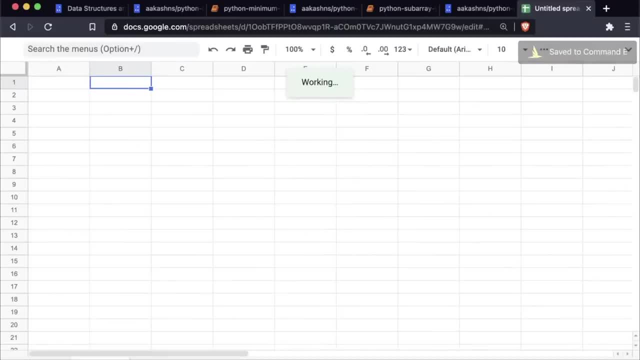 And in this sheet let us put the two words: which is intention, жел塔. Difference between aче. It's like I'm not going to explain it later, Maybe one minute before the date. That's the first thing, Okay. 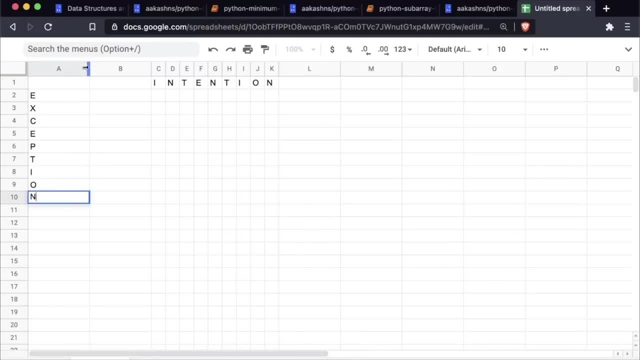 And let's put the word exception As well. There you go. It's like that: Let's move this down to and let's also put in the indices. Ultimately, this is what a dynamic programming looks like. Programming problem looks like you are ultimately going to create a table here. 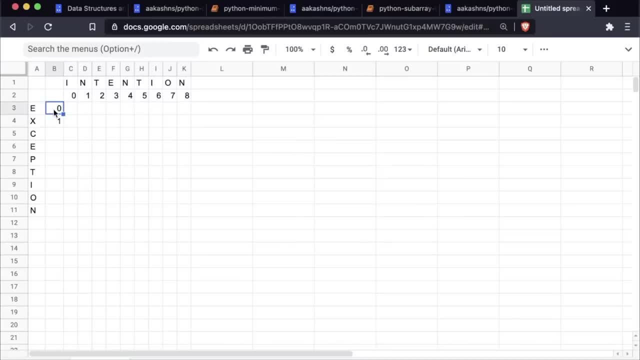 and how we'll start filling the table is the I J element. So let's say this element: I N T I N T E, E X C E. So this element represents the edit distance or the number of operations required to convert I N T E into E X C E. 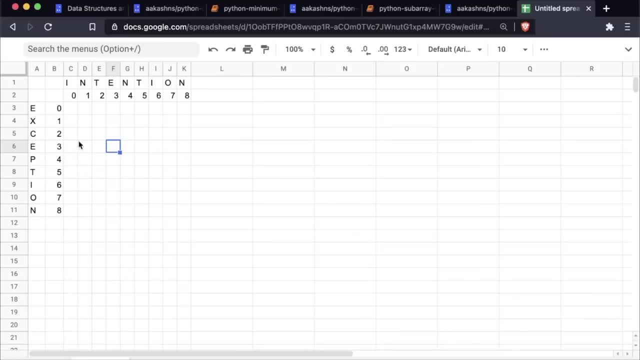 And how do you check what the solution is? now, you know that E and E are equal, so the final elements are equal. So what that means is we look at this value, then this value should tell us what is the minimum edit distance between E X C and E X C. now, since we can simply add E, 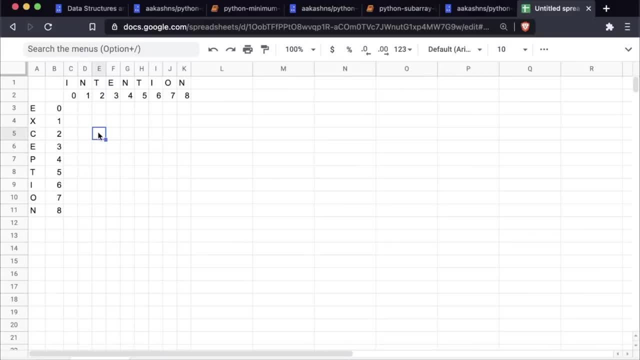 to each string and get this solution. that means this solution is equal. This value should is equal to this value, All right, So in the case where the corresponding elements are equal, we simply copy over the value diagonally left top left value onto the current cell. 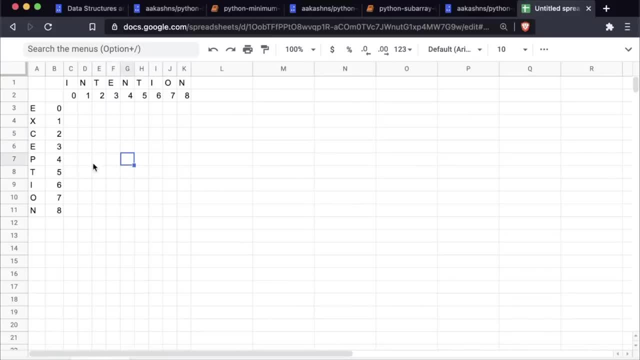 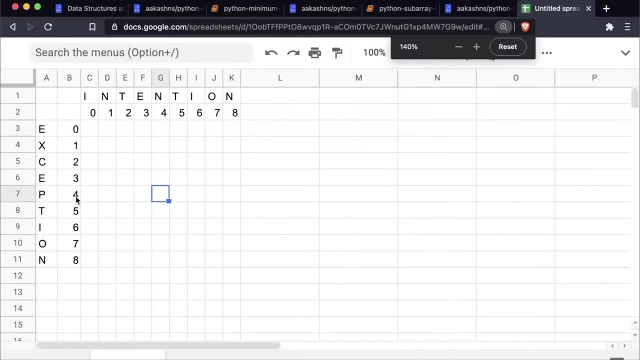 The other Option is if they are not equal. So let's say, if we are here where, here you have N and here you have P. now there are three possibilities. you want to find the minimum edit distance between I, N, T, E, N and E, X, C, E, P. now N is not equal to P and this is the original. 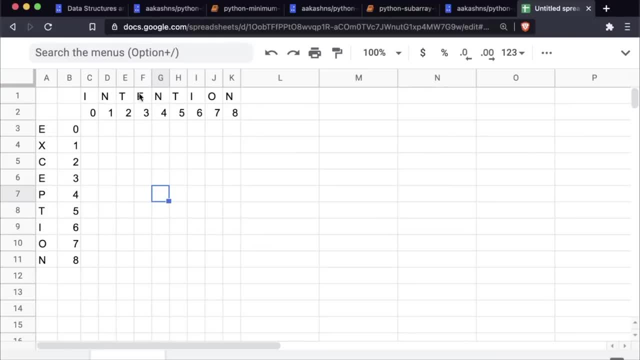 string. so either we delete N Now. if we delete N, then we need to find the solution for I, N, T, E and E, X, C, E, P. so if we delete N, then this value will become one plus this value. That's one possibility, or another possibility is that we swap N. so we swap N for P. 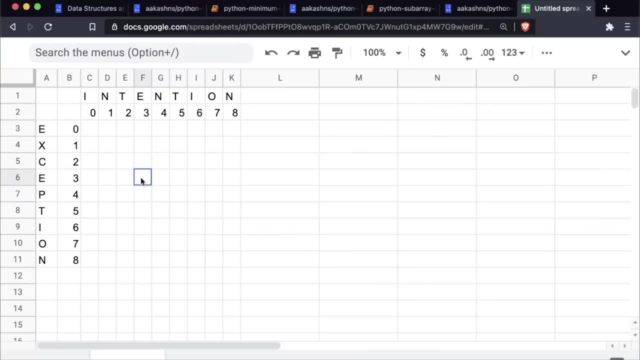 So now you get this becomes P and this becomes P, So this value becomes, will become one plus this value, because now we can ignore the P and simply get this previous solution for E, X, C, E and I N T E, So this value becomes one plus this value. or the final option is that you can insert something. 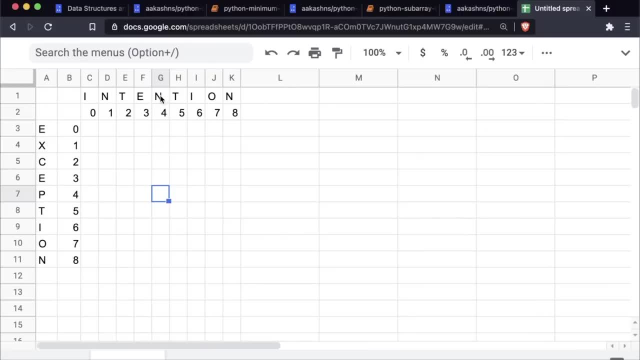 Just before N. So if you insert something just before N which is going to be P, So if you insert P just before N- sorry, you insert P just after N, not before. If you insert P just after N, then you have P after it already. 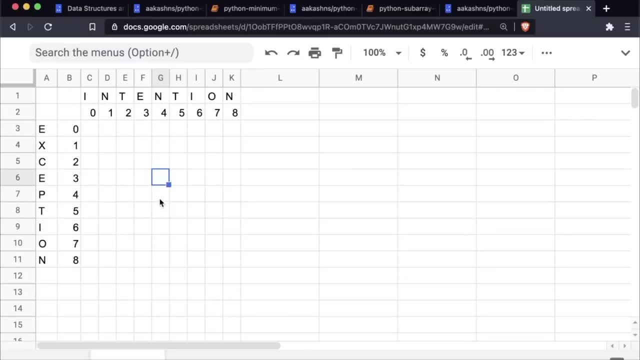 So you can just look at this value, and this value is going to be one more than this value. In the case that you Insert something, insert P after N, right? So there are three ways to come to this value: either by deleting N or by 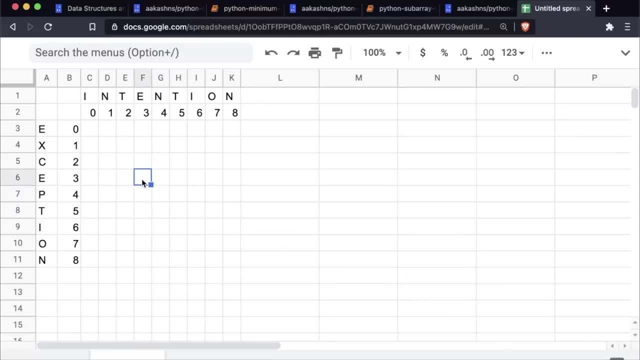 inserting P or by changing N to P, And what you can do is you can take the minimum of three values- three or these three values- and add one to obtain this value. So that's the logic, roughly speaking, and you start from the left. 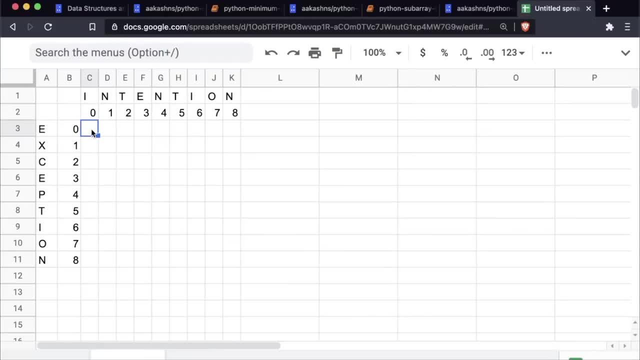 So you see, okay, E and I, they're unequal. So you need one operation to change them and there's nothing else to consider. So that's done. Then E and N, they are unequal. Now you need what you can do is you can either delete N. if you're delete N, then 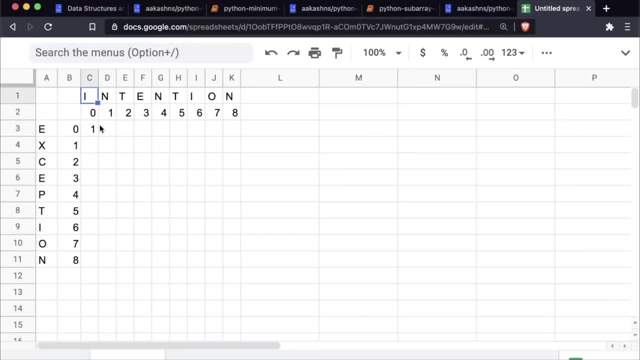 you simply need to check E and I and you know that the solution for E and I is one, So this would be two. Another another option is that you could possibly insert something, but if you insert something, the length of IN is going to increase. 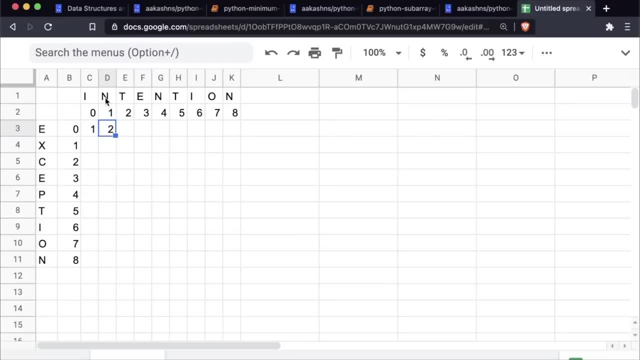 So that's going to cause a problem. So you can't insert. Another option is you change N with E? but if you change N with E, then you will no longer be able to. if you change N with E, then you will no longer be able to use this solution, right? 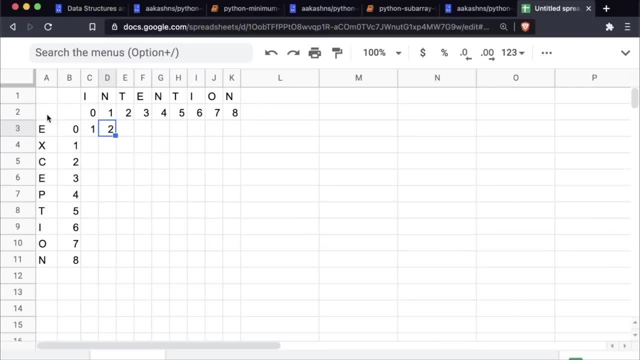 Because now you will have to match I with the empty list, So that's going to be one as well. So overall you end up with two and this is how you start filling the list. So you start filling up from left to right, and left to right, and keep going top to bottom. 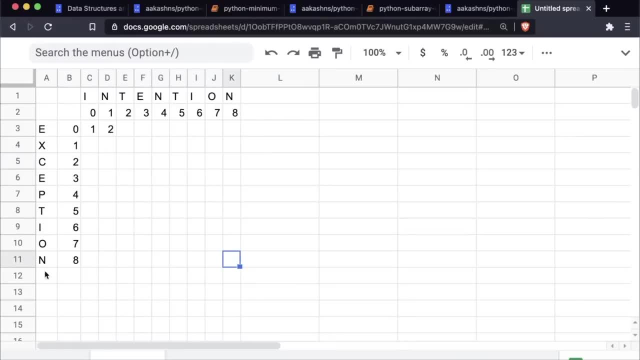 Okay, Okay, And as you fill out this list, finally, you will fill out this final value, exception and intention, and that will be your solution. So that's the dynamic programming solution, And you can see that it's getting tricky to convey the entire solution because there are so many cases involved here. 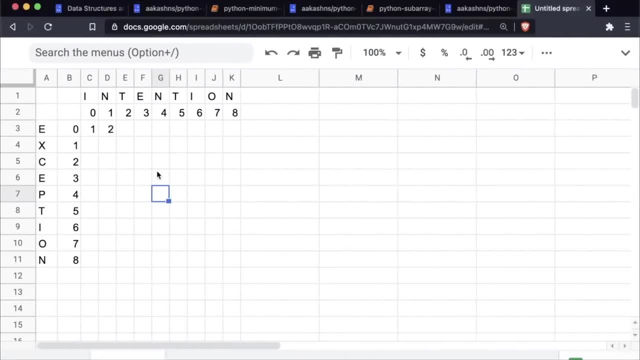 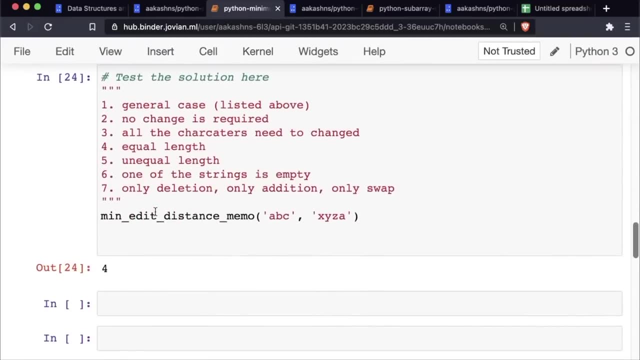 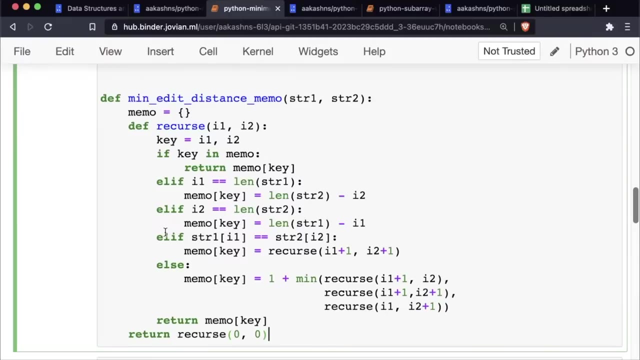 So typically you will not find dynamic programming solutions to requested in interviews and it will help you to just stick to the memoization solution. All right, So with that we have covered two common interview questions And you can keep going. So the idea here is to just apply the method. 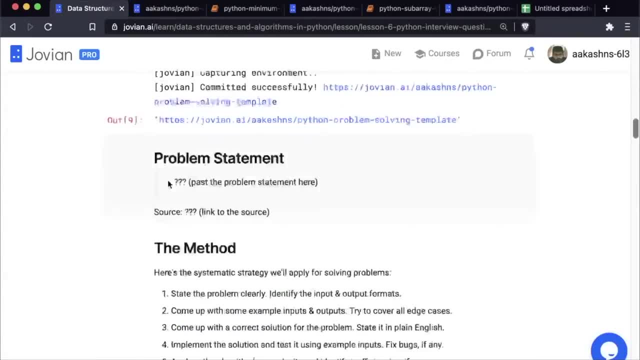 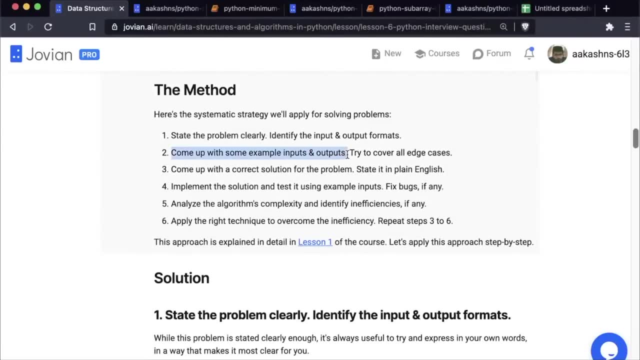 Remember them. remember the method, the problem solving template that we've covered. state the problem. identify input and output formats. write a function signature. come up with some example inputs and outputs, or at least the scenarios. come up with a correct solution stated in plain English. implement the. 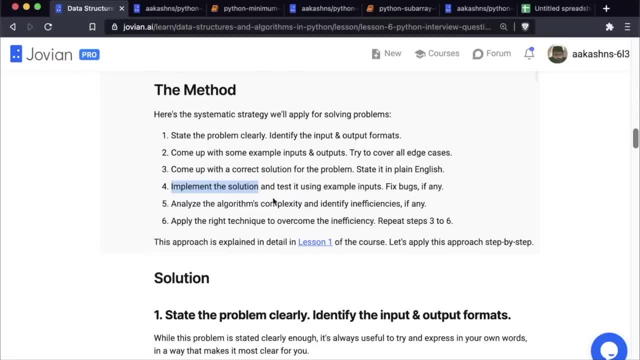 solution, tested using example inputs and fixed bugs. If you face any, then analyze the algorithms, complexity and identifying efficiencies And finally, a Apply the right technique to overcome the inefficiency And you repeat the process, going back and stating the solution, implementing, analyzing and repeating. 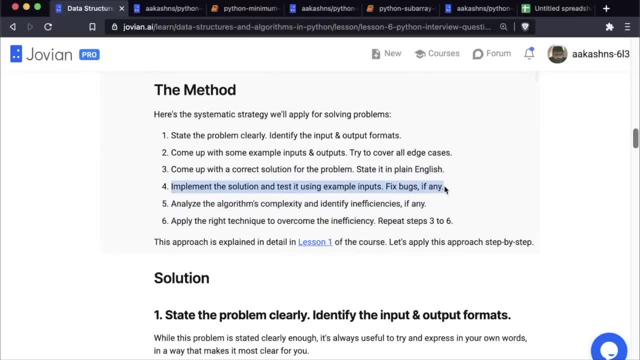 Now you. in some cases you do not need to implement the brute force solution if you don't have the time, but when you're working with the recursive solutions, it always helps to implement brute force first before you do memoization or dynamic programming. 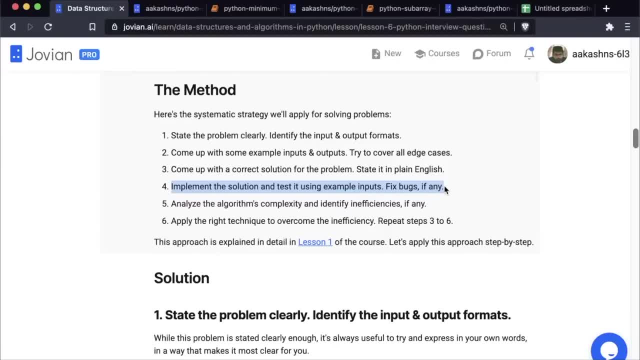 And some tips. ask questions, as many questions as you can, as many as you need to clarify the problem. show an example, Follow the method. Don't panic If you get stuck at a certain point. give it a couple of minutes. 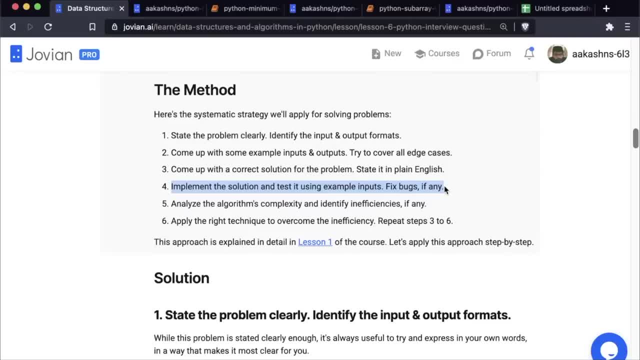 Sometimes you can even ask the interviewer and they may be able to tell you that maybe what your error is, or maybe you're not stuck at all What you're, you're simply assuming something incorrectly. but beyond a few minutes, what you want to say is that let I'll fix this later. 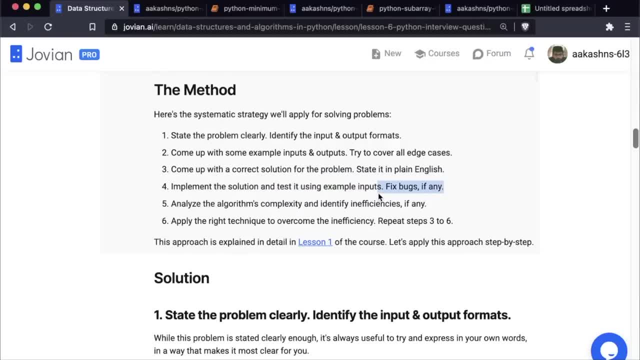 Assuming this is correct, Let's move on And then talk about complexity And and optimization and such and such. Very important is to state the brute force solution to the interviewer, And if you are unable to figure out a more optimal solution, then the best thing you can do is to offer to implement the brute force solution so that you can at least demonstrate that you are able to write code. 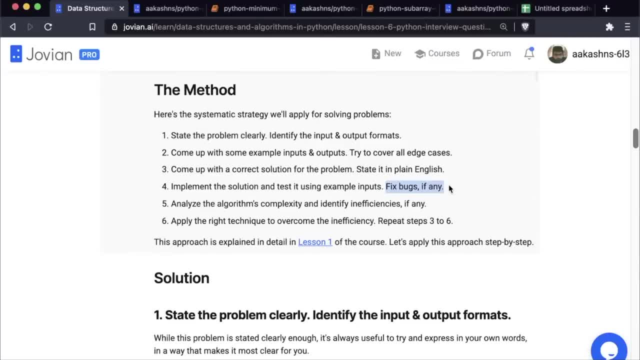 And it's all right. In a lot of cases you will not be able to figure out the optimal solution, And in some cases there may not be an optimal way, but there are some. there are certain problems where there is just one way. 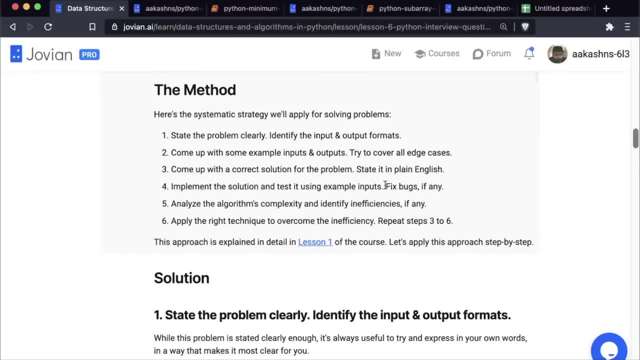 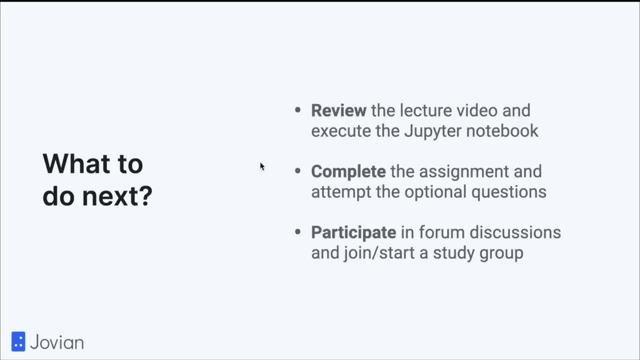 And that is The hard way or the brute force way, And this is typically very true with a family of problems called backtracking, something we've not really covered in a lot of detail, but it is also another form of recursion. So what do you do next? 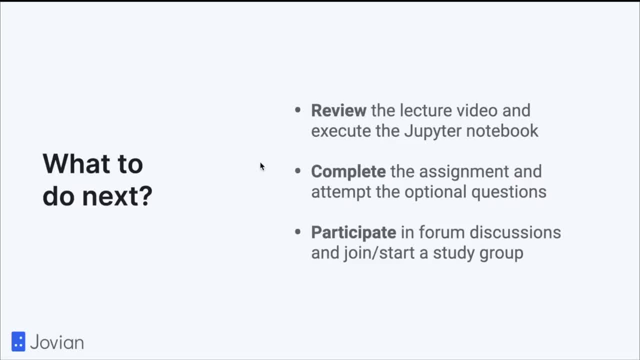 So the next step for you is is to review this lecture video and solve these problems yourself, or take more problems. Ideally, what you want to do is you want to take all the five different techniques that we've Covered and let's quickly review what those five techniques were. 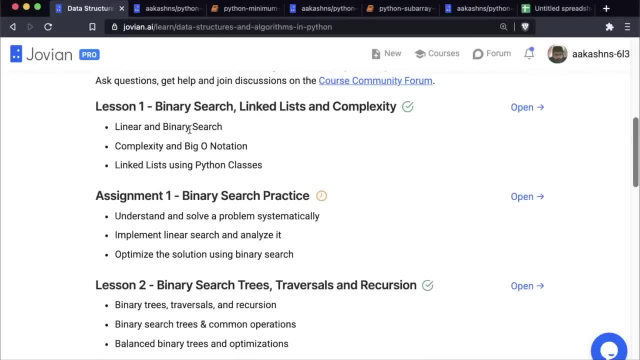 The first one was binary search. So we looked at linear search and binary search, which is a form of divide and conquer, And along with that we also understood the complexity and big O notation. And then you had some homework on linked list and Python classes. but binary search is something that comes up often. 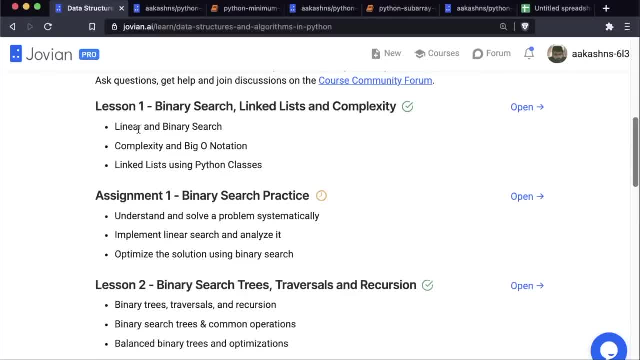 And the hint to detect binary search is simply to look for order. whenever you see something being something being mentioned, mentioned As sorted. Now that is an indication for you that this may be binary search. Sometimes what you may have to do is you may have to get things into a sorted form, maybe by taking replacing elements by some of values. still that element or so on. 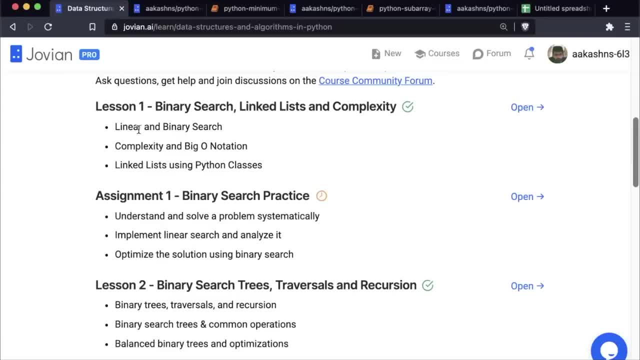 And once you get things into a sorted form, maybe then you can do binary search. That's one way to go about it, And once again, just two, five to 10 problems on binary search and you will be able to identify pretty much any binary search question. 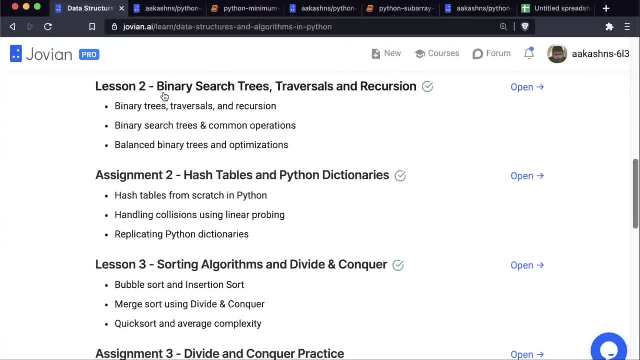 Okay, Okay, Then the next topic that we looked at was binary search trees, traversals, and here is something that is generally asked very directly. So you will be given a question like binary search tree- do something with a binary search tree- and you can answer that question directly. 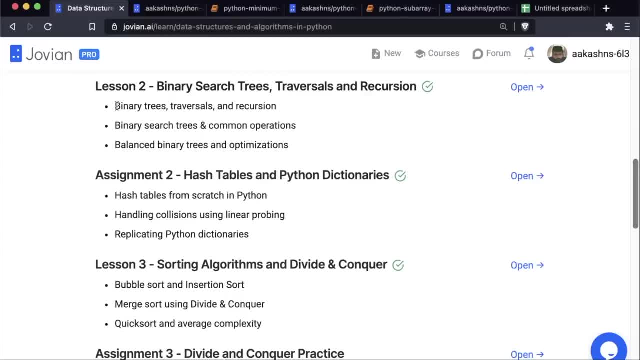 We've covered a lot of different things here, So do check out lesson two for all the different things you can do with binary search, trees, traversals, balancing, and most of these are recursive solutions, So it's also a good exercise on recursion. 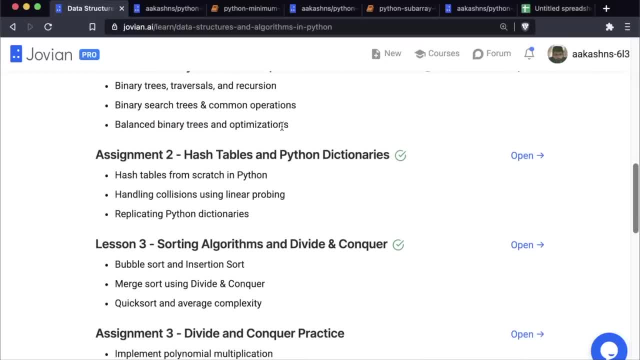 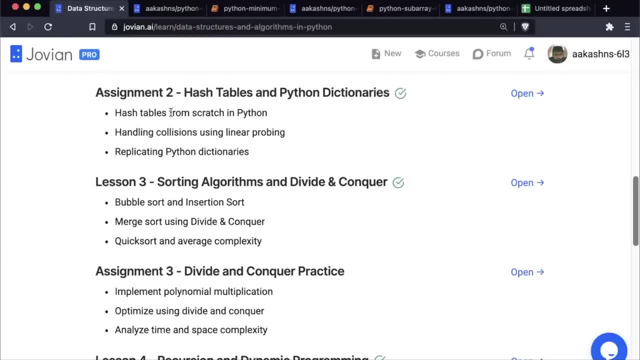 Okay, And we've also looked at balanced binary trees and how can we optimize them further. Then you had an assignment on hash tables, So hashing is again a common question that is often asked. So we built hash tables from scratch in Python and we also handled collisions using a technique called linear probing. 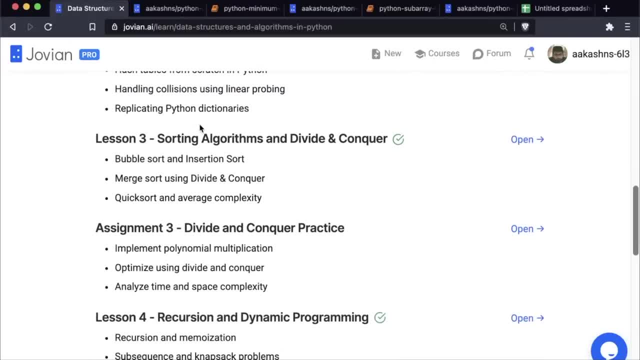 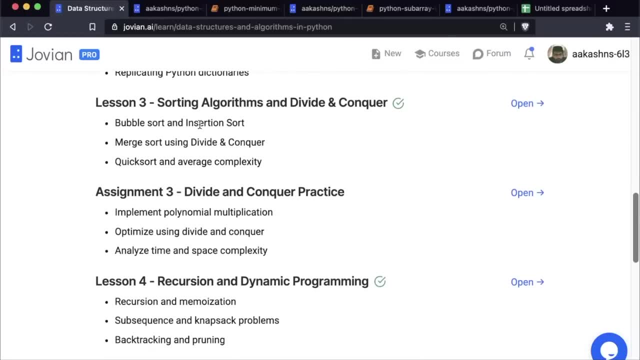 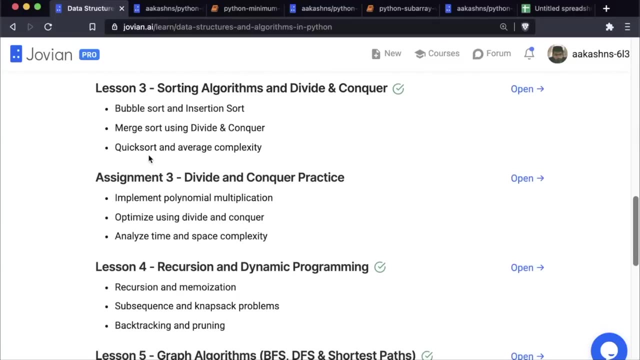 And so this is something you can check out in assignment two. So you may get asked just to implement a hash table in Python or implement collision resolution in a hash table, in which case you can use linear probing. Then you have the sorting algorithms, where we looked at bubble sort and insertion sort, merge sort using divide and conquer and quick sort, where we had a quadratic worst case complexity but a logarithmic average complexity. 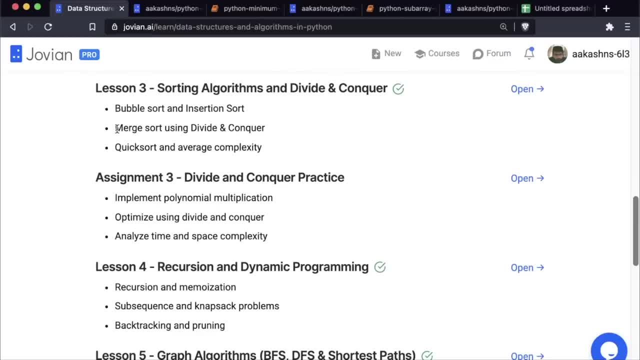 And that's a good thing because merge sort, although it is logarithmic in the worst case, it still takes up a lot of space and space allocation is slow and you may also not have the memory. That's why we sometimes use Prefer quick sort over merge sort when we are constrained for space. 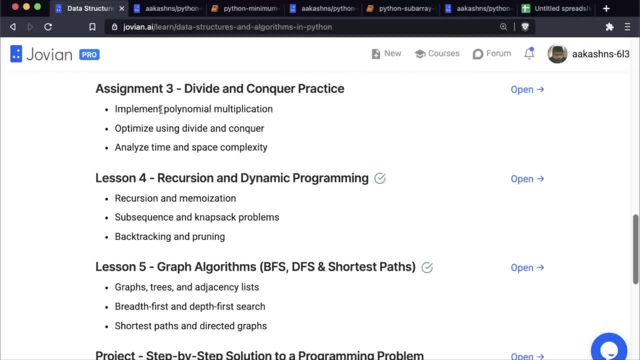 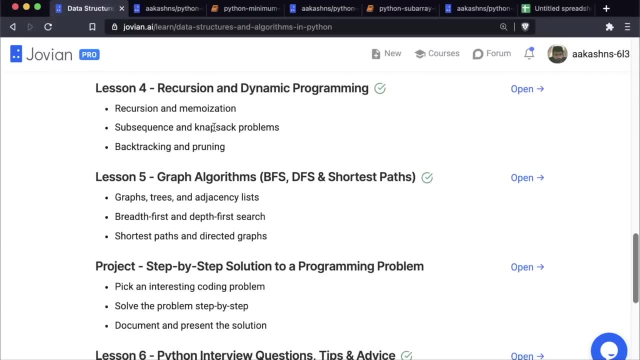 Then assignment three is pretty interesting, where you will implement an optimal algorithm for polynomial multiplication using divide and conquer. So do check out assignment three as well. Then we looked at dynamic programming. We looked at recursion, memoization, subsequence and knapsack problems. 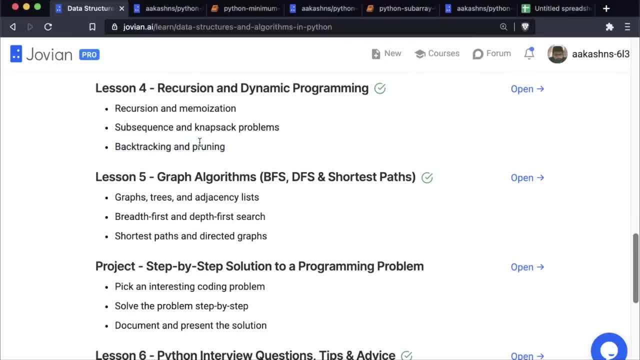 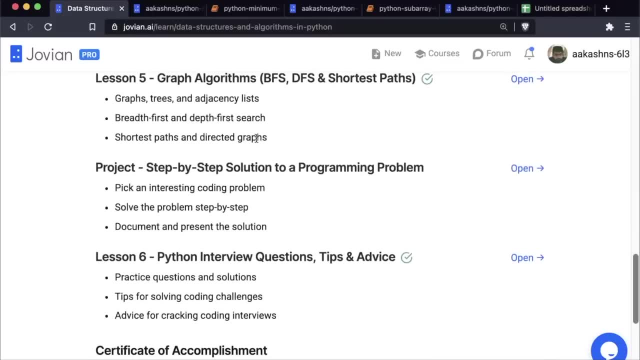 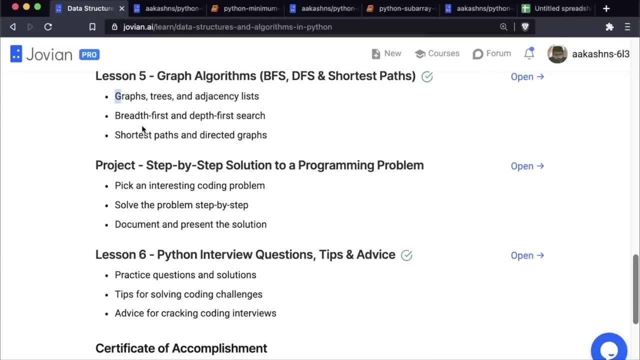 And then we finally also didn't cover backtracking and pruning, but we'll. there are some questions there in the lesson notebook which you can try out, which use backtracking And pruning as well. Then we looked at graph algorithms- the last time, which was graphs and adjacency list and adjacency matrices. 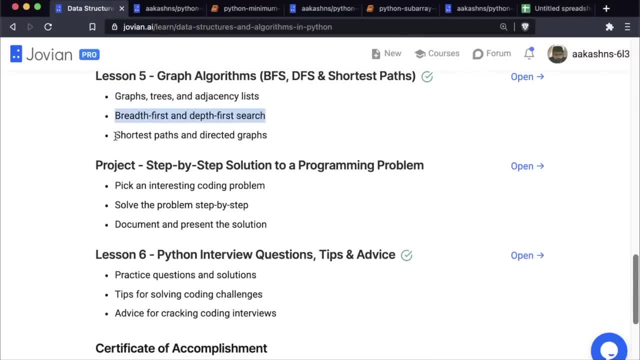 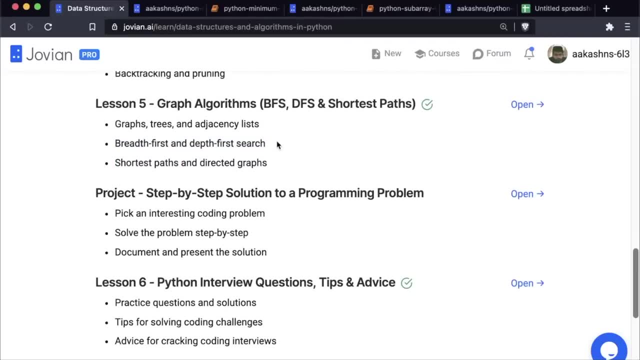 We looked at the depth first and breadth first search and how to implement them, And we also looked at shortest paths and directed and weighted graphs. This is a very important topic: breadth first and depth first search. You will get many questions related to these. 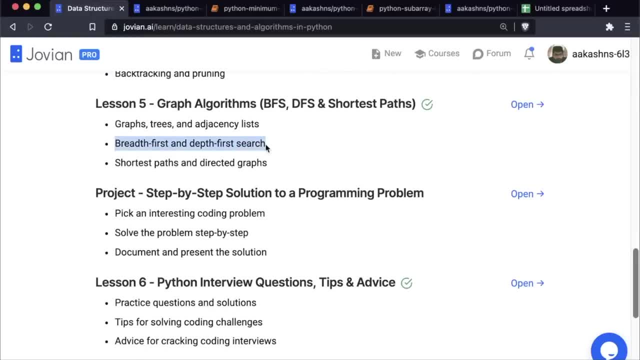 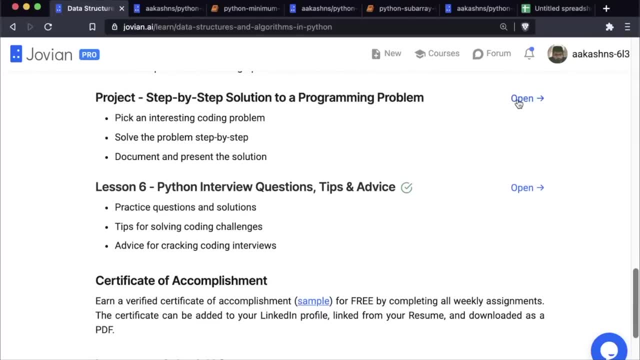 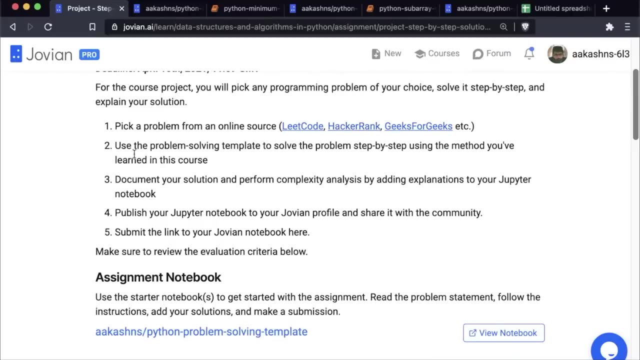 So do solve maybe five questions on each of these topics and you should be good with most graph problems asked in interviews. Now this project for you- the course project, if you haven't seen it already- is to pick a coding problem. So you can pick a coding problem from an online source like lead code, hacker, rank, geeks for geeks, et cetera. 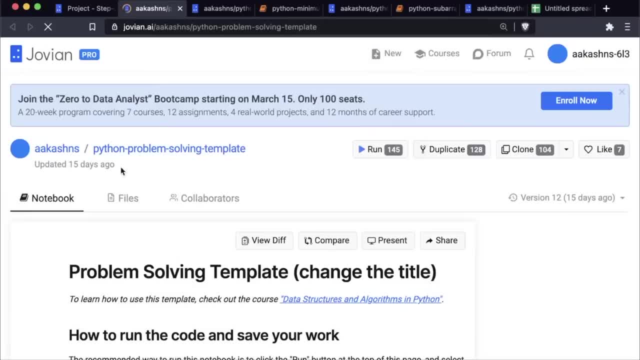 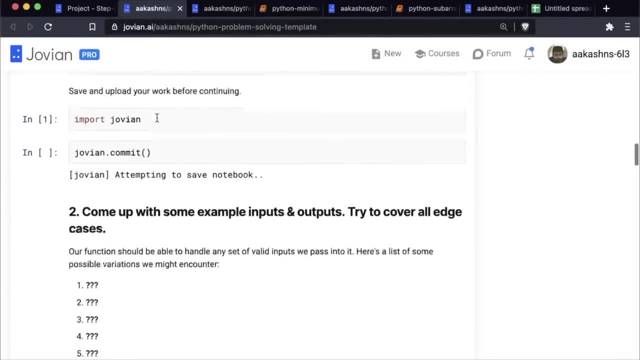 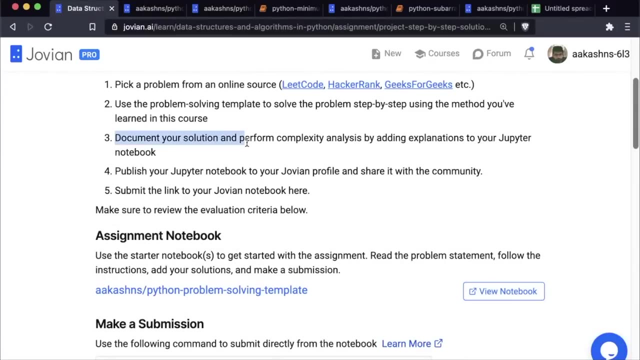 And then use the problem solving template that we've shared with you- this problem solving template as a starting point, So just give it a name and then write the problem statement and implement the solution step by step. We use the problem solving template to solve the problem using the method you've learned in the course. then document your solution, add explanations. 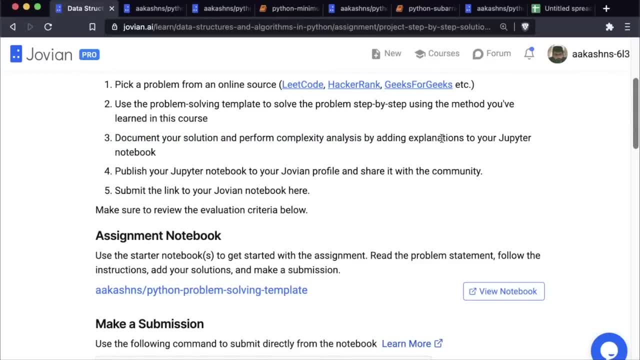 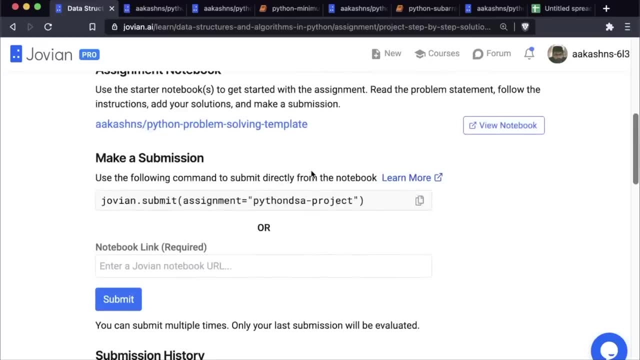 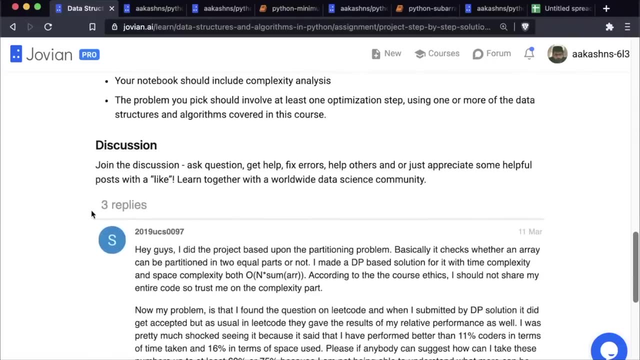 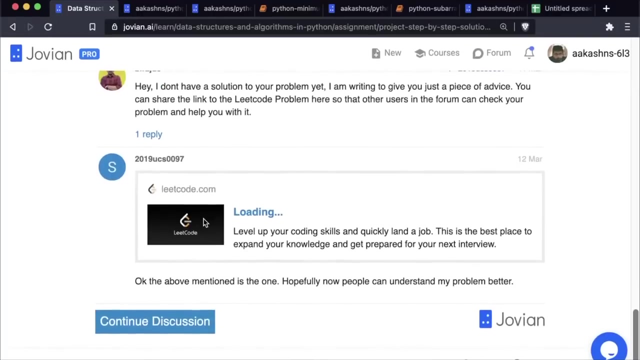 wherever required, perform the complexity analysis. all of this you should add in the Jupyter notebook and then publish your notebook to your Jovian profile. And finally, you can submit the link to your Jovian notebook here. Do submit the link to your Jovian notebook here and you can check out the discussion where you can change a way we can post what you, what you're working on. 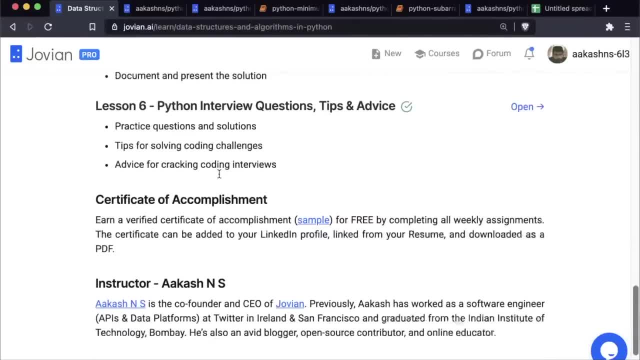 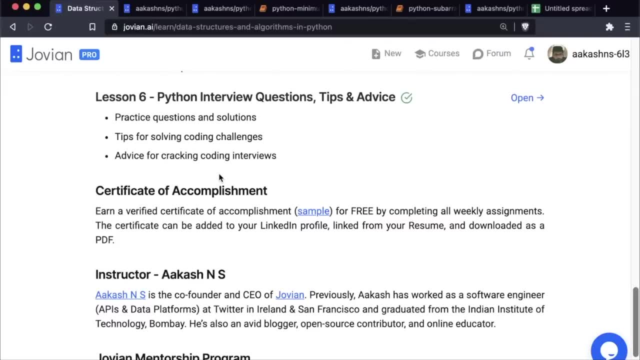 So do post your notebook as well. And finally, today we have looked at A couple of real interview questions from Amazon and Google and how to go about solving them, And we also addressed a few issues that we faced along the way. So that was a helpful exercise and that's it. 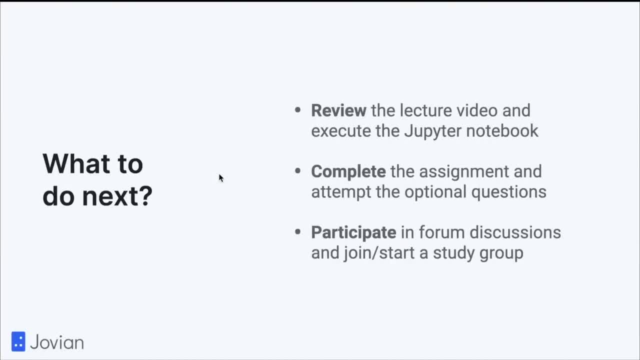 So now you can review the lecture video, execute the Jupyter notebooks, complete the assignments and attempt the optional questions so that the topics that we've covered, they get consolidated and you do not ever have to look at this Lecture again, right?